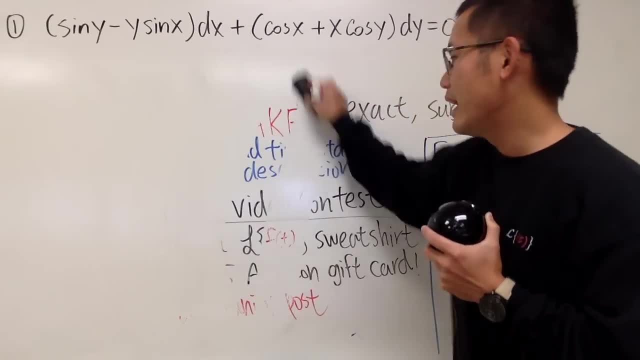 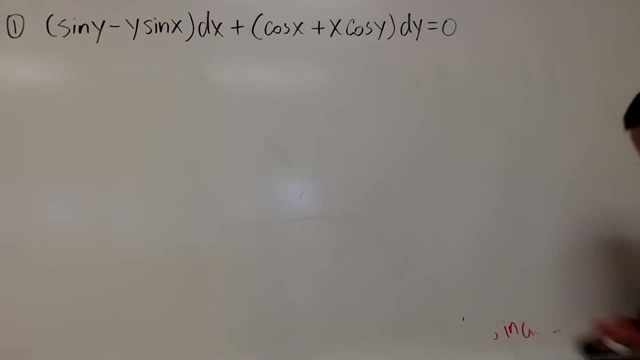 Stay healthy, stay safe And let me know how you guys are doing. And yeah again, best wishes to everybody. right Now, let's go ahead and get started With the first one. Yeah, the equation is this long. 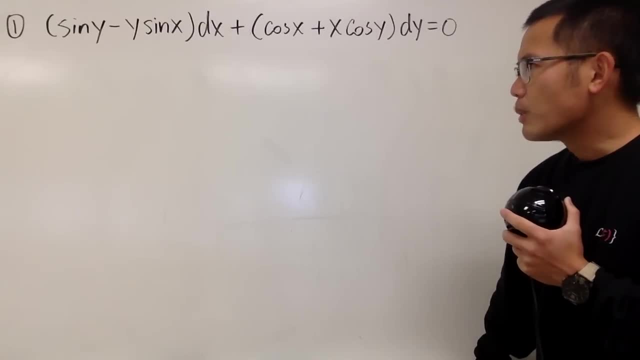 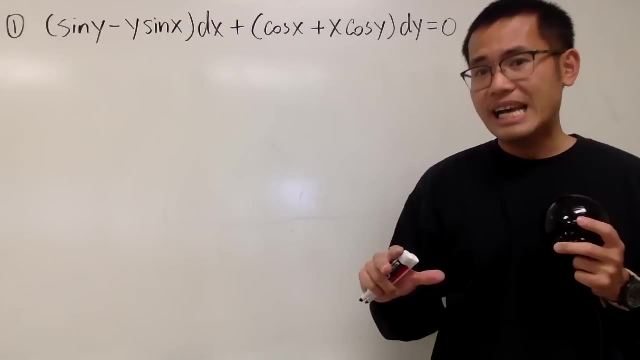 All right. so here is the deal. Sometimes, when people write down a differential equation in this form, maybe the person is trying to give you a hint that this is in the exact form, And what I mean by that is: hmm, just think about it. 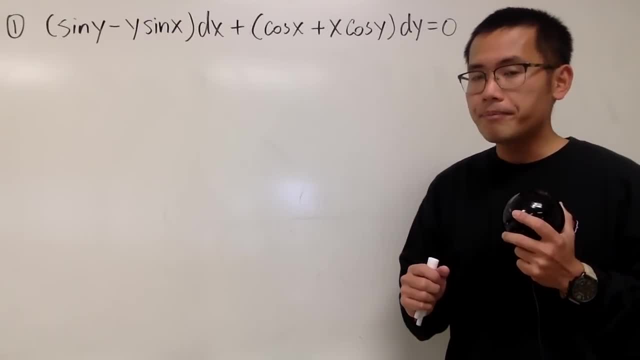 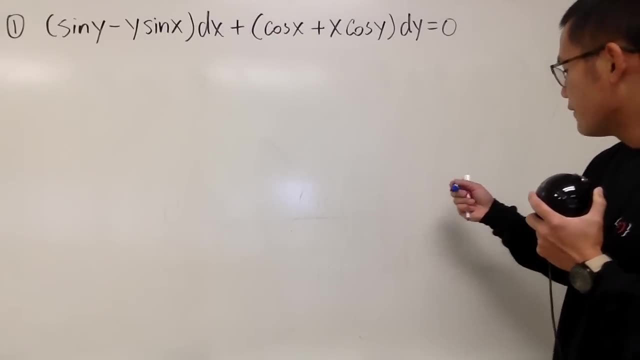 If you have a function in terms of both x and y. well, if you do the total differential. let me just write this down right here for you guys. I'm going to write it down in blue. When you have a function, let's say f, of x, y, and you can just kick the constant to the right-hand side. 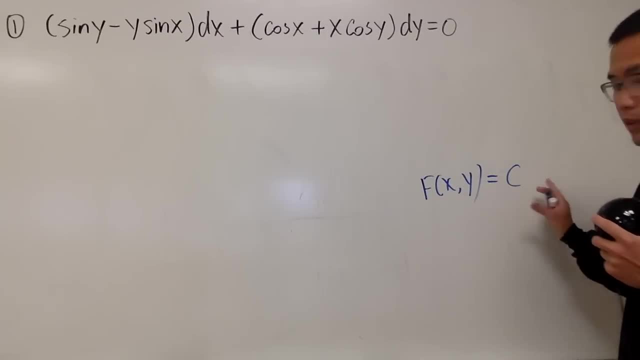 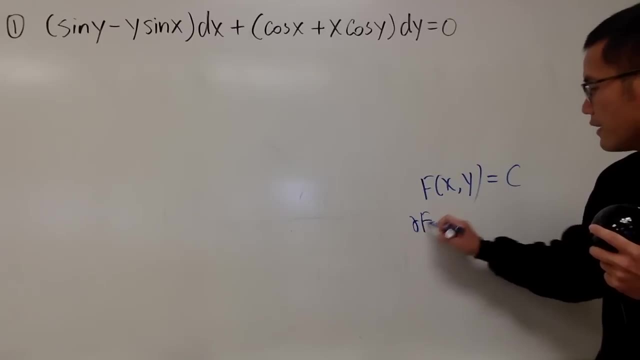 So it doesn't really matter if you have the constant or not. You can always kick that to the right-hand side, like this: Anyway, if you look at this, you can do the total differential of this And you can just get the partial of f with respect to x, like this: 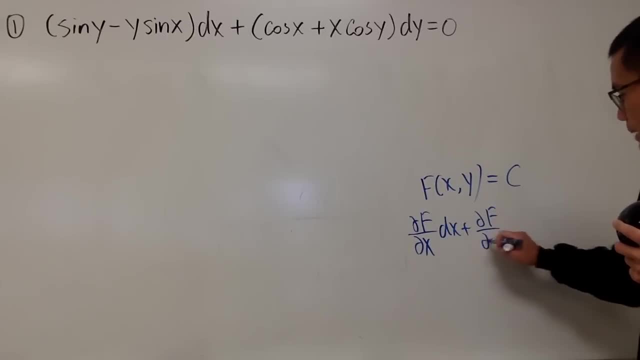 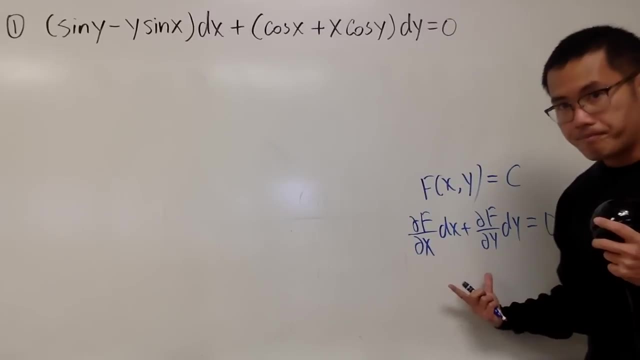 And then dx plus partial of f with respect to y, dy, And that will be equal to 0. And you see this right here. it's in this form, So you can check to see if this right here is exact or not. 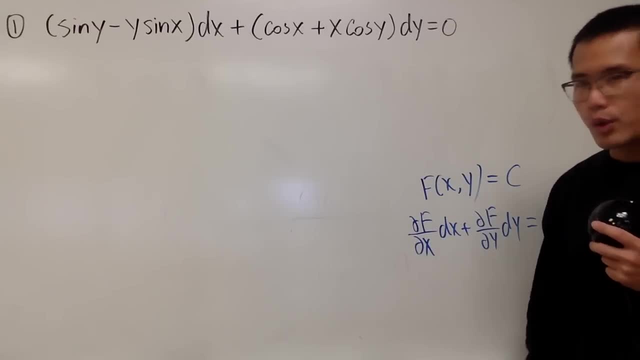 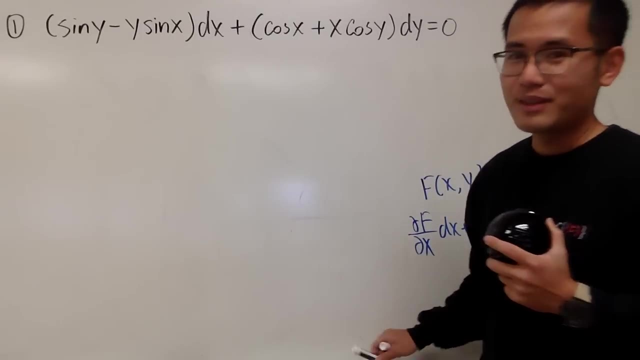 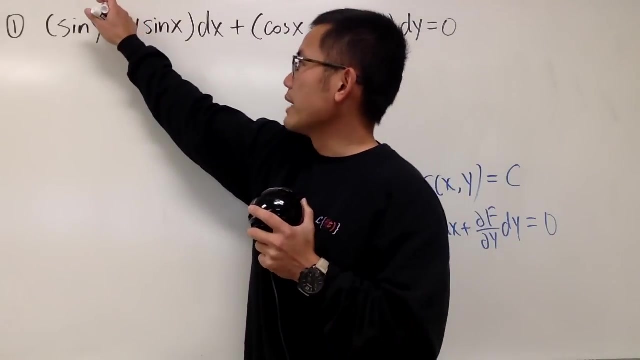 And this is an example of a possible exact differential equation. And again, it's just because, if the creator of the equation wants to give you a hint, I'll go for exact first. So here's the deal, though Suppose this is exact, which I actually don't know yet- 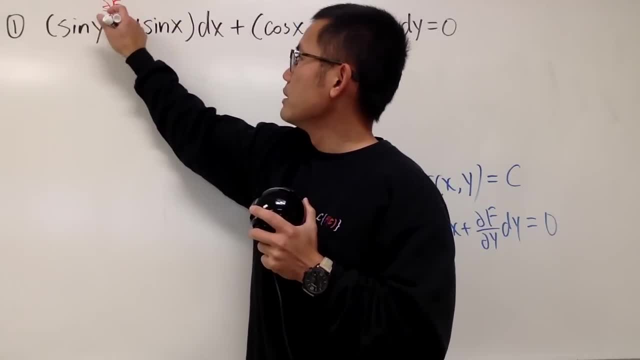 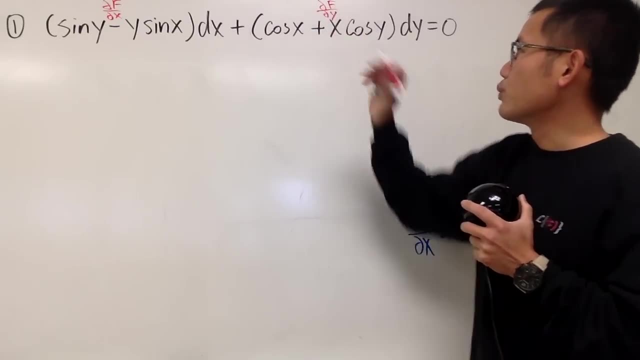 The idea is that this right here represents some function's derivative with respect to x, And this right here represents the partial of f with respect to y, right, Just like this and that. How do we know if this is exact or not? 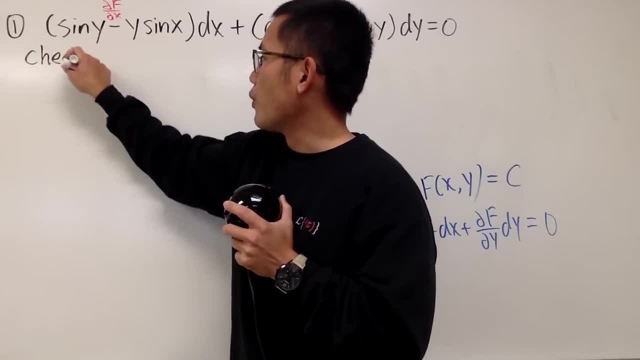 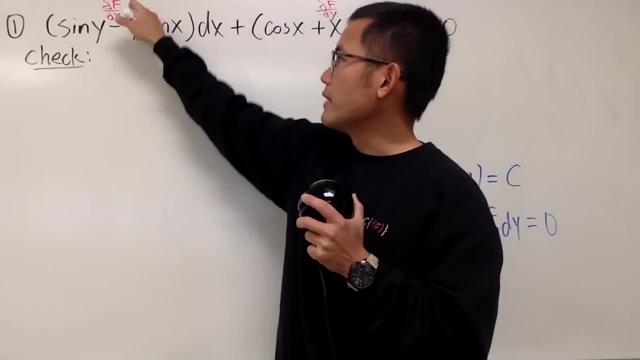 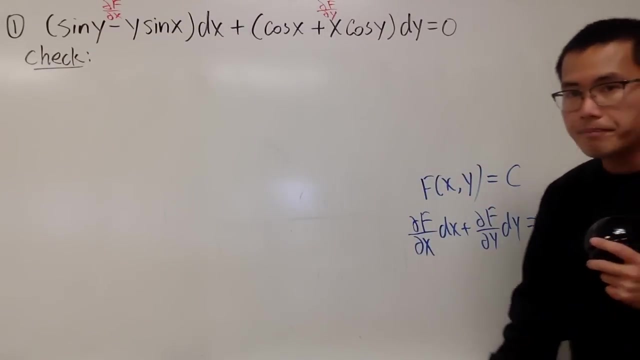 Here is the check And I'll, of course, write it down right here for you guys. The check is this: right here. Hopefully it does represent the partial of f with respect to x, But remember that the mixed partial of a multi-variable function most likely. 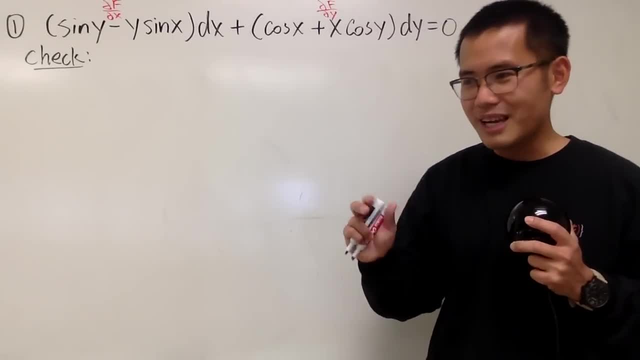 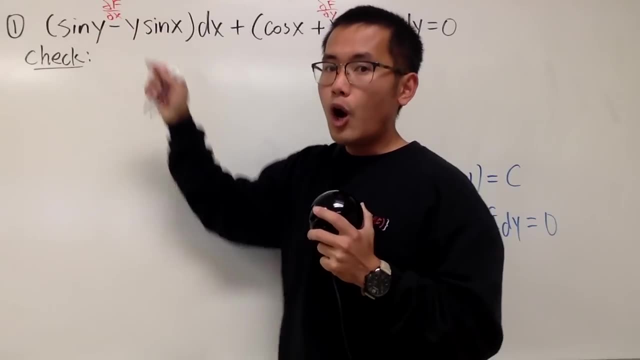 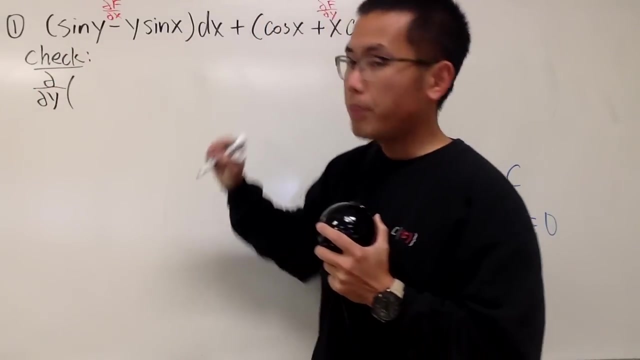 they will be the same right, Because you know it's just like one real stuff that will happen. that's not the same. So just check for the mixed partial. So this is with respect to x. already All we have to do is go ahead and check the partial with respect to y of this part. 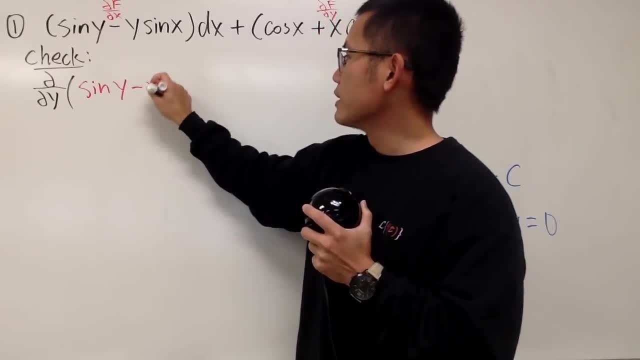 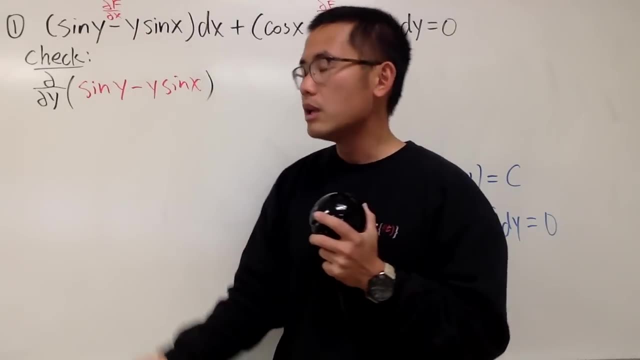 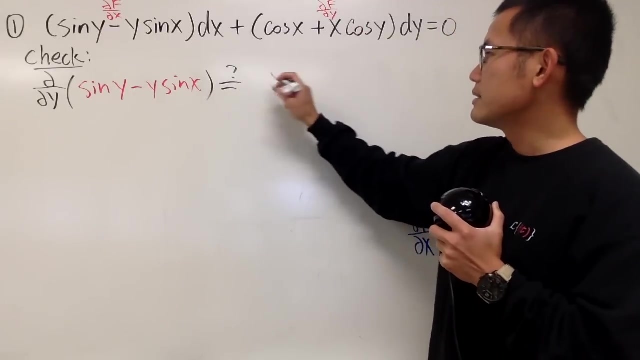 which I will just enter sine y minus y, sine x, And you see, this is with respect to x. already You want to do the mixed partial, So you do it With respect to y, namely the opposite, And hopefully this right here is the same as the partial of this function with respect to x. 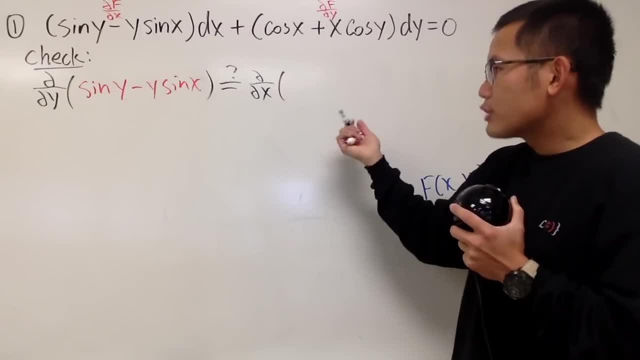 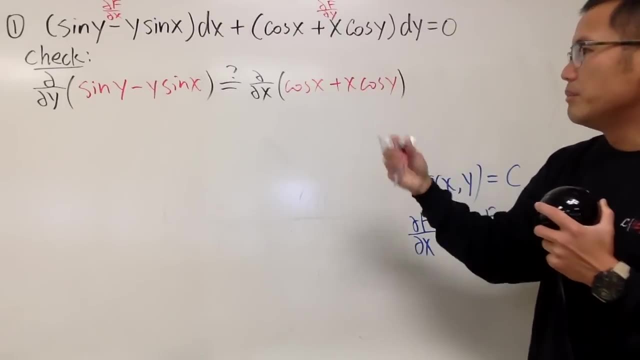 Because this right here is with respect to y, already And again, I'm not sure yet. Usually, when the question is presented this way, just go ahead and do the mixed partial, Just do the derivative real quick and hope for the best. I'll say. 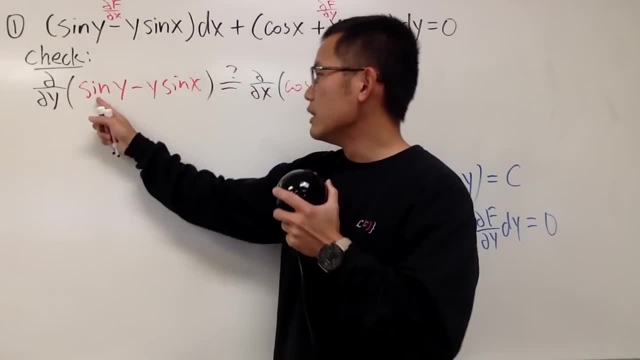 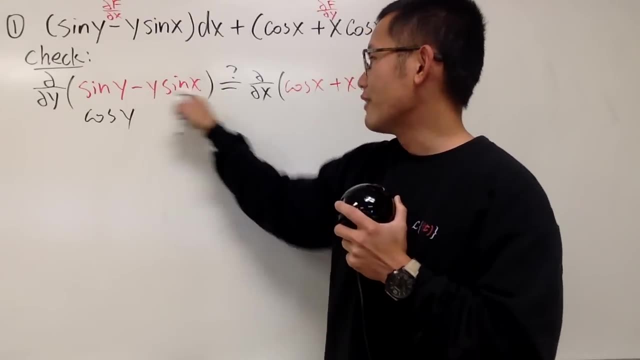 Now here's the deal. Go ahead, Differentiate this In the y world sine y will give us cosine y. And then differentiate this. Well, differentiating y, we just get 1.. And then we have minus sine x. 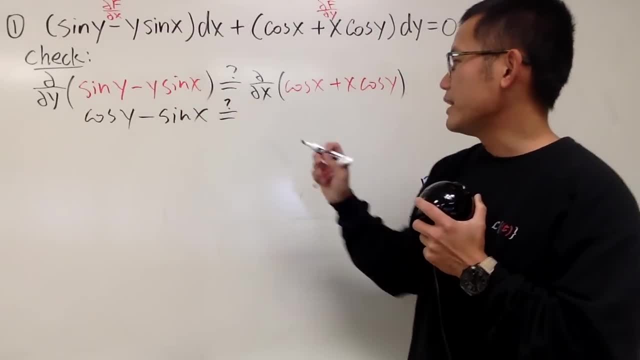 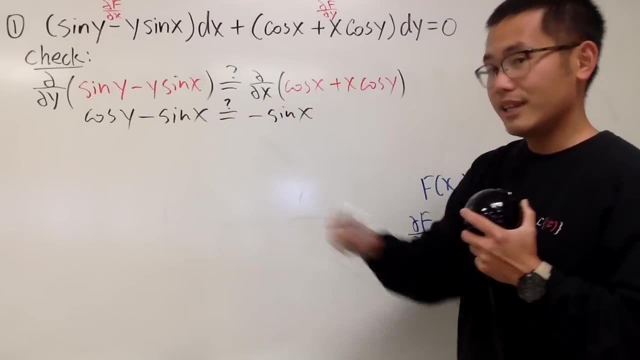 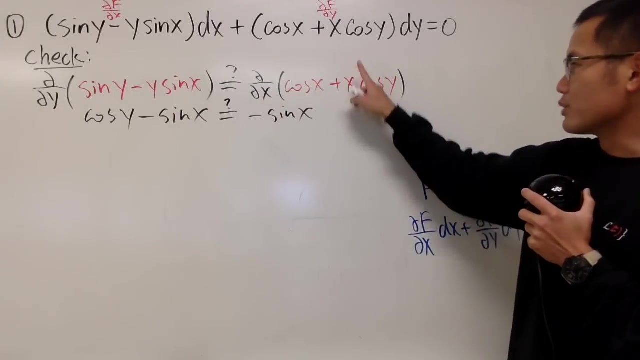 That's all we have On the right-hand side. well, I don't know if they're equal. yet Differentiating this with respect to x, In the x world we get negative sine x. Hey, it looks good. Now, differentiating this with respect to x, the derivative x is just 1.. 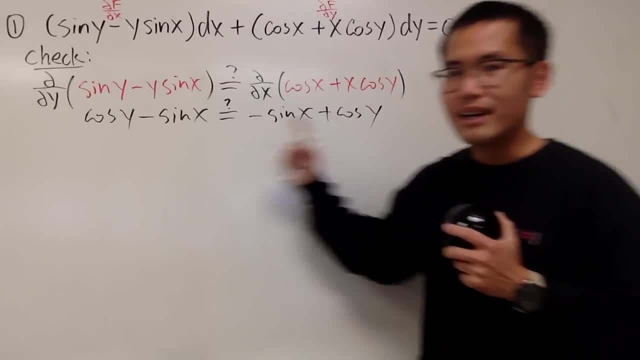 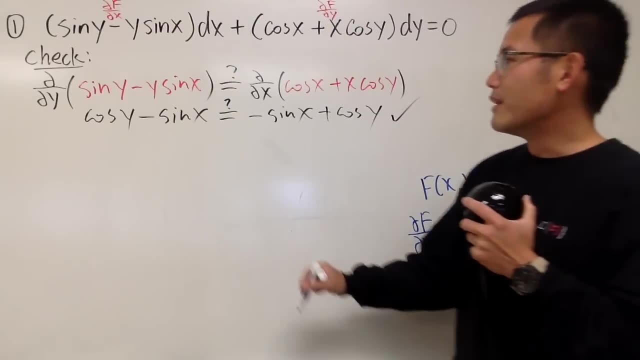 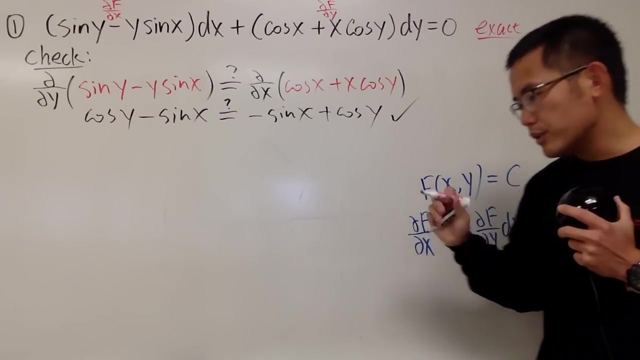 So we have plus cosine x And then we have minus sine y. It does match. Of course, the order does not matter. So it is exact, Right. So this right. here again, this is an exact differential equation And I will show you guys all the details for this question later on. 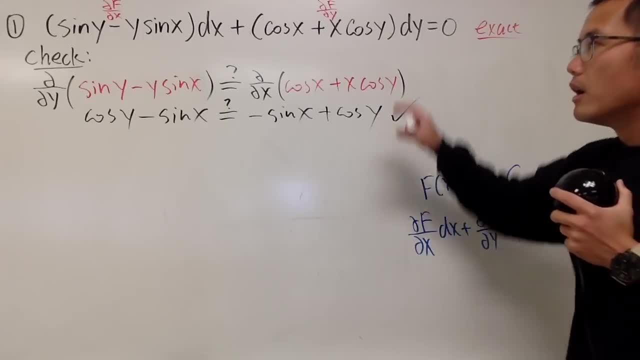 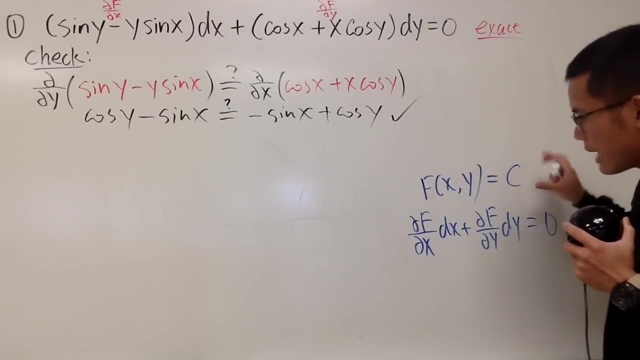 We'll just do it much quickly, of course. Now, here is the thing. Now we can be sure that this came from the total differential of some multi-variable function In this form. yeah, This right here again, is the partial of f with respect to x. 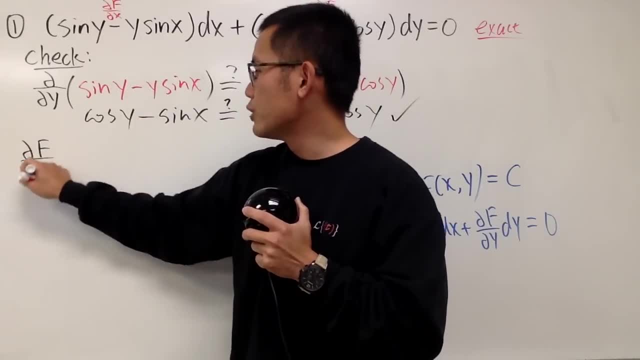 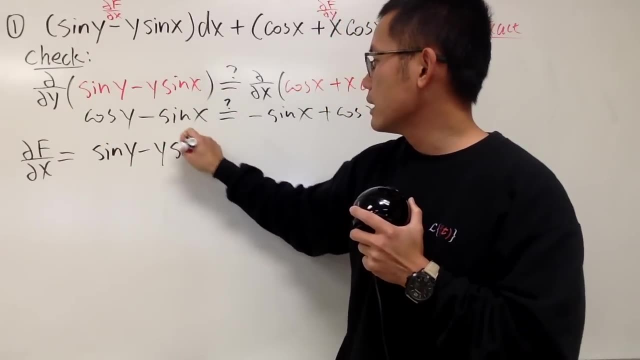 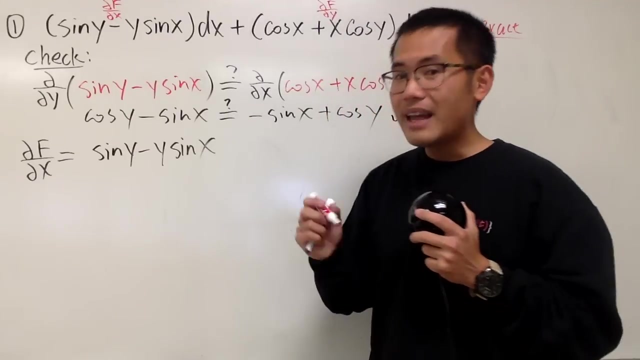 So this is how we are going to start. We write down partial of f with respect to x, like this, And we will just begin to write this down, which is sine y minus y, sine x. And if you want to start with this, this is also possible, but let me just do it for that. 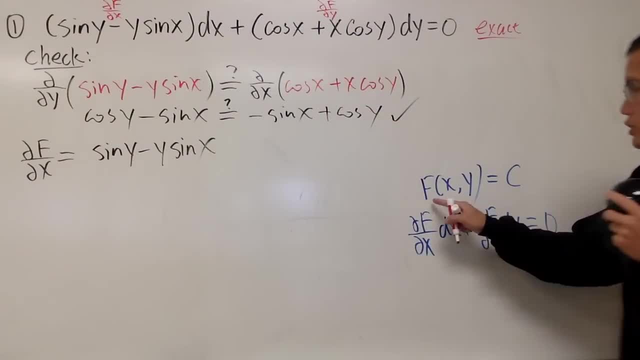 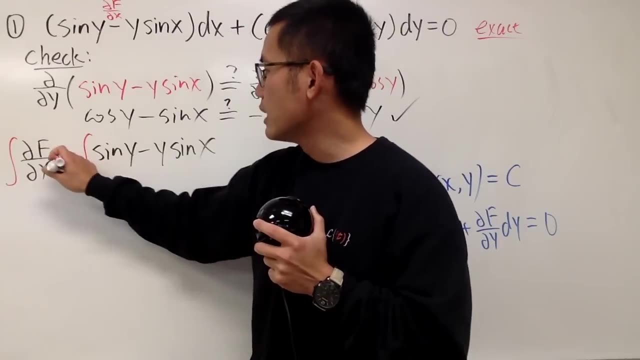 Now what we're going to do is, of course, to get back to the original capital F. we will just have to integrate, And this right here is with respect to x. So we have to integrate both sides with respect to x, just like this. 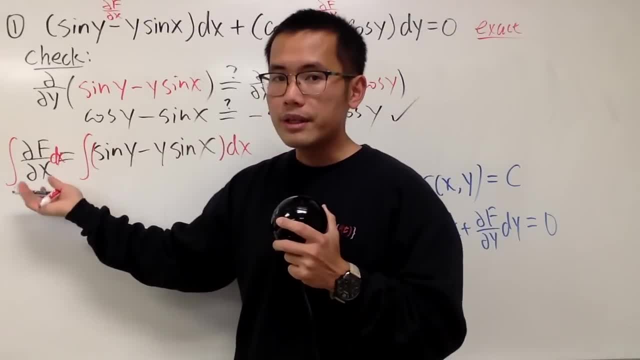 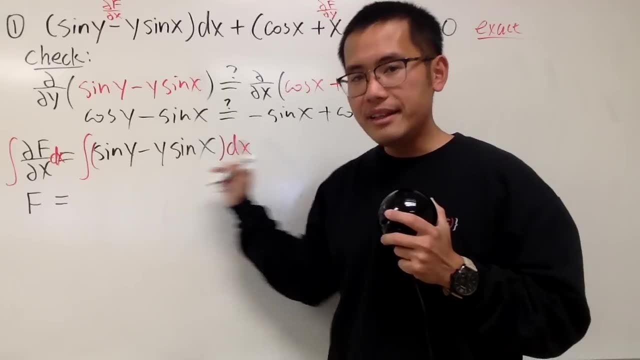 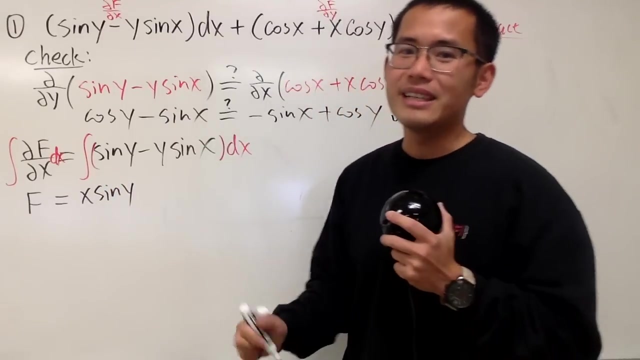 Right. So now on the left-hand side, when we integrate this, of course we just get capital F And then this is equal to well, integrating sine y in the x-world. it's actually very easy. It's just x times sine y, because y is a constant in the x-world, right. 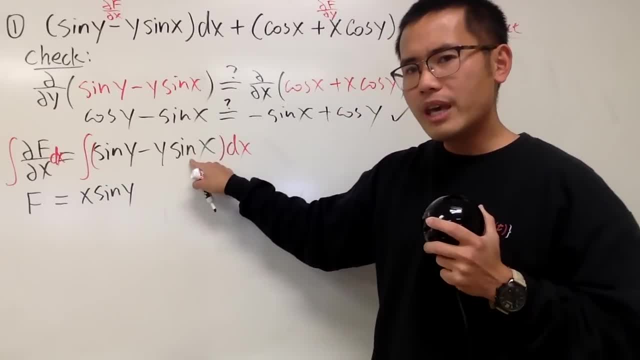 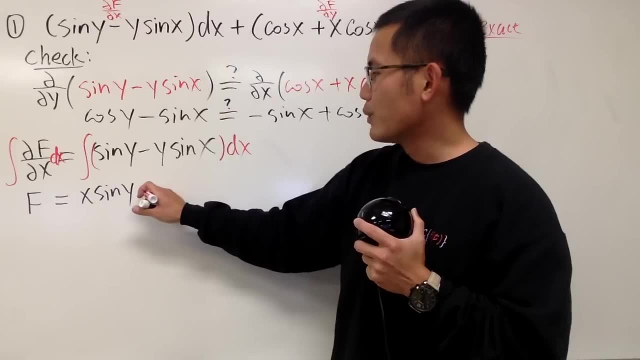 And then, of course, integrating sine. well, we get negative cosine. So this right here will actually be negative, negative. so we'll actually get. okay, let me just write down negative and then I will have to put down another negative, so it's actually plus. 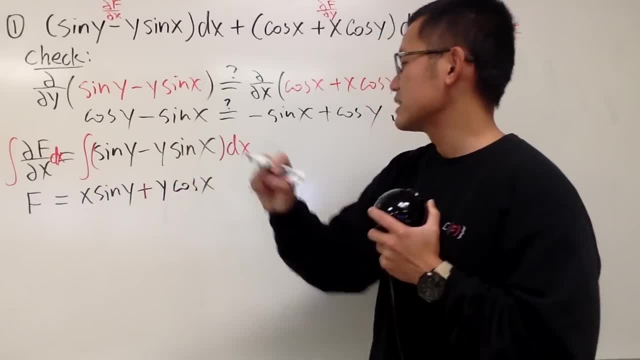 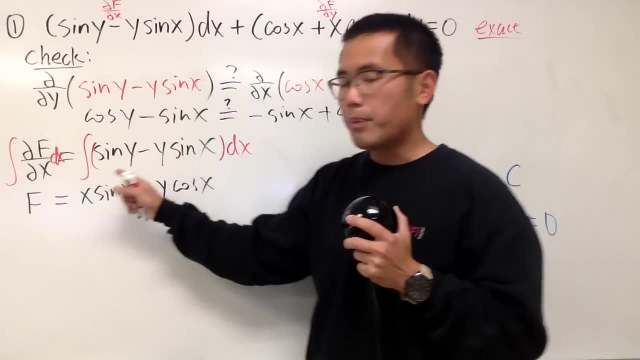 and then we have y and this is cosine x, just like this. Well, in the x-world, y is a constant. Usually, when we integrate both sides, we just put a plus c. but since y is a constant, so we are not going to just put down plus c. So we are not going to just put down plus c, but since y is a constant, so we are not going to just put down plus c. So we are not going to just put down plus c, but since y is a constant, so we are not going to just put down plus c. 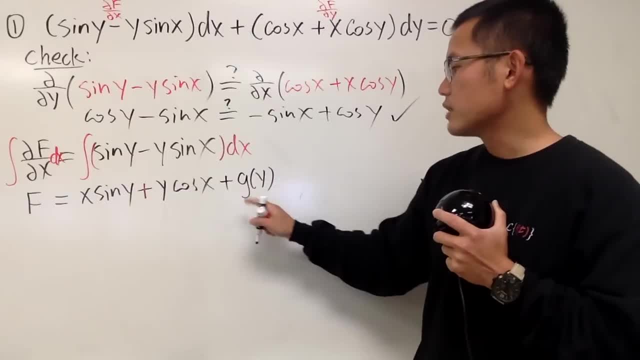 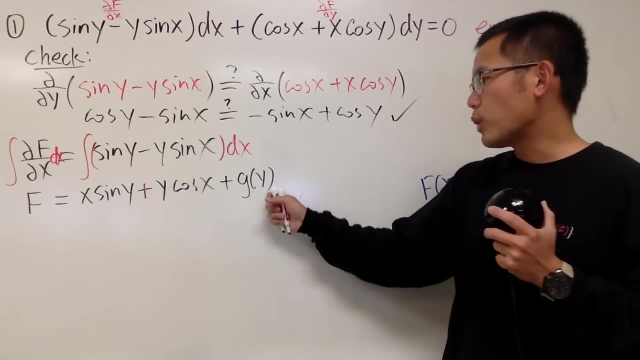 In fact, we'll put down plus a function in terms of y, So usually we write it as g of y, like this. So this is how capital F looks like, but I don't know what g of y is. This is the part that we are going to utilize, this part of the information. 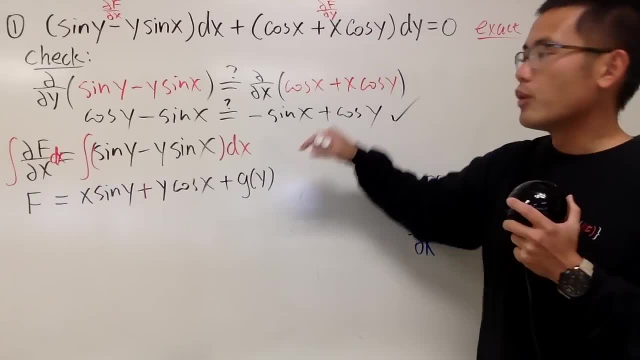 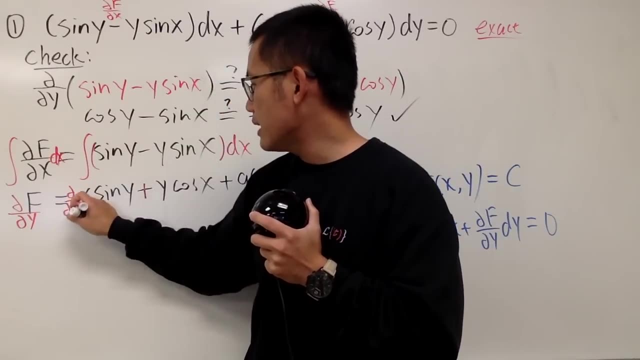 This right here represents partial f with respect to y. Well, now we have to do the partial of f with respect to y on both sides, so let's go ahead and do that. So on the left-hand side, we have a partial of f with respect to y on both sides, so let's go ahead and do that. 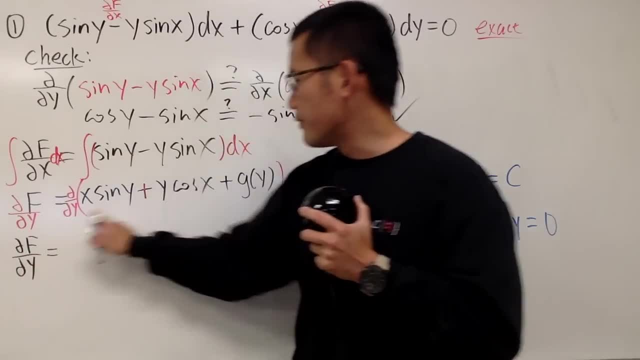 So on the left-hand side we have a partial of f with respect to y on both sides. so let's go ahead and do that, Differentiating this with respect to y, the derivative of this. well, we get x. stays, it's just a constant multiple. 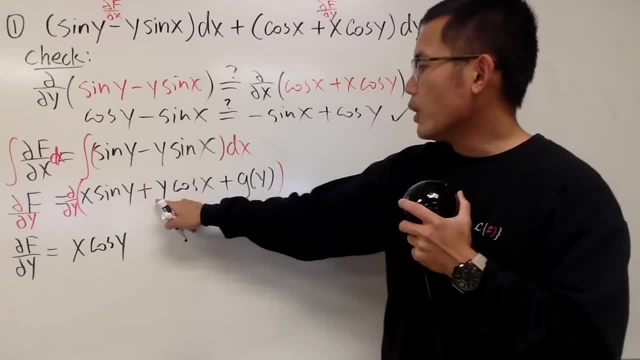 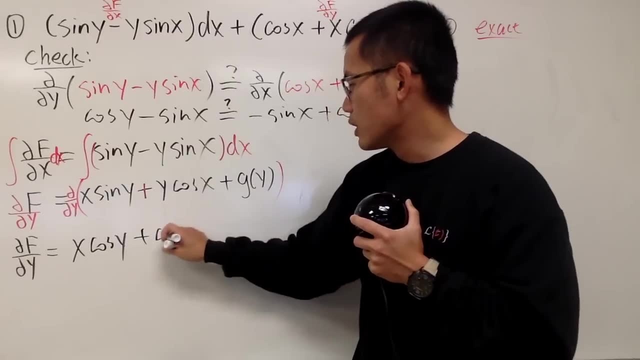 The derivative of sine y is cosine y. Well, differentiating plus y cosine x, this is just going to be constant multiple. so we actually just get plus cosine x And then plus. the derivative of this is just g prime of y. 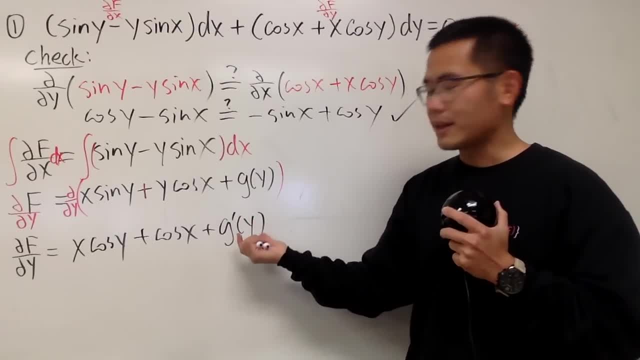 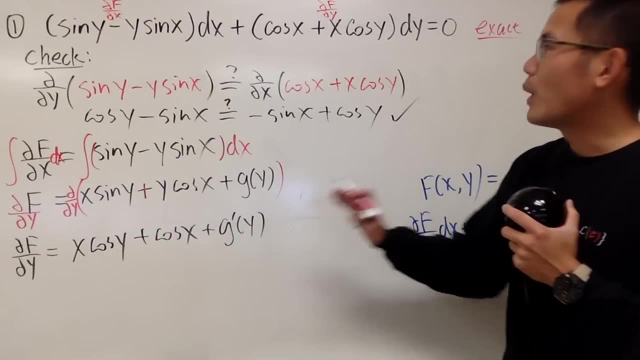 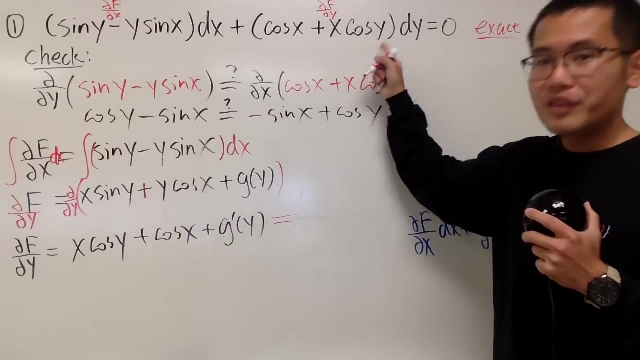 And keep in mind this right here: it's a single variable, not calculus, It's a function. Capital F is a multi-variable right. All right, so now this is what we have, and this right here, yeah, this right here should be equal to what we have here. 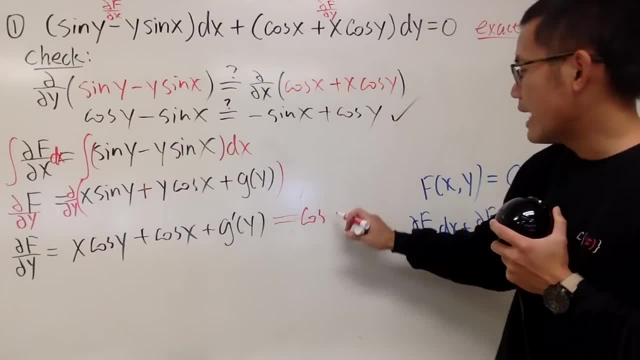 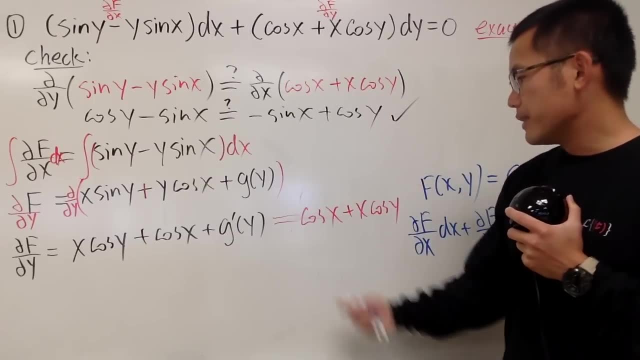 So that's how we can make the connection. and then let's go ahead and just write this down: Cosine x plus x, cosine y, like so Well, well, cosine x match This and that also match. so what does that mean? 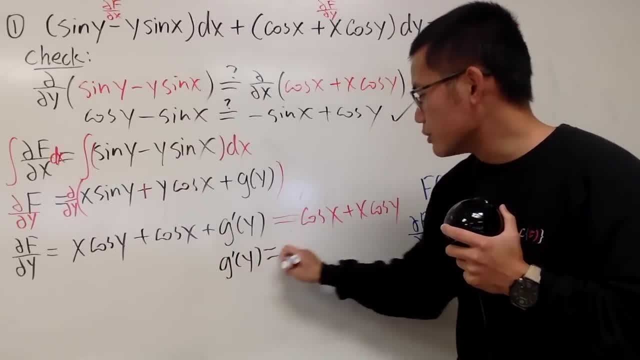 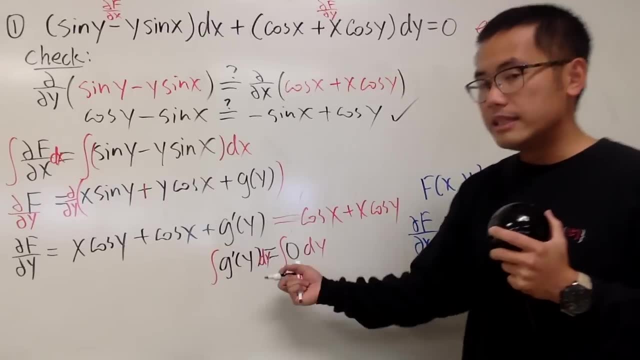 That means g prime of y has to be equal to 0. And then from here we can just go ahead, integrate both sides with respect to y, But this is just going to give us in this a constant c. So we get g of y is just a constant. 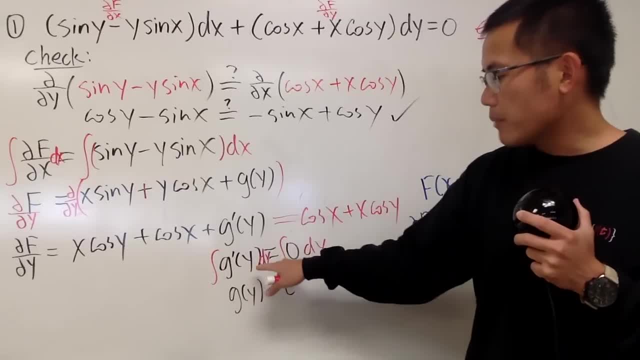 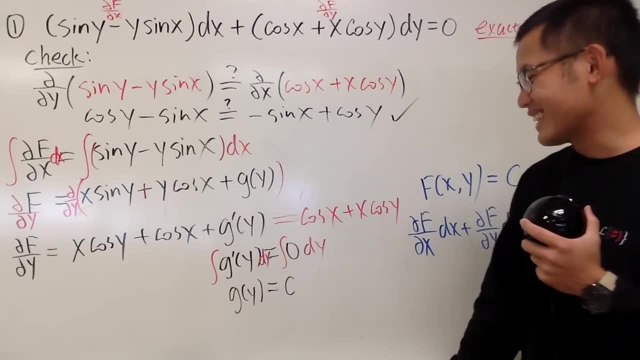 And the reason we write down constant is again this g prime of y. the function g is just a single variable function, So we just get a constant. So it's normal x in this case. So that's pretty much it. 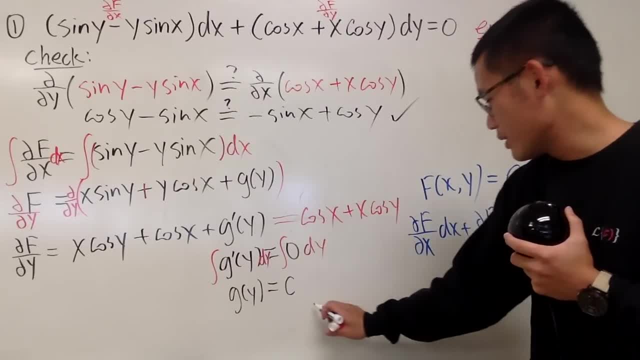 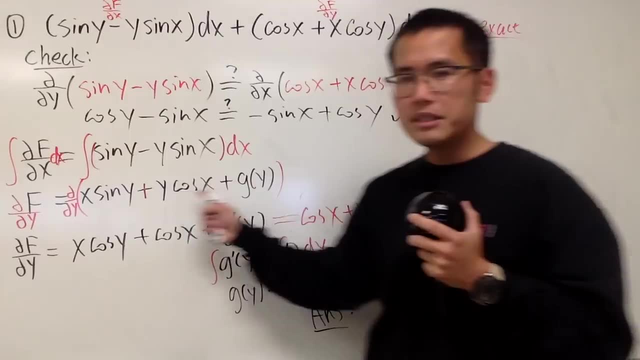 And all right. So what we have to do next is just write down the answer. I will put it down right here for you guys, And this is how you are going to write down the answer. Look back to our capital F, which was in this form, and then we know g of y is just a constant. 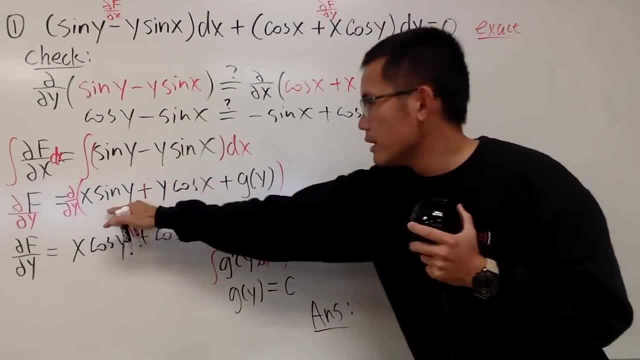 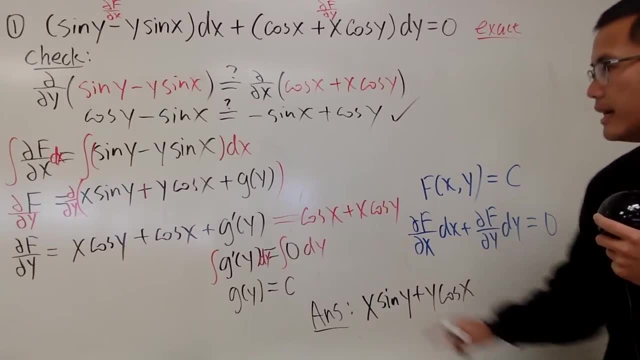 So let's write this down, and we'll put this down in this form later, You'll see. So let's write it down. We have the answer x sine y plus y cosine x, And then this right here is the constant, so we can put down: plus c. 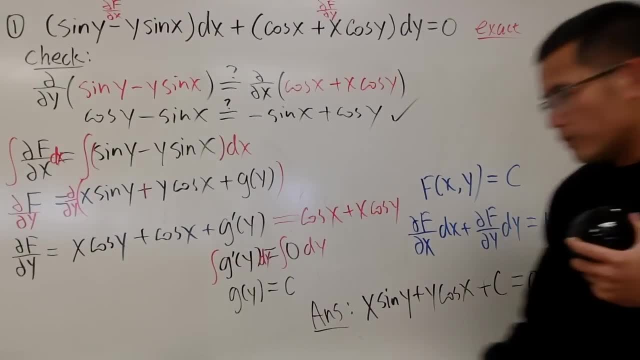 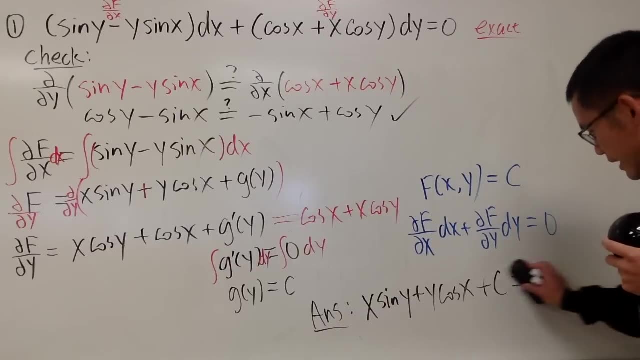 And this right here will be equal to 0.. Well, again, this right here is OK. but usually we will put a c to the other side And when we do that it looks like we have negative c. But since c is a constant, negative c is also a constant. 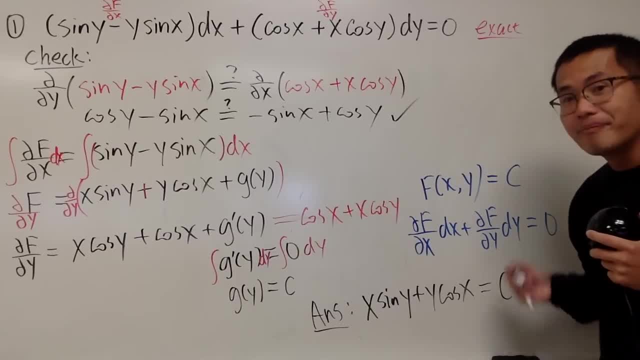 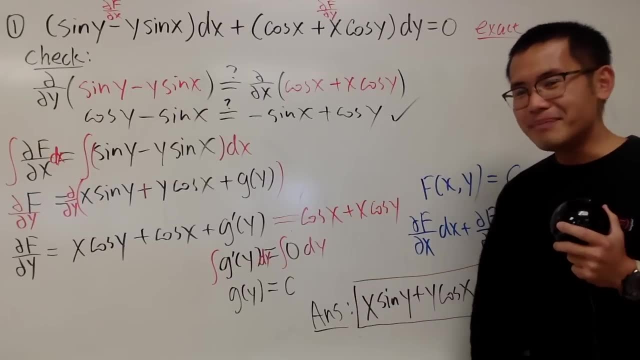 When we write down our final answer, just put it as c. That's all. It might be confusing for the first few times that you're doing it, but after a while you'll just get used to it. And to make it simple, all you have to do is just write down the function part. 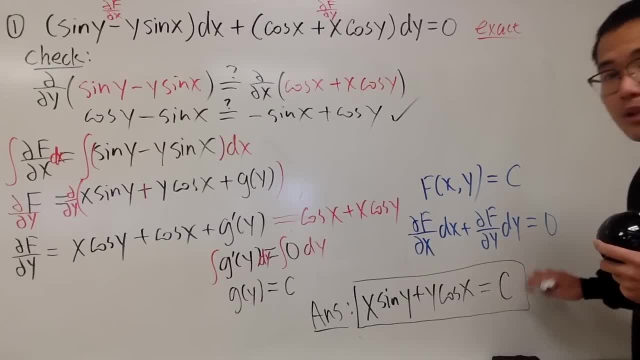 On the left-hand side and then make this equal to a constant on the right-hand side, And that will satisfy this, just like this. So this is an example of an exact differential equation, just like that. Very good, huh, It took the whole board already. 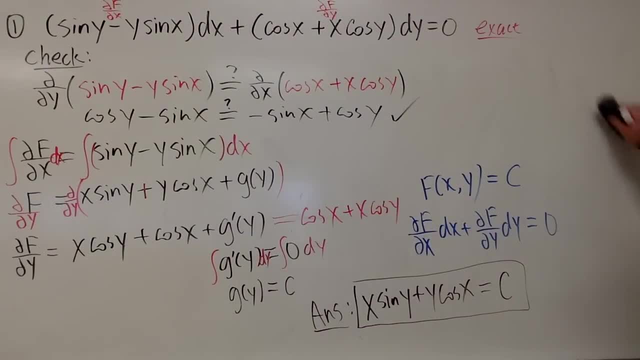 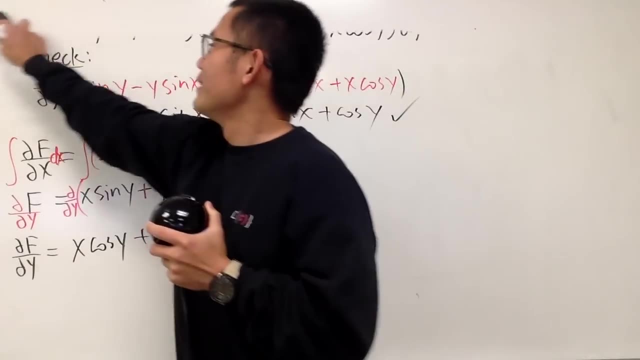 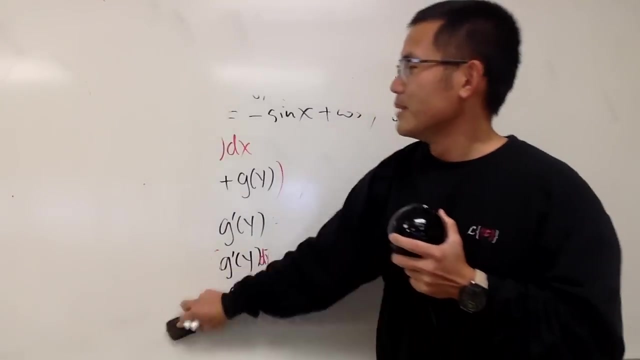 Let's see 10 minutes, All right. So yeah, we have 23 more to go, Let's see. And then, after Laplace, transforms, I don't know, Maybe second-order differential equations, and that's going to take even longer. 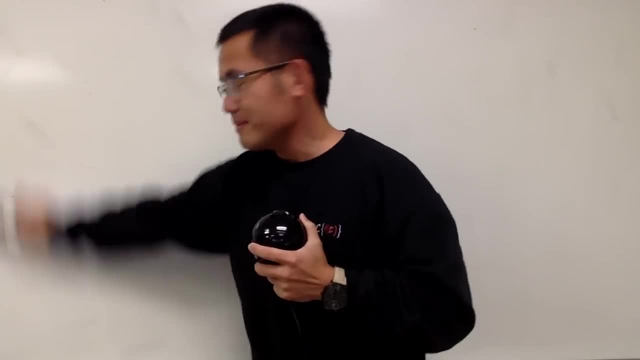 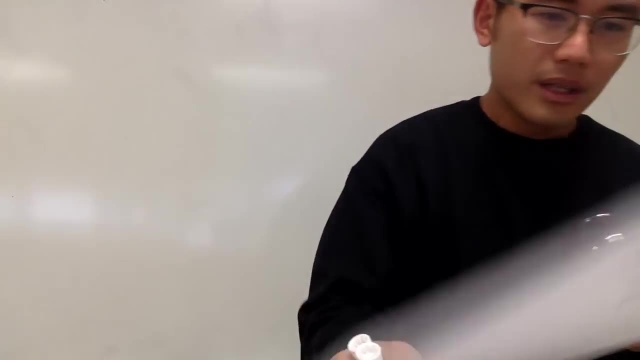 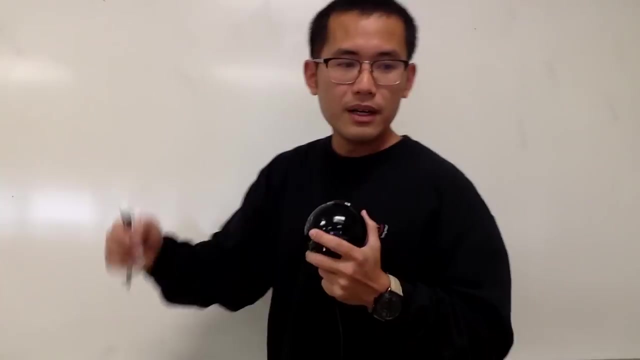 But we'll see. Let me know what you guys would like. things in 24 differential equations, I'll see. OK, So here we go. Number 2, right here. We have an initial condition here, So let me just make sure I write down the equation correctly. 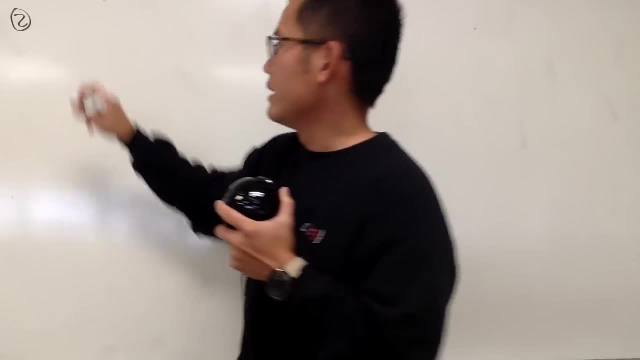 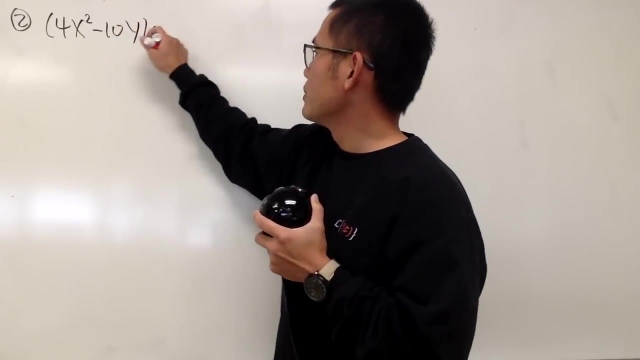 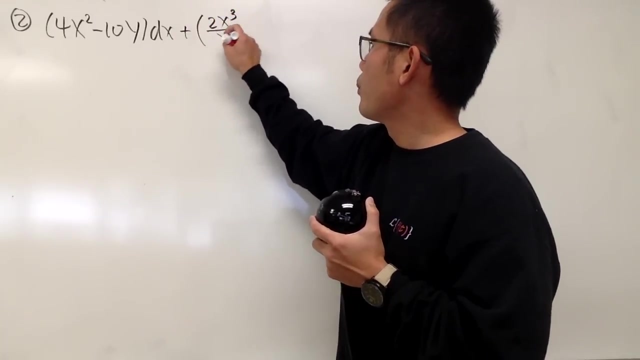 Because otherwise I will cry if I realize I spent like 20 minutes to do one question and then realize hey, I actually just had the wrong question in the first place. That's not funny. Plus 2x3 over y, minus 15x dy. 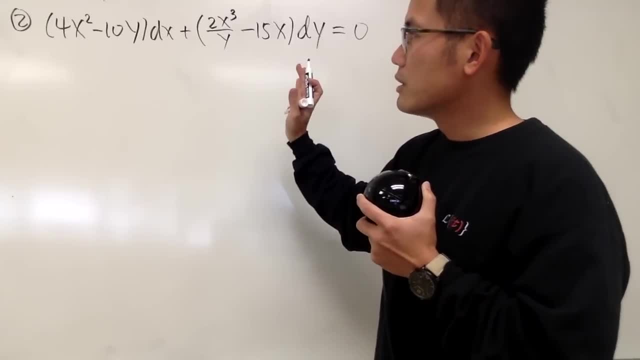 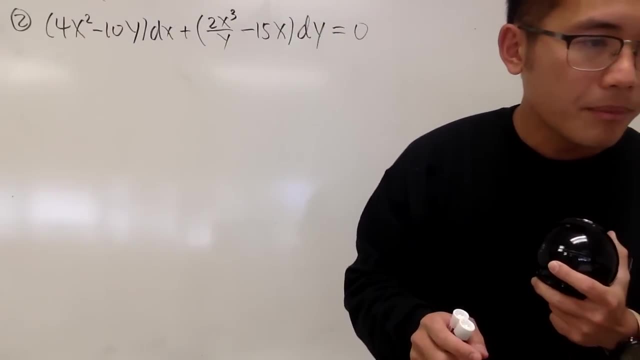 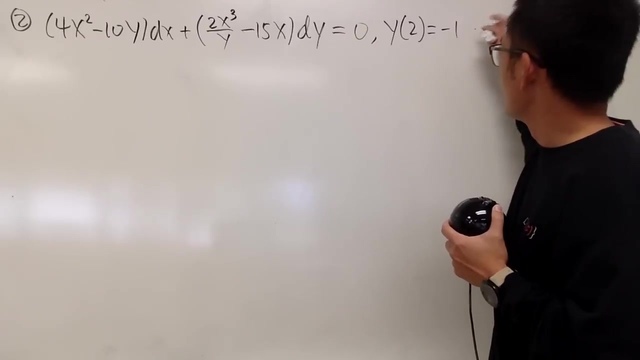 And that's equal to 0.. And again, just let me make sure, Make sure that I have the correct question, Because the questions are really long. Yeah, All right, y of 2 is equal to negative 1, like this: 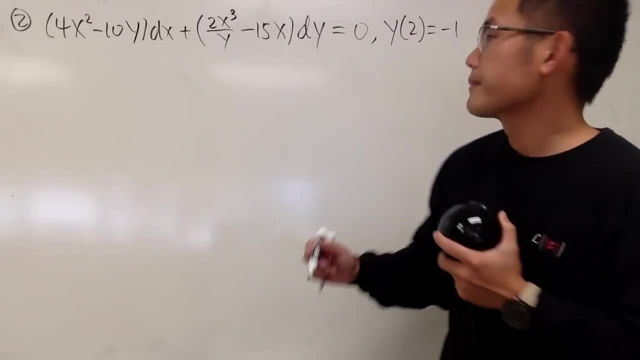 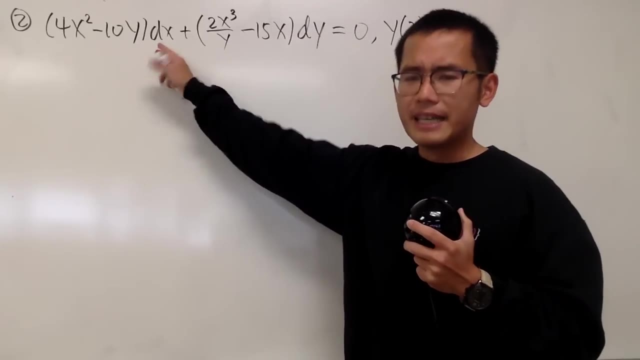 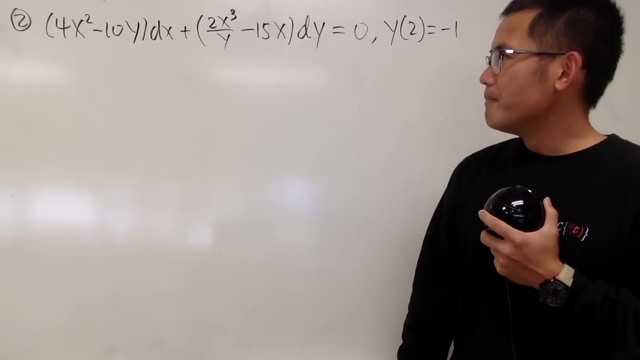 So yeah, OK, All right. So here's question number 2.. And now it seems like again it's like in this form it's suggesting us that this might be an exact differential equation. Let's do the check real quick, right. 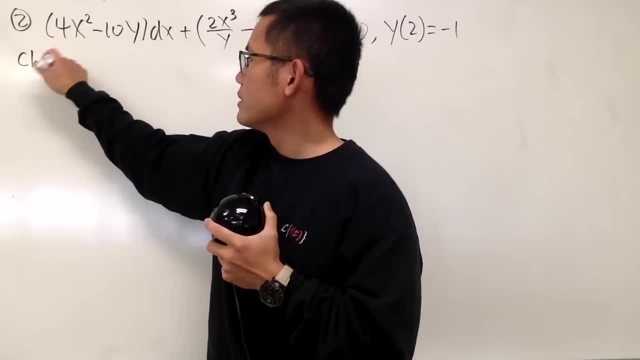 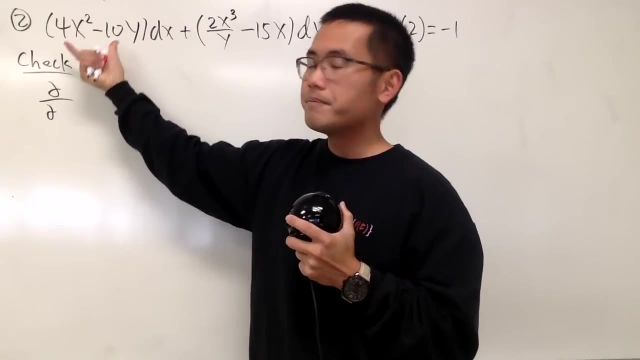 So let's just do the check. Let me just put this down. Here's just a quick check. I'm going to do the partial of this expression right. this function here. this part Depends how you want to say it. This is with x already. 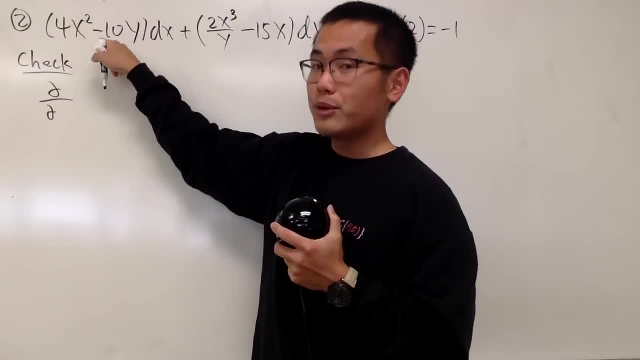 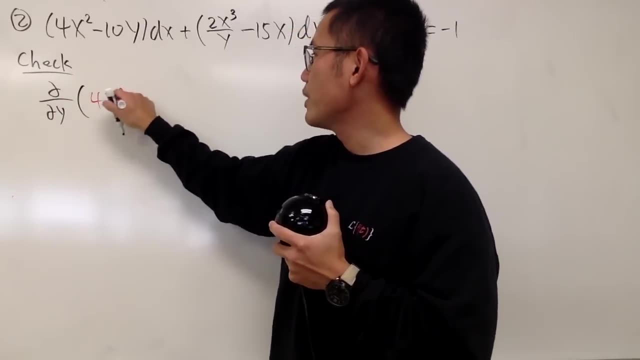 And remember this was partial with respect to x, And again you have to do the opposite. So you check this with respect to y And you put that down: which is 4x squared minus 10y, Is this equal to partial of this part with respect to x? 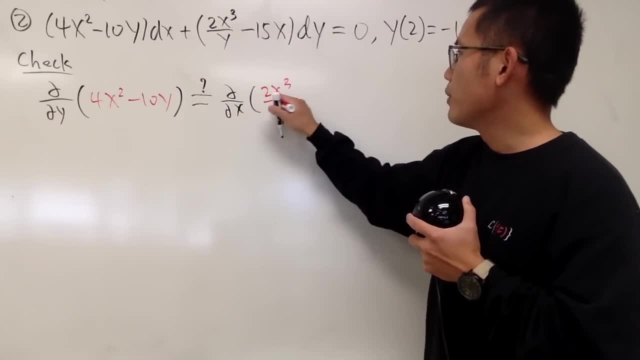 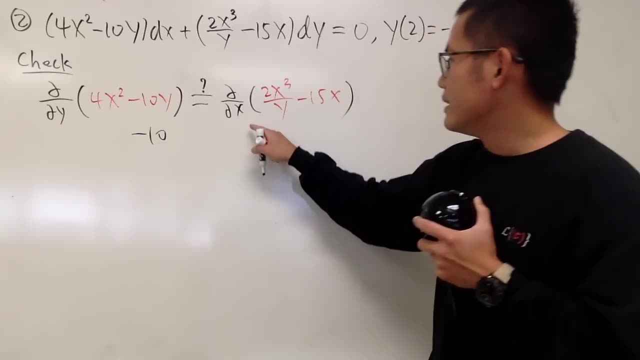 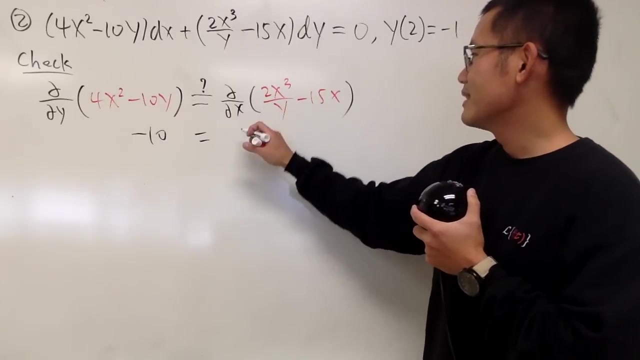 And then you write that down: 2x3 over y minus 15x, like this: All right. So let's do this real quick. Do that. We get negative 10.. No, It's just not possible. Like 6.. 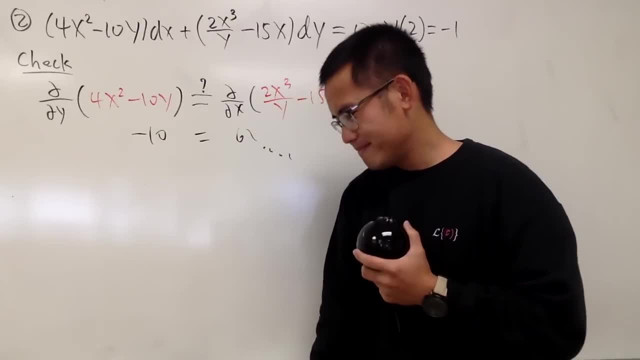 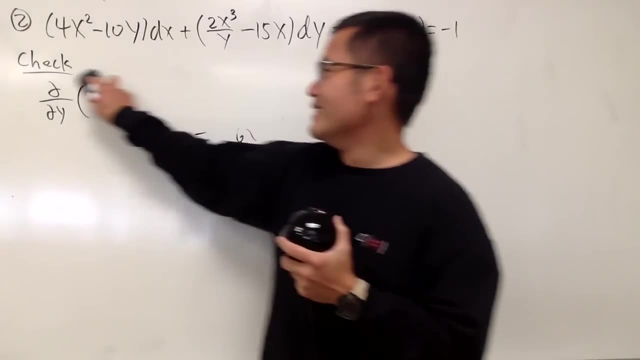 No, No, no, no, no, no, No. This is not exact. So it's not exact. Of course. you do not just write down not exact to be on the test. Do not just write down not exact and then just move on to the next. 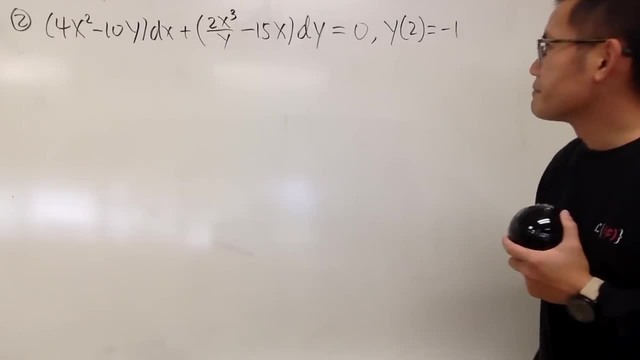 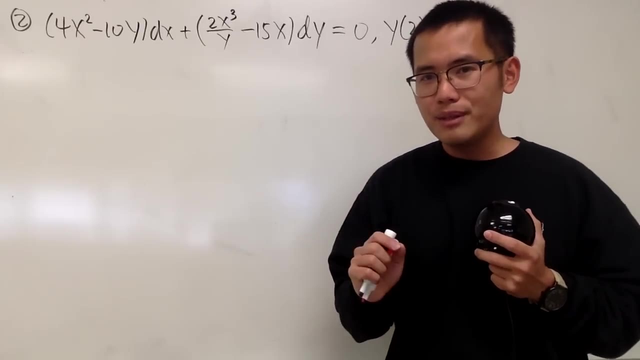 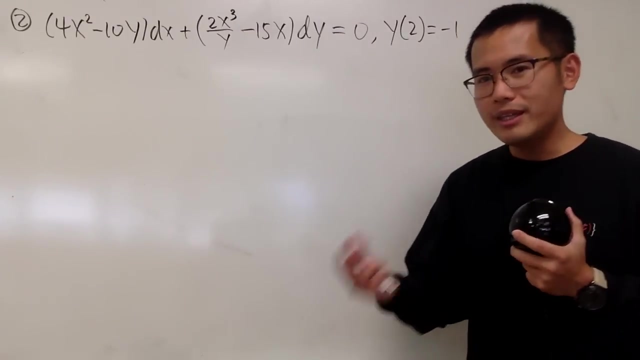 No, You have to actually solve it. So here is the deal. Sometimes, when you have a differential equation, if it's not exact it might be almost exact, And usually, when I have an almost exact differential equation, it depends on what we call the integrating factor. 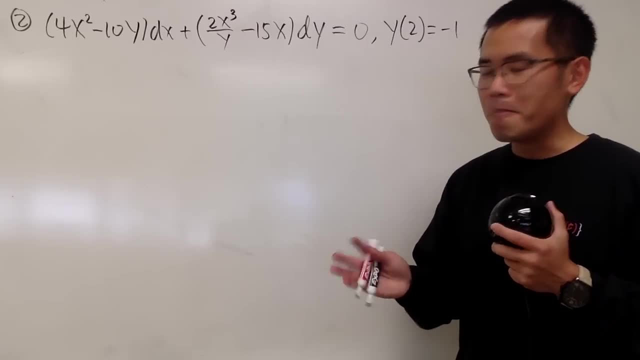 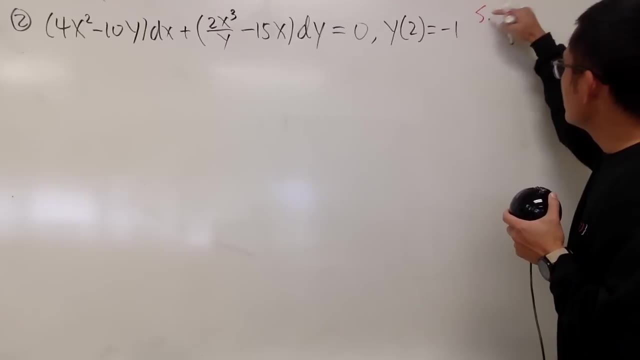 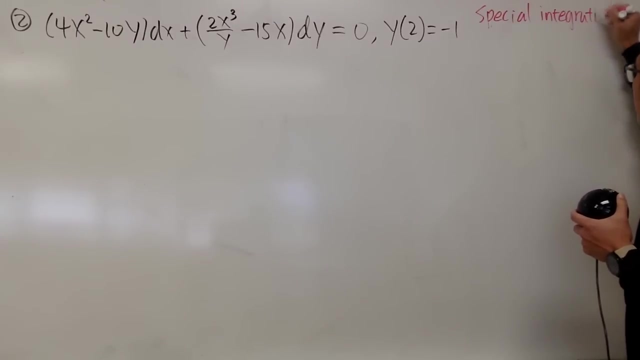 And if the integrating factor is like, hmm, Too crazy, I will usually give my students some hints. So in this case, in fact, we do have what we call the special- Let me just actually write it down Special- And we have what we call the integrating factor. 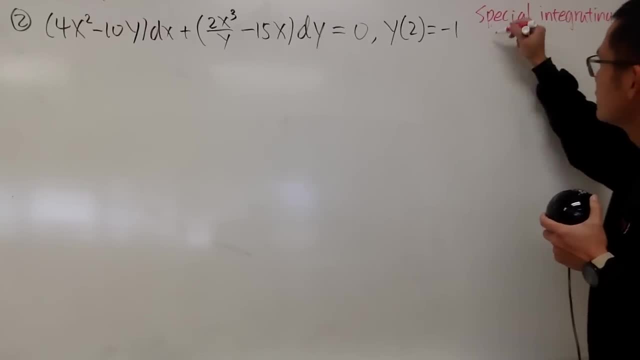 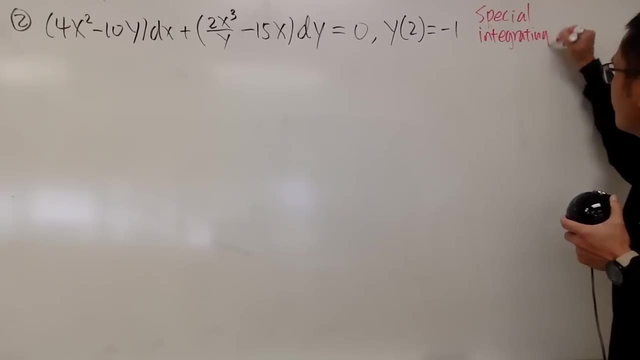 Right, Integrating factor. Let me just put it something like this: We have the special integrating factor, And when we have that, Let me just put it something like this: And when we have this, Again, it depends, And it depends on the form. 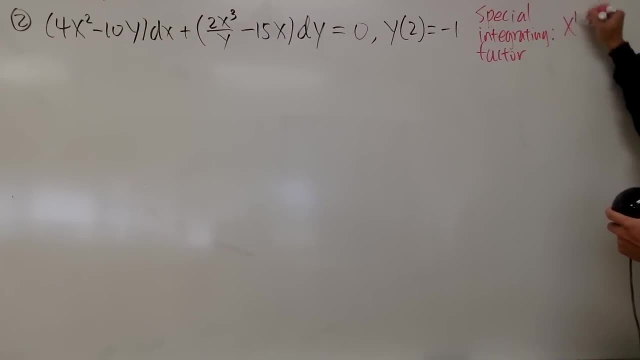 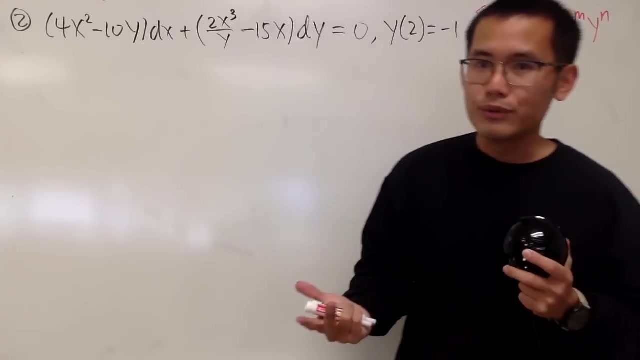 But in this case I will tell you, the form is actually x to some power m times y to some power n. This is not that easy to figure out, So I will have to give my students some hints sometimes, And the idea is that we are going to figure out what m and n are. 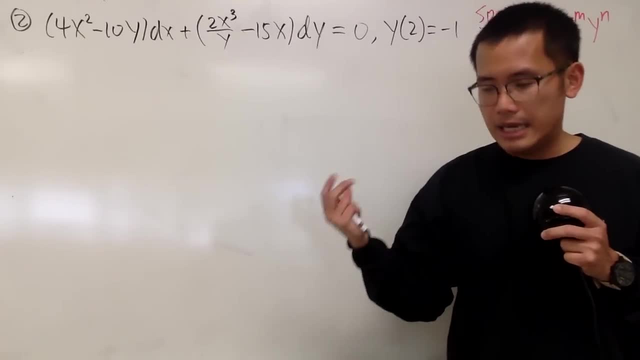 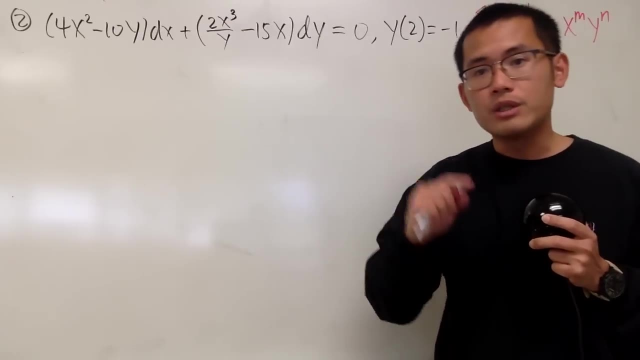 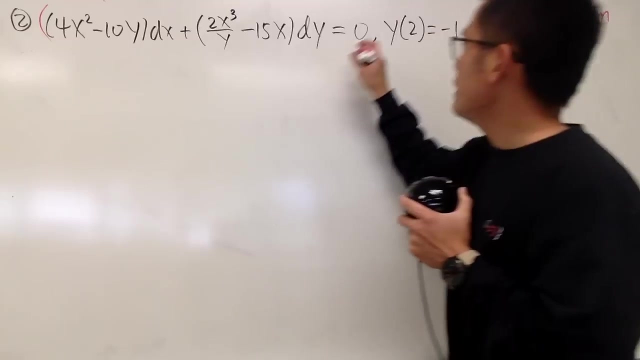 And then we'll multiply everybody by that, And that will become exact. So I want to figure this out. How can we do it? We have to utilize the idea that we talked about earlier, But for the special integrating factor, the first move is that we will just go ahead and multiply the entire equation by this form. 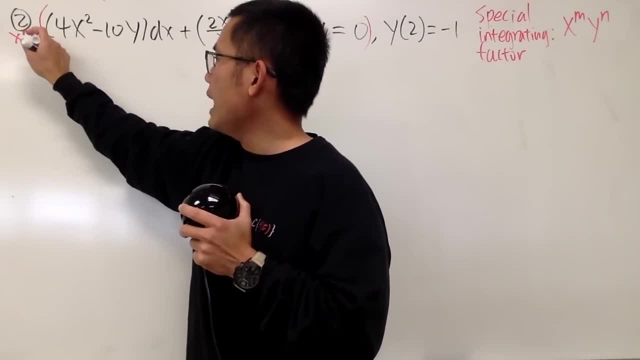 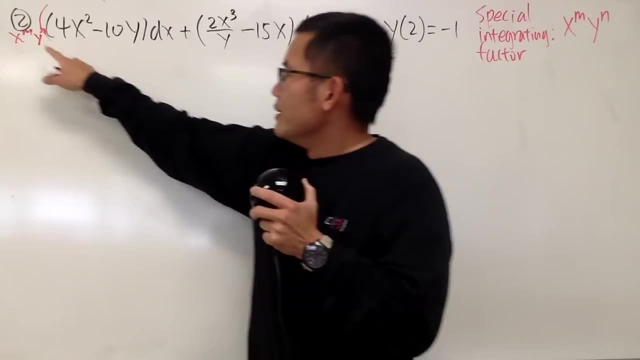 So let me actually just write this down right here: Multiply x to the m, y to the n, throughout this expression, Throughout this equation. So here we go. All right, Let's see x to the m times this, So first part we have. 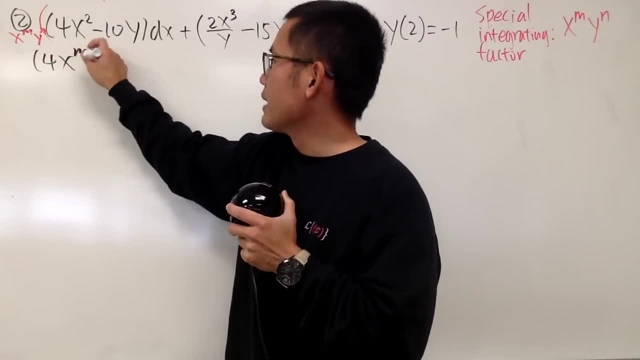 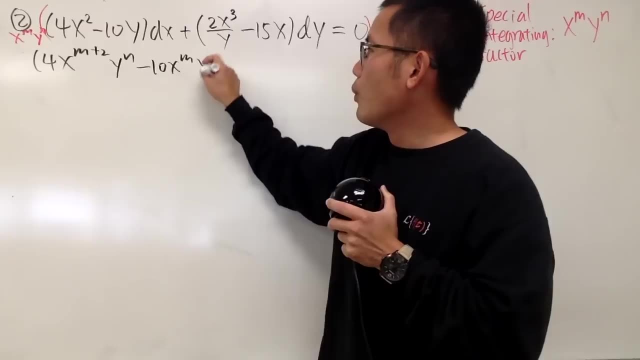 4.. And then, of course, we add the exponents, So we have m plus 2. And then this, and that which is just y to the n, And then we do this times that which is minus 10.. x to the m, y to the first. 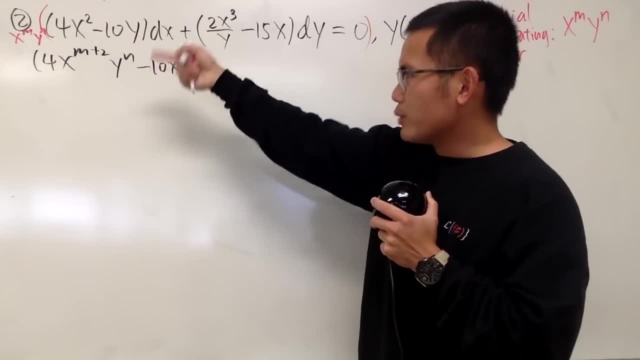 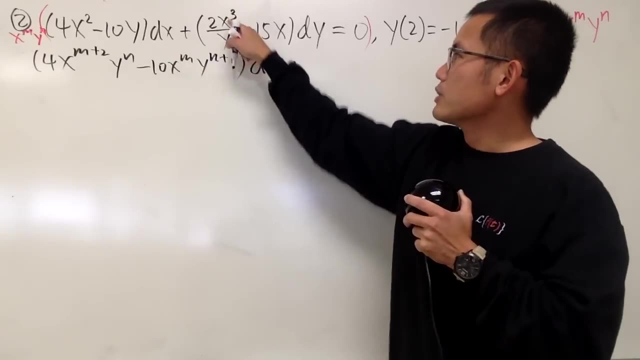 And then y to the n, So it's m plus 1.. So that's it for the first part. dx that, And then we add this, times that, So we have 2x3 and x to the m. Yeah, here. 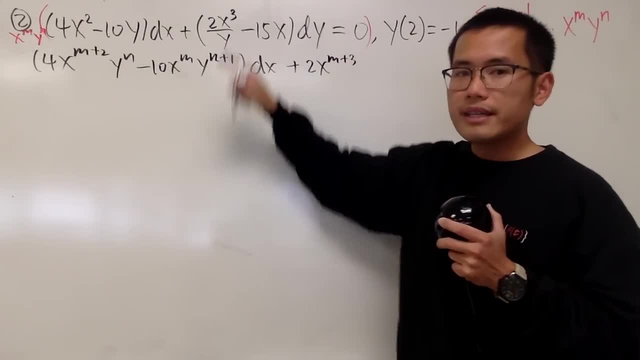 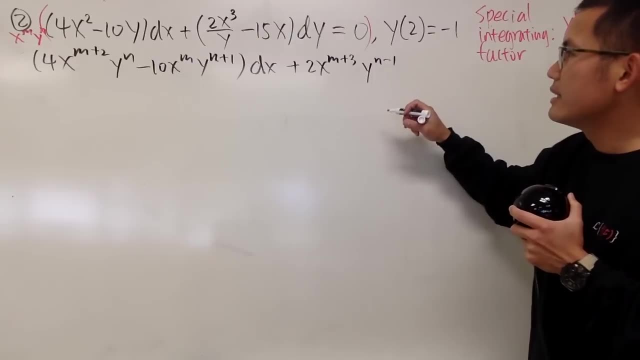 So we have m plus 3.. And this is y to the negative 1. And this is y to the n. So we have ym minus 1 times. yeah, just like that. And last part, we have minus 15x to the first. 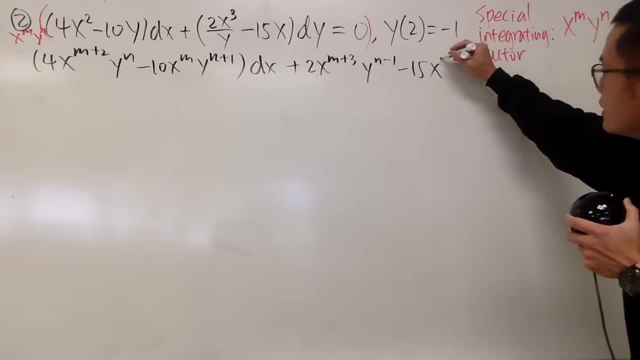 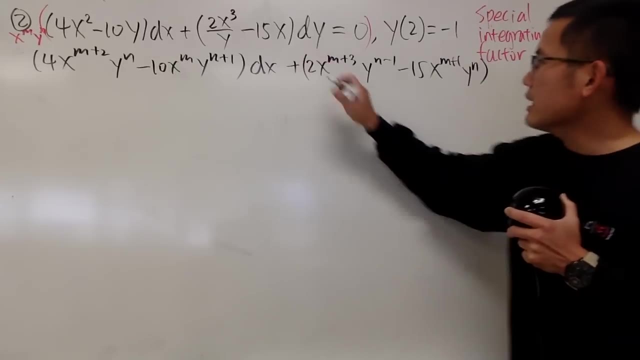 And that's m, So we have m plus 1.. And then we have y to the n, So that's the second part, And this is with dy, And that's equal to 0 times that, which is still 0, like this. 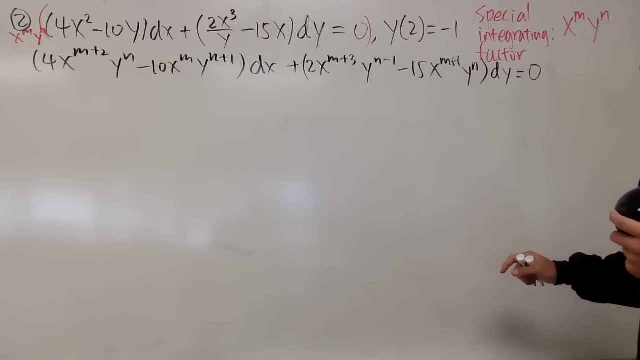 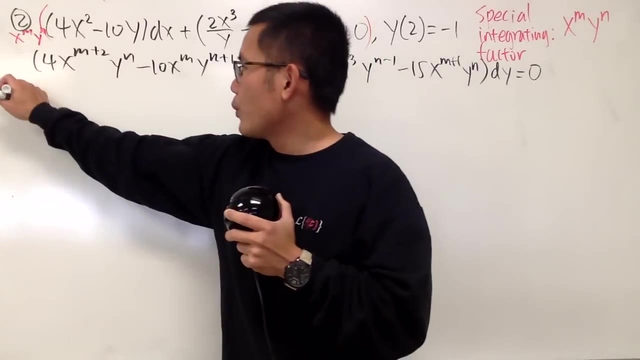 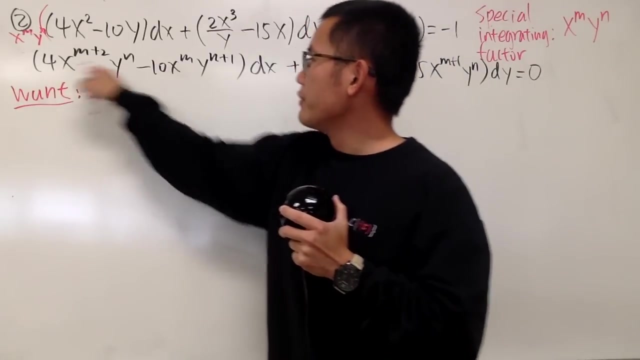 Let me just check, And I think this is okay. Now, this is how we are going to make this exact. Well, this is what we have to have in order to have this happen. Yeah, We want to have the partial of this part with respect to y. 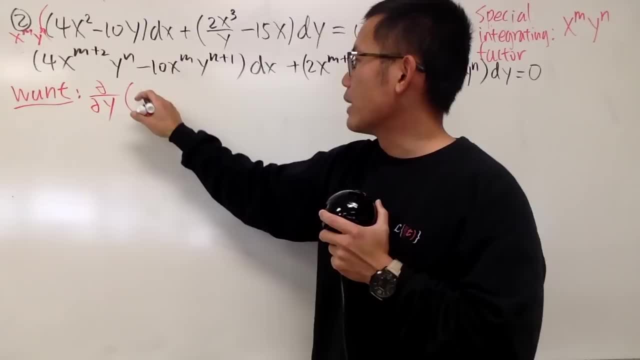 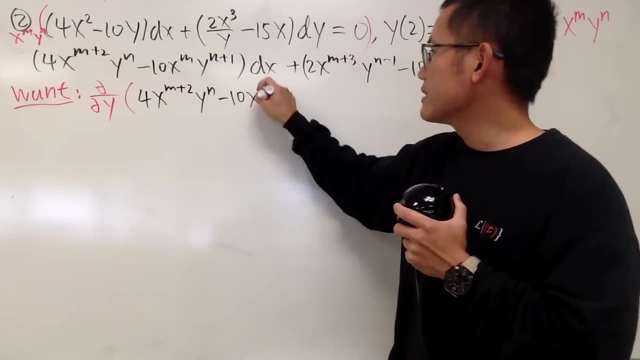 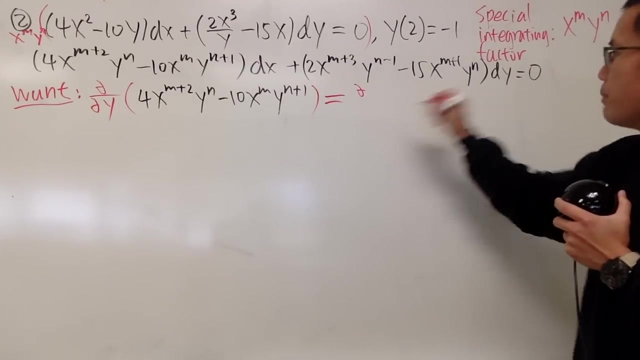 Again, you do the opposite. So I will just write this down, which is, again just write it down- 4xm plus 2. 2yn minus 10xm, ym plus 1. This part, we want it to be equal to the partial of this part with respect to x. 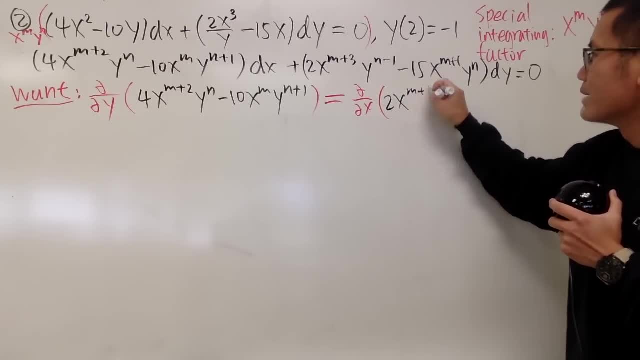 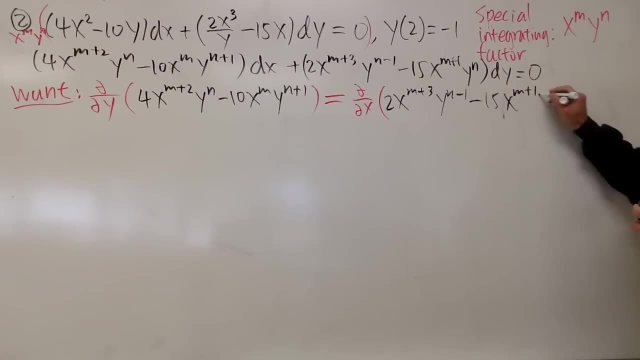 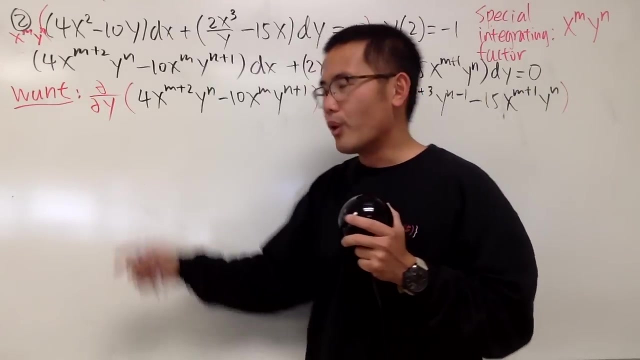 So let's see, Let's write it down: 2xm plus 3yn minus 1 minus 15xm plus 1yn, like so. So, yes, let's do our derivatives now, Differentiating this in the y world. 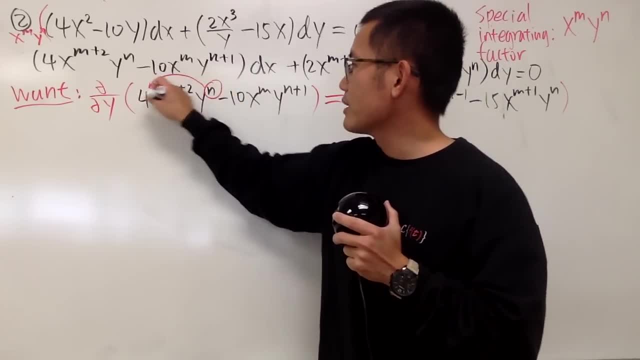 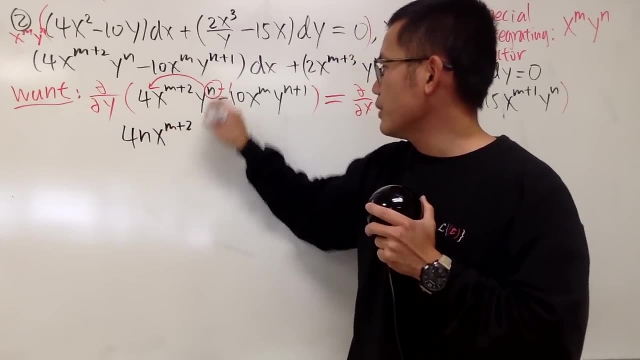 Here is the variable y and to the nth power. So I will just bring that down to the front and minus 1.. First part: we get 4nxm plus 2yn minus 1.. So that's the first part that we have. 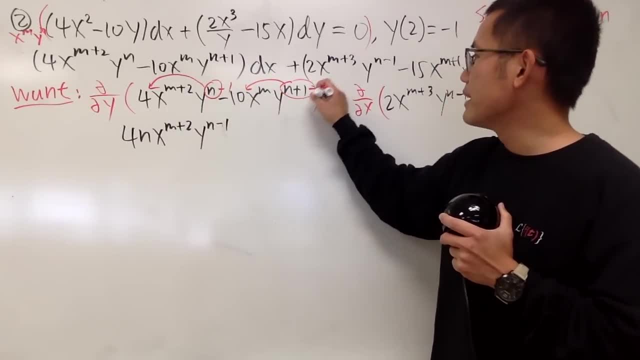 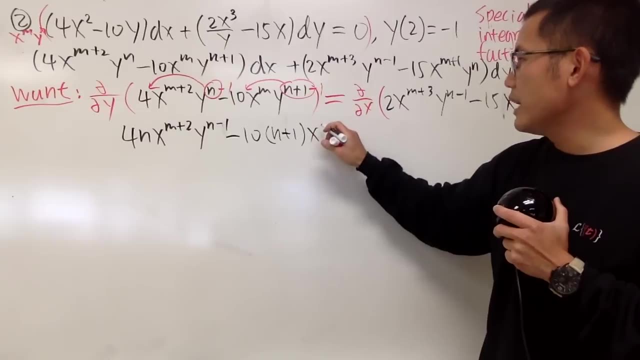 For the second part, I will bring this to the front and then minus 1.. So we have minus 10, parentheses, that m plus 1. And then we have x to the m And then y to the n, only because you know, minus 1 after that. 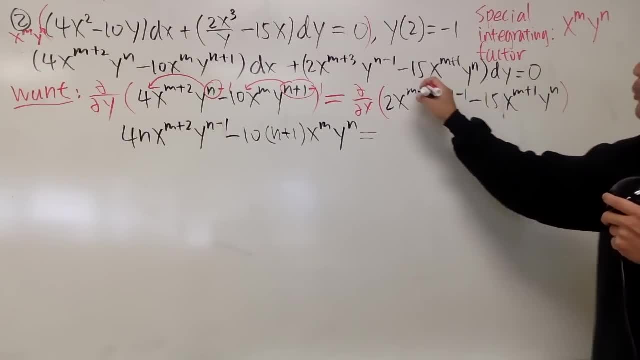 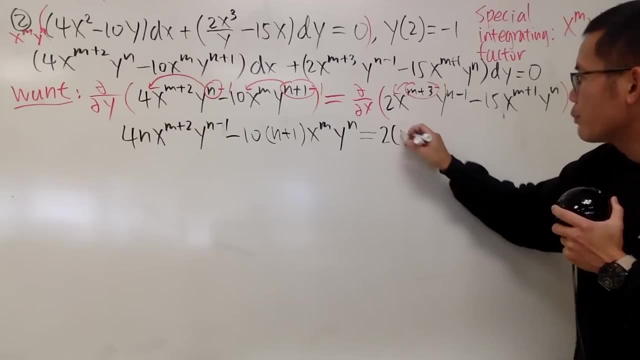 And again we have to make this equal to the right-hand side. Bring this to the front and then minus 1.. So you know, we're differentiating this with respect to x. So here we have 2, parentheses, m plus 3, x to the m plus 2.. 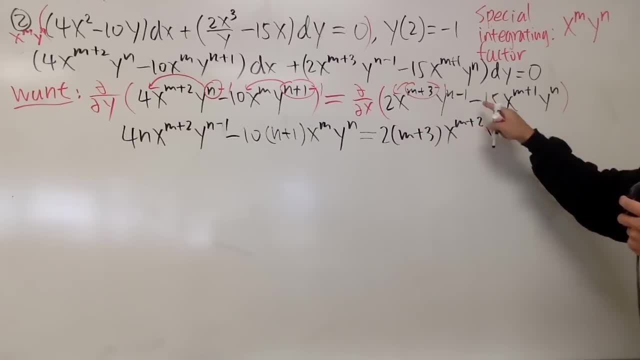 Good. And then this right here stays: ym minus 1.. And then, for this part, bring this to the front, and then minus 1.. So we have minus 15.. 15, parentheses: m plus 1.. And then x to the m, y to the n. 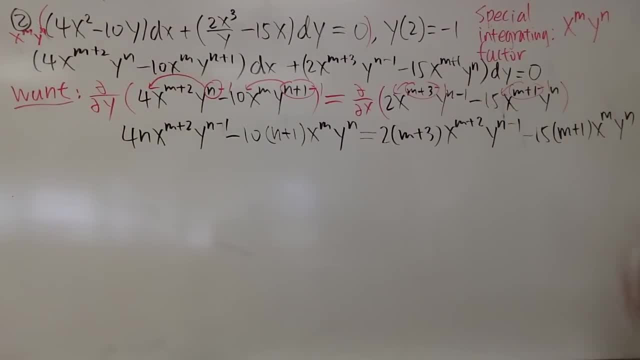 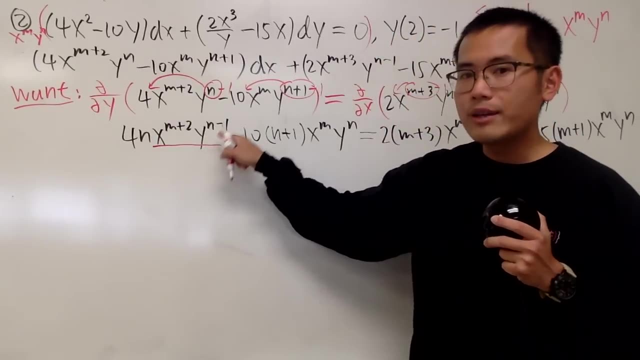 Phew, like this right, So have a look. Now. here's a good thing. You see this part. this is x to the m plus 2,, y to the n minus 1.. It matches with that. That's good. 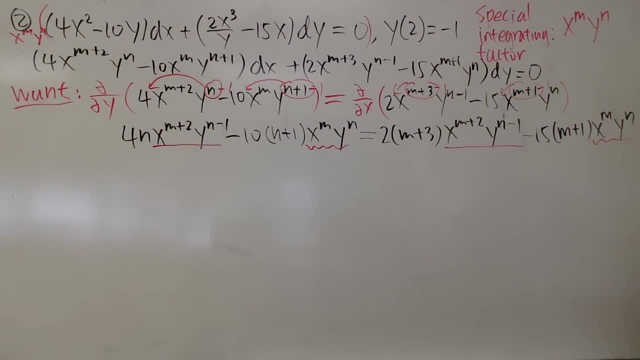 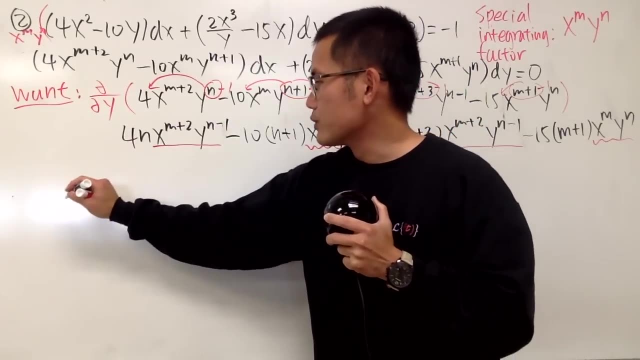 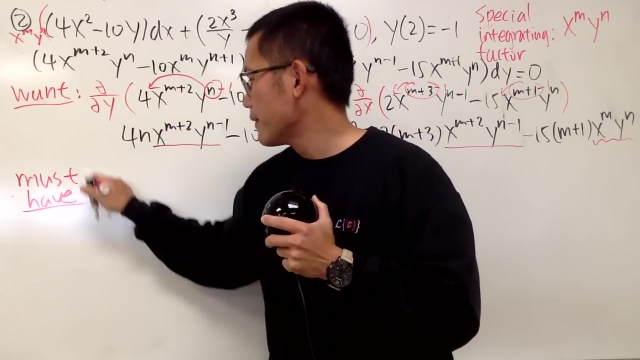 Likewise, this matches with that. So what that means is that the coefficient of those terms have to be equal. In another word, first we must have- I'll just write this down: We must have, must have the following: First thing I need to have 4n being equal to what we have right here. 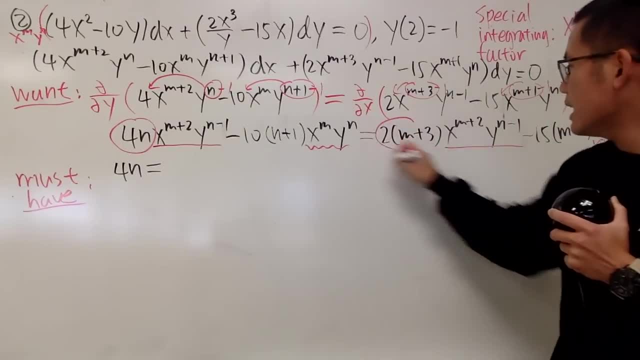 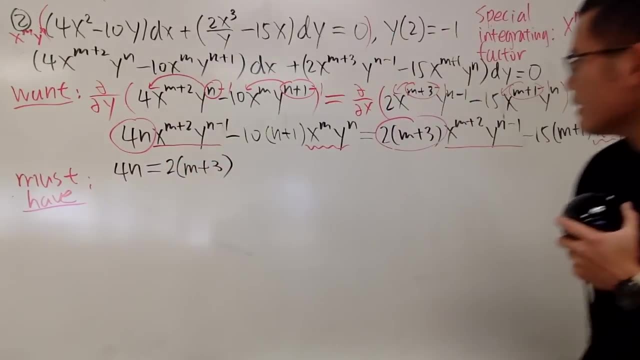 So, again, this has to be the same as that, And of course I will just multiply this out. Why not? Actually, I'll just put it down and then we'll multiply it out in our head. Next we have this: 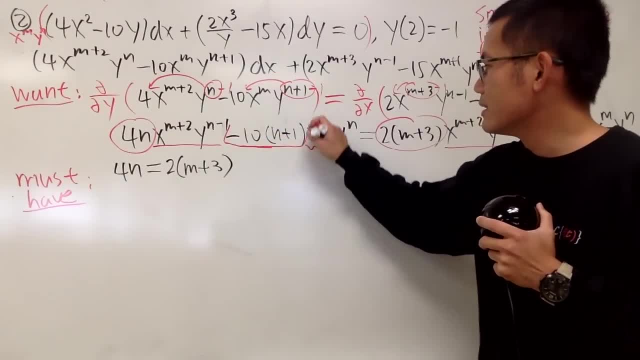 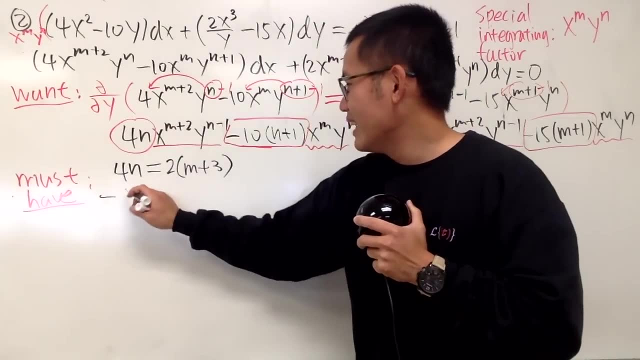 Actually, don't forget the negative. So we have: this Has to be the same as that. Well, thankfully they're both negative, So you know they cancel each other out. That's nice. Anyway, I'll still put the negative though. 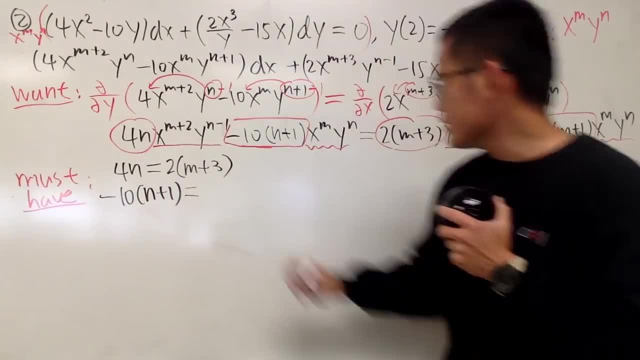 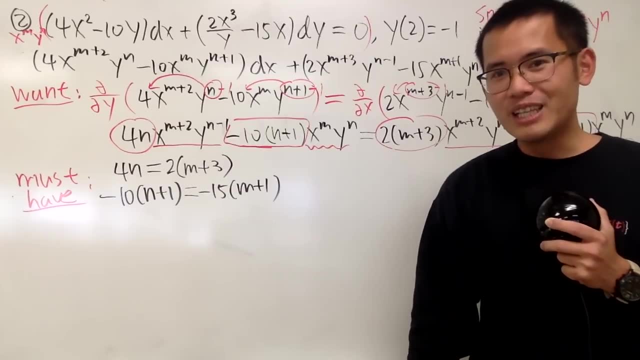 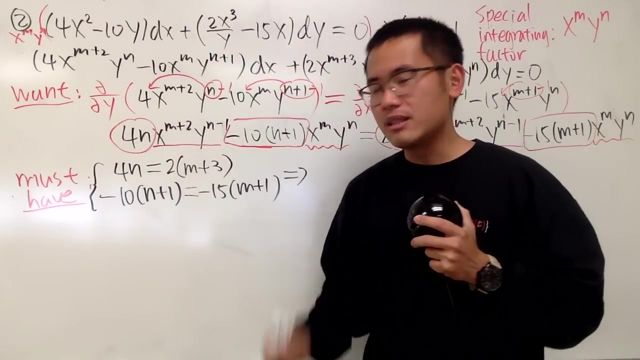 Negative 10 n plus 1 equals negative 15 m plus 1.. Like that, Yes, system of equations in the differential equations. Yes, let's go ahead and do that. This is just a baby system of equations And let's put things in order. 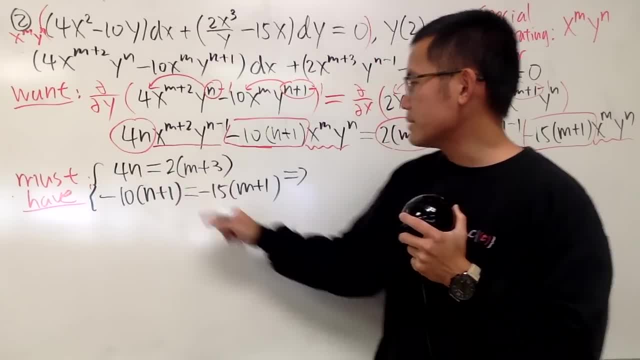 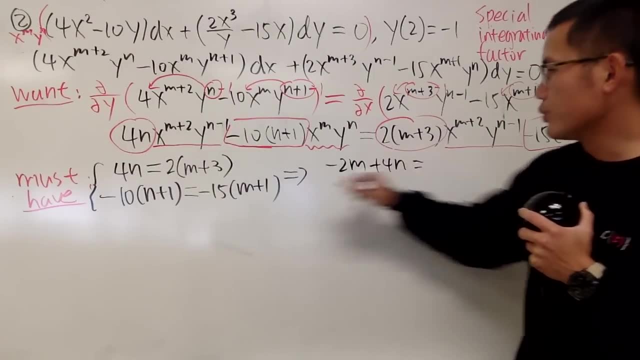 So I will put down: m goes first, So this is 2 times m. Kick that to the other side, We have negative 2m plus 4n And that's equal to 2 times 3, which is 6.. 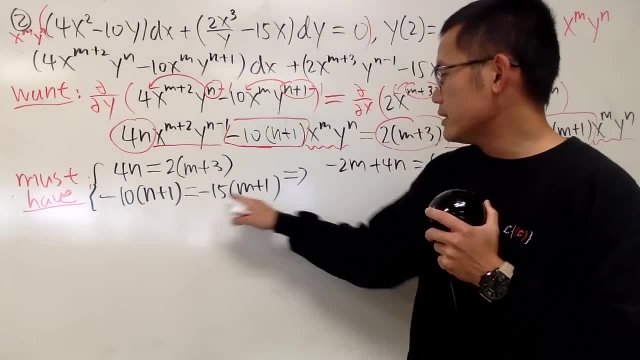 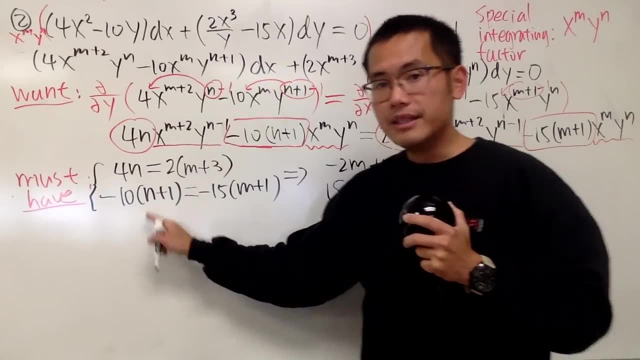 And for the second equation, this is negative 15m. Kick that to the other side Becomes positive 15m, Yeah, And then we have this and that which is negative 10n, And that's equal to this, and that is negative 15.. 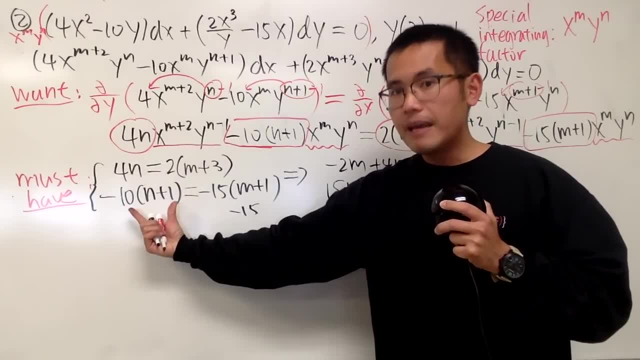 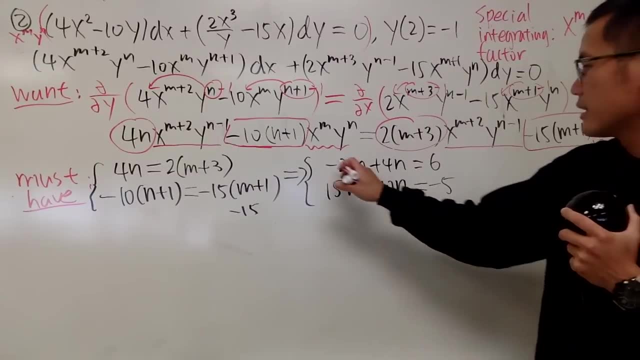 Bring it down. This and that is negative 10.. Add the 10 on both sides, we get negative 5.. Yes, Now let's see, Let's multiply the top and bottom. Let's see, I want to get rid of the n. 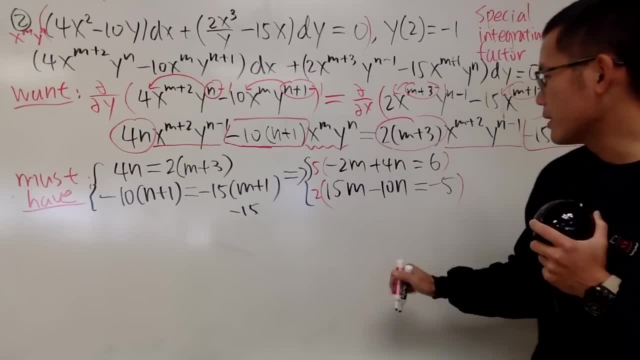 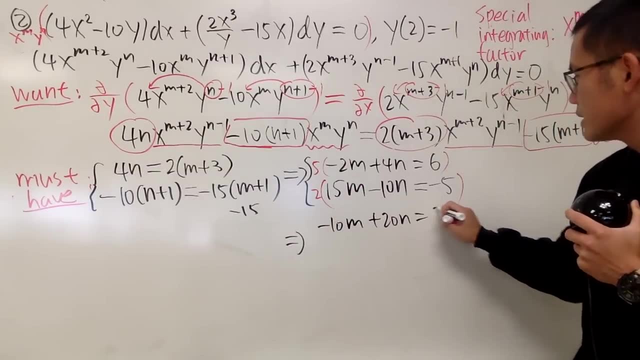 It's easier. So let's multiply the top by 5 and then the bottom by 2. So we get the following: We get negative. 10m plus 20n equals 30. And this- and that is 30m minus 20n- is equal to negative 10.. 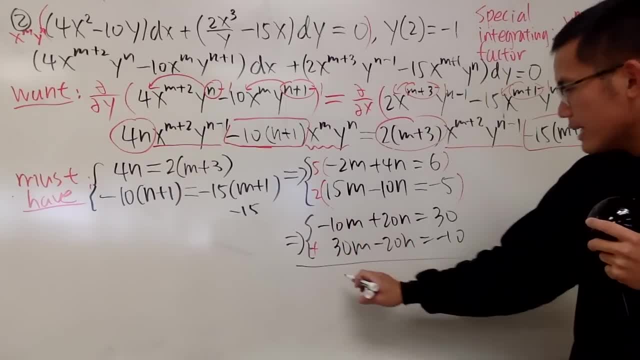 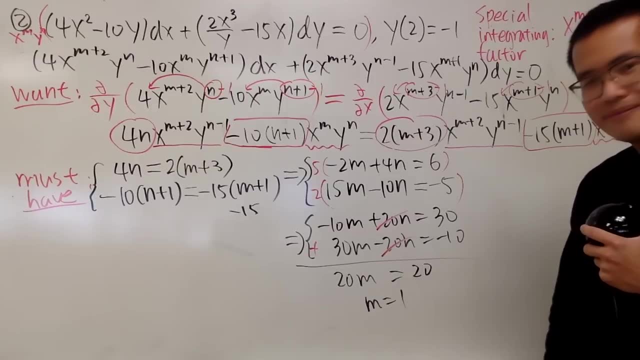 And let's see, We add: OK, All that is 20m. This is equal to They cancel And we get 20.. So m is equal to 1.. Seriously, All the work for m is equal to 1.. 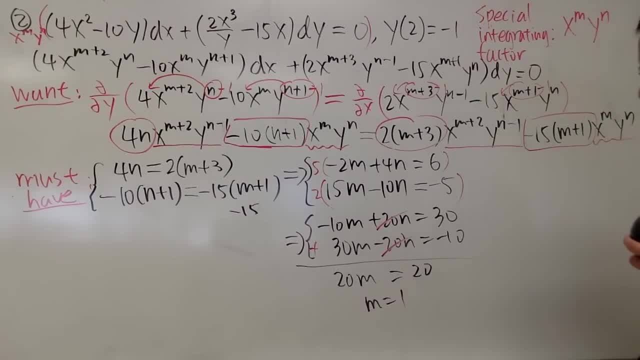 Don't tell me n is equal to 1.. Seriously, All right, Otherwise I'll just feel so sad. Anyway, m is equal to 1. And I'll just plug it into whatever equation I want. So that's it, right here. 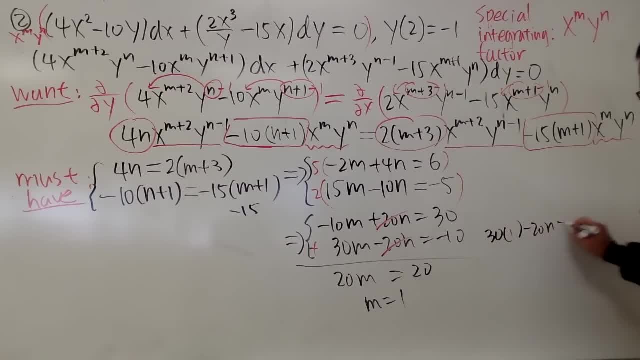 So we have: 30 times 1 minus 20n is equal to 1.. OK, 1tn is equal to negative 10.. So let's do this in our head: This is 30 minus what will be negative 10?? 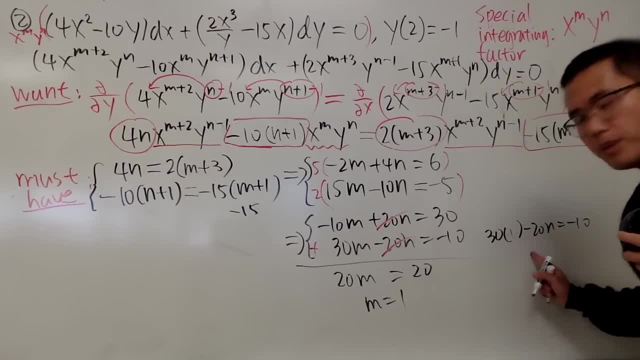 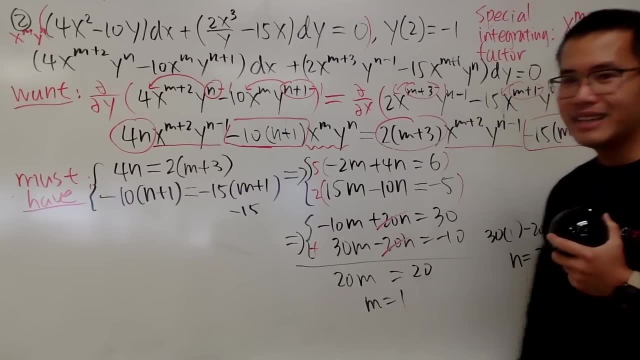 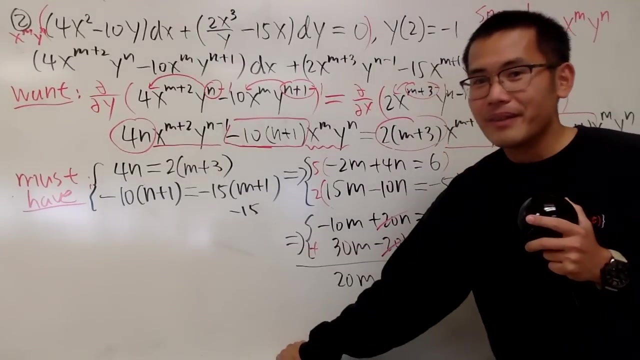 30 times 30 minus 40 will be negative 10. So that means n is equal to 2. m is 1.. n is equal to 2. And in fact we're not done yet. So now, what we know is our special integrating factor. we know: 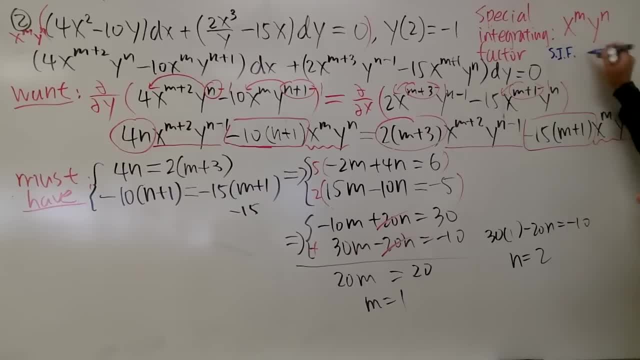 I'll just put on sif Like this: It's going to be x to the first power, y to the second power, right, Because we found it, We made that happen, So of course I need more space. Let me just erase all that. 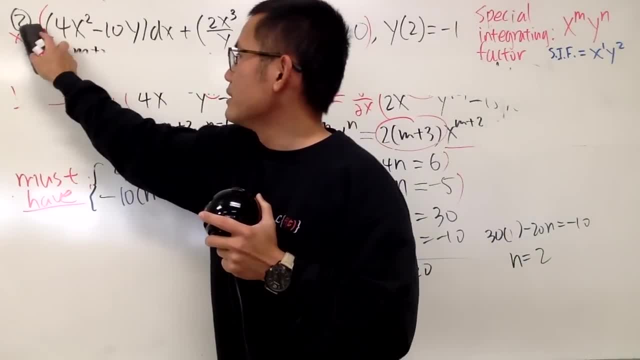 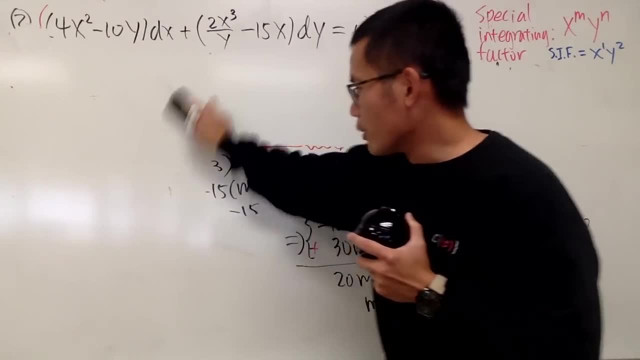 And then, don't forget, we still have initial condition to handle. So this is not a short question, of course, And again, for the purpose of the integrating factor is that we'll multiply everybody by that, And then it will become exact. 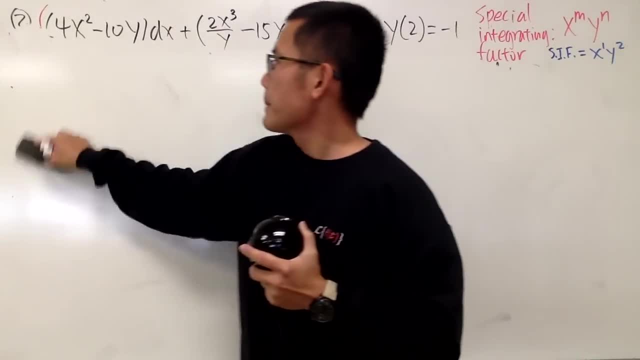 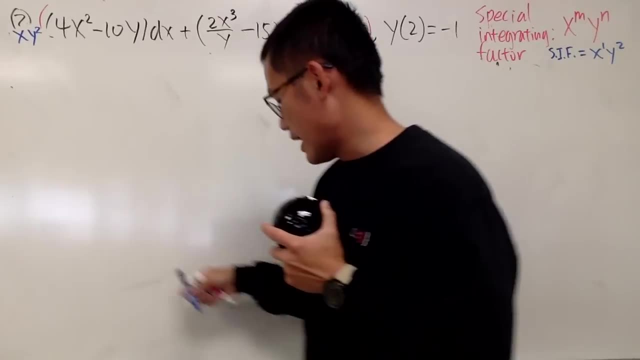 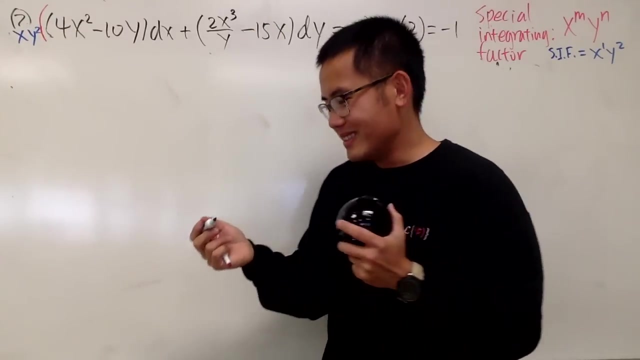 So this is the special integrating factor. This is the special integrating factor. OK, So here we go. Let me just write it down. We multiply by x to the first power, y squared like so, And then let's go ahead and just do the crazy algebra and all that stuff. 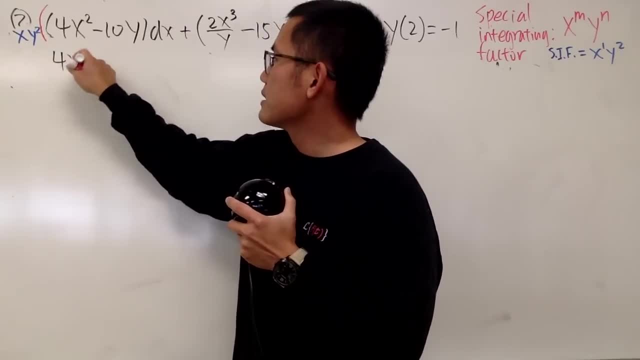 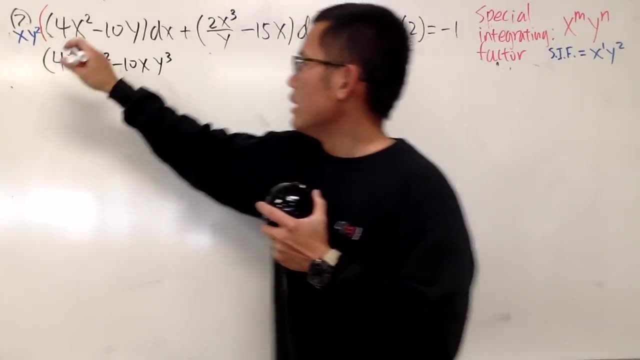 Anyway, here we go. This times this: we get 4x to the third power, y squared- and then minus 10xy to the third power, Yes, Times dx plus. this times that We have the y's cancel out. 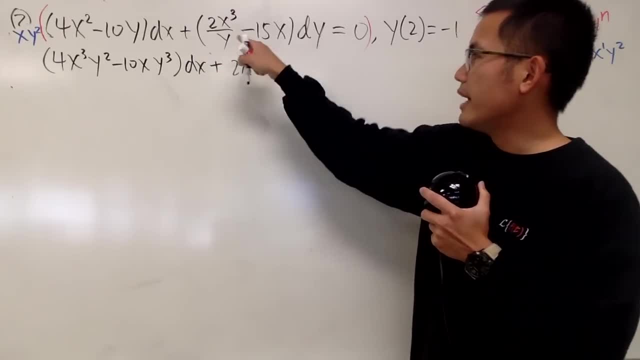 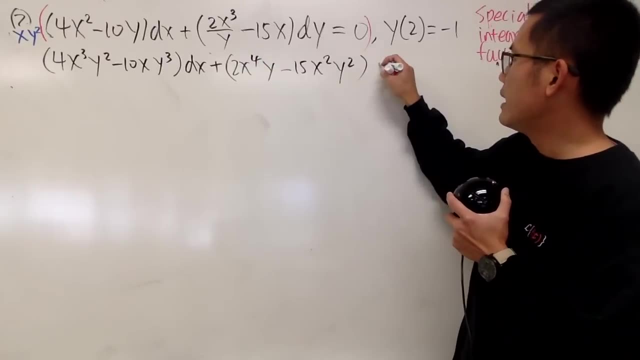 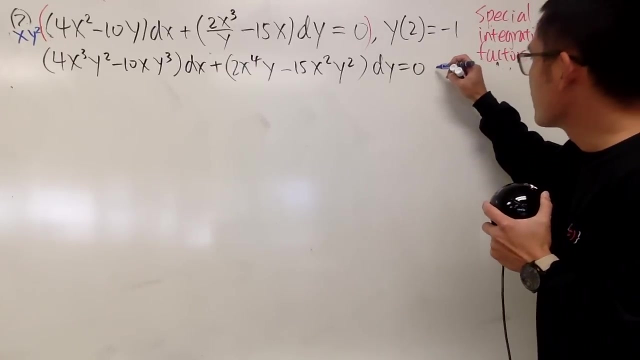 We have 2x to the fourth power, and then 1y left, And then minus 15x, squared y, squared, like all this And divide that, and this is equal to 0.. And I will promise you after all this, of course, this right here has to be exact. 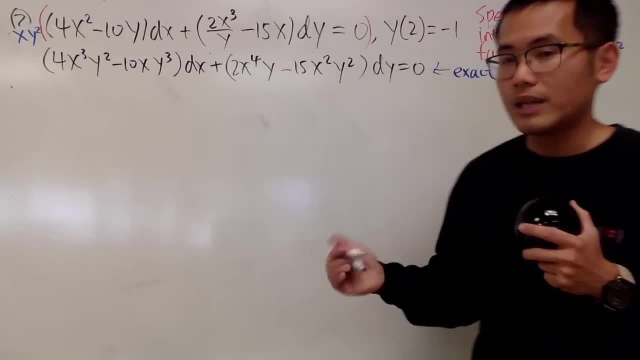 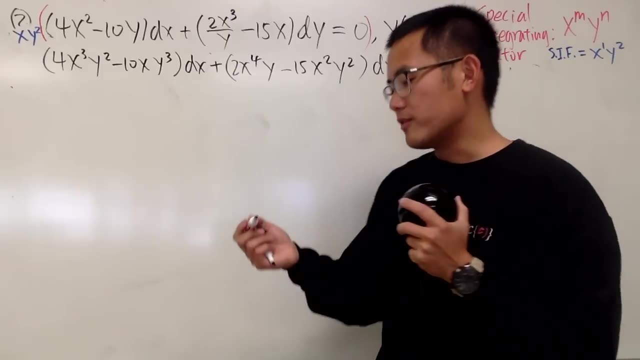 Right Guaranteed. And, of course, if you want to do the check, go ahead and do that. But I know for sure, So we'll repeat what we did earlier. This represents the total differential of some multifarible functions. capital F. 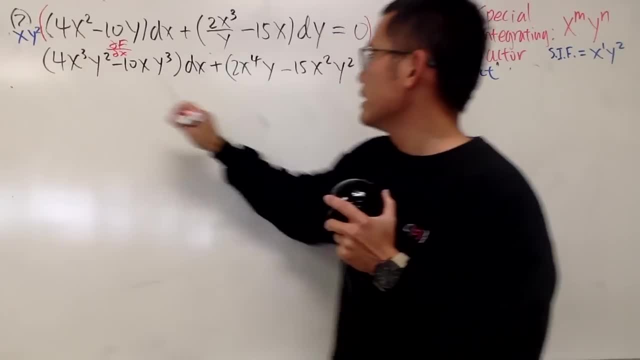 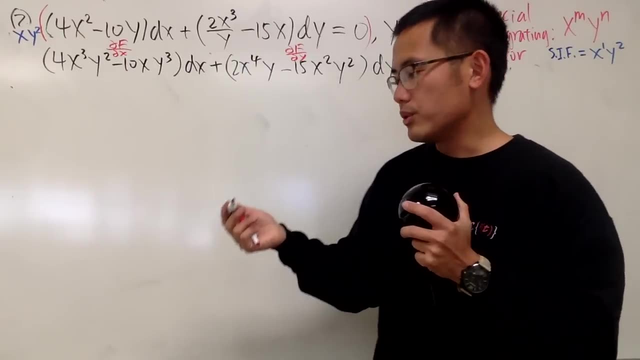 So I'll just say this is the partial of capital F with respect to x, And likewise this is the capital F with respect to y. Right And again, depends on which direction you want to do it. Maybe I'll just show you guys, if you want to start right here. 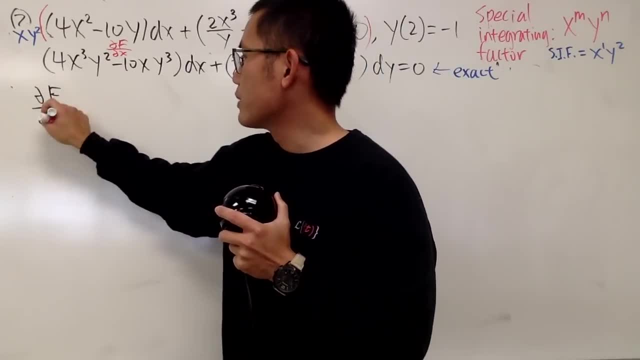 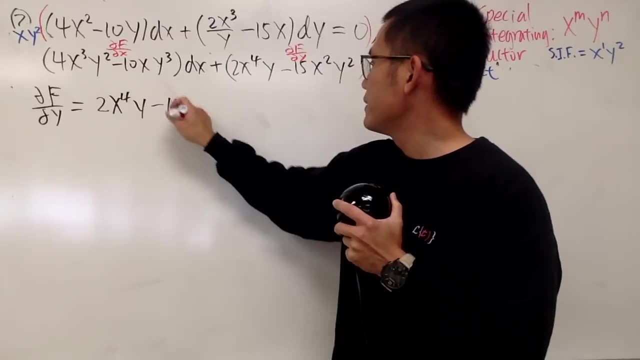 That's totally OK. So partial F with respect to y, this is equal to that. Now you know for sure. So this is 2x squared, This is 2x4 minus 15x2y2.. And then let's go ahead, integrate both sides. 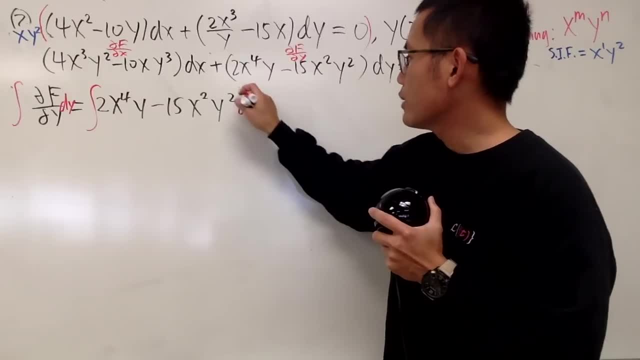 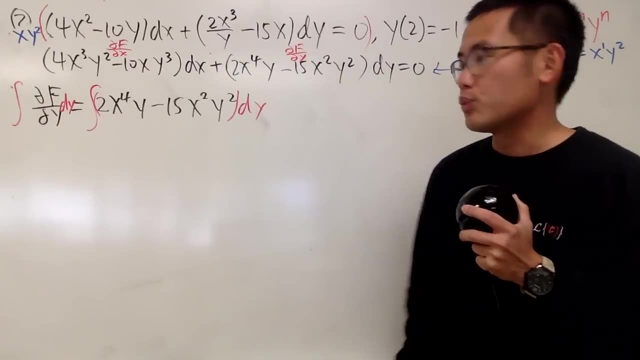 And we have to do this with respect to y, So you have to really know which part you are picking, And then you know this was with respect to y, So you have to integrate it with respect to y. Anyway, so here we go. 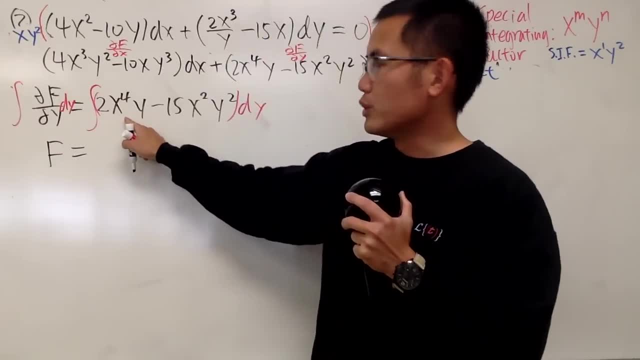 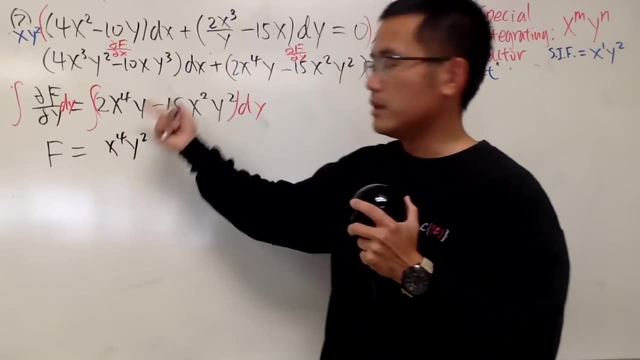 On the left-hand side, we get the capital F And integrating this with respect to y, you just get this is going to be y squared Right, And then the x to the fourth power is just going to be, you know, staying the same. 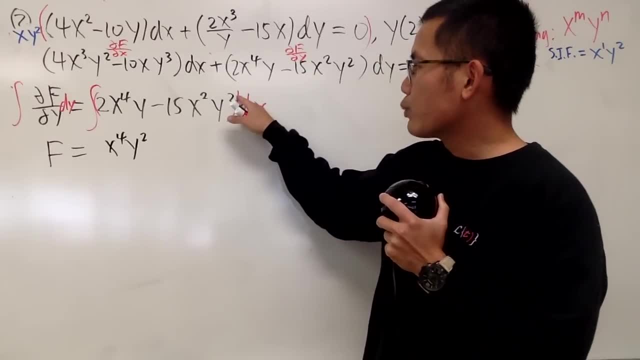 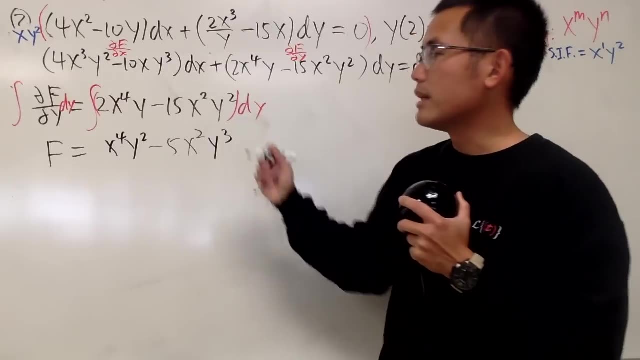 It's the constant multiple, And for this we have to add 1 here, which is 3. And then divide it by that, which is going to be minus 5.. This stays x squared y to the third power, like this: 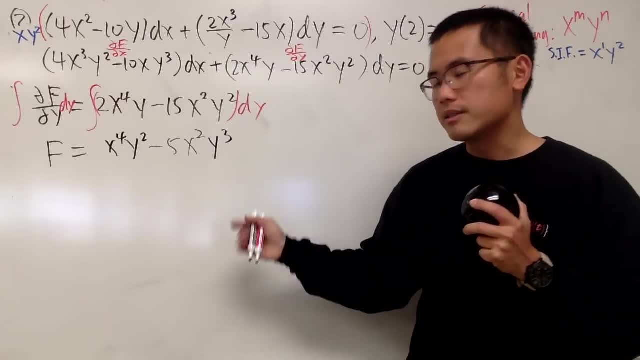 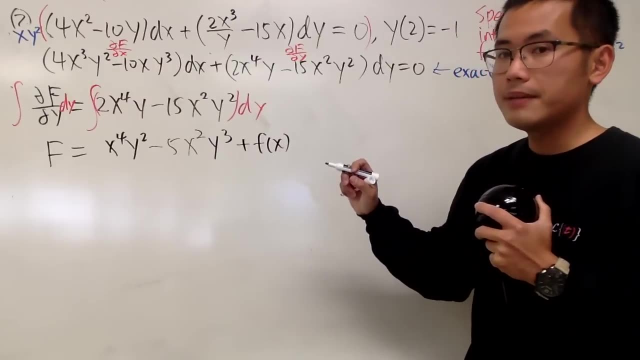 Now, in the y world, x is considered constant, So we'll add some function in terms of just x. So I will put an F of x like this Right. Well, to figure this out, all we have to do is just go ahead and do the partial with respect to x. 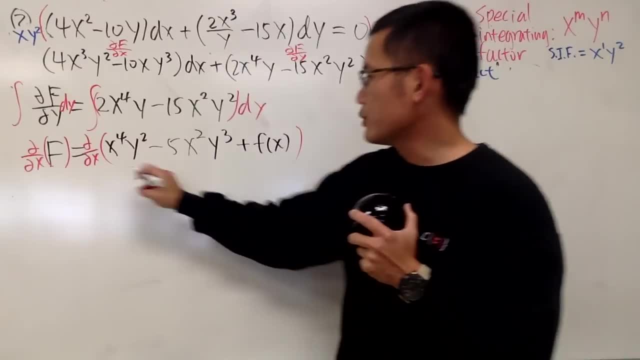 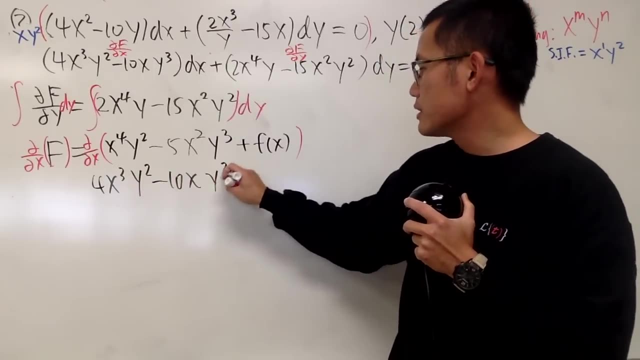 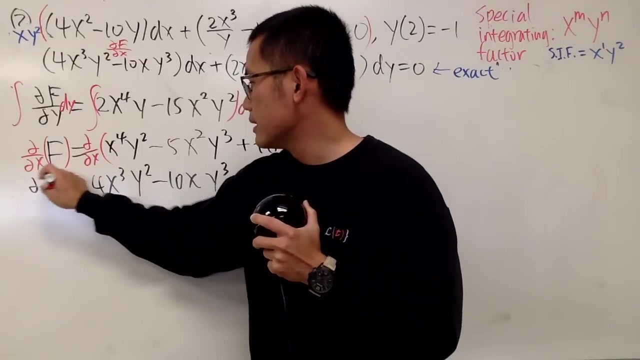 On both sides. So you see, when we do that, we get 4x to the third power, y squared stays, And this is minus 10xy to the third power, plus F prime of x. This, right here, is our partial of F with respect to x. 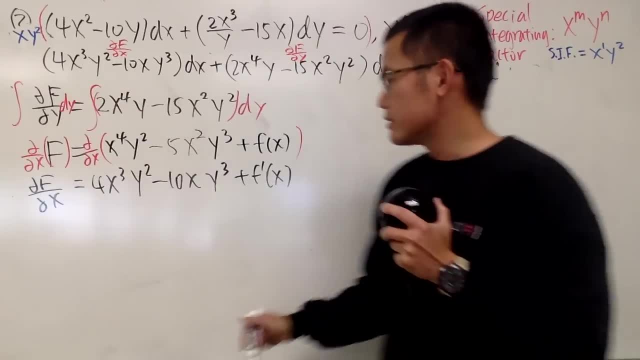 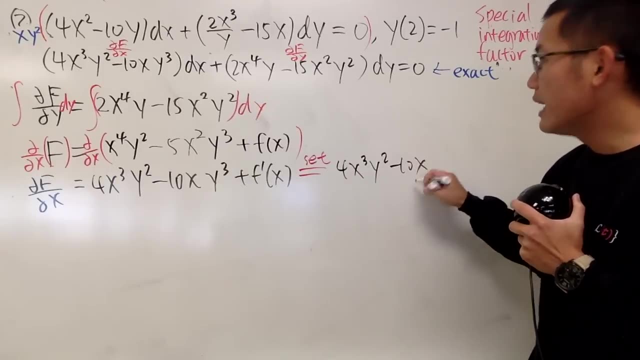 And this part has to be the same as this, Right? So we have to set Again. we have to set: This is equal to 4x cubed y squared Minus 10xy cubed, And the good thing is that this matches with that. 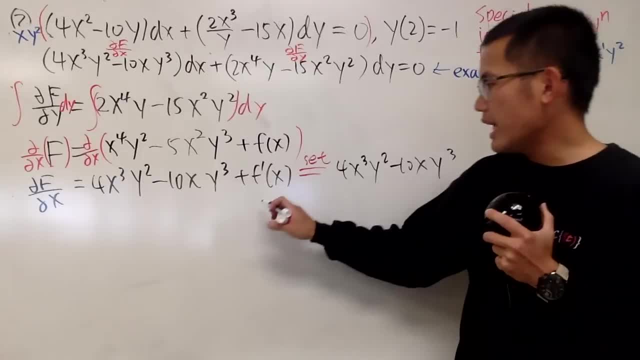 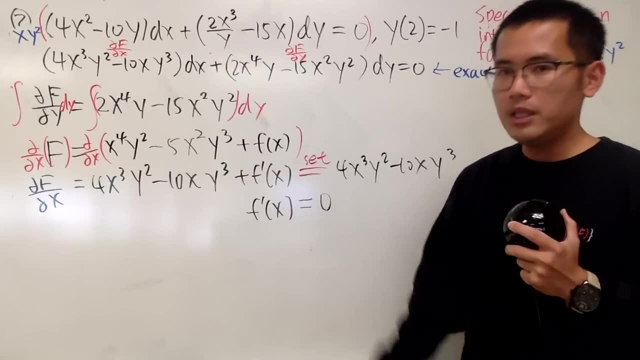 This matches with that. So again, in this case, F prime of x has to be equal to 0. And now you might be wondering: is this always going to be equal to 0?? Not necessary, Because you can imagine if I have plus sine of x right here, for example: 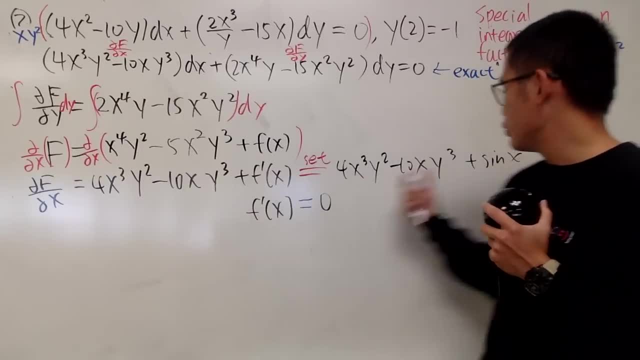 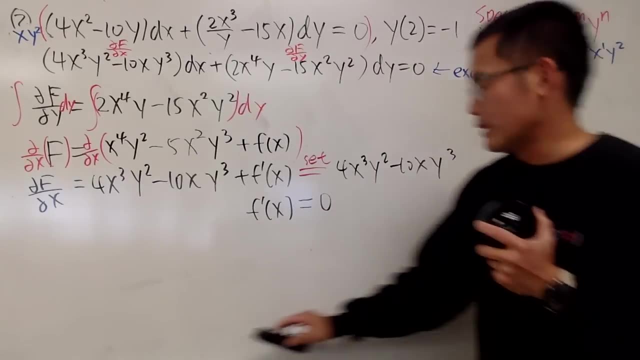 Then you will have to set F prime of x to be this sine x, And you just have to integrate that. And I do have another example in that situation, But that will be for later on. So in this case, though, it is equal to F, prime of x equal to 0.. 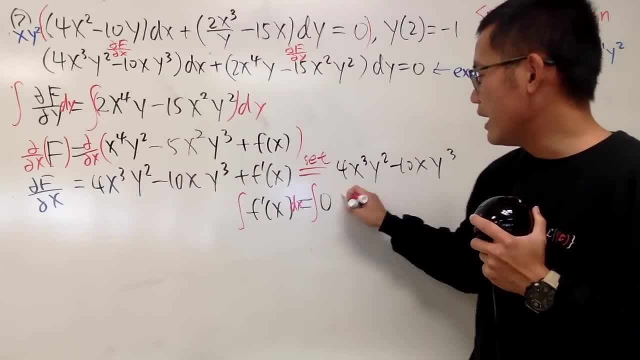 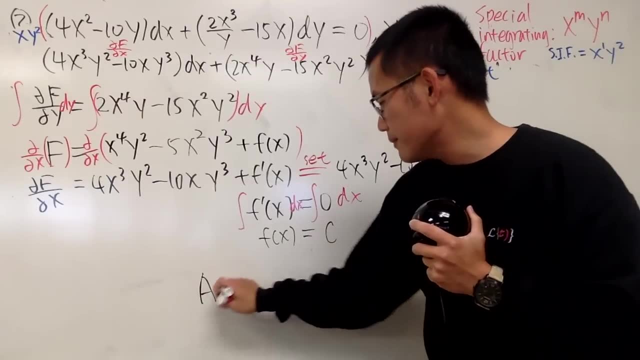 And, of course, just go and finish that, Integrate both sides, And that means our F of x, little f of x, is just a constant c. So now let's write down the answer. All we have to do is the following. 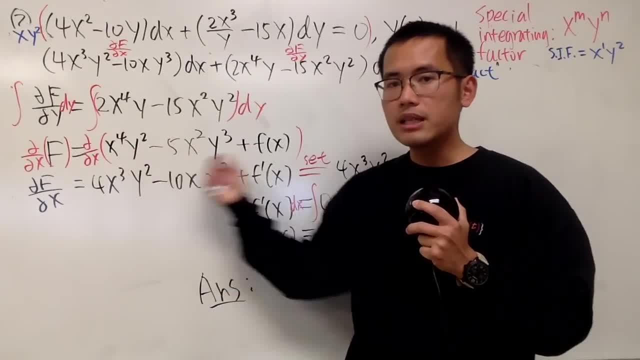 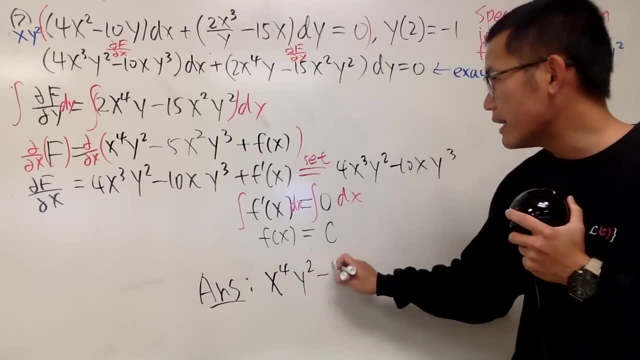 Look at the capital F. This right here is the function part. This is just a constant Kick out to the other side. So I'll just put this right here: x to the 4y squared minus 5x squared. y to the third power. 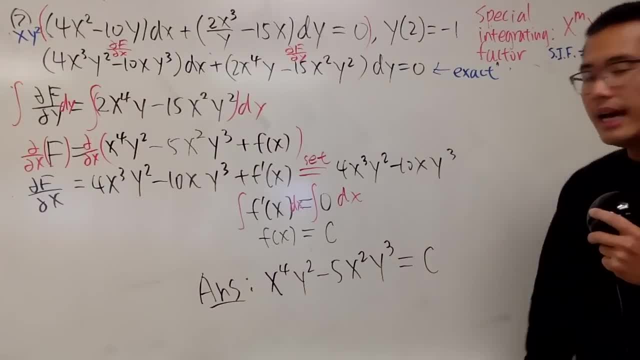 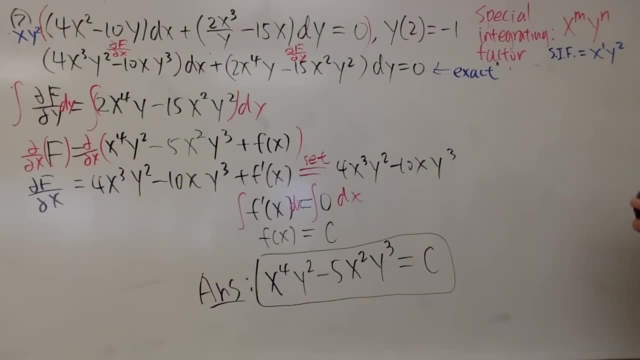 And again I will just say that's equal to the constant c. And guess what We are done? Let's see how long this took. Yeah, 15 minutes or so. So it's just like this right: The longer the question, the better. 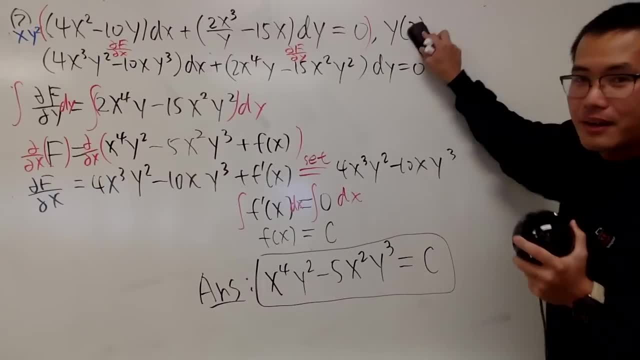 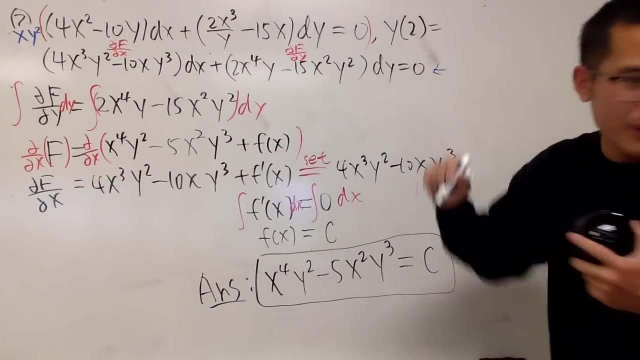 So anyway, this right here is it, But this is not it. Sorry, sorry, sorry, sorry, sorry. Initial condition: Sorry, my bad. And y of 2 is equal to, I forgot That's negative 1.. 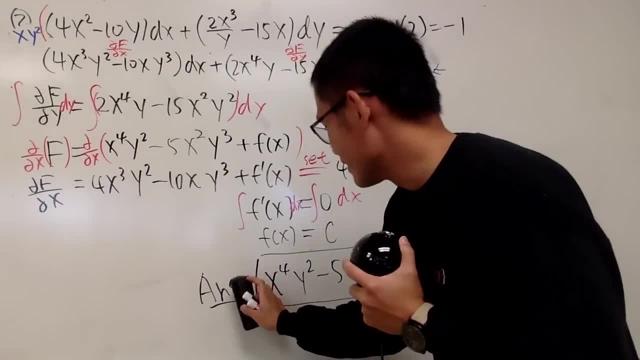 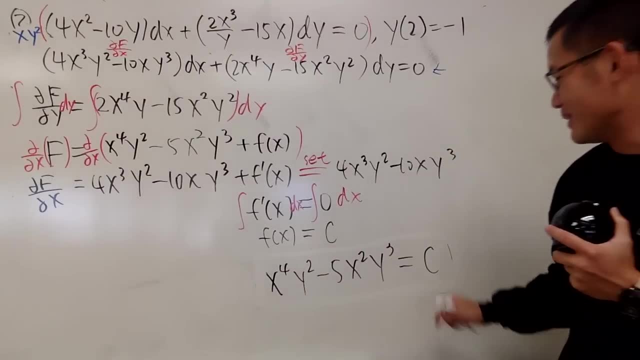 Almost forgot, Almost forgot. So this is not the answer yet, So I'll just write this down right here. Sometimes you get too excited, You just seriously forget about what happens. All that stuff, All right. So when we have initial condition, 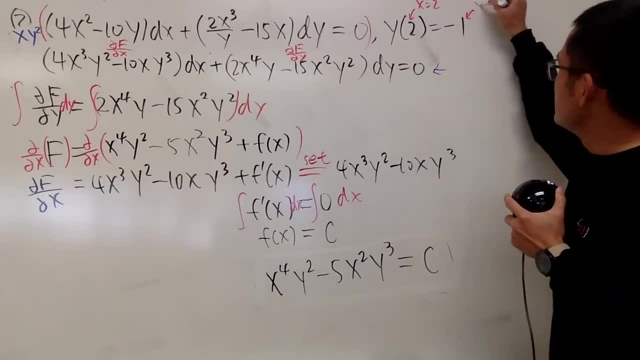 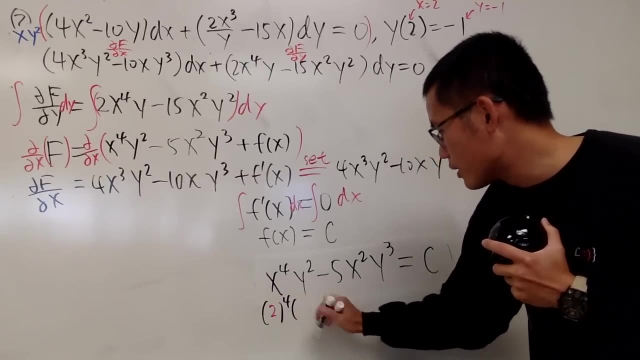 this means when x is equal to 2, y has to be negative 1.. Yeah, So I'll just put this down right here. We have 2 to the fourth power, negative 1 squared minus 5, fourth power: I mean 4 to the second power. 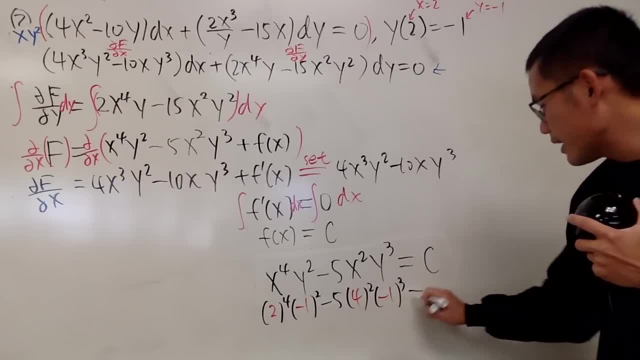 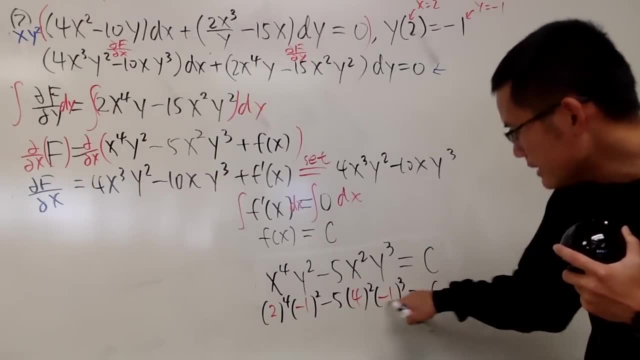 and then negative 1 to the third power, And that has to be equal to the constant c And of course you can just work this out- This is going to be 16 plus- Oh sorry, This is supposed to be 2.. 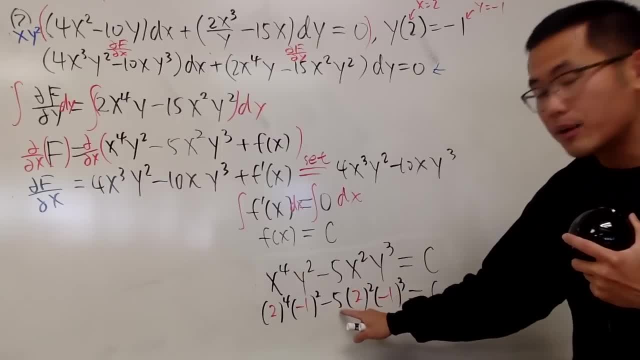 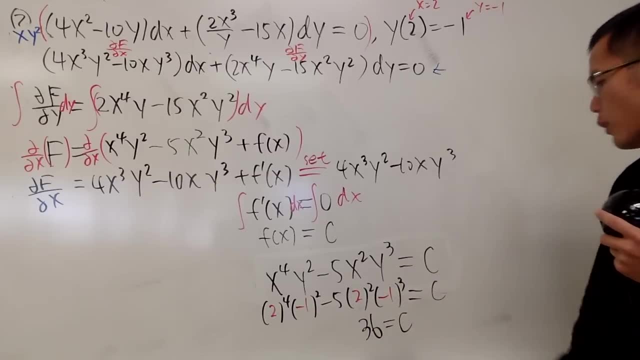 x is 2.. Plus this right here is 4 times that, which is 20.. So altogether this is 36 equals c Right. And this right here will also explain the following right. Let me just write it down. 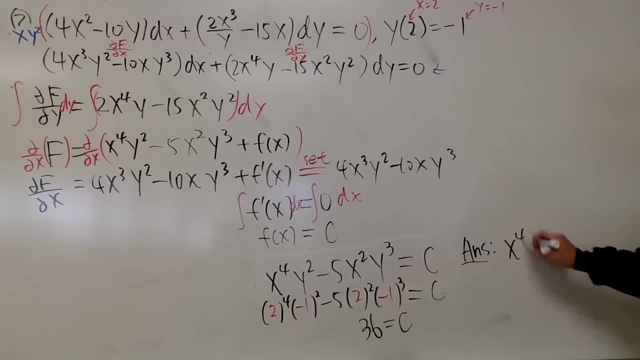 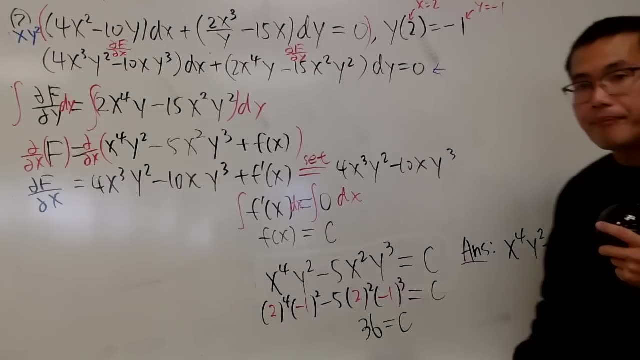 The answer is going to be this: which is x to the fourth, y squared minus 5x squared y to the third, power equals 36.. Just like that, And earlier, if you put the c on the other side. 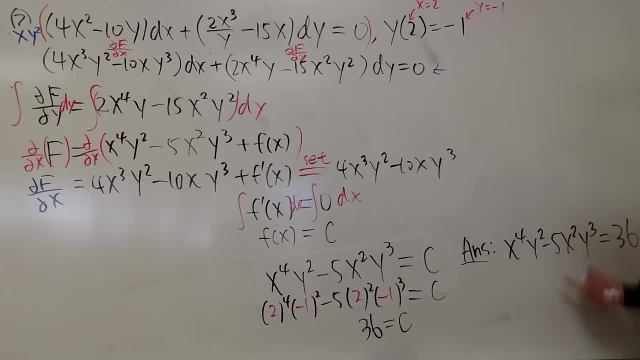 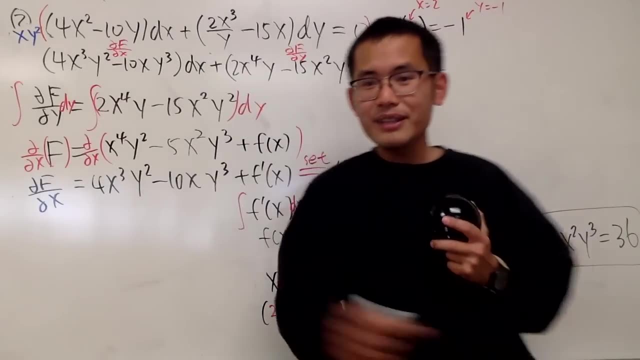 you would just end up with this minus 36,, which is equivalent. So that's why we can always just put a constant on the right-hand side, like that. Right? So that's the idea. So have a look, Have a look. 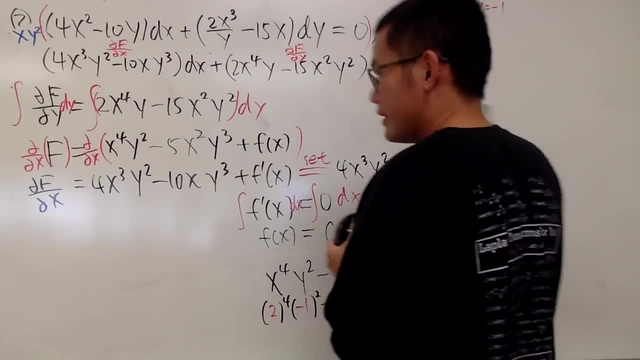 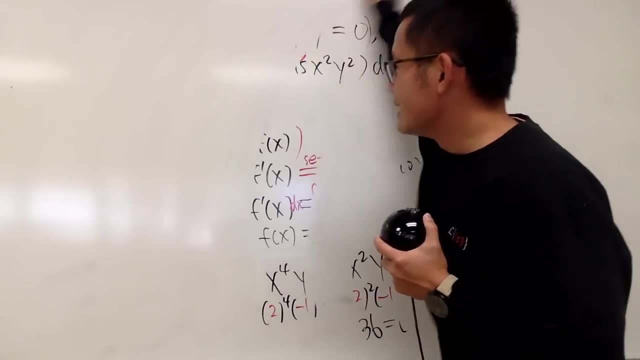 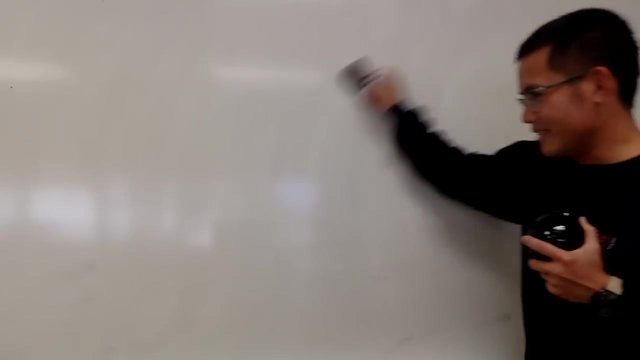 This is the final answer. All right, good, And now let's see. We have 22 more to go. We have a lot more to go, actually. In fact, this is not the first time doing this, because, in fact, yesterday I did it. 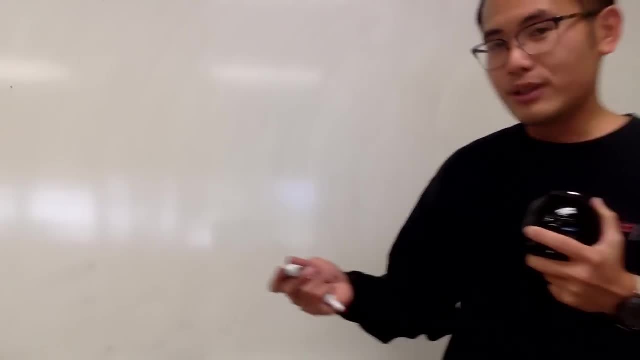 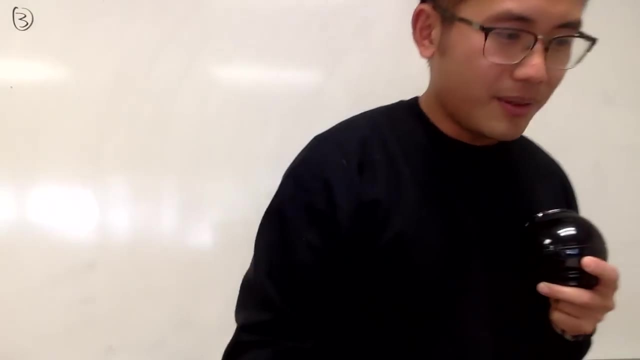 and I wasn't so happy so I stopped it somewhere. I will upload a video if you guys want. So I kind of just spent, Spent two hours, almost two hours, and didn't satisfy. I was not satisfied, so I will do it today. 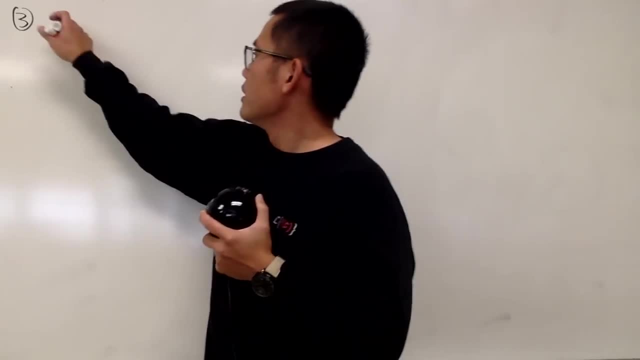 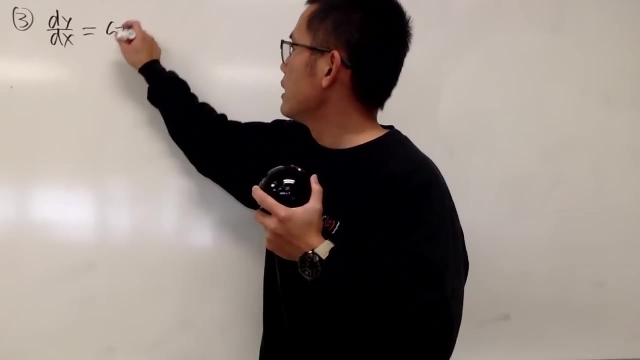 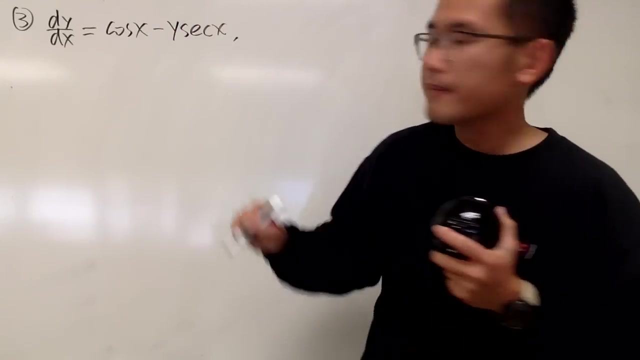 Anyway, here we have this Number three, dy dx. Ooh, the dy dx is by itself. and then we have cosine x minus y, secant x, And this is also an initial value problem. so we have: y of 0 is equal to 2,. 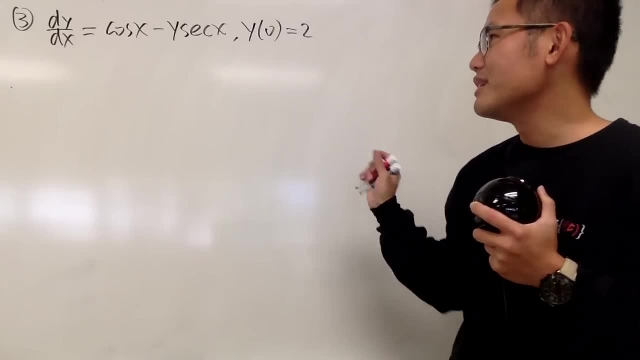 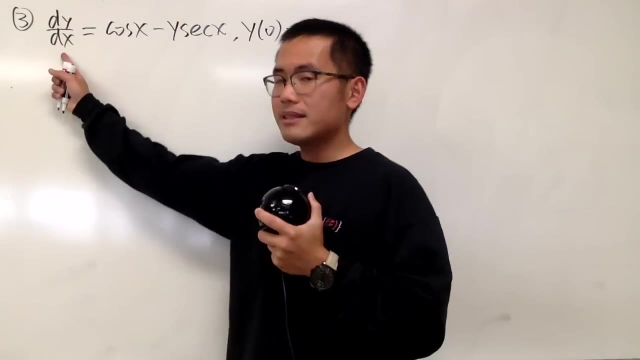 and now remember that will actually solve this before I erase any part of the answer. All right, so now? what kind of equation is this? Have a look, We have dy, dx, and this right here is y to the first power. 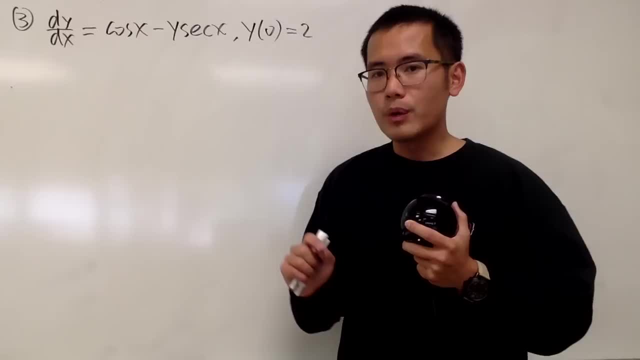 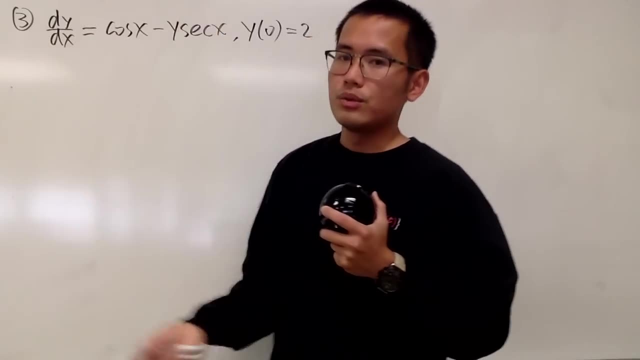 and there's no other y anywhere. This, right here, is what we call the first-order linear differential equation: y to the first, dy, dx, of course that's to the first. So in that case we can do the following: Let me bring this to the other side. 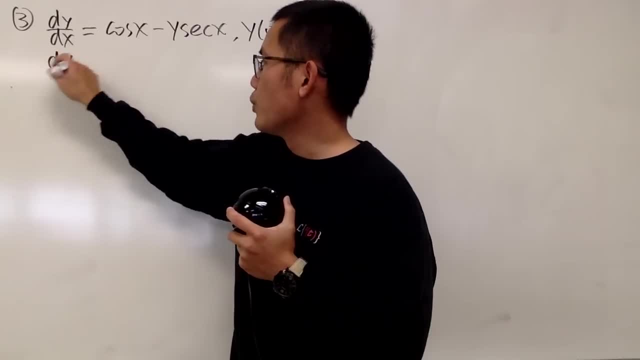 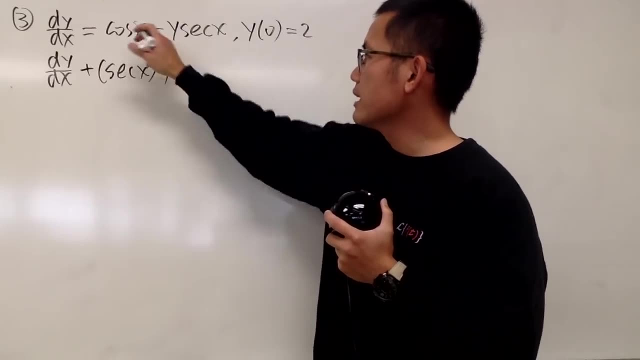 so we can put this in the standard form. I'll write this down for you guys: dy dx. and then we add- let me put down parentheses- secant x and then the y after this, and that's equal to cosine x. 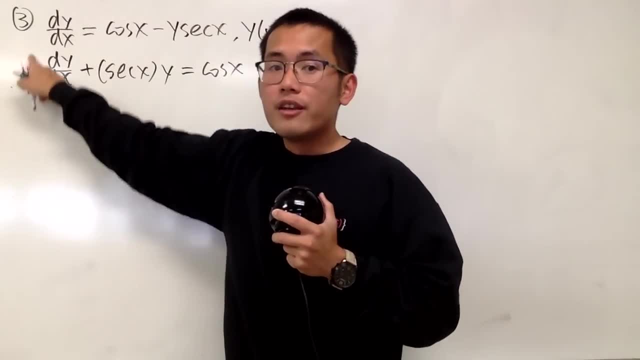 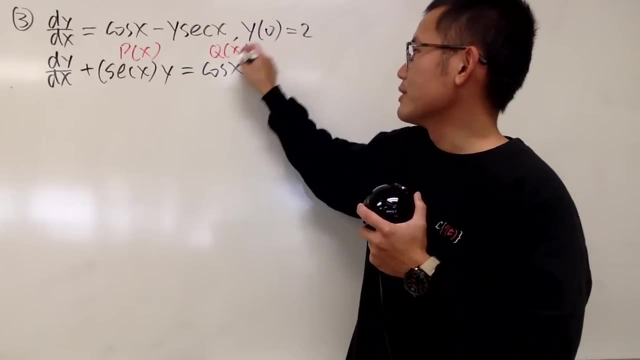 This right here is the standard form One in the front of dy dx. This part is called capital P of x and this part right here is called Q of x, which is actually doesn't matter, just a name For this kind of situation. 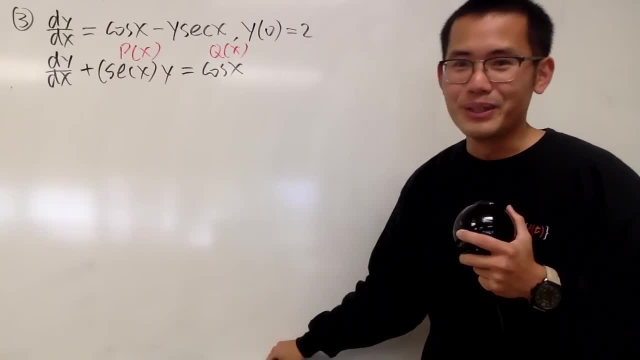 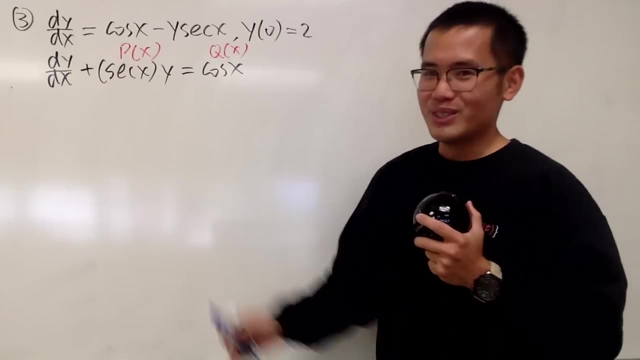 what we are going to do is integrating factor, But this one is actually not so bad because we actually have a nice formula. It's going to work every single time, unless the differential equation is not solvable with regular functions. But anyway, I'll write down the formula for you guys. 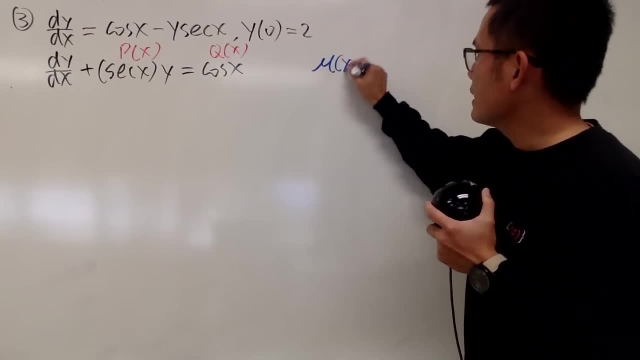 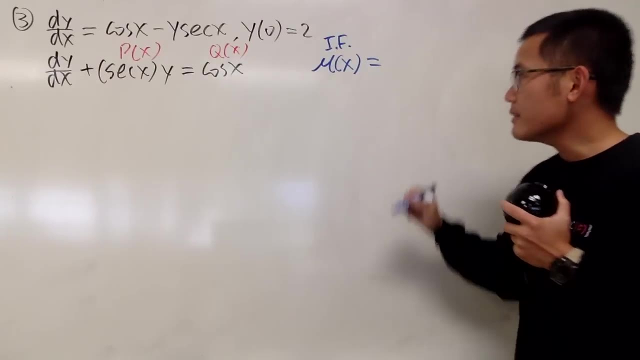 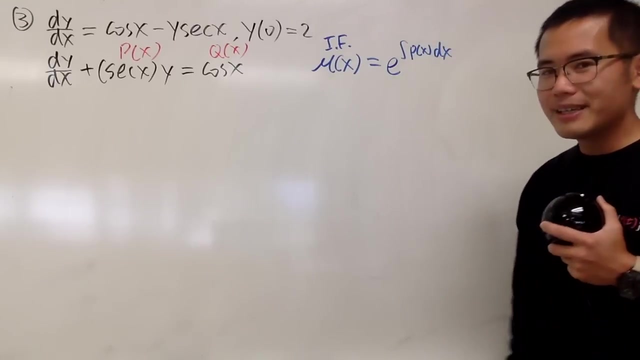 and I'll put this down right here: Mu of x- that's the notation for the integrating factor- is e raised to the integral power of P of x, like this- And you guys can see my old videos- I proved this three years ago already. 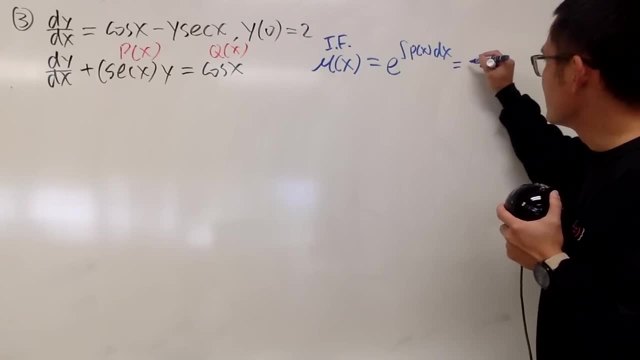 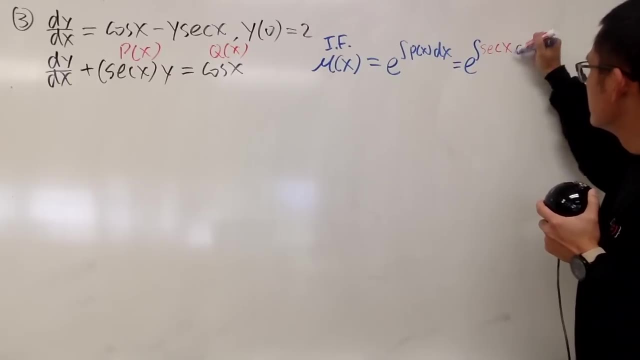 so go and check that out to see how we can do that. Anyway, all we have to do is integral, I mean e, to the integral power of secant x, dx, Because, remember this, right here is our P of x And you really have to make sure that. 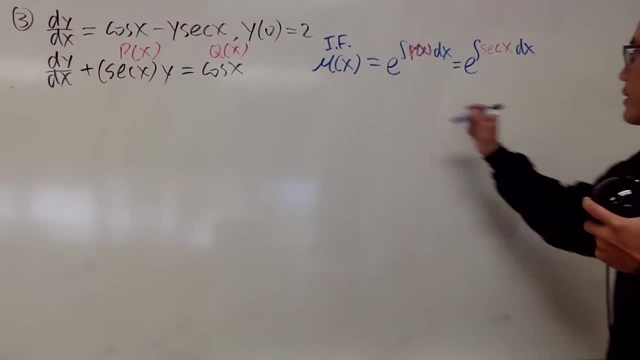 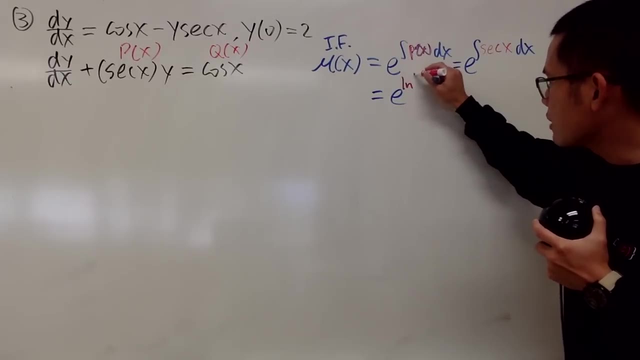 we have a one in front of the dy dx, which we do. that's good, Alright. so e is just e. and then integrating secant x. that's a standard integral, which is just natural log: absolute value: secant x plus tangent x. 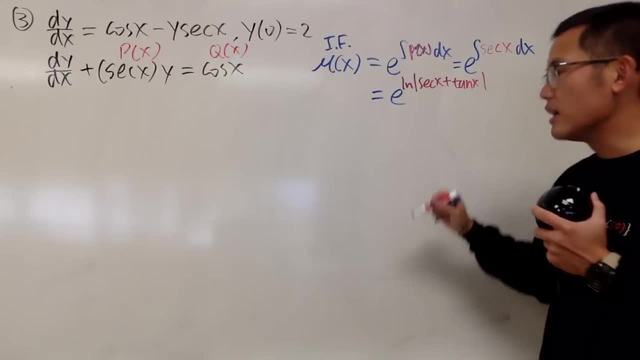 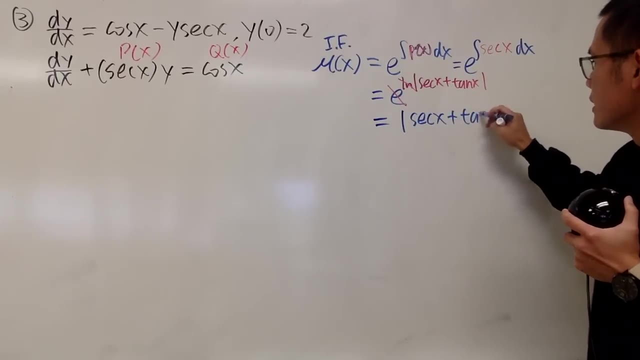 like this: And, nicely enough, this and that will cancel each other out. So finally we get absolute value, secant x plus tangent x like this. Now here's the deal. You can actually just get rid of the absolute value. 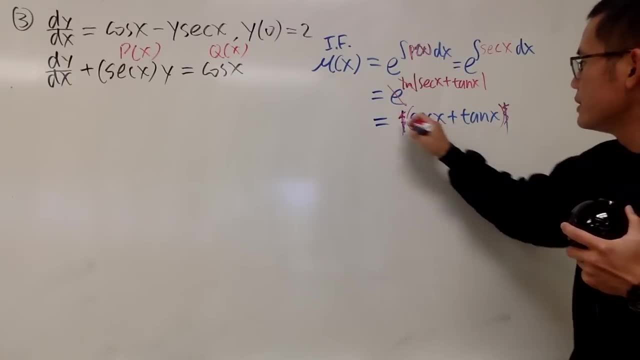 But when you do that, of course you have to just put this as plus minus. And now you have two choices for the integrating factor: Either the positive version of this or the negative version of this, And let me tell you, both of them will work. 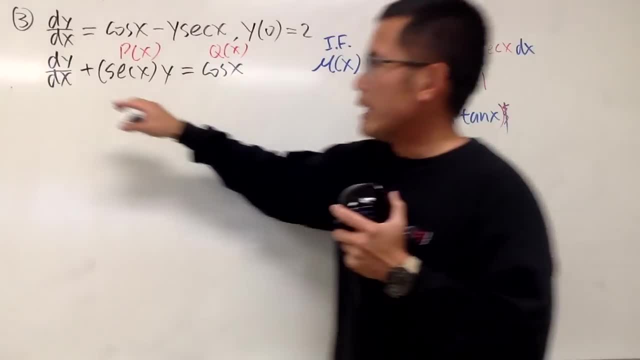 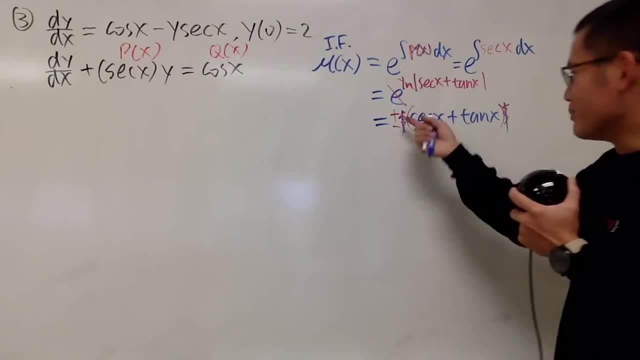 If you use the negative version, that means you multiply this by a negative, by a negative, by a negative. all we have to do is divide everybody by negative one. So it's the same as you multiply by the positive version. So in fact, I'll just use 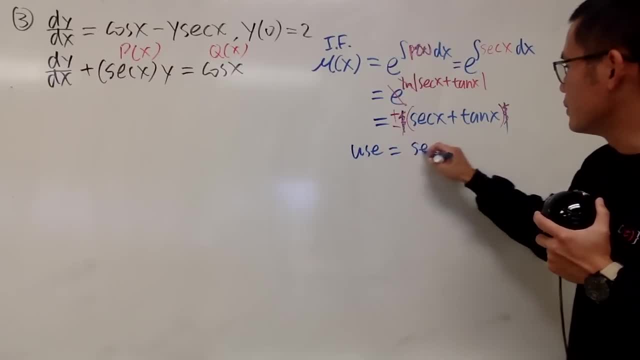 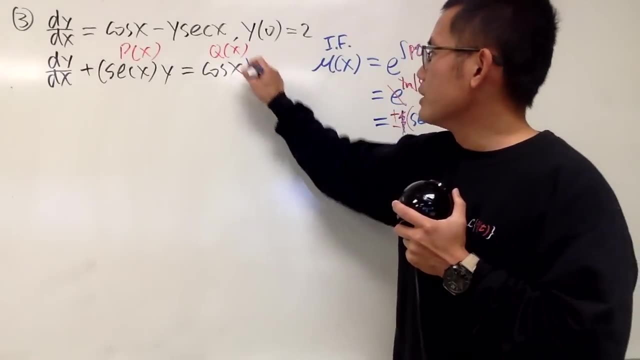 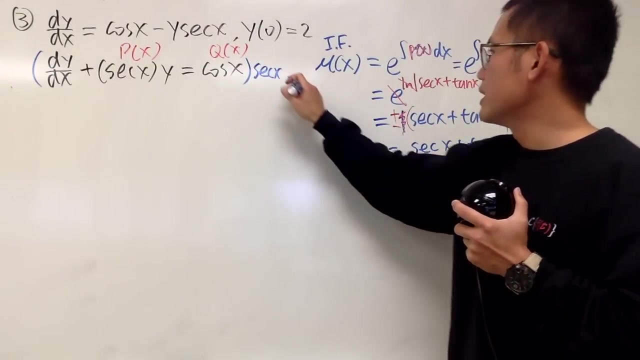 I'll just say: use the positive version, which is secant x plus tangent x. That's all Alright. So what we do is, of course, we multiply everybody here by what we are going to use, which is secant x plus tangent x. 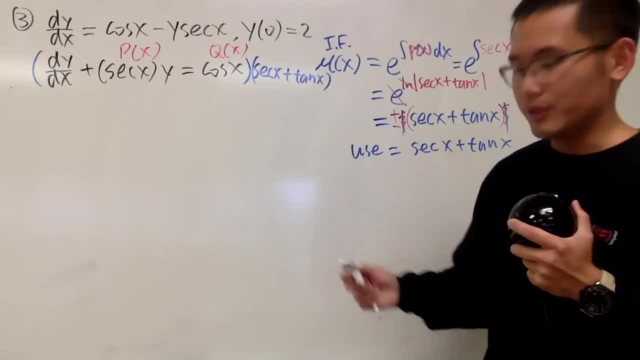 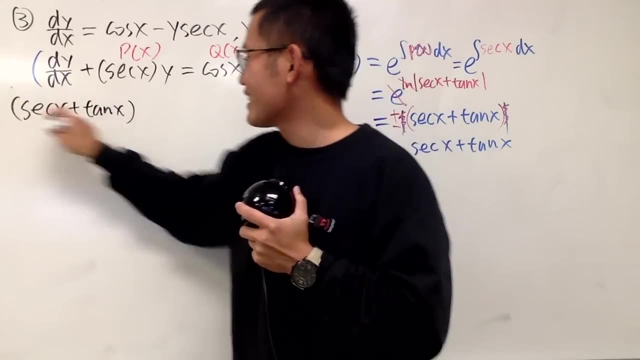 Right, So that's going to work out very nicely. you'll see, This times that we get secant x plus tangent x and then divide the x at and then plus secant x, times that just, of course, work that out. 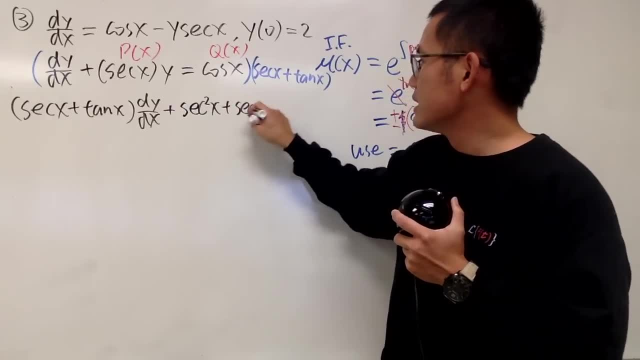 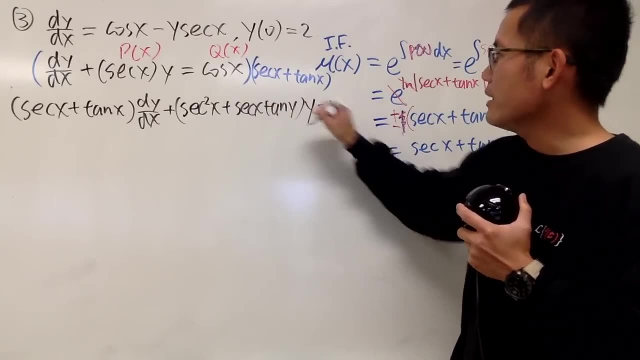 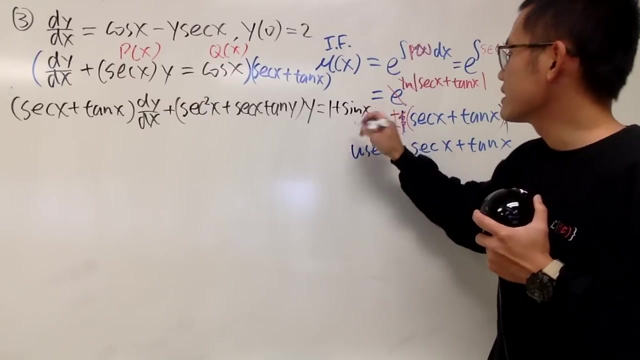 we have secant squared x, plus secant x, tangent x, y, and then this times, this is one right, Because this is one over cosine and this is sine over cosine- times that we just get plus sine x. 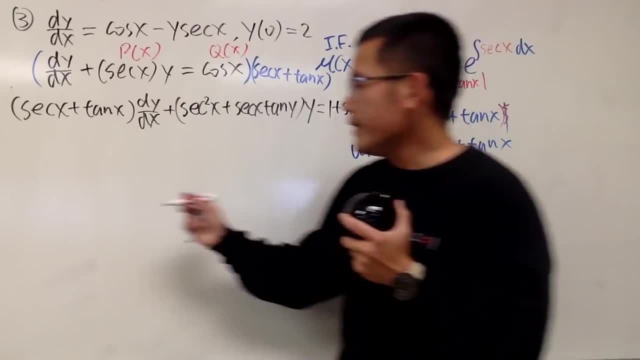 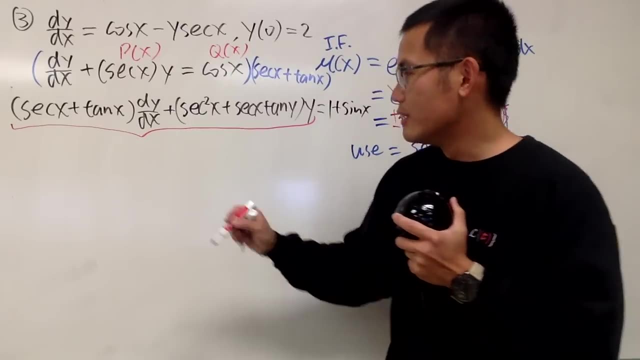 Very nice, Right. So now have a look here. This is so wonderful because the left hand side, in fact, is the derivative of a product of two functions. So I'll tell you this right here is actually the derivative of two functions. 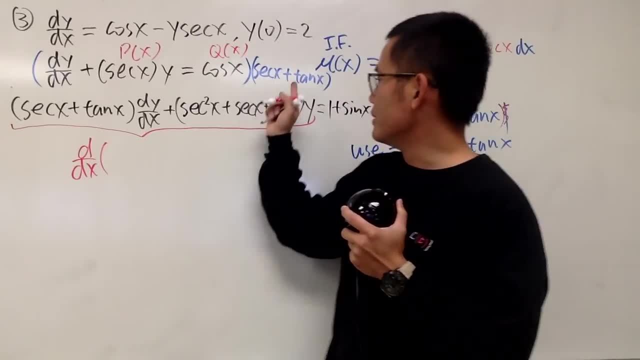 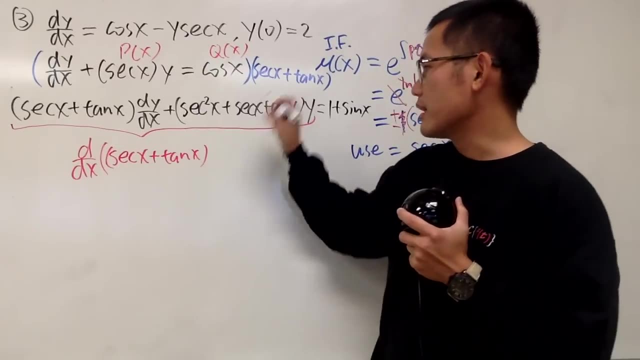 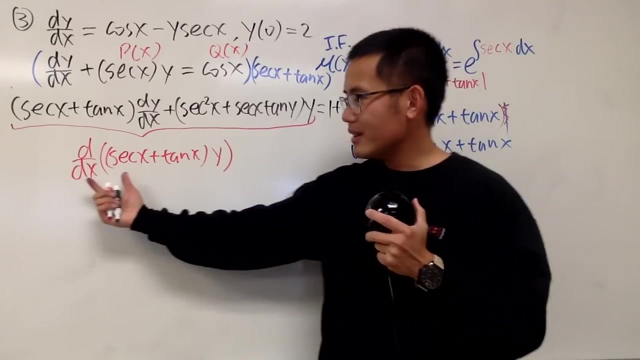 and these two functions are precisely your integrating factor, which is secant x plus tangent x, And the second function is precisely our y, like this Every single time. You can go ahead and check that out When you differentiate this product. rule in action. 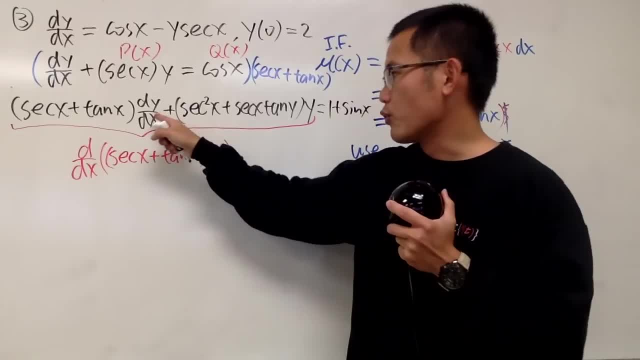 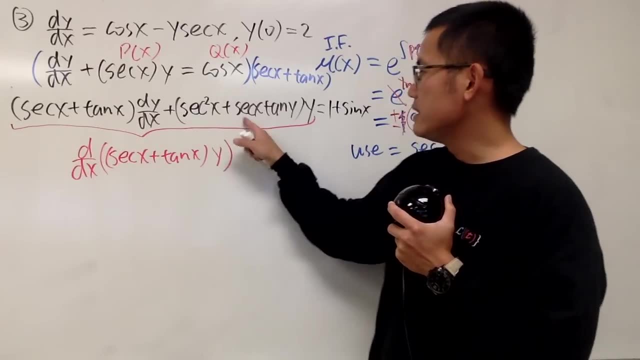 Keep the first function, which is that, and differentiate the second derivative of y is of course dy, dx. and then you keep the second function, which is y, and you differentiate the first. The derivative of secant is secant tangent. 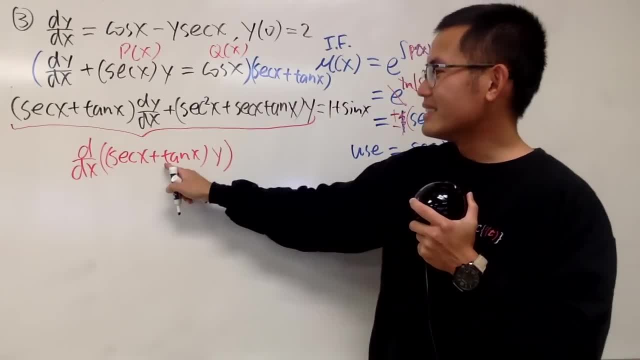 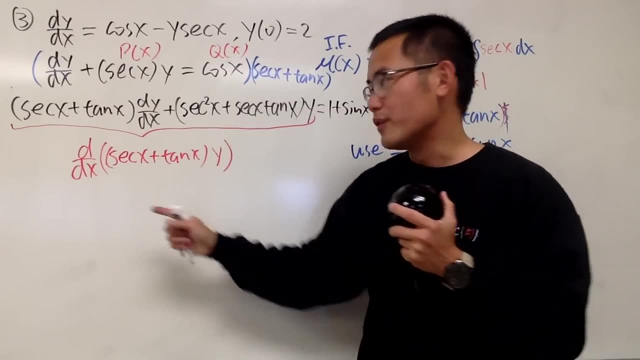 oops, tangent x, sorry, tangent x. And then derivative of tangent x is secant, squared x. So we're good. So the left hand side does represent the derivative of a product of two functions, So we can just combine that. 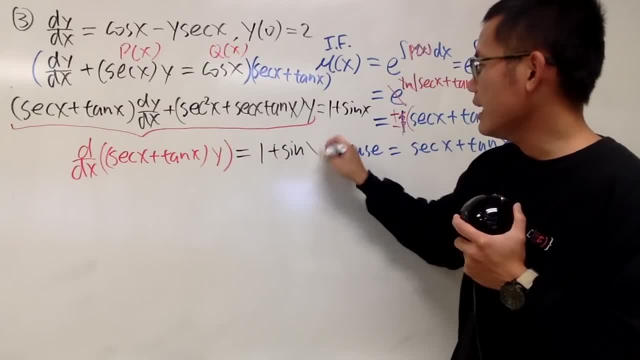 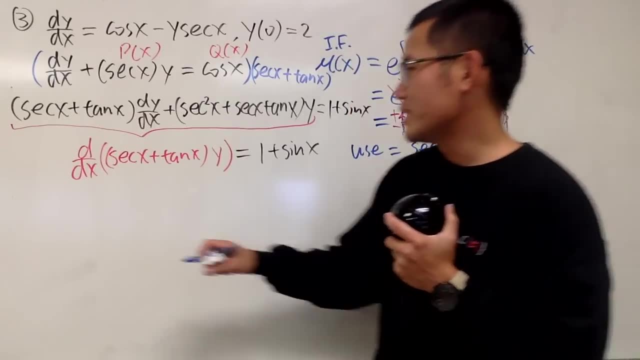 and then this is equal to that which is one plus sine x. Now I want to get the y by itself. Well, we have a derivative. to get rid of the derivative, of course, we integrate. integrate both sides in the x-world. 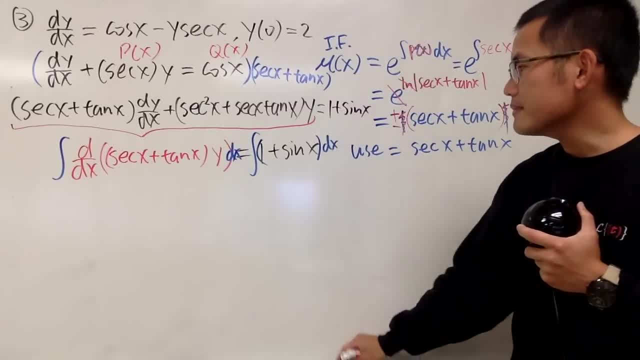 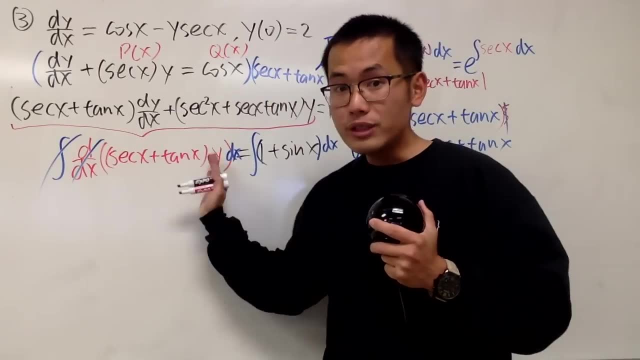 So let's go ahead and do that. Yep, So the nice part about all this is that derivative and integral cancel and you just have the inside. Don't forget to write that down again, So I'll put this down. 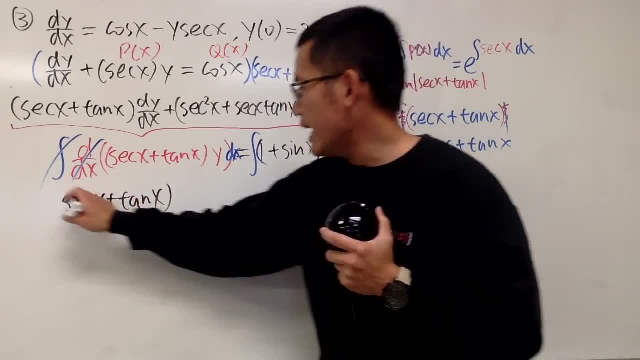 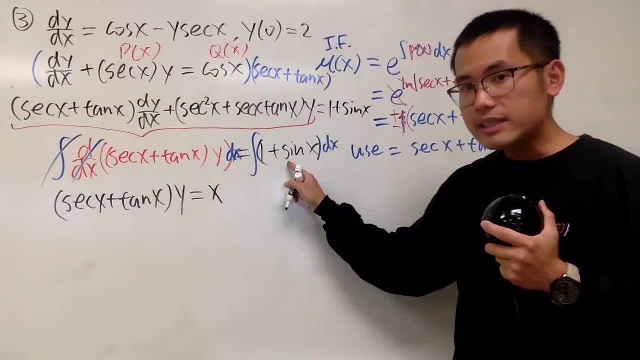 Secant x plus tangent x, and then times y, and that's equal to integrating y in the x-world. we get x. and integrating sine x, we get negative cosine x. And don't forget the plus c. So 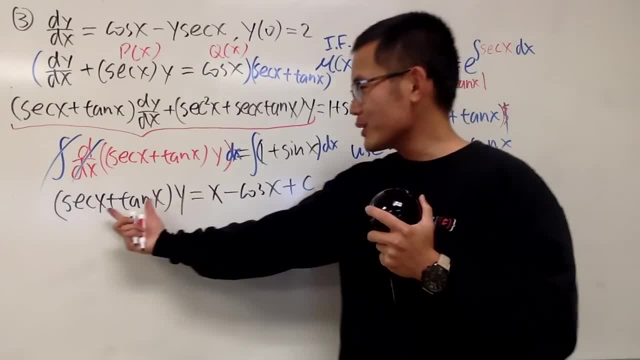 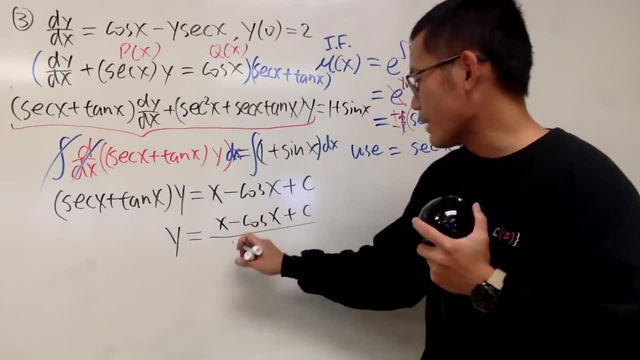 here you put on the plus c. Now of course we can just divide this on both sides. So finally we can see that y is equal to x minus cosine, x plus c, all over that which is secant, x plus tangent x. 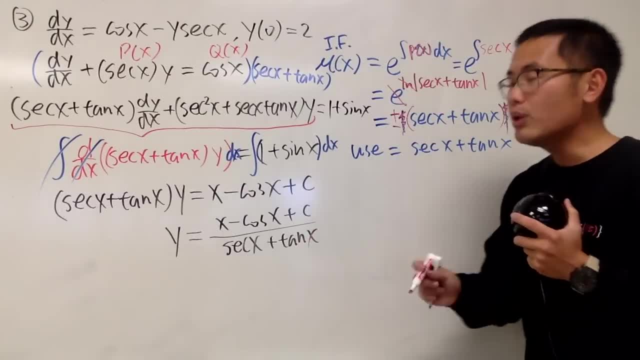 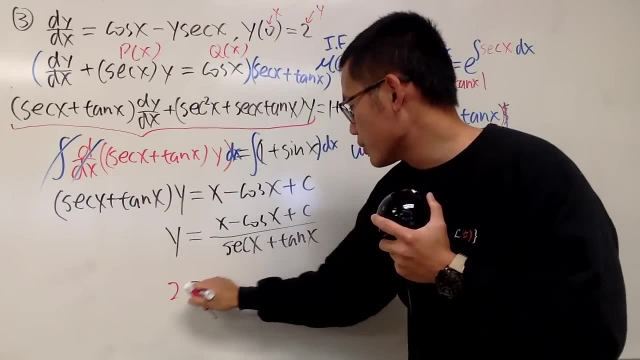 like that And we do have an initial condition. So this right here is x and this right here is y. Go ahead and put that in. So we have two is equal to zero minus cosine of zero plus c. 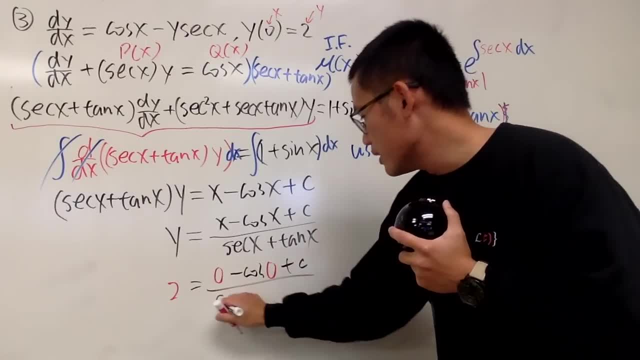 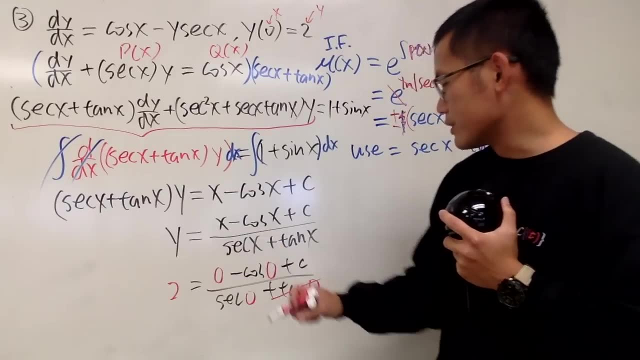 all over that. So plus c over secant zero, plus tangent zero, Well, this is zero and that's of course zero And this is one. So we have two is equal to negative one on the top. 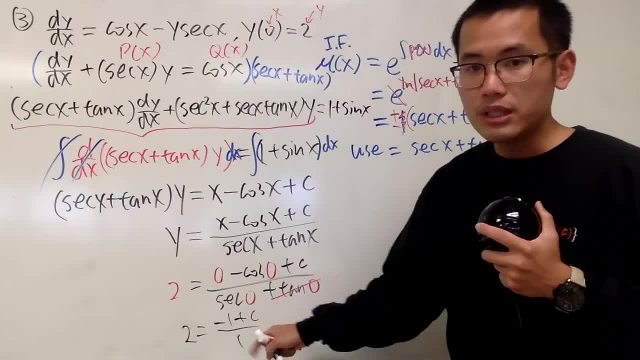 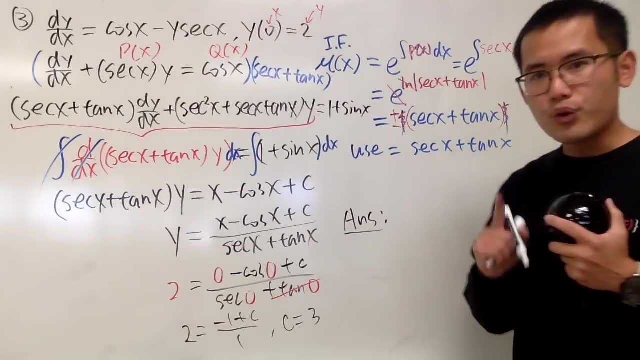 plus c on the top over, this is one. So we have all this. So that means just add one on both sides. So we have c is equal to three. So final answer. I'll just write it down right here: 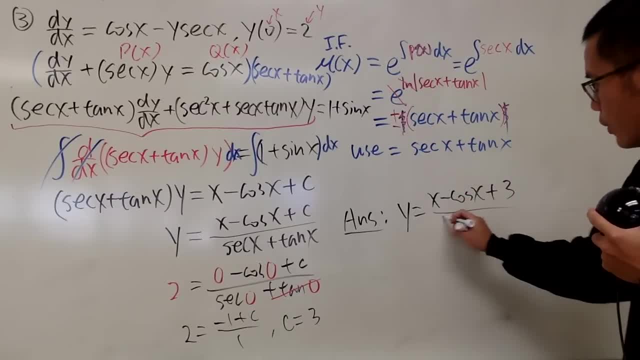 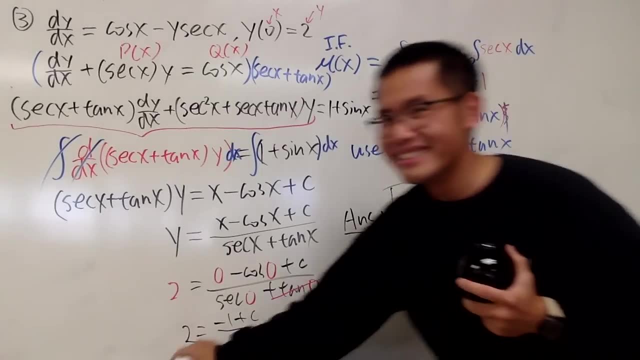 for you guys. So we have x plus three all over that guy, which is secant x plus tangent x like this, And we are done Just like that. Very cool, huh, One of my favorite ones. 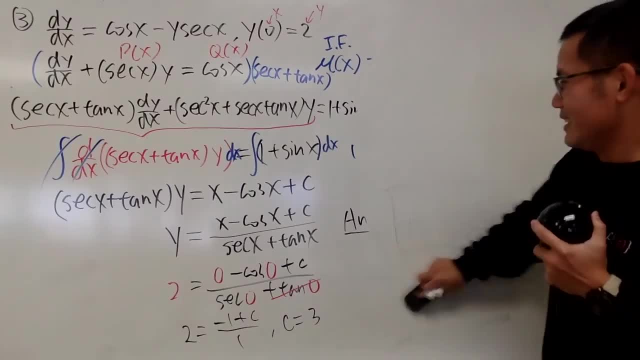 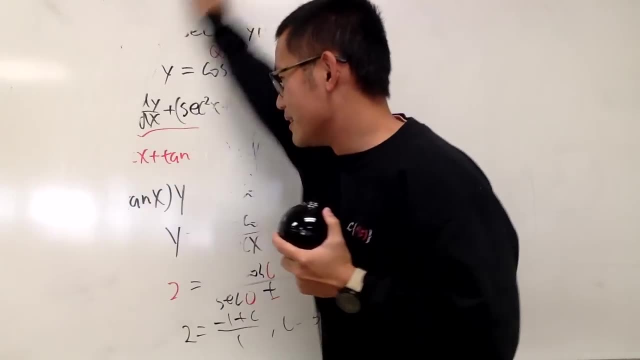 the linear differential equation. Actually, a lot of the differential equations are my favorite, The ones that are solvable, actually, Because sometimes, of course, differential equation will be insolvable, just like integrals, and then differential equations. 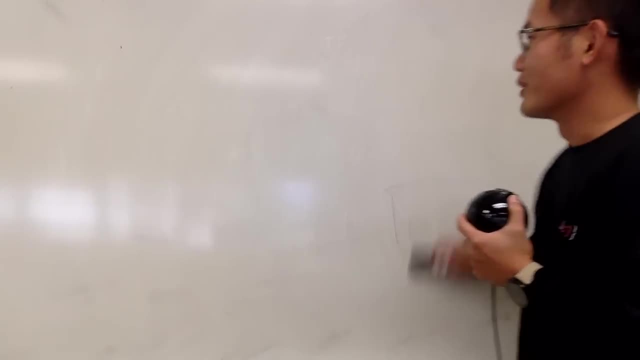 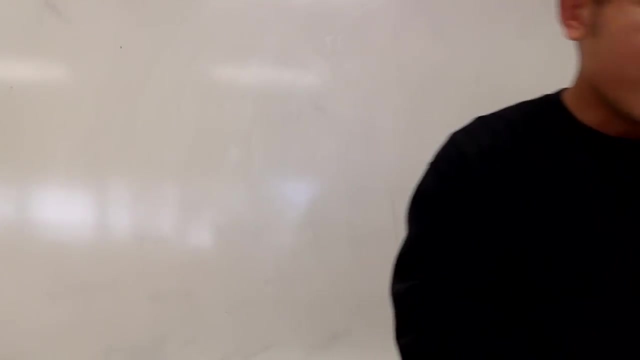 are much harder than integrals, because not only you have to do integral one time, but sometimes you have to do it multiple times in your differential equations. All right Enough talking. Number four, of course. So here we go. 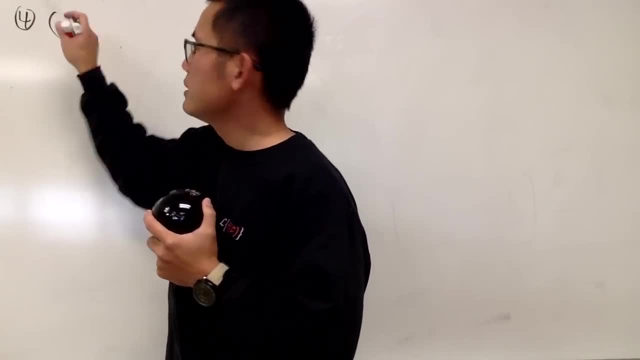 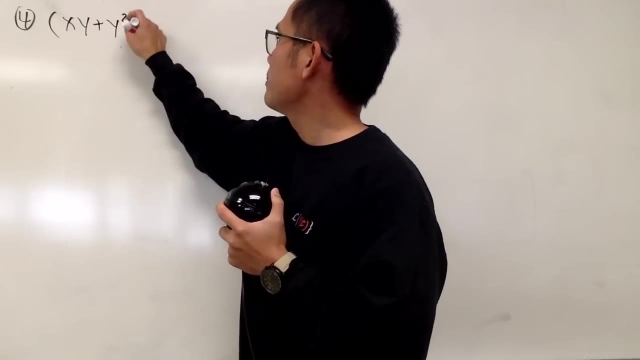 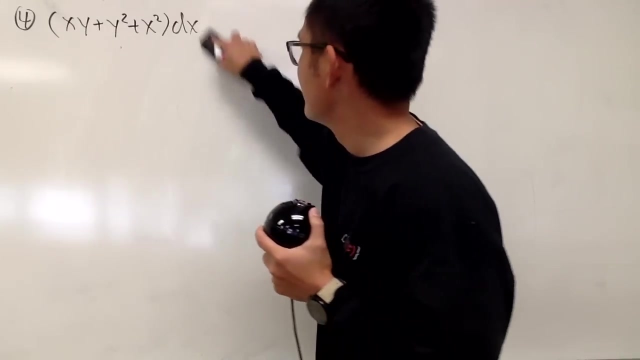 So let me write this down right here for you guys. Number four, parentheses: x, y, x, y plus y square plus x square dx, that x square dy, which is equal to. 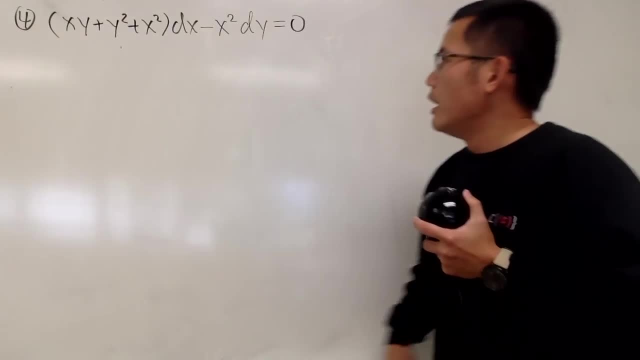 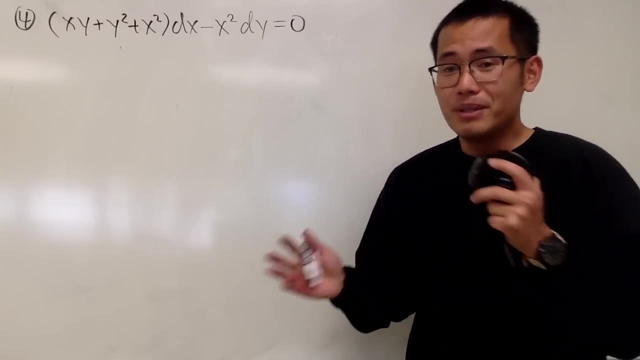 zero, Am I right? Yes, Okay. So, just like what I told you guys earlier, this right here looks like exact because it's in the seems like it's in the total differential form. So 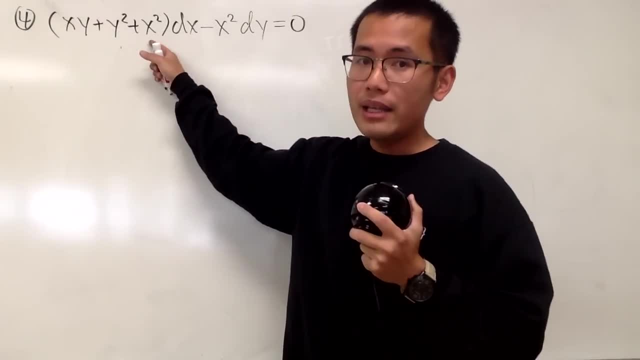 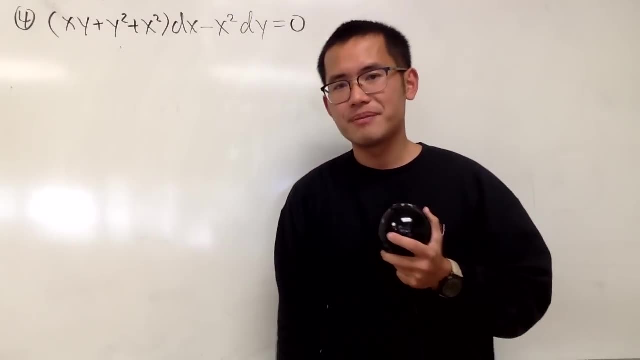 go ahead and check for exactness, But if you differentiate this with respect to y, you get x plus two y, And if you differentiate this with respect to x- not exact, Do we have a special integrating factor? 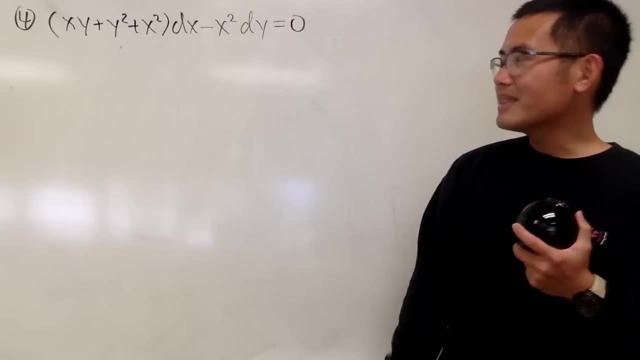 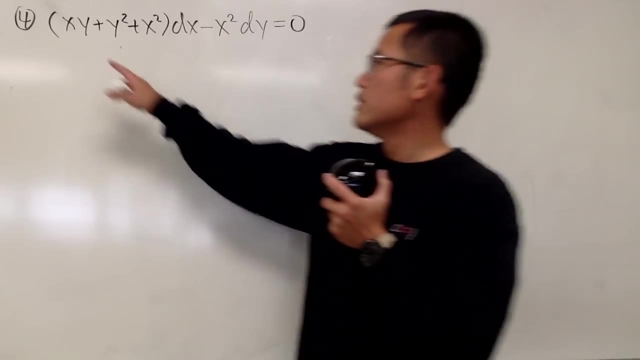 Maybe I don't know, And let's not go there because that's sometimes it's going to be pretty hard. right Here. it's actually a very good situation because you look x to the first, y to the first. 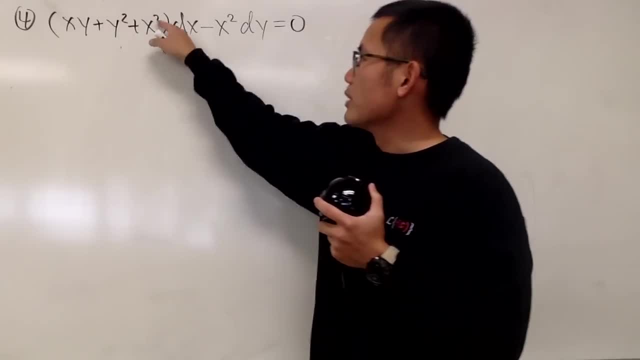 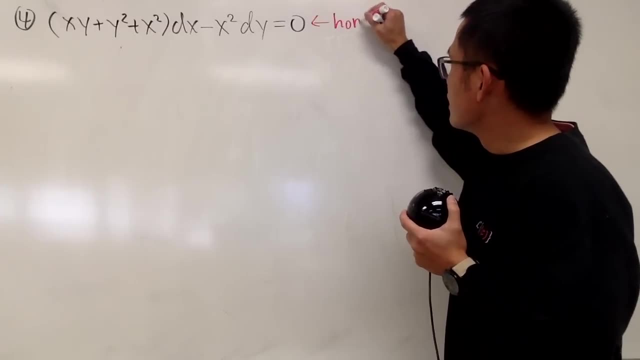 so the total degree here is two: y to the second, x to the second, and this is x to the second. This right here is a special case. this is called a homogeneous situation. Homo- genious differential equation. 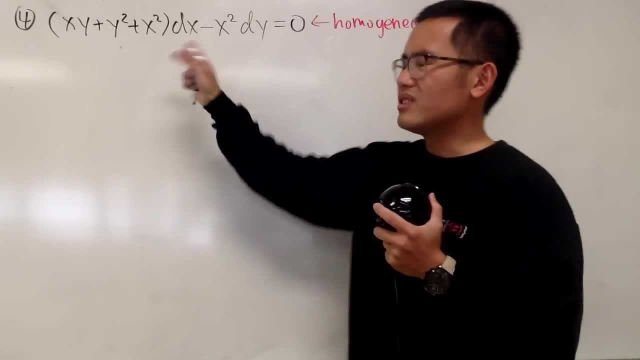 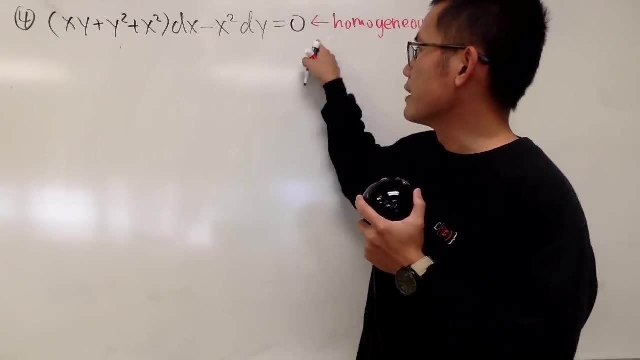 So this is how we can make this work. If you see, the degrees are equal, like this for all the terms, go ahead and do the following: I'm going to isolate the dy dx, so let me put this to the other side. 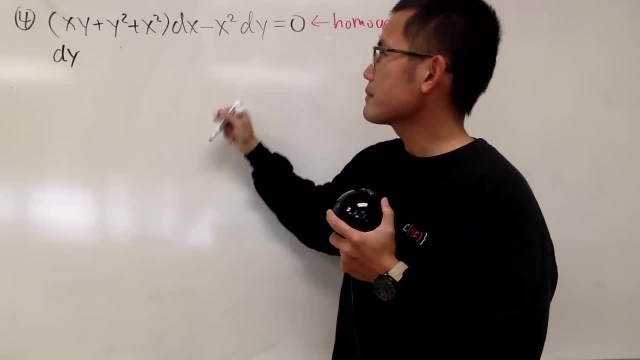 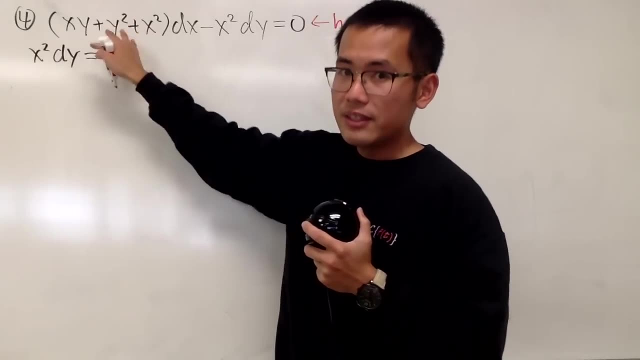 so I get- let me just write down the dy first. yeah, So I put this to the other side and I have the dy power, which is x squared dy, and that's equal to this, which will stay on the left hand side. 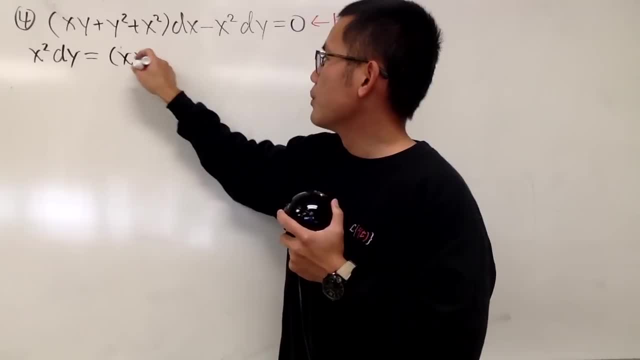 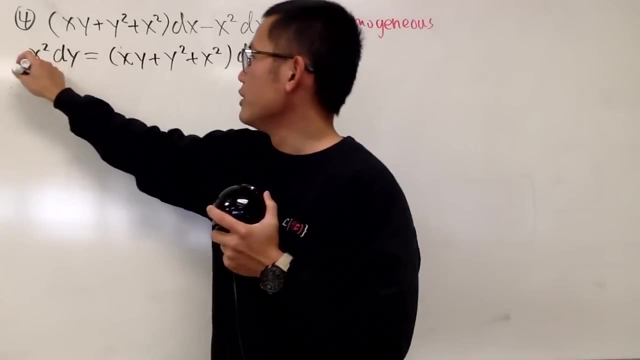 but it's positive. alright, Just go ahead and do the algebra and all that stuff: x, y plus y squared dx, that, just like this. Now I want to divide both sides by x squared. So divide this part by x squared. 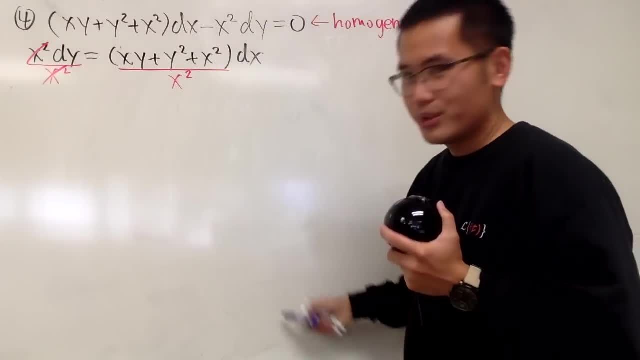 so that of course they can. so let's cross that out, because it's you know, it's pretty satisfying when you do that. And of course, let's divide the dx on both sides so they can. so let's move this here. 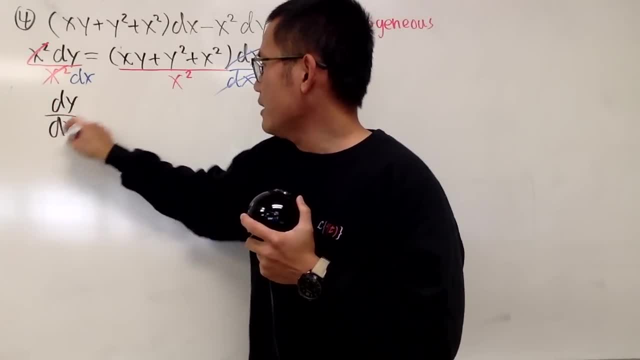 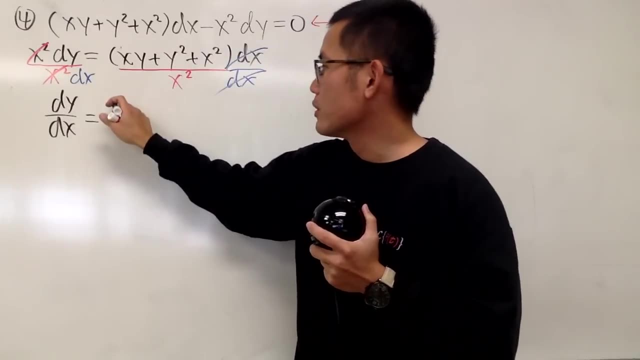 of course that's very nice. Anyway, dy dx, here is the deal. I'm going to split the fraction and you'll see this. over that, we get y over x to the first power, So it's y over x. 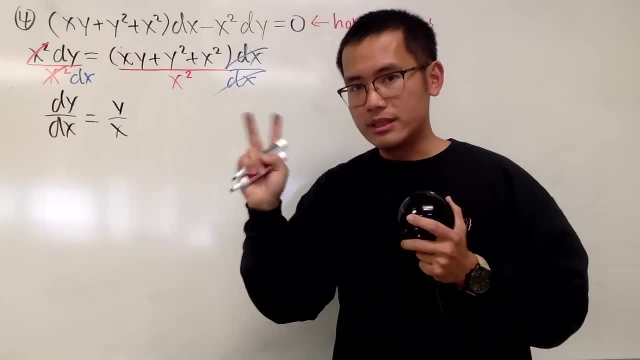 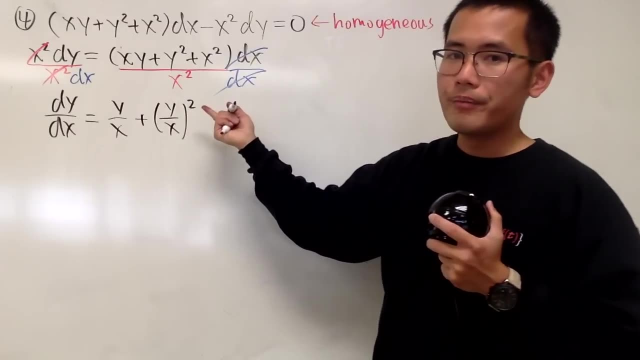 So next this, and that both of them with degree two. So I will actually write this as plus y over x, degree two, right to a second power. Lastly, this, over that we have plus one, just like this: 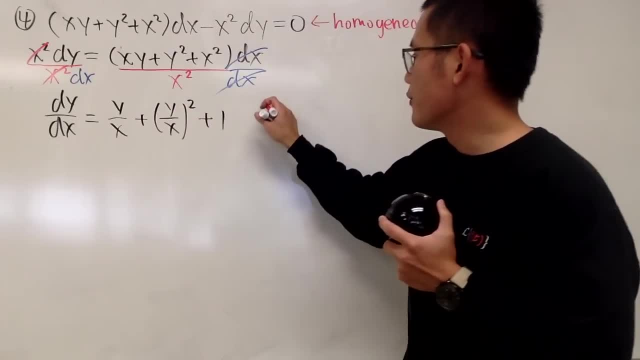 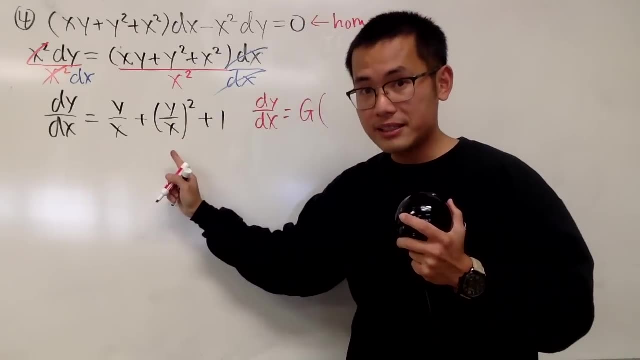 Now this right here. right, this right here is in the form of dy, dx equal to the right hand side, as g as a function of y over x, The right hand side, you can see. the input is this: 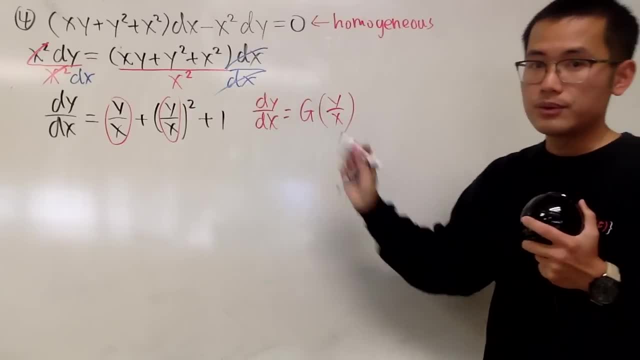 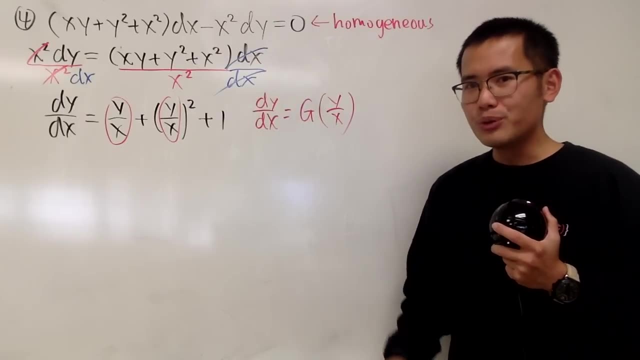 just that, right, So homogeneous differential equation. And the strategy to do this is that we will just do some substitution, just like how you do the? u substitution back in the days for integrations, right, And I will go ahead and use v? 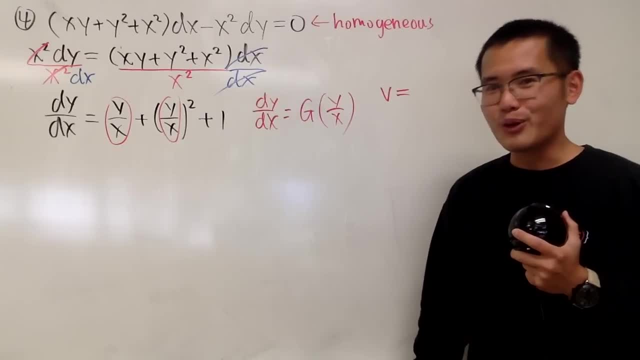 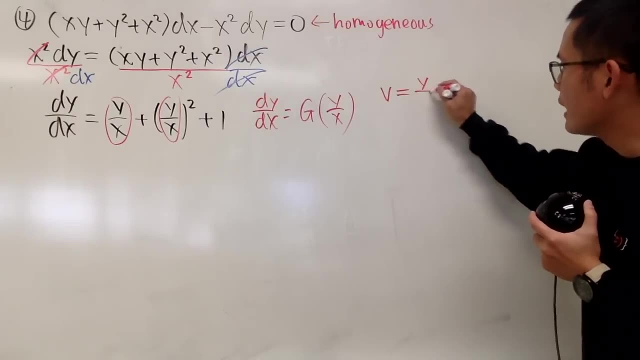 this is the standard notation in the differential equation textbooks. You can use u, of course, Use v and let v be the input which is y over x. like this, We'll be doing a lot of substitution sometimes, yeah. 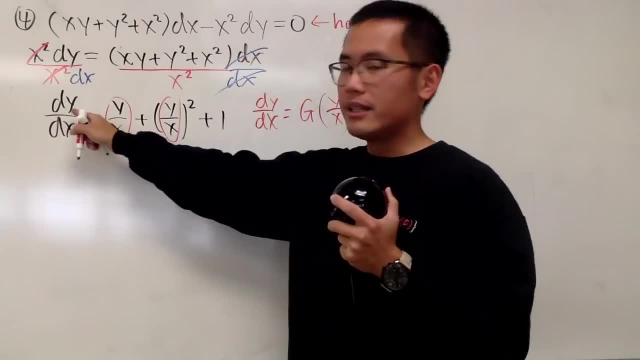 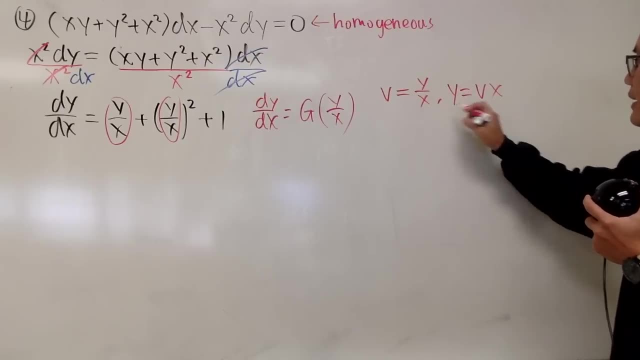 So this is the first part and of course do the usual thing. I need to get the dy dx, so perhaps let me just multiply the x on both sides. that means y is equal to v times x. 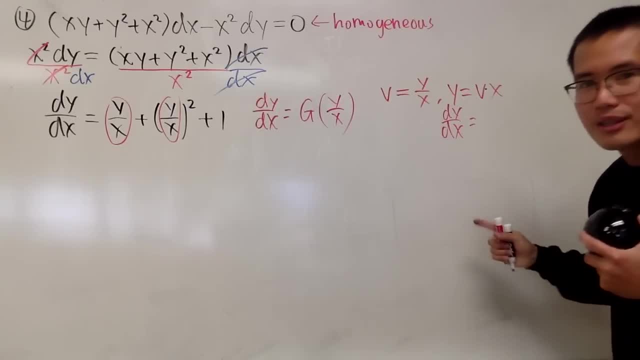 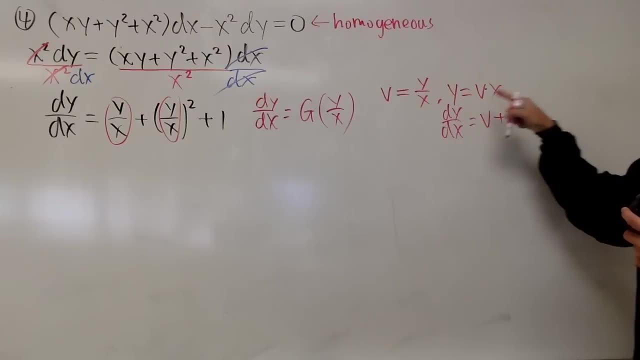 and then differentiate that dy dx. hey, Prada-Lew in action, Go ahead, keep the first function derivative of x is just 1, good, plus the second function, which is x times the derivative of the first. 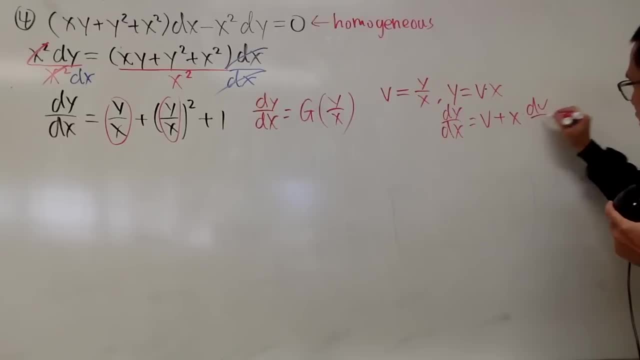 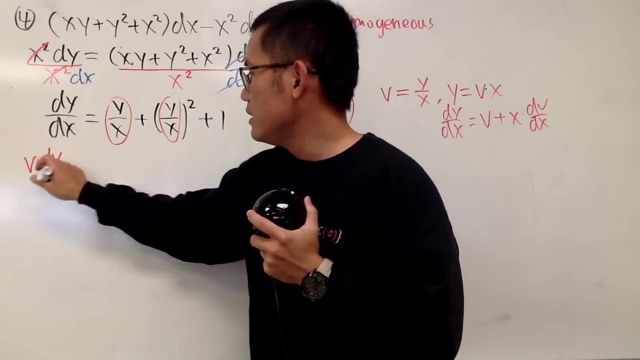 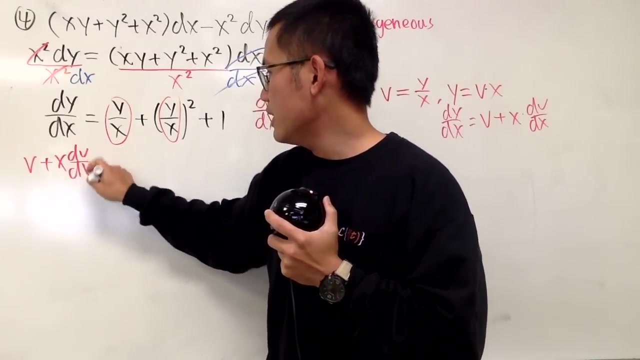 v is a function of x, so derivative of v is dv, dx, like this: Now bring this to here, so we have v, dv, sorry, v, plus x, dv, dx, dv, dx. 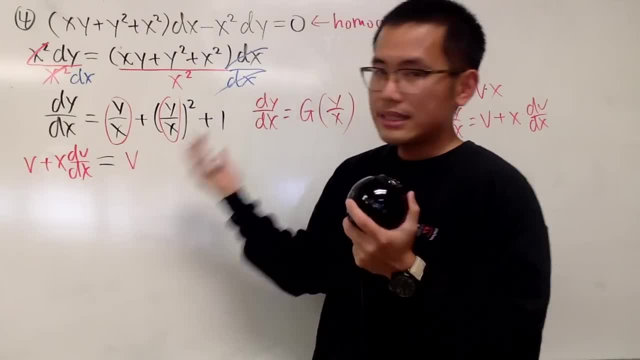 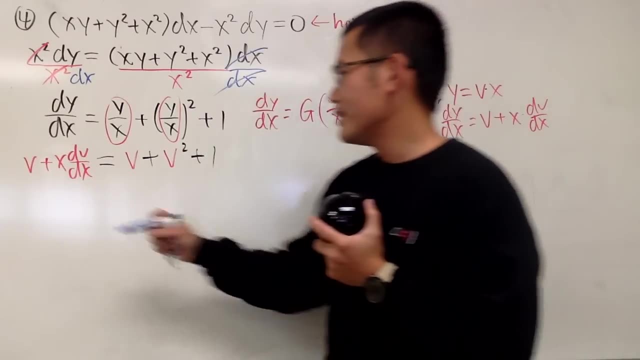 this is equal to this part. you see is v, So that's the input. very nice, Plus this right here, so it's v squared and then plus 1. Very nice, You know what's nicer? 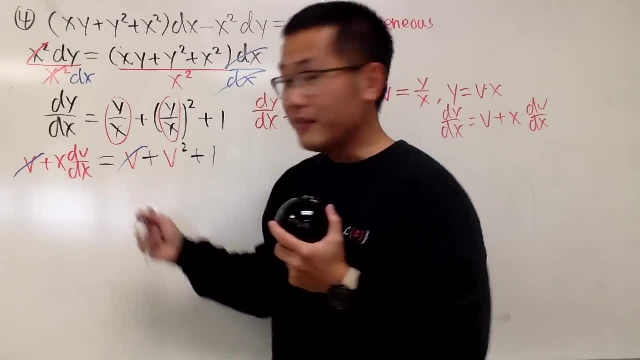 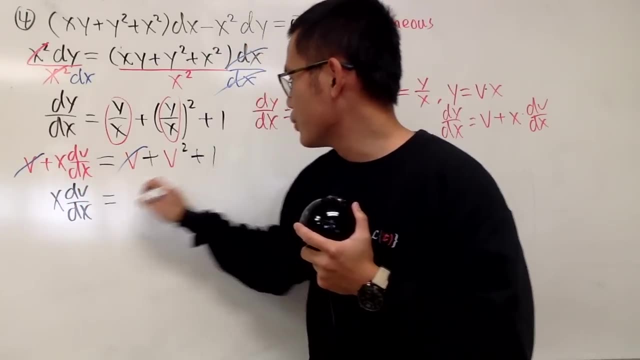 This and that comes out Very good, huh. So it becomes separable, Because you can see we have x, dv, dx, and that's equal to v squared plus 1. And of course, this is the quantity by itself. 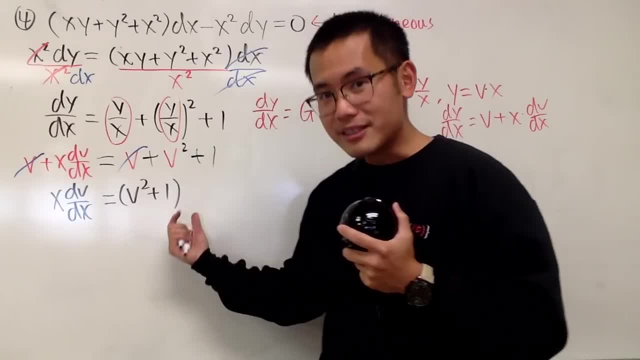 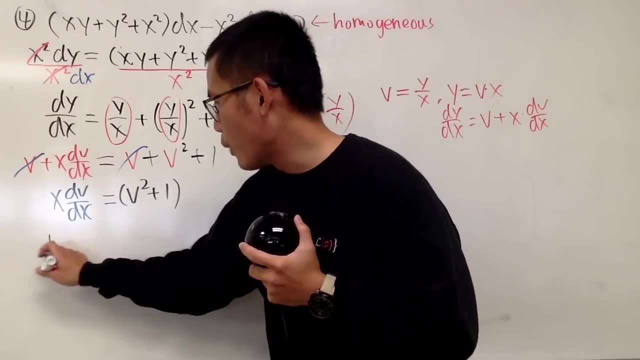 yeah, We can multiply the dx on both sides and also bring the x to the other side and divide that by to the other side. So let's do this part first. Bring this to the other side, I get 1 over. 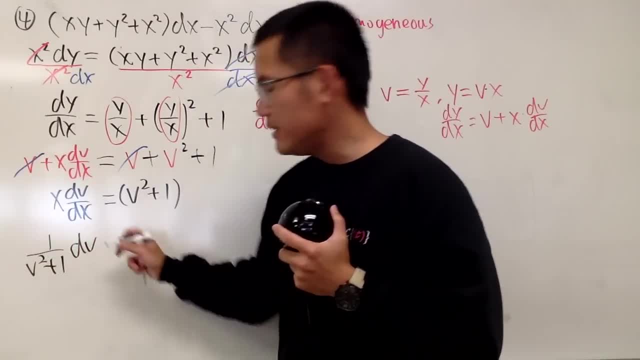 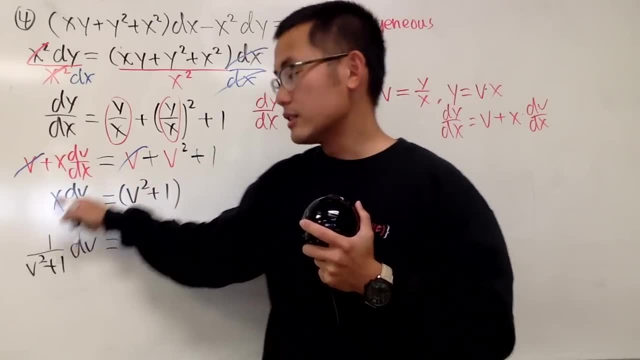 v squared plus 1, and that's in the v world. Here it's going to be equal to dx. on the other side it was x. so the other side. you have to divide the x on both sides. 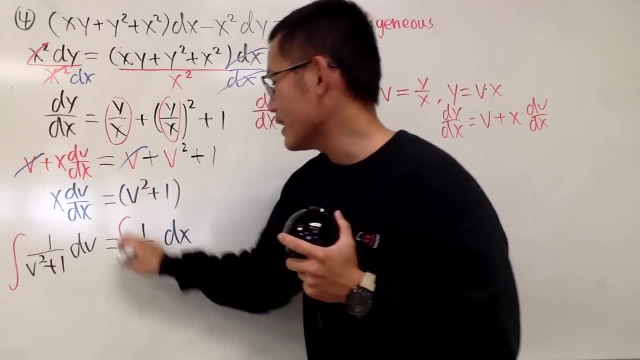 so it becomes 1 over x. like that It's separable. Very nice, Integrate both sides now and you see we have the differential already: dv and dx. What's the integral of this? Know your derivative really well. 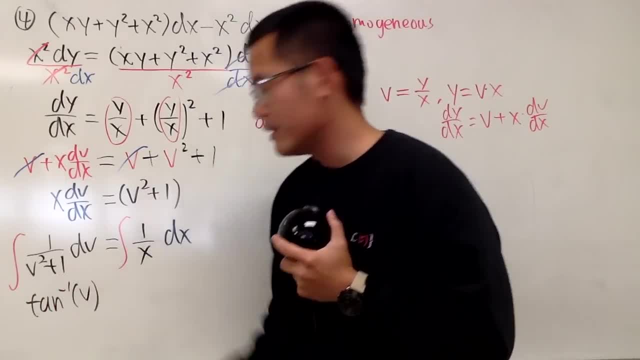 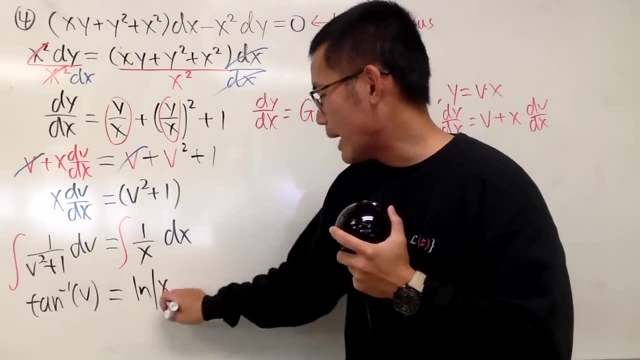 This right here gives us inverse tangent of the input, which is v. Don't worry about the plus c, just worry about the plus c on the right hand side, Integrating this. well, it's classic ln of absolute value of x. 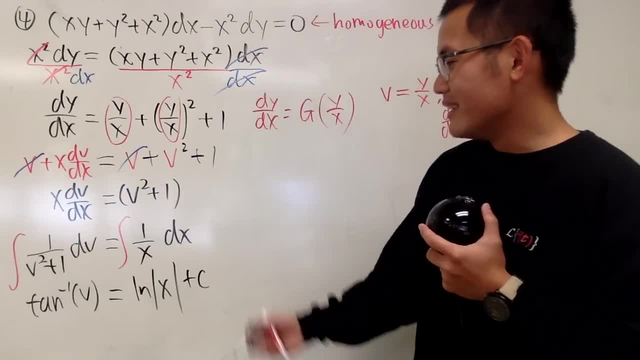 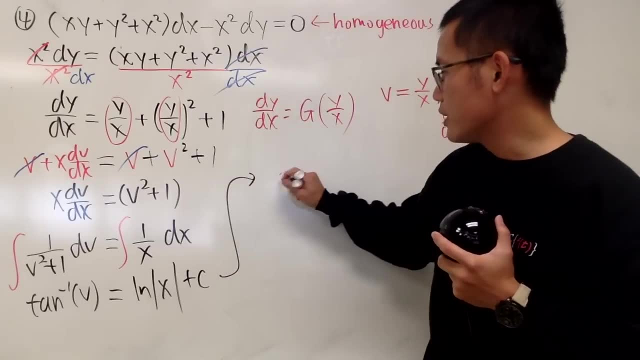 And then don't forget the plus c right here. Okay, so let's take the original tangent on both sides, because this will tell us v the original tangent right. v will be the original tangent of the right hand side. 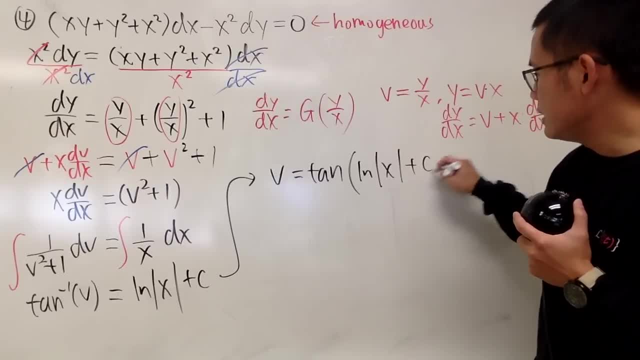 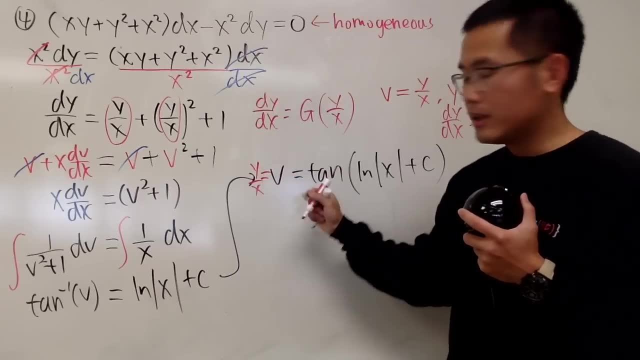 which is ln of absolute value of x, and then plus c, like this: But what's v? v is y of x. so don't forget, you care about v, but more importantly, you care about y. y over x is equal to that. 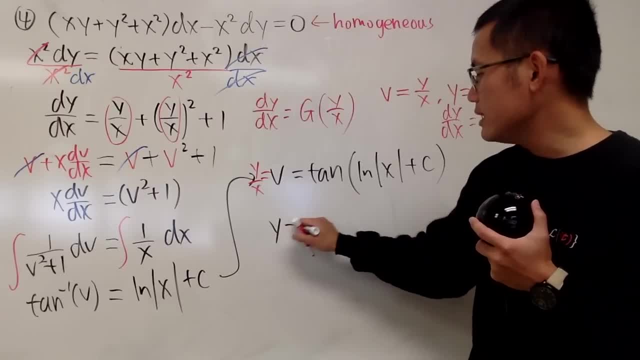 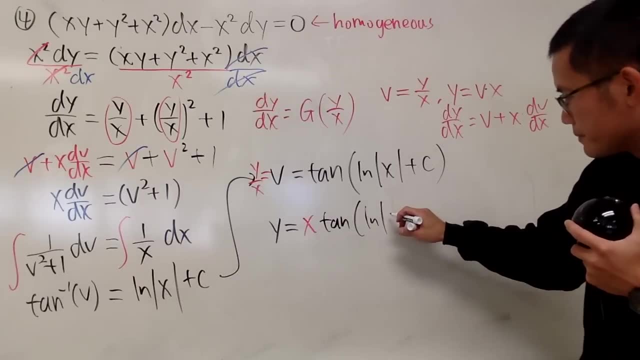 so of course you can multiply the x on both sides, so y is equal to x, right here. and then tangent of inverse, so tangent of ln, of absolute value of x plus c, like this: 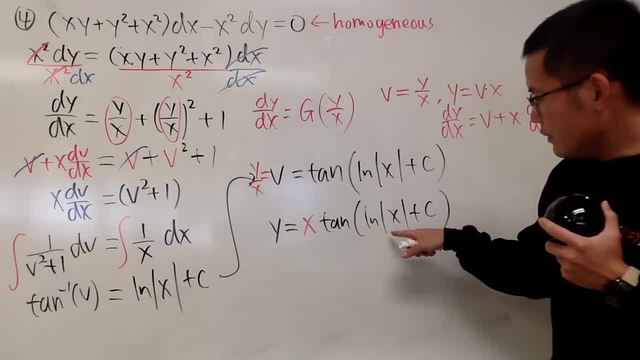 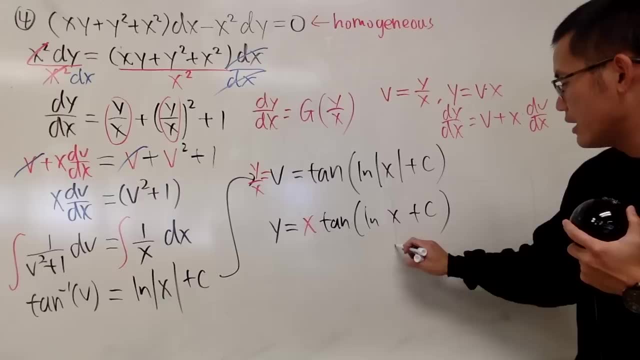 Okay, And here's the little thing: sometimes if you specify an interval, the domain for the solution, you might not need the absolute value. so if you would like, you can get rid of this and then just say x is greater than zero. 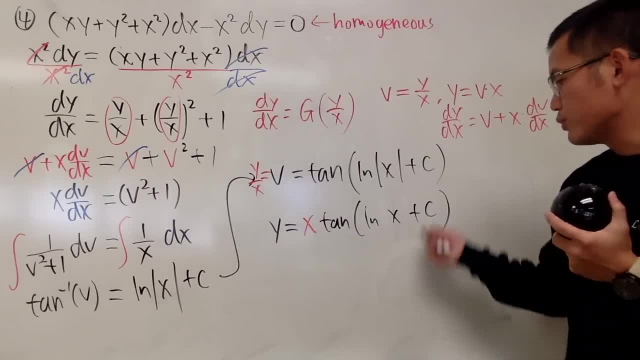 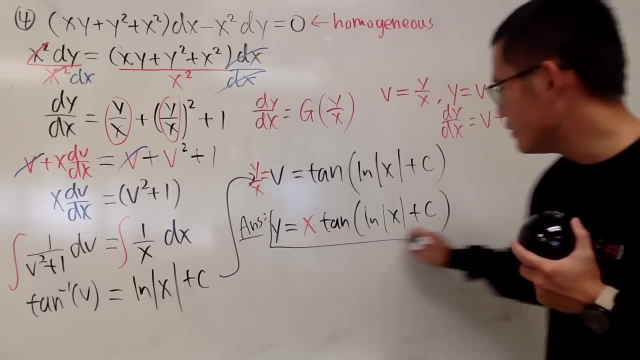 That it's okay. it depends on the situation, that how you want to solve the differential equation, But I'll keep the absolute value right here. This, right here, is the answer. Very, very nice, huh, So just like that. 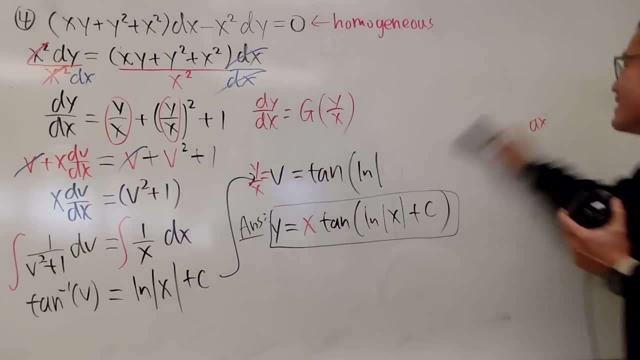 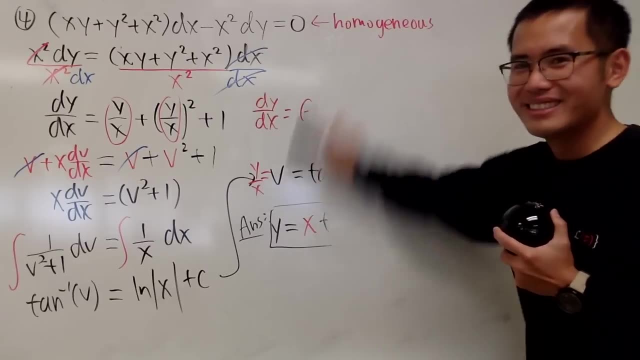 Okay, cool. Number four: homogeneous differential equation. In another word, it's actually just substitution. There are a lot of things just substitution, just like integrals, seriously, But sometimes some of the substitutions, they are not so obvious. 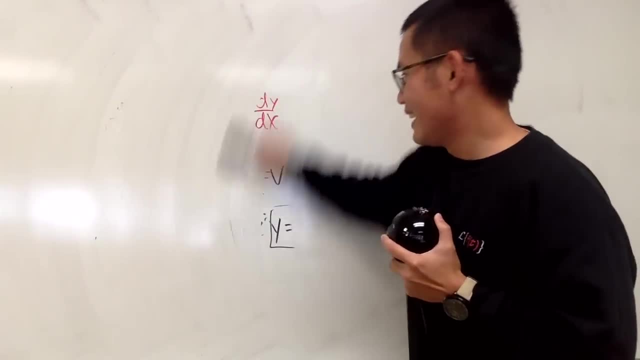 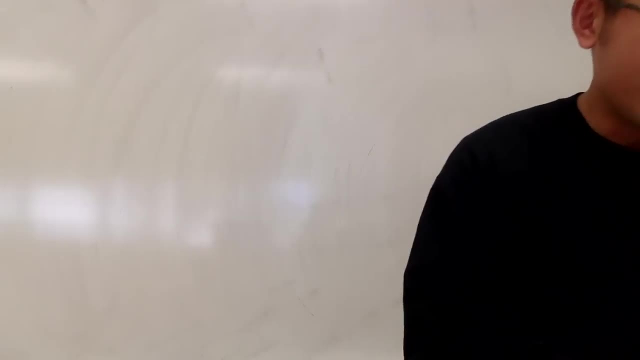 and I'll tell you this, which one that we have, and it's going to be really exciting, right? Okay, number five. What's after four? Of course it's five. Let me just make sure that we have. 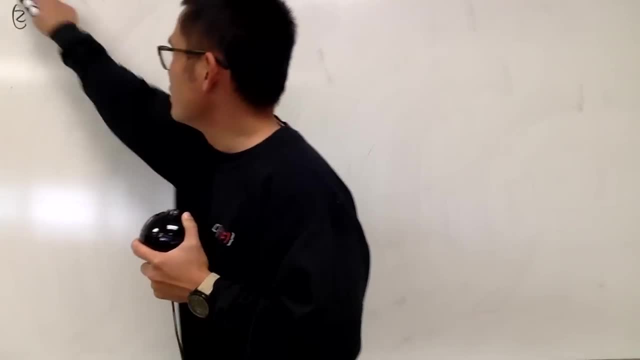 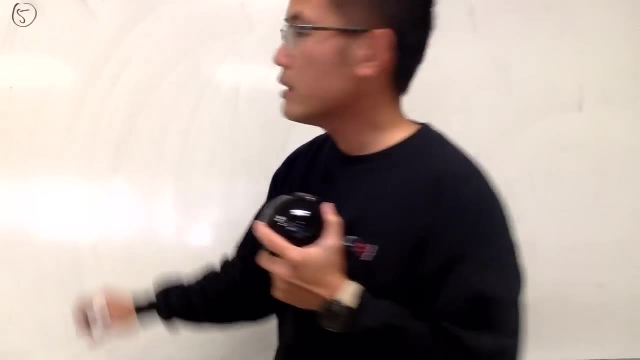 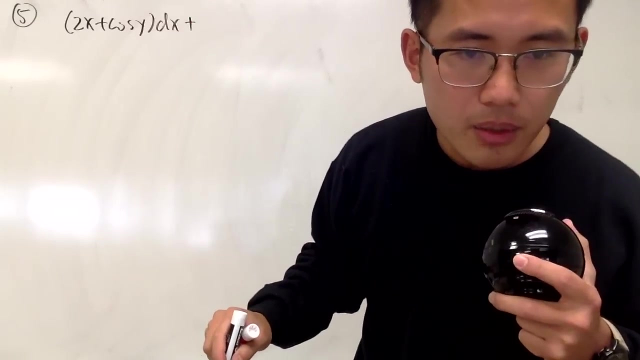 this right here? No, why do you have random two, Five, Two x plus cosine y, Dx plus, and we have x squared, tangent y. Oh my god, Tangent y and cosine squared. 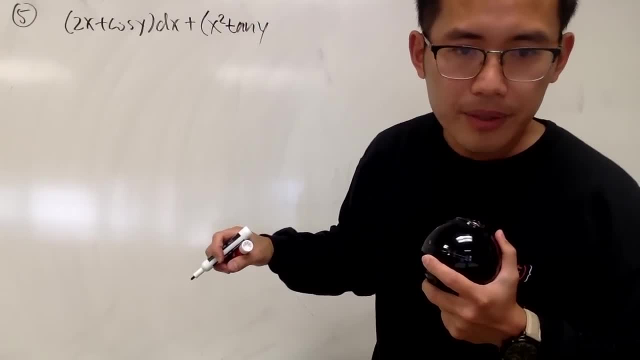 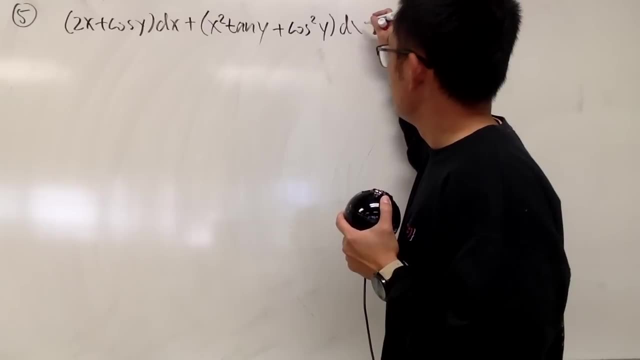 y dy equals zero. Now looking at the equations, and then again I don't want to mess it up. So we have x squared y dx plus, and we have x squared tangent y. 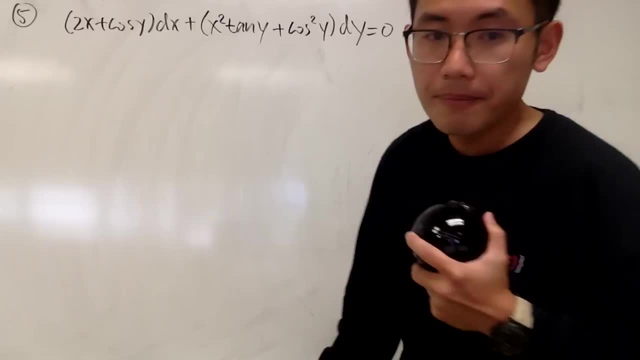 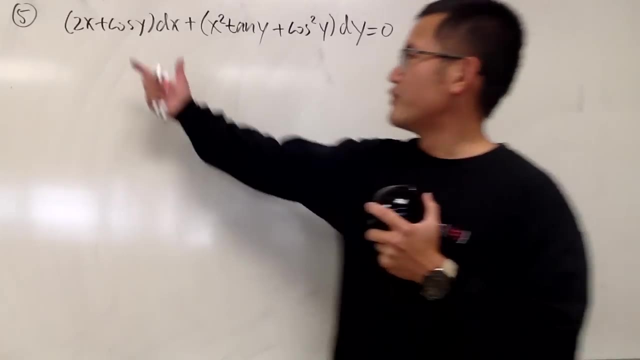 Oh, let me see. Let me see, All right, good. Hmm, What should we do? Check for exactness. Okay, do this in your head. Differentiate this with respect to y. we get negative sine y. 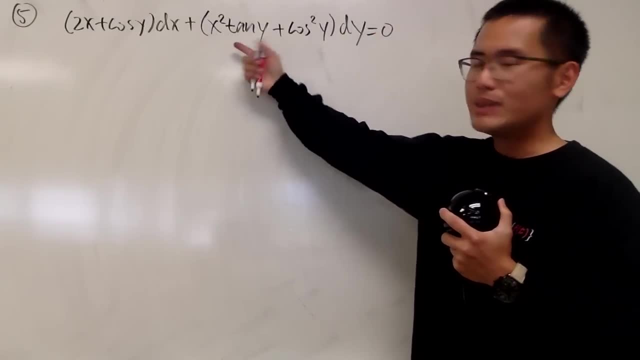 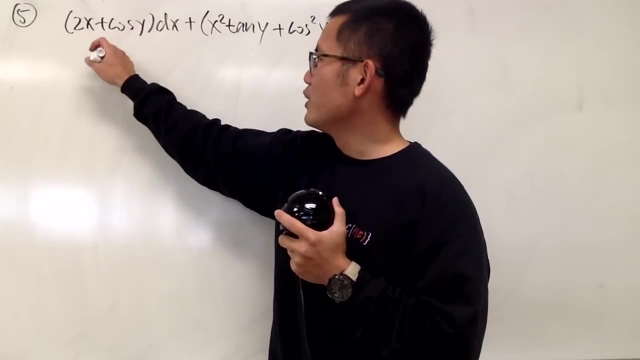 Differentiate this with respect to x. We get two x tangent y. But hold on, hold on one sec, hold on one sec, Right here. this is when we differentiate that we get negative sine y. 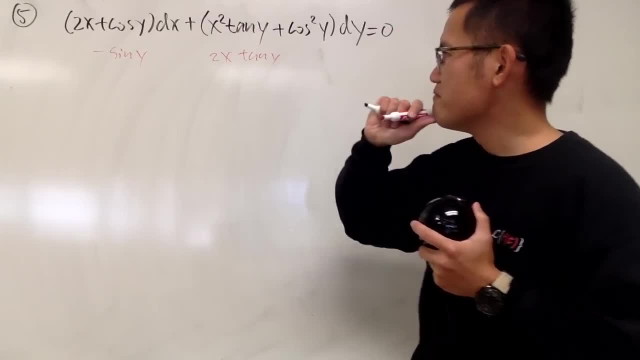 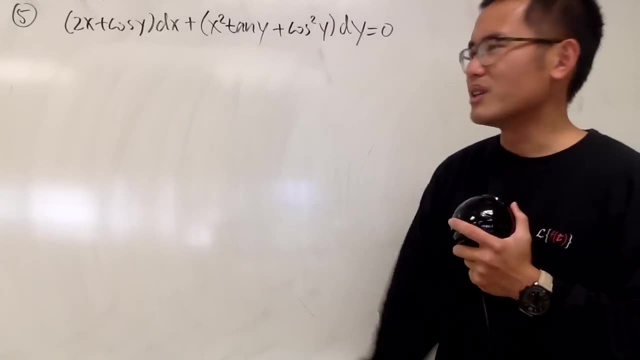 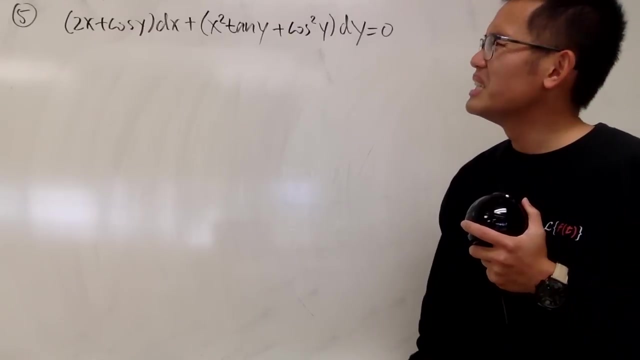 When we differentiate this, we get tangent y. Hmm, Okay, Not, not, not, not, not, not, not too alike. yeah, It's not linear, because cosine y and then tangent y, all that stuff. 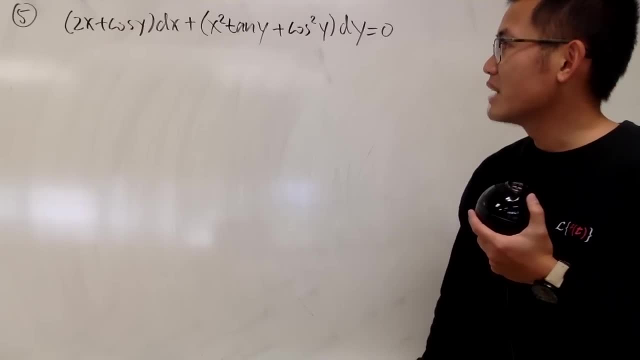 It's not homogeneous. It's not like the situation that we did. It's not separable, because you can try, it's just not. But in this case it's almost exact, Right. How do we know? 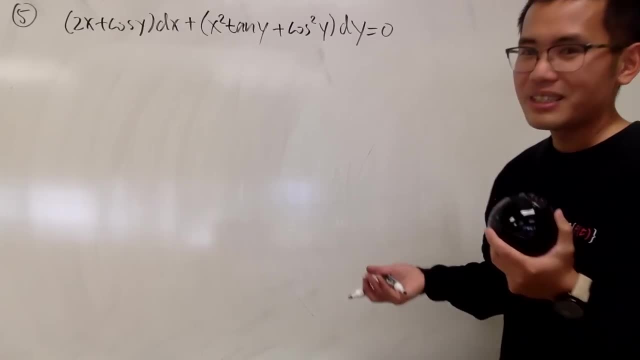 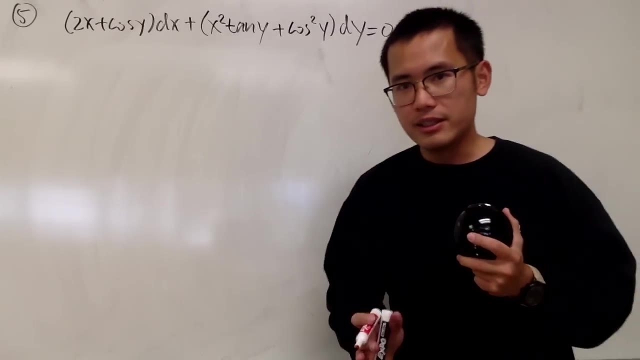 Well, sometimes we don't know, we just have to try it, And um, yeah, And now here is the deal. If I don't give a hint and if this question seems like uh, out of nowhere, 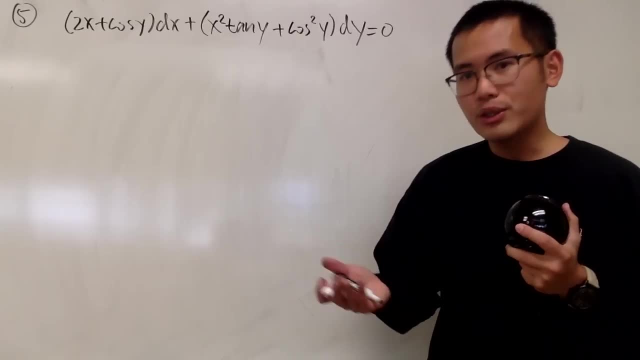 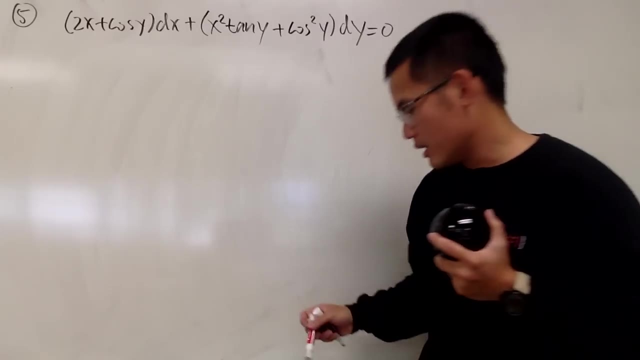 then the special integrating factor. it will just be either in terms of x or in terms of just y, So we'll see which one. the situation is Right, So I will have to write this down. 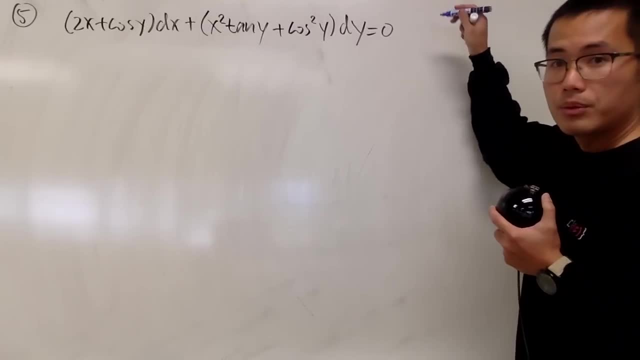 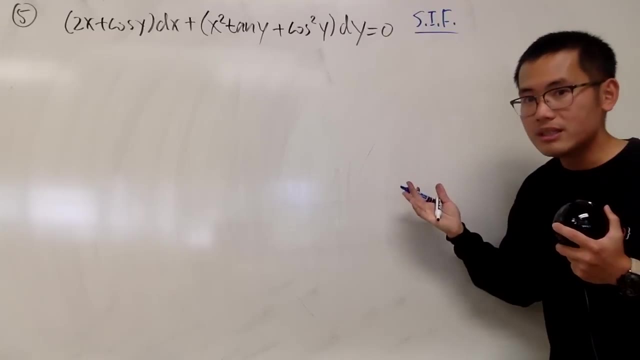 right here for you guys, So I'll put this down. Here is the special integrating factor, And I'm not going to prove all this in my in this video, because I did that three years ago. 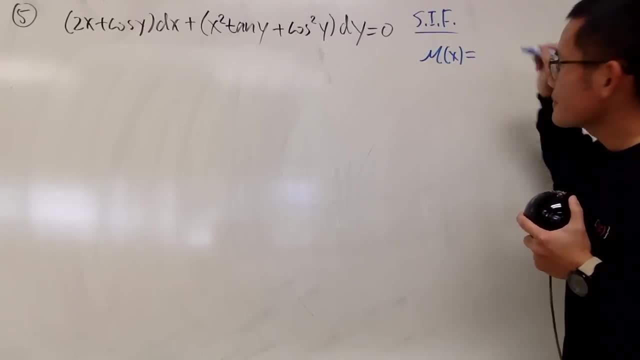 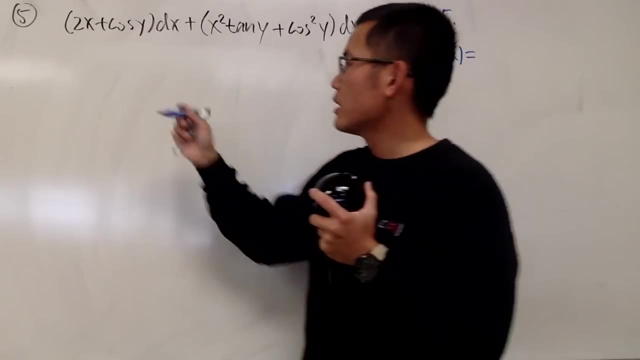 for you guys already. So go ahead and check that out. Mu of x. When you have a total, differential, full situation, this one right here, it's more bizarre. First, this right here. we call that to be m. 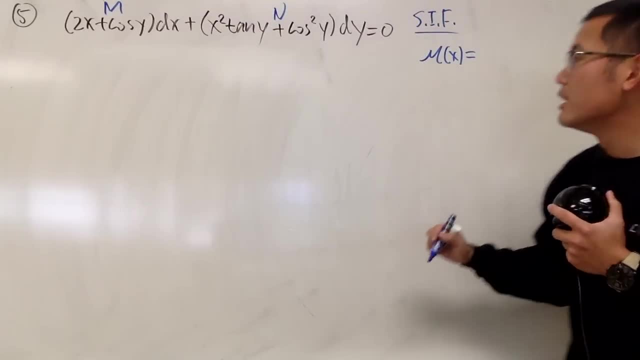 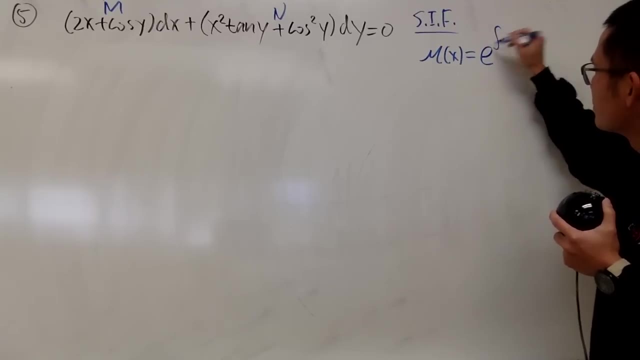 We call this to be n? Yeah, Just notation. purpose: Mu is the special integrating factor in terms of just x. In that case you have e to the integral power. It's not like the one that I showed you guys. 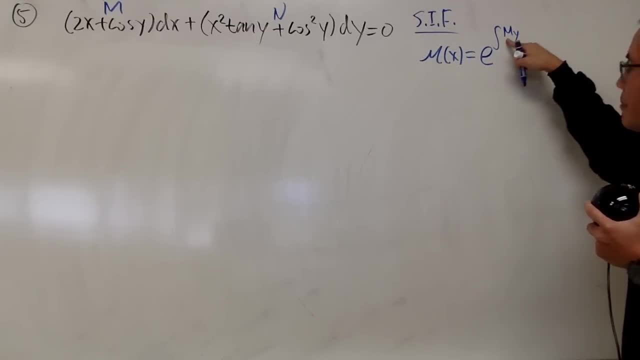 earlier. This right here is m sub y, Meaning the partial derivative of this part with respect to y Minus n sub x, Similar right Divided by original n, And hopefully this expression: 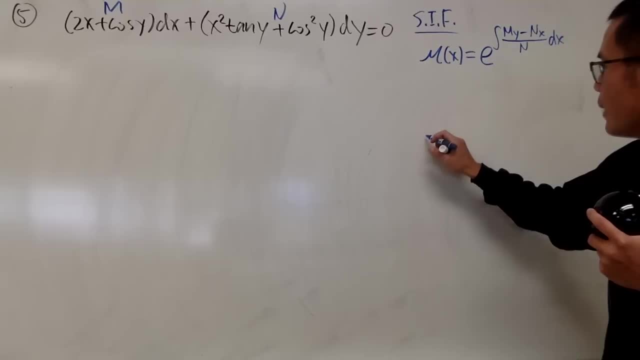 will integrate that part, Alright. And then the other one is. I'll put it down here: Mu of y is similar e to the integral power And you actually have n sub x minus m sub y. 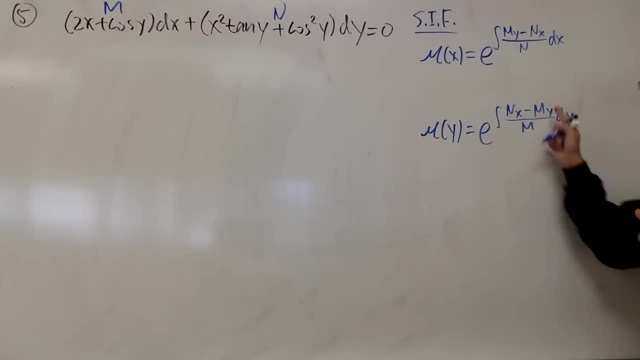 over m, And this right here, hopefully, is in terms of just y, And in that case, then that will be it. Okay, So now let's see: E is e, Integral is integral. m sub y. 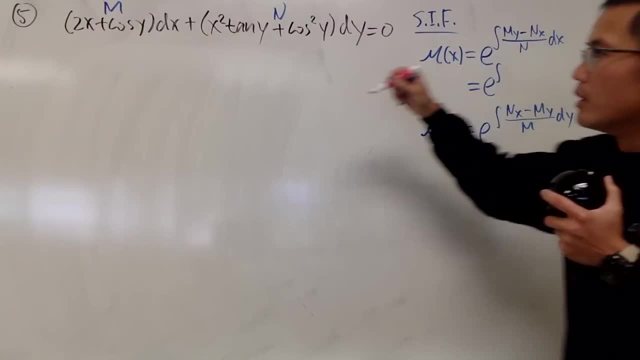 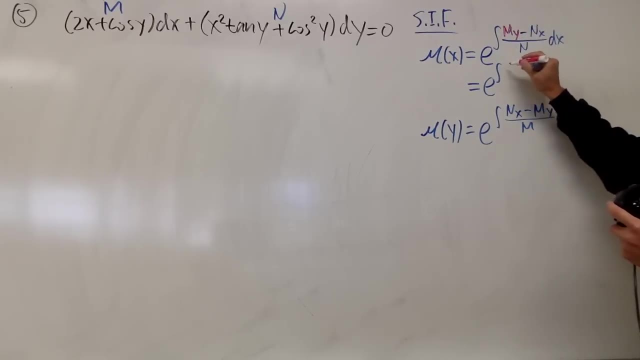 Meaning that, this with respect to y. So let's see m sub y. I will just write it down right here for you guys: m sub y. We get negative sine y, as we mentioned it, And then 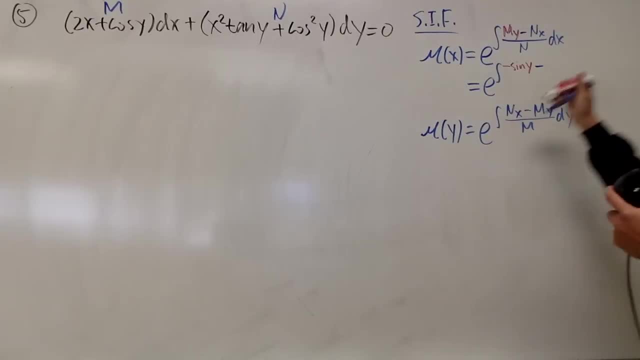 minus n sub x, Which is this part- and we did that earlier- Which is two x tangent y. Okay, And then divided by n, which is that, And we have. let me just write it down right here. 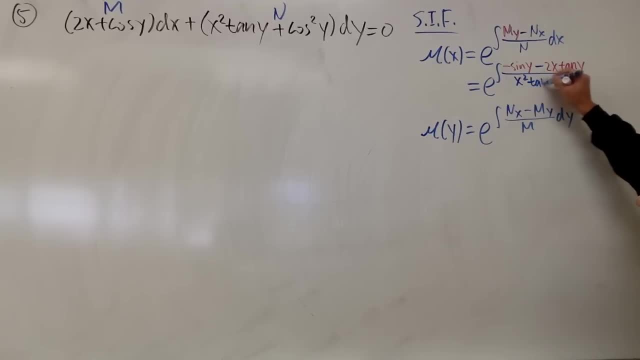 Yeah, x squared tangent y plus cosine squared y dx, like this. Now, by looking at this, can we simplify it? Hmm, Uh, well, let's see. Hmm, Not so much that we can do. 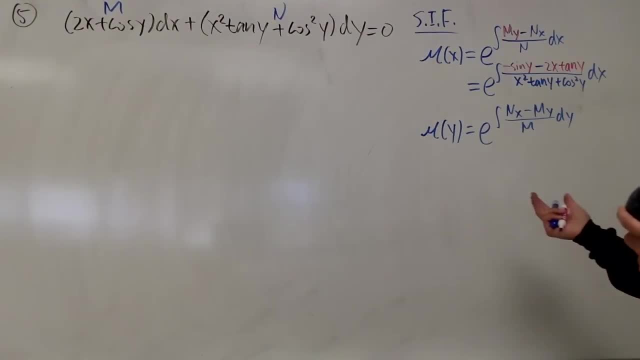 I, I don't really think that we can do too much right here. Uh, in the meantime, let's also write this down. So, uh, let's see, This is the e integral n sub x, which is that: 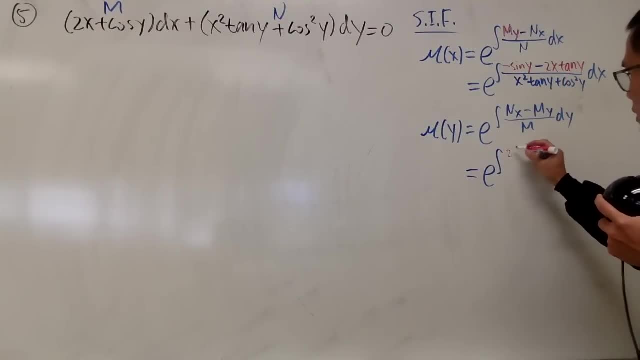 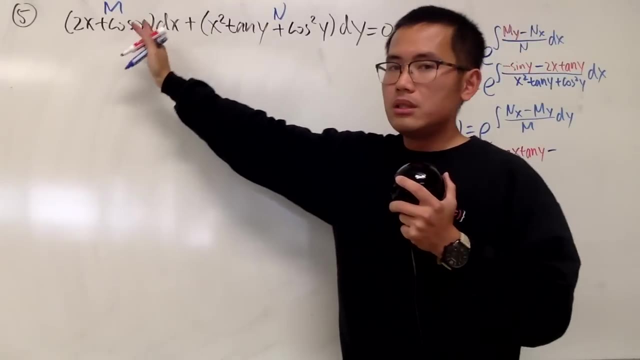 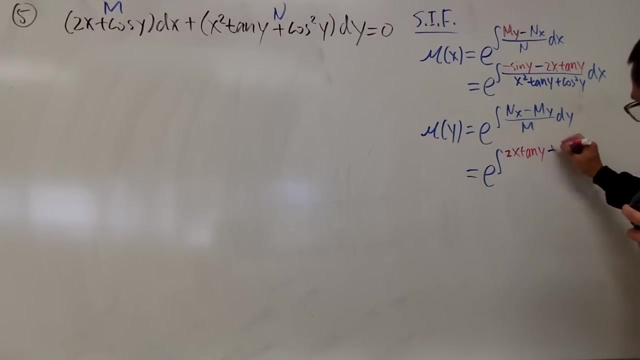 We have uh derivative of that, which is two x. Let's write down two x uh tangent y minus m sub y, which is going to be, um well, negative sine, yeah So. 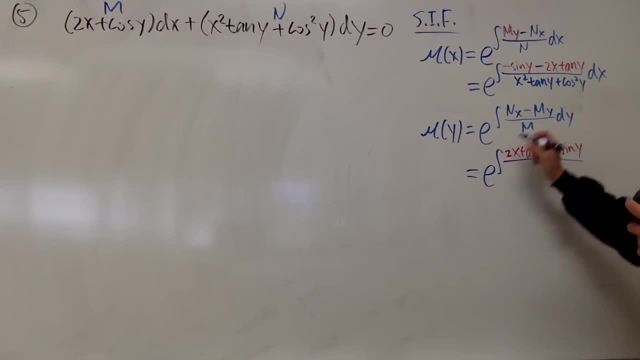 negative. negative becomes positive, and we have the sine y over m, which is the original two x plus cosine y, like so Okay. So now we just have to think about how can we simplify one. 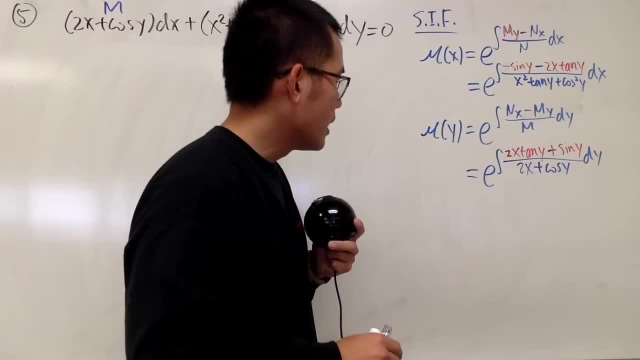 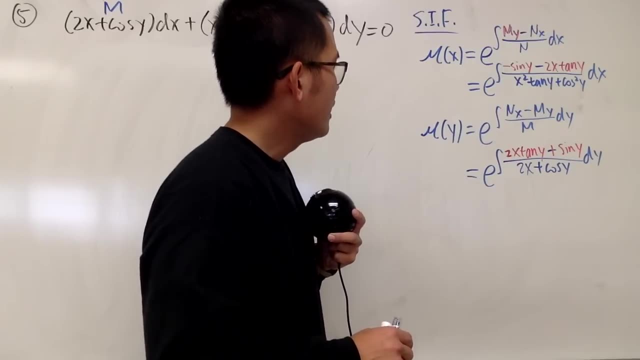 or the other, and then hopefully that's the situation And, hmm, Um, let's, uh, let's um. you see, right here, this is two x, this is x squared. I don't really think we're going to do too much. 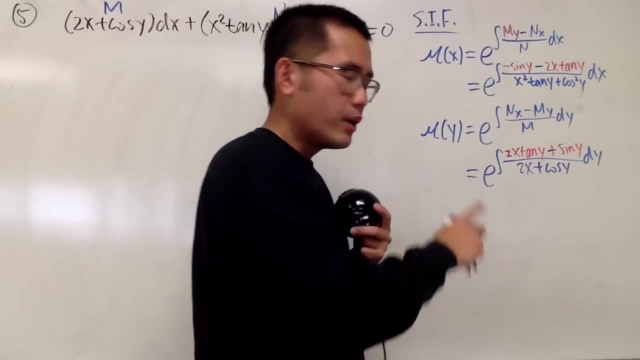 but I think we have a better hope, because this is two x and that's two x. So maybe this is the one that we can simplify And let's just do some trig identity business and all that stuff And 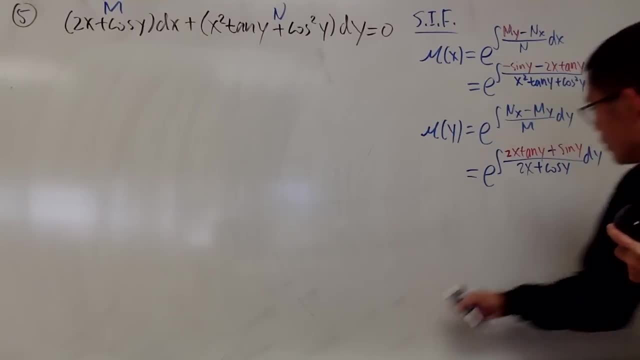 of course, as we all know, tangent y is the same as sine over cosine, So we can look at this as sine y over cosine y, And in that case you see, both of them have the. 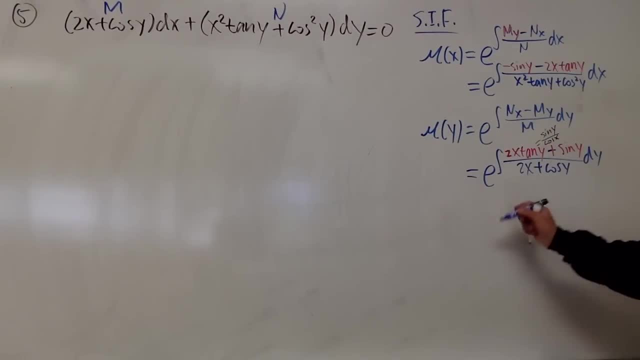 sine y, So we can factor that out. So let's do that, So we will have the e integral And let's factor out the sine, And we get a complex fraction. that's not what we like. 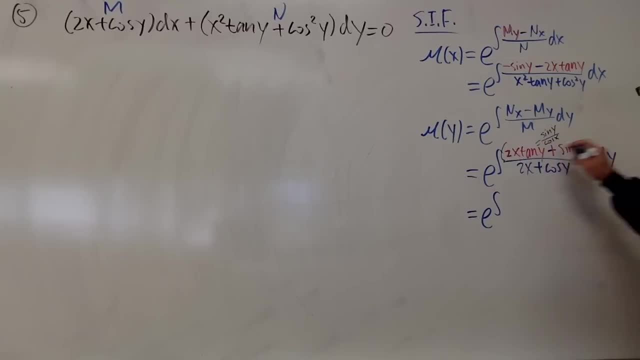 yeah, So let's go ahead and do the following. This right here is dy. Let's multiply the top and bottom by cosine x. And again, the purpose of all this is just to simplify this guy. Okay. 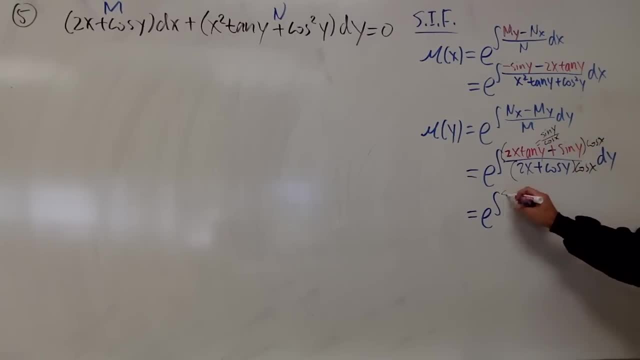 So I'm going to factor out the sine y right here. Focus Here: we have the sine y And then the y is out. The sine y is out, And then cosine, cosine, cancel. So 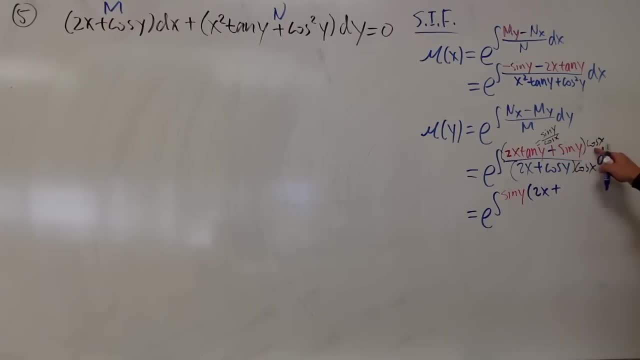 we just have two x left, Yes, And then plus original, the sine y is out. But we are multiplying by cosine, So it should be cosine y. It should be cosine y, Because this right here is supposed to be cosine y. 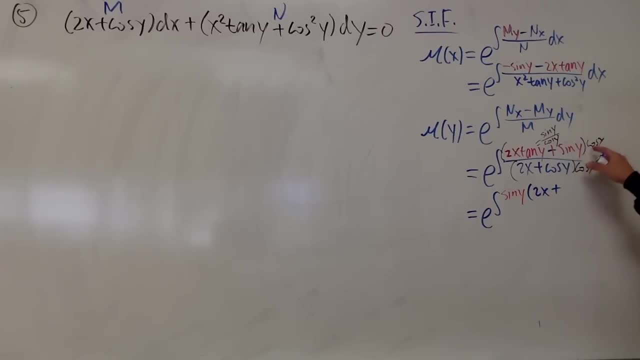 This right here is supposed to be cosine y, So cosine y, cosine y sine y is out This times. this, So we have two x plus cosine y. Ah, I see this, I see this, I see you. 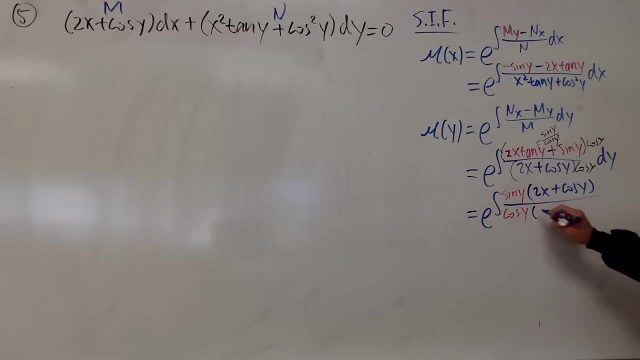 I see you. And then, divided by here, we have that cosine y- I'll just put that in the front- And then we have this part which is two x plus cosine y. Ah, This is so satisfying. 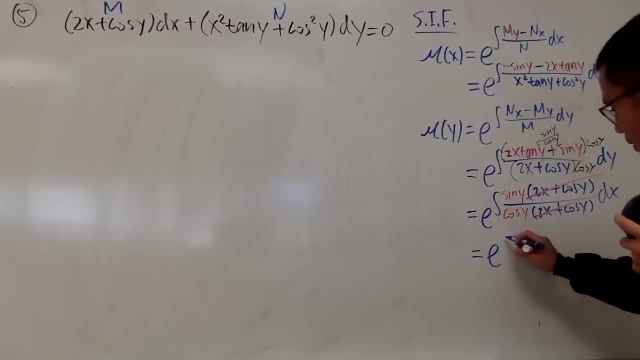 Because this and that cancel each other out. Yeah, So here we just have the integral, I mean the y, And of course the integral of tangent y is just ln absolute value of secant y. 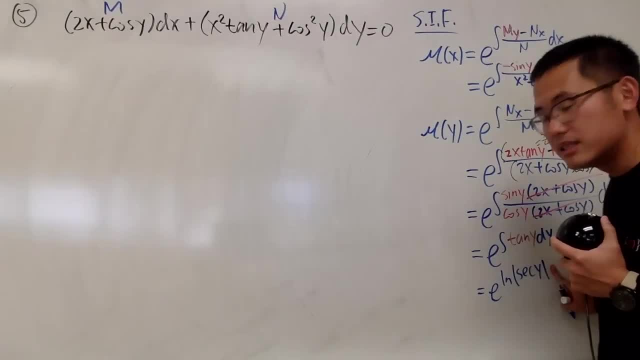 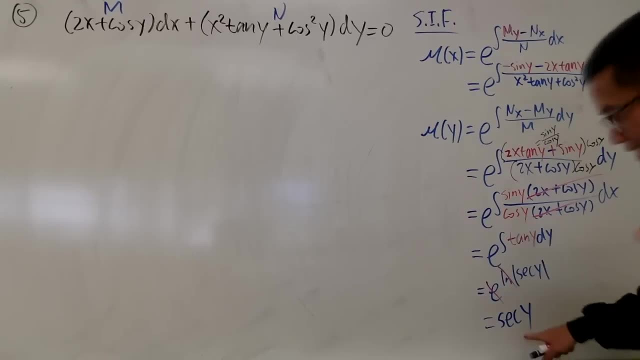 like this: And again, don't worry about the plus c, Don't worry about the absolute value, Just cancel them out And you actually get secant y. This is pretty sexy. Well, there's no. 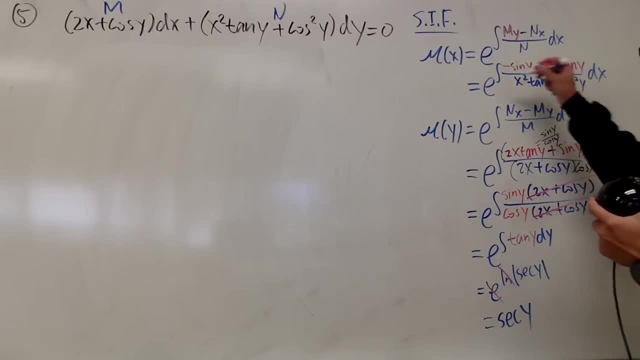 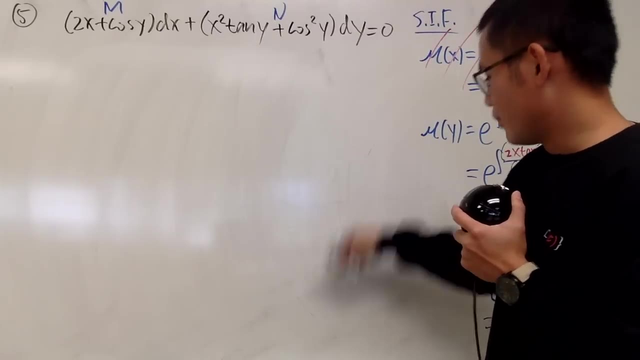 x sound or whatever. Anyway, secant y. So unfortunately, before we need it, this is So we'll come here and multiply everybody by secant y. So let's put this right here: Multiply. 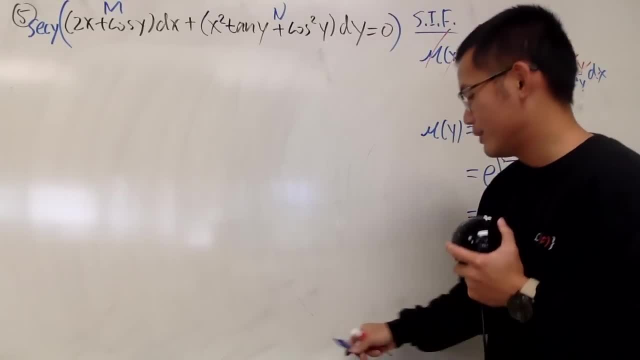 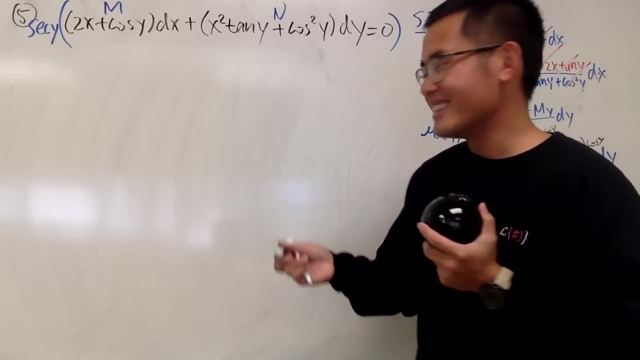 everything by secant y. Whew, Okay, So now continue. That took a while to figure this out, So imagine all the stress on your final exam track. Anyway, this times this we get two x. 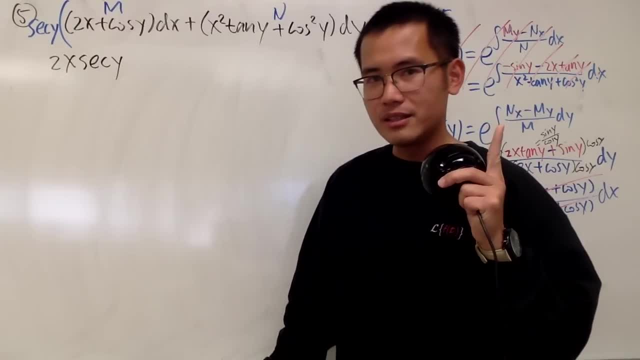 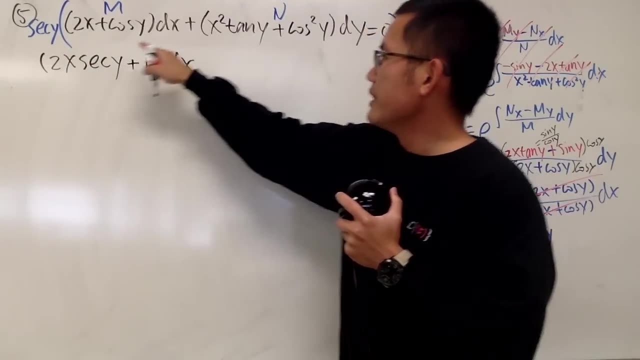 secant y. This times this, we get one, Because one over cosine and both of them is with y inside. So we have that dx this, and then this times this, And I will not. 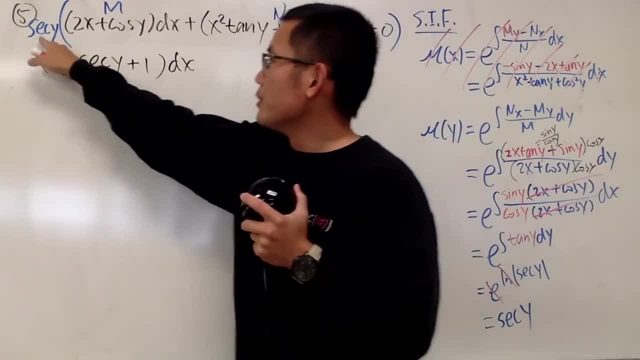 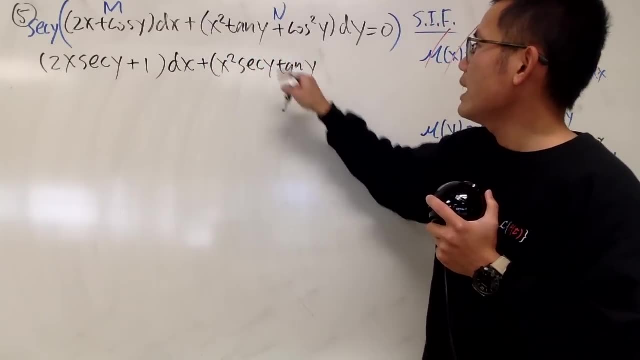 write tangent this sine over cosine, Because we'll be doing derivatives. I will be just writing them down, So I will plus x, square secant y, tangent y and lastly this and that Well. 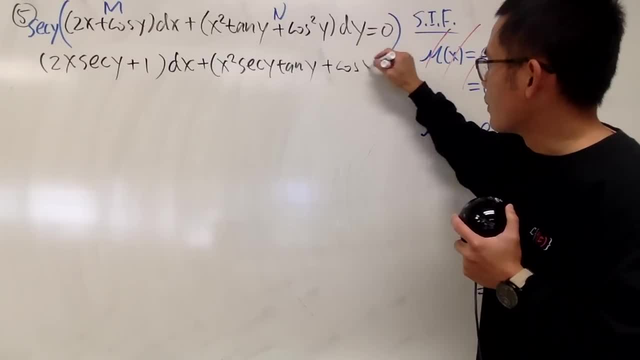 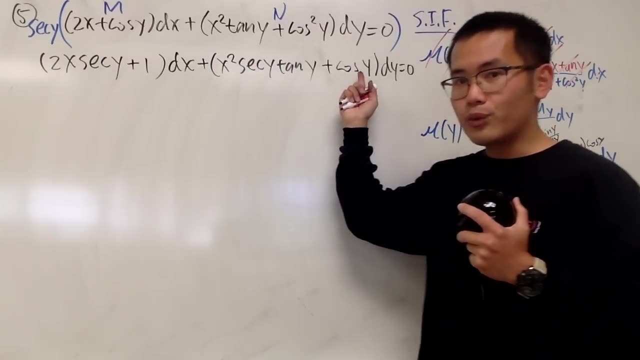 I'll cancel one of the cosine here. So this is plus cosine divide, that that's equal to zero. Alright, so again one over cosine y and that we just have cosine to the first power. This is guaranteed to be. 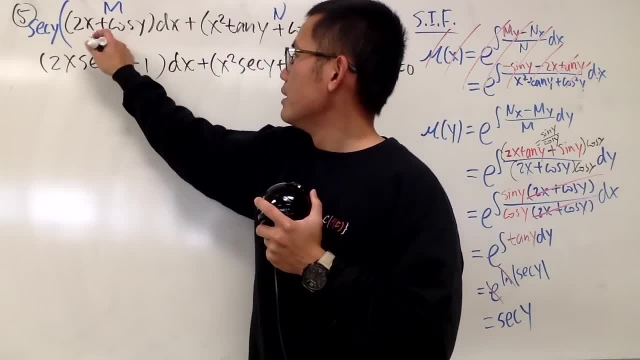 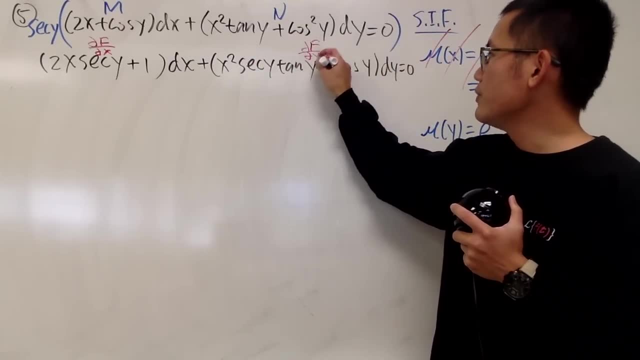 exact. So that means there is some function. if you differentiate that with respect to x, And you'll get that part, And this is the part that. if you differentiate that with respect to y, Let's do that part. 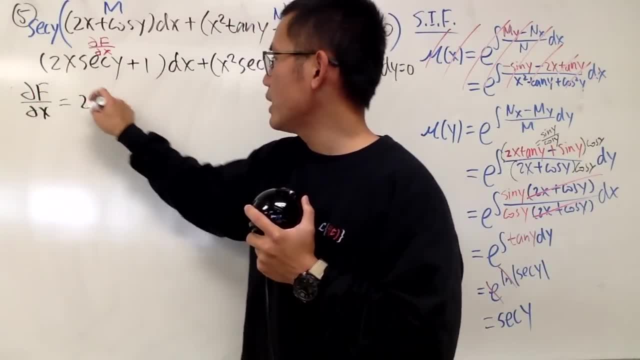 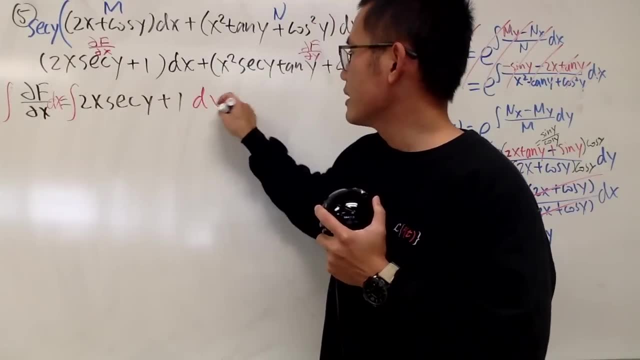 So I'll write down partial f with respect to x is equal to two x and y plus one. Integrate both sides, dx, ah, in the x world. So go ahead and dx. that Here is. 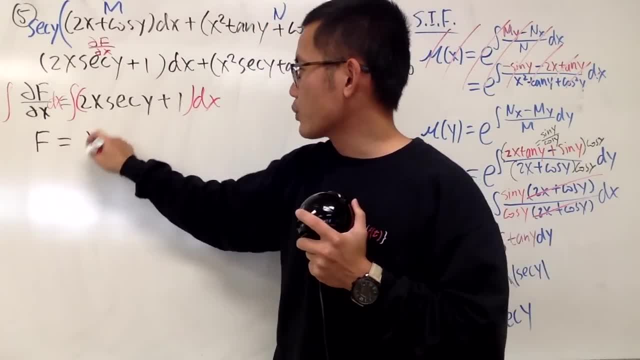 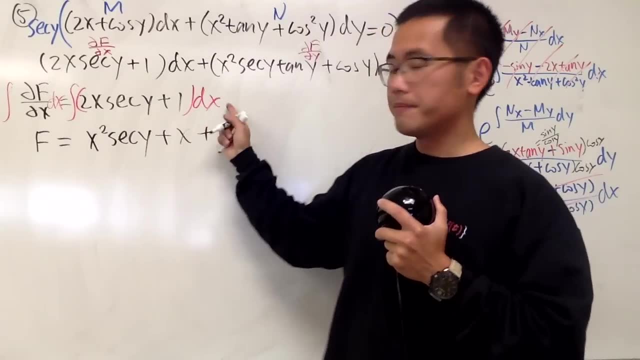 how capital F looks like. Well, this right here will give us x squared. and then this is just a constant multiple. just keep it The one in the x world. when you integrate that, you get x, And 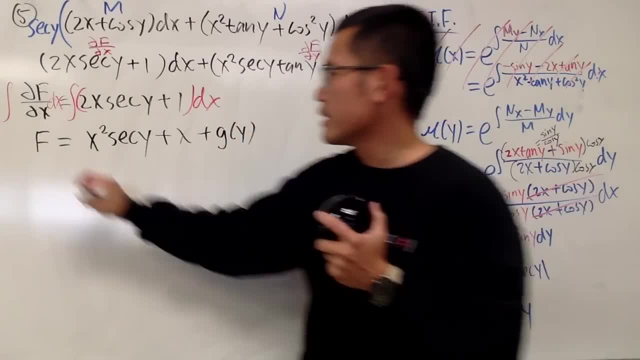 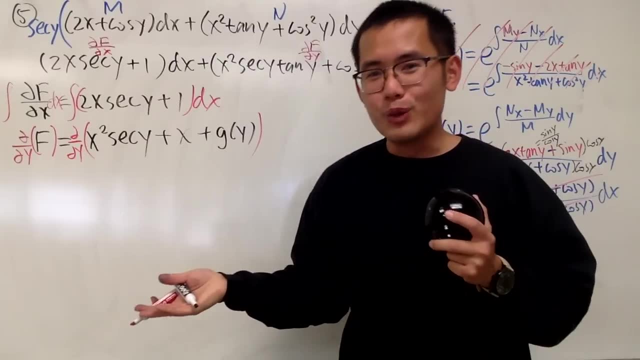 don't forget, y is the constant in the x world. So we have to add a function in terms of y, like this: And then I mean, do the partial of f with respect to y, And then we'll get. 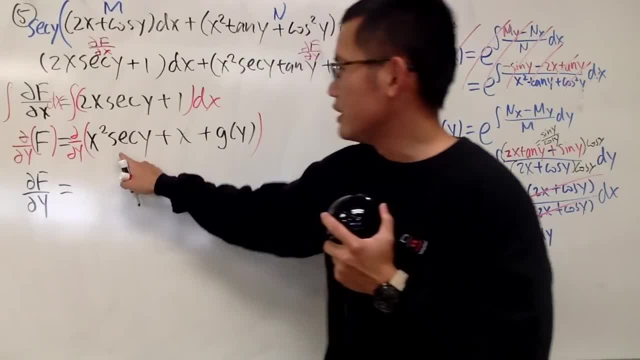 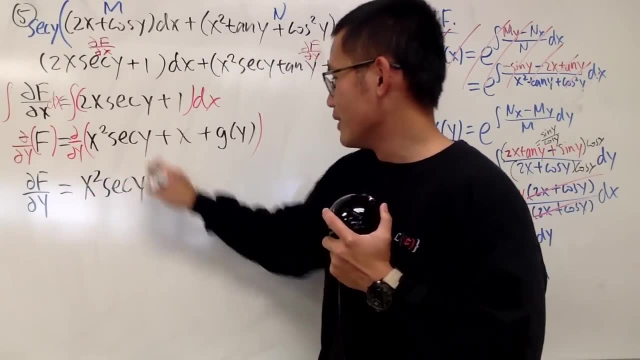 the partial of f with respect to y equals differentiating. secant y. we can secant tangent. Look at that And the x squared again is just chilling in the front. So secant y, tangent y. 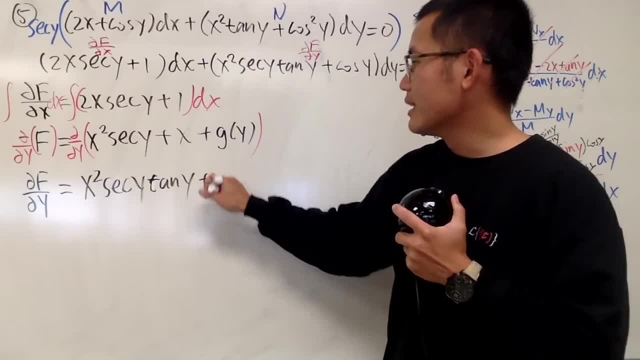 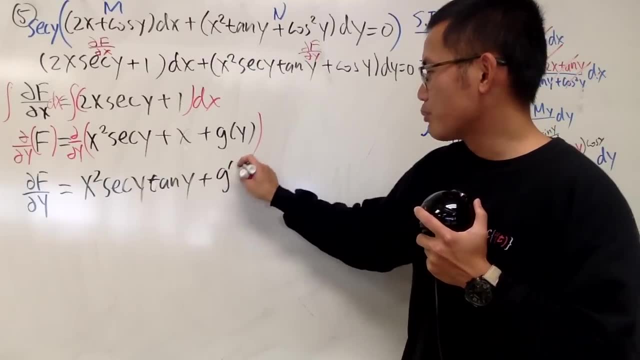 like this, And then we add: the derivative of this is what? Nothing, Because we are in the y world, So it's just nothing. And then we add y. Now, this is partial of f with respect to y. 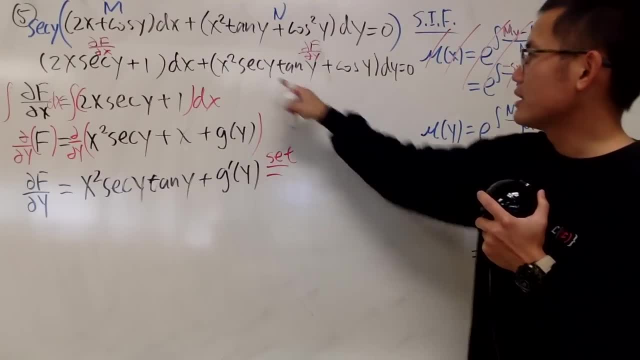 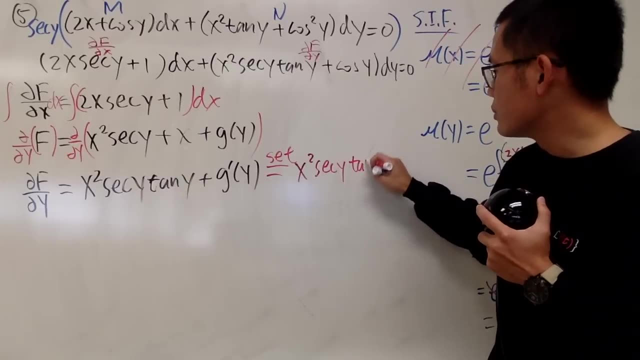 We have to set this to be the right hand side here, Like this part. So we have x squared. let me just put this on here: why not x squared? secant y, tangent y plus. 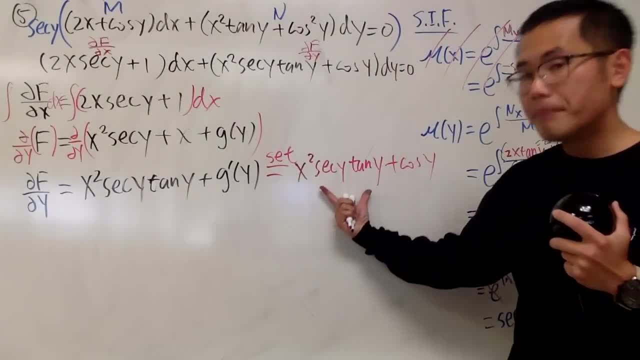 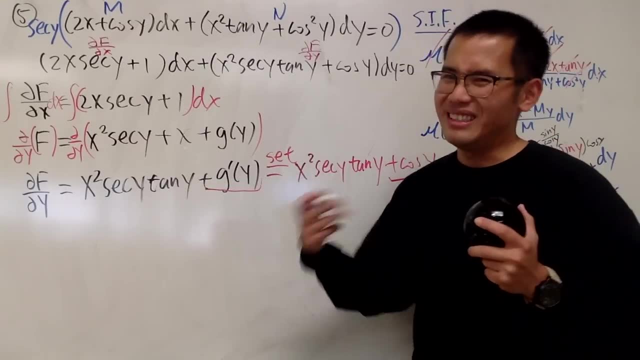 cosine y And, as we can see, this part, that part match. So that means this part has to be the same as that. So f prime, just like the one earlier. they are not always equal to zero. 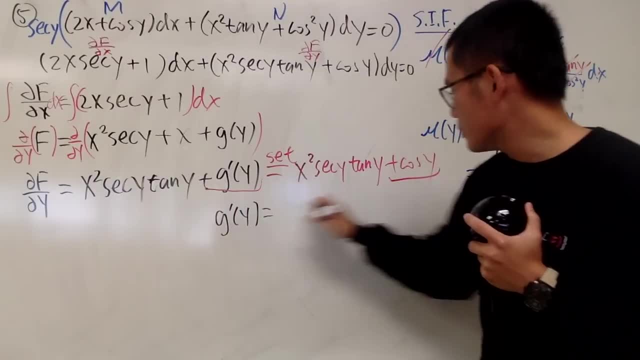 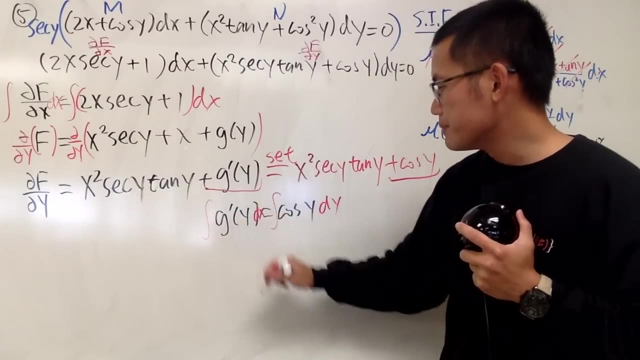 This right here, we know g prime of y has to be equal to that, namely cosine y. Of course, go ahead, integrate both sides in the y world. So this right here is just g of y. 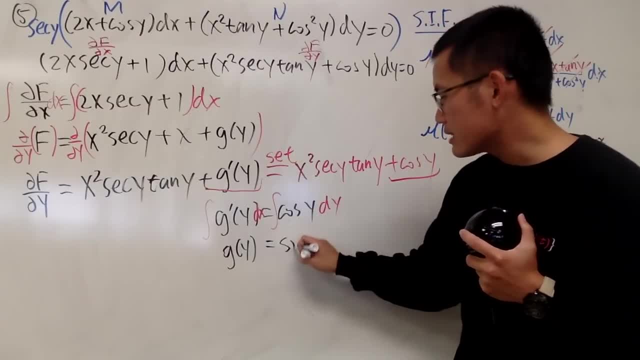 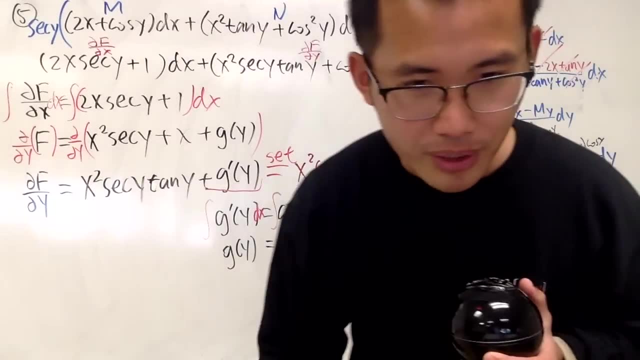 The derivative of y will give you cosine y. The answer to that is positive, sine y. And of course you can put down the plus c, but again kick the c to the other side. We are done. There's no initial condition. 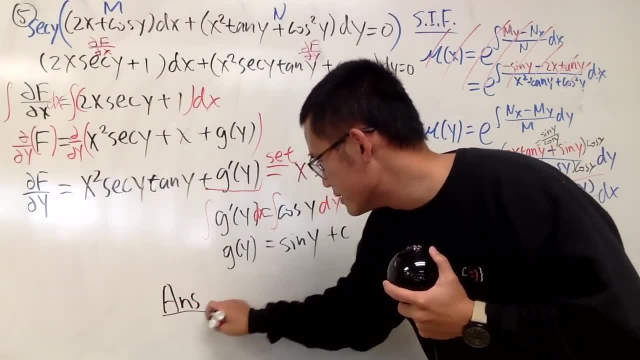 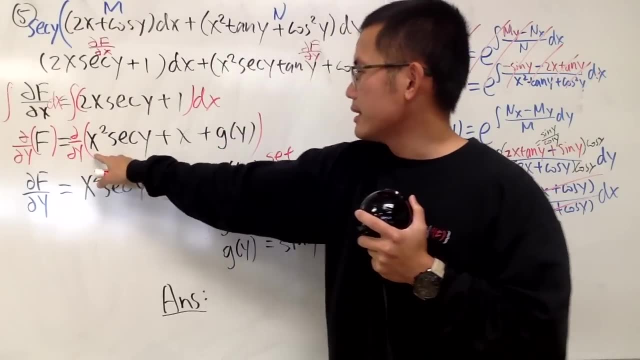 right, Okay, so finally, here is the answer. Let's see, let's see, let's see, Here is my capital F, right Original F, in black, and then this that let's write that down first. 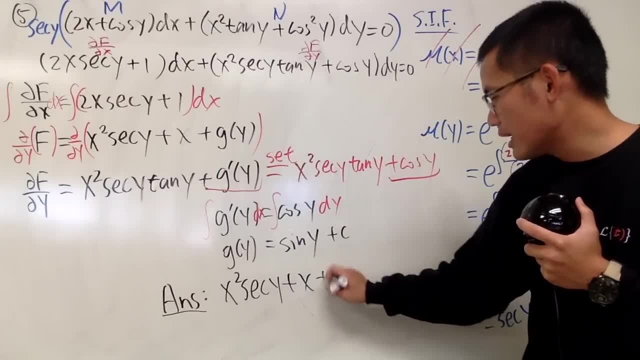 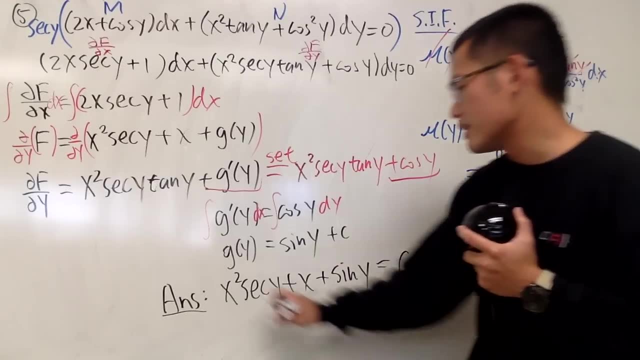 x square secant, y plus x, and then this guy is just plus sine y. And again I'll put the c to the other side, and still just a constant. It's not because we are messing on the algebra. 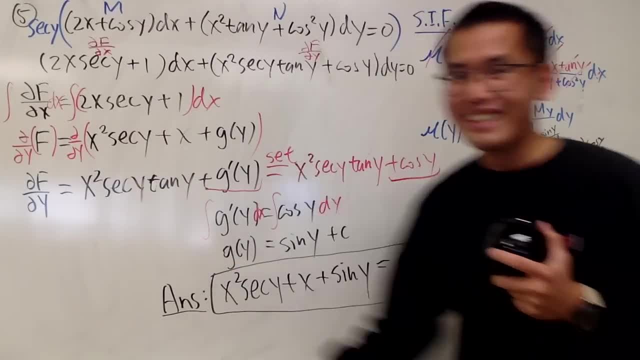 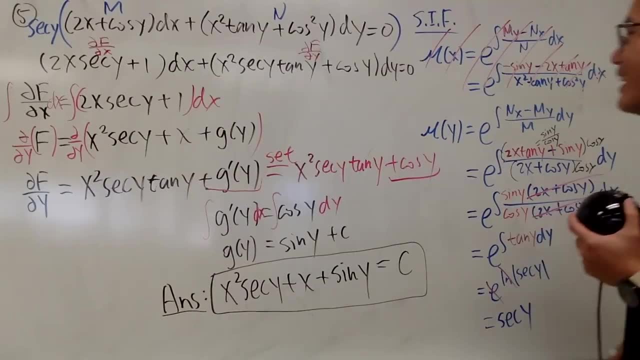 it's just constant. you can do whatever you want, the operation is still constant. All right, so I'll step out a little bit, and this right here is the answer. Very good, huh, Okay, so that's pretty much it. 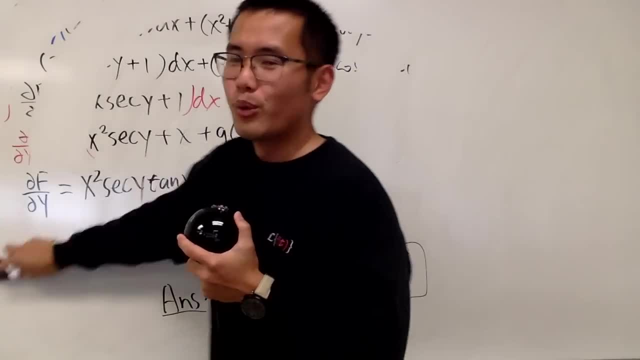 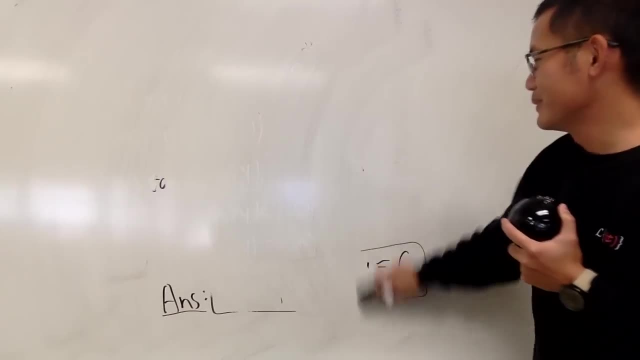 So yeah, I pretty much tried to erase the board like 24 times. Imagine how long 100 differential equations will take, right, So don't ask me to do 100 differential equations. 24, I think is just about right. 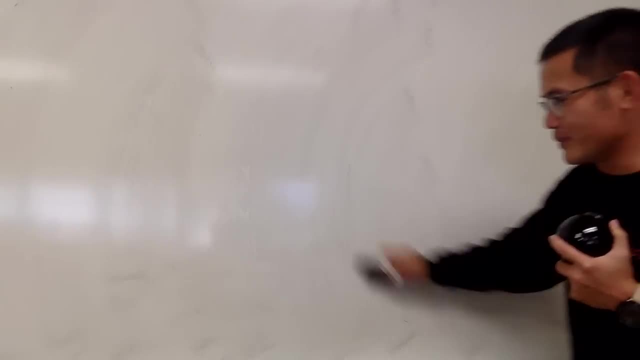 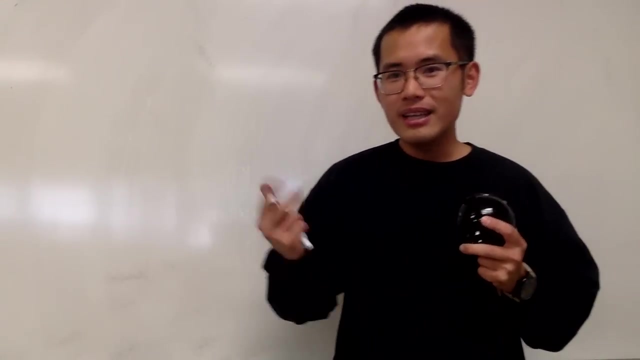 And you'll find this to be helpful. right, I'm doing all this for you guys, Especially for my former Cal 2 students. right, Shout out to Brett, Brian, Eric and the rest of you guys. 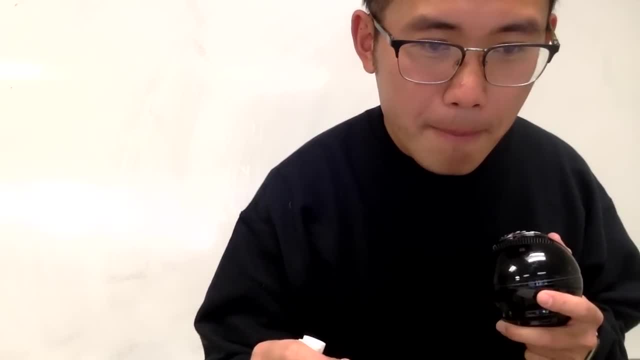 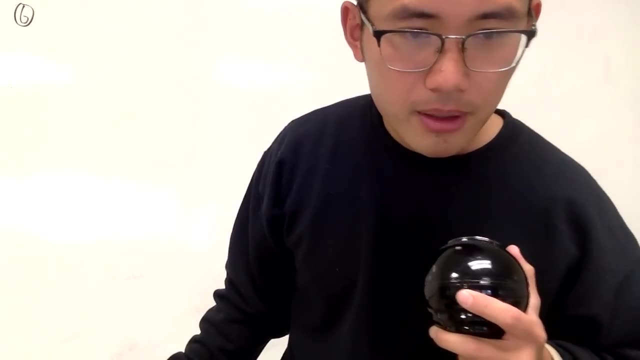 And I miss you guys. and best of luck to you guys, Best wishes and all that stuff. Number 6.. Here we go. Number 6, we have parentheses: x squared plus 1, dy dx. 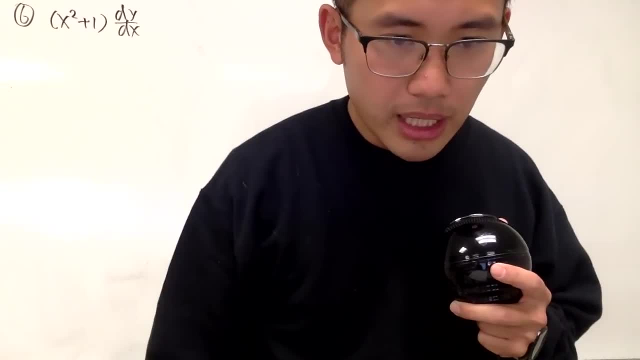 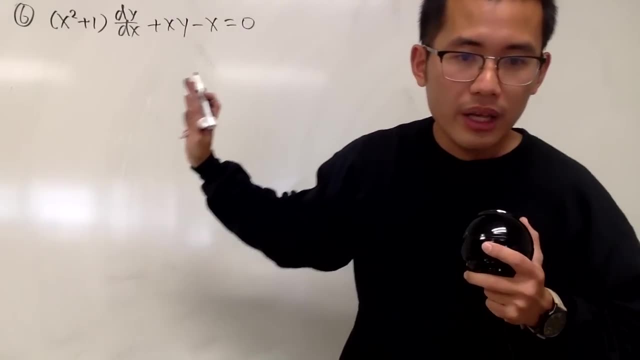 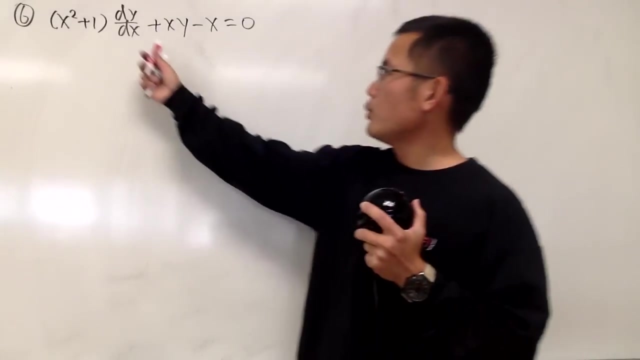 So dy dx. And then we have plus x, y, minus x equals 0. And thankfully there's no initial condition. Good, Hmm, We have the dy dx, We have the y to the first power. 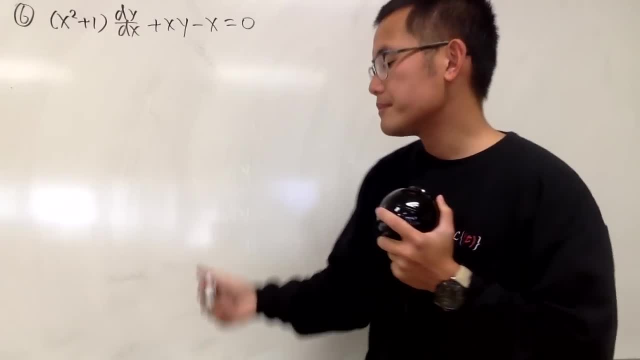 and there's no other y's, So this, right here, is a linear situation. What we have to do first, though, is to put this in the standard form. I will have to get rid of this, So I want to. 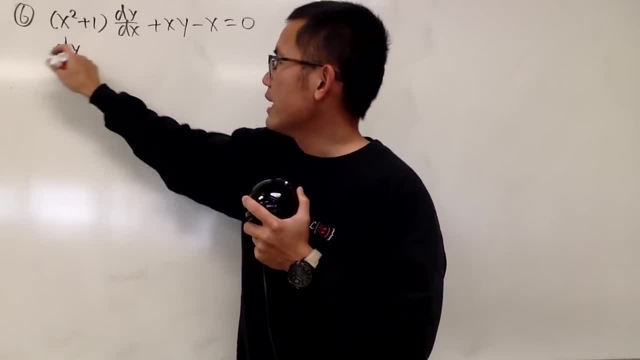 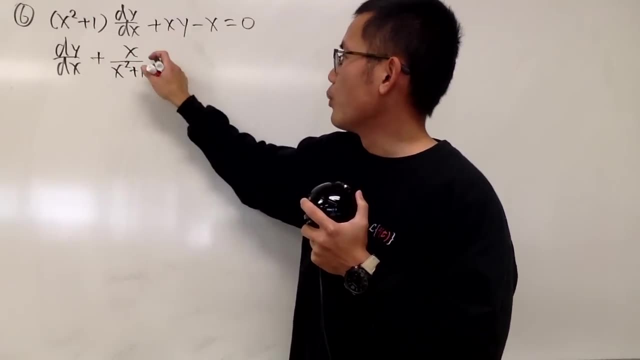 divide everybody by this guy. So we get dy dx plus x over that x squared plus 1.. And then the y, And then I will bring this to the other side, So it becomes: 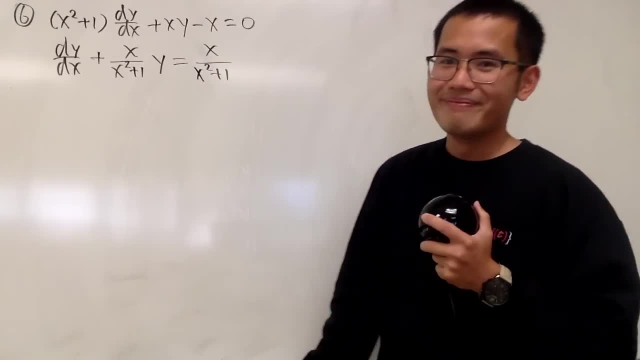 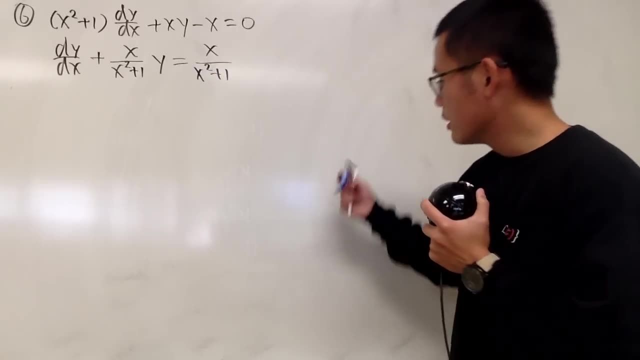 plus the x over that. So just like this. Good, Now the special integrating factor. I will put this down in blue, Because why not? So I'll just write this down right here. I should have enough space. 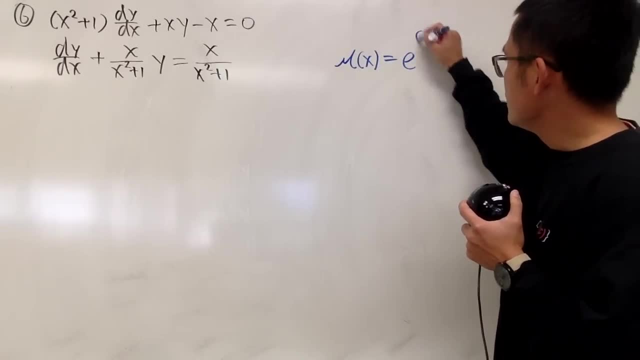 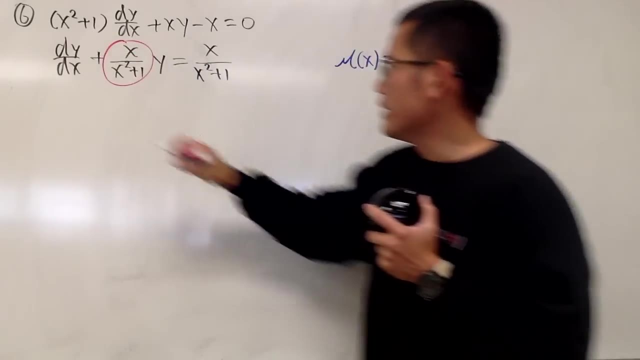 to do all that. So put this down, Okay. So this right here is e integral and we have x over x squared plus 1.. Because, again, this right here is the p of x. 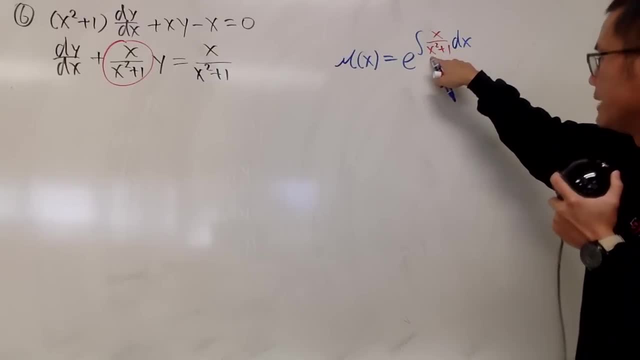 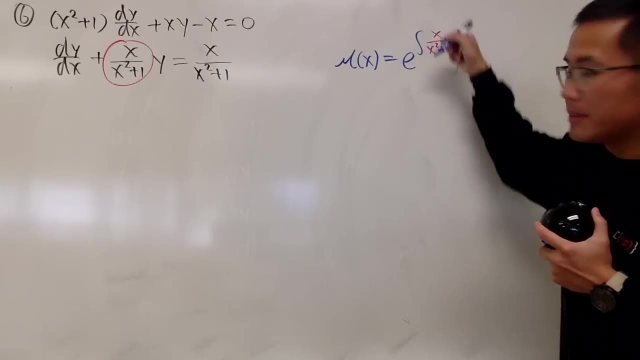 And we are in the x world. Go ahead and integrate that Right. So do this in your head. Let u equal to the denominator x squared plus 1.. So you can divide this here by dividing by 2,. 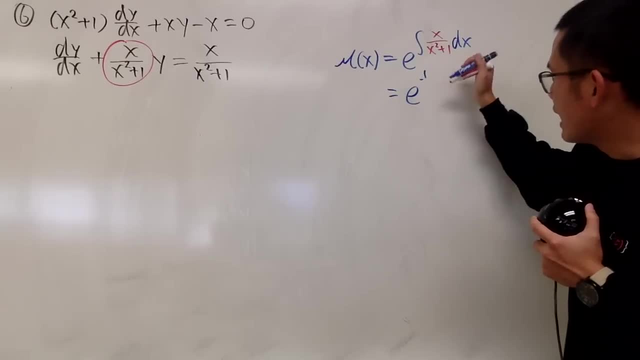 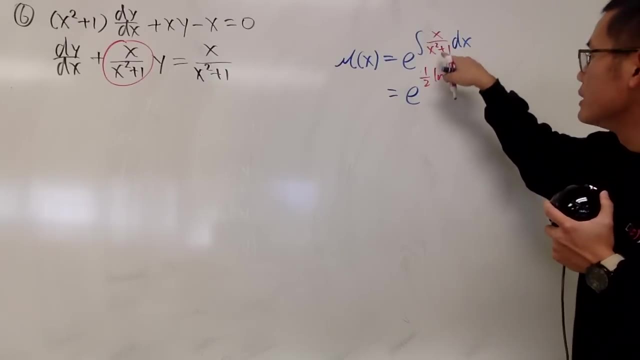 right, But anyway, all in all, you will get e and the result of the integral is 1 half. Let me actually write this down in red: The result of the integral is actually 1 half ln. 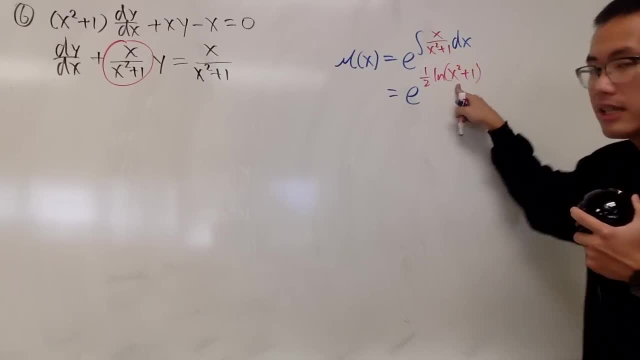 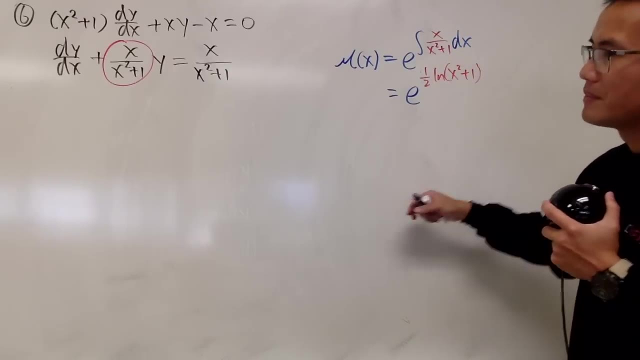 u and the u is that which is just x squared plus 1.. Here I don't even need the absolute value, because the inside is always positive, Just a cultural stuff and so on. And then 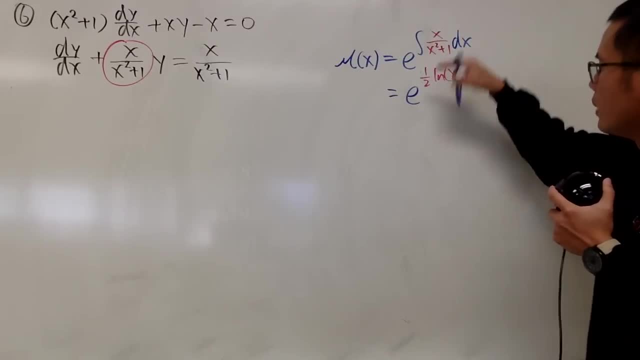 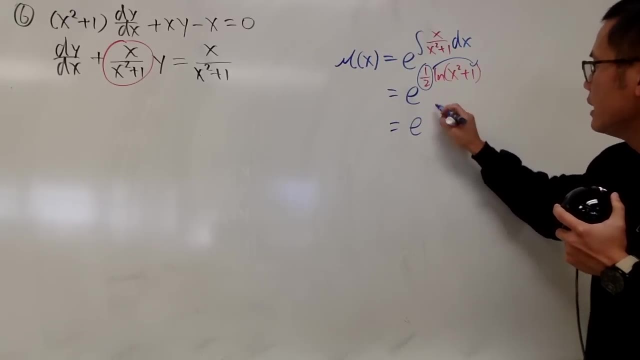 don't worry about the plus e, right? Don't worry about that. In order for us to get rid of the e and ln, though, you have to bring this up here, So you actually have e- ln. 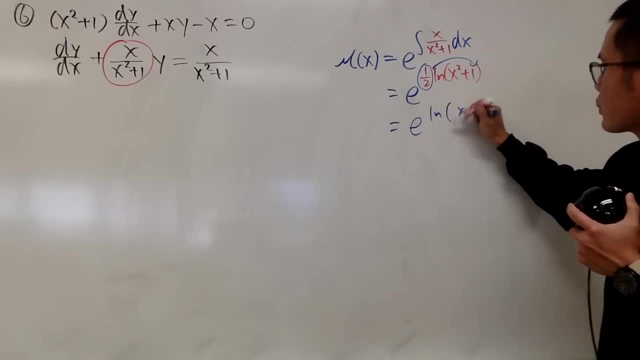 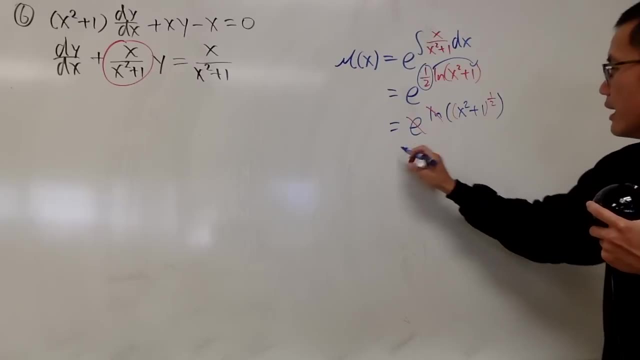 parentheses, and this is uh x squared plus 1, to the 1 half power, like this: And of course, now you can just get rid of this and that, And the 1 half power is of course. 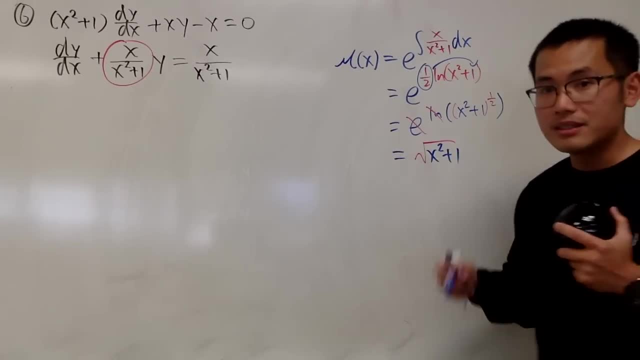 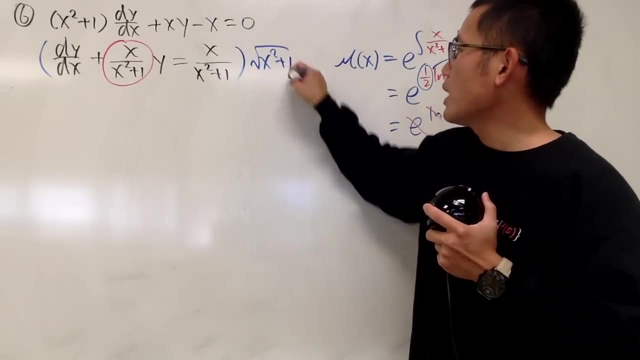 the same as square root, so square root of x squared plus 1.. So this is the integrating factor. Go ahead, multiply everybody by the integrating factor: square root of x squared plus 1.. Good So. 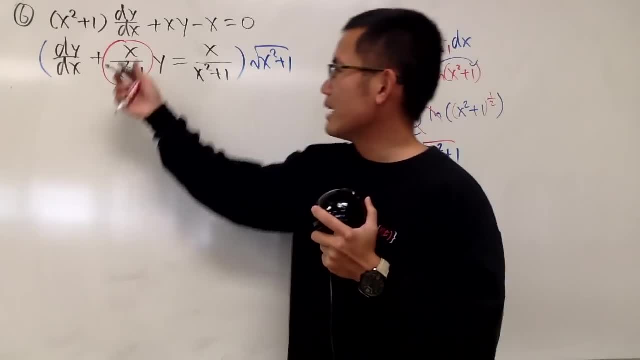 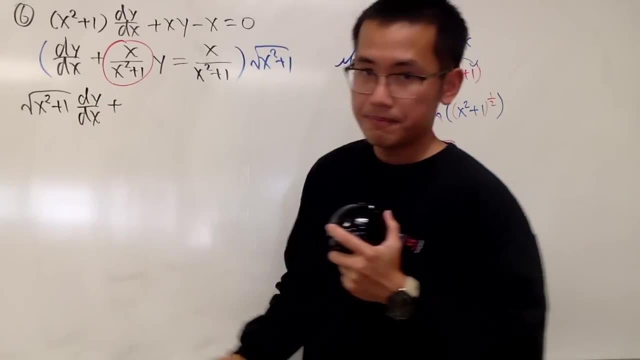 black pen, I mean blue pen, can take a risk now. Now, this times the first part. we have square root of x squared plus 1, dy, dx plus. now here's the deal x over this. 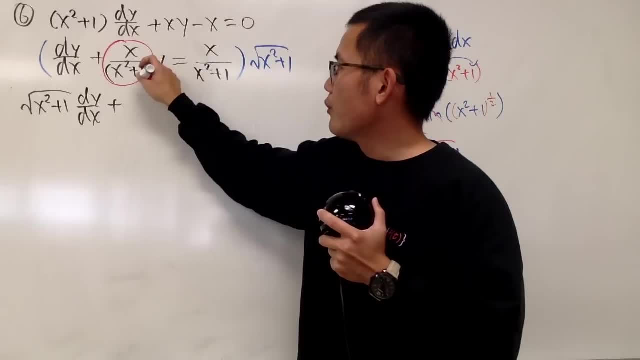 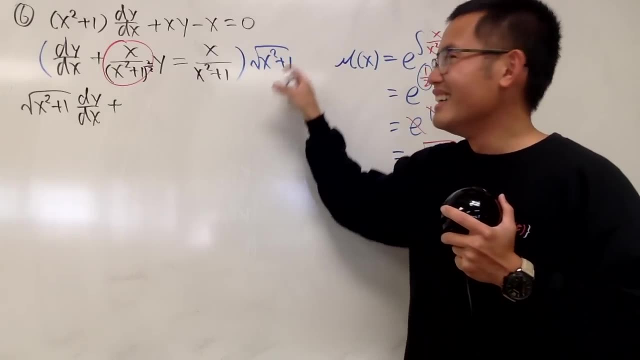 this input and that input are the same. This right here is the same as saying: to the 2 over 2 power: yeah, To the 1 over 2 power, 1 over 2 minus that. so you have another 1 half power. 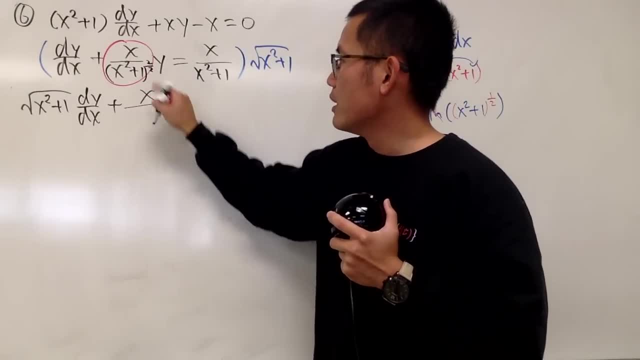 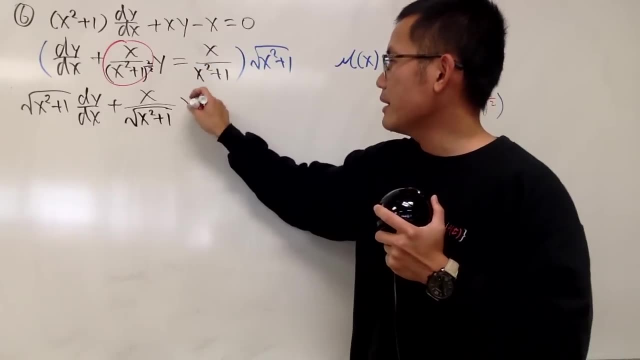 on the bottom. So this times that we get x over, which is just the square root, x squared plus 1.. Right, So this and that, And then we have the y, and then that's equal to. 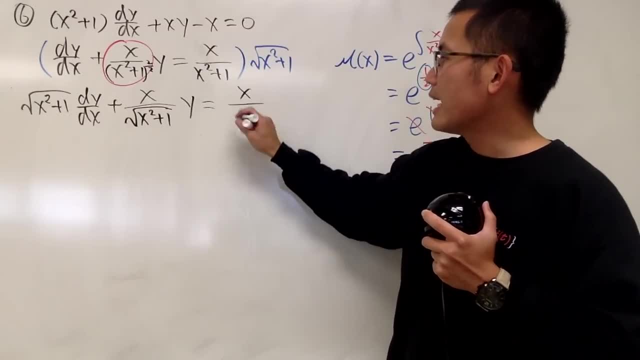 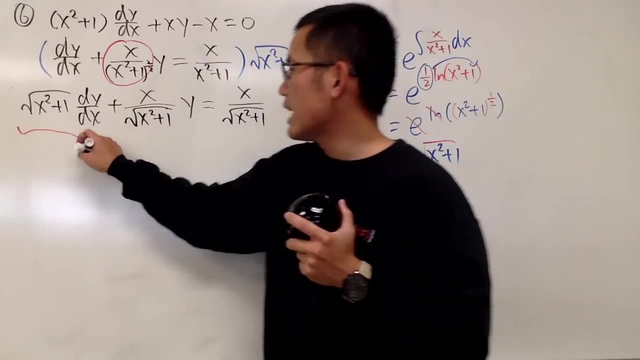 again same business. x stays on the top over this and this divided by that, you have the square root, x squared plus 1.. Now I promise you, the left hand side is the derivative. 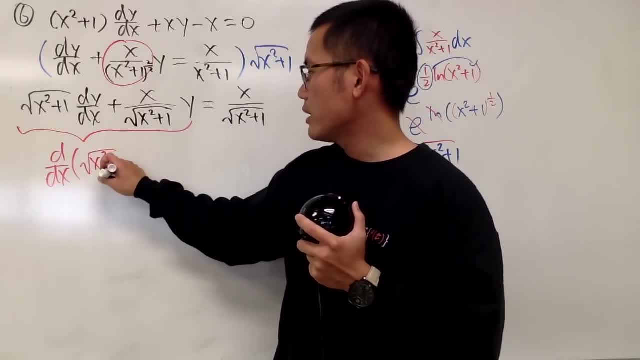 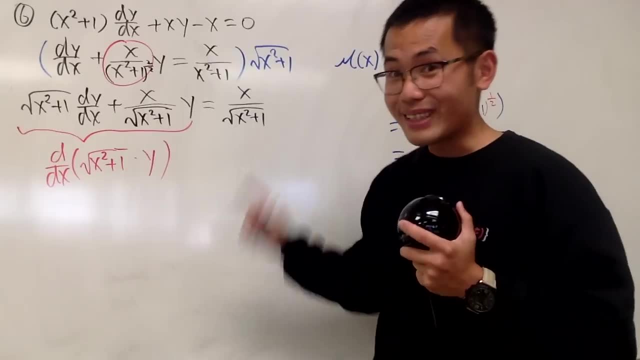 of a product of two functions and we have x squared plus 1 in the square root and then the y, Guaranteed The integrating factor, and also the y. That's why the integrating factor works. It's always like that. 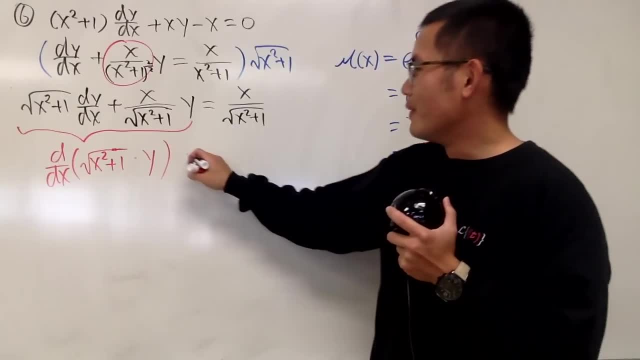 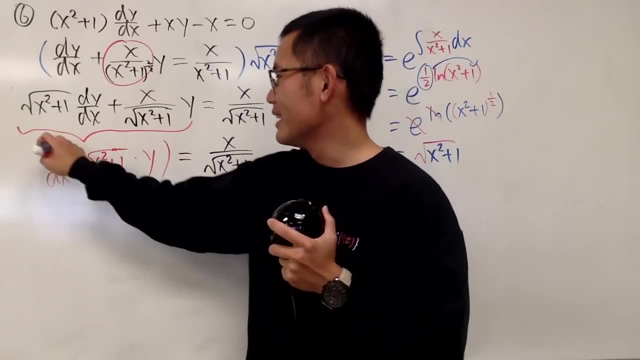 Right, It works so magically. And the right hand side. we have x over square root of x squared plus 1.. Now let's go ahead. use the blue pen again, integrate both sides in the x world. 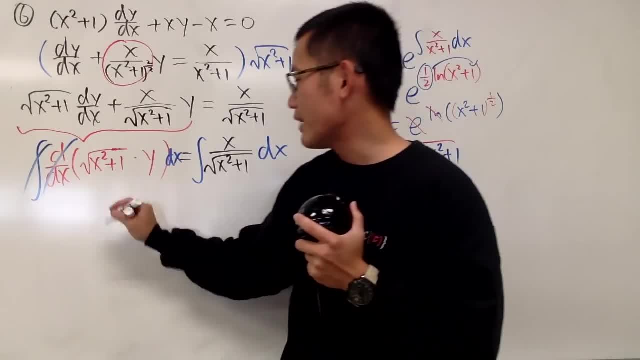 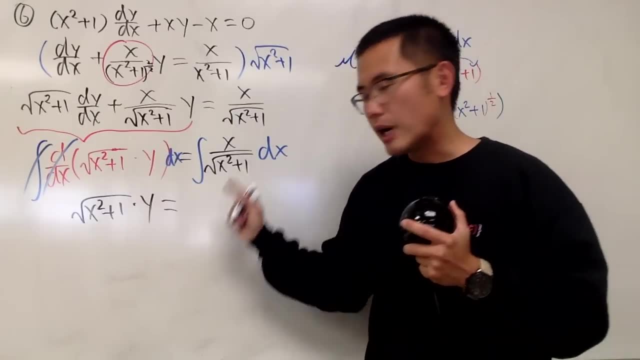 This and that cancel very nicely. and here we just have this inside, which is the square root of x squared plus 1, times y, That's equal. to integrate this in our head, we get square root of. 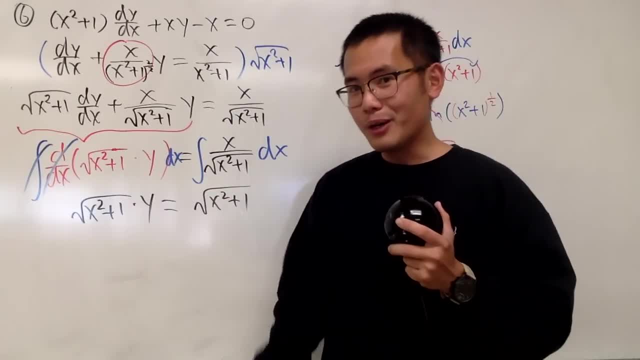 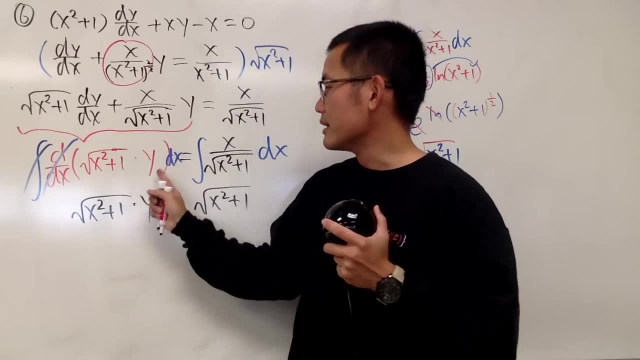 x squared plus 1.. Why? Because I know it already. You see, right here, The derivative of this is the first function times the derivative second plus function times, the derivative of the first. So the derivative of this. 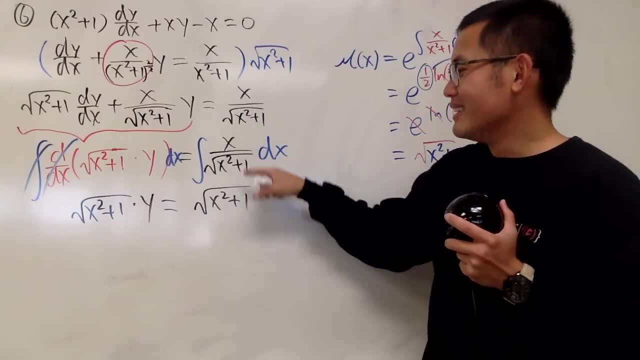 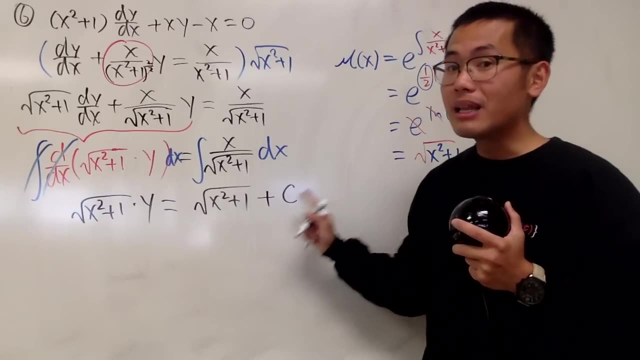 is equal to that. It just happened to be right here. The derivative of this is equal to that, so the integral of this is equal to this. Easy, Then don't forget to put down the constant of plus c. 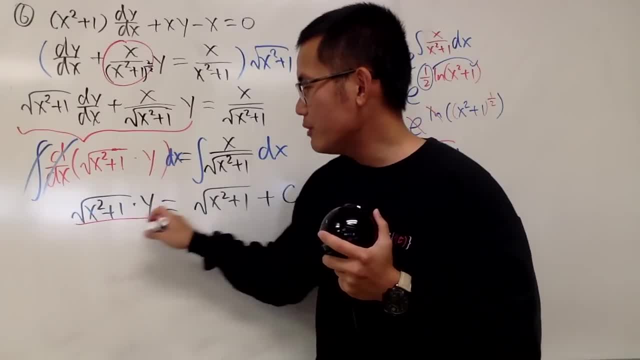 right here, Because if you don't have the plus c, it's going to look something weird. Because now we have to divide everybody by this. I will just show you guys the work. because why not Divide everybody by this? 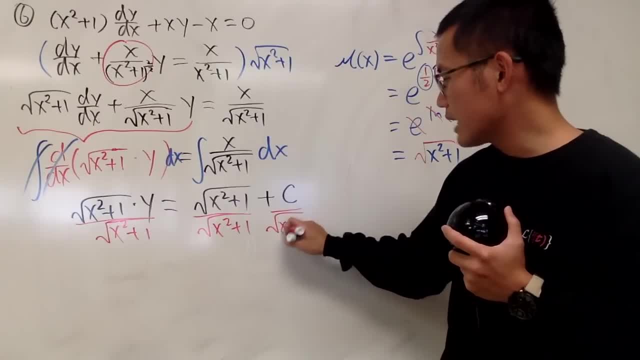 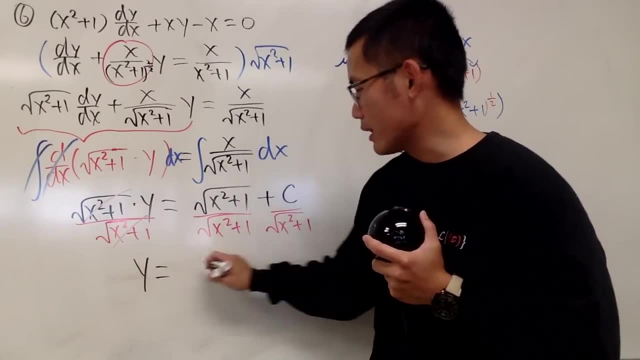 Divide everybody by this And you see over this guy. If you forget the plus c, then it looks like you will just end up with y is equal to 1. Which is seriously does not make sense. 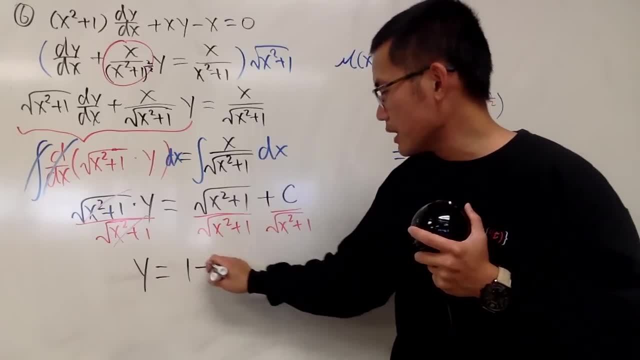 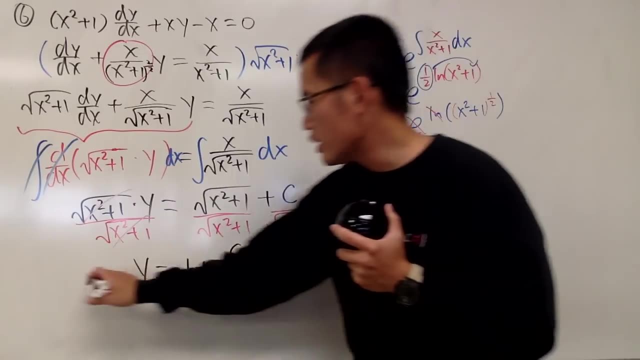 to the original differential equation. You can go ahead and try it. Don't forget this part: plus c over square root of x, squared plus 1.. That's the answer. This is the general solution to the. 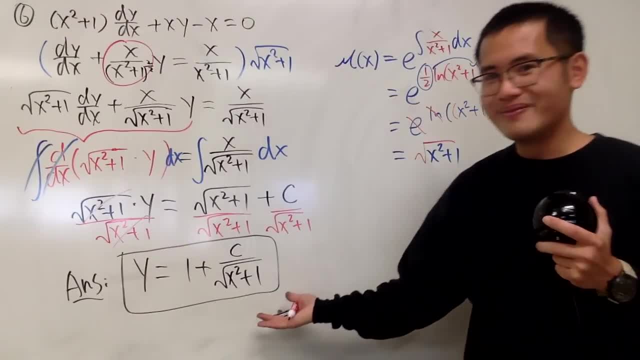 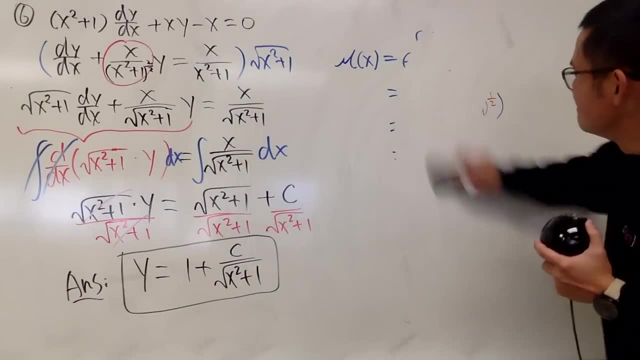 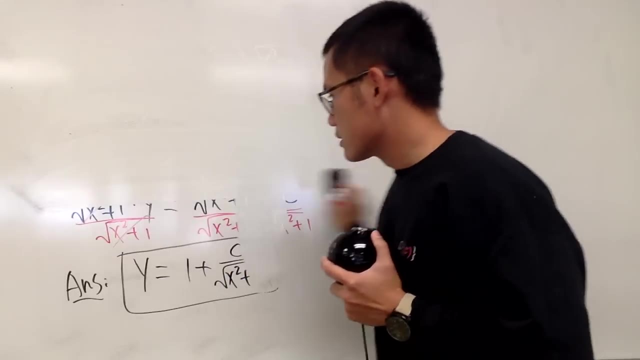 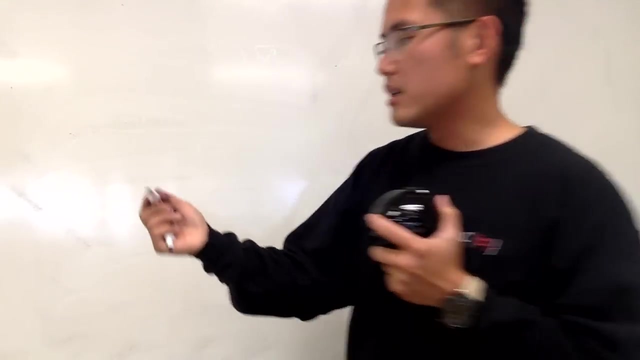 first world differential equation that we have over there. So this is it. So have a look, have a look, have a look. Okay, Right Number 7. Here we have, we have dy. 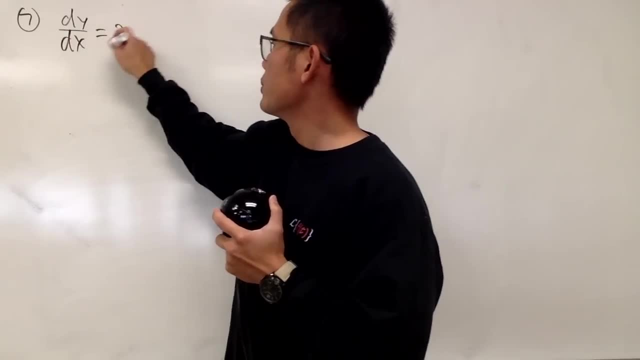 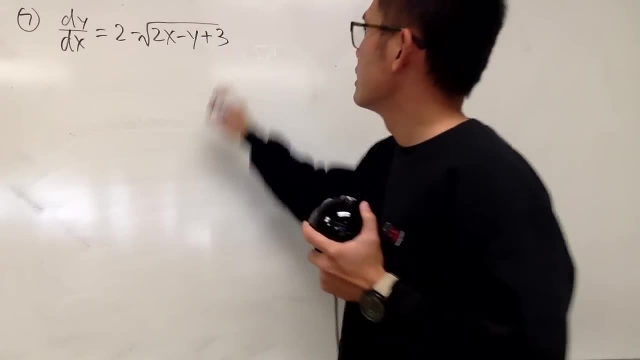 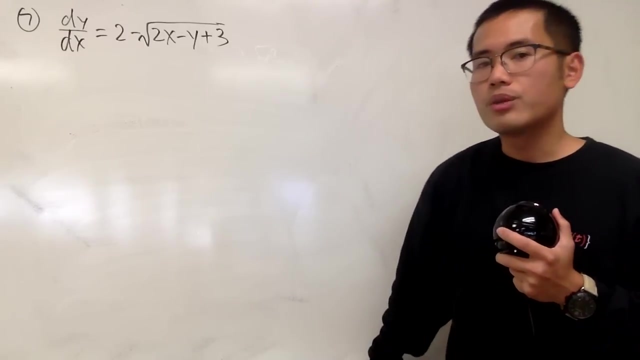 dx. Okay, good, dy dx. that's equal to x minus y plus 3.. Yes, Just like this. No initial conditions. So now let's take a look, and all we can do is this: 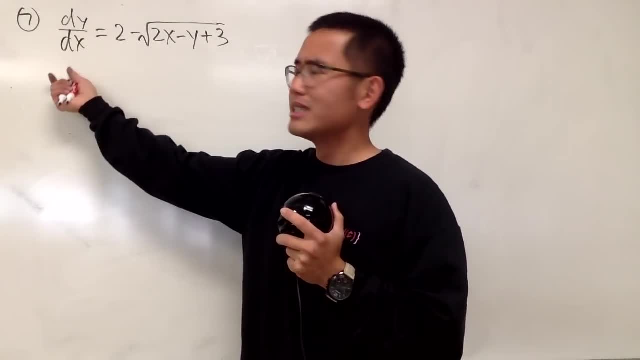 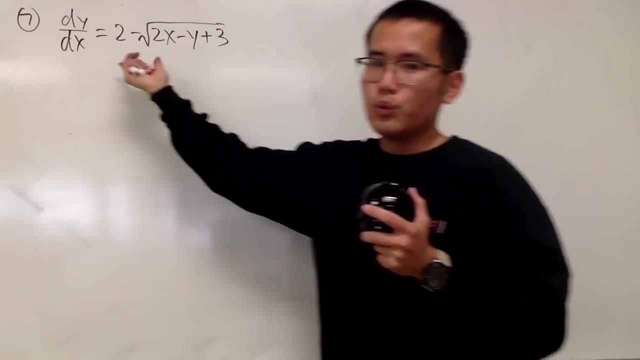 Usually when we have just this kind of things. it's not exact. I say usually, Because if you multiply the dx on both sides, you see there's nothing in front of the dy besides 1. So if you differentiate that with respect to x, 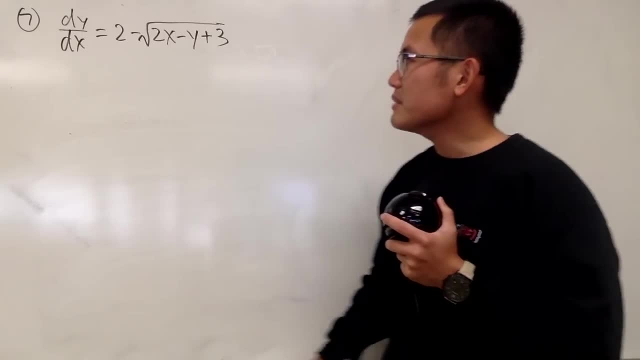 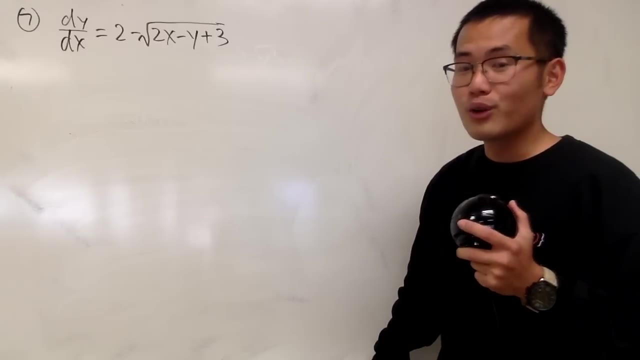 you get 0. If you multiply that with respect to y, you get something crazy right. So it's not exact. Don't go for the almost exact. Don't go for special integrating factor if you don't have to. 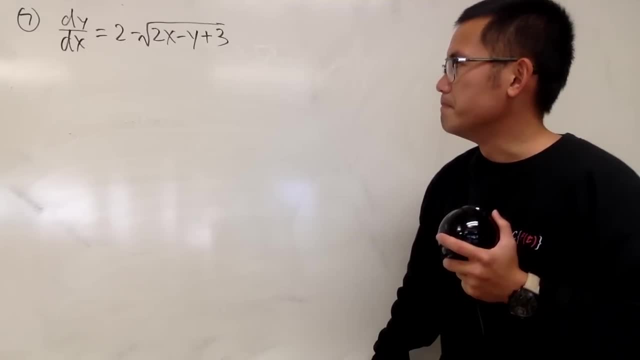 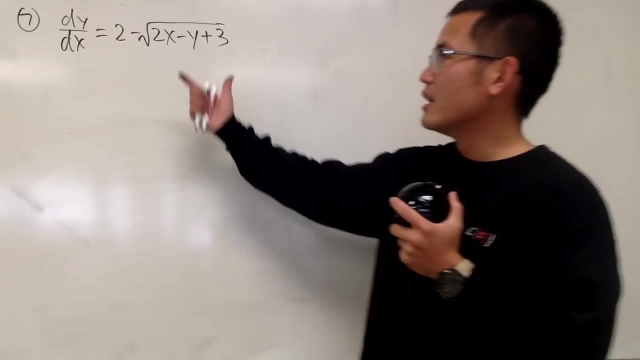 Life doesn't have to be that hard sometimes. Hmm, It's not linear, though, because we have the square root. Man y is inside of a square root. no good, But have a look here, This square root of 2x. 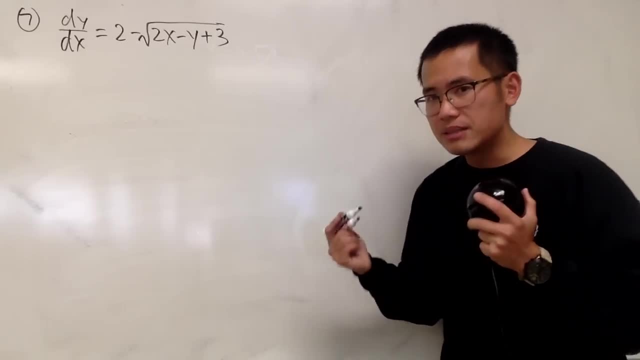 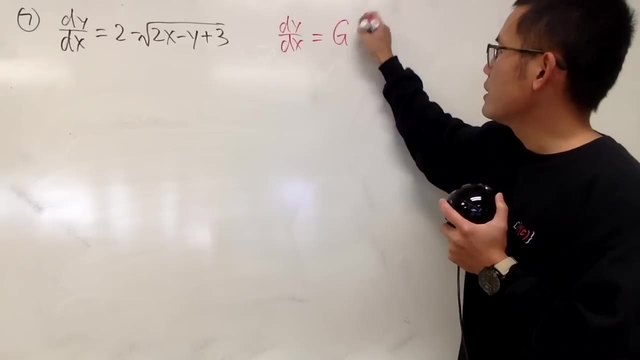 minus y plus 3.. In fact, this right here is in the special form. Let me write this down right here for you guys. We have dy dx. that's equal to some function in terms of ax plus. 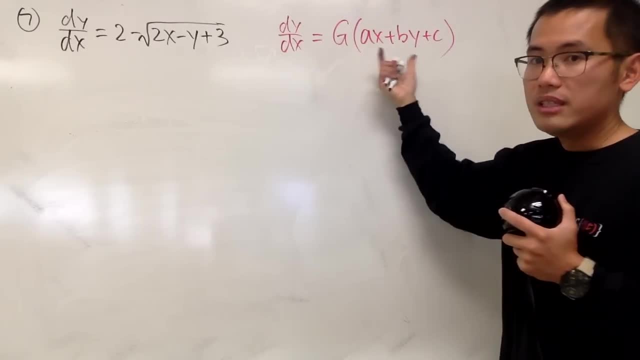 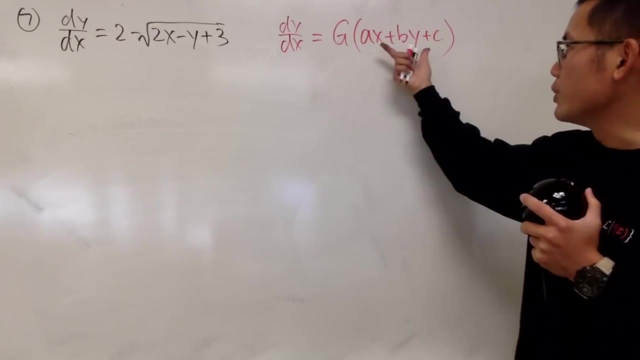 by plus c. This right here is just a linear combination of all that right Ax first, plus by first and plus the constant, like this, And we do have this as the input right here. Whenever this happen, we can go ahead and try. 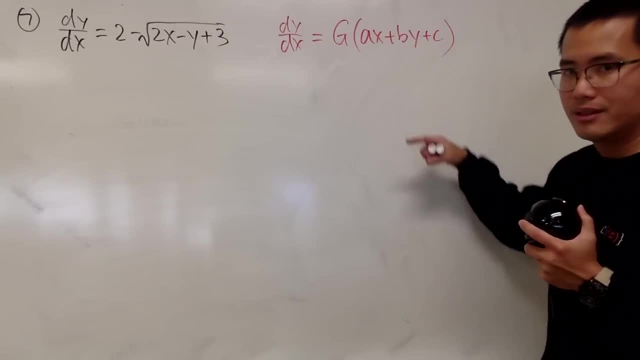 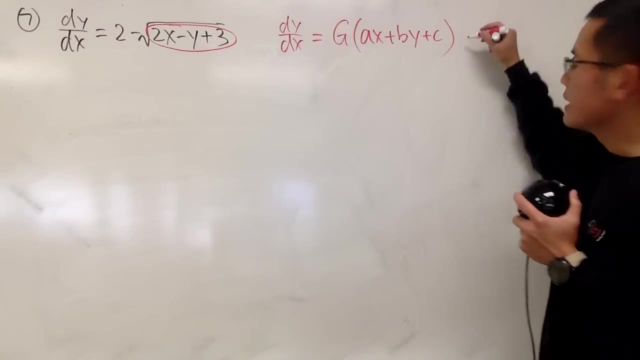 to do a substitution for the input, And that's exactly what we'll do In our situation. we have this, So I will just say: go ahead and do the following. I will put down this right here in blue. 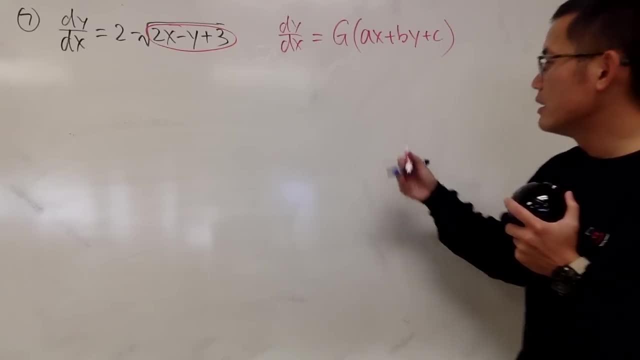 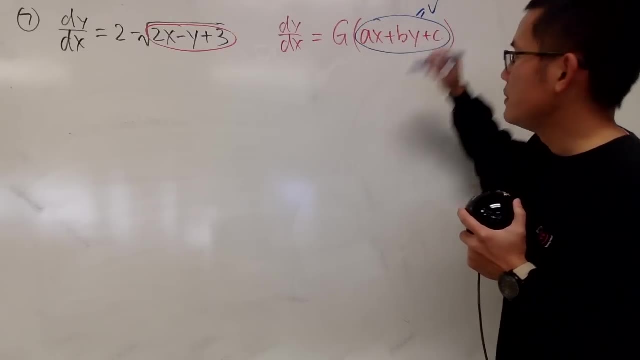 I'm going to let v equal to that, So let's see So again. usually when you have this, just go ahead and let this to be v, So I'll probably match my color. This right here is the. 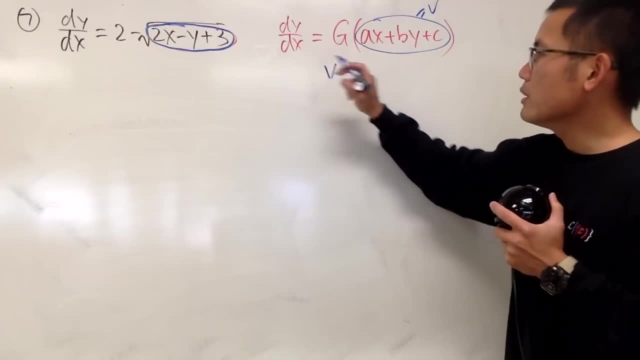 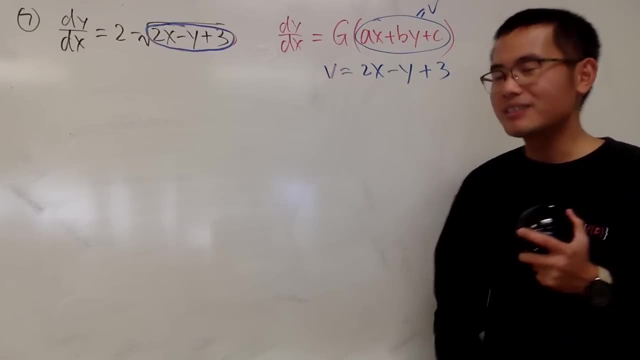 v. So let's go ahead and do: v equals 2x minus y plus 3. And hope for the best. Seriously, we do have to hope for the best sometimes. Anyway, go ahead, do the usual business. 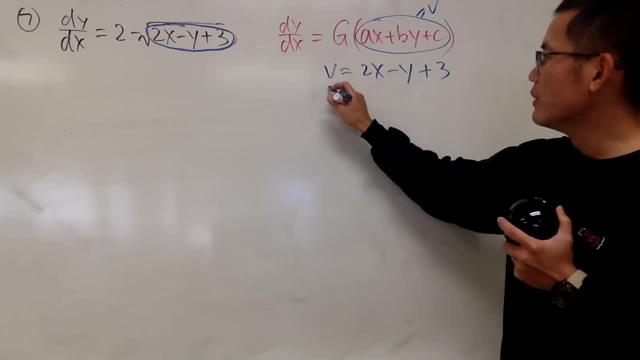 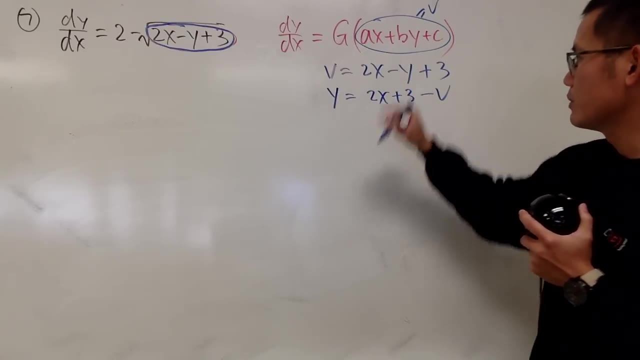 Perhaps I'll move the y to the other side and then move the v here first, So we actually get y equals 2x plus 3, and then minus v. Yeah, Do all that stuff, And then this is dy. 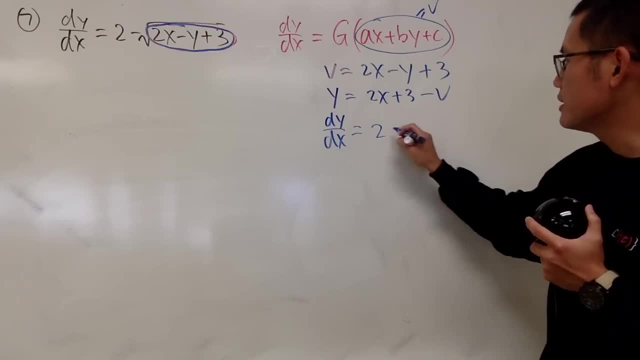 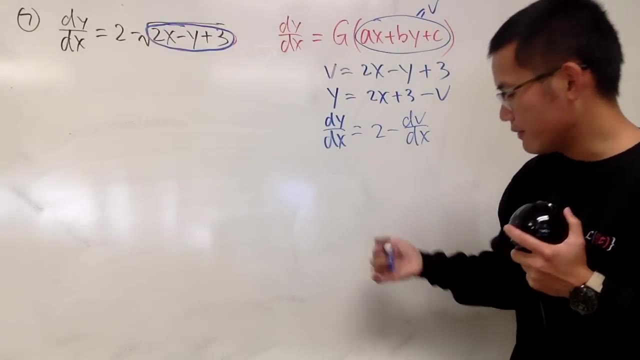 dx equals. derivative of this is 2, derivative of this is 0, derivative of this is minus dv. dx Like this. Now go back there, and we will have the following: Bring this with us, though We have. 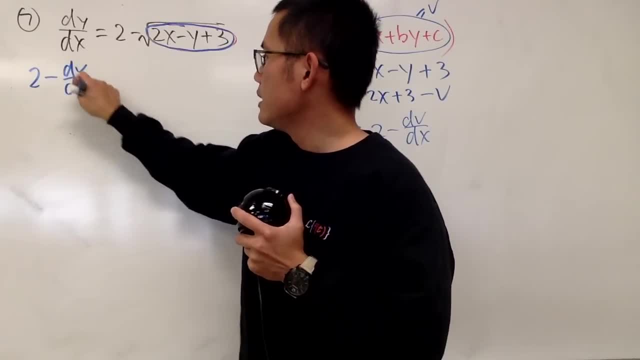 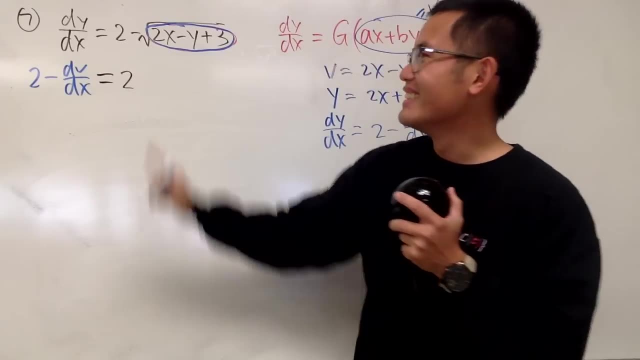 2, minus dv, dx for the dy dx, And this is very nicely equal to 2,. right here, Very nice, This right here, minus square root of what v, Because that's what we have for the input. 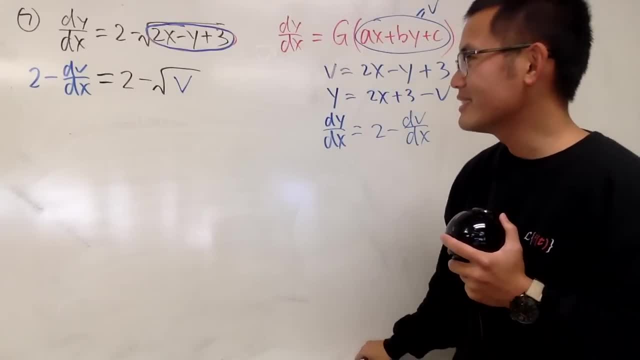 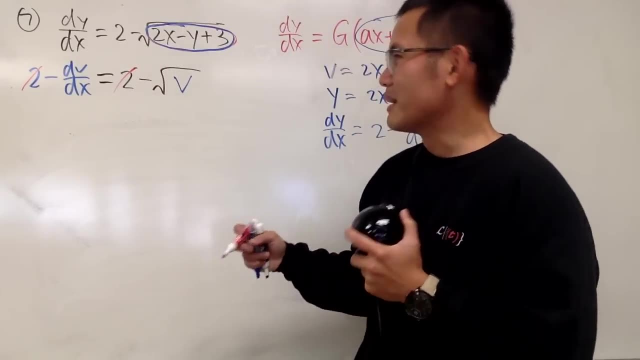 This is seriously very, very nice, Because the 2's the 2's cancel out. Imagine if you have something crazy in the front. maybe it's not so nice anymore, right, But maybe it's still doable. 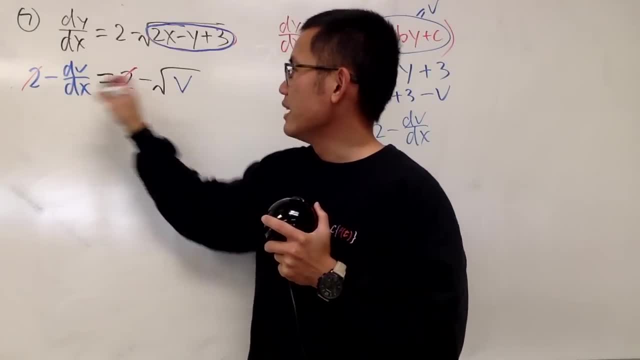 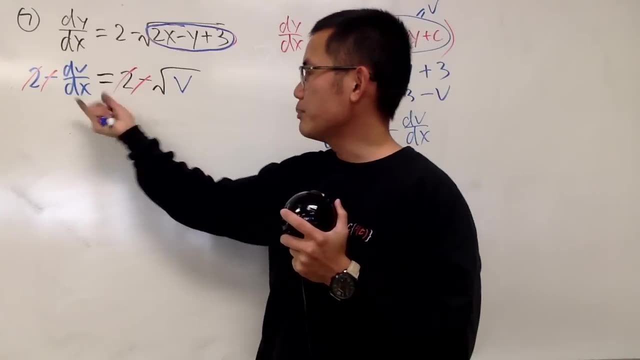 we don't know, unless we try, Anyway, and we'll be left with the negative. negative, of course they can cancel. And guess what? This is a separable differential equation. Very easy stuff, Because we can bring this to the other side. 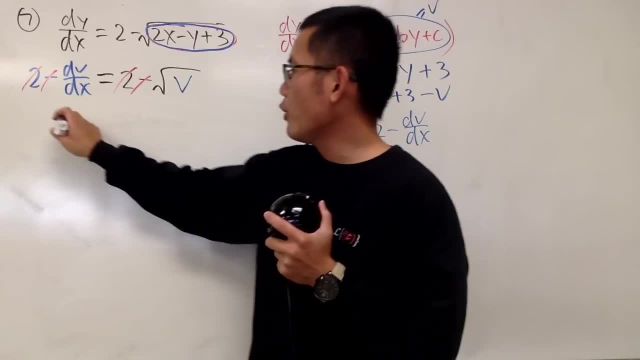 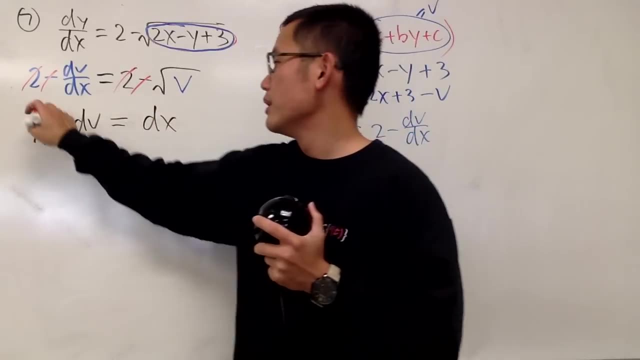 bring the dx to the other side. So here we have 1 over square root of v is with dv and that's equal to dx. Separable, Integrate, integrate. do this in your head: Integrating that. 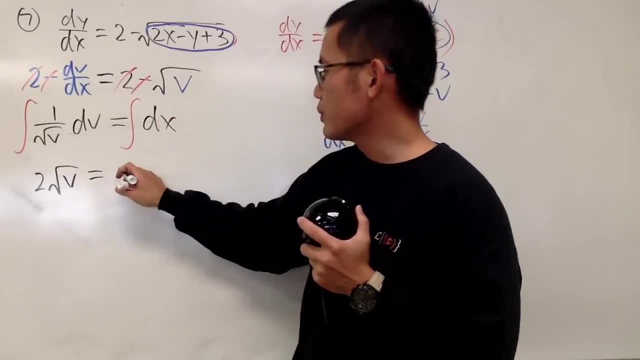 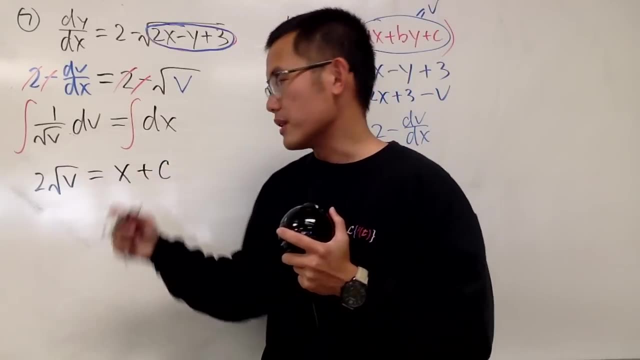 we get 2, square root of v, and that's equal to do this, which is actually what This is like: integrating 1.. In the x world, we get x, Don't forget the plus c, And now let's go ahead and solve for the v. 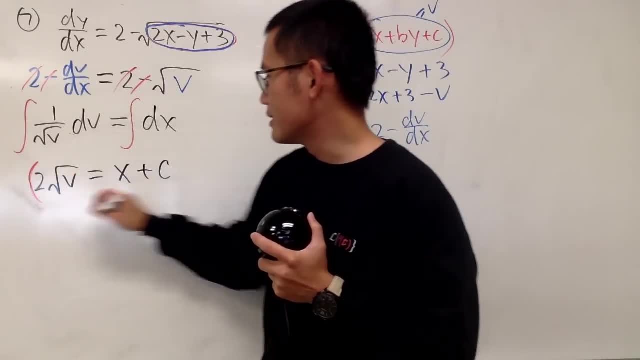 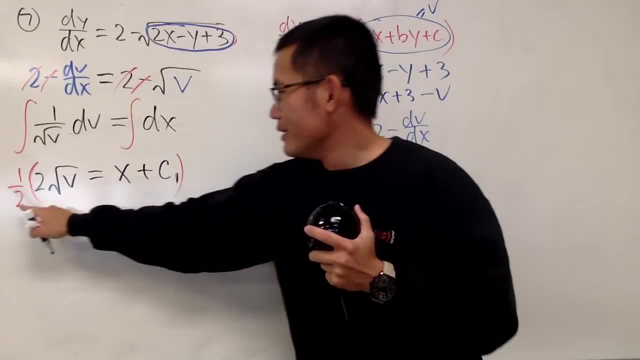 So divide everybody by 2. And I will show you guys the work, because this is going to be slightly funny. Here is the deal. Technically, I'll write this down as c1.. And here we go, This times that. 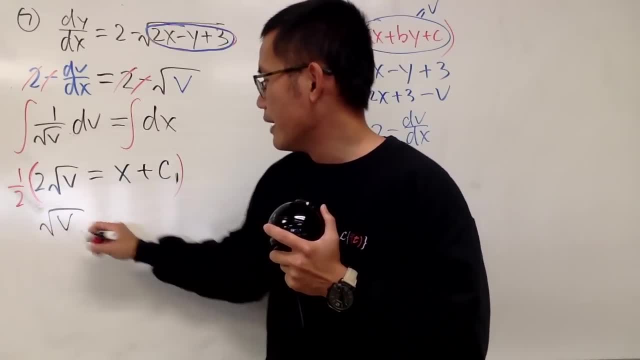 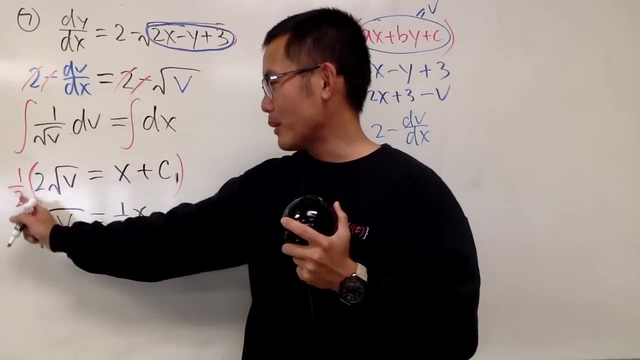 which is just square root of v and 1 half times x, I will still have the radius 1 half x And c1 is a constant. Multiply by 1 half, it's still a constant. So let's call that to be another constant. 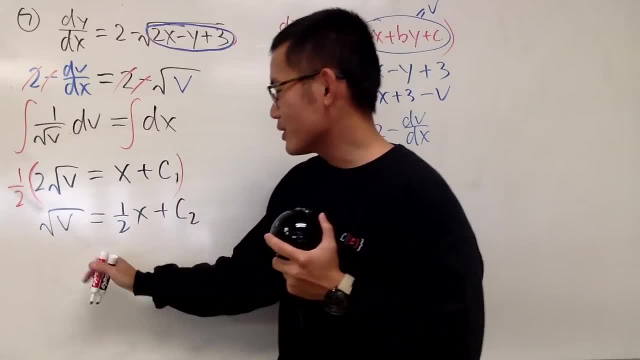 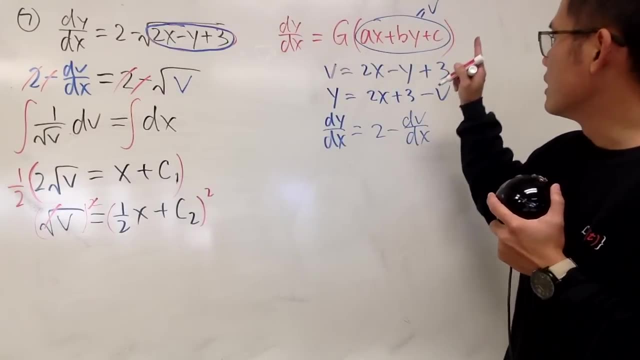 and be c2.. Very nice, Right, And of course we can just go ahead and solve for the usual thing: square both sides and all the good stuff, And in the meantime though, v is um that, so I will put that back. 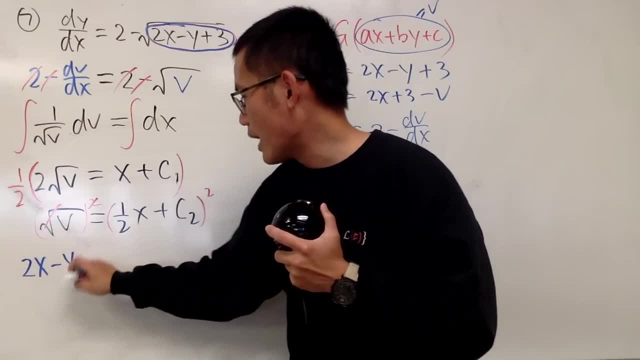 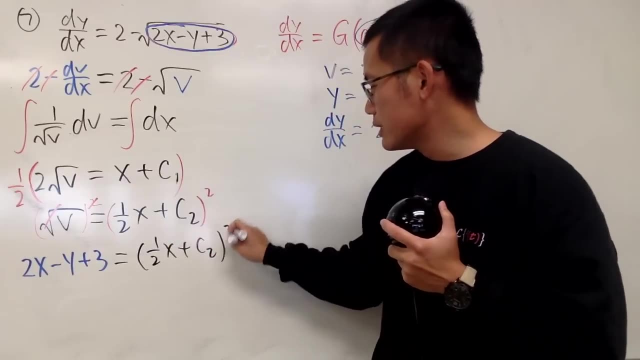 which is the 2, x minus y plus 3, and that's equal to the this side, which is, parentheses, 1 half x plus c2, squared like this: Finally, we just have to isolate the y. 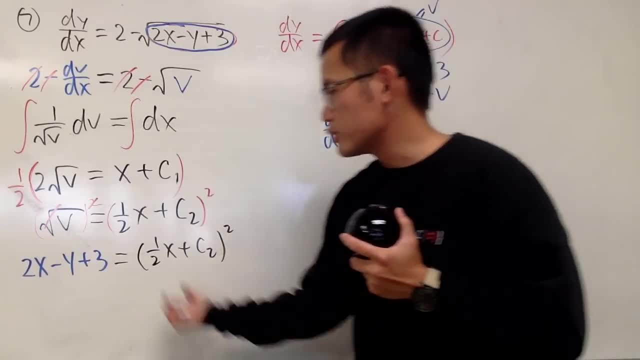 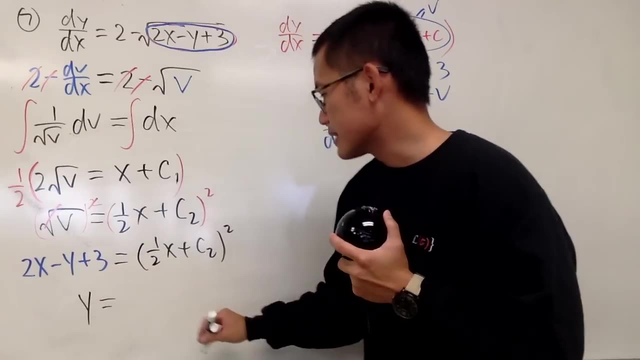 I'll bring the y to the other side so it becomes positive. I'll bring this to the other side so it becomes negative, And then, um, I will write down the y first, though, So it becomes y equals this: 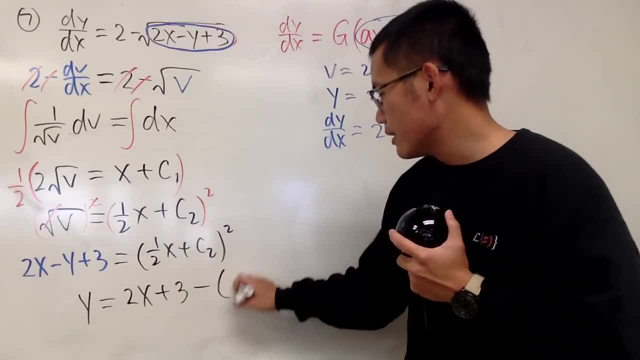 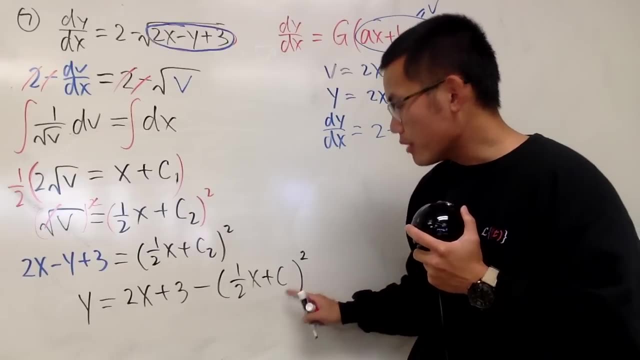 this and minus that. yeah, So we have 2x plus 3, minus this guy, 1 half x plus c2, squared. But the reason that I'm not putting down the 2 right here is because 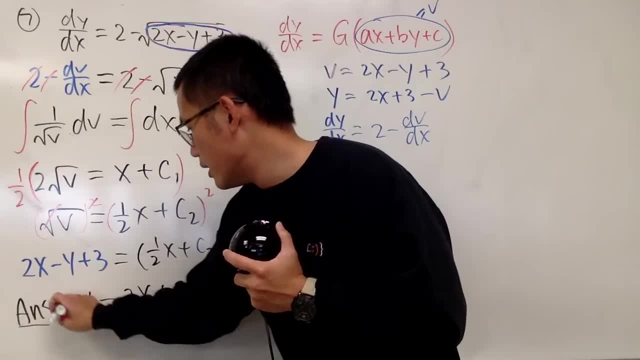 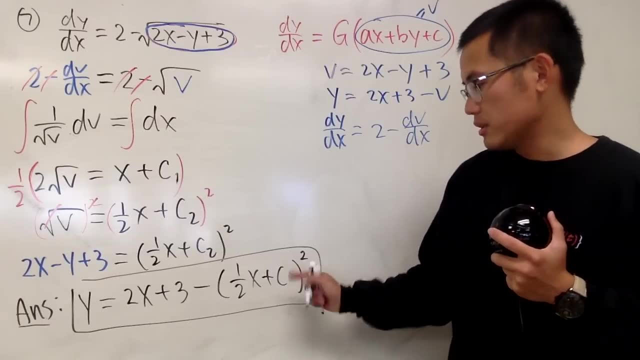 this is the answer. So, finally, I will just use the c for the final answer. That's it. You don't have to write down the subscript anymore, because this is the answer that we're presenting. So that's it. 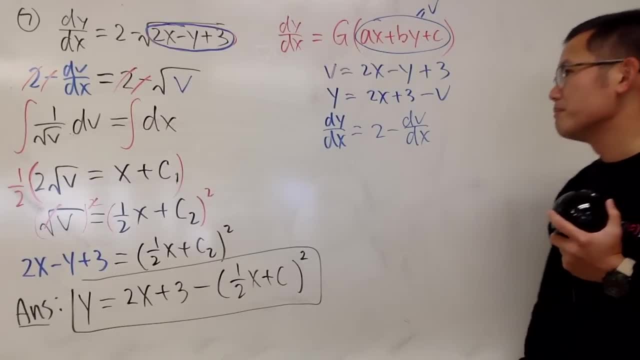 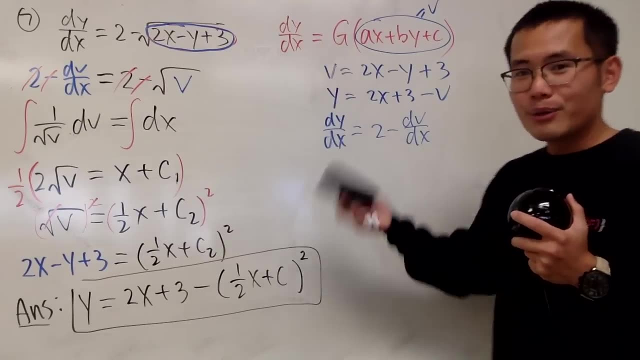 Not so bad. And again, substitution is the key. um, when we cannot really approach the differential equation with another method, Just hope for the best with substitution. Maybe there's another way. I don't know, but let me know, Okay. 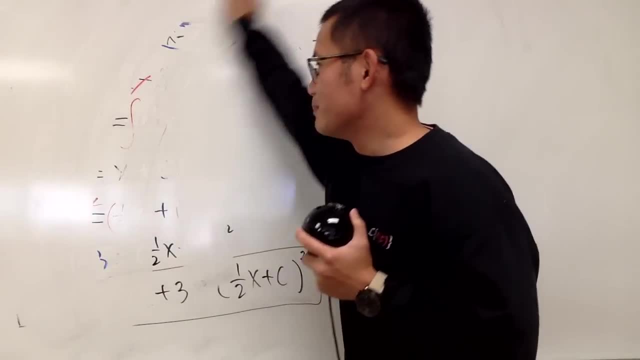 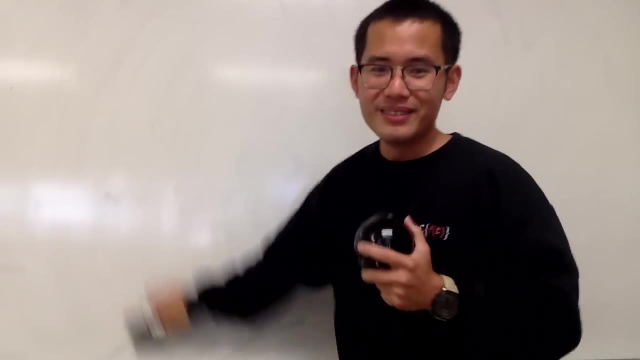 So that's pretty good. I think the most evil one is the almost differential equations. of course, right, But I don't know. You guys can let me know. That was number 7, and here we go, we have number 8.. 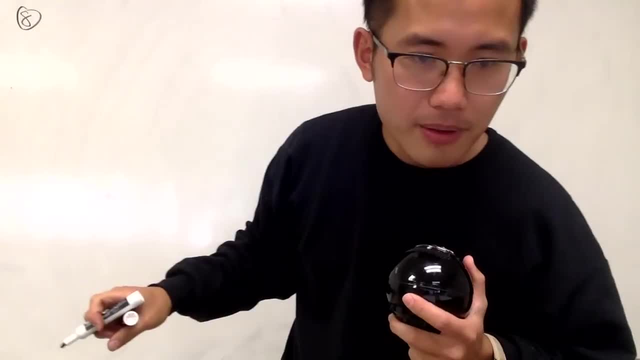 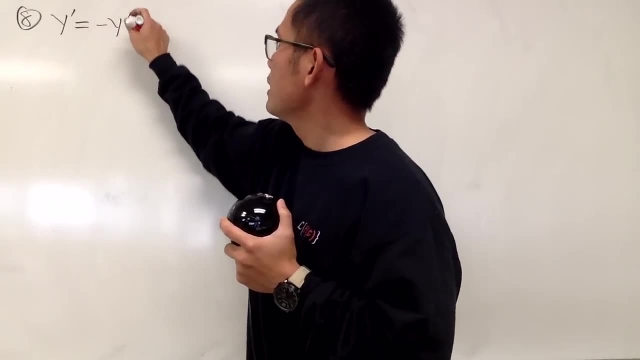 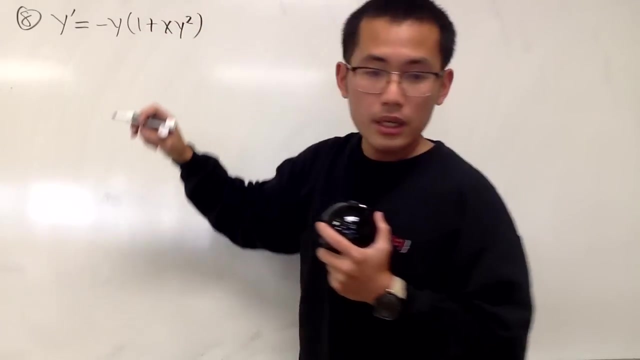 Right here. This is: y prime equals y prime is of course the same as dy dx and this is negative y, 1 minus um, 1 plus x y square, and we have an initial condition which is y of 0 equals 1 half. 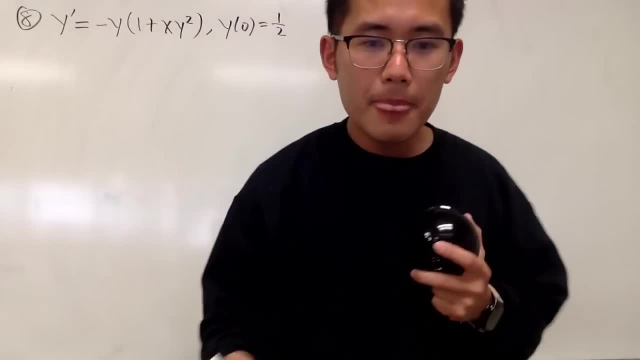 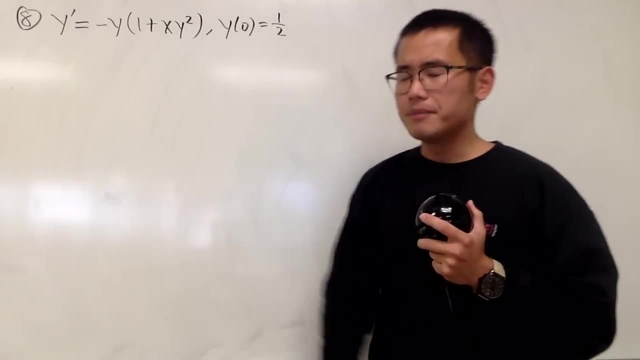 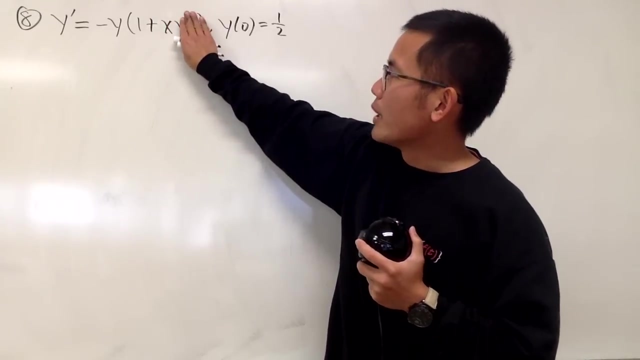 Okay, So you guys can see: All right, Not linear, because we have the y square and then multiply by y. Not linear, Not separable. If I don't have the x, that's separable If I don't have the y square. 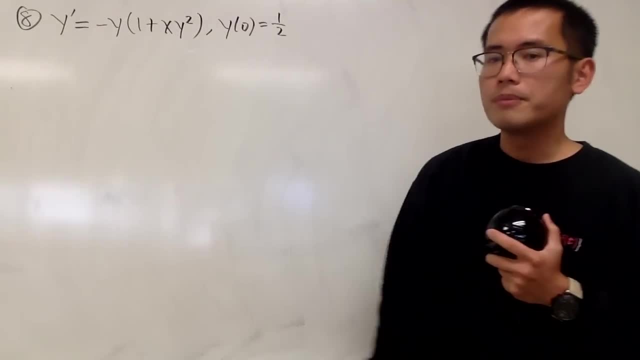 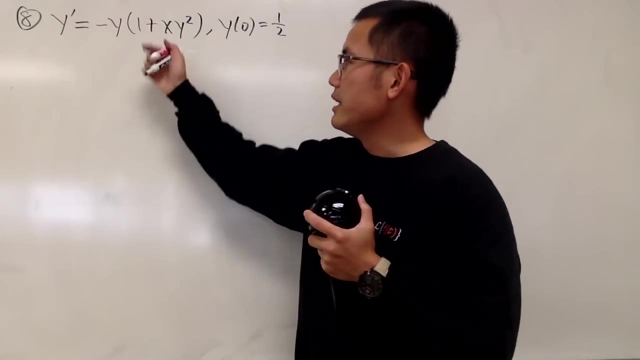 this right here is also separable, But with this not separable. You can try if it's um exact or not, but I don't think so. But if you multiply this in, you will see that. 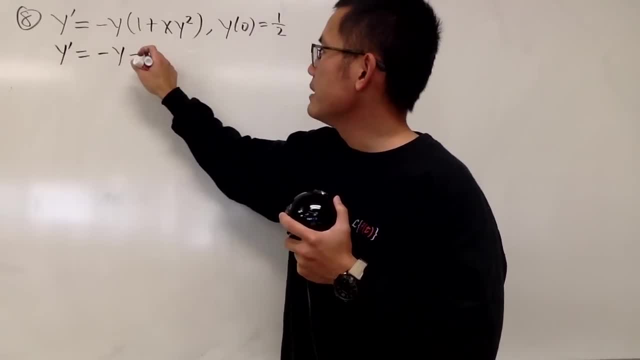 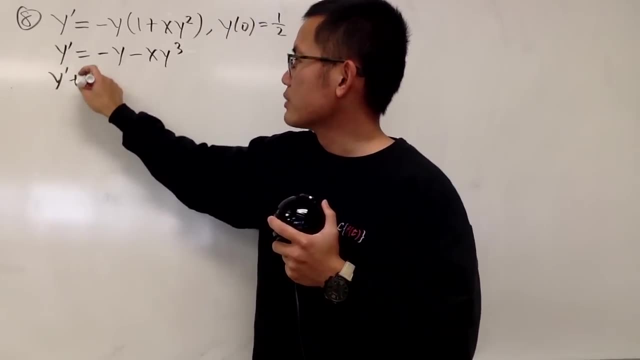 we get: y prime is equal to negative. y minus x. y to the third power: Yeah, If you bring the y to the other side, this is y prime plus y, which looks really similar to a linear differential equation. But 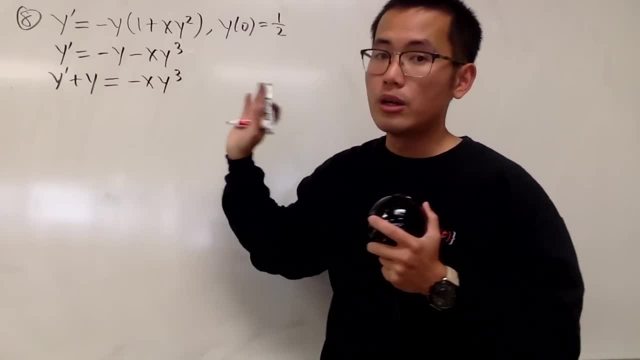 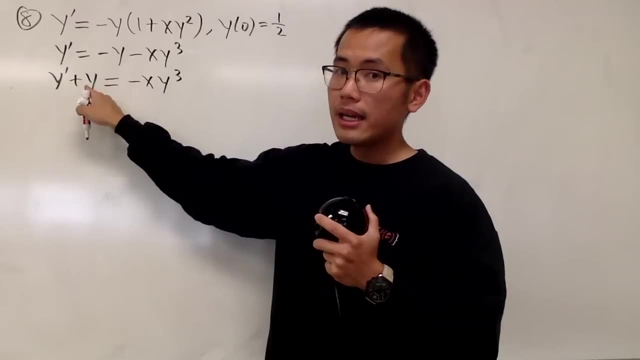 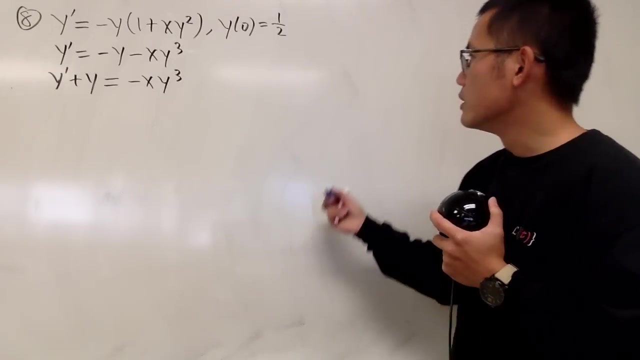 the right hand side, we have negative x, y to the third power. Here's the deal. You see, right here we have the y and right here we have a function times y to the power. This is what we call Bernoulli's differential equation. 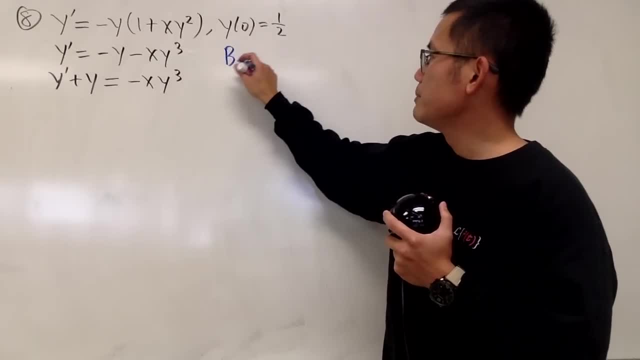 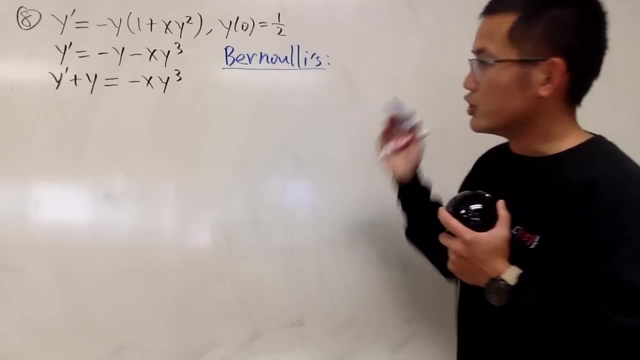 So let me just write it down right here. So I just put this down. If I spell Bernoulli wrong then I'm very sorry. Bernoulli's The general form. it's very similar to the linear differential equation. 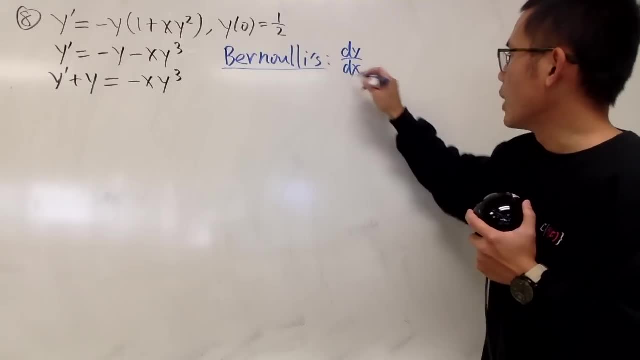 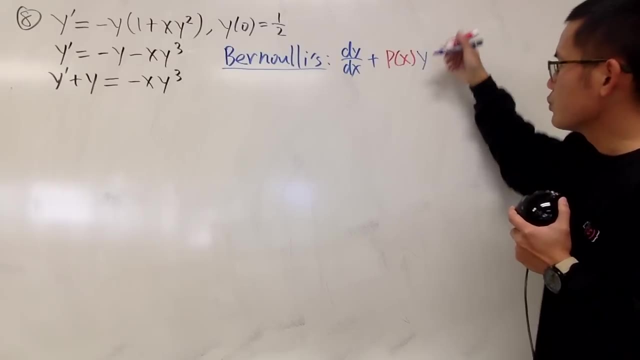 which I will just write it as dy dx, which is the same as y prime plus some function and again very similar to the linear differential equation. so I'll just use p of x And this is equal to q of x. 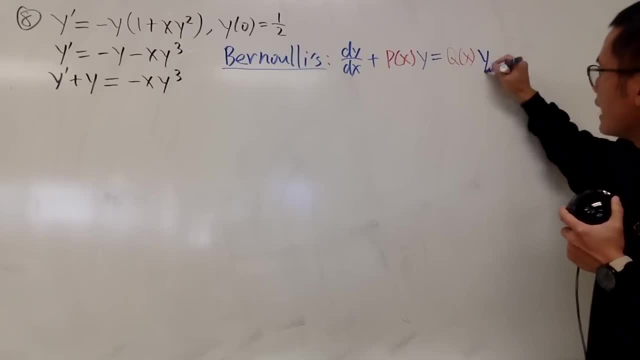 It can be whatever function, hopefully nice enough times. y to some power, r Okay, And the reason I'm using r is r can be any real number, It doesn't have to be a whole number, it doesn't have to be positive. 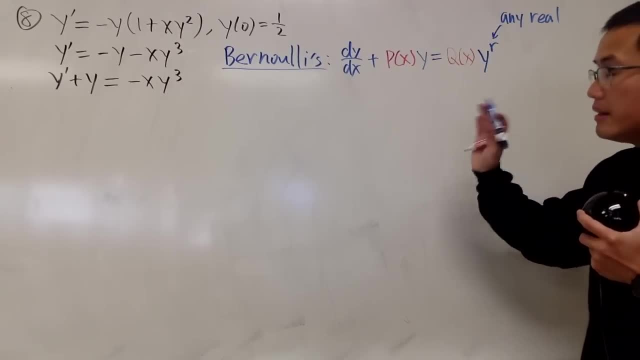 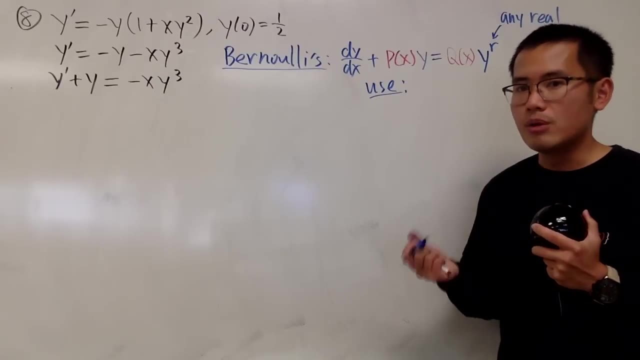 it doesn't have to be negative whatsoever. In this situation, what we are going to do is we are going to use a substitution, and this is not so obvious. you just really have to remember it and have to know it. 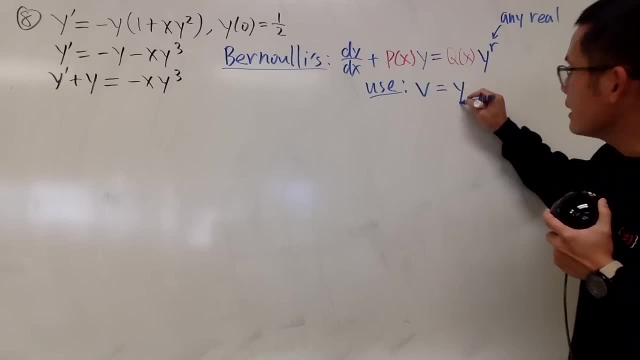 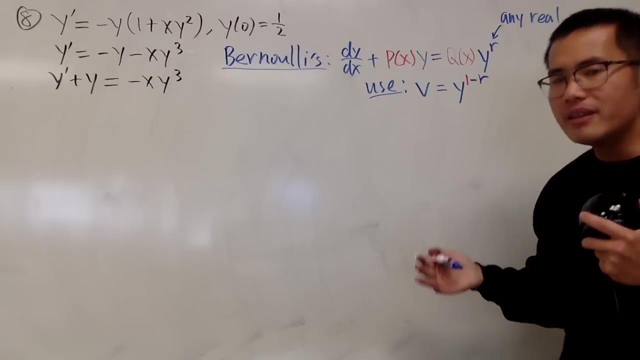 The substitution is that take v to be y, raised to the 1, minus r's power, like this. And you might be wondering: how is this going to work? How do I know that? Well, first of all, you have to study this to know that. 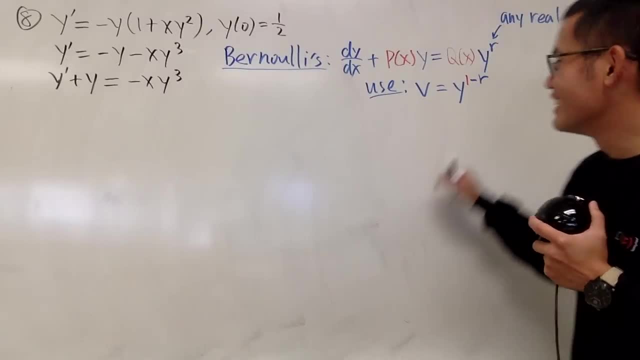 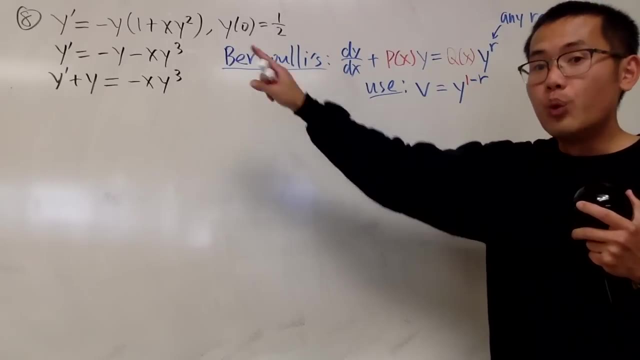 And, of course, I will tell you guys why the 1 minus. it's actually very genius. I will tell you guys, though that's not linear yet. It will be linear after this substitution. Okay, So in our situation here, 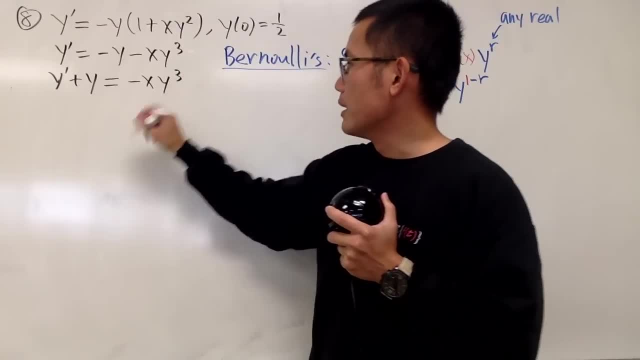 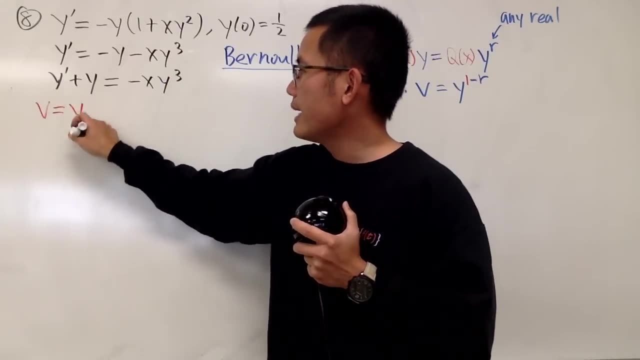 of course, I will just write this down right here just to make it nice for you guys. We have v which is equal to: this is my r, so I will actually do y raised to the 1, minus. 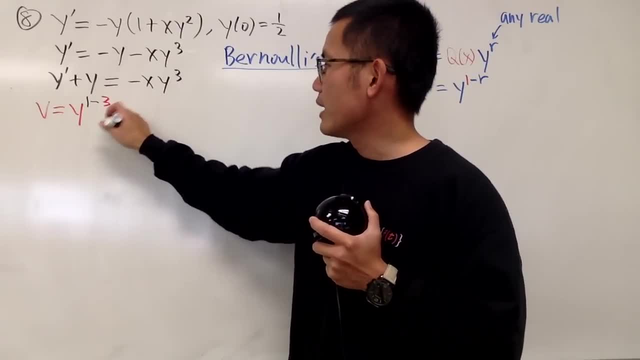 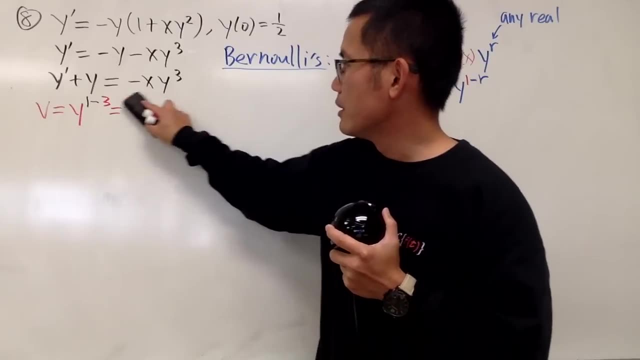 third power like this, And of course you can just work out this is just going to be y to the negative 2.. Well, when we have, v is equal to y to the negative 2.. Actually, let me just write it down like this: 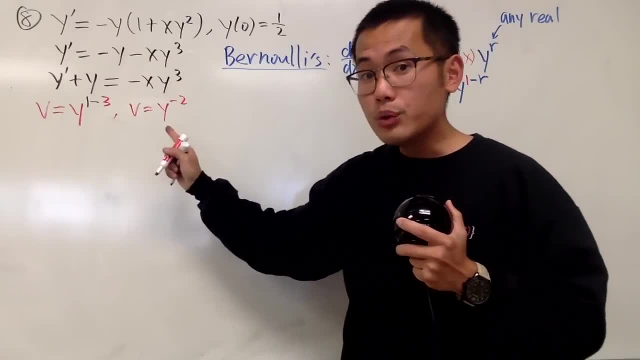 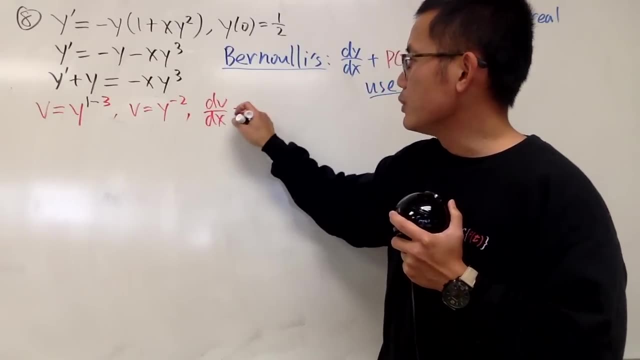 v is equal to y, to the negative 2.. What I will do is I will just look at this and differentiate already, So you will see that the v- dx is equal to. of course, bring the power to the front. 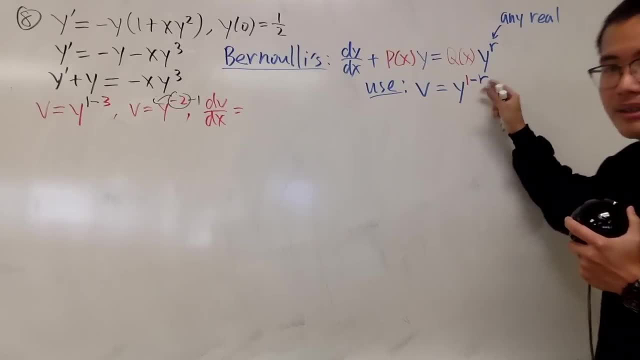 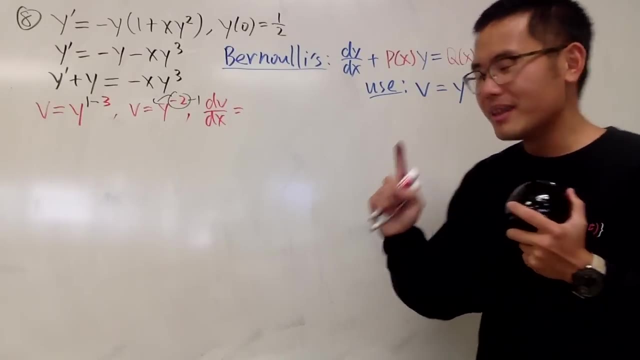 minus 1.. And you see, this is the reason why the 1 minus It's very cool. It's very, very cool. You see why it actually works out so nicely. That's why you have to use the 1.. 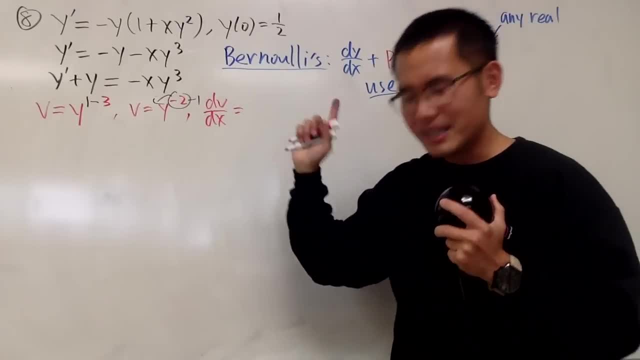 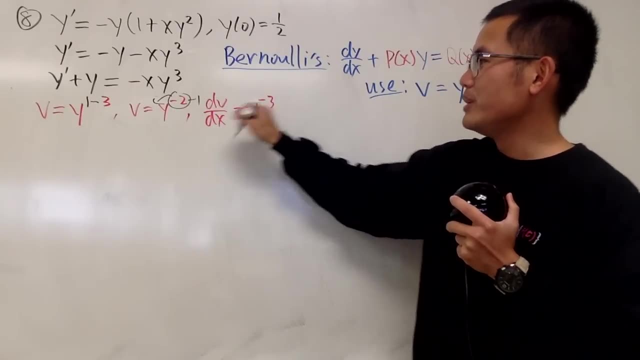 That's 1 minus r, But you'll see, I know the word is wrong, but it works out really well. Anyway, enough talking, enough excitement. This right here is y to the negative 3.. And don't forget. 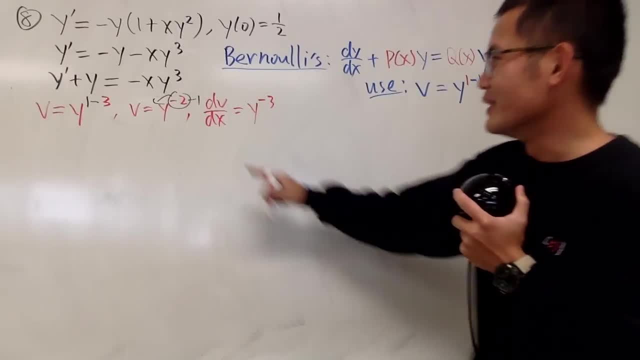 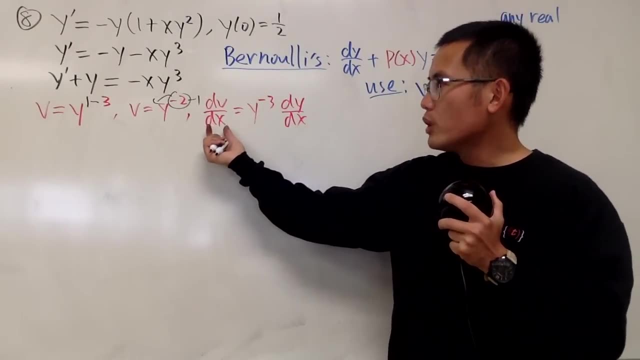 use the chain loop Man, first time in this video seeing the chain loop. Don't forget to multiply by dy dx. Alright, So here's the deal. In order to produce dv dx, we have to have: 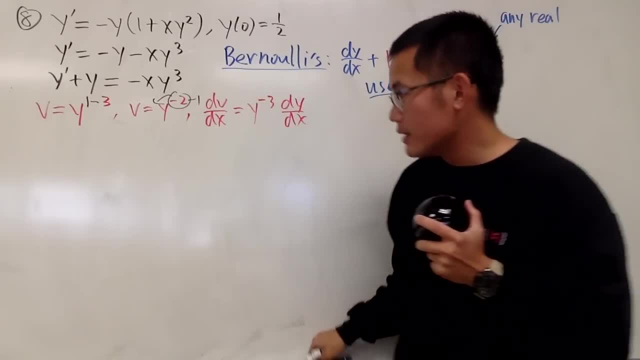 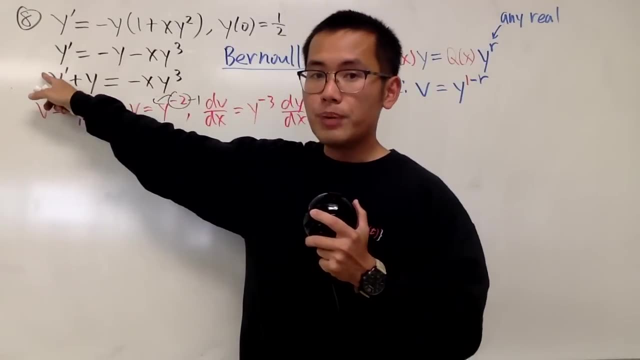 y to the negative 3, right, So this is what we'll do. If you look at this equation, I do not have y to the negative 3 power in front. I want to have that, So let me multiply everybody by. 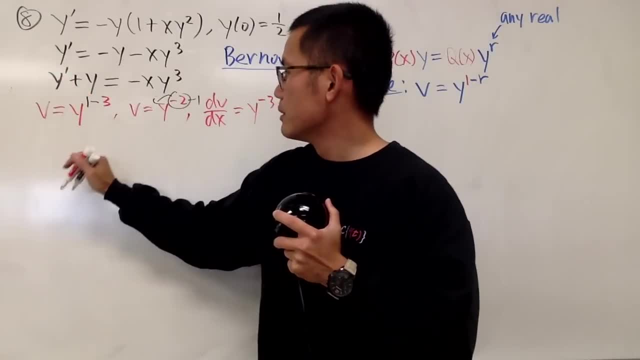 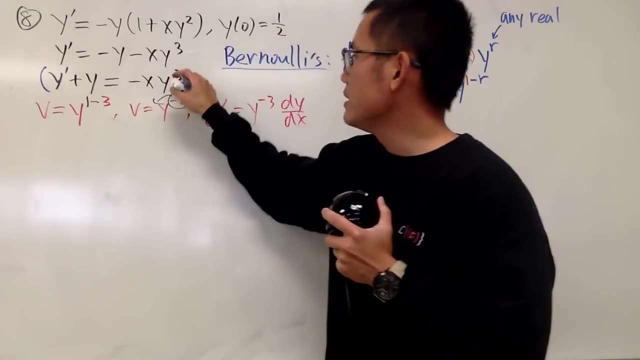 y to the negative 3.. So I will actually just- let's just do that right here. Let me multiply everybody by y to the negative 3.. Right here, And you'll see when I do this. 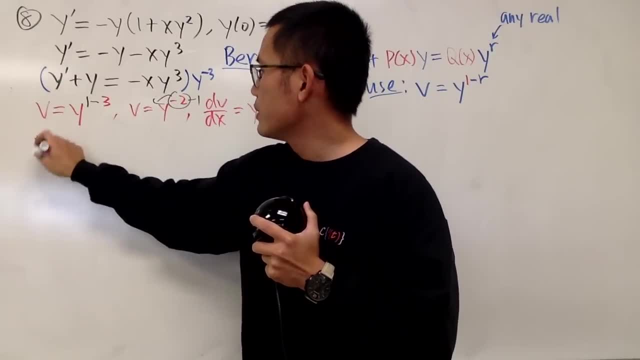 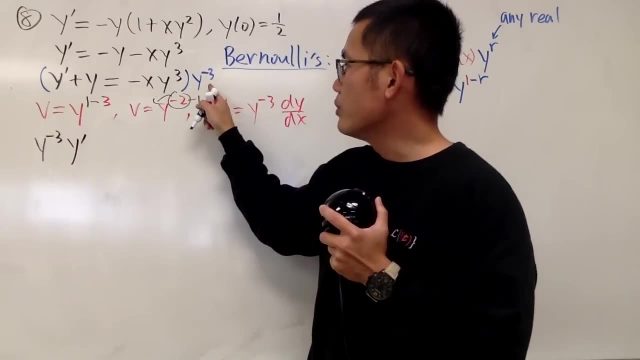 times 3, times that I will end up with y to the negative 3, and then we have the y prime, which is just exactly our dv dx, And then just continue. this times. that is plus y. 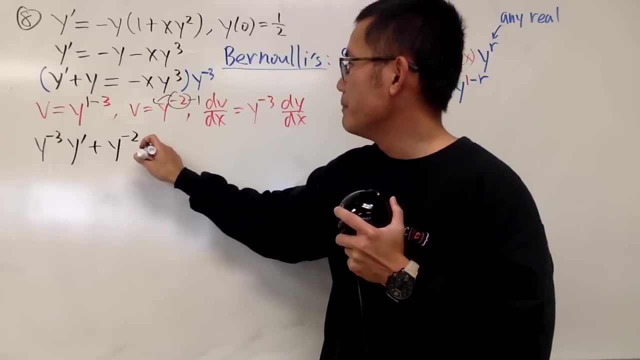 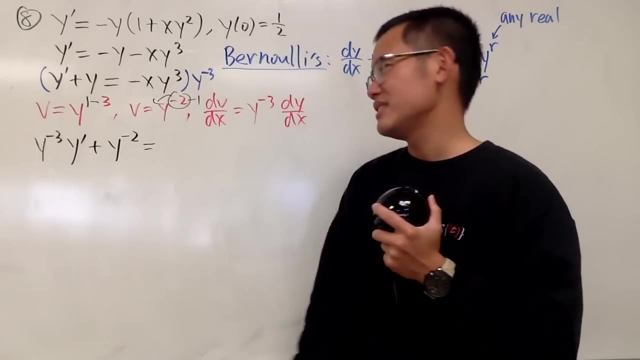 to the negative 2.. And then equals this and that The y's cancel out. Very cool, huh. You see This and that the y's just cancel out. so, so, so nicely. This is like a prediction. 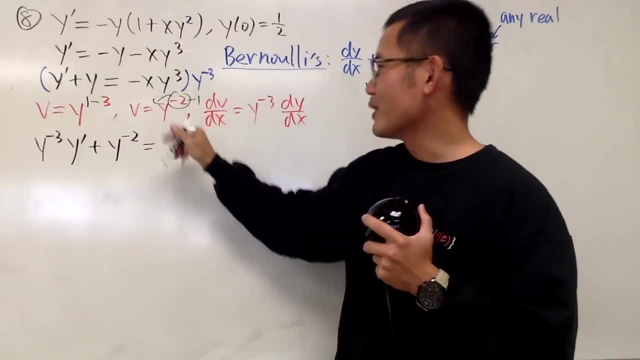 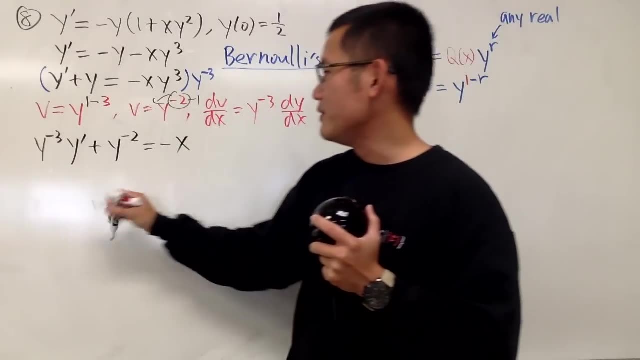 When you do always cancel out, guaranteed it, They cancel out and you have the minus x right here. Now, here's the best part. This is precisely our dv dx, So let's just go ahead and write that down. 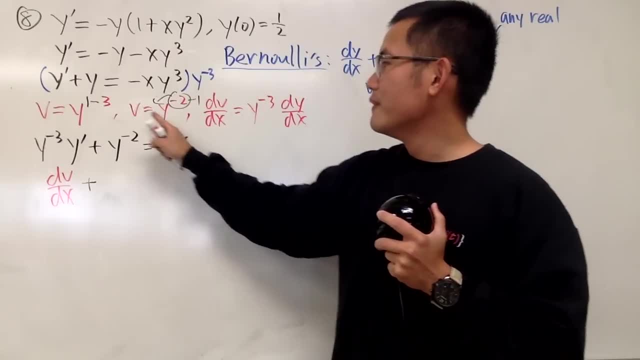 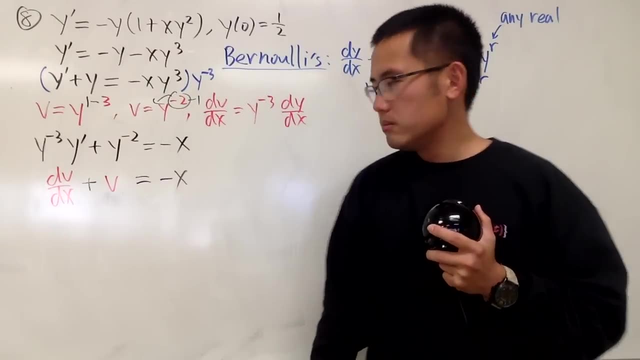 Plus, this is precisely our v, And this is just negative dx. So that's what I have. But yes, this is linear. That means we have to use the integrating factor, But it's not so bad. 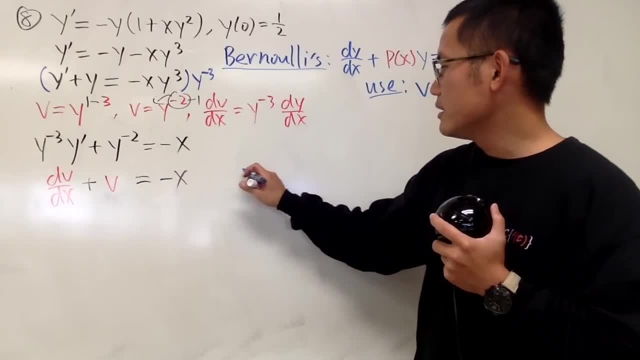 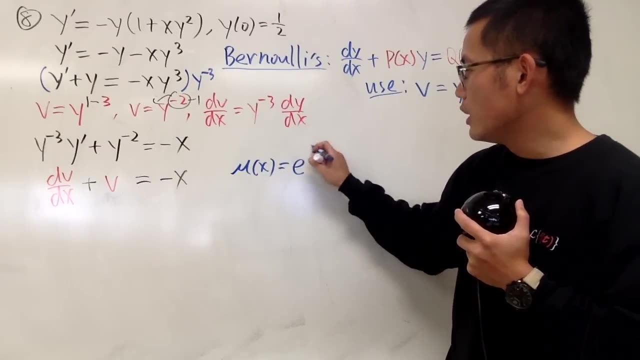 This is not a crazy integrating factor situation, right? So here we go. Here is the linear equation. So the integrating factor is mu of x, which is e integral, and we just have a one right here. 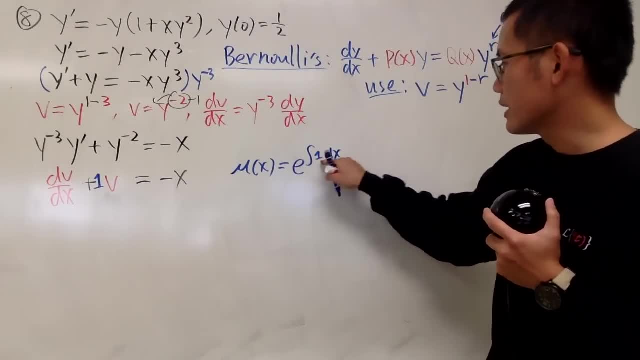 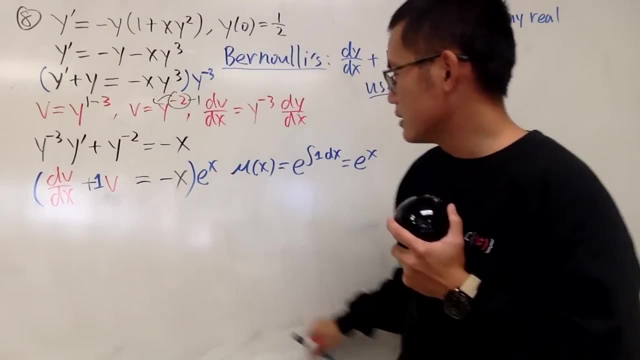 I believe, Yeah, So integrating one in the x world, so that's just e to the x. Just like this. Very cool, huh? That means multiply everybody by e to the x. Of course. let's go ahead and do the work. 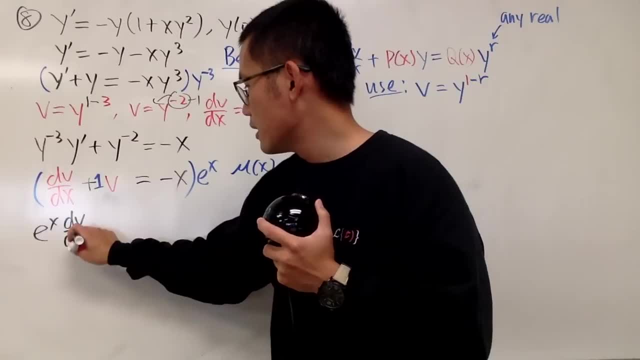 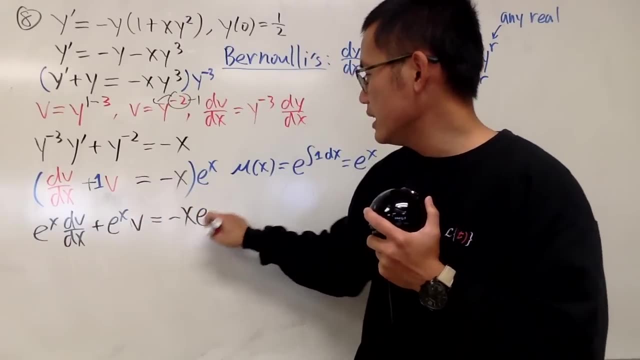 Here we have e to the x, dv, dx, plus this times that which is e to the x, d, and that's equal to negative x. e to the x, Like that, Yes, the left hand side. 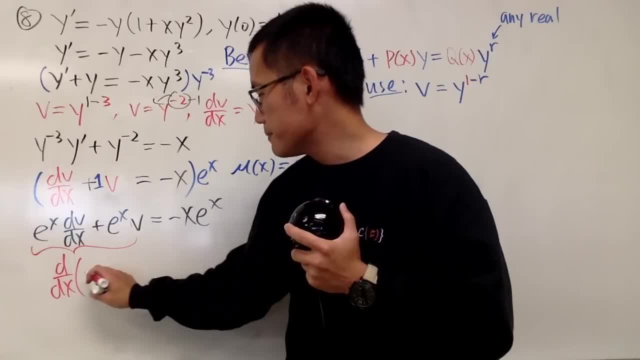 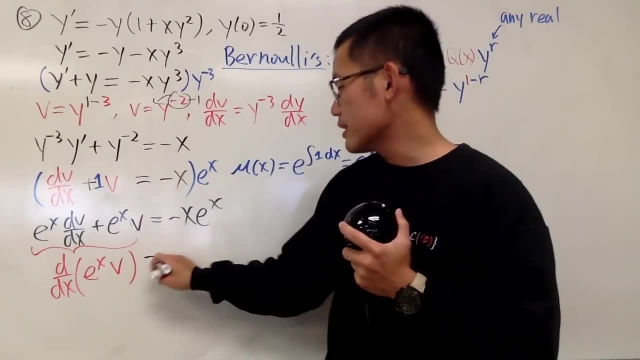 is still the derivative of a product of the linear, of an integrating factor, namely e, to the x and also v. You can of course go ahead and check out, And the right hand side is just the right hand side. 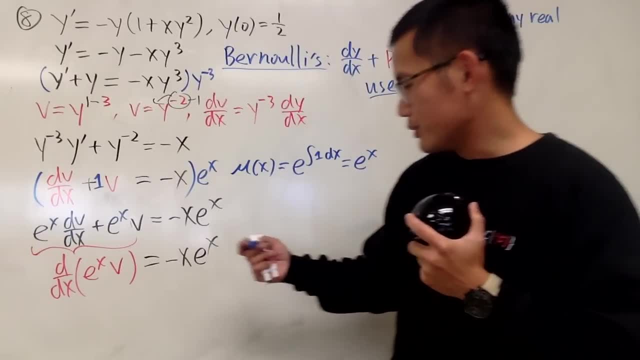 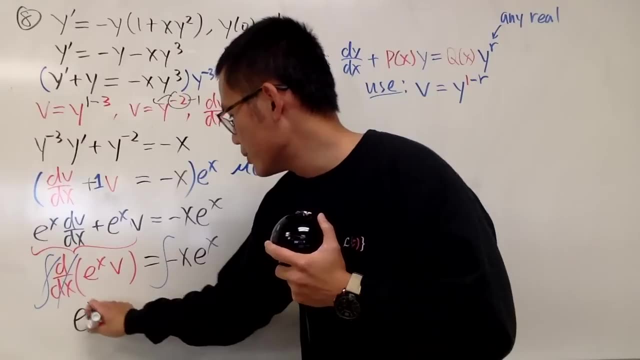 e to the negative to the positive x. Well, how do we do this? Of course, integrate both sides. they cancel. So here we have e to the x times d. that's equal to this guy. 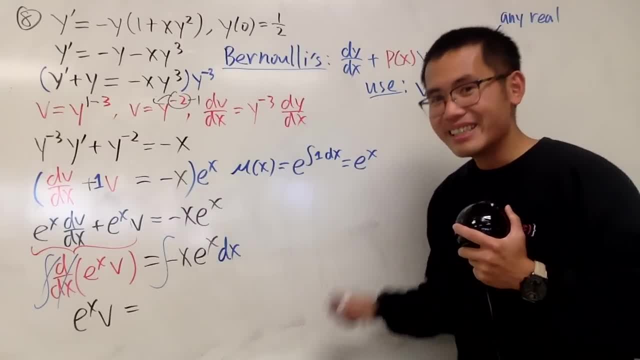 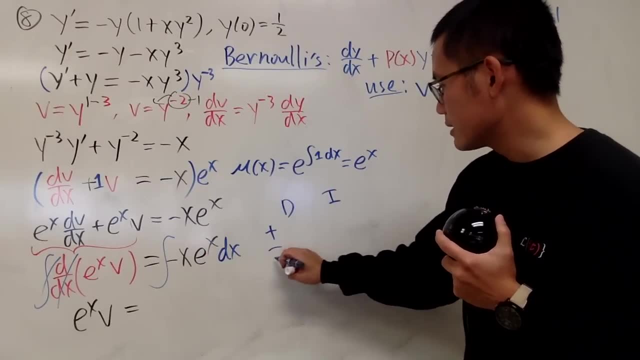 Man, we have to integrate this. How do we do it? Yes, d, i method. right, Because we are doing the integration by parts. So I'll just put down the d and also the i, right here. So 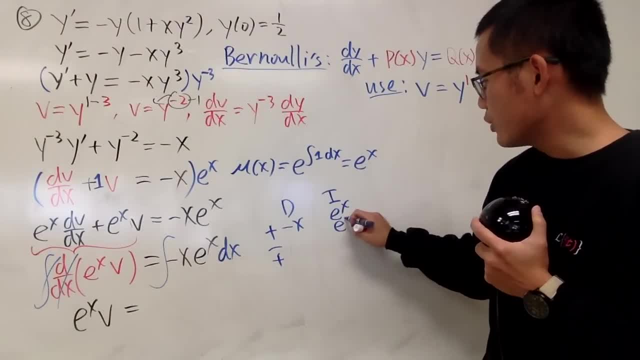 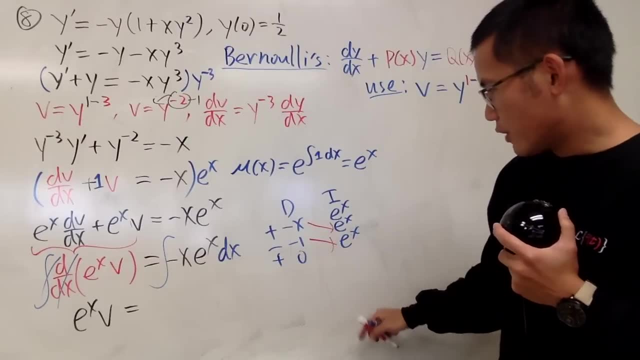 plus minus, plus Negative x. I can do that all day, all day, yeah, And this right here I can just do negative one and then zero. so done So this times this, this times that. First part of the answer. 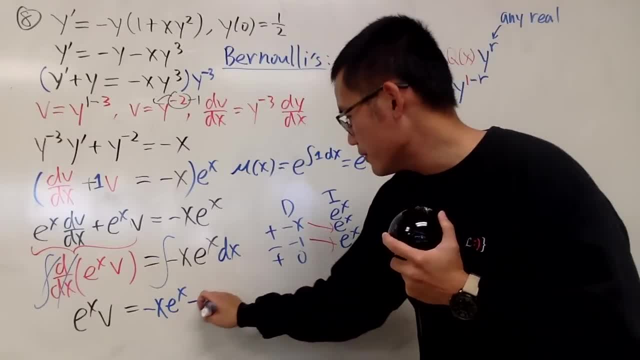 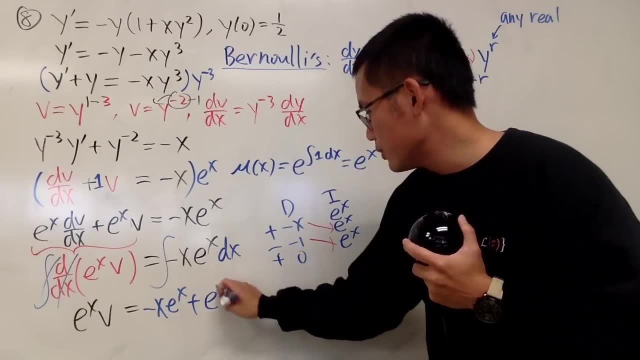 we have negative times, that which is negative, x e to the x Next, this times that is positive and again I took the negative into consideration already, right This times that and the negative so positive, and we have 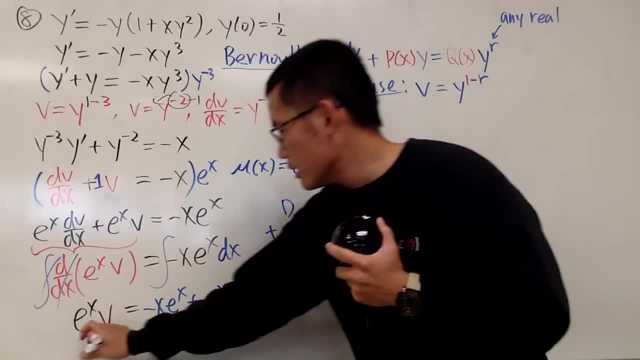 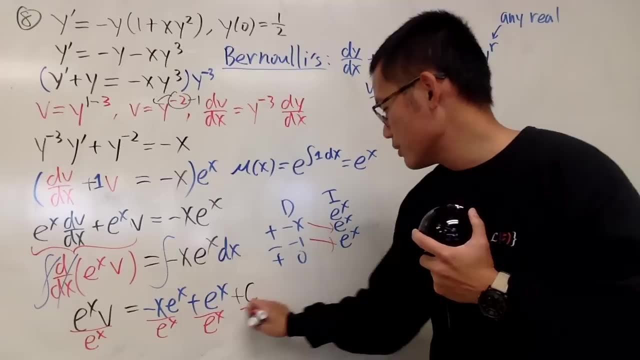 e to the x, And don't forget the and. again, if you don't have the plus, you'll see something really funny. You'll just get like negative x plus one, which is not true. Right, Define everybody by. 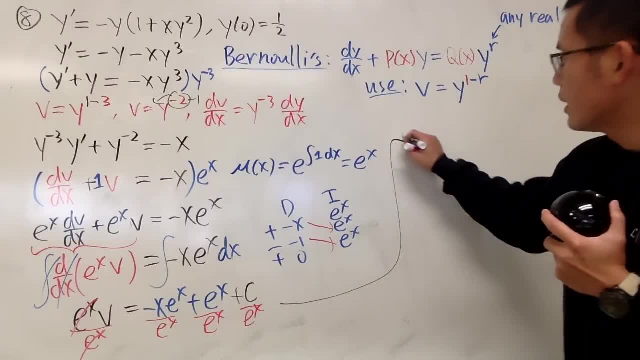 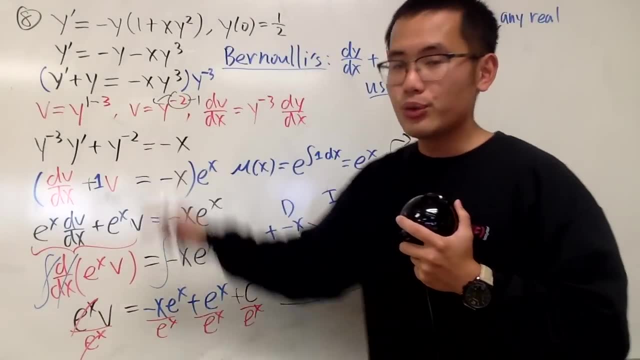 e to the x. So that's nice. Now I'll come here and we have v, which is y to the negative two. So again for the v, I'll just write it as y to the negative two. 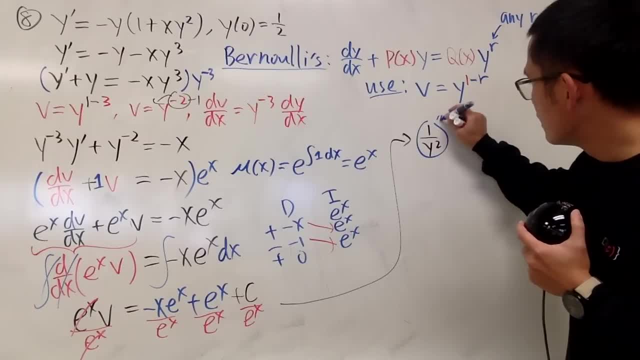 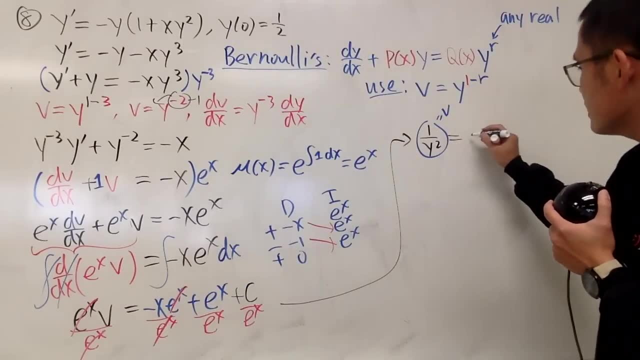 which is one over y squared. So again v, right For v, And this is equal to the right hand side. this and that cancel, so we have negative x, and then this and that cancel plus one. 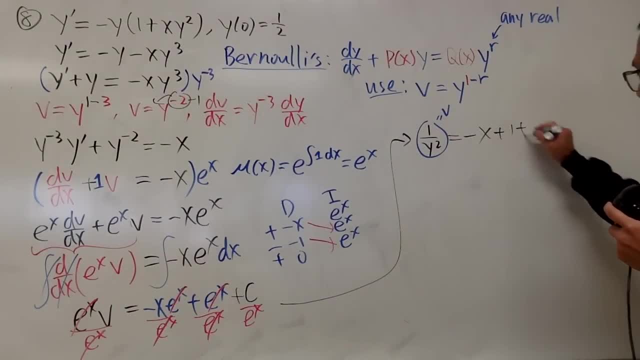 and then I will use negative exponent right here, so it's plus c e, negative x, like that. Pretty good, Now I will just go ahead and do the reciprocal and then also take the square root. 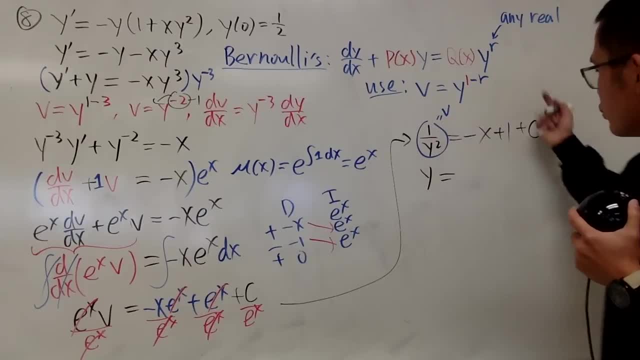 and you'll see, we'll just get y and do the reciprocal, so you have one over all this guy, which is negative x plus one plus c e negative x, But it was to the second power. 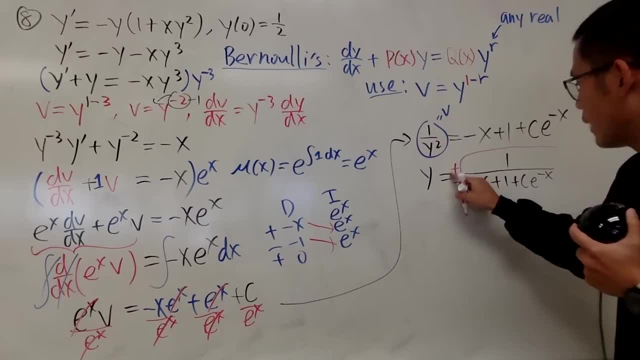 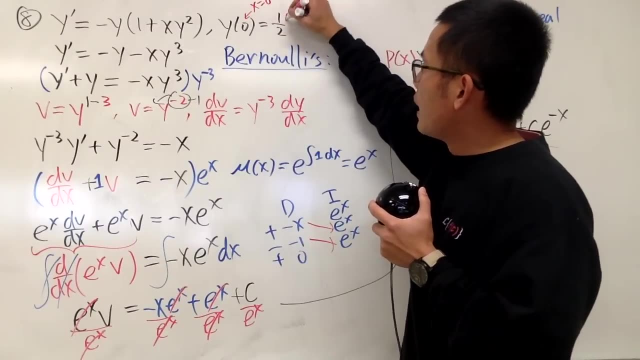 so you do the square root and technically you should keep the plus minus. so I will keep the plus minus. Now look here: x is zero, y is negative, y is positive one half. So I just put the one half. 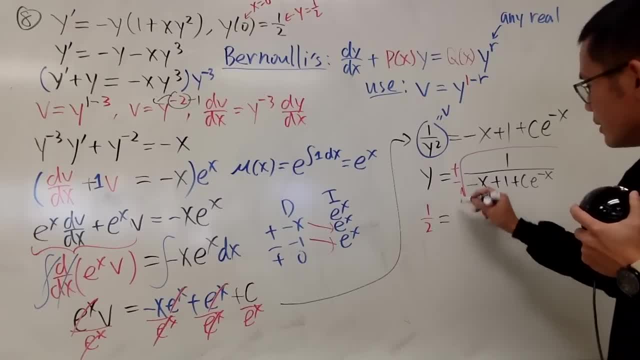 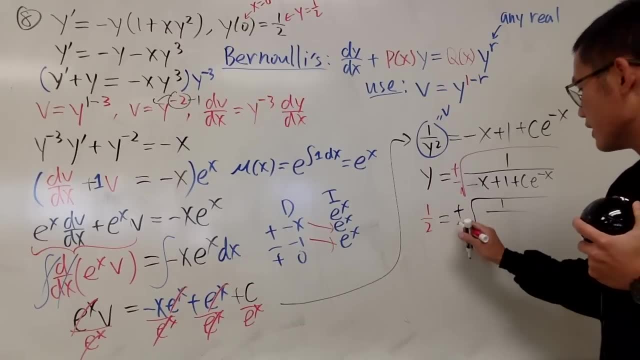 right here equals. well, which one Is it- plus or minus- of the square root? It has to be the plus because the one half is positive, so do not use the negative And again just plugging zero into all the x. 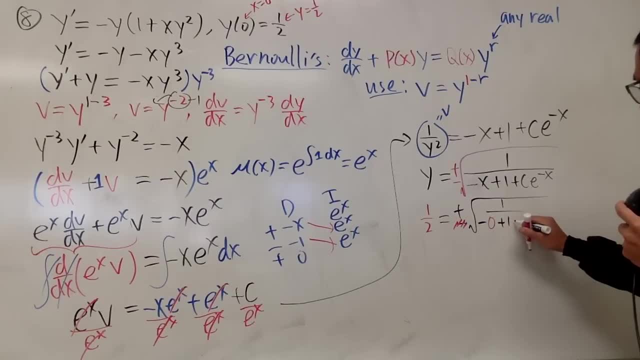 so here we have negative zero plus one, plus c, we don't know- e to the negative zero's power, which is just one. So now this right here is one half plus the square root. 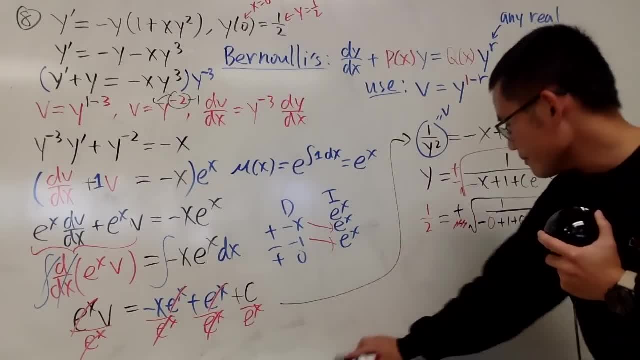 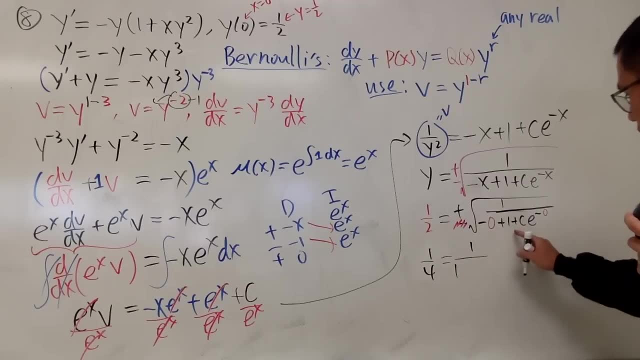 ah, I'm going to square both sides. I'm going to square both sides, so I get one over four and we have one over. this is zero, this is just one, and then this is plus ah c. 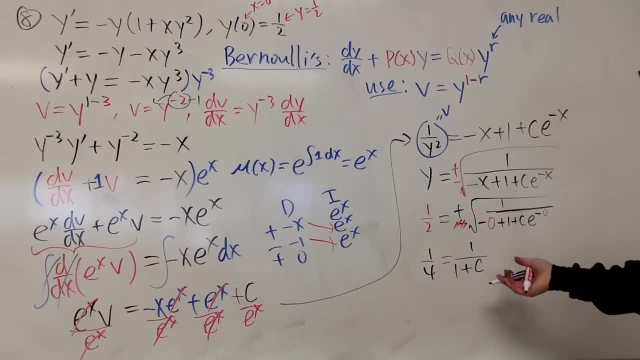 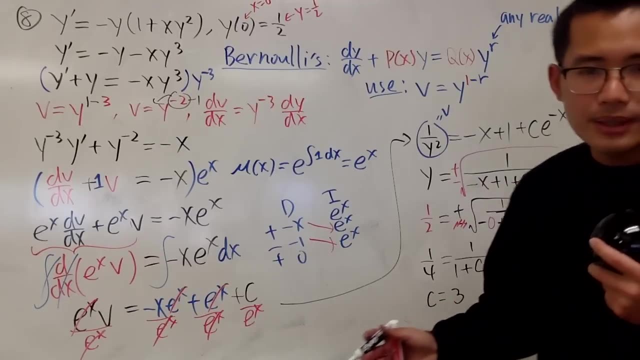 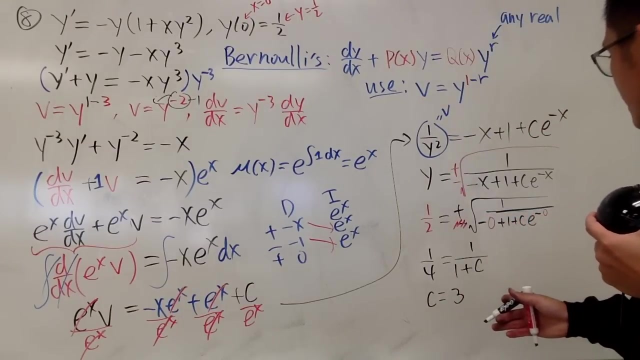 just like that, So you can see that ah c is equal to three. like this: Yeah, Am I right? Let me see. Let me see, let me see, lung ah c. I must have done. 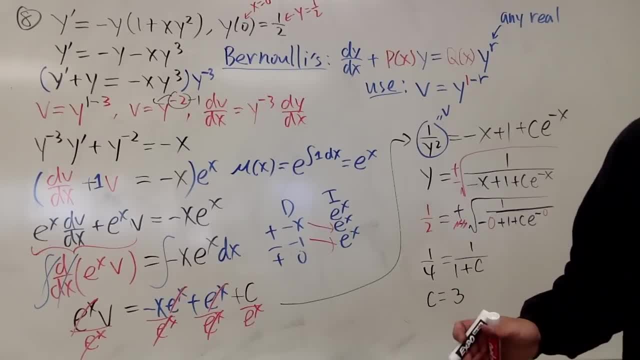 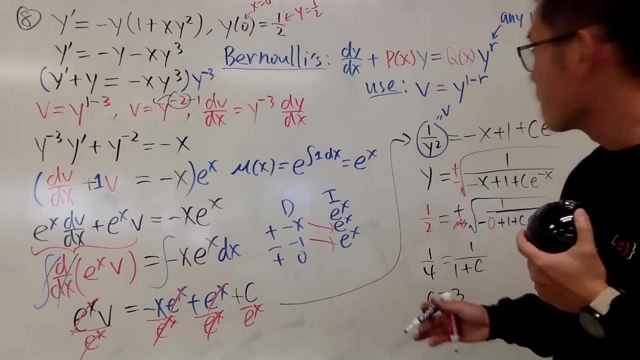 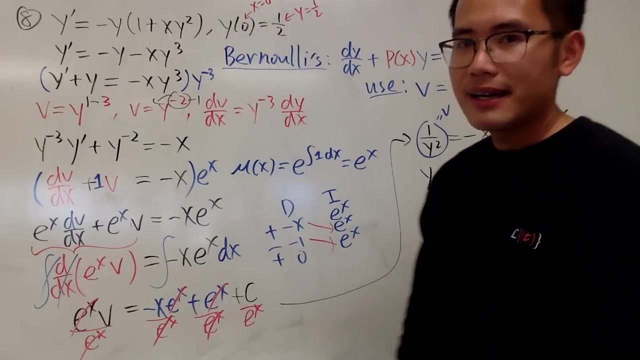 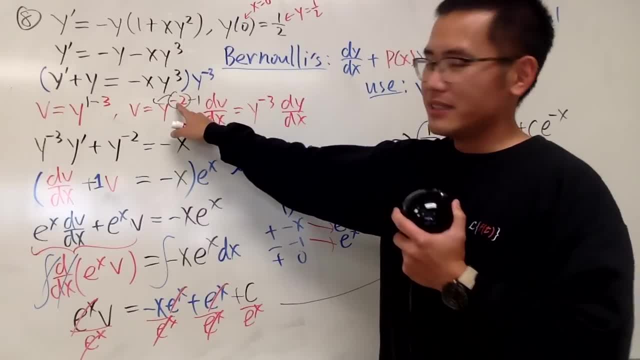 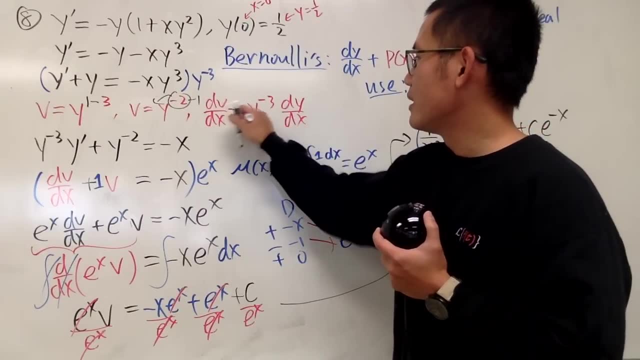 c, c, c. This right here is negative 2, bring that to the front. Man, I'm mad at myself. Negative 2, bring to the front. I should have a negative 2 right here. I should have a negative 2 right here. 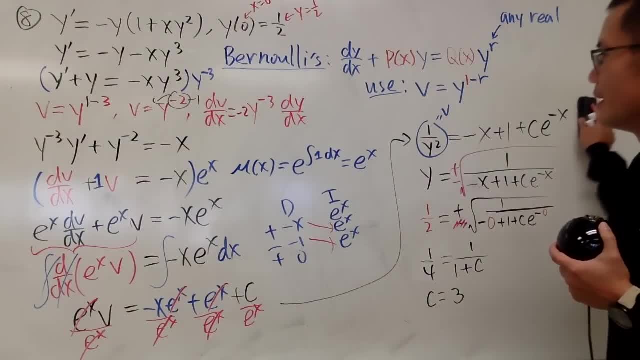 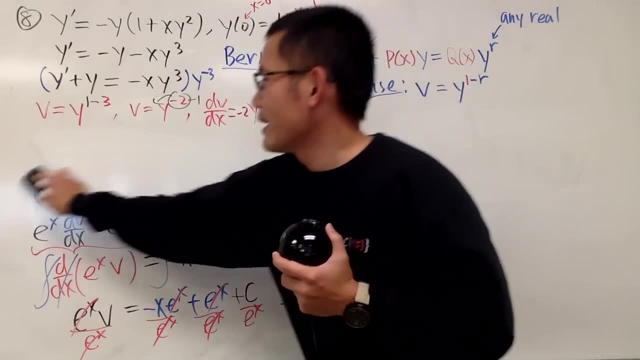 I'm sorry, I'm very, very sorry. So, man, let me just do it again. Let me just do it again, Let me just do everything again And again. I'll speed up a little bit, And I don't know if I should cut it, but 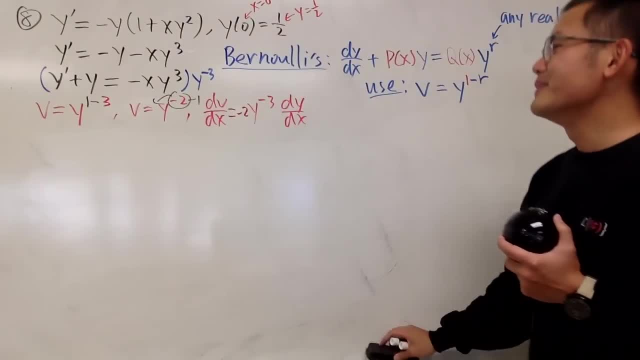 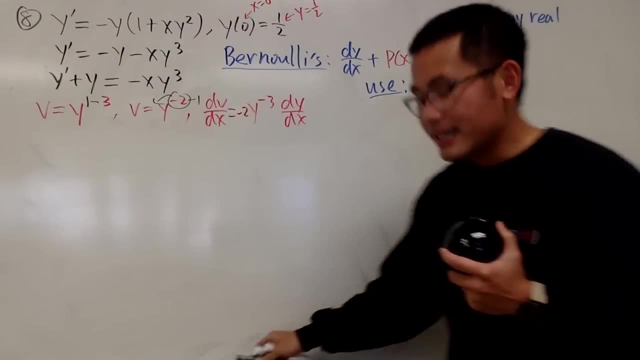 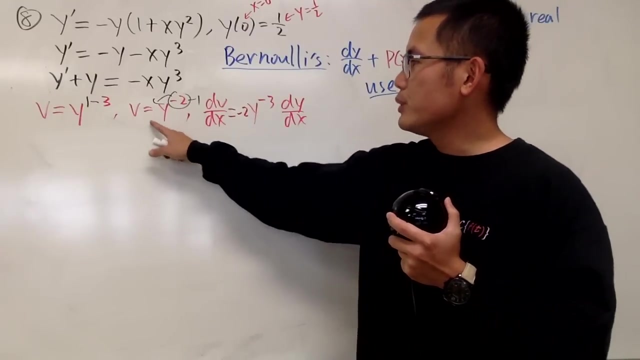 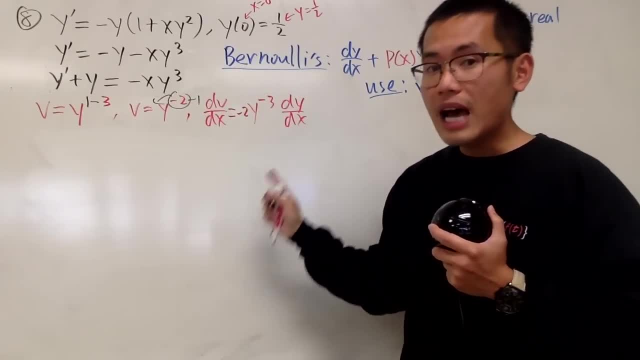 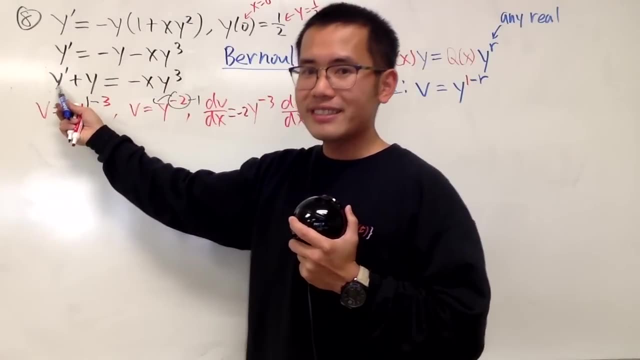 and then minus 1, so I'll have this and it's equal to dv dx. So now what we can do is look back to the equation and you see, this is just the dy dx. I need to have this so that I can. 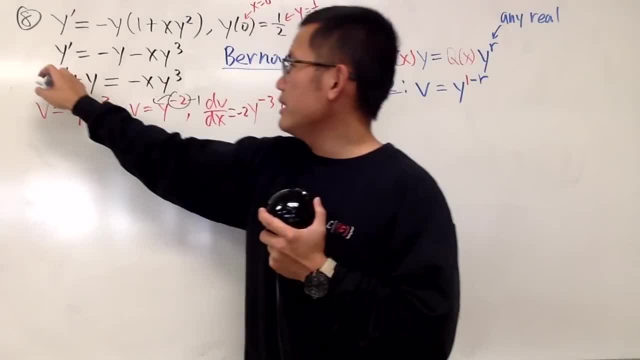 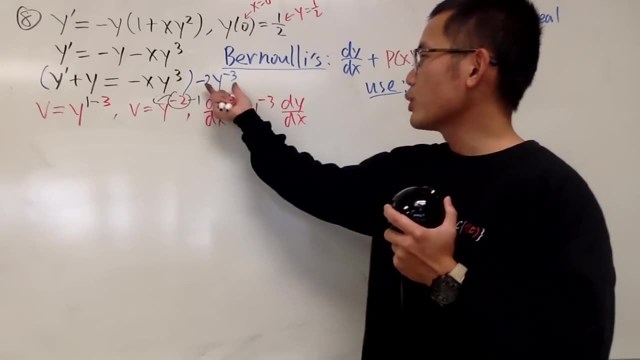 I can produce dv, dx, yeah. So let me look at this equation and multiply everybody by negative 2y to the negative 3.. This is gonna be so nice, because when you multiply this and that, you will see you get negative 2y to the negative 3,. 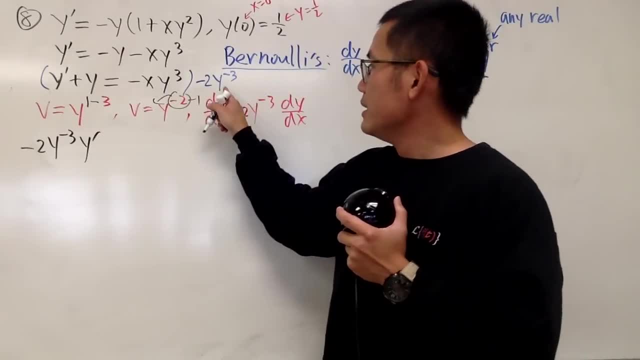 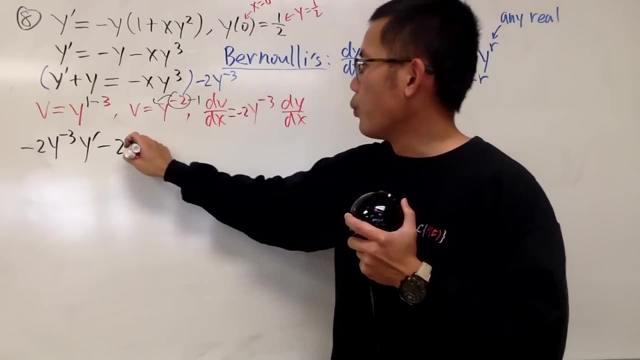 and then that's of course, just our dy dx. And then you see, this times that of course now becomes negative 2, and then we have the y to the negative 2 power. That's good And this, and that you check this out, check this out. 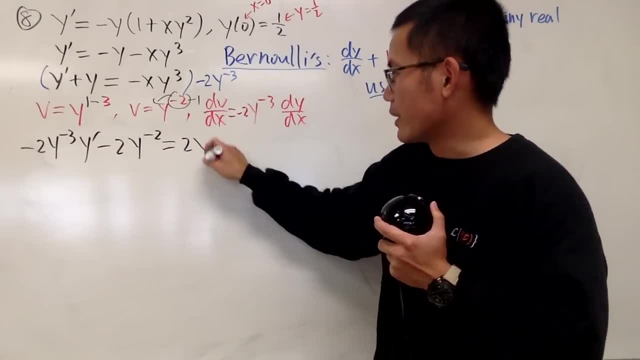 You see, negative times negative is positive. so we have 2, and then the x. yeah, right here, which is good, But y to the negative 3, and y to the negative, y to the negative 3 and y to the positive 3,. 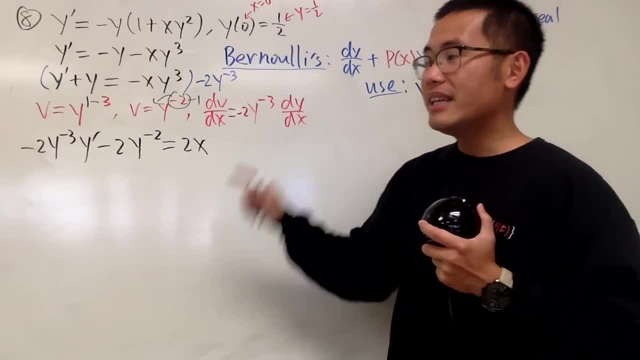 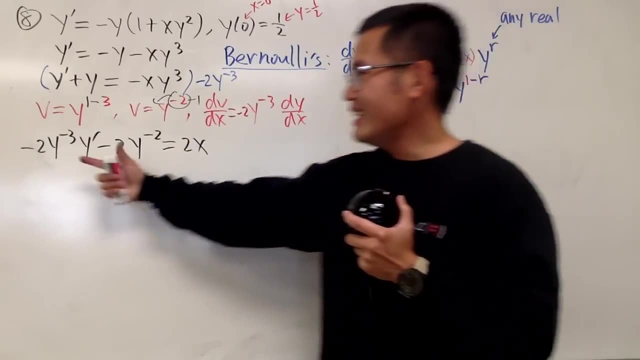 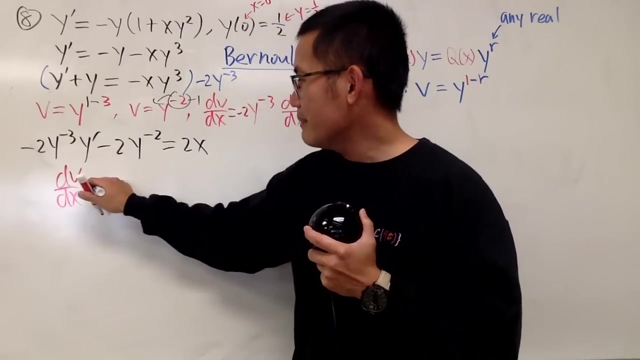 they cancel each other out very nicely. So we actually just have this, and this right here is linear. You'll see, it's gonna be linear very good, Because this right here is precisely our dv dx, And then minus 2, and the y to the negative 2 power. 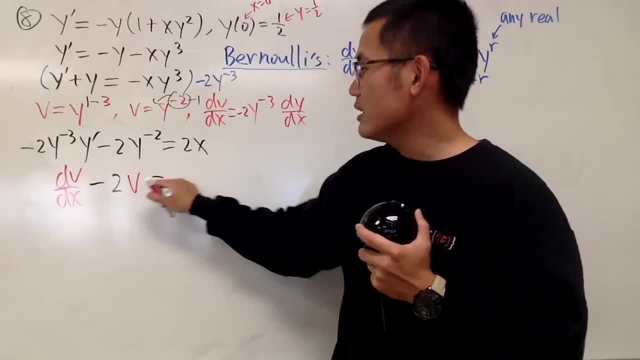 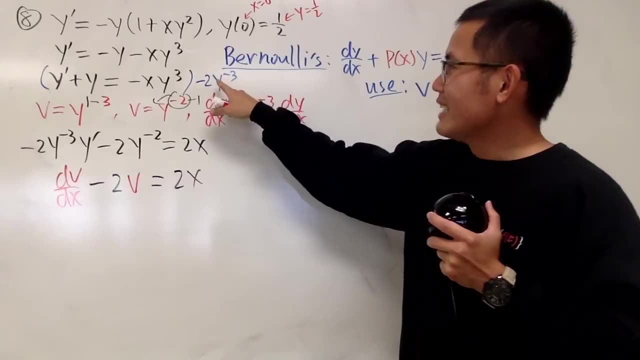 is precisely our v and you see, that's equal to 2x. And you see, Bernoulli is a genius: when you have the 1 minus And that, which is this part, they will cancel out. Right, they will cancel out because of the power rule. 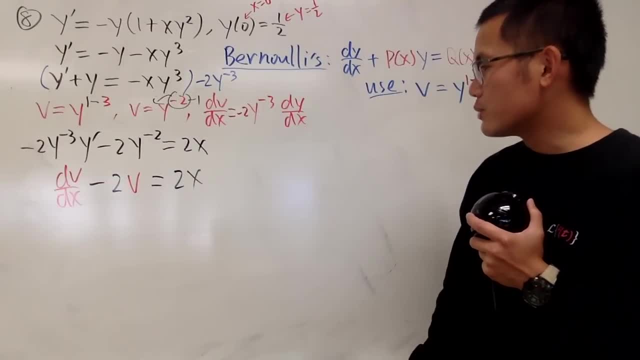 so that's why you have the 1 minus right. So we have this right here, and then let's see, of course we have to do the integrating factor right. So we have this right here, and then let's see, of course we have to do the integrating factor. 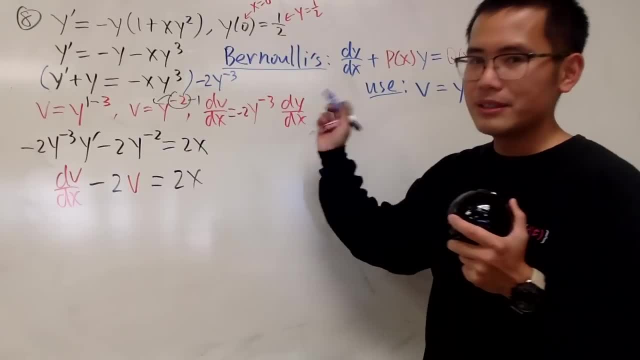 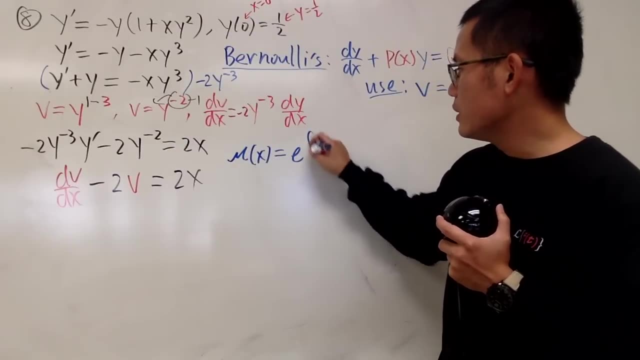 so let's go ahead and just do that. I know I made that mistake earlier, so I'll just do it real quick. Our integrating factor here is gonna be mu of x, which is e, integral of this, which is negative 2,. 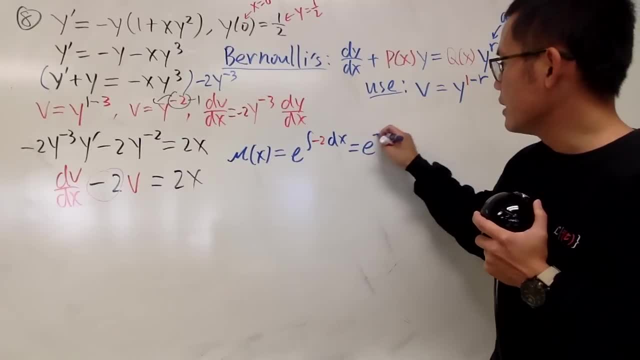 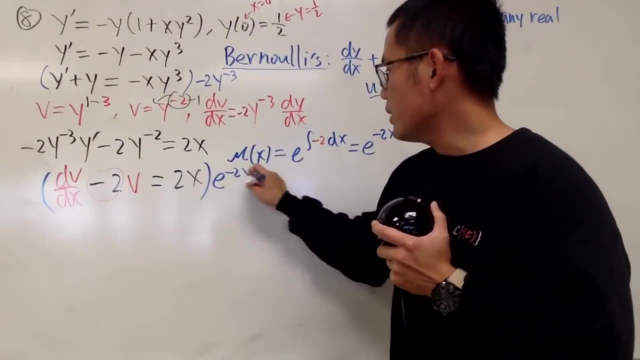 and this is dx. so that will be e to the negative 2x power. And don't worry about the plus c. that's all. Let's go ahead. multiply everybody by e to the negative 2x, So we will get e to the negative 2x. 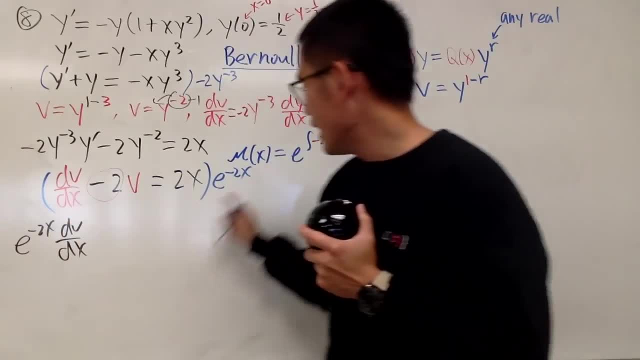 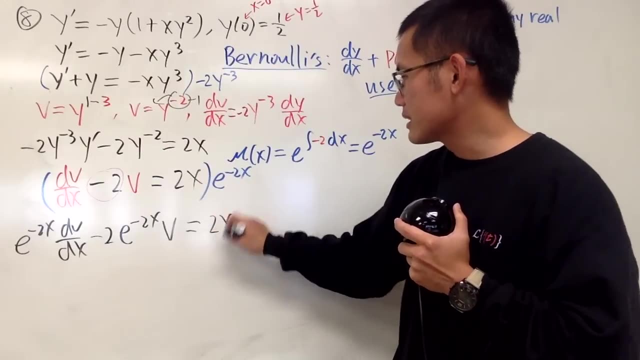 and then we have the v, v, dx and this, and that is minus 2e to the negative 2x and v, and then this is equal to all that which is 2x e to the negative 2x, like this I believe. 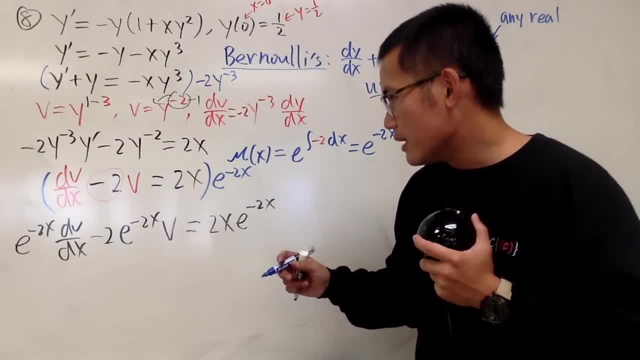 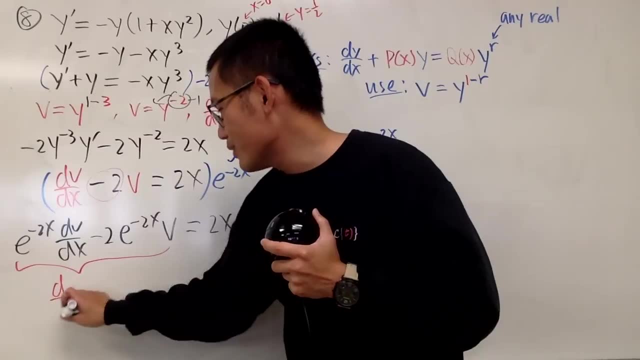 Well, good, Yeah, and then let's see. well, the left-hand side is precisely the derivative. This is still the same as the derivative of a product of two functions, and the first function is going to be the linear linear. 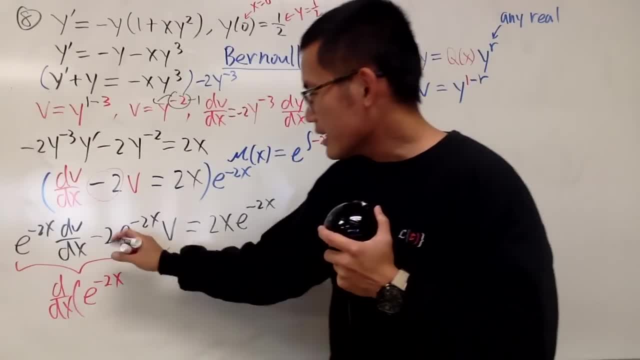 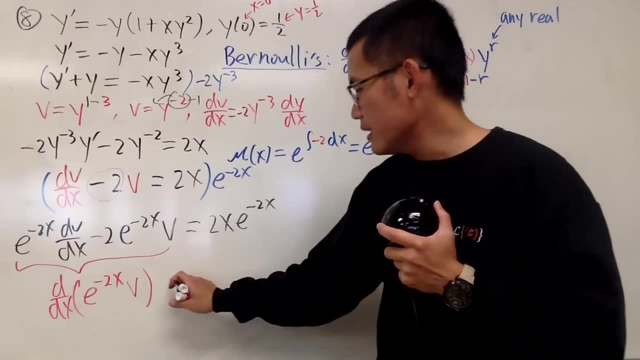 this is going to be the integrating factor. and then the second function is the v right, You can go ahead and check that out and, I'm sorry, wrong column. All right, and then the right-hand side. this is equal to this, which is 2x e negative 2x. 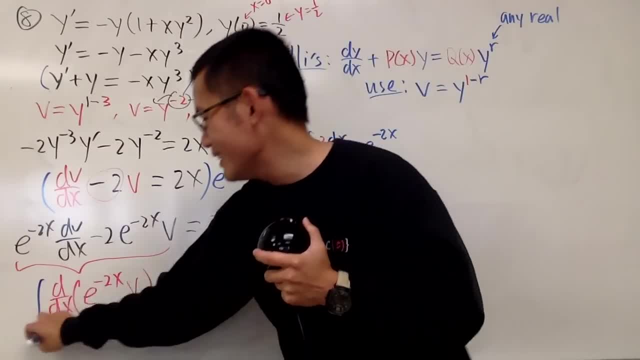 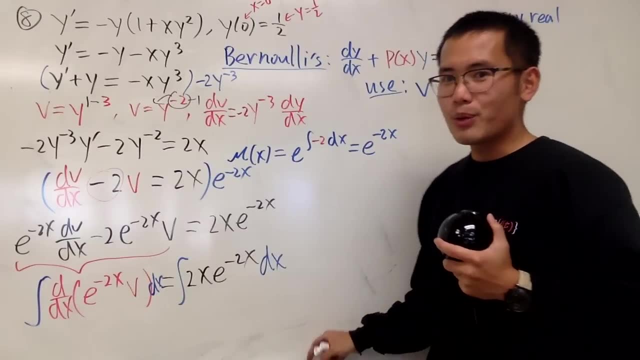 Good, Now to get rid of the derivative, of course. integrate, integrate, dx, dx. When you make a mistake, it's okay, we just do the same equation twice and then you'll get this, you know, double of the enjoyment. much better, right. 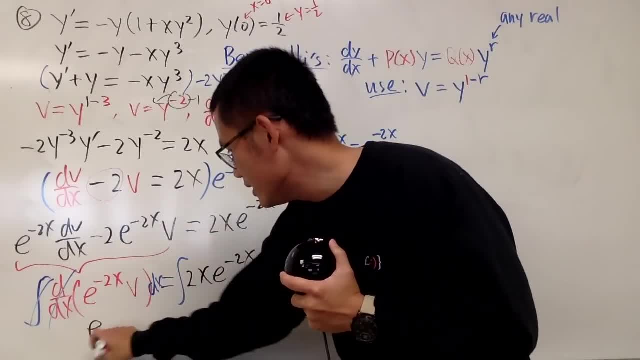 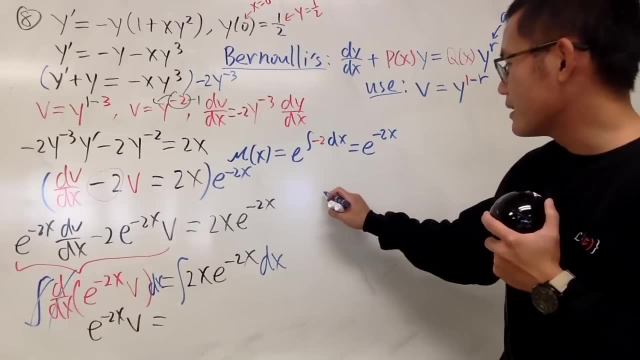 So, anyway, cancel, cancel. and here we have this, which is e negative 2x, v, and that's equal to this. right here we have to do integration by parts and of course we do that by the DEI method. 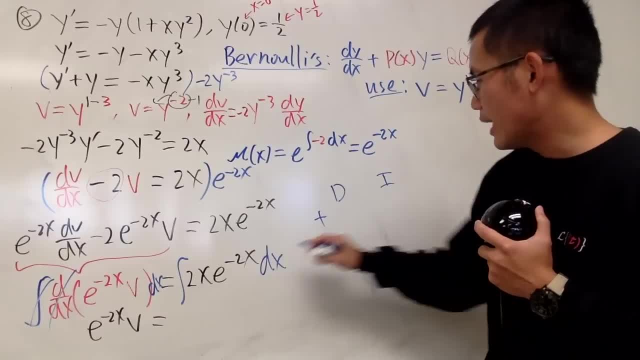 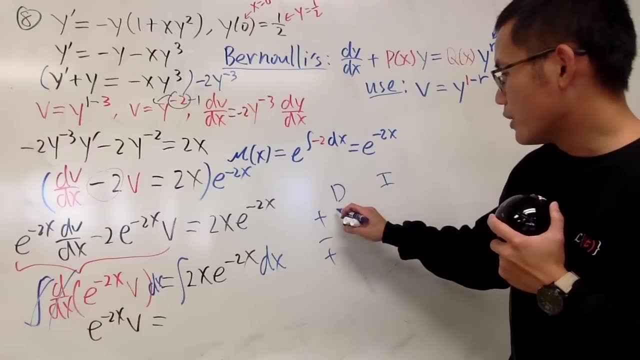 So DEI plus, minus, plus, and I will differentiate and I will differentiate. let me just make sure I don't. yeah, I will differentiate 2x here, and then I will integrate e to the negative 2x. Differentiating 2x, we get two. 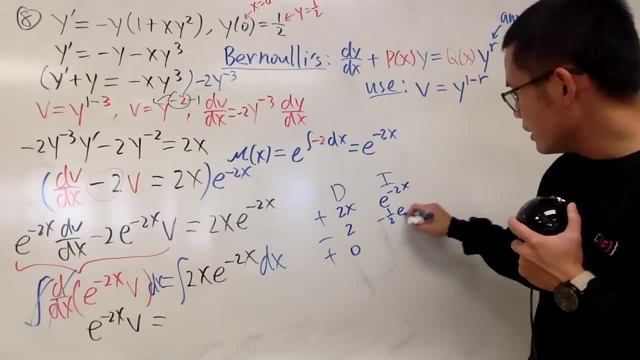 and then do it again, we get zero. Integrating this, we get negative one over two e to the negative 2x. and do it again: we get one over four e to the negative 2x, right, Good. 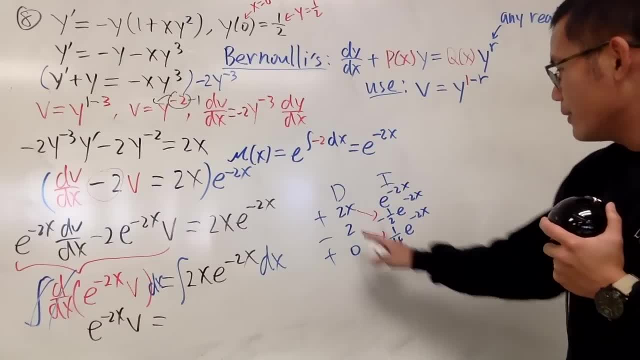 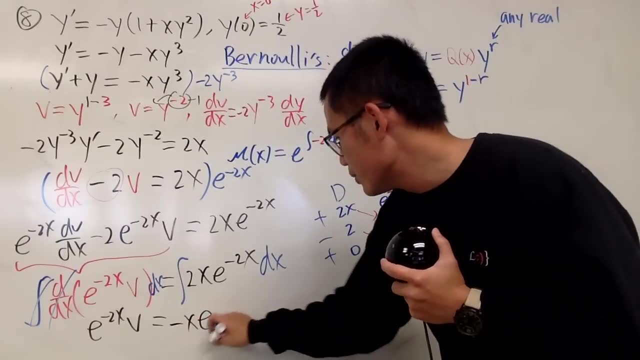 And then we have the answer already this times, this, this times, that Now, this times this: the two cancel out, and that's negative x. So we have negative x, and then we have e to the negative two power, and then also the x. 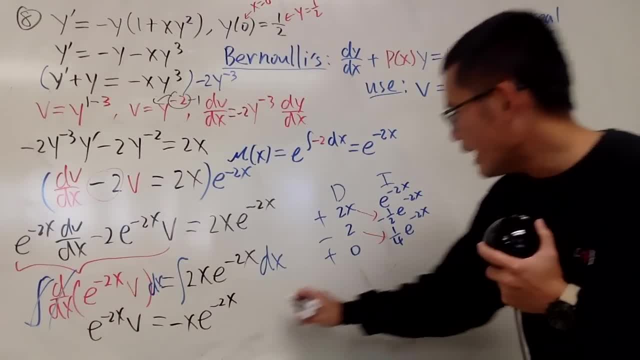 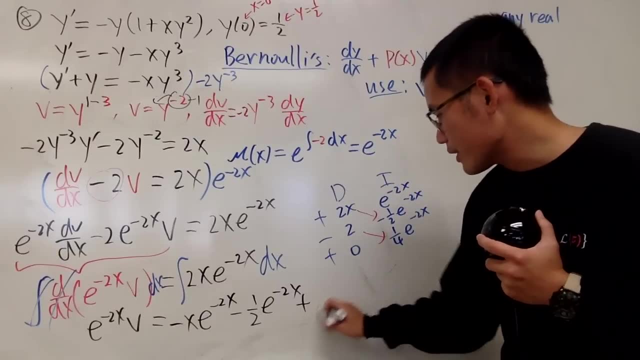 and then the next one is this times that which is negative one half, and then we have e, and then this is negative, and then we have e to the negative, two x like this, And right here, don't forget the plus c. 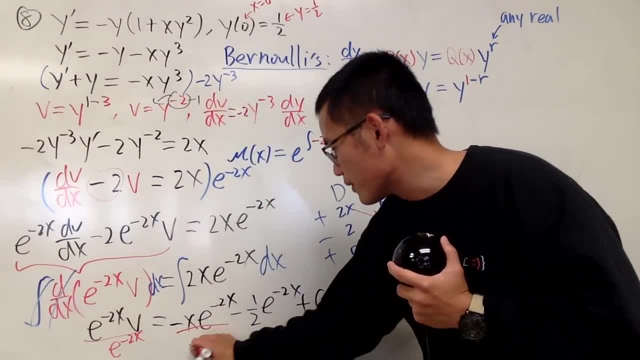 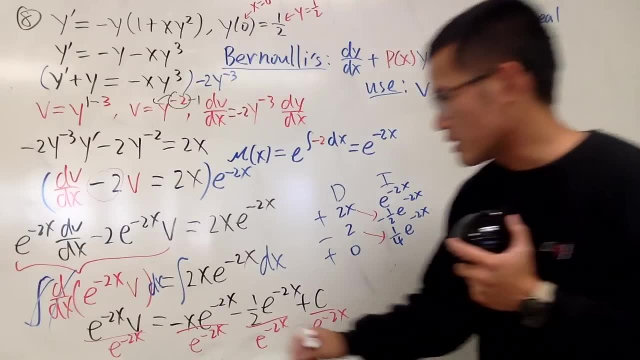 Now I will clean things up. divide everybody by e to the negative two. So just do it carefully, because we have negative exponents and also there's some a lot of like weird fractions. so let me just write down everything. 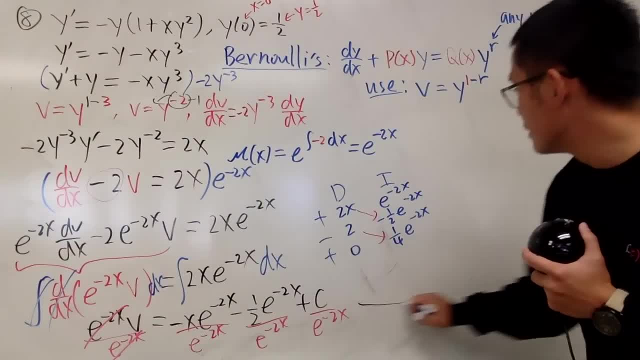 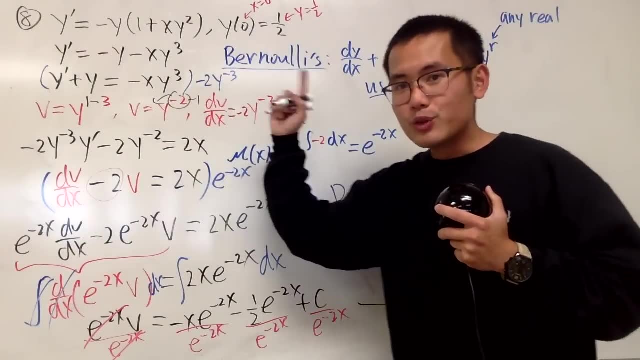 just to make things clear for you guys. Okay, so we have the phi right here. So now it's like a deja vu, because I know I did this earlier already. Anyway, phi is the same as this, which is one over y squared. 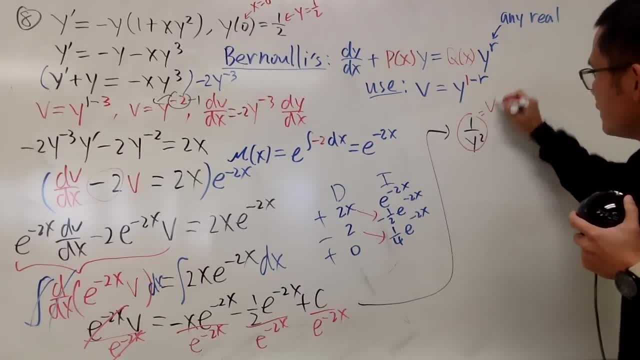 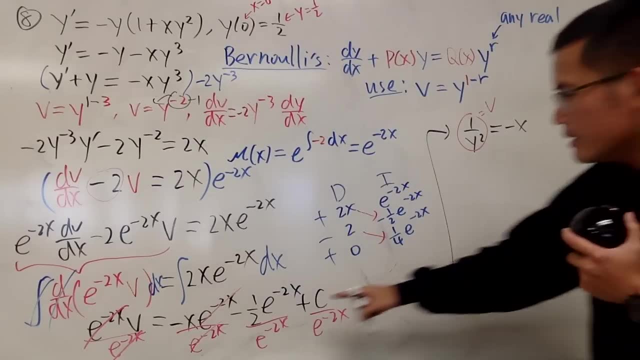 So let me just write down one over y squared, and then I'll do it again Again. this right here is the v, That's equal to the right hand side. This and that cancel, so we just have negative x. And then this and that cancel as well. 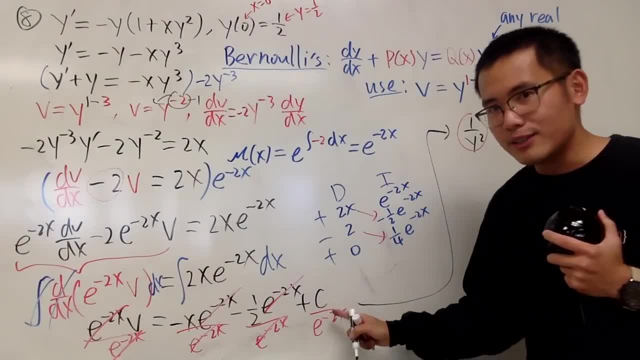 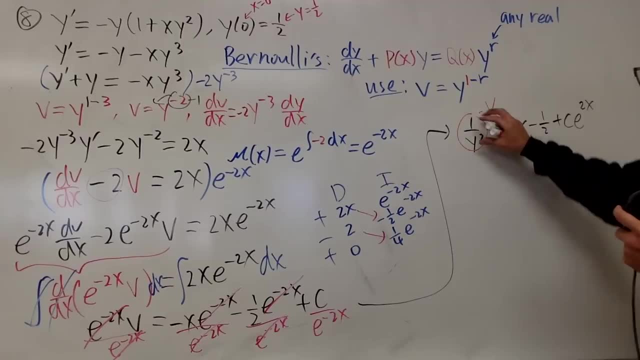 so we have minus one half. This right here cannot be canceled, but you can bring this up so we have plus c e to the two x power, like that. Now I will do the reciprocal on both sides. so we have y squared. 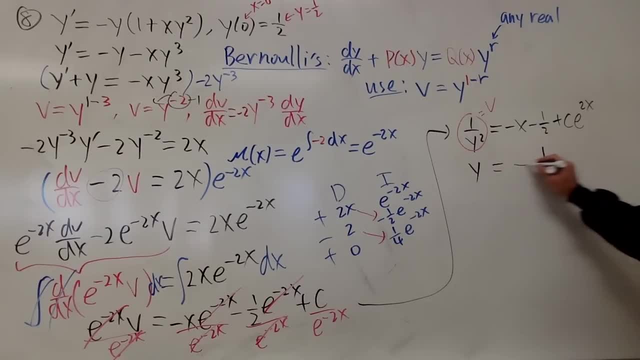 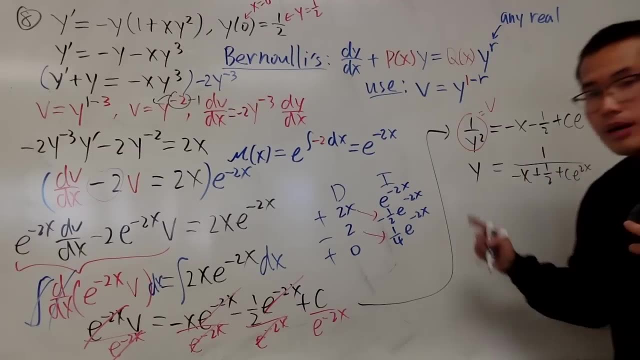 and I know I have a square, but just keep that in mind. Do the reciprocal, so I have one over. let me just write down negative x plus one half plus c, e to x. Well, I have the square, so I will take the square root. 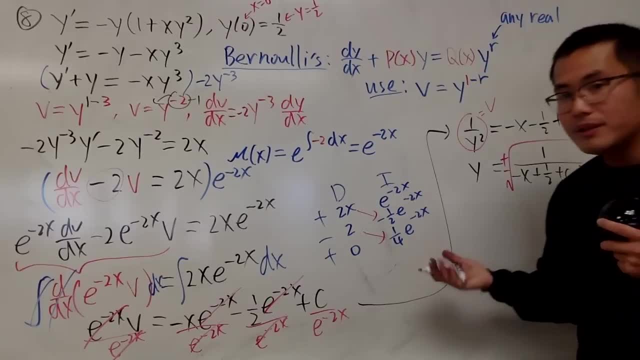 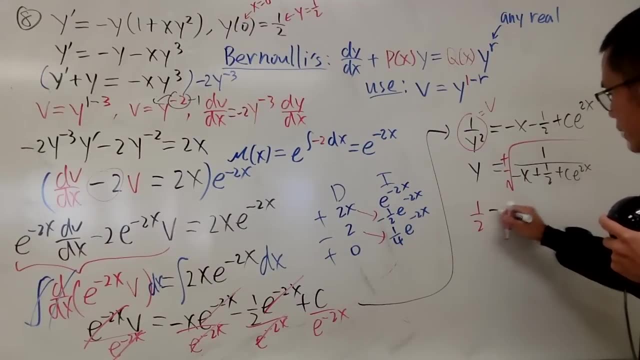 and I'll just do the square root right here And don't forget the plus minus technically. But again, x is zero, y is one half, So when I plug in I get one half. This right here is equal to plus minus square root. yeah. 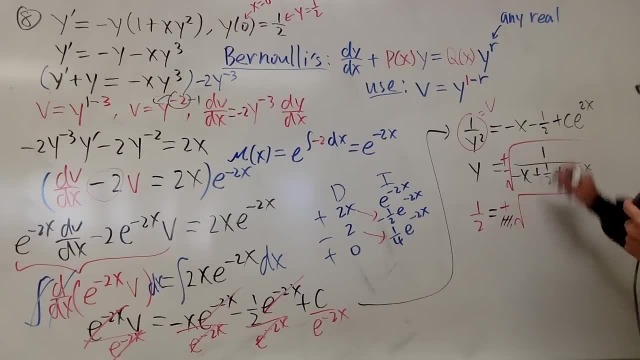 But this right here is positive, so I have to just use the positive version. Anyway, one over. keep this right here in black Like this: yeah, And again, negative, x is zero and then plus one half, and then plus c and then e to the two times zero's power. like this: 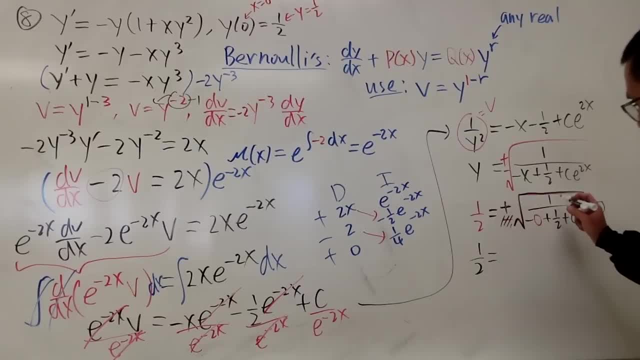 Here is one half. This is equal to the positive square root, So I will square both sides. So this right here becomes one over four right, And then this is one over. This is zero, doesn't matter. so this is one half. 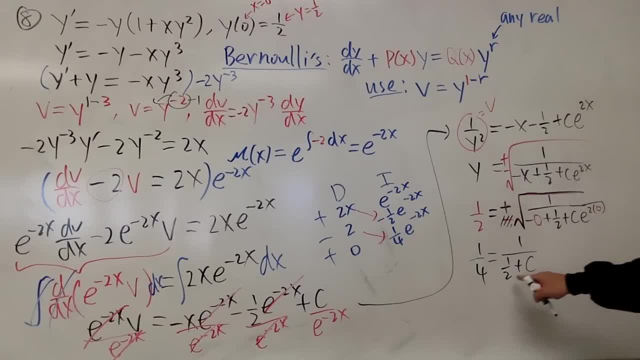 plus this: right here is c. So, of course, right here, this has to be equal to that right. So, of course, right here, this has to be equal to that right. So, of course, right here, this has to be equal to that right. 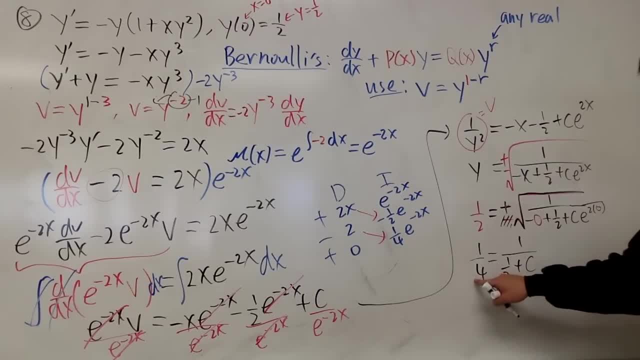 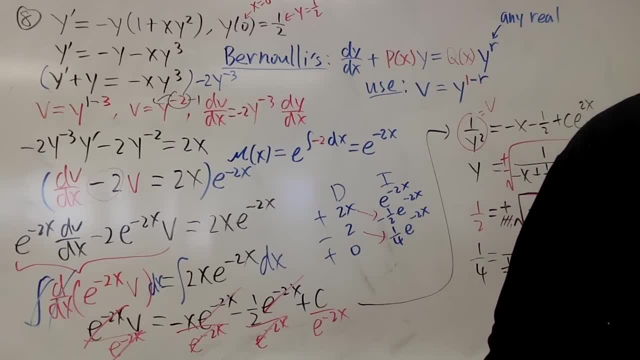 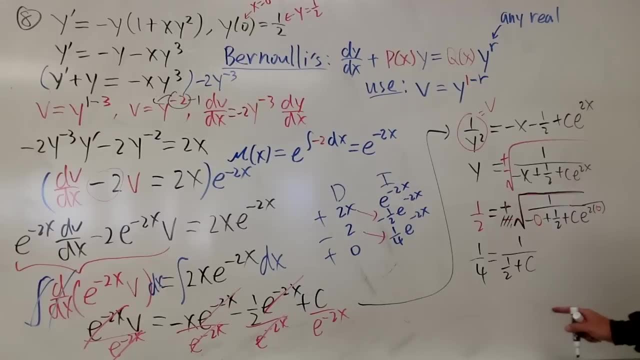 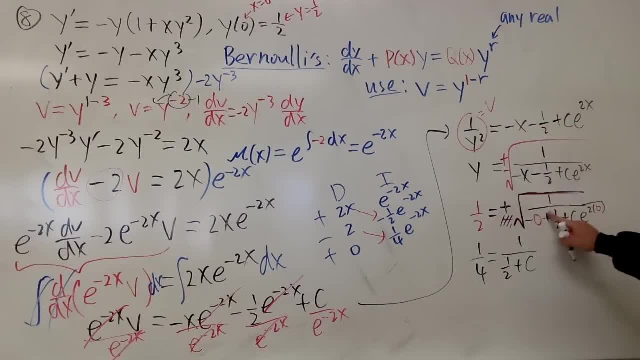 I'm so sorry For this question, man. I'm so sorry, Okay. Anyway, negative one half, so this right here is equal to x, and then plus one half right here is equal to that. so this right here is the same as 8 over 2 is equal to that. so that means 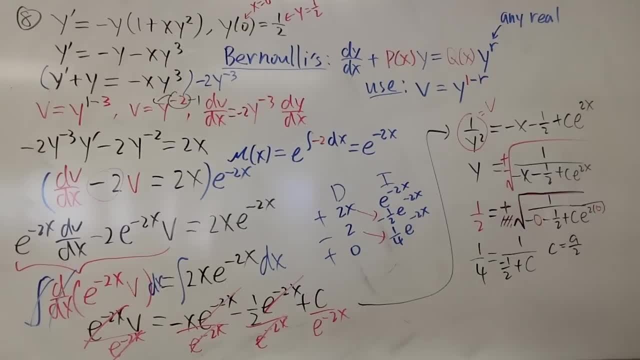 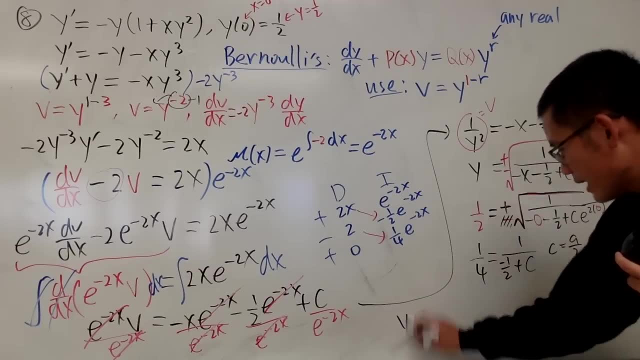 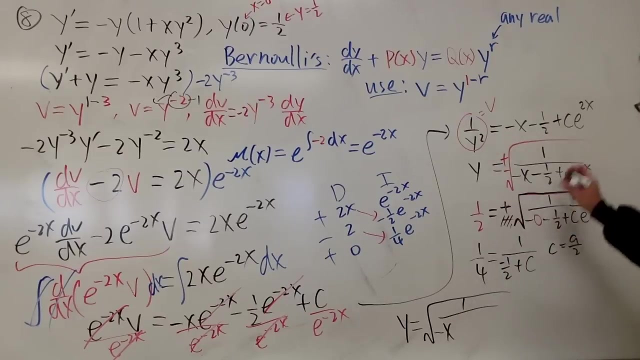 c has to be 9 over 2, like this, right. so finally, i'll see if i can write this down- we have y- i'll put this down here- y, which is the positive square root, and then we have 1 over negative x, and then minus 1 half, and then this is plus, c is 9 over 2, and then we have e to the 2x power, like this right. 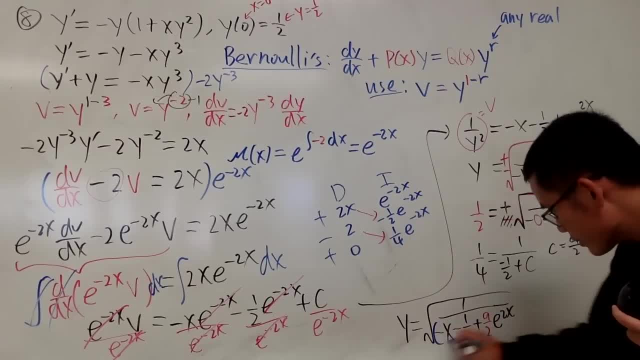 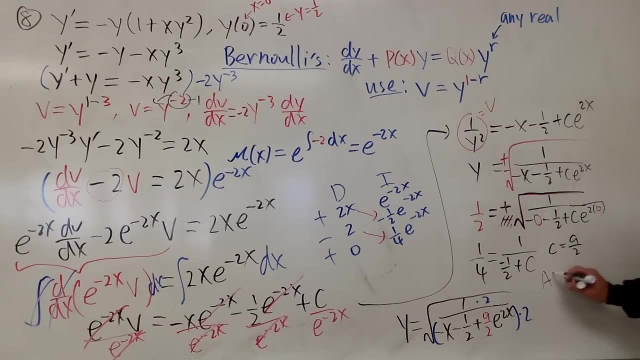 so of course in the end here we can just do a little clean up so that we can avoid use complex fractions. so to multiply the top and bottom by 2.. so finally, i'll write this down right here: answer all right. this right here is done for sure. right. y equals on the top of square root of 2. 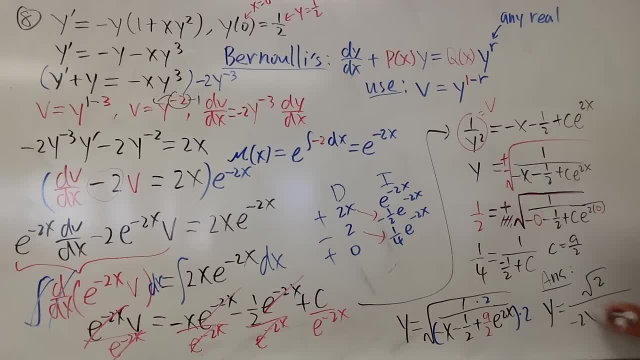 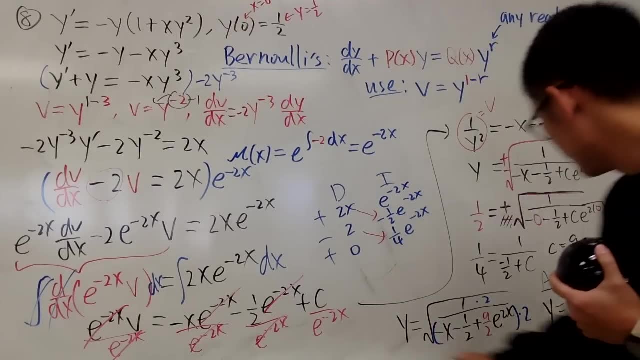 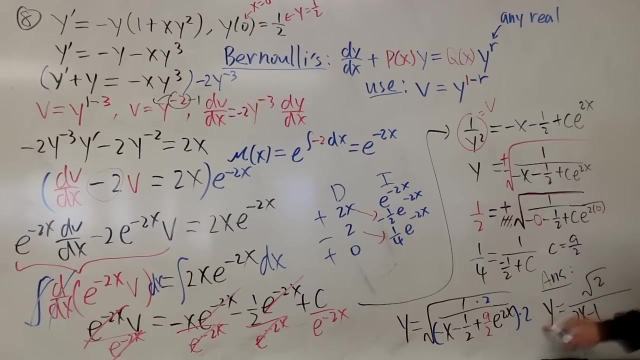 on the bottom 2 times, that is negative 2x. this times this is minus 1, this times this is plus 9. and then we have you guys cannot really see anymore. let's see negative 2x minus 1 and this and that is plus 9. e to the 2x power like this: 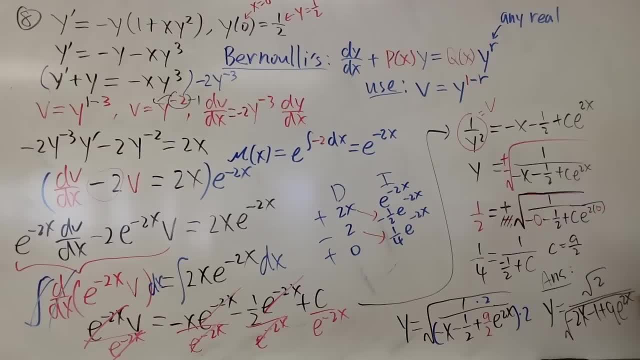 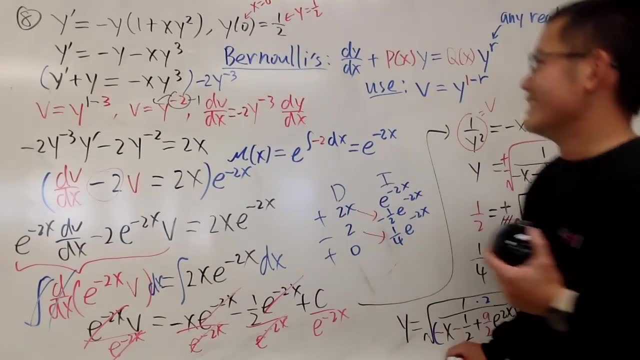 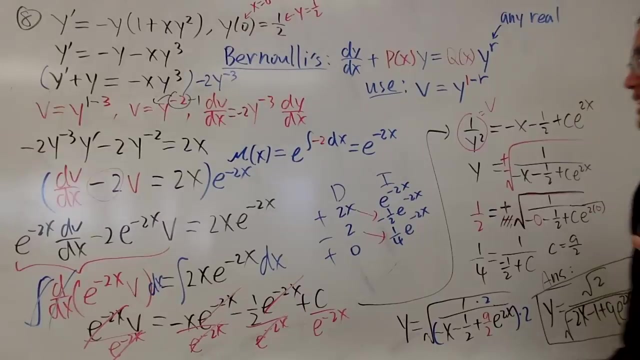 and again the button also has the square root. okay, so here is the answer. here is the answer. man, hopefully this is okay. i don't know make two mistakes, that careless mistakes and that kind of just ruins the whole thing. so be really careful. i make mistake too, even though i did. 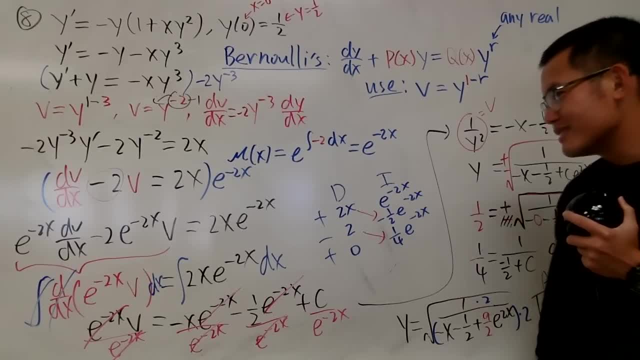 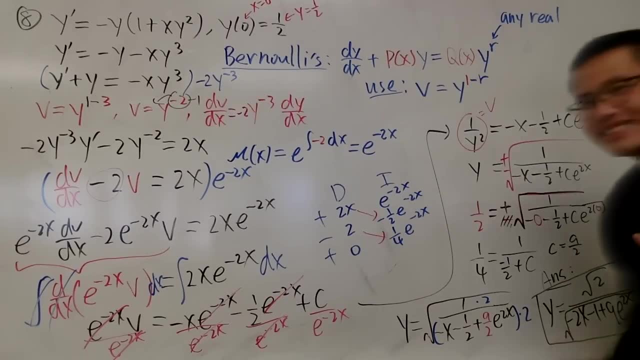 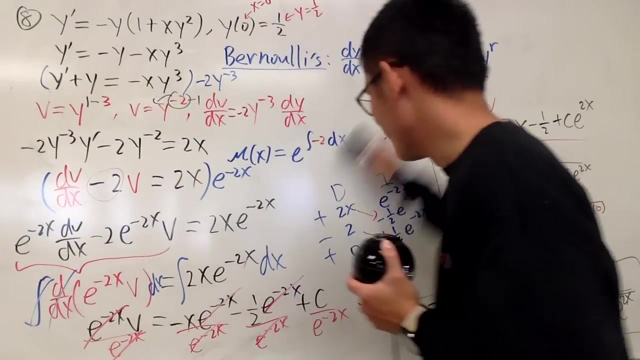 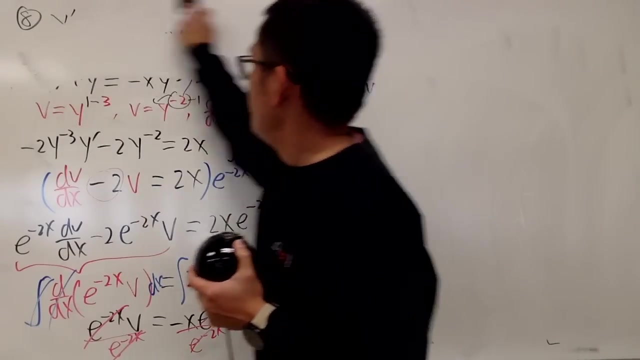 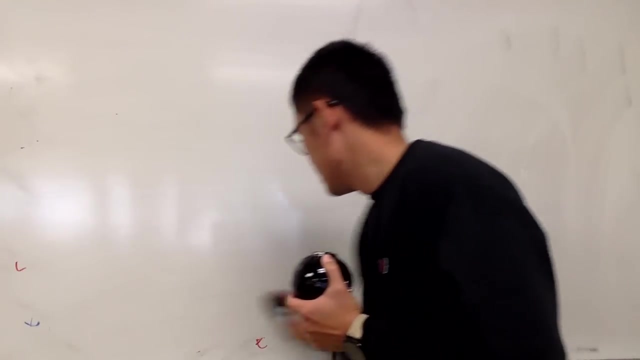 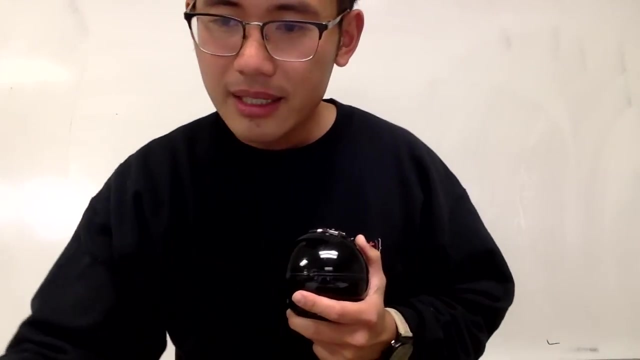 this questions beforehand, so that's how i know something was wrong. but yeah, so go ahead. look over this again. so final answer and no mistakes. yeah, okay, number eight and let's see. hold on. am i taking one hour and 37 minutes of time? Okay, so stay strong, yeah. 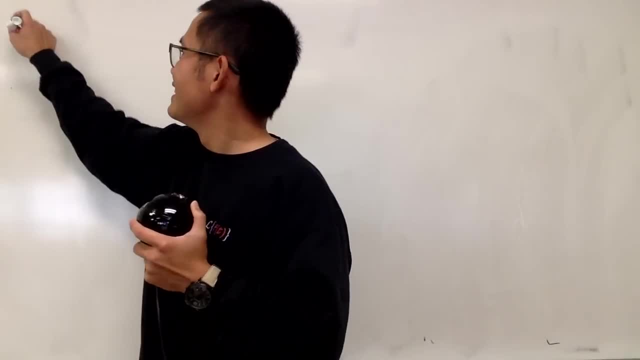 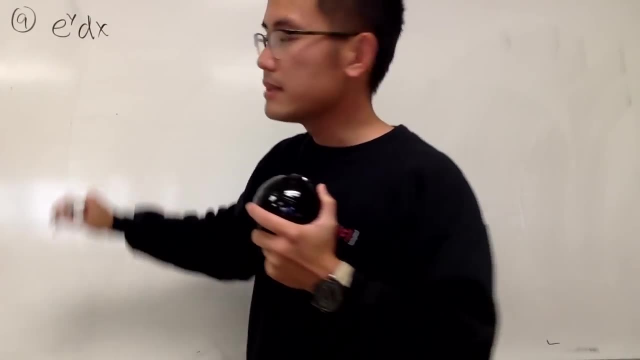 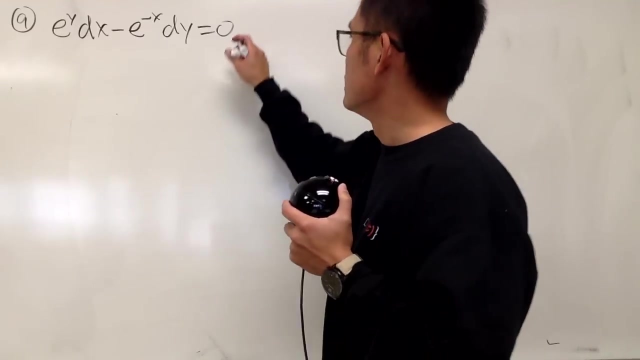 So now number 9, right here. So here we have e to the y dx, and then minus e to the negative x dy, that's equal to 0, and we have y of 0, it's equal to 0, like that right. 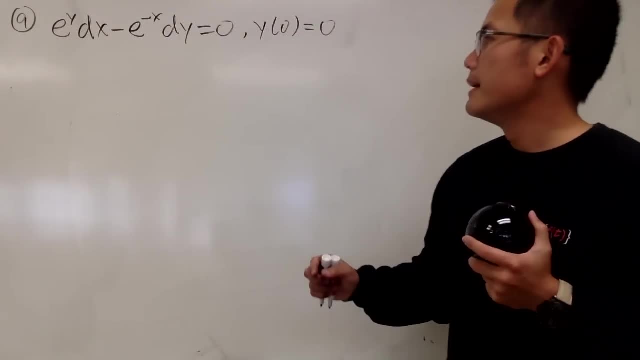 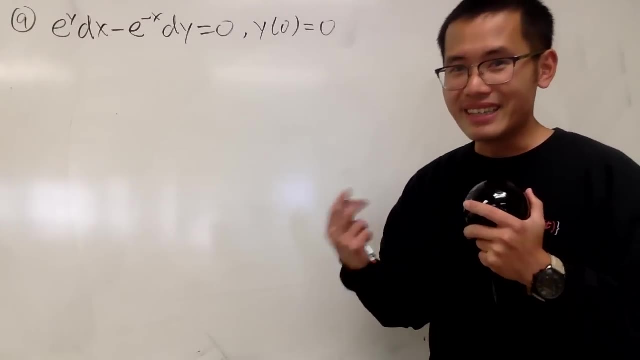 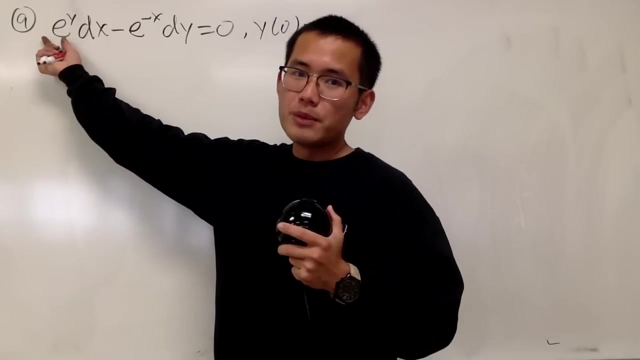 So let's see, hmm, is this exact? Technically it will be, if you just arrange it. You can arrange it in a careful sense, but this right here is actually separable. And one thing that you notice: this is just a function in terms of y, only with dx. 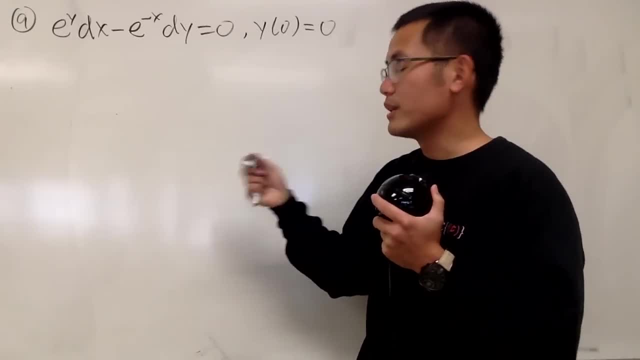 The function in terms of x only with dy, so it's separable. So you can just go ahead and do the following, separating the variable. So let me bring this to the other side and I'll make this positive. 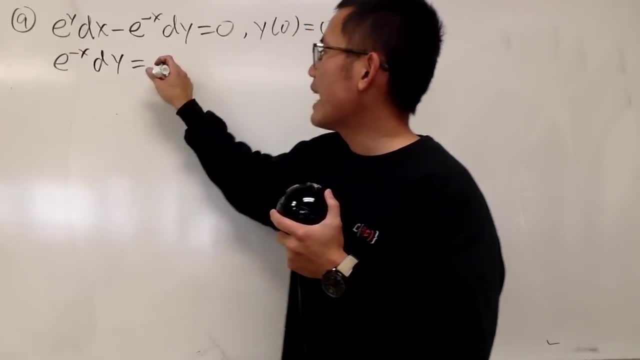 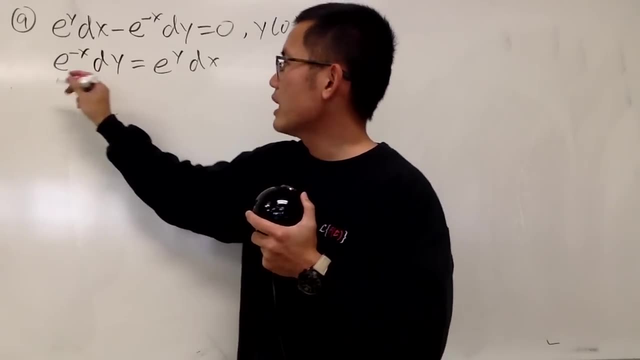 In other words, e to the negative x dy, that's equal to that guy, e to the y dx, like this, And I will just bring this to the other side. bring that to the other side. Do it carefully though. 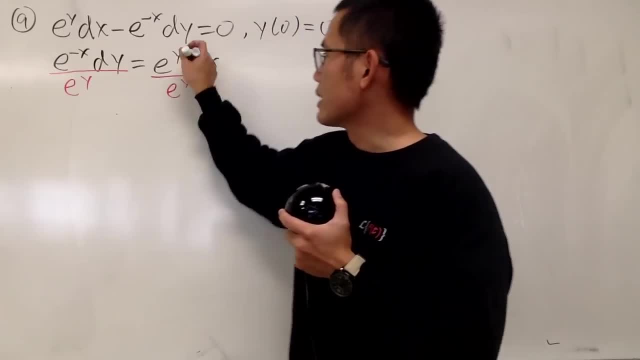 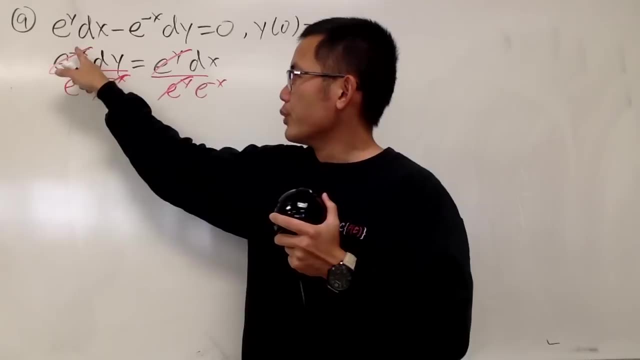 I'm going to divide both sides by e to the y, so that this and that cancel. and I'll divide both sides by e to the negative x, so that this and that will cancel. So here's the deal: To integrate 1 over e to the y. I will write this as e to the negative y dy. 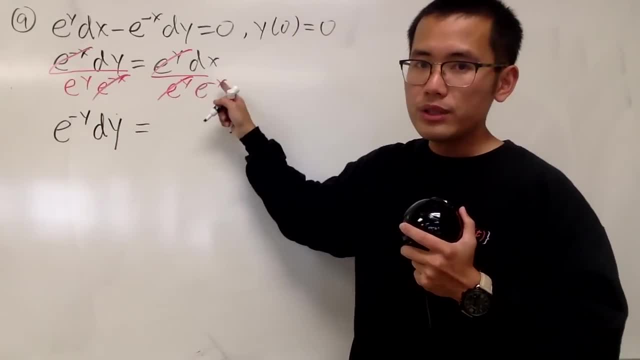 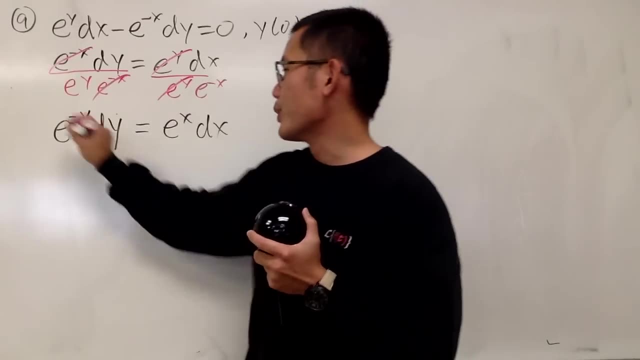 That will be the same as 1 over e to the negative x, which is going to be positive x right here, yeah, And then dx, like that. So now we can integrate. integrate With any separable differential equation. it's also exact, so that's fine. 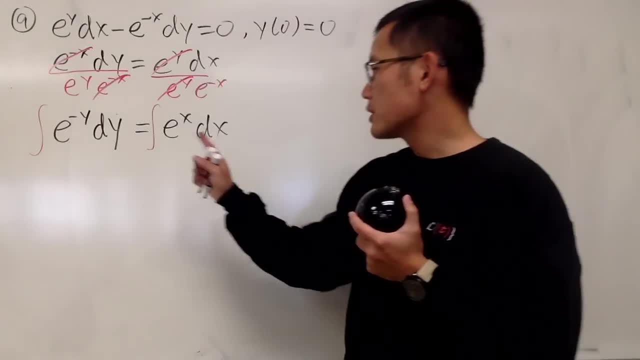 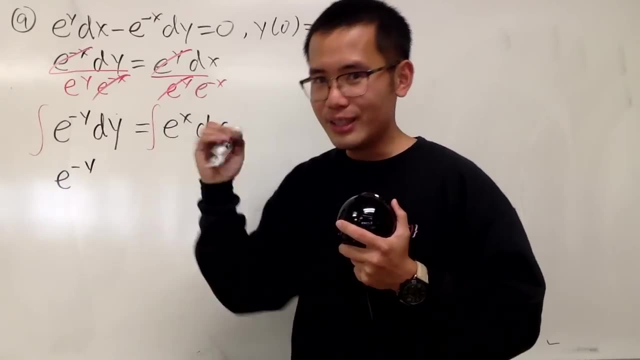 But you have to do arrangement first. Okay, so here we go, Integrating e to the negative y. well, we just get e to the negative y, but don't forget the Lu-Chen, the reverse of Chen-Lu. yeah, 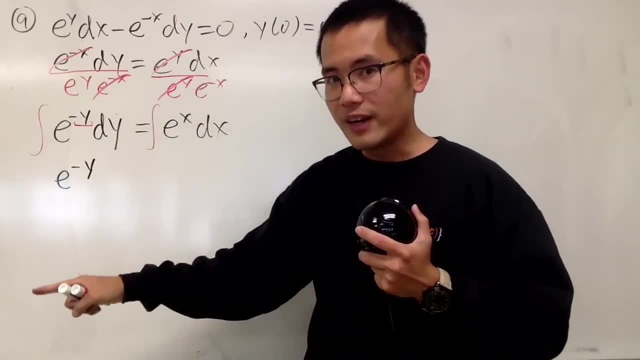 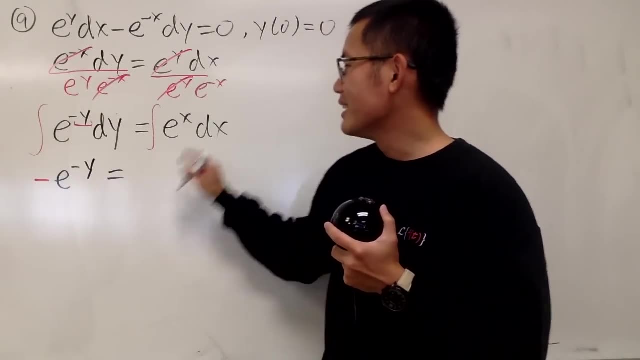 The derivative of negative y is negative 1, so we have to divide it by that constant. so you just have to have another negative right here. Don't worry about the constant, just put that on the right-hand side. Integrating e to the x is just e to the x. 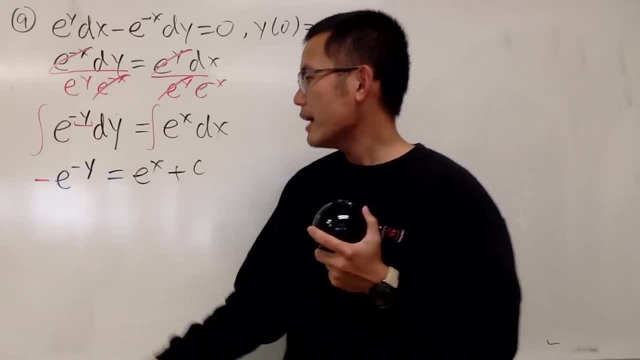 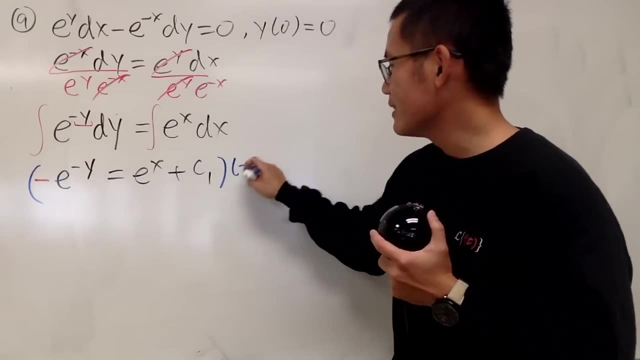 Now plus c, like that. Now I want to isolate the y. so here's the deal. Let me say this is c1, because I'm going to multiply everybody by negative 1. When we do that, we get e to the negative y. that's equal to negative e to the x. 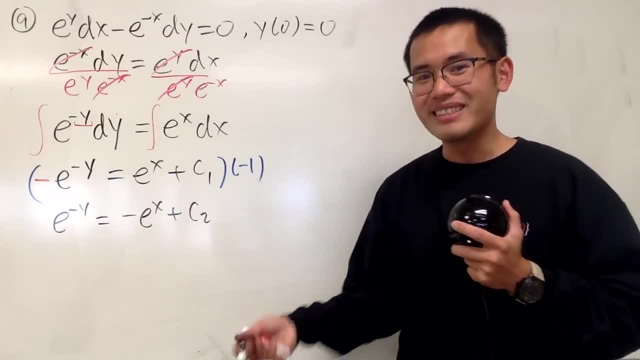 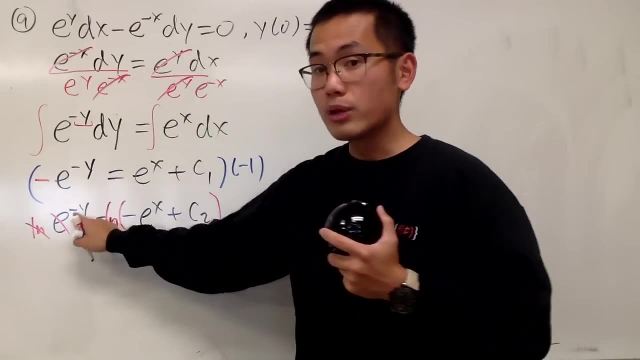 This and that is plus c2.. Just call that to be another constant. yeah, Alright, so now of course we can do the natural log on both sides, so they cancel, and I will also divide the negative on both sides. 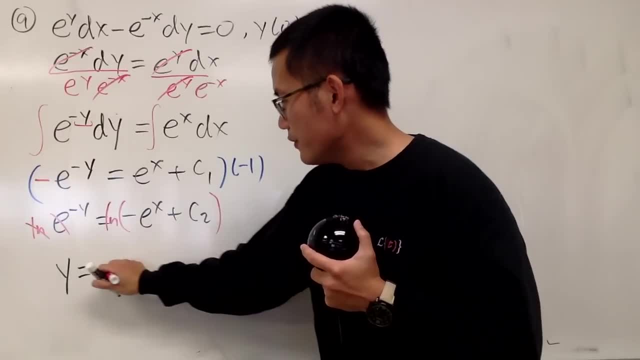 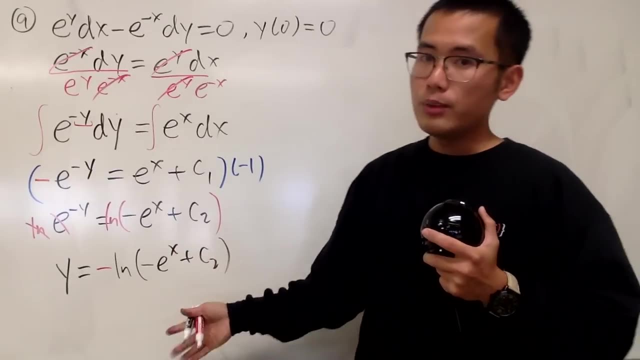 So I get: y is equal to negative, and then we have ln parentheses, negative e to the x plus c2.. And this is pretty much the general solution, so you don't have to have the subscript 2.. But we're not done yet, because we have the initial condition. 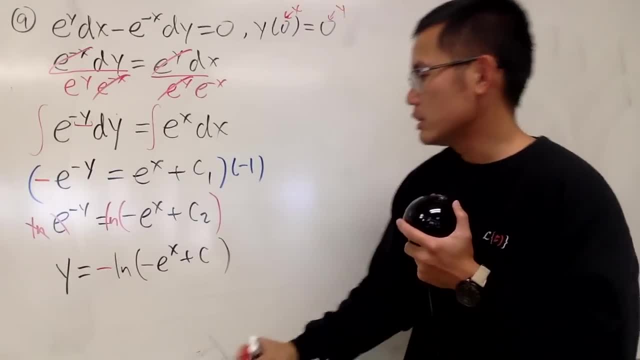 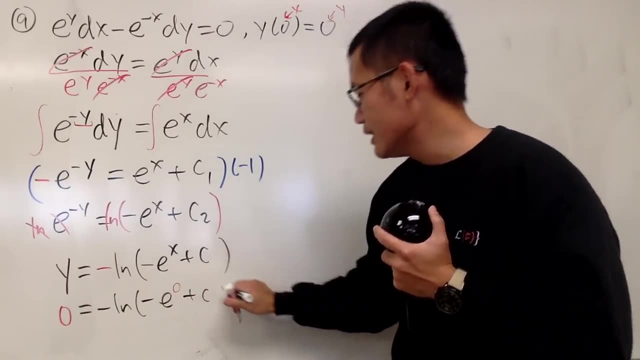 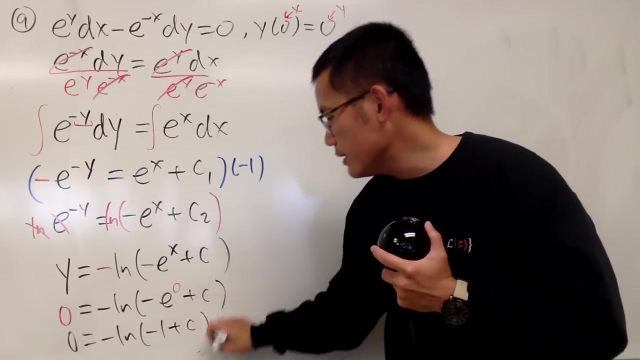 So x is 0, y is also 0. So here we have 0 equals negative ln. parentheses negative e to the 0th power, plus c, like that. So here we have 0 equals negative ln of negative 1, plus c ln of what will be 0?. 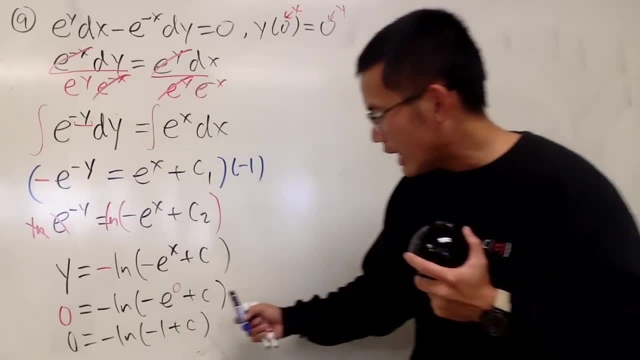 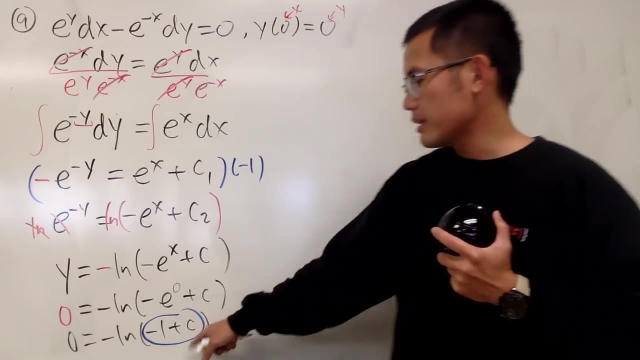 The input has to be positive 1.. But here we have negative 1 plus c already. so that means c has to be positive 2, right, Plugging 2, you will get 0.. So finally, I'll just write down the answer right here. 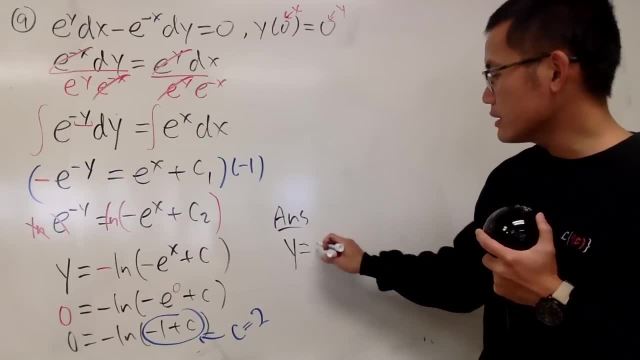 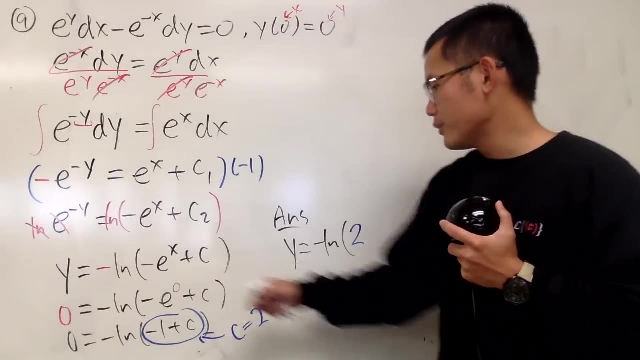 For you guys. this right here we get y equals negative ln parentheses. perhaps that's right on the c. that's right on the c, which is 2 first. yeah, That's right on the c first. and then we have 2 minus e to the x power. 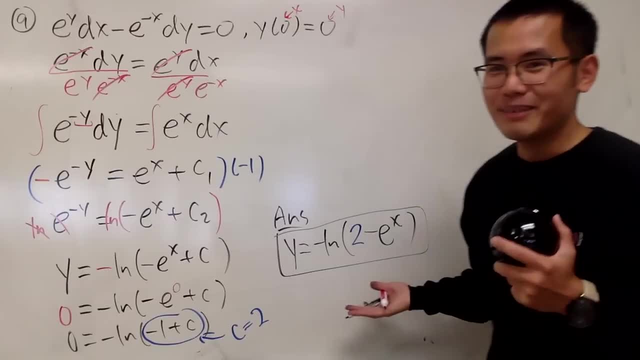 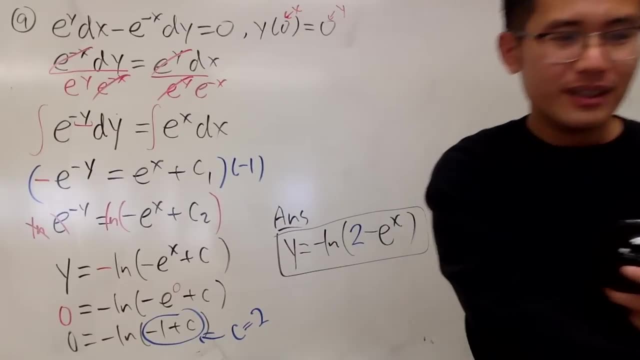 Just like that. Much, much better than the Bernoulli equation, huh, Alright, so yeah, I'm also checking to see if I that my answer key is right or wrong. huh, So just let you guys know, Yeah. 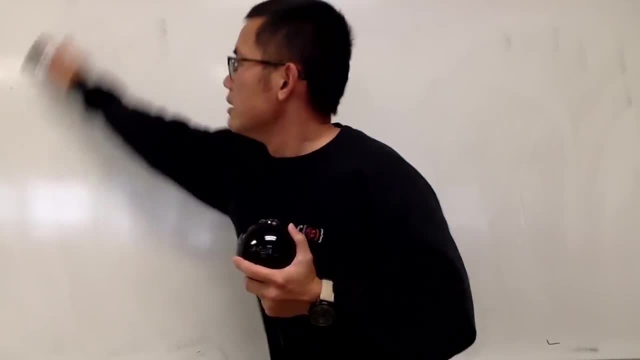 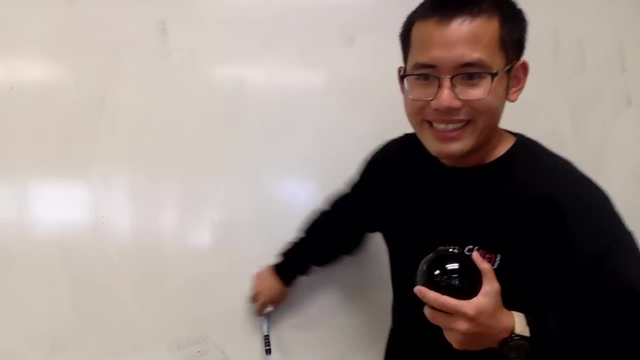 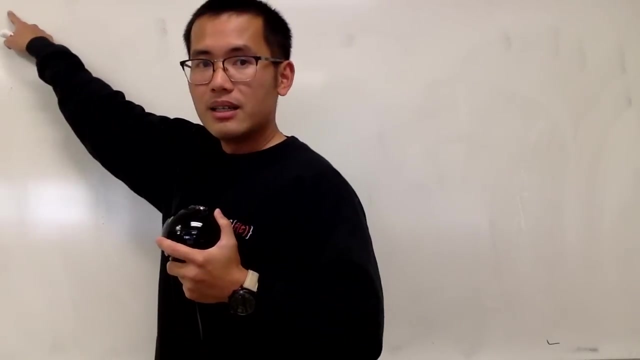 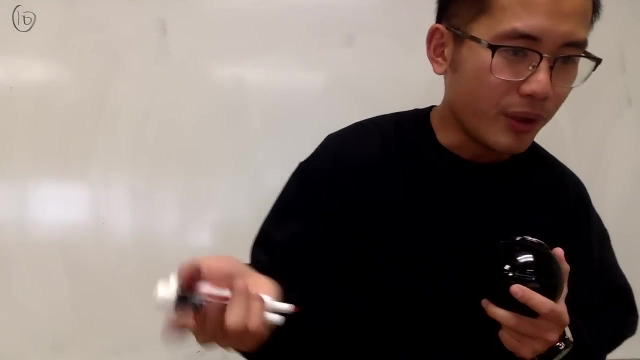 Alright, so number 10.. I'll try not to look at, uh, my answer key, But I will try to see if I have the correct answer key before I, before it gets downloaded. so that's why I wanted to also check that stuff. 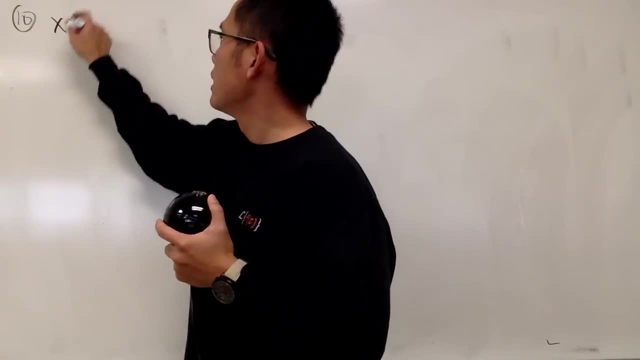 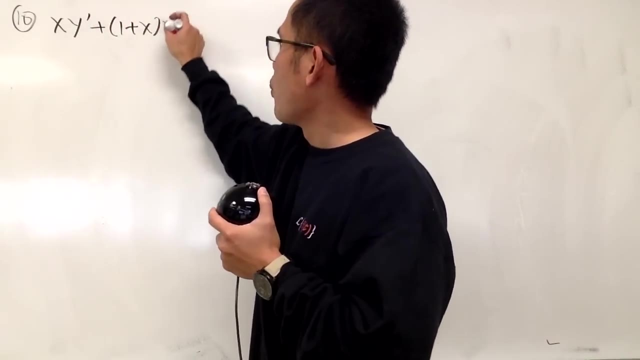 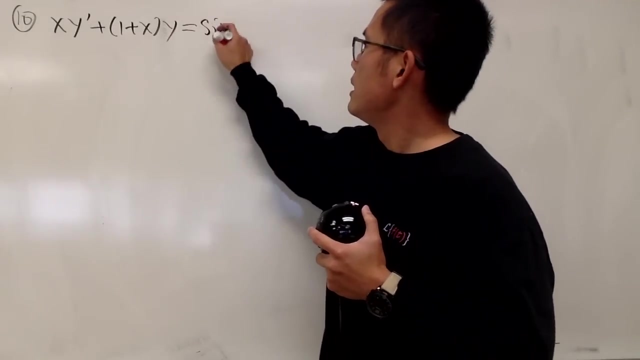 Anyway, number 10, we have x, y, prime And uh, plus parentheses, 1 plus x, y, and this is equal to sine x. Yeah, just like that. Now here is the deal. This is linear, yeah. 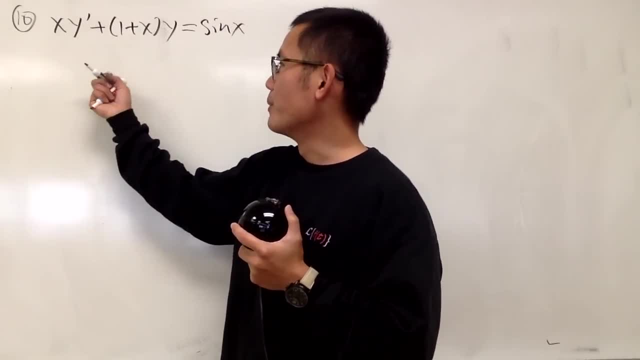 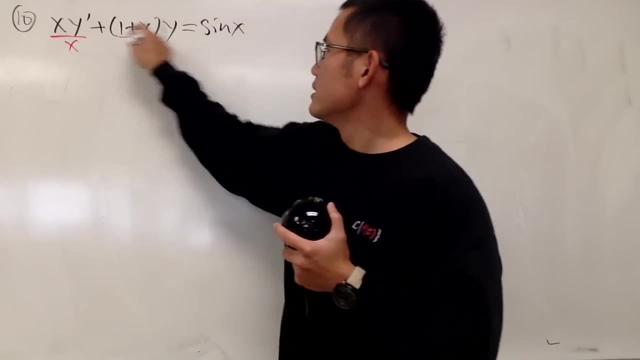 But it's not in the standard form, so let's go ahead and make that into standard form. So that means I will just have y and actually let me do the following for you guys: I would like to divide everybody by x so I can put this in the standard form. 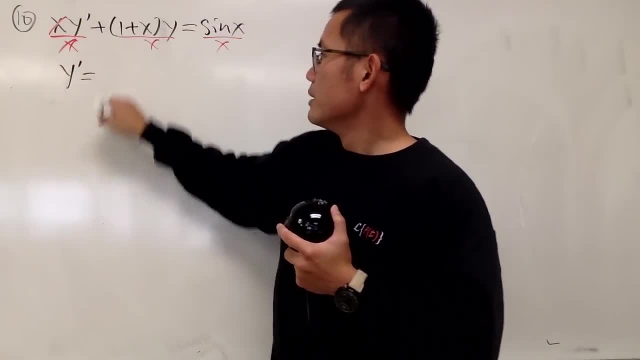 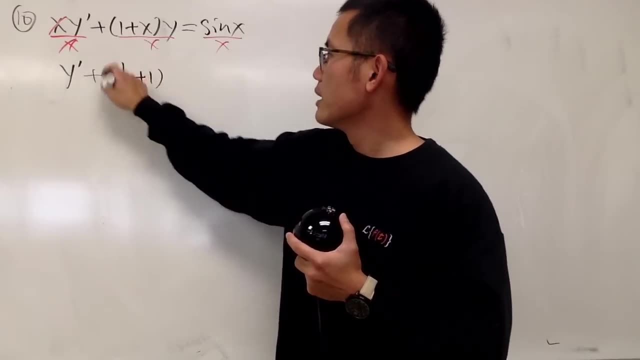 So of course that and that will cancel. We get y prime. that's what's the plus. This over that is 1 over x. This over that is plus 1.. And then we have the y, and this is equal to sine x over x. 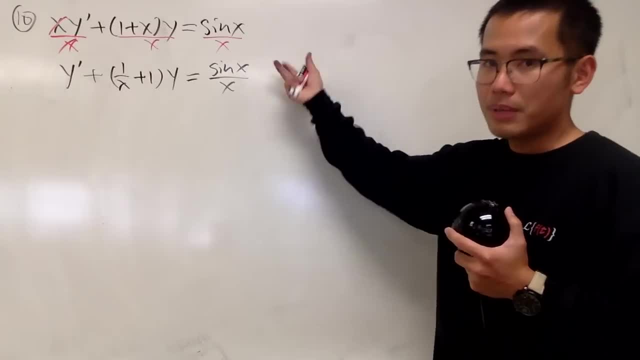 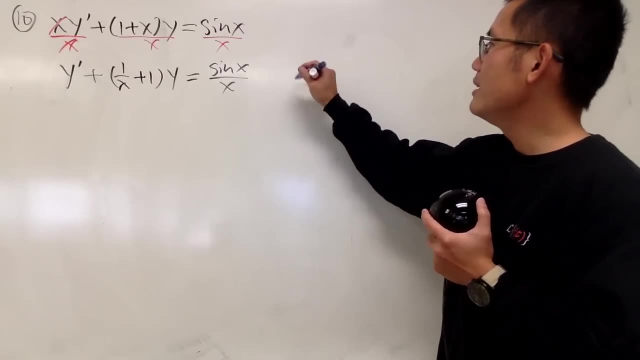 This is not Bernoulli. Bernoulli is with y to some power, but this is just that by itself. So this is slightly better. It's just linear right away, And here is the Linear integrating factor. So I will write this down right here. 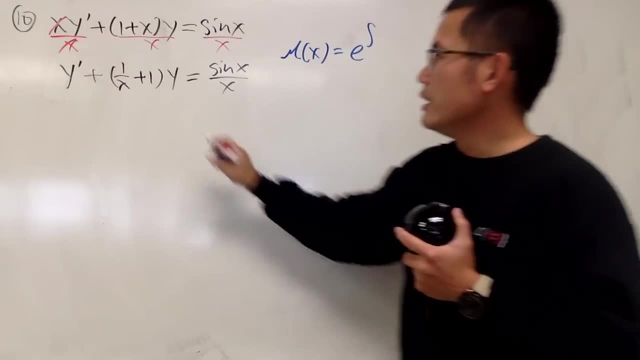 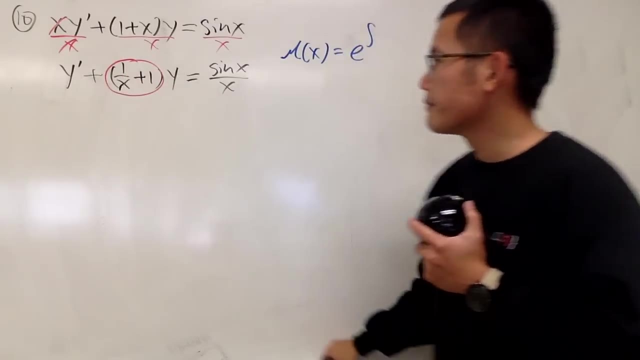 So let's say mu of x, which is e integral, And this is the p of x, and with both parts right, with both terms. So be really careful with that. So let me write it down: 1 over x plus 1, and then we have to integrate that. 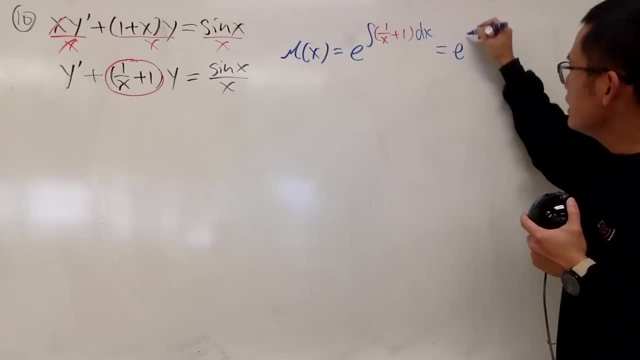 Well, well, here we go. That's e, and then we have natural log of x- Good, And then plus the integral of 1. It's just x, And technically you can put an absolute value, but again, it's not needed later on. 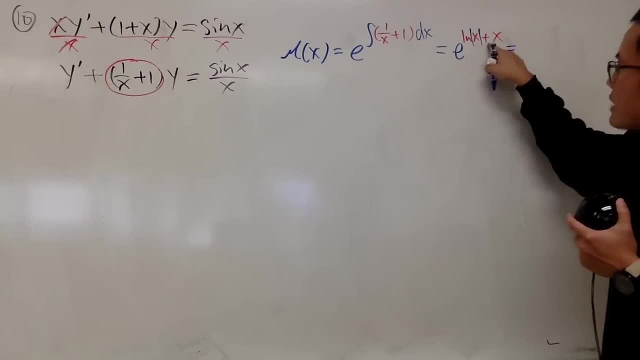 Now this is how you're going to break this down: e to a sum right. This right here is a sum of two powers, So you can write this as e to the first times, e to the second, Just like that. And for this right here, if you have the absolute value again, you can just cancel them out. 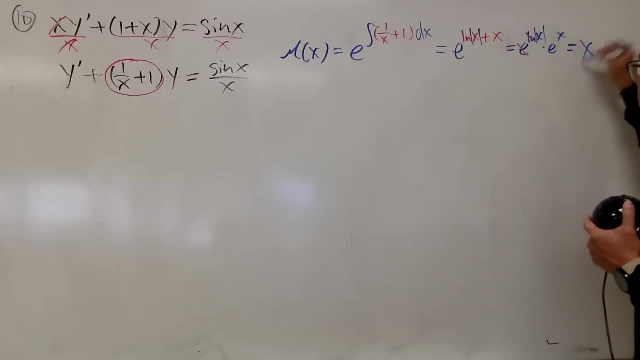 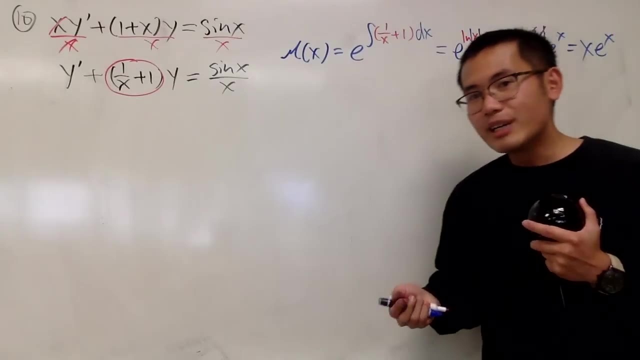 And again, this right here gives us x. Just use x. Yeah, just use x. Just get rid of that, Doesn't matter, Doesn't matter. And then e to the. So this right here is our integrating factor. Okay, go ahead, multiply everybody by x. e to the x power. 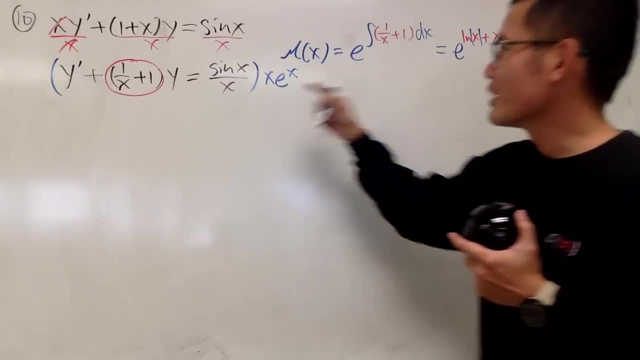 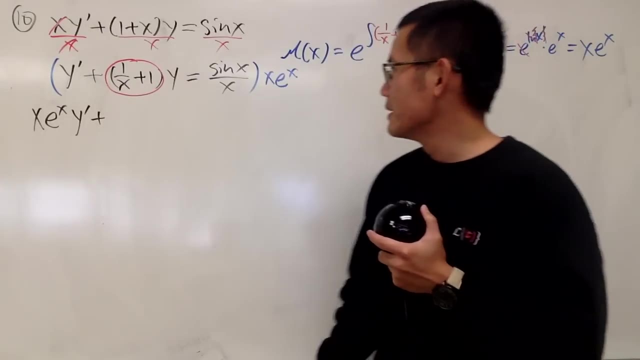 And now let's see what we have left. All right, so now we have x, e, x, y, prime plus this times that. Okay, so do it carefully, This times that the x cancels out. so I will just have e to the x. 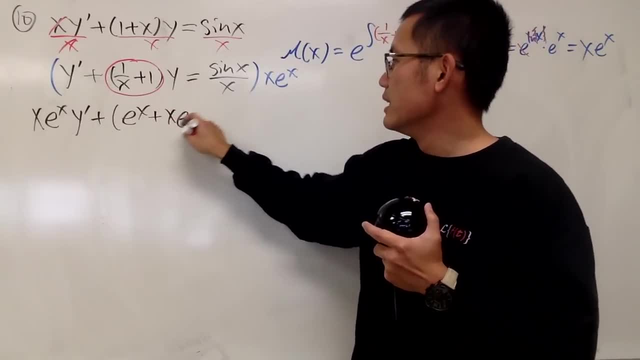 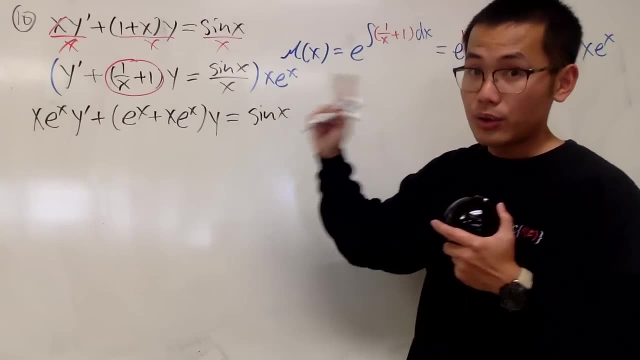 Next, this times that I will have plus x, E to the x, And then y. This times that the x cancels out. so we just have sine x. But don't forget, we still have the e to the x. 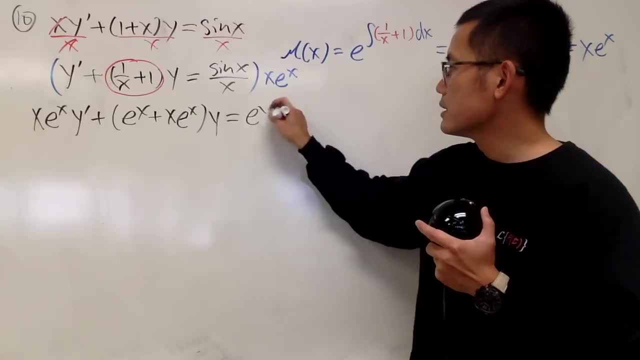 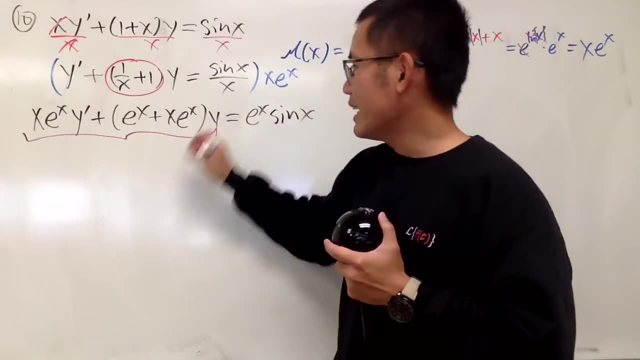 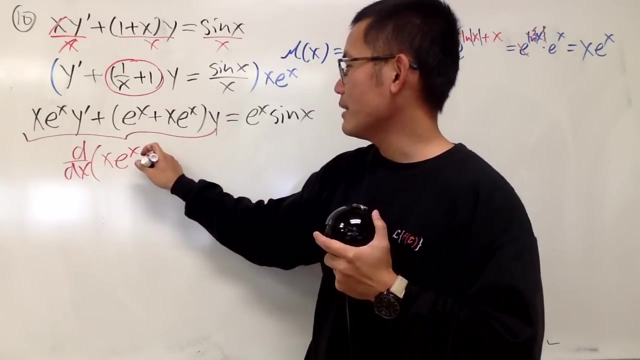 So I will actually write this as e to the x, first Cancel, and then we'll have the sine x, Like that. Okay, so the left-hand side: yes, it's a derivative of a product. It's going to be the x e to the x times y. 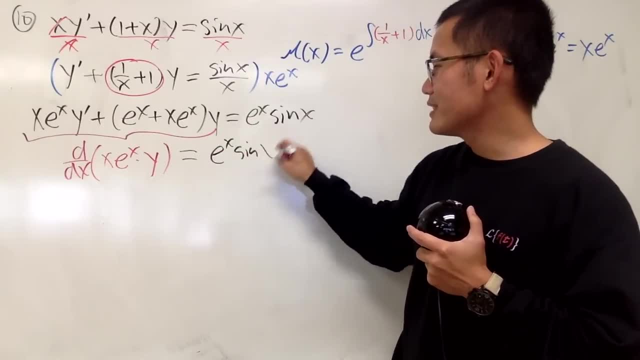 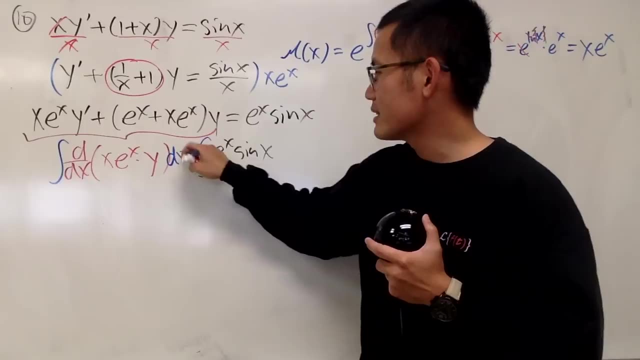 And then the right-hand side is still just Just the right-hand side, e to the x times sine x. And then, of course, we are going to do the integrals on both sides: Integrating, integrating dx, this, dx, that. 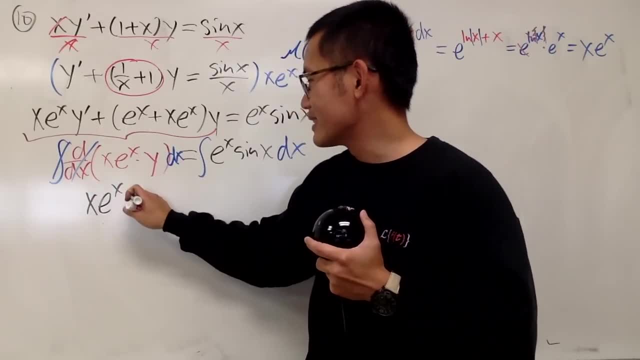 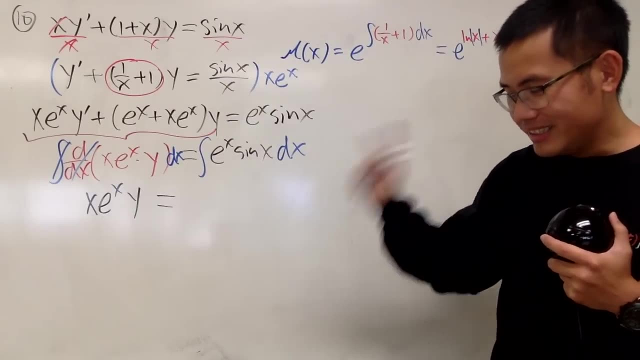 The left-hand side is easy because you just write it down: x e to the x y. But the right-hand side, yes, we have to do integration by parts, with partial, With DI method, and this, right here is a repeating situation. 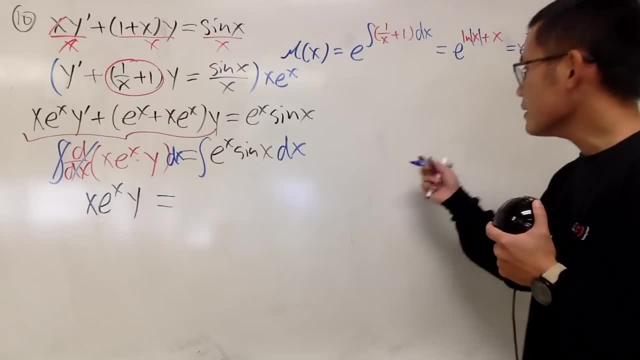 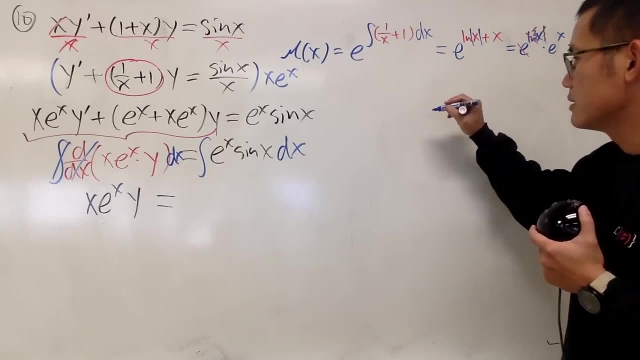 So let's go ahead and do that right here. So let me put this down here. Let's see, let's see, let's see. I should have a space right here d and also the i and plus, minus, plus. 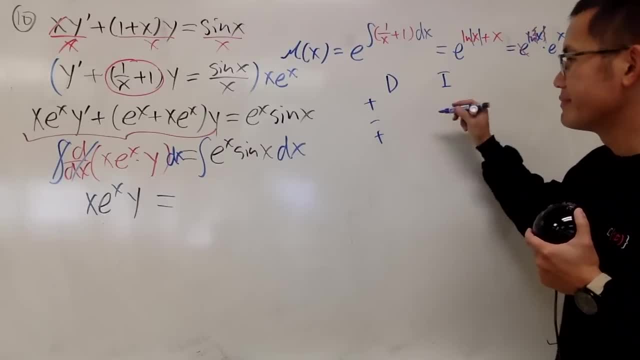 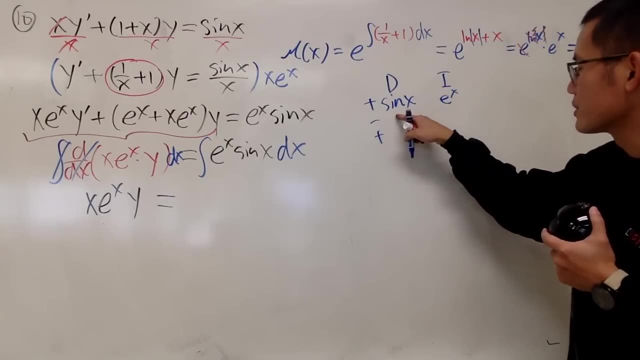 I'm going to be differentiating sine x. Why? Because I like to do the trick. It's easier to think that way, but it doesn't really matter, because both of them will give you the same result if you switch the word. Anyway, differentiating sine x, you get cosine x. 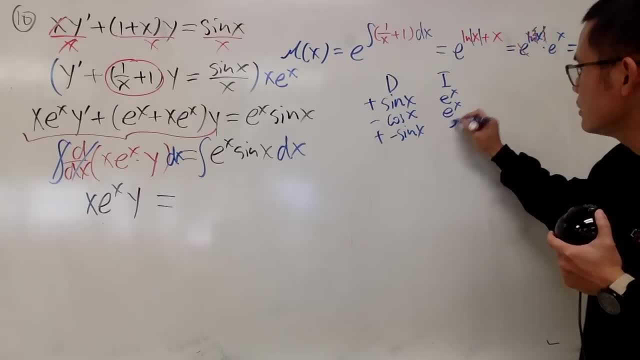 Do it again, you get negative sine. So you see It repeats e to the x, e to the x, all that, This, this, yeah. So, with this being done, this means the integral of e to the x, sine, x, dx. 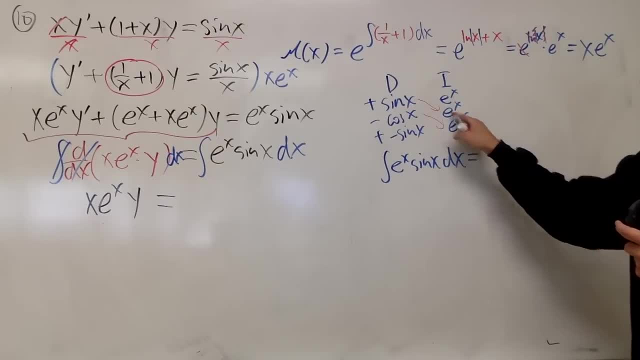 This is equal to the following: First part of the answer is e to the x and that, so I'll just write it as e to the x sine x. Second part of the answer is this and that It's negative. so it's negative: e to the x cosine x. 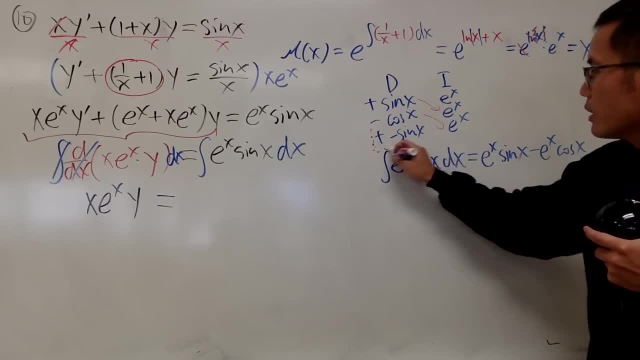 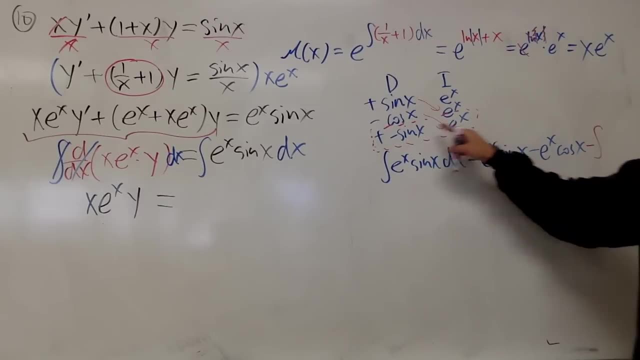 But don't forget the third row. when you multiply by a row, this right here is still an integral. So pay attention, This is negative integral and when you multiply, this is e to the x, sine, x, dx. All right. 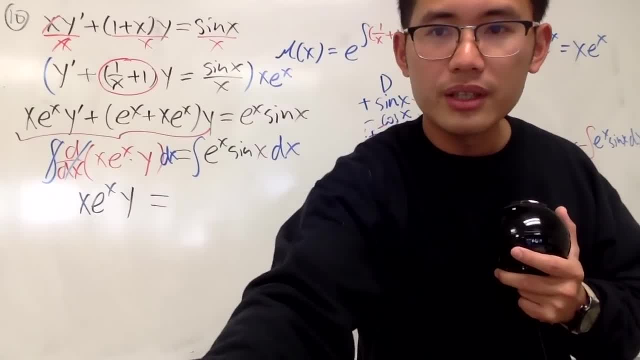 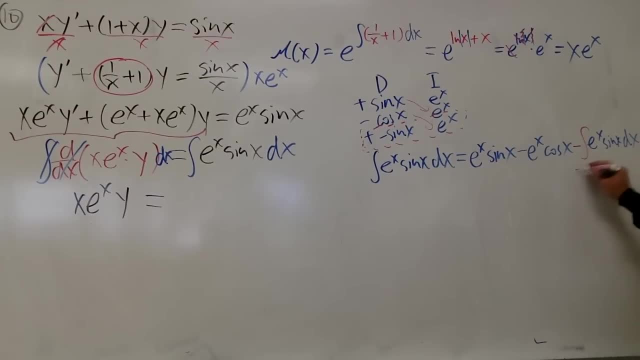 So this right here is a repeating situation like that. So what we'll do is we'll just bring this to the other side. So you just go ahead and add this on both sides: integral e to the x sine x, dx that, so they cancel. 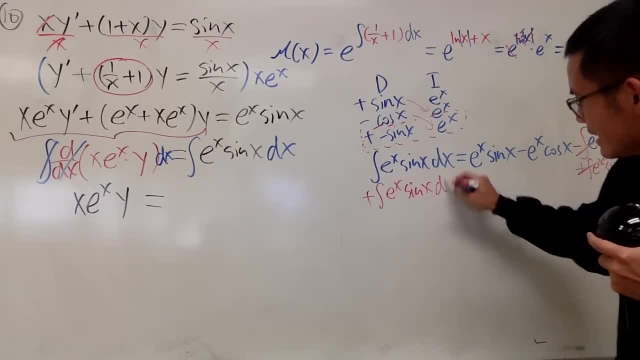 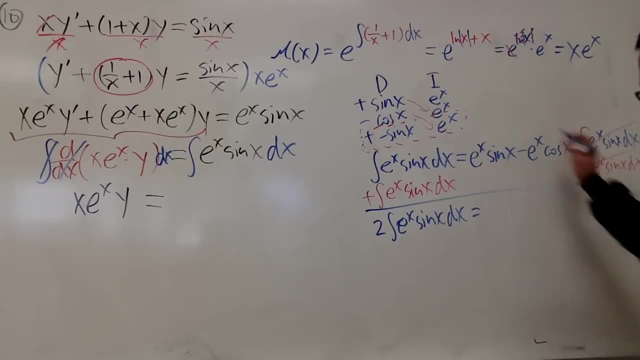 And then just go ahead and do that, Do the same thing again like this, And then you get two integral e to the x sine x. dx is equal to all this, which is e to the x sine x minus e to the x cosine x. 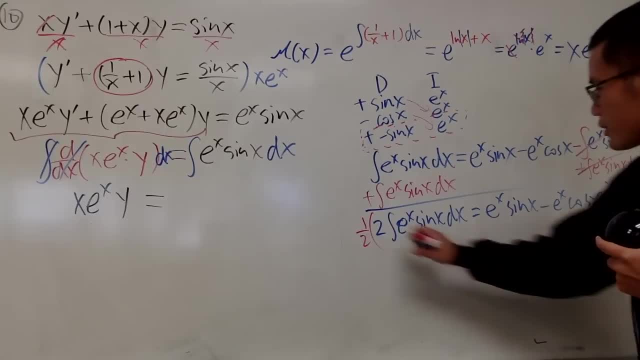 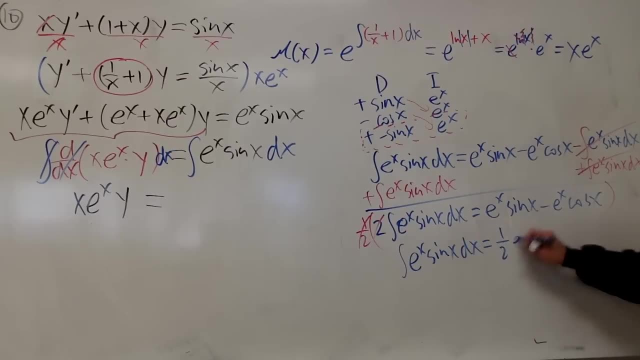 And then in the end, of course, multiply everybody by one-half so that you actually get the answer. So finally, integral e to the x sine x dx is equal to one-half e to the x sine x, and then minus one-half e to the x cosine x. 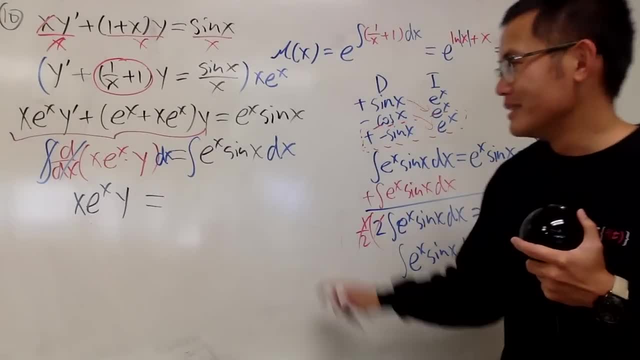 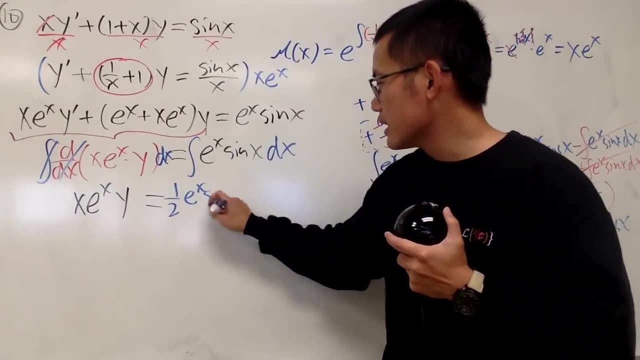 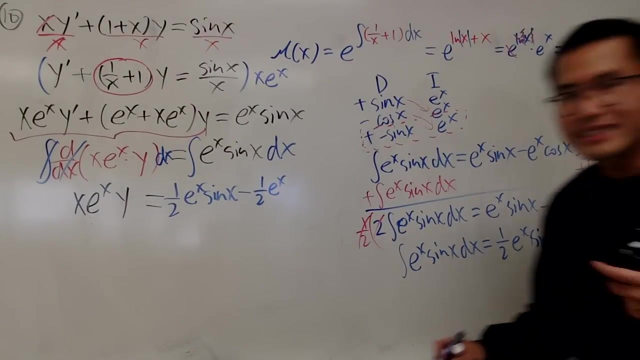 And don't worry about the plus c, because this is not the main deal. This is So anyway, this right here is equal to that. So I'll just put this down right here for you guys: One-half e to the x, sine x, minus one-half e to the x, cosine x. 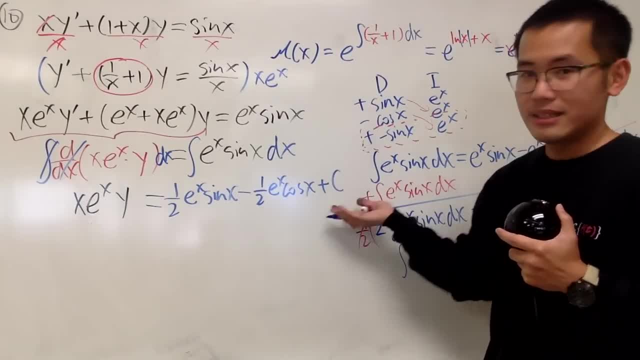 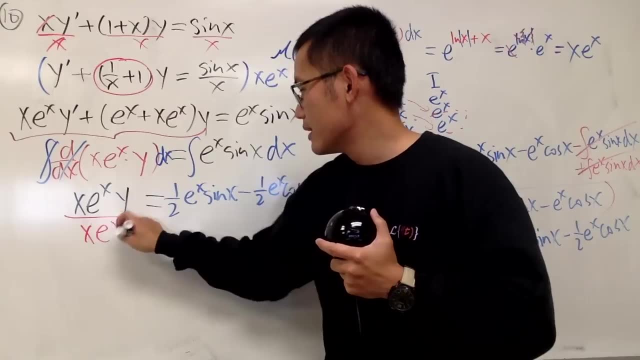 Yeah, And then here I'll put down the plus c, because, as I said, this right here is the main deal. Okay, Then what we'll do is, of course, just go ahead and divide everybody by x. e to the x. 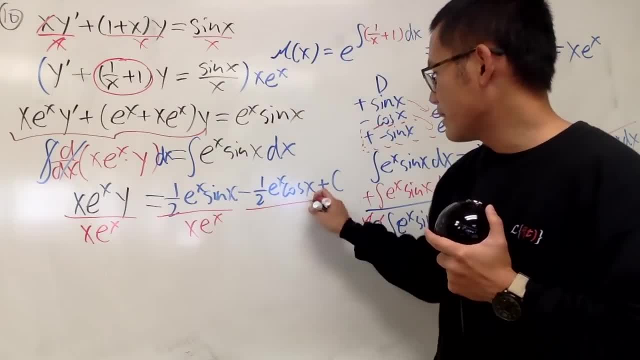 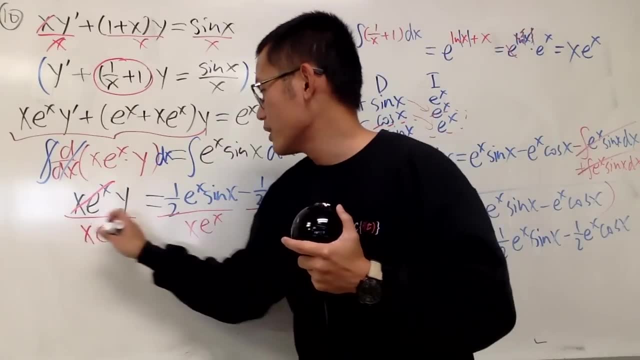 So divide everybody by x e to the x, Divide this by x e to the x, And also divide the c by x e to the x. This is a very common mistake that people just don't forget, People just don't remember. 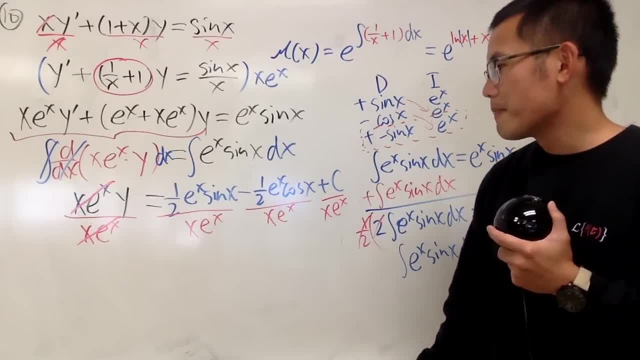 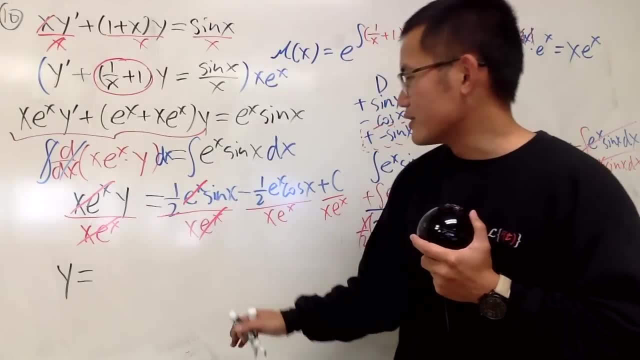 People just tend to forget this part. Anyway, we're done. Let's, of course, write down the final answer in a nicer way. Okay, So here we have the e to the x cancel, And man, we have the x on the bottom. seriously, 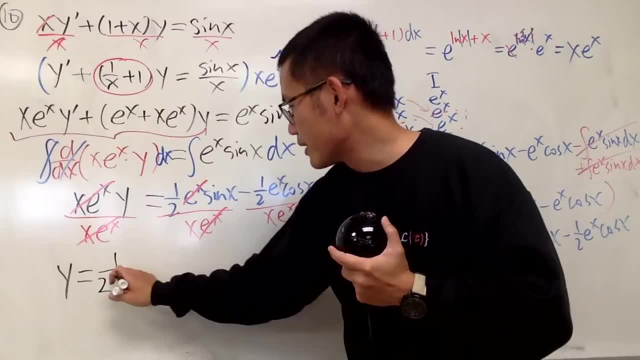 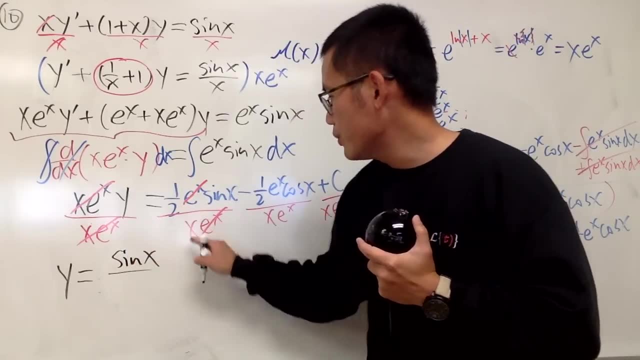 So I will just put down one over two and then the x right here, And then perhaps I will just write it as a whole fraction: Sine x on the top over two, and also the x on the bottom, Yeah, And then the second part is this and that cancel. 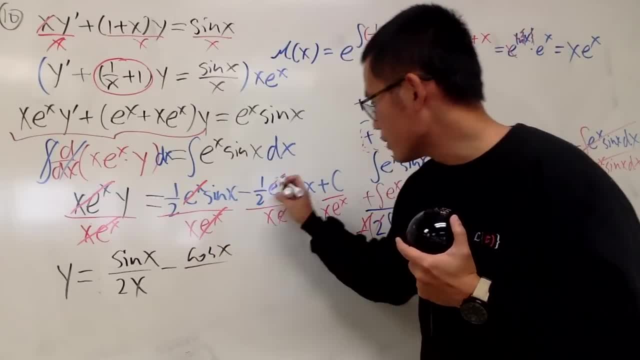 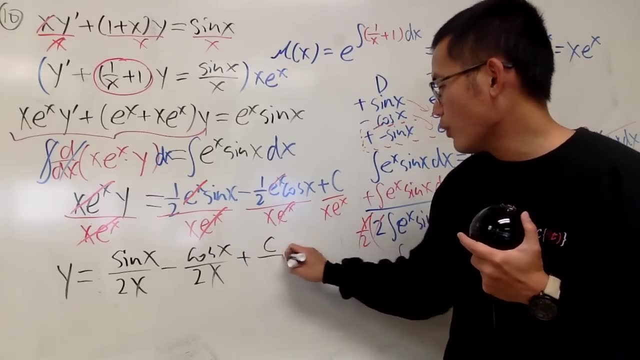 We have minus cosine, x over two and x on the bottom. And lastly, if you would like, you can put down this as plus c over x And it depends on where you want to have the e to the x. I can write it as e to the negative x. 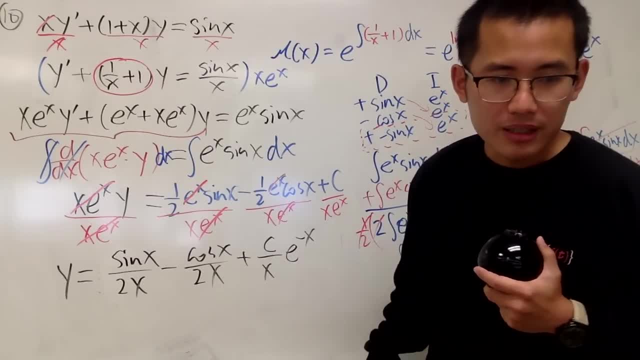 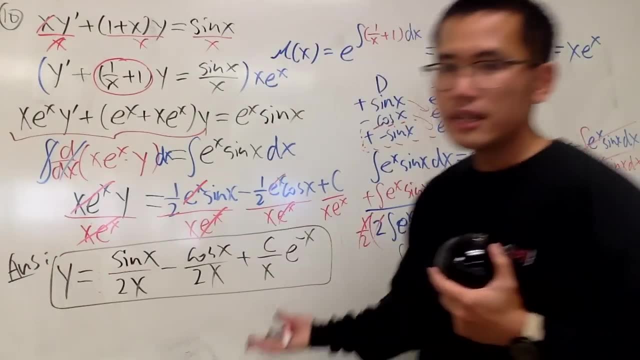 I think that's okay. How did I write it down there? Yeah, I wrote it down like that. So, yes, Here is the final answer. All right, So don't forget your integration by parts. Don't forget your integrals. 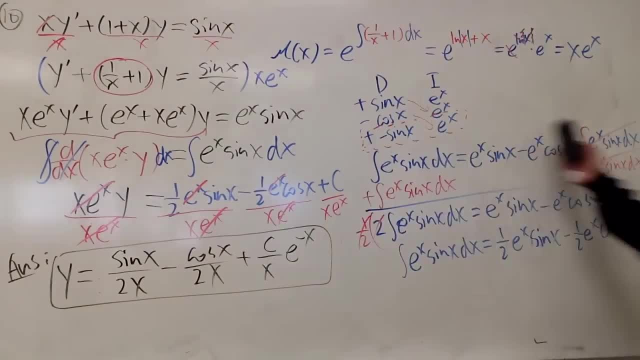 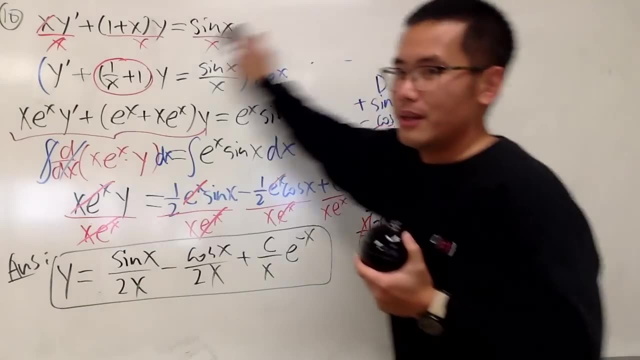 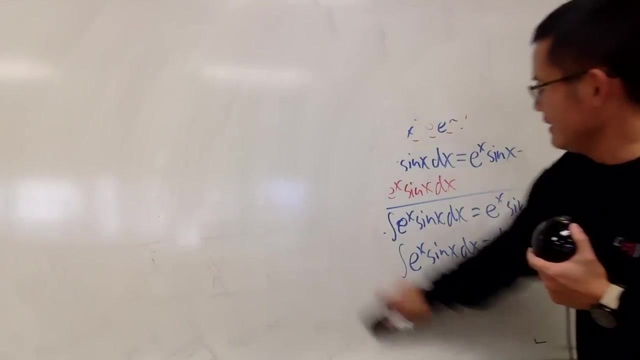 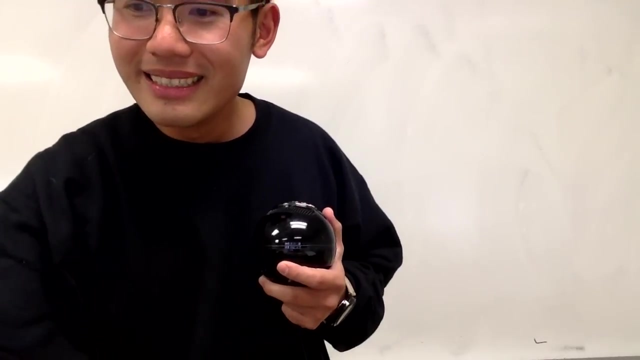 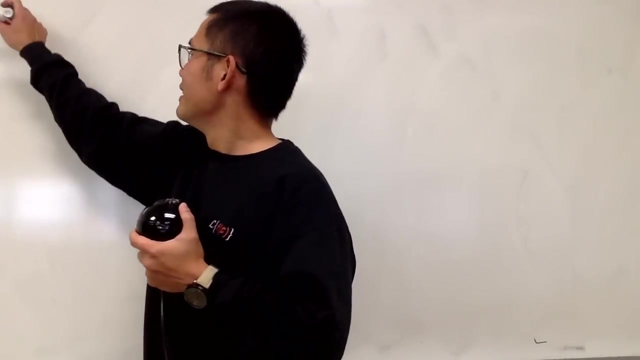 That's the prereq of a differential equation. So have a look at all this. All right, 10 questions, 14 more to go. Not so bad. Not so bad, All right. Okay, Number 11.. It's like a face. 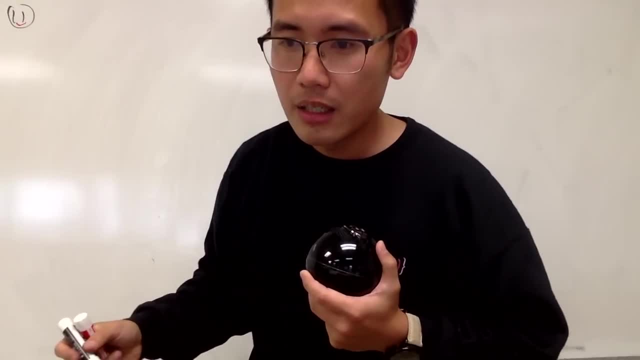 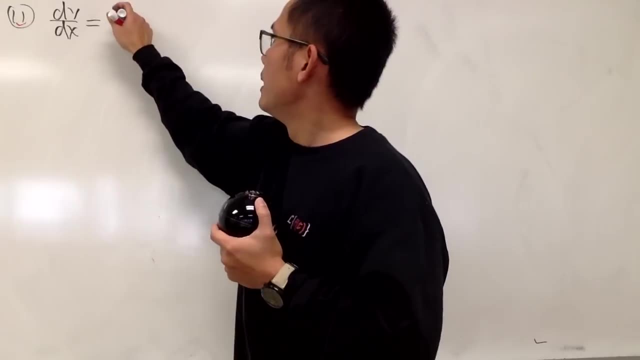 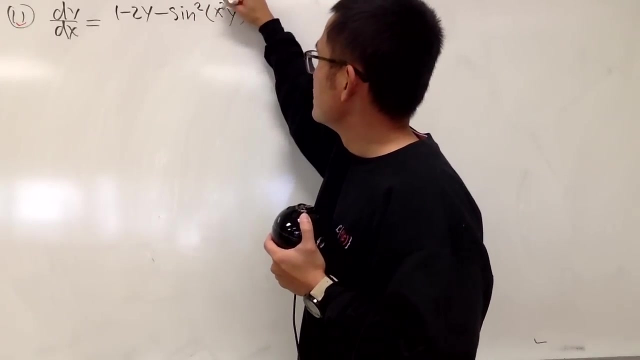 Look at that Again whenever it's number 11, give a little face. We have dy dx, It's equal to, And then we have 1 minus 2y, And then we have minus sine squared of xy, And this is x squared inside actually. 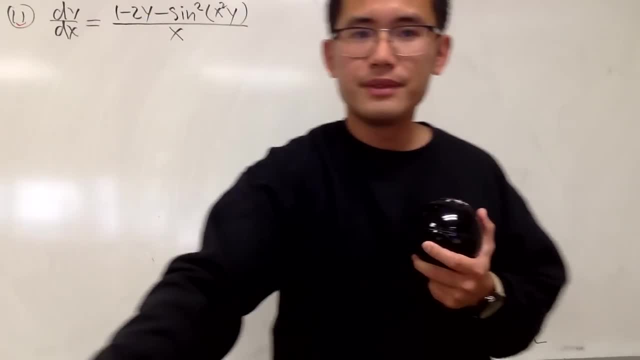 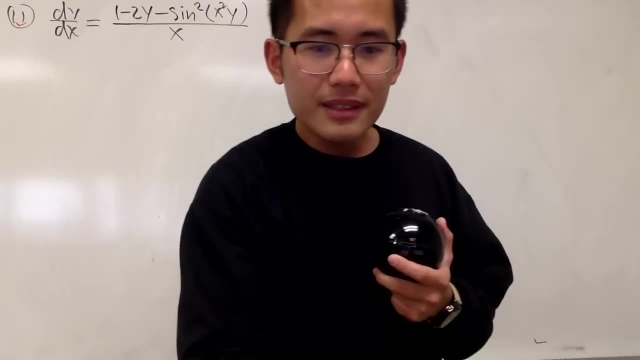 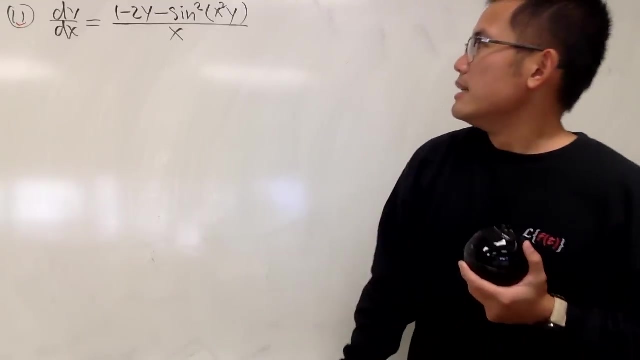 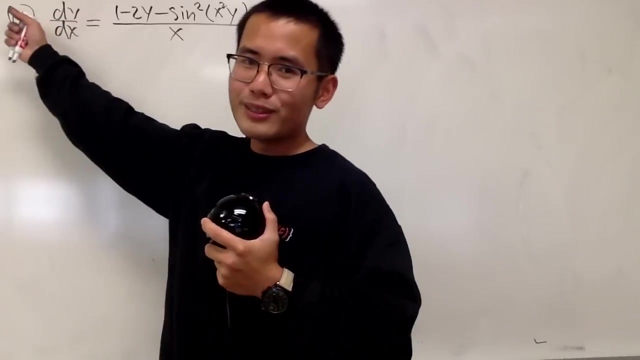 And then all over x. So that Can you do. that You can all see that, Yeah, Okay. So have a look, Let's think about it. Is this exact? You can try it: Multiply x on both sides. 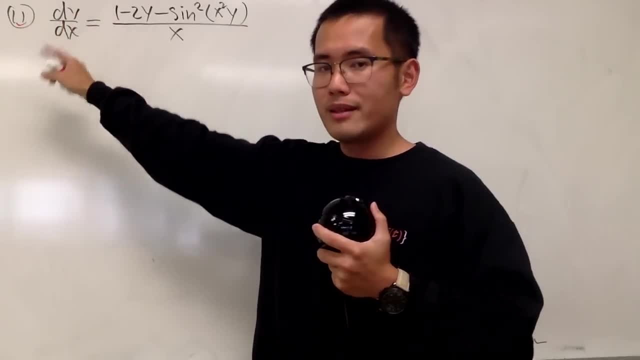 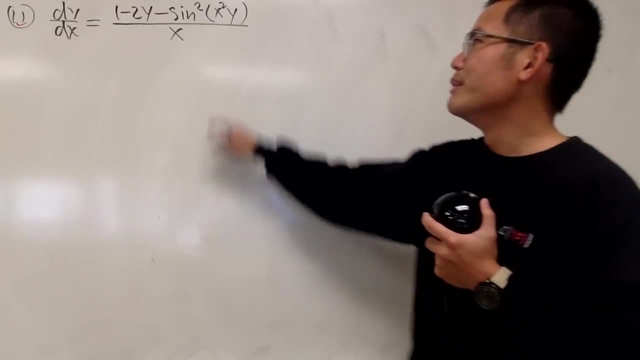 So you have xdy. If you differentiate that part with x, you get 1.. But if you have that, No, it's just not Go ahead and try it. No, Is it linear? No, Because you do have this portion right. 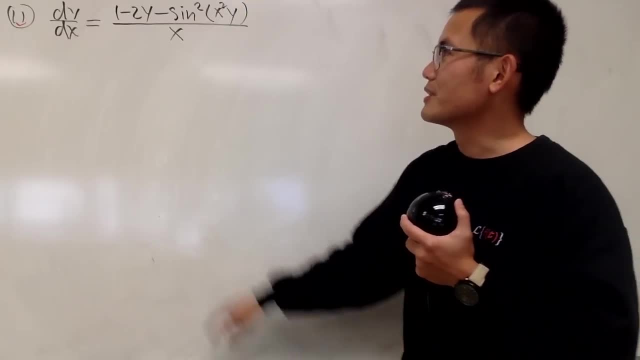 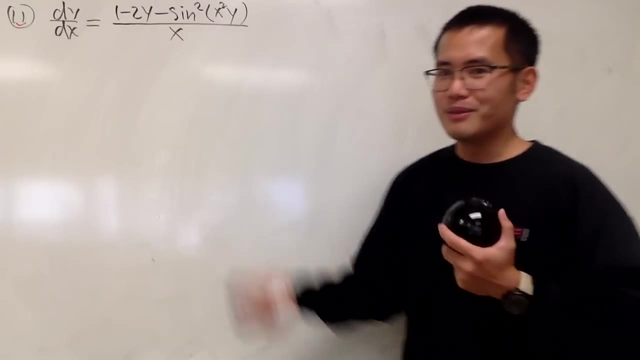 So no good. Just to say, though, if you don't have this portion, you have the y to the first power. So maybe linear, You know it's linear, But if you don't have this portion, maybe this: it would be super hard. 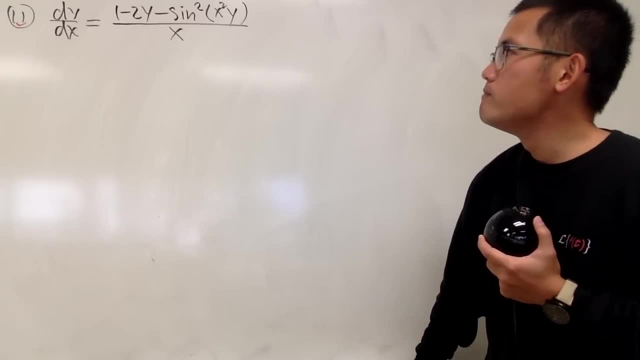 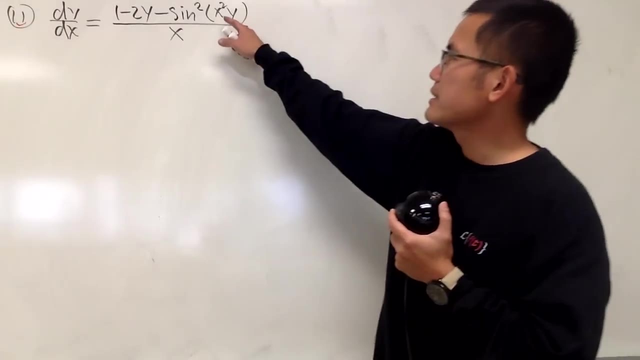 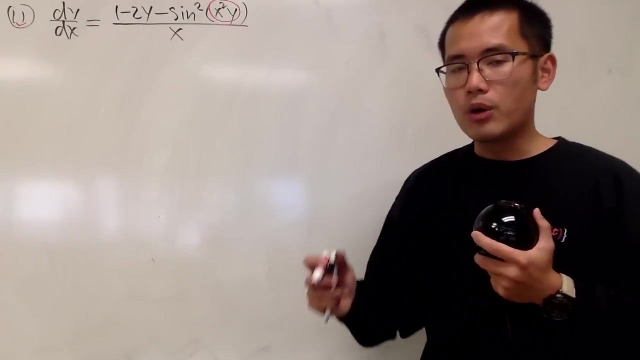 I don't know. Hmm, Well, this right here, maybe we have to do some substitution, because we have both the x squared y inside of the sine, Yeah, So maybe it's a good idea to pick that to be our new letter, new function. 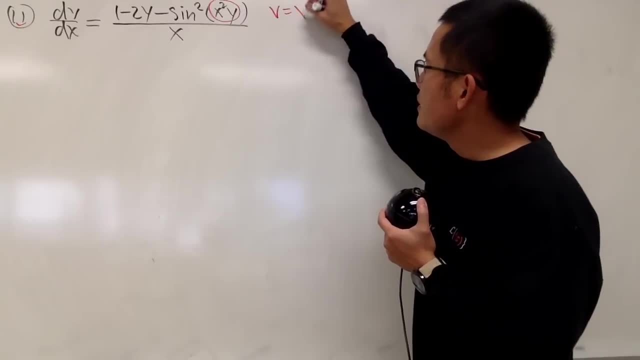 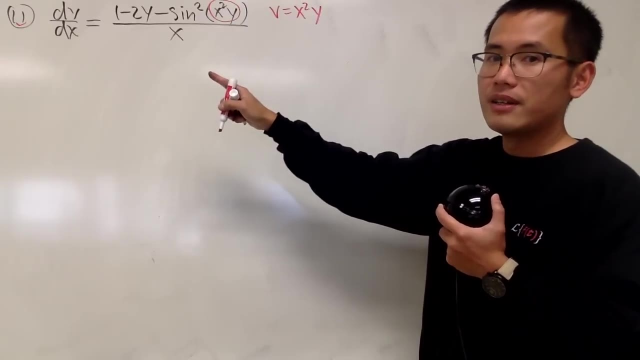 So let's go ahead and do that. Call this to be v. v is equal to x squared times y, And what we'll do is: I want to get the dy dx by itself. Yeah, So let me actually just divide this on both sides. 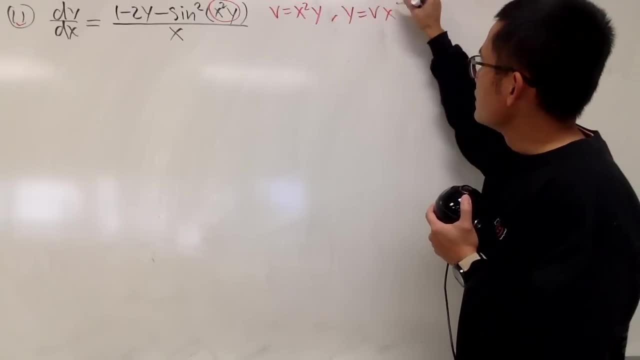 So I'm looking at this as y equals v, x to the negative 2.. Let's just look at it like this, Because this way I do not have to use the quotient rule. We can just use the product rule. Yeah. 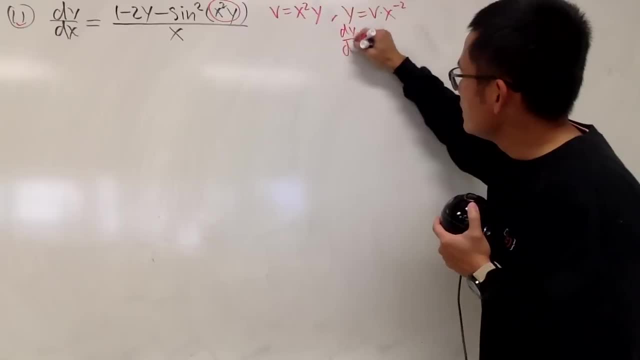 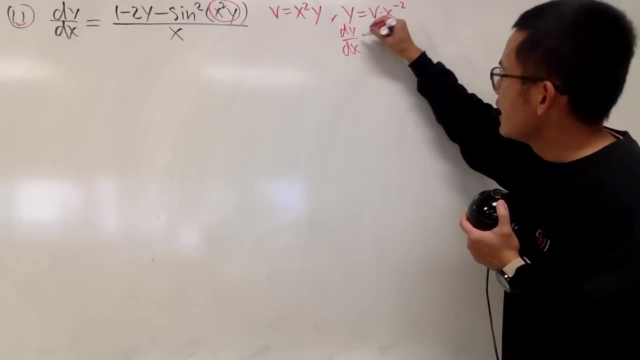 So go ahead and do that. So I want to get the dy dx Product rule in action, Differentiating. Well, keep the first function, which is v, And then differentiate the second. Bring the negative 2 to the front. 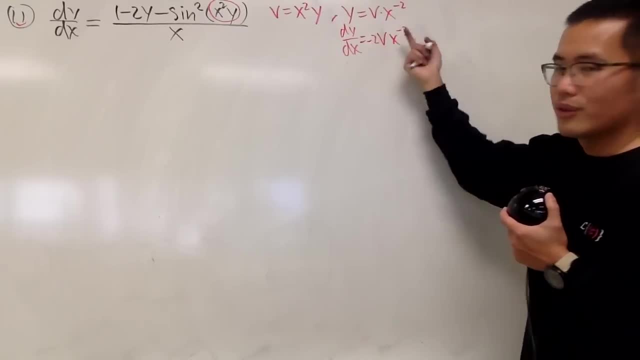 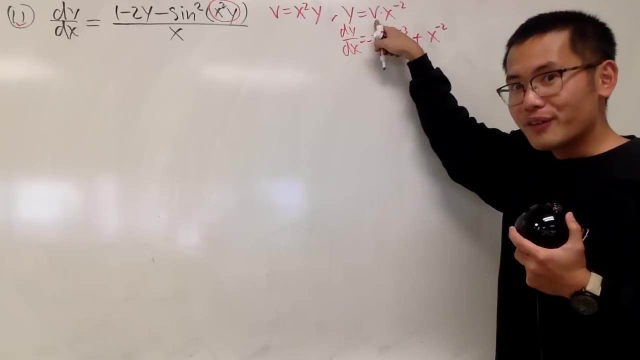 And then x to the negative 3.. Now I remember to bring the negative 2 in the front. Yeah, Anyway. And then we add the second function, which is x to the negative 2.. And then the derivative of the first function is dv, dx. 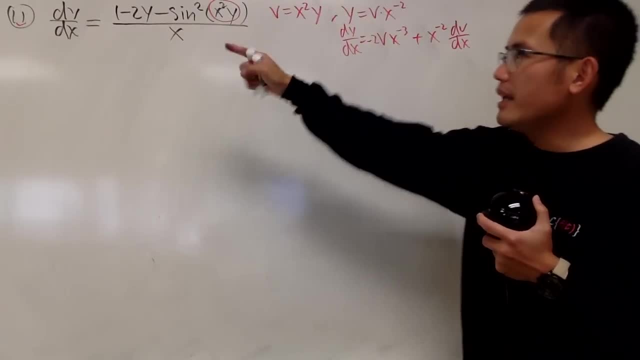 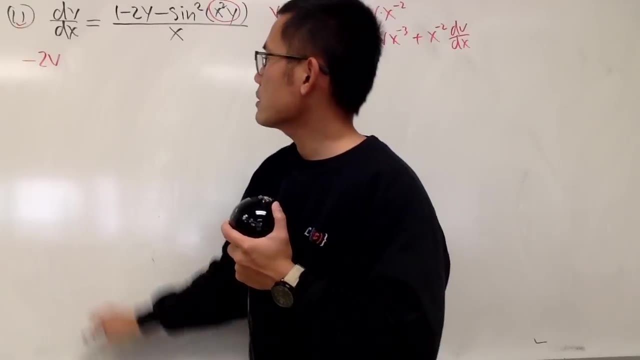 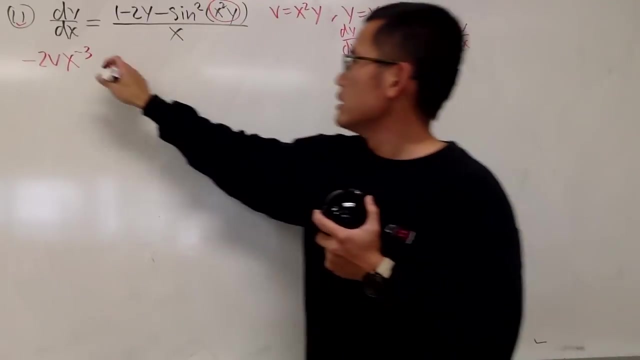 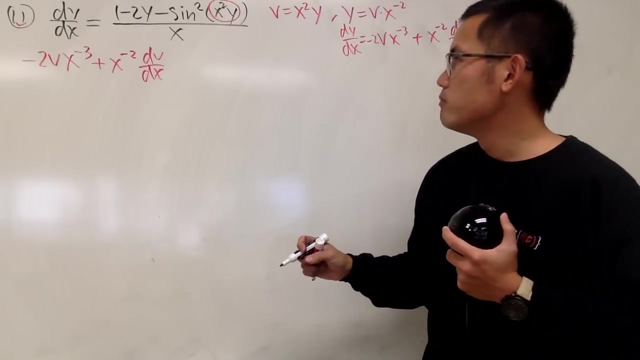 Like this. Very good. Now I'll put this right there. So we have negative 2vx to the third power And then plus x to the negative 2 dv dx. That's for dy dx. Okay, Technically, you can do whatever substitution that you want. 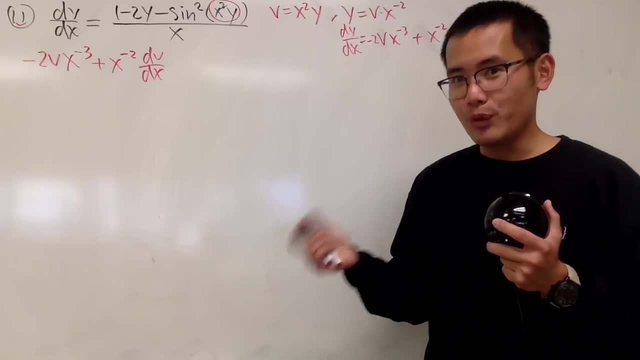 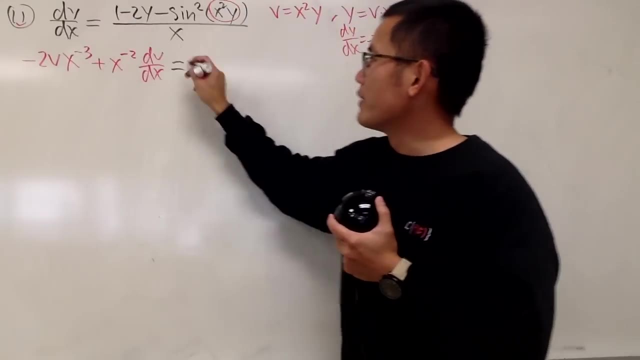 It's just that if it works or not, right. So let's see on the right-hand side. Hmm, Let me just split the fractions and hope for the best. Here we have 1 over x. Good, Here we have negative 2y over x. 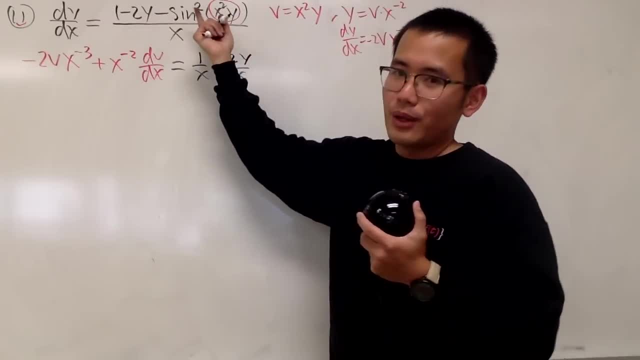 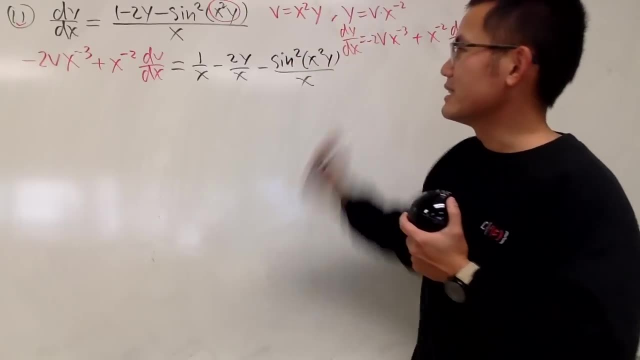 2y over x. Good Well, I don't know what will happen actually. And then next we will have minus sine squared of x, squared y over x, Like this. Yeah, To be honest with you guys, the reason I stopped my try yesterday. 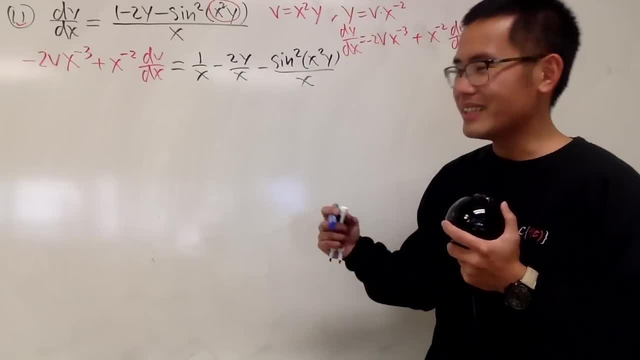 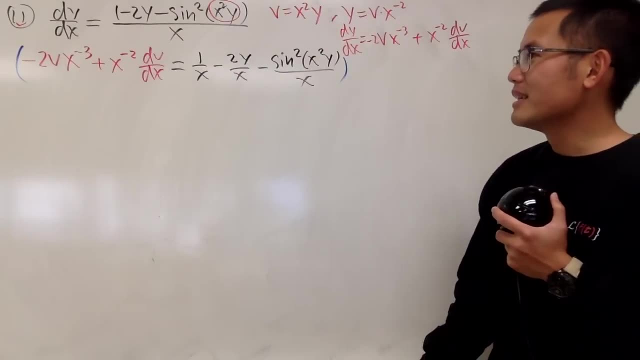 is because I forgot to divide it by x And I just made some mistakes And then it's. I just hate it. If you guys want to see it, you can go check out the other video. Anyway, Go ahead, We'll multiply. something else: 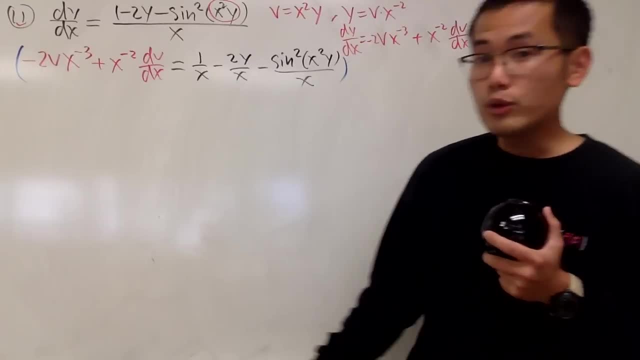 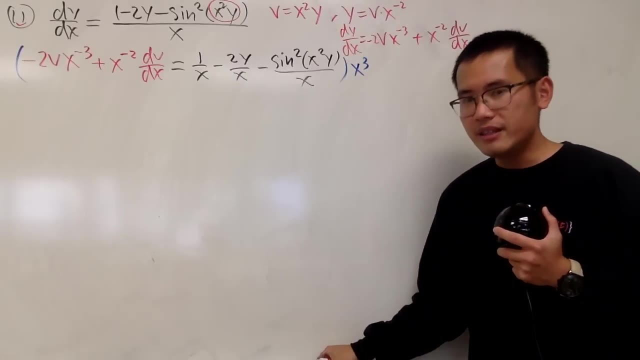 Here's the deal. We have fractions And also x to the negative 3 power. Let's multiply everybody by x to the 3rd power, So we can clean up the negative exponents and also the fractions. So have a look. 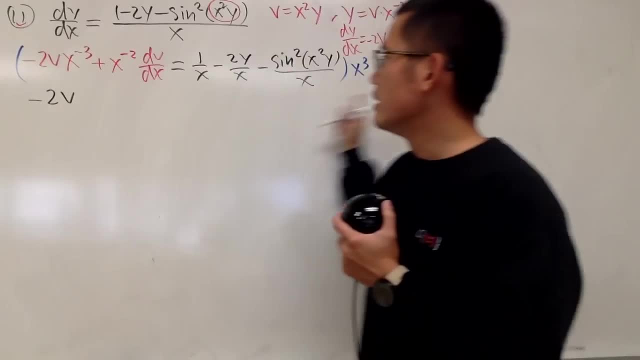 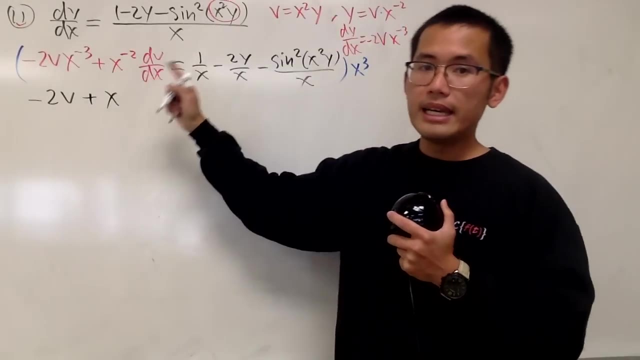 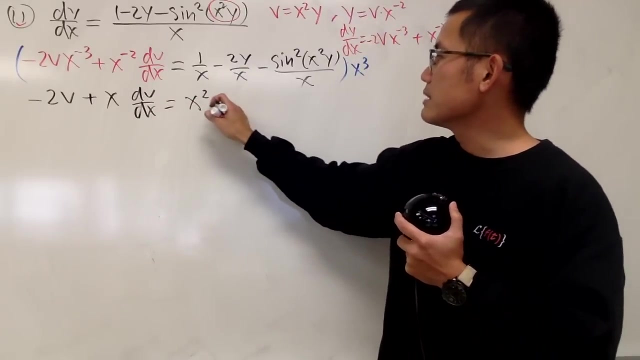 This times that we get negative 2v, This times that we get plus x, Huh, Plus x, And then dv dx, This times this is x squared And this times this is minus. We have x squared, huh. 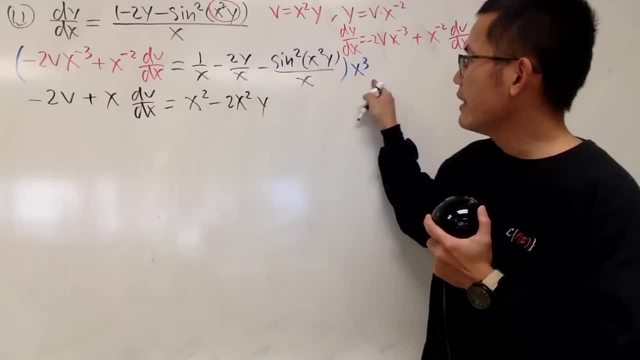 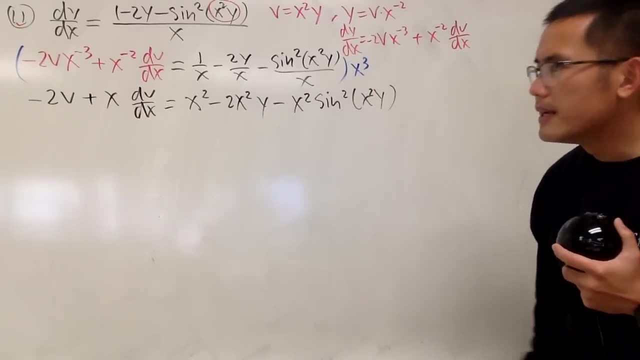 We have 2x squared, right x squared, and then the y, And then we have minus x squared, And then this is sine squared: xy, x squared y. Like that Is this going to work? Have a look here. 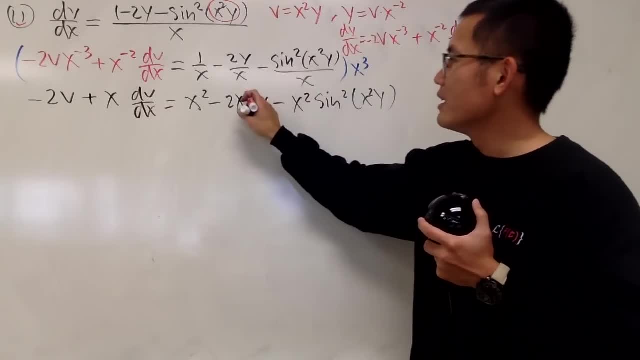 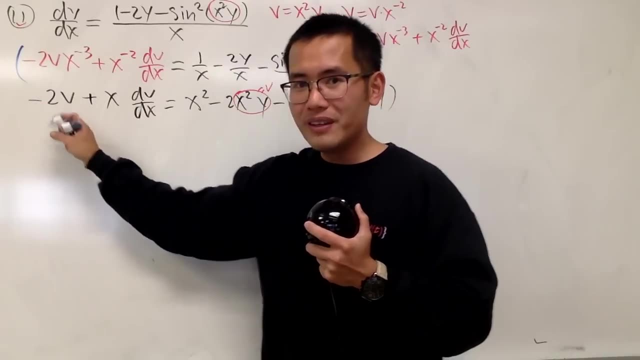 What's x squared y? That's precisely our v. Now, this right here is precisely our v. What's so good about this? Here we have negative 2v, And here we have negative 2v, So of course, this is so nice. 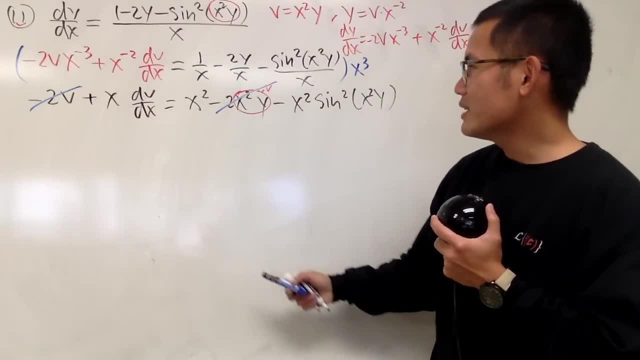 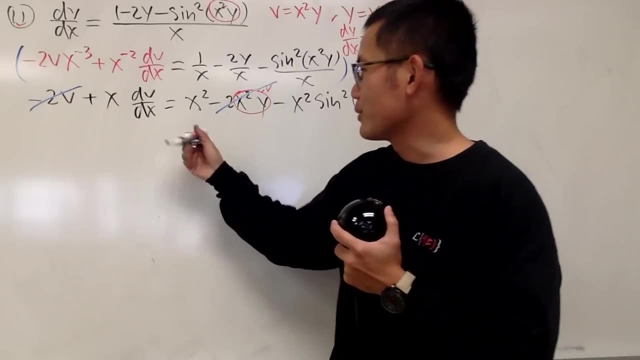 Because this and that cancel each other out. And then, as you can see, everybody now has dx, So perhaps we can just divide everybody by x, So let's go ahead and do that. In that case, well, just do that in your head. 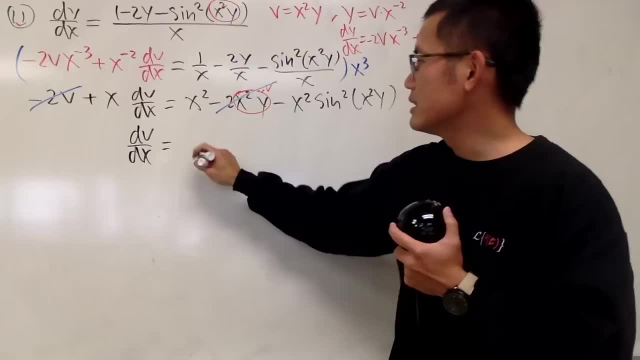 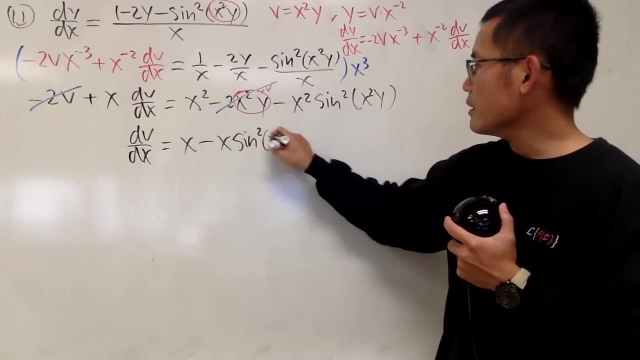 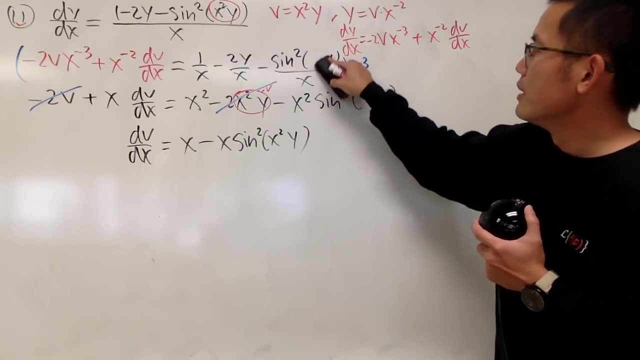 So I will just write it as: dv, dx equals. This is just going to be x. Divide everybody by x, And then this is minus x, And then we have sine squared of x squared y. Oh sorry, So this right here. the input is the v. 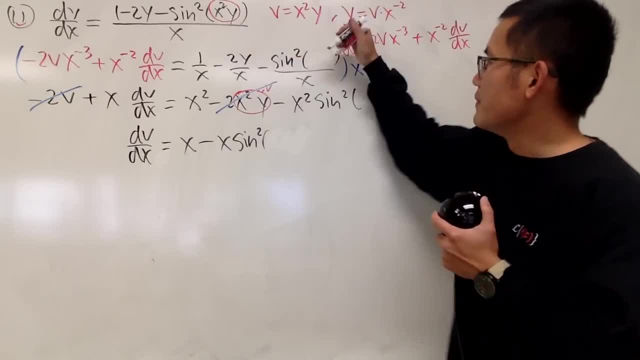 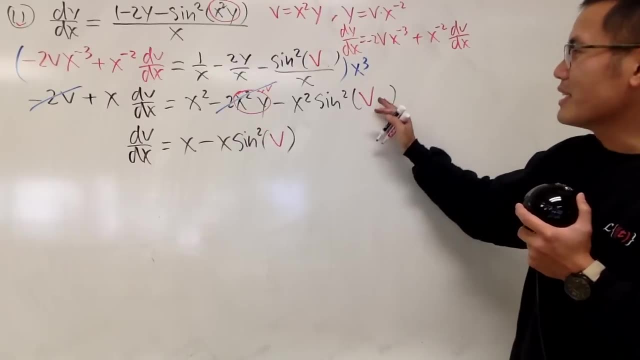 Because I want to take this to the v world. So the input is the v, So let's go ahead and write that down. Just some small mistake. Hopefully I'm not making any crazy mistake this time. So this right here is v. 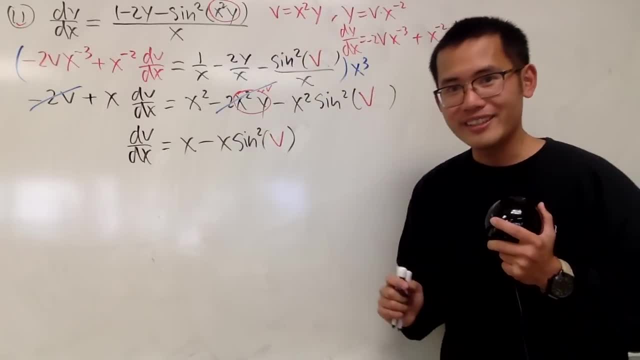 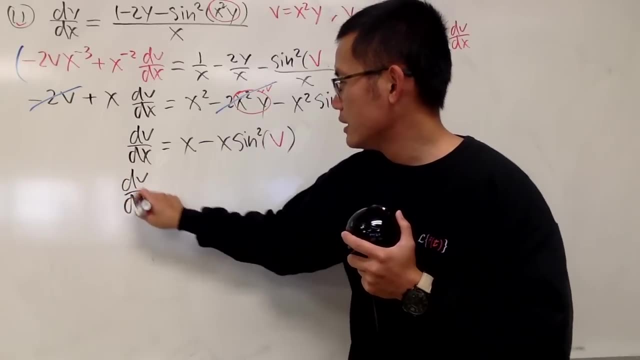 Because that was the input. This is so nice Because this is actually separable. now I can factor out the x. So we have dv, dx equals. factor out the x And then we have 1 minus Sine squared v. 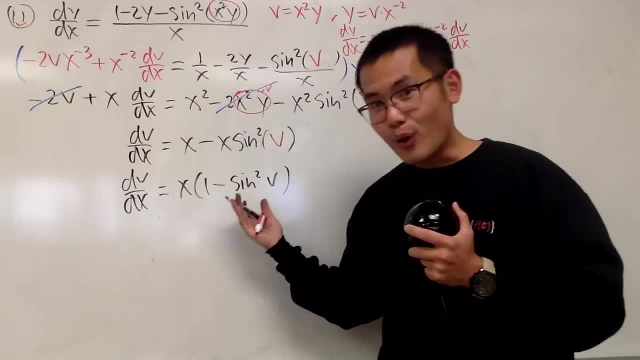 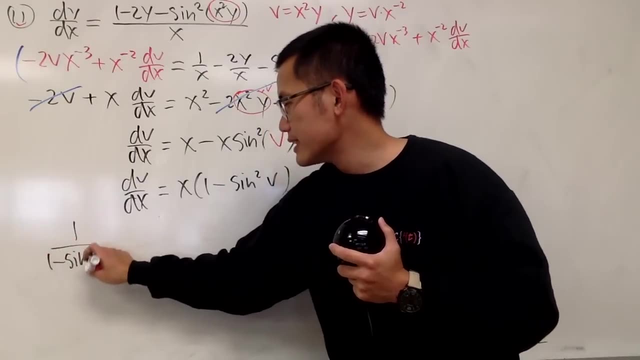 So perhaps I don't want to use the parentheses anymore, Of course, separating the variable. Put this to the other side And put the dx on the other side. We have 1 over 1 minus sine squared v dv. That's equal to x- dx. 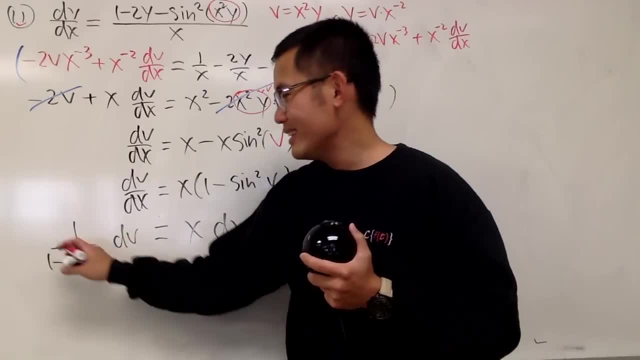 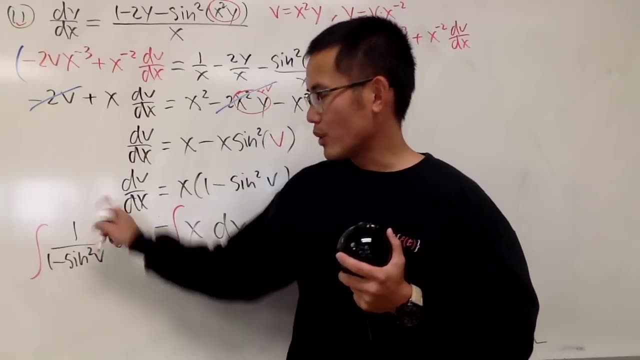 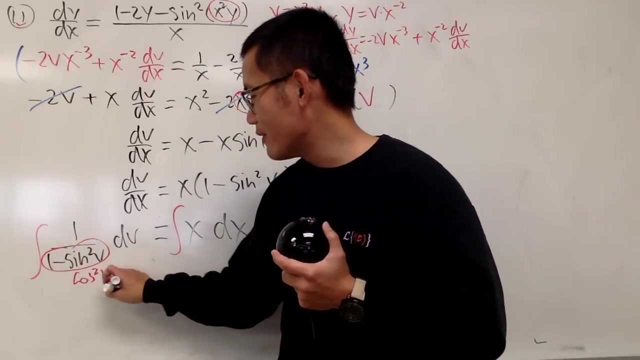 Very nice, isn't it? Now, integrate both sides. yeah, Integrate, integrate. How do we integrate 1 minus sine squared v on the bottom, Like 1 over that, This guy? it's very nicely equal to cosine squared v, isn't it? 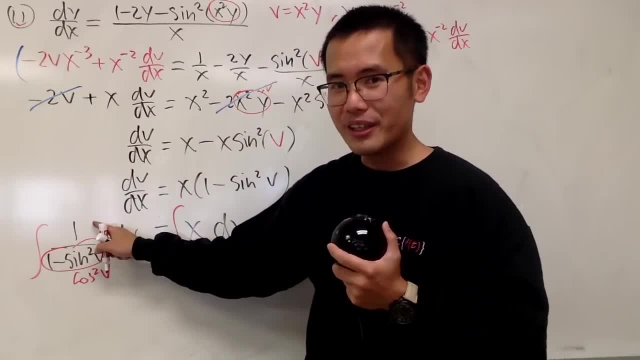 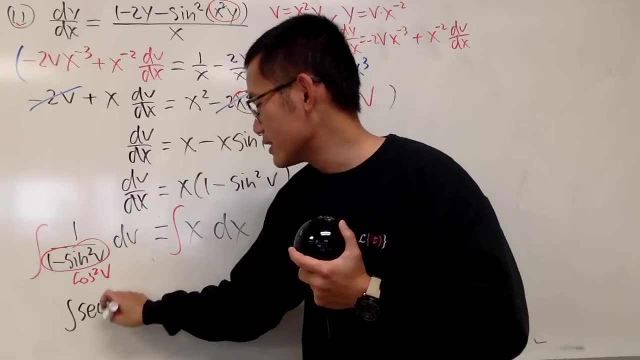 Yes, it is. So what exactly are we integrating? 1 over cosine squared v? So let me write it down. What's 1 over cosine squared v? It's just secant squared v dv. Yeah, Isn't it? 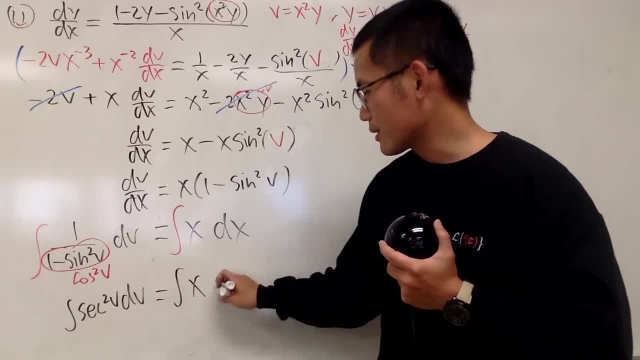 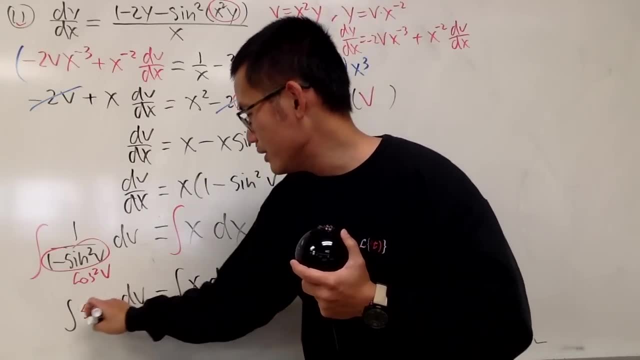 So yeah, let me just write this down. I'm not doing the integral yet, So of course you just fix the inside Like that. So perhaps make this in red To make it prettier. Okay, Integrating this, we get tangent. 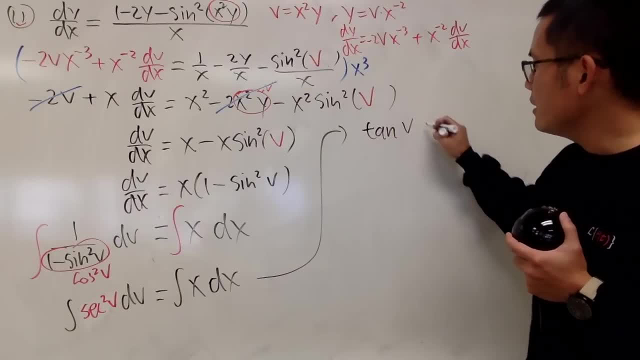 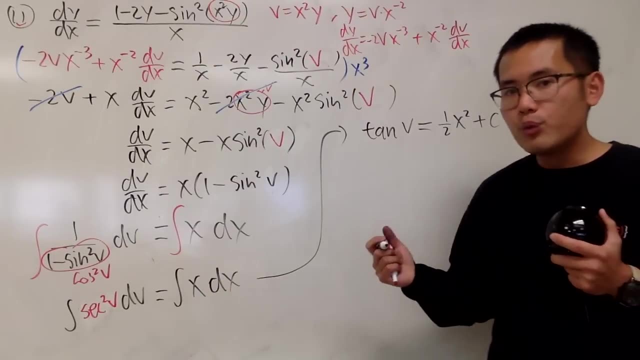 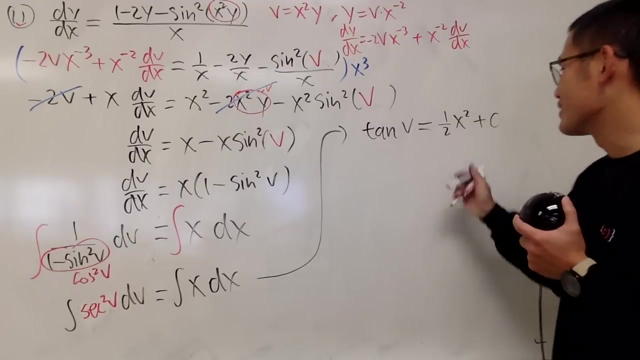 And this is the original tangent, v, And that's equal to integrating this. we get 1 half x squared plus c. Now, if you want to, well, we should get the y by itself. So let's go ahead and take the inverse tangent on both sides. 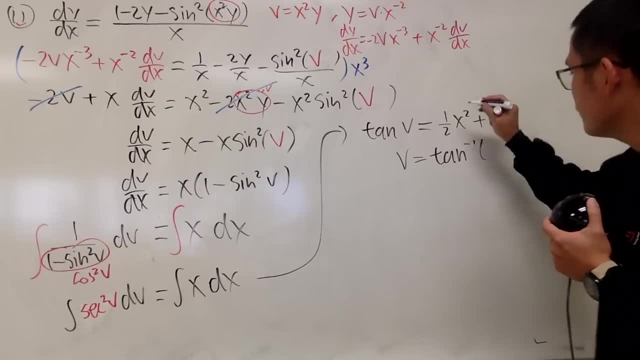 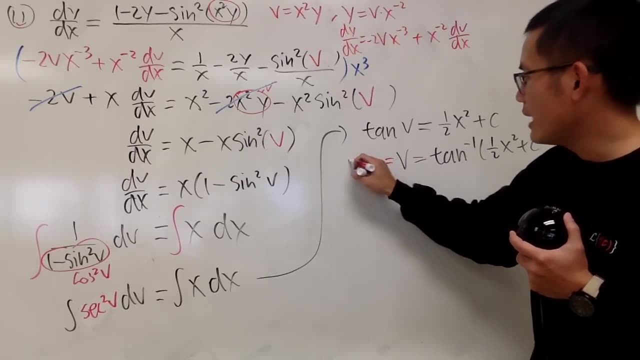 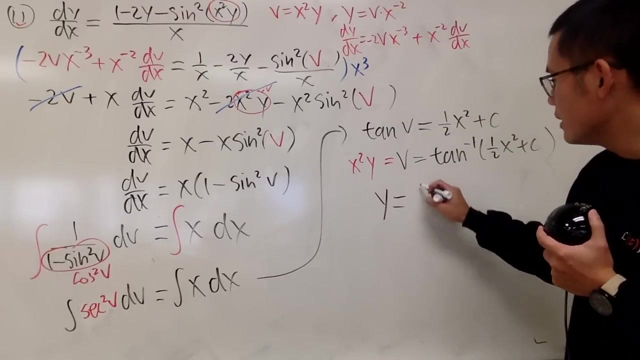 So v is equal to the inverse tangent of 1 half x squared plus c. And then v is equal to x squared times y. Yeah, So finally, of course, we can just divide the x squared on both sides, So we can see that y is actually. 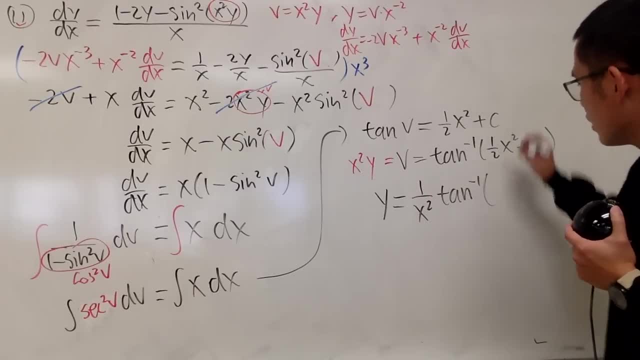 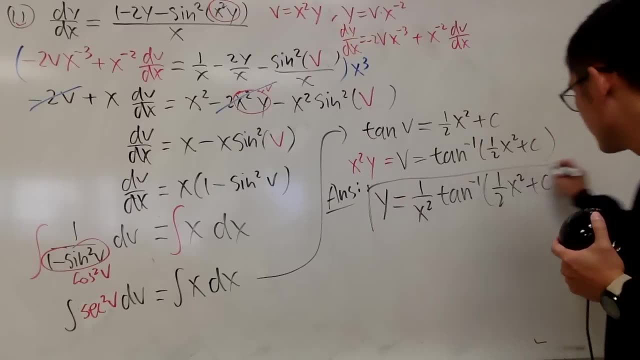 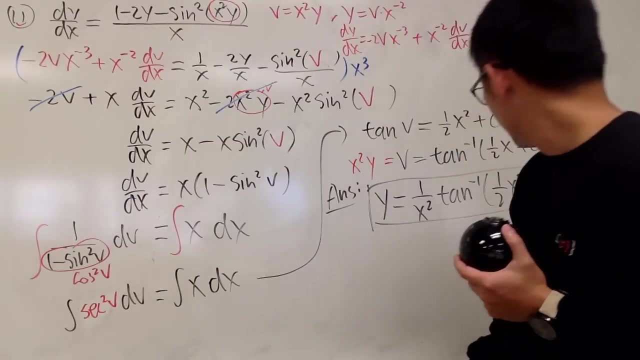 1 over x squared times the inverse tangent of 1 over 2 x squared plus c, Like this, And we are done Very good right, So check. Very good Yeah, And you might be wondering how this substitution works. 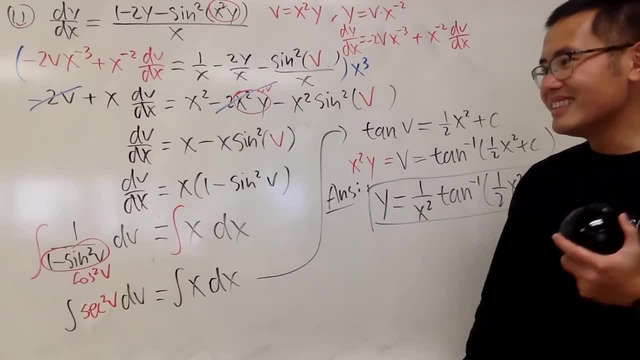 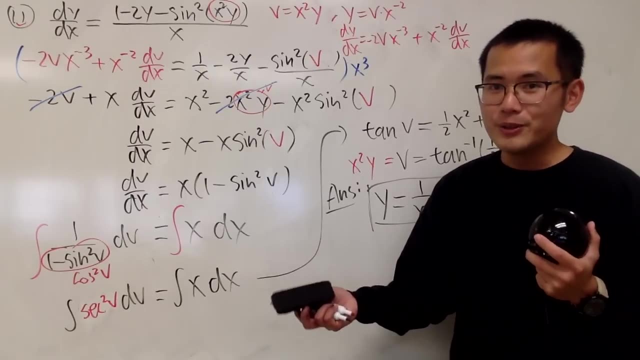 In fact, I created this equation and I will also show you guys how to create it. And yeah, you can check out my other video from three years ago where, if you guys would like, I'll show you guys how to create some exact differential equation. 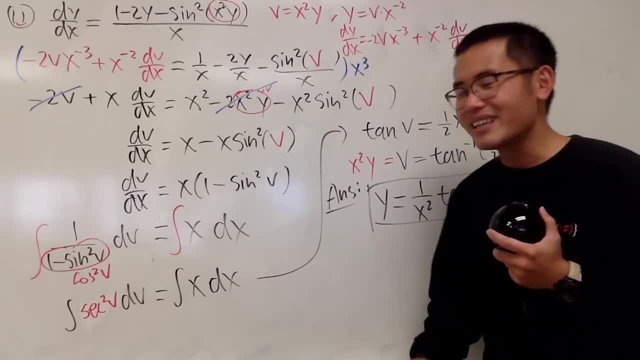 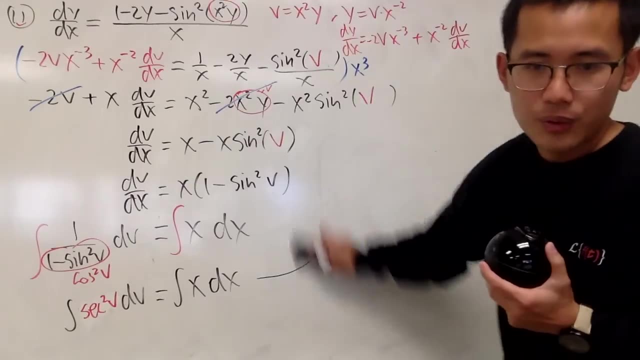 Also, I'll make another video on how to create your own differential equations and all that. If you want to see that video, just let me know. I'll do that for you guys. Anyway, this right here is it? Okay? So we have number 11.. 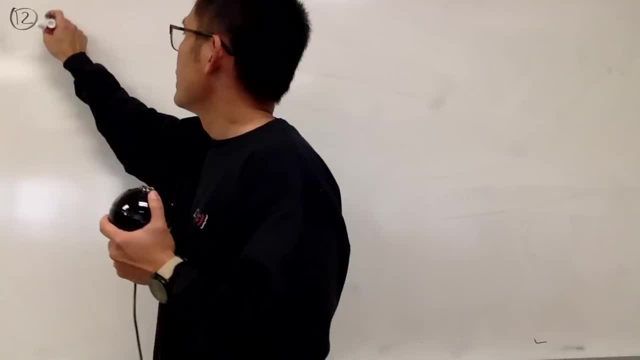 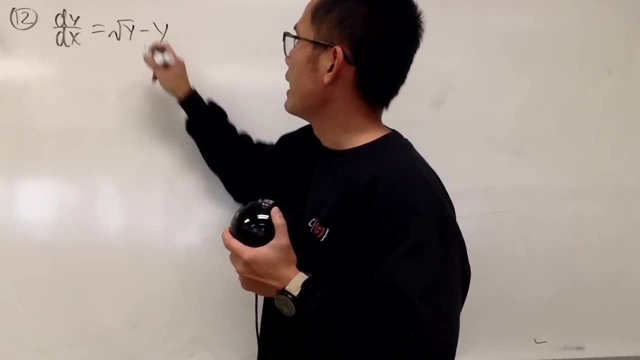 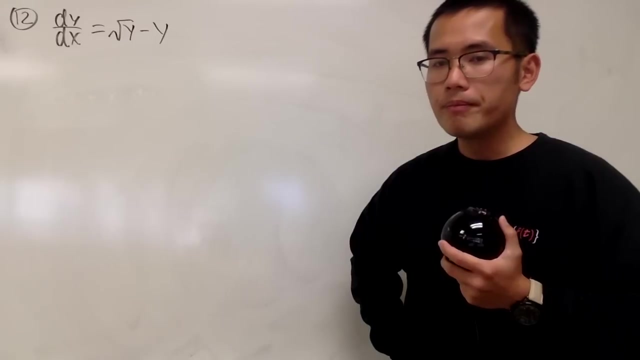 So now here is number 12.. So here we have dy, dx equals and we have square root of y minus y, like this: Hmm, This is separable. You have two ways to do it, Of course. you can separate the variables. 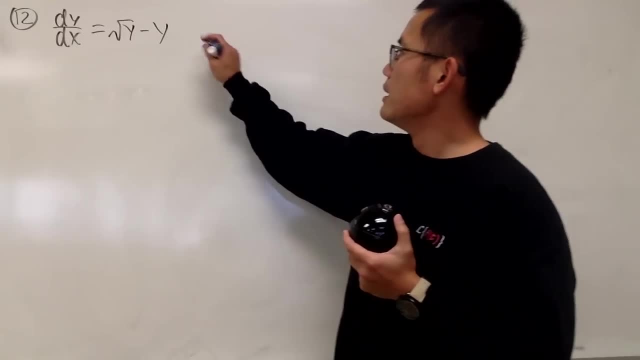 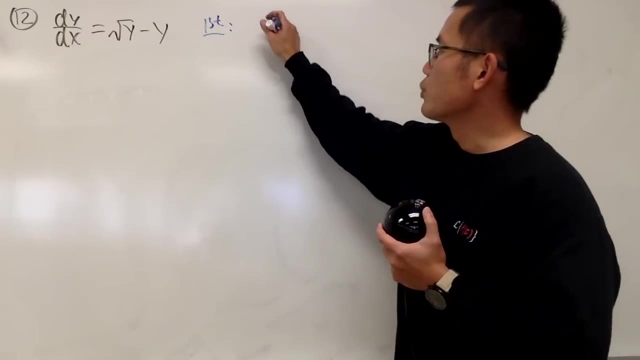 So if you would like, you can write this. So I'll just tell you guys, the first method is that you can write this. bring that to the other side. So if it's 1 over square root of y minus y, dy equals dx. 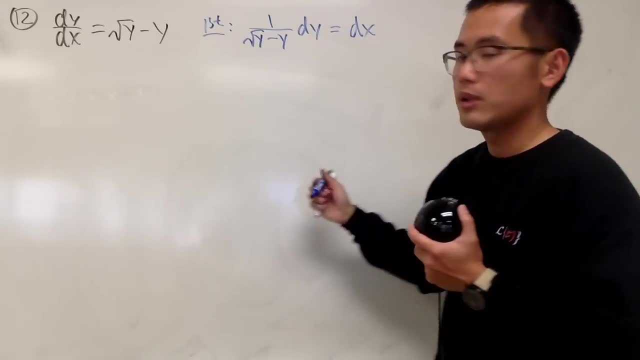 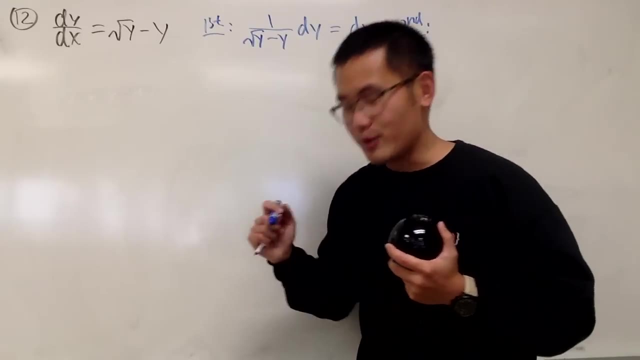 You can separate the variable and then you can just integrate both sides. And secondly, this right here, it's actually Bernoulli's differential equation as well. In that case we can bring the y to the other side and you get this. 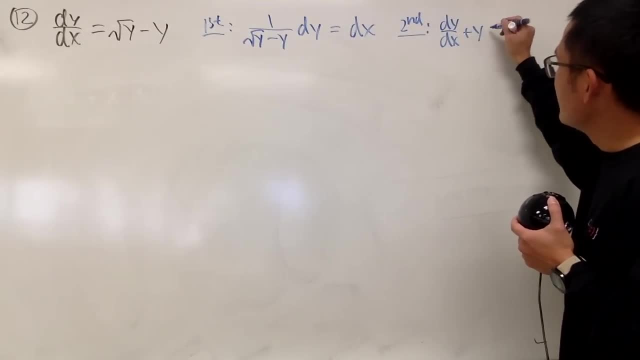 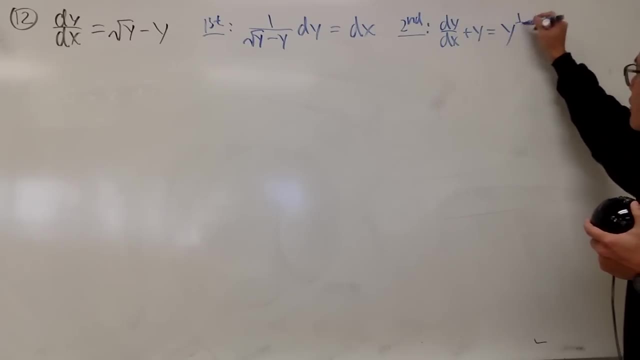 You get dy dx plus y, that's equal to y and you see the square root, which is the same as 1 half power, The square root which is the 1 half power, Like that. So it's also Bernoulli's. 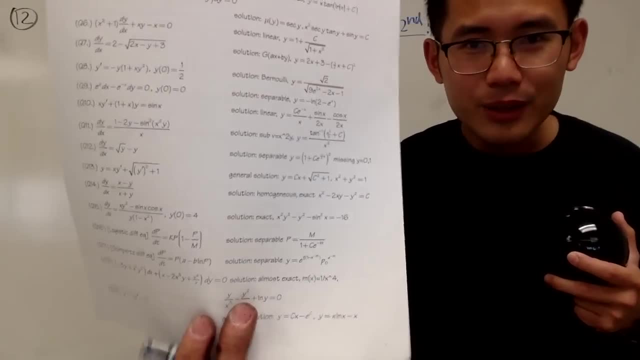 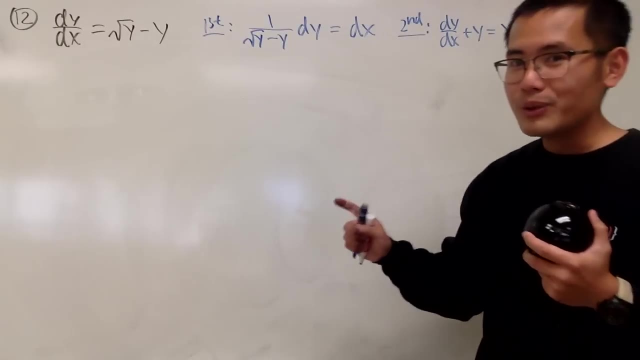 So one or the other. And on my answer key I have a note that I want to do this as a separating variable, But since I made a mistake for the Bernoulli's differential equation earlier, I will do this with the Bernoulli's differential equation. 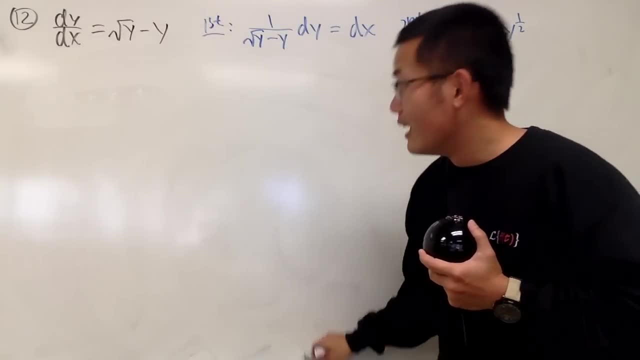 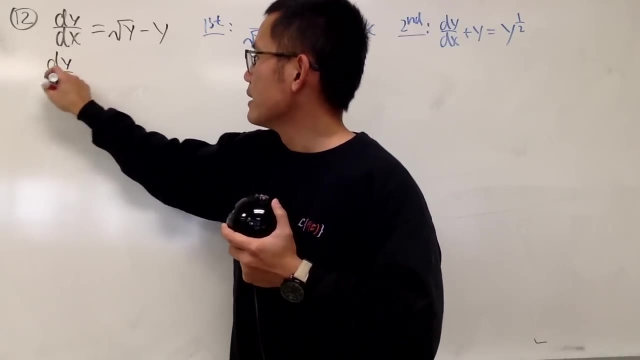 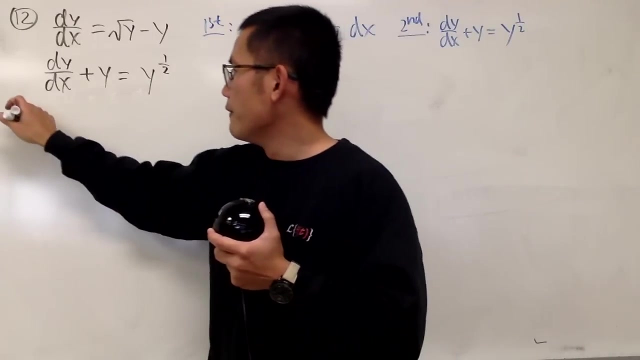 So here we go. Let's see, Right here I'll do the second way. I'll write this down right here: dy dx plus y equals: this is y to the 1 half power. Now v is equal to y 1 minus this power. 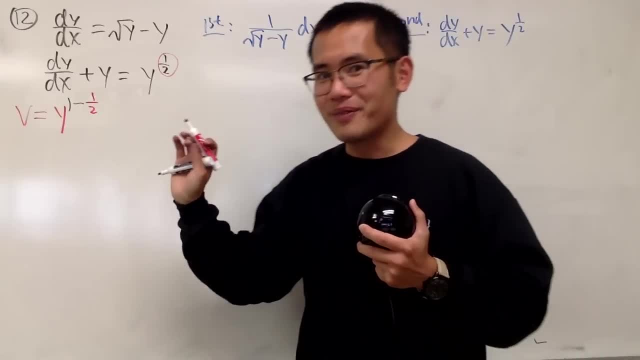 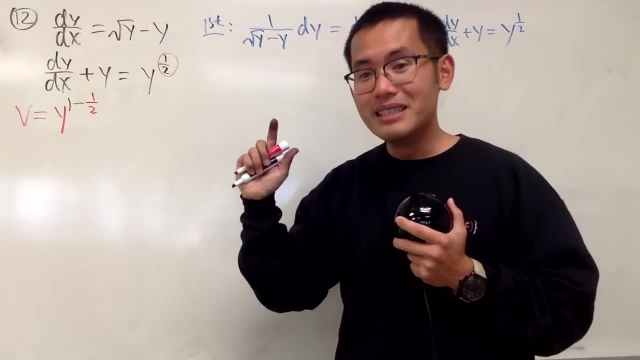 Which is 1 half. So this is the genius part of the Bernoulli's differential equation. And again, if you just work this out, you'll see that this later on will become linear. There we go, So that's why the 1 minus. 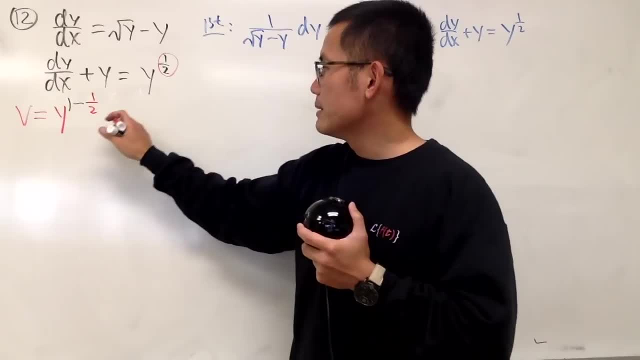 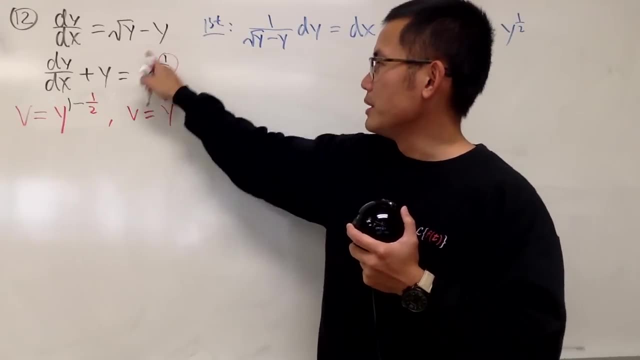 because of the power rule and all that stuff. So have a look. Anyway, let me just write this down again: v is equal to 1, minus that, It's just 1 half power. So it's not because I'm taking v to be this. 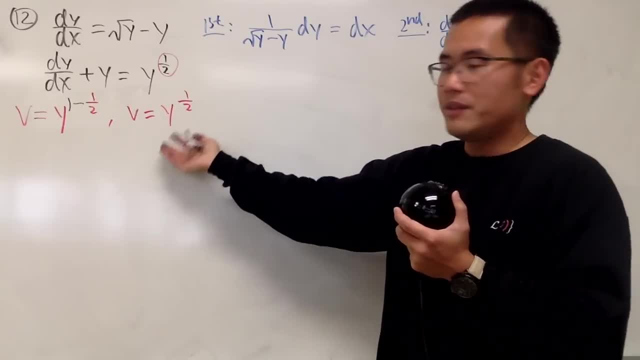 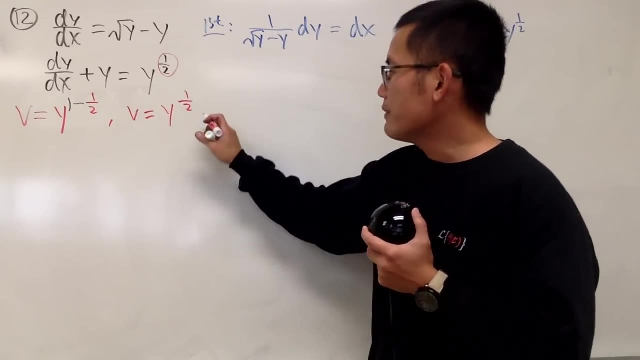 I'm actually working this out, So that's how I end up with. v is equal to y, to the 1 half power. It's a coincidence and they are equal in this case. But anyway, have a look, I will differentiate that. 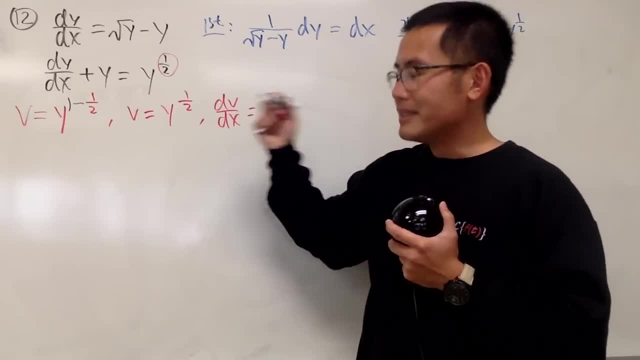 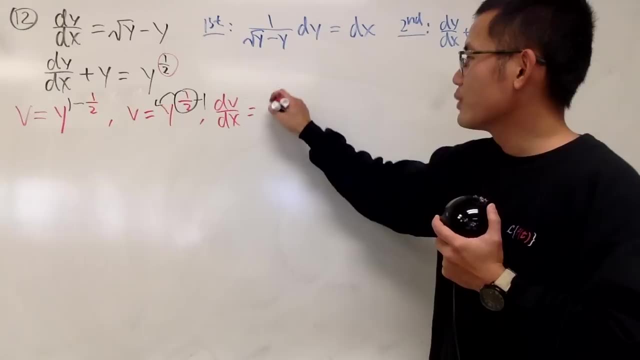 So I get dv dx equals bring down the power first. That can represent bring down the power first and the minus 1.. So I will get 1 half and then y. this minus 1 half is negative 1 half. 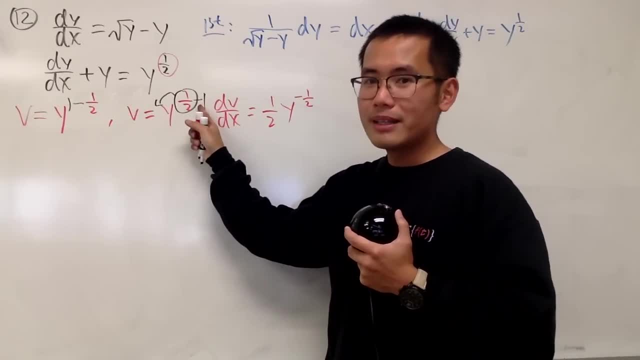 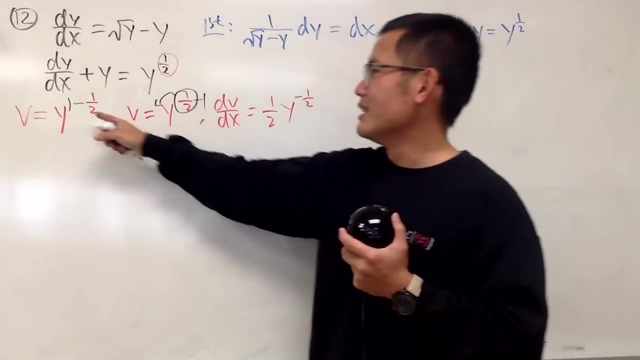 You see, Right here you do the power rule, you have the minus 1.. Yeah, And here you have that extra 1. So they cancel out Very nice stuff. And then you will see you negate the power, so they will cancel. 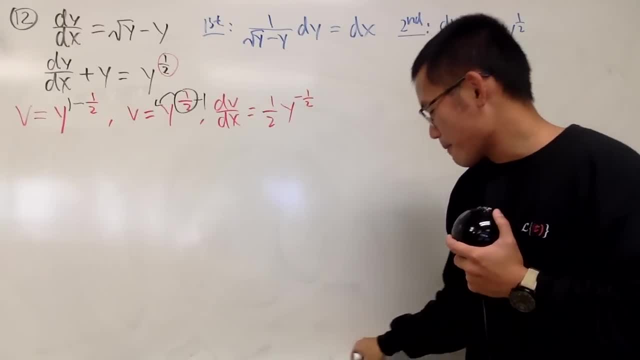 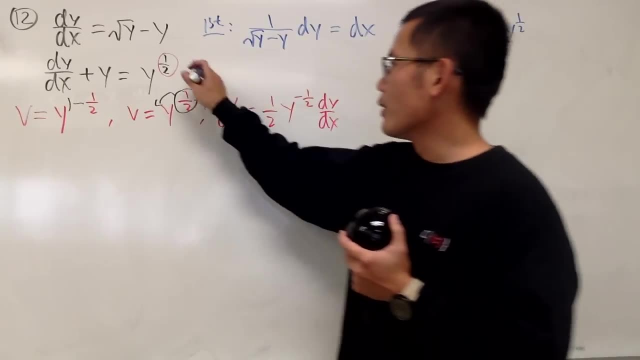 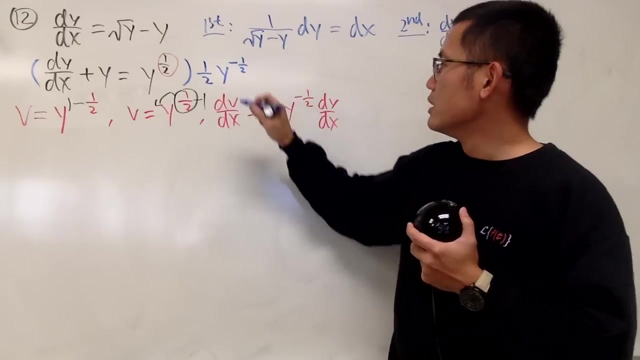 Very nice stuff. All right, enough talking. I forgot the dy dx though, There. Okay, So here we go. Multiply this equation by this extra part. This is my recommendation whenever you are doing the Bernoulli substitution. It's easier this way. 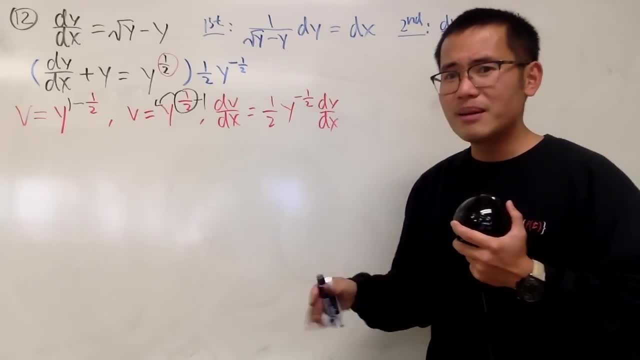 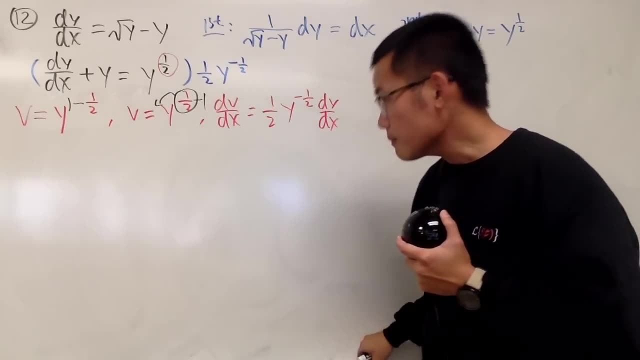 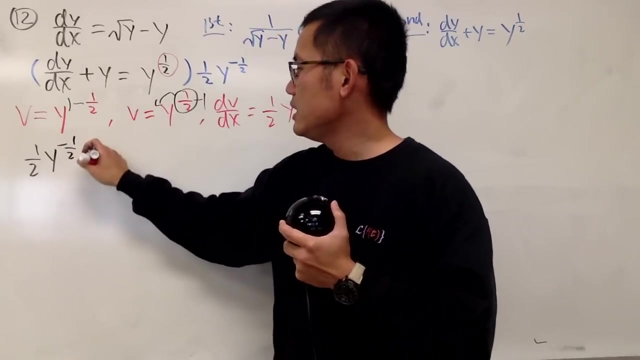 in my opinion, You don't have to deal with rational exponents, sometimes negative exponents, sometimes. This right here is better, Anyway, this times that we get the following, which is positive: 1 half phi, negative, 1 half dy, dx, This and that. 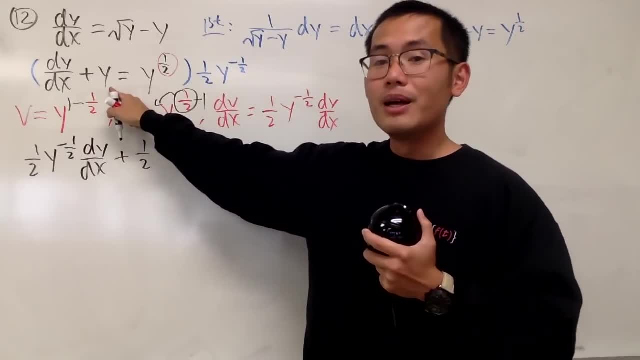 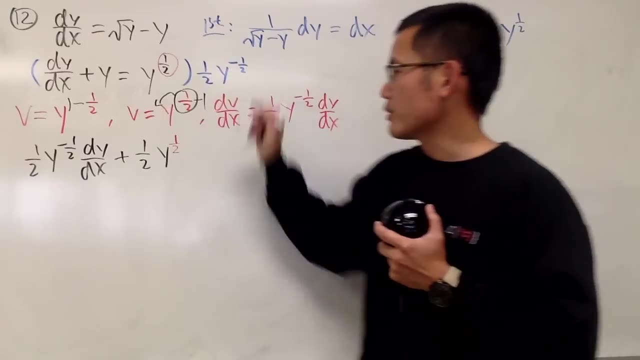 is plus 1 half. This and that is what. This is the first power and that, so it's y to the positive 1 half power. Just make a note on that And this and that cancel out, but we still have 1 half. 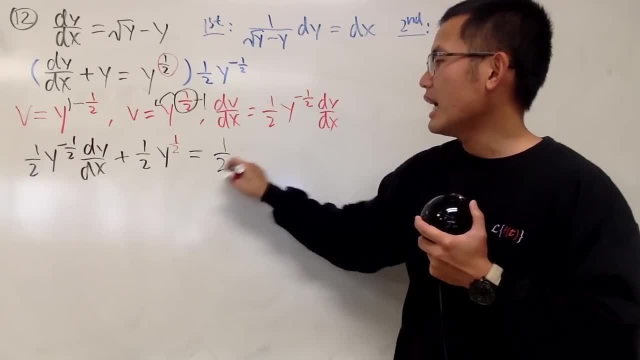 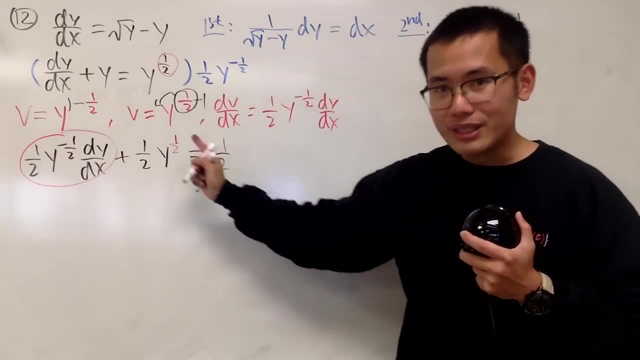 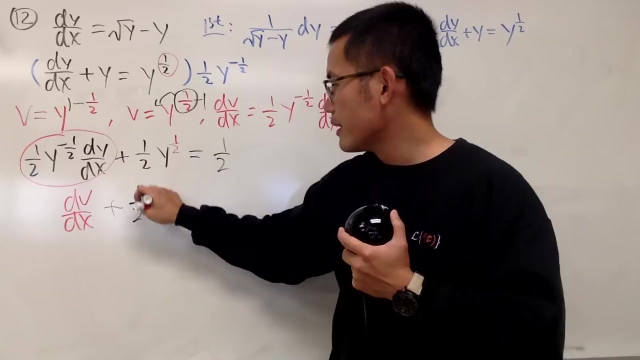 So this is equal to 1 half like this, Very nice stuff. Now have a look. What's this? That's precisely our dv dx- Very good dv dx plus 1 half, and the y to the 1 half power is our phi. 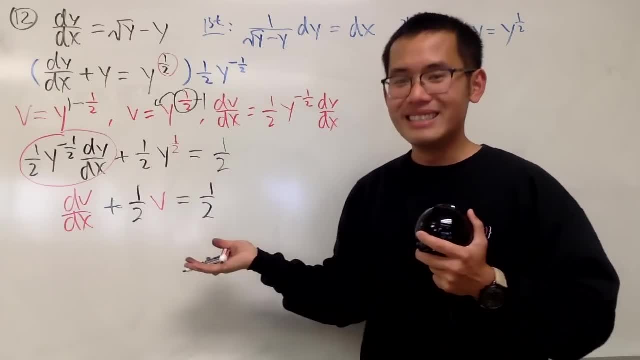 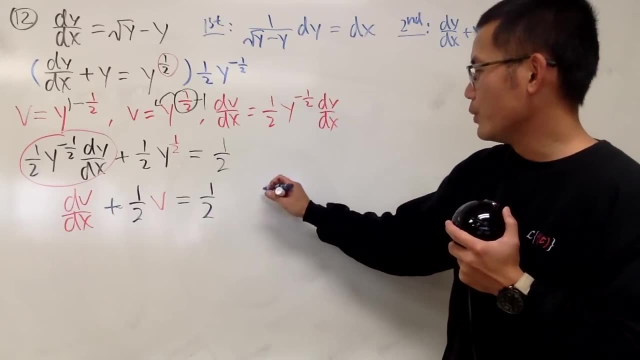 And this right here is nicely equal to just 1 half. It's linear in the d and x world, Like that. Okay, so integrating factor. So here we go. We will have to do this right here. Let me see I should have the space right. 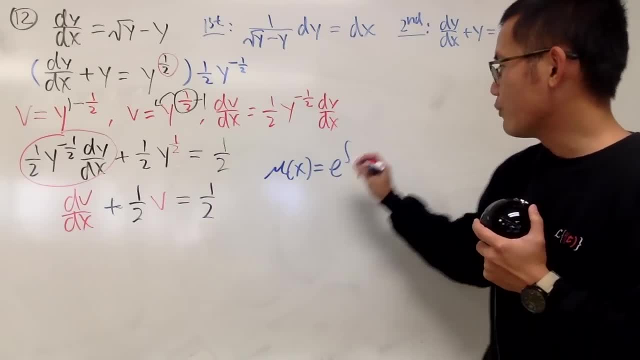 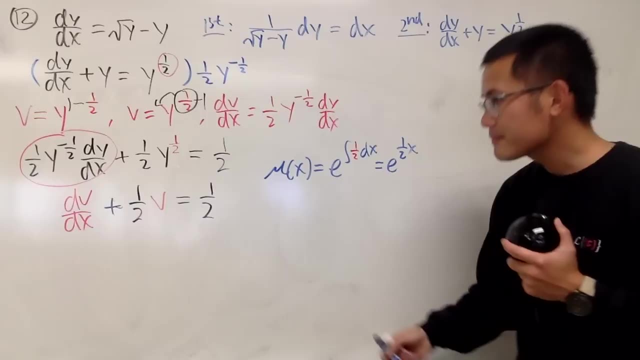 Nu of x is equal to e integral, and we have 1 half right here, and then dx that, So it's just e to the 1 half x power, like this. So, with that being done, let's go ahead and multiply everybody by e to the 1 half x power. 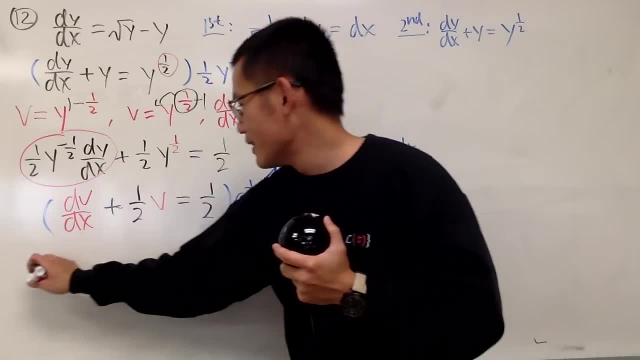 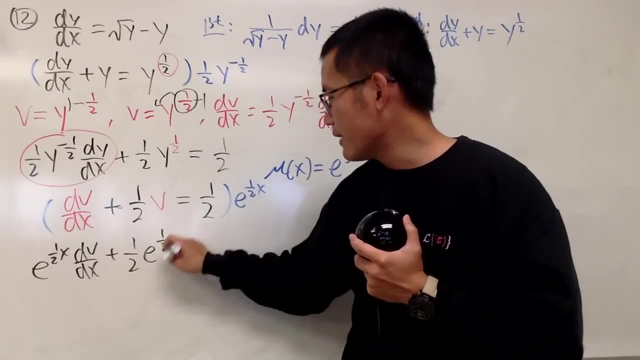 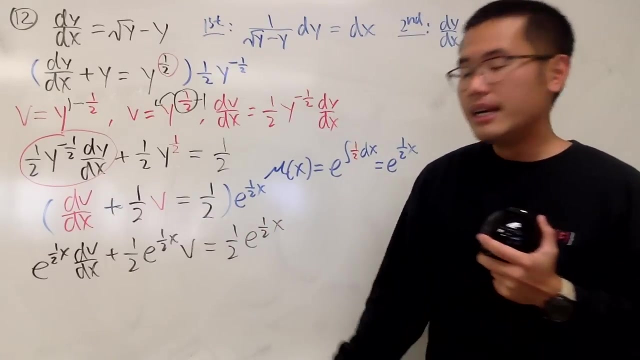 And we will see the following: We will have e to the 1 half x dv dx, plus 1 half e to the 1 half x v, and that's equal to 1 half e to the 1 half x. like this, Yes, on the left hand side. 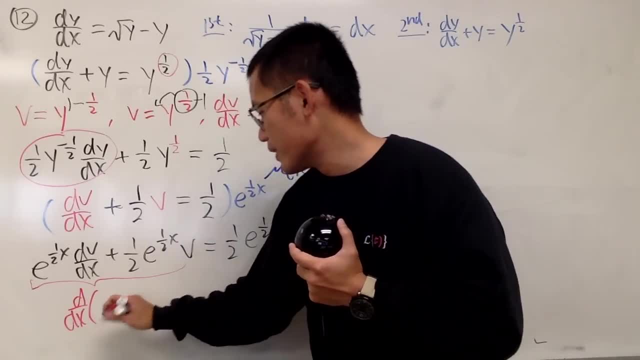 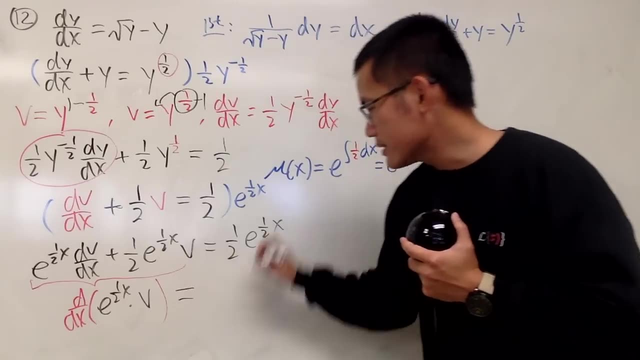 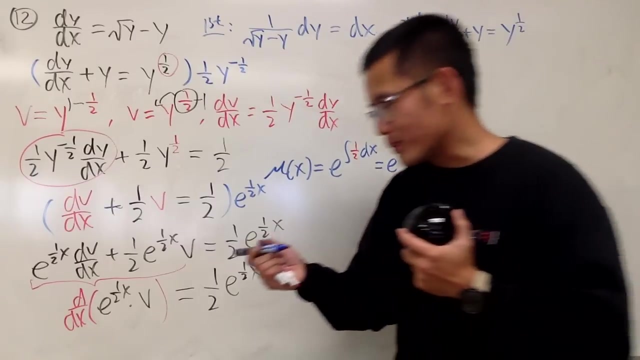 is our favorite derivative of the integrating factor, which is e to the 1 half x times d. And again, you can check it And the right hand side is this: 1 half e to the 1 half x power. like that Now we can integrate both sides. 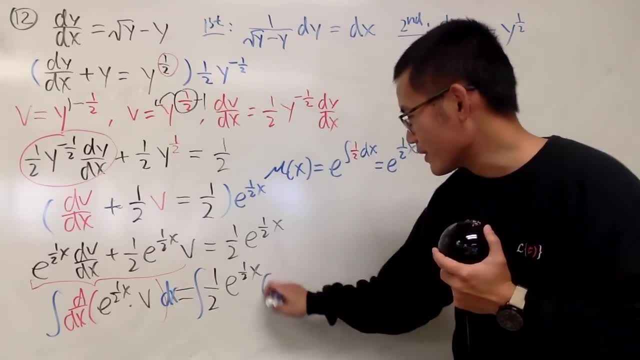 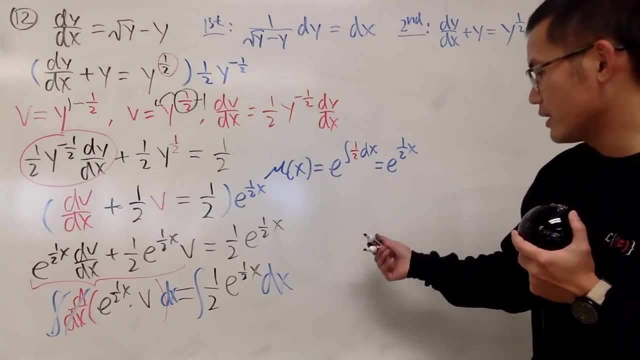 So integral, integral in the x world. So don't forget that, Otherwise people will get mad at me. Okay, So cancel those things out and then I will just see if I can. I'll just do it right here. Let me see. 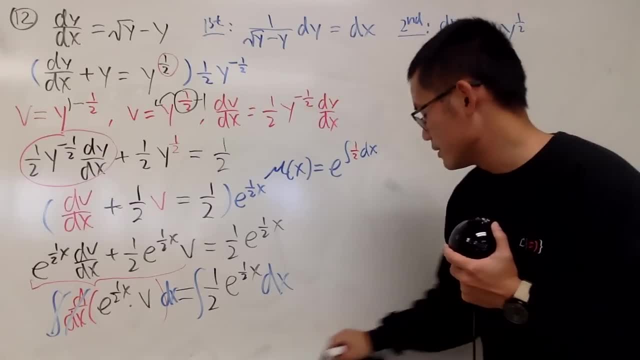 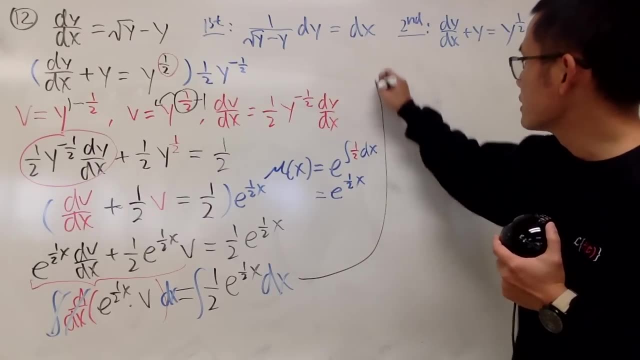 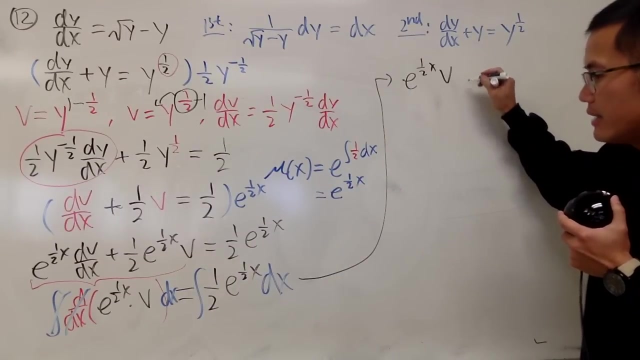 Let me just organize this a little bit. This right here is e to the 1 half x, and then let's do it like this: Study: more space. All right, Here we have e to the 1 half x, v, and then this is equal to: 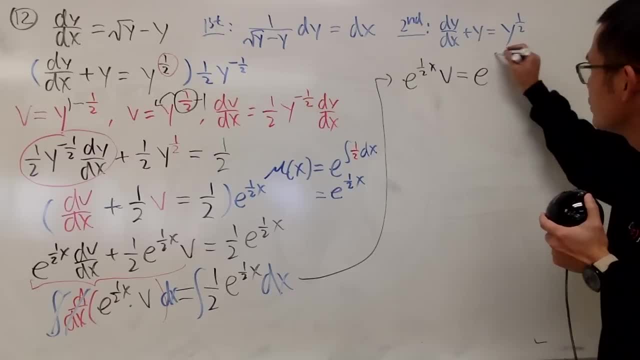 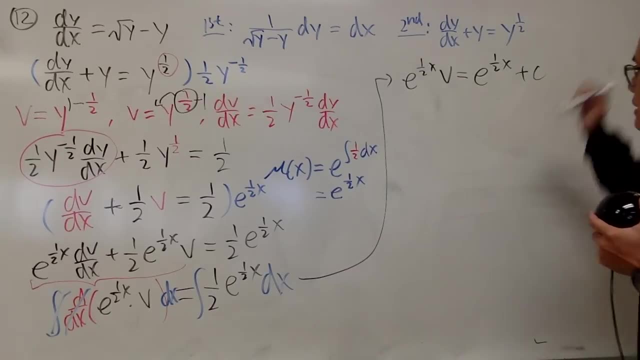 integrating this. It's very nice. We actually just get e to the 1 half x. Why? Because the derivative of this is precisely that. Very nice. And then don't forget the plus c. Yeah, And then let me divide everybody. 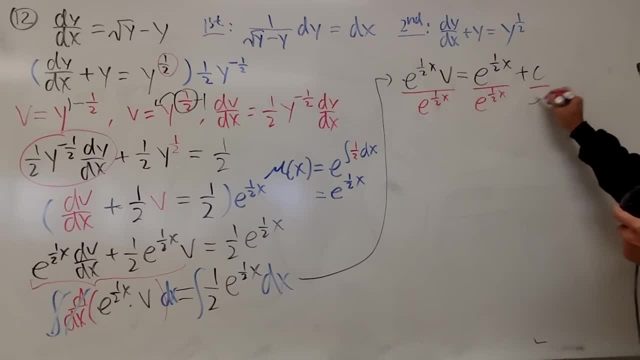 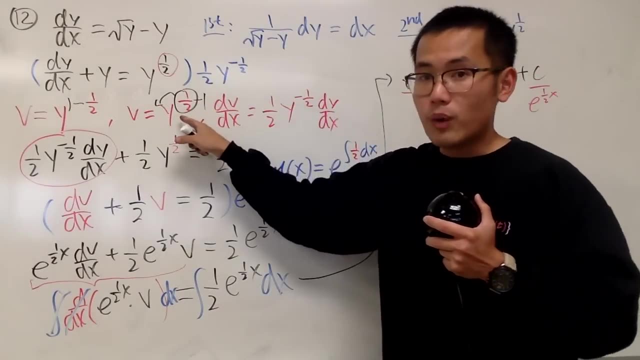 by e to the 1 half x, Divide everybody by e to the 1 half x and divide everybody by e to the 1 half x. This and that cancel out nicely. v is equal to square root of y. Yeah, Pretty much. 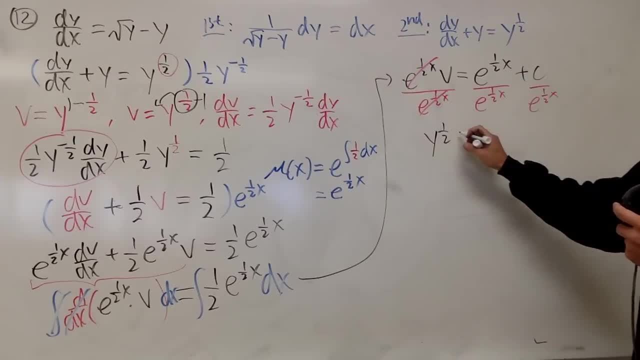 So let me just write it as y to the 1 half power: Yeah, For now. And then this is equal to this and that cancel, It's just 1.. And then this, right here, I will just write it as plus c e, negative 1 half x power. 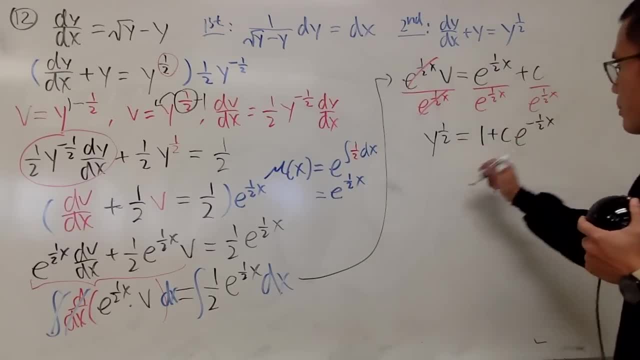 Right Negative power And finally, of course, we can square both sides. So we have our answer And whenever you have c, this is called the general solution And of course we just get y equals parentheses, 1 plus c, e negative, 1 half x. 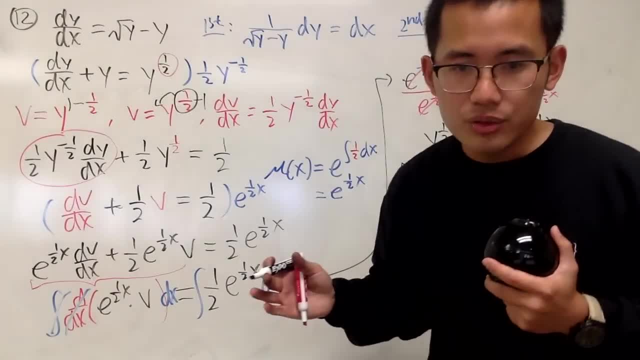 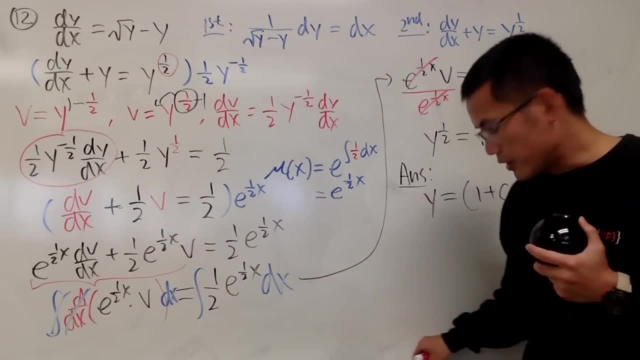 And then we square that, And I didn't give you guys any initial condition. So this right here is, is it? Yeah? However, though, in this situation here I want to address something. Notice that earlier, if we divide both sides by this, we have that. 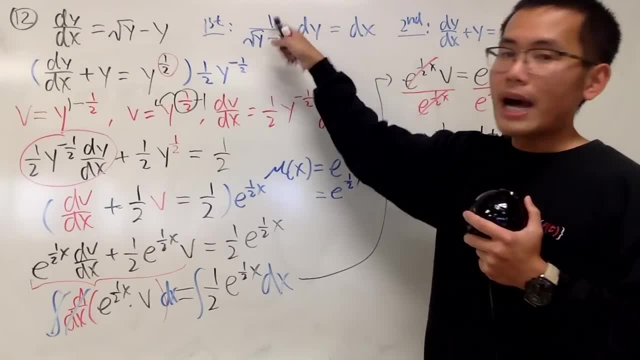 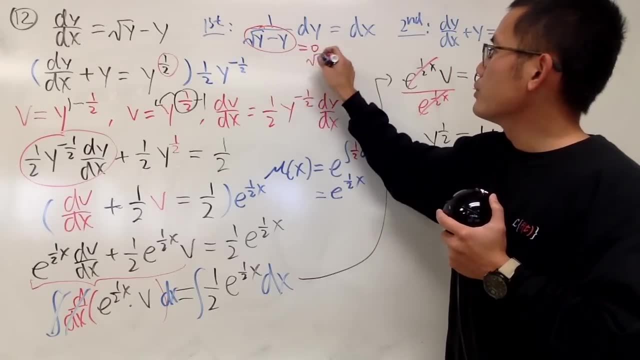 right here. right And notice, the denominator is just with y. In this case, what we will do is the following: Put this to be 0.. Square root of y is square root of y minus y is equal to 0.. Solve for this equation. 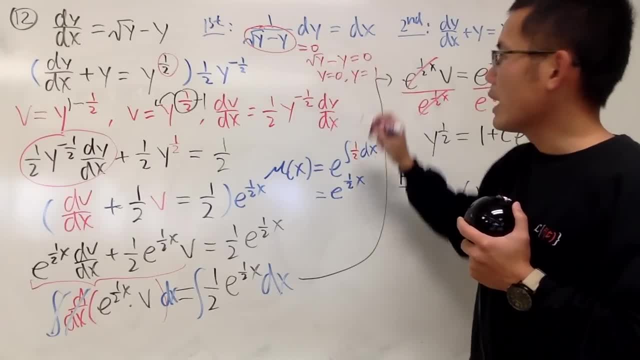 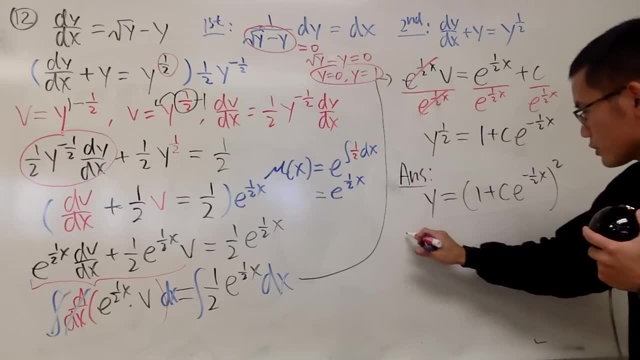 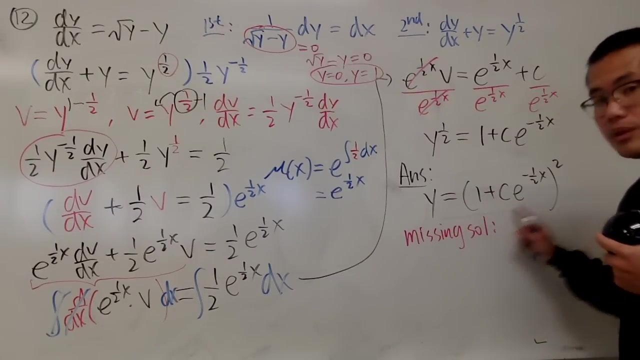 and you will get: y is equal to 0, y is equal to 1.. This two right here, they are the missing solutions. So I just write this down here for you guys Again earlier, that's why I mentioned it. when we have the c right here. 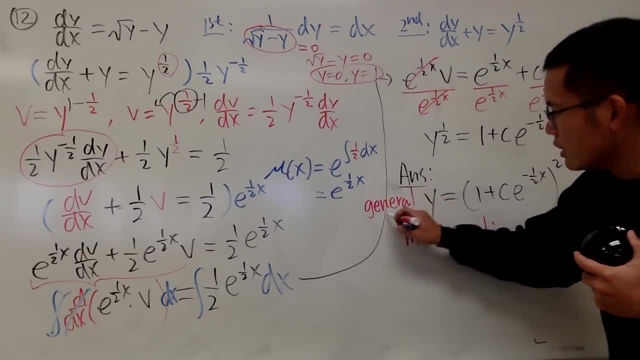 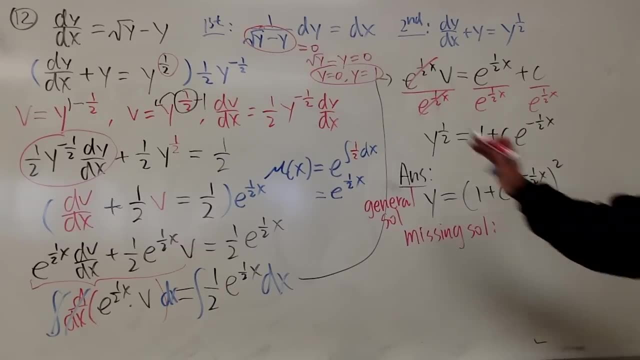 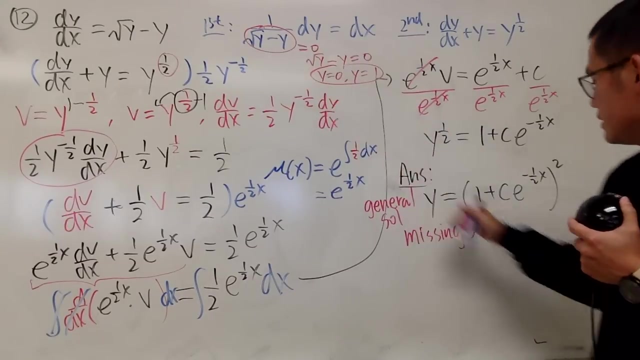 this is called the general solution. General solution Whenever. you have all that, But here is the missing solution and if you do this, you will see when you have this right here, when y is equal to 0 and y is equal to 1, they are the missing solution. 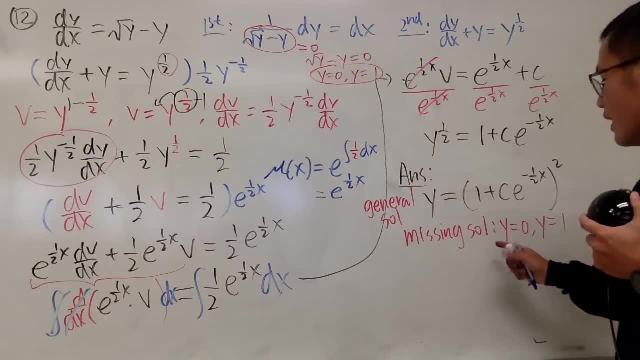 And in fact this is the crazy part, right? What we mean by the following is this: When you have the function- this is the function- y is equal to 0- you can plug into the original Square root of 0 is 0 minus 0 is 0. 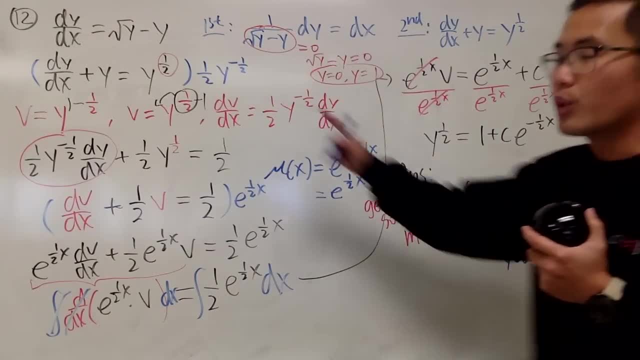 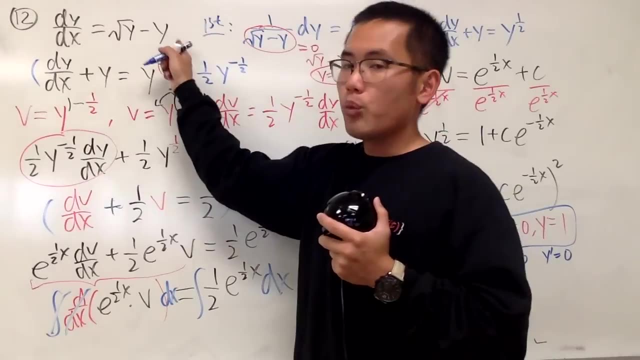 and the derivative of this is also 0. So it works. Yeah. Likewise y prime. the derivative of 1 is also 0. if you plug in 1 and 1, you also get 0. So that's the missing solution part. 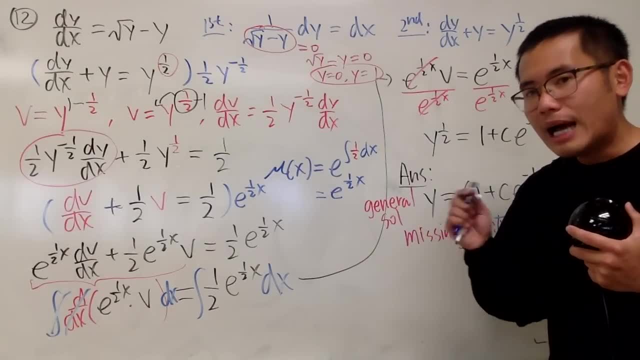 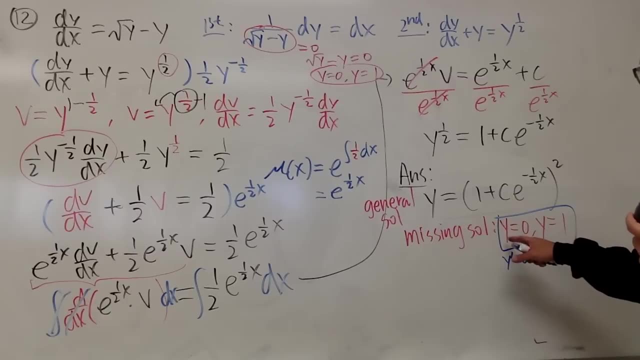 So usually this is the thing that you will have to do, however, though sometimes the general solution might include the missing solution. So here is the deal. Is it possible to this to be endowed with 0? and let me put down 3 equal signs. that means 3 lines. 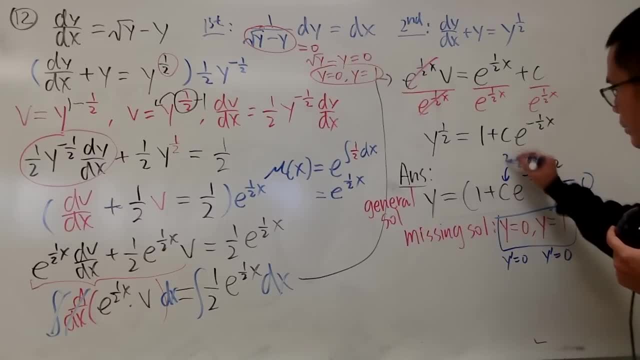 meaning identical equal to 0.. Is it possible? So can you pick a c value to make this identically equal to 0? Not possible, Why not? Just not possible. Just maybe put c to be 0, then you have 1 square. 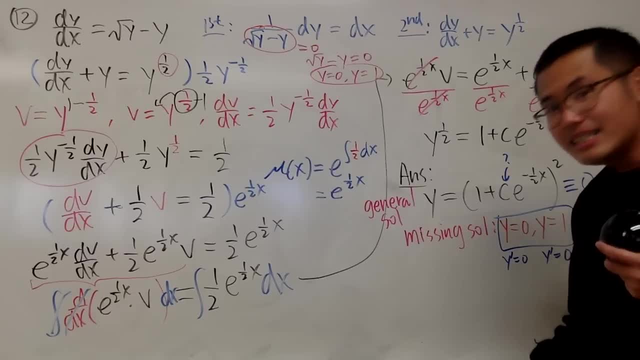 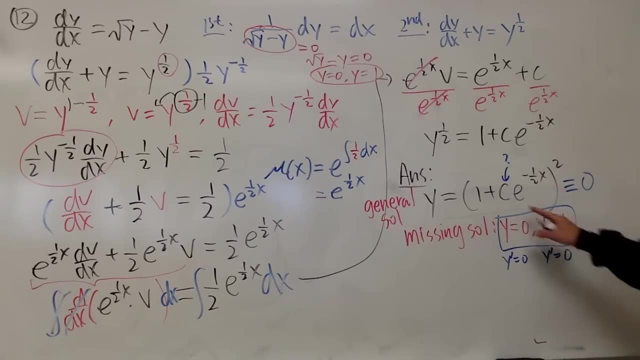 It's not possible. Yeah, And I mentioned it, if you put c to be 0, you actually get 1.. Yeah, So in fact, this 1 it's actually including this general solution. So here is the deal. You usually do this. 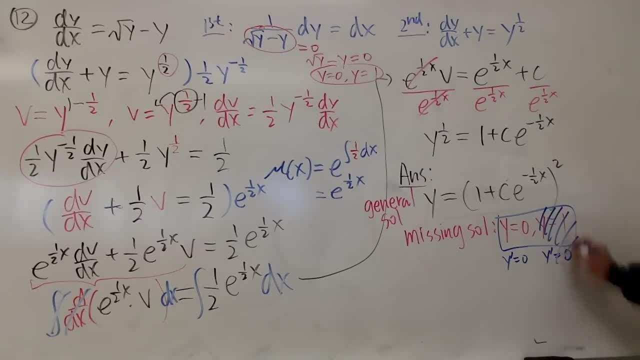 but this 1, it's actually included in the general solution. I will actually write down the following: Um. So let me see, let me see, let me see how should I write it down. So let me just rephrase it, Right. 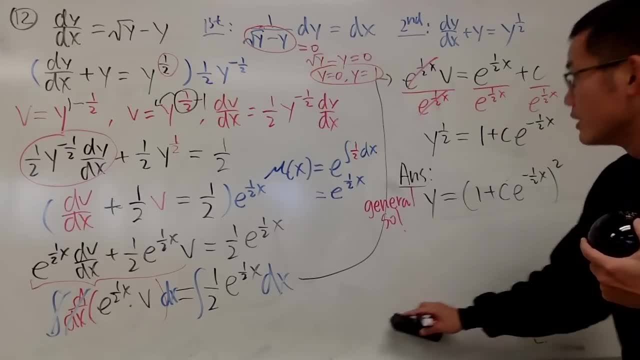 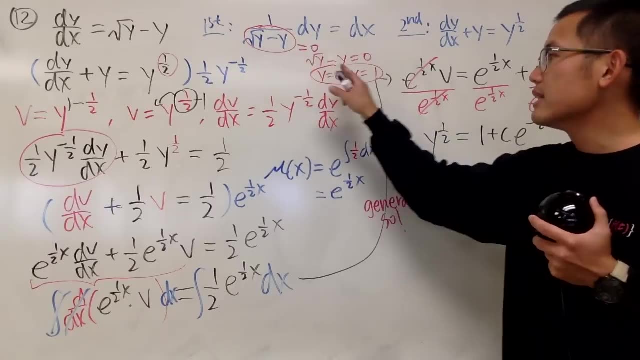 Whenever you do this, pay close attention. both of them are the constant solutions. they will work, But sometimes this might be in the general solution already. So I will just tell you: the only missing solution is from: y is equal to 0. Again, that's the constant solution. 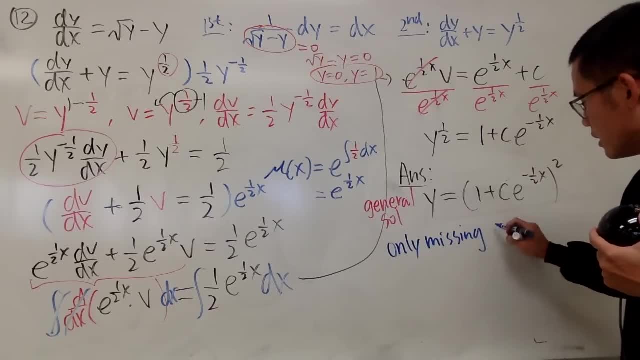 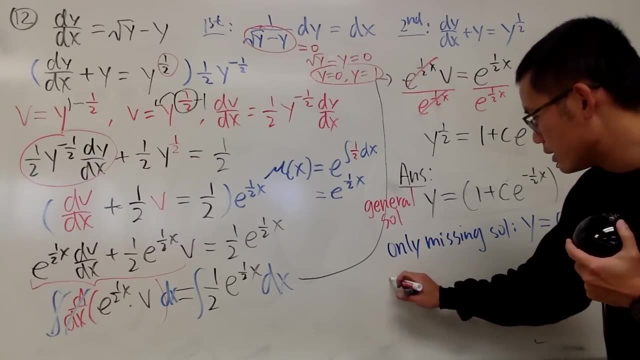 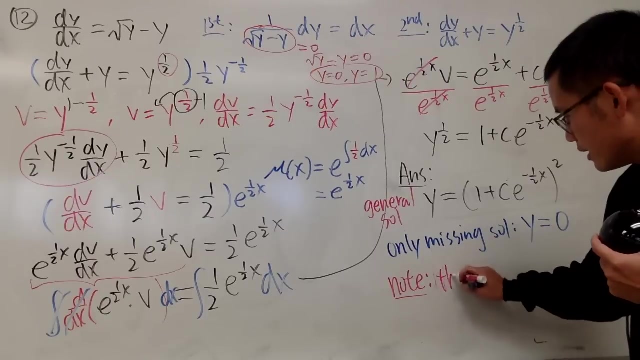 So I will just tell you, the only missing solution is from: y is equal to 0.. Again, that's the constant function. And note the solution. uh, let me just write this down like this: The solution y is equal to 1 is in. 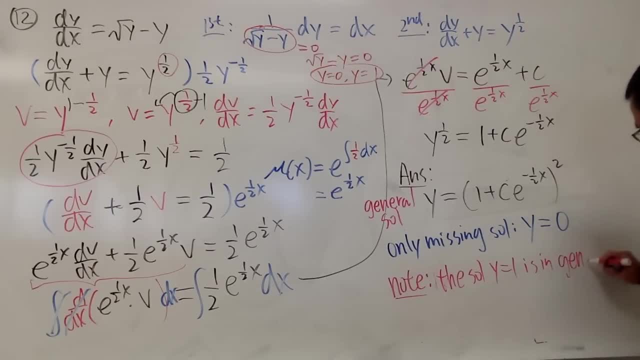 the general solution already when c is equal to 0. So for example, if you have y is equal to 1 plus you put 0 in here and you have e negative 1, half x square. this right here gives you y is equal to 1. 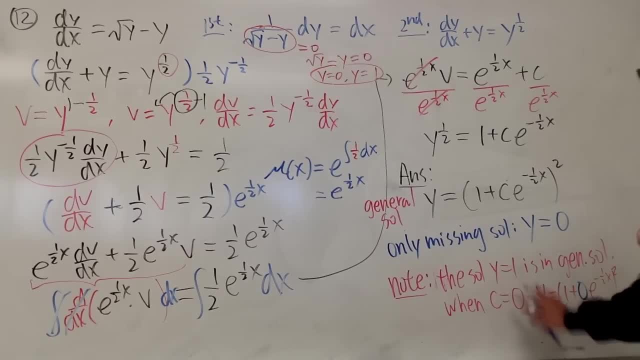 already right. So this is not considered a missing solution because it's included in here. But this right here is. So that's what I was trying to say. So depends, right, Depends on what the question is asking. Sometimes, if you have to find out all the solutions, 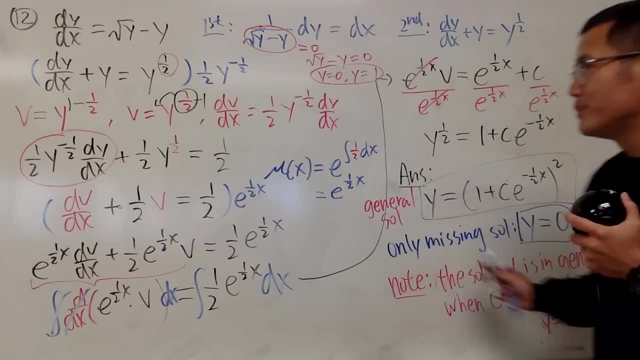 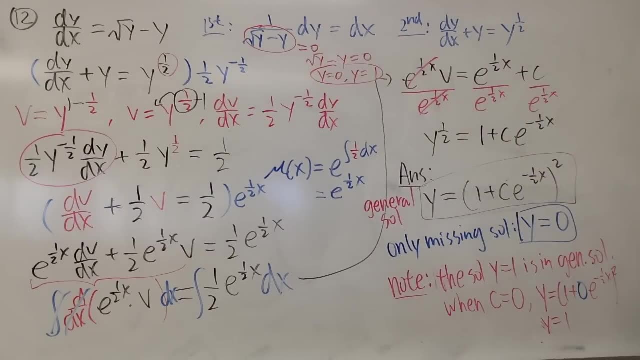 then you have to do this and also include that And really be really careful, because not both of them are the missing solutions. So that's what I was trying to say. So have a look, Have a look, And sometimes to avoid this kind of confusion, 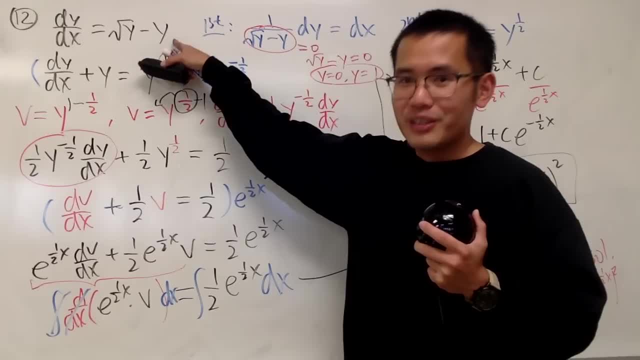 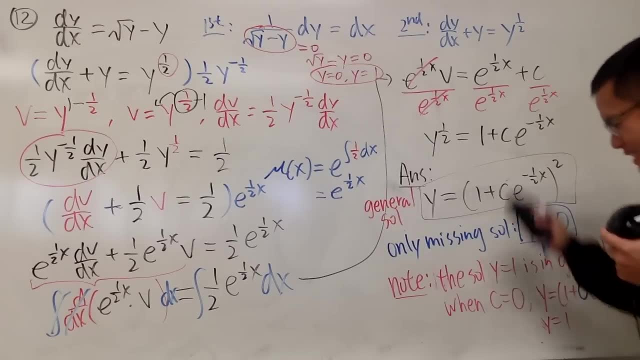 the best thing to do is provide an initial condition. Let's say, y of 2 is equal to 5 or something like that, And in that case you will just have to have a general solution for that, A specific one for that, Anyway. 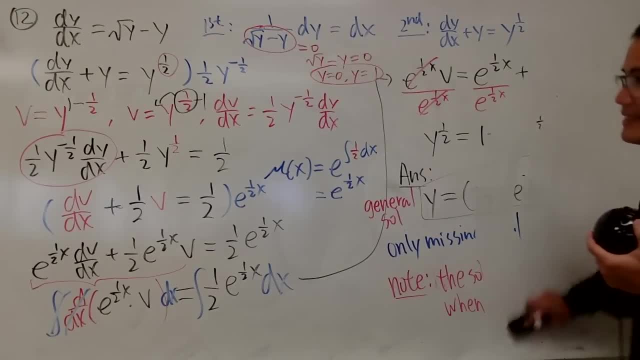 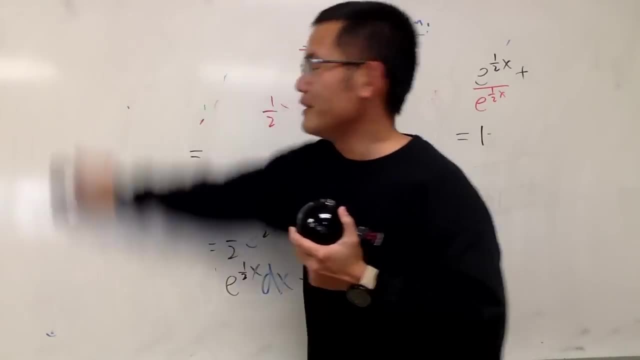 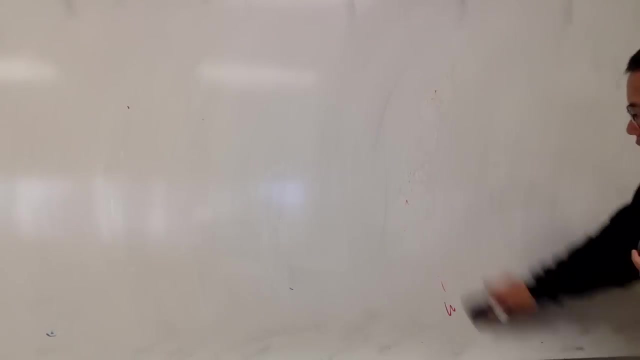 that's it. And, of course, feel free to do this question with separating the variables. And let me know, In fact I did that already for you guys. You guys can go check it out- three years ago, So I created some of the questions. 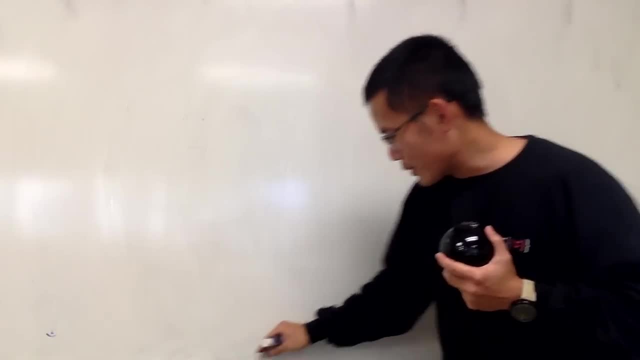 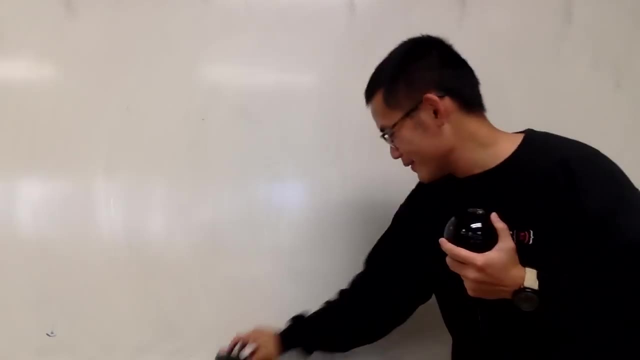 just for this video, And I also have some questions that I have done a while ago. I haven't taught differential equations for a while, So I feel really good to do differential equations again, Or halfway done. Let's see what time is it? 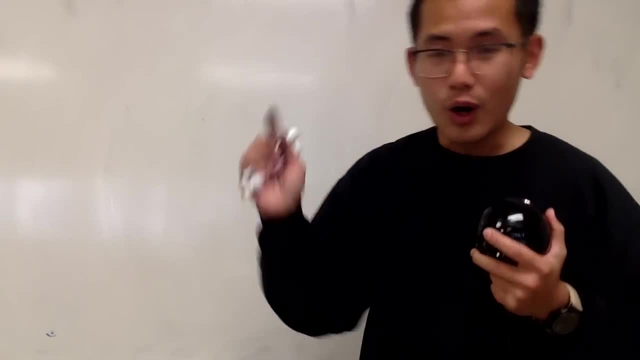 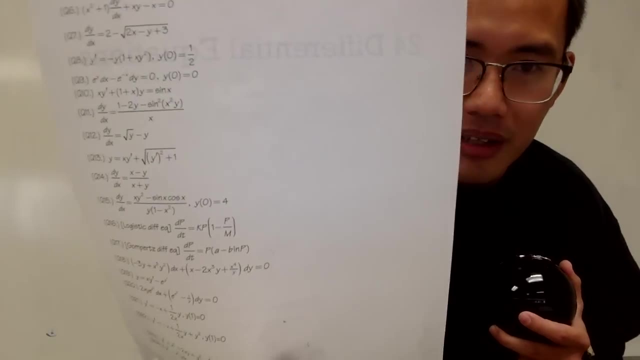 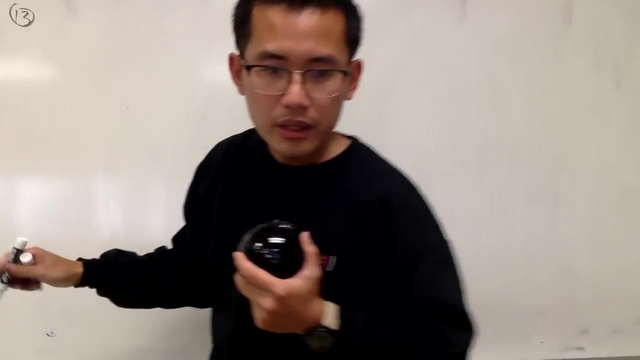 What time is it? Two hours, So four hours will hopefully will do it. Okay, Number 13.. This right here is a very cool one, Right? So I'll try to do this. Let's see number 13 here. Here we have. 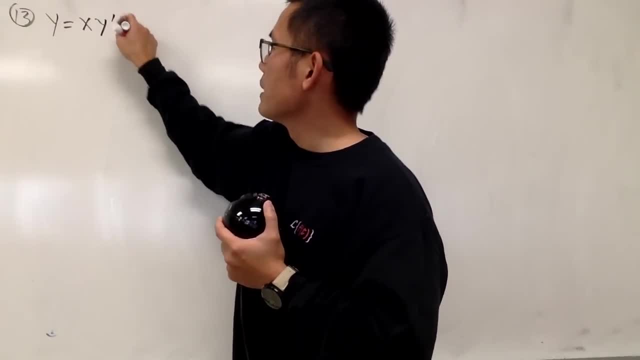 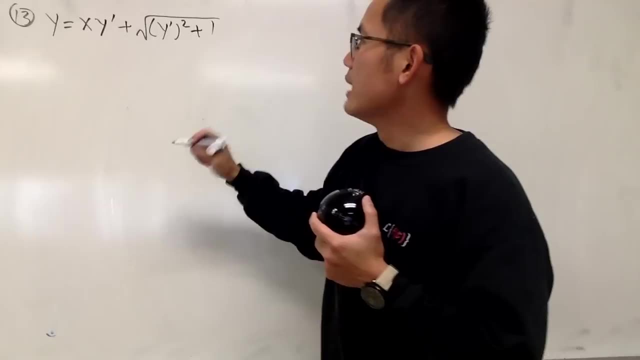 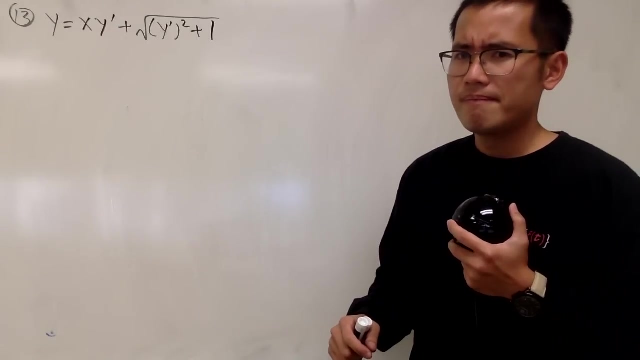 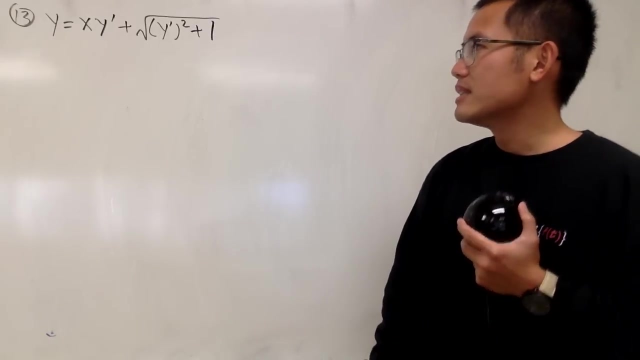 y is equal to x, y prime plus square root, And we have a parenthesis: y prime square plus 1.. Like this Seriously: y prime, which is the first derivative, and you square that guy, God. Now, even though this right here looks crazy. 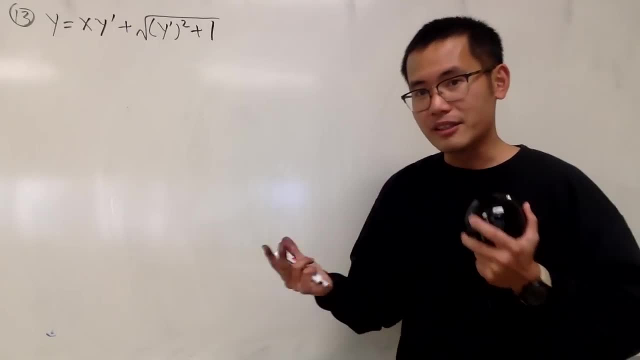 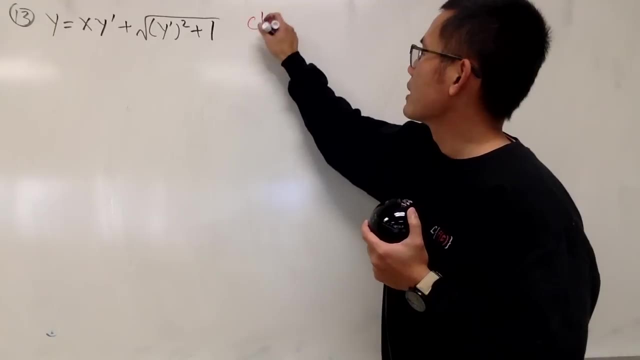 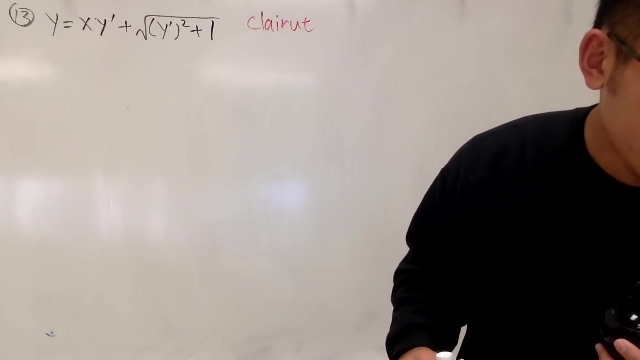 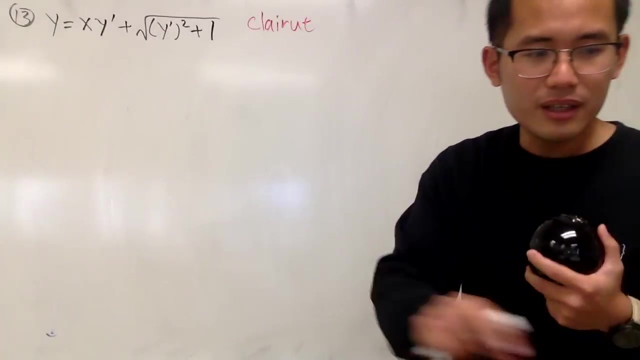 but in fact this is actually a rather famous one because it has a name. This is called the not clear, This is called the clear out. Let me see if I spelled it right: Oh clear and the out Clear. I missed the a. 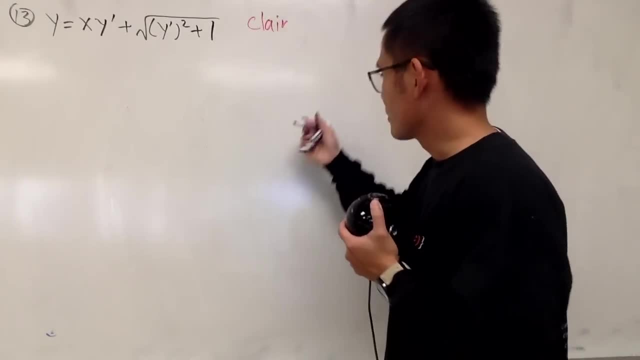 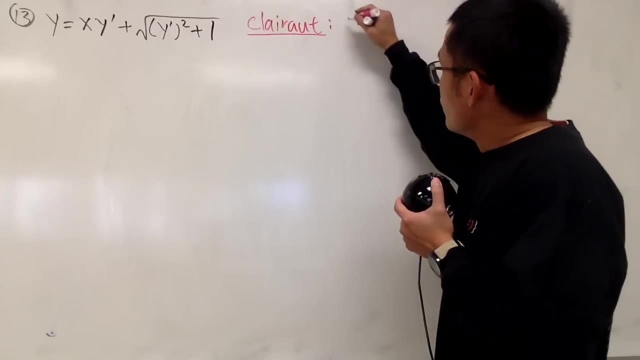 I'm sorry. I missed an a, So I checked my notes for spelling out Clear out. There we go For the clear out. it's the following: Right, It's y and that's equal to x times y prime. So this part. 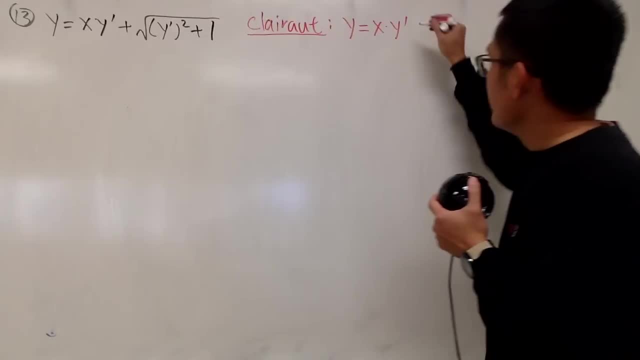 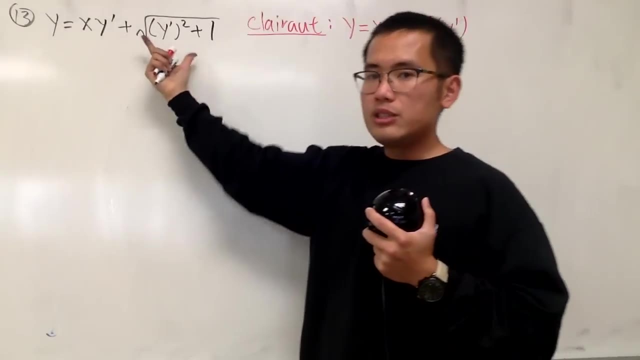 is the same as that. And then, whatever you're adding, it has to be a function, and usually people write it as v of y prime. So this is just a function in terms of y prime. Crazy huh, You can have sine of y prime. 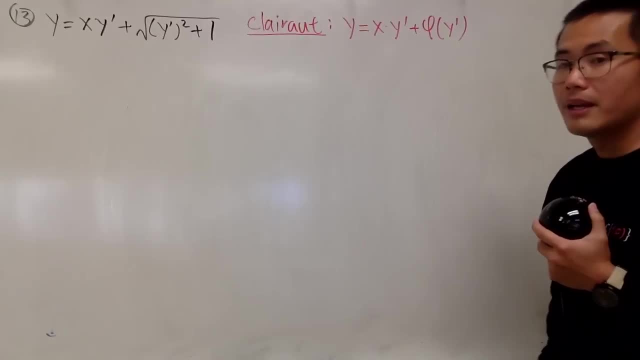 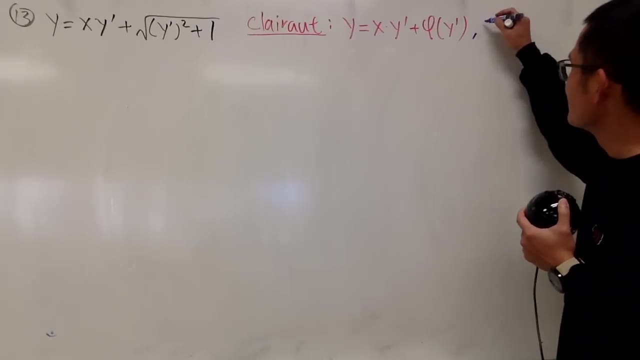 cosine of y prime or whatsoever, but all that stuff. And in fact there is also a just as famous one as well, but that's even crazier. I'm not going to do any of that. It's called the La Grunge. I'm just trying. 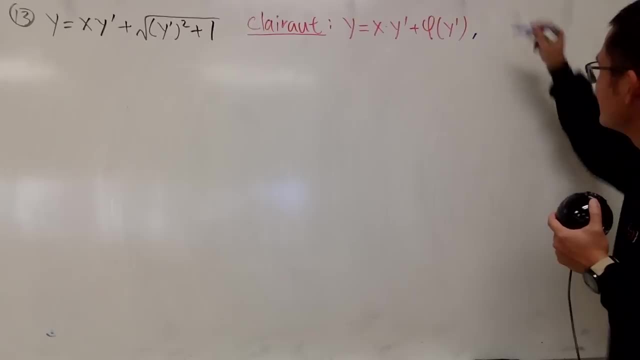 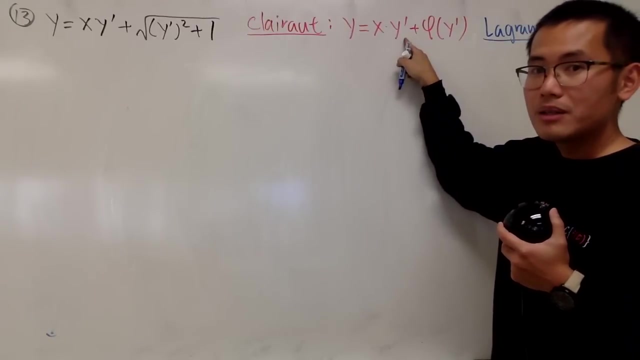 La Grunge. How do I spell that? I didn't prepare this? actually La Grunge, Something like this. Anyway, La Grunge differential equation is the following: It's that instead of the y prime here, right, You actually just get a function. 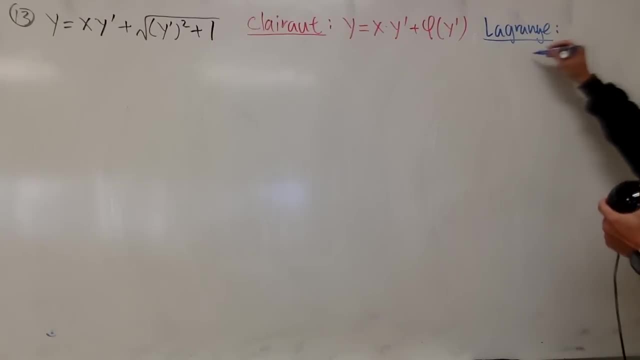 in terms of y prime as well. So the La Grunge situation is: when you have y is equal to x times, I think, they use sine and then y prime and then plus phi of y prime, And I forgot which that, but it doesn't really matter. 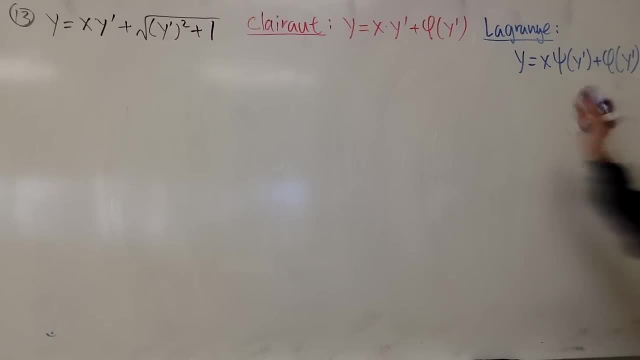 It's just a Greek letter anyway. So yeah, Yeah, I don't know how to pronounce the phi or the psi or whatever, But anyway, this is actually just a special case of that, You see, Because you can just take this to be the identity. 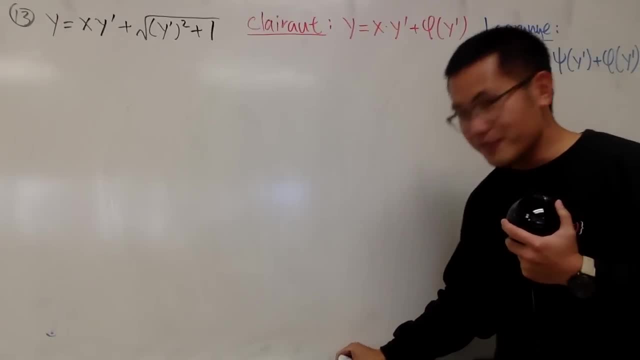 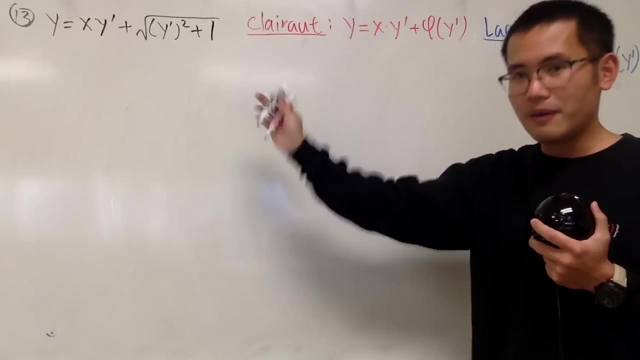 Right. So that's just some some fun fact I will say. But anyway, the reason I bring this up is you can just solve it the following way, You don't have to do it the usual way that when they introduce this, This is pretty bizarre. 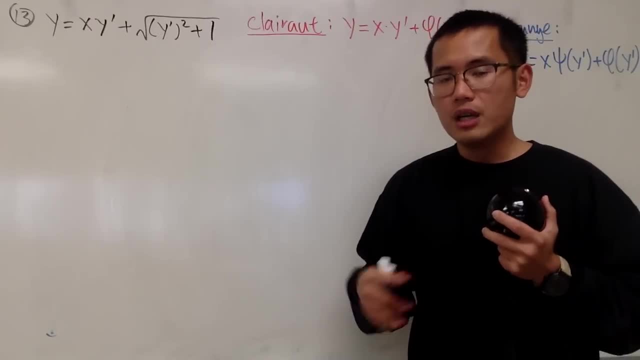 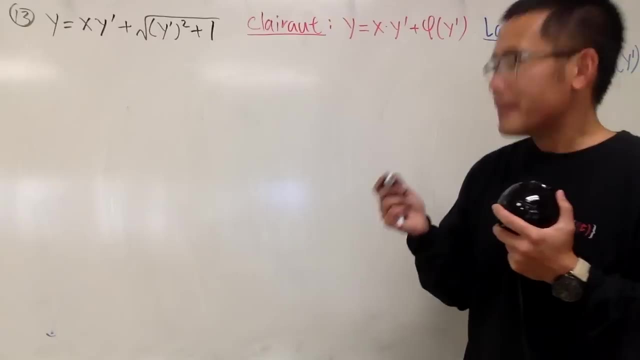 You will have to do, you have to, you have to come with the parameter and all that stuff. But life doesn't have to be that hard sometimes. Go ahead and check this out. Here is the deal When you have a clear out, not clear, okay. 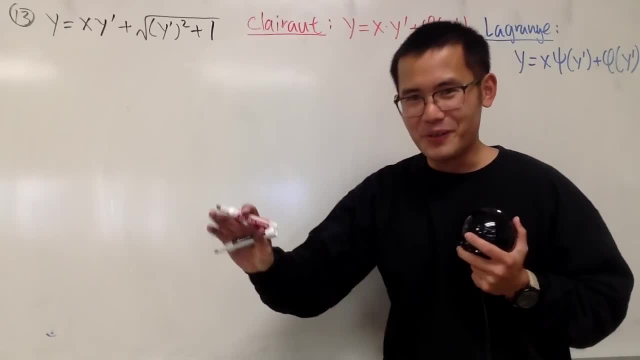 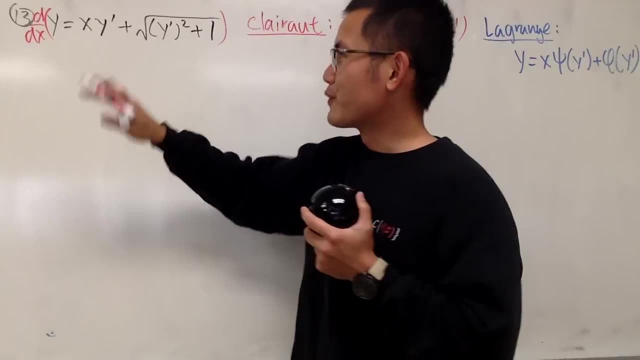 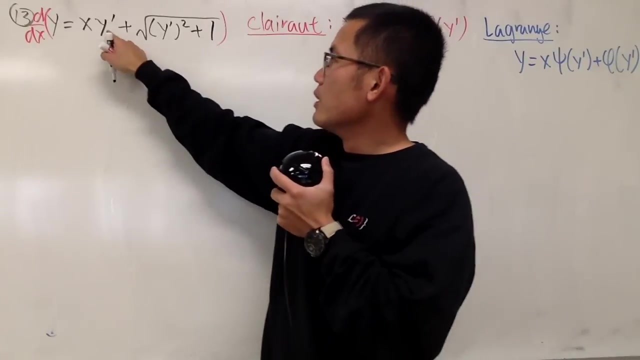 clear out differential equation. you want to differentiate that equation first, So I'm going to go ahead and differentiate this Right. Differentiate this with respect to x right away. And the reason this is not partial derivative is because y prime is dy dx. 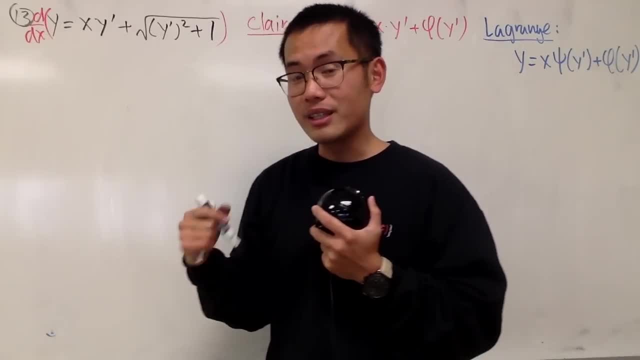 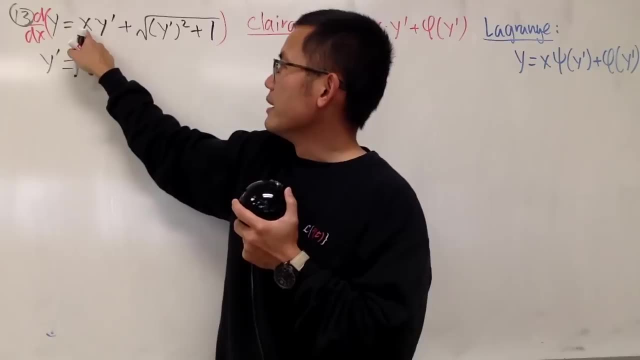 I want to just differentiate this with respect to x again, So I get a second derivative, Right? Anyway, here we go. Differentiating y, we get y prime. Okay, Differentiating this, x times y prime, of course we have to use the Prada loop. 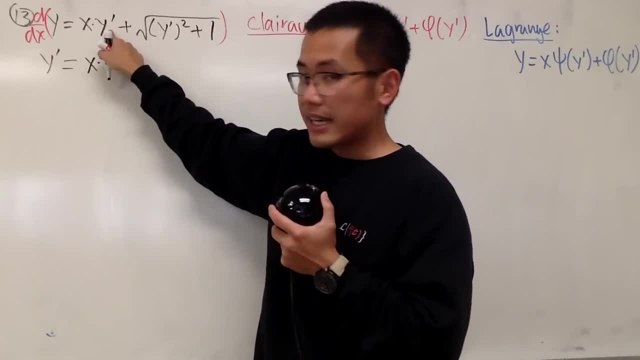 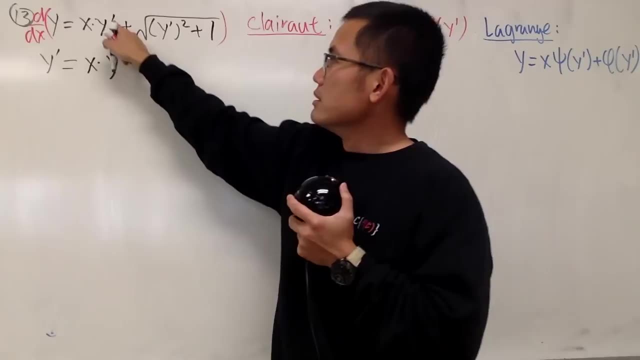 Keep the first function, which is x times the derivative of the second Derivative second of y prime. Right, It's just y double prime, Like the second. The derivative of this is just y double prime. Yeah, Plus the second function, which is the y prime. 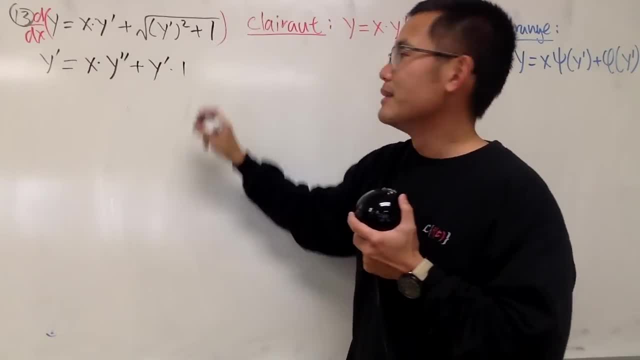 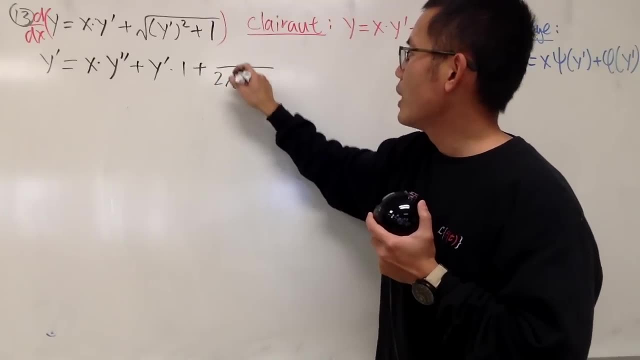 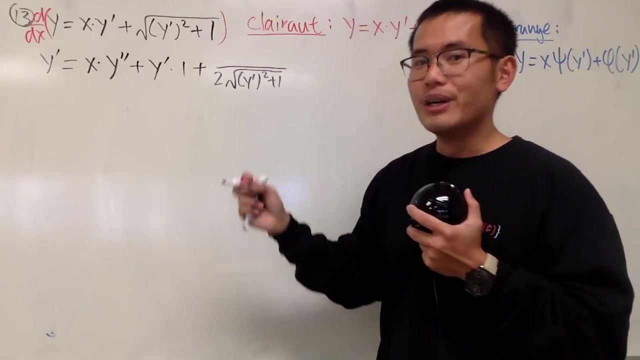 right here, times the derivative of the first, Just like this. And then plus the derivative of this Derivative of square root is one over two square root of five inside. So let's just write that down. And then don't forget the Chengdu. 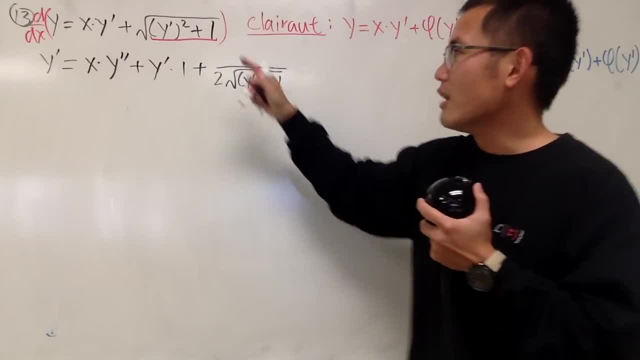 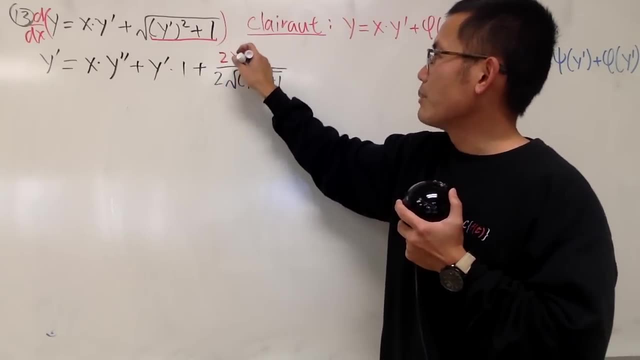 Multiply by the derivative of the inside Derivative of this. bring the two to the front, So we have two, And then the input state is the same. So y prime, And then to the first power. But let's do the Chengdu. 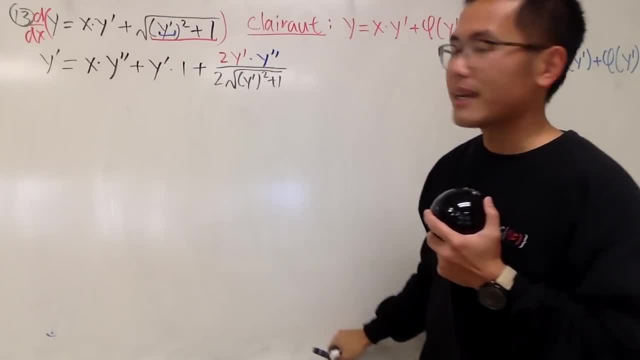 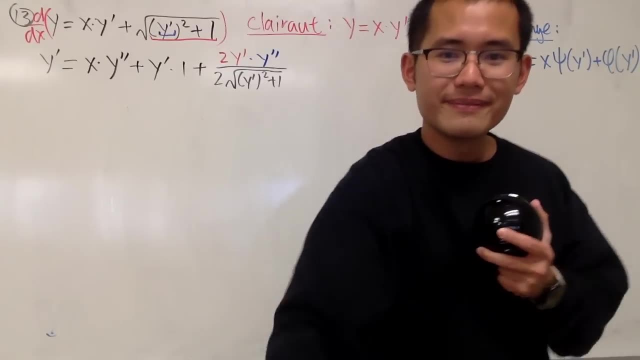 of Chengdu. again, Derivative of that is y, double prime, Like that- And of course the derivative of one is zero. So that's why we don't need to worry about anything on that. Yeah, So that's pretty much the first step. 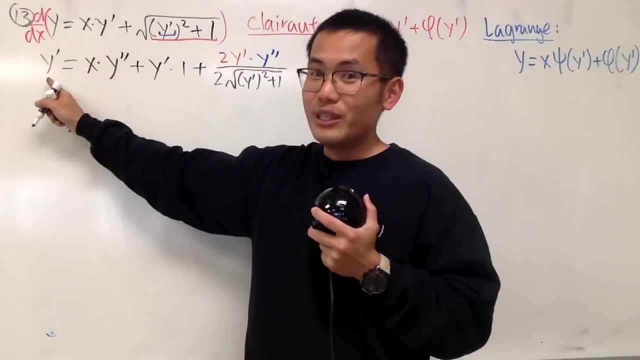 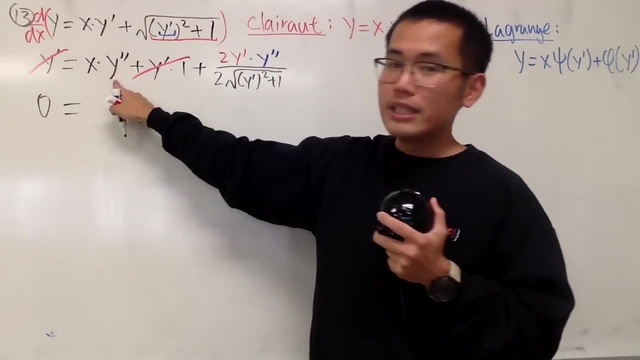 Now check this out. It's really crazy. First, it's really nice right here: y prime, y prime. So they cancel. Very nice, Yeah, So we have zero on the left hand side. Notice both of these guys. they have the y double prime. 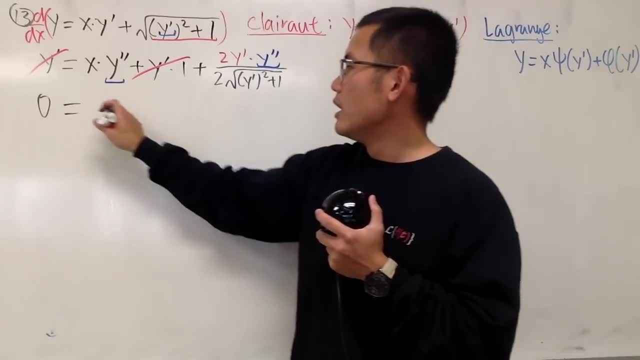 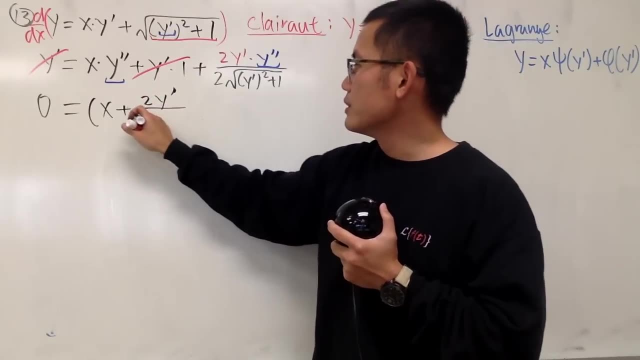 So what we can do is, of course, we can factor that out, And when we do that, I will just have x, and this is plus, and we have over this, which is two square. no, just cancel the two already. Just cancel the two already. So. 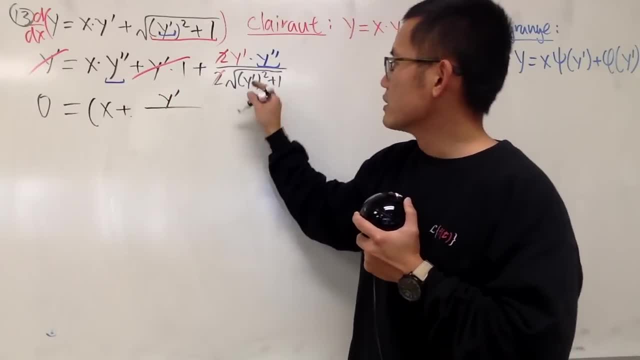 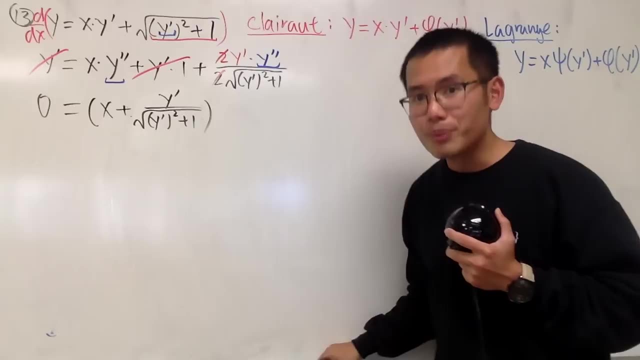 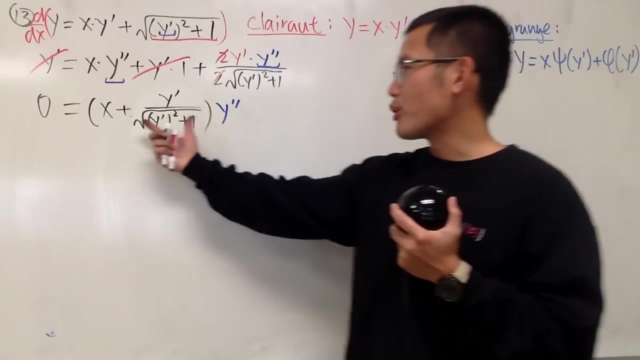 plus y prime on the top over square root of y prime, square plus one, Yeah, And then we will put the y double prime at the end like this, And, as you can see, when we have a product of two things, it's equal to zero. 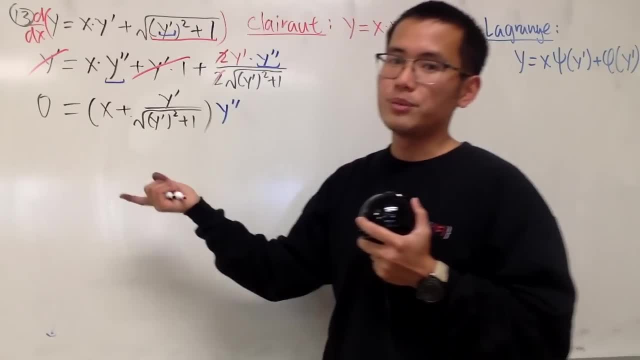 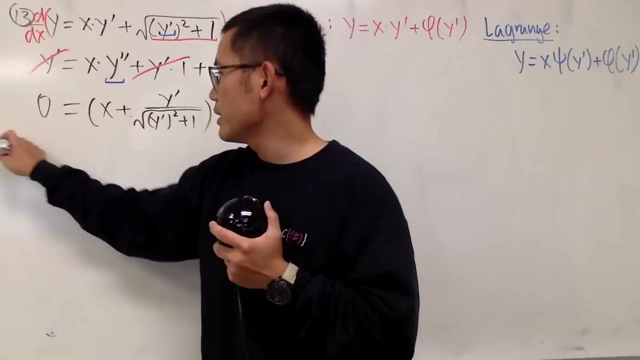 That means what? That means: the first has to be zero or the second has to be zero. Right, Let me first write this down right here. This implies, this implies, let me just tell you guys, this implies that we will have one of the factor. 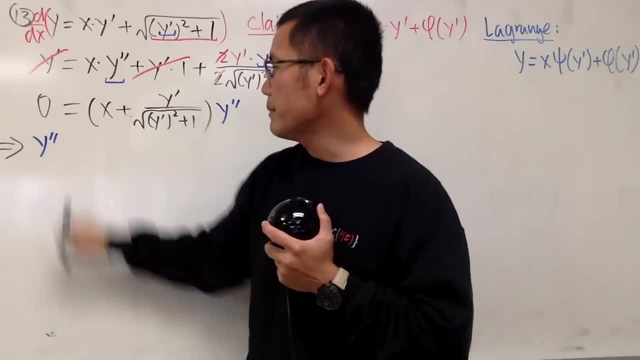 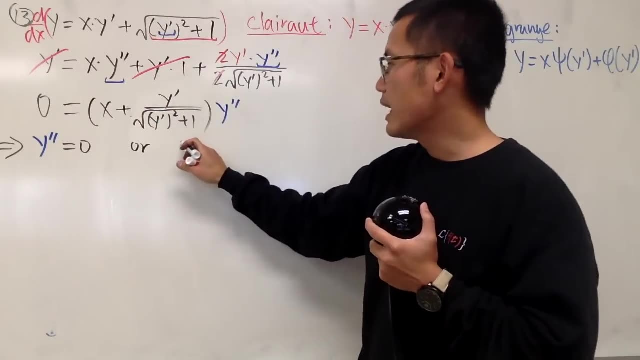 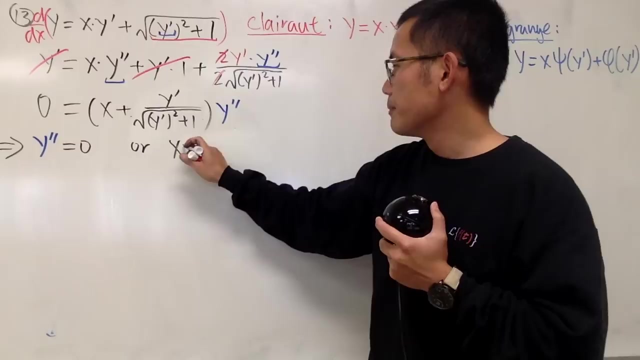 let me write down y double prime. it's: either this is equal to zero, or the other one, which is this part. I will write down x plus y prime over all that, x plus y prime over all that, x plus y prime over all that square root of. 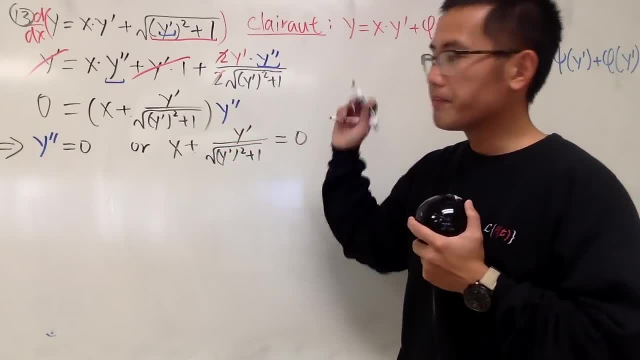 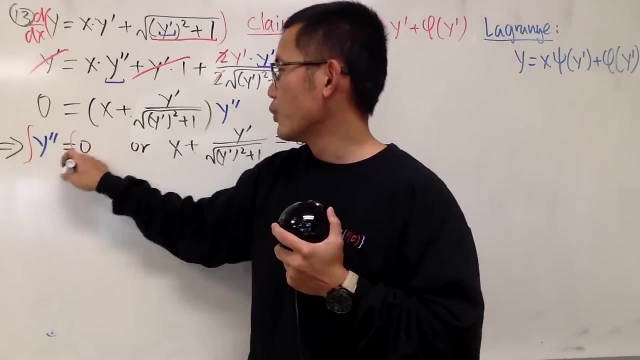 y prime square plus one is equal to zero. Yeah, So it's either this or that. This is easier, so let's go ahead and do that. first, Of course, we can just integrate both sides with respect to x, So integrating y double prime. 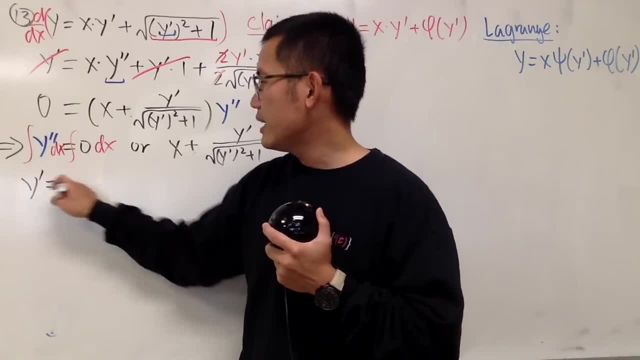 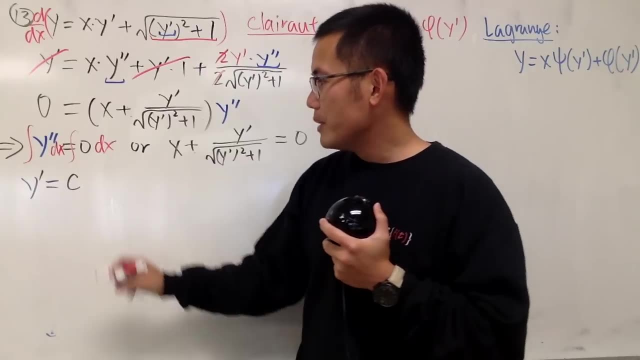 we just get y prime. that's pretty easy, And we will just end up with constant. Yeah, Integrating zero, we get constant. Now here is the deal. Be really careful with this. Actually, I'll put this down in blue When we 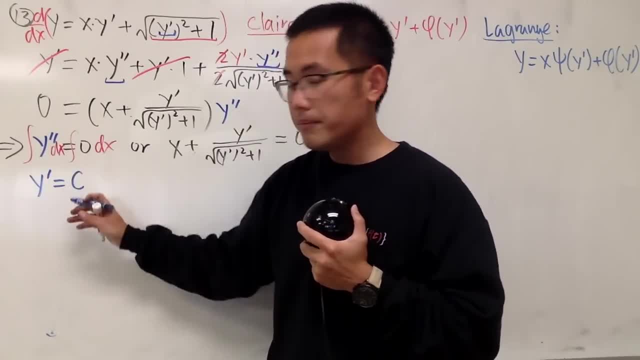 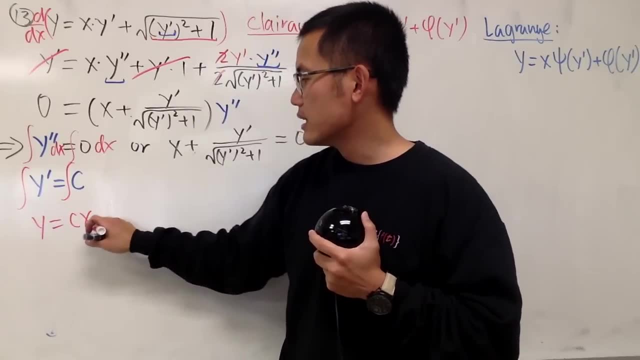 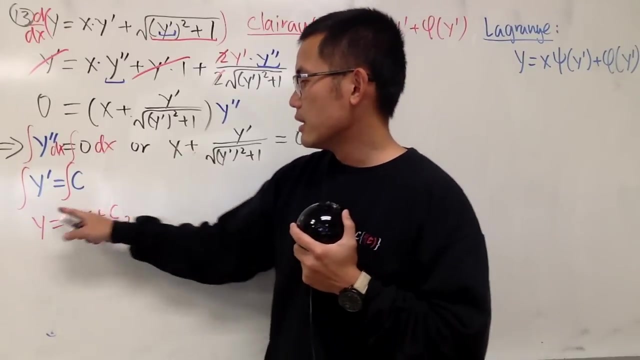 integrate this, we get y prime to be c. Be really careful with this. Do not integrate again and say y is equal to cx plus another c And maybe you can say this is c1 and c2.. Do not do that Why. 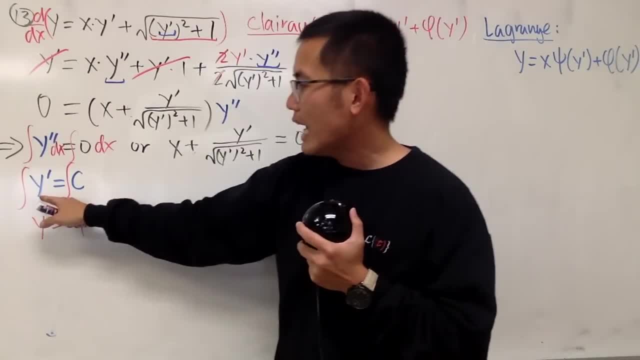 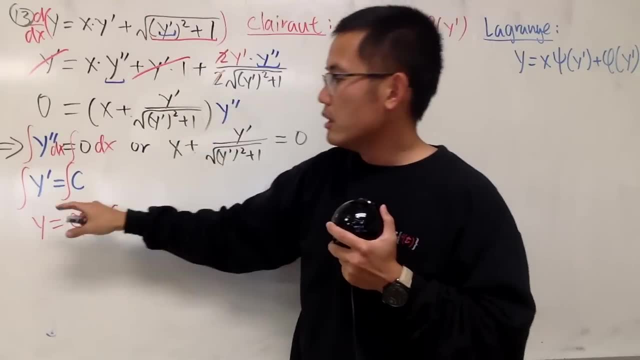 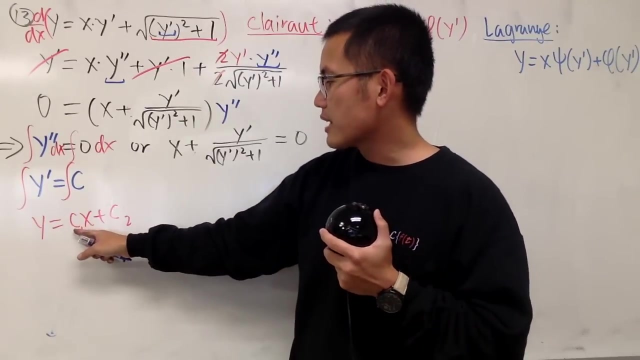 Because y is detected by the original equation, y prime already. You see, y is detected by y prime, the original already. If you say y prime is equal to c, you will just have to plug in c into here and here. That is it. You will still get. 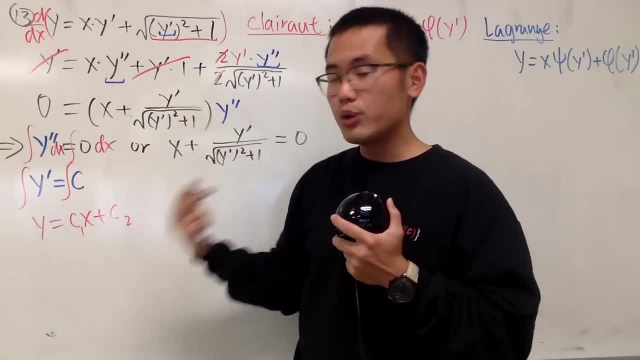 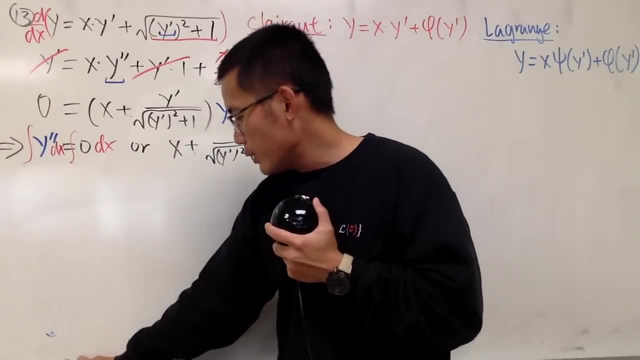 the constant times x. That's good, But this part will actually tell you what c2 is. So this is actually what we are going to do. So here we go. Here we have y. prime is equal to c. We will integrate that. 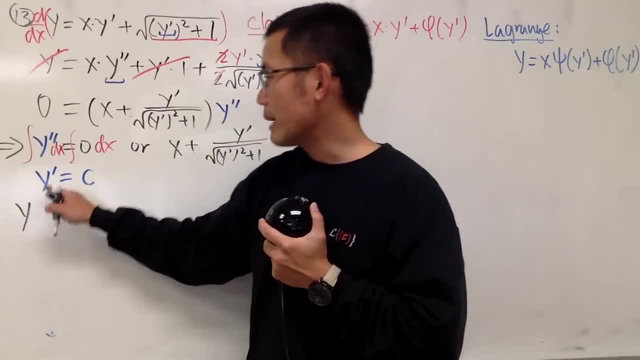 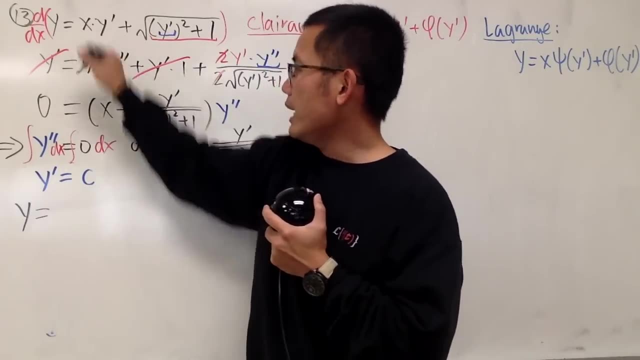 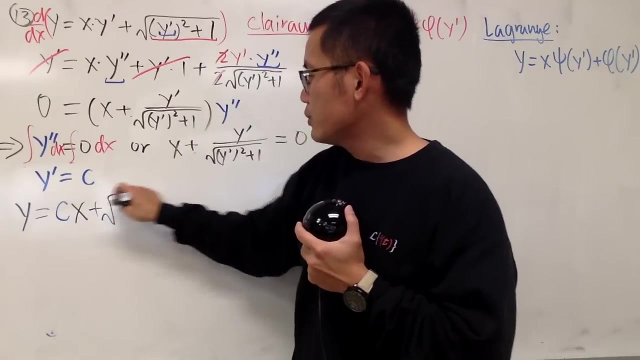 Now together. y do not do not integrate again. All we have to do is plug in c into here and here. So you see, y is equal to x times y prime, which is the c and then the x, And then plus square root, this right here. 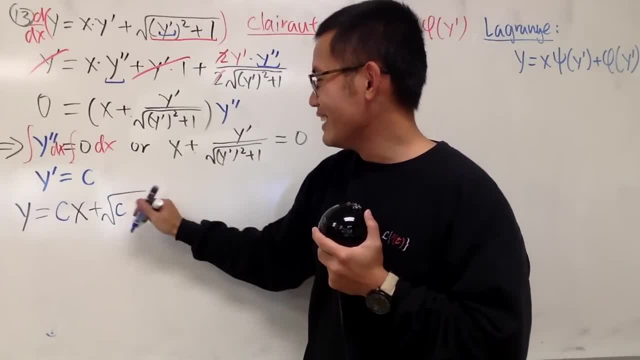 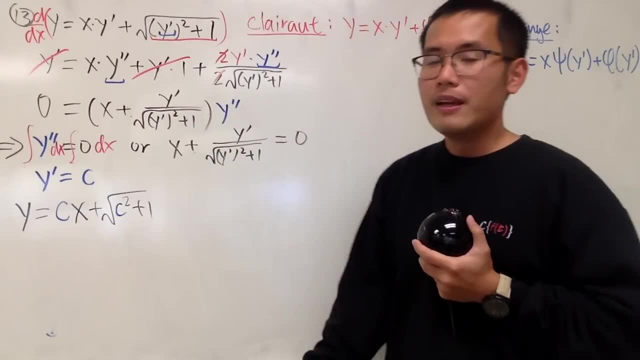 It's my c, It's your c, It's everybody's c. So c square, You see it. And then plus 1.. Just like that, Very good. And now you might be wondering, seriously, we have second derivative. How come we don't have two constants? 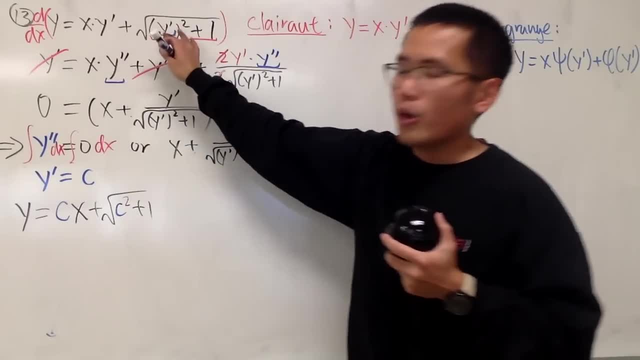 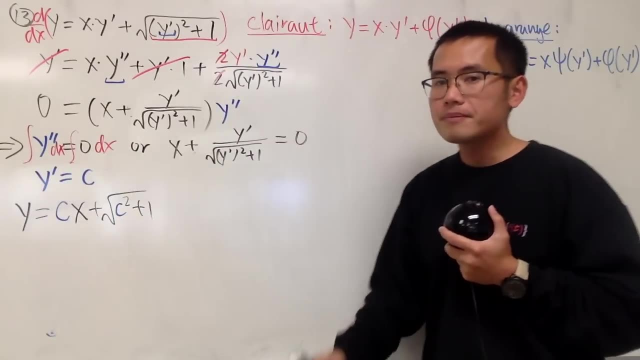 But you have to keep in mind we are trying to solve the original differential equation. We are not trying to solve this differential equation by itself, Right? So keep that in mind. And the idea is that sometimes, when you do extra things, maybe you end up with 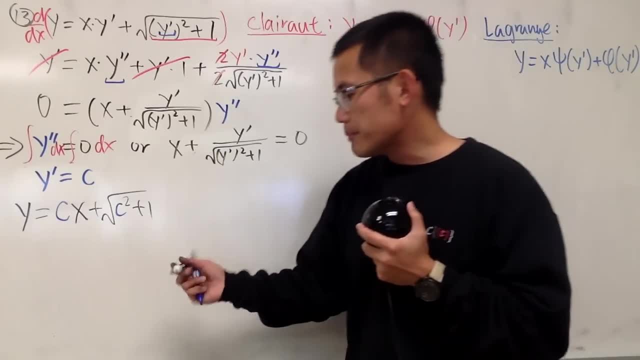 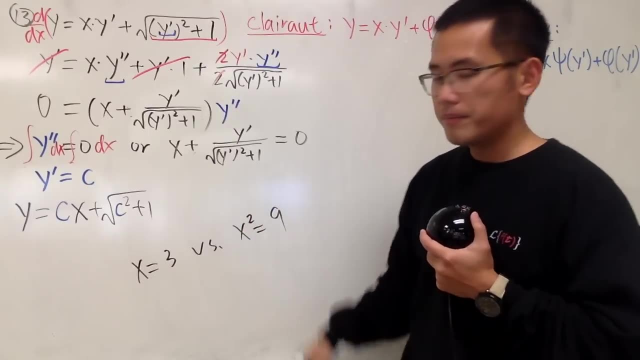 extra solutions, but be really careful with it. For example- just a real quick example- If you have x, it's equal to 3 versus x squared, it's equal to 9.. Do they have the same solutions? No, This right here is the equation. 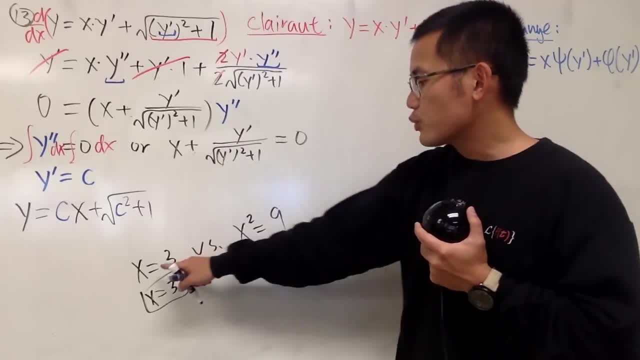 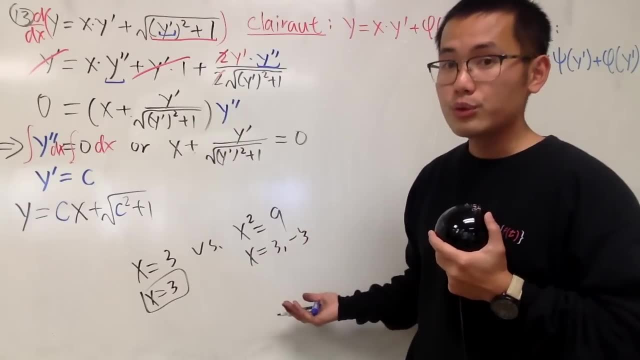 x is equal to 3, and you are done. But here, if you square both sides, this equation is no longer the same as that. Is x equal to 3 or negative 3? You have two solutions, right here? Right, But again you are trying to do. 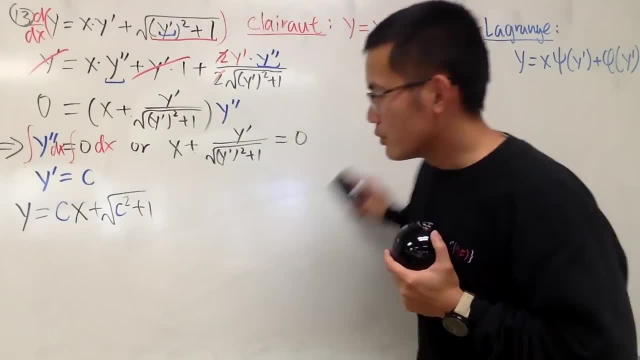 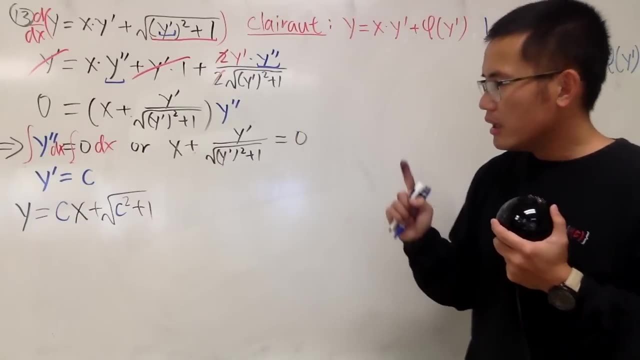 the original one. So keep that in mind. Do not have too many constants. If you only have first order, we can only have one constant. Well, that's going to be really weird, because we still have to solve this right here. Right, Okay. 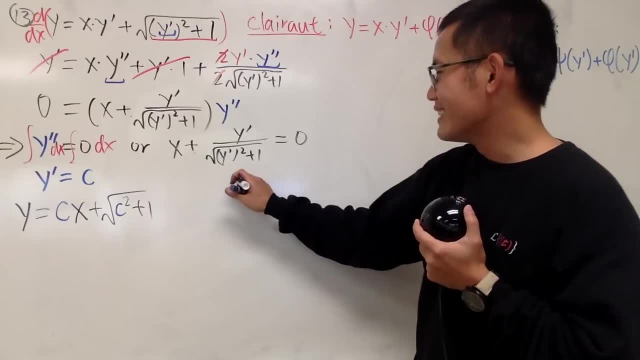 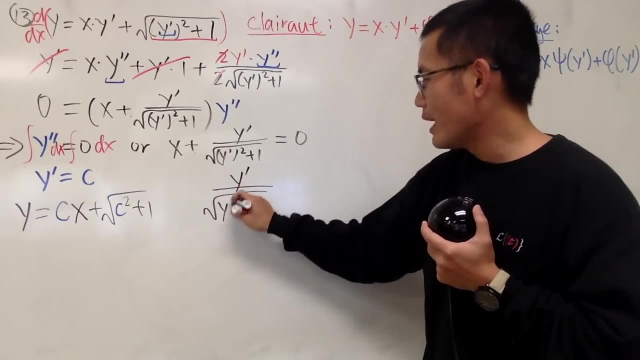 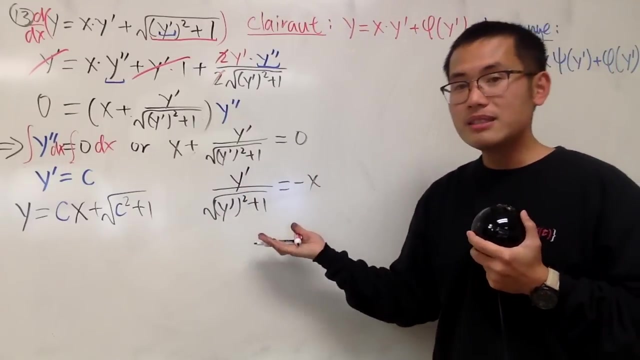 Let's go ahead, bring the x to the other side. This is so weird: y prime and that's divided by square root of y prime, square plus 1, and that's going to be negative x. By the way. does this make sense? Yes, it does. 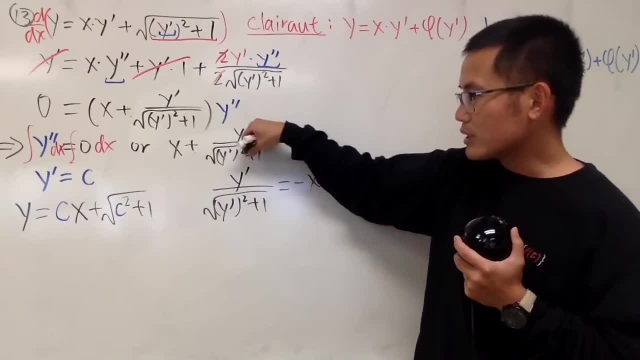 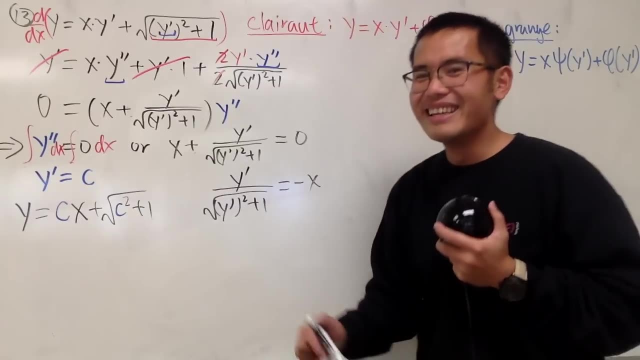 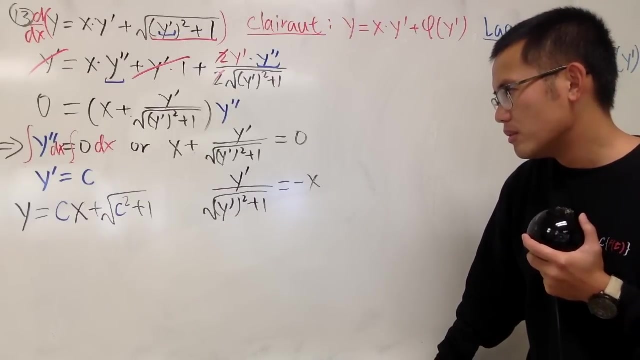 Because y prime could be negative If I just have 1 over square root of something equal to negative x or negative. actually, it still makes sense, because x can be negative, Never mind. All right. So how to do this, though? Well, y prime. 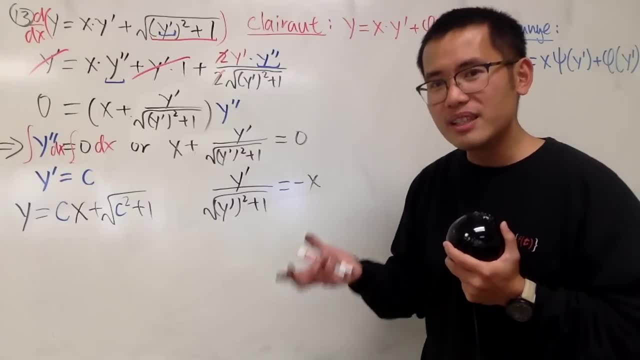 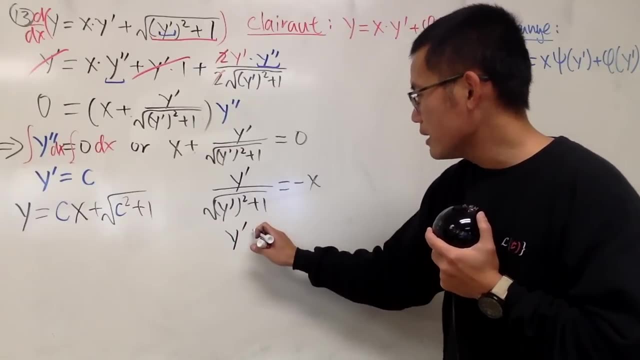 y prime. maybe you can solve for y prime so you can get the dy by itself like the derivative. So here's the deal. Do our algebra Multiplies on both sides. So we're looking at y prime. it's equal to negative x times the square root. 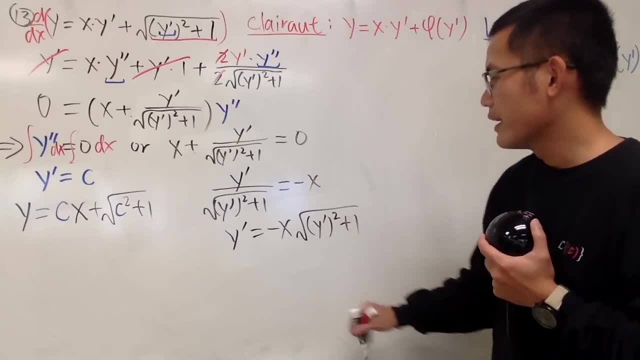 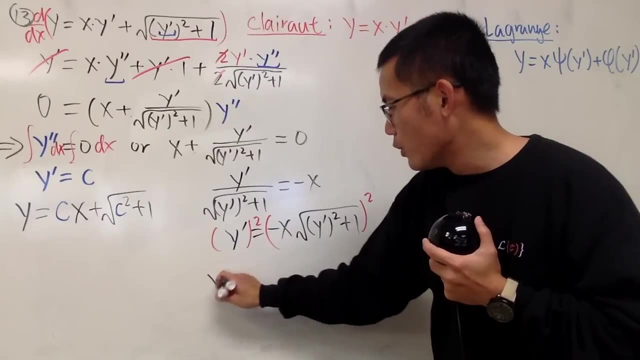 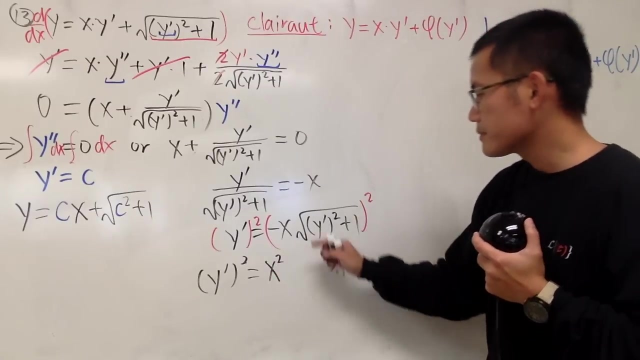 parentheses: y prime square plus 1.. Yeah, And then I will square both sides. Have a look Here: we will get y prime square and that's equal to negative x square. we just get positive x square, square root, square root, cancel. but don't forget. 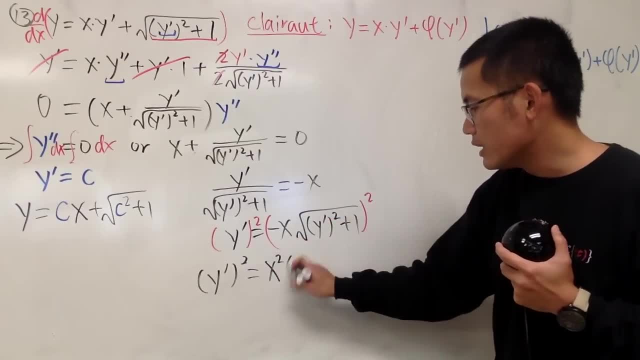 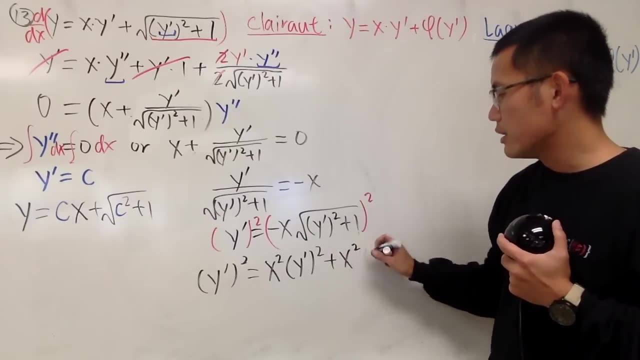 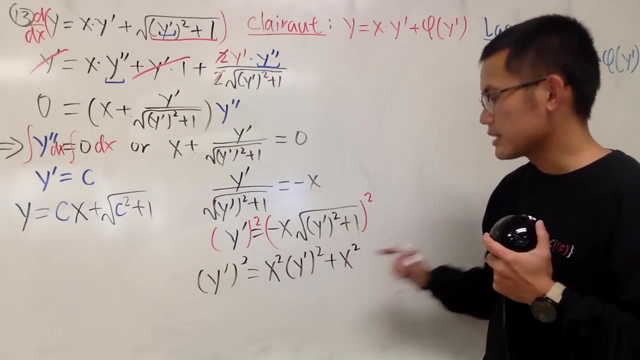 we have to distribute x square, So x square times- this guy is parentheses- y prime square. x square times 1 is plus x square. Again, the negative becomes positive already. So make sure x square, this is the x square, and distribute, distribute. that's how we get that. 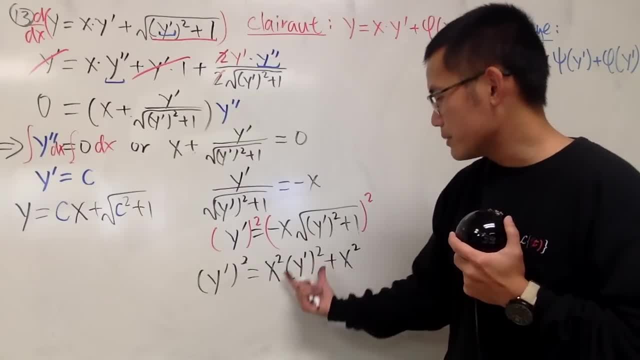 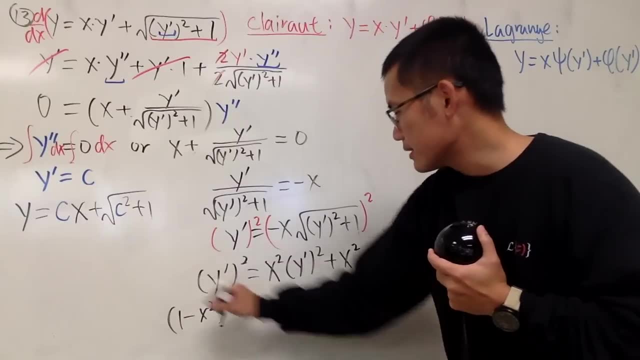 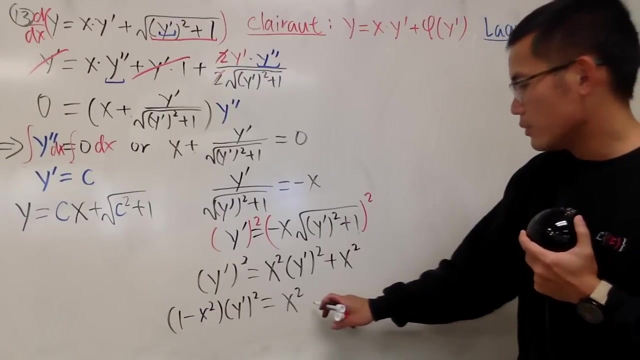 It's very nice because both of them are of y prime, so I can move this to the other side. So I get 1 minus x square right, 1 minus x square, parentheses, y prime square positive, x square, like this, And then let's see: 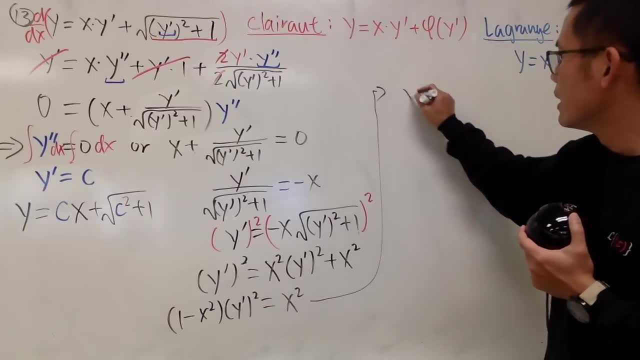 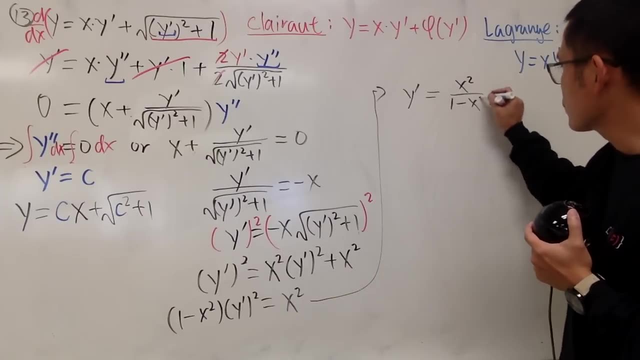 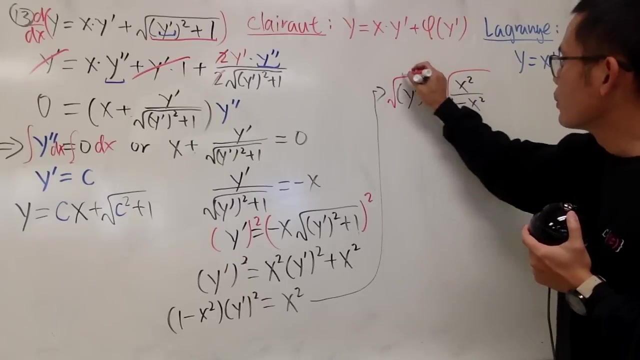 we can just go ahead and do this y prime square. I will write this down first, which is the x square over 1 minus x square. actually, let me just keep that square and then I will just do the square root on both sides. Cancel. cancel. 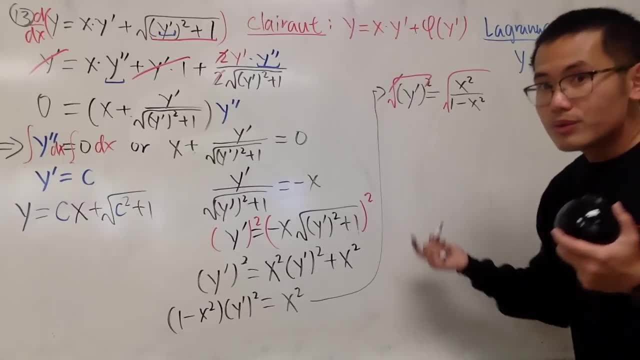 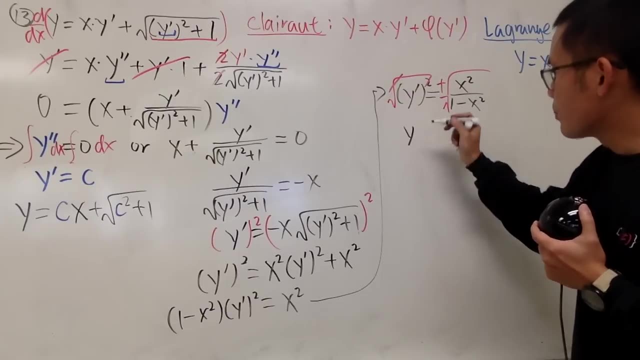 and now you might be wondering: do I need a plus or do I need a negative? the truth is, it doesn't matter. I'll show you both. So let's just keep that. And then we get a y prime, which is just our dy dx. so 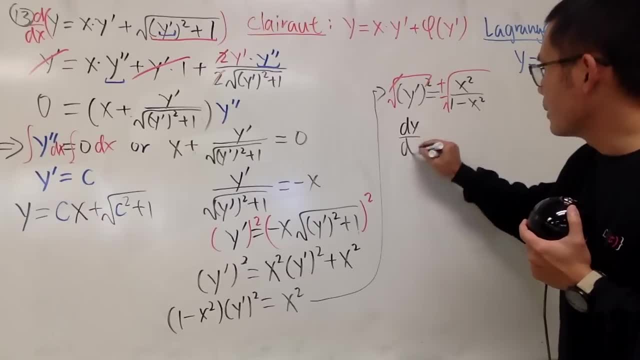 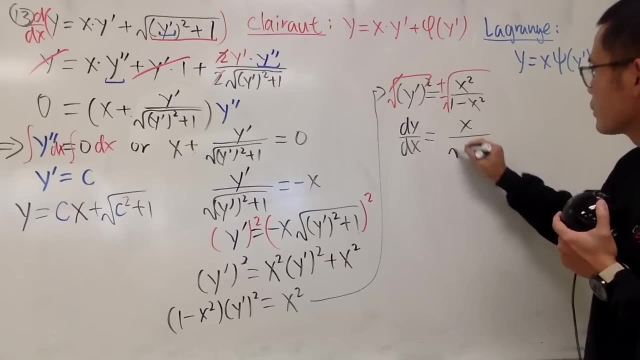 let's perhaps write that down already. This is the dy dx for the y prime. This: take the square root of x square. it's just x over this right here. square root of 1 minus x square. yeah, and then I will still keep the plus minus. 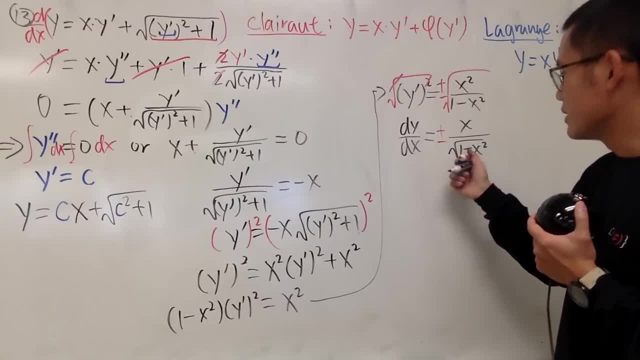 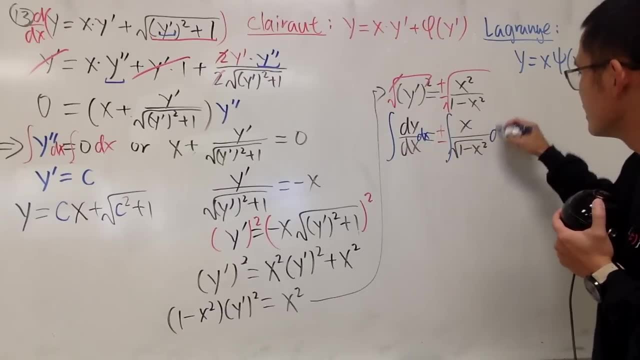 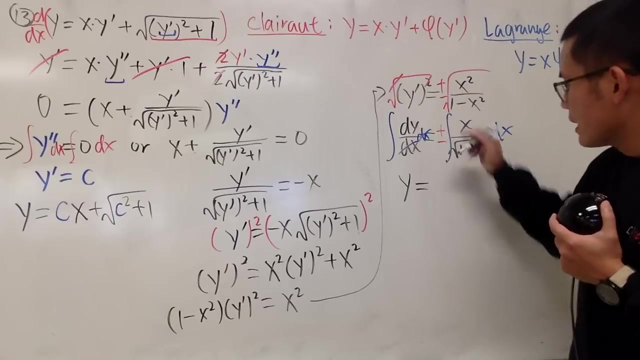 okay, and of course I can just multiply the dx on both sides, so I will just go ahead and do that right here, like this: integrate dx, integrate dx and of course, this and that cancel. Now, based on this, we get y and that's equal to plus minus. 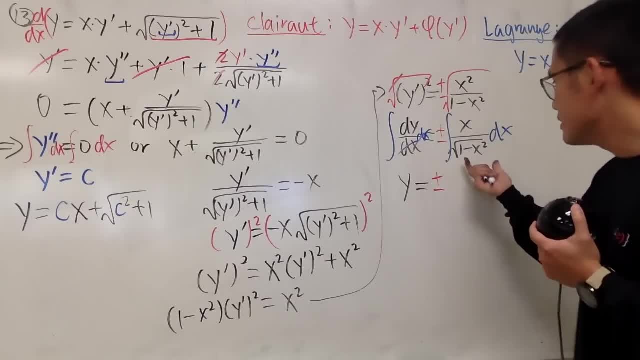 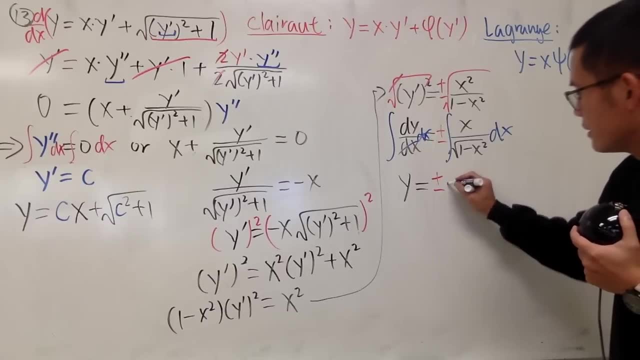 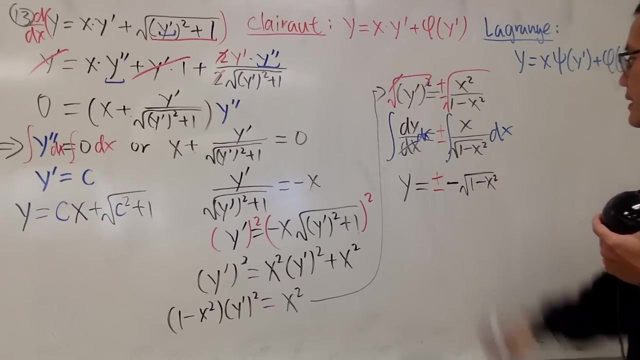 stays, and I'm going to leave this to you guys. you guys can work this out in your head whatsoever. You will end up this integral being equal to negative, being equal to negative square root of 1 minus x square, like this, right? and hmm, let's see. 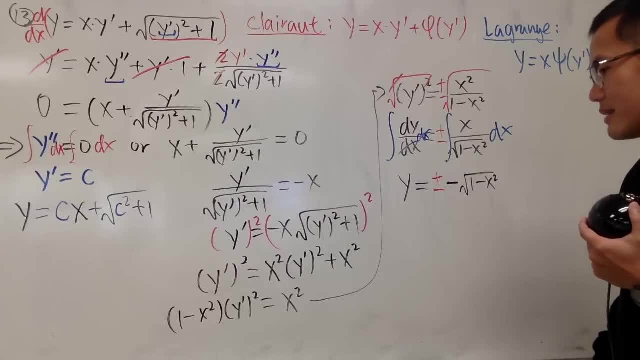 do I want a plus or minus? does that matter? Yeah, it really doesn't matter. it really doesn't matter. and let's be, it's weird, but this part you get negative square root of. but I still have the plus minus in the front. Now, here is the deal. 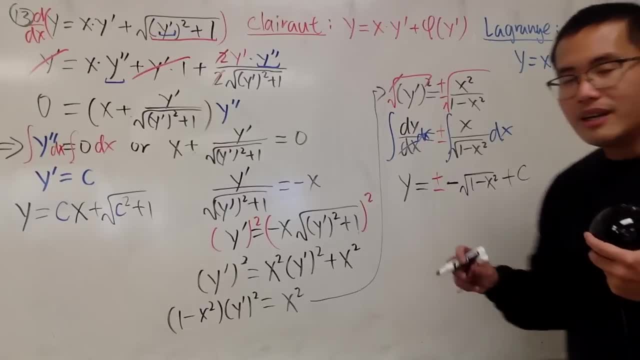 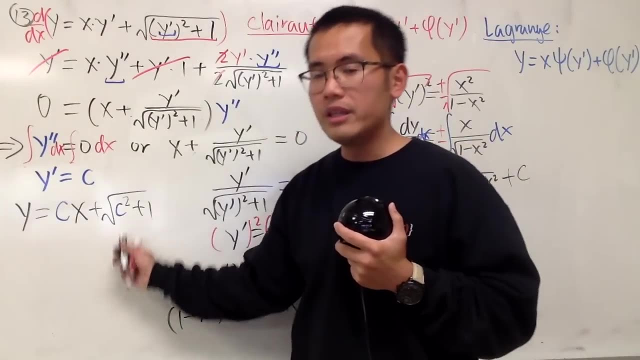 you might be wondering: do I need to put down a plus c? The answer to that is no. the answer to that is no right. Why? Because we have the c right here already for the original differential equation. If you want to put a plus c right here, 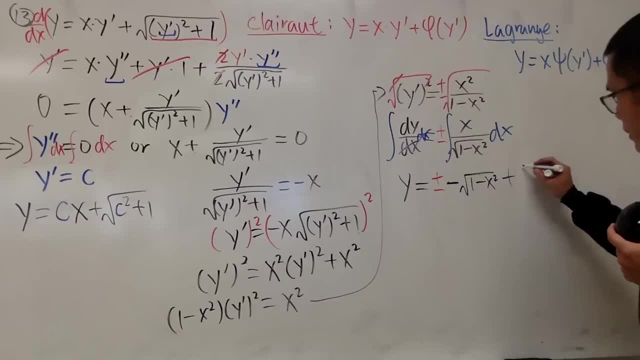 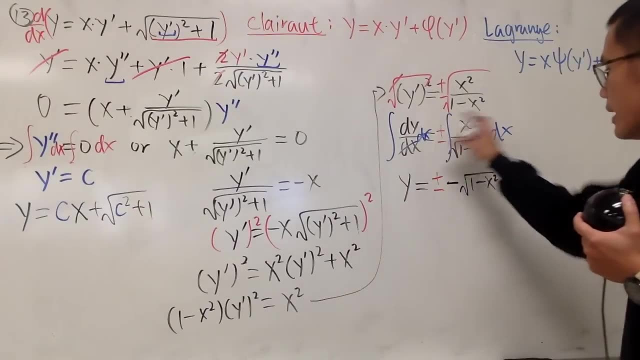 and just not to confuse this c with that c, I will put down plus k for the constant and I will tell you guys that this constant will always be zero, alright, So I will just keep that right here for you guys, if you would like to see that. 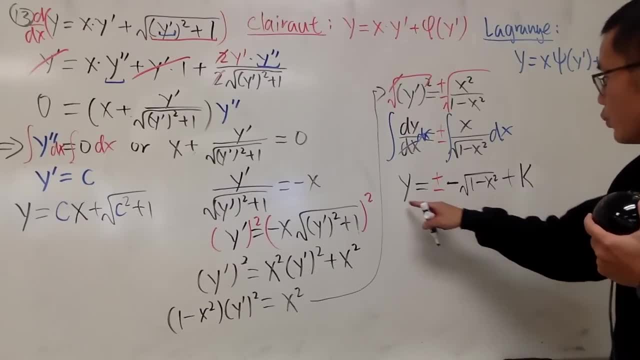 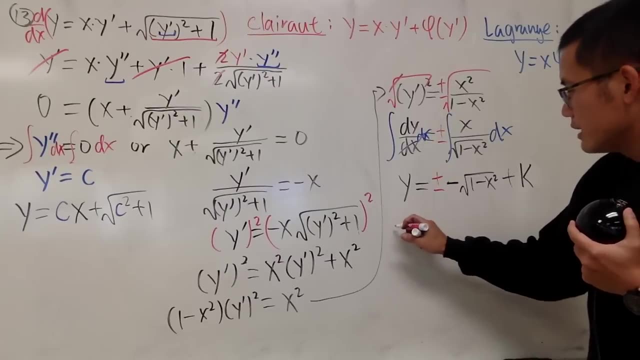 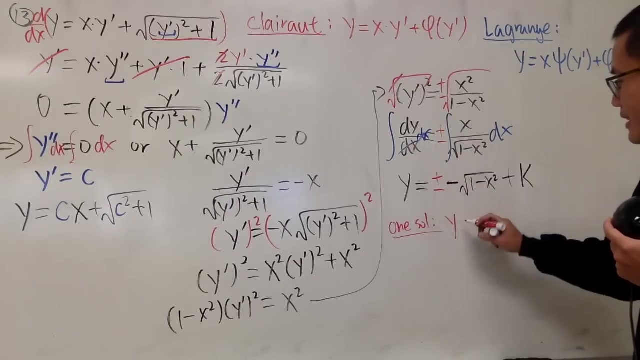 But anyway, here is the deal. we solved it already, yeah, So you can see that we have a solution and let's just take the positive version first. so you can just see that it seems that we have one solution: here is y, and let's take the negative. 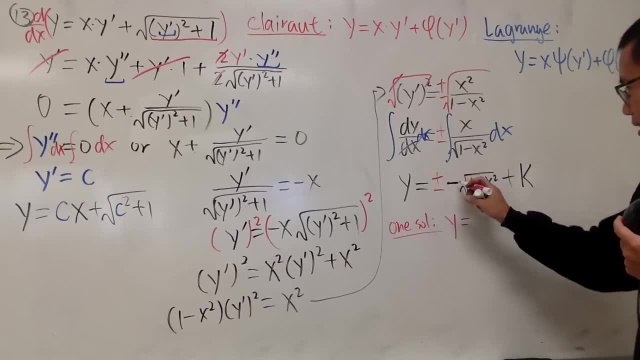 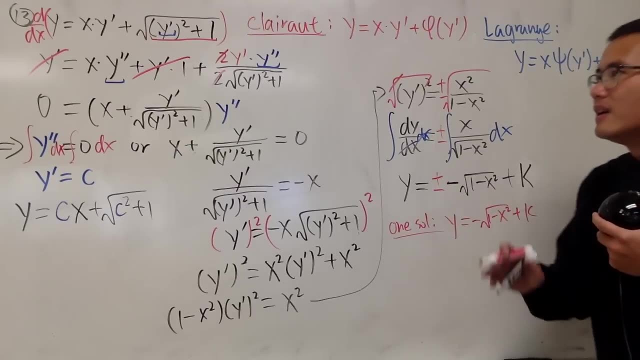 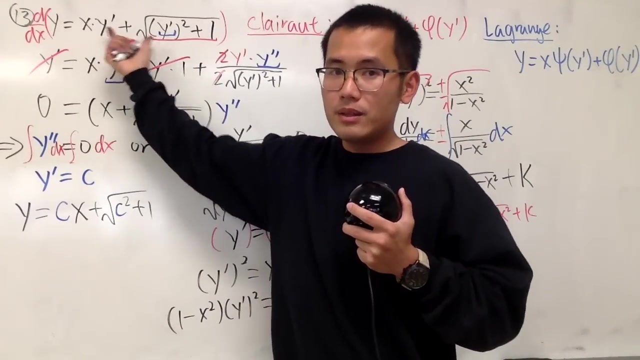 let's just take positive, positive times that. so it's negative: square root of one minus x. squared plus k: yeah plus minus one solution like this. now I will check with the original differential equation, and to do so I will have to get y and then you see the derivative. 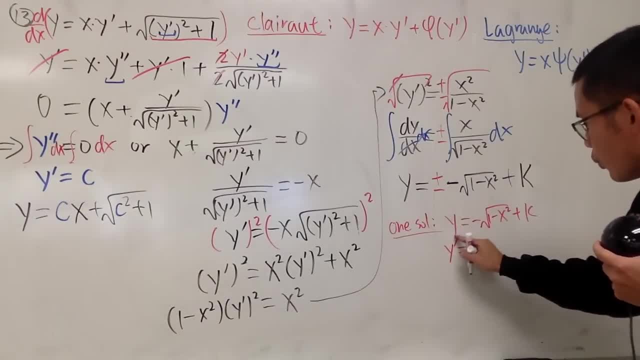 with this being done, you see that y prime, when you differentiate this guy, you get negative and the derivative of this is: over two, one minus x squared, and use the Chengdu and you get negative. two x, yeah, and then negative, negative, cancel, two and two, cancel. 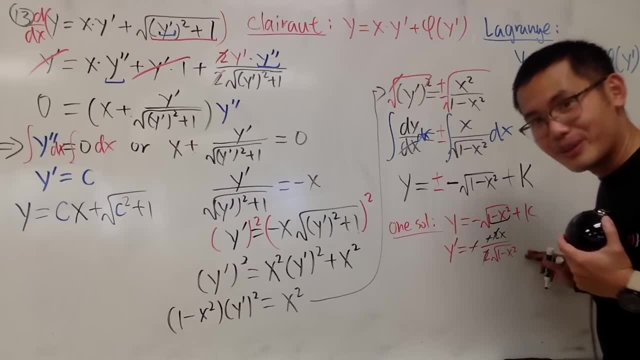 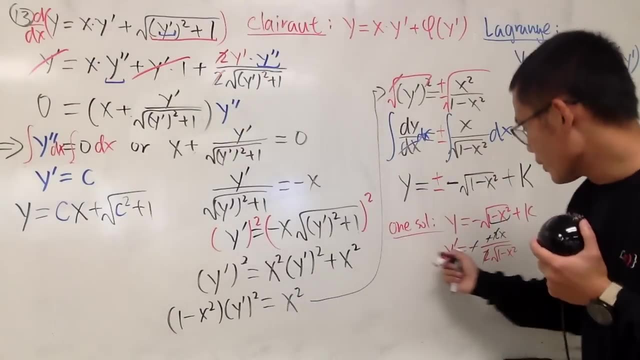 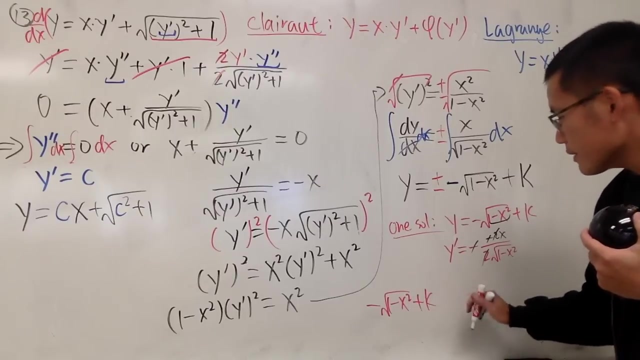 and then the k is zero. right, when you do the derivative. now put this to the left hand side. we will get the y being equal to negative square root of one minus x squared plus k. and then the right hand side: I will have to put the y prime. 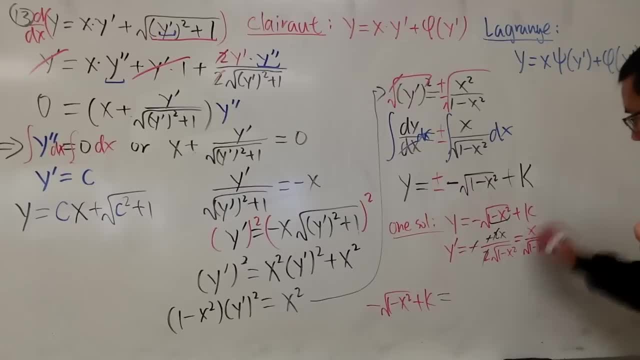 which is x over square root of one minus x squared. this is my y prime. yeah, I will have to put the y prime in here and here. so I get x times x over square root of one minus x squared, and then plus square root of x plus. 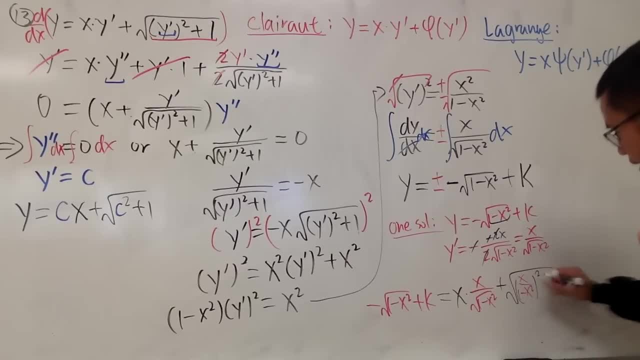 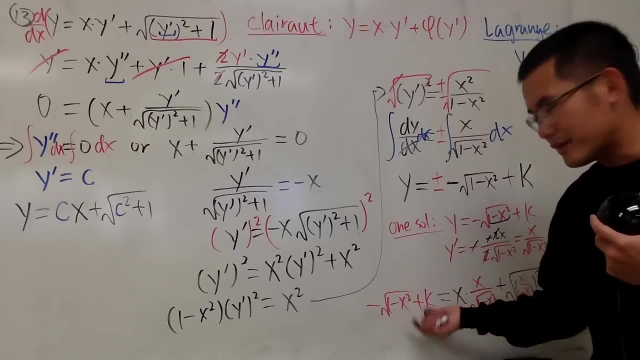 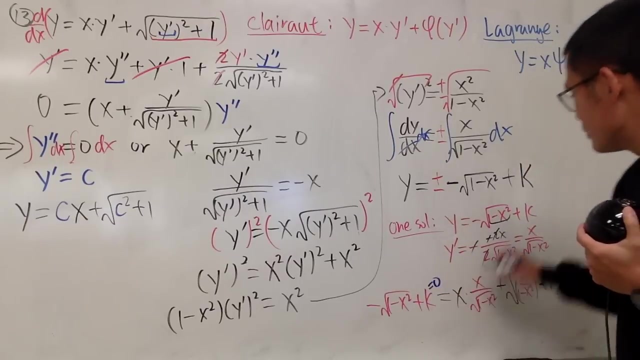 one minus x, squared, squared plus one. right now, on the right hand side, you have no k. on the left hand side, you have the k. there is no way for k to be a whatever number besides zero, so hopefully you can see that the k right here is zero. 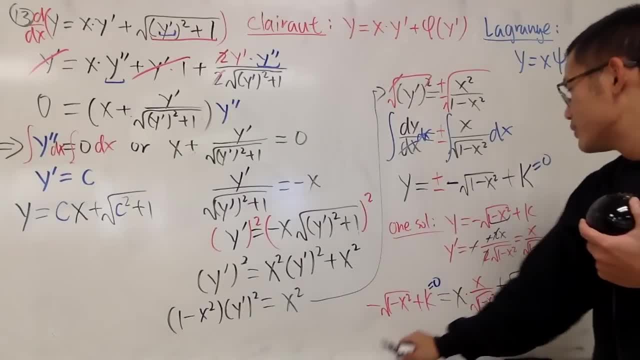 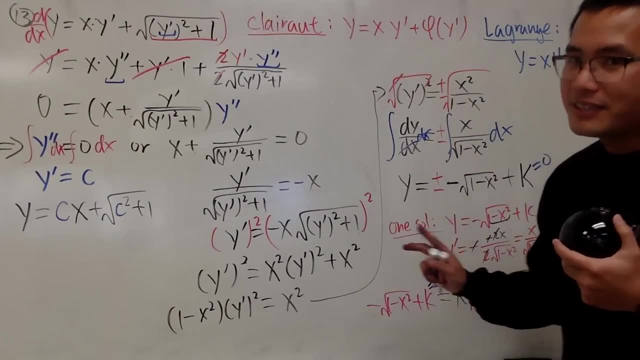 the k right here has to be zero right, so you actually don't have to do this part, the k part. so just keep that in mind. this right here is a strange situation, so I'm going to just pause for a little bit. look over this right. 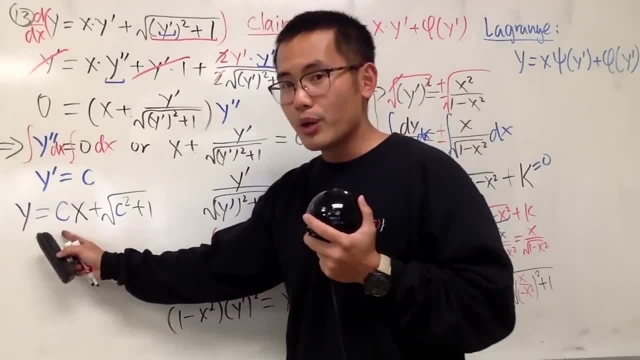 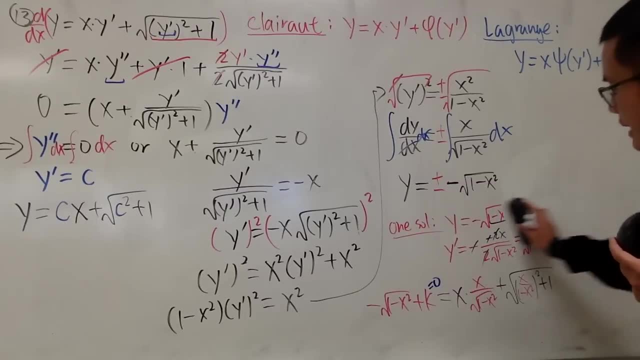 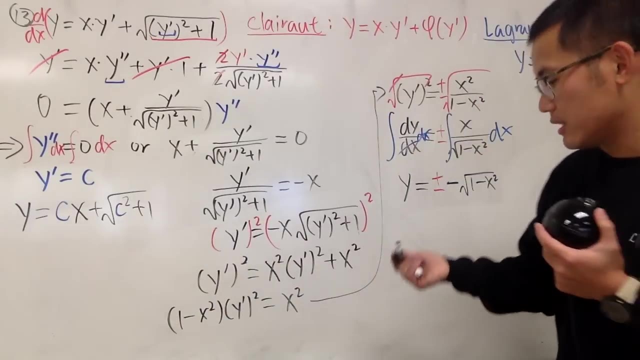 and I will erase this part. first thing is that when you have the c right here already, even though you integrate both sides, do not put down another constant anymore. okay, so this, finally this, and that they actually have names. this solution is actually the general solution, as usual. 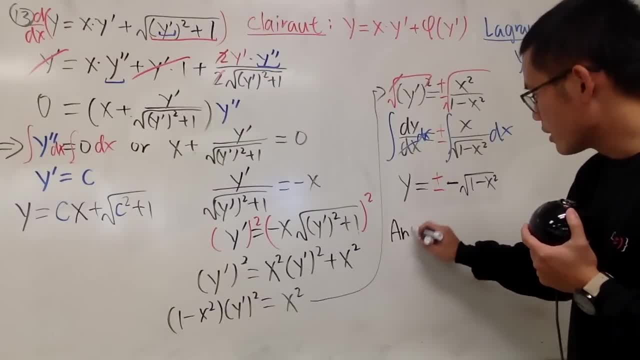 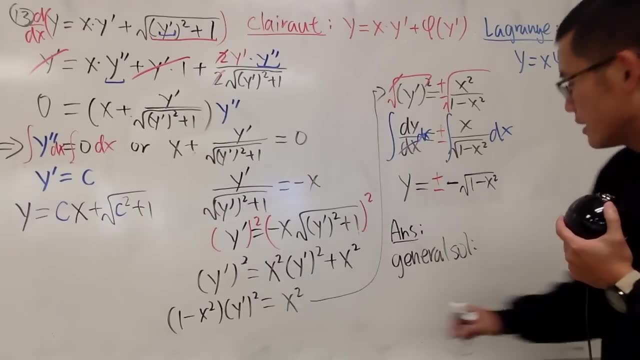 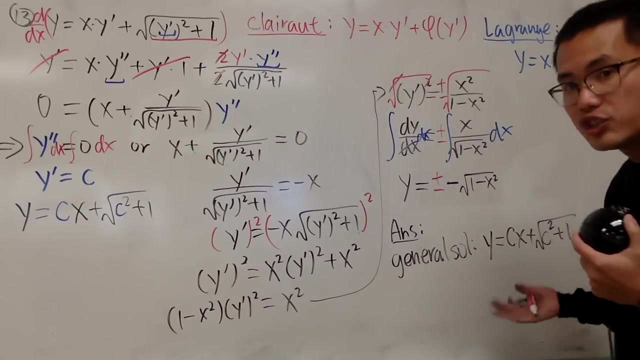 you have the c, so here I will just write this down right here for you guys. the general solution is that, namely, y equals cx plus square root of c squared plus one. this, right here, is the general solution. and what's this, though? this is kind of like. 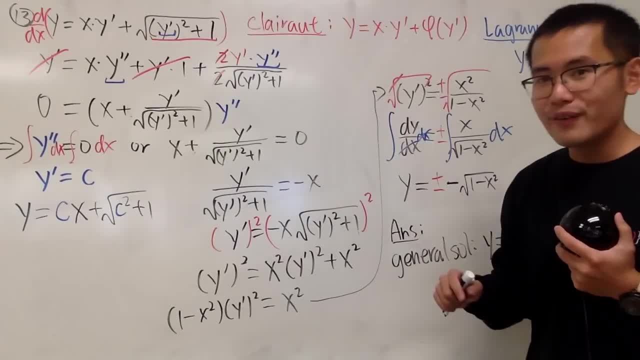 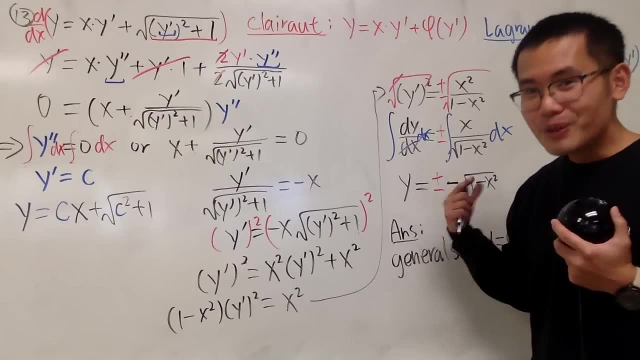 the missing solutions that we were doing earlier in question twelve. that's why I spent the time to give you guys some warm up for the missing solution idea. but this right here has a cooler name. this right here is called the singular solution, and let me just write this down. 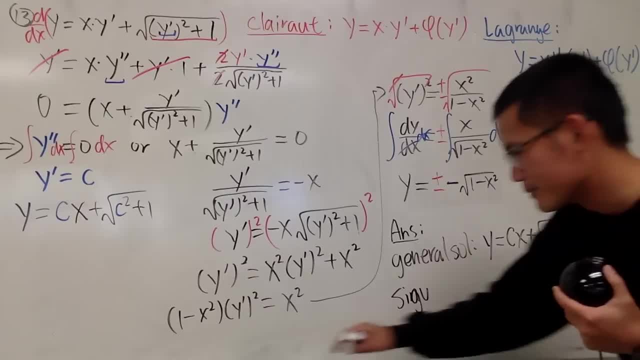 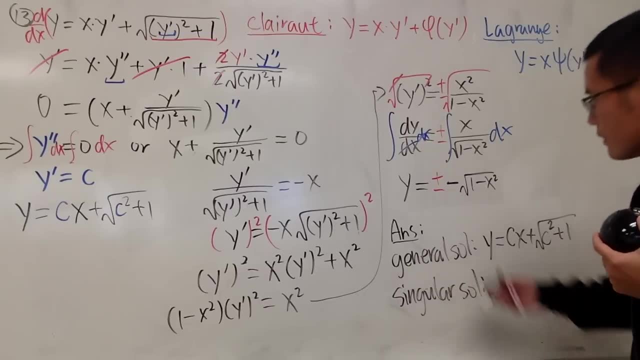 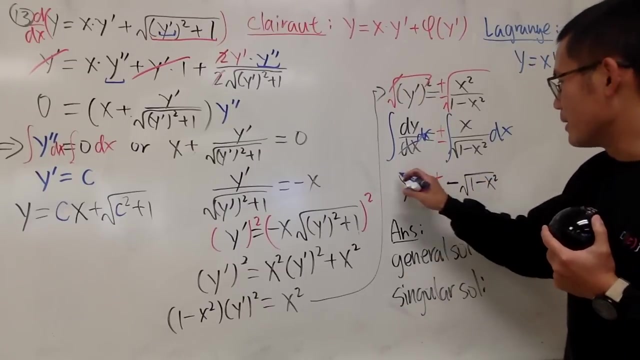 sin, not even sin sin. no singular solution, which is just this. but have a look here. you see that I was kind of like worried about if I do the plus or minus, don't worry about it, let's just square both sides for the function, though it was the derivative earlier. 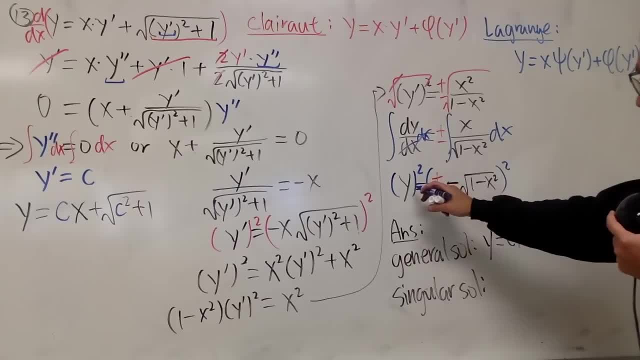 now I'm squaring the function. you will see that this is going to give us y squared equals. now don't worry about the plus minus anymore. this is just going to be one minus x squared, and of course, you can move the x squared to the other side. 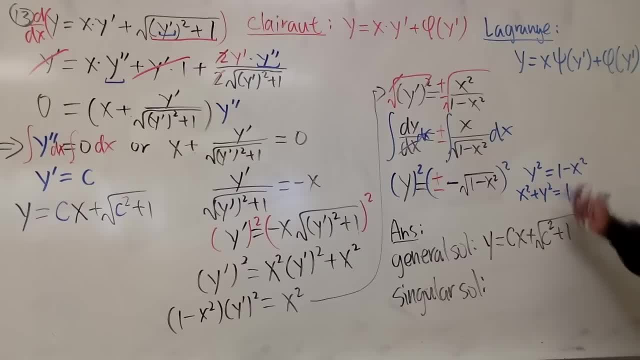 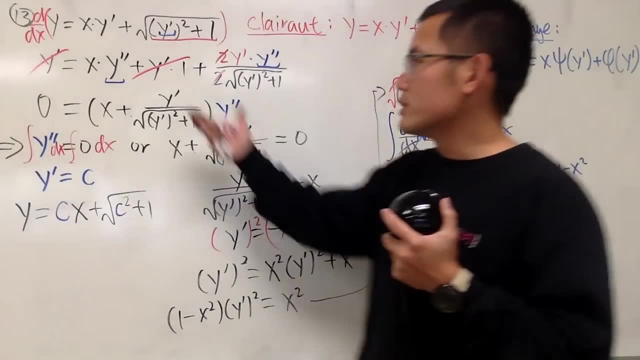 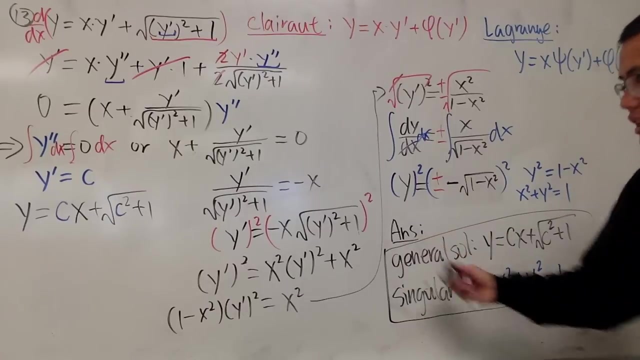 x squared plus y squared is equal to one. this is the singular solution: x squared plus y squared is equal to one. when you are dealing with a clear, old differential equation, most likely you actually have to find both the singular and also the general solution. you might notice that 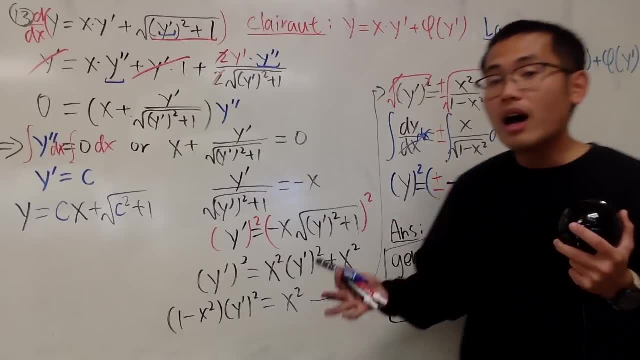 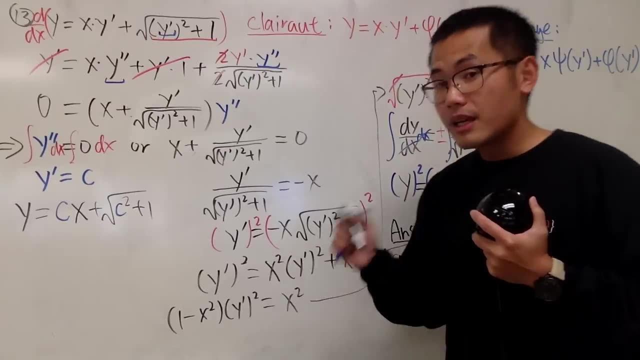 this right here is a circle, this right here is a bunch of lines. what are the connections? well, hopefully I will use that space. that's enough space for me to explain all that. so here is the singular solution, which is just a unit circle. I will just put that down. 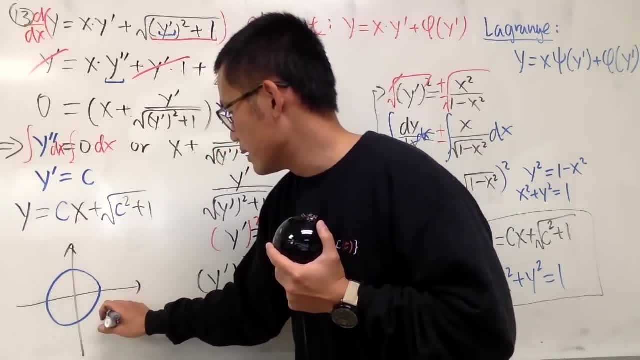 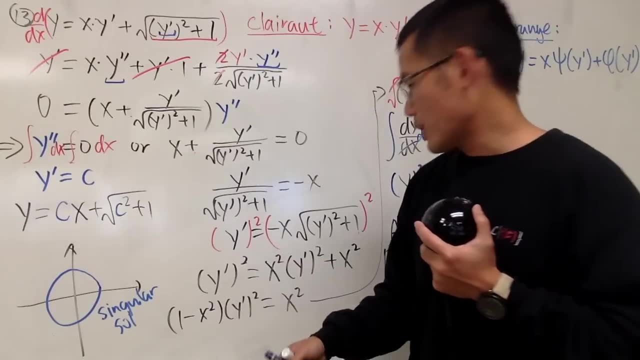 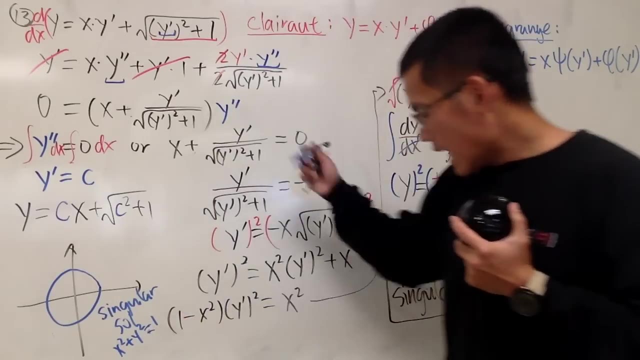 right here for you guys. this is the singular solution, which is: x squared plus y squared is equal to one. so x squared plus y squared is equal to one. very nice. now, in our situation, we actually do not have an initial condition, so I don't know what the c actually is. 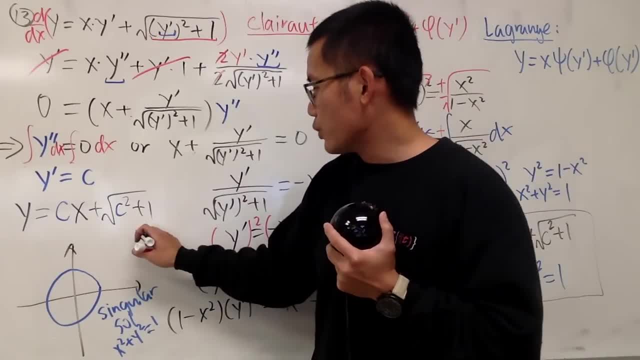 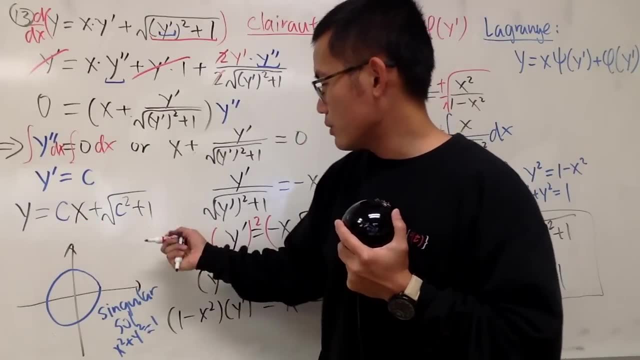 but if you pick whatever c you want, if you have c is equal to one, then you will get y is. let me see. if you have c is equal to one, let me see if I can do this right. if you have c is equal to one, then you are saying: 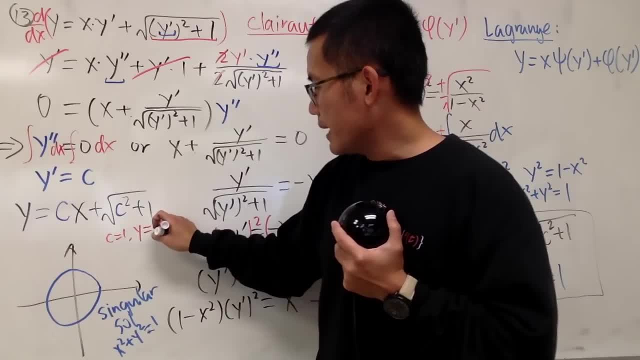 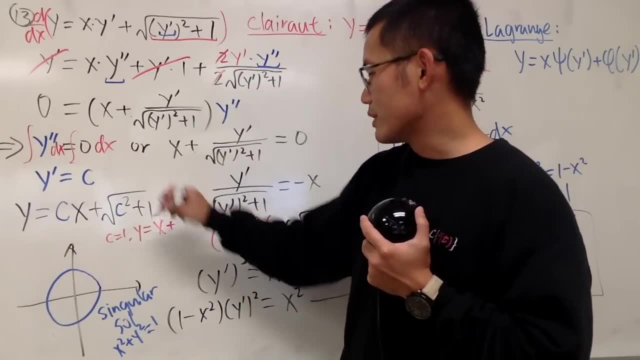 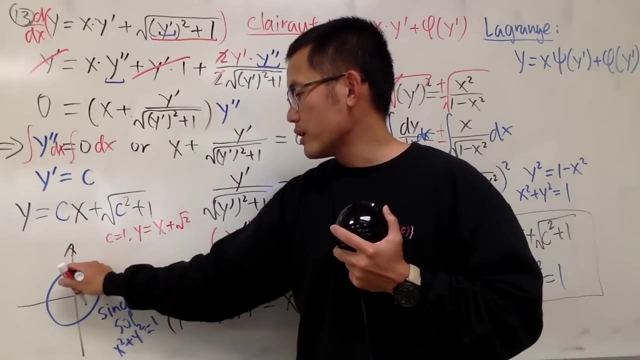 y is equal to x. yeah, you are talking about x plus one. squared is just one plus square root of two. so square root of two is about right here, because this is this is one right here. so square root of two is right here. one is the slope. 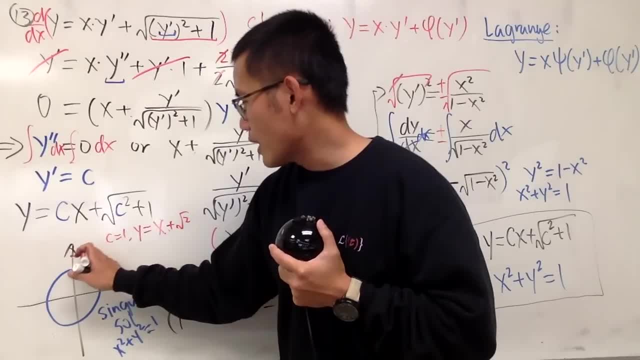 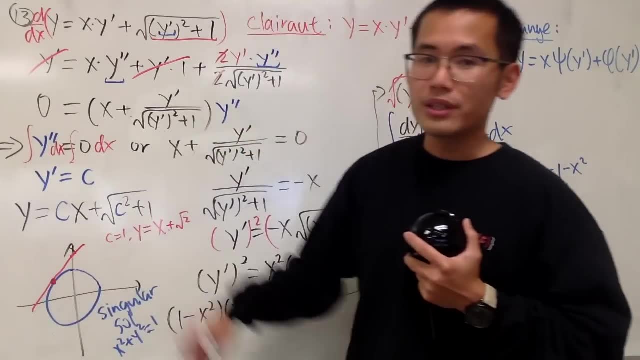 of course, and if you graph it, you will get, and if you graph it, in fact, you actually get this. and the truth is, this line will be tangent to the singular solution. and if you pick another c- let's say c is equal to zero- then this is zero. 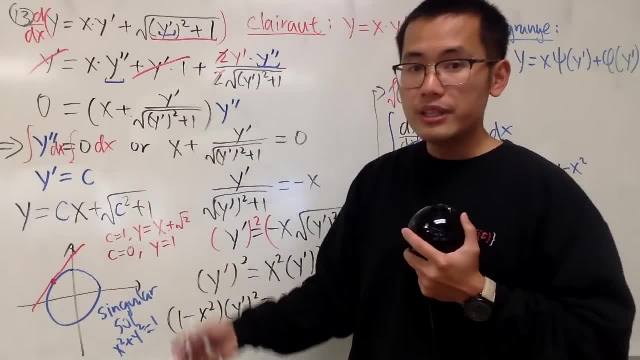 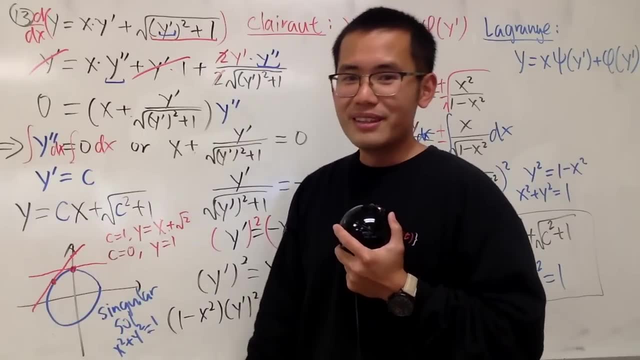 so that means y is equal to one. yeah, and you actually get a horizontal line, and of course they will touch each other right here, because, uh, that's a unit circle and if you pick c is equal to negative one, you get y equal to negative x plus. 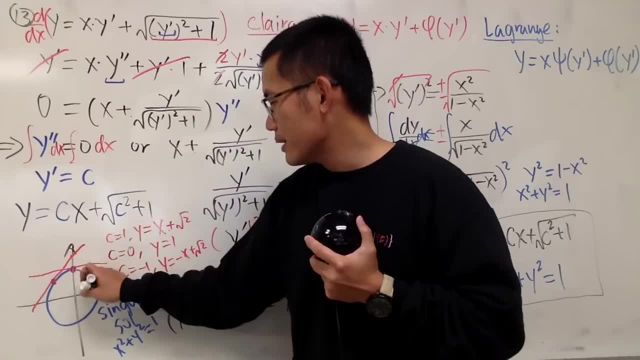 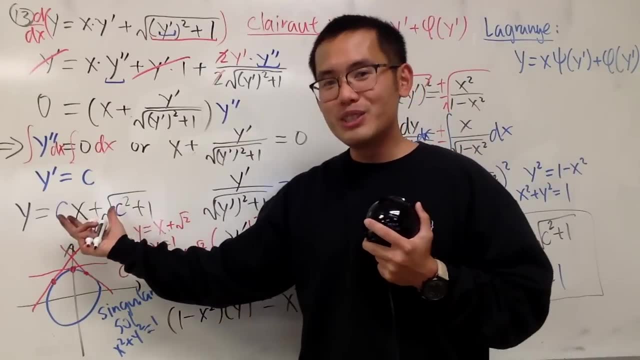 square root of two. that's just like this, but the other side right, and then you can just do like that. the idea is that you can just pick whatever c you want and the line will be tangent to the singular solution. very cool stuff, in this case, we call that. 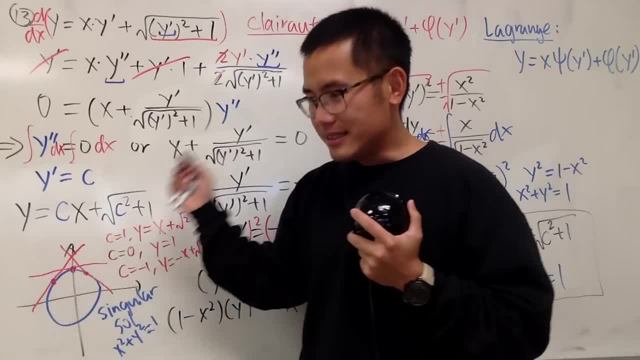 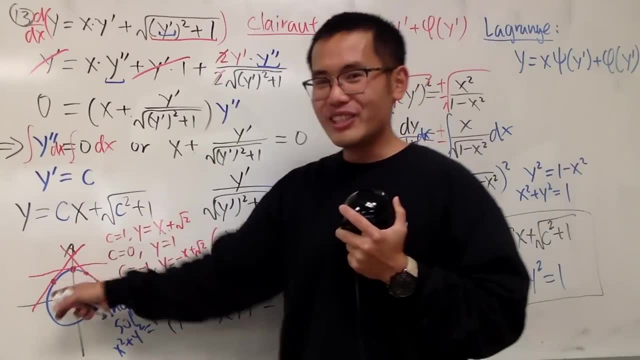 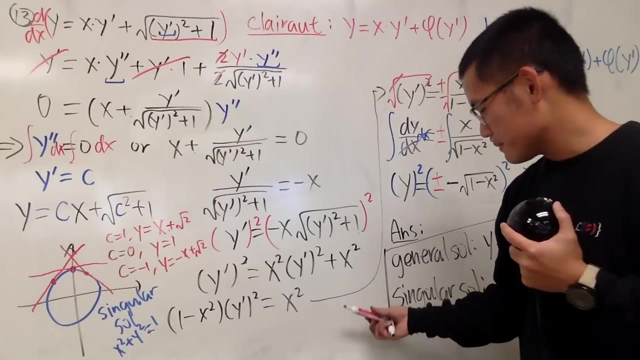 this right here. it's an envelope with our. this is the envelope with the for the for the general solutions. it's just like everybody in the general solution, everybody in the family, uh, it will just be tangent to the singular solution. very cool stuff, yeah. so that's pretty much it. 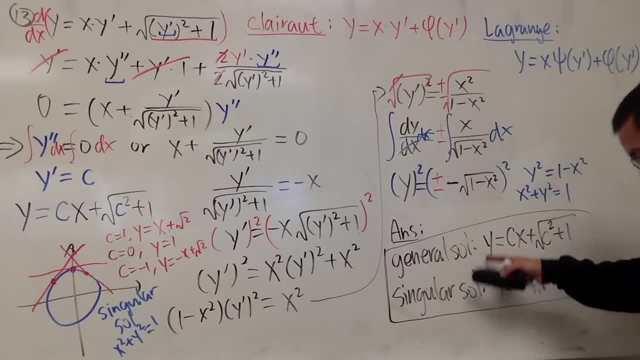 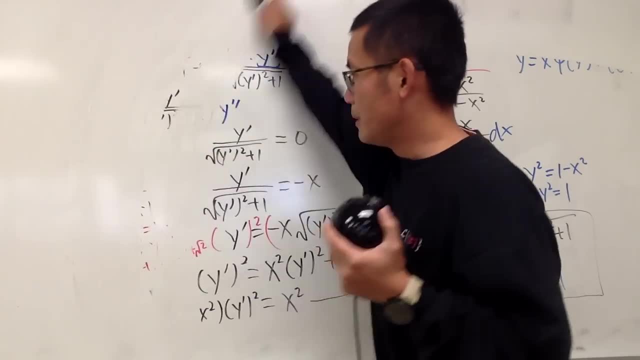 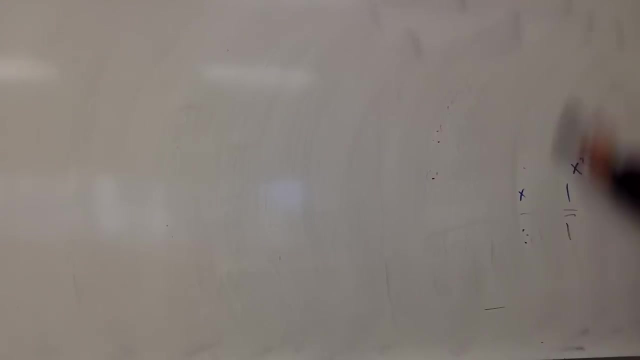 right, that's pretty much it right. so that's it. but most importantly, do this and do that, all right. so, again, that took a while, but, um, maybe you haven't seen before, so i want to just show you guys that one, which is some really cool stuff. 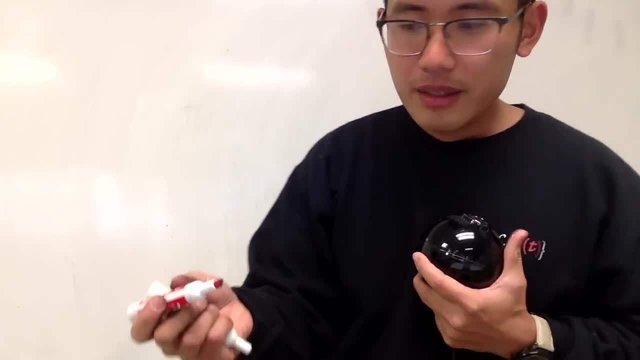 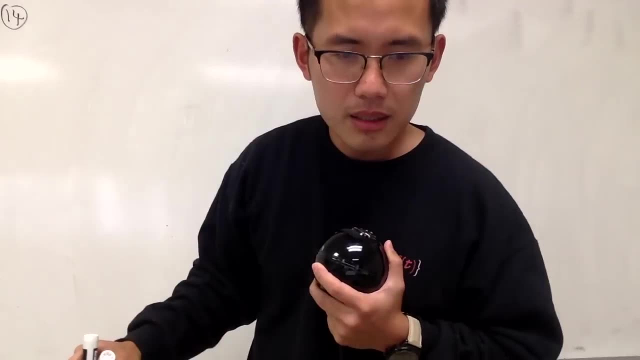 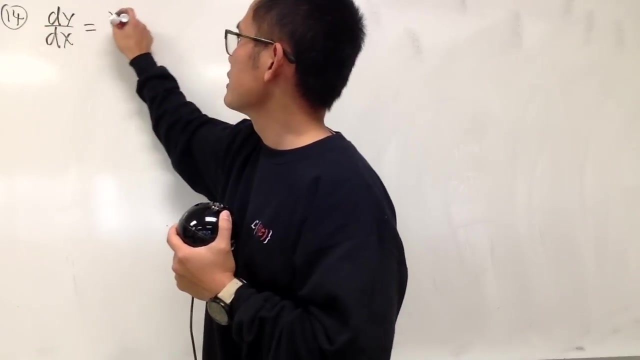 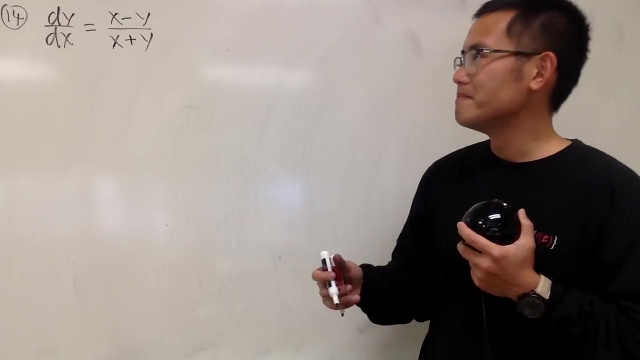 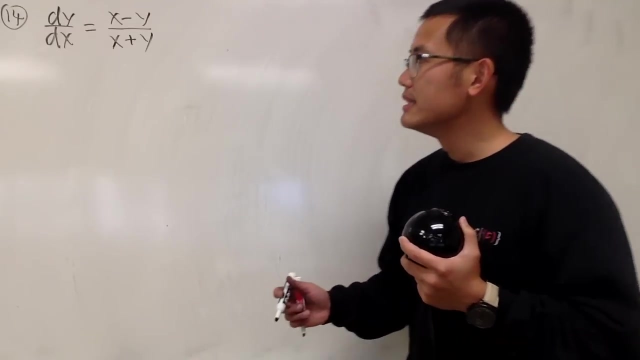 number 14: ah, this one looks pretty nice. dy tx- that's equal to x minus y- over x plus y, looks innocent. yeah, um, not so much. um, what's this? is it exact? uh, you can try it, and i think it's actually exact, but i want to show you, guys, another way. 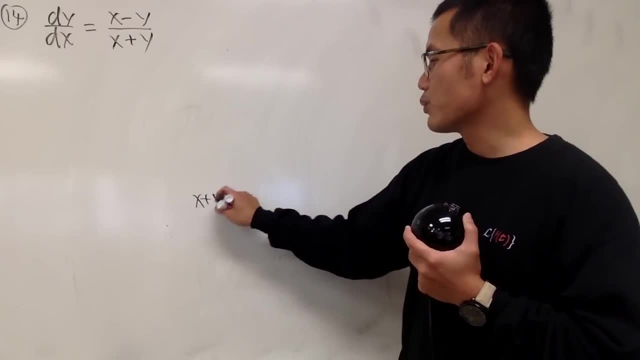 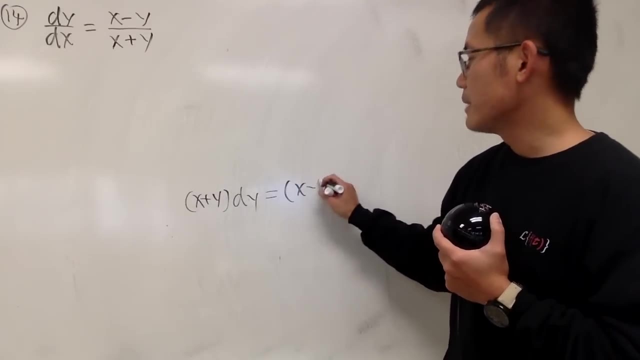 so in fact, if you try it, you will see this is x plus y and then you have the dy right if you multiply down both sides, and that's equal to parentheses, x minus y, dx, and you can bring that to the other side. so it's x minus y. 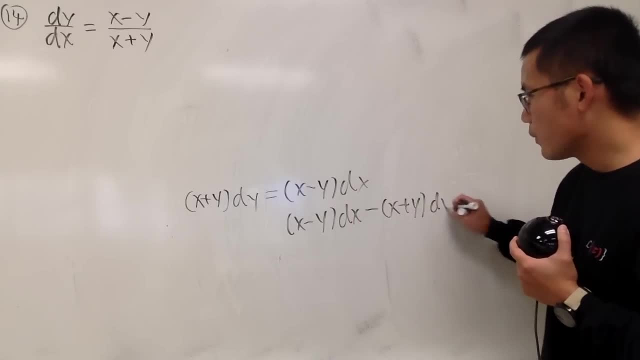 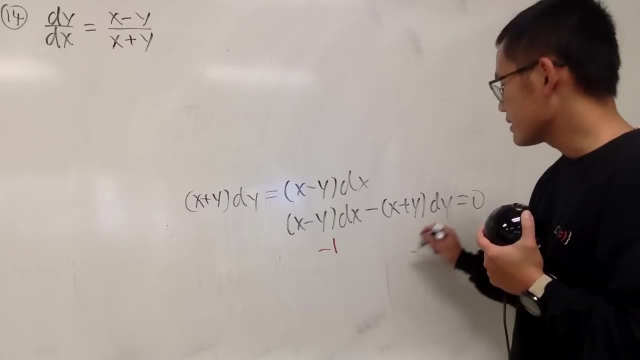 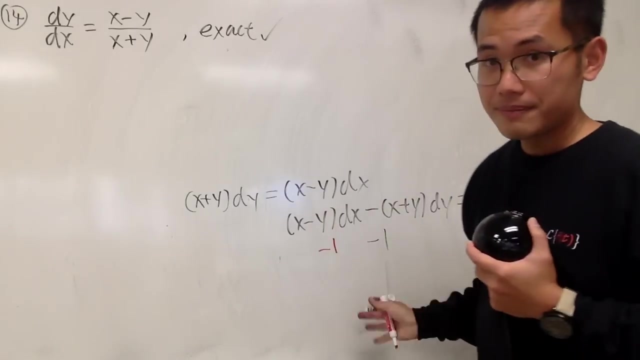 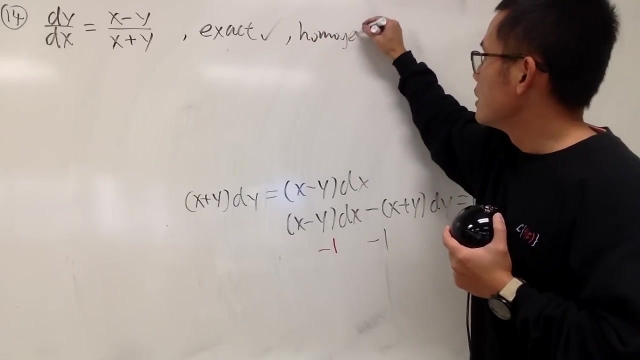 dx minus x plus y dy, equal to zero. differentiate this with respect to y: you get negative one. differentiating this with respect to x, you also get negative one. so this right here is exact. right, it's exact, but this right here is also homogeneous, and in fact, 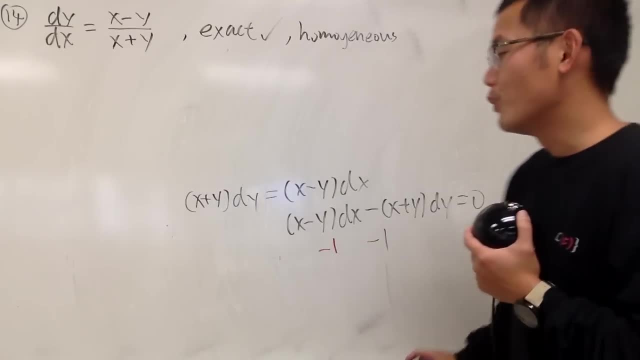 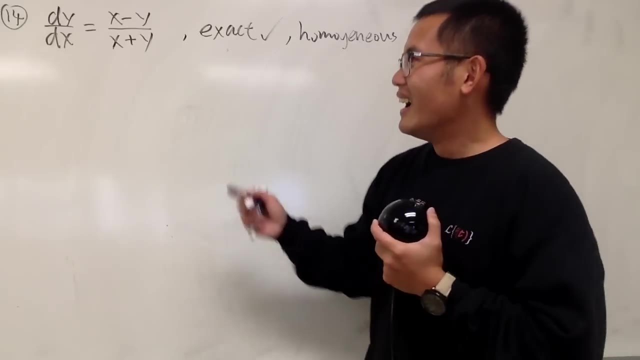 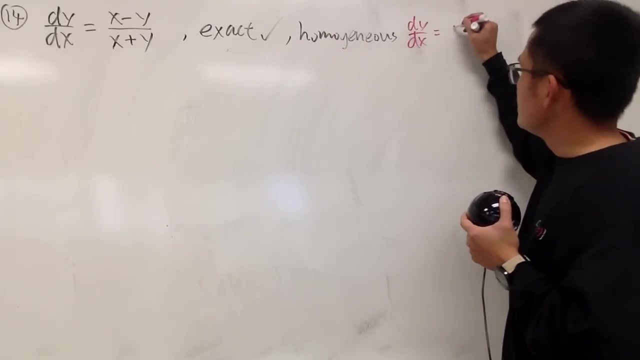 let me show you, guys, how we can do this with the homogeneous way to do it right. just have some extra practice with the homogeneous differential equations. all right, here is the deal for homogeneous differential equation. our goal is to have dy dx to be a function in terms of 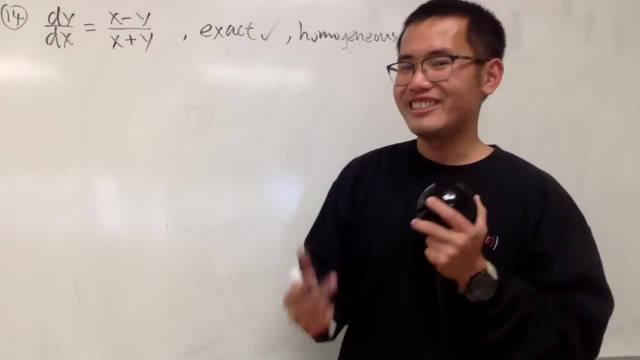 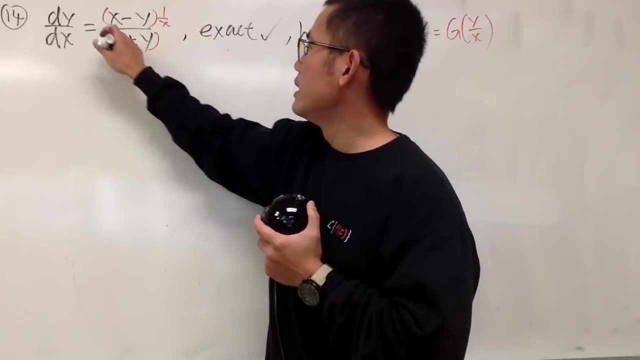 y over x, isn't it? yeah, so on the right hand side, we have to make some change. all we have to do is divide everybody by x, so i'll just go ahead and do this and do that, just on the right hand side, of course. then you see that. 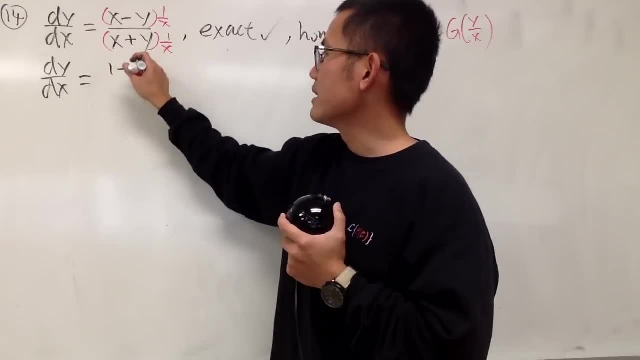 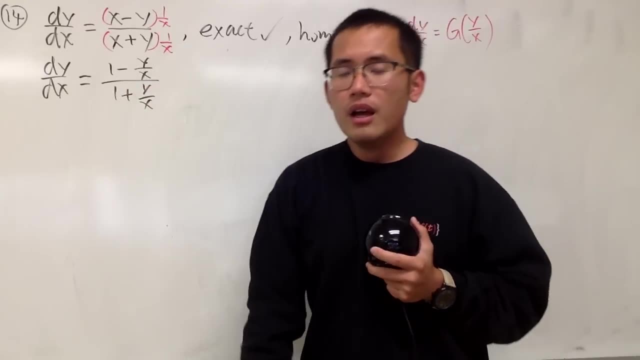 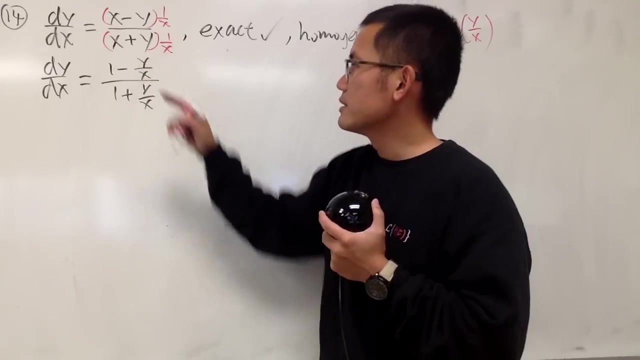 we have dy, dx, this and that is one minus this, and that is y over x, this and that is one, this and that is plus one, i mean y over x, and exact might be easier, but again just for extra practice for the homogeneous differential equation. so here is 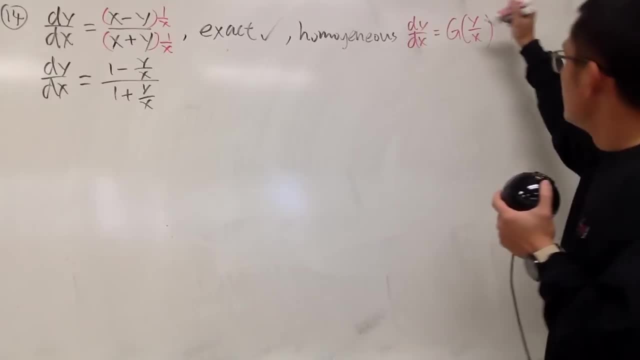 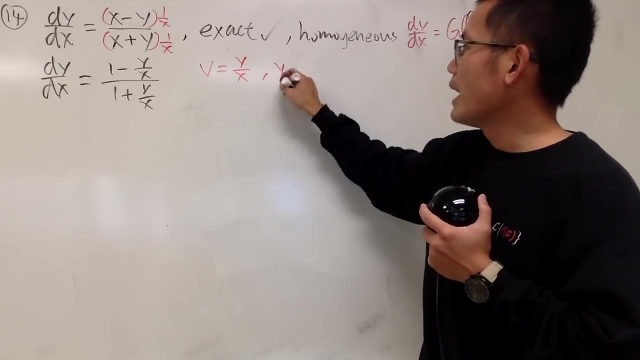 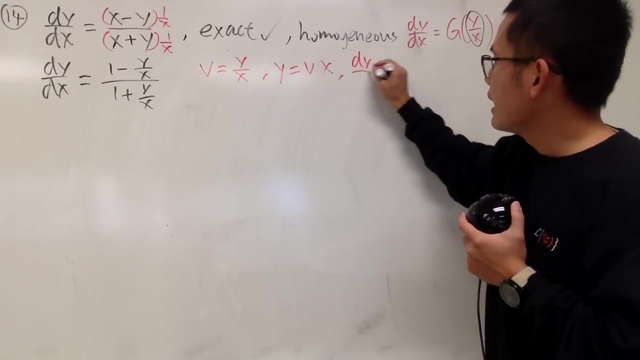 the deal right here. i'm going to do the substitution right, so i will just say phi is equal to y over x. so in another word, y is equal to phi times x. so here we know. let me just write it down right here: dy, dx is equal to: 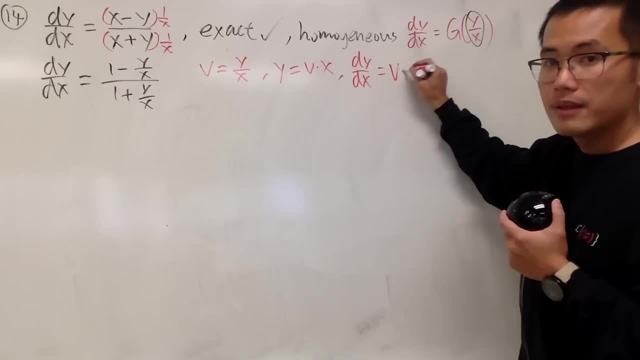 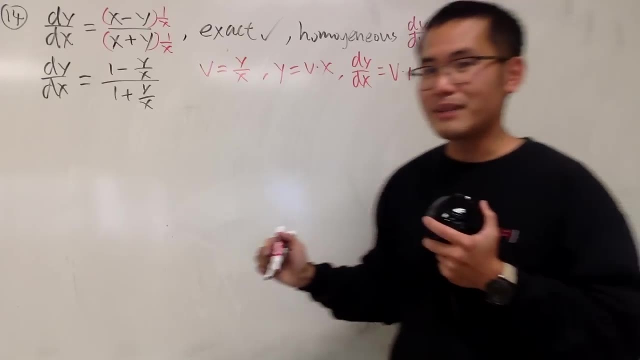 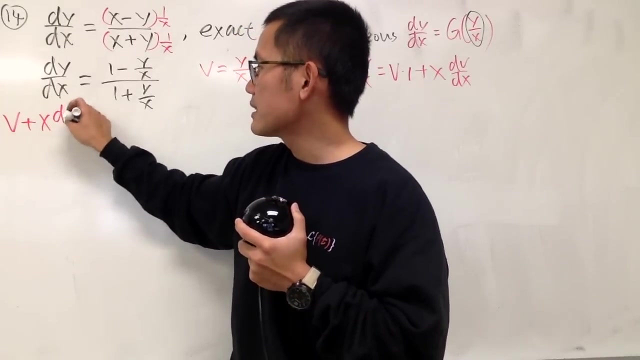 product of the action. so first function times the derivative of the second, plus the second function, which is x times the derivative of the first. same stuff, like last time. now, okay, go ahead and get to work. dy dx is v times one plus x times dv dx. great, 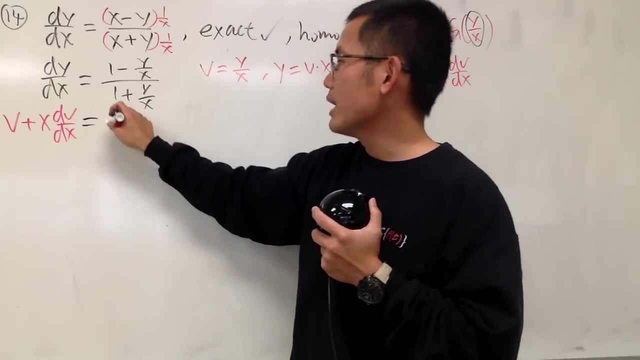 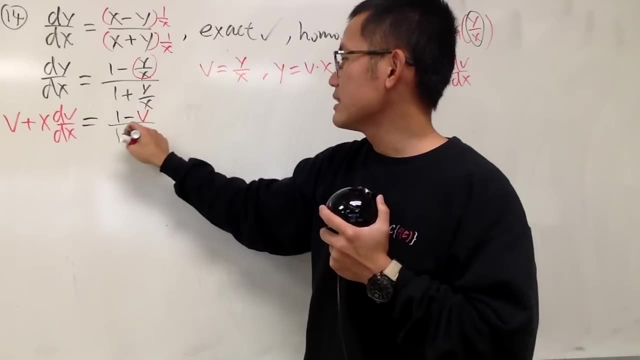 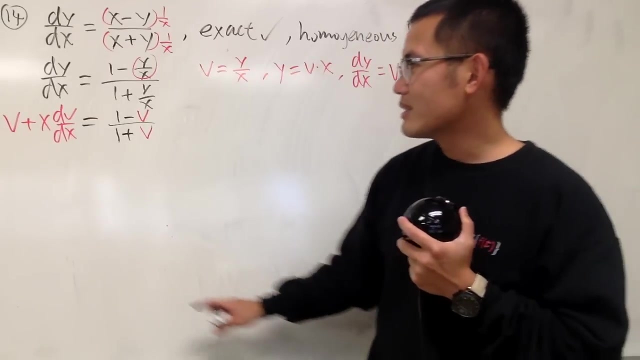 now, on the right hand side, this is equal to: on the top, we have one minus on the here is phi. on the bottom, we have one plus this right here is phi, just like that. and i promise you, this is a separate differential equation. but to do so, though, 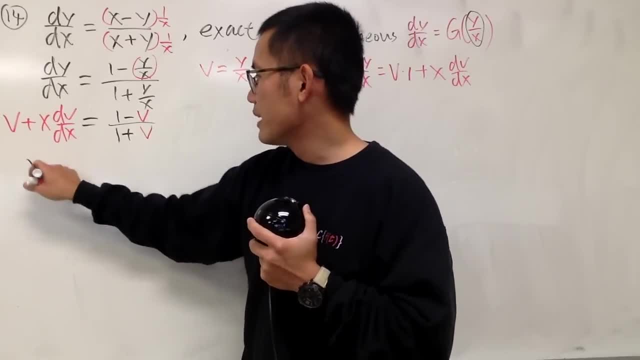 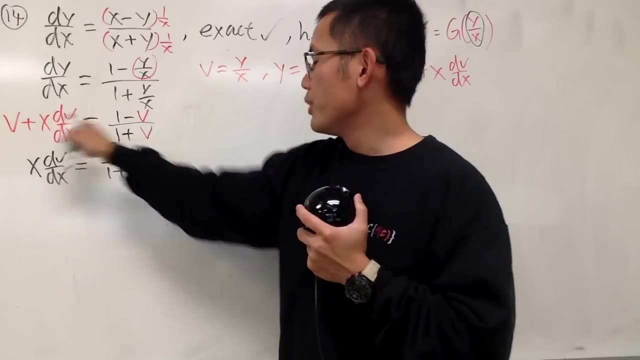 we have to actually bring the phi to the other side. so we are looking at x, dv, dx. that's equal to one minus phi over one plus phi. bring the phi to the other side and again, of course, we have to get a common denominator to combine these things. 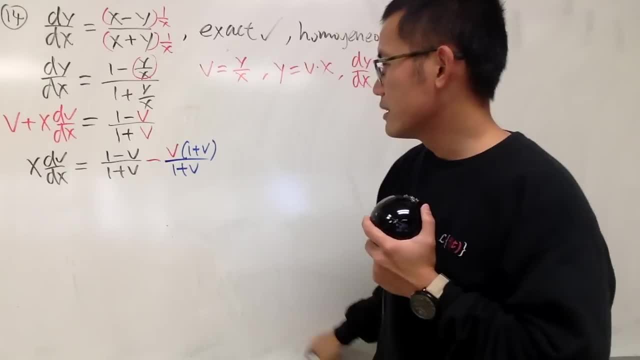 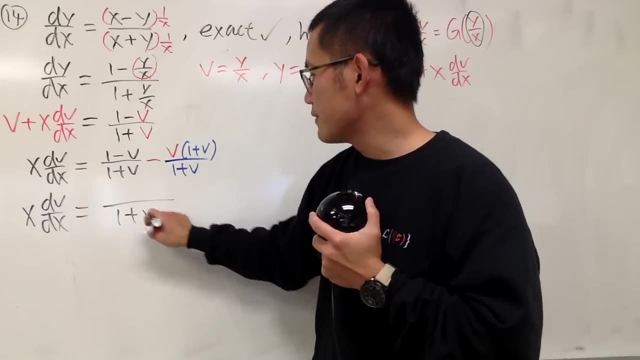 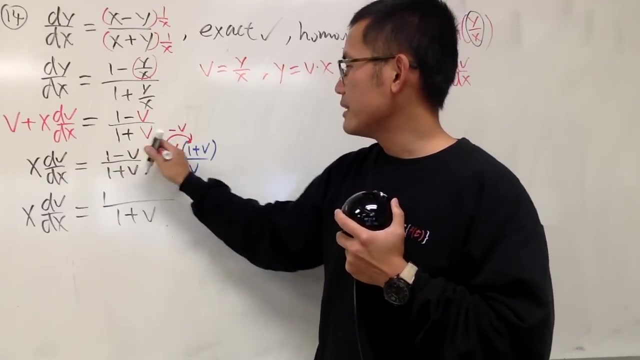 so one plus phi and one plus phi, and here we have x, dv, dx, that's equal to one plus phi. this is one minus phi and then another minus phi. yeah, so we have minus two phi. so just keep that in mind. and then we have this times that 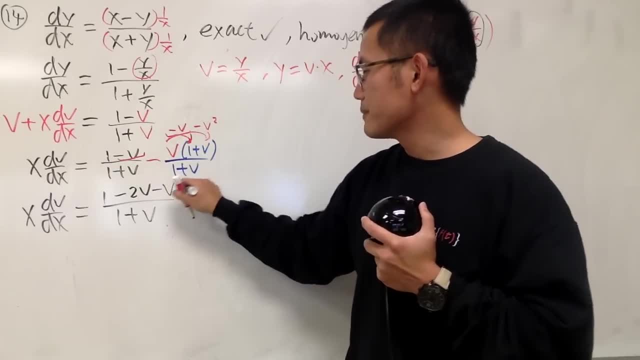 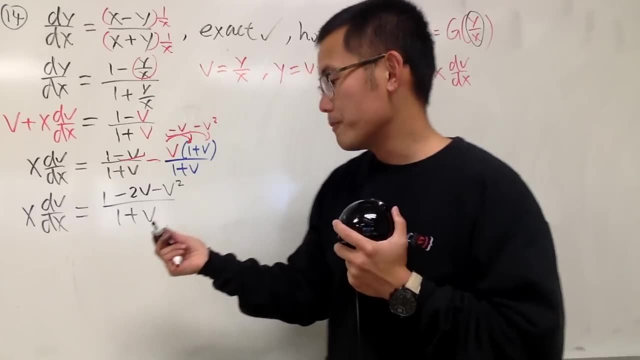 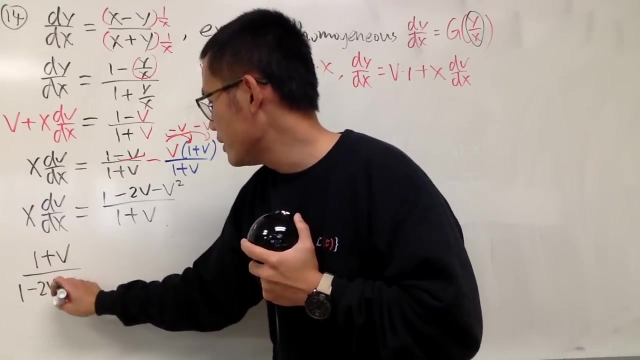 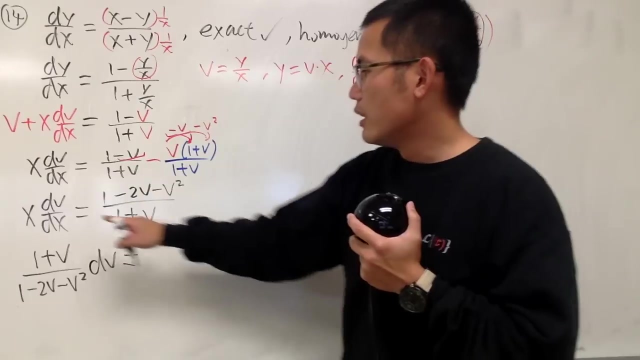 is d squared, so it's minus phi squared here. okay, now we can separate the variables. bring that to the other side, but it becomes the reciprocal. so here we get one plus phi over that, which is one minus two, phi minus e, squared with dv of course, and that's. 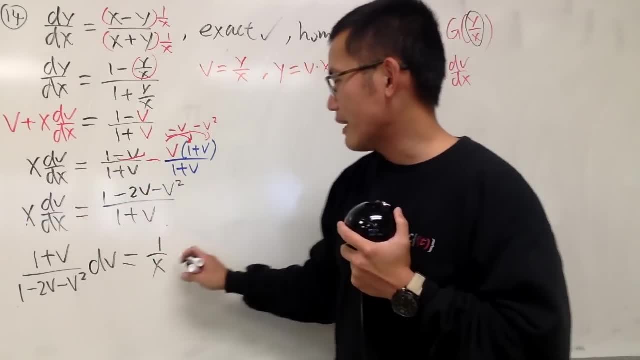 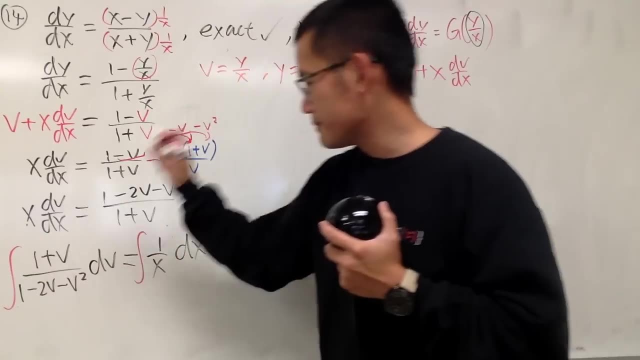 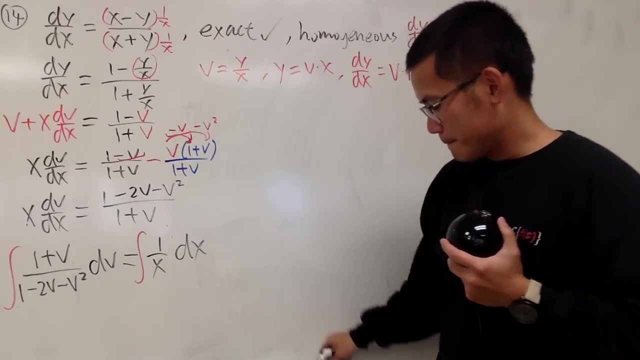 equal to bring this to the other side, becomes one over x, and then we have, just like that, now integrate both sides. very, very nice. depends on your personal preference. I think it's going to be easier. but okay, that's it. extra practice. all right, here's the do. 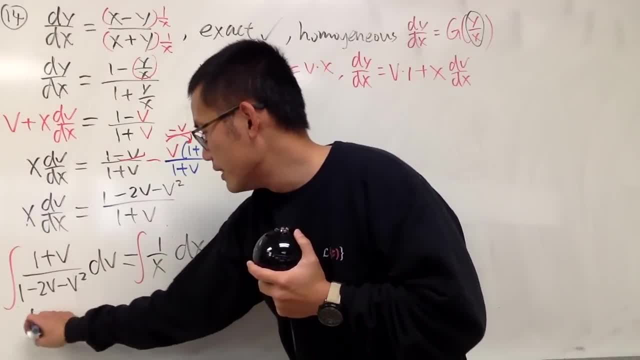 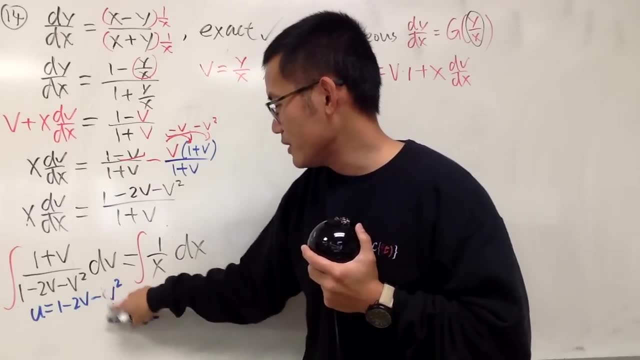 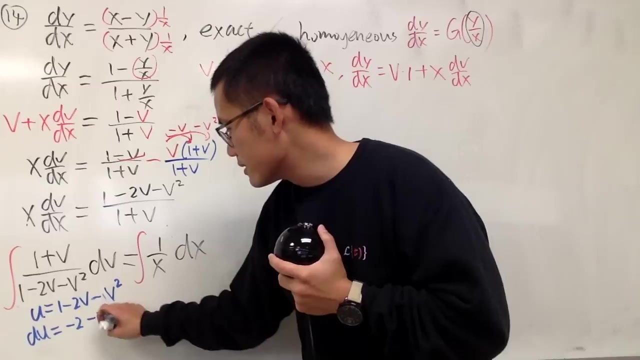 right here. this is actually very nice. we can just do u sub. let u equal to the denominator one minus two. phi minus phi squared. this is horrible. phi and you see that du is equal to. this is negative. two minus two v dv like this, so you can see that. 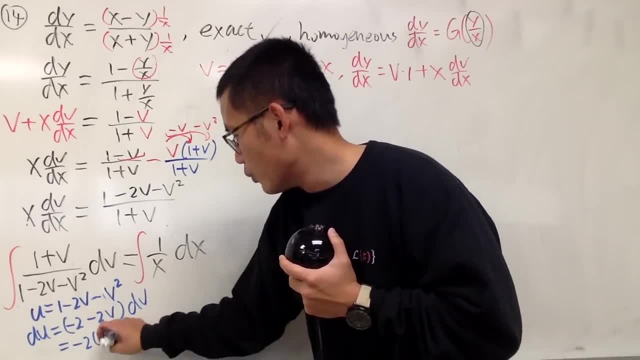 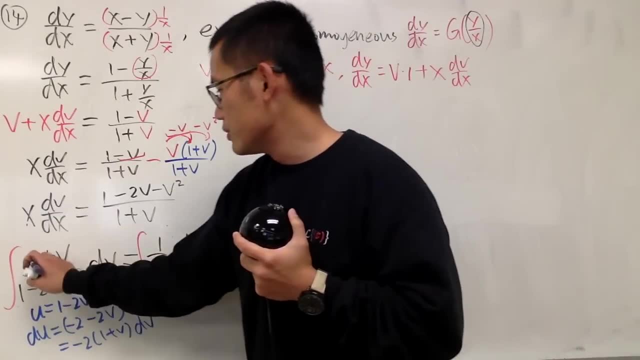 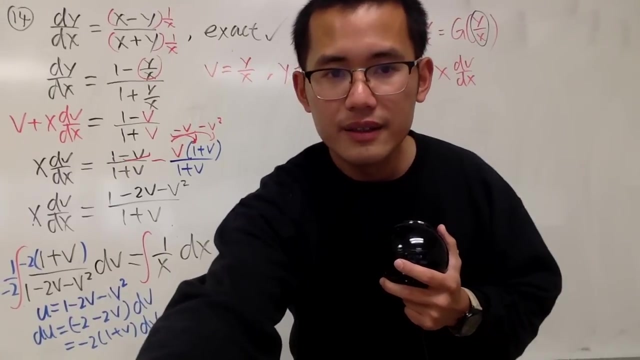 this is actually the same as negative two, one plus phi dv. so you might not see the negative two right here, but all you have to do is just multiply this guy by negative two and then divided by negative two. so that's pretty much the idea. so have a look. 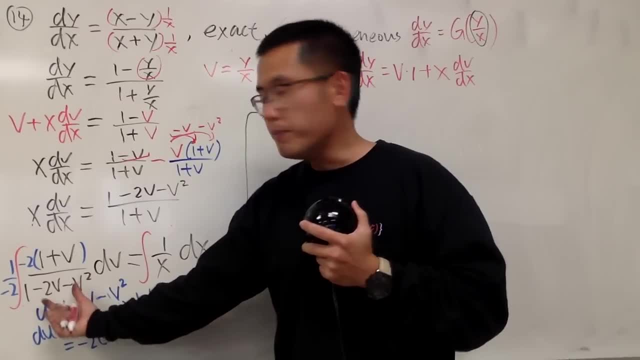 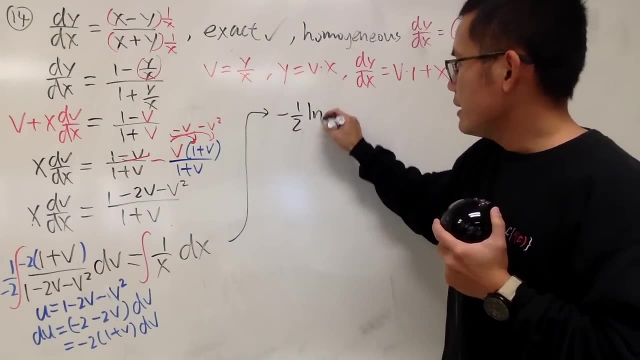 I will have the integral right here for you guys. this is going to be the? u, and then we'll have the du already. so here's the constant: we have negative one half and then it's going to be ln of u and the u is that? so we just put. 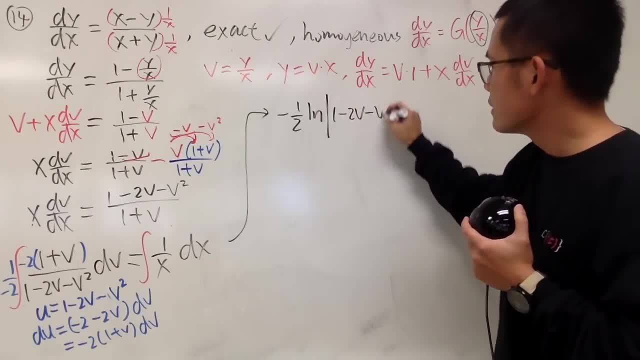 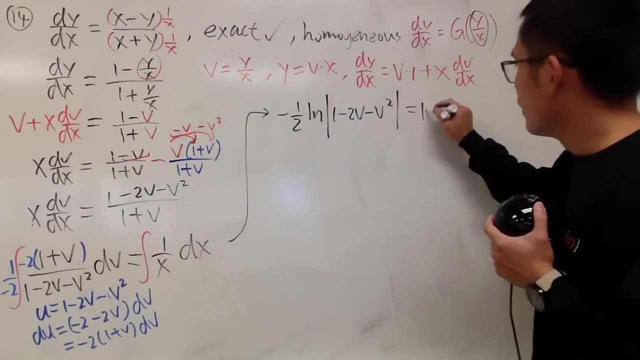 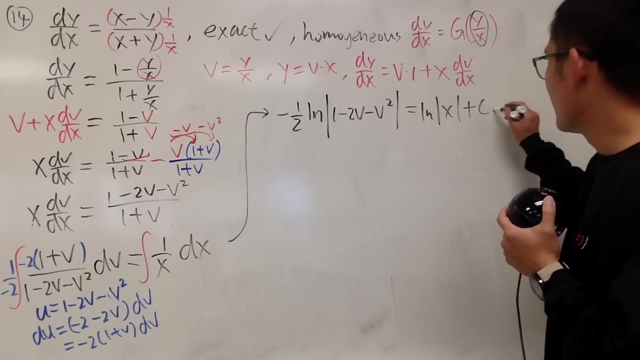 the ln absolute value one minus two, v minus v, squared like so. and then, on the right hand side, integrating this, we just get ln absolute five, x and then plus z, like that. good, okay, then clean things up, because I'm going to multiply everybody by negative two. 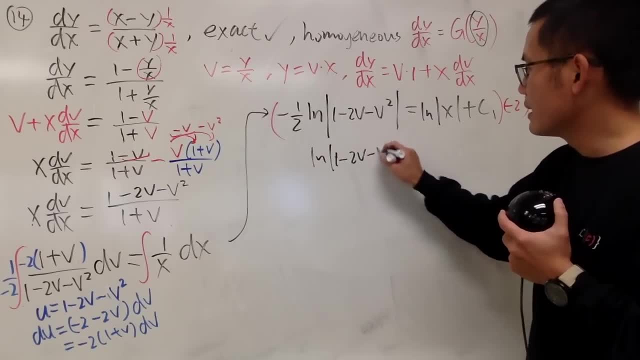 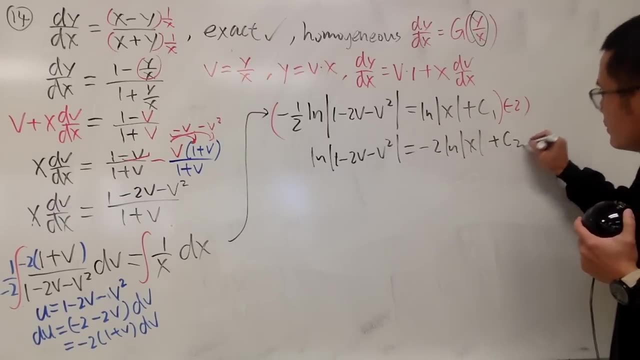 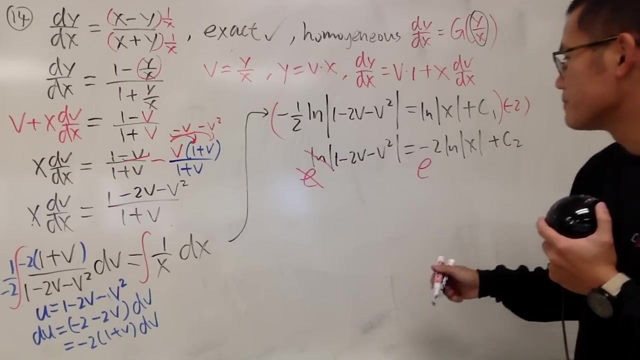 so I will get ln absolute value one minus two, v minus v squared it's equal to this times, that is negative two. ln absolute value of x, this, and that is c two, and then I will do e to this power and e to this power, so that this and that. 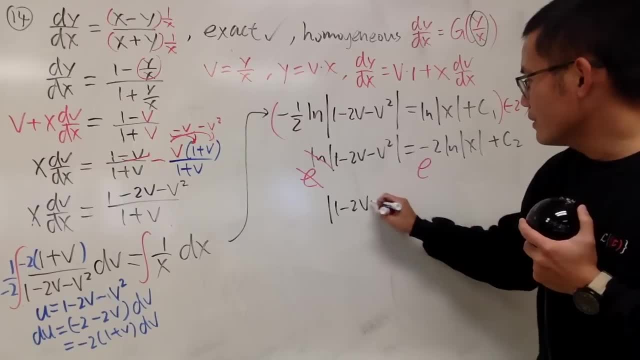 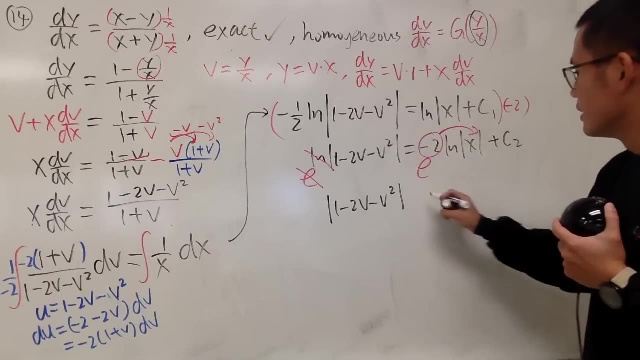 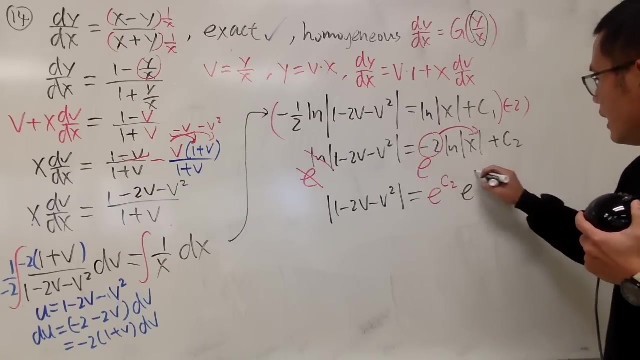 will cancel and you might keep the absolute value for now, v squared like this. so here's the thing. I'll bring this to here, and this is as saying e to the c two. yeah, e to the c two. and then this is as saying e to the. 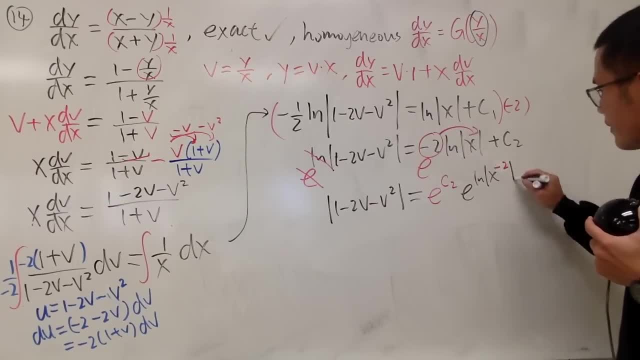 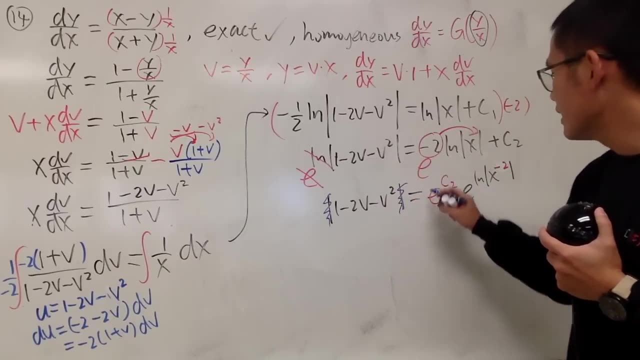 ln. absolute value of x to the negative. two like this: yeah, okay, now we have the absolute value. how can we deal with the absolute value? well, just get rid of that. get rid of that and then we have the plus minus. so just like that, no big deal on that. 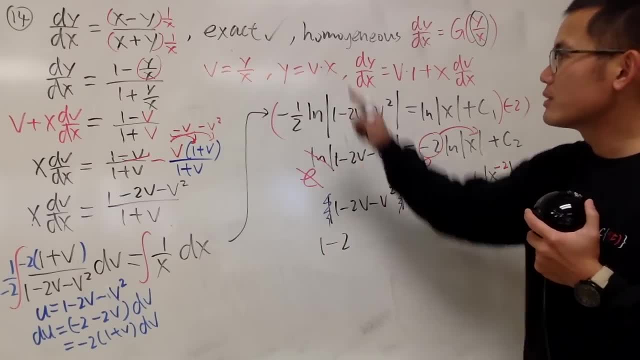 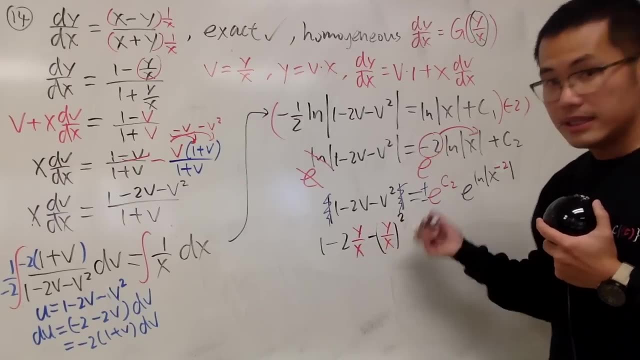 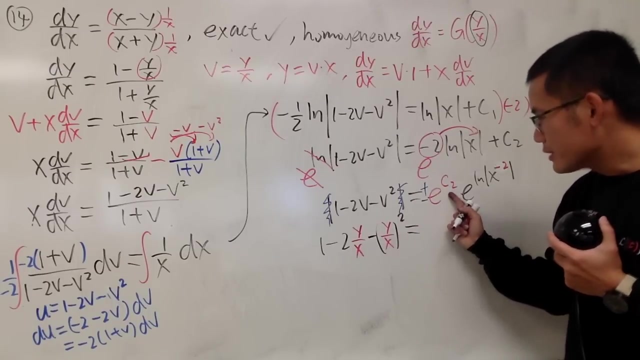 here is one, minus is two. d is y over x minus y over x. square this guy, yeah, like this. and then, um, this is equal to okay. here c two is a constant, e is a constant. so e to the c two is also a constant. that's good. 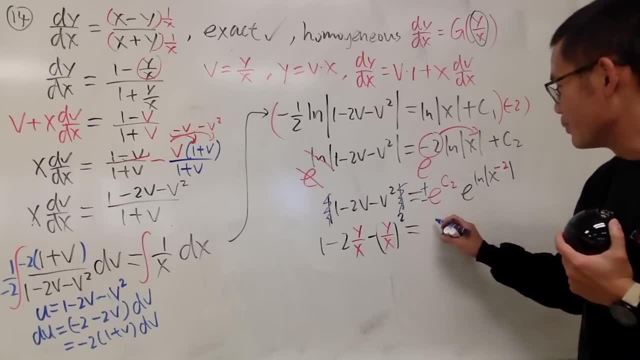 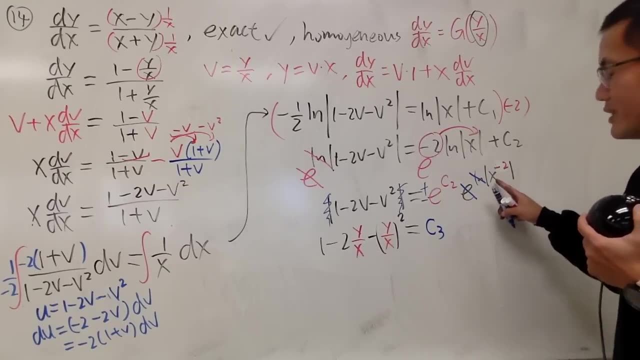 so c three. but plus, minus is just another constant, so I'll make it blue c three, like that. okay, and then for this one we have x to the one, and the truth is, you see, we have x to the one, negative two power, so in fact the absolute value. 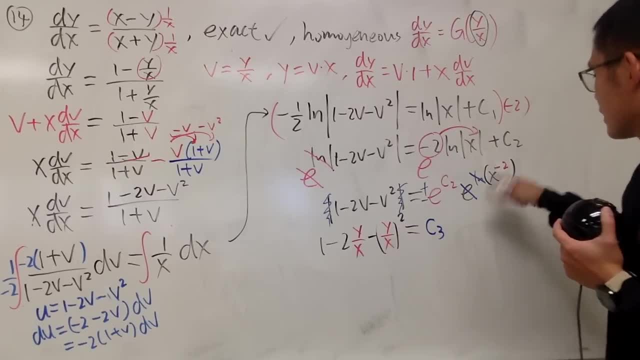 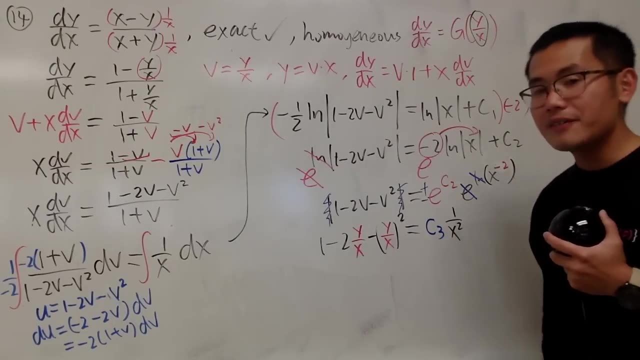 was not needed, because the input will be always positive anyway. so cancel them out. we have x to the negative two already is one over x to the second power like that. so that's what we have. if you don't like uh denominators like that, all we have to do. 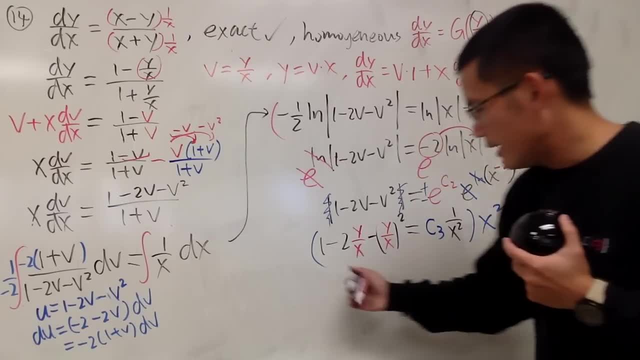 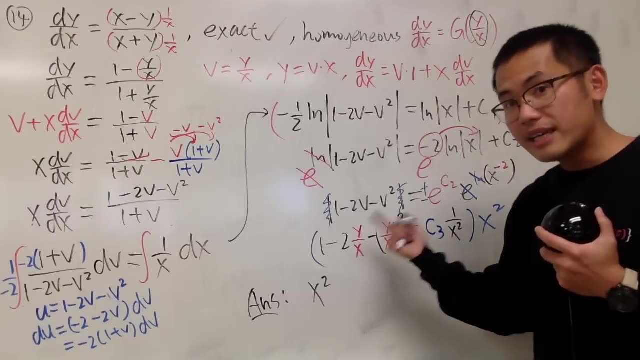 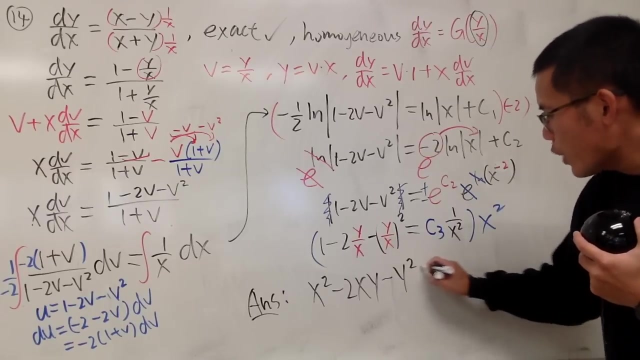 is just multiply everybody by x square and we'll get the answer. here is the answer. so this times that we get x square, this times this, we have x, one more x, so it's minus two x y. this times this x square: cancel, so we have minus. 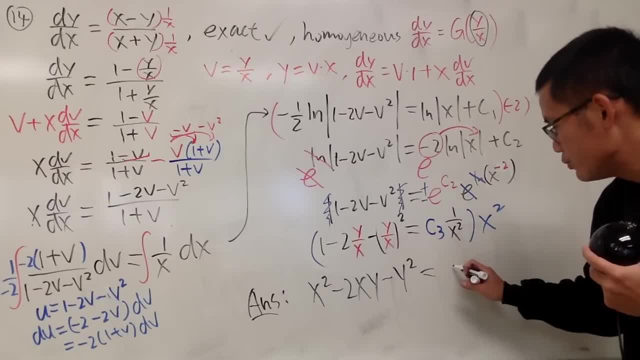 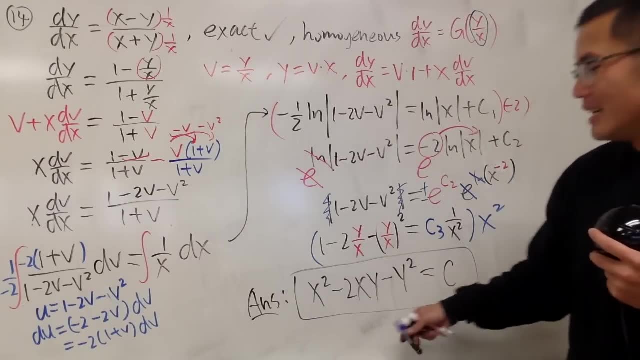 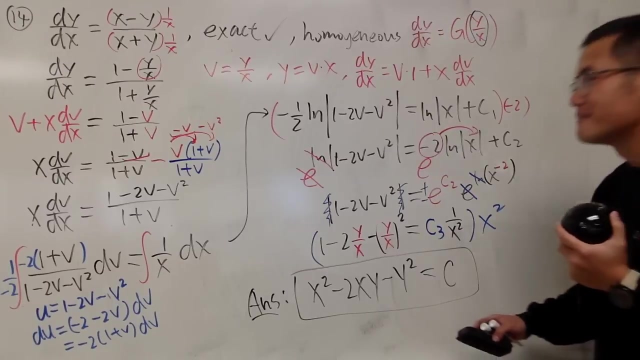 y square. this is equal to that. cancel we are done. so don't put down c three. just put down c and we see it. here is the answer for that. very good, I seriously think that's exactly. it's easier, but homogeneity: we need some practice, alright. 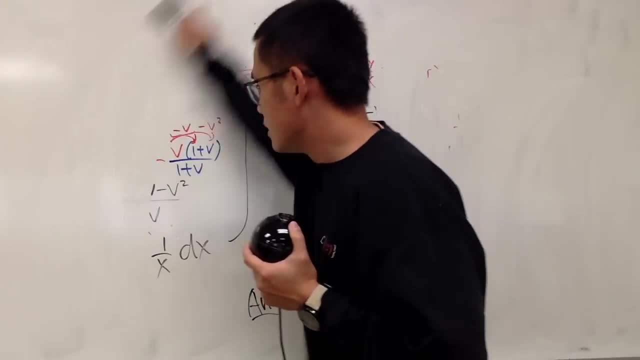 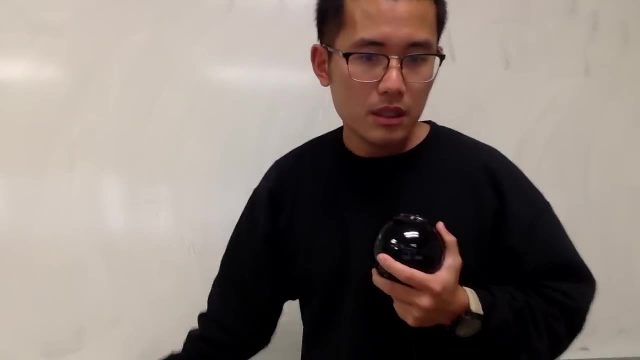 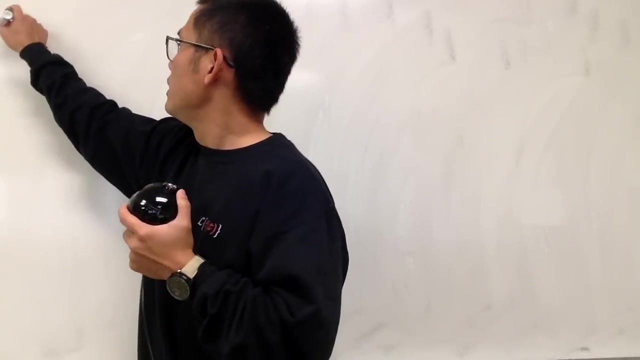 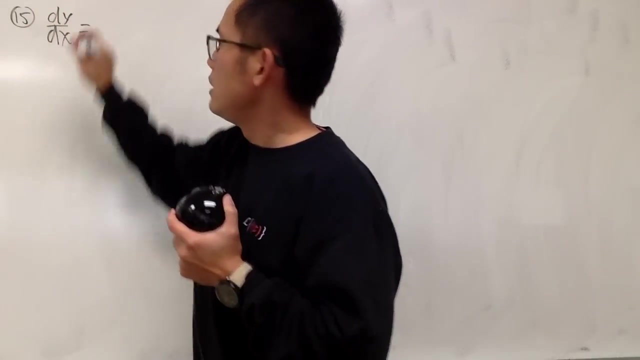 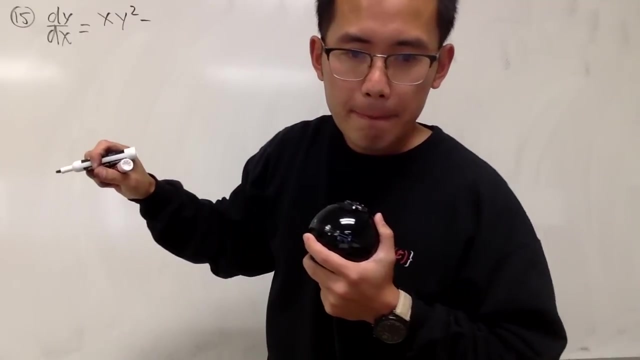 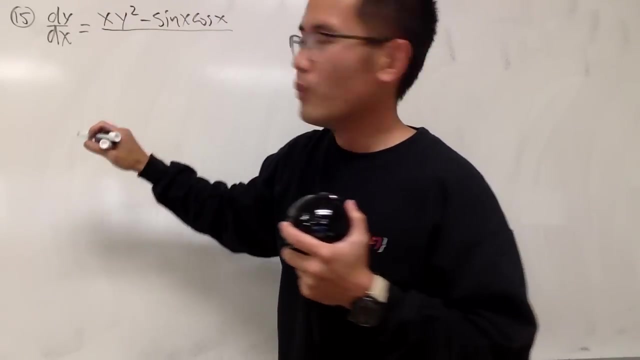 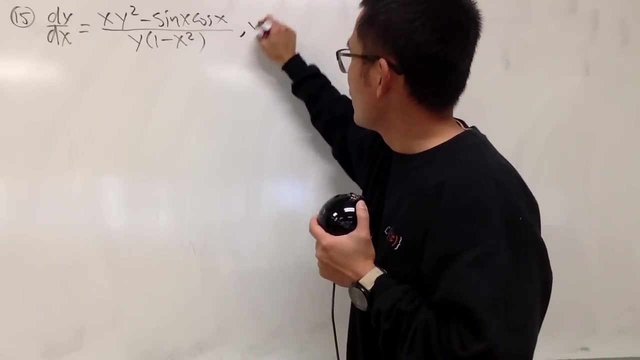 number fourteen. what's number fourteen after number fourteen? of course number fifteen. number fifteen, it's right. here and uh, we have the y over the x of x square. I mean x- y square minus sine x, cosine x over y one minus x square. initial condition y of. 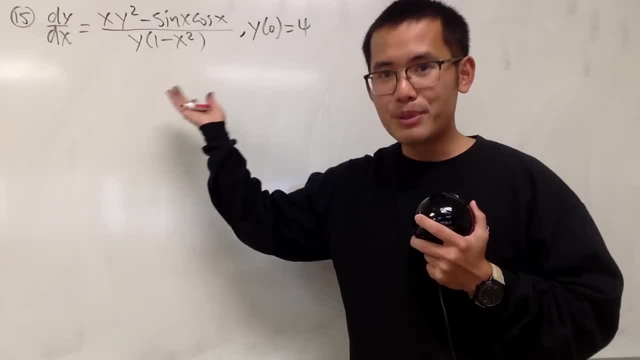 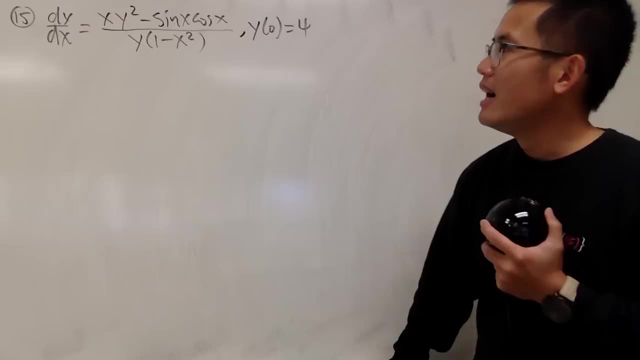 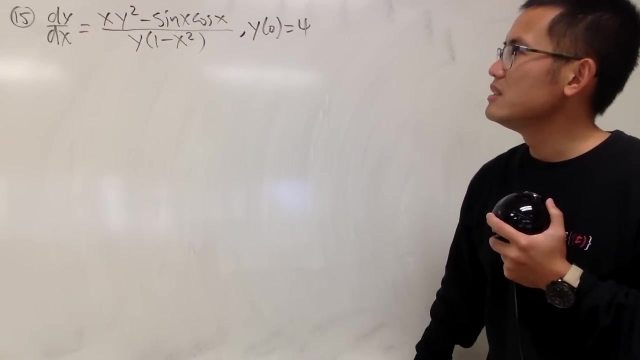 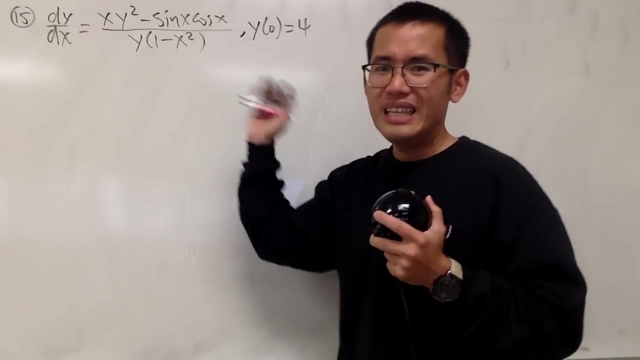 zero is equal to four. okay, so number fifteen right here. not linear, for sure, not separable neither. yeah, because you have this and that, the y is there. so, out of I'm not aware, not homogeneous neither, not Bernoulli's substitution, but the input. this is not like. 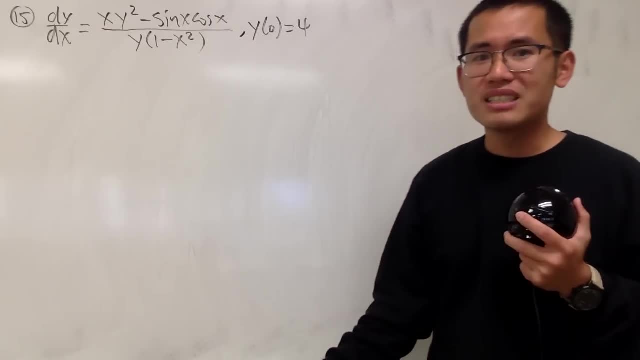 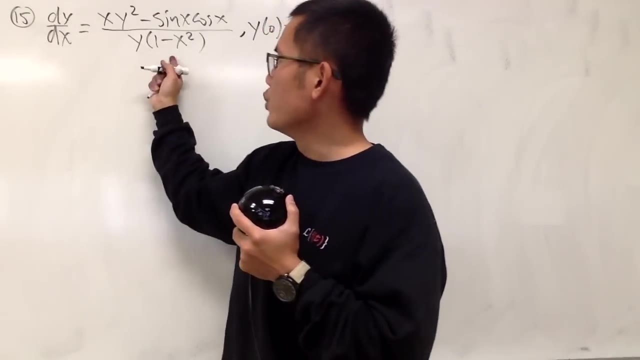 this input function right. so how about exact? so again, to check if it's exact or not, we have to make sure this is in the correct form. yeah, so let's go ahead and do that. rewrite it this over there, which is y times one minus x square. 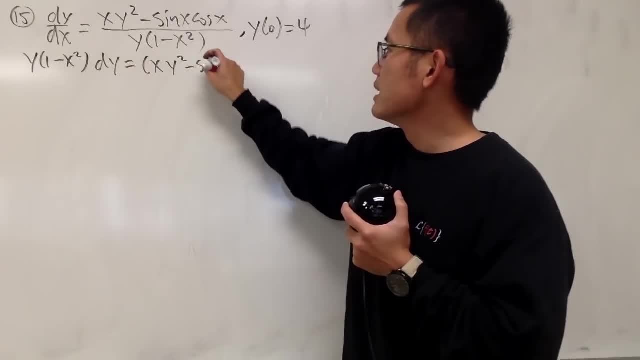 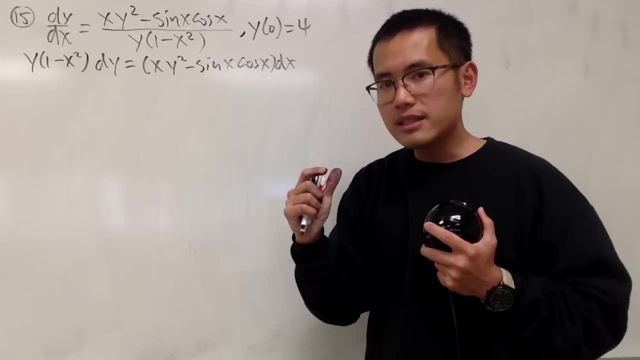 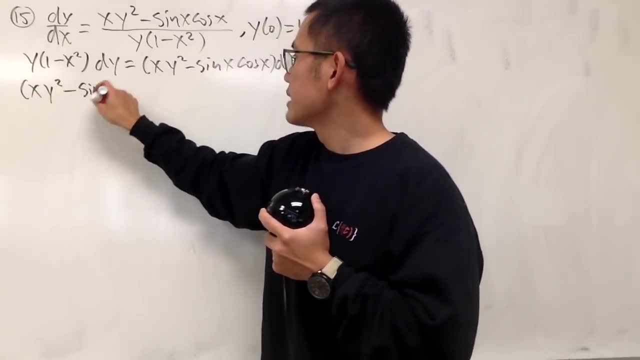 and then we have the dy that's equal to this times all this, which is, parentheses: x, y square minus, sine, x, cosine, x, dx. and yeah, and remember, for the exact differential equation the dx part goes first. so I'll write this down first: x, y, square minus. 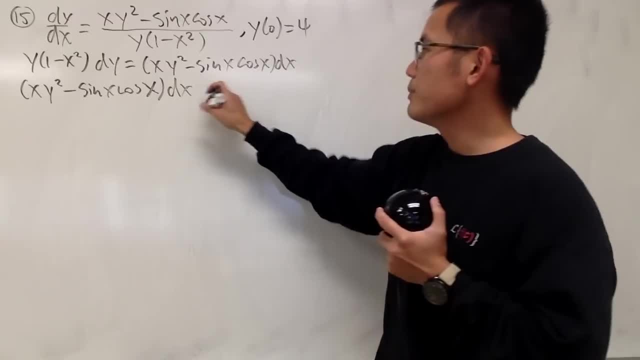 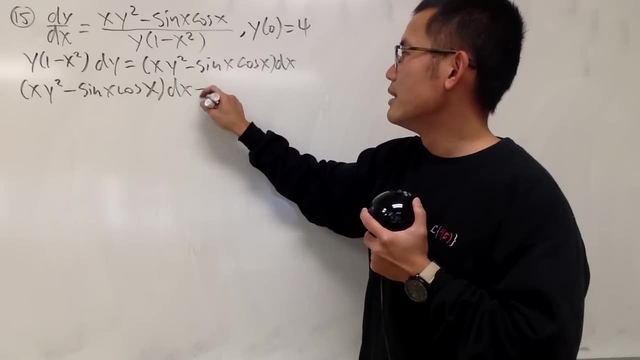 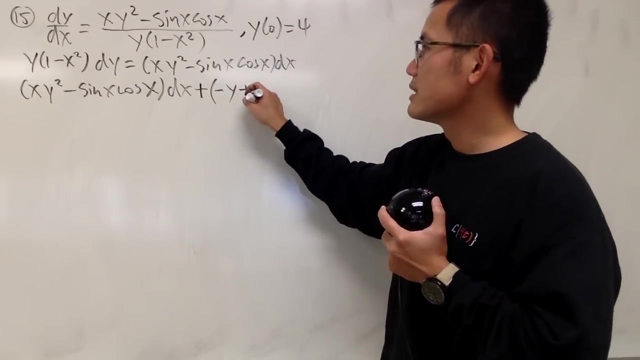 dx, bring this to the other side- becomes minus, and let me just distribute. let me just distribute. so minus, let's do this plus. but it's a minus y, right, it's minus y, and then plus y, x, square y, right. so again, if you have this, this is: 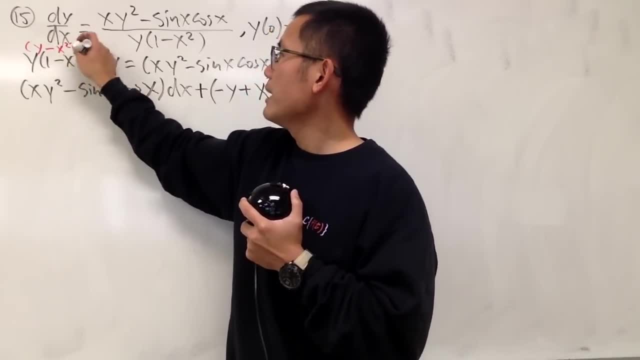 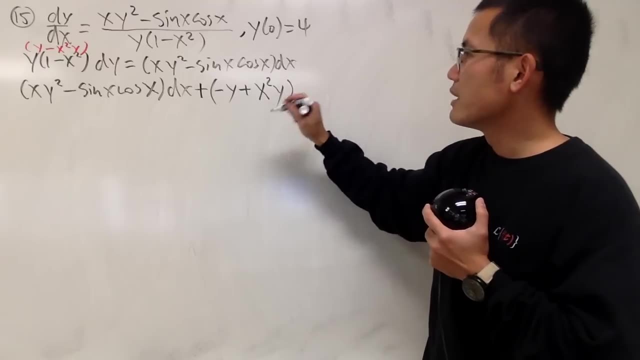 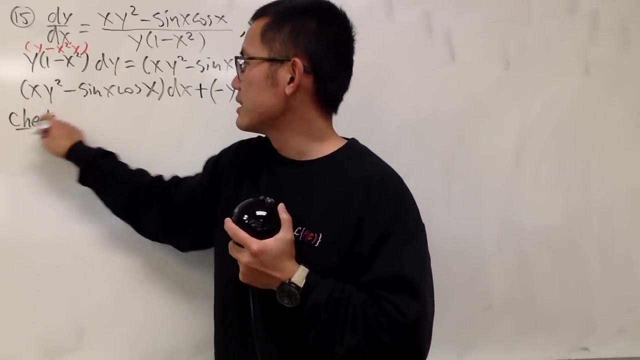 y minus x square y. bring this to here, so it becomes minus. bring that to here, so it becomes plus. and then we have the dy here and that's equal to zero. now here is the check for exactness. this right here it's with the dx. you do the opposite. 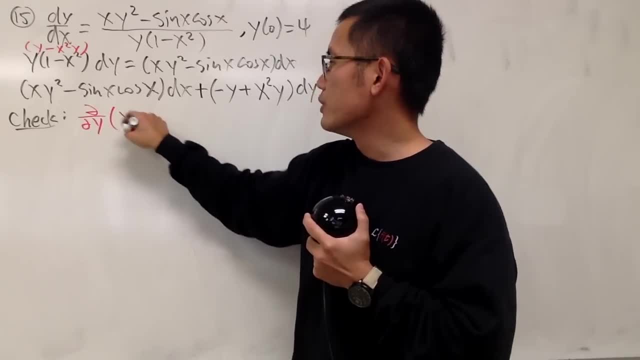 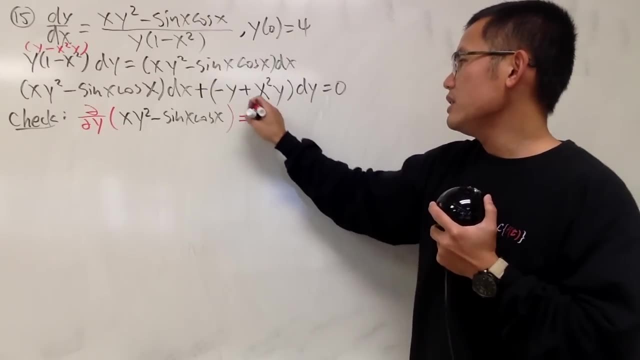 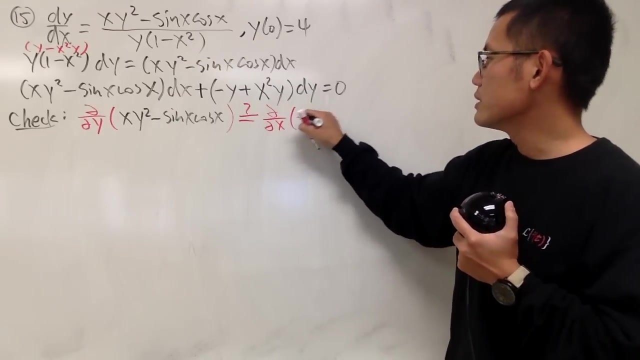 so go ahead, do the partial with respect to y of this guy, which is x y square minus sine x, cosine x. hopefully this right here is equal to the partial with of this with respect to x, which is the negative x. I mean negative y plus x square y. 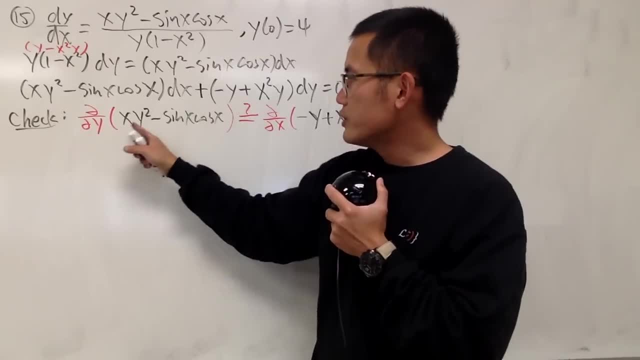 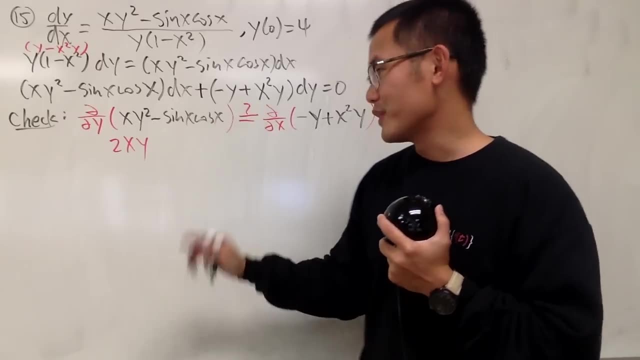 inside. let's go ahead and check differentiating this. well, bring the two to the front, so we just get 2xy. and guess what? this right here? the derivative is zero, so very nice. so probably just write it down right here: 2xy is this equal to? 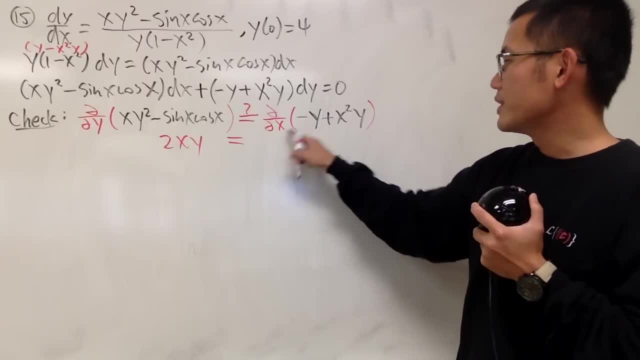 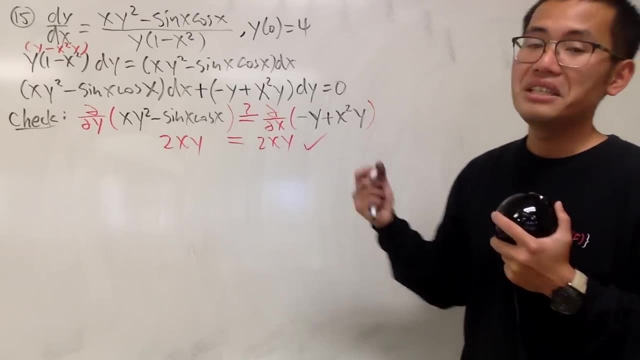 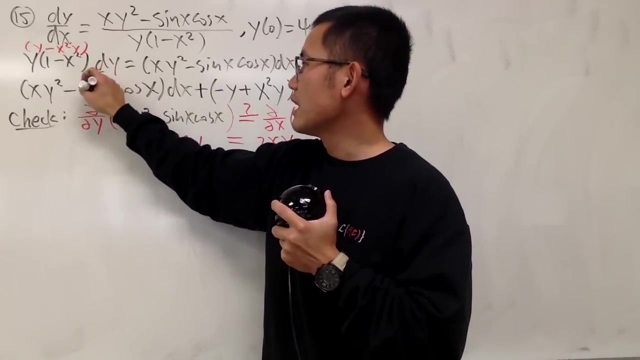 the derivative of this with respect to x. the derivative of this is just none, nothing. the derivative of this- bring the two to the front- is 2xy checks. it is exact, right. so here's the deal. this right here represents the partial of some capital: f with respect to x. 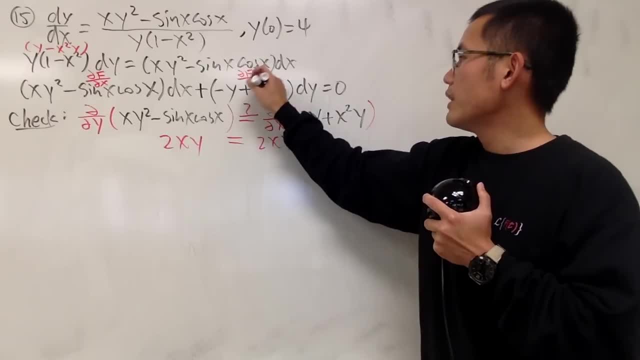 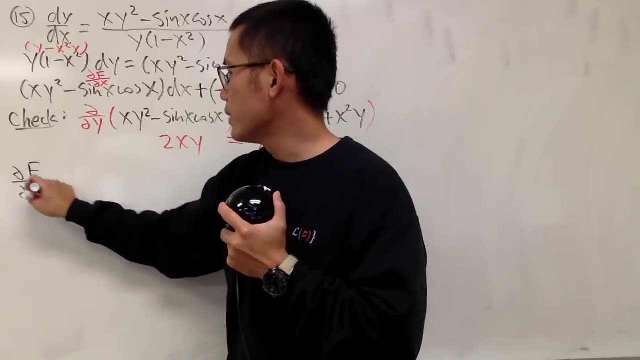 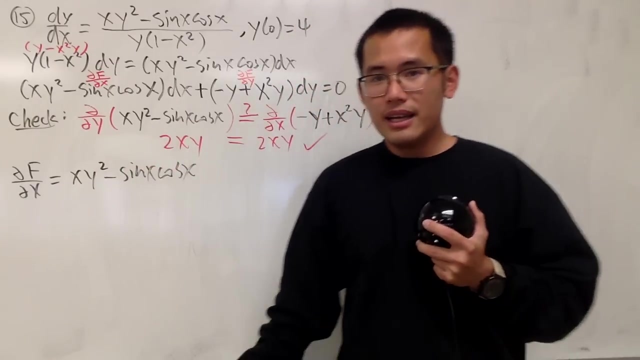 and this right here, it represents the partial of f with respect to y. go ahead and write this down. we have partial f with respect to x. equals xy square minus sin x, cosine x, like this. and here we go, of course. go ahead and do our integral in the x world. 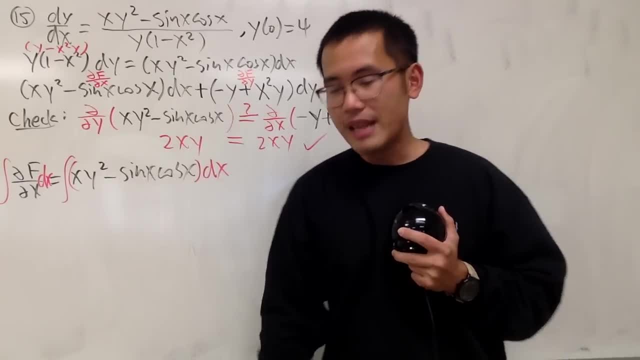 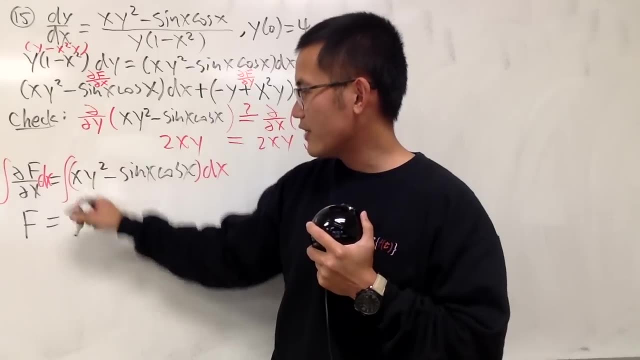 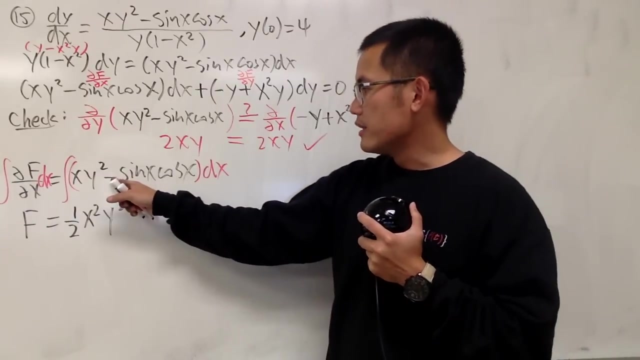 in the x world. now, on the left hand side, we get the capital f, integrating this well, x to the second divided by 2, so we have one half x square y stays the same. okay, differentiating this. well, we have minus. check this out, bring down the minus. 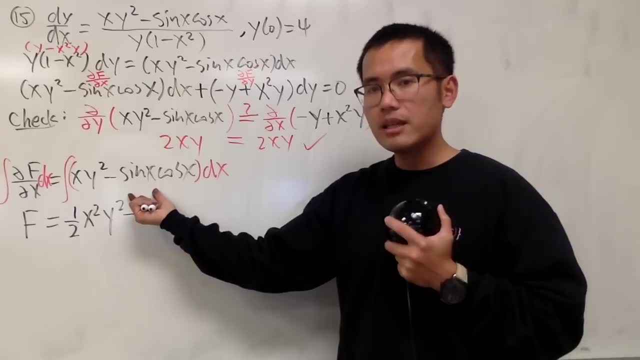 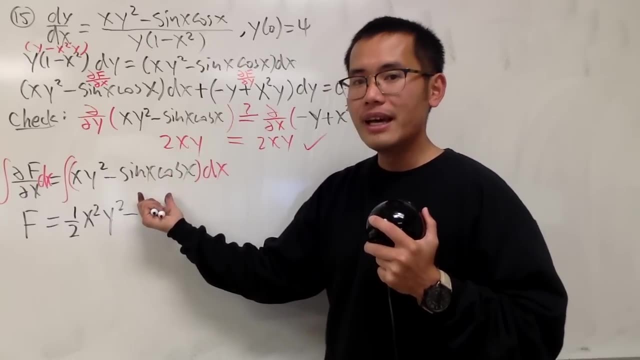 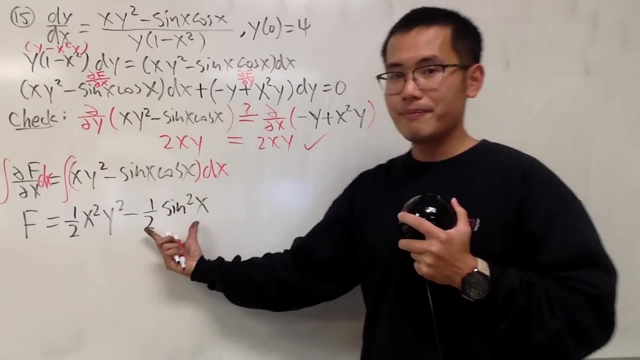 and now I'll do u sub. let u equal to sin x, because derivative of sin x is cosine x. very good, so we just have to integrate u in the u world and that will be one half u square which is sin square x, like this, and you can go ahead. 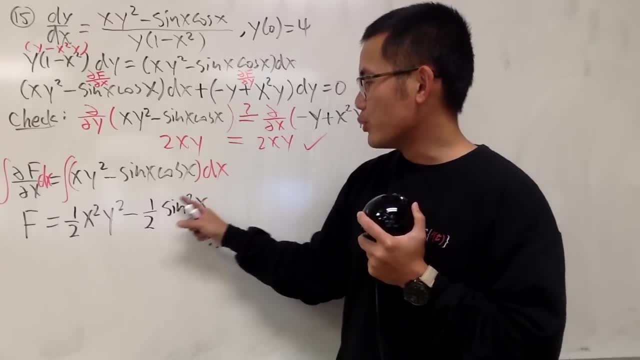 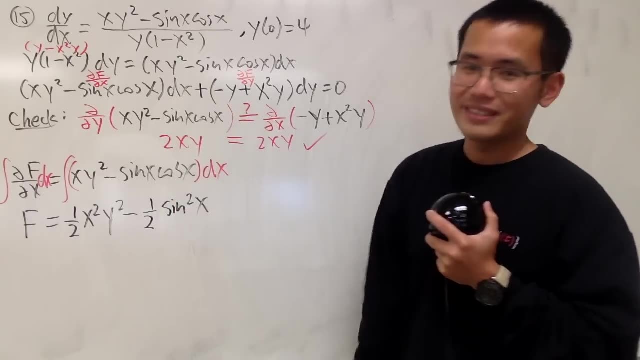 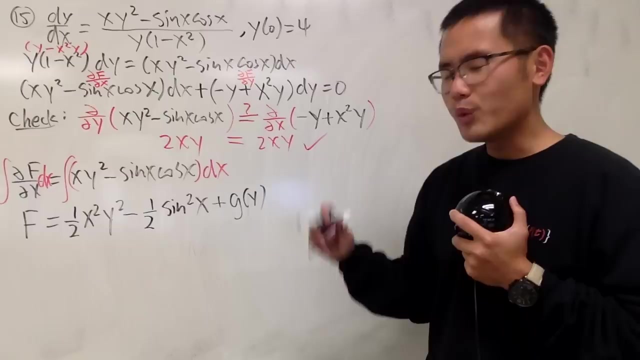 and just do this in your head and then differentiate this in your head as well to check. okay, so we have the sin x to the first power, but don't forget the chain loop. the derivative of sin x is cosine, so this works, okay, don't forget plus. 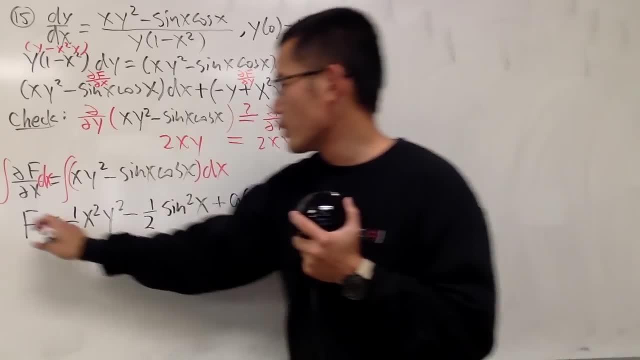 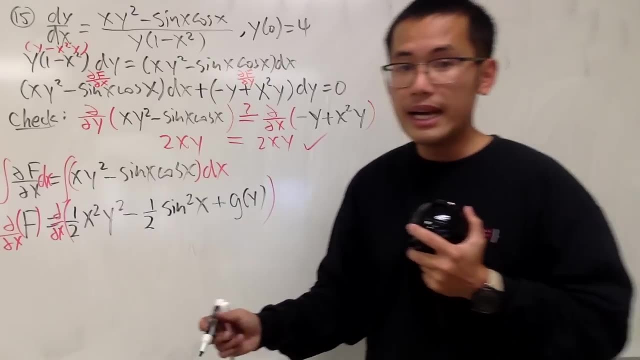 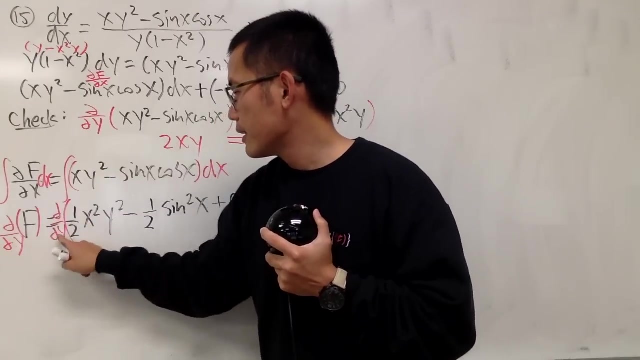 g of y, because in the x world y is also world. y is a constant. so to make use of that we will have to do the partial on both sides with respect to x and we will see no with respect to y. so on the left hand side, 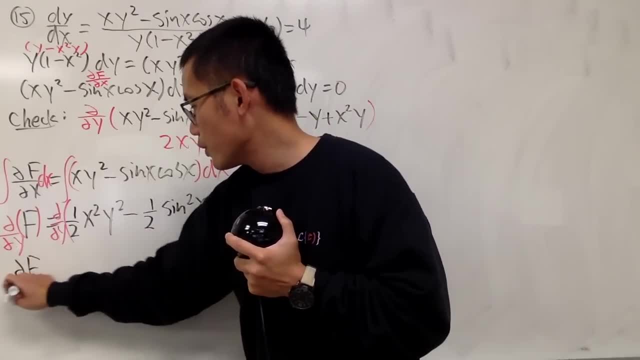 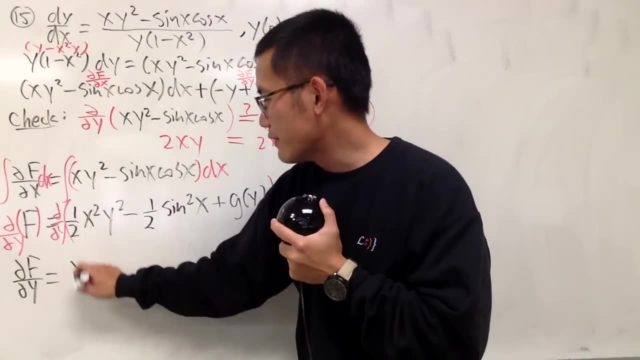 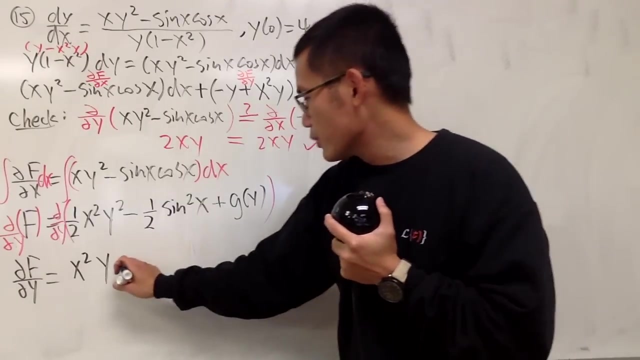 we get the partial of f with respect to y. that's equal to well differentiating this part. put the two in the front, so we just have x square and then y, like this, and then differentiating this part is gone. so that's good and differentiating this. 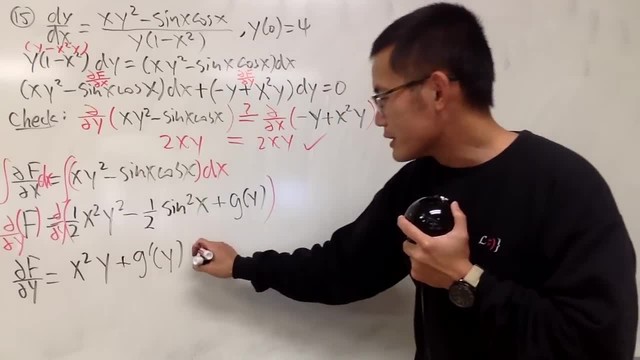 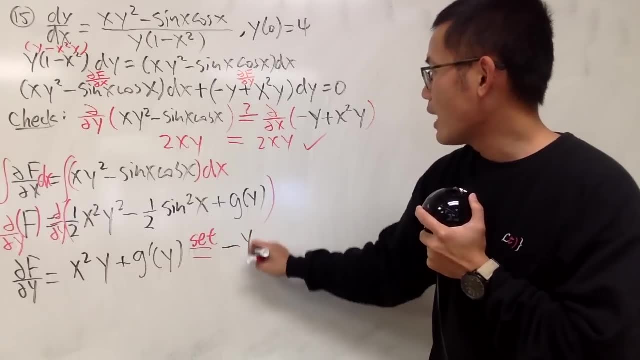 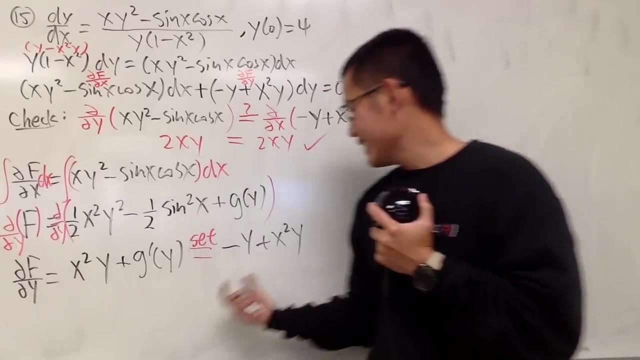 we get plus g prime of y, like that. now we have to set this to be this, which is negative y plus x square y, like that. alright, and let's see this: and that are the same already. so that means this has to be equal to that g prime of y. 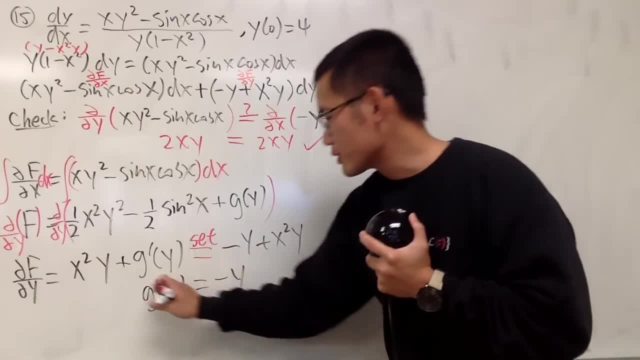 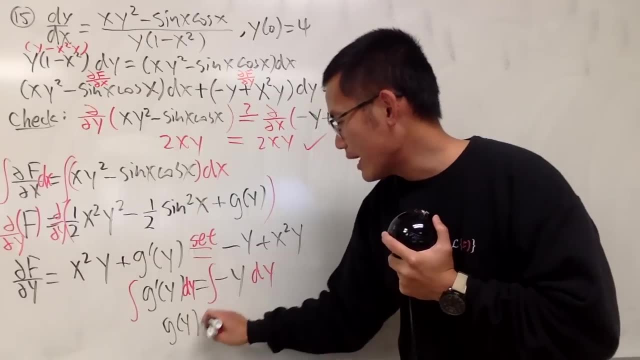 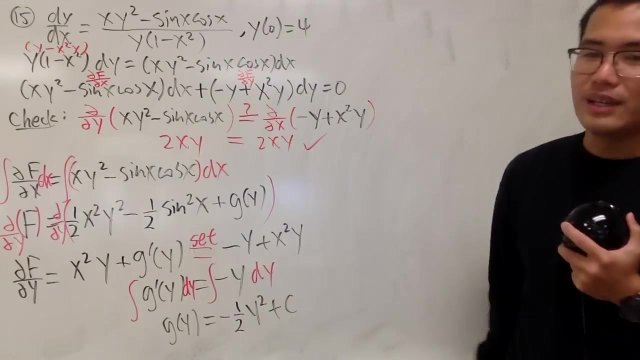 has to be the same as negative y and of course from here we can just go ahead, integrate both sides in the y world, so we will get g as a function of y being equal to. we get negative one half y square plus a constant right, and then we'll kick the constant. 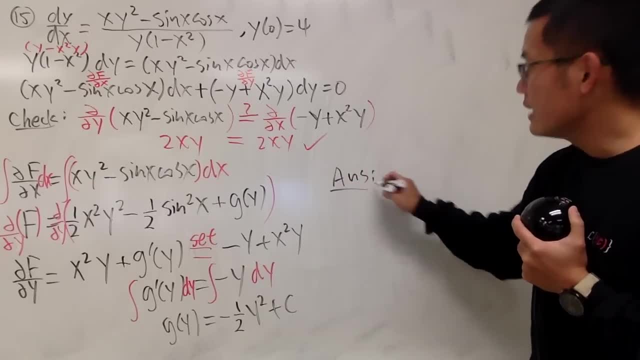 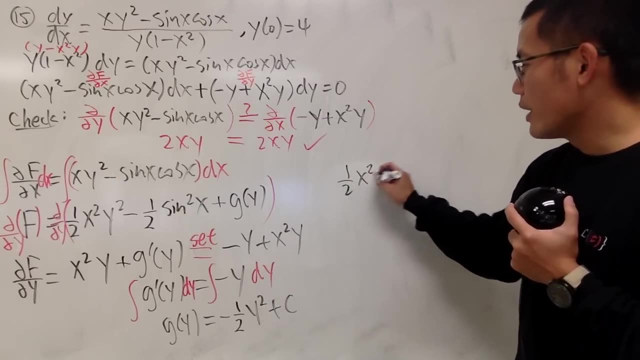 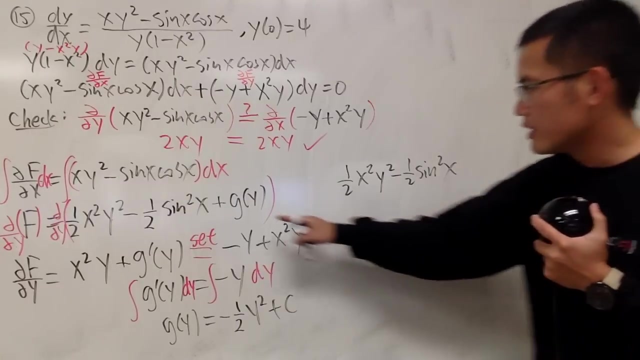 to the right hand side. okay, so that's pretty much it. finally, here is the end. oh no, finally we know the function f. I will write down: one half x square y square minus one half sine square x, and then the g of y is this: so I'll just write down: 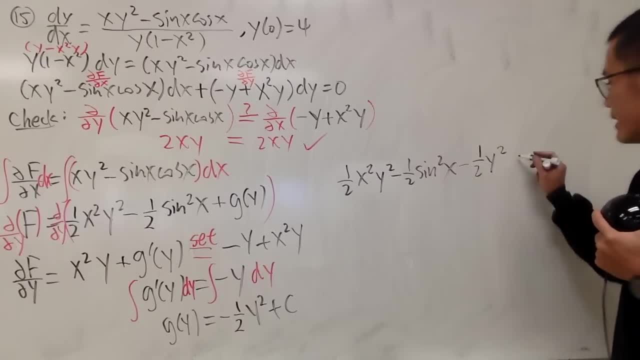 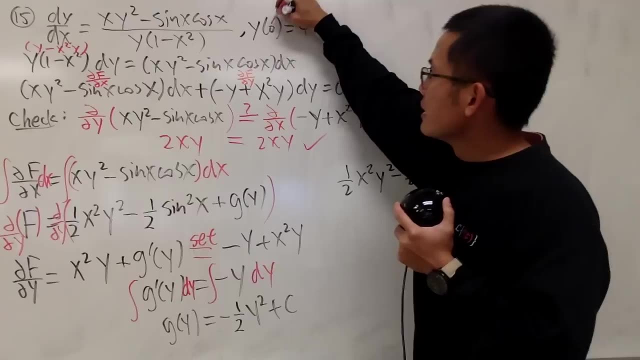 minus one half. you can put a plus c here, but I like to put a plus c right here. so this is what we have, but we do have the initial condition. so again, here is the x and here is the y, so that means I go ahead and plug in numbers. 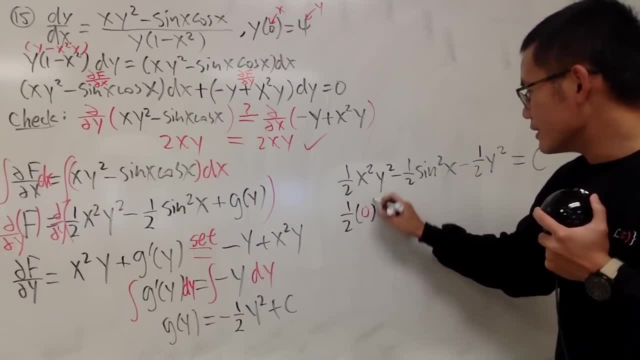 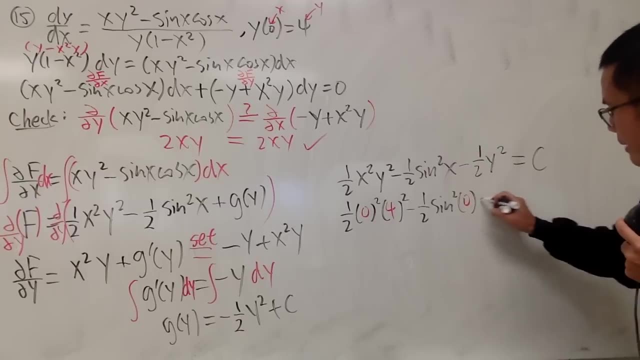 one half times zero square. and then we have four four square minus one half sine square of zero, and then minus one half four square equals zero. this is zero. this is also zero. this is sixteen divided by two is negative eight, which is equal to c, just like that. 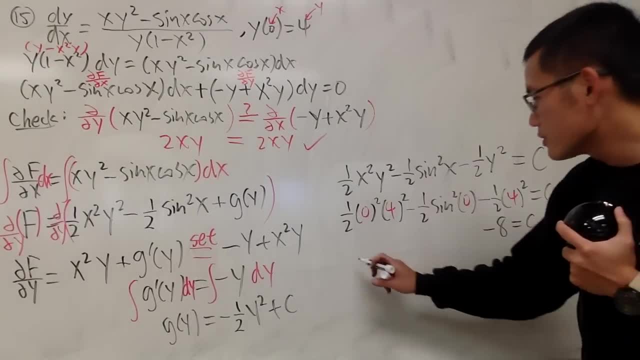 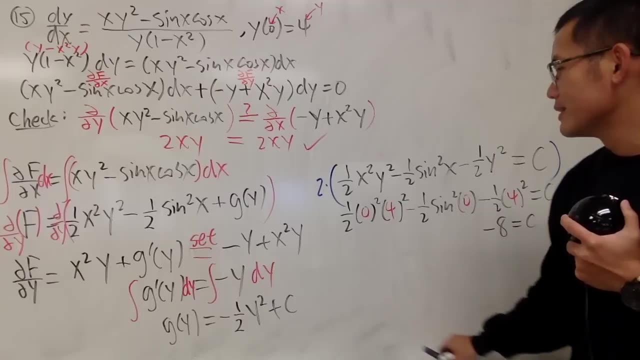 so finally we have all this, so we can just plug in, but I prefer to not have the one half. let me actually multiply everybody by two, because why not? so two times all this, here is the final answer. two times all this, we get x square, y square. 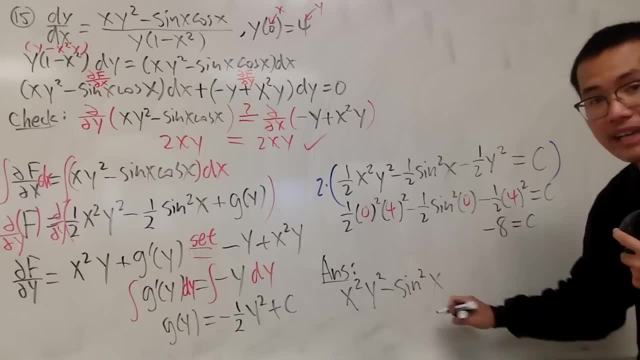 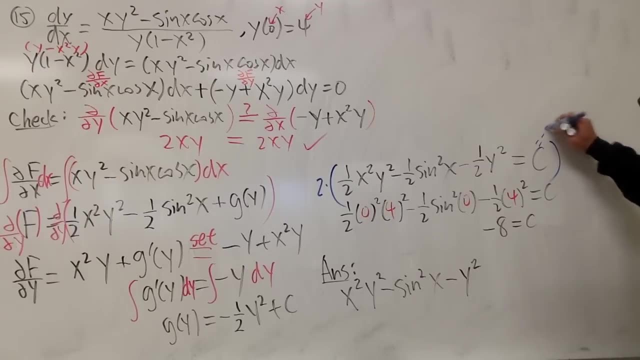 minus sine square x, and then, this times that we get minus y square now, because we know c is equal to negative eight multiplied by two, we actually end up with negative sixteen, right? so here is the answer. here is the answer for that, and I'm going to change. 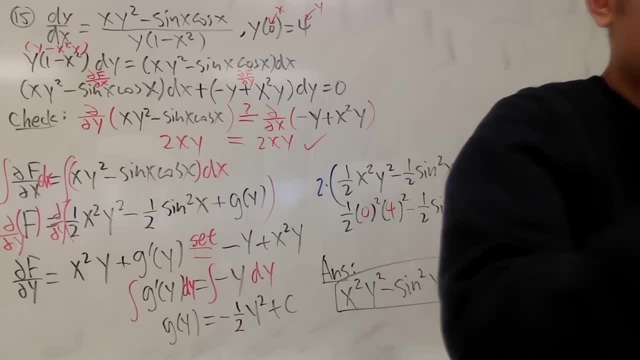 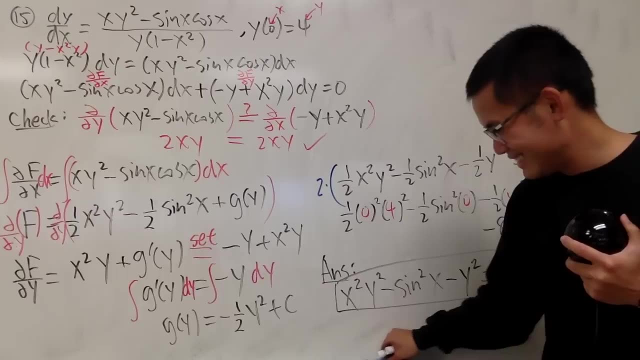 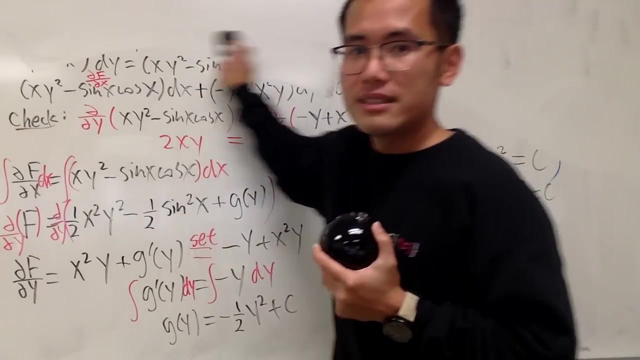 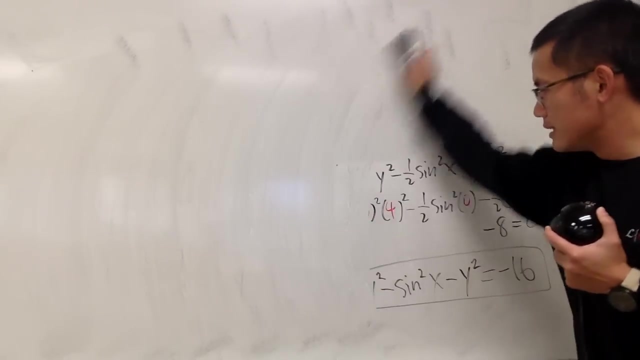 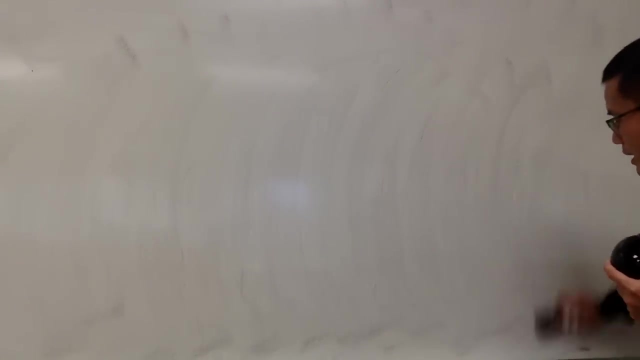 my marker, because it's kind of getting the light thing is getting low. so you do that, so that's it okay, so good, alright. so another exact differential equation. let me see if I can erase the board, if I can make the board cleaner. so you guys will have. 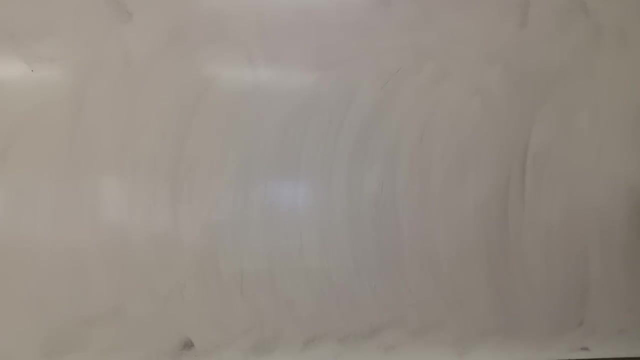 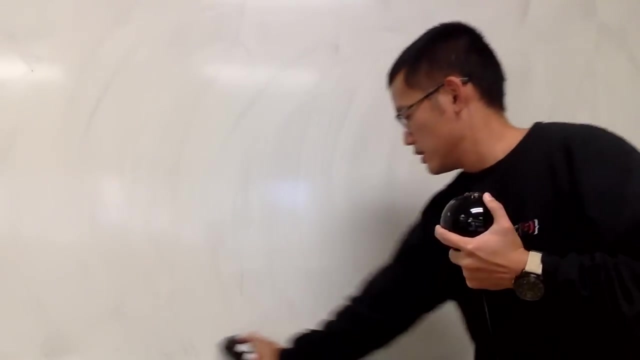 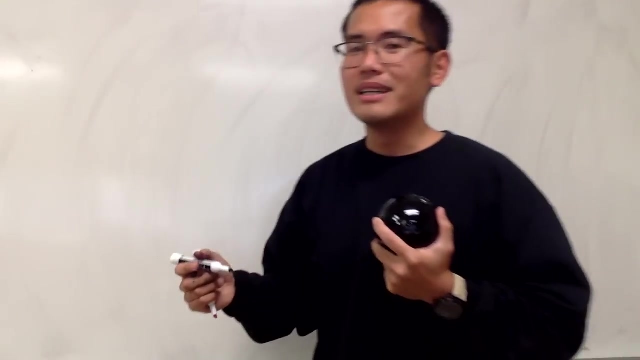 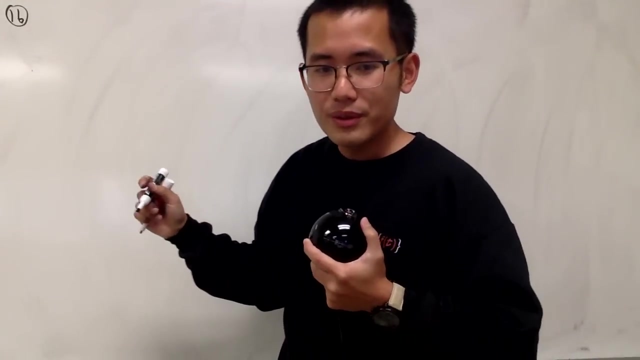 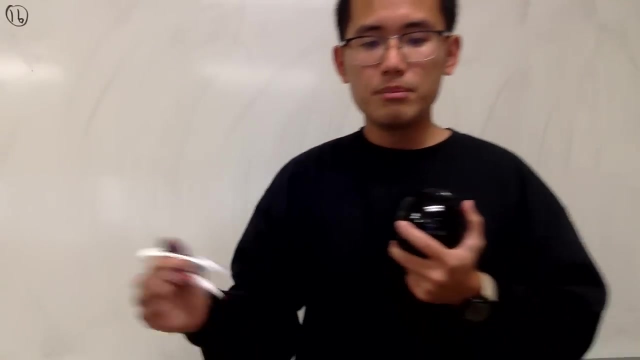 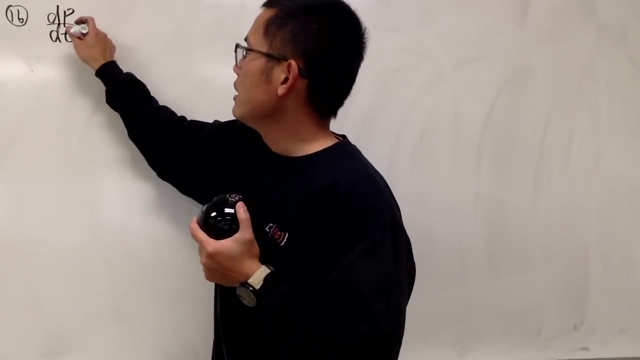 a better watching experience. alright, good number sixteen. so yeah, sixteen plus eight is equal to twenty four. so yeah, this right here I want to show you guys how to do some classic growing models. so this is the logistic differential equation. so we have dp, dt that's equal to. 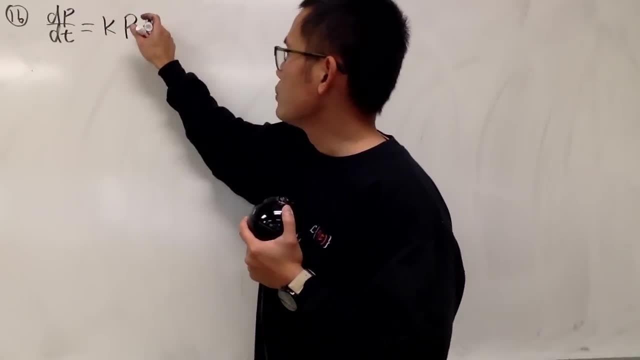 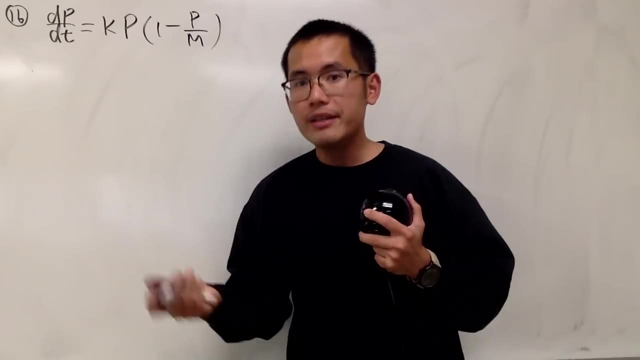 k, which is the constant of proportionality, and then p, which is the population, and then we have to multiply one minus p over m, and m is the carrying capacity. and I will also tell you: p of zero is equal to p zero. it's just the initial. 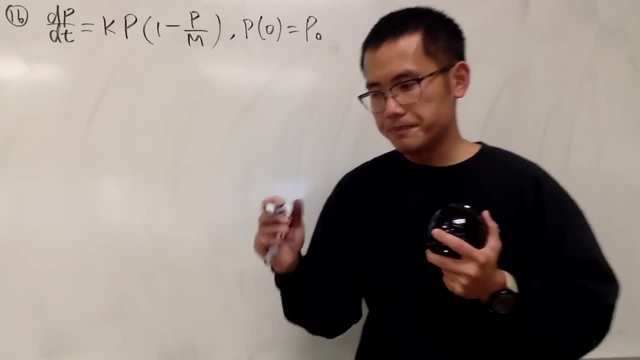 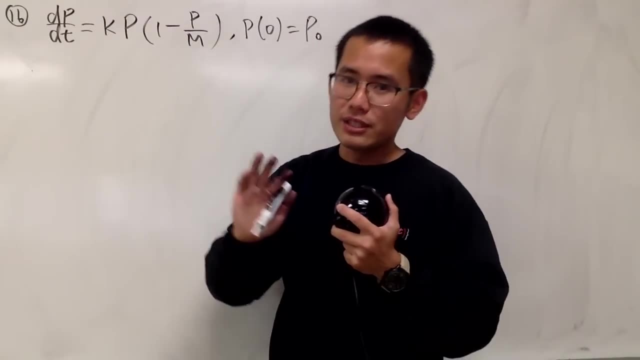 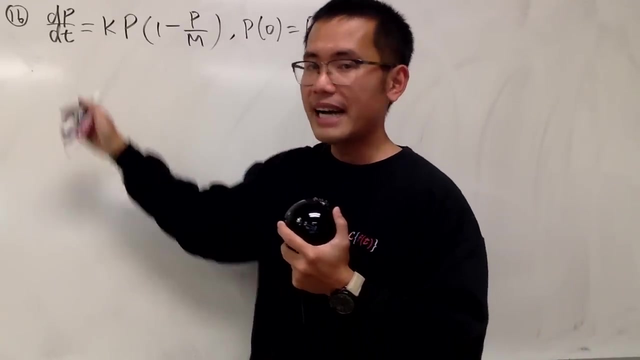 population. so I will come up with a general formula for you guys for the logistic. here we go. this is so separable k and m, they are just constants, so don't worry about that. so now, here we go. I will bring this to the other side, so I will have 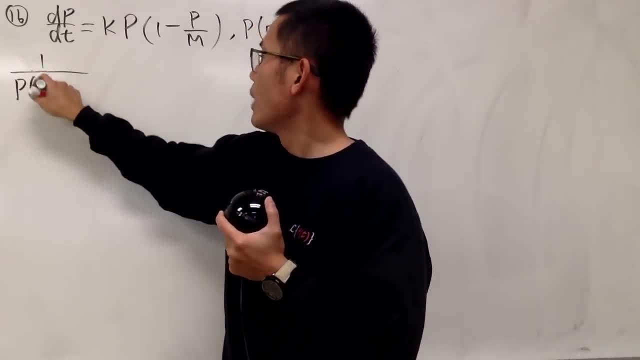 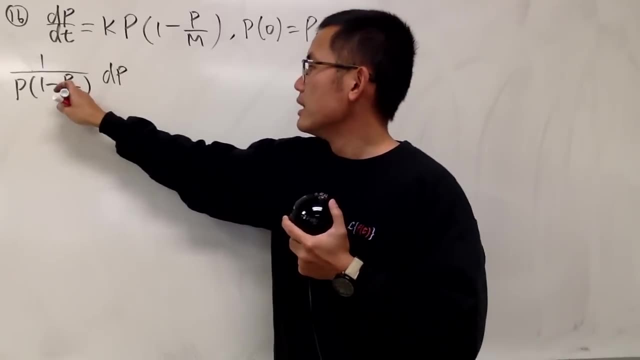 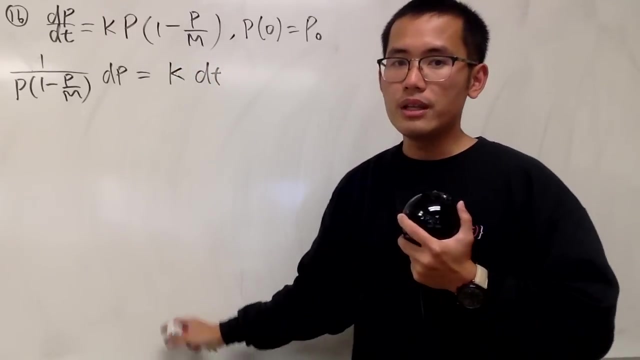 one over p times one minus p over m, like so it was dp here, and then this is equal to k and then dt. and remember a constant, if any constant is invited to in any world. so that's good. now, before I integrate this, I will clean things up. 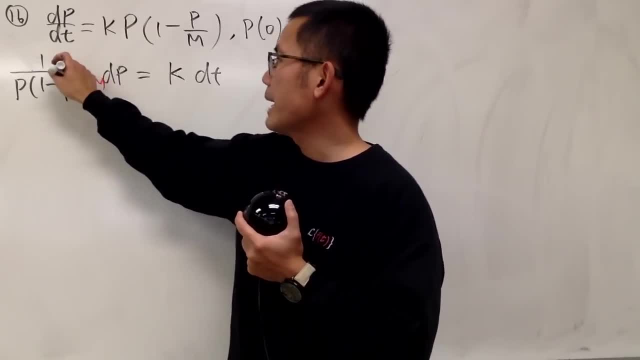 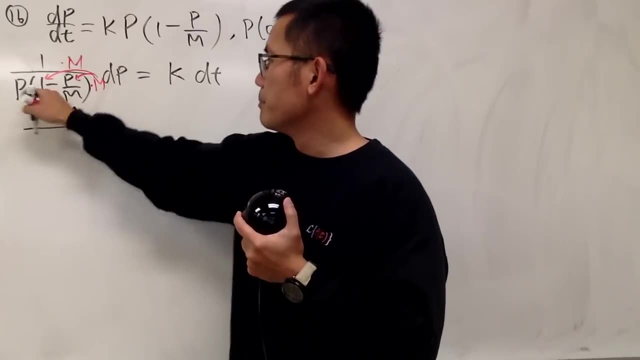 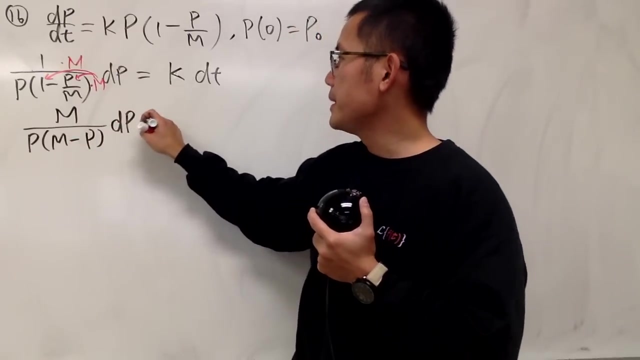 because this right here is a little complex fraction, so what I will do is just multiply the top and bottom by m. right, so if you distribute the m right here, right, so we actually get the following capital: M over p in the front times, m minus p and then. 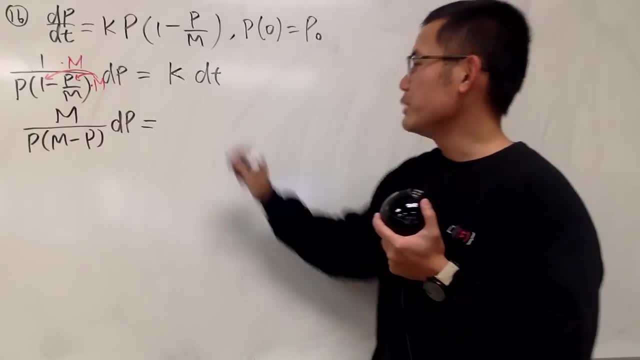 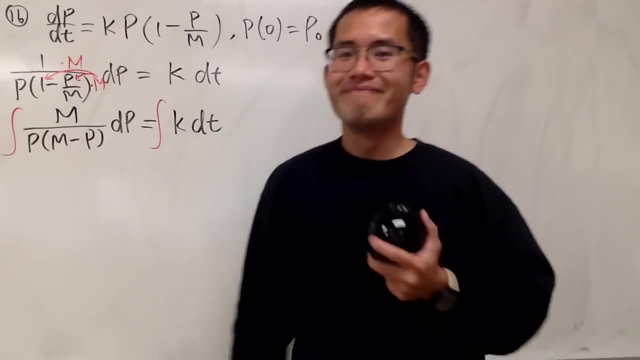 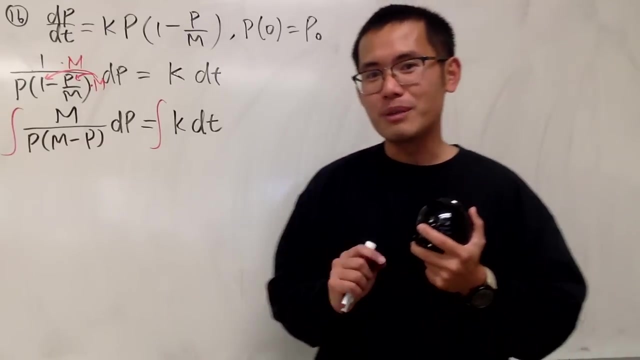 this is the only number is one or maybe zero. anyway, k is k and then dt. now integrating both sides here and here. and if you notice, I haven't shown you guys any partial fractions. I know, but here it is. this is where we have to use the partial fractions. 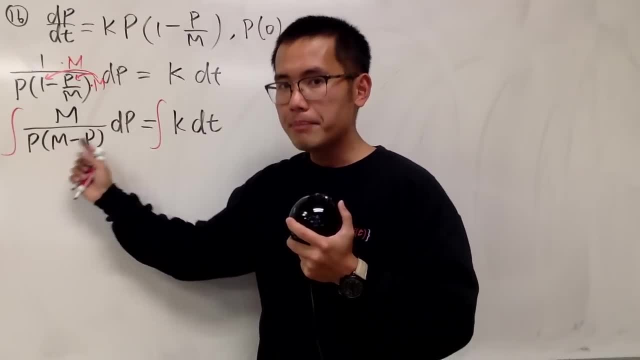 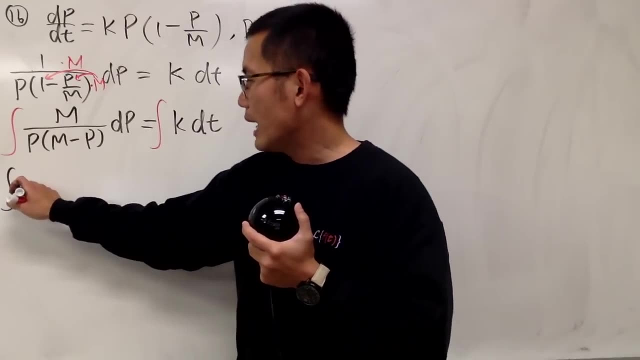 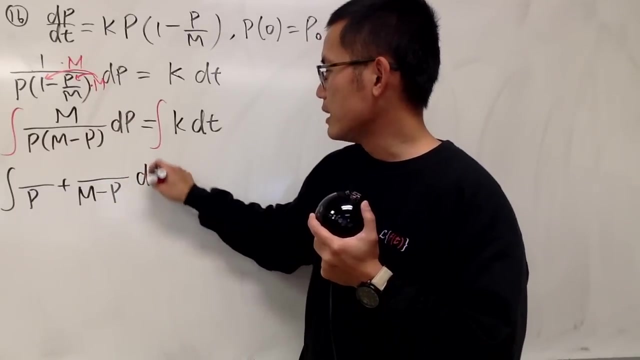 notice: this is p to the first and this is also linear right m minus p to the first. so I will actually just write this down again. we have to integrate. I will have to first get over p plus something else, over m minus p, and we have the dp. 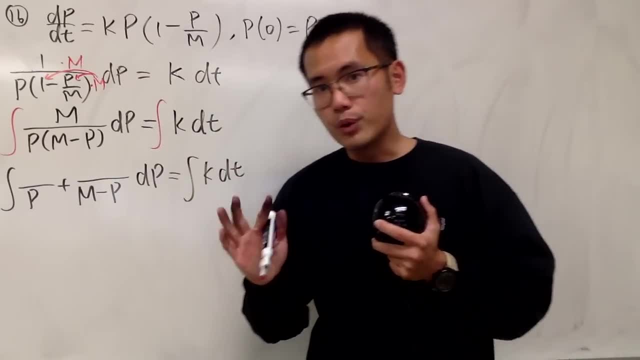 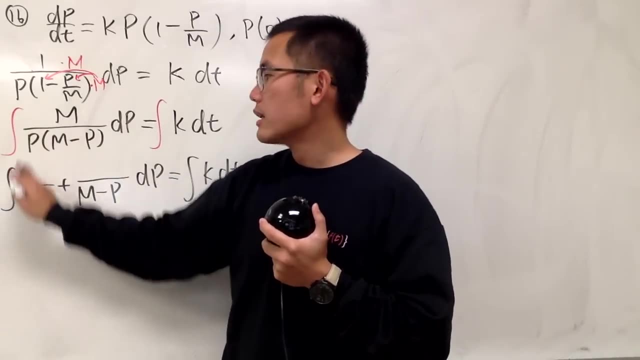 right here and we still keep the integral k dt, like. so now we will integrate. we will do the partial fractions by the cover up. to figure this out, I will come back to the original cover. the same denominator, which is the p, and how can we make p equal to zero? 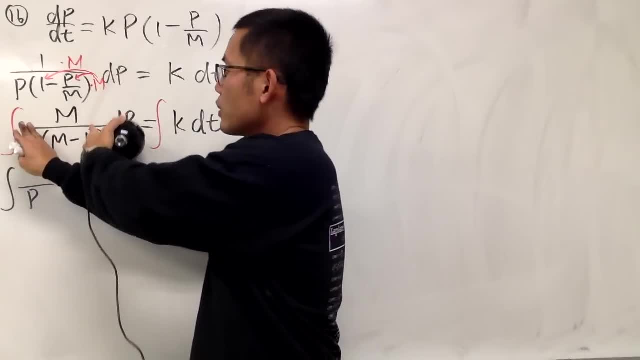 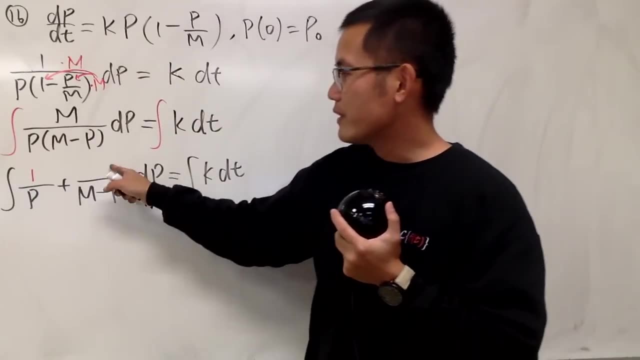 p has to be zero. then we put zero in here for the remaining p over m, which is just going to give us one. so the number that we need is one right here now to figure this out, I will go back to the original cover. the same denominator. 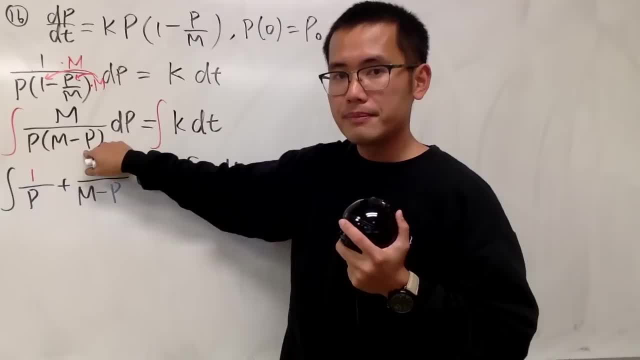 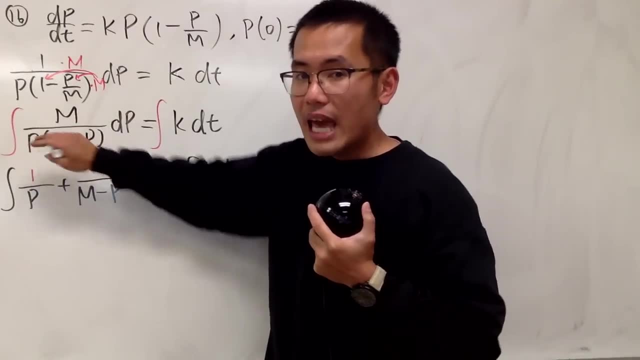 how can I make m minus p equal to zero? p has to be what p has to be. m right, so you have to put m in here and you get m over m again. you have one, which is very nice. so that's what we have and now we can just go ahead. 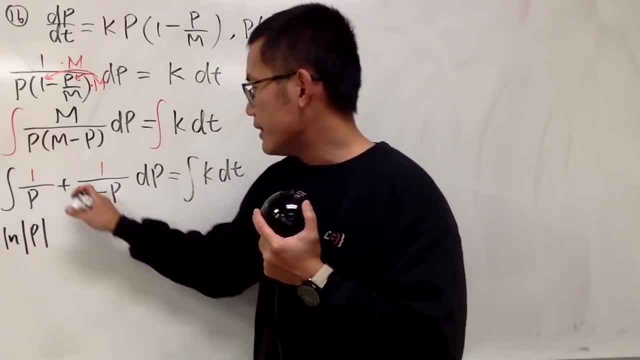 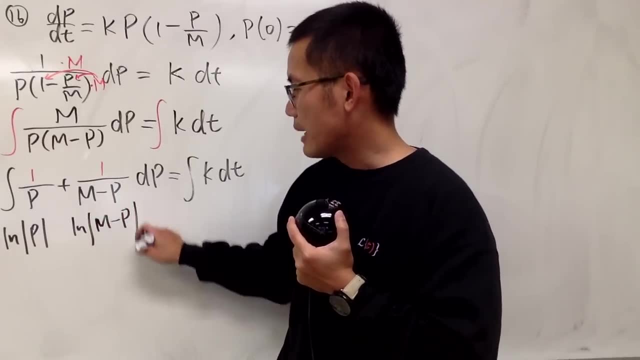 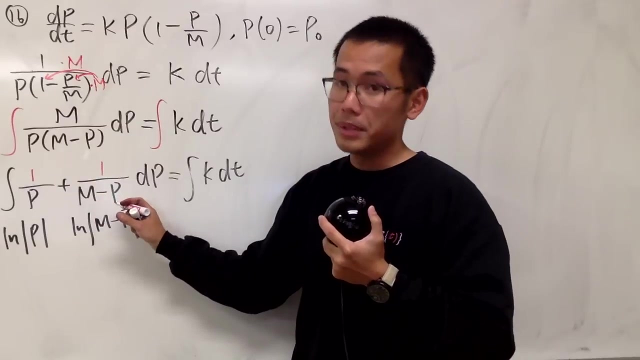 and integrate this part, we get ln absolute value of p and then we are going to have this part which is ln absolute value, m minus p. but again, don't forget the Lu chain, the backwards of chain. Lu derivative of m minus p in the p world is negative one. 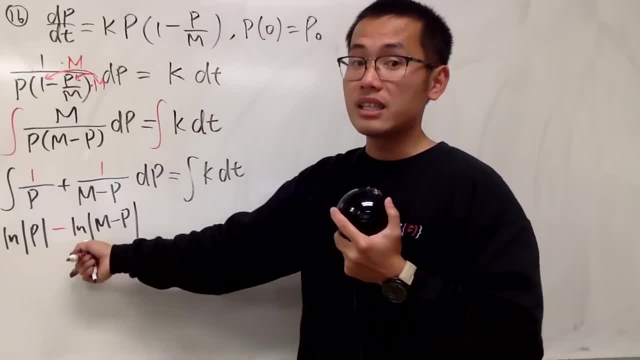 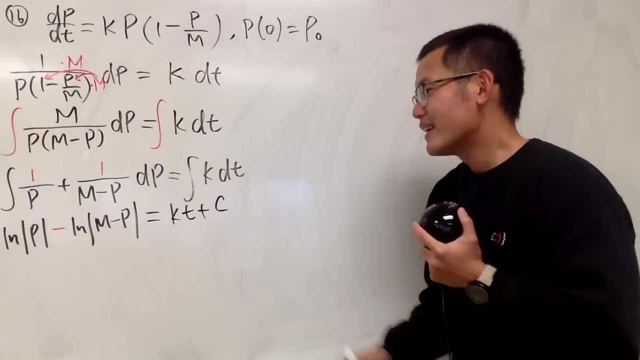 you have to divide it by negative one. divided by negative one is the same as multiplied by negative. right there, so it becomes negative, right there. right, you don't see any numbers right here. alright, so this is the idea. now I want to isolate p. to do so. 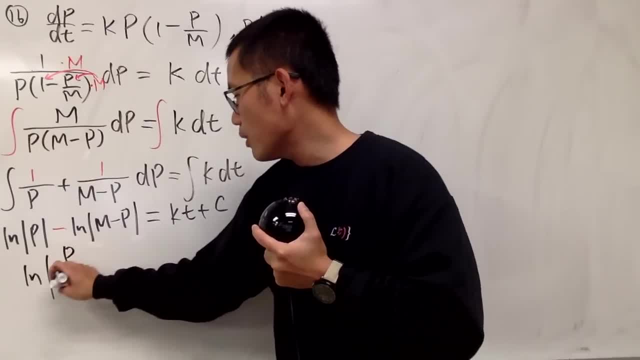 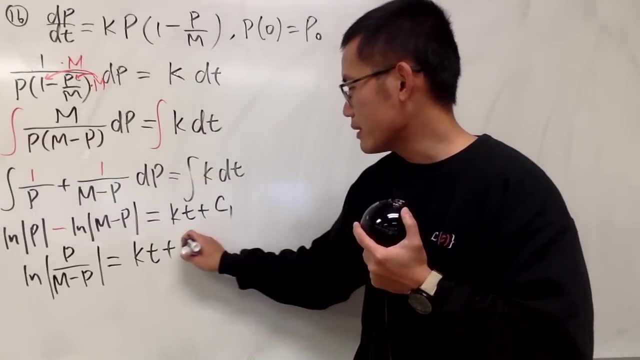 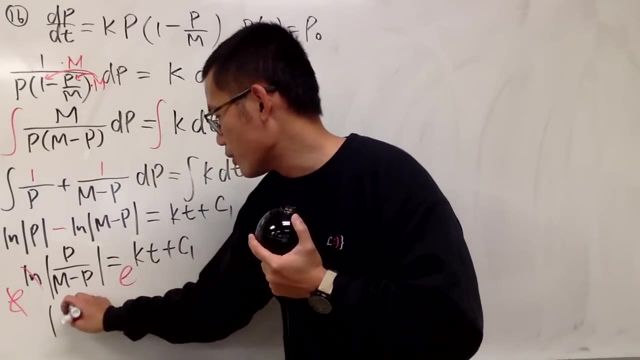 combine the natural logs ln and we will just put p on the top over m minus p, and that's equal to k, t plus c, c one. let's put on c one. then I will just do e to this power, e to that power. they cancel, and then I'll have 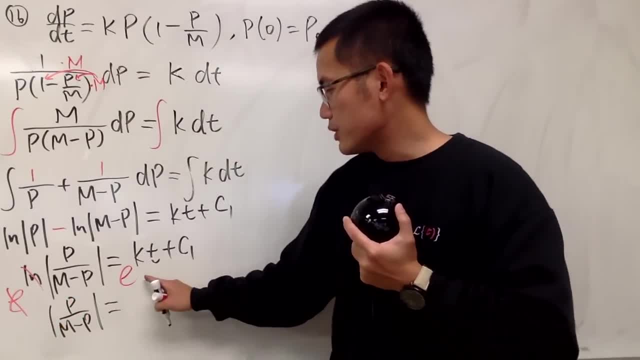 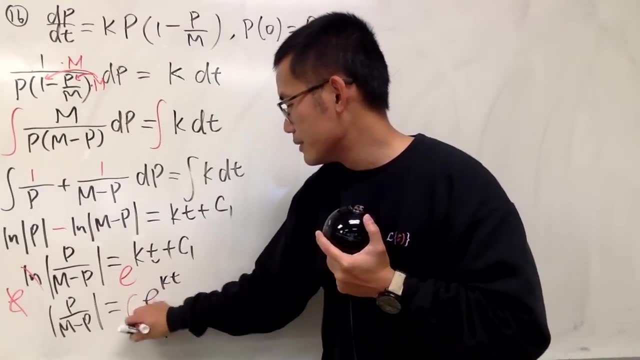 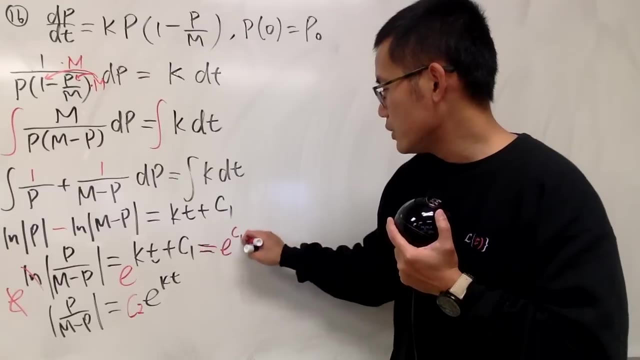 the absolute value of p over, because this is just the function part, so keep it. but e to the c one is just c two, right, because remember, this is the same as saying um, this is the same as saying e to the c one times e to the. 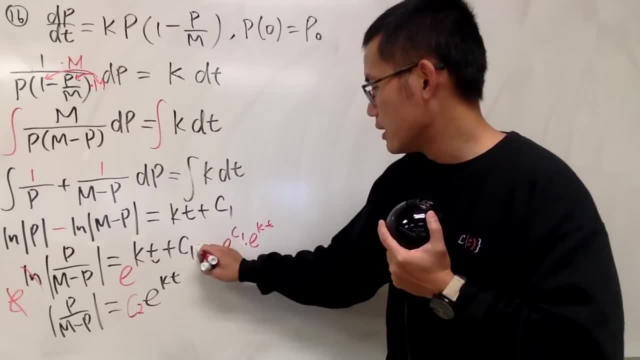 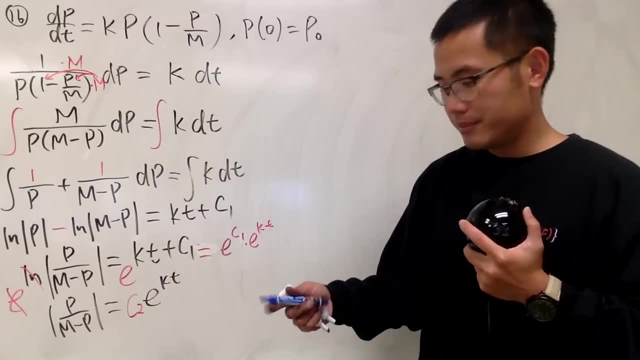 kt, right, so this part is the same as that. so that's why this is the same as c two. now how can we get rid of the absolute value? I'll pick you out later. I will just get rid of the absolute value literally, but don't forget. 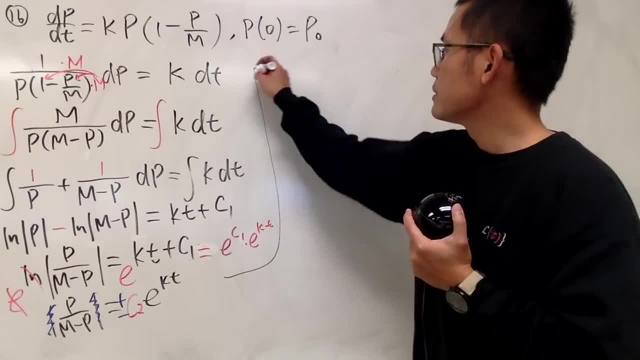 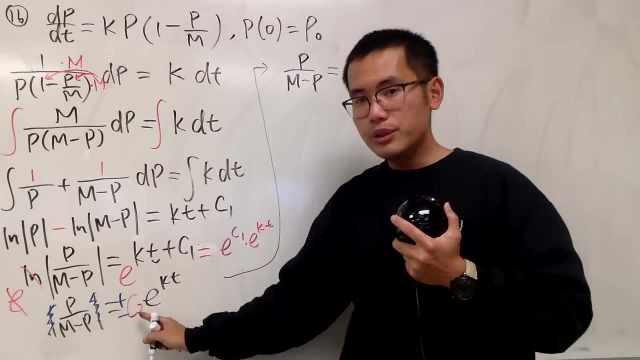 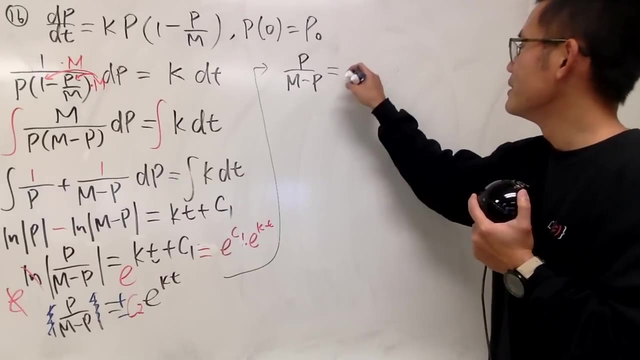 the plus minus. so we will have the following: p over m minus p equals c two is a constant minus c two is also a constant. that's called out to be c three. so here we have c three. put that in blue, why not? and then kt e to the kt power. 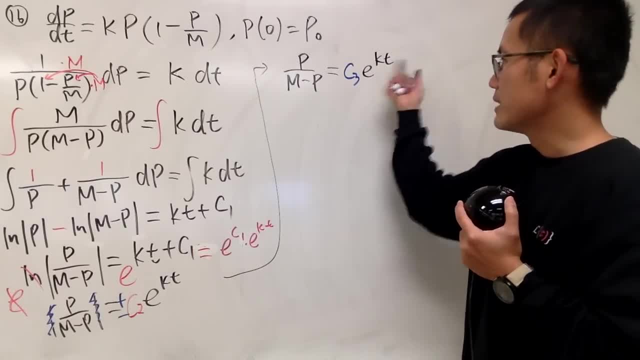 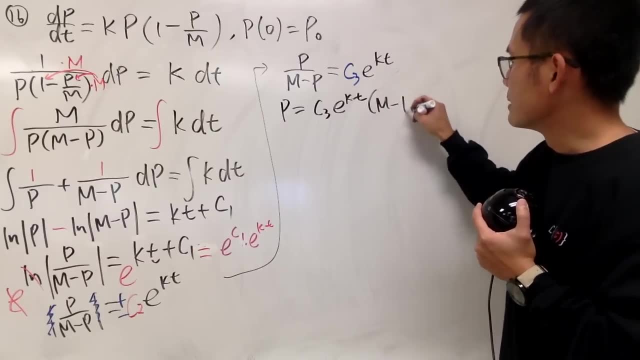 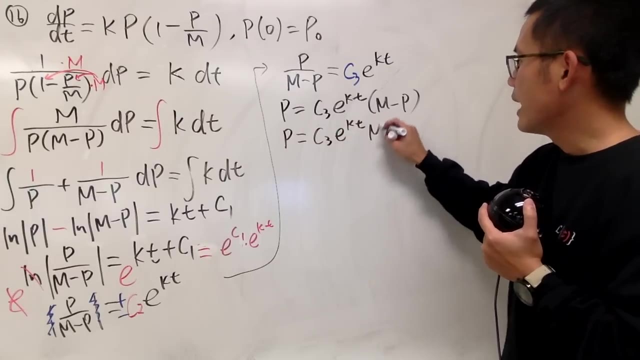 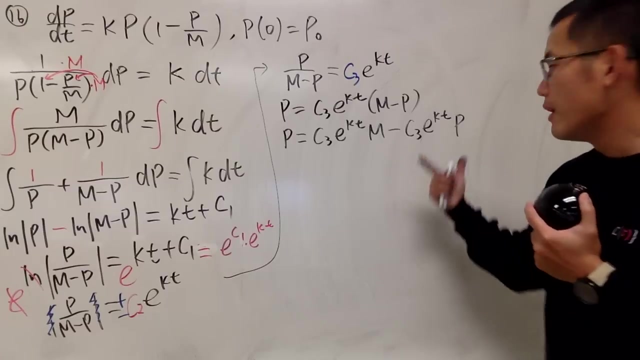 like this: now we can actually isolate the p multiplies on both sides, so we have p equals c three e kt times m minus p, like. so of course, distribute that p equals c three e kt times m minus c three e kt p like that. now bring this: 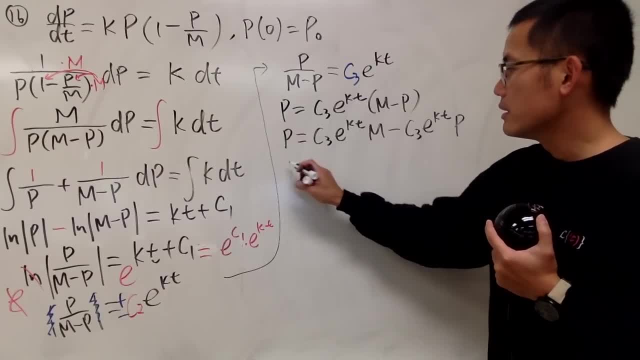 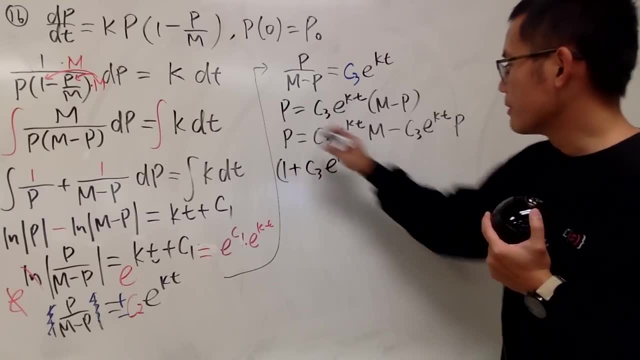 to the other side, then both of them have p. so a factor of p- this is one. the other side becomes positive c three and then e to the kt and then we have the p. put that at the end, and this is equal to c three, e, kt. 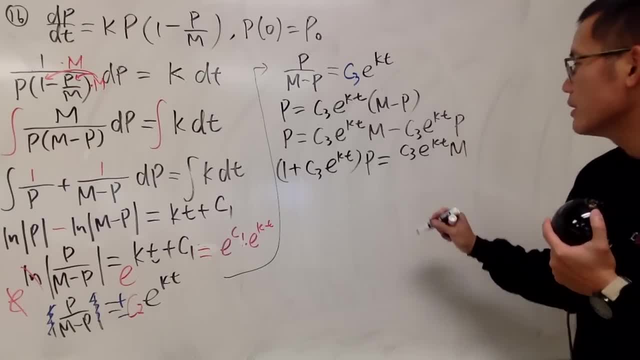 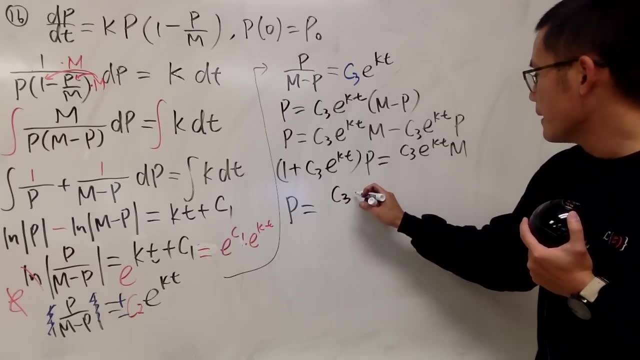 and then we have the m- m is now in the exponent, okay. and finally we can just divide both sides by this. so we have p equals over this, which is c three e to the kt power times m over this, which is one plus e to the kt power. 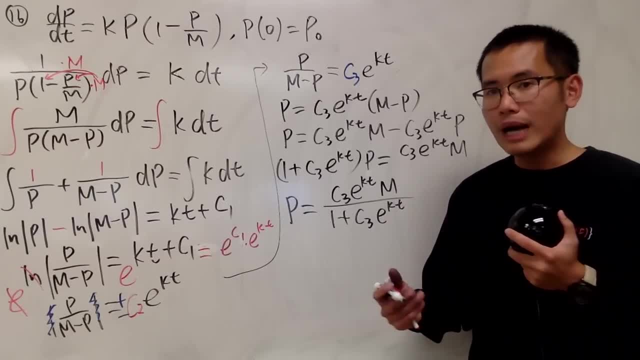 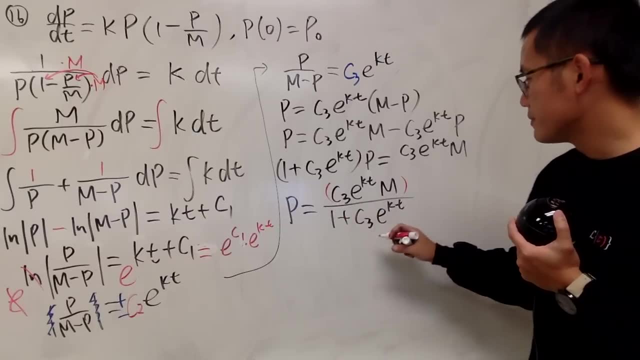 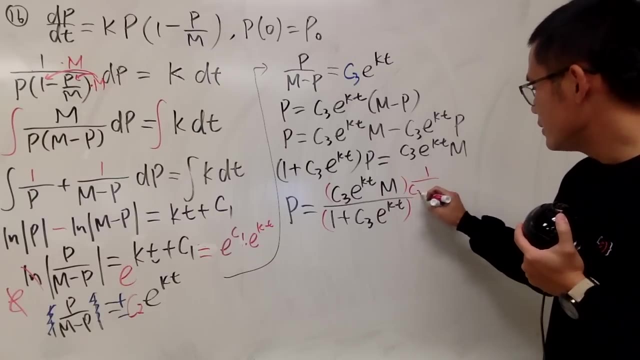 like that. so this is pretty much it, but usually we like to have just one e to the whatever part to do. so we are going to multiply the top and bottom by well, you can just do this. we are going to divide the top and bottom by this part. 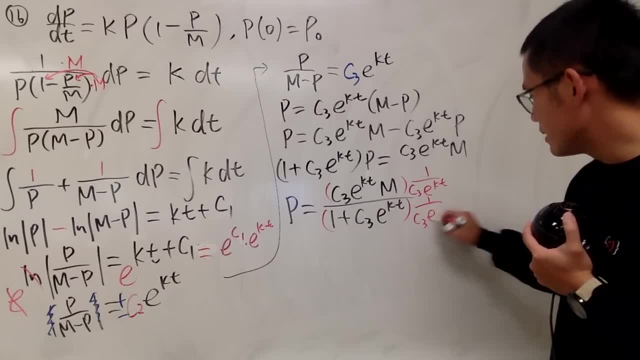 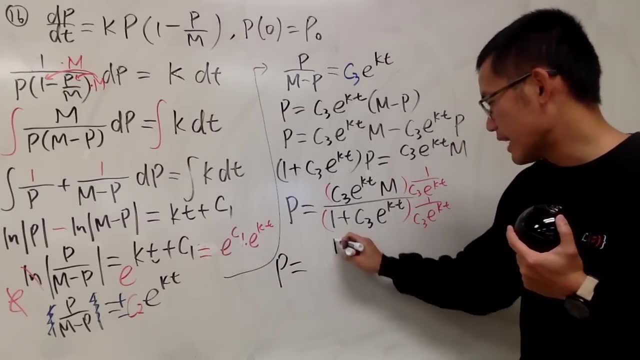 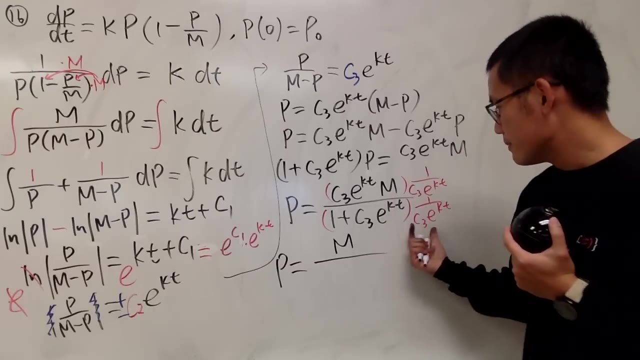 c three e, kt. c three e, kt right. divide both sides, the top and bottom, by this. so finally it's just m, that's nice, very nice. the bottom this times that is just nicely equal to one right and this times this: I will write this down first. 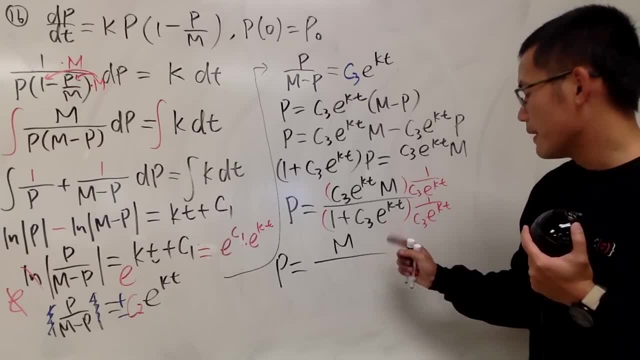 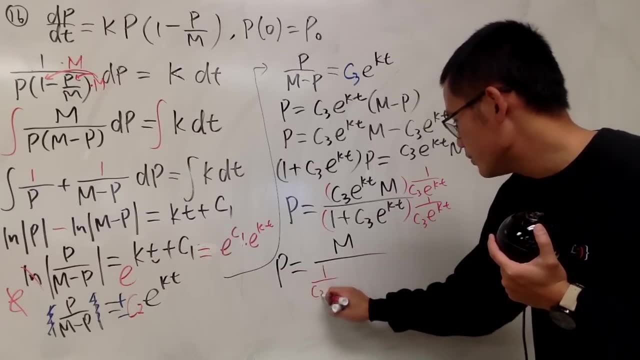 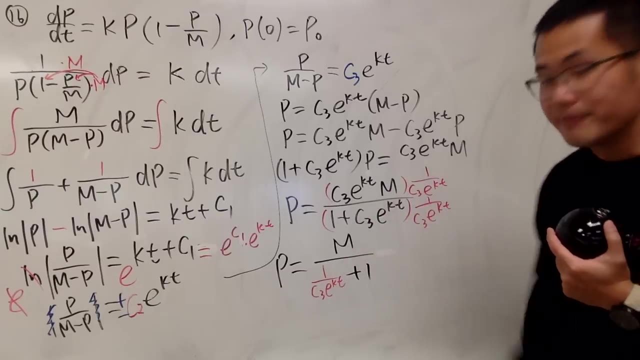 I will write it down like this: this right here is: this times that is just one over c, three e, kt, and this times this is just plus one, like that, yep, good, and of course I will rewrite it a little bit: this right here I have the m. 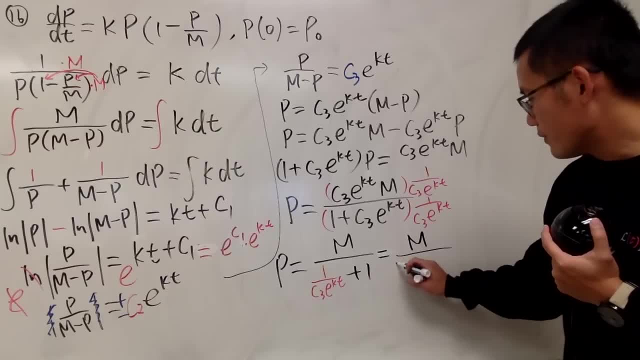 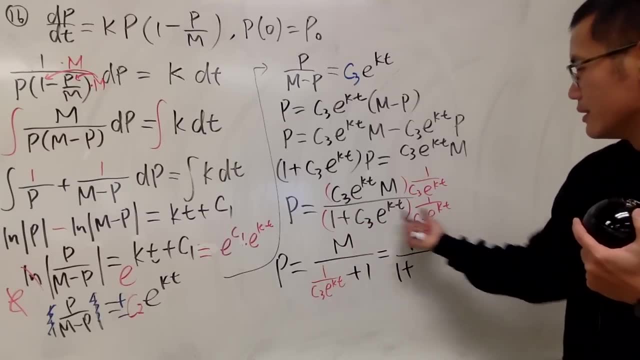 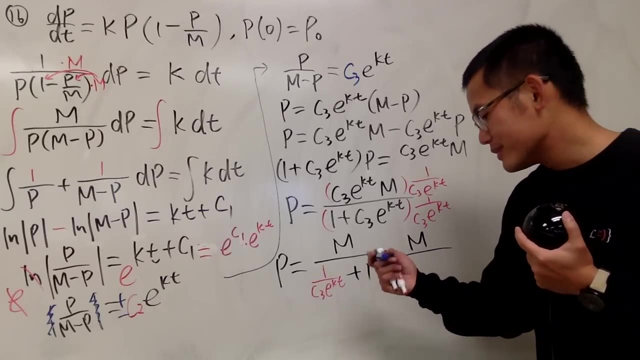 on the top over. I will put down the one first, and the reason I didn't do that earlier is because I don't want to confuse the with the one and one. yeah, anyway, it just worked out, algebra stuff. anyway, here another thing I want to show you. 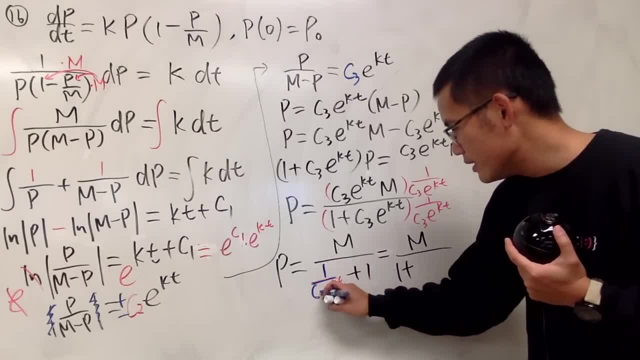 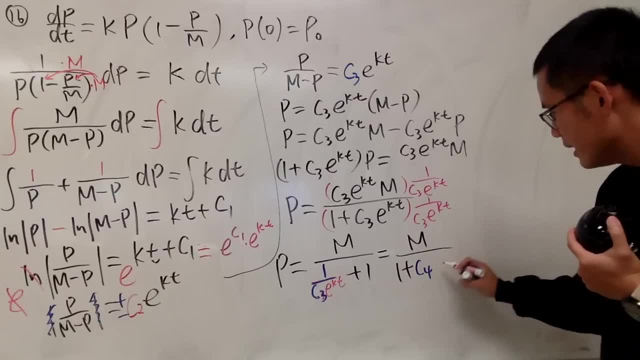 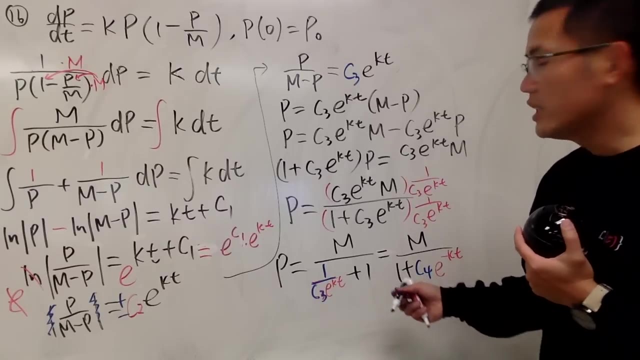 c three is a constant one over c three, so I just put out to be c four, like this. e to the kt in the bottom. I will write it as e to the negative kt, like that. so this is the general form for this, so the general solution. 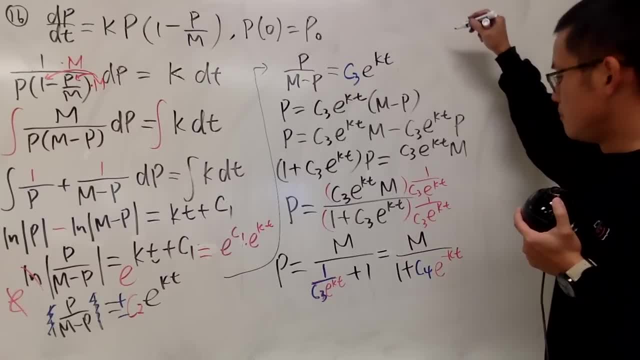 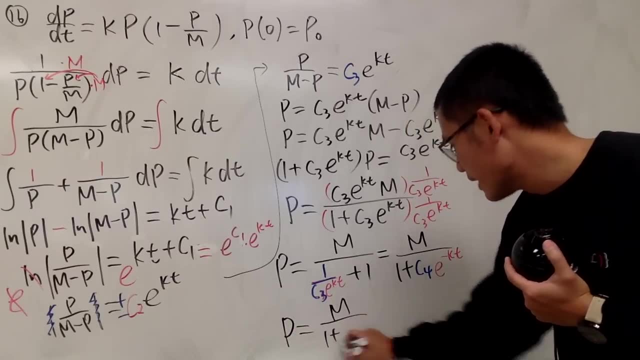 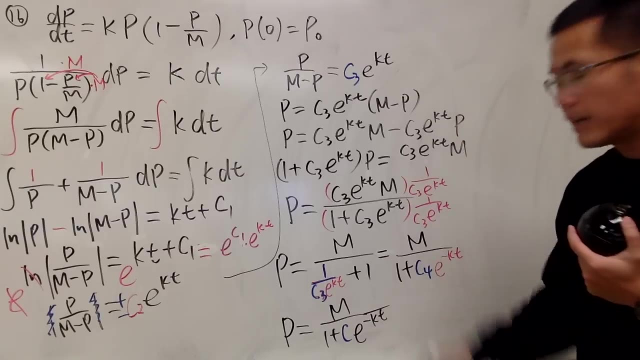 is. let me write it down. hmm, let me just write it down like this: p equals m over one plus. finally, I will just put this as the legitimacy. and then we have the e to the kt power like this right. so this is the general solution. now, how can we figure out the c? 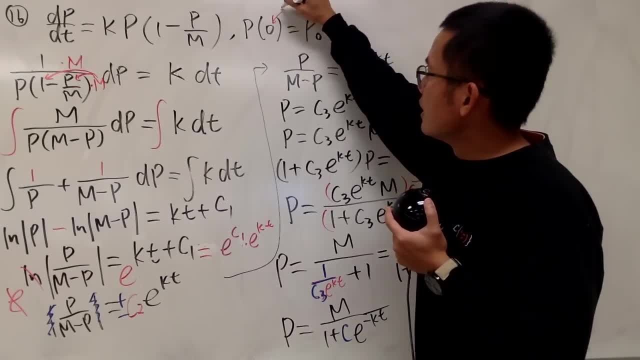 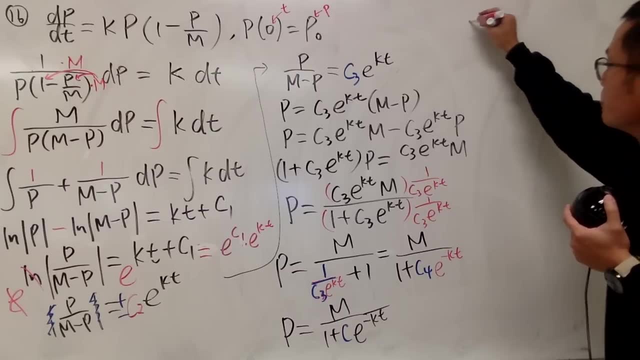 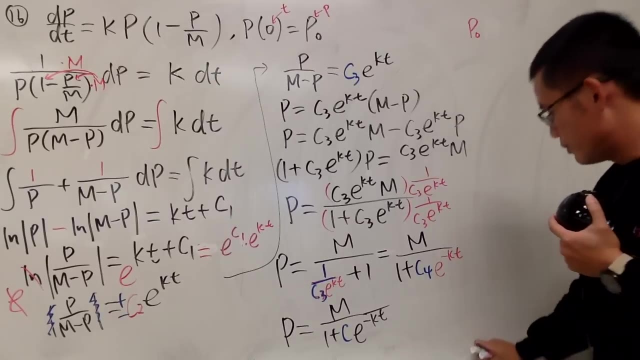 well, here is our work. this is the t and this is the p value, right? so on the eleventh side, I will have p zero. that's equal to, and we have to plug in zero into the t. so here we have the m. let me just emphasize this in blue. 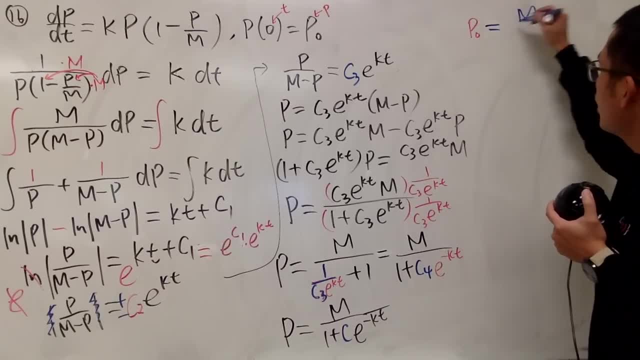 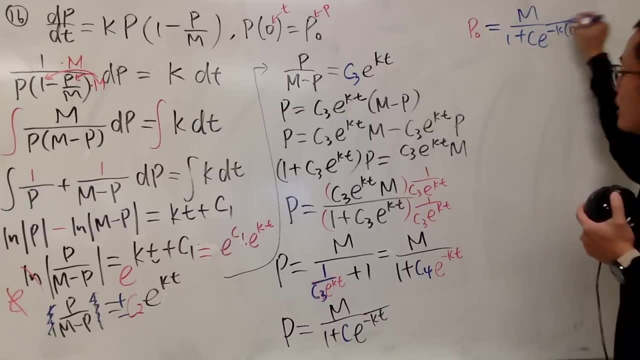 this is equal to m on the top over one plus c is c, and then e to the negative k times zero, like this: now, this is good because this is just one. so we have p, zero, equal to m over one plus c, and then I just have to get the 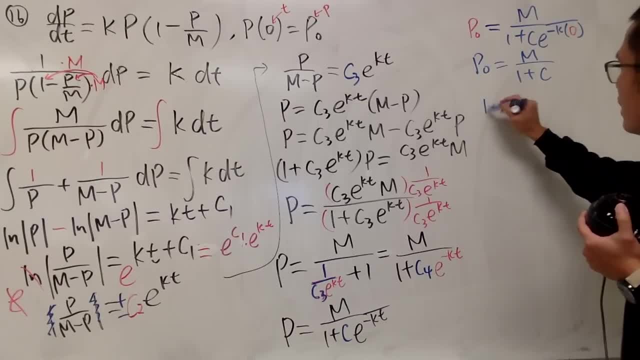 c by itself. let's do the reciprocal on both sides, so I get one plus c over m equals reciprocal, so it becomes one over p zero. and then I will just multiply the m on both sides, so one plus c equals m over p zero minus one, so c is equal to. 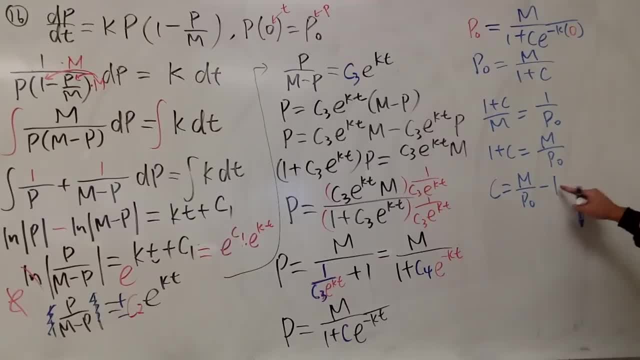 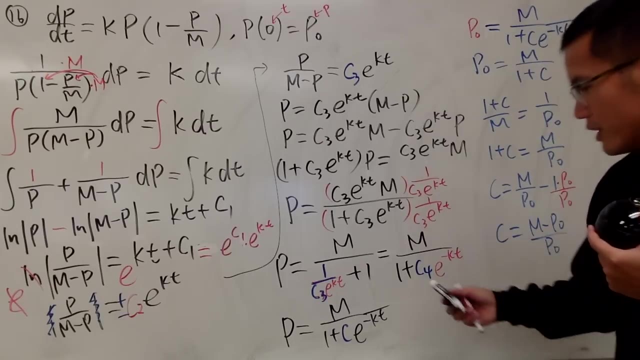 m over p zero, minus one, which I will just multiply this by p zero and p zero or p naught and p naught, depends how you want to say it. finally, c is equal to m minus p naught over p zero, like this. so here is the general solution. 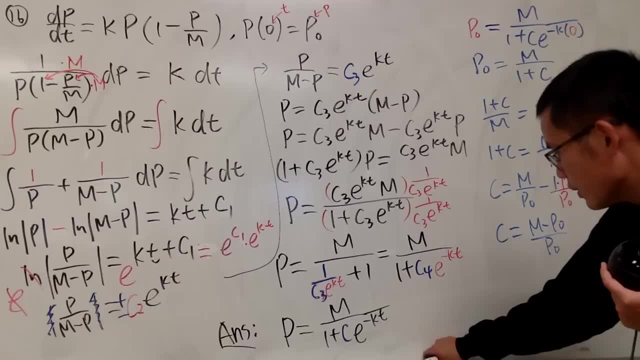 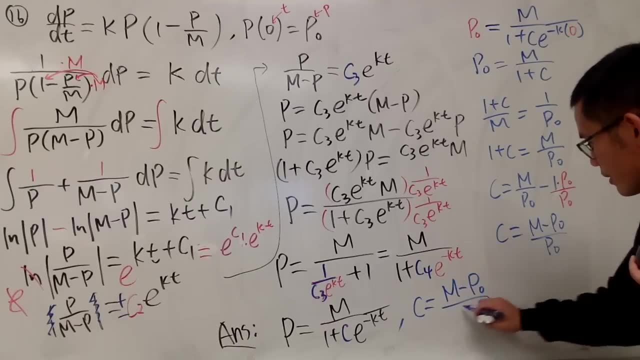 here is the answer. this is the general solution, along with the c. I will just include it right here for you guys. c is equal to m minus p naught over p zero. usually I don't like to put this back there because it gets too messy. you can just work that out. 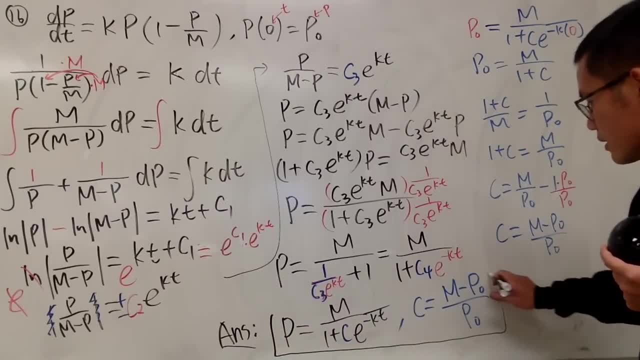 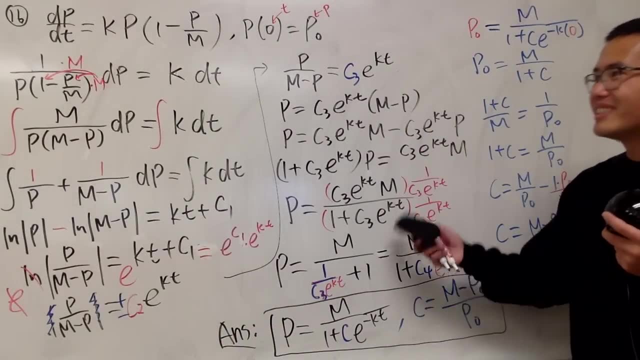 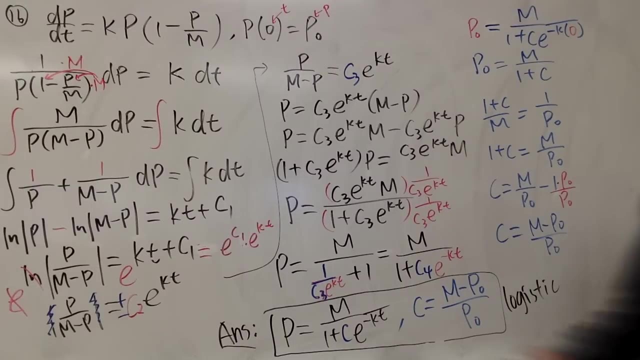 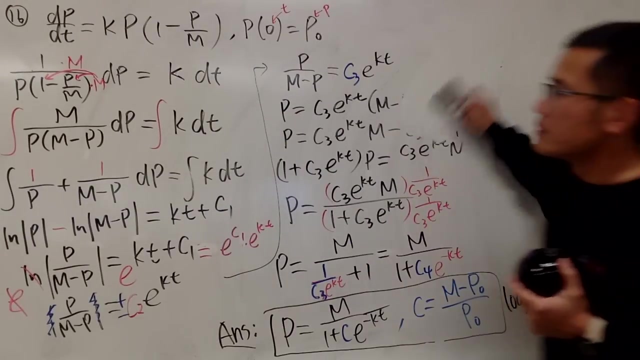 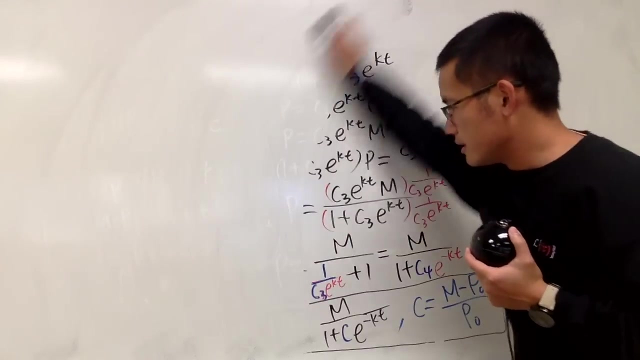 and then put that at the end. so personal preference. yeah, you can put. just work it out on your own, whichever way. anyway, this right here is it the joystick differential equation. perhaps I should write it down somewhere. I will write it down here, the differential equations. okay, good, 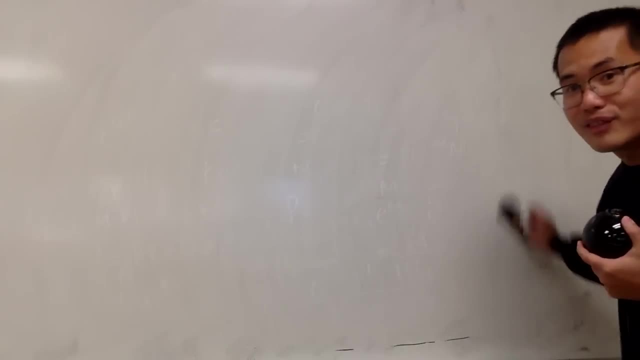 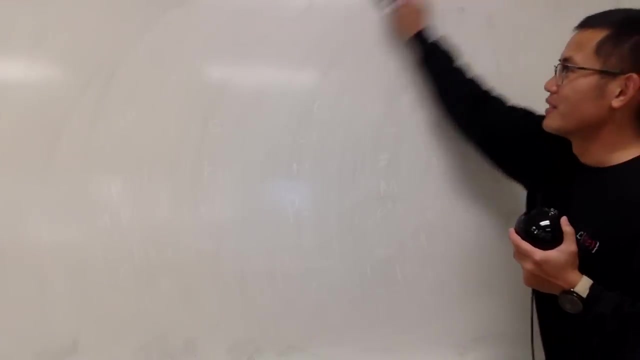 oh, by the way, there is like a missing solution for that as well, but I do have the initial condition, so I don't have to worry about the missing solution, because with the initial condition you actually get a curve and all that stuff. so all right, so let's do another growing. 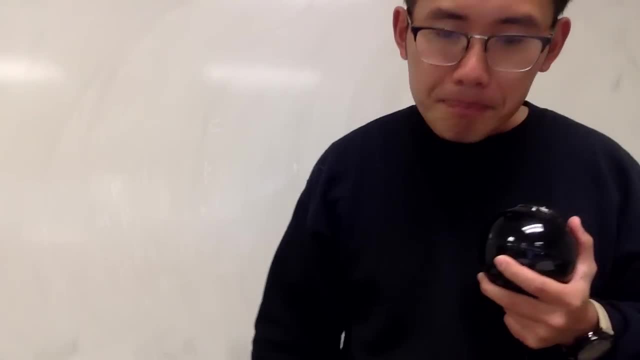 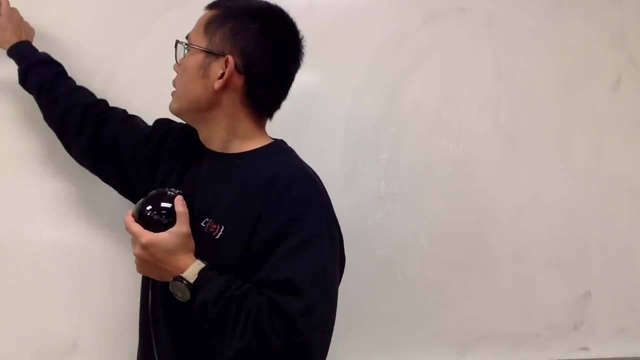 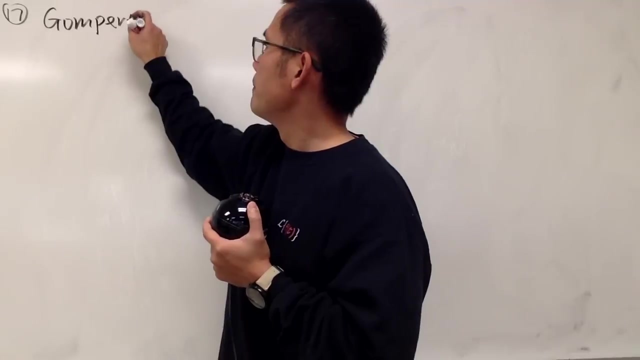 thing. this is called a compass, com, gumpast, gumpast. so this is number 17. here we go, number 17 right here, so I will write this down right now. gumpast, yeah, differential equation. so I will write this down right here for you guys. 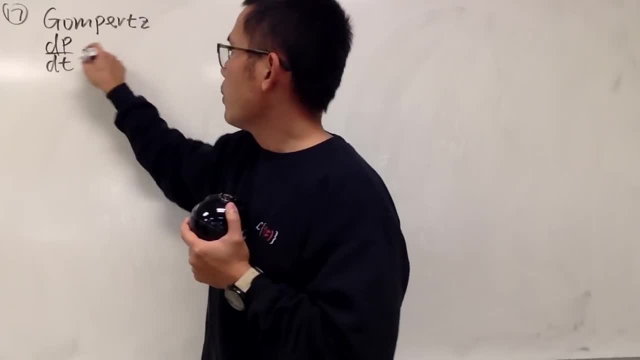 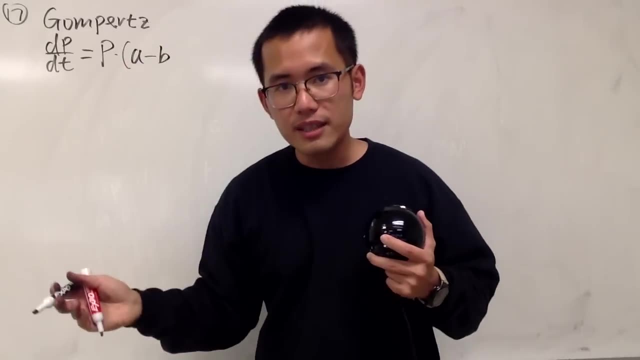 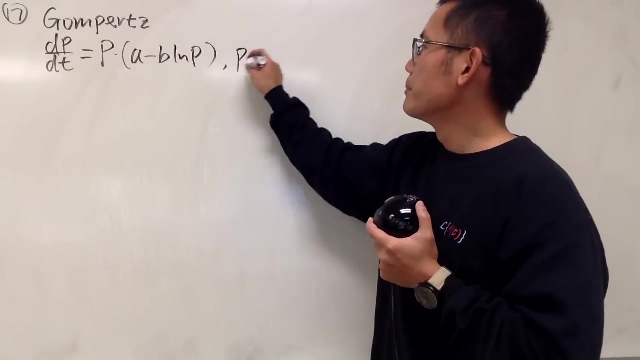 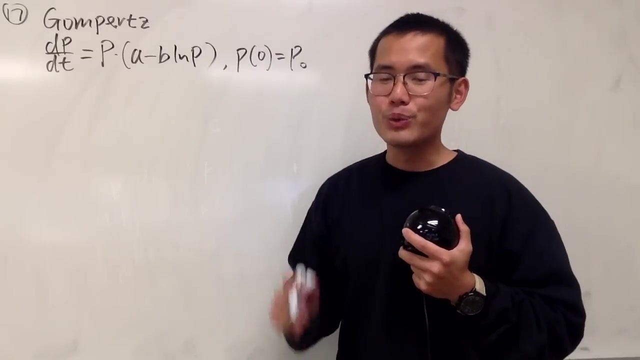 we have p, p equals- this is personal, but bear with me- p times apprenticeship round. a minus b, and that is the constant. Then we have ln of p, and let's also have the initial condition where P of 0 is p, not like that this. 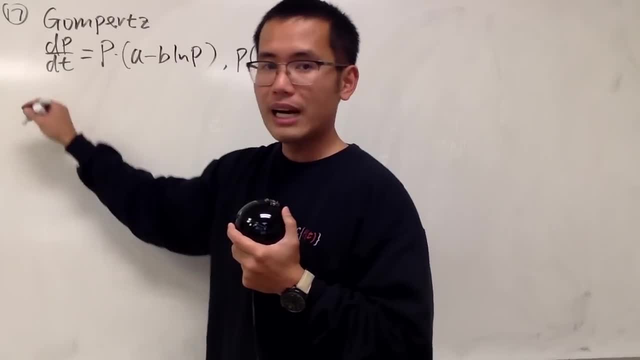 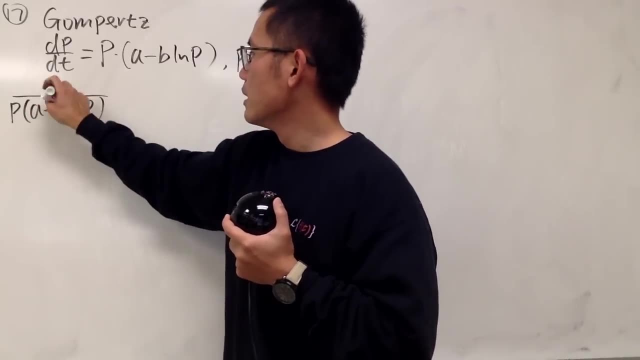 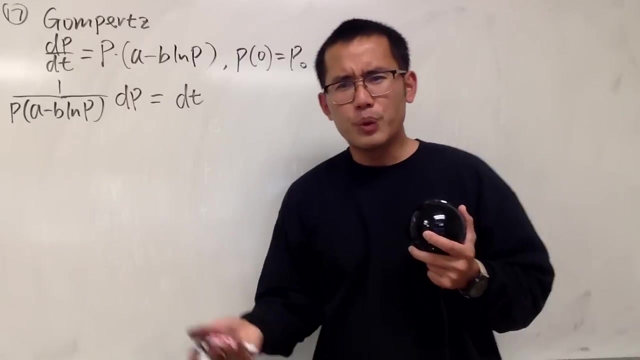 looks crazy, but it's not so bad. 1 over p times a minus b, l and p like this, And we are in the p world. so we have the dp here and that's equal to dt. And you might be wondering where's the k, where's the constant proportionality? 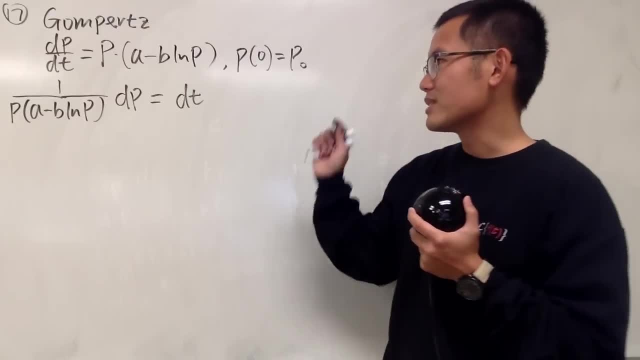 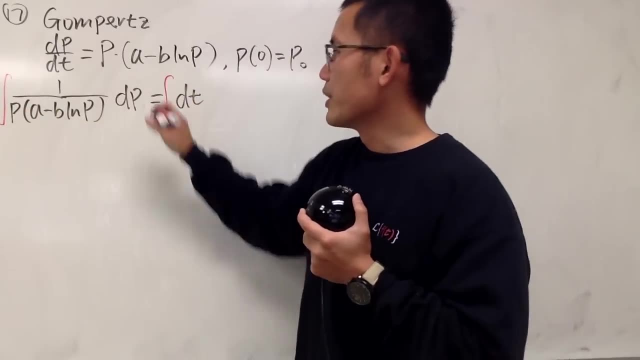 Don't worry, it's a and b, that kind of thing, right? Yeah, let's just take care of that. Okay, so this is what we have. and then, of course, let's go ahead and integrate both sides. Integrate here, integrate here. 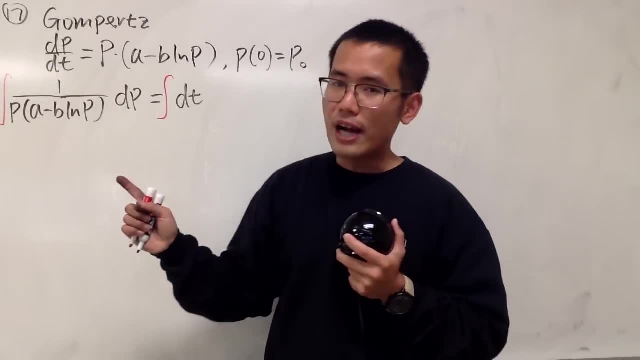 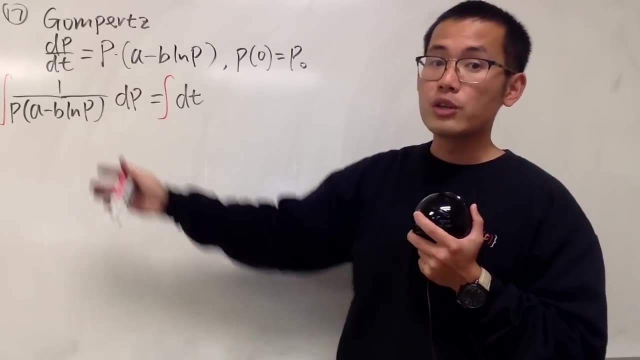 Do we do partial fraction here though? No Partial fractions, it's only good for rational functions. Here you have l and p, so it's not polynomial. This is not a rational function. Don't do that. But better yet, we can just do u sub. 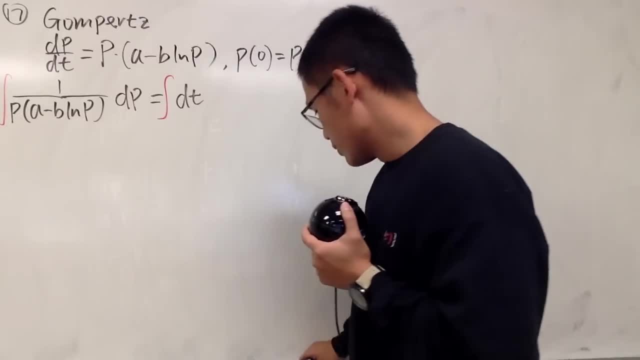 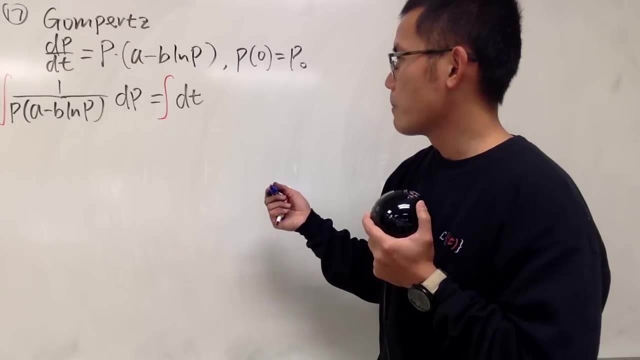 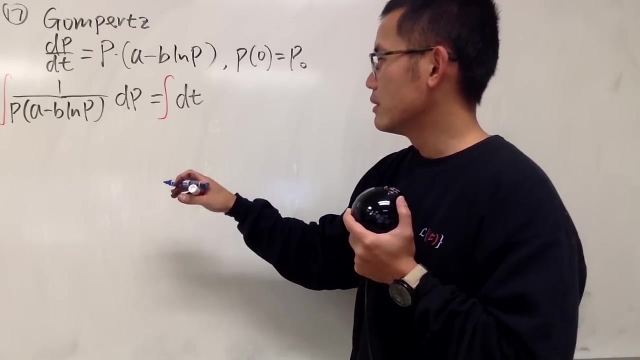 I'll show you guys all the work here, though Right here I will do this in, I'll just do this in blue. Let's see where I can do that. I will do it here. Let me see. Oh, that's just. let me just do it here. 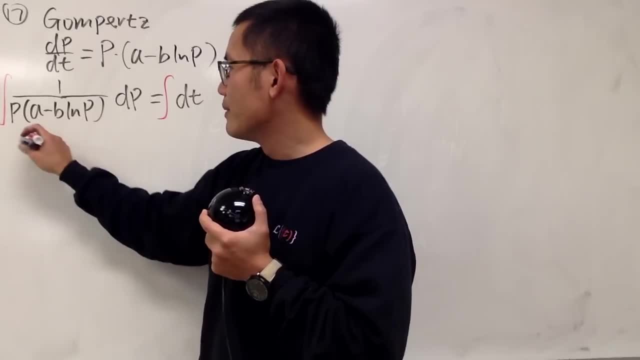 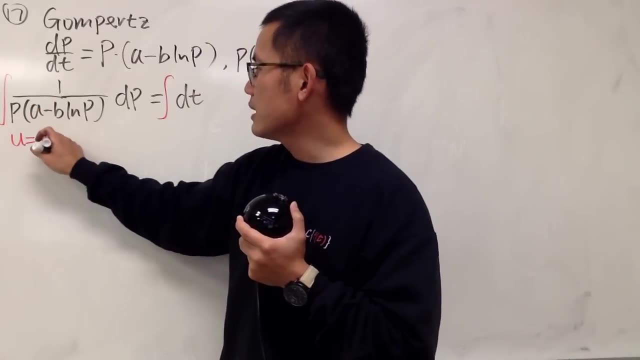 All right, here we go. Oh, I'm still doing it, never mind, I'm sorry. All right, let's go ahead and do that. u equal to the input, which is this: a minus b, l and p. 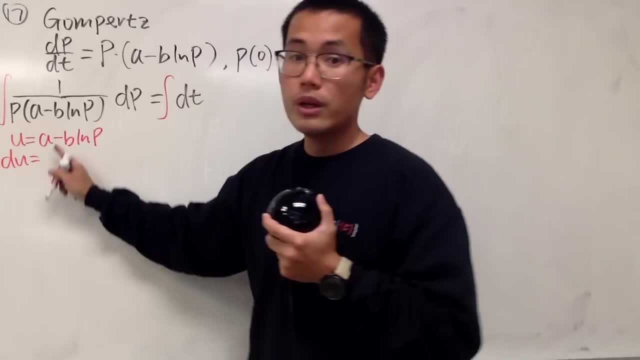 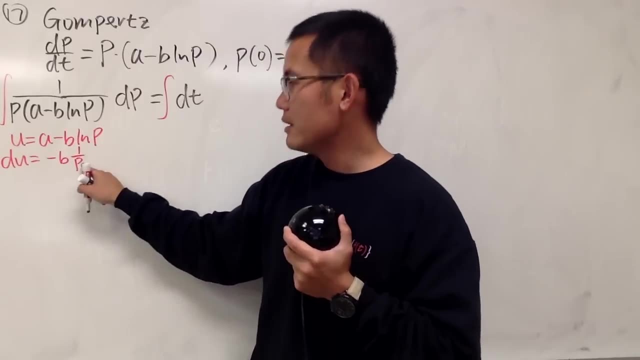 And then you will see that du is equal to. the root of a is 0, the root of negative b in that is negative b times 1 over p. right, the root of p is just 1 over p. dp like that. 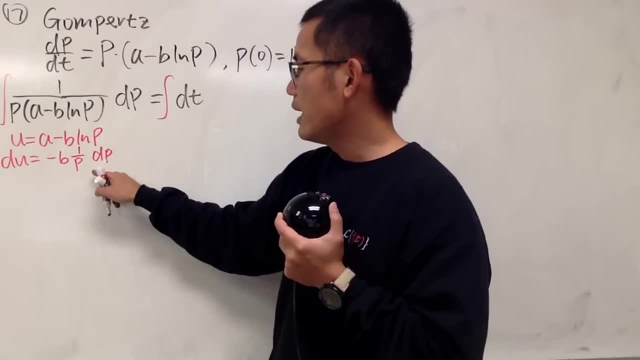 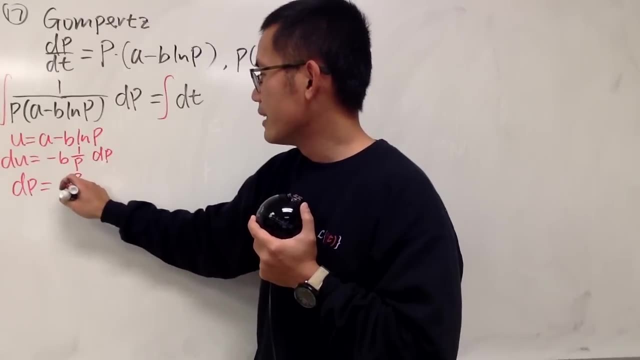 And if you would like, you can solve for dp, and this is crazy. dp is equal to you multiply p on both sides and then negative and you divide the b on both sides and then you have du, like that. 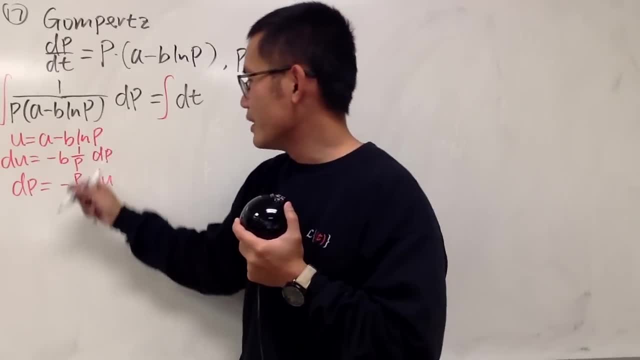 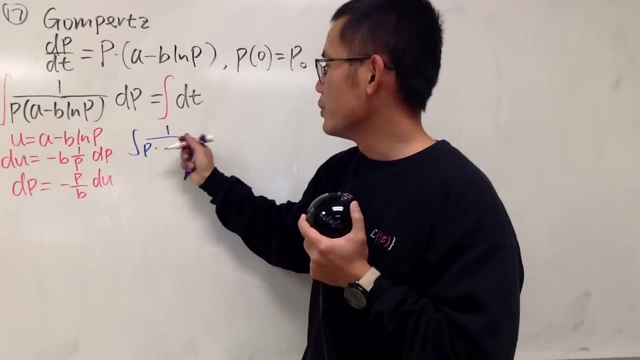 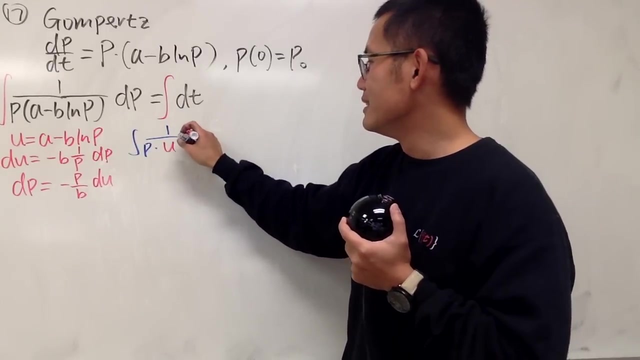 Again, there's no number in this equation, So here is the integral. You will get the integral to be integral 1 over p times u, and then you have the dp, dp as negative, p over b and du like this: 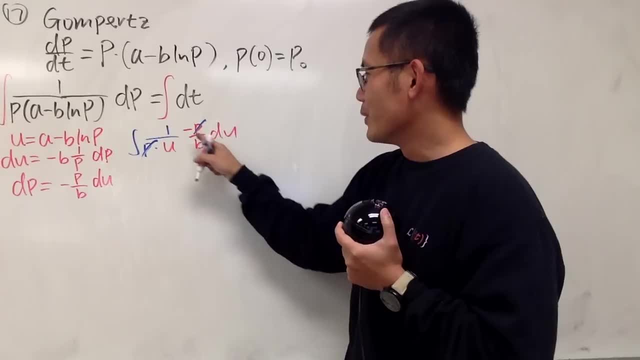 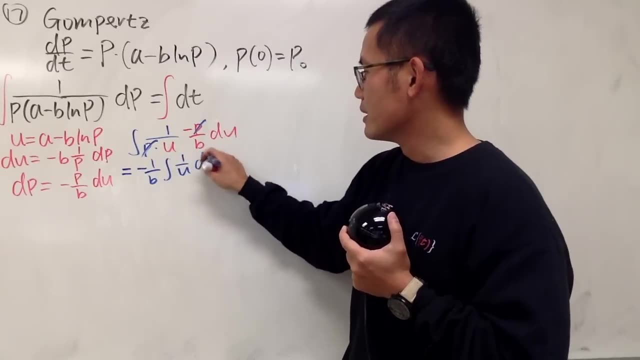 And then you will see that this and that can solve very nicely And we will have the constant multiple which is negative, 1 over b. Just put that in the front and we have the integral 1 over u. du like that. 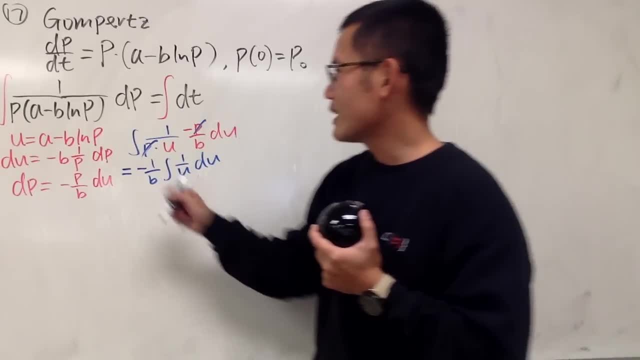 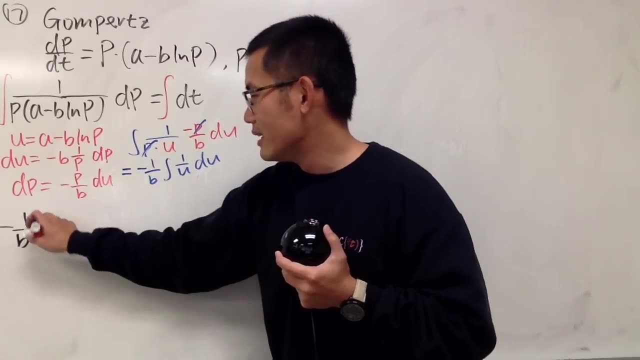 Right, so just kind of work that out. That's pretty much it, And of course I will just write down this right here: We have negative 1 over b, integrating ln. Integrating 1 over u is ln, u and the u is that. so I will just put an absolute value with the u inside. 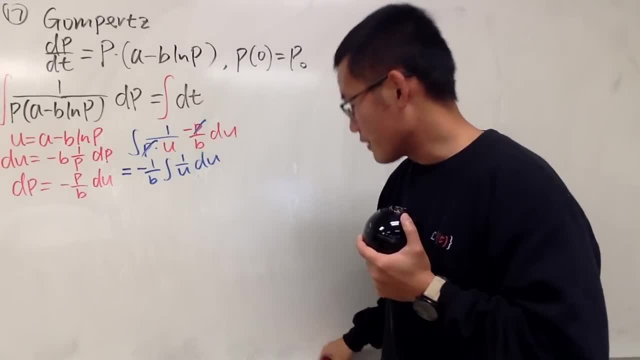 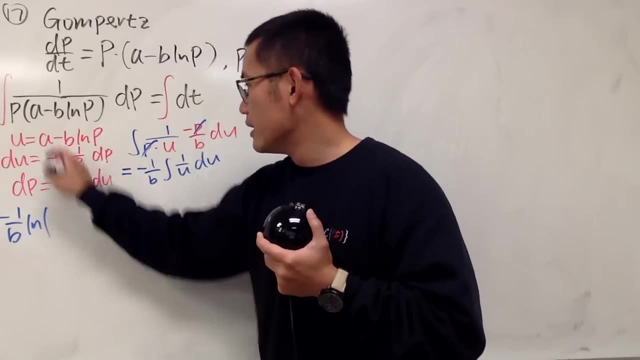 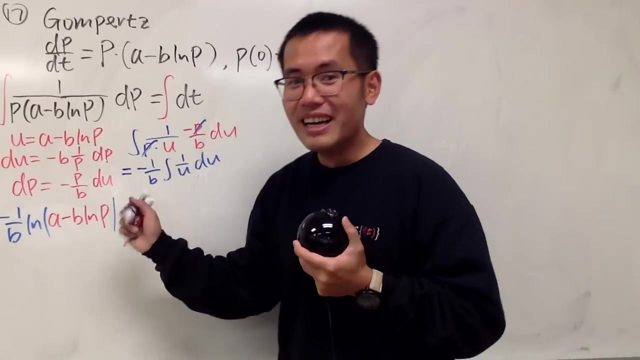 Actually, let me just put this in blue so you can see where I picked off. So this is negative 1 over b ln u, which is that a minus b ln p. Seriously, that's so many letters. So we have all that, and then that's good. 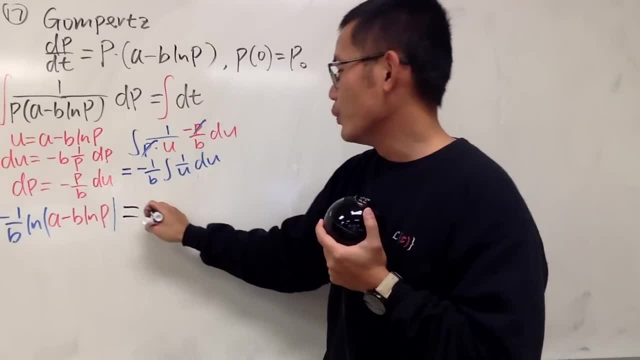 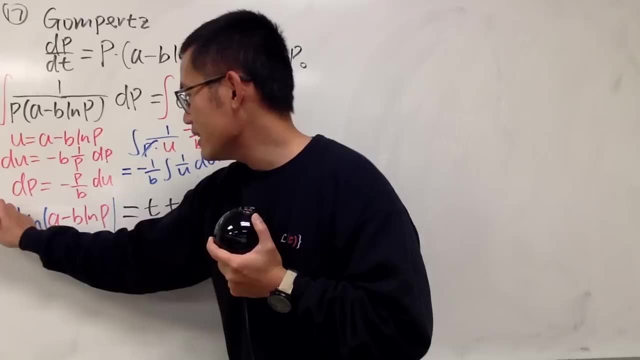 That's equal to the right-hand side. integrating 1 in the t-world, We get t. And don't forget the plus sign, That's c, c1, maybe? Yeah, Now I will multiply everybody by negative b. Why? 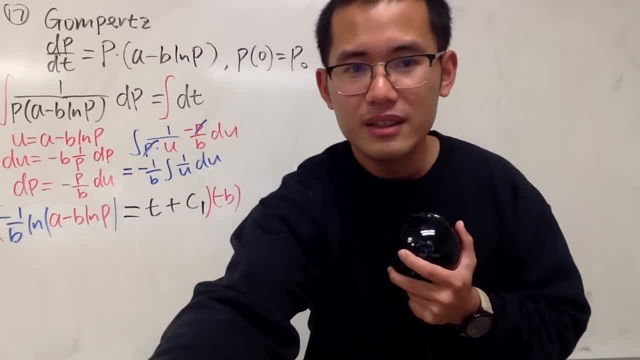 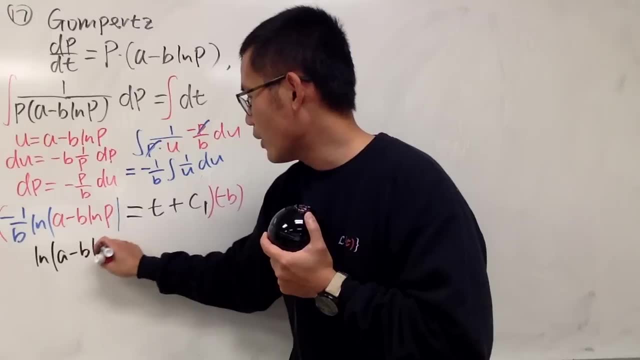 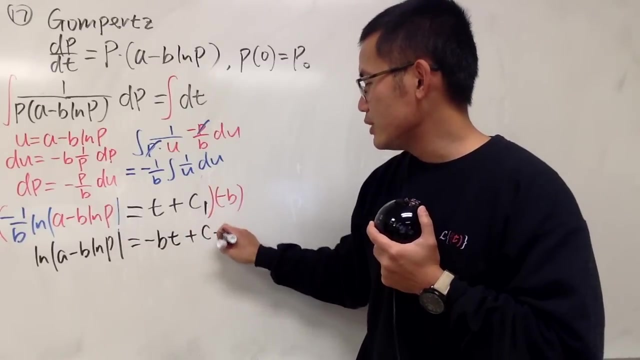 Because I will cancel that out right. So we get negative This times. that is out. So we have ln absolute value a minus b, ln p and multiply this and that We get negative bt And this and that is just plus c2.. 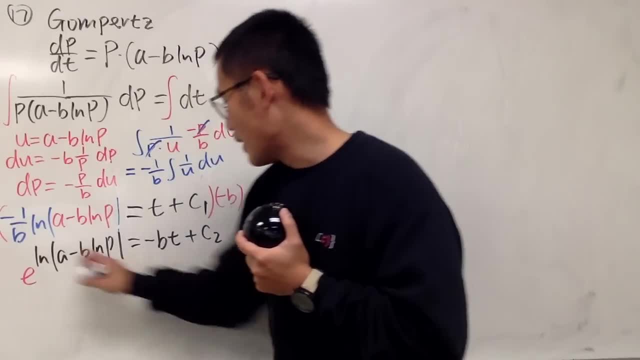 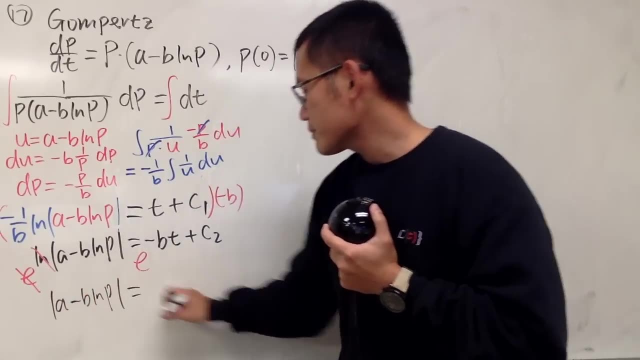 We have done this many times already. Then we do e to this power, e to that power, They cancel. And then we have absolute value of a minus b ln p. absolute value: This to this power stays. e to the negative bt. 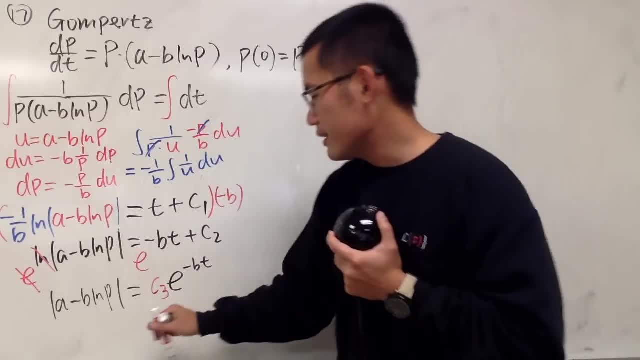 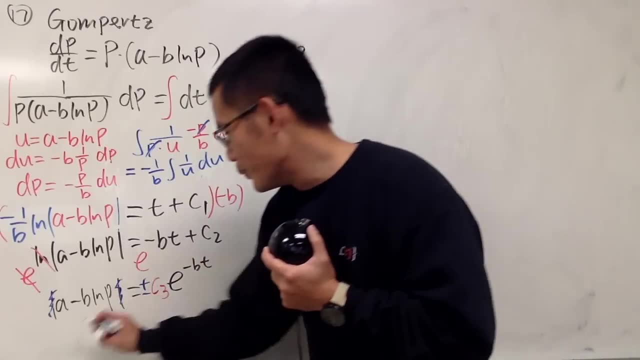 This to. that is another constant, so it's c3.. And then again you can just get rid of the absolute value And then don't forget to put down the plus minus. So that will be another constant. So we have a minus b ln. p is equal to that. 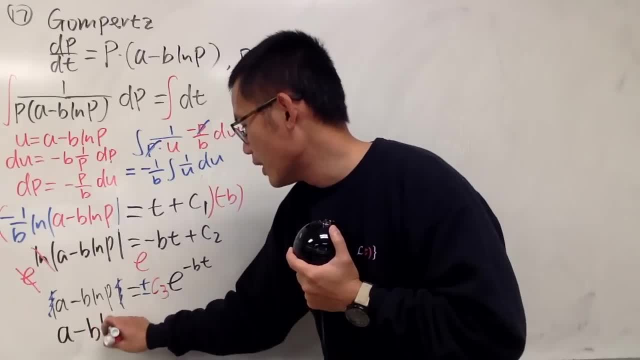 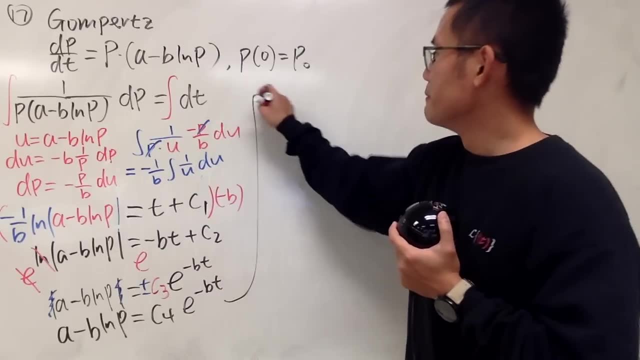 So Let me just write it down. Let me write it down one more time: a minus b, ln, p is equal to c4, e to the negative bt. Yeah, Okay, good, Now bring the a to the other side, becomes minus, and then I will divide everybody by. 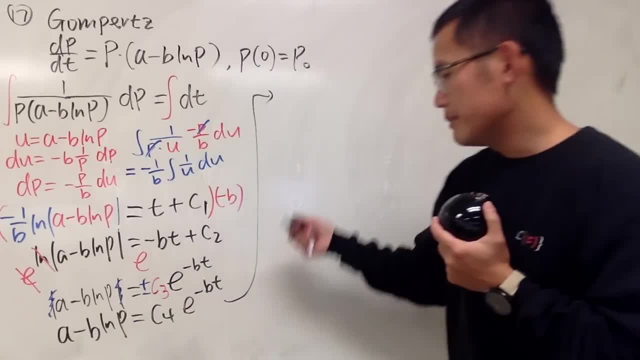 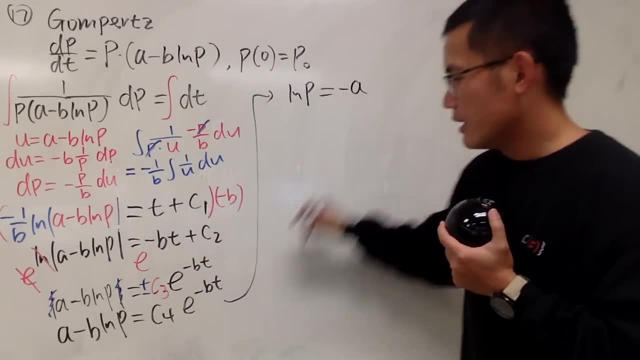 negative b, Right. So be really careful. Let me just write down this right here, and then we'll do a few things in our head. Bring the a to the other side becomes negative a, and then we still have the plus c4, e to. 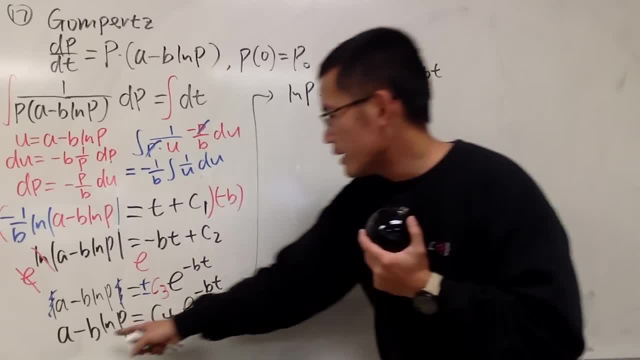 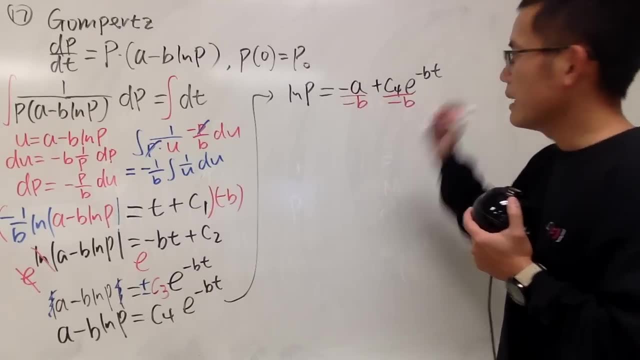 the negative bt. Yeah, So far, so good. And then I'm dividing negative b everybody, So I'll divide this by negative b. I'll divide this by negative b. yeah, So that's pretty much. it Work this out real quick. 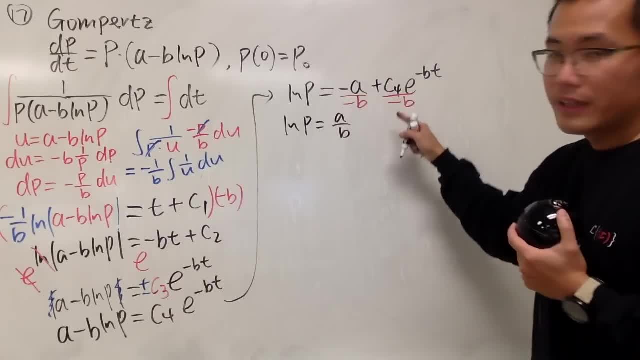 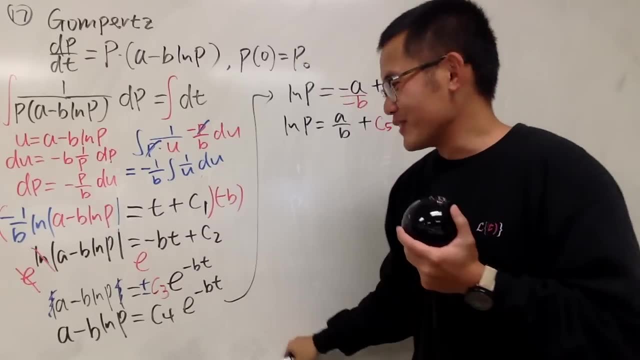 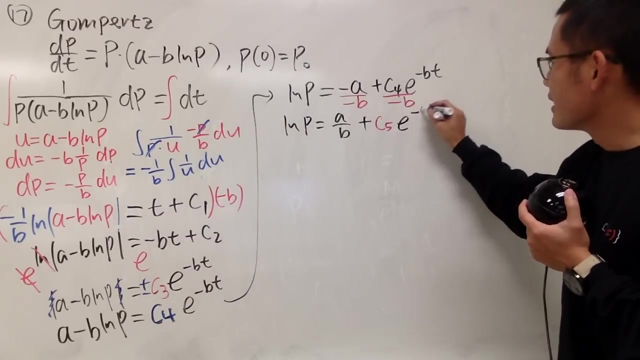 ln, p is equal to a over b. This over that is c5.. So plus c5.. No, it's just so much fun to do all the constants and probably let me just change this to blue. Anyway, c5. So this is e to the negative bt. 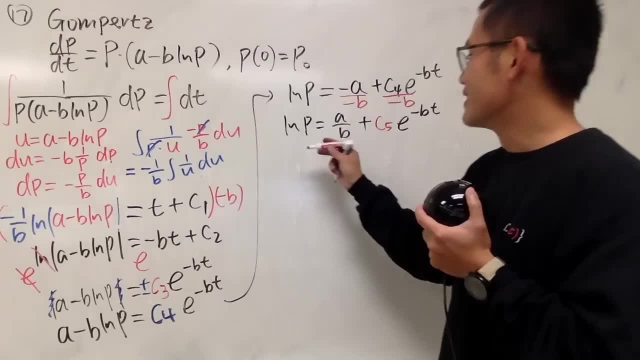 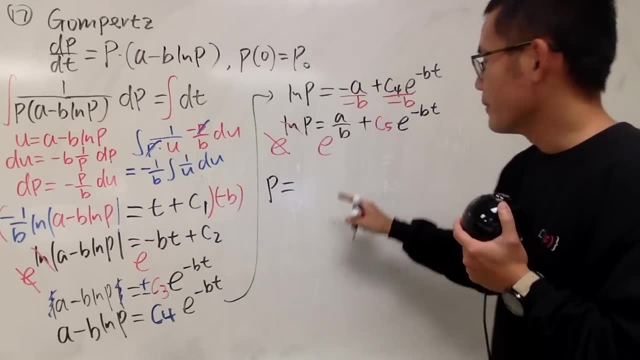 How can we get rid of the ln? Yes, another e. So we do another e. e to this power and e to that power. This and that cancel, and we get p is equal to okay, check this out. e to the ab. 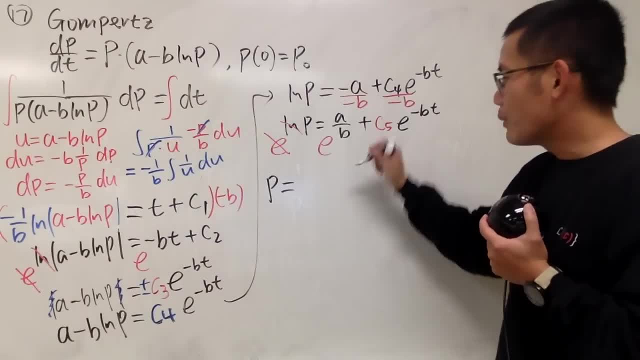 ab are from the original, so you cannot just call them to be different letters, So I will have to write it down: e to the a over b. yeah, e to the ab power. yeah, e to the a over b power. 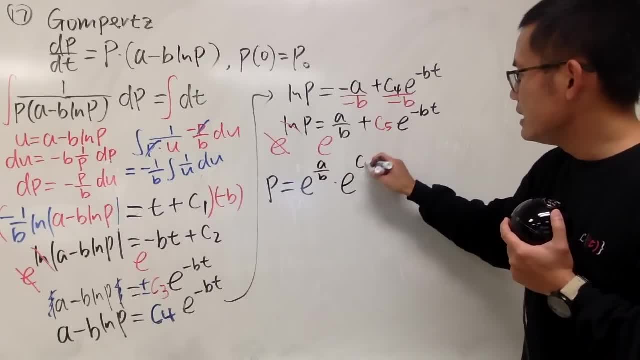 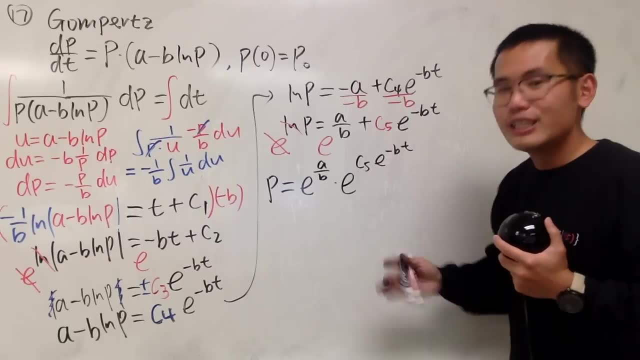 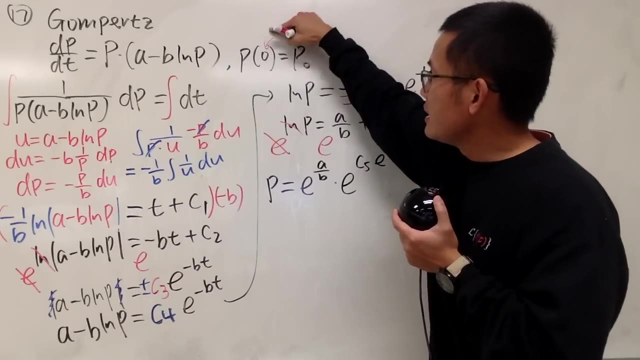 Let's add it. e to this right, e to the c5.. e to the negative bt power. Yes, this is the exponent in the exponent that thing. All right now. this right here is the initial condition. so we have t and also p, so of. 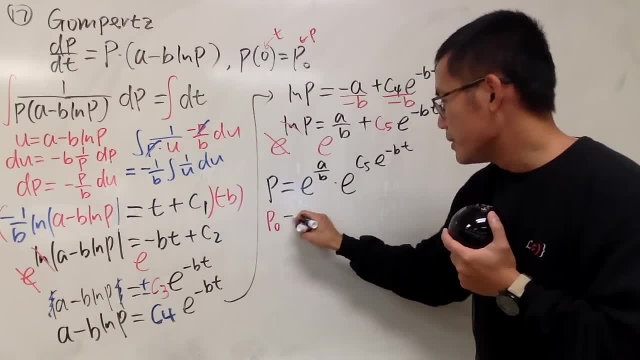 course, let's draw things in. This is p0, p0, if you would like, if equal to e, to let's do this in glue, so you guys will know that I'm doing the…. no, I'm doing this in glue, so I'm not trying to get into. 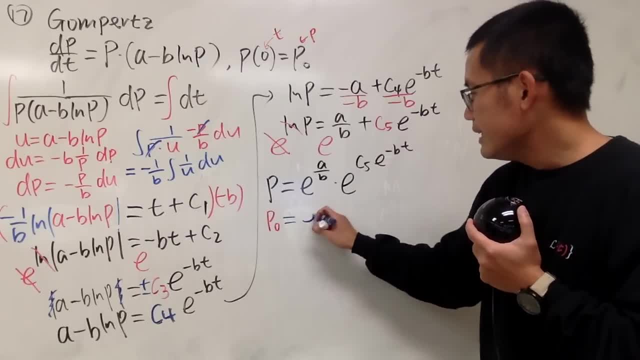 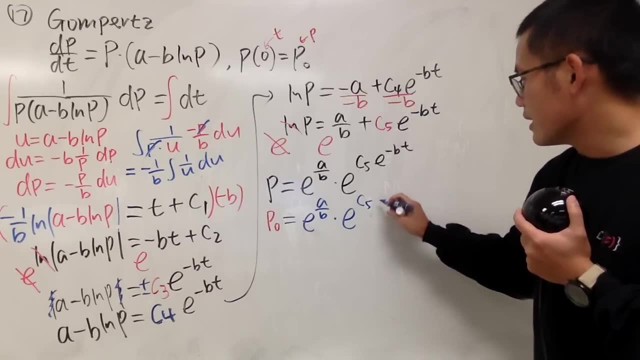 initial condition. here. this is equal to e to the a over b times e to the c5, well, let's just c5,, why not? and then c5 times e to the negative b times 0, right, so it's like. 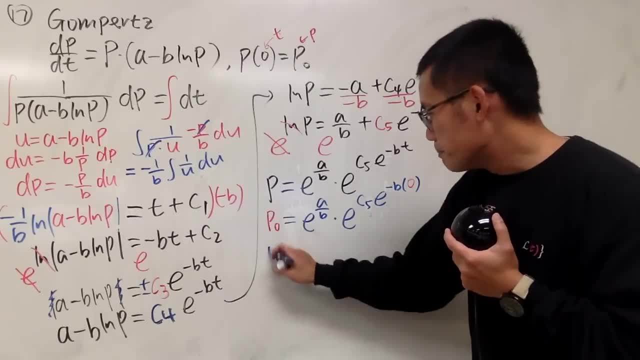 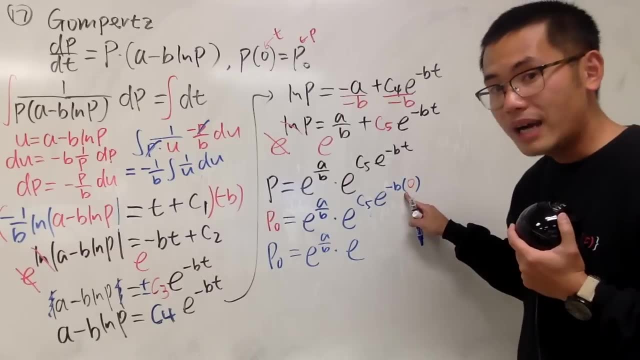 this. I know it's crazy, but that's just how it is. and then this is: p0 equals e to the a over b times e, and this right here is 0, this right here is 1, so we just have c5 like that, yeah. 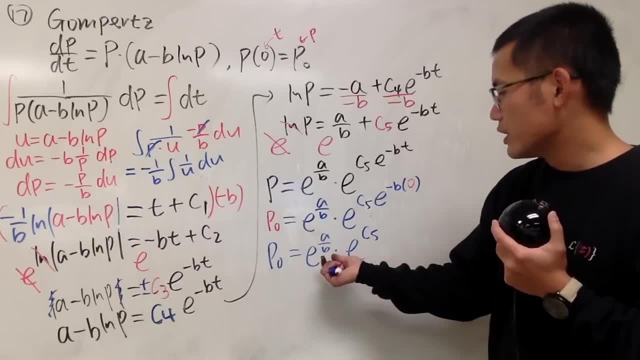 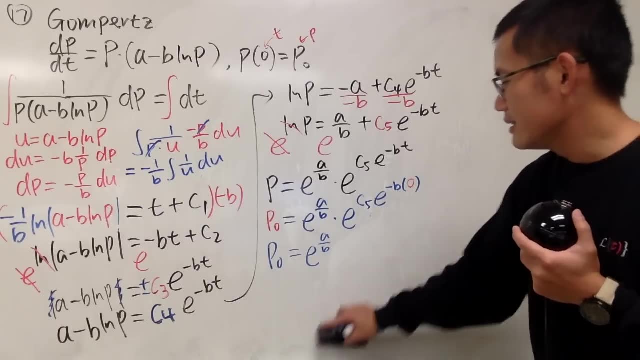 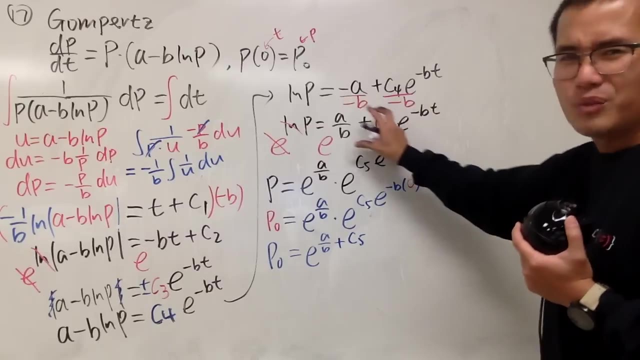 now to isolate c5, all we can do is just let's see: okay, I'm going to just combine them, because this and that they're both with e, so I'll just say this is plus c5, same thing. it was like this. now, I think it was easier if you do it this way. 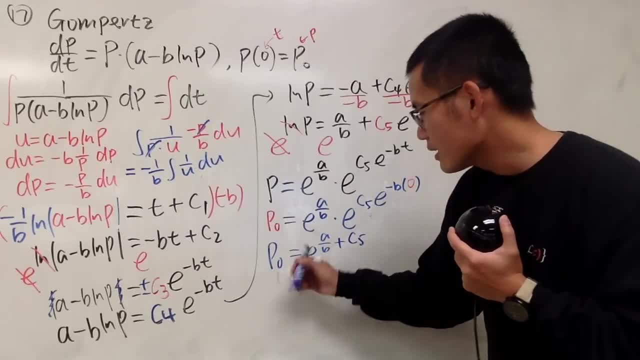 but anyway, this is what we have now, and then of course, you can take a natural log, so I will show you guys a natural log here, natural log here. so be really careful. so this and that cancel out completely. so we have. 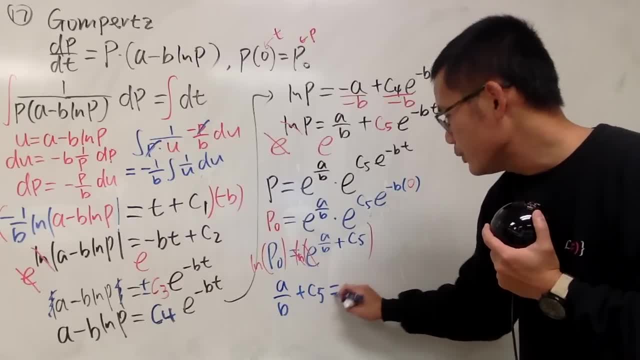 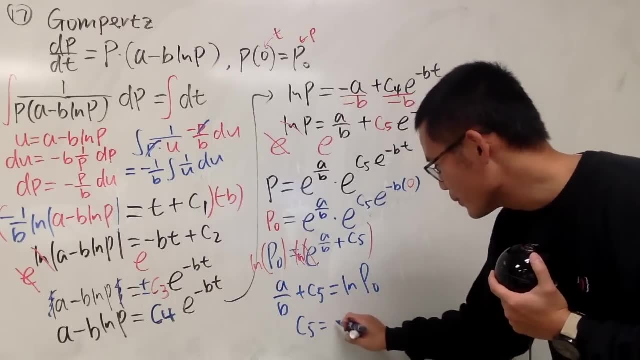 a over b plus c5, that's equal to ln of p0, and of course we can just minus the a over p. on both sides, c5 is equal to negative a over b plus ln p. actually, let me write it down like this: 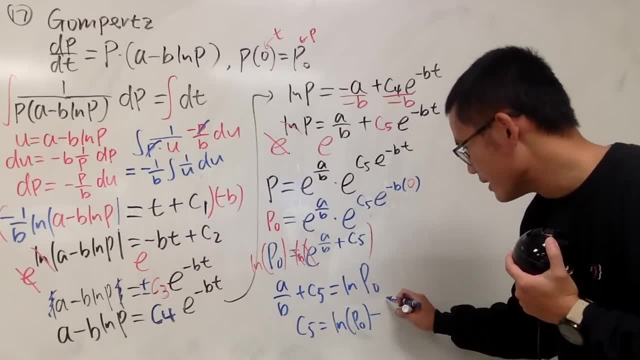 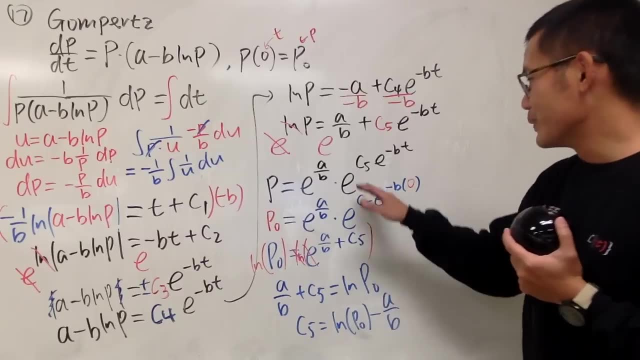 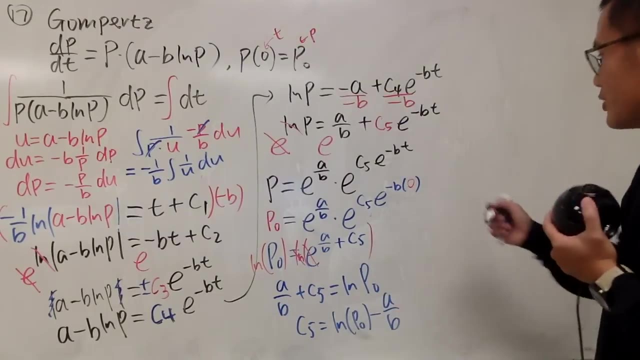 ln p0 minus a over b. all right for this one. I'm going to actually plug it into the c5 here, so it gets the final form right inside cell. the final form, all right. Dragon-Bosy reference. 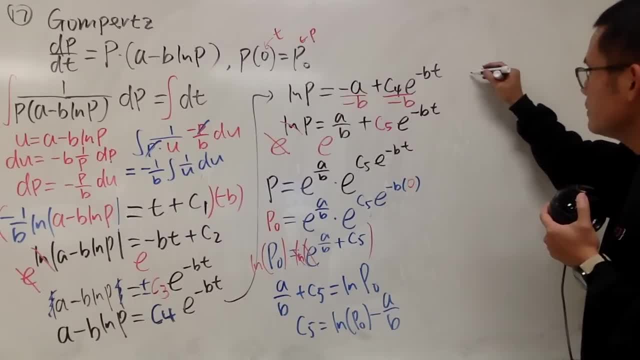 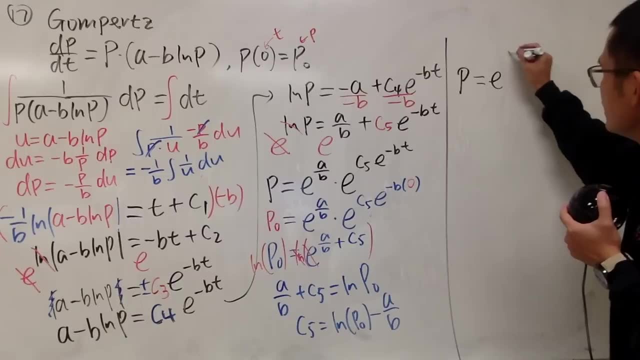 so finally, let me see I should be able to write this down. so finally, p. so I'll just draw a line like this: p equals we have e to the a over b power and we have times e, and then this c5 is: 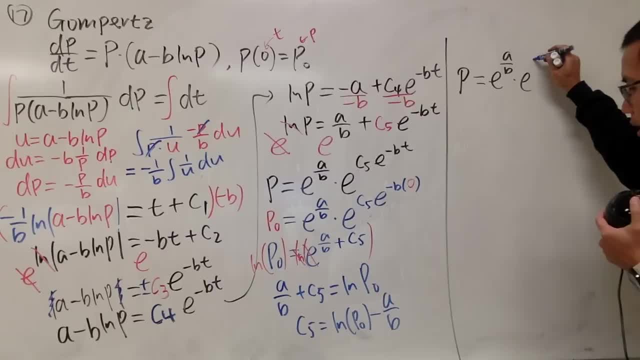 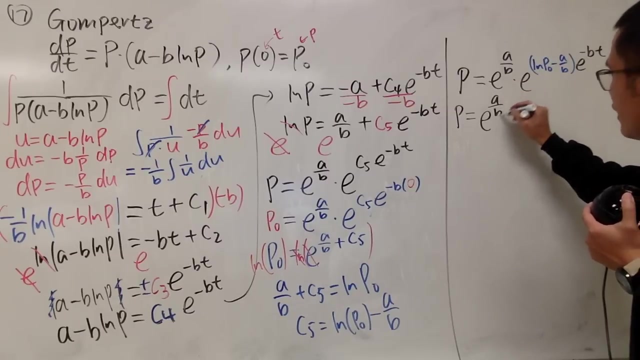 which is pretty crazy. we have ln, p0, and yeah, and then minus a over b, this is the c5,. right, this is the c5, and then we multiply by e to the negative bt, like this: okay, now, this is what I will do: p equals e to the a over b, and I will distribute. 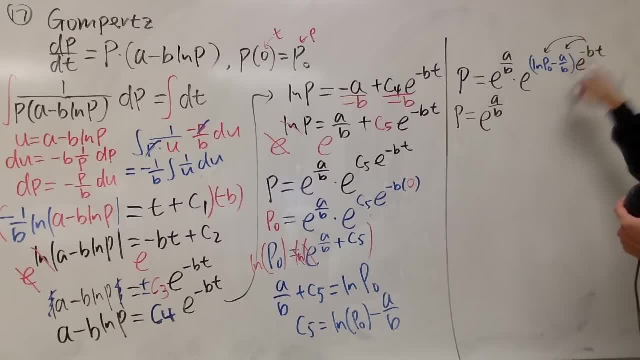 this guy in here and here, so now, no, no hard building, okay, so I will put this down first this times: all right, I will do this this times that, which is e, and then we have e to the negative, b over t, so e to the bt times, ln, p0, okay, so this times that. 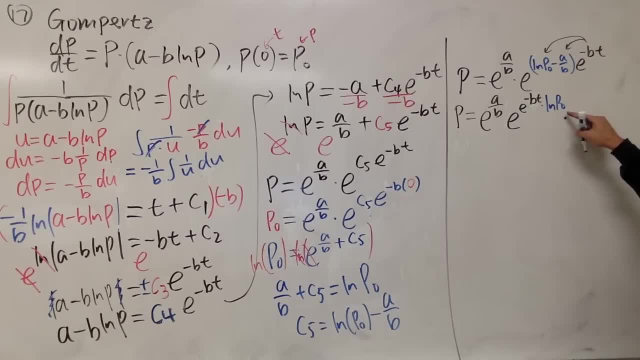 and then multiply by yeah, because this is just negative. so let's multiply by e and then I will just do this times that which is negative, a over b, and then e to the negative, b over t power. can we see? 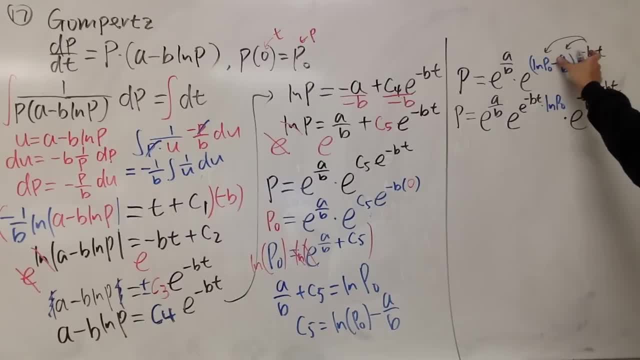 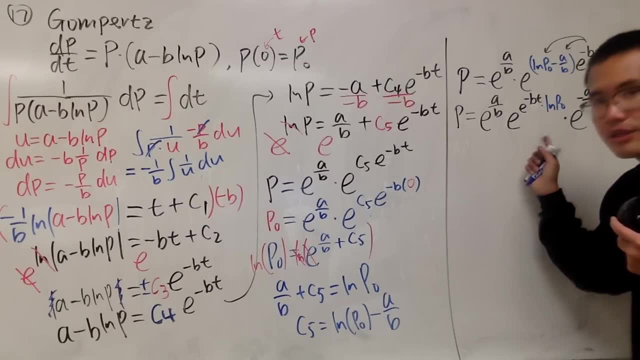 Yeah. so again, this times, this is negative power, but just break it down into, because if you do, this times that you just combine the powers. so that's what we have Now. this is the part that you can simplify, because when you have to simplify, 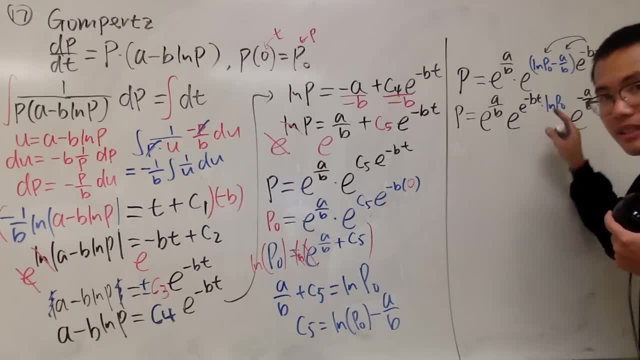 and this is the dance chart right. this is the dance chart right. this is the dance chart that we have time. what temperature it should be. at 30°, when you have the product of two things, you can do the following: So this is: p equals e to the a. 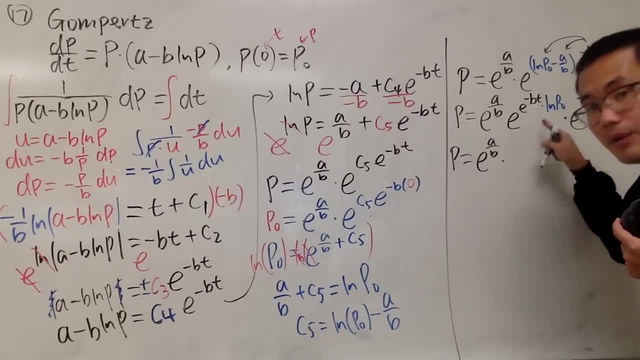 over b power times. let's do this as the following: e goes first, and then you raise to the ln p0 like this, And then you raise that to the e negative bt power. And again why we can do that? Because when you have a power to a power, you just multiply the powers. you get that. 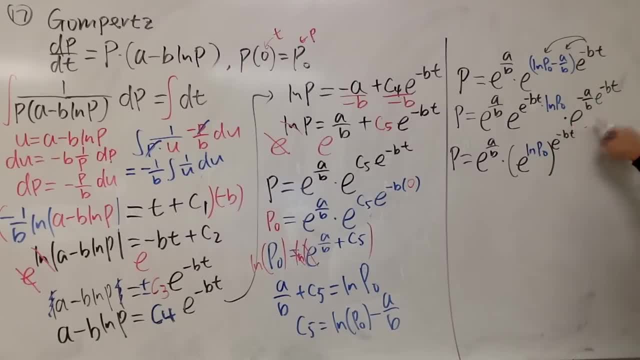 and we're just doing this backwards. And then here you have times e: negative a over b, e to the negative bt power. Okay, good, Now the best thing that we can do is that e and cancel. So, yes, that's right. Okay. so finally, this is the answer. already I promise I won't. 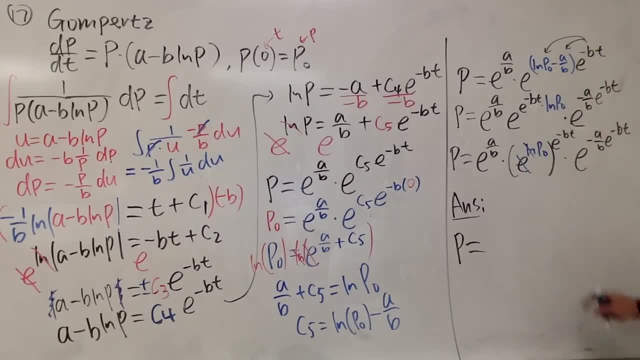 simplify it anymore. Here we have p, that's equal to and, if you would like, you can put this down first. So p 0, right, this is just p 0. Take this and then raise that to the e, to the negative bt power. 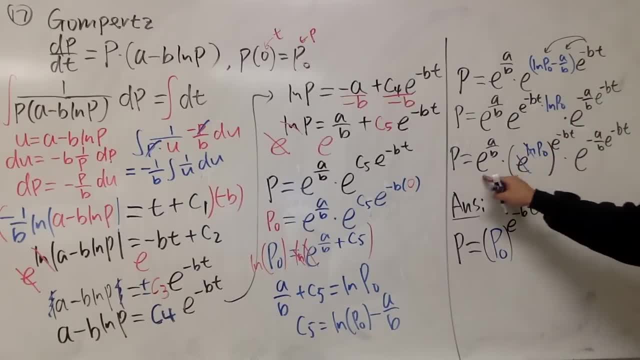 I'm not kidding, This is just that part, And then this, and that I can just add the exponents. Well, you add a negative, so it's actually multiplied by e, And then this is a over b minus a over b. 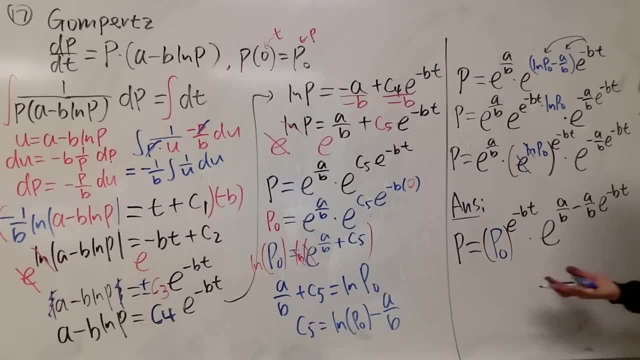 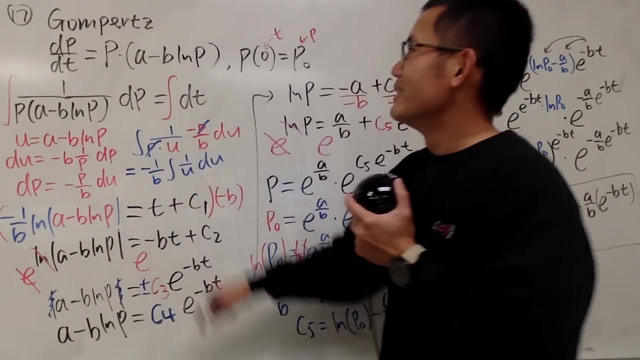 And then you have e to the negative bt power, like this, And if you would like, you can factor out a over b, but seriously don't make it, Don't make me do that anymore. So this, right here is it. Yeah, So let me just make it clear: It's like this, And then this is the huge power here, And then this is like the power, like that. So uh, uh. 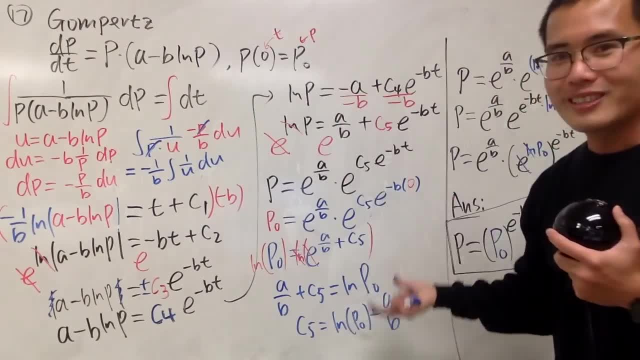 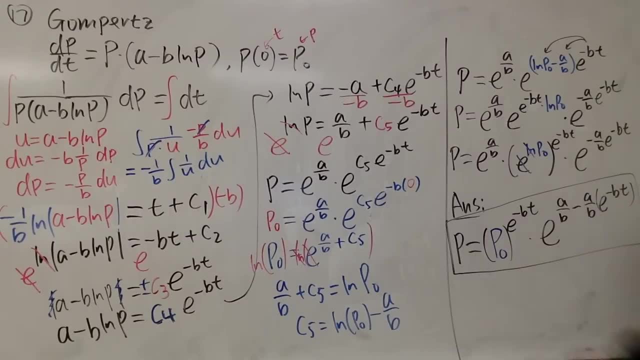 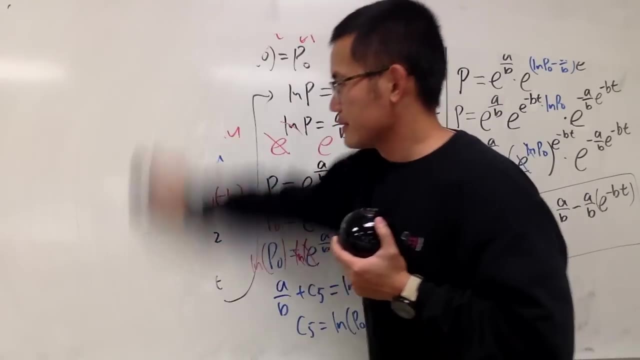 compassed differential equation. It's like this: This is so colorful. How many letters have we used right here? So just have a look right here. So pretty cool, Okay, Okay, Okay, Okay, Okay, okay. Can I finish this? It's in like 4 hours, I don't know. 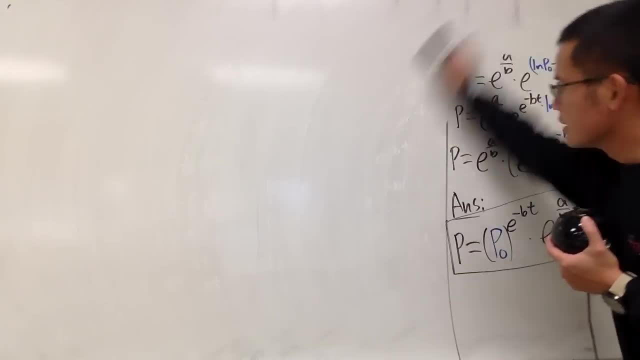 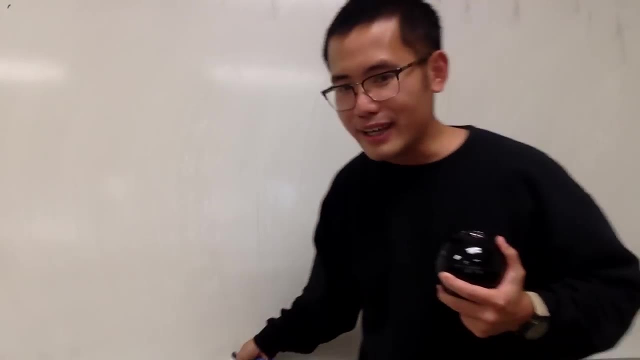 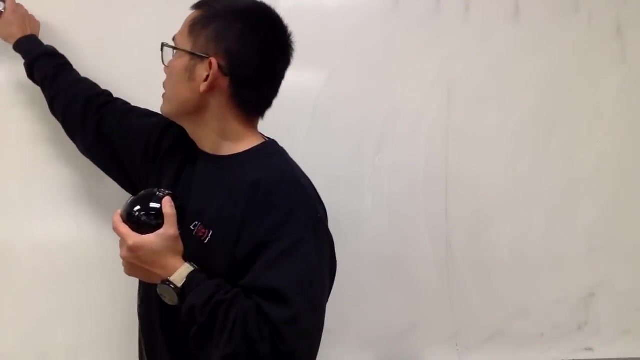 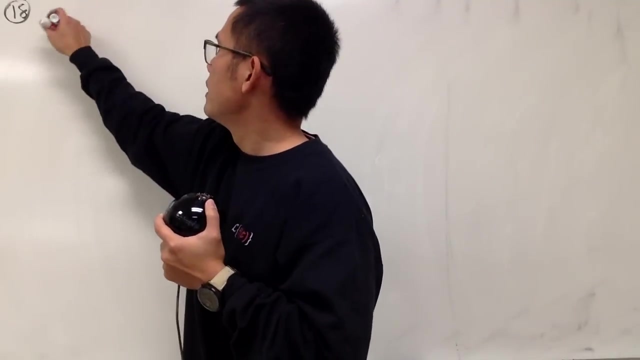 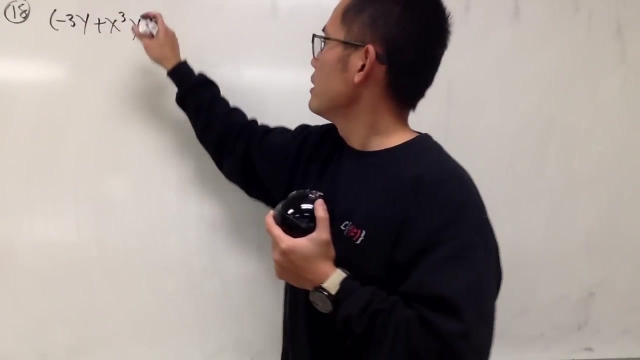 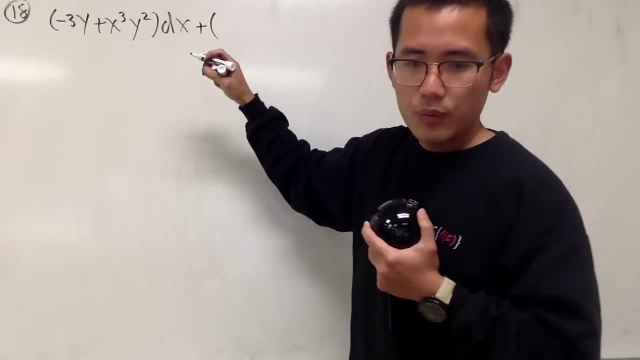 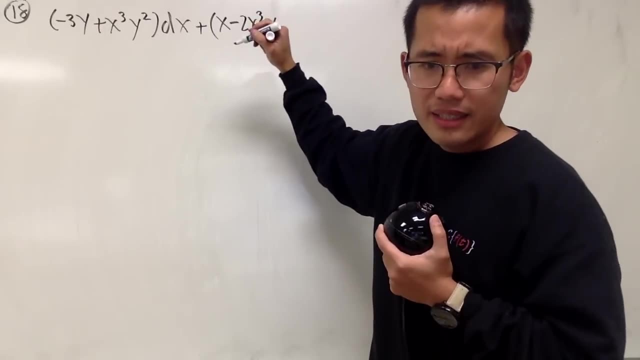 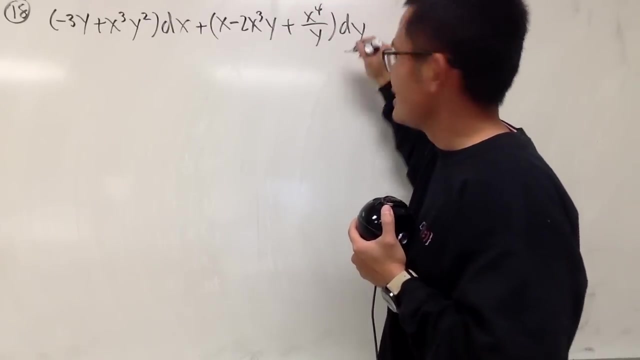 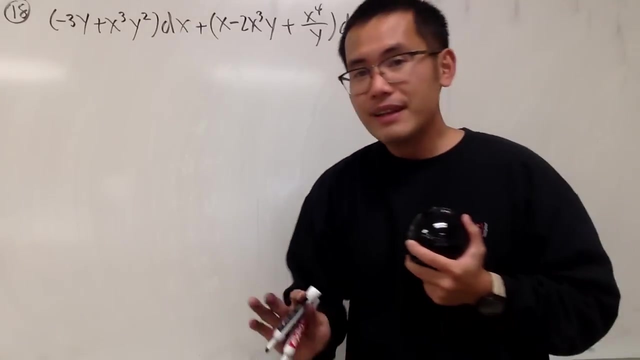 and then plus parentheses and we have x minus 2x cubed y and then plus x to the 4 over y. oh my god, dy is equal to 0, so yeah Again. usually when somebody gives you this, like try to go maybe for exact. 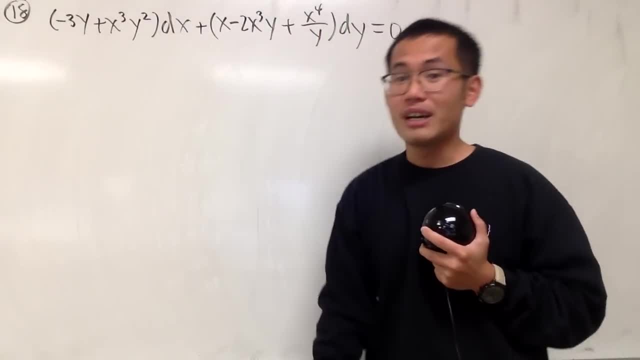 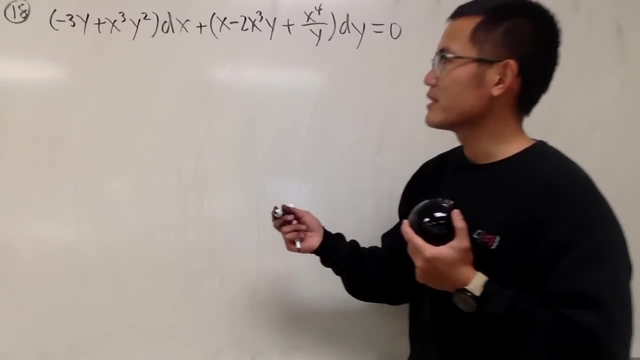 especially. you see, the degree here is 1, degree here is 5, so not homogeneous. And again, let's see exact Or not, Let's go ahead and check it out. So go ahead and do the derivative right here. with respect to y. 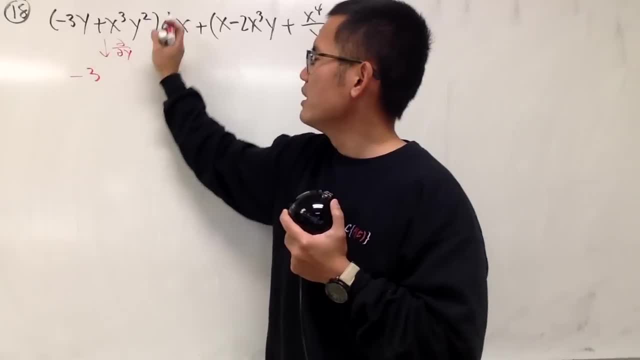 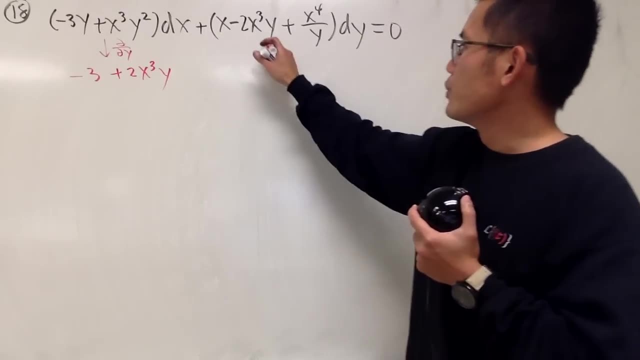 so do partial with respect to y, and in that case we get negative 3, and then we get plus 2x cubed and then y. Okay, But if we do the derivative right here with respect to x, this is 1,. this is minus 6x. 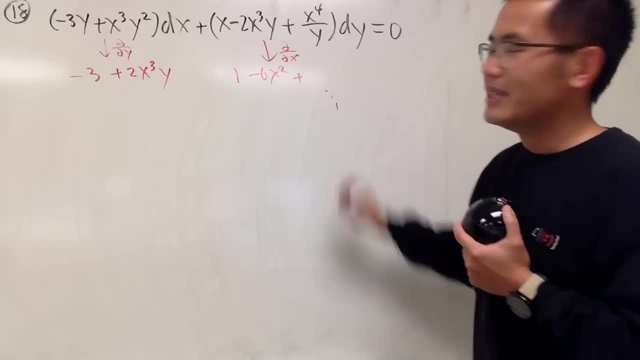 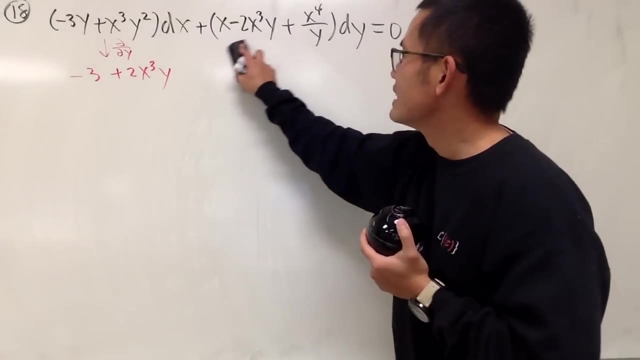 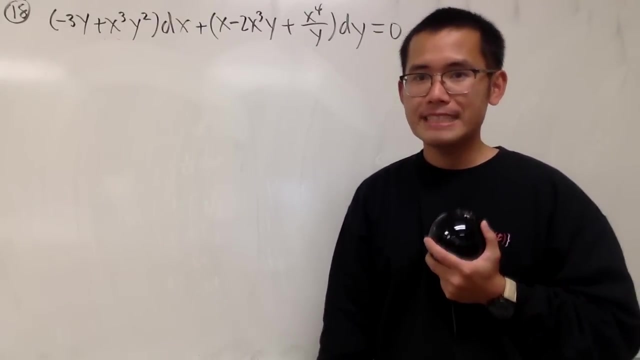 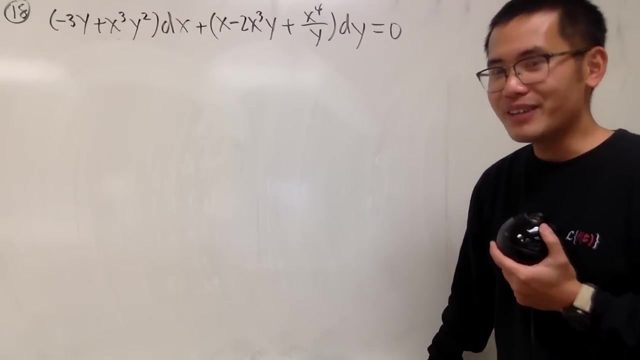 so no, no, it's just a no. It's just a no, So not exact. Hmm, what should we do? You can pause the video and give this a try. all right, This is just what you should be doing, so don't just say. 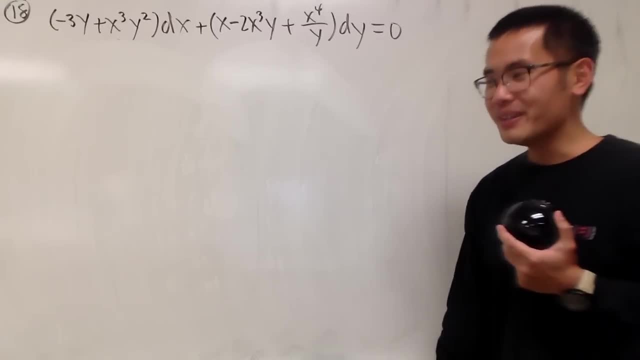 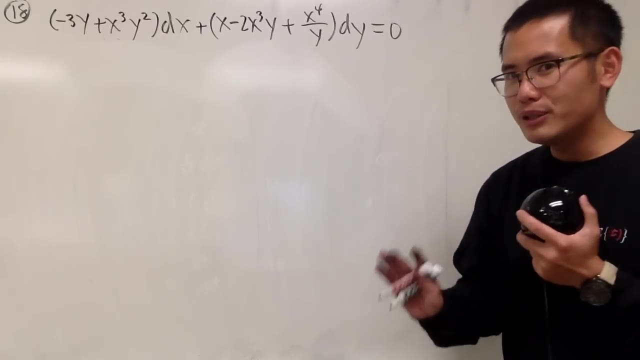 look at the solution, even though this is like a movie, like a marathon, math marathon or that differential equation marathon. but give this a try, So we'll try to do it. Okay, So we'll try to do some special integrating factor. 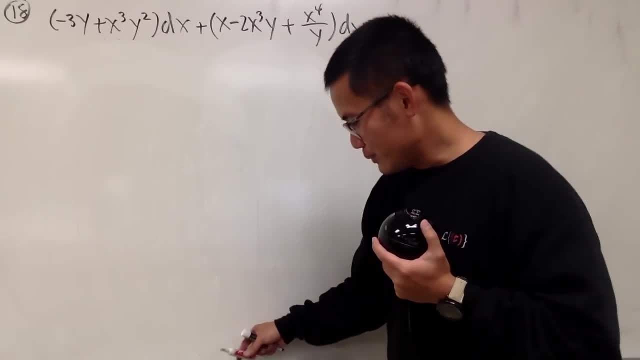 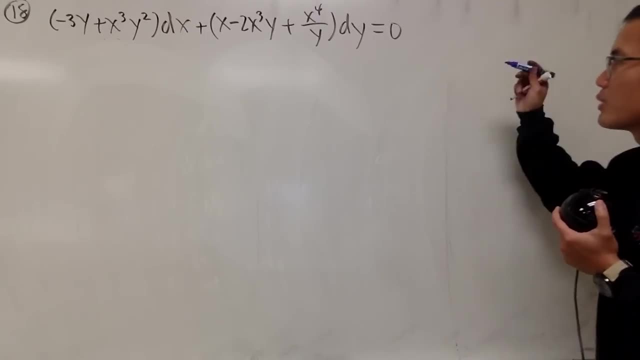 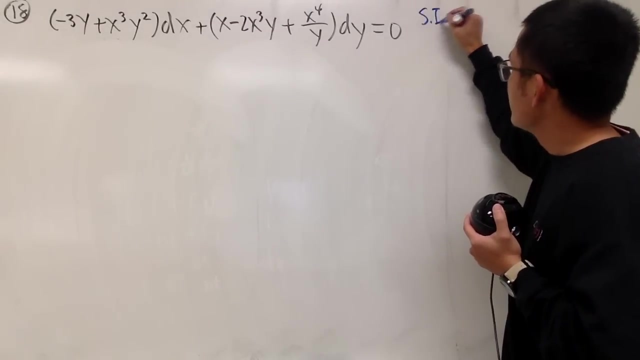 and the answer to that is yes, we should. Okay, So, just like earlier, I will try to squeeze in all the work on the right-hand side, on the right side here. So special integrating factor, let me just put on S I F right. 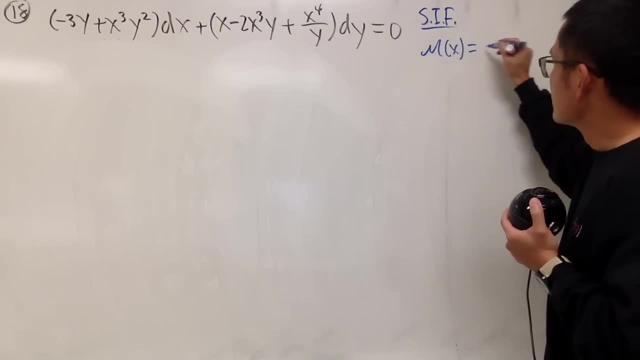 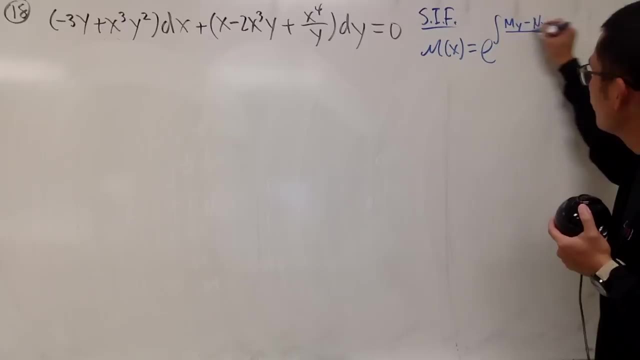 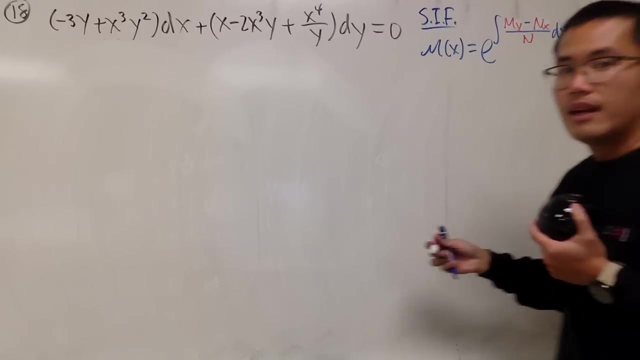 And the first one is: we have mu of x, That's integral, that's e to the integral of m sub y, minus n sub x, over nx, I mean just over n. Let me just put my columns: m sub y, m sub x, and then over n dx. 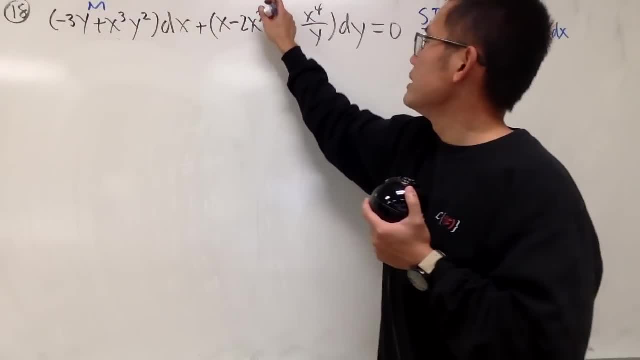 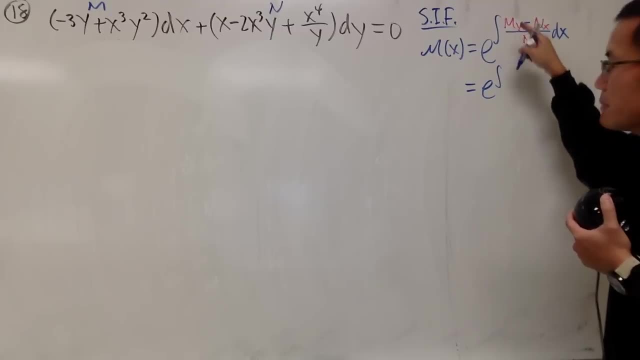 And right here here is the m, then this, right here is the n. Like usually that's the notation. Let's see if this works out or not. e, integral m sub y. so go ahead and differentiate. I need more space for sure. 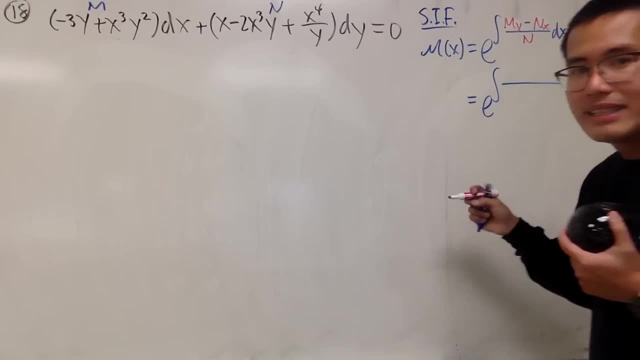 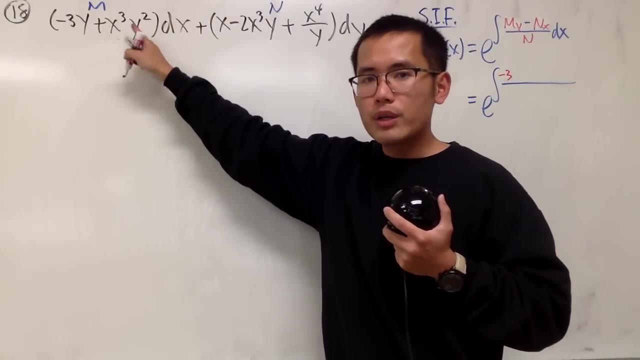 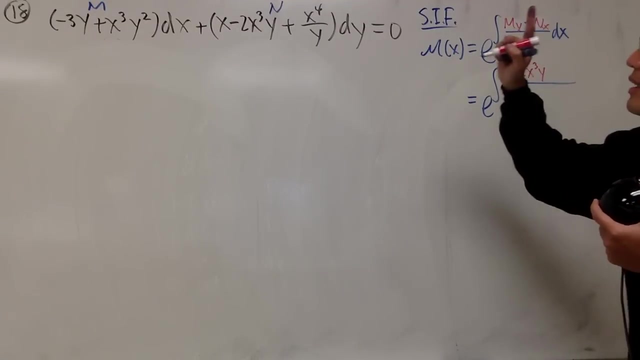 e integral m sub y is negative 3, and then differentiate this with respect to y, we get 2 x cubed y- Good, And then n sub x. so that's a minus. can we see? Oh, yeah, I think so. 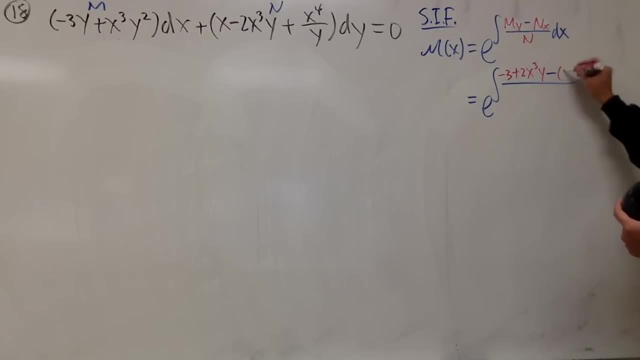 So right here I get 1, but this is a minus, so okay, put parentheses there. Minus 1, minus derivative of this is 6 x squared y. Good, And then lastly differentiate this so we get plus 4 x cubed over y. 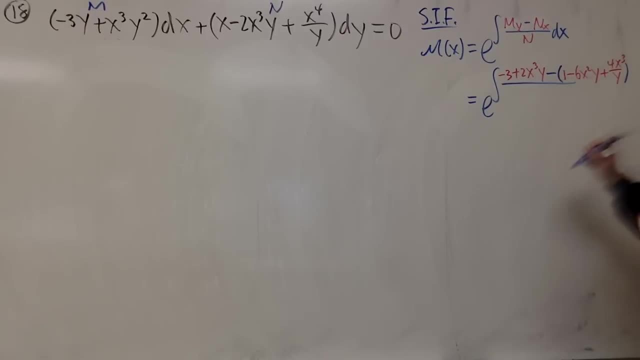 Yeah, So that's this part. Oh good, we still can see this as dx, hopefully. And then the n is now: oh my god. So we have x minus 2, x cubed y plus x 4 over y. 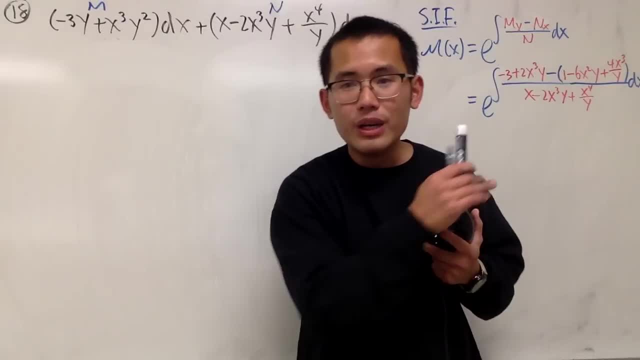 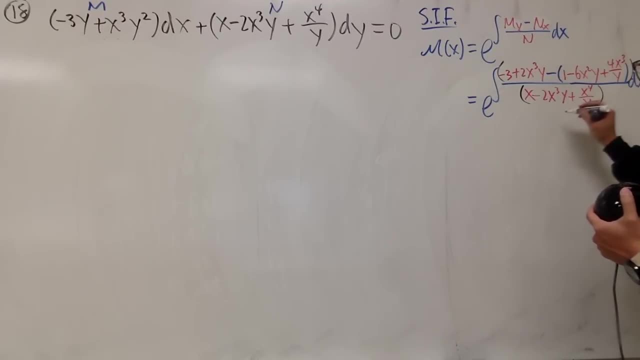 Okay, here's the deal. As we can see right there, we have a complex fraction, So let's go ahead and clean things up, And the way that we'll do it is multiply the top and bottom by x, And I mean y. let's see what will happen, right. 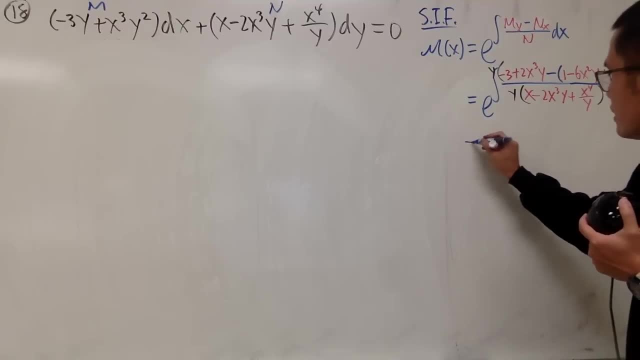 Let's hope for the best and all that stuff. So here is e integral, And then this is negative 3y, And then plus 2 x cubed, And then y to the second power- Yeah, Good. And then y minus y times. this is minus y. 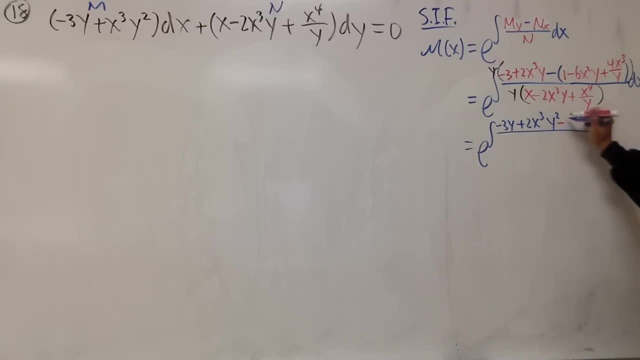 So I'll change the sign. So don't forget. Don't forget that Minus y And then minus minus, so it becomes plus. Also, you should do it the other way, Because originally it was red, And then multiply by this. 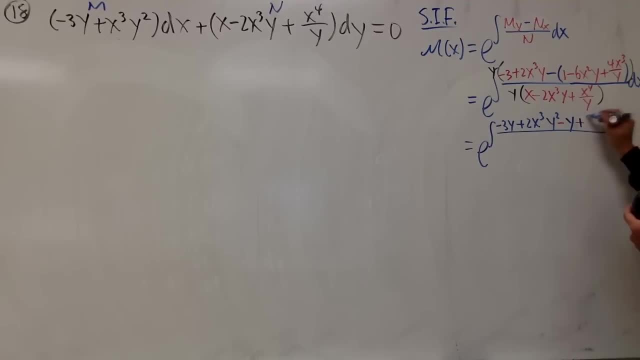 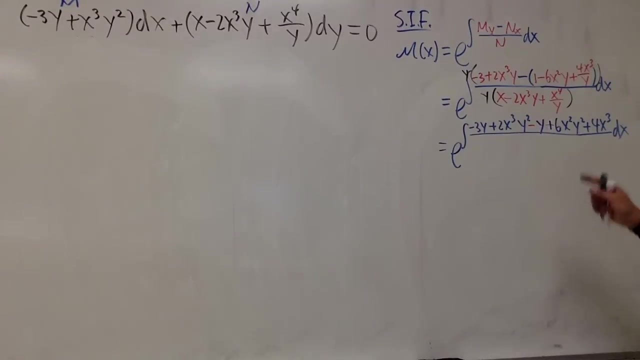 Yeah, Anyway, y times, that is 6 x squared, y squared, And that's the plus 4 x cubed dx. All right, So I'll put this back later on. Actually, I'll just leave it like this for now. 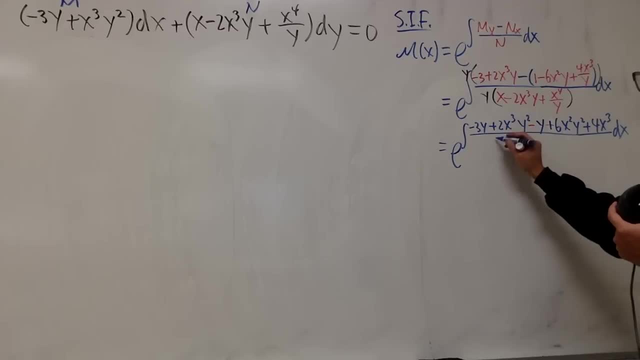 So this is what we have, And then multiply all this by y, So we have xy minus 2, x cubed, y squared, And then plus x to the fourth. Okay, Okay. So let's see, Don't panic. 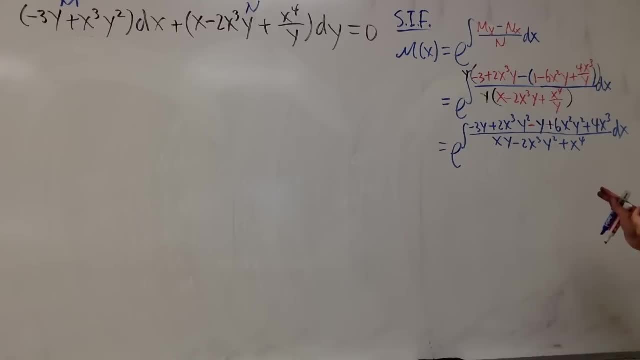 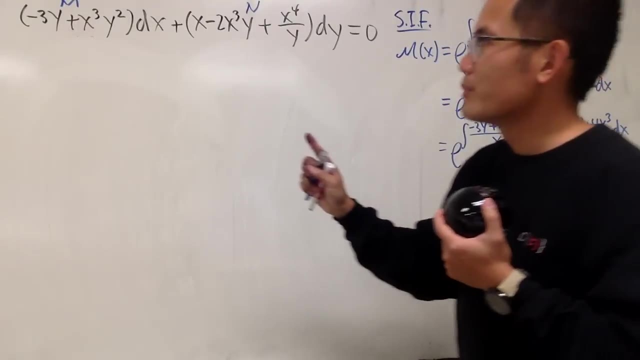 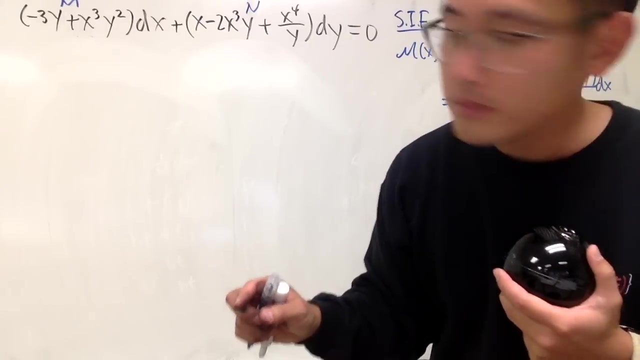 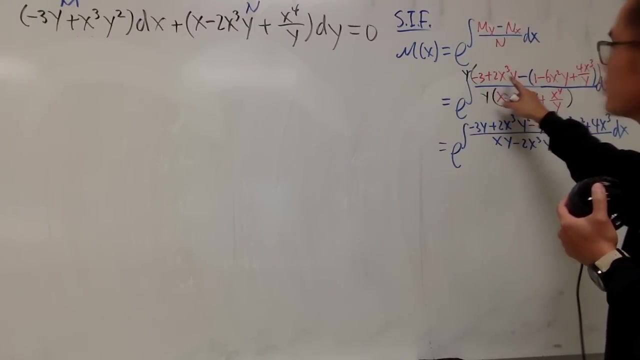 Don't panic, I'll really make sure that I don't have any careless mistakes. Square Okay, Then y is this, And then Square blah, dah, dah, dah, dah, dah Go down the same thing. 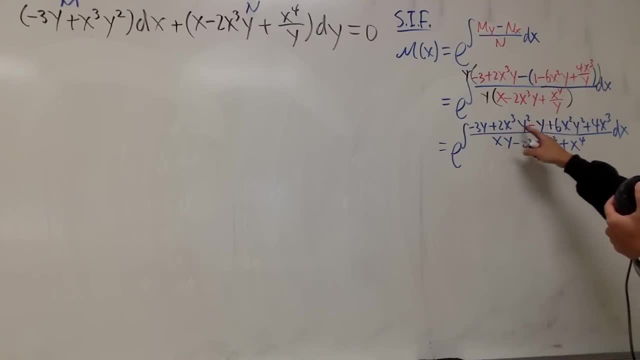 Okay, And then multiply by y- Good, Multiply by y- Good, But I cannot combine any terms on the top. What the heck? Oh, hey, I can. I can get rid of this and that. Ah, that's all. 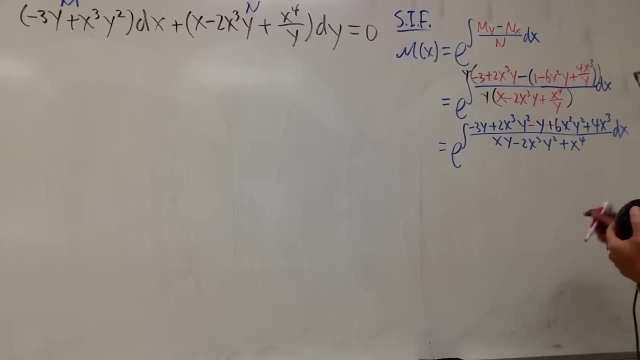 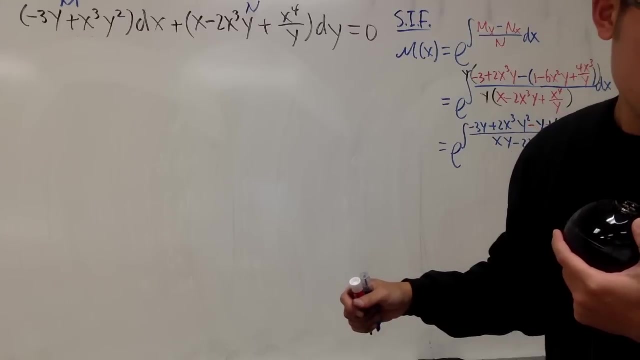 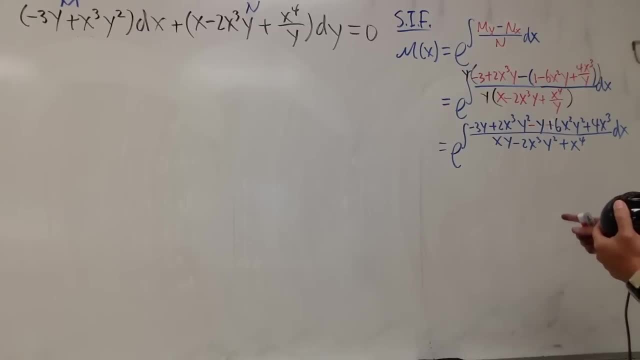 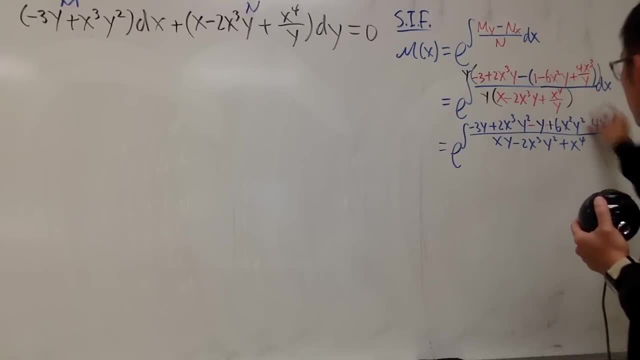 Oh, by the way, this is negative. Negative, so it becomes minus. Okay, That's, that's good. I can count a little mistake, but it doesn't really help. That's good. Okay, That's good Okay. 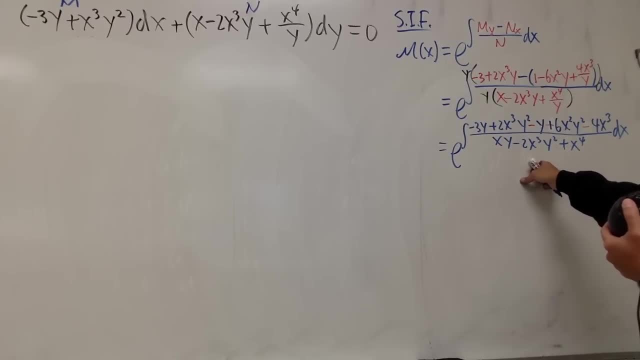 Okay, Okay, Okay, Okay. m sub y, x, y, y x x. I feel like I had to factor things out in order to cancel things out, but I could be wrong. So if I factor out, oh man, this is bizarre. 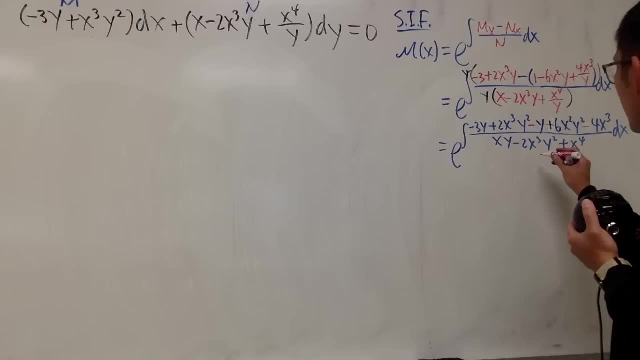 If I factor out, if I factor out the x, what will happen? If I factor out the x on the bottom, this is x, and then I get y minus 2x squared, y squared plus x cubed. That's the bottom of this. 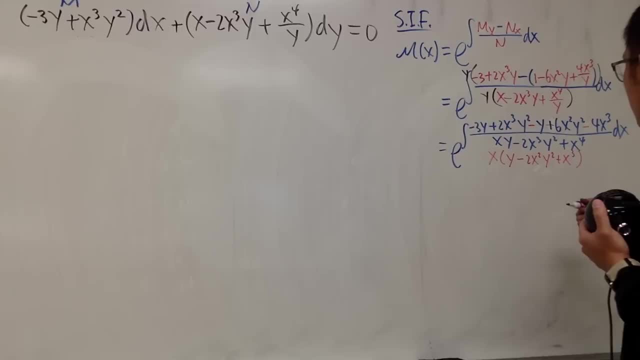 But the top is is so messy. I thought it would be a nice simplification when I come up with this equation: So e integral, and then this, and that I can do a negative. So what? This and that is negative 4y, but nothing too crazy. 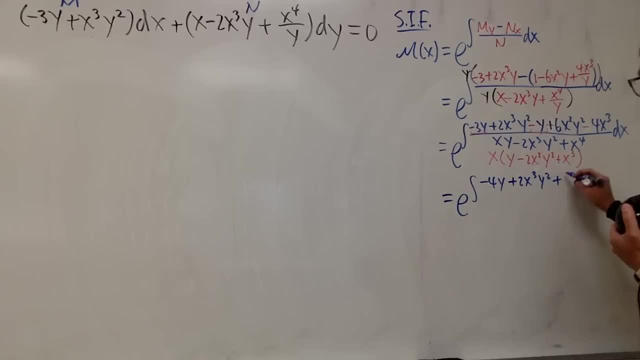 Plus 2x cubed, y squared, and then plus 6x squared, y squared, minus 4x cubed. This is kind of suspicious. Hey, this part and that part can be. Let me try this. Okay, let me try this. 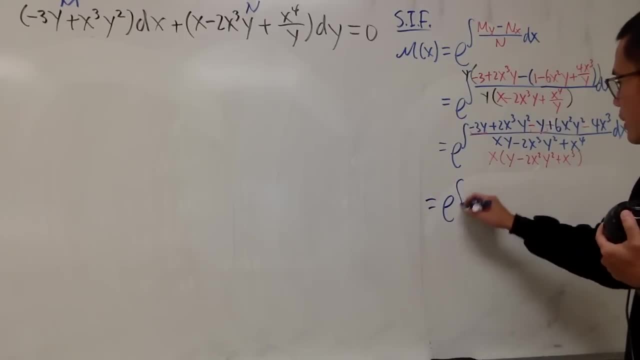 It might not work, but I will try it anyway. So here is e integral, and then this, and that is negative 4y. I seriously don't think that this would be a negative 4y, but I really don't think. 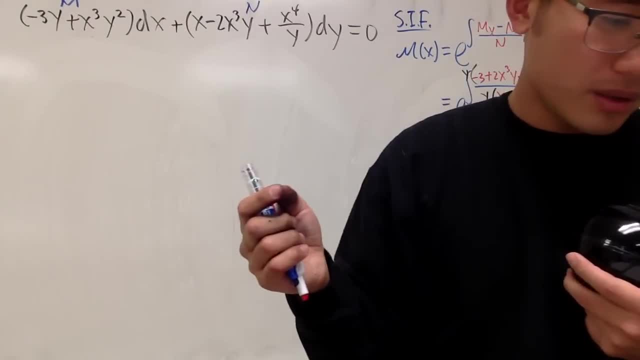 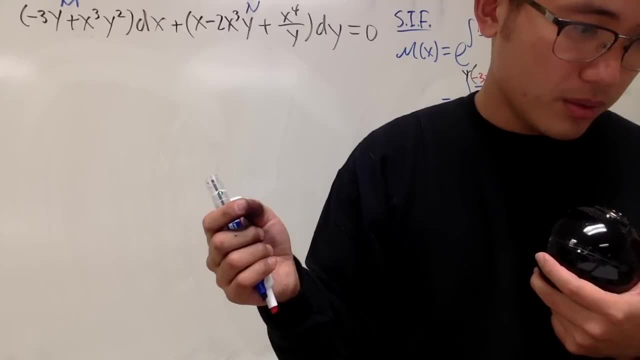 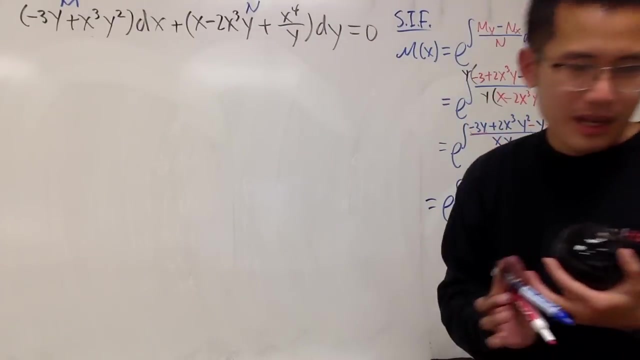 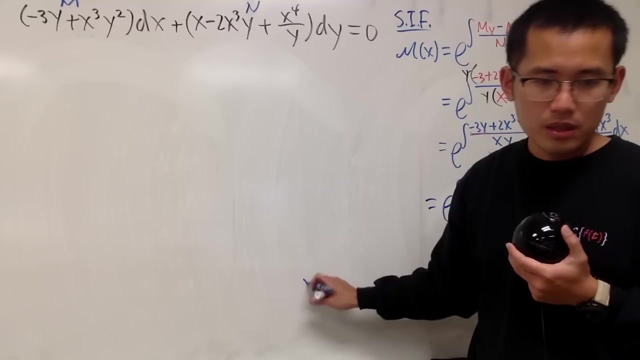 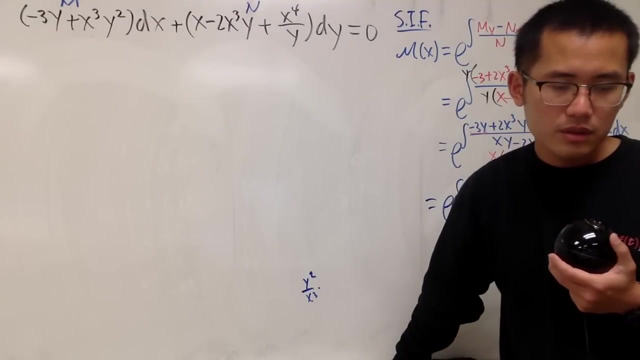 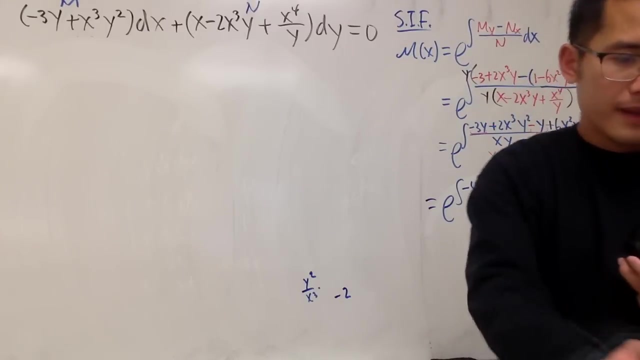 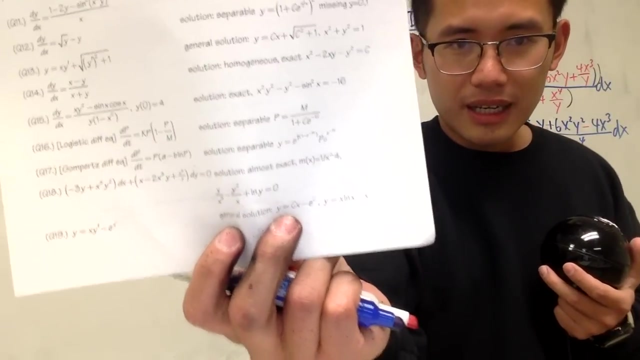 Okay, I have the answer. Let's see Negative 4x. Okay, I am going to do this before I continue. So let's see, this should have been negative 2, you see negative 2.. Okay, so this is the answer that I have, but I am thinking, maybe when I type out the question. 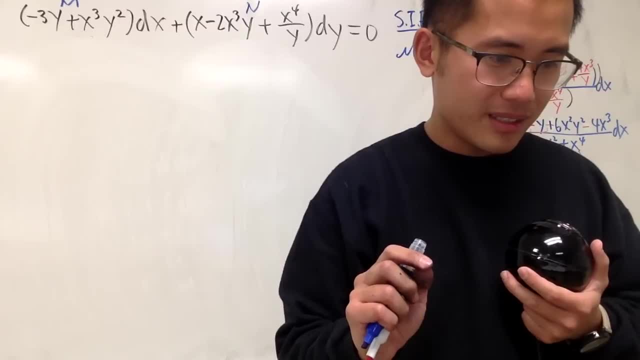 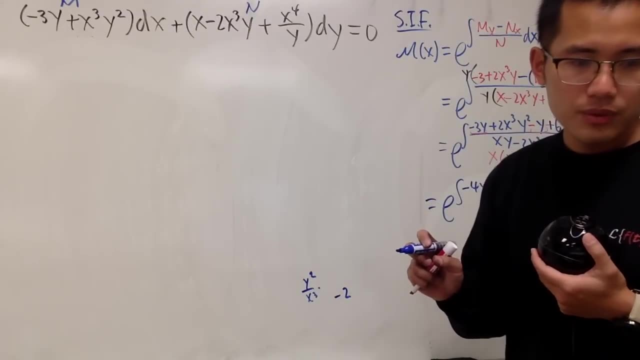 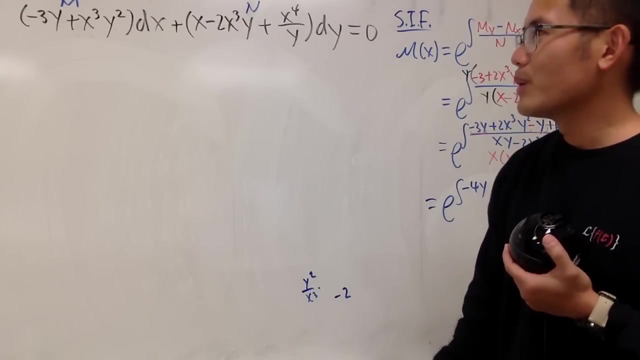 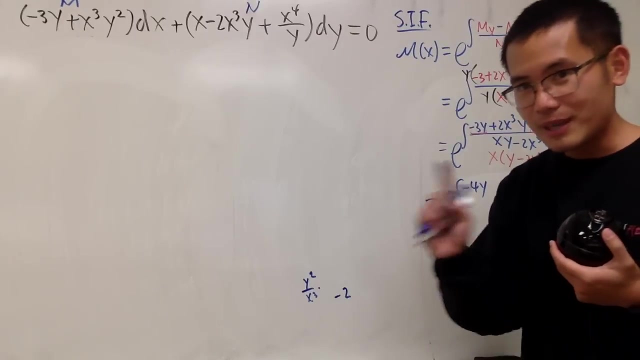 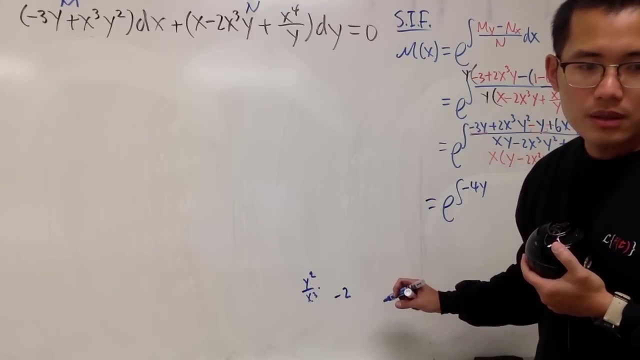 I make a calculation mistake. Okay, so I think I will do the following for you guys, for number 18.. Because unless I am just- let me just- okay, 10 more seconds. Well, actually, no, I need to find that, I will just do it. 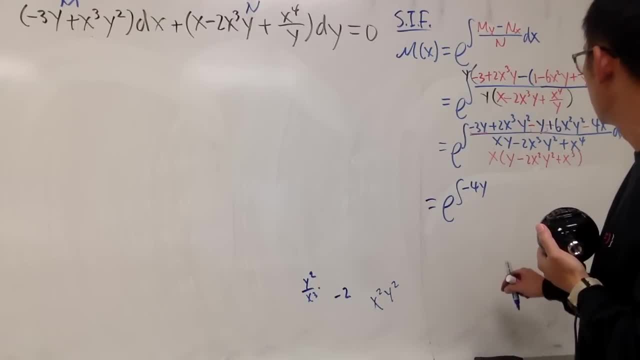 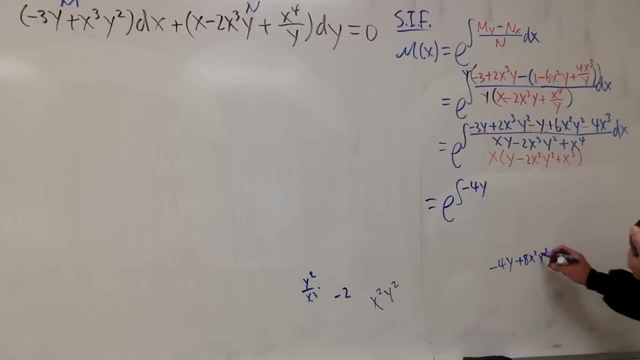 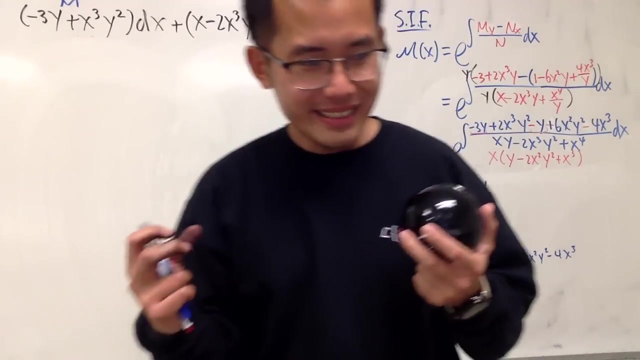 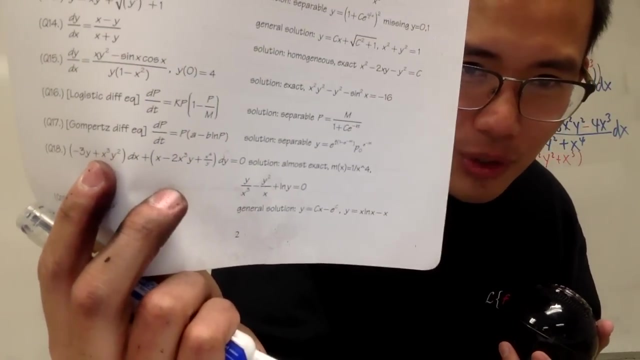 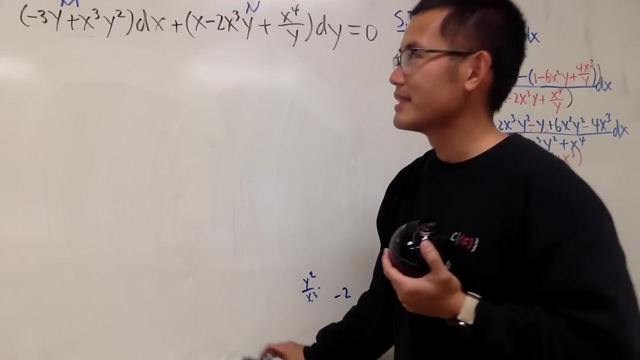 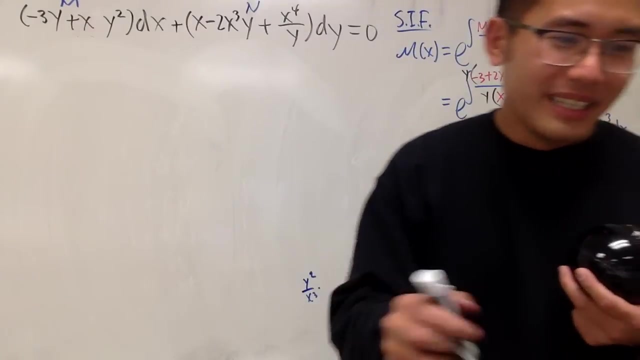 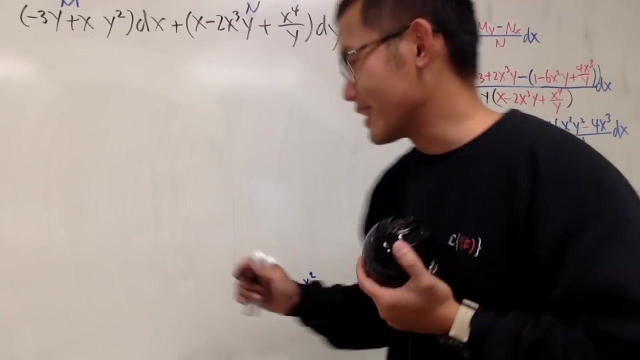 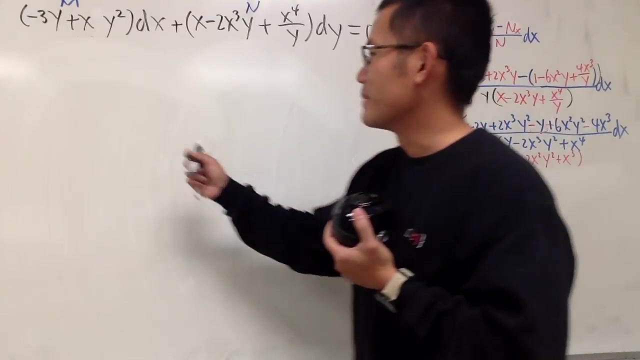 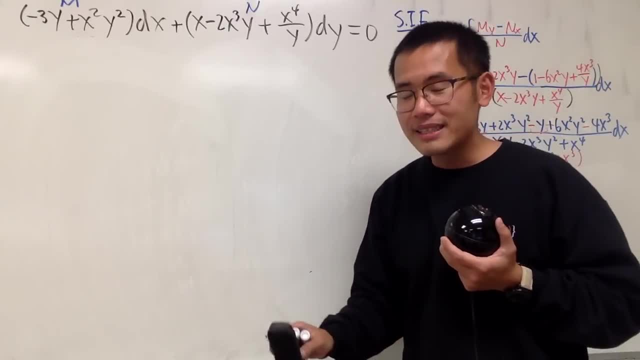 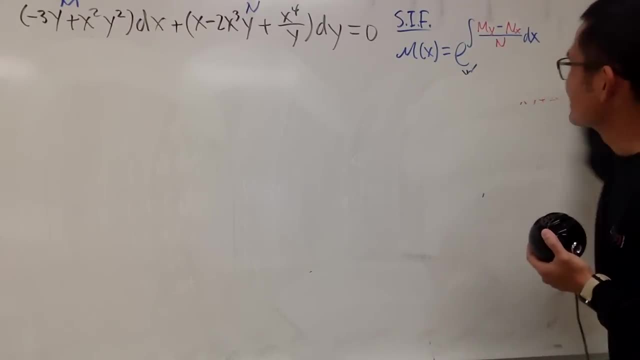 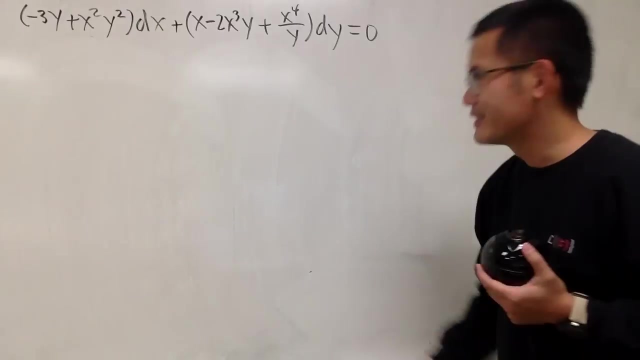 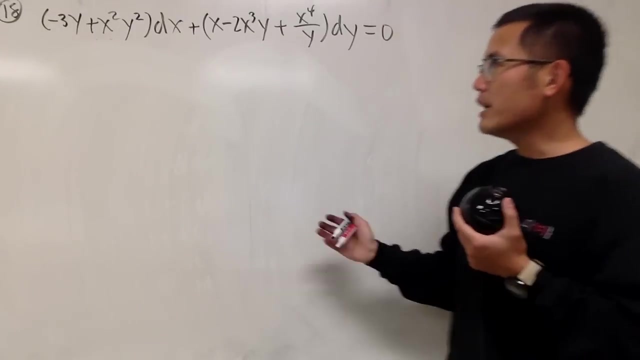 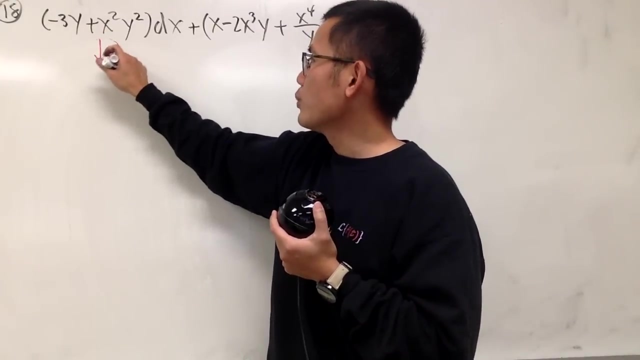 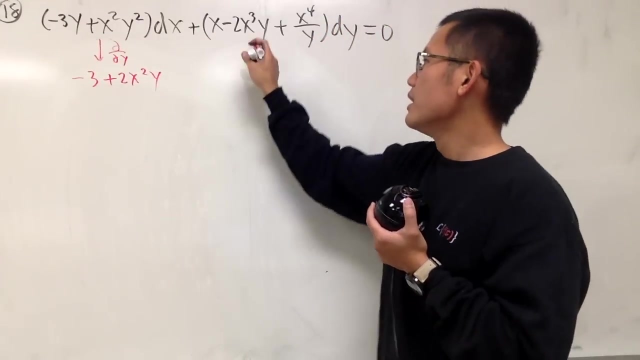 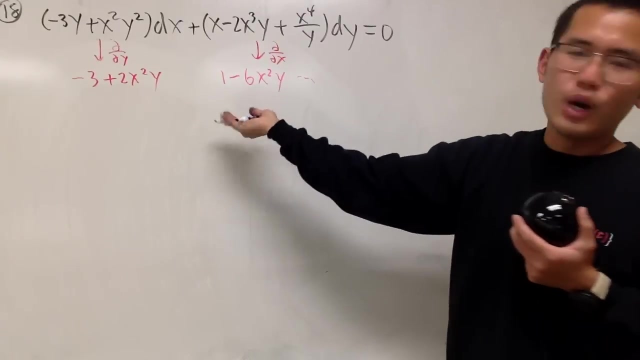 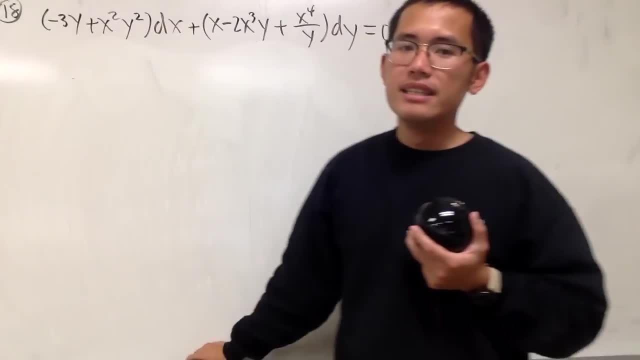 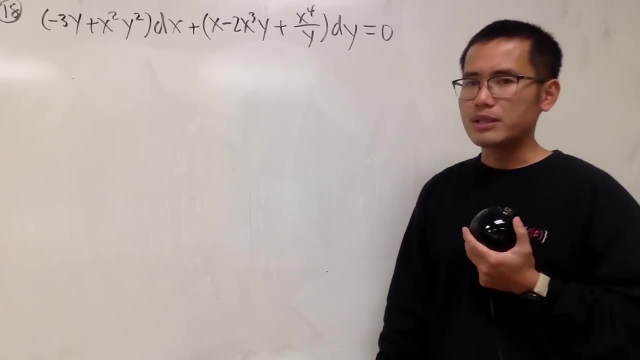 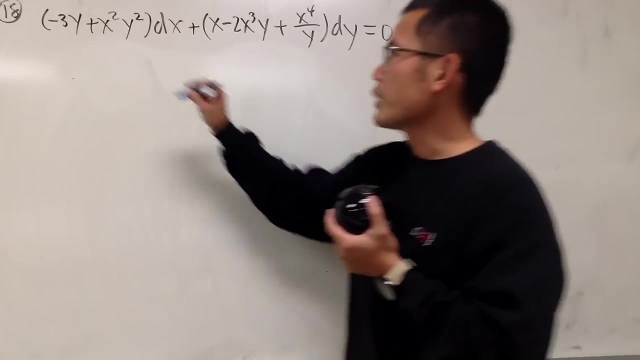 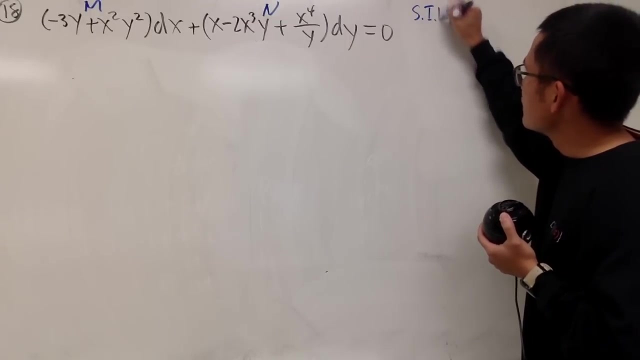 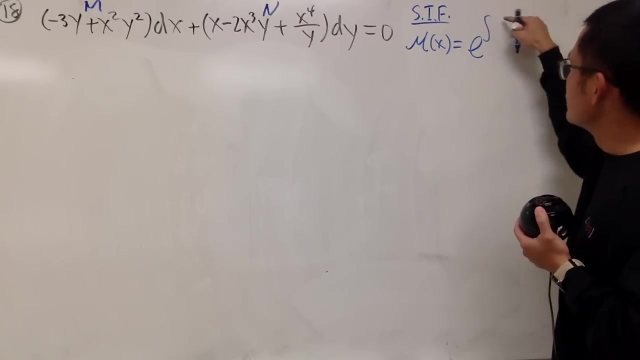 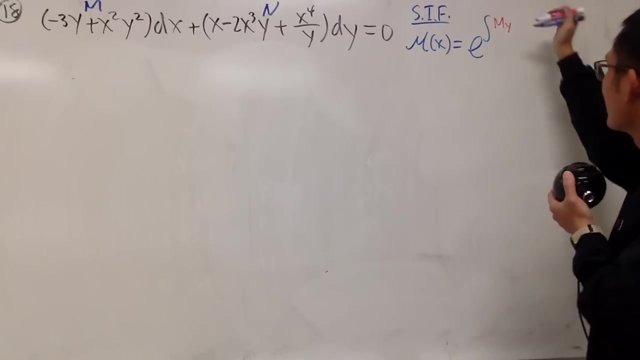 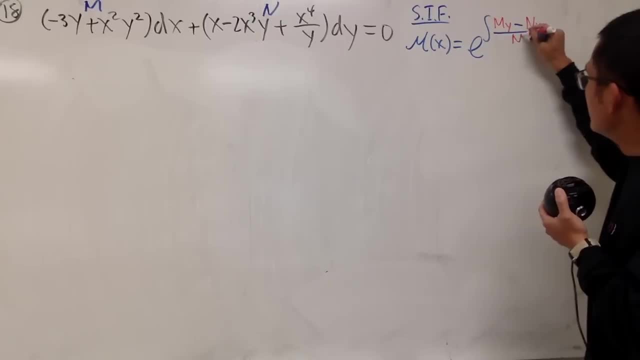 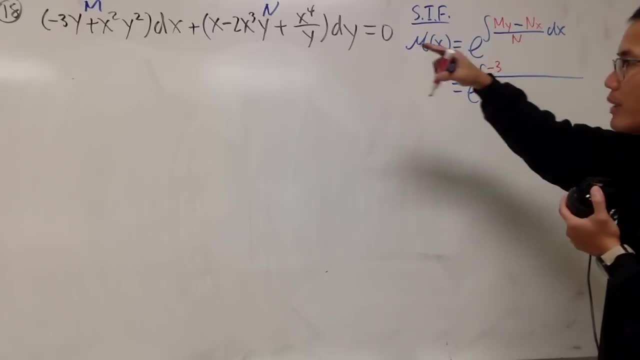 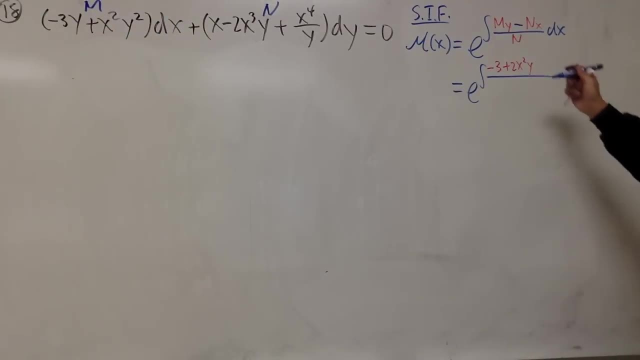 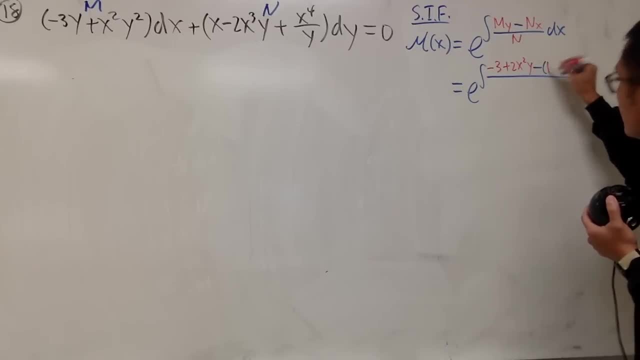 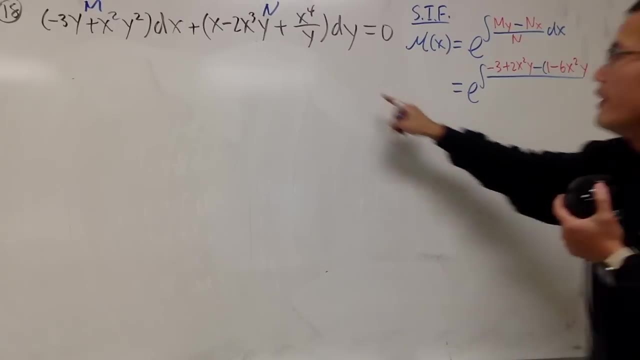 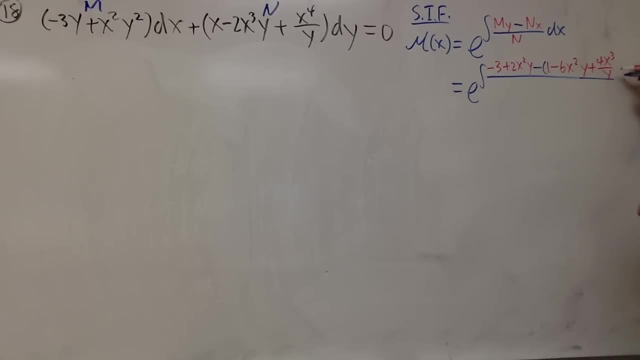 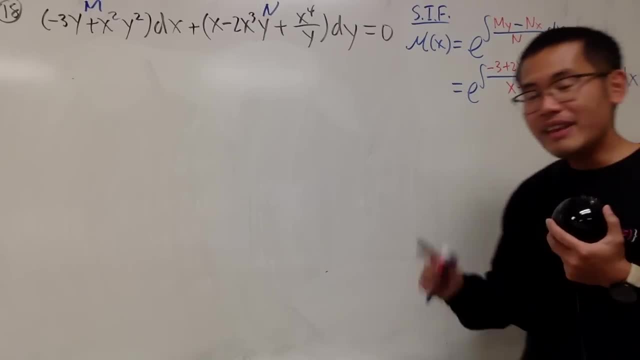 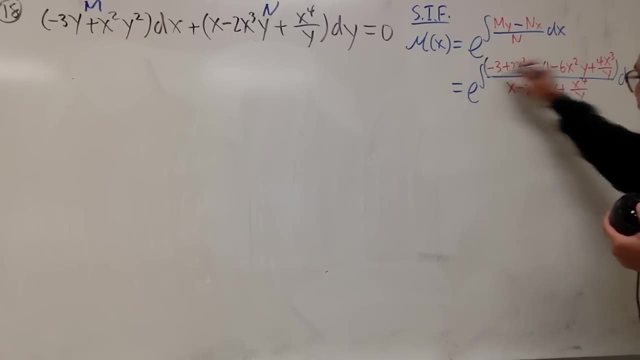 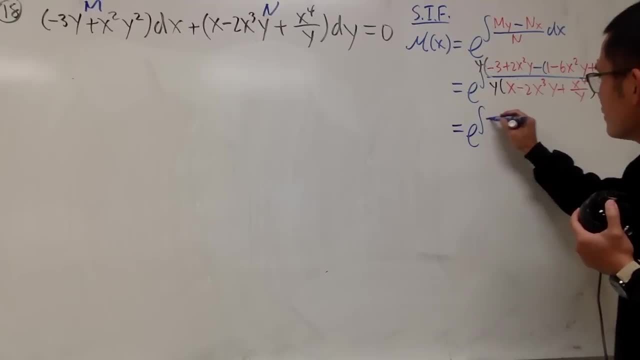 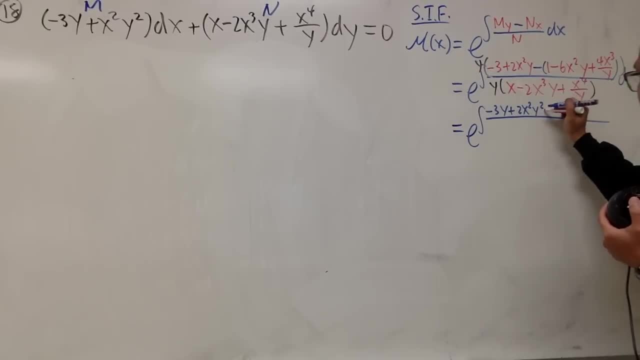 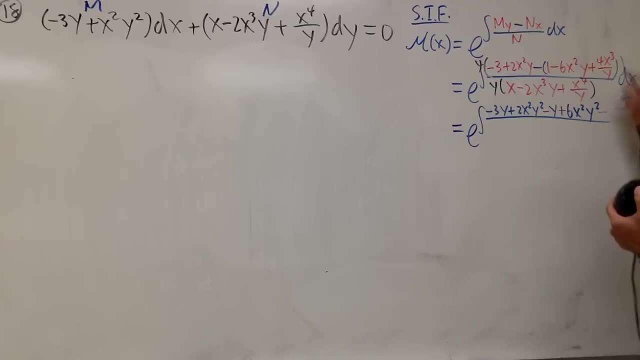 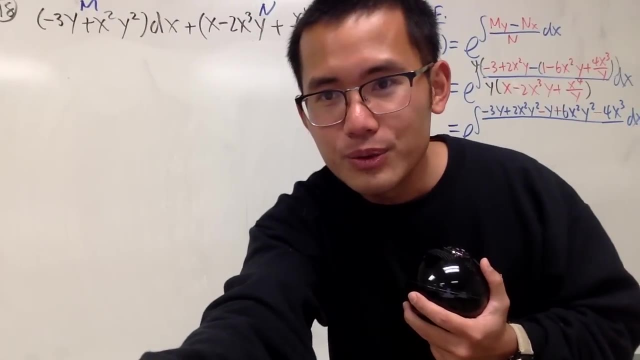 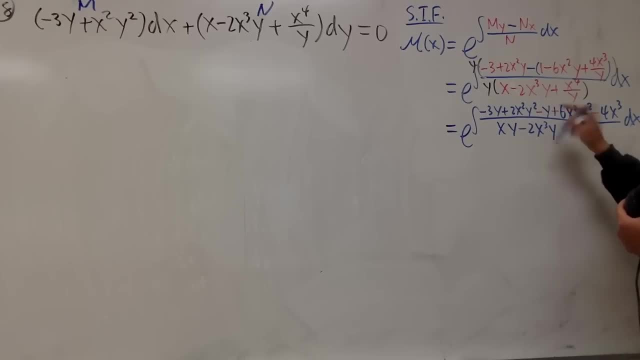 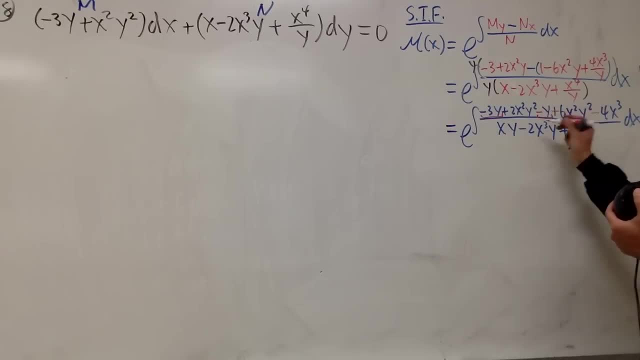 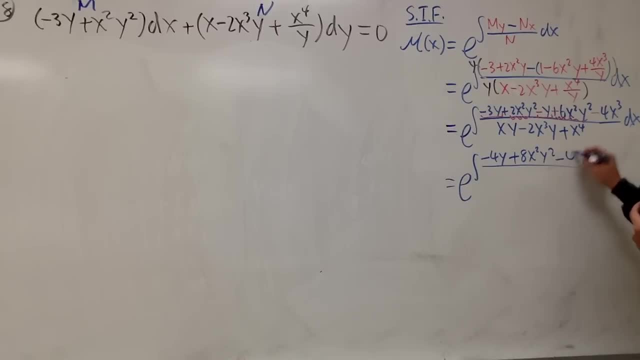 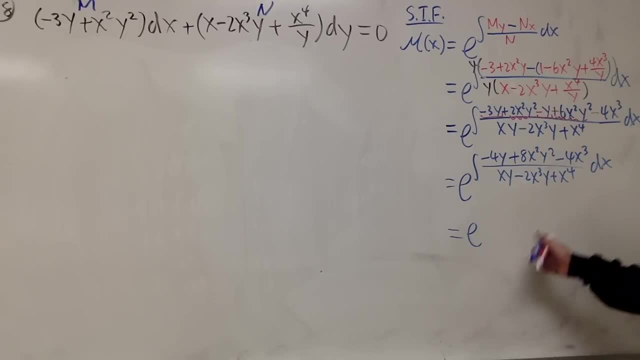 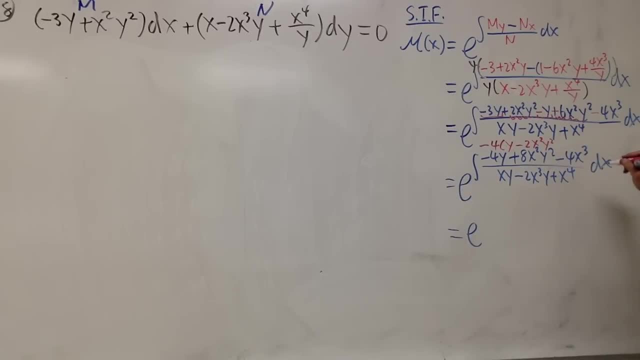 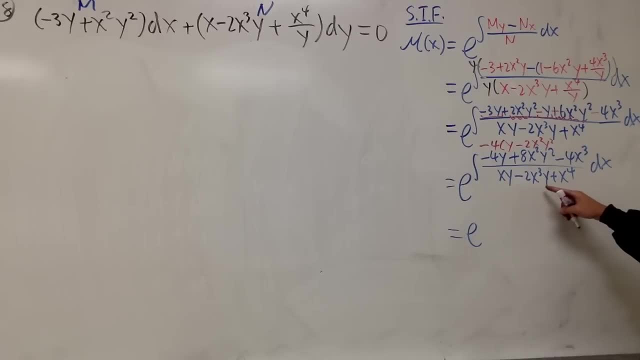 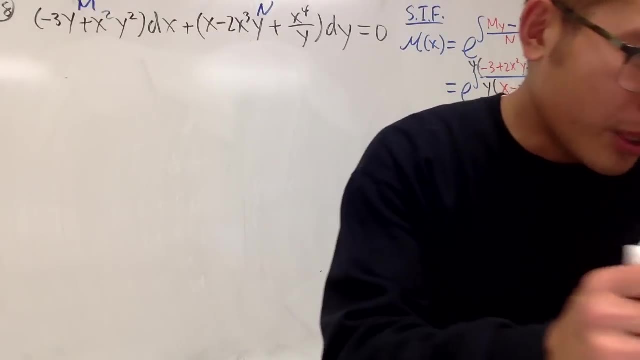 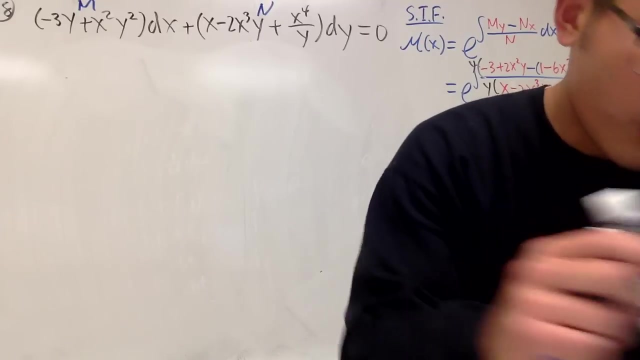 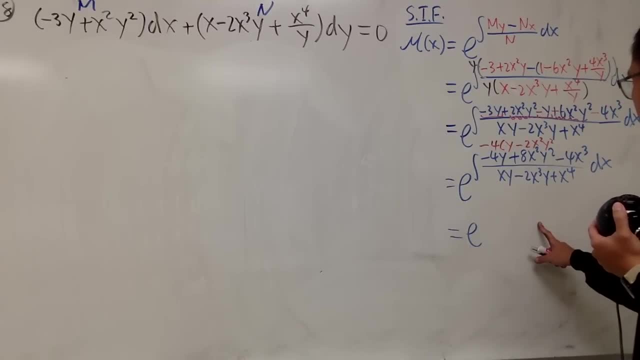 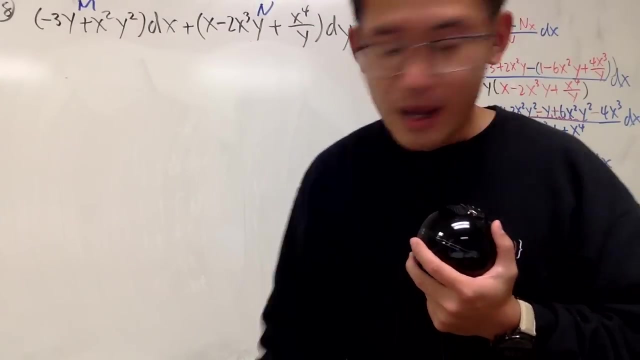 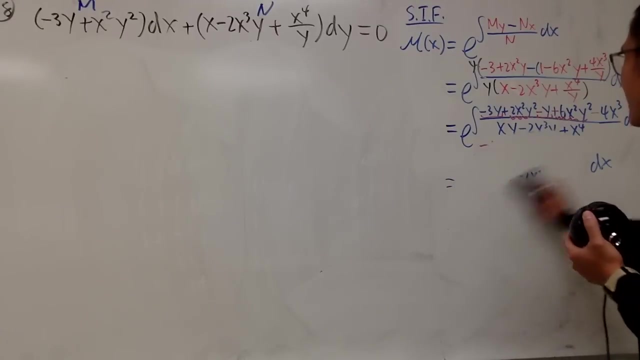 Ah, this is so bizarre. Hmm, All right, No, Okay, I'm not going to solve this. I'll show you guys how I was trying to create this question, right? So I really- oh, I cannot see After like three hours of differential equations. 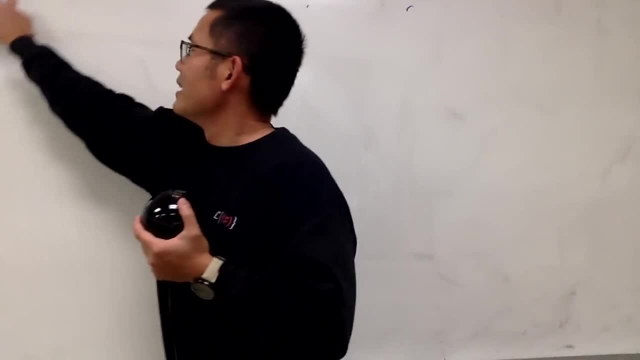 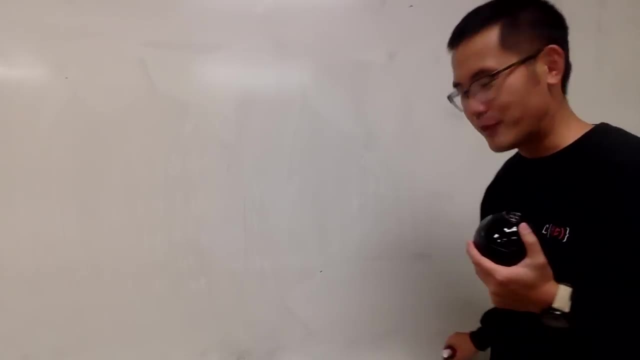 maybe there was just some small typo that I cannot see it, But anyway I will. you know, I will still, uh, make this as fun as possible for you guys. Here is question number 18.. Let me show you guys the following: 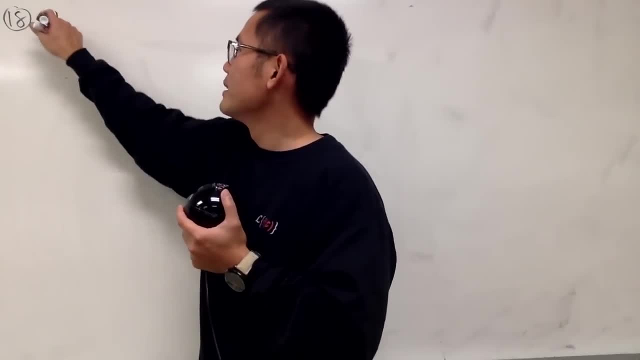 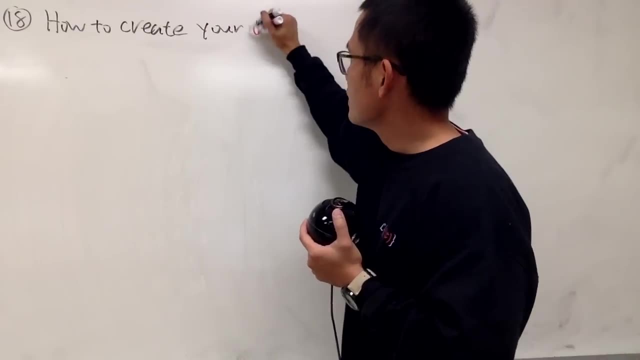 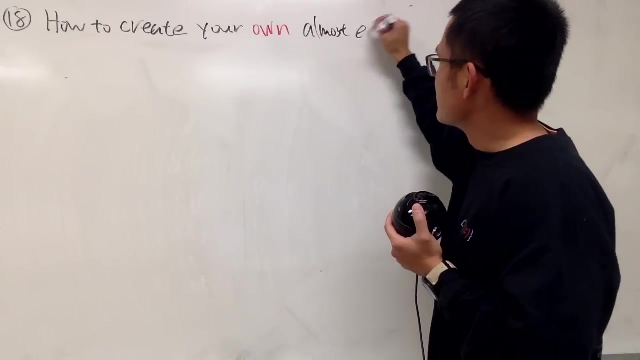 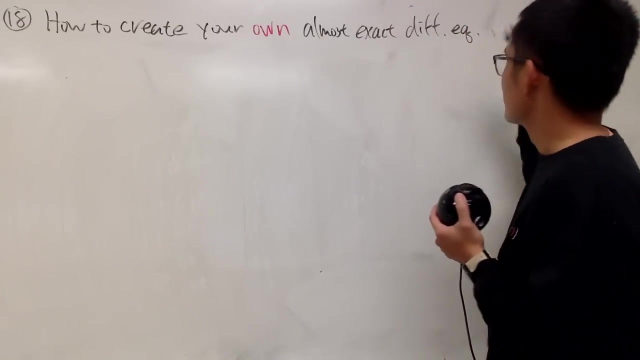 Number 18, I will show you guys how to create, how to create your own, your own, your very own almost exact differential equation, So you guys will see, like, how the uh things works. So I will tell you guys what it means. 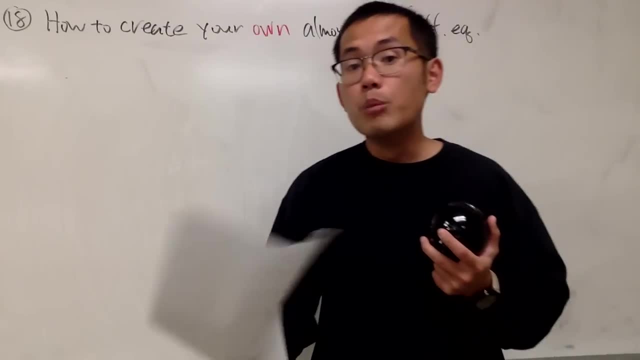 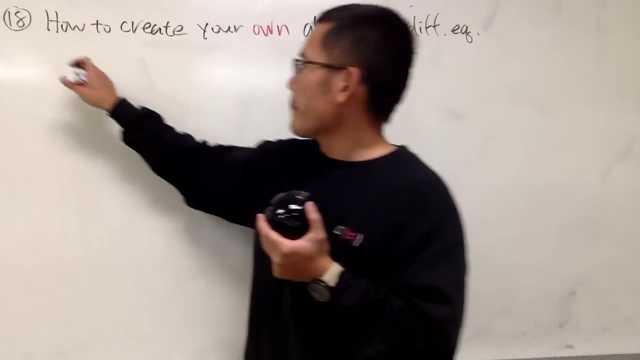 So here is the idea: You should have a function in mind, multi-variable, with both x and y. So this is the one I have in mind. All right, I will do this. So, um, we'll start with. um. a function is equal to whatever number. 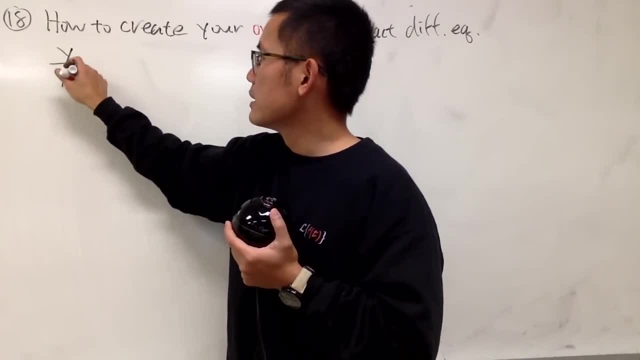 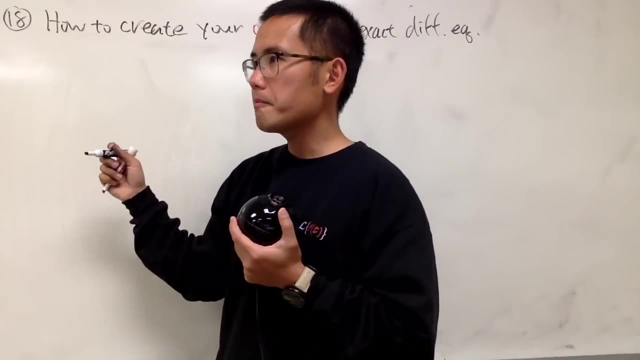 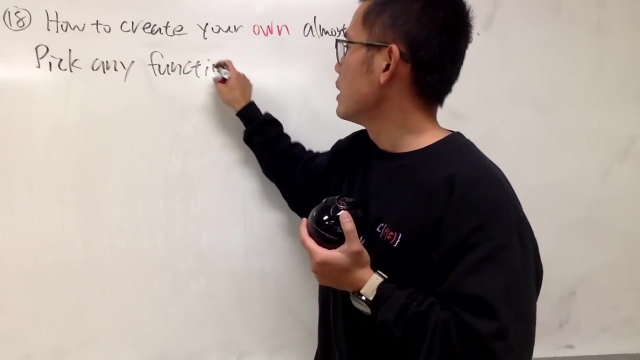 So I'll just write it down: We have y over x to the power, um, so this is just a just a. uh, pick a function, just a. pick a function, right. Pick any function right, And the one that I did was this: right. 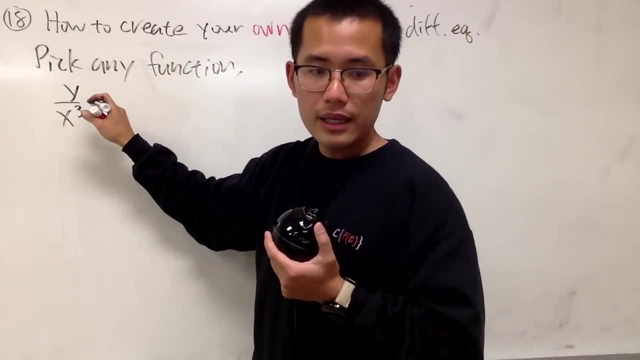 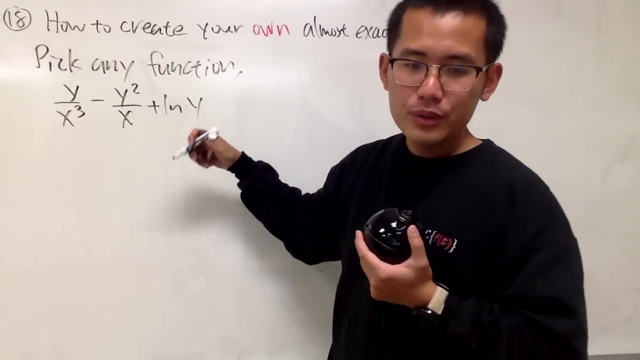 So I'll just say y over x cubed and minus y squared over x plus ln y And you can make this equal to whatever number that you want, but technically that's just a constant on the right-hand side It's not 0 that you guys see. 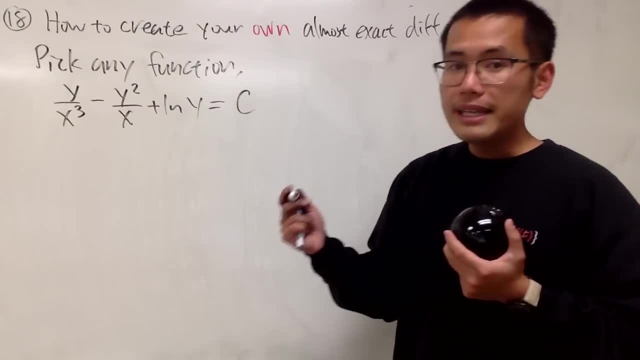 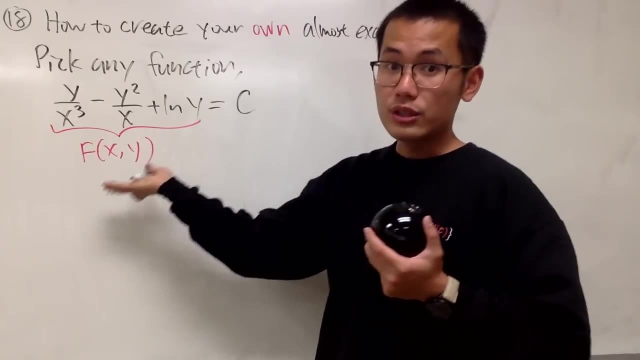 That's your change. that was just a constant. So the idea is that this part is the uh f of x, y, Right? So it's just a function in terms of both x and y, Like that. And now what you want to do is do the total differential. 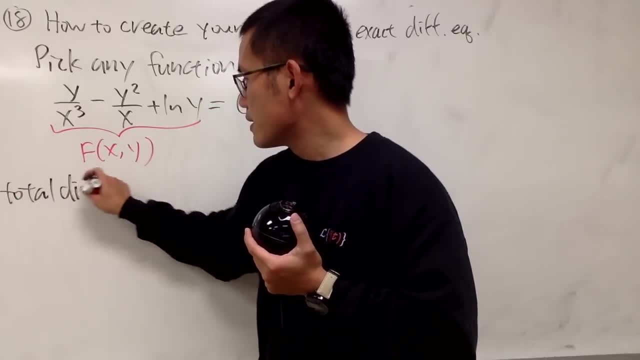 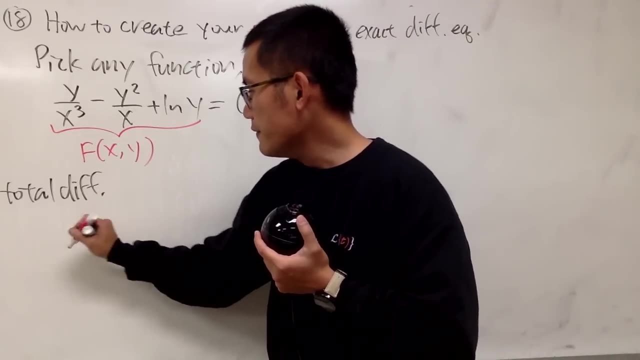 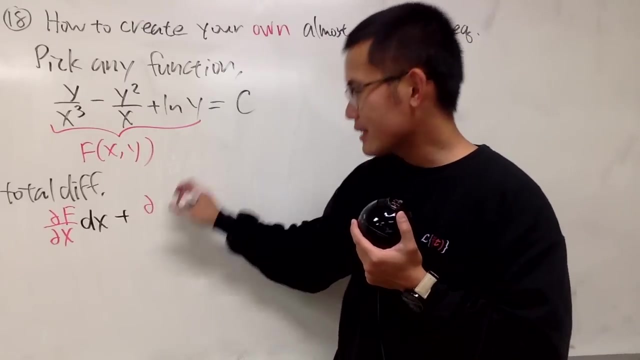 So here is the total differential, And the total differential is the calculus 3 idea. what you do is you do the partial of f with respect to x and then you multiply by dx and you add the total, Then you add the uh partial of f with respect to y. 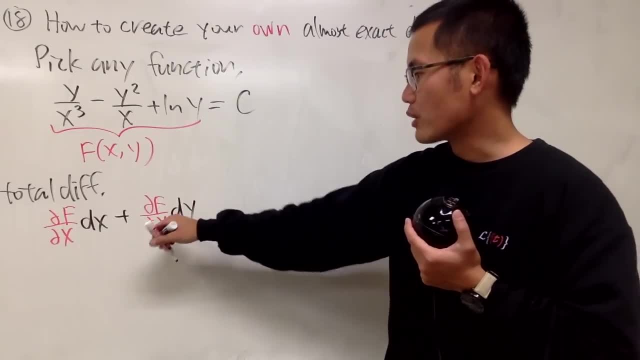 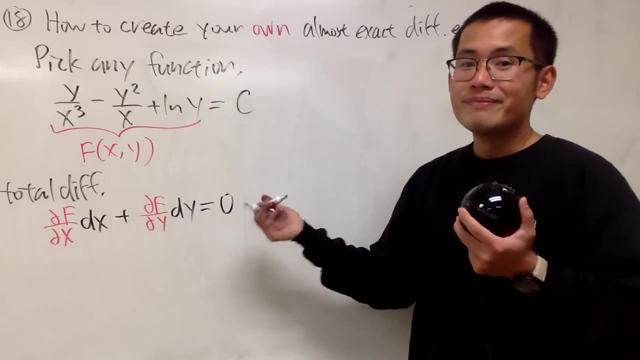 and then you do that with respect to y, so partial y and dy, And if you do the total differential, you're differentiating this, differentiating that constant, you will always get 0. That's why the exact differential equation is that equal to 0. 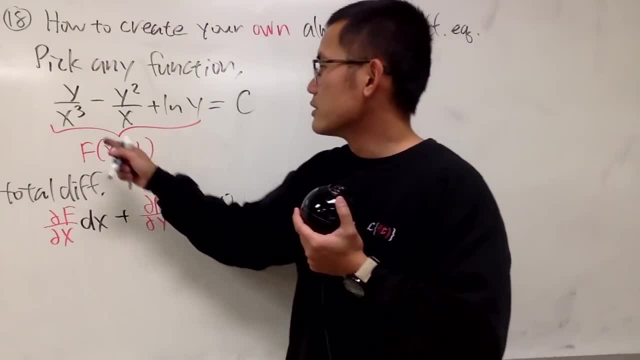 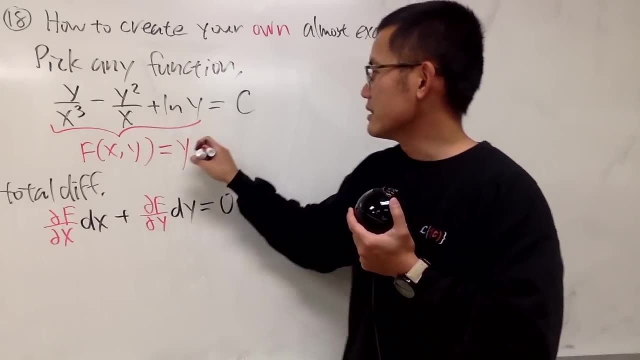 All right, so now let's just do this in our head. So here is the thing. This right, here is what I have, and let me just write it down in red. So we will have y, and this is x, to the negative 3.. 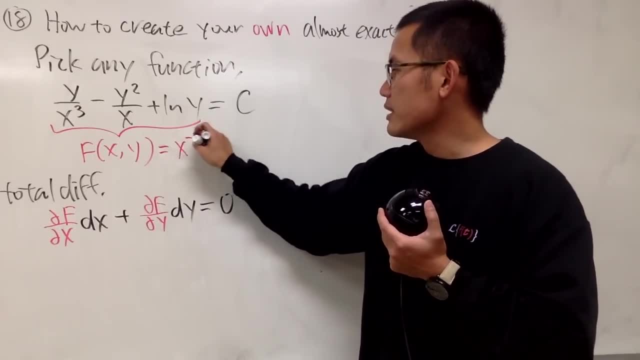 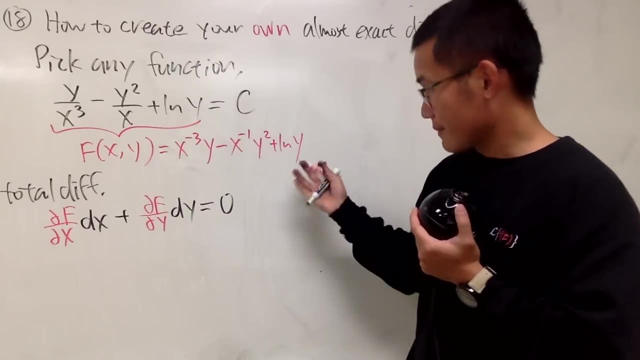 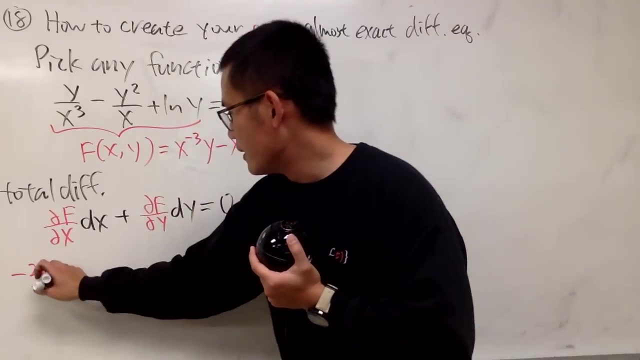 Let me actually write it down like this: So x to the negative 3, y, and then minus x, and then to the negative 1, y squared plus l and y. Now, differentiating this with respect to x, I will get negative 3, and then we have x to the negative 4, yeah. 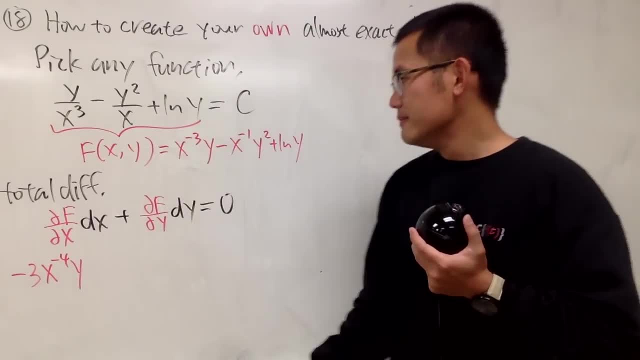 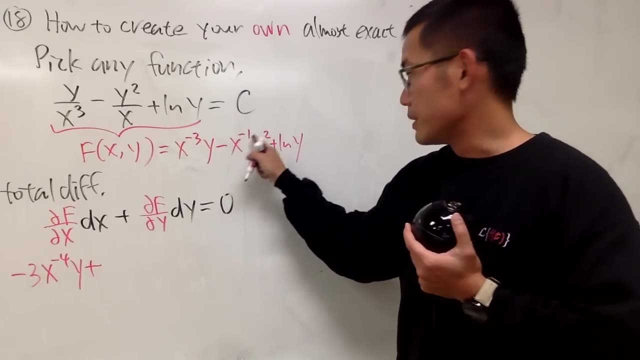 And then we have the y, like that Good. And then I will have to differentiate this. I will get plus and do the power rule so it becomes plus, and then we have x to the negative 2, and then we have y to the second power. 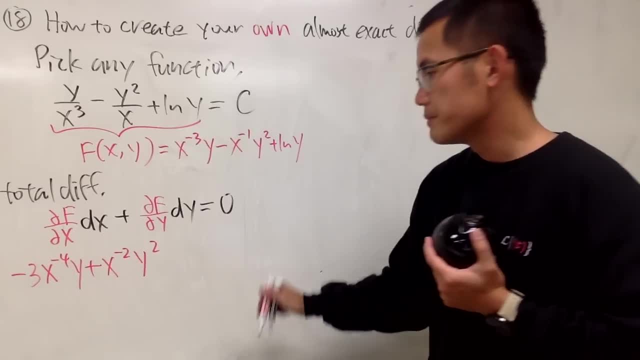 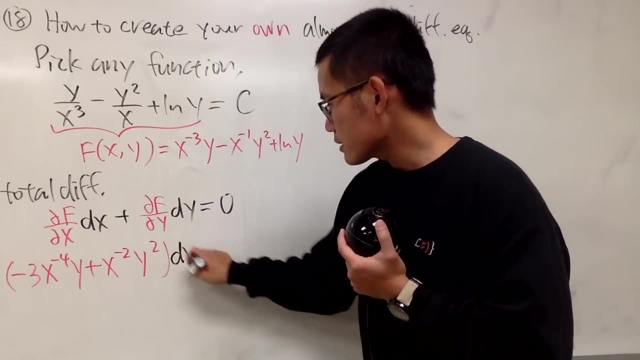 Good. Differentiating this with respect to x is 0. So we are good. This is partial f with respect to partial x, And then you multiply by dx And then you add: well, for the partial of f with respect to y. 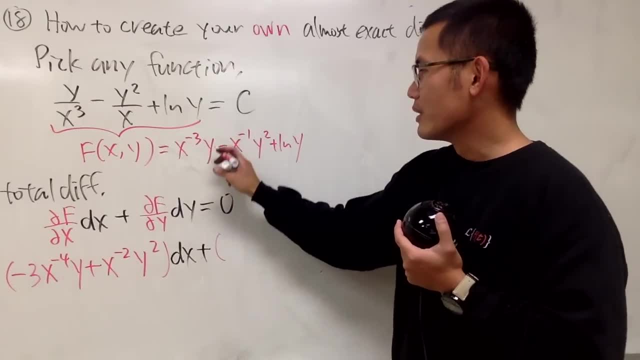 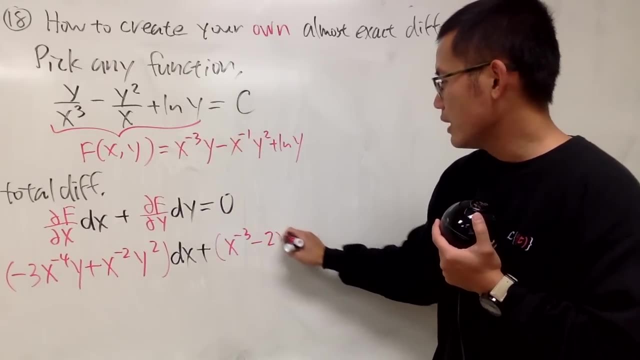 all you do is look at this and differentiate this with respect to y. So this right here will just give you x to the negative 3. This is out. This right here brings the 2 to the 5. So you have negative 2, x to the negative 1, y to the first. 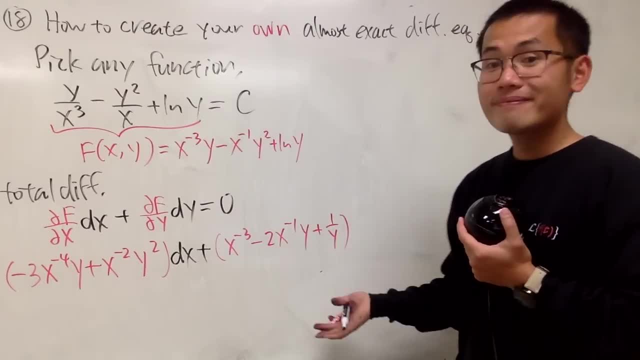 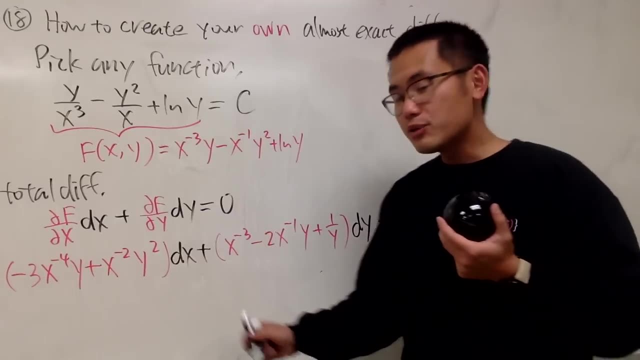 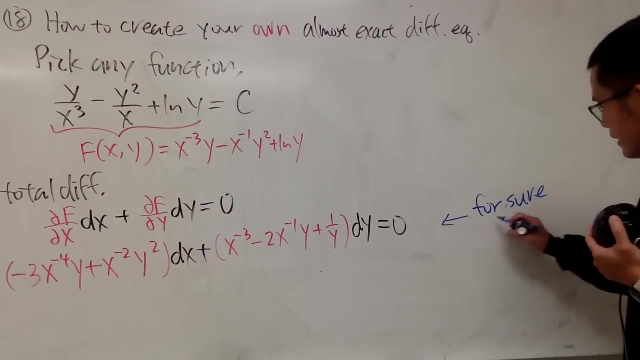 Lastly, you add 1 over y, like this, All right, And then dy, and that's equal to 0. So that's good. Now this right here is exact. I'll just tell you: for sure, Exact. This is for sure exact, no problem at all. 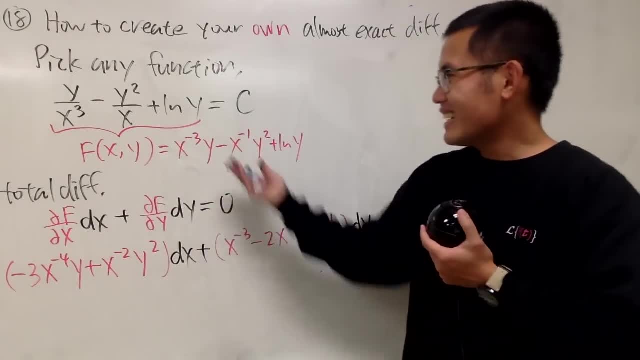 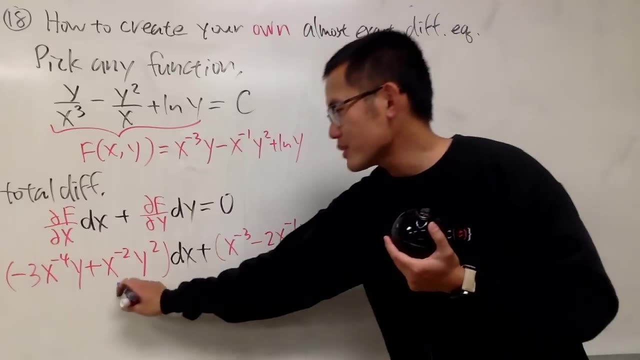 You can go ahead and check it, but Woof, woof, woof. This is exactly how I got this in the first place. Why did you even check? And yeah, you do the partial. If you do the mixed partial, go ahead. mixed partial with respect to y. 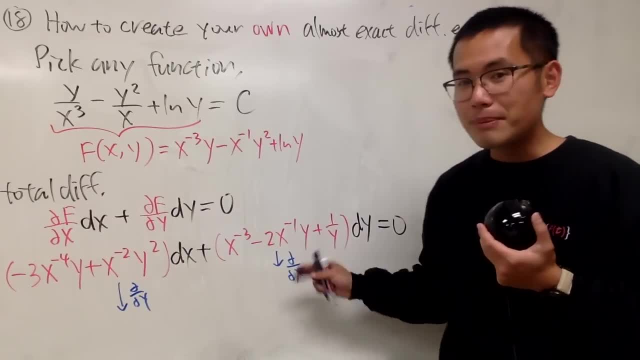 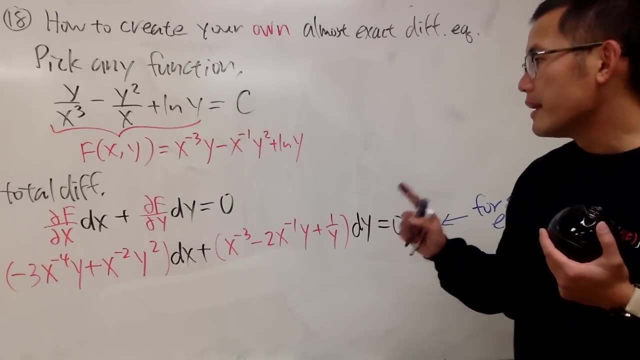 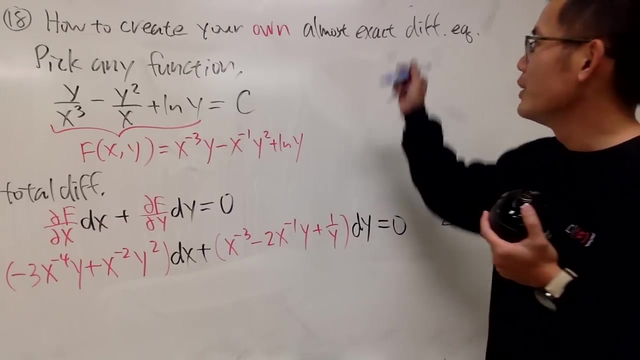 And then go ahead and do the mixed partial with respect to x, Do the opposite, You will see it's the same Guaranteed Promise. All right. Now here is the diodo. This right here is exactly exact. Good. But if you want to create your own, almost exact. 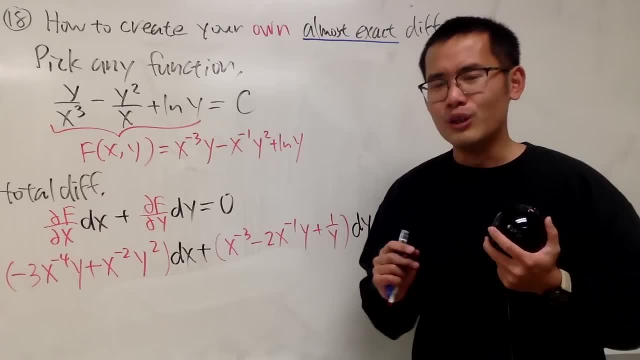 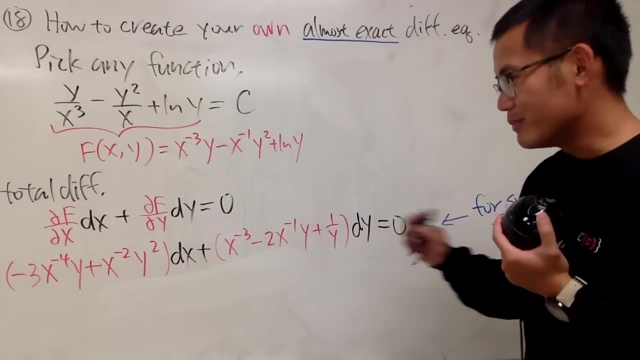 this is what you have to do. You just have to be evil sometimes. You just have to come here when people cannot see. you Just kind of make the change. Of course, you have to make it so that it's still equivalent. What you can do is- and this is what people like to do- 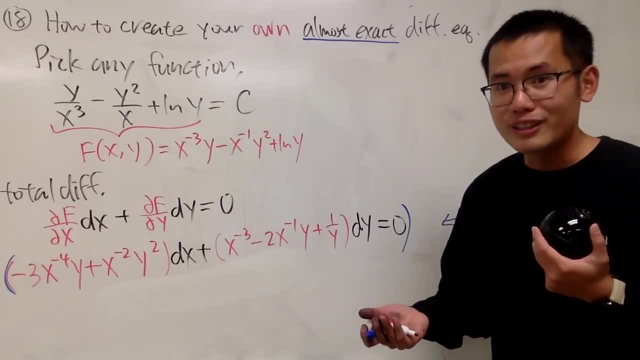 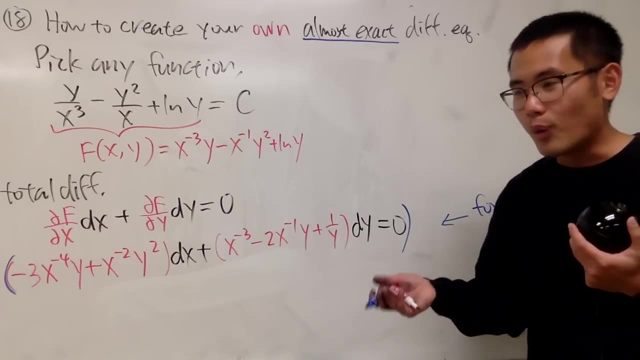 you multiply the entire equation by whatever factor that you want. You can multiply by sine x, You can multiply by tangent y, You can multiply by x over y to the 17th. power Up to you. But I'm not going to be too evil. 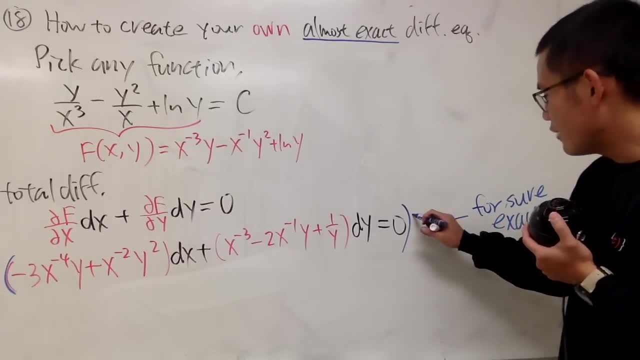 I'm just going to see: hey, this right here is x to the negative 4, so I will multiply everybody by x to the positive 4.. So this is my evil step When I multiply everybody by x to the 4,. 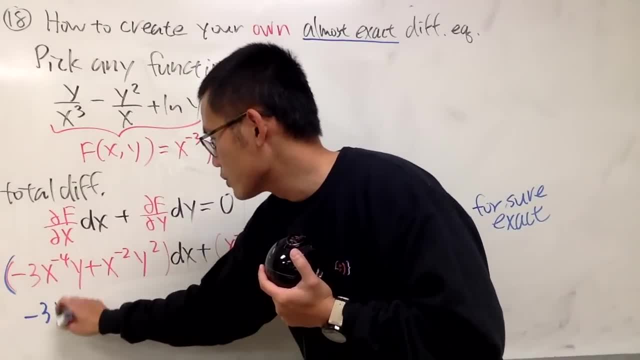 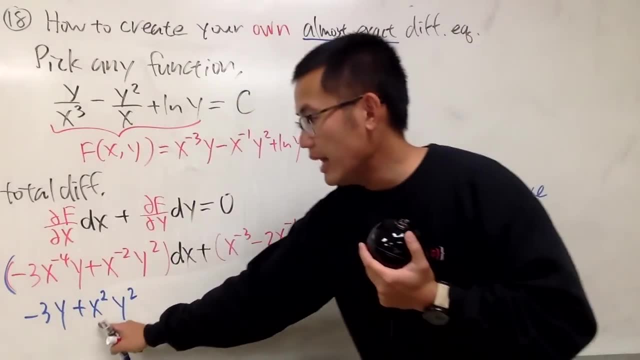 this right here we get negative 3.. That will be out, so it will be negative 3y. And then I add x squared, y squared. This is why it should be x squared right here, right, Yeah? And then go ahead and dx that. 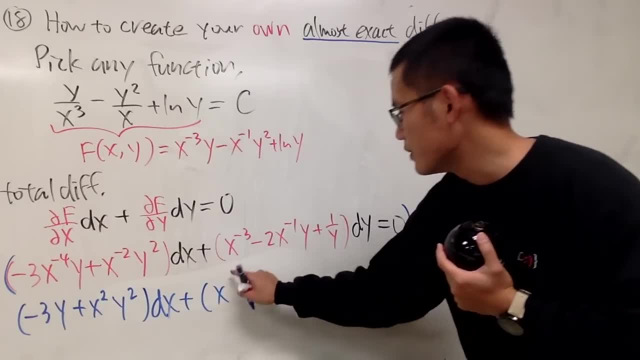 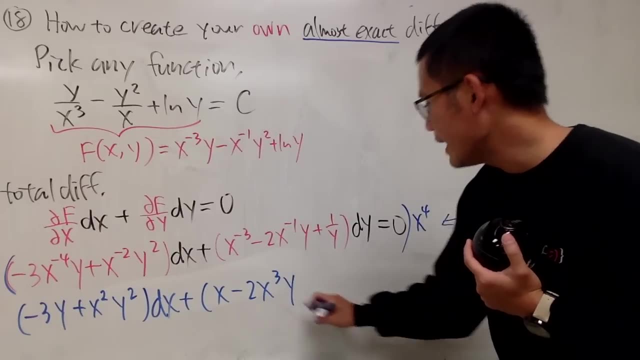 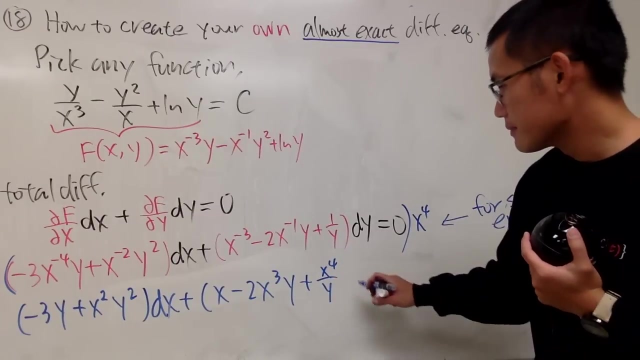 This times this, We get plus parenthesis x to the first power And this times that we get minus 2x cubed y And finally I get plus x to the 4 over y. like this, And dy dot is equal to 0.. 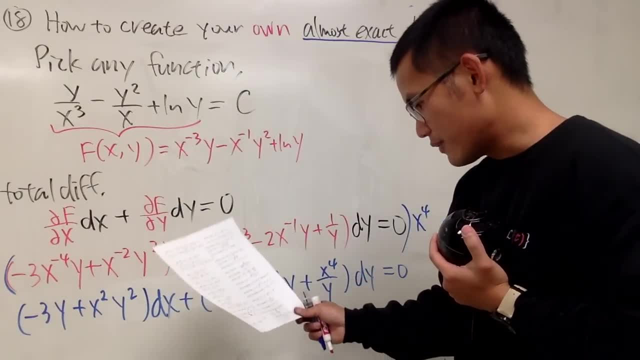 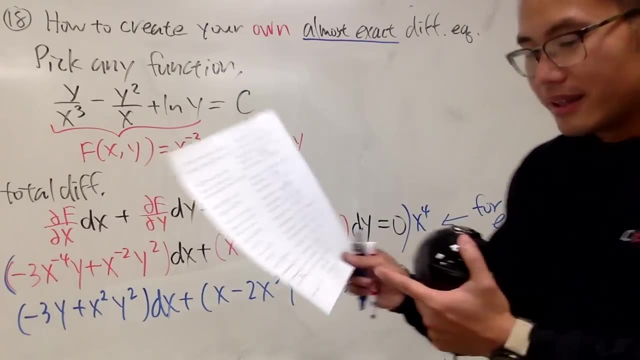 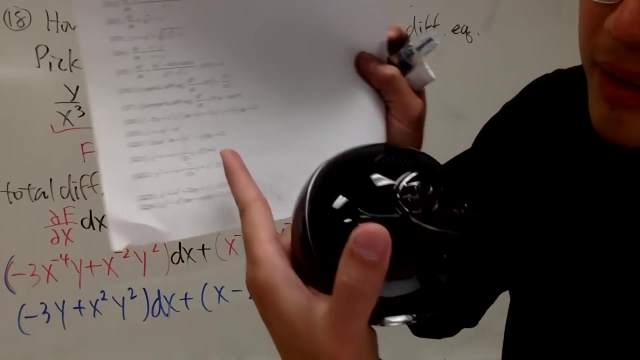 So this is how we create an almost exact differential equation, And it seems like there's nothing wrong with this. I don't know, I think I just have something wrong there. But anyway, this is why this right here- You see, this right here- should have been x squared instead of y squared. 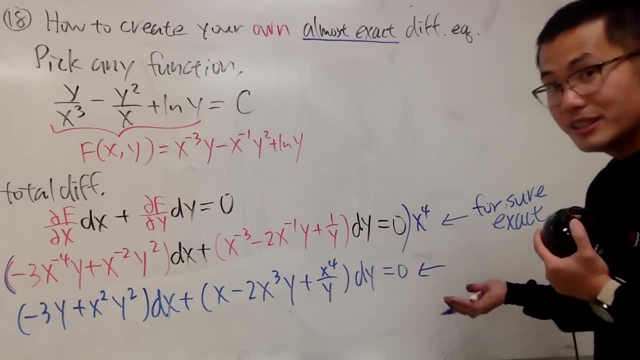 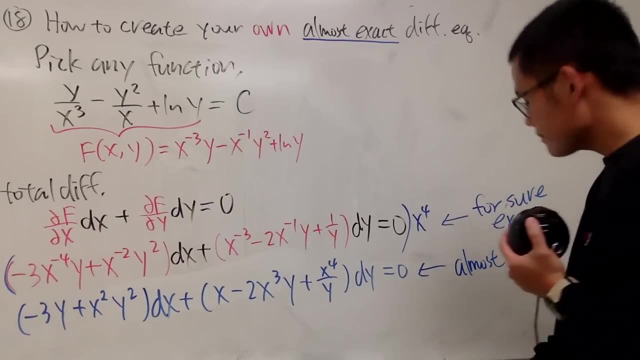 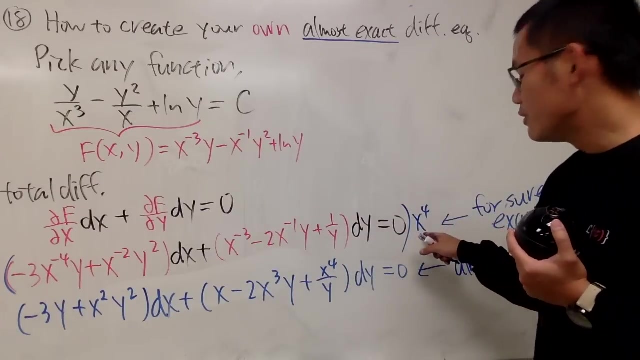 So, anyway, this right here, I will tell you that's how I create the almost exact differential equation. This is almost exact. Well, what does it mean? almost exact? Well, because it came from an exact differential. And I will show you that it's an exact differential equation by multiplying everybody by x to the fourths. 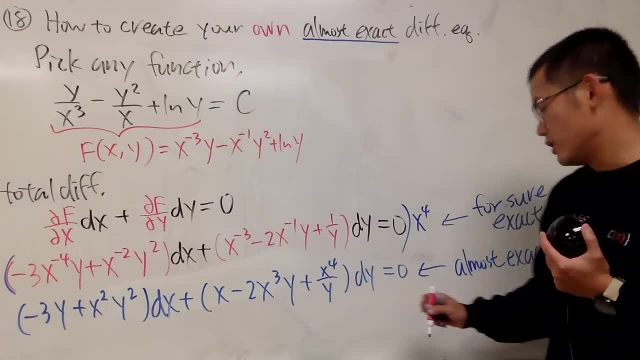 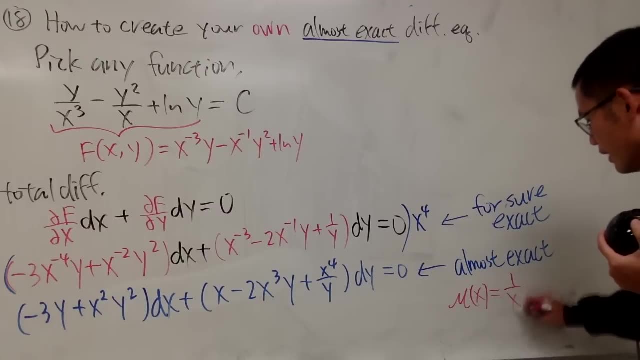 How can you make this exact? then Just go ahead and define everybody by x to the negative 4.. So you know, this is almost exact, And you will know that the special integrating factor is equal to 1 over x to the fourth right. 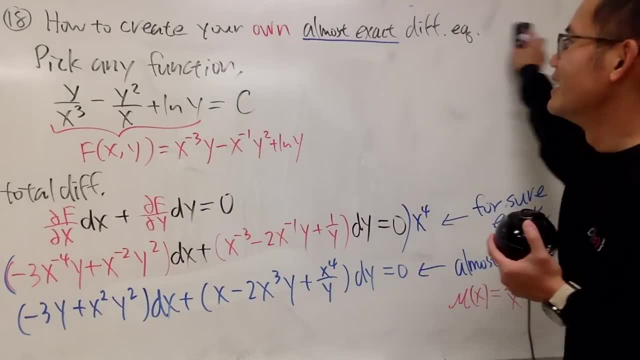 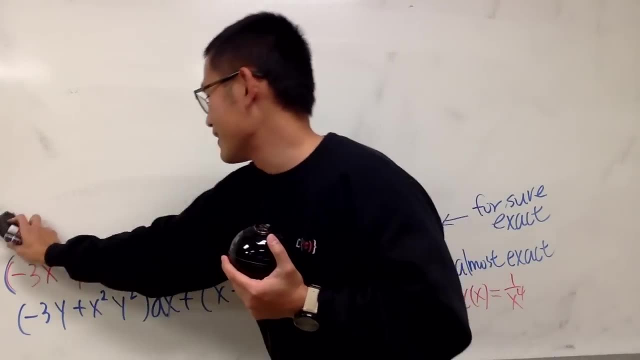 So you know this for sure. Now I'm going to stop this right here, because, Alright, Third try, I'm not going to mess this up one more time. right, I'm not going to mess this up again. Okay, so here we go. This is question number. 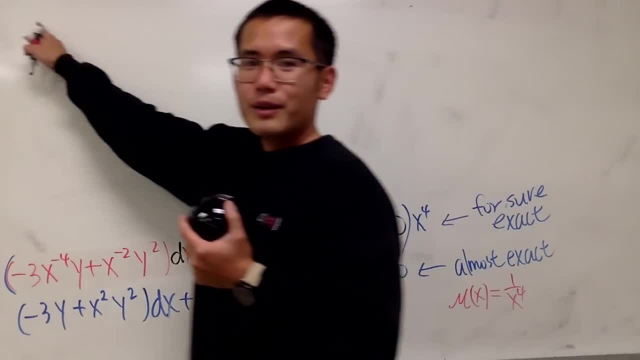 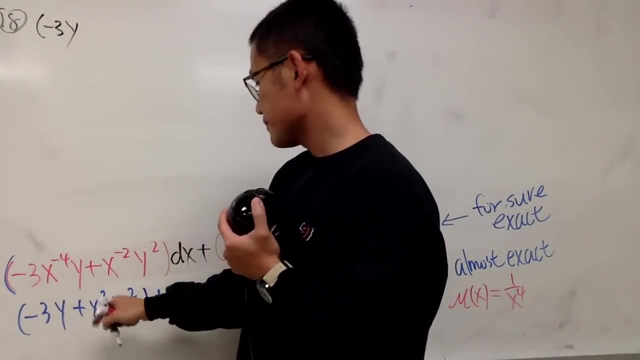 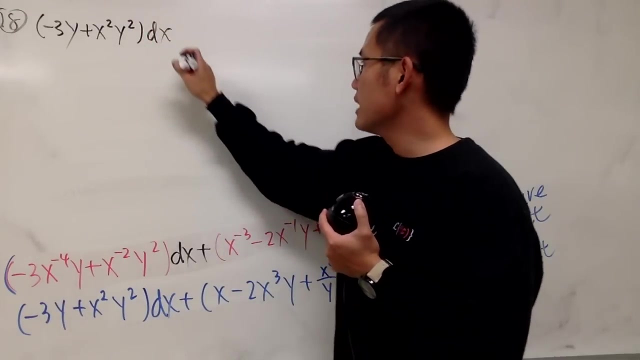 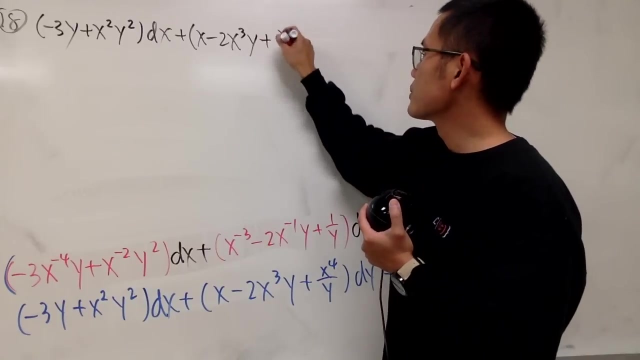 18.. Alright, question number 18, right here I'm going to have negative 3y plus x squared, y squared, and then dx that, and then we have plus parenthesis, x minus 2x, cubed y, and then plus x to the fourth over. 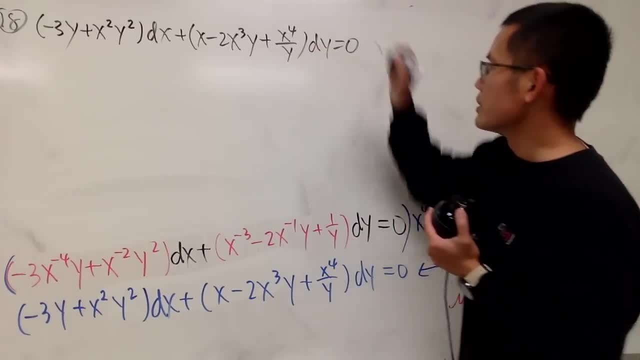 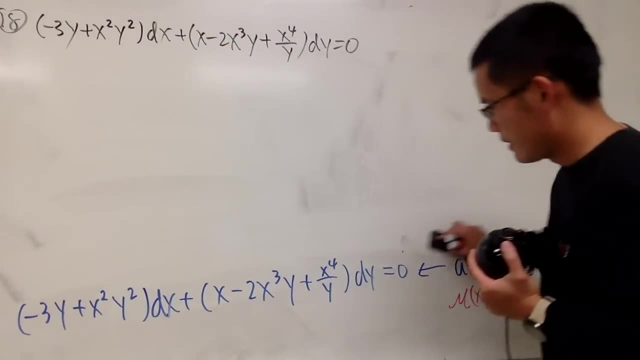 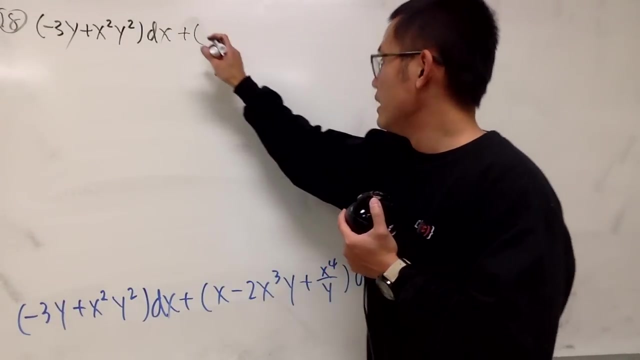 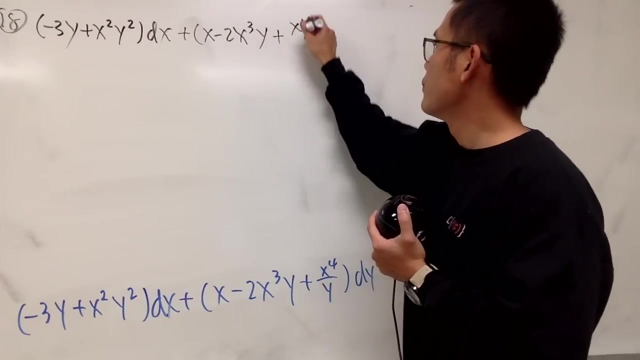 y and dy, this is equal to 0.. Alright, so now here is the dR. Actually, let me write it down better, because this is not plus parenthesis, x, minus 2, x cubed y and then plus x to the fourth over y. 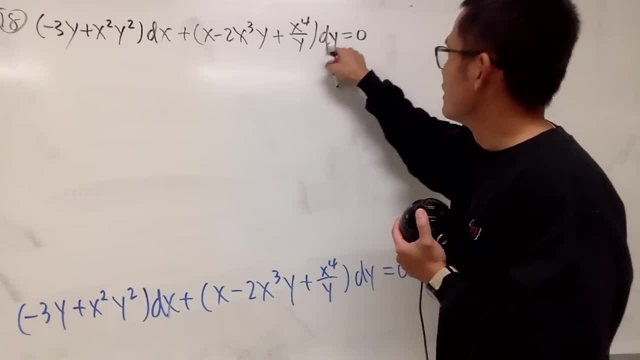 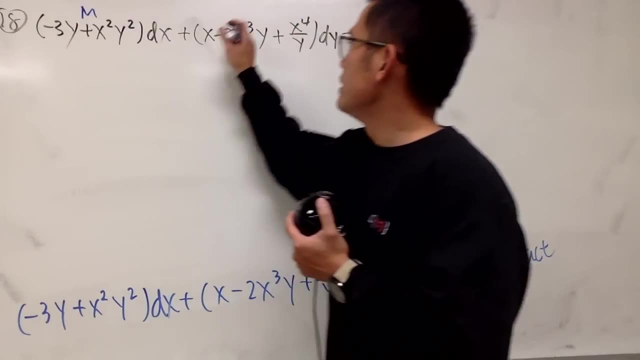 dy equal to 0.. I'm going to have to solve this for sure. Okay, here we go. This is m, this is n, this is almost exact, and we will have a special integrating factor, which is the following Special 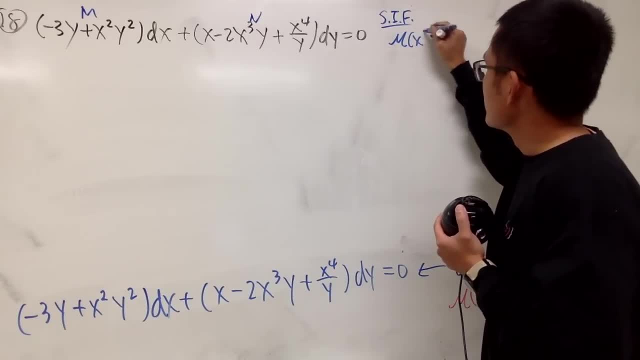 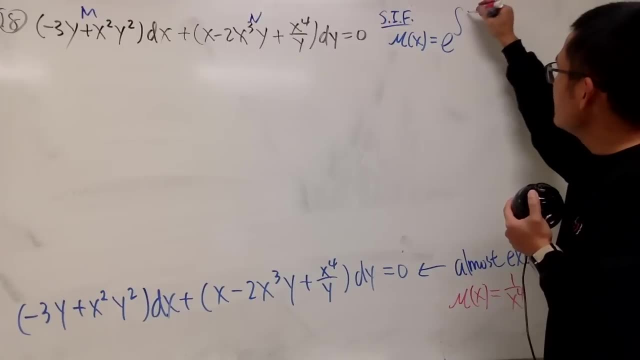 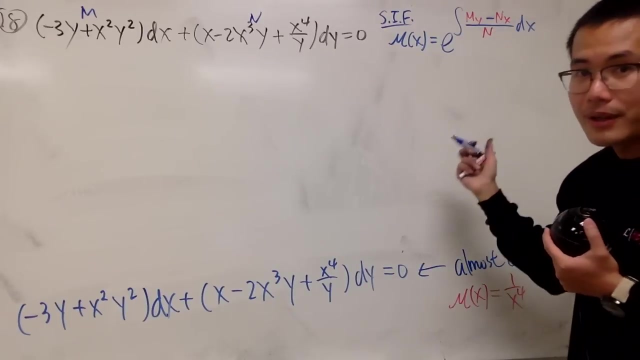 integrating factor mu of x is equal to the following: e is e, integral is integral. and then we have m sub y into m sub x over n dx. Okay, and let's go ahead and work that out. So, mu of x. 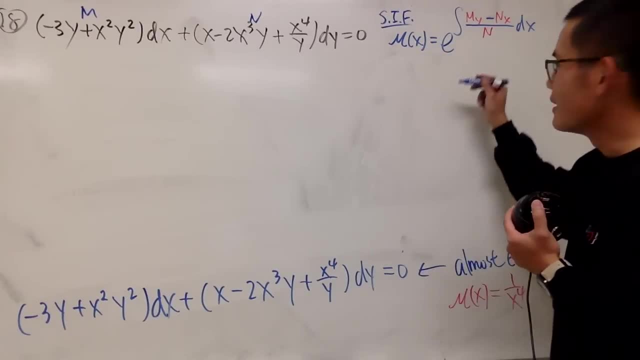 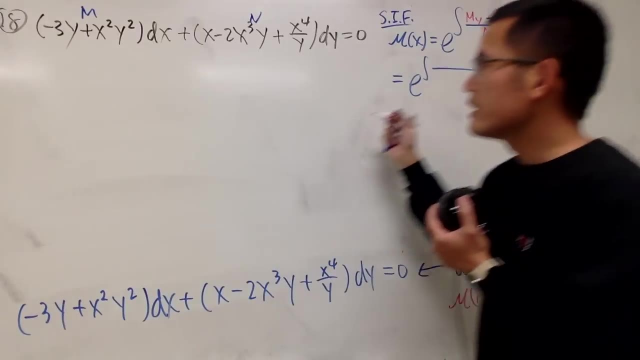 actually I'm not going to write that down again. So this right here is equal to e integral m sub y. Okay, I'm going to focus: This is negative 3y, so differentiate that we get negative 3.. And then I add: 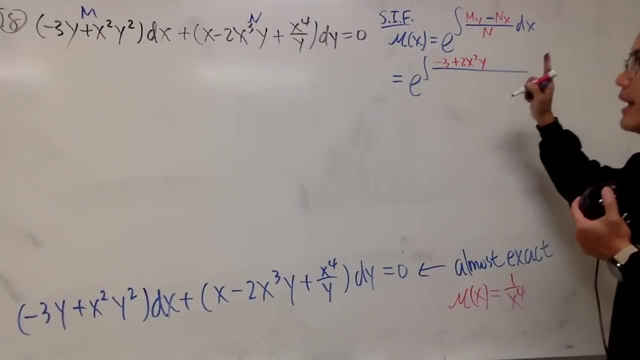 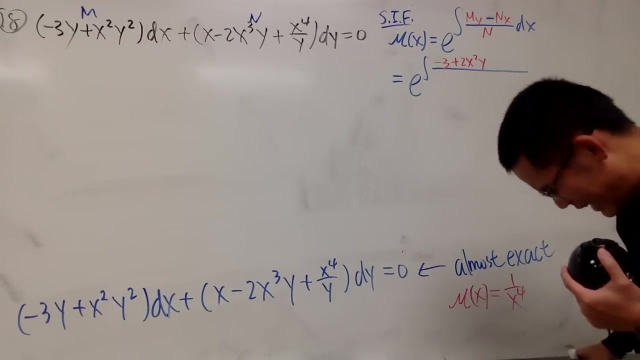 2x squared y to the first. Good, And then I will wait, let's see, let's see, let's see. I think I know why I made the mistake earlier, but I, I, I, I think, I know, yes, yes, yes, I know I forgot to that multiple. 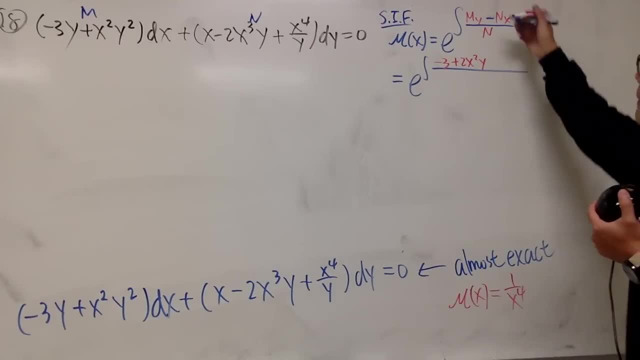 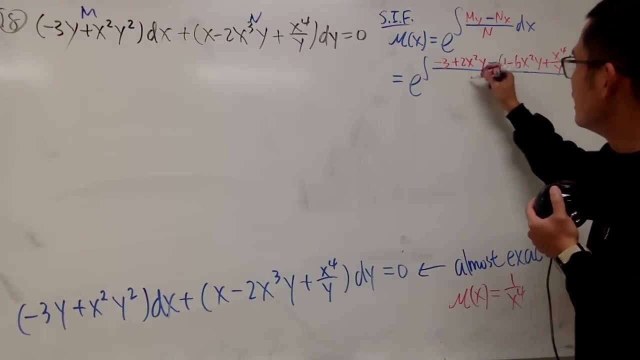 okay, just do it all right. so we have this, and then minus m, sub x, which is this, and you differentiate it with respect to x. so we have parentheses: 1 minus 6x, squared y plus x to the fourth over y, like this, and then dx and the n is all that stuff. so we have x minus 2y, cubed y. 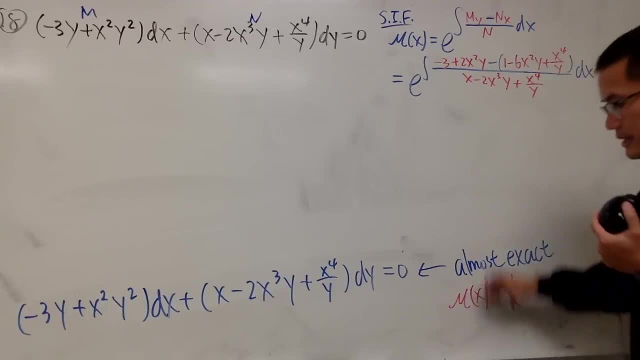 plus x to the 4 over y, like this. now this is the third time saying this. we see that we have a complex fraction, so I'm going to multiply everybody by y, so we don't have to deal with the complex fraction. that's good. 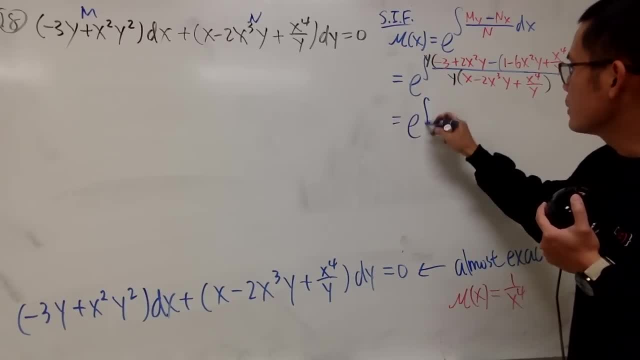 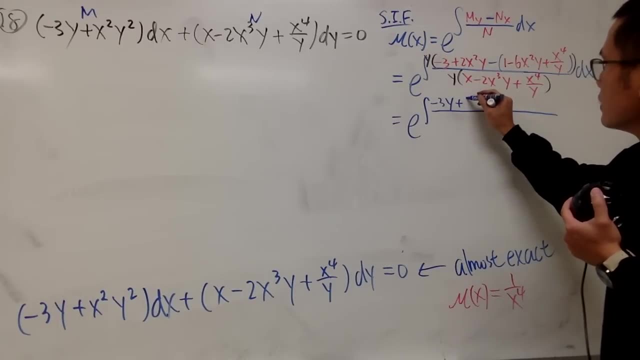 so then we see that this is going to be e integral on the top. this is negative 3y, this, and that is plus 2x squared, y squared, and then this, and that is negative times 1, which is negative y, this, this, and that it becomes minus. minus is plus, and then we have 6x. 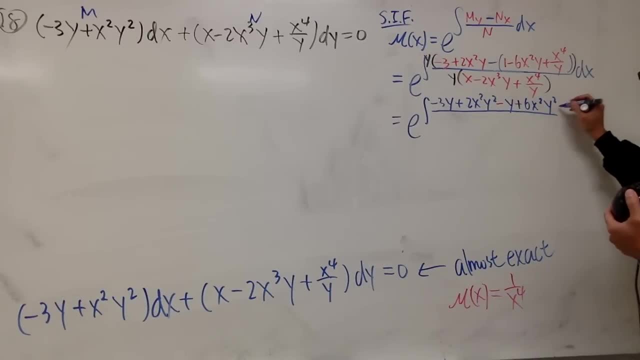 squared, y squared, and then the y cancels out. so plus x to the fourth power, like that right, and then on the bottom: this times this is xy, this times this is negative. 2x. cubed, y squared. there you go, there you go, there, you go. y times this is plus x to the. 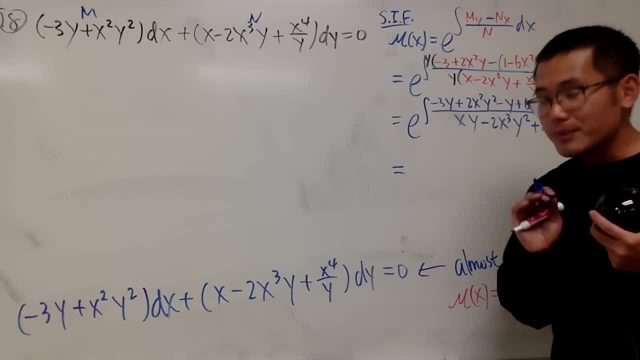 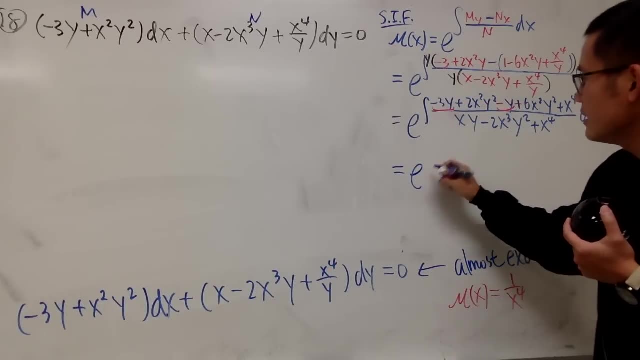 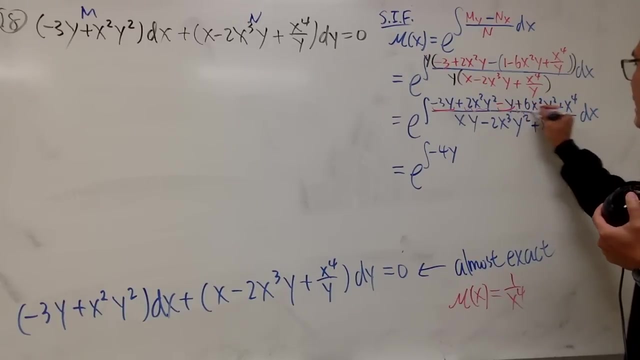 fourth power like that: good, now guaranteed. this will work on the top. we can combine the terms this and that, this is going to give us e integral. this, and that is negative 4y, and then this and that is plus 8x squared, y squared, and lastly, we have the plus x to the 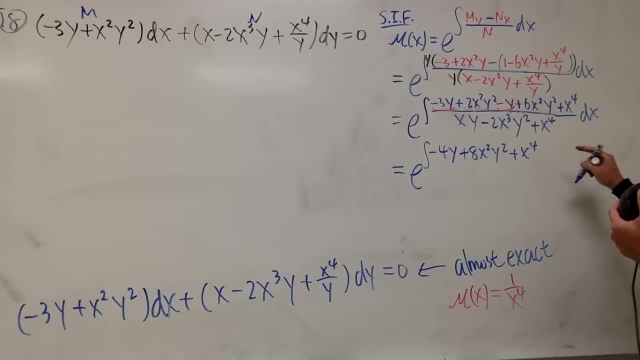 fourth power, like that. good, yes, yeah, over. this is the x. oh, by the way, negative, negative again. it should be positive here. I mean negative, positive should be negative. sorry, okay, I'm not going to make another mistake. that's, that was. that will make me cry big. 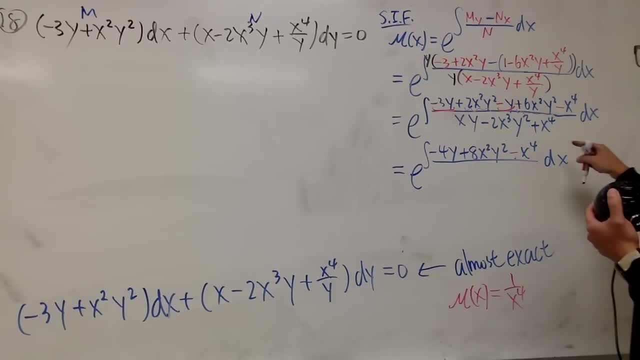 time. but what happened to my 4,? seriously, okay, another mistake. this is horrible. I'm so sorry. all right, but this is just a tiny mistake. n sub x, differentiating x to the fourth over y. this right here should have been 4x to the third power. okay, 4x to the. 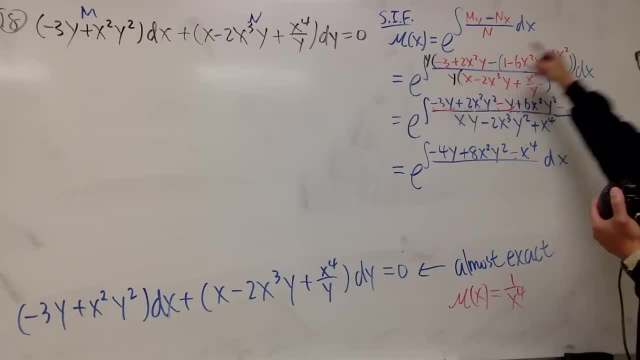 third power. I'm sorry, yeah, so when you multiply like this, by that, you get 4x to the third power, and this right here should have been a minus. yeah, minus, plus is minus and this is still a minus and this should have been. 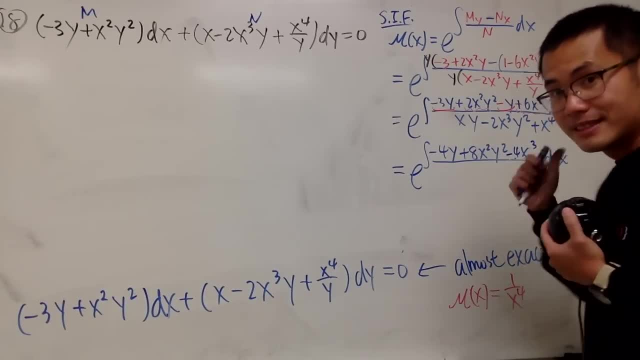 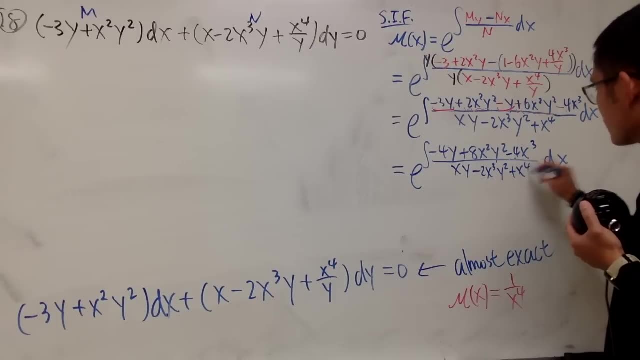 a 4x to the third power. we're good on the bottom. let's just keep it xy minus 2x, cubed y squared, plus x to the fourth power. okay, now on the top we can factor things out. 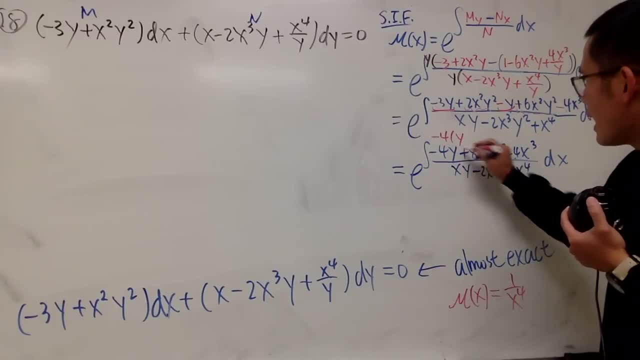 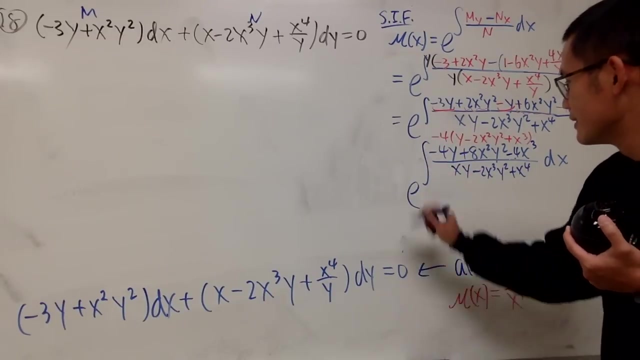 we can factor out negative 4, and then we get y Watts, y minus 2x squared, y squared, and then plus x to the third power. yeah, good on the bottom, this right here. you made the integral longer. that's horrible on the bottom. 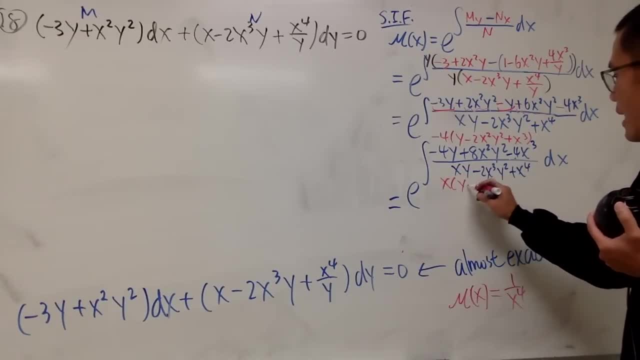 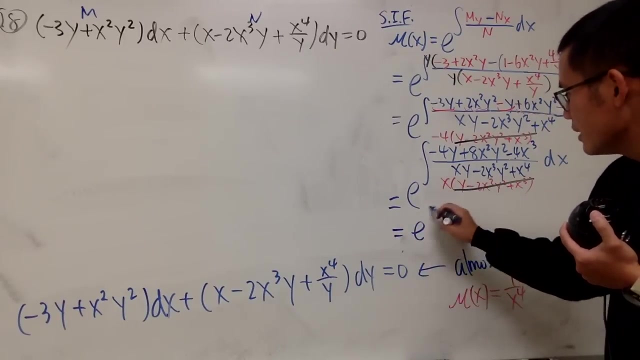 we can factor out an x, so factor out the X and you get y minus 2x squared y squared plus x. to the third power. third power, oh my goodness, this and that are finally the same. so this. cancel out with that, thankfully. and this is equal to e, to the integral of negative 4 over x, dx, which is the same as. 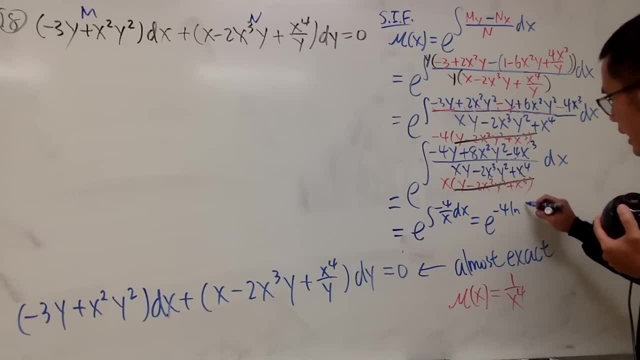 saying e to the negative 4 and you have ln absolute value of x. but again you bring this to the front and bring this back here, so you get e, ln x to the 4 negative and then of course you can just have the absolute, you can just have the parentheses and this and that cancel finally your 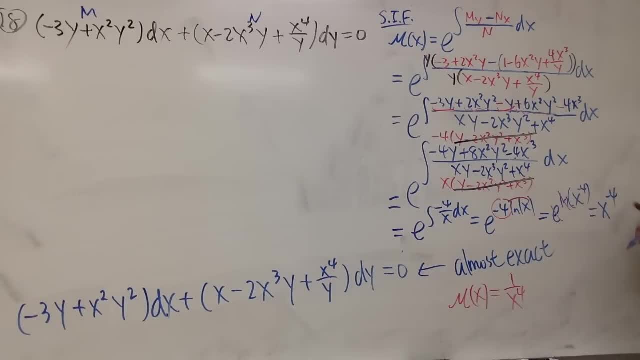 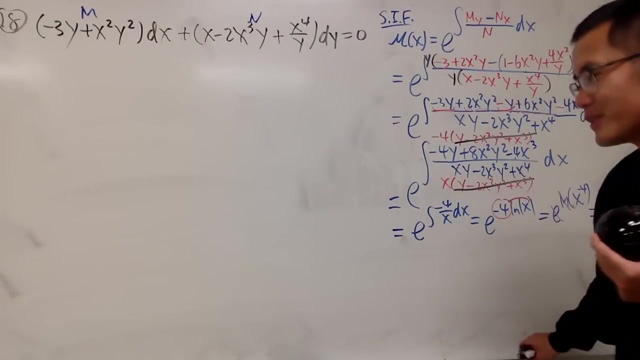 new prime is x to the negative 4.. thank god, so this is x to the negative 4, right? so that's how i got the almost exact differential equation. so sometimes, um, don't boot, don't, don't do it bad things, you know, this is what happens when you like uh have a, when you ruin somebody's. 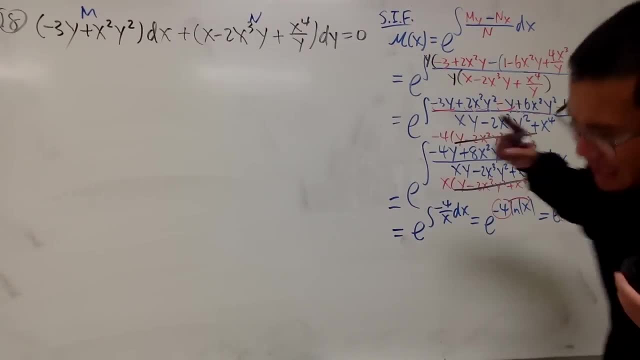 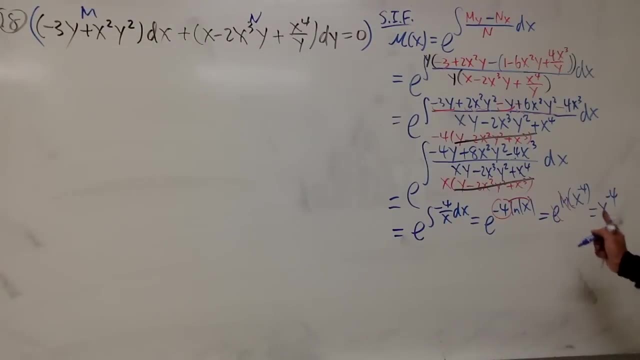 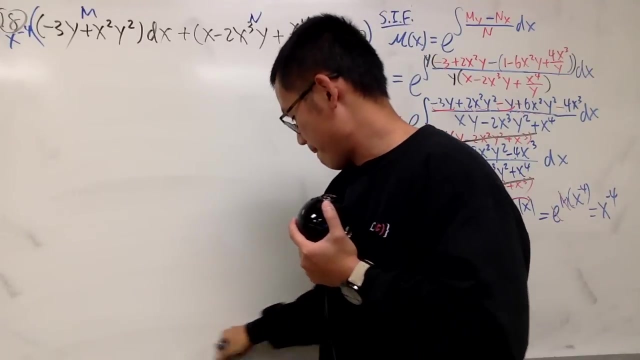 exact differential equation and that would be really bad. anyway, we are ready to solve this guy. go ahead, multiply everybody by this, so i'll write the s x to the negative 4 all the way in the front. yeah, so here we go. so when we do that, we will have negative 3, x to the negative. 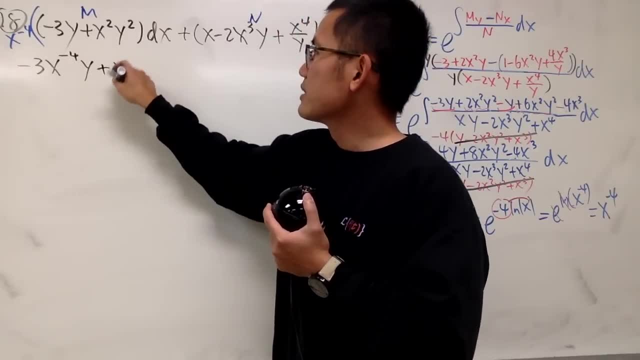 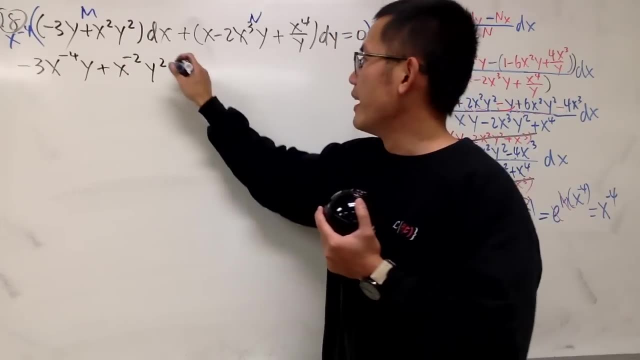 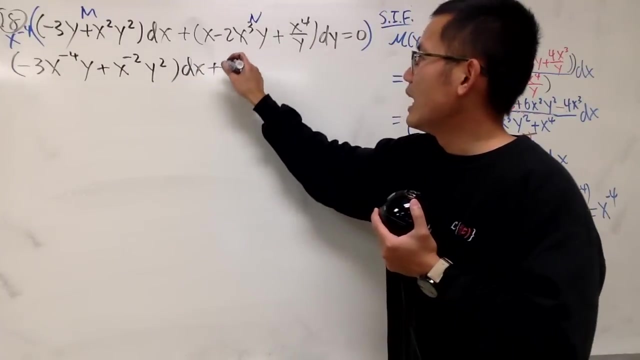 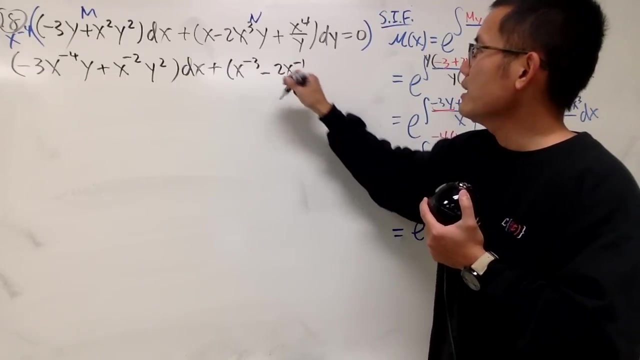 4 y. this times this is plus x to the negative 2, am i right? yes, and then y square. yes, and then i have the dx here and then plus this times this, we have x to the negative 3. this times this is plus. i mean minus 2x to a negative 1 y. they cancel. so just plus 1 over y dy. 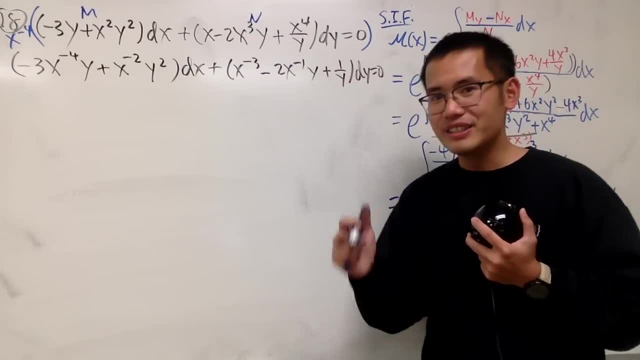 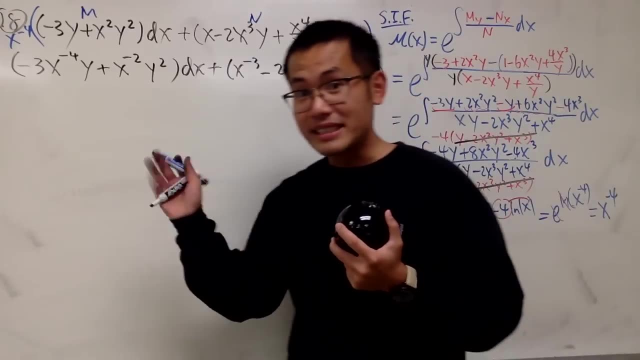 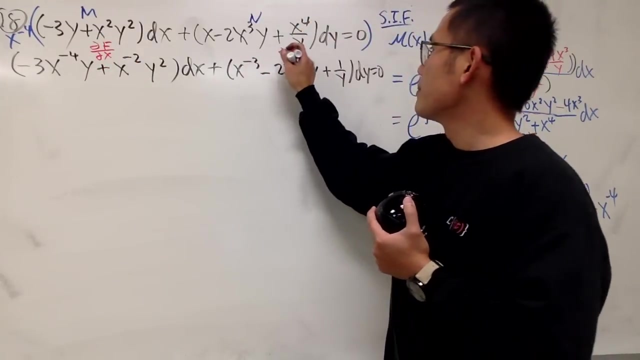 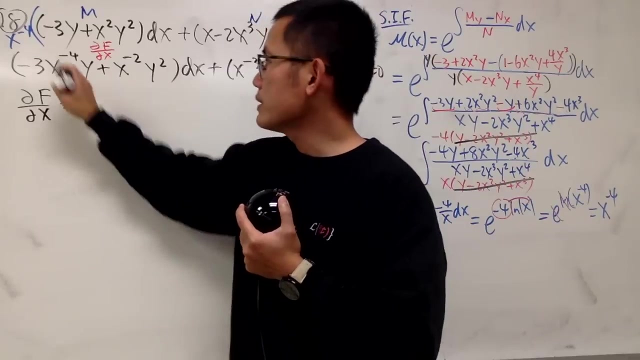 dy equal to 0.. that is good. now, uh, let's go ahead and do the following. this is exact for sure. so we know this is partial of some capital f with respect to x. this is some partial of f with respect to y. write this down: partial f with respect to x equals this: negative 3. x negative 4. 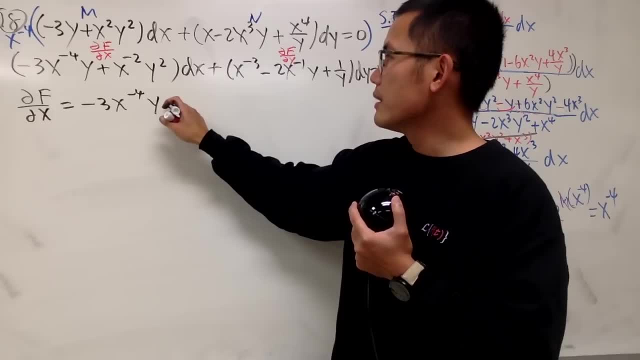 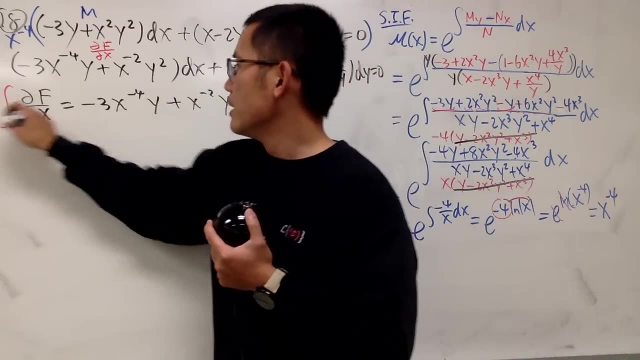 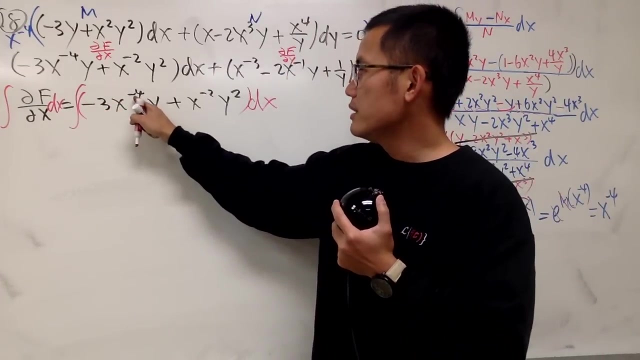 y and uh, plus x, negative 2, y, 2. Yeah, like this, Go ahead and integrate with respect to x. Okay, so for this one, do it carefully. This is negative. 4. Do the power rule is plus 1,, which is negative 3,. 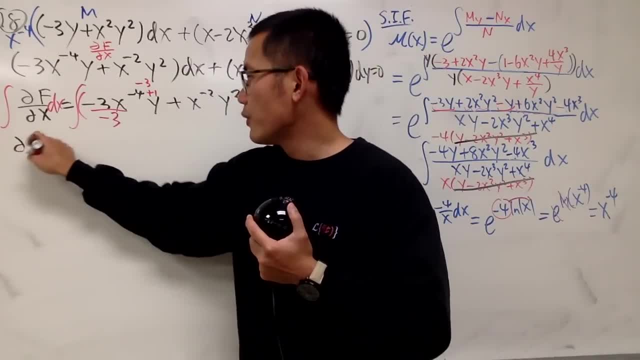 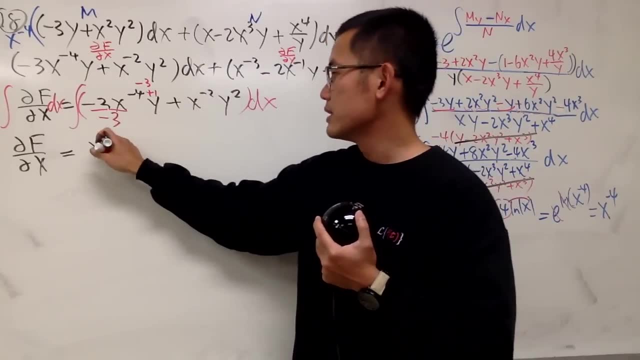 and you divide it by negative 3.. So you get partial f with respect to x, equal this cancel. so you just get x to the negative 3 power first, And then the y is just a constant multiple, so you just multiply it like this: 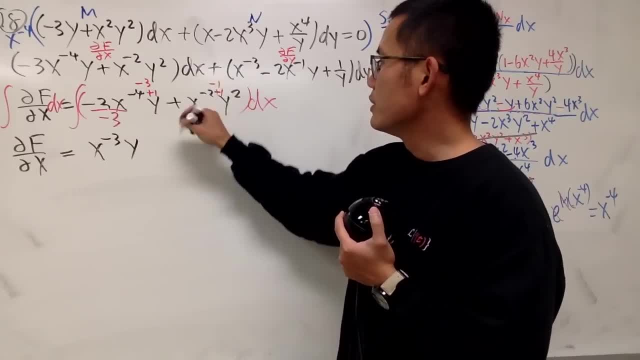 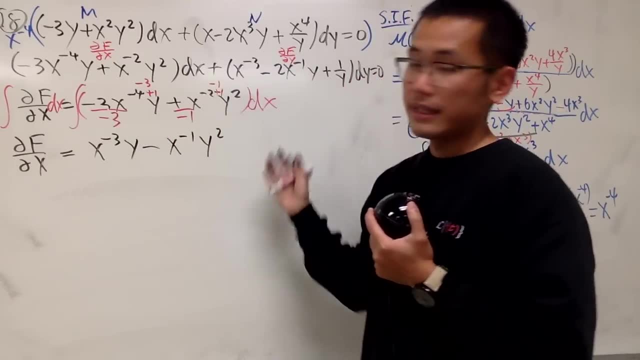 Next you do the same thing. You add 1,, which is negative 1.. You divide it by negative 1, so it becomes minus and you have x to the negative 1, power and y squared like that. But in the x world y is a constant. 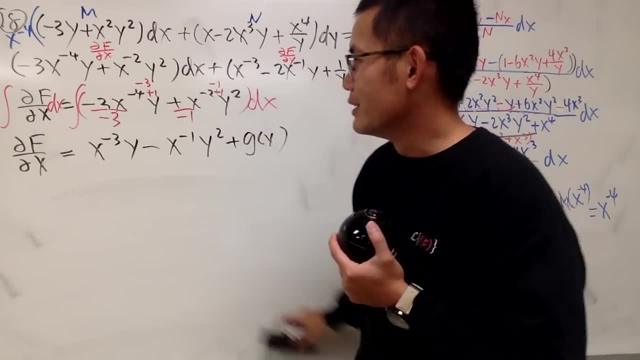 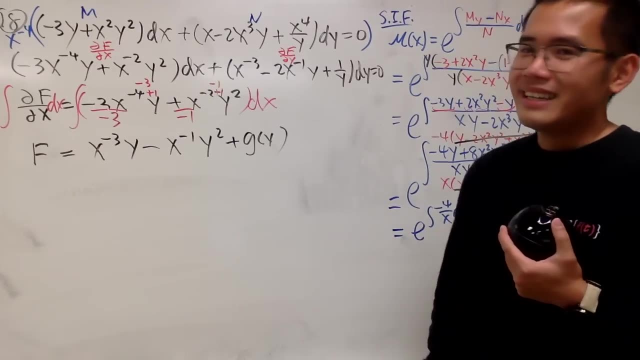 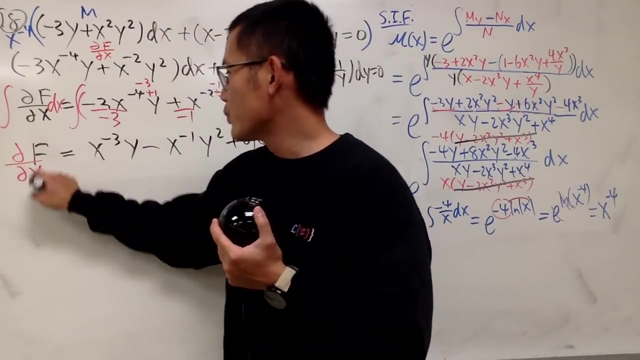 so you add g of y, Then, sorry, this right here should be just f, Integrate that. you just have f. I think I'm cursed with this question. I have so many mistakes. Okay, no time to complain. Differentiate this with respect to y. 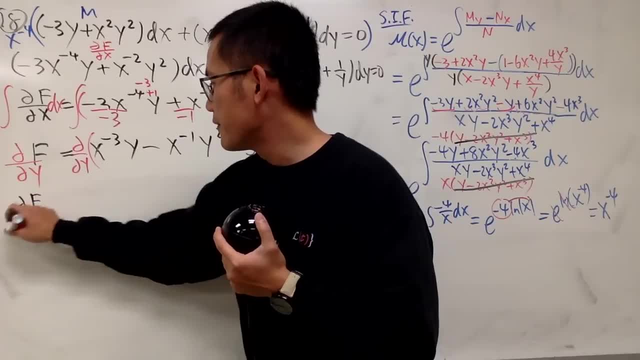 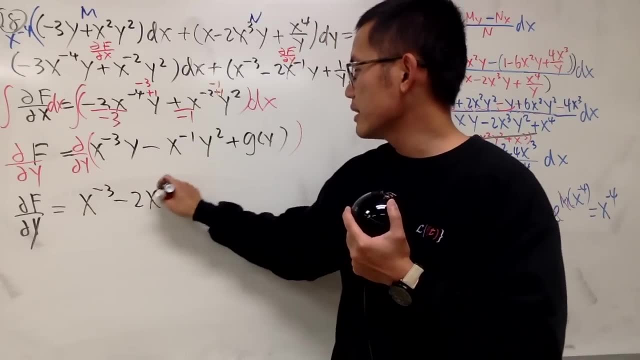 So when we do that, we get partial f with respect to y equals. do this: we get x to the negative 3.. Do that: we get minus 2x, negative 1, y to the first and then plus g prime of y. 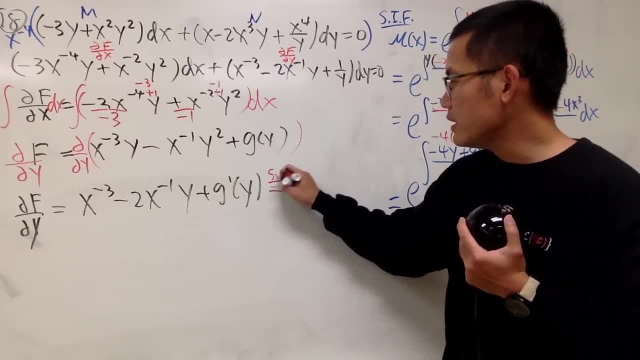 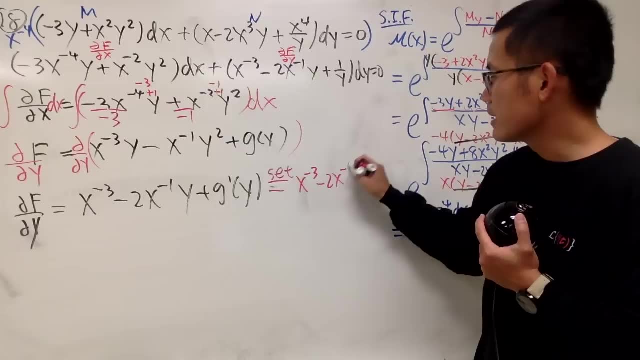 Then we are going to, we are going to set this to be the same as whatever we have right here. So, as you can see, x to the negative 3, minus 2x, negative 1, y, and then plus 1 over y. 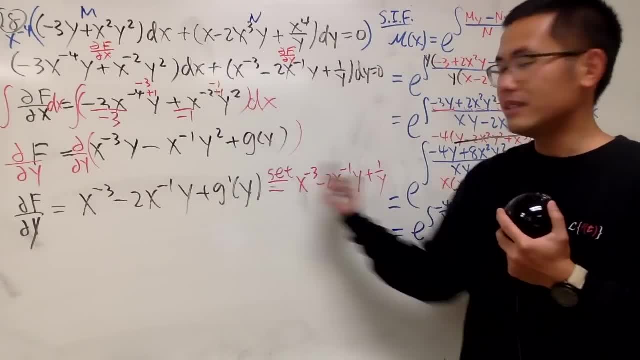 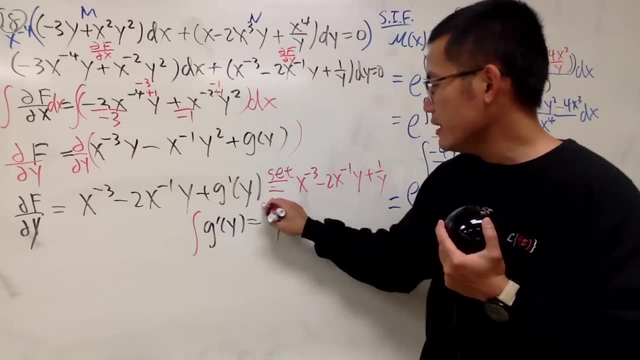 Have a look: This match, that match and this has to be the same as that. Therefore, we know g prime of y has to be 1 over y. Integrate, integrate with respect to y. So g as a function of y is just natural log of y. 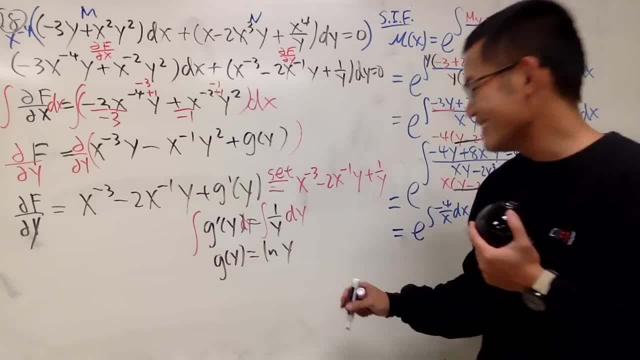 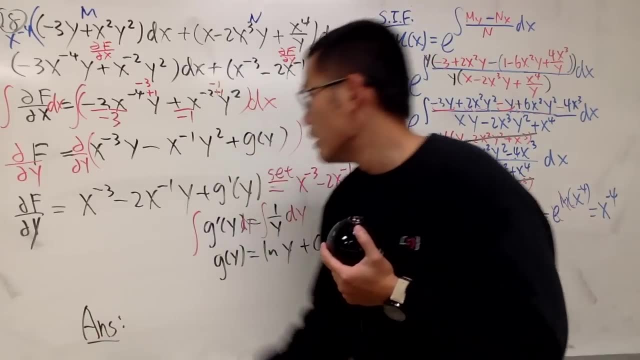 As we predicted. Well, how did I predict it? We created Plus a constant, if you wish, If you wish, Anyway, finally, I'll write down the answer for you guys. Final answer. I will just put this down right here for you guys. 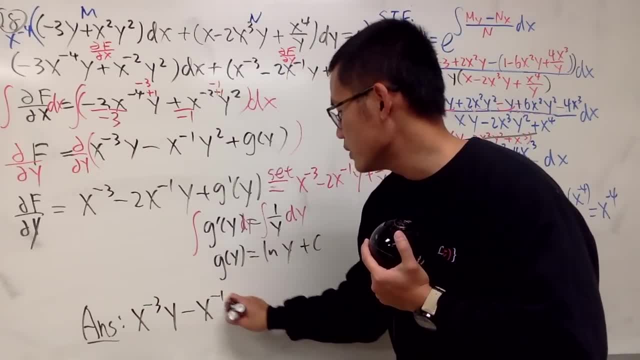 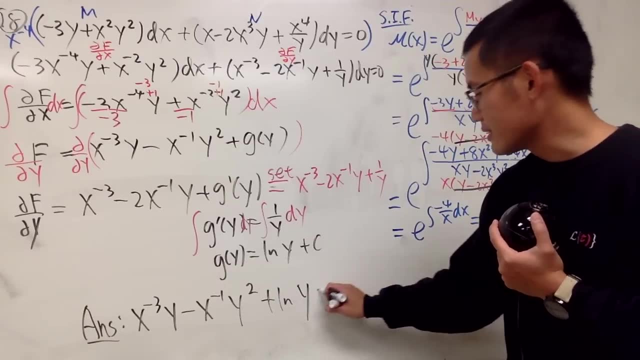 We have x negative 3, y minus x negative 1, y squared g, is that? so it's plus ln, y and I'll kick the c to the other side. So plus constant, like this, If you want to bring that to the bottom. 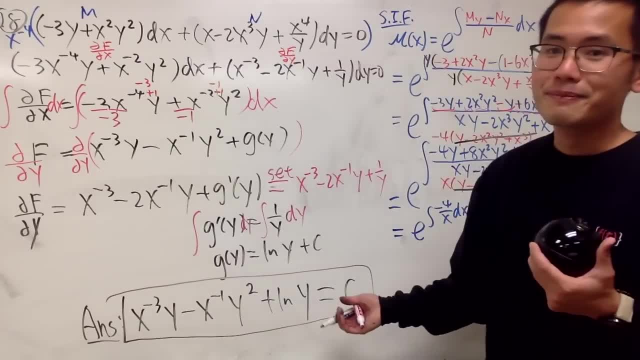 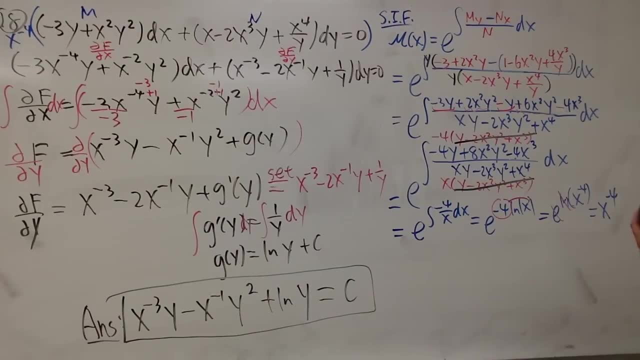 no, I'll leave that to you guys. That's it, Number 18,, number 18.. Have a look, I have a look. So yeah, Sometimes it happens to me too, even though I'm the creator of the equation, right. 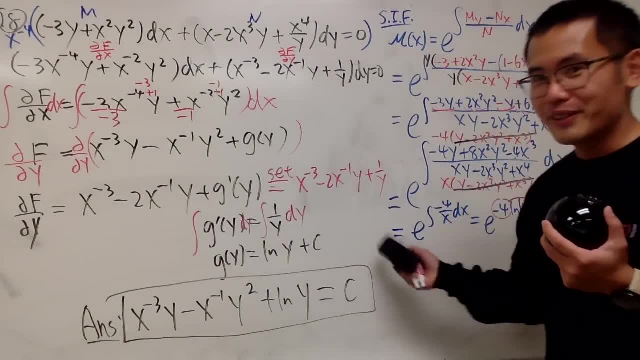 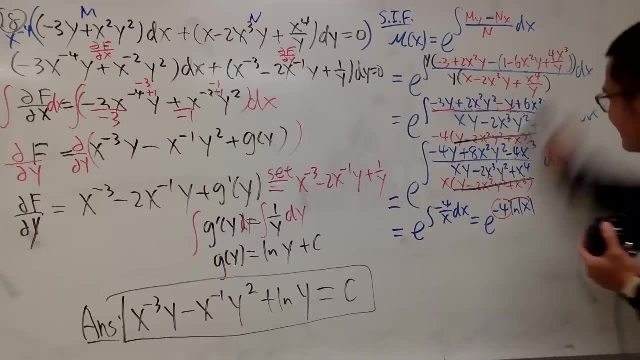 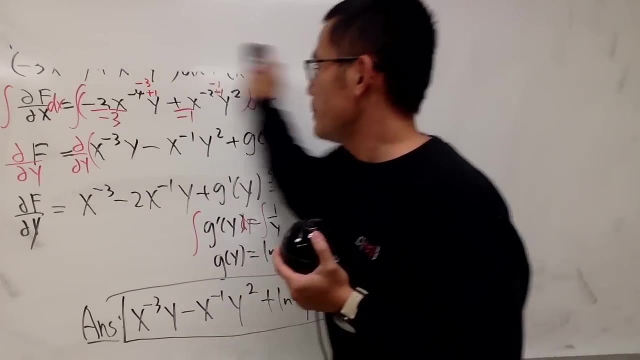 So don't feel discouraged that you cannot solve differential equations, because it's hard, It's not easy, Even though I created this equation, but I still messed up so many times, right, Okay, So not so bad, not so bad, not so bad. 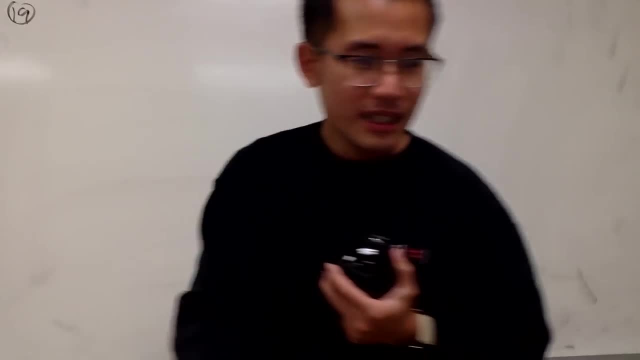 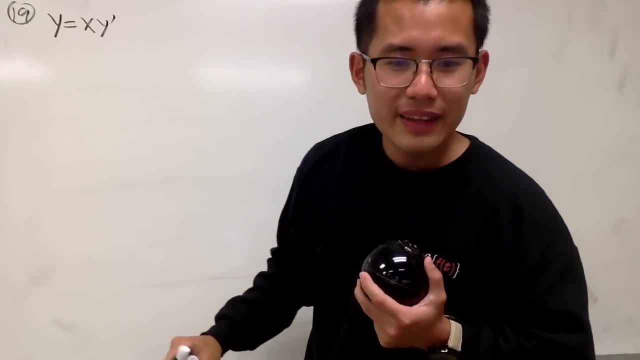 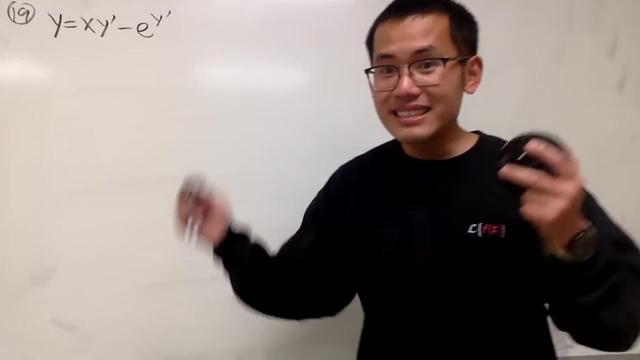 Number 19.. Finally, we're moving forward. Number 19.. y equals xy prime. Hmm, And then minus, yes, minus e to the y prime power. Yes, clear out again, right. So this is the get. 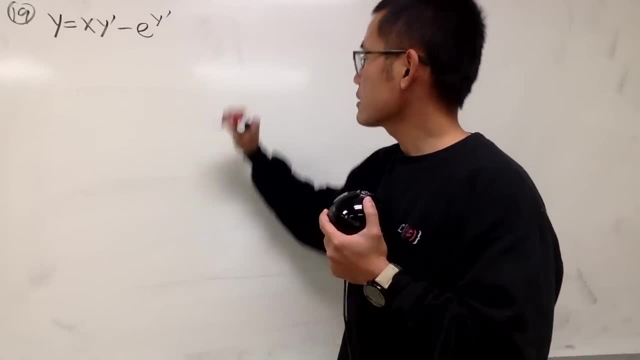 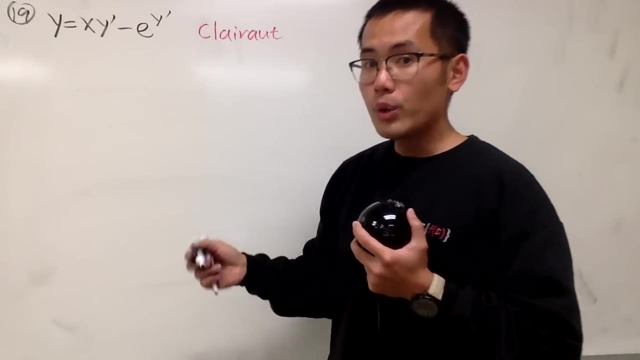 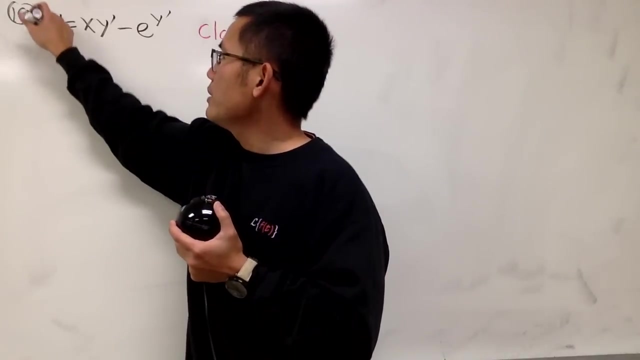 this is the clear out differential equation. So all we have to do is the following: Look at this. I'm not going to show you guys the parametric equation way to do it, but I'll just show you guys the usual way. 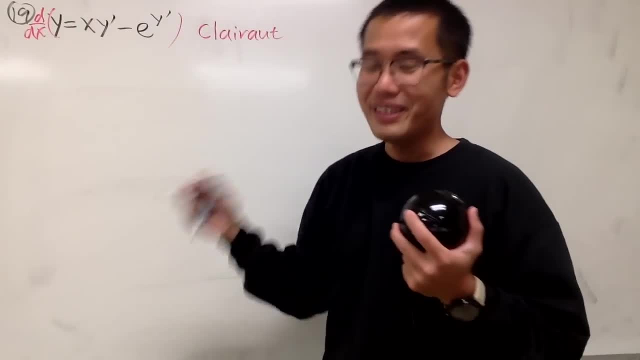 You can just go ahead and differentiate this. I know we have a differential equation, but I'm not going to show you guys the original equation already. but differentiate this anyway. Left-hand side: we get d no already as y prime. 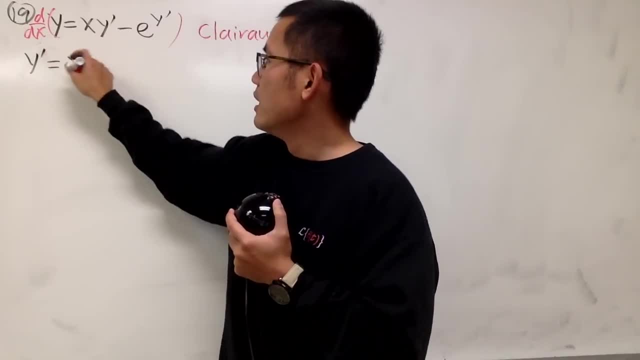 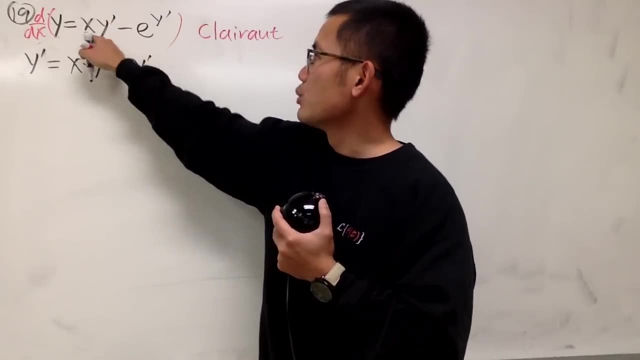 Left-hand side, we get y prime. that's equal to differentiating this. Keep the first function, differentiate the second, then that will give us y double prime plus this function, which is y prime times d, derivative of the first. 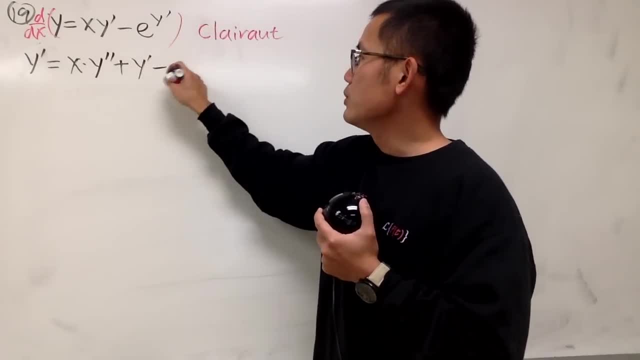 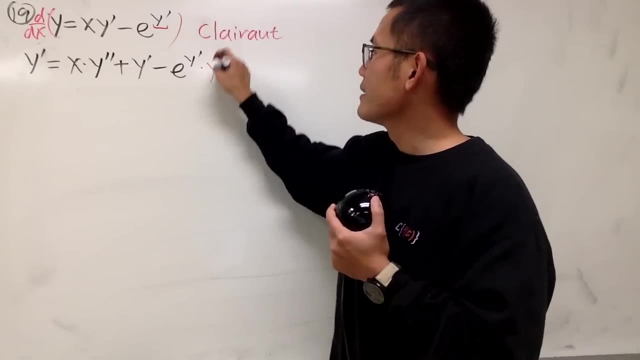 which is 1, doesn't matter. Then. derivative of this is just e to the negative y prime. and use the Chengdu right Chengdu says: multiply by the derivative of this, which is y, double prime, Like that. 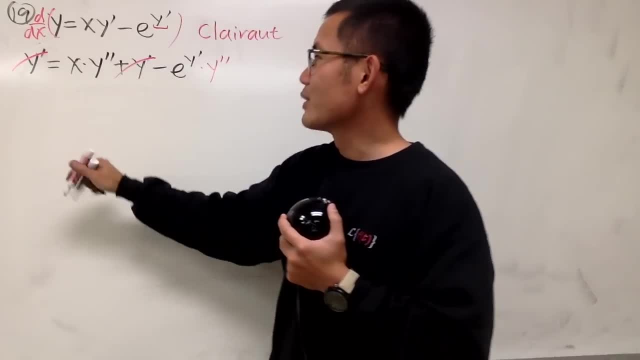 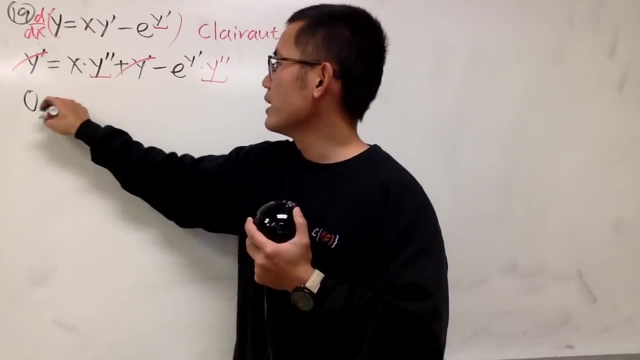 Now you see that this and that cancel nicely, so you have a 0. Good. And then we have y prime here, y double prime here, y double prime here. so we can look at this as parentheses: x minus e to the y prime. 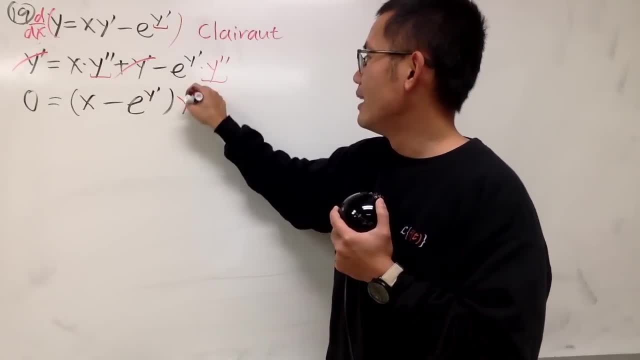 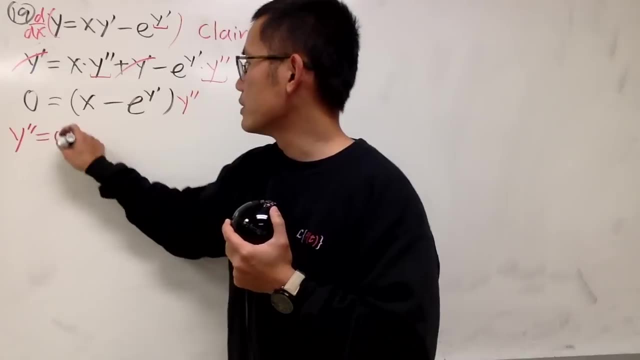 and then we have the y double prime right here Now two choices. First choice is when we have y double prime is equal to 0, or the second choice is when we have x minus e, y prime is equal to 0.. 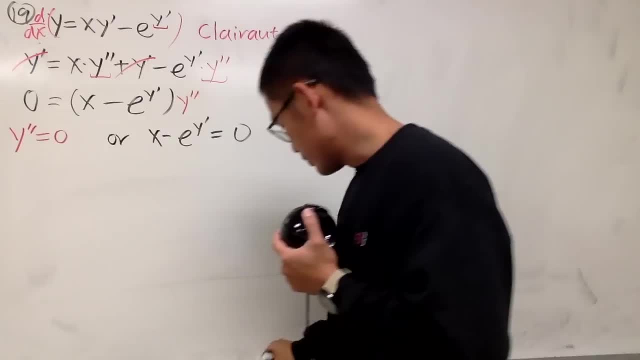 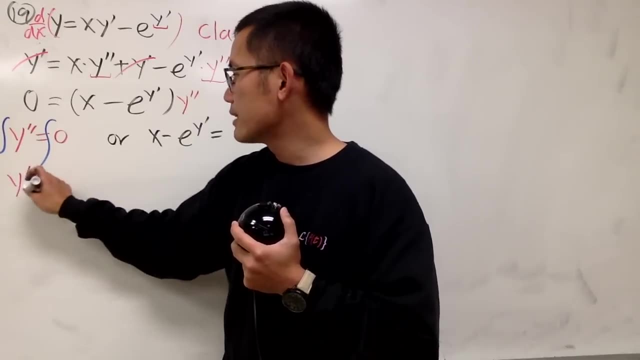 For this: go ahead, integrate that, and perhaps I'll do this in blue: Integrate, integrate. we know y prime has to be a constant, but keep in mind when you are doing the clear-out differential equation: do not integrate again. 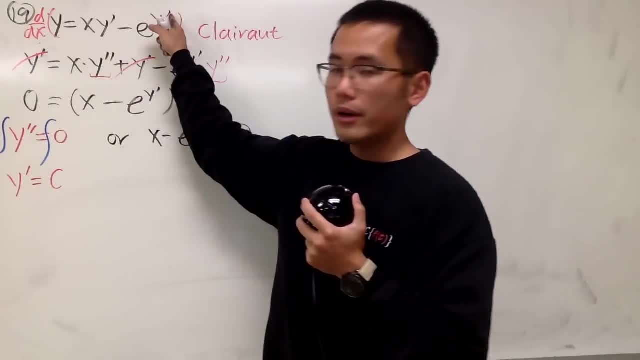 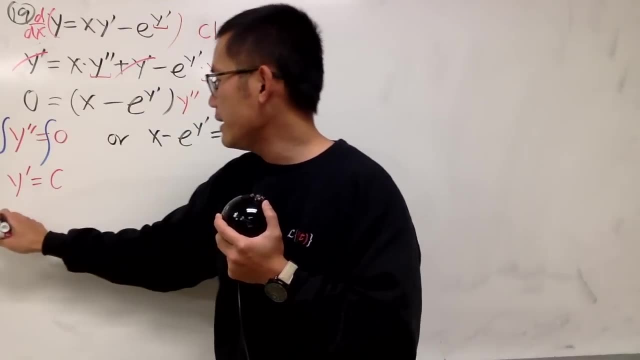 All you have to do is put a c here and here, because y is based on the y prime. You have the y prime already, so you actually know that y is equal to put a c in here, so it's cx. 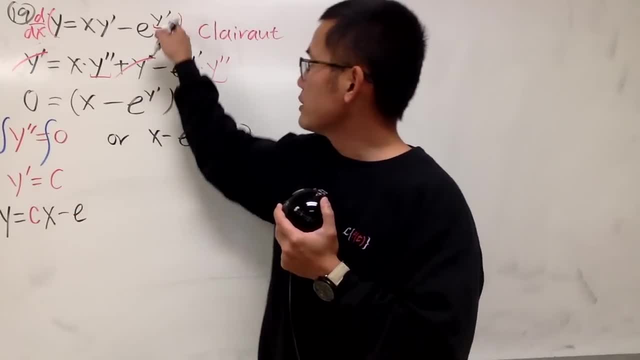 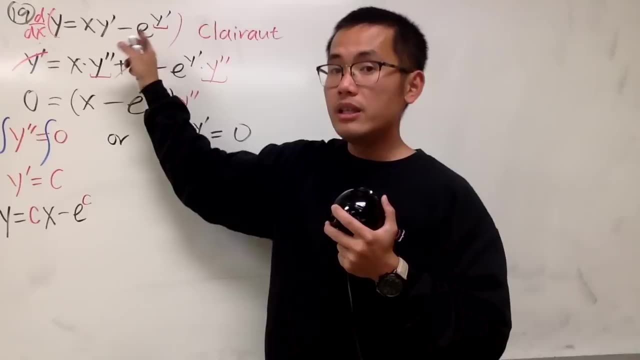 and then you have minus e raised to the c's power, like that, And do not write this as another constant. Don't do that because originally it's just the first order, so just keep this as how it is right. So that's the first part. 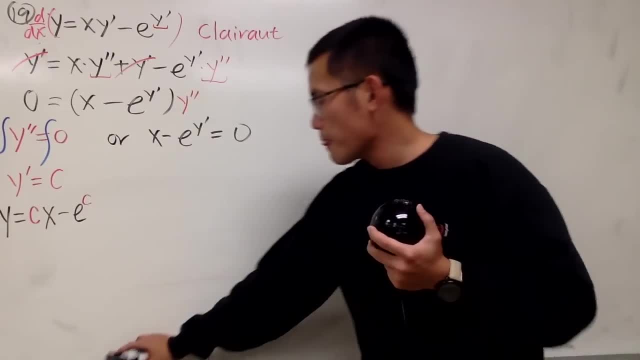 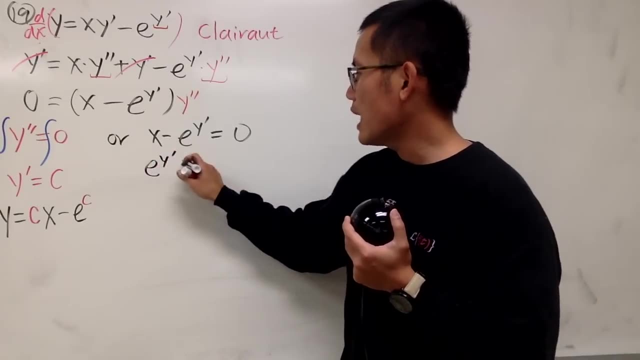 Now for the second part. Of course, to integrate this, we should isolate the y prime. To do so, I will just move this to the other side. In another word, ey prime is equal to x, ln, both sides, yeah. 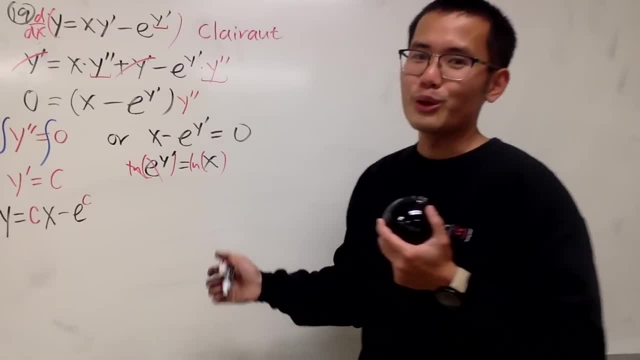 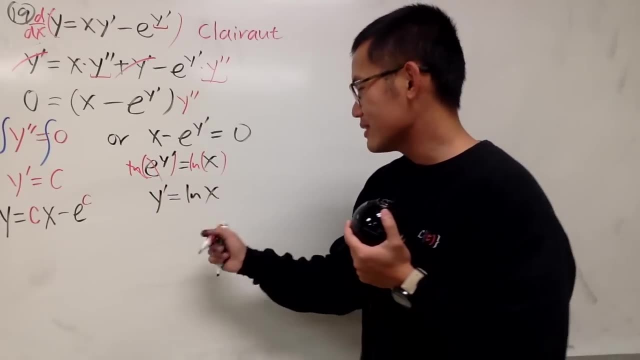 It's pretty fun because we're doing tons of algebra in differential equations and also tons of calculus in differential equations. very fun: y prime is equal to ln- x. How do we get this? Well, integrate both sides with respect to x. 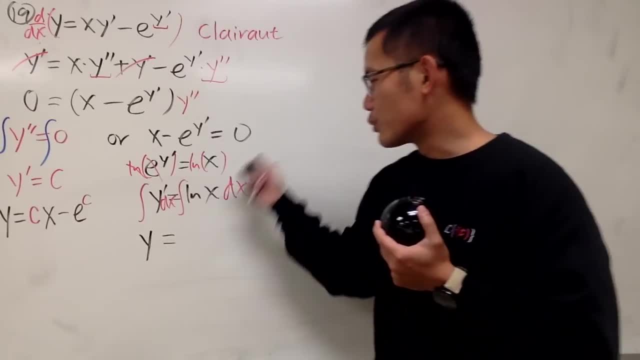 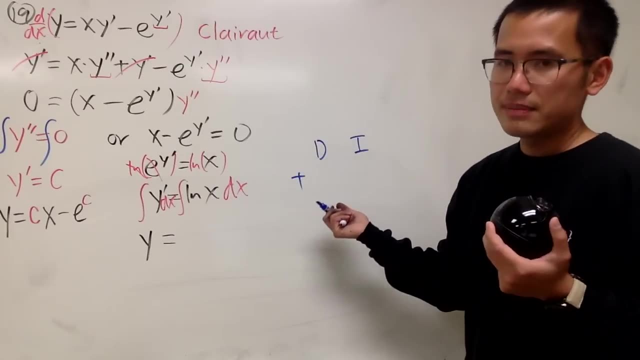 So we get y. and what's the integral of ln x? Well, let's just do it real quick. The i method it's x, ln x minus x, But I'll show you guys. anyway, This is ln x integrate 1.. 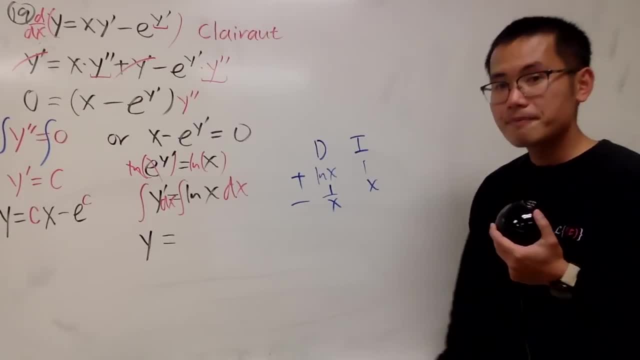 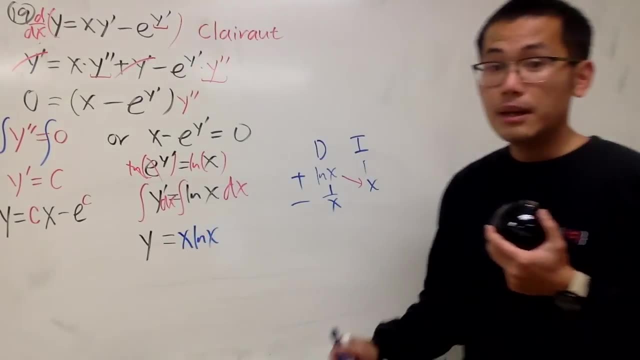 Integrating 1,, we get x. Differentiate this: we get 1 over x. First part of the answer is this and that. So we have x, ln x. But don't forget, you still have to have an integral when you multiply a row. 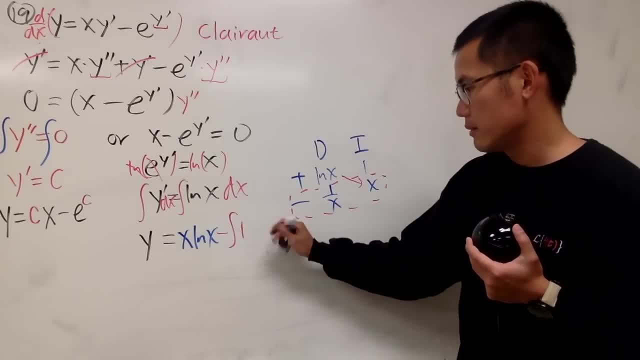 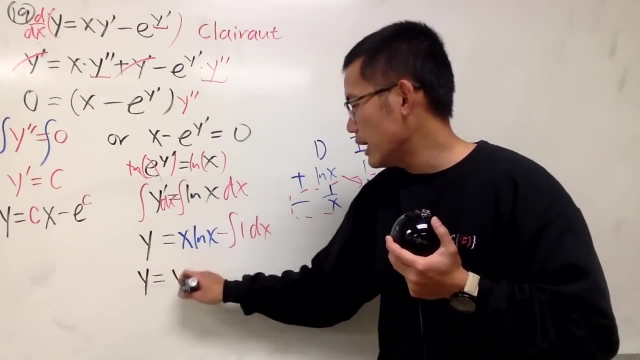 Minus integral. this times this you have to integrate 1 in the x world. This times this is 1.. So you can see that the answer is y equals x, ln, x minus x. Do you need to put down the plus c? 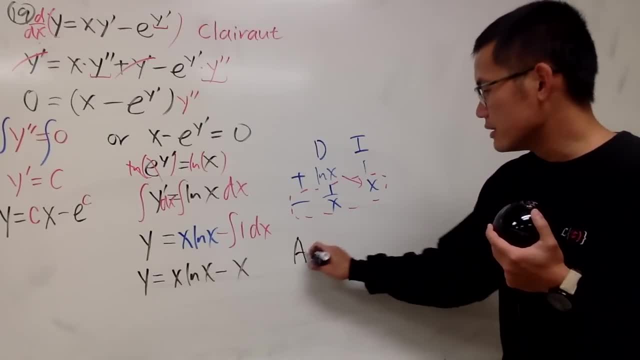 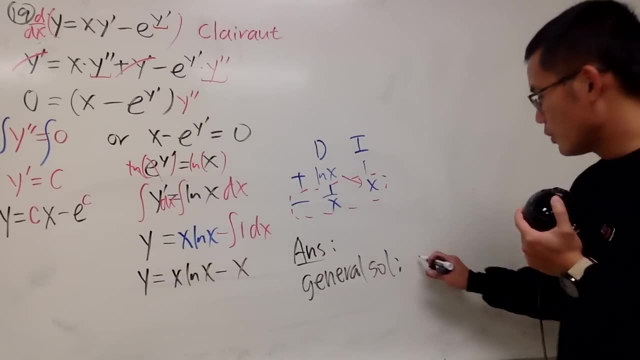 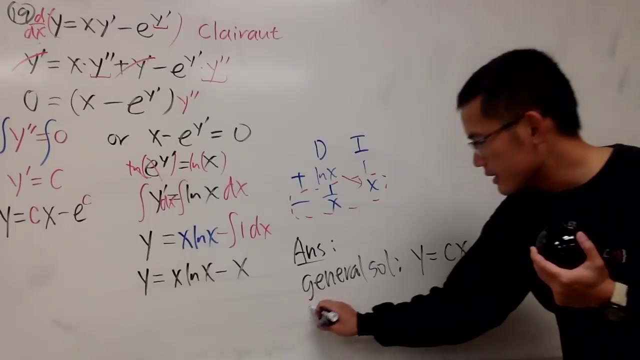 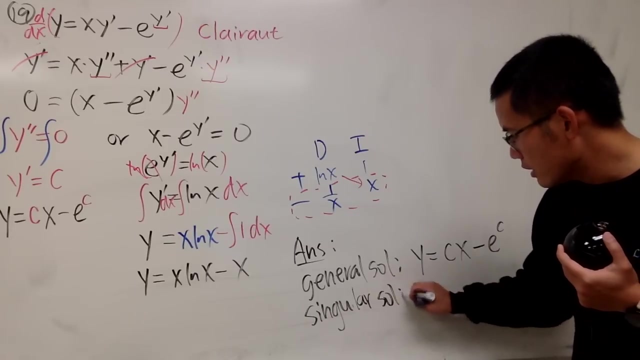 No, you don't have to. Here is the answer. This is how you answer it. You write it down. The general solution is that y equals cx minus e to the c's power, and then the singular solution is that: And for the singular solution. 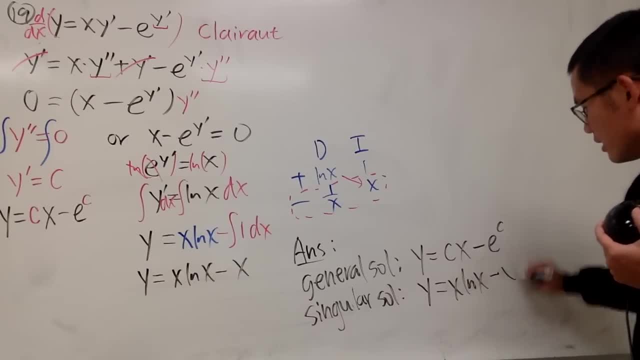 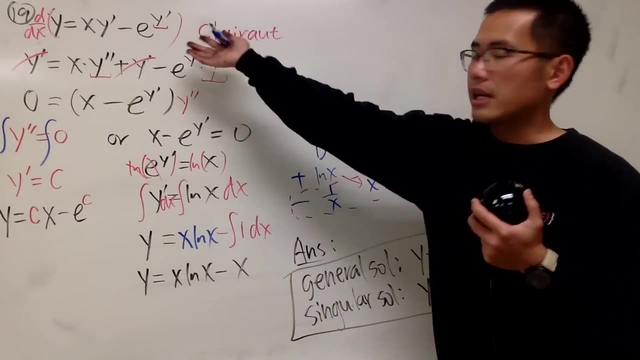 do not write the plus c or plus k. In fact, the constant will be 0, guaranteed. If you have the plus constant, plug it into the original. it will be 0.. So this is it, And the cool thing is that. 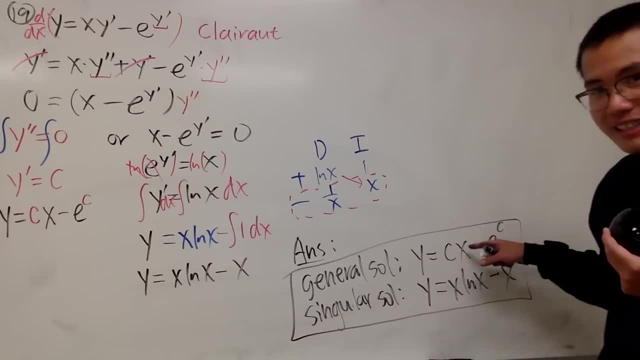 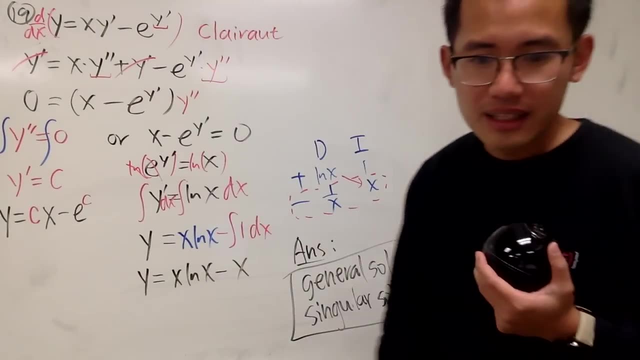 if you graph this and graph that, you can see that this is just a bunch of lines and the lines will be tangent to this curve. Right here, Very cool stuff, Right? So number 19. Done All right, All right. 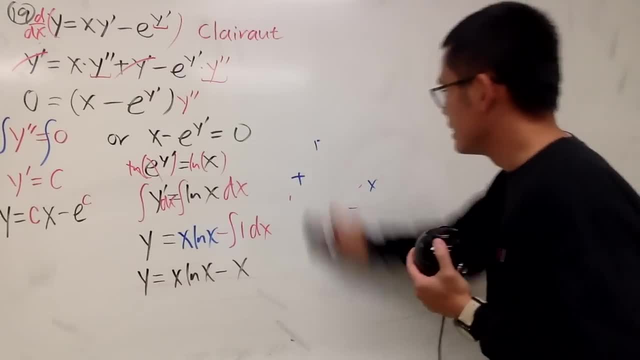 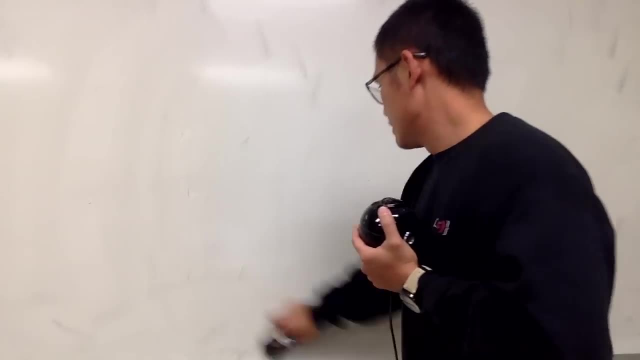 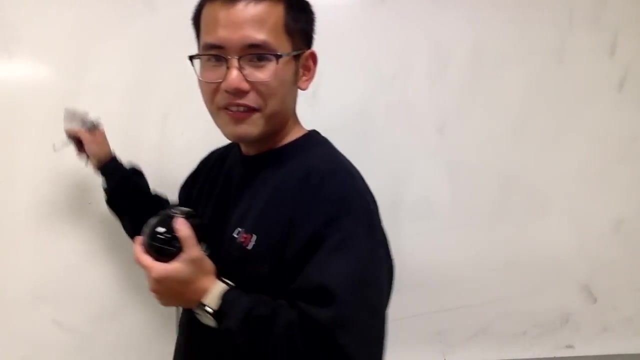 All right, Very good, Very good, The 20, and then just 5 more to go. Thankfully, I'm not doing the 100 differential equations, So I'm doing the 100 differential equations seriously. man And 2x. 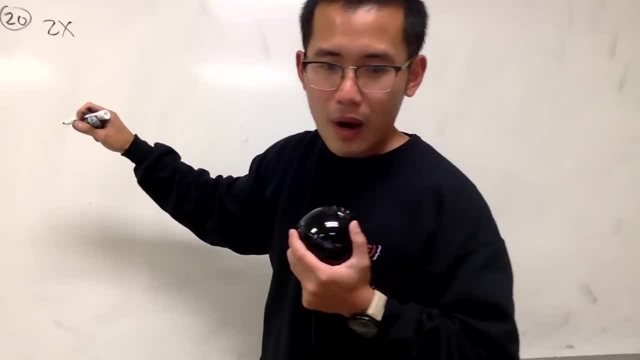 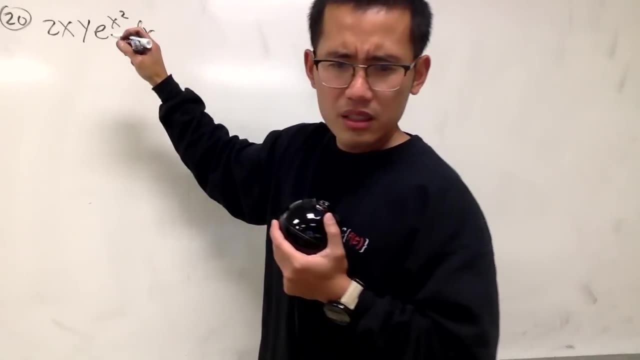 and then we have y, e x squared, and then we have dx, and then plus e x squared and minus 1 over y, and then dx. that's equal to 0.. Hmm, Looks like an exact, doesn't it? 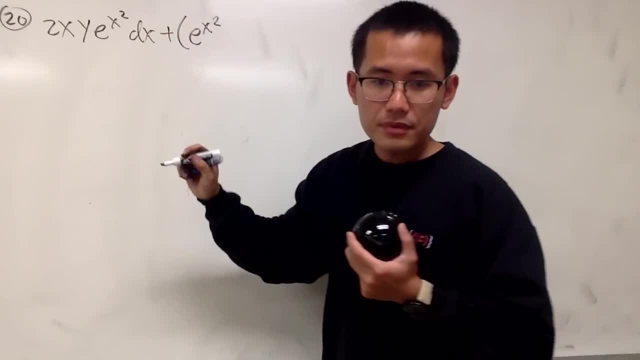 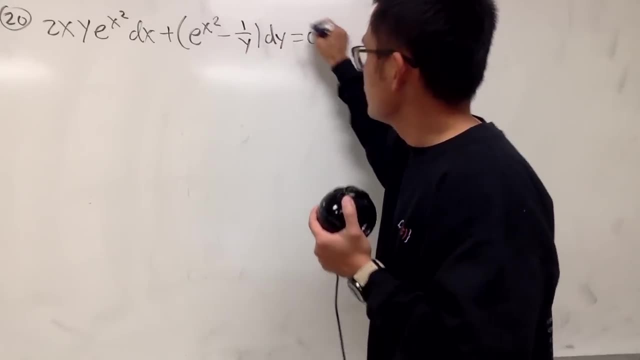 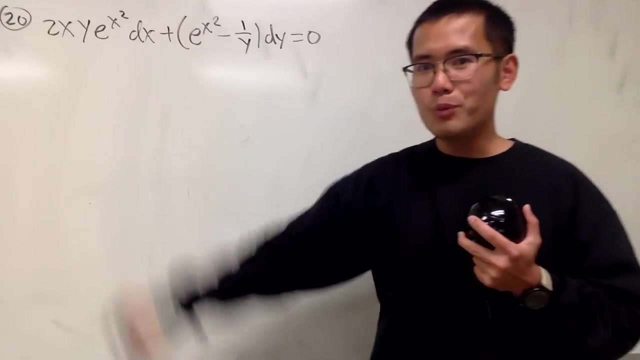 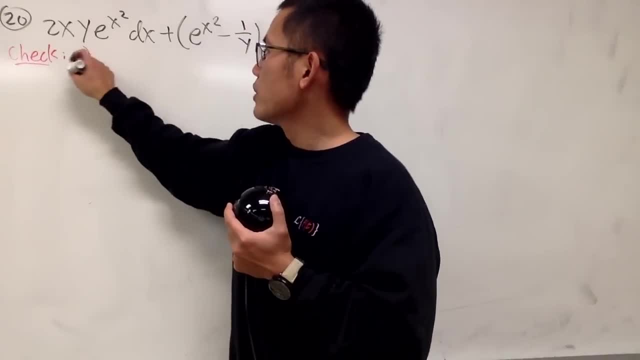 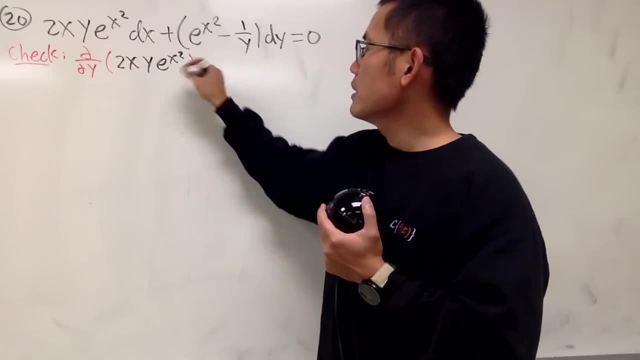 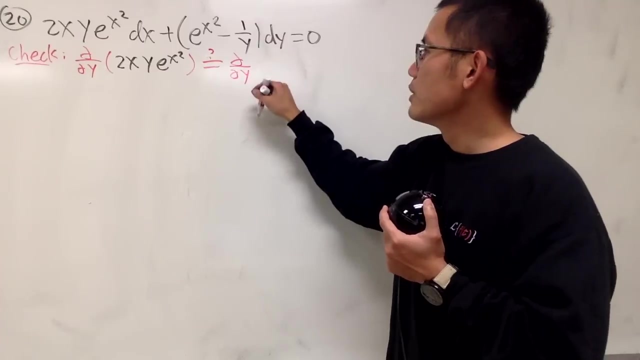 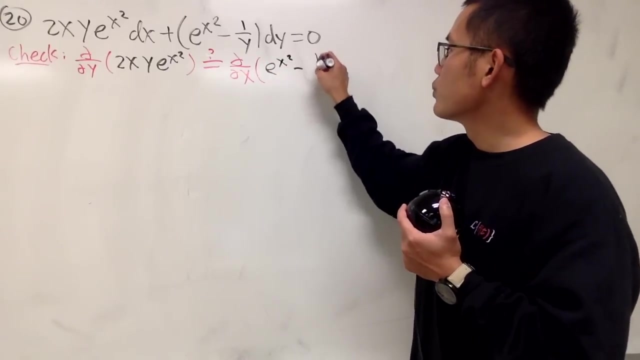 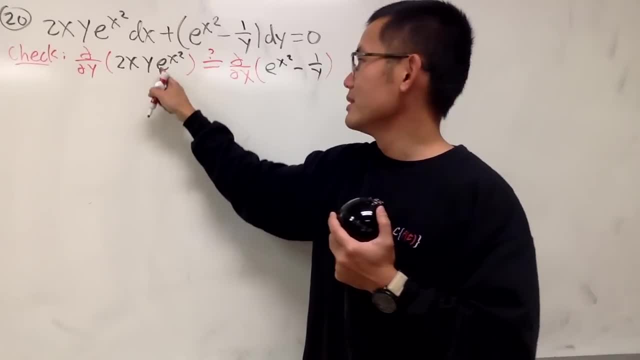 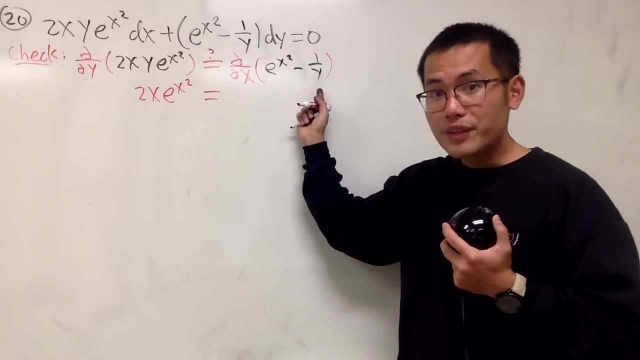 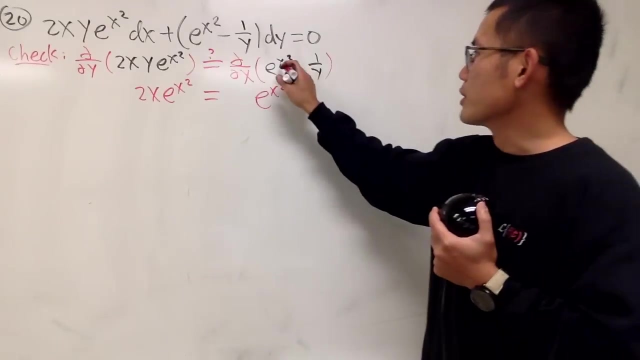 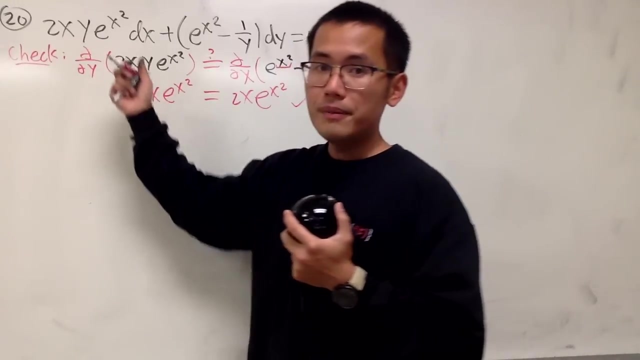 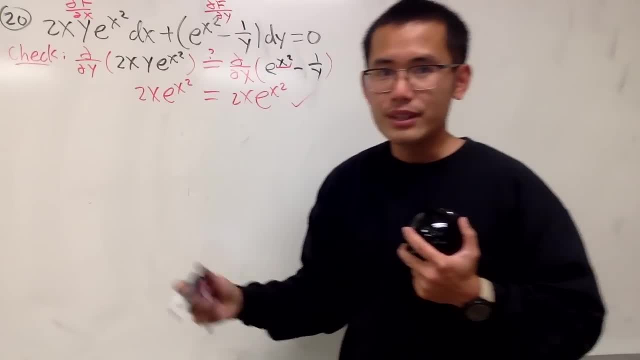 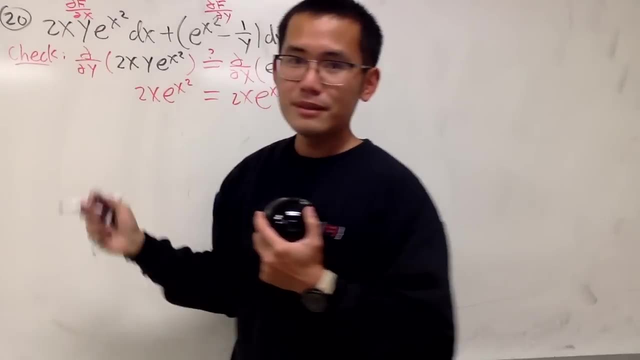 partial of f with respect to y. So let's go ahead and work that out. This right here. the f should be more feasible for you guys. Better, Yes, Okay. so now of course, you do the same thing, So we 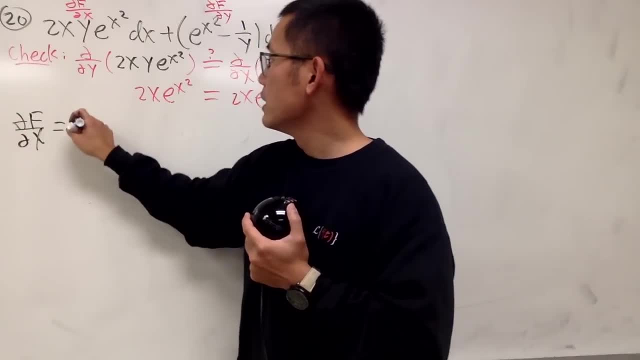 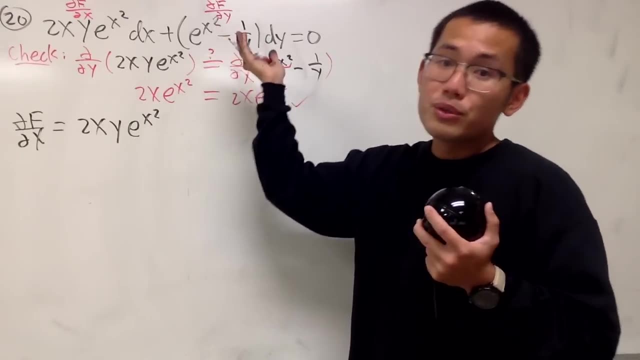 have partial f with respect to x equals 2xy e, x squared. And again, if you want to start with this, it's okay, too up to you. It's actually easier if you do it this way, but I will do it. 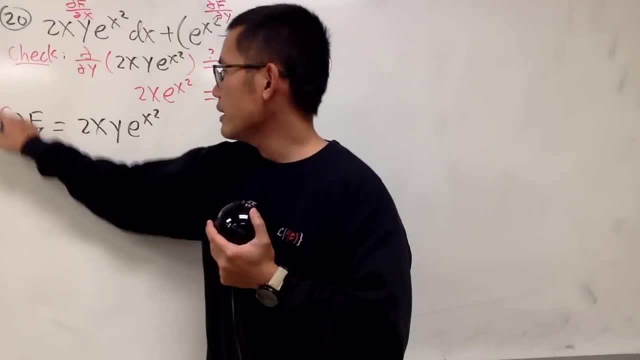 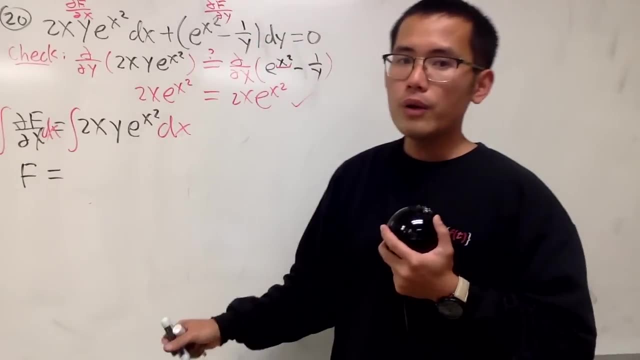 I wrote it down already, so All right. so integrate. integrate in the x world, So we get capital F equals well. y is just a constant multiple. that's good. and notice that the derivative of x squared is the derivative of x squared, So we get capital F equals well. 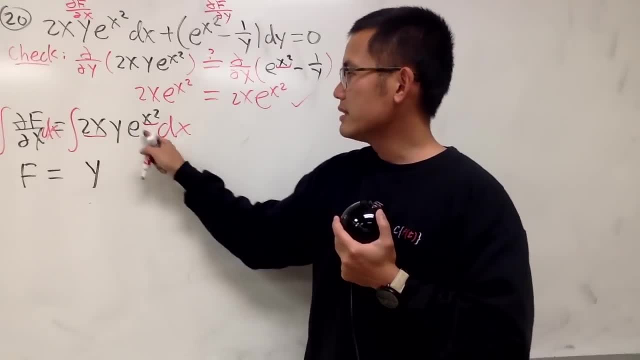 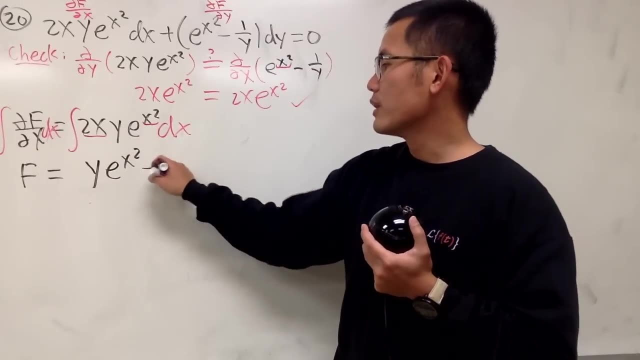 it's precisely 2x, So the integral of this, and that is nicely equal to e, to the x squared power, just like that, And that's it. And of course we have to add a function in terms of y, so g of y. 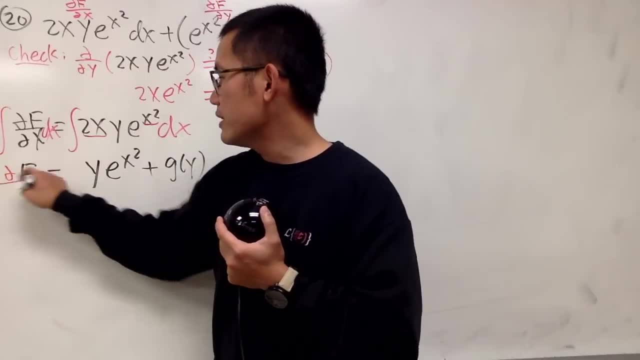 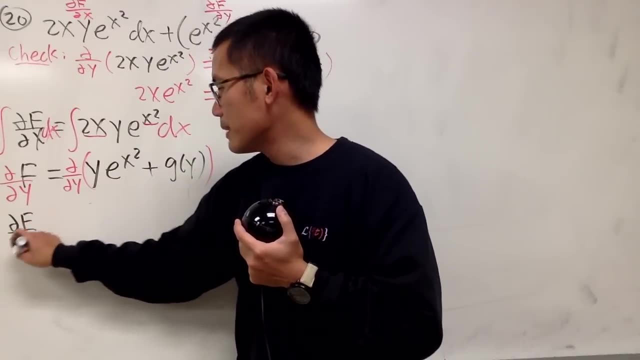 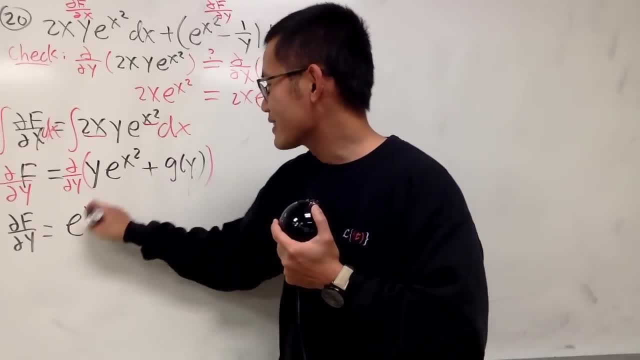 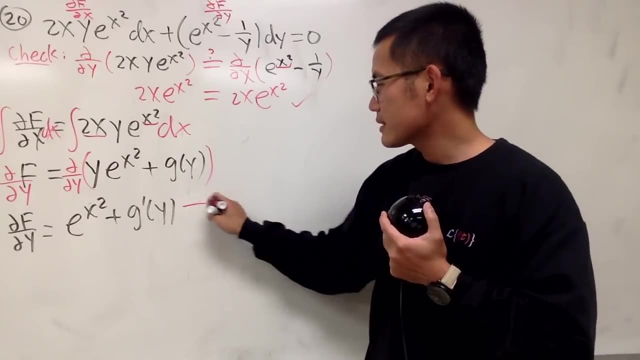 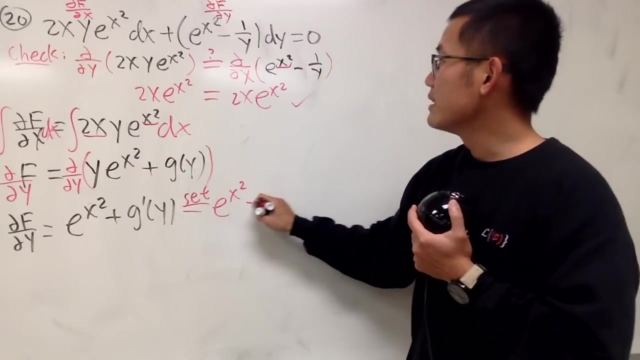 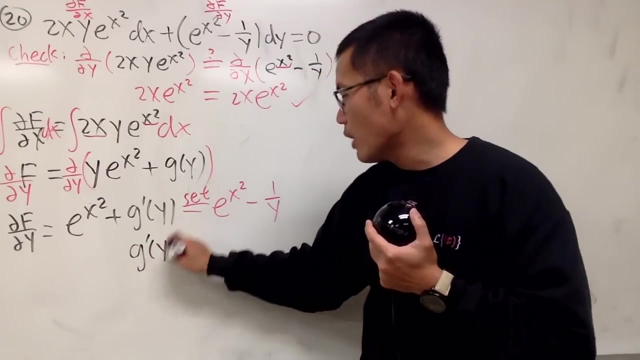 do this with respect to y, we get e x squared plus. derivative of this is g prime of y. that's equal to well, I have to set. I have to set this equal to that which is e x squared minus 1 over y. yeah, Same same. So we know g prime of y is equal to negative 1 over y. 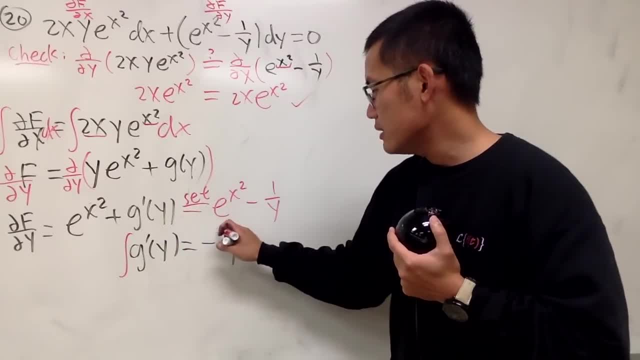 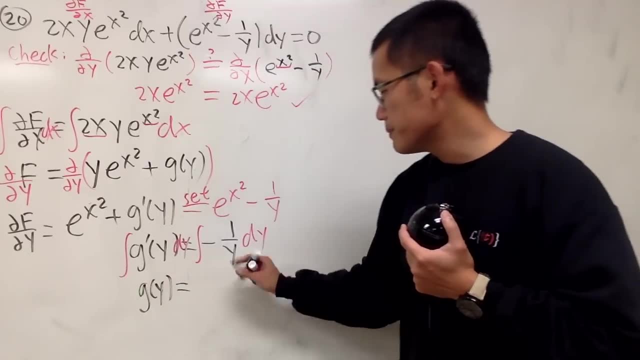 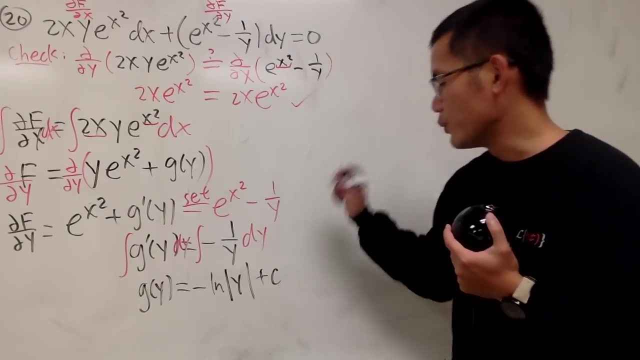 and then, of course, integrate both sides. let me just integrate this right here, and then dy, dy. so we know our function g of y is equal to negative ln absolute value of y, like this, Finally, or plus c, if you wish. 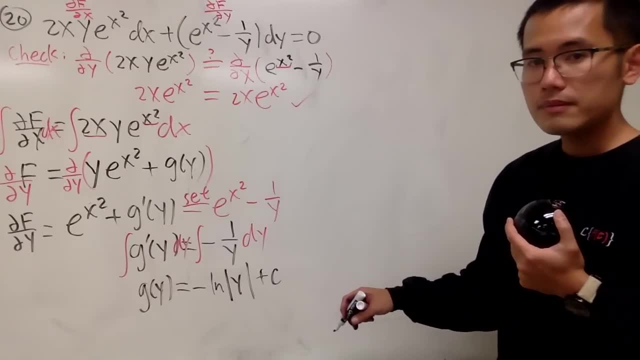 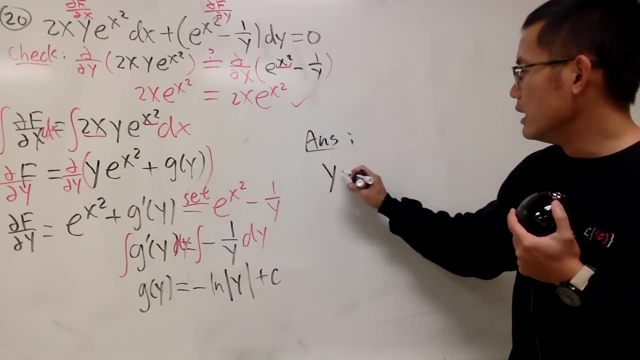 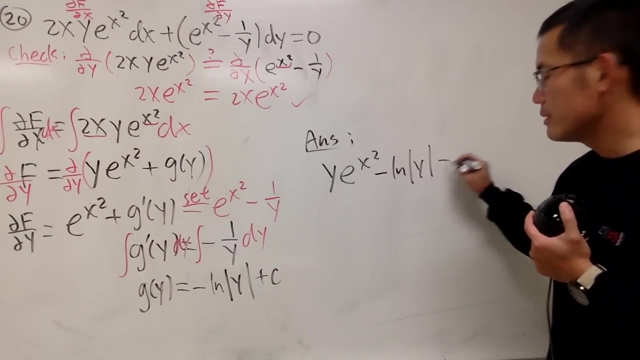 doesn't really matter at the end right here, I'll put it down here. Answer. This is my function. part y: e, x squared this right here is that? so we have minus ln absolute value of y and then put the c to the other side and we are done. 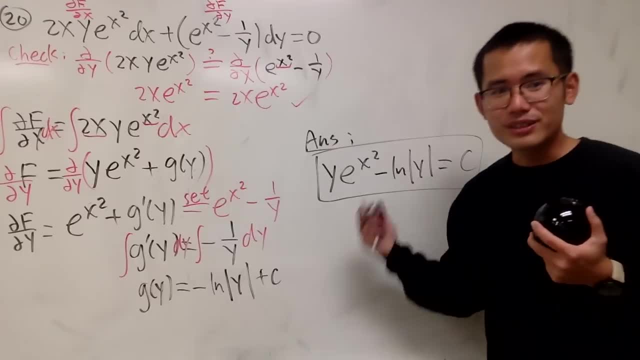 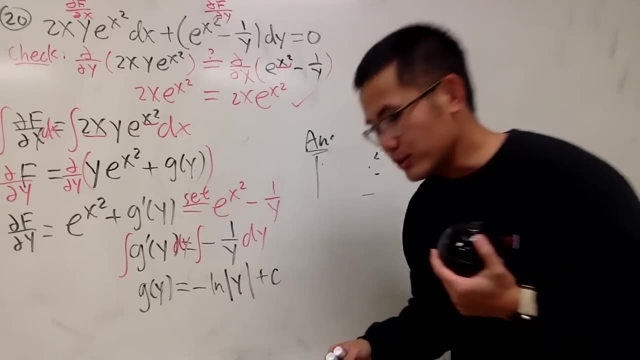 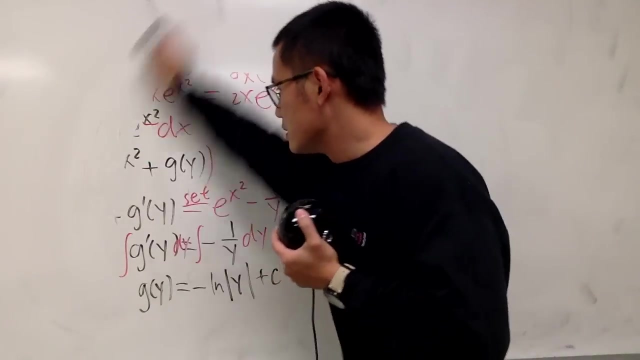 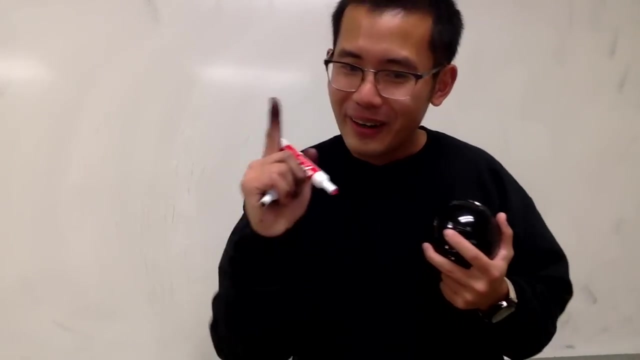 Just like that, Right. So just like that, All right. so number 20 done. I should go pick out the cap, but oh well, Okay, Okay, Okay, Okay. Now here are the fun ones. right, Here are the fun ones. 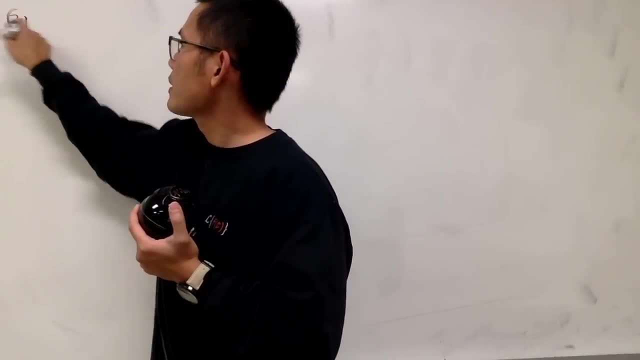 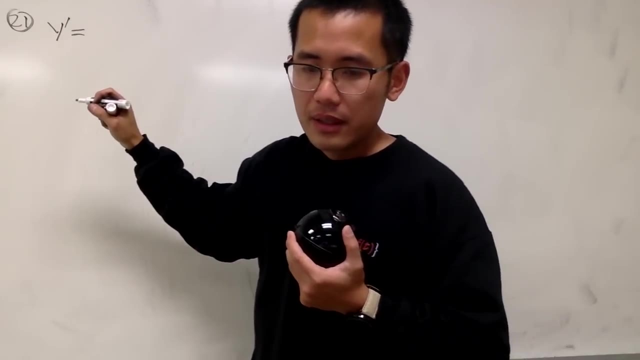 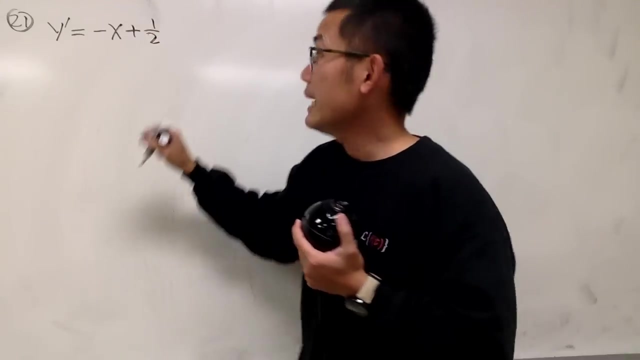 Number 21.. Just a couple more to go. Number 21. We have y prime that's equal to, and we have negative x plus 1 over 2, and then we have x on the bottom, okay, And then y, That's it, And then y of 1 will keep the sum okay. 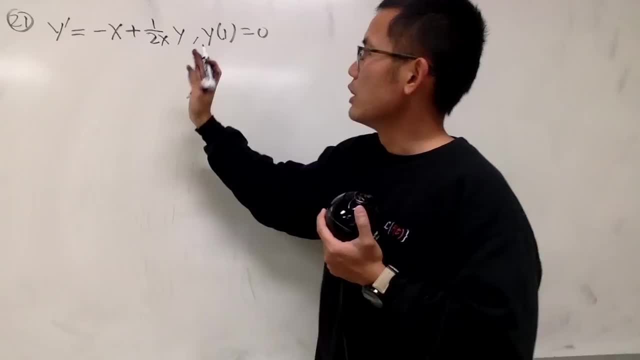 That's it. And then y of 1 will keep the sum. okay, We will just have to multiply that in order to see the answer give you 0.. So this is the one we have and you can have a little preview. The one next: 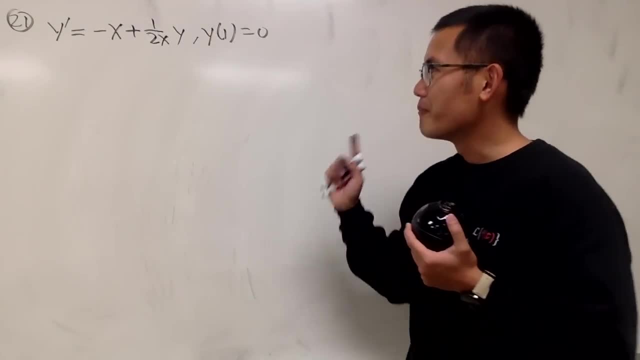 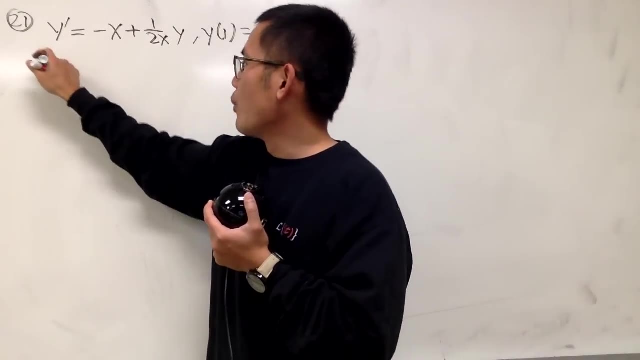 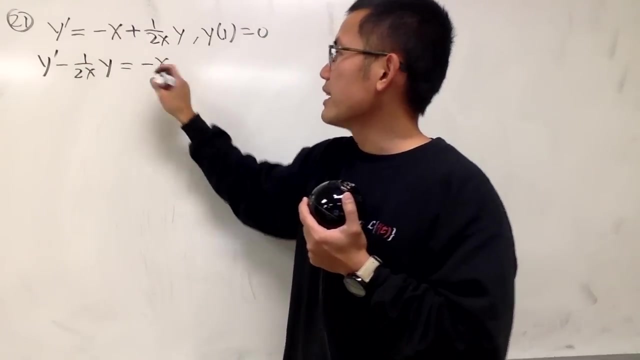 to it. we add a y squared after that. Very cool stuff. So now this is so linear, isn't it? Bring this to the other side first. So here we have y prime, and we can write it as minus 1 over 2x, and then we have y, and that's equal to negative x. Very good stuff. 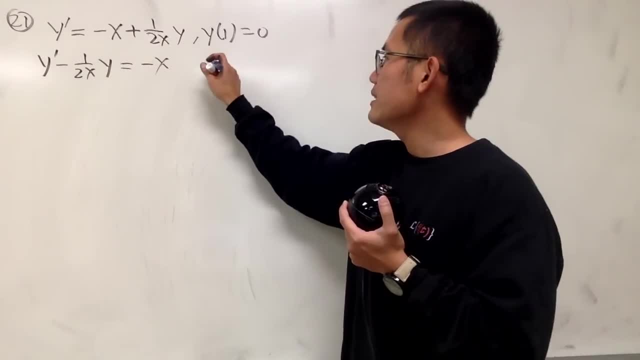 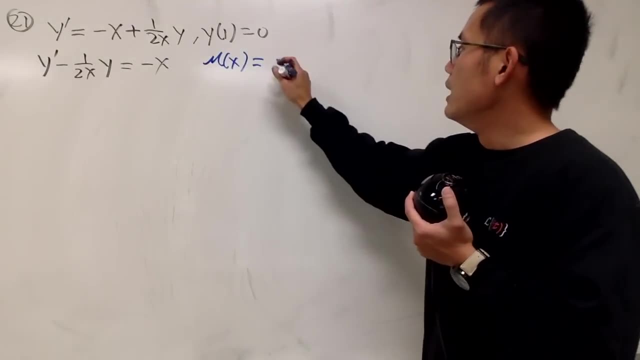 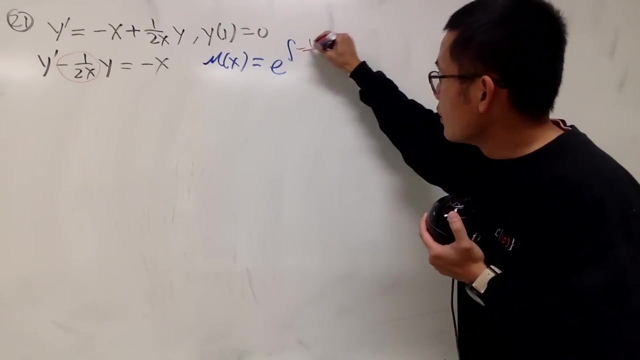 Now let's do the integrating factor on this side, mu of x For the linear integrating factor. it's much easier. It's going to be e, integral power, and then we have this. don't forget the negative, though, which is negative 1 over 2x right here, And that will give. 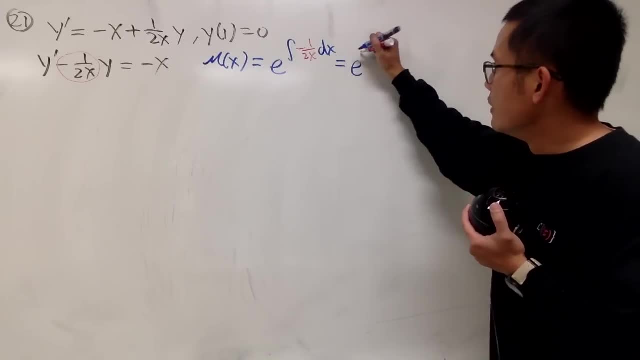 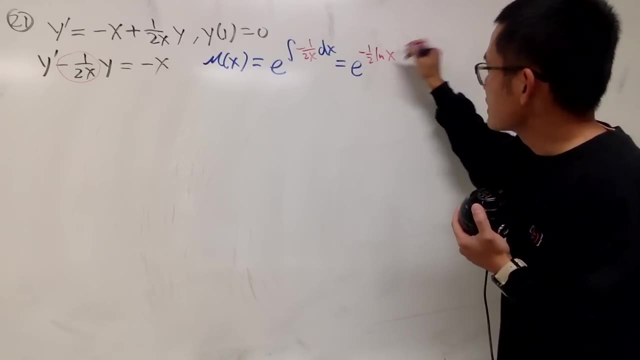 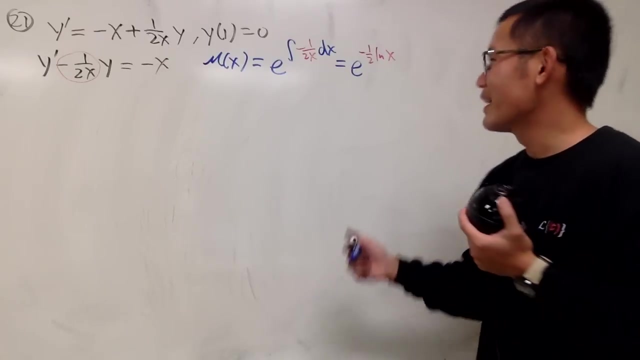 us this negative 1 half state. so we have e negative 1 half, and then, of course, you integrate that which is ln, x. Don't really worry about the plus c, alright, So just go ahead. and I mean, don't worry about the absolute value. Anyway, put this right here so you 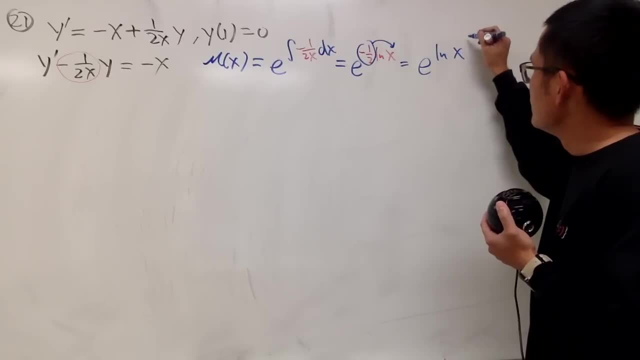 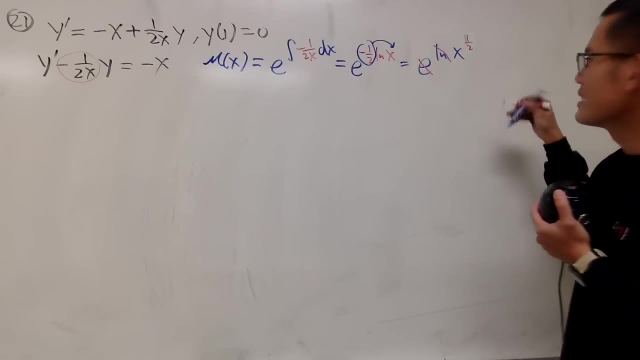 can see. this is e ln. x to the 1 half power should be in red, But anyway, cancel. So finally you get x to the 1 half power. Wow, Do you want to write it as square root? No, x to the 1 half power is much better. 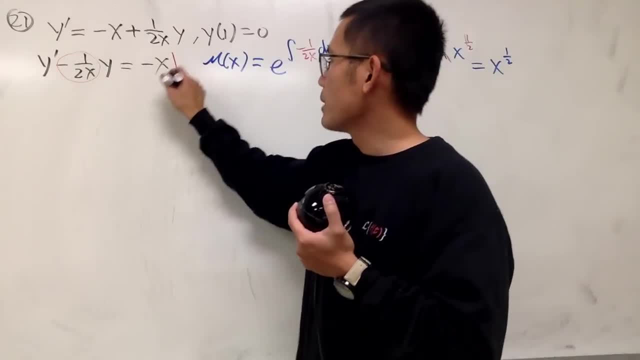 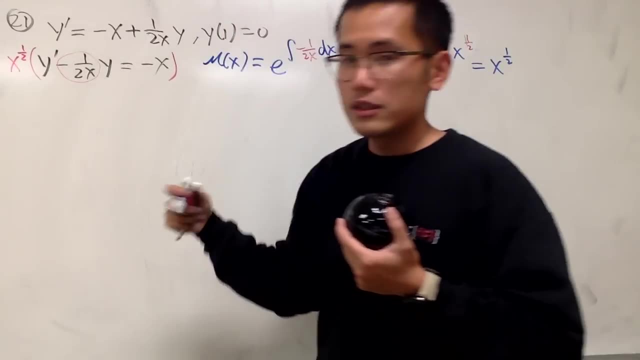 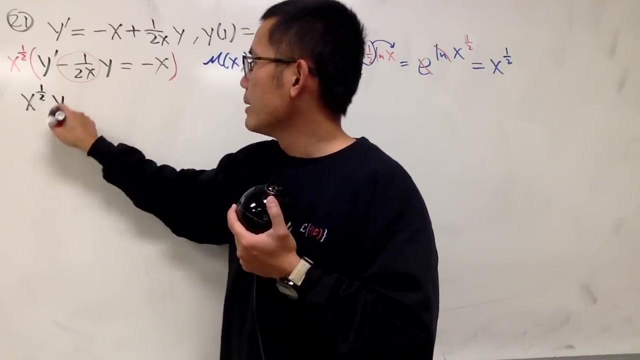 So this right here is the integrating factor. I will come here and multiply everybody by x to the 1 half power. Let's put it down in the front. So go ahead and work that out. We will get the following: x to the 1 half power, y prime- This times that is minus 1. 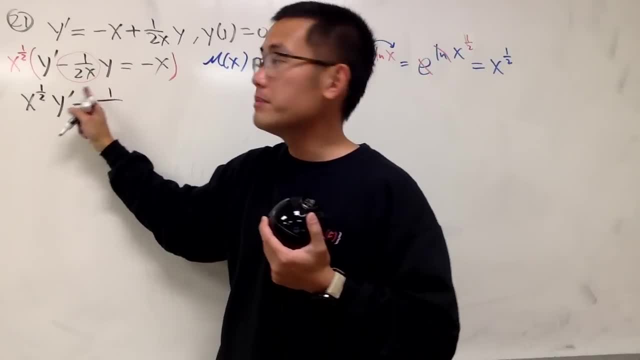 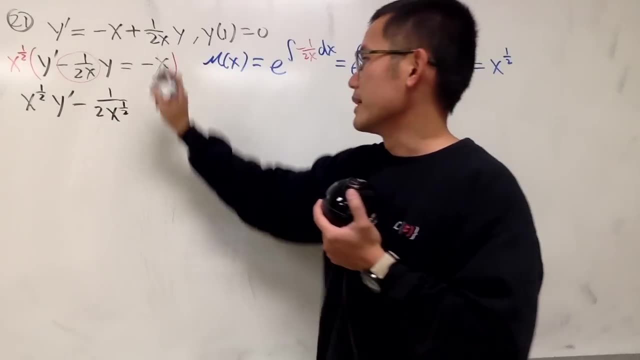 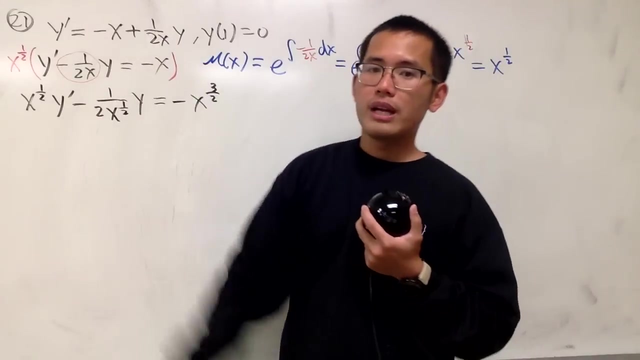 over 2.. And this is x to the 1 power on the bottom, 1 half on the top. so we can reduce: is x to the 1 half power on the bottom. Just do the algebra. I know that y that's equal to minus this and that is x to the 3 half power. 1 plus 1 half is 3. 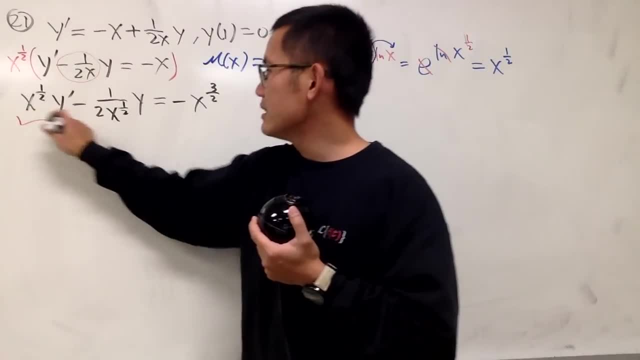 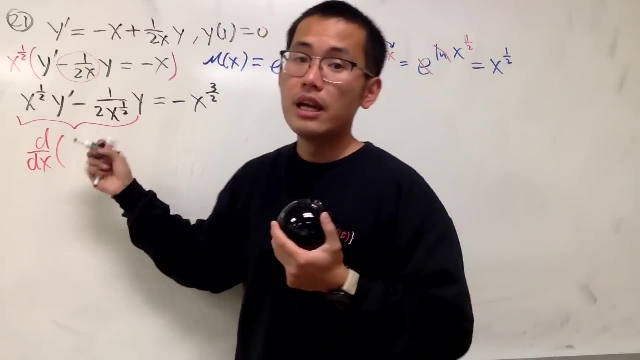 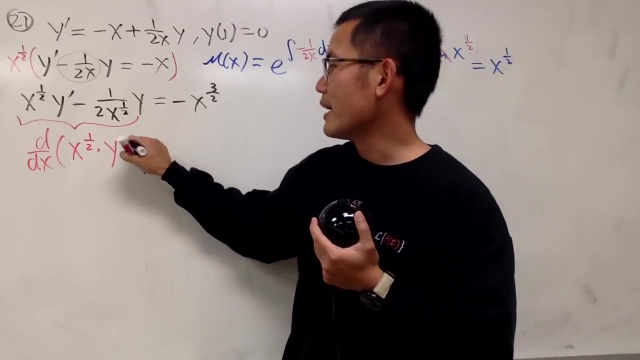 half. That's what we have. Yes, the left-hand side is still a very nice derivative. yeah, Is the derivative of a product of two functions And of course, that will always be the integrating factor, which is x to the 1 half power, and the second function is the y guaranteed. 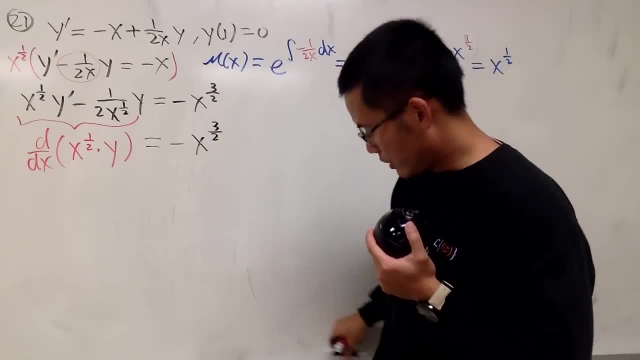 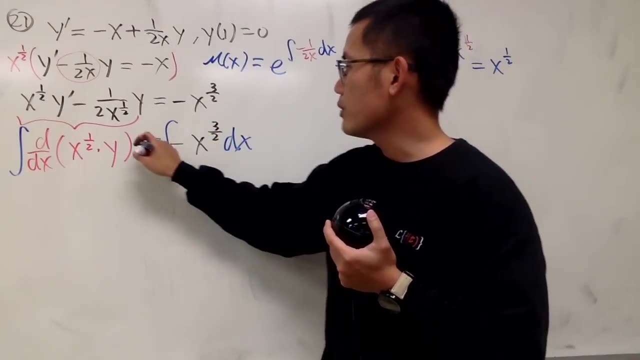 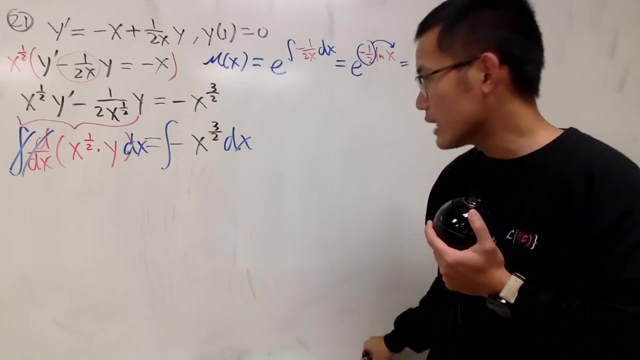 And the left-hand side. we have negative x to the 3 over 2.. Good, Now let's do the integral, Integral here, integral here in the x world, So that this and that will cancel, Very nice. And then we will just have the following: This is x to the 1 half power times, y and. 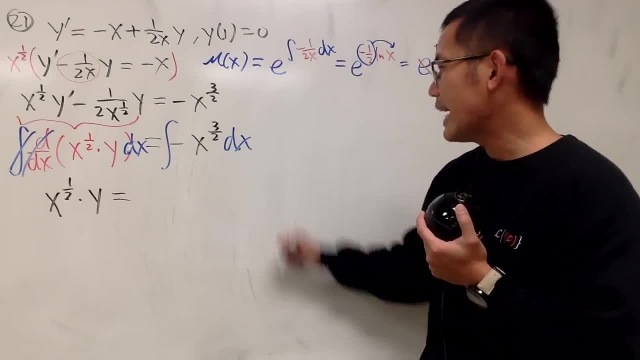 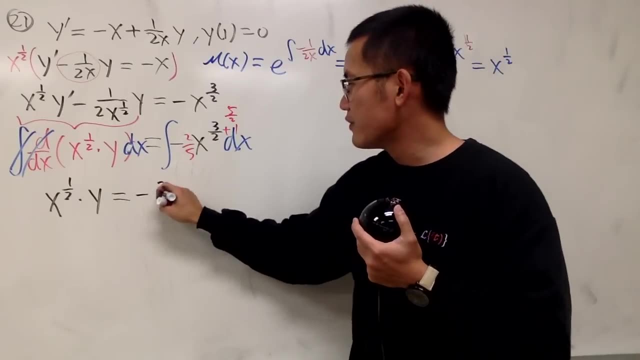 that's equal to. Now for this, go ahead and add 1 to the power, which is going to give us 5 over 2, and divide it by the new power, which is 2 over 5.. So we get negative 2 over 5, x to. 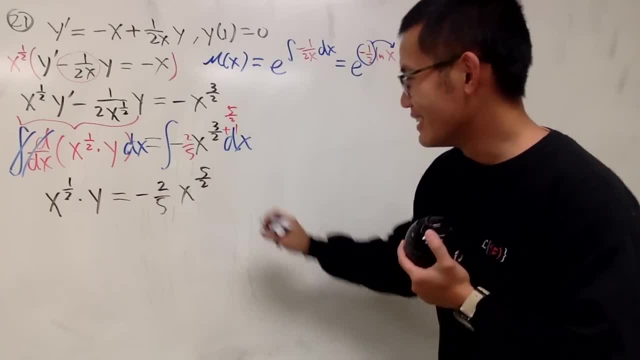 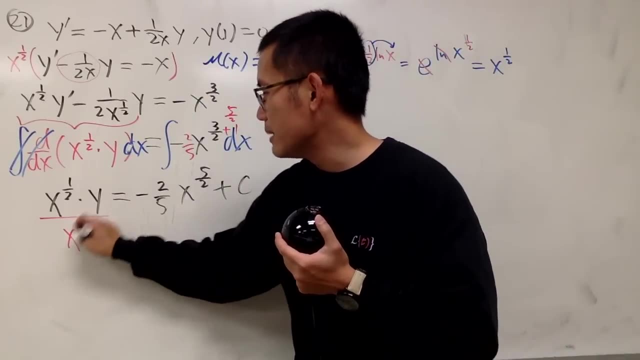 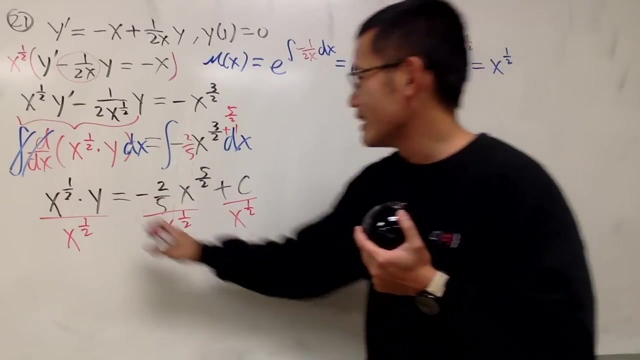 the 5 over 2.. Don't forget the plus c, even though I'm not wearing the plus c shirt, but I still remember the plus c, Plus c, right here. and then I will be done. after we divide everybody by x to the 1, half power Done as to get a general solution. okay, This and 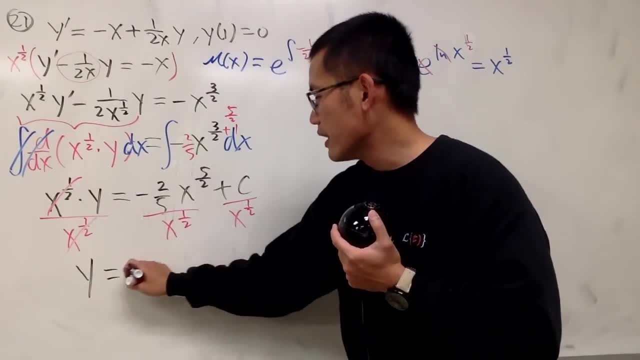 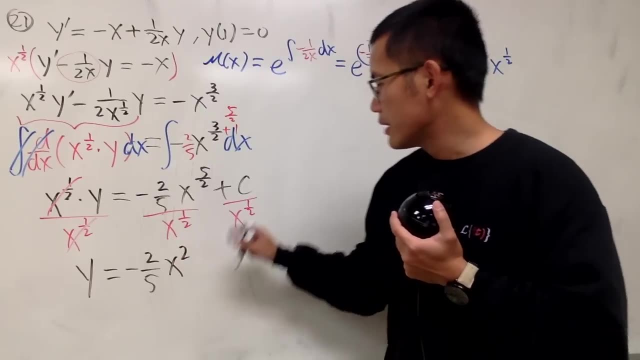 that can be done. So very nice. y equals negative 2 over 5. That's 4 over 2, which is x squared like this. and then this is just plus c over square root of x, if you would like. So that's what. 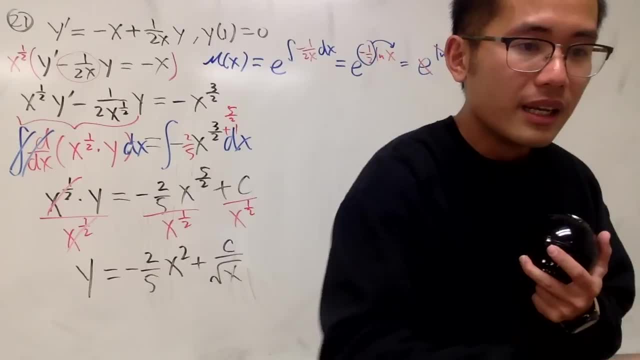 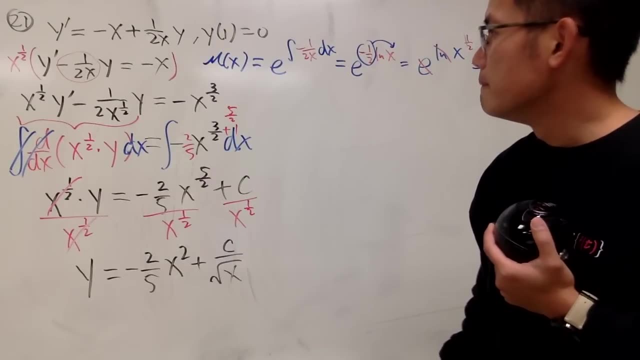 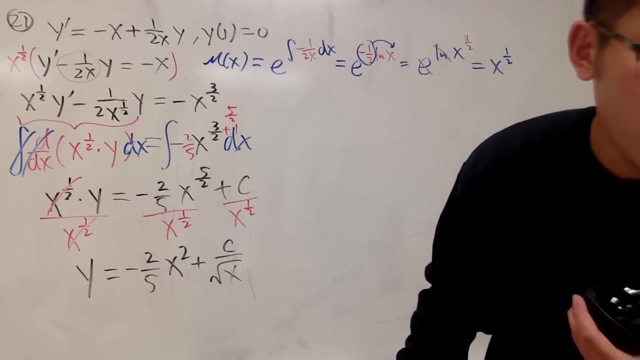 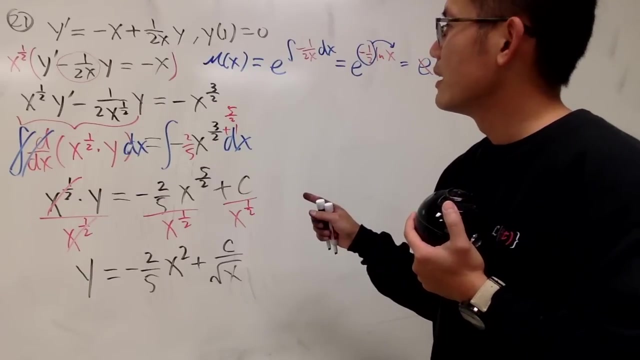 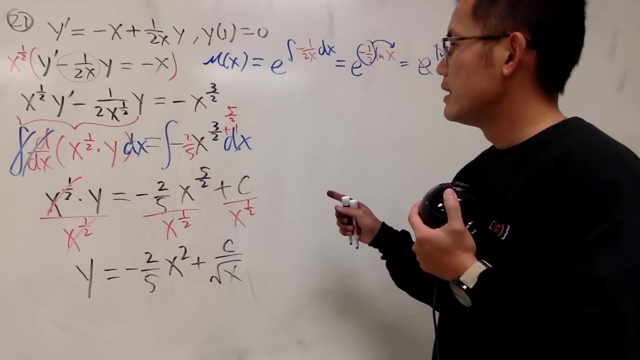 we have, And let me just double check if my numbers are looking good. Hmm, Okay. so let's see, I have the 1, x to the 1 half we have. Okay, So, as you can see, x to the 1 half, so I have the 2 over 4, and then I have sin squared. 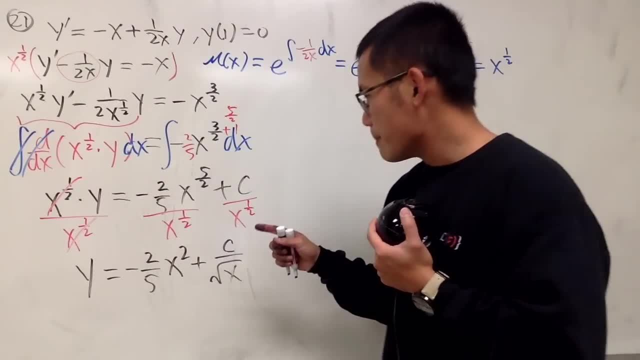 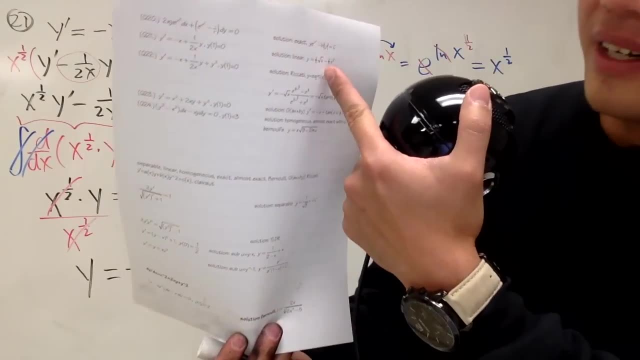 I have 2 over 4.. Okay, So that's what I'm talking about. Okay, Okay, Okay, Okay. Ah, scary, On my answer key I have a minus 2. 3rd. I don't know if it's just a typo when I was doing it. 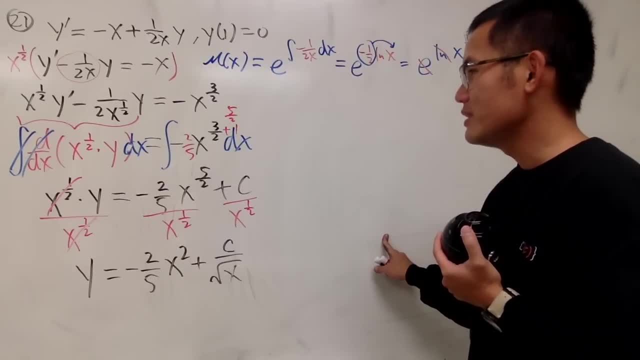 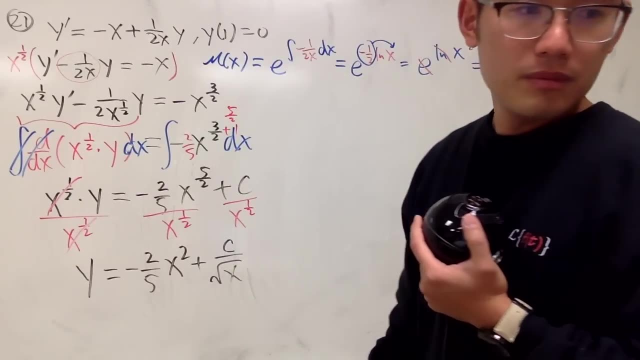 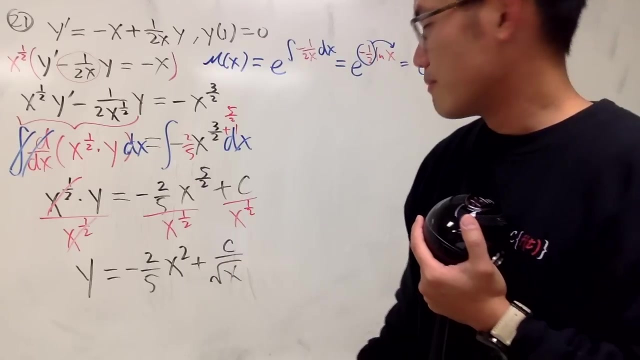 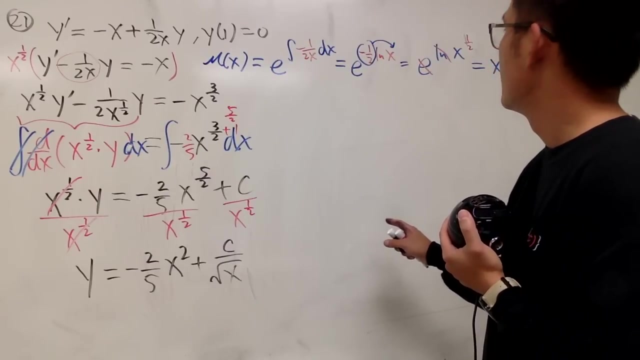 or maybe I'm doing this wrong right now. So I'll double check before I proceed. And I still have to find a C for you guys. Okay, let's see, let's see, let's see To the other side. So I have a negative. 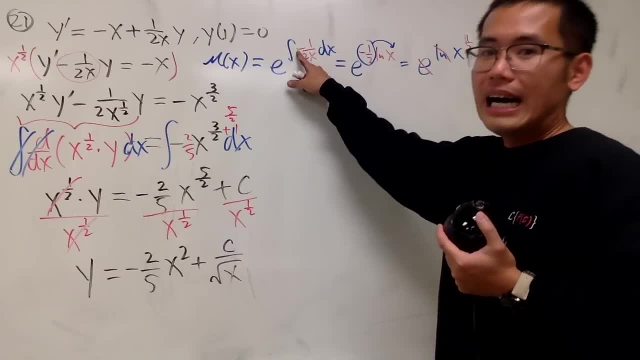 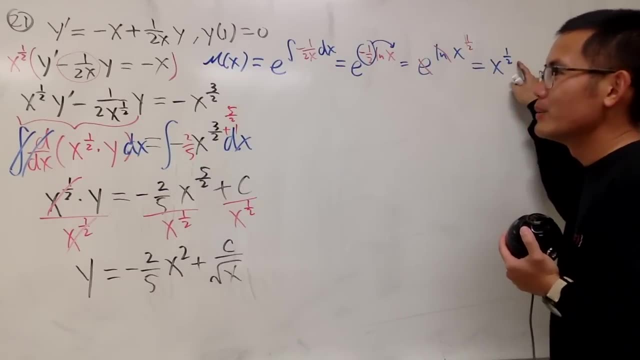 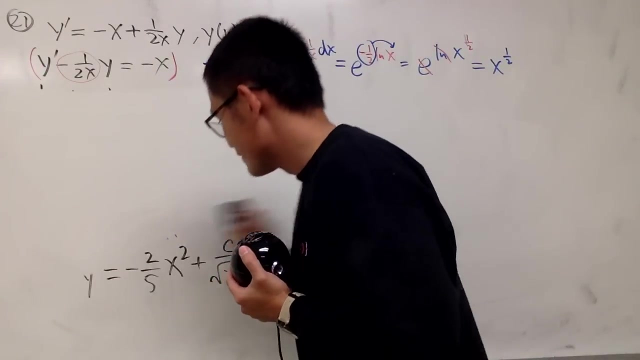 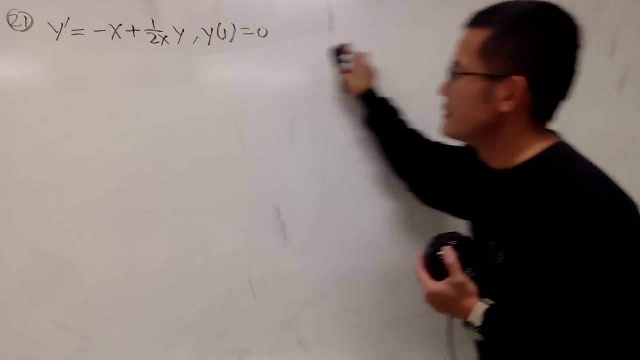 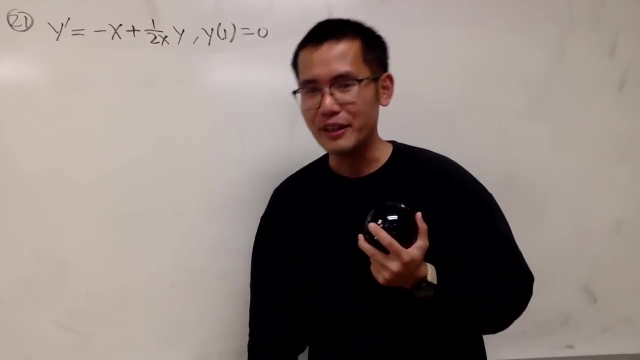 I have a negative, I end up with a positive. Oh no, Okay, I'll redo it. Okay, question number 21.. As you can see, this right here is so linear, isn't it? Yes, it is, But I will have to put this to the other side first. 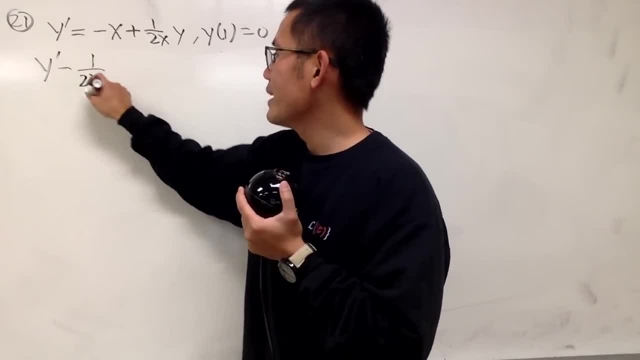 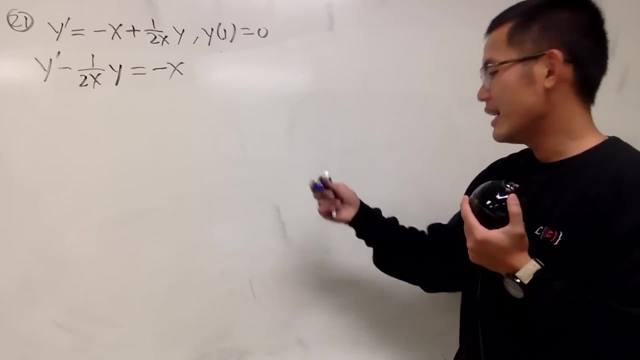 So here we go. We have y' Minus 1 over 2x y, And that's equal to negative x, like this. And of course we can just find a linear integrating factor, And I will do that right here for you guys. 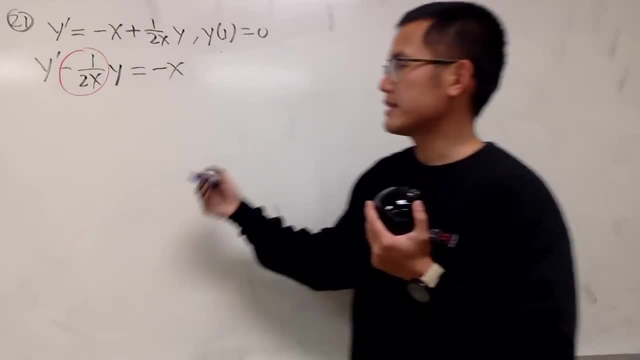 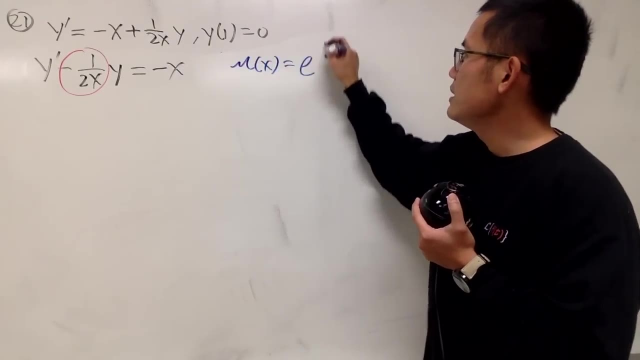 Pay close attention though. This right here is our p of x, right. Good, We don't have the, we just have a 1 in front. So here is the mu of x is e integral And we have negative 1 over 2x to be differentiated. 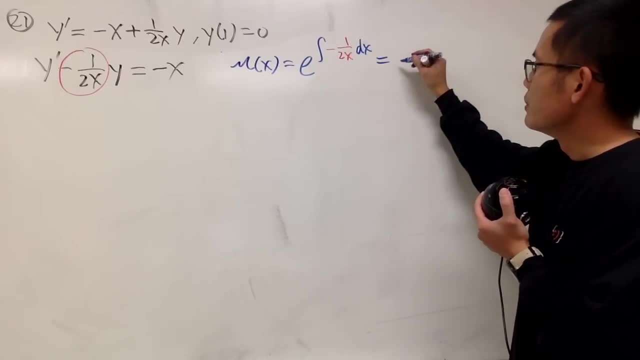 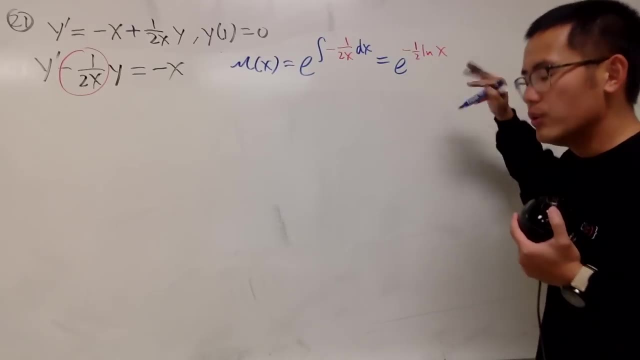 I mean to be integrated, And then we will just pretty much have e, And this is negative 1 half, And then we have ln, x. Don't worry about the absolute value, Don't worry about the plus c. Put this in here. 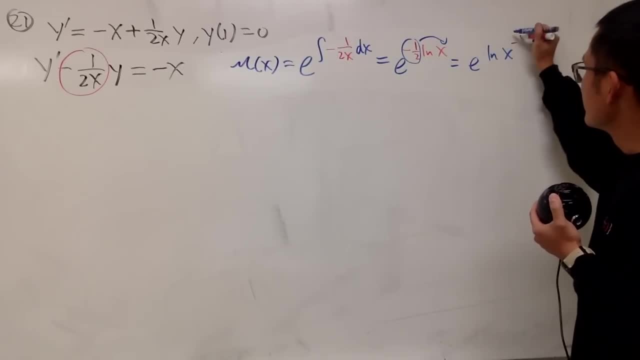 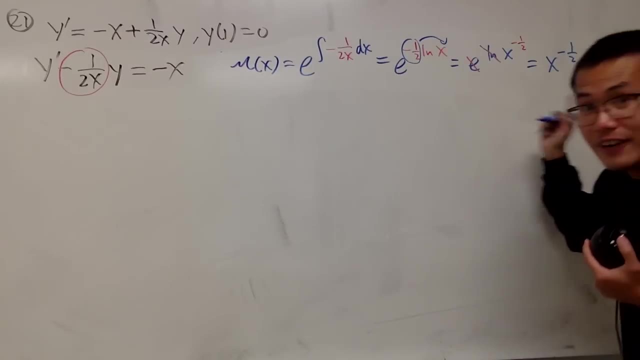 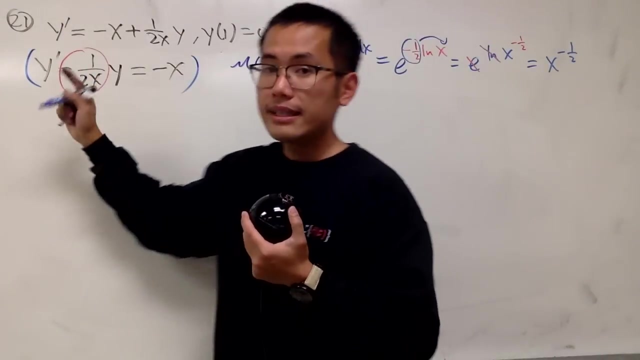 So we have e ln, x to the negative 1 half And they cancel. So finally we just have x to the negative 1 half power. Very good stuff. Now I will come here and do the following: I will multiply everybody by x to the. 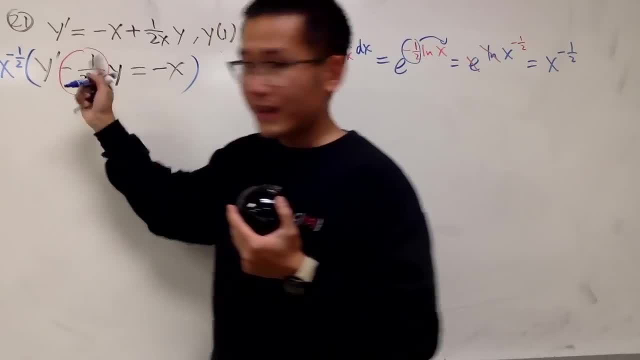 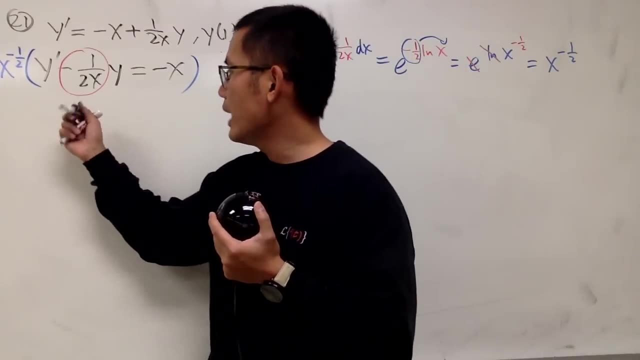 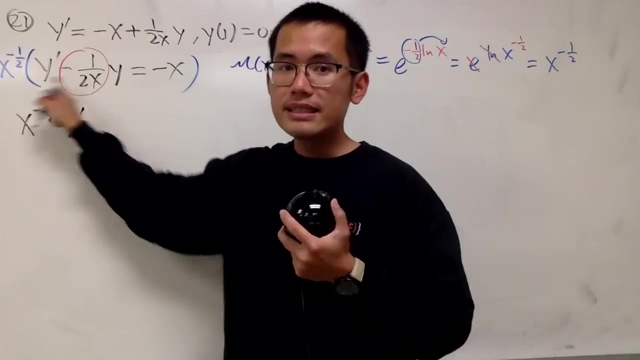 negative 1 half right. Okay, x to the negative 1 half. So now put on black and red, of course. So now, here we have x to the negative 1 half. power times, y, prime, Good. And then next, this times this, we have negative 1 over. 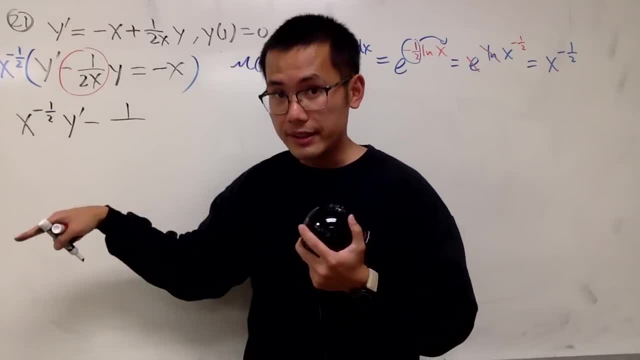 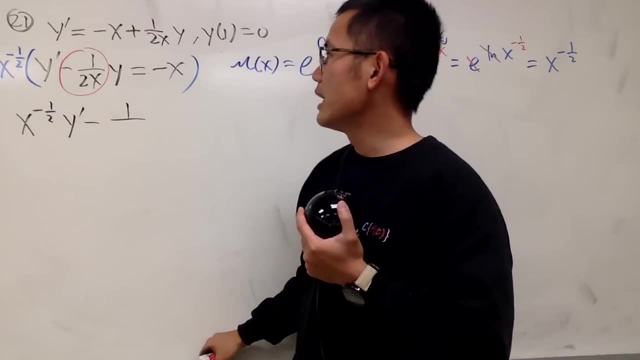 hmm, this right here is negative 1 half. Bring down to the denominator right. So we can write this down as: bring this down to the. let's do it like: okay, that's, that's okay, we can handle this in our mind, huh. 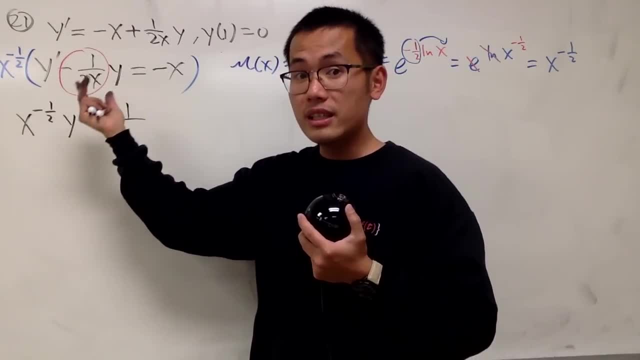 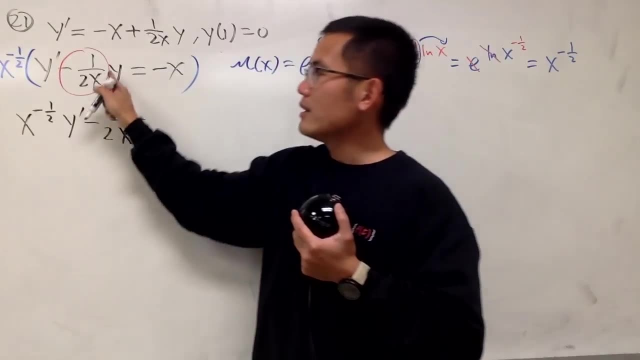 This is negative 1 half. This is negative 1's power, So it's negative 3 half. Bring that down. So you have this 2 right here, And then x to the 3 over 2 power, right, So bring this down. 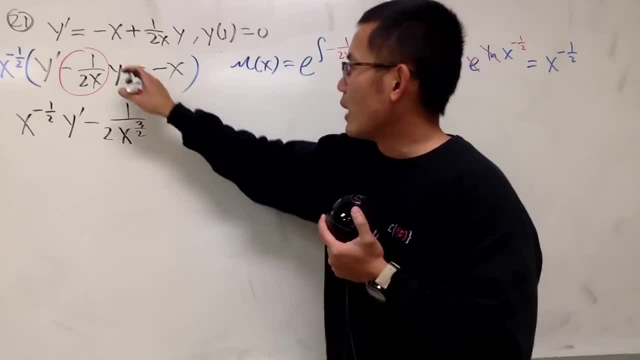 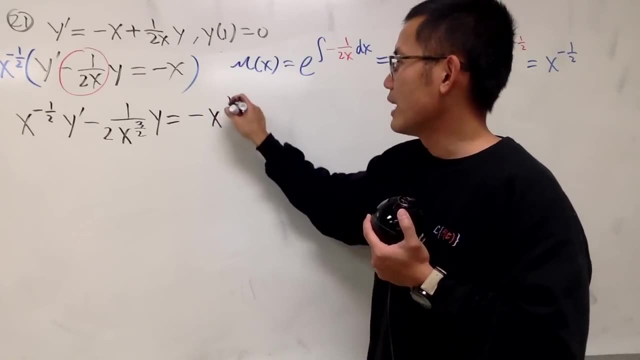 Just 1 plus 1 half. That's all Like this. And then y, that's equal to negative. This is 1.. This is minus 1 half, So we have x to the positive 1 half, Like this: 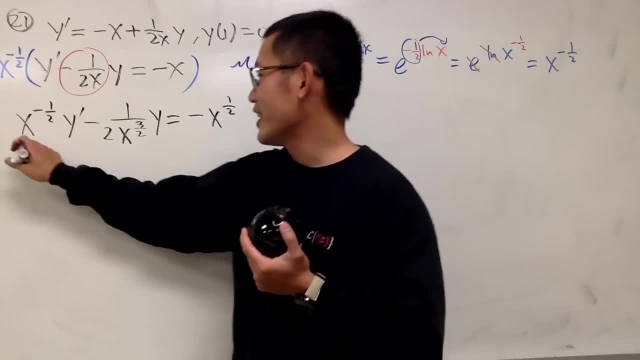 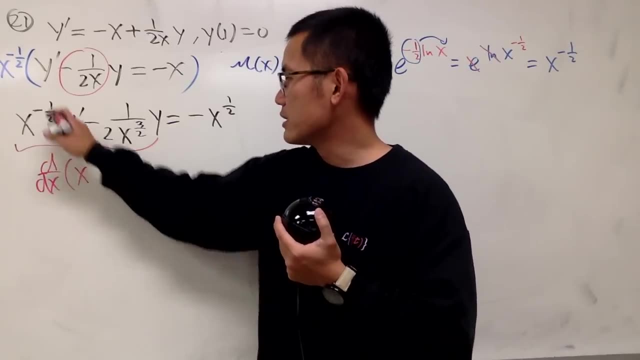 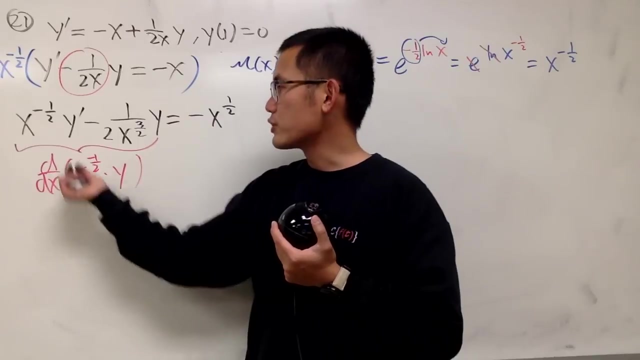 Now I should have totally done the check earlier, right? So this right here is the derivative of the product of functions. Name the x to the integrating factor, which is negative 1 half times y. Go ahead and check: First function times, the derivative of the second, plus the second function times, the derivative of the first. 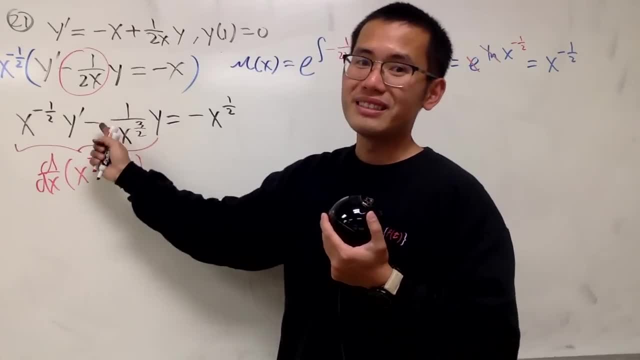 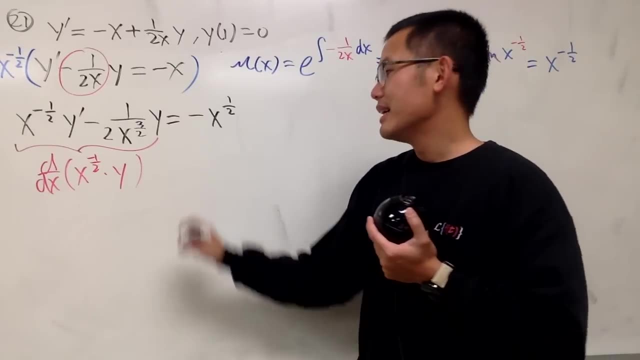 But if you bring the negative 1 half in the front it becomes minus Negative. 1 half minus 1 is negative 1 half. This is negative 3 half, which is the same as x plus 3 half power, Like that. 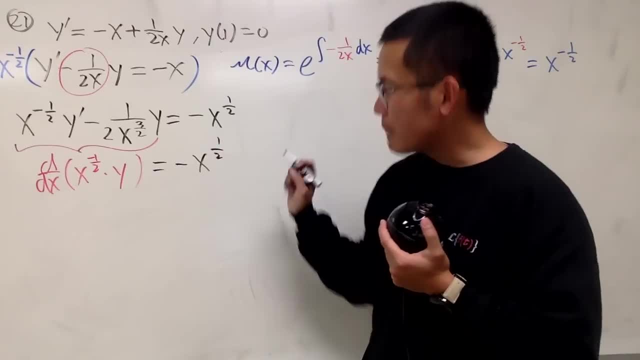 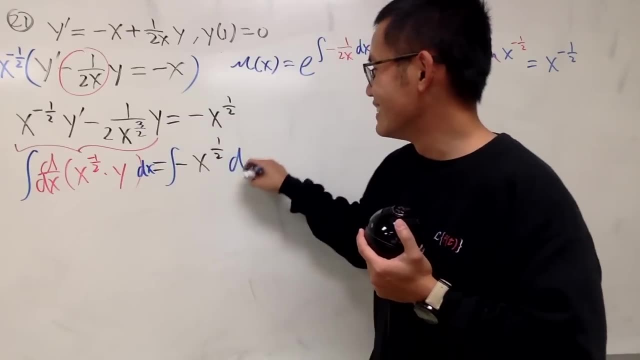 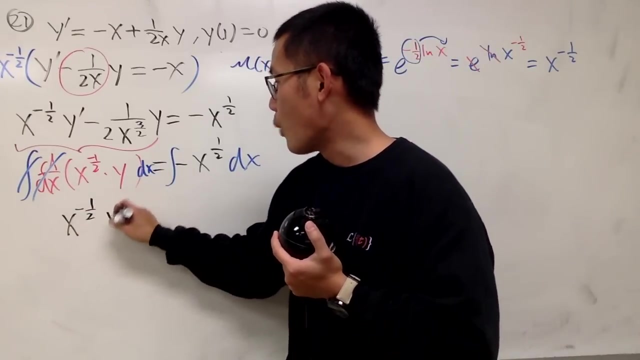 Okay, So here we have this: equal to negative x to the 1 half power, And then we can just go ahead and integrate both sides with respect to x. So this and that will cancel Very nice This. here we will have x to the negative 1 half y. 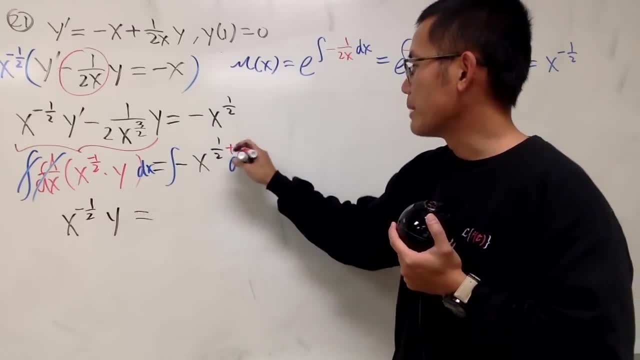 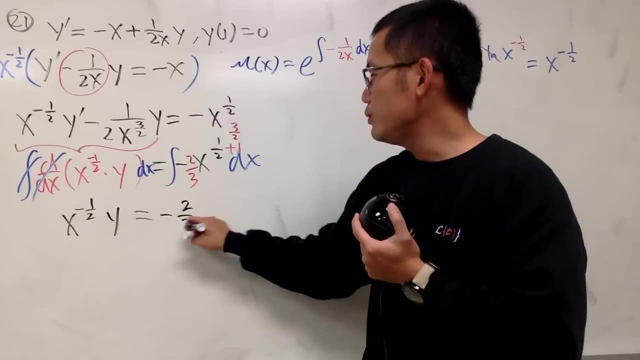 That's equal to right. here I will just add 1 to the power, which that will give us 3 over 2.. And then divide it by the new power. So we have negative 2 over 3, x to the 3 over 2.. 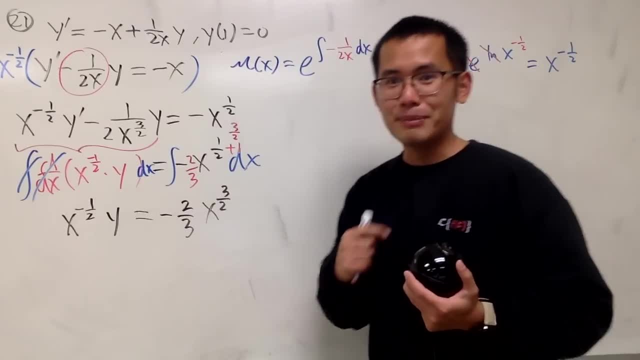 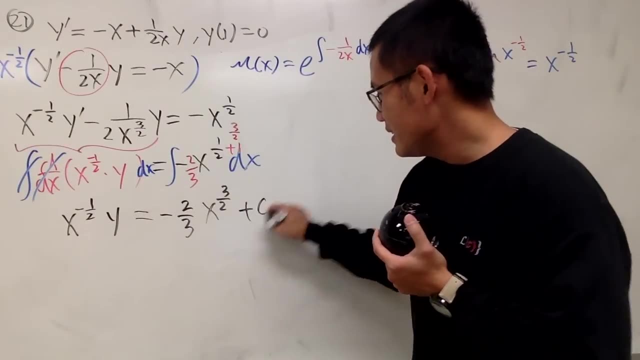 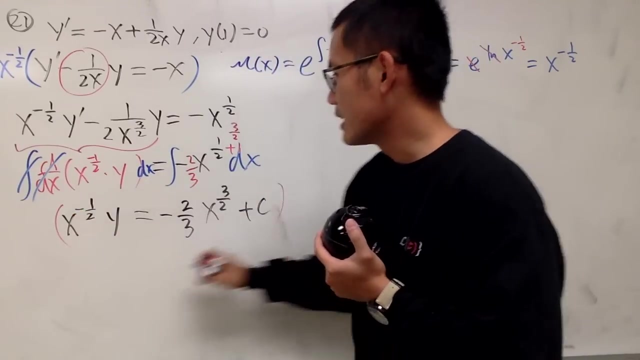 Like this And don't forget the plus c. Even though I'm wearing the Laplace transform shirt, I still remember the plus c. I still remember the plus c. So plus c here, and then divide everybody by this, And since this is negative exponent, so I will actually just multiply everybody by x to the positive 1 half. 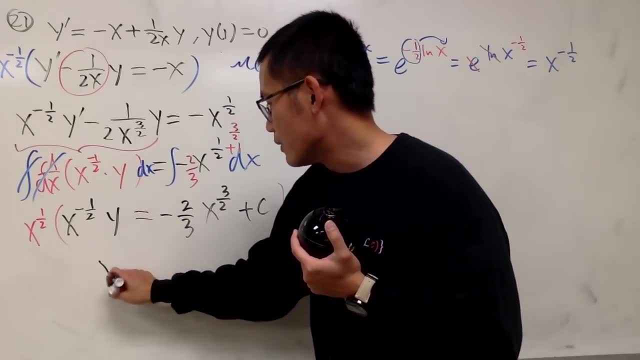 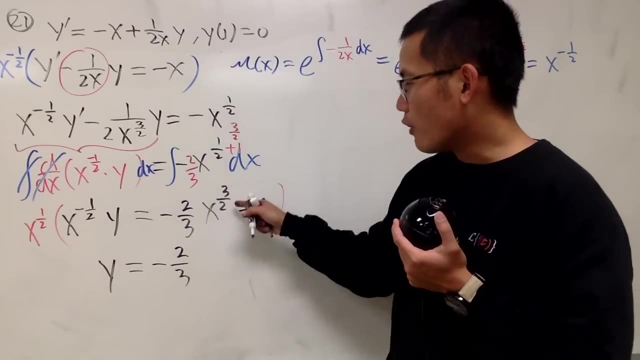 So this and that will cancel, And then I will just have y. That's equal to: this is negative: 2 over 3.. 1 half and this is 4 over 2, which is x squared. This times. this is plus cx to the 1 half power. 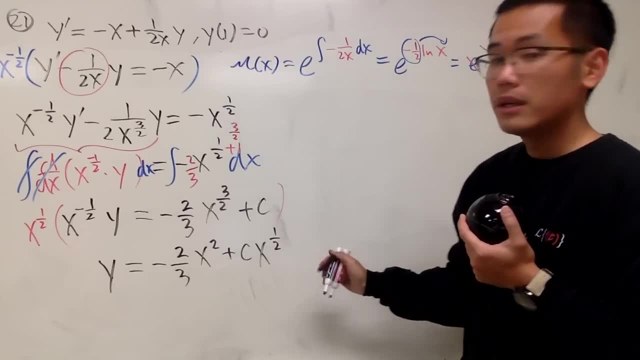 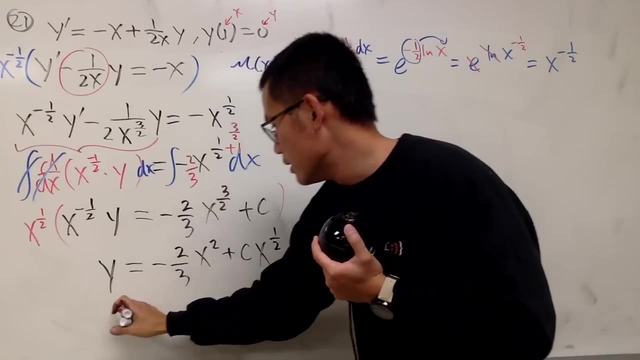 This is the general solution, But we do have the initial condition. So here we go. x is 1.. That will give you y being equal to 0. So we have- let me just do it right here, Because right now we have enough space. 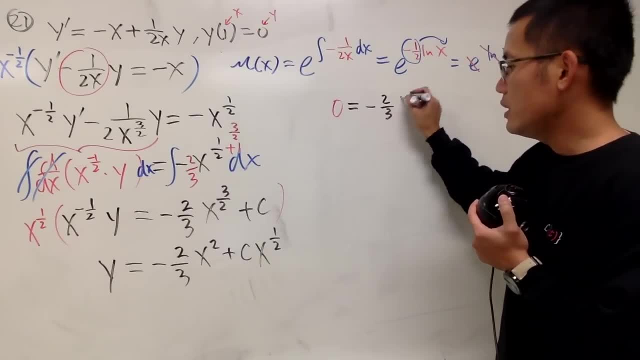 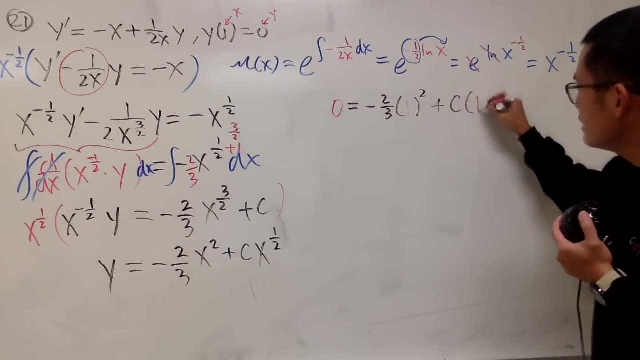 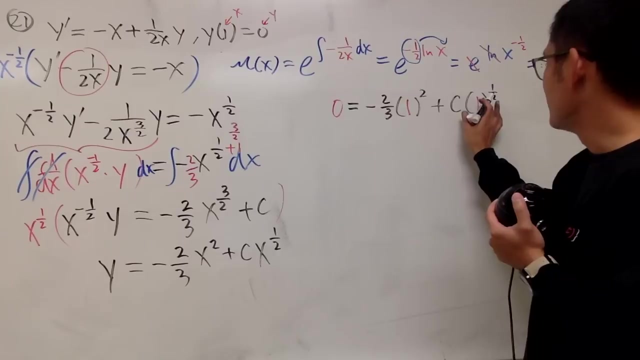 0 is equal to. It's equal to negative, 2 over 3.. 1 second power plus c times 1.. And then we have the 1 half power here. Yeah, And then this is just c, And then bring that to the other side. 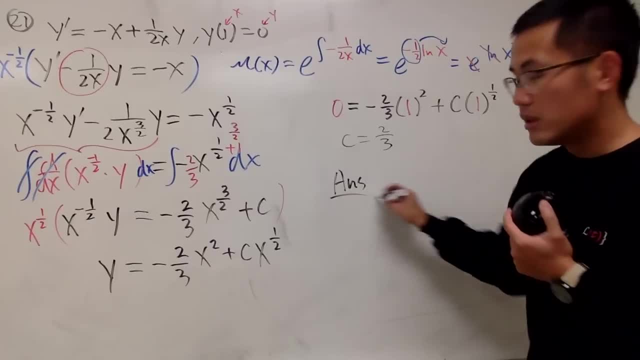 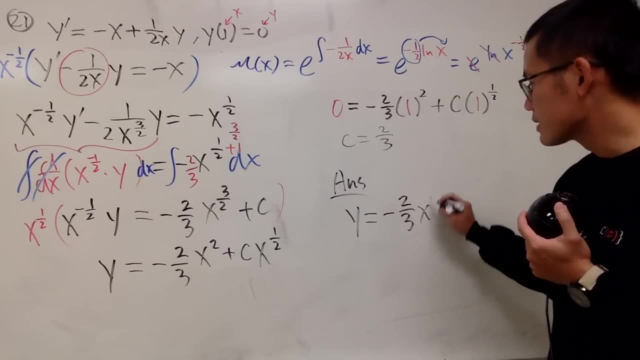 So c is equal to 2 third. So finally, I will write down the answer for you guys. We have this: y equals negative 2 third x squared, And then c is that. So it's put on plus 2 over 3.. 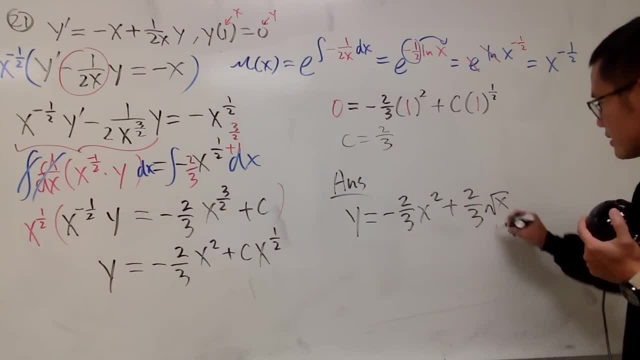 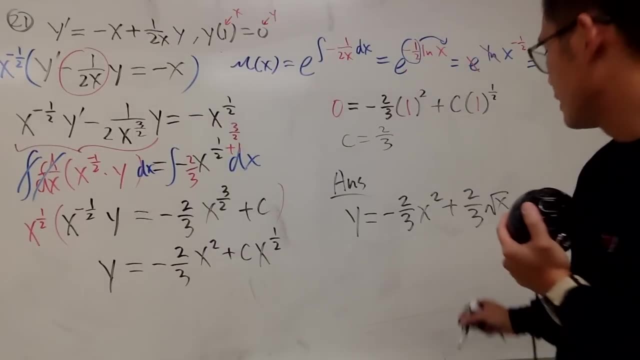 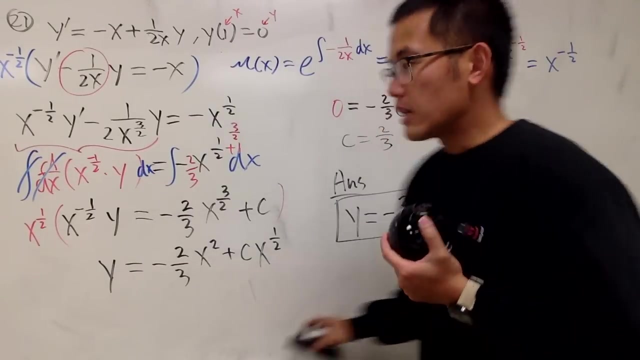 And for this you can learn the square root of x. So this right here is it. So that's pretty much it. Yes, So that's it. Good Couple more to go. So have a look. This is question number 21,. yeah. 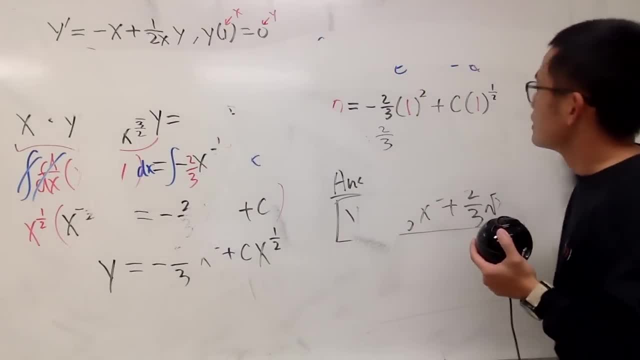 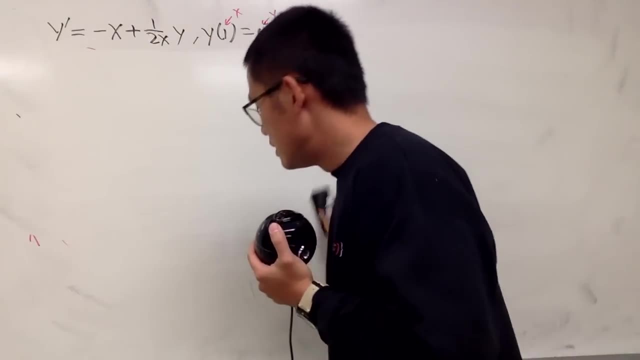 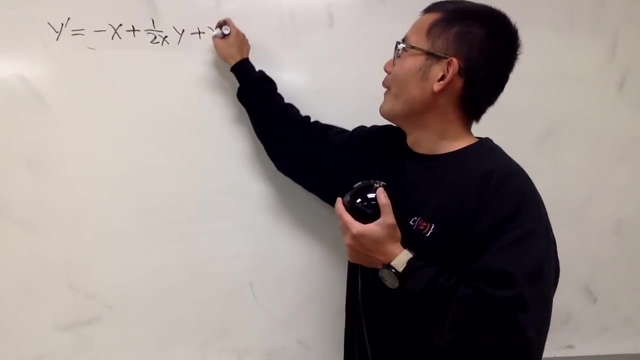 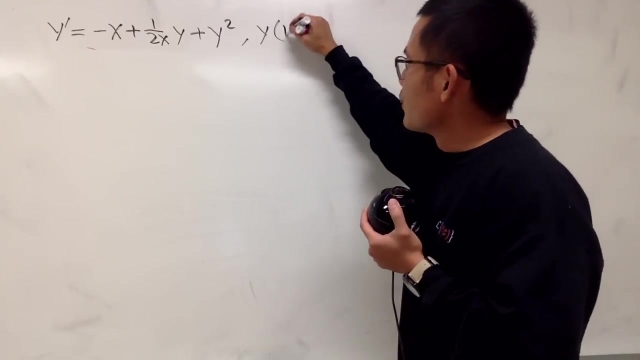 And this is what I will do for question number 22.. Plus y squared. And that was tricky because the initial condition, because- why not Anyway? y of 1 is equal to 0. And this is question number 22.. I believe that's what I said. 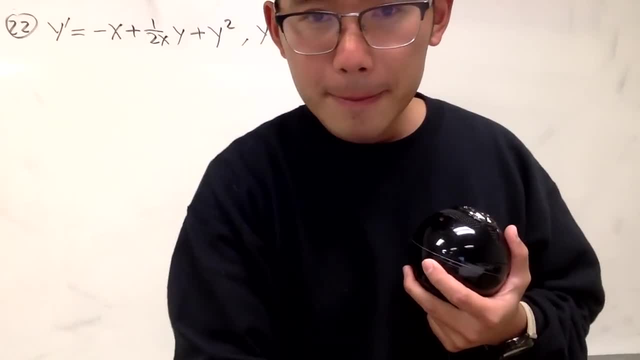 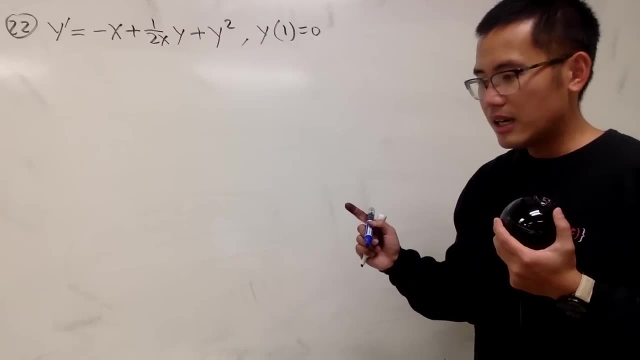 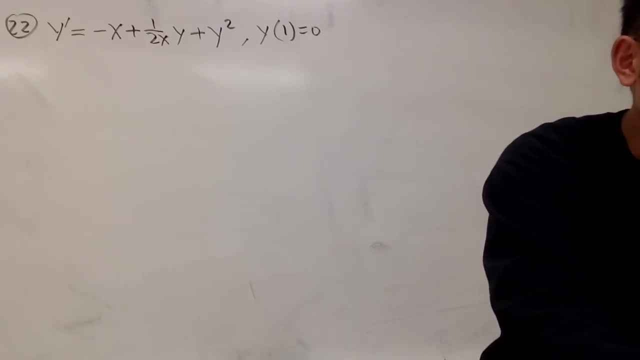 This right here is going to take a while. Okay, It's four hours already. Anyway, this right here has a name. This is called Riccati. I don't know how to use it. How do you say that, Riccati? 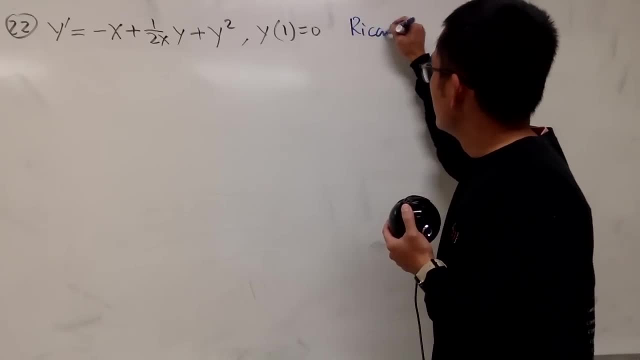 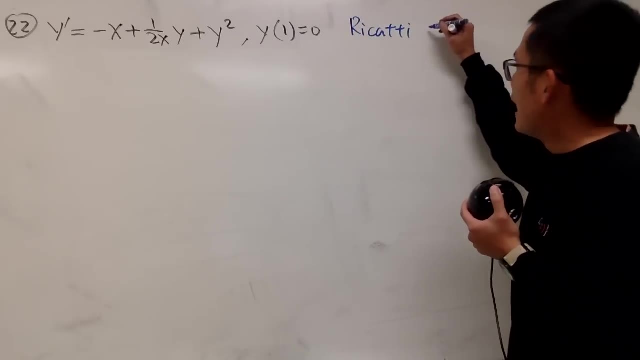 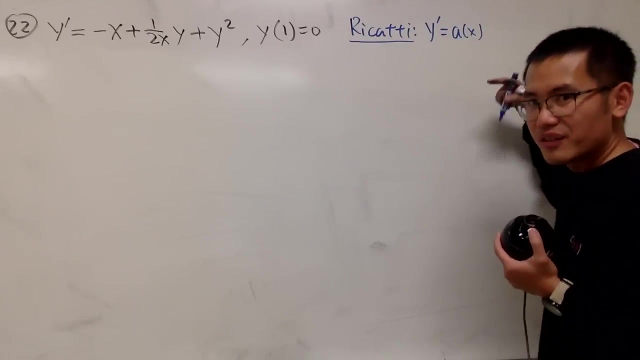 Yeah, This is called the Riccati. This is the Riccati differential equation. This right here has the form y prime. So y is equal to the function of x. So a of x. I just say a of x. 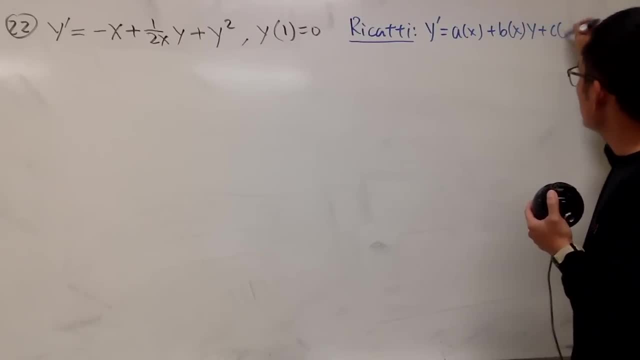 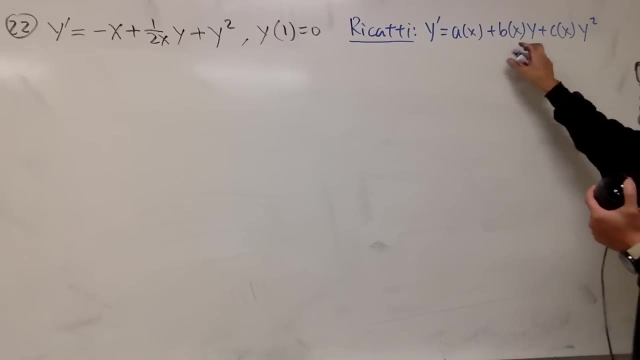 Plus some function in terms of x times y plus some function, And you have the y squared like this, So you have the coefficients being the function of x and then you have the quadratic in terms of y. That's pretty crazy, all the stuff. 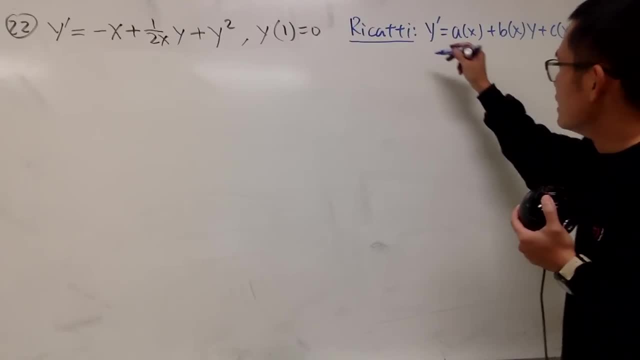 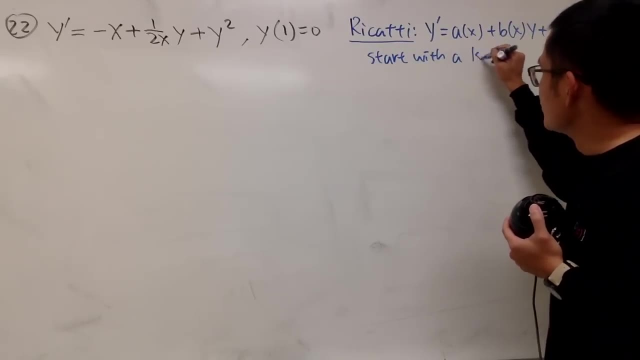 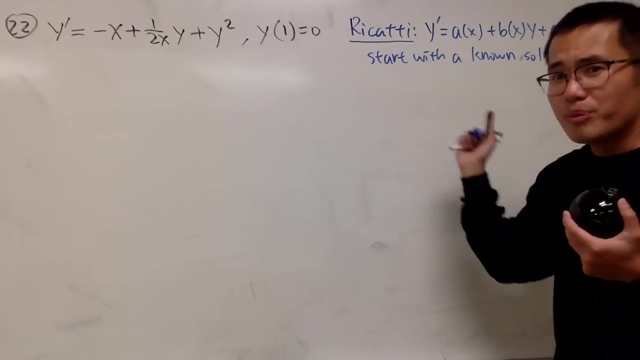 So here is how you are going to get it. first, You have to start with a, A known solution. A known solution, So it's like a particular solution that will make this work right. A known solution can be like something simple, hopefully. 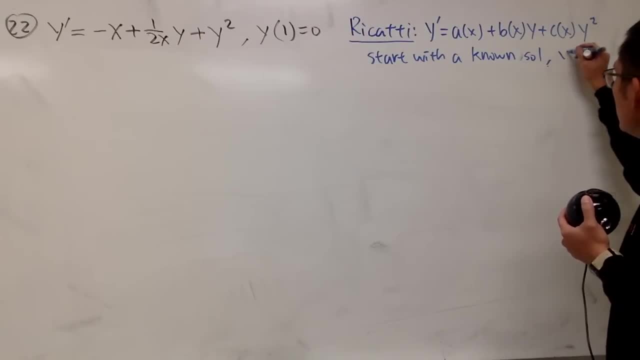 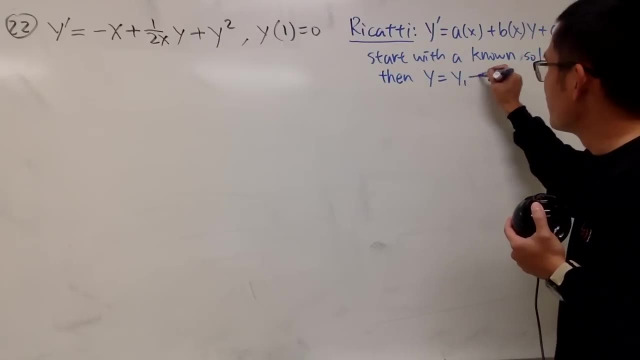 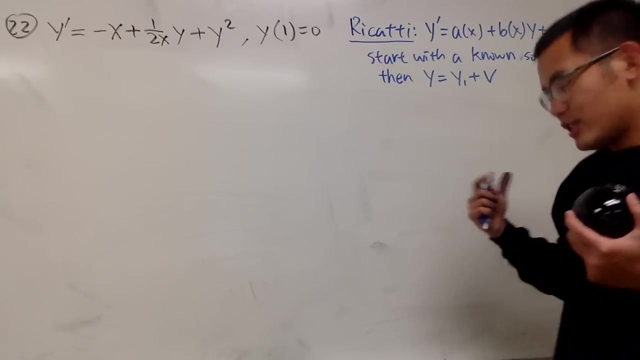 And let's say call it y1.. Start with a known solution. Let's say it is y1. Then y is equal to y1 plus some other variable. Let's say v, And then you just continue from there. So this procedure is not so bad. 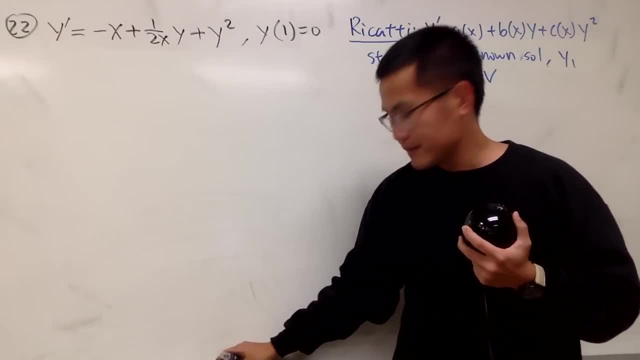 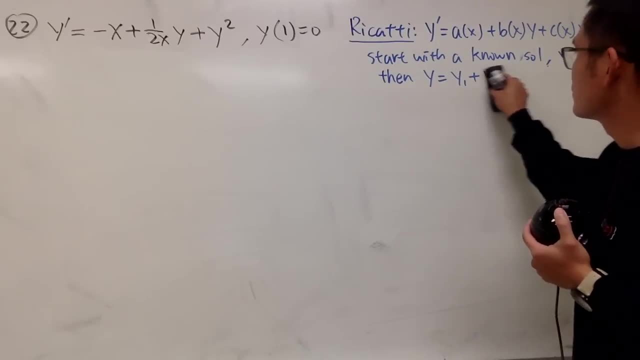 And you end up with the time Bernoulli, And then I will try to fit everything onto this whiteboard because it will be so satisfying if I can do that. So I will make sure I have enough space. So I have to do this. 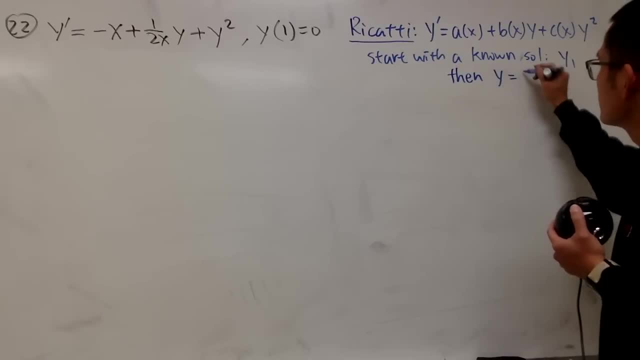 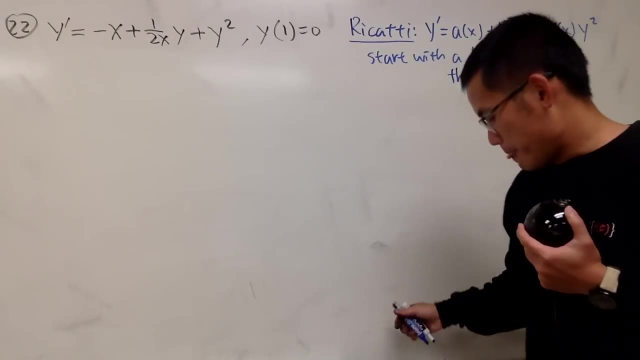 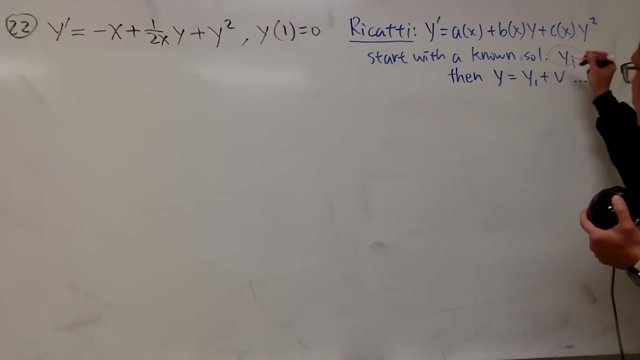 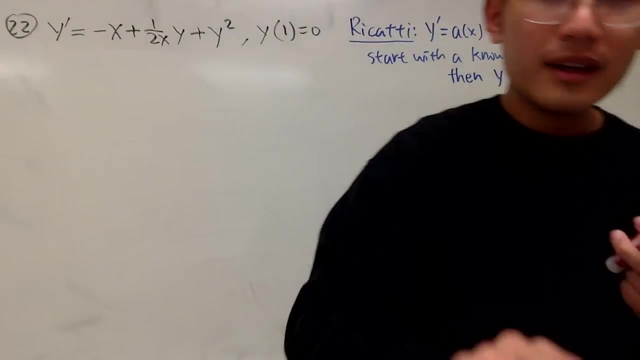 Then y equals y1 plus v And then continue. Okay, Here is the deal. We have to start with some known solution like y1.. And the problem is that that's not easy And just I don't have a good red pen. 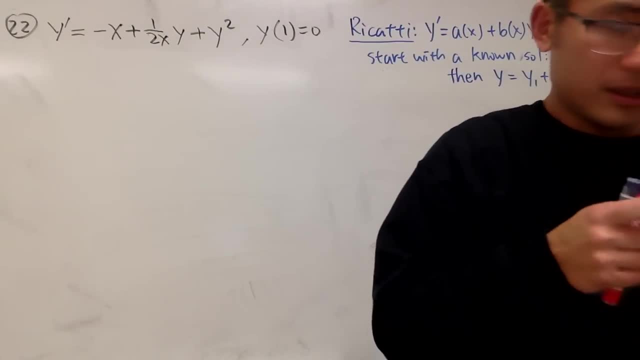 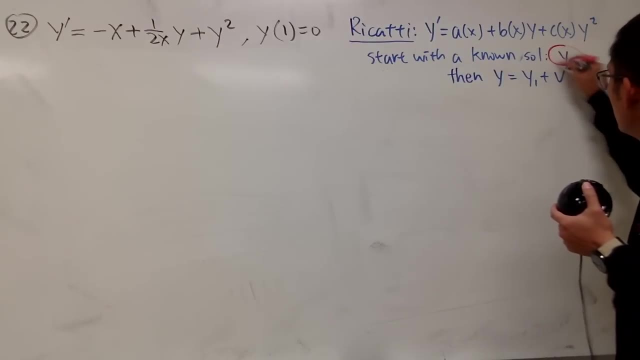 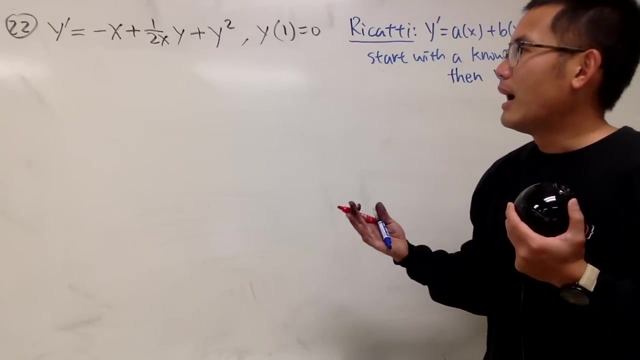 That's not easy, I will have to get another one. We want to have a Much better. We want to have a known solution y1. That's not easy, So right here. usually if I have to assign this question, or so, I will give people hints. 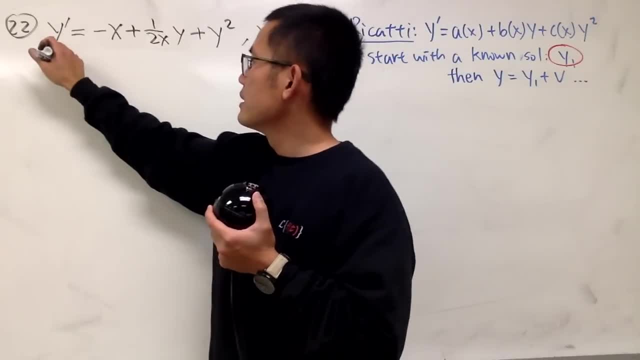 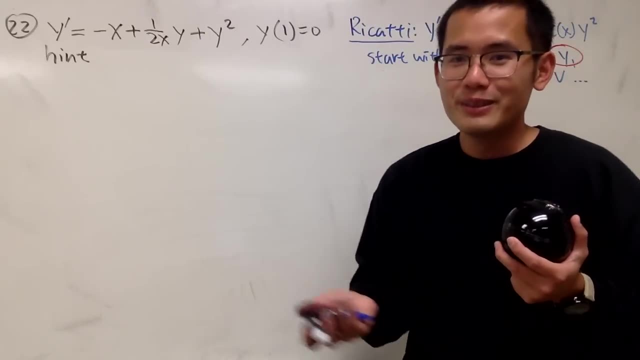 So I will just say the hint. And here is the hint for you guys: Whenever you are taking a test, if there's a hint, you have to use it right. Otherwise, no, This wouldn't make sense, unless you can come up with some super genius way to do it. 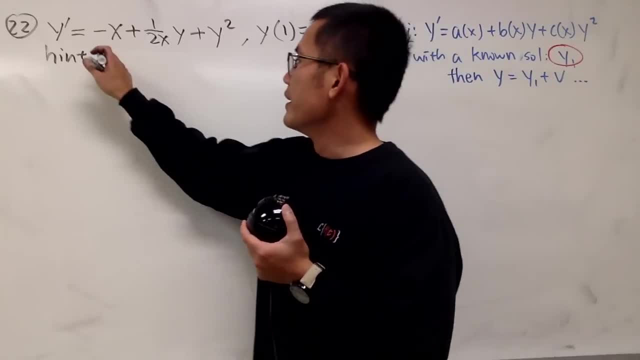 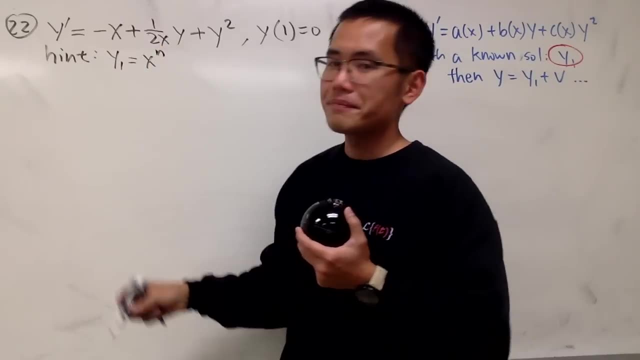 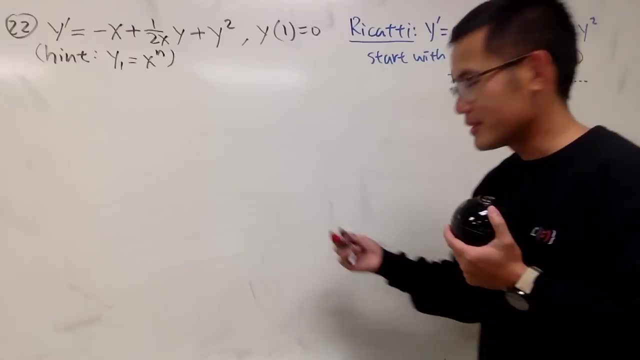 But if you have a hint, use it. Why not? The hint is that y1, I will tell you it's in the form of x- to some power n Yeah. So this is the hint that I will have for my students if I am assigning this kind of questions. 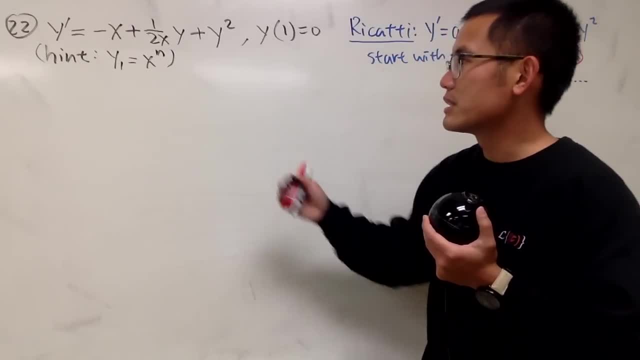 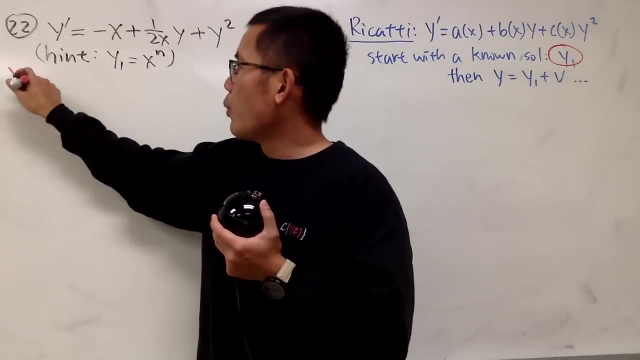 So I'm going to use this hint and then I will just kind of come up with: what function do I have for the particular solution, right? So here we go, Starting with y1 being equal to x to the n. then I know, y1 prime is just going to be nx to the n. 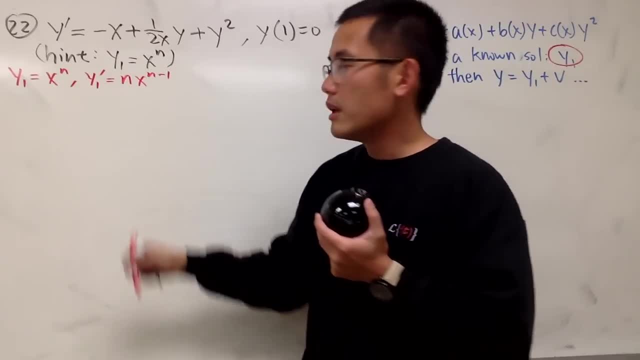 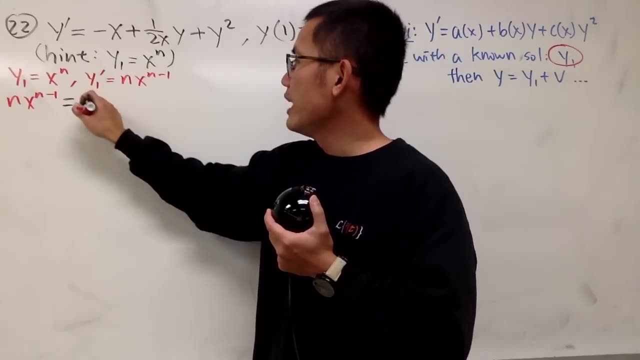 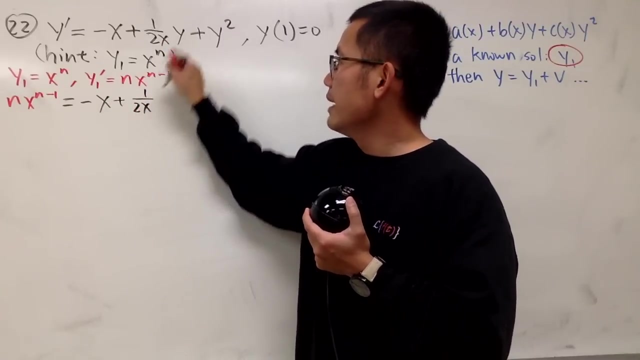 nx to the n minus 1, because that's just the derivative. Now I put this back, so I will get nxn minus 1.. That's equal to negative x, It's just x, And then plus 1 over 2x. 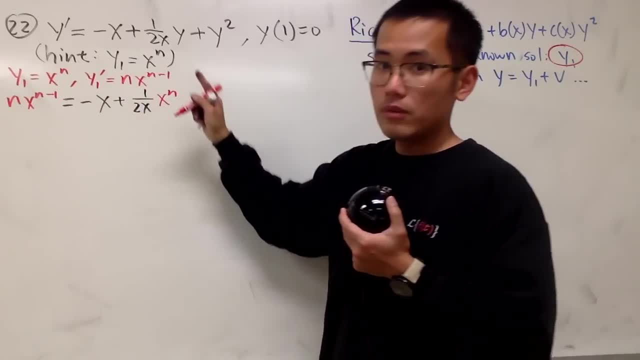 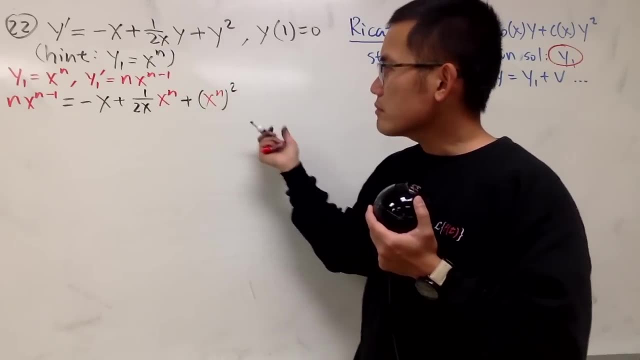 And then the y is x to the n, And y is x to the n, And then we add x to the n to the second power. So just like this. And now here's the hard part for this. This right here does not always work right. 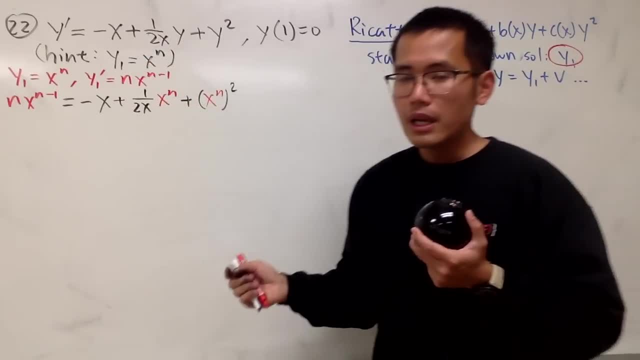 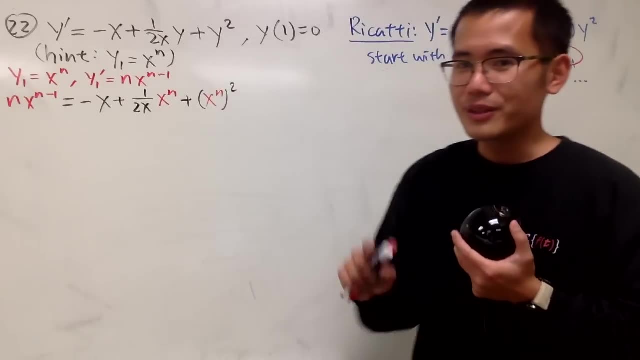 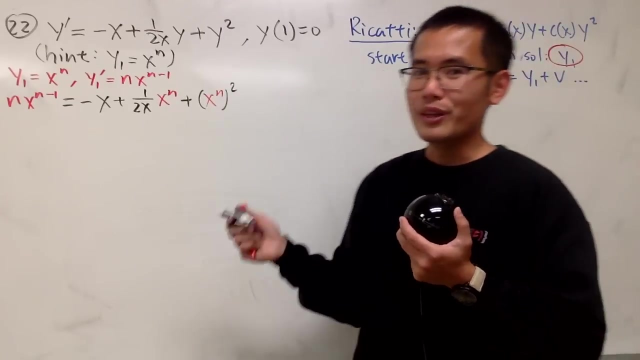 Because you can imagine, if you have sine x, then it's not this for sure And we just have to see. Let me see if this is working. Yeah, Am I still recording Good? We just have to see if we can actually come up with a good value or not. 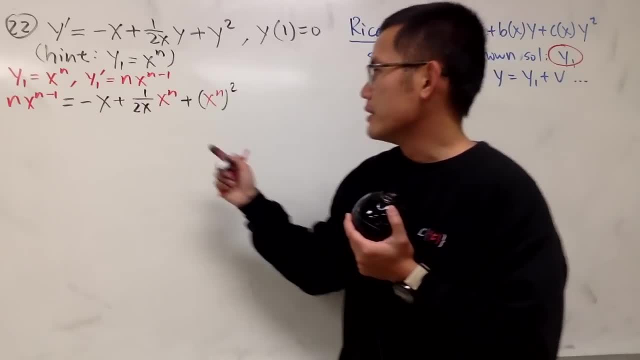 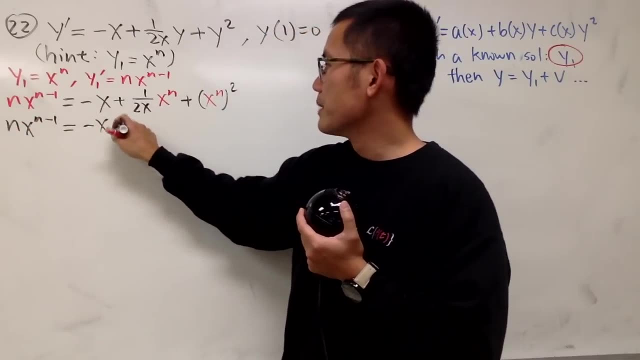 and hope for the best, I'll say Okay. So here we go. Notice: this is x, This is nxn minus 1.. This is negative x plus. this is 1 half n minus 1, yeah, x to the n minus 1.. 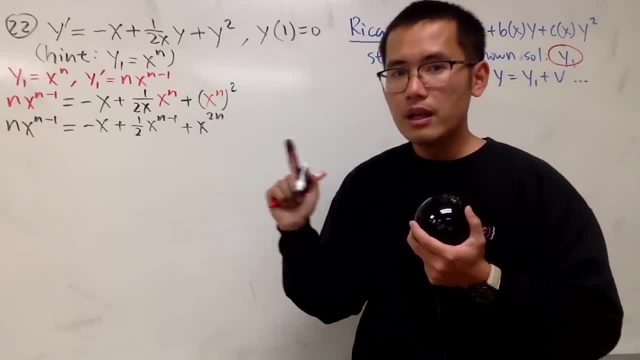 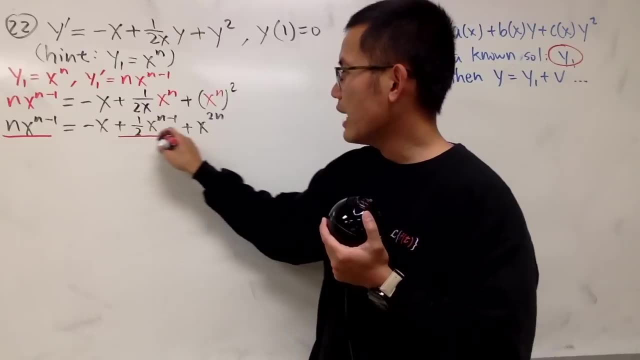 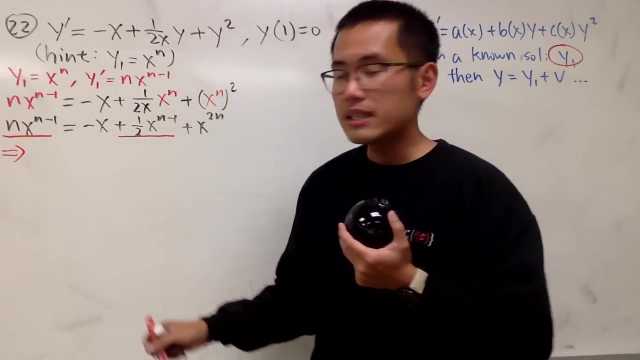 And then plus x to the 2n. Good, Now, on the left-hand side, we have nx to the n minus 1.. On the right-hand side, we also have that nx minus 1.. So wouldn't this suggest us that, based on this, wouldn't this suggest us that? 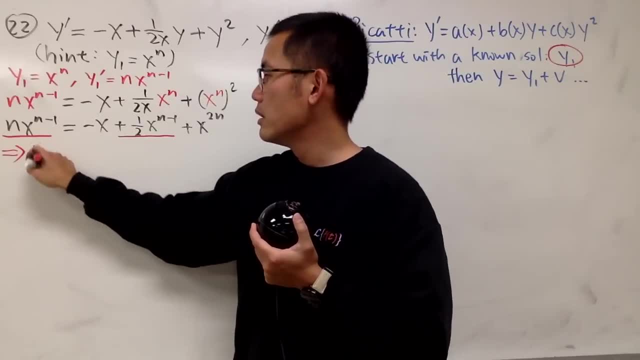 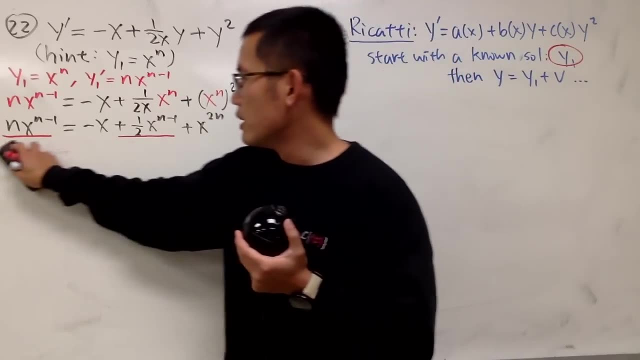 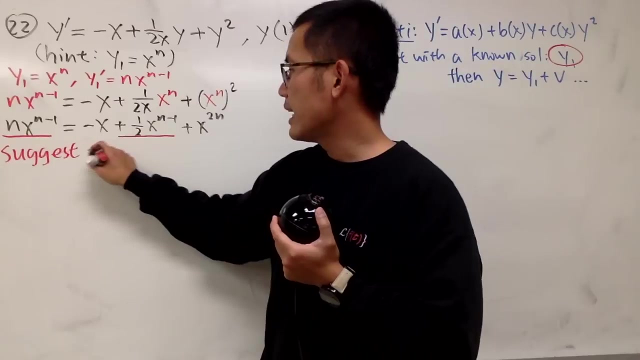 n has to be 1 half. This right here suggests us. it just suggests: okay, I'm not, I shouldn't draw the arrow, I will just say: based on this and that it suggests us, suggests that n is equal to 1 half. 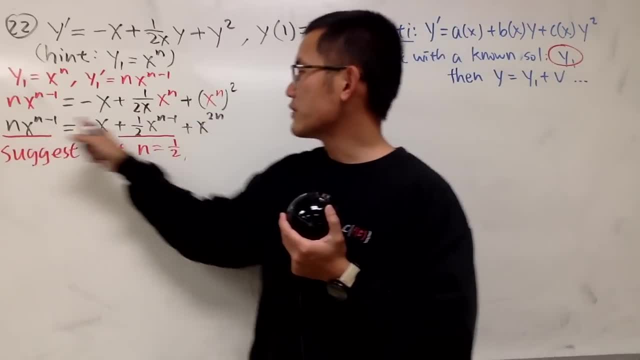 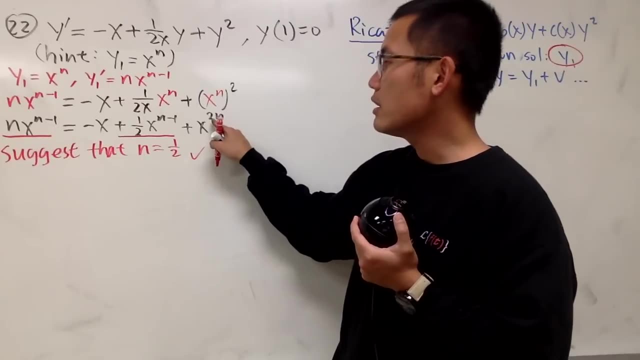 Well, does this work though? Because if n is equal to 1 half, it works for this and that. But does it work right here? Yes, it does. It just happened to work, Because if you put 1 half in here, 2 times 1 half is 1.. 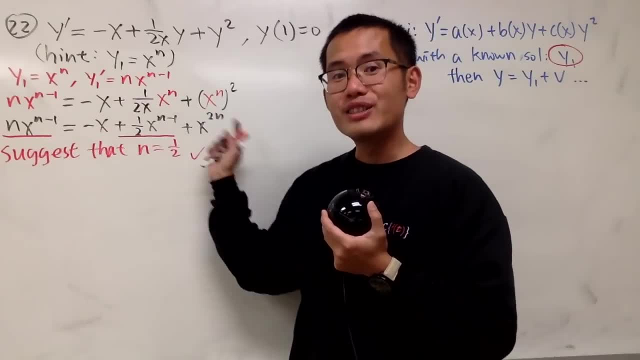 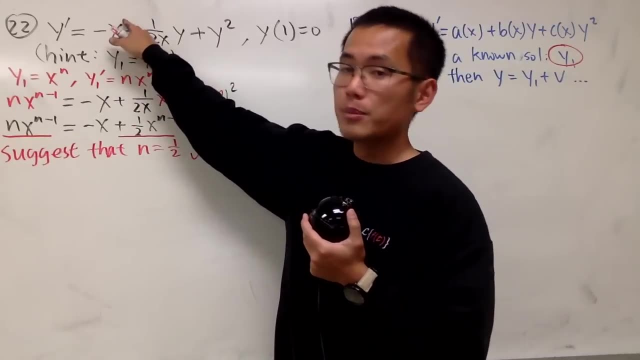 x to the first power and this is minus x. they cancel. So the left-hand side is indeed equal to the right-hand side. You can imagine this wouldn't work if this was minus x to the third power. This, right here, wouldn't work. 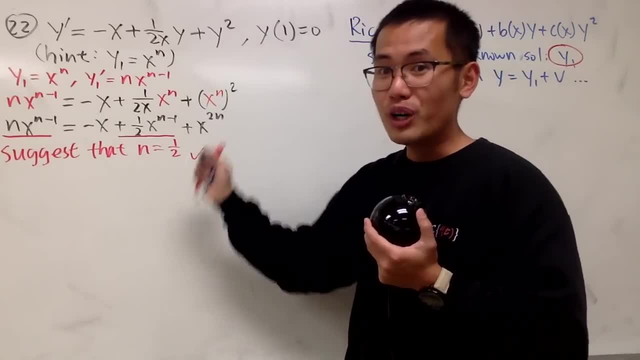 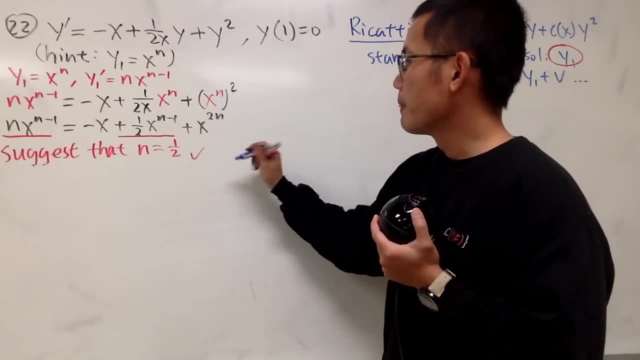 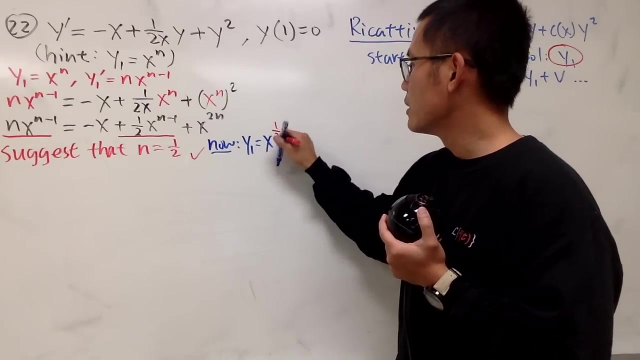 So I'll just say: suggest n is equal to whatever. If it works, it works Alright. So we know now why 1 is equal to. So now y1 is equal to x to the 1 half power. Now we know right. 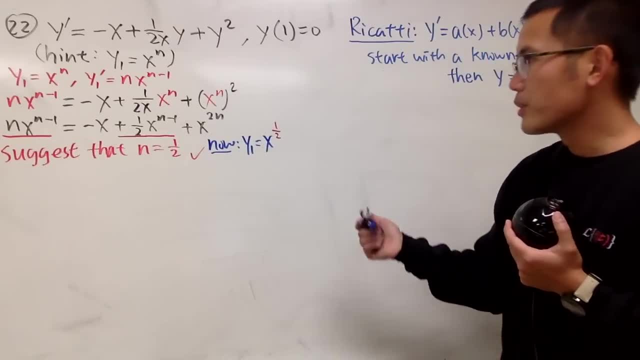 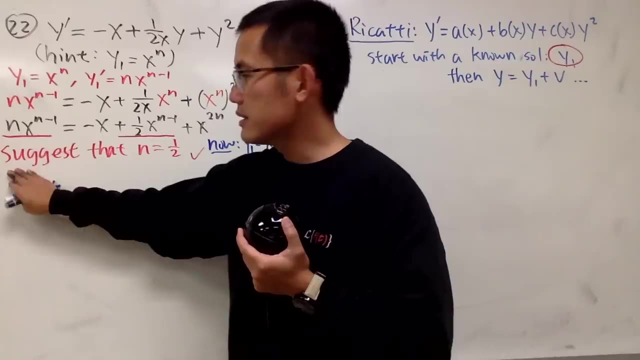 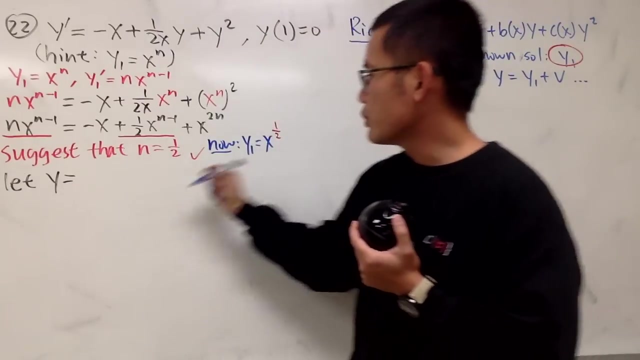 Now we know. now That's good, So I'm going to do the following. I will just pretty much do the usual thing. So now the solution is going to be y. So here's the substitution. So I'm going to let y equal to y1, which is this, which is the square root of x. 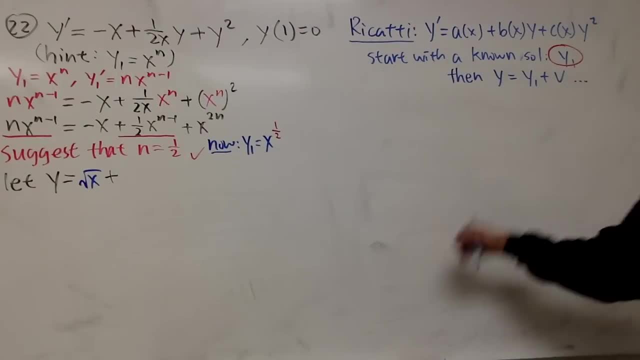 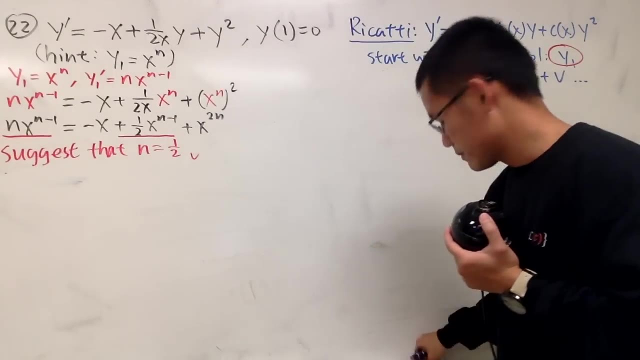 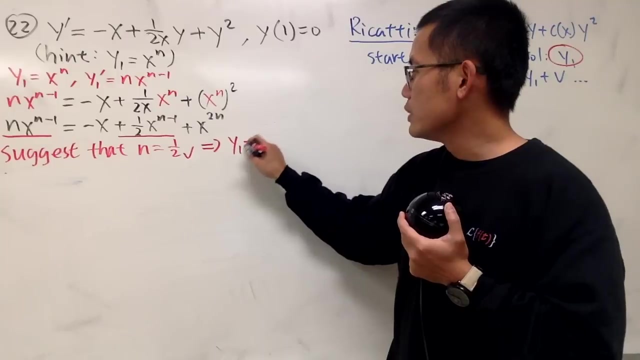 plus, plus some other letter, which is v, and I will just put this down right here. Let me see- Actually let me do this right here, Sorry- n is equal to 1, half, It checks. So this means y1 is equal to x to the 1 over 2 power. 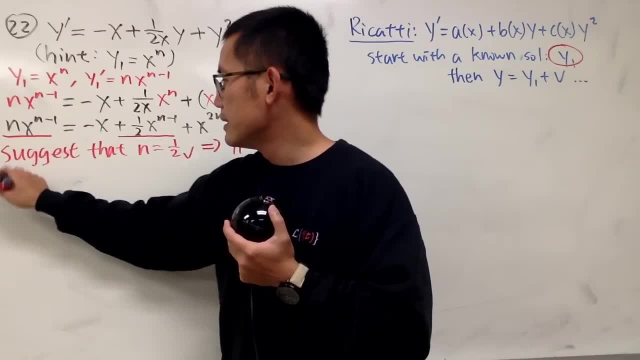 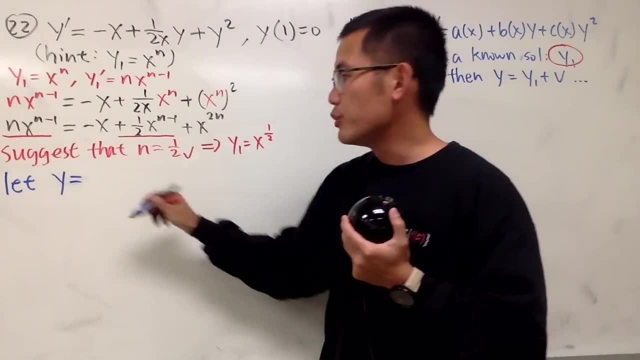 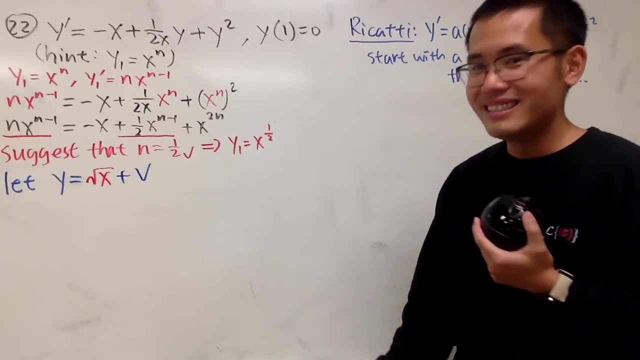 Alright, Now I'm going to let y equal to y1, which is x to the 1 half power, and that's going to be square root of x, And then plus some other letter, v, Yeah, And then I will just do the usual thing. 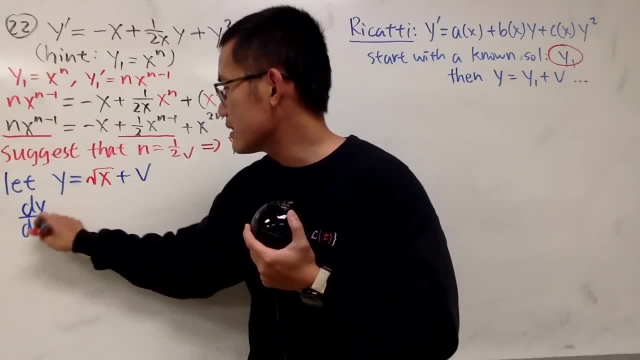 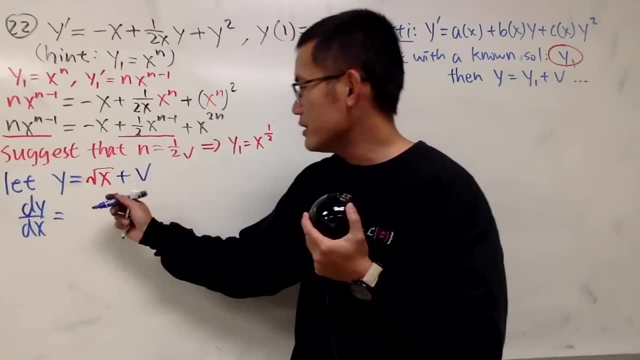 So let's go ahead and differentiate this guy. So we get dy dx. That's equal to Differentiate this guy. Actually, I will change that to black, I'm sorry. Oh, don't change it to blue. Differentiate this guy. 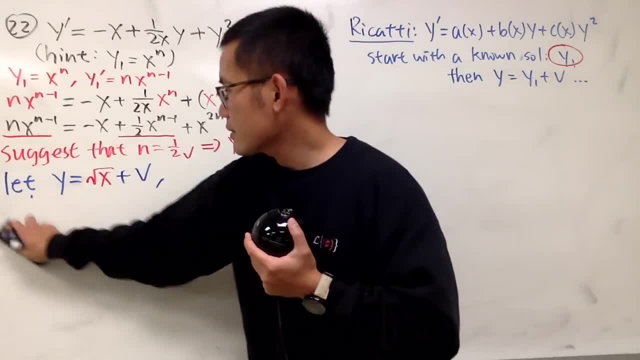 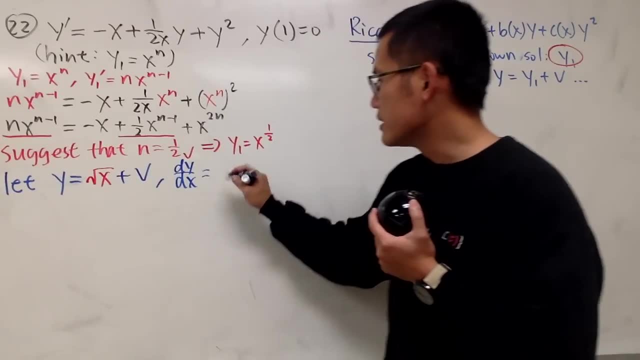 Get this and this is Sorry, sorry, sorry, sorry. I will differentiate this guy. I will get dy dx. That's equal to: The root of this is 1 over 2, square root of x, And differentiate this. 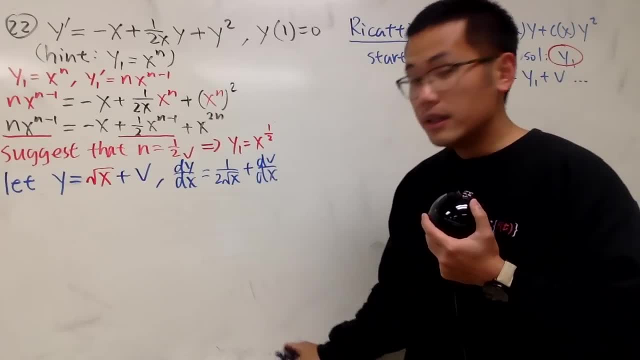 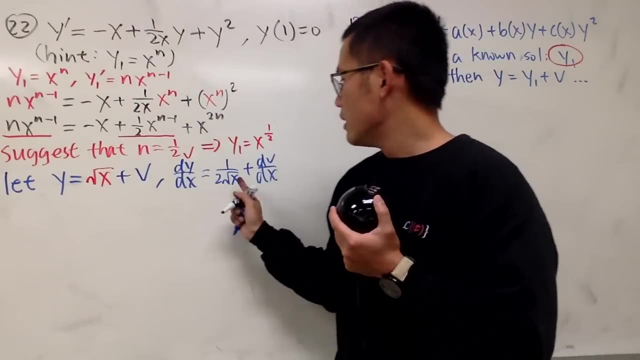 We get plus dv dx, Yeah, So now I can put this in here and put that in there and all that stuff. So have a look. First I will put this right here: We have 1 over 2 square root of x. 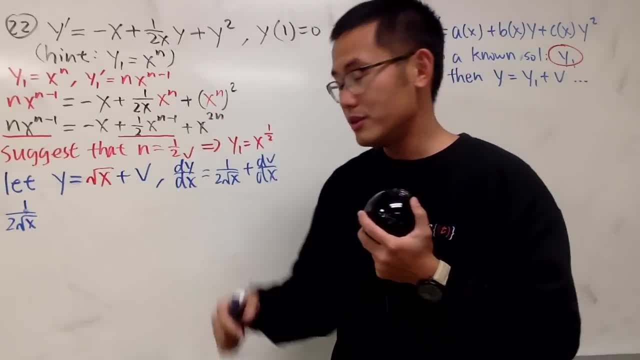 I can also show you guys how I create this equation. okay, If you want, let me know, And if you are still watching, let me know. Anyway, Plus dv dx, That's for that Y prime, of course, And then this is equal to negative x. 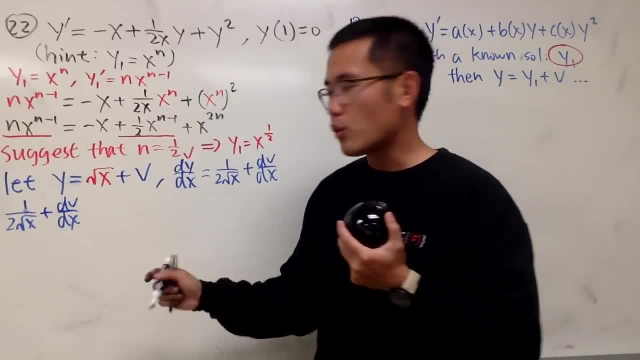 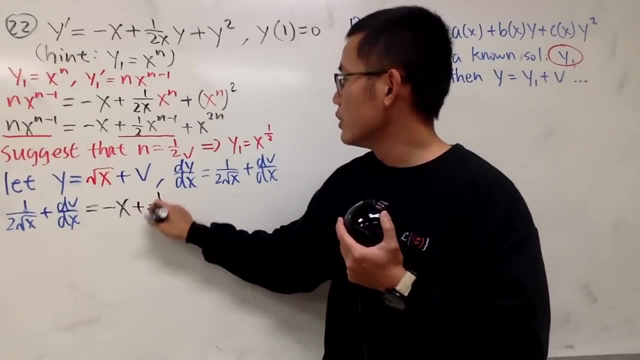 It's still negative. x Plus 1 over 2x, and the y is this. So I will just put that down right here: The y is square root of x plus v, And then, lastly, we have the v square, which is: 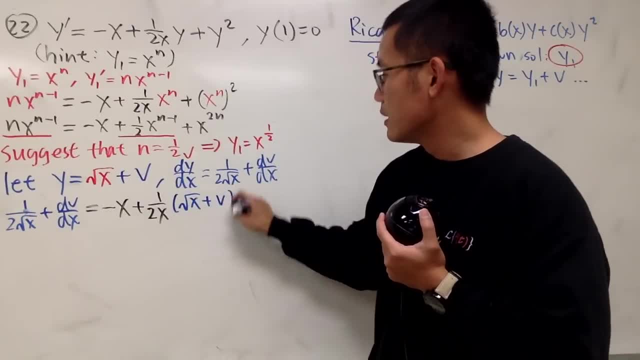 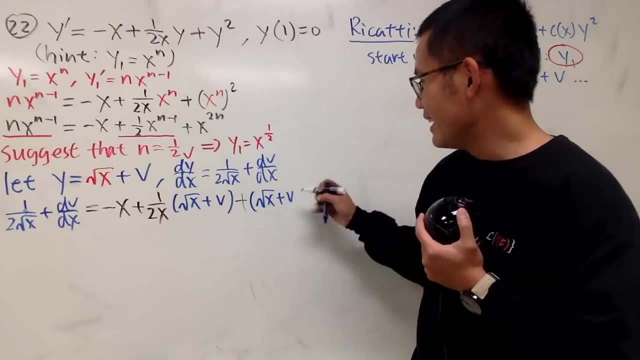 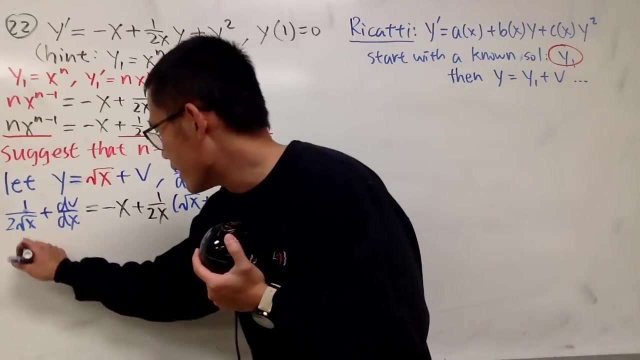 Square root of x plus v. So you know, this is the value square which is square root of x plus v, and then we square that. Okay, it's not so bad, we can handle it. Okay here, 1 over 2. square root of x plus dv. dx equals: 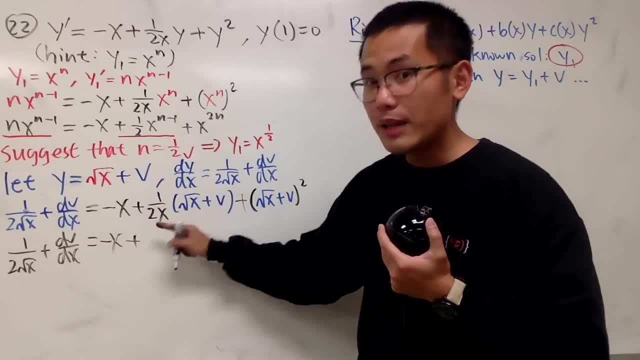 negative x and distribute this guy. okay, this over that. you still have the square root on the bottom, so you have 1 over 2 square root of x. Hey, look at that, they are the same. we can cancel. 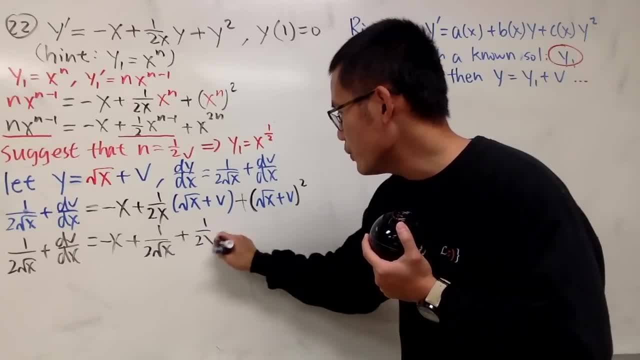 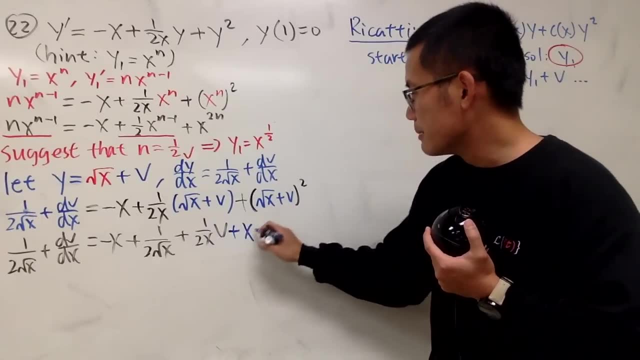 things out good: This and that plus 1 over 2x times v, and this, of course. just multiply this out, we get- I will show you this thing squared- which is x plus 2 times this and that which is. 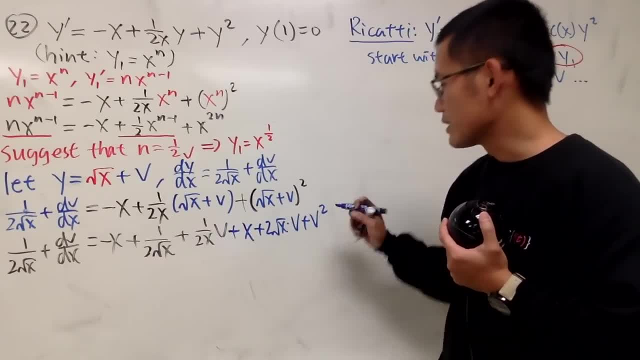 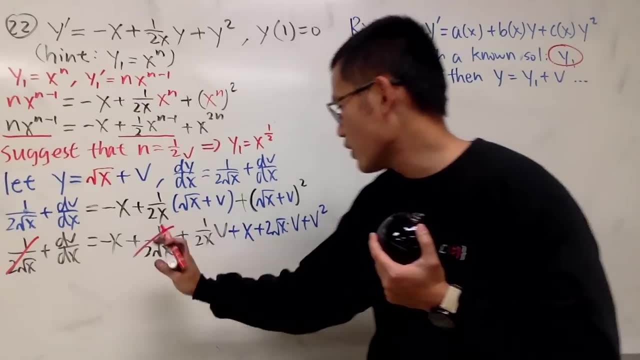 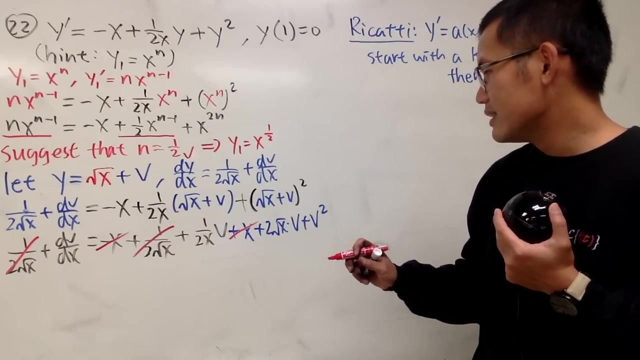 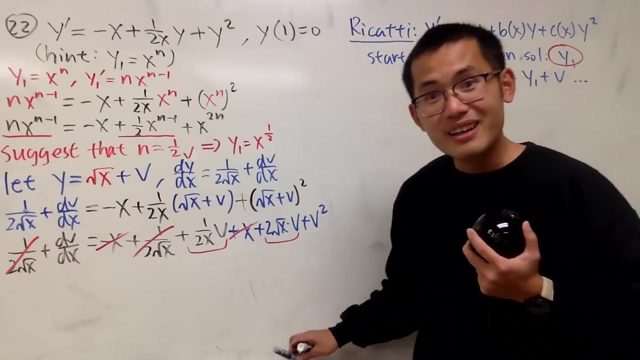 2 square root of x times v and then plus v, squared on our side like this: Very good Now, very good stuff, This and that cancel, negative x, positive x, cancel and uh, yeah, and then this and that, we can combine and we have the v squared This right here in v. 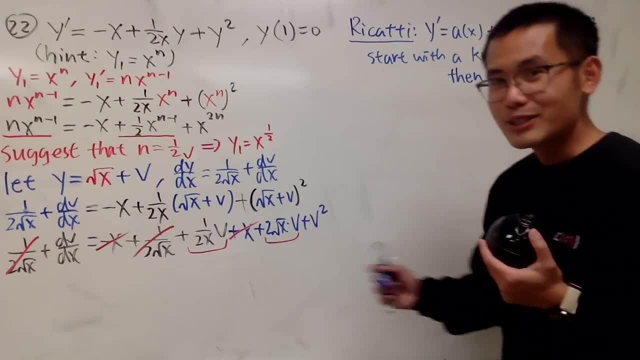 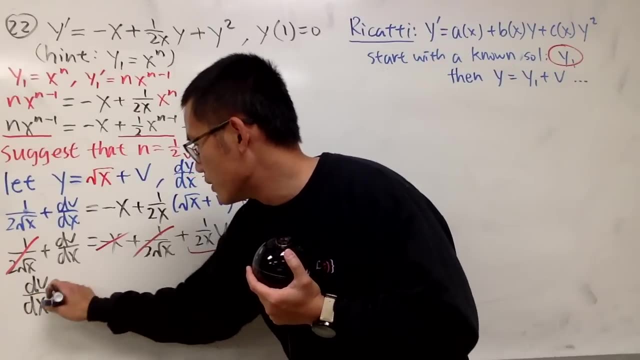 it's a Bernoulli's differential equation. that's why I have to save all the space. That's why I was so picky about all the space. Alright, now here I will just write it as: dv dx. I should have used 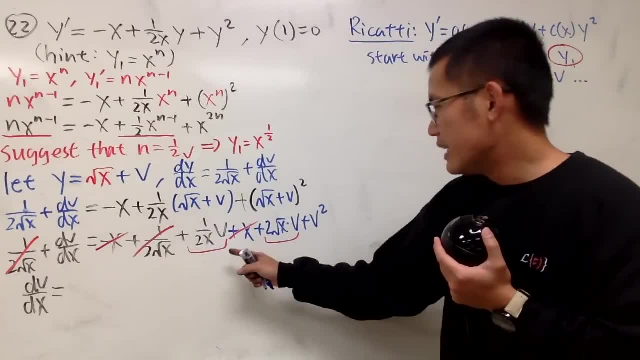 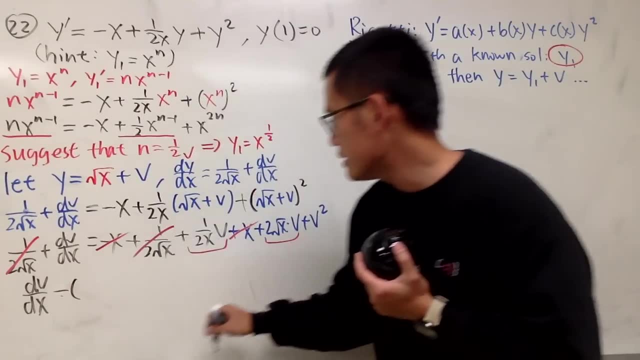 you god. but whatever, dv, dx and uh, this right here is this plus that, but you brought it to the other side, so let me actually make it minus parentheses, this and that. so I will just get 1 over 2x and then plus 2. 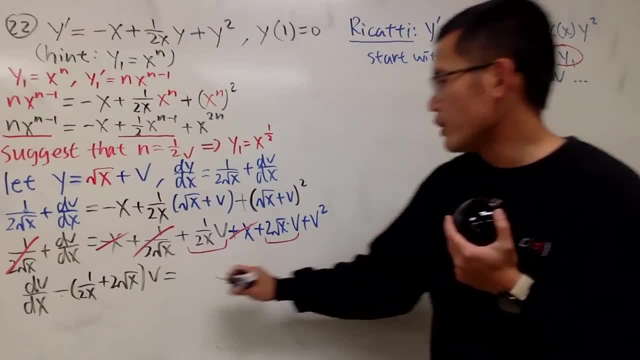 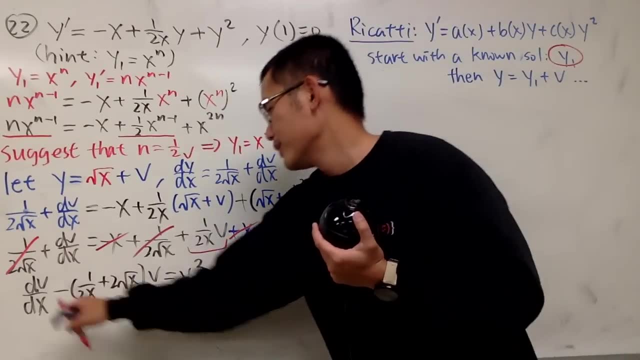 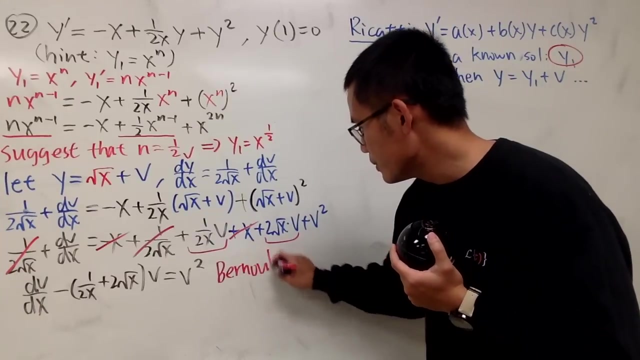 square root of x, and then v, and this is equal to v squared on the right-hand side. Yeah, just like that. Okay, look at this guy. Okay, Bernoulli's, now Ber-nu-li, So it's Riccati, and then 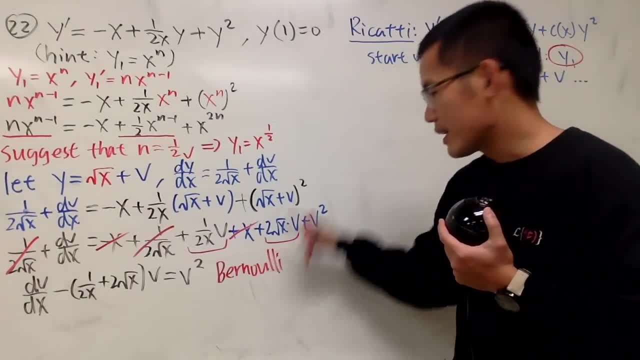 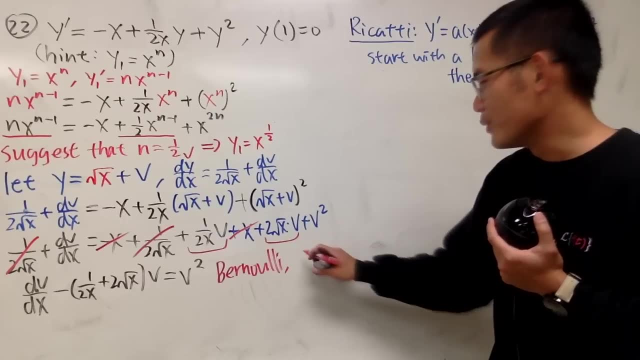 Bernoulli, They go together. What's the relationship? I have no idea. Alright, so here uh, I used v already, I don't use u, otherwise it would be too confusing. Let me use w- w is equal to v- and then I will do 1 minus. 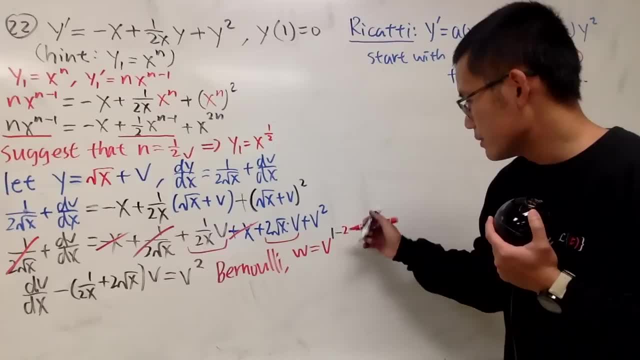 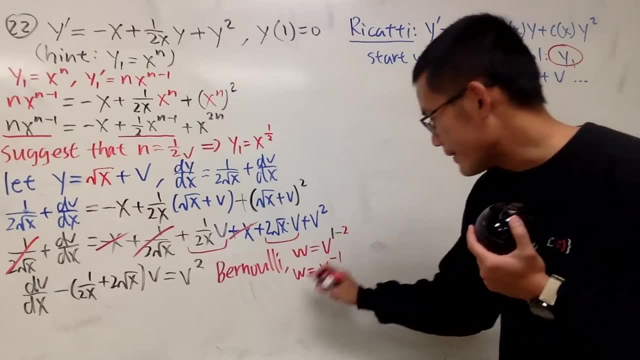 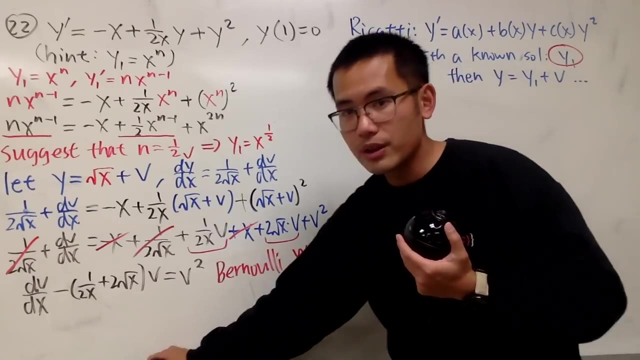 uh, that which is 1 minus 2, which is w, equals v to the negative 1 power, and I'll differentiate this right here, right now. so I'll get dw, d, d, x. Let me see, uh, how can I save more space? 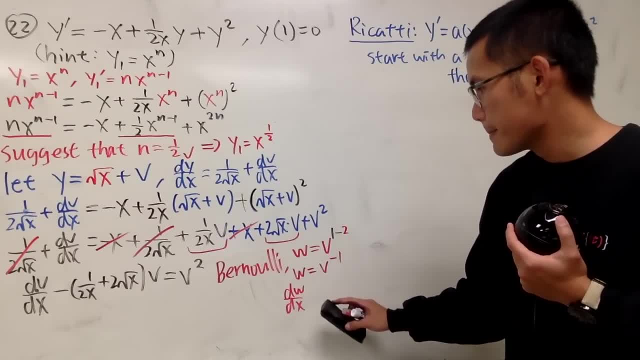 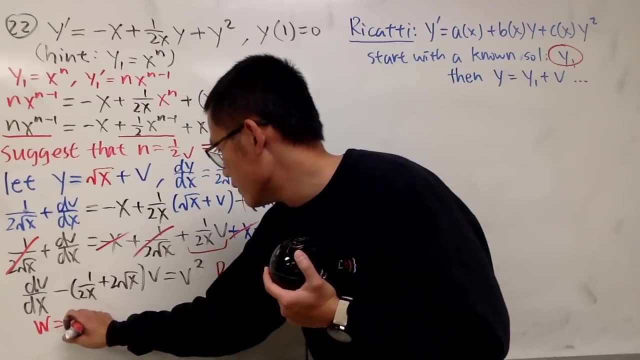 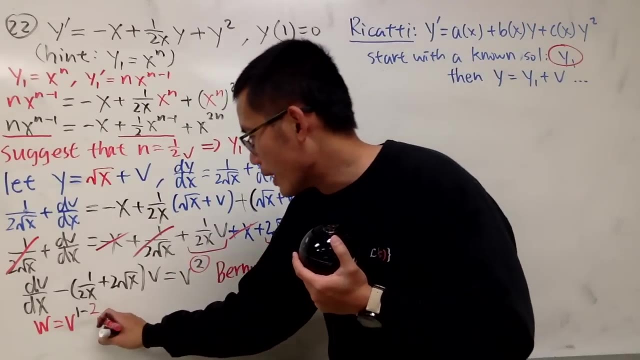 Uh, actually, you know what This is, Bernoulli. now I will write it down right here. It's actually better, So I'll do: w equals v 1 minus 2, right, This is 2.. And then, right here, this means w. 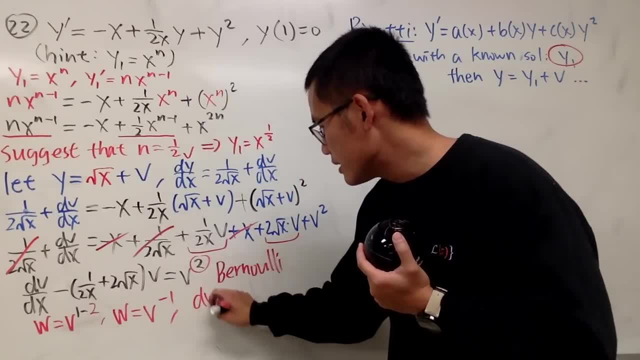 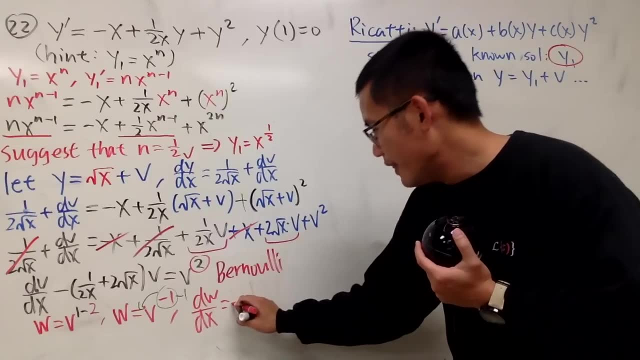 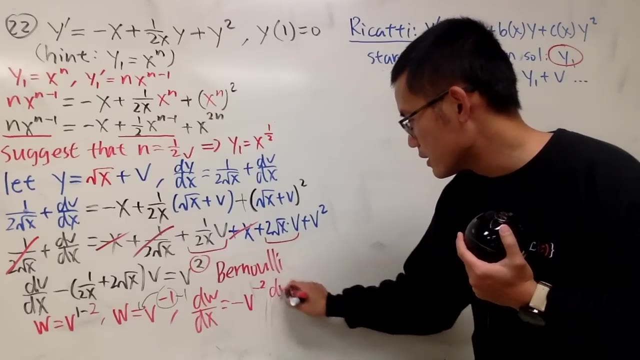 equals d to the negative 1.. This means dw over dx. equals. differentiate this guy, and I will make sure I bring the negative to the front. negative v, negative 2, and then we have dv, dx like this Amazing stuff. 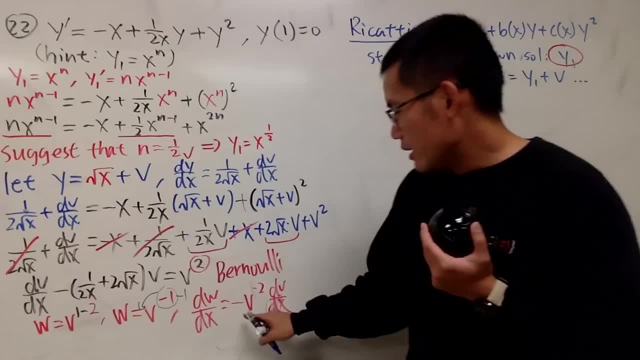 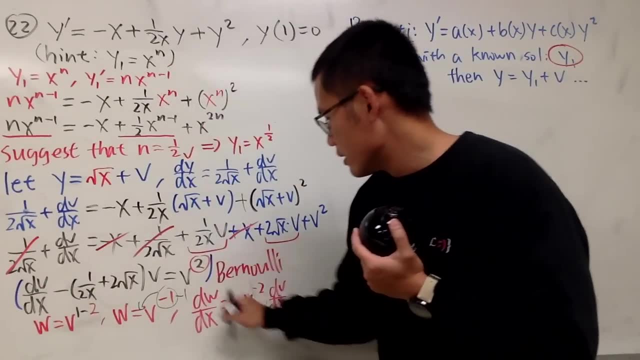 So that's what we have Now. here is the DO You see, we have dv dx, and in order for us to produce the dw dx, we should have this in front. So let's multiply everybody right here by negative v, squared like that. 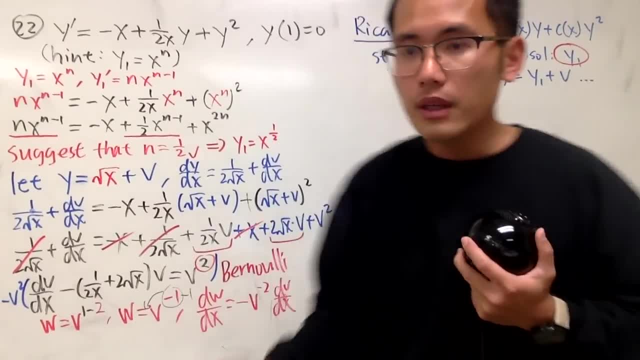 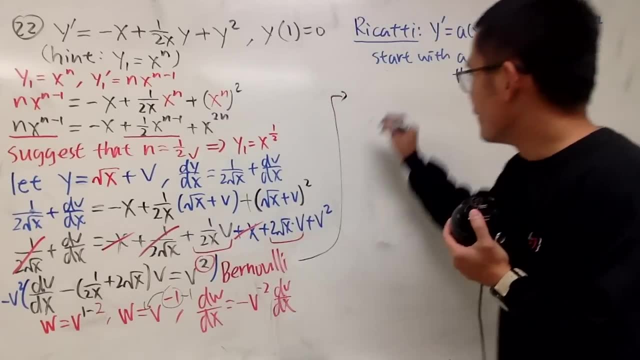 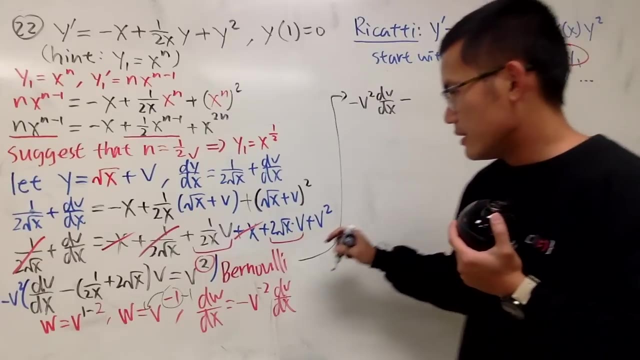 Negative v squared. That's a negative v squared. Okay, now I will go ahead and do the following. So pick this up right here. We have negative v squared: dv dx minus. okay, okay, okay, okay, okay. 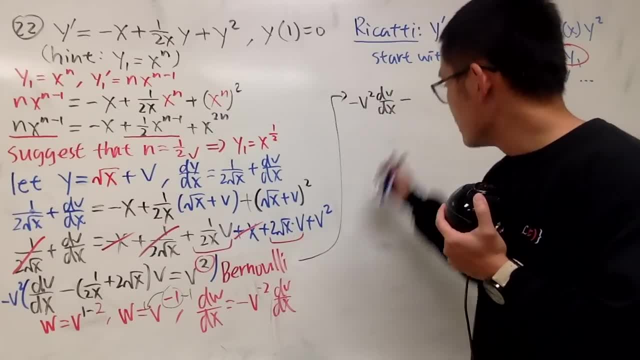 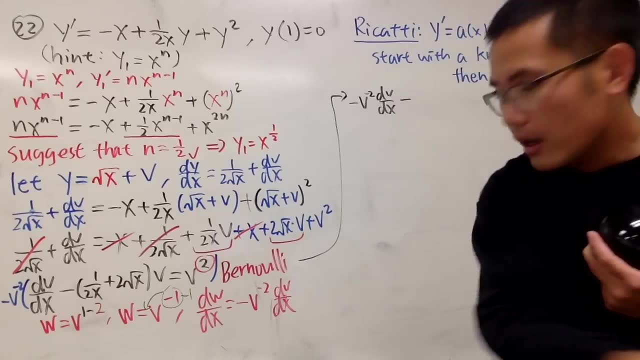 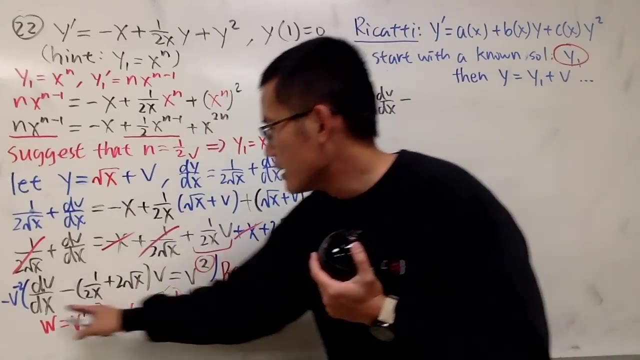 No, it's a negative v, negative 2.. Sorry, this should have been negative 2, and this is a negative v, negative 2,. okay, So it could help. Alright, multiply everybody by this guy, So we have this right here and next. we do this times that. 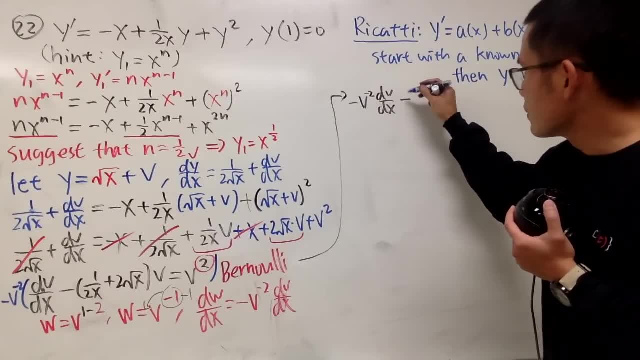 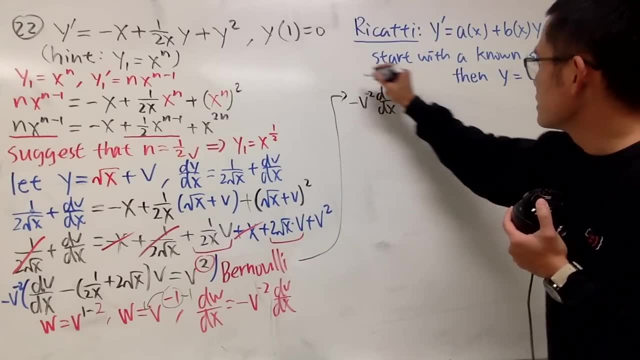 and you see, negative, negative becomes positive. so just bring that down, become positive, and then the x part stays. I'll just make it. I'll just make it keep it, stay, and then just make sure I have all the stuff right here. 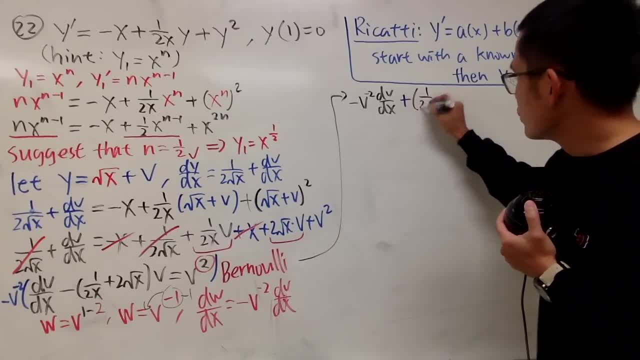 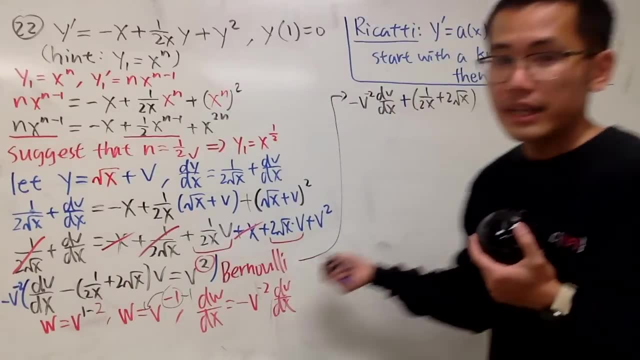 We have 1 over 2x plus 2 square root of x, and then v times v to the negative 2 is v to the negative 1, so we have v to the negative 1, and this is equal to what. 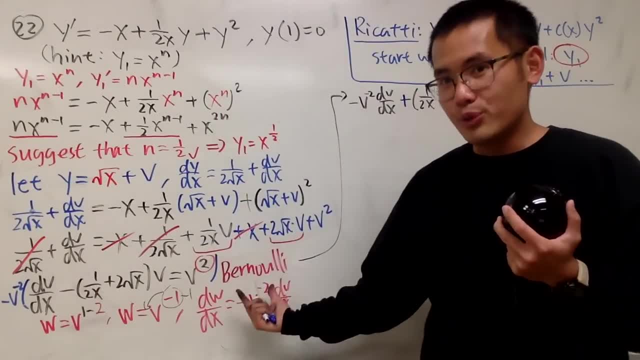 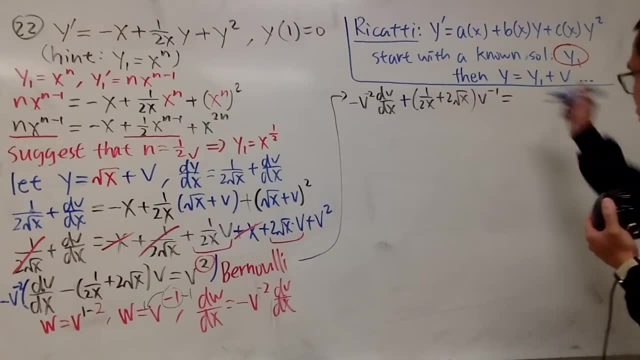 Guess what This times that they cancel. that's the genius Bernoulli. I explained that earlier, like three, four hours ago, and don't forget. we still have the negative right here, Negative, negative. okay, So this right here on the right-hand side is equal to negative 1.. 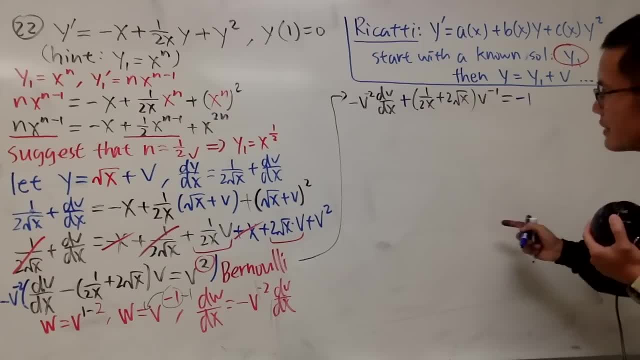 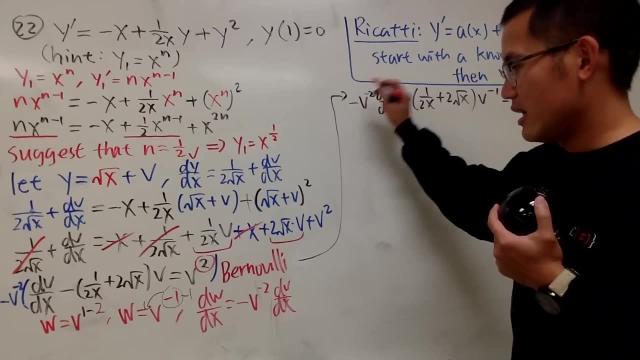 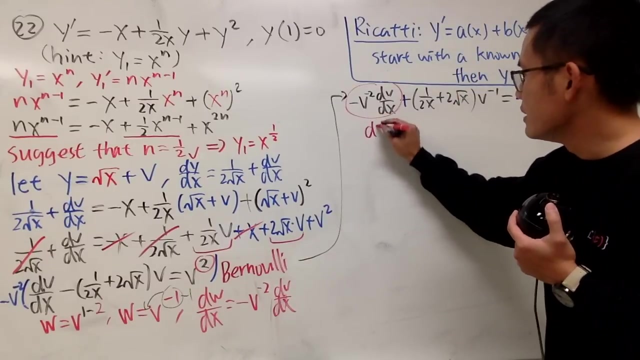 Uh good, Now, ha-ha-ha-ha-ha-ha-ha-ha-ha, wah-ha-ha-ha. this part is what? This is precisely our dw dx. So this right here is that I'll just write down dw dx. 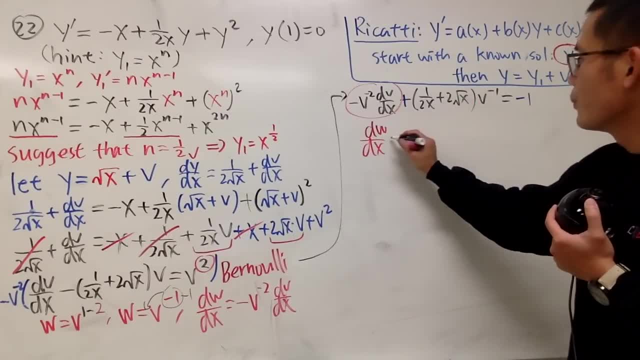 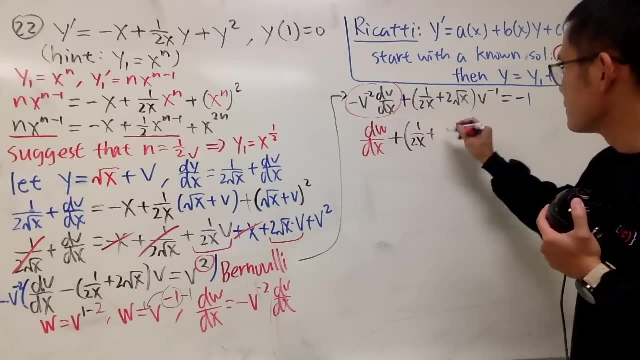 and then for this part, well, we don't have anything. I'll just write this as 1 over 2x plus 2 square root of x, and then the phi to a negative 1, well, this guy is precisely our w. 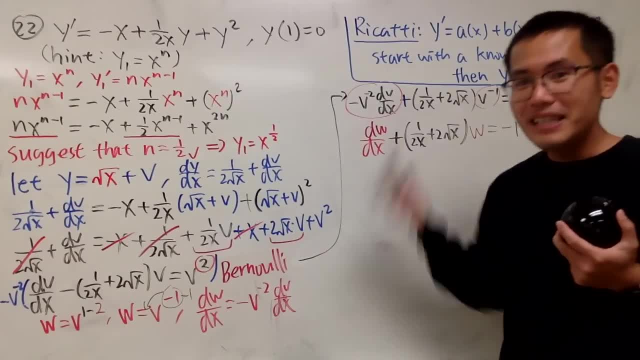 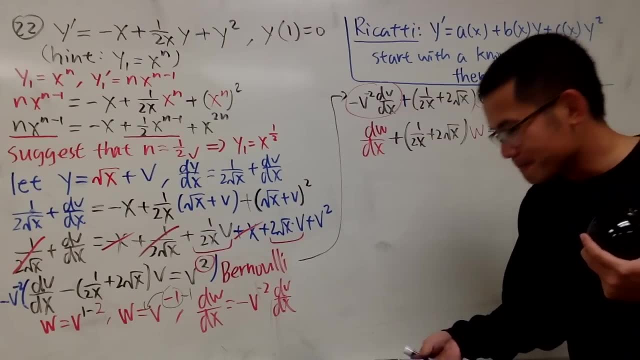 And that's equal to negative 1.. And guess what? This becomes a linear God. how many times do we have to substitute this guy? I don't know, man, But anyway, what do we do? What do we do? 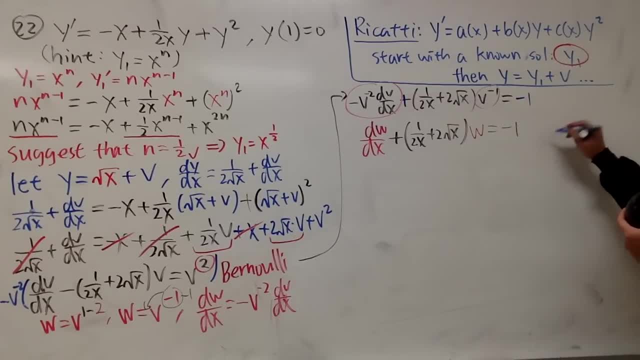 Integrating factor, right, Linear integrating factor. So let's go ahead and do that. So right here I will just do mu of x, That's equal to e integral power. And then we have this guy which is 1 half x. 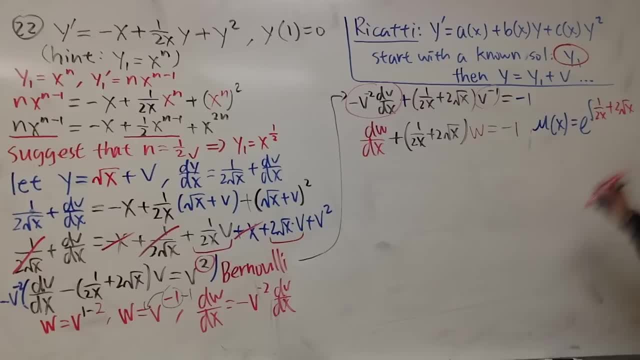 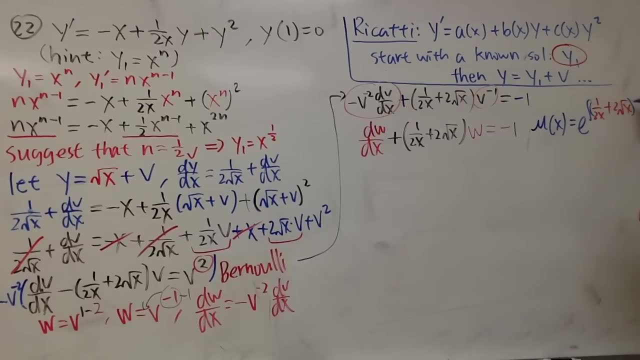 And then plus 2 square root of x, Yeah, and then maybe you guys cannot really see it, And then I'll just have to squeeze in a little dx just to be legitimate. Can we see it? That's a dx, right. 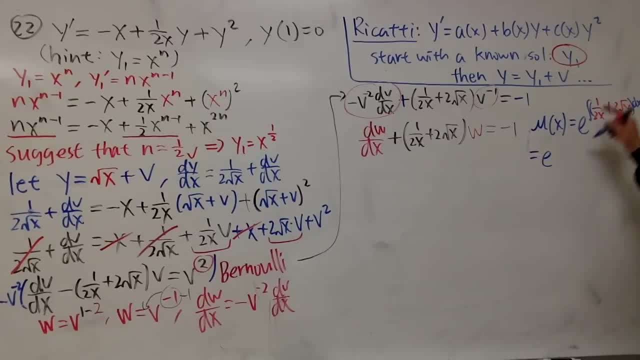 So now, anyway, this right here is going to be e 1 half stays And you have natural log of x And I explained that a lot of times already, so I'm not going to tell you enough to put, but I just did. 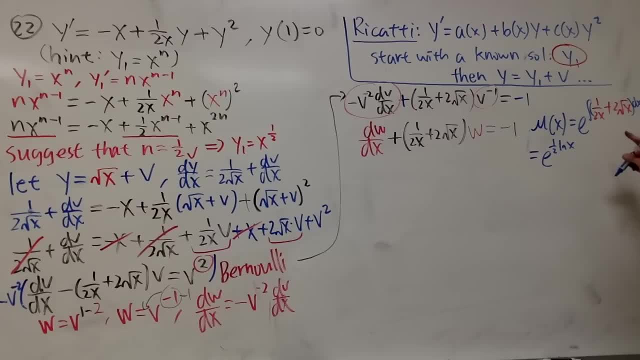 Don't put the f's before you, Don't worry about the plus c. And then this right here: integrating 2 square root of x. yeah, This right here is the same as saying integrating this as 1 half power. You add 1, which is 3 half. 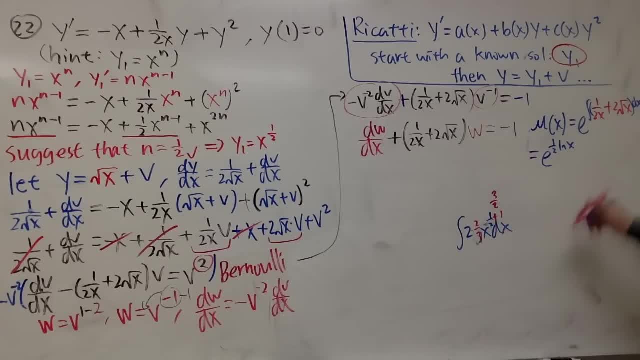 and divide it by that, so it's 2 over 3, like this: yeah, So you get plus 4 over 3.. And then you have x to the 3 over 2.. Just like that, okay, Just like that. 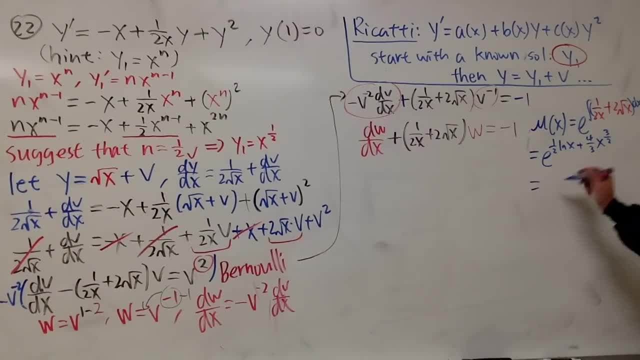 Some crazy stuff I know. Now break this apart. First you bring this up here and then you have e, ln x to the 1 half power, And then this is adding in the exponent, so you can just multiply e to this power. 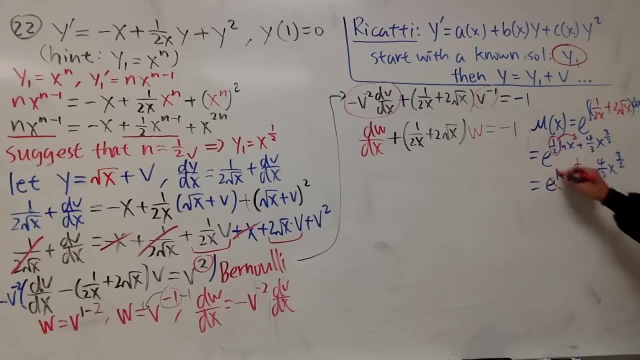 4 over 3, x to the 3 over 2.. This and that cancel. This is square root. so we have just the square root of x times all that: e, 4 over 3, x to the 3 over 2.. 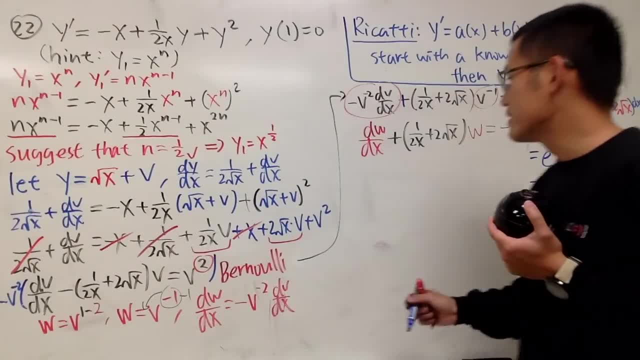 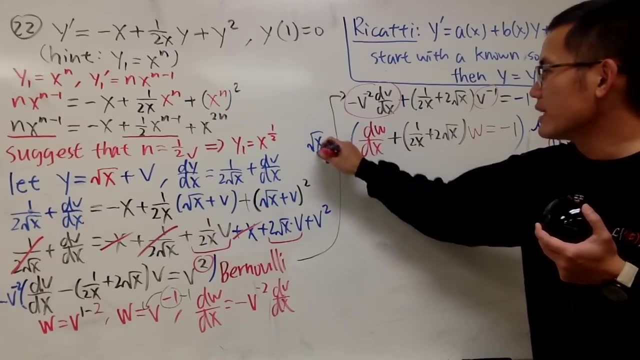 All right. So this, right here, it's an integrating factor. Crazy stuff. Now multiply every party by this guy which is right here, square root of x, e, and then we have 3 over 4, x to the 3 over 2.. 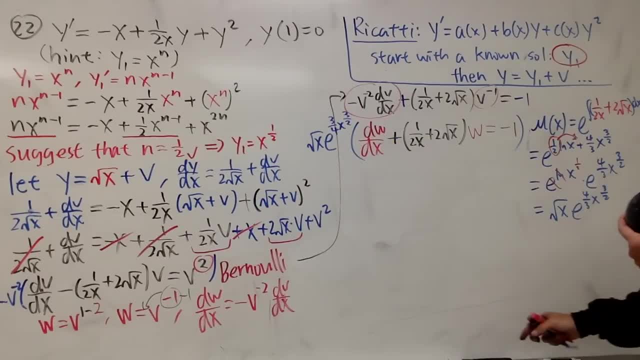 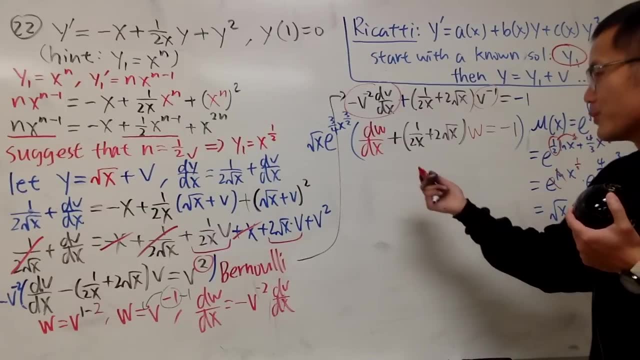 Like this. okay, So now, as I said, I will try to fit in everything, because this is going to be the most satisfying Man. some space, actually. Oh, what a bad. This times this. Now do this in your head, yeah. 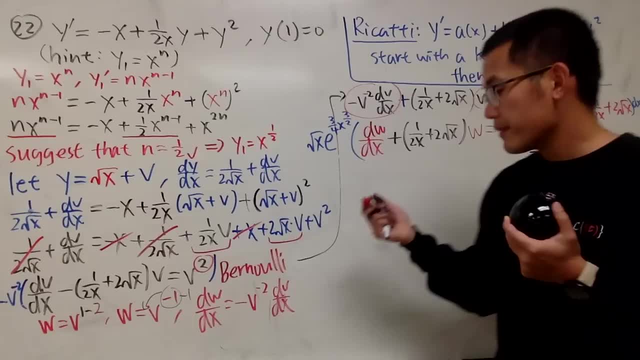 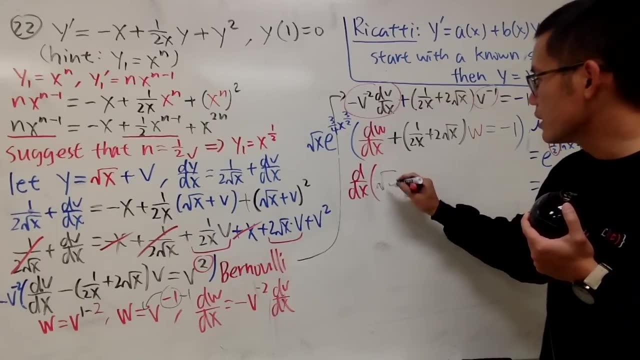 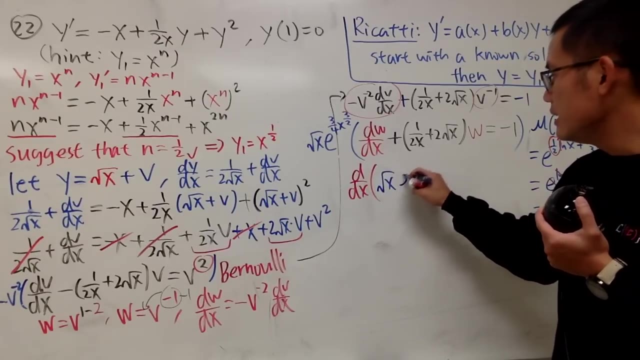 This times, this, this times, this is going to give you the derivative of a product of the linear integrating factor, which is the square root of. Let me just Which is that, I'll just write it down better: Square root of x, e to the 3 over 4,. 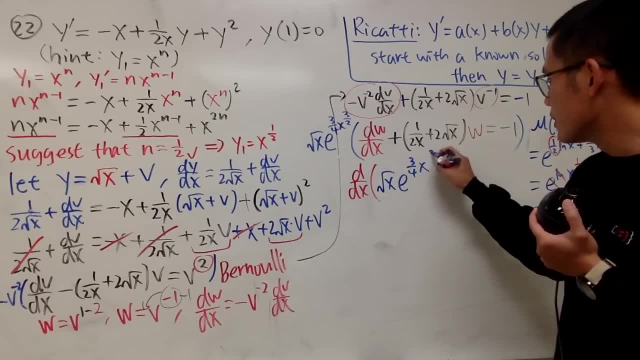 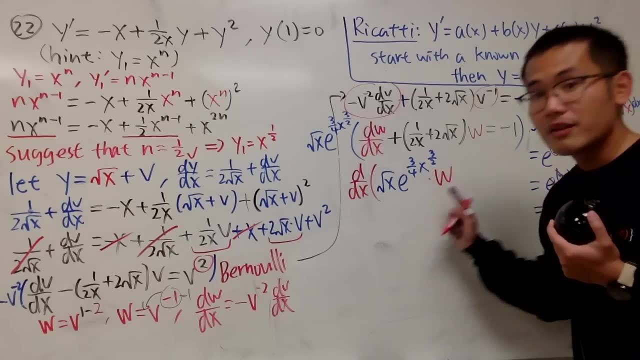 x to the 3 over 2.. Yeah, So we've done this so many times already. and then we are going to multiply by w, so the product of these two functions- and I know this is also a product, But then you do this times that- 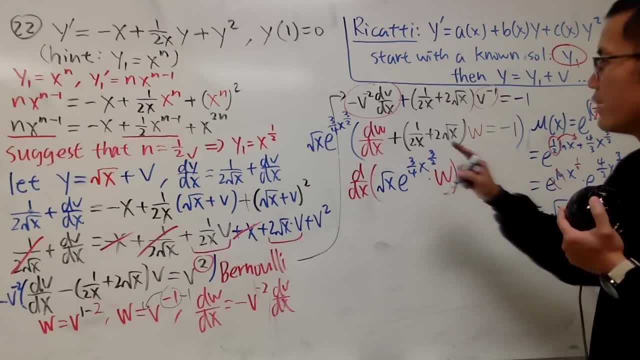 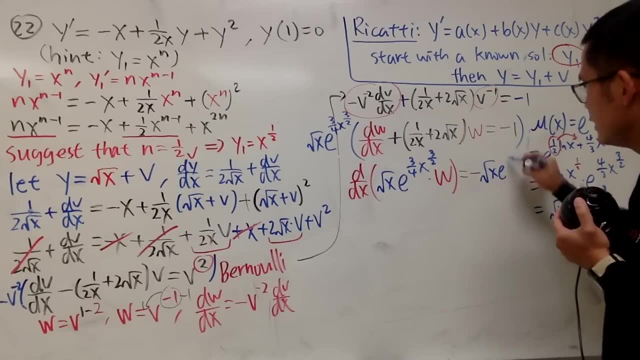 so be really careful. Here we have negative and then you have, Uh, The square, All that stuff, Square root of x, e to the 3 over 4, x to the 3 over 2.. Right, So not so bad, not so bad. 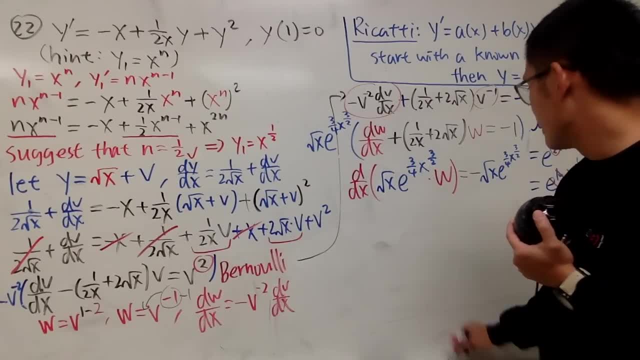 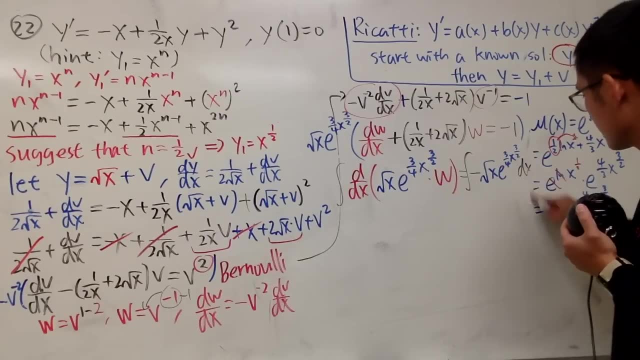 Now, as usual, you integrate both sides, So you're going to just integrate this, integrate that, dx this Right. So this and that, cancel, Very nice. And you're going to just do a few things in your head. 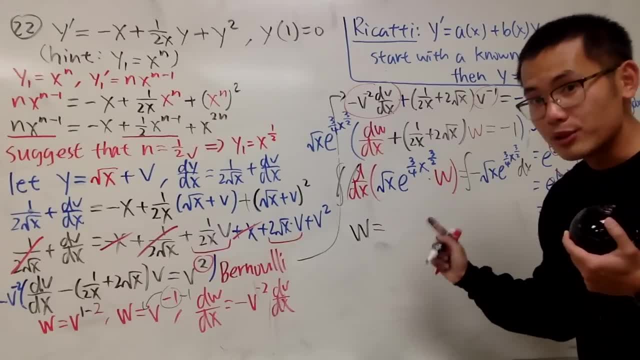 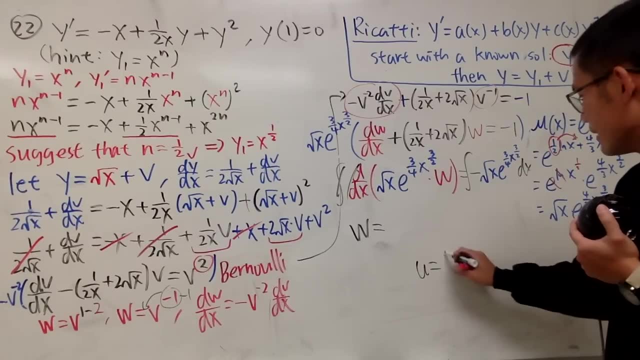 w, it's going to be the following: right w is going to be the following: Integrating this, guess what You can do. u sub Let u equal to 3 over 4, x to the 3 over 2.. 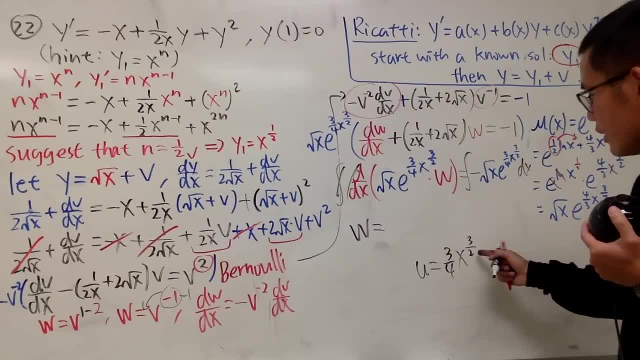 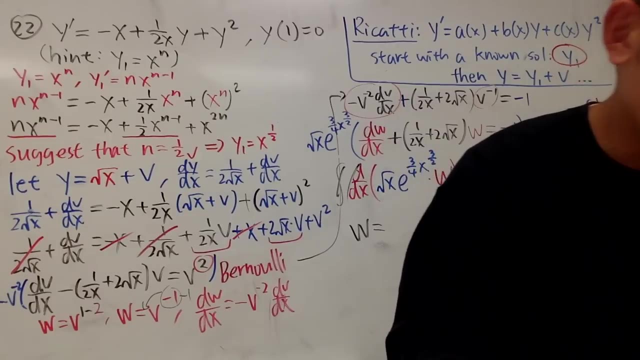 Yeah, And when you integrate, when you differentiate this guy, you bring that to the front, so you get du equal to 9 over 8.. Okay, So I have the 3 over 4.. Let me just double check it before I continue to. 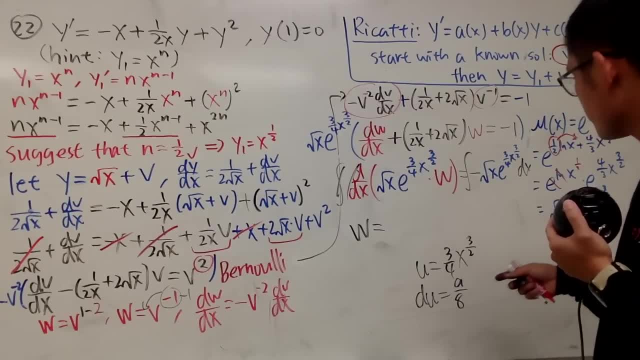 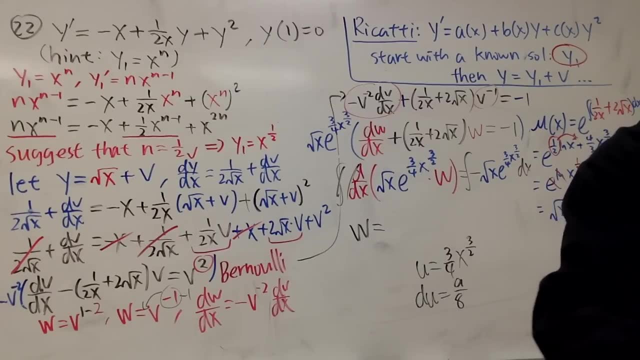 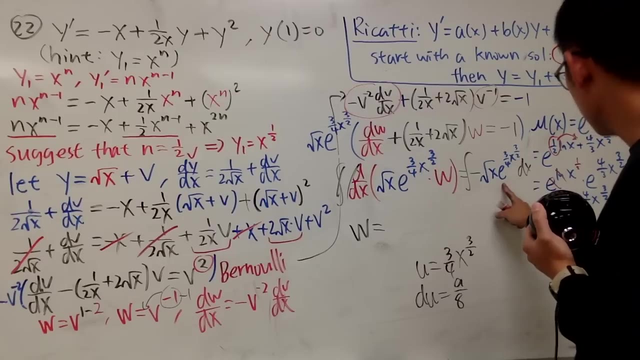 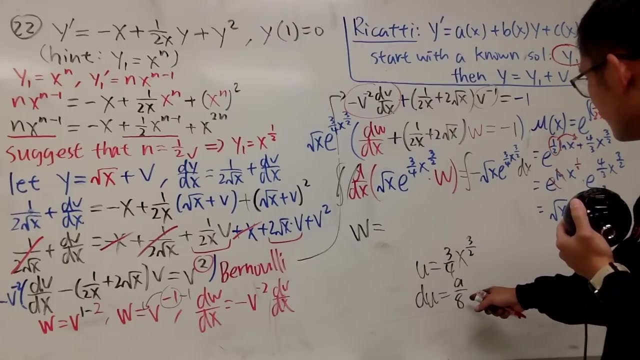 So far, so good. Yeah. And then if you differentiate this guy, I get this. and then Let's see, I have to integrate this guy. And if I integrate this guy I will get this ugly number Seriously 9 over 8, and then x to the 1 over 2.. 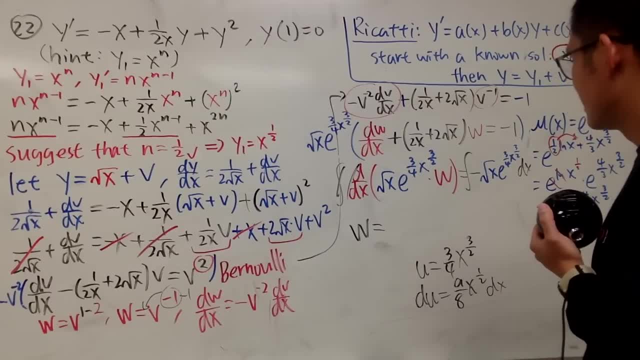 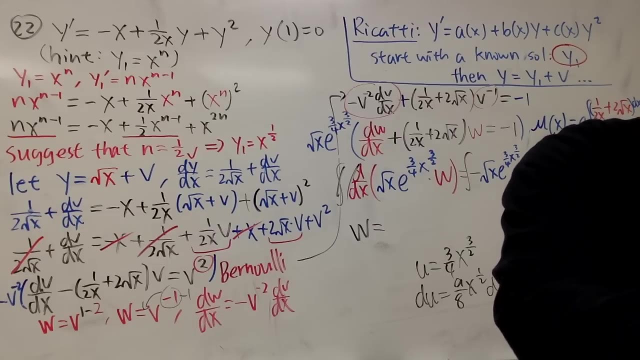 So we end up with 9 over 8.. That's not. That doesn't look right. Oh, I do have initial condition, So maybe that's why, Oh God, Ha, ha, ha, ha, Okay, okay, okay, okay. 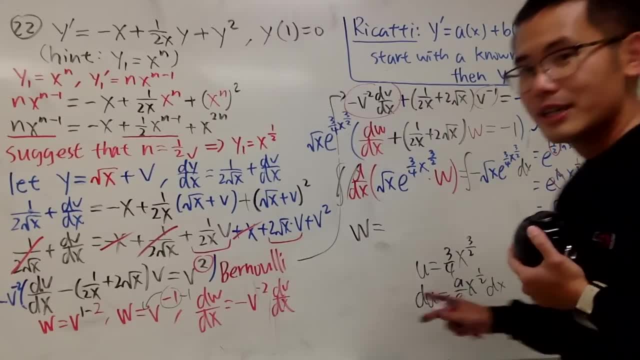 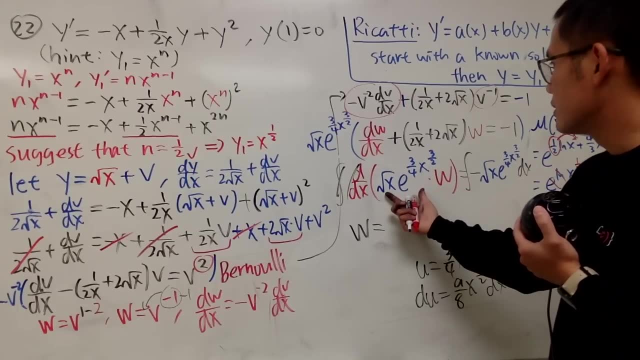 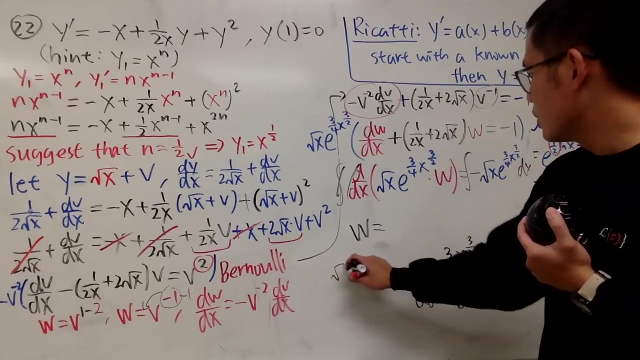 Just let me triple check, because this right here it's not a joke. So let me triple check. Okay, If I differentiate this, it's the linear factor, right, If I differentiate this first function, Okay. Square root of x. 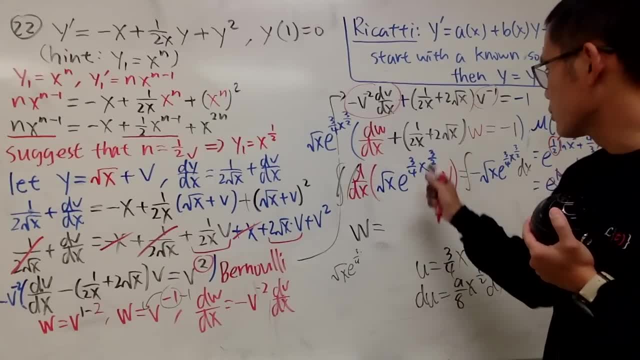 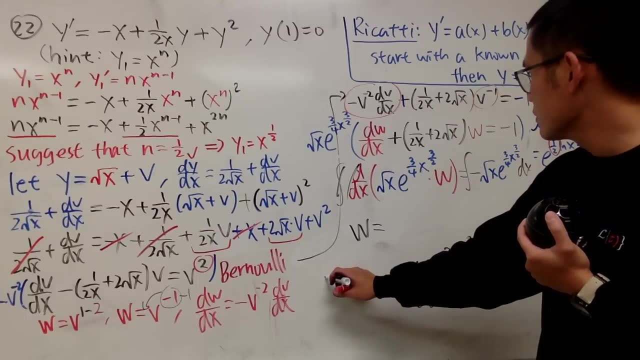 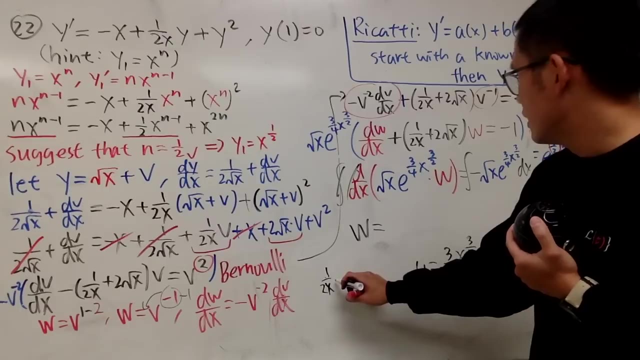 4. It's the first function times the second. That's right. So the second times the derivative of the first. If it's the derivative of the first, I will see this is 2x. No, no, no. 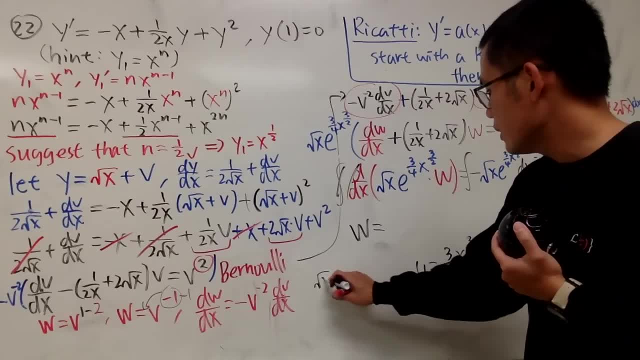 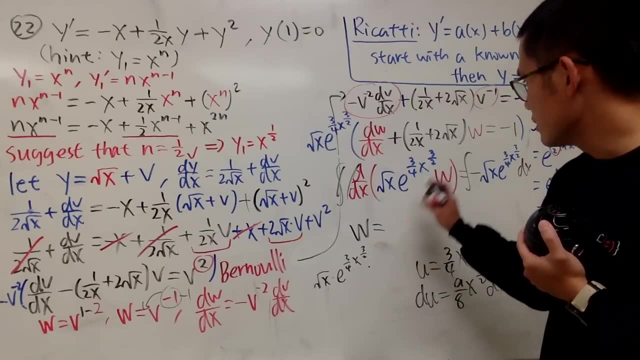 I'm going to do the derivative of this right here, which is square root of x times e3 over 4x to the 3 over 2 times. I don't think it's right Times the derivative of this, which is: 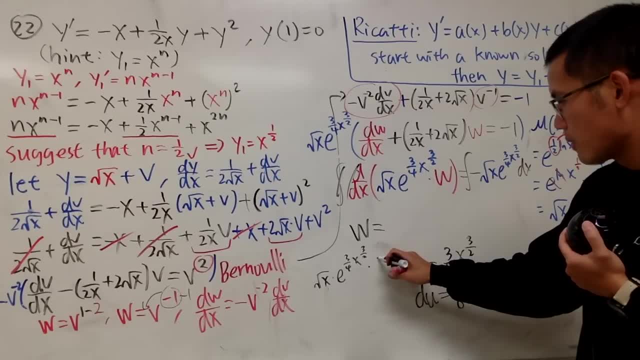 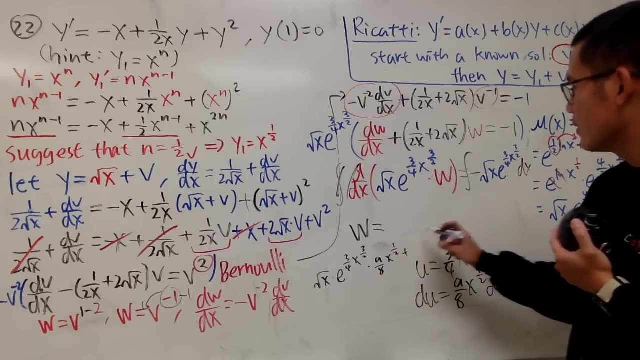 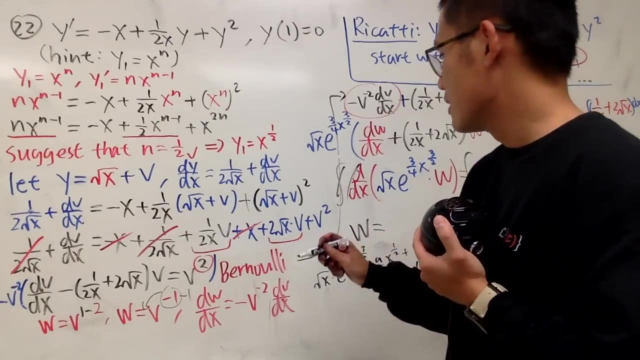 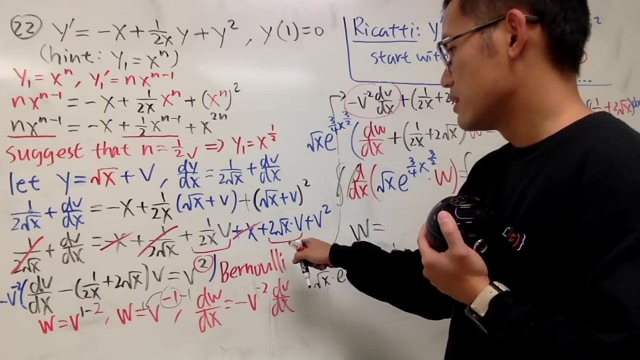 9 over 8x to the 1 half. And then, Yeah, Uh-oh, Let me see, Let me see I have the 2x. Uh-oh, I'll do it again. Everything is right, I believe. 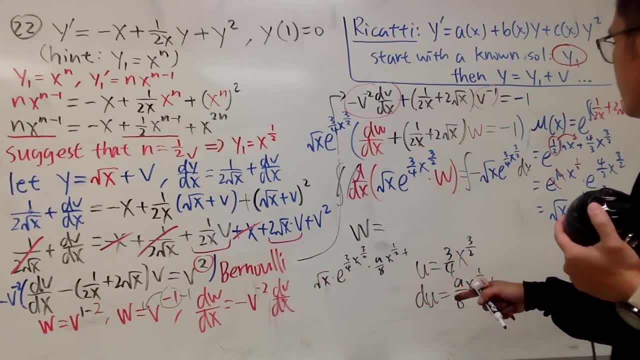 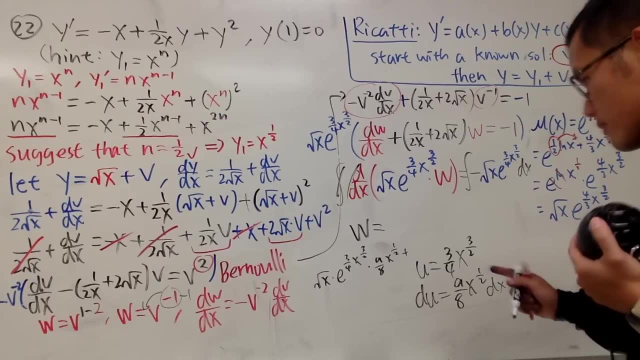 Yeah, Okay, Now it's like this, I can do it like this. Yeah, like this. Uh, Like this. It's like this. It's like this. Now I can do it like this. It's like this. 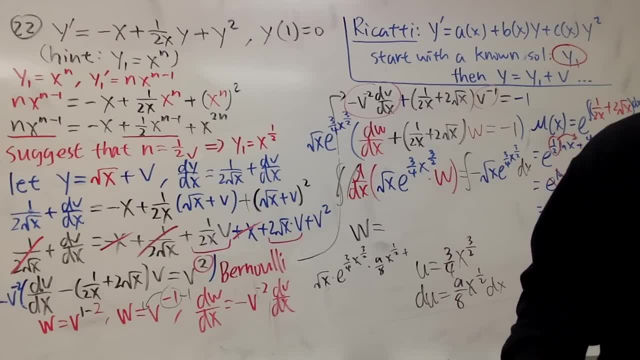 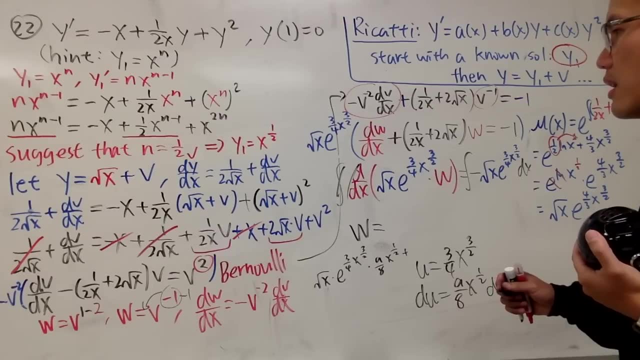 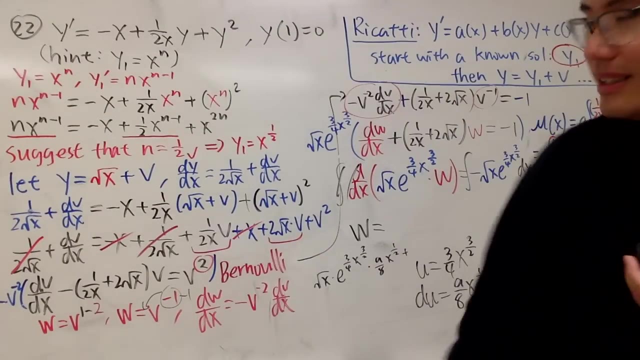 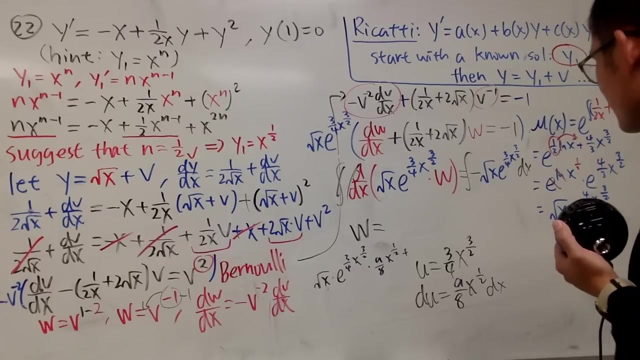 Yeah. Now If it's 0,, 1,, 1, yeah, I only have the answer key, right, Just so? you guys don't have the answer key And I don't know where it is, Unless this is right, and then I just don't see. 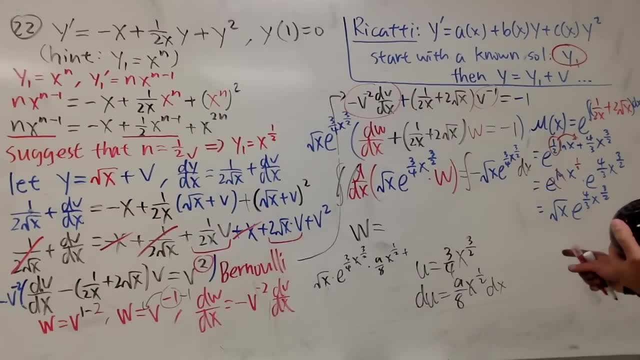 I don't see the integrity part is right. Let me triple check again. I have a 2., 2, and then So it's x to the 1 half, So it's 3 over 2. Has to be right. 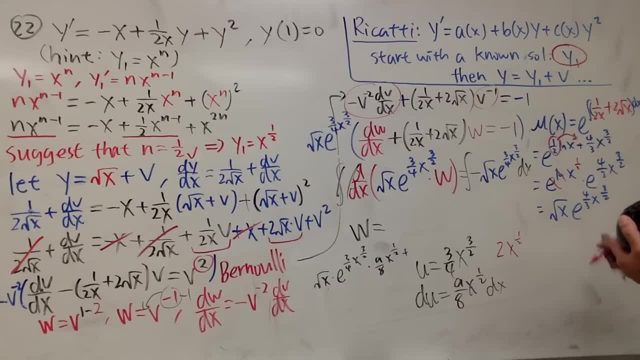 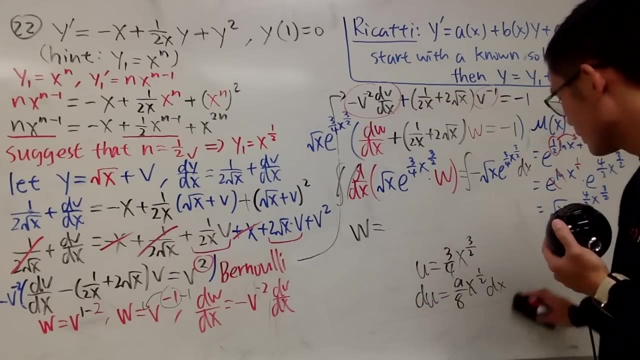 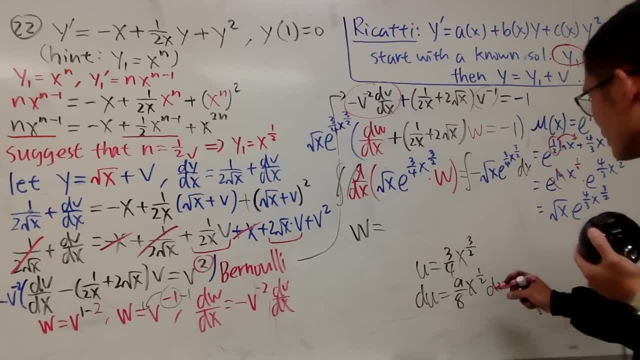 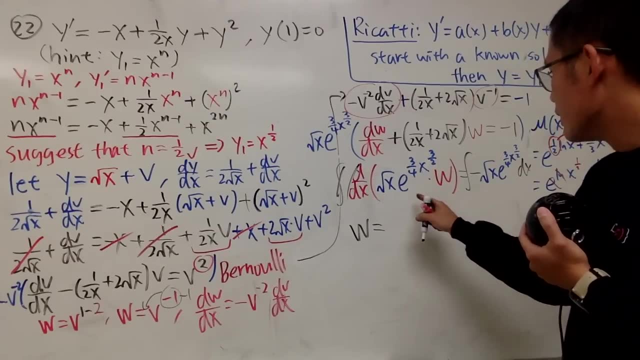 Hopefully it's right. Okay, So I will just go ahead and continue then, But hold on, hold on, hold on. Let me just see, let me just see Right here if I do the product rule right. So it's the second function times, the derivative first. 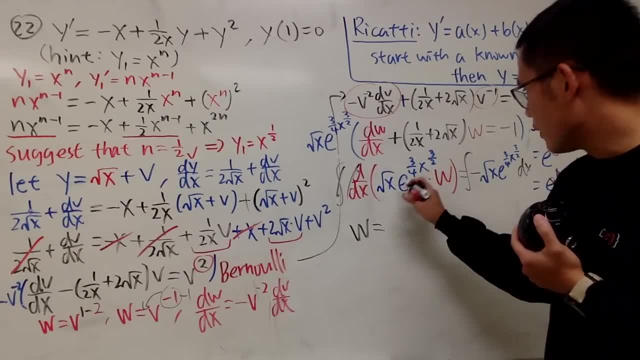 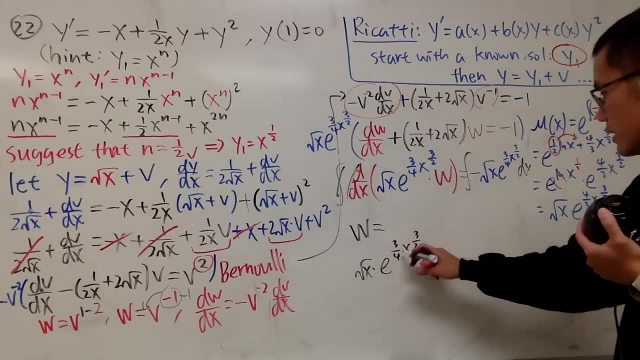 Do I get this times that? So let me just do this real quick. The derivative of this guy is square root of x times e3 over 4x, to the 3 over 2 times the derivative of that, which is 9 over 8.. 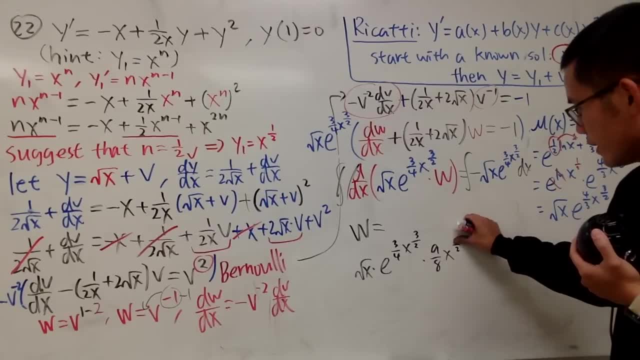 x to the 3 over 2.. No 9 over 8.. x to the 1 over. yeah, like this. And then I add the second function, which is this: e3 over 4x to the 3 over 2 times the derivative of the first, which is 1 over 2.. 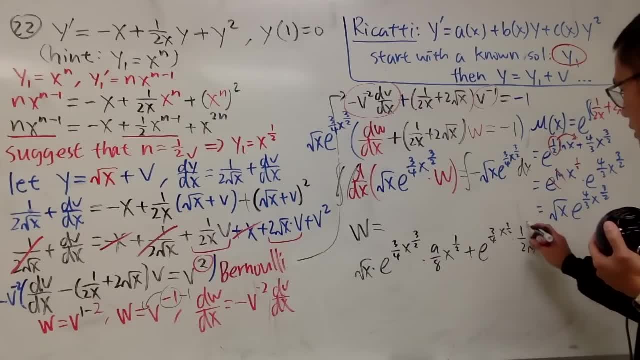 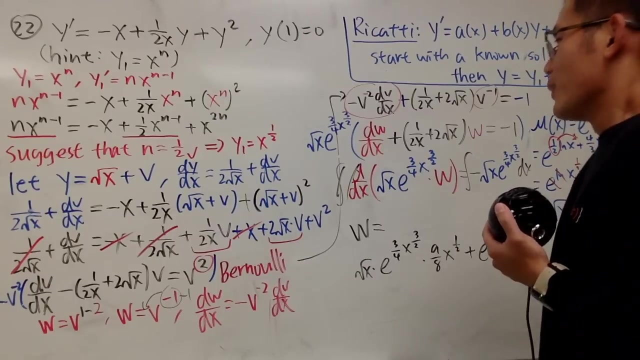 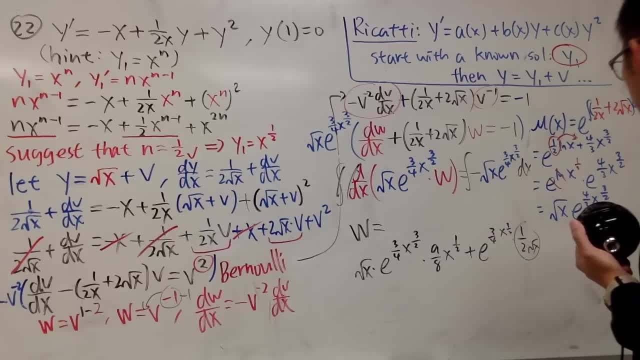 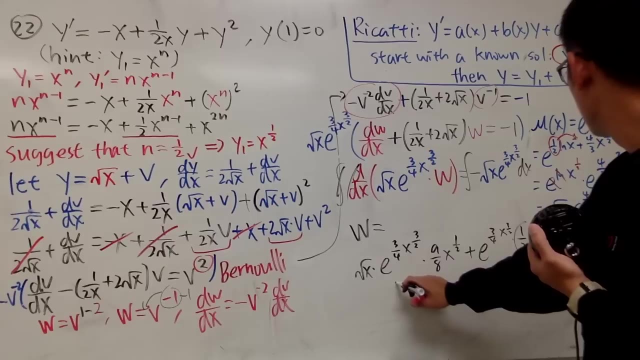 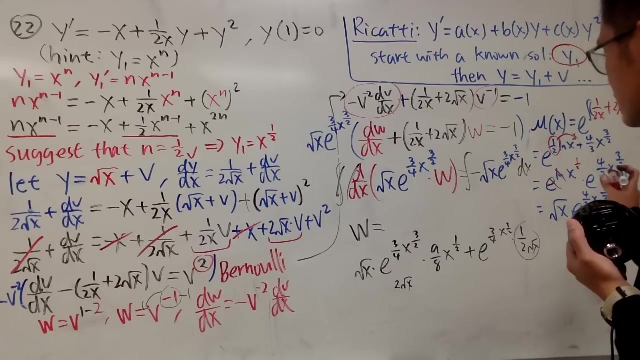 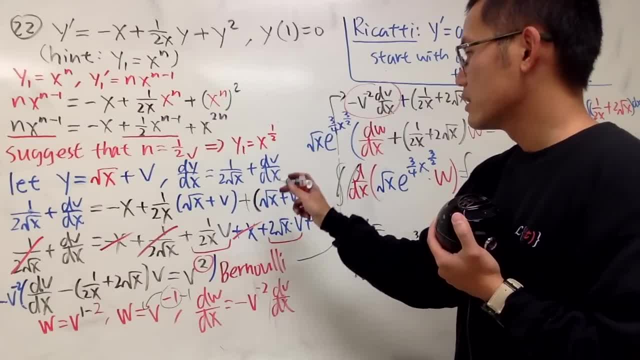 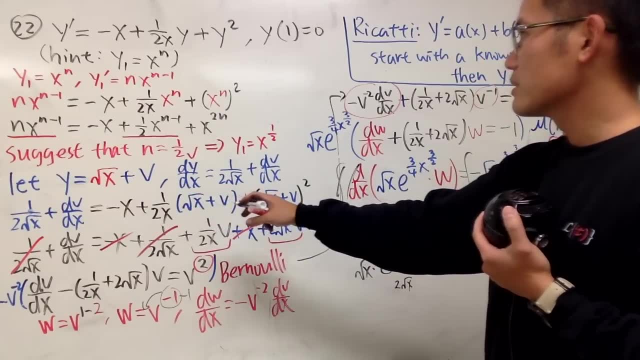 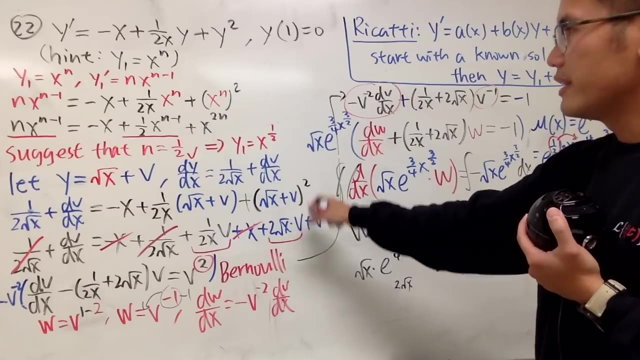 x is 1 over half. that's right. So that's right. then put that back there and that's right, minus25.. Okay, Okay, Thank you. So the purpose is to stop for v and then you put that back and then it's y1 plus v, that's all. 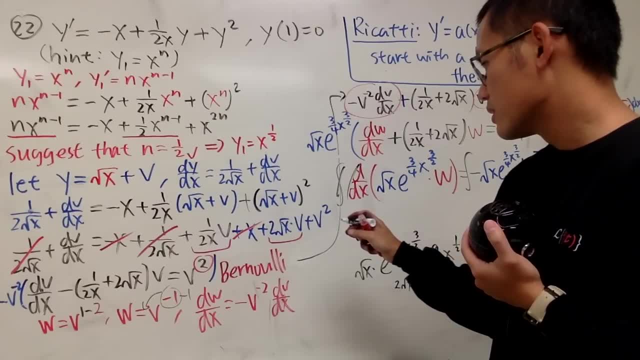 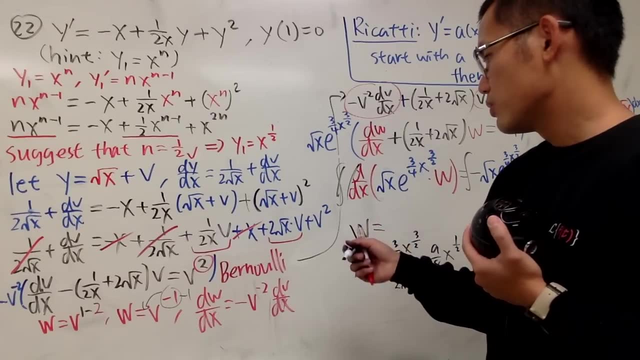 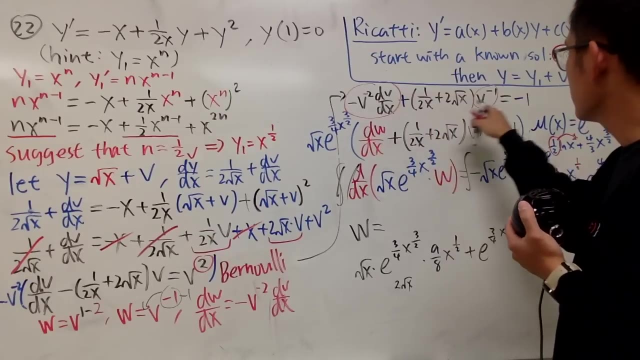 So now I just have to focus and then just get a right answer. You should be right. So this is negative and negative times. that is positive and all that is negative. 1. Good, Okay, one thing is wrong For sure. I don't know. 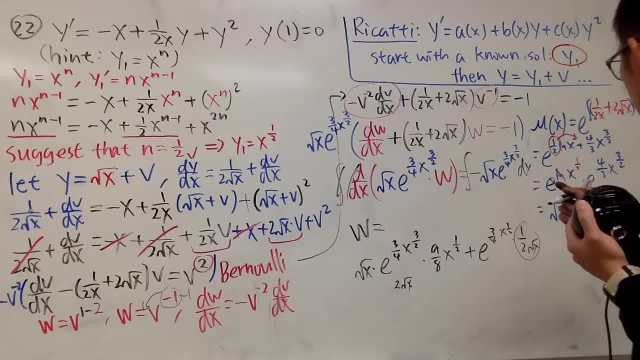 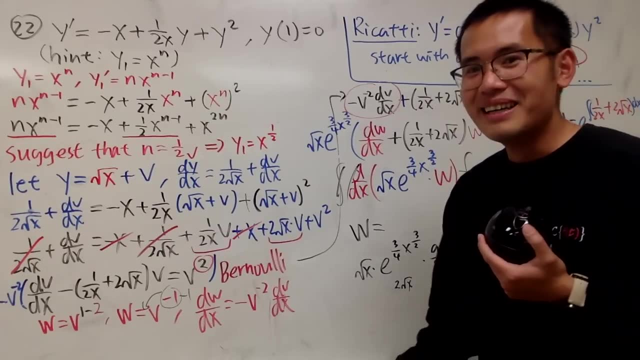 Or maybe I'm just tired. Oh my god. Oh my god. Oh my god, Nothing wrong, I just already done wrong. I'm so sorry. Okay, so this right here. I put it as e to the 4 over 3.. 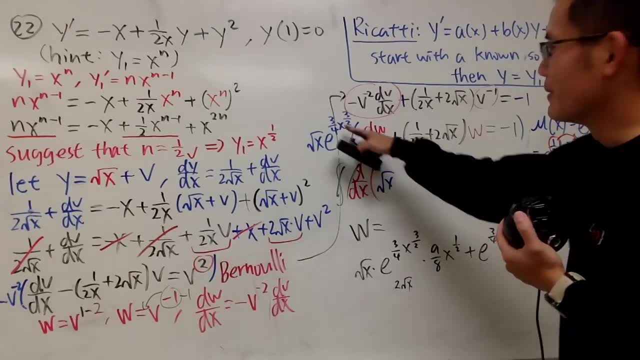 And then I screw up so badly. Right here I put it as 3 over 4, that's why I said, ah, something's wrong. Anyway, Okay. So it's not a major mistake, right? So just chill everybody. 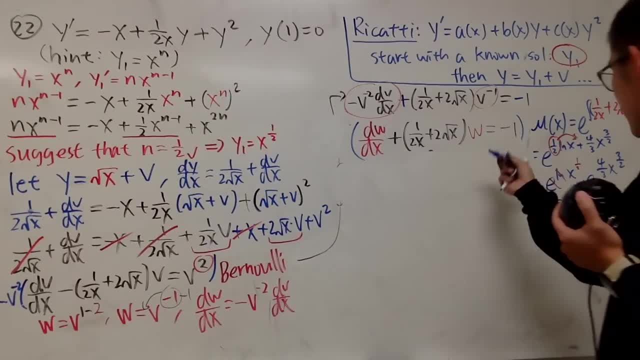 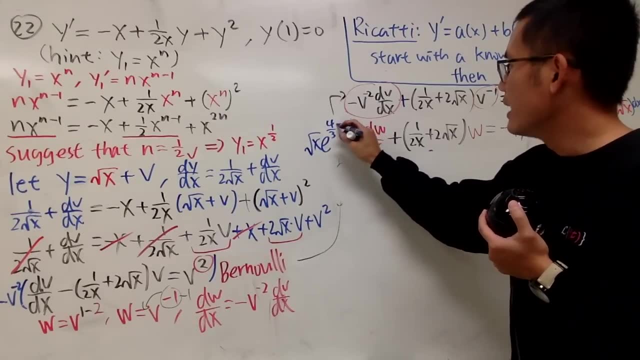 Chill, chill, chill, chill, chill, All right. So this, right here, is our integrating factor. Let's multiply everybody by square root of x: e to the 4 over 3,, x to the 3 over 2.. Like that. 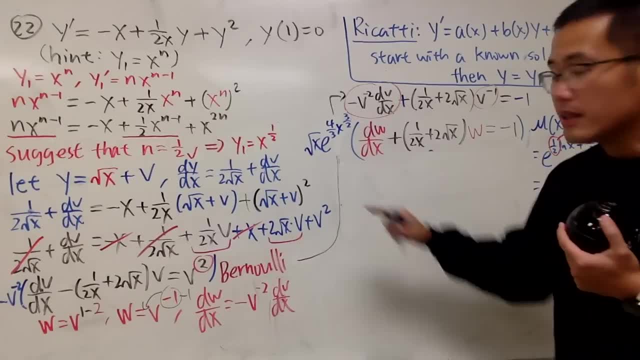 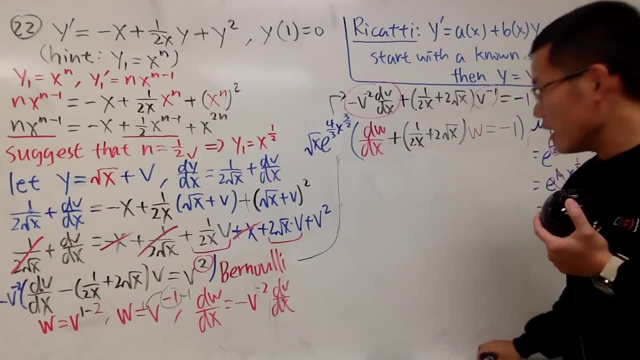 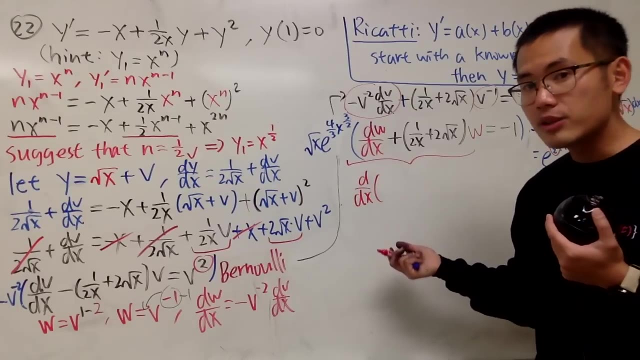 Right. So this, right here, is the idea Now. so we multiply the integrating factor here, And when you do this, times that you know this part is going to be what. This part will be the derivative of a product, Okay, And the product is going to be well, this and v. 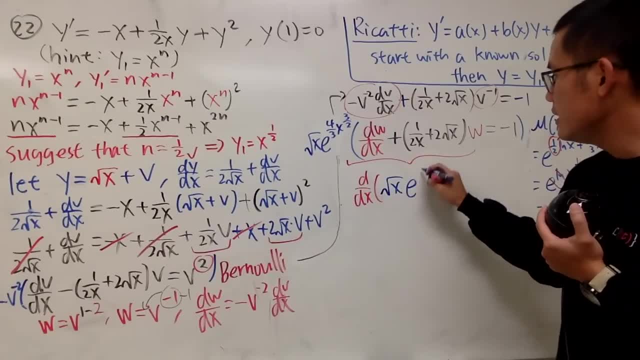 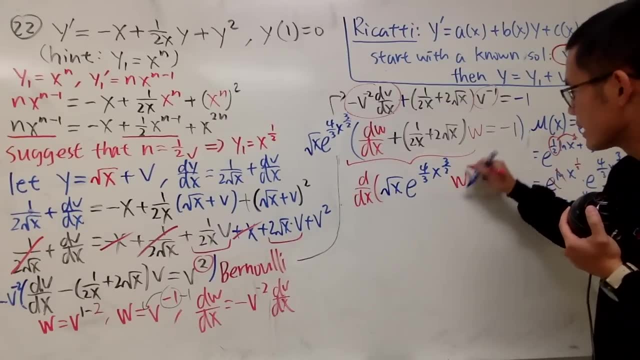 So I'll just write this down here for you guys: Square root of x: e to the 4 over 3,, x to the 3 over 2.. And then, sorry, and w- I mean w The second function is w right. 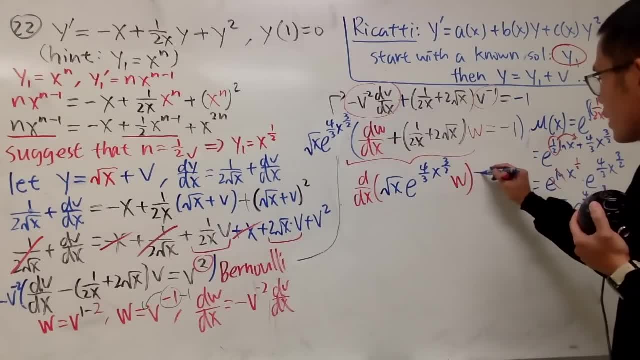 So that's good, And then don't forget to do this times that, though, And that's the part we actually have to integrate. So when we do that, this is equal to we have negative times that, So it's negative and square root of x. 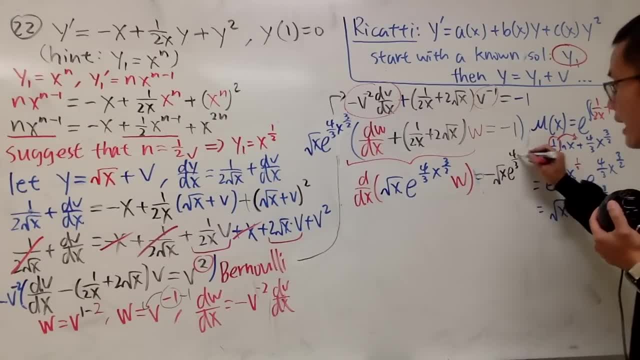 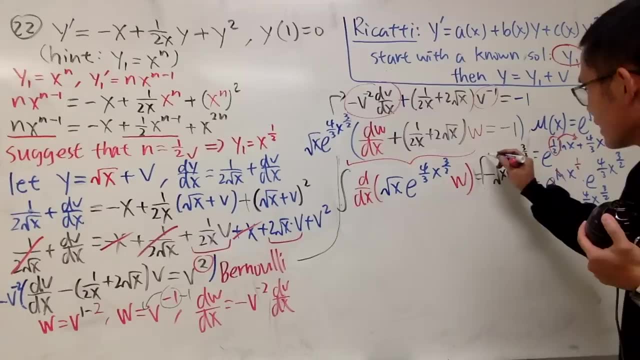 E, 4 over 3, x to the 3 over 2.. Like that. And now, of course, we have to integrate both sides. Integrate both sides Like this In the x world, So that this and that will cancel and integrate this right here. 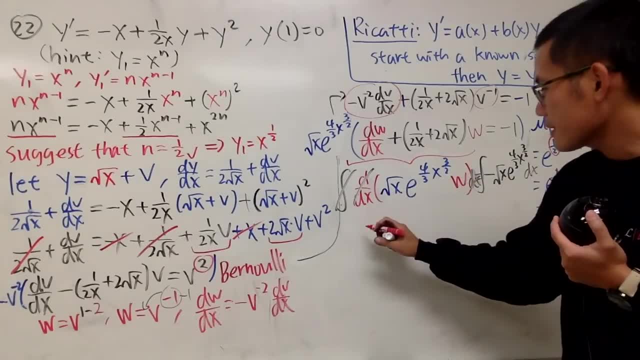 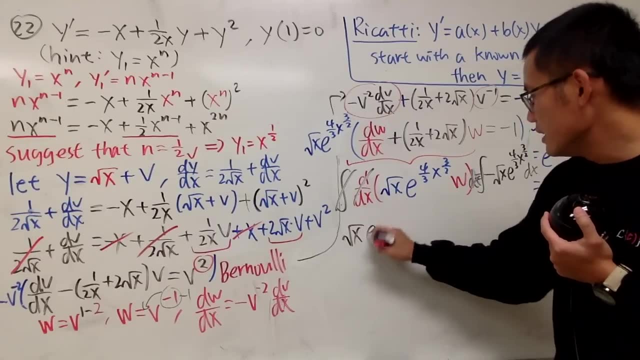 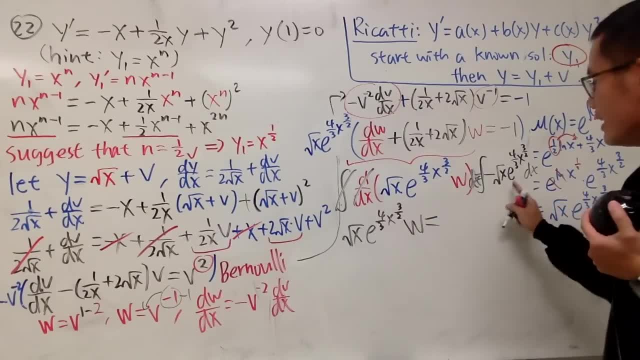 So it's the square root of x, e to the 4 over 3,, x to the 3 over 2.. W and that's equal to integrating this right. We can do u sub. Here is the choice for u. 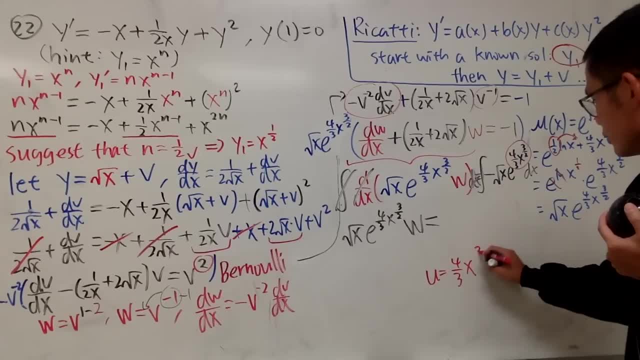 If you let u equal to 4 over 3, x to the 3 over 2. You will see that du will be this in the front, So the 3 will cancel. so you just have 2x and a minus 1.. 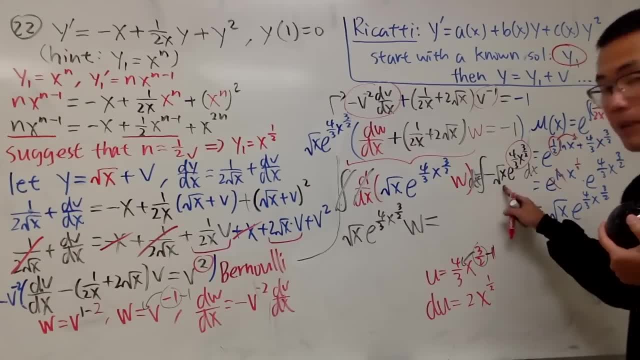 So that's going to be 1 half power, And the 1 half power will cancel, but you have to have the 2. So you just have to divide it by 2.. So again, you just have to divide it by 2.. 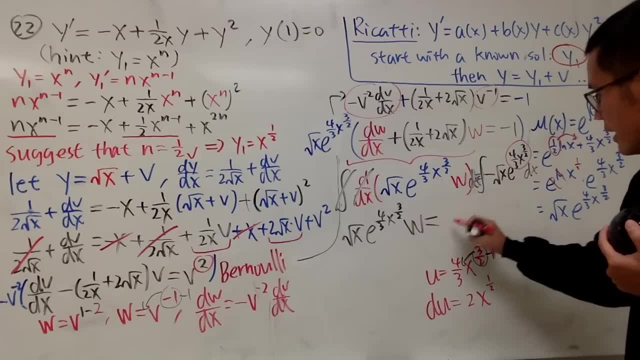 And then you have to have a negative right here. So put down the negative and then again divide it by 2. And then it's just going to be this part which is e to the u, which is that which is this: 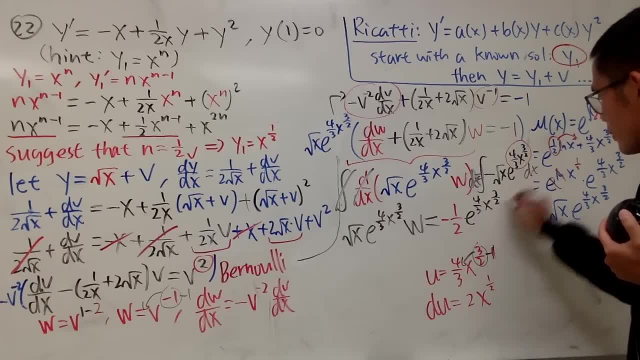 4 over 3, x to the 3 over 2, like this, But don't forget the what Plus z, right? So don't forget the plus z And you can do this in your head. so you know, I didn't erase any work. can you call me? 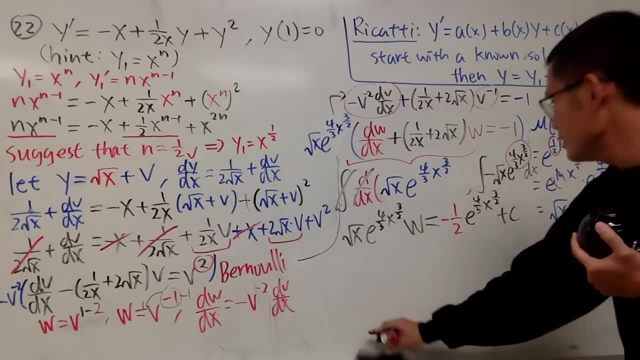 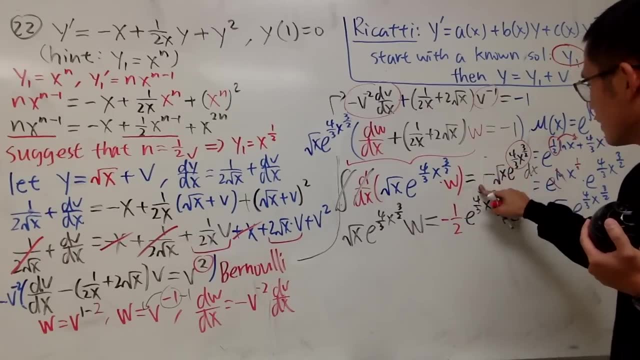 All right, so let me just write it down better for you guys a little bit. This is w times w, and then this is this, and that's the equal sign. Okay, so that's what we have Now. I will divide everybody by this. 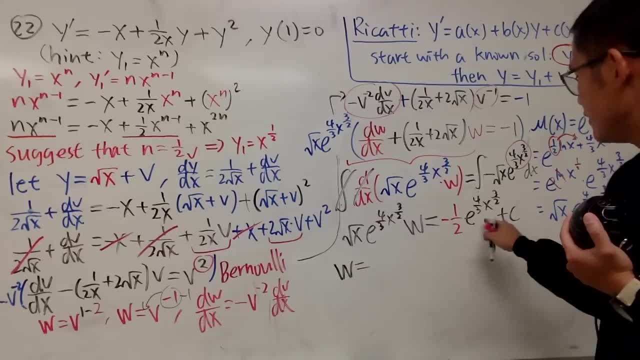 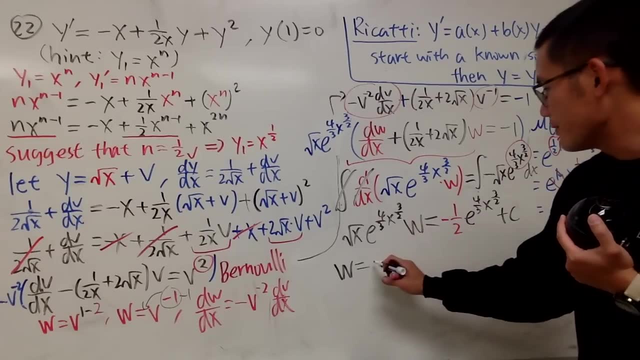 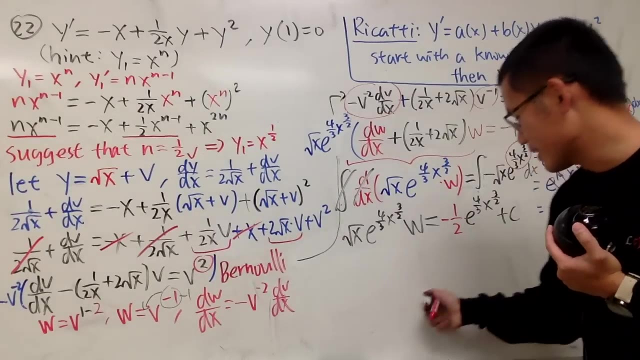 So I see that w is equal to this divided. well, they were just this power cancel, so we just have negative 1 over 2. And then you will have the square root of x, And I don't know if I should show you guys the work. 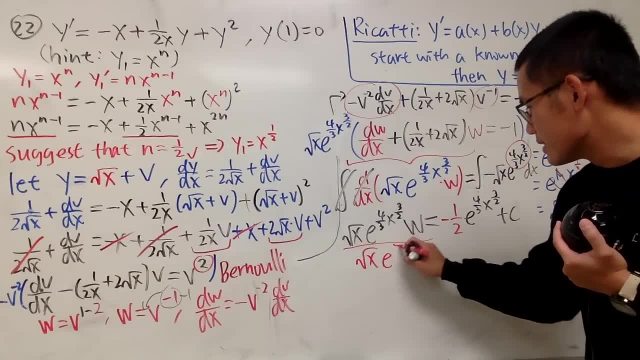 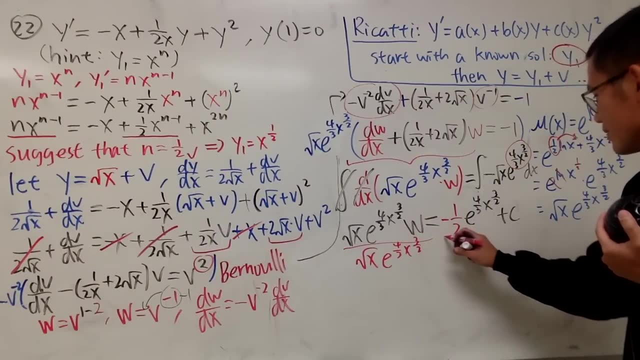 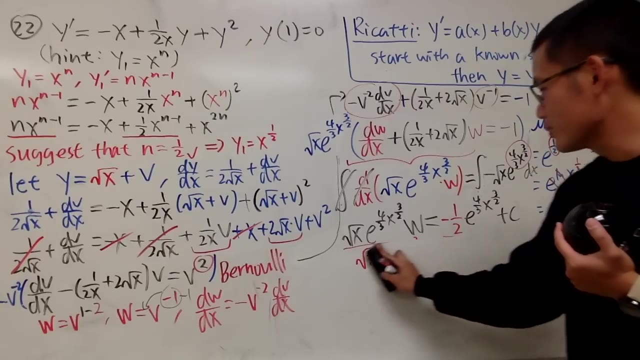 Okay, I cannot fit in everything here. Divide everybody by this 4 over 3,, x to the 3 over 2, and divide, Just divide everything. Oh well, there's so many things to write. No, I will just. no, just just, let's just do this in your head. 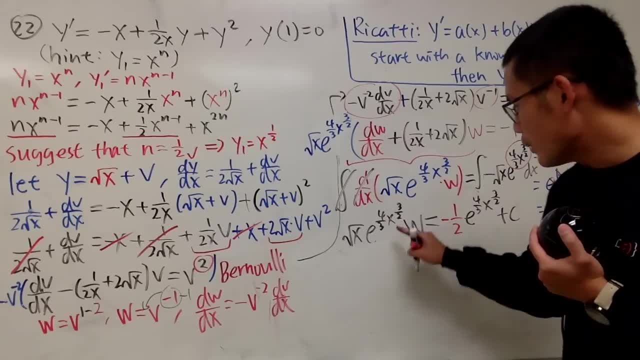 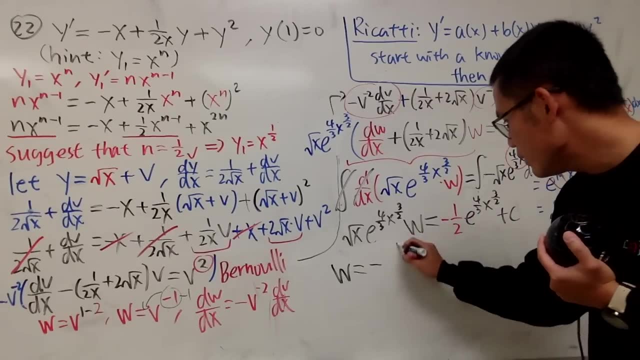 Yeah, let's just do this in your head, All right, so divide this right here. I will isolate the w And that's equal to This will be out, but we have the square root of x on the bottom, So we have negative 1 over 2. square root of x. 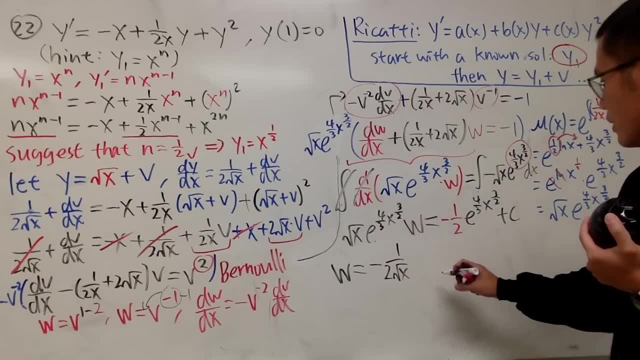 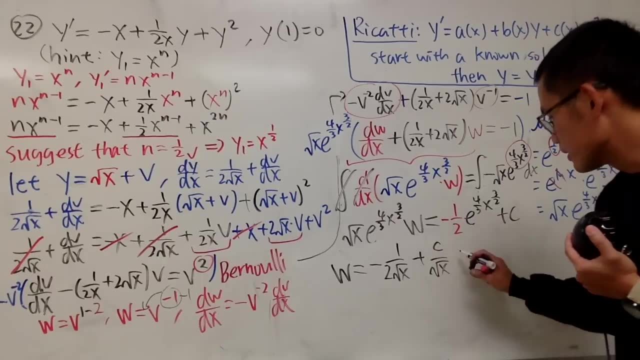 Yeah, and then c over this guy. So I will write down plus c over square root of x And for this I will write it as negative exponent. So we have e negative, 4 over 3, x to the 3 over 2,, like this: 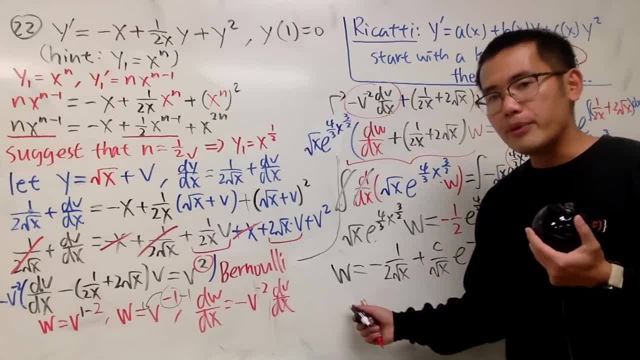 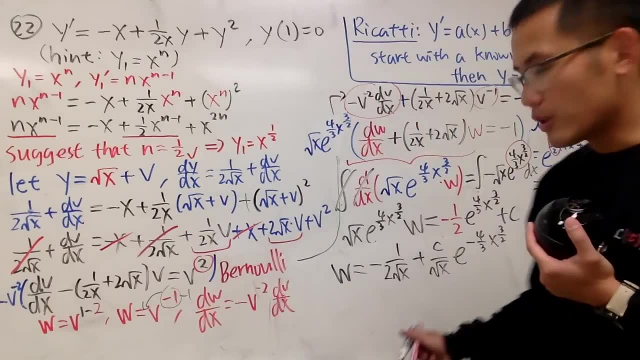 And you think we're done? No, because this is just w And we have to go back to the v. W is equal to v, to the negative 1.. So you see this right. here is actually 1 over v, right? 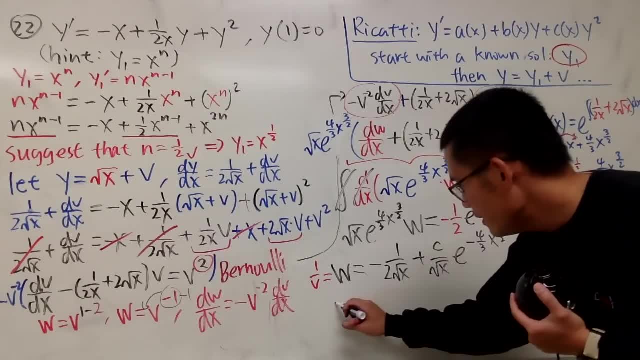 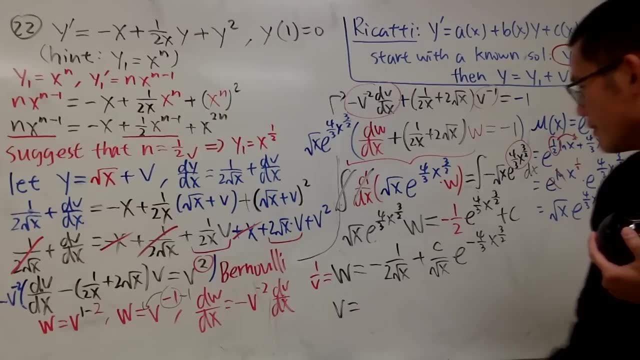 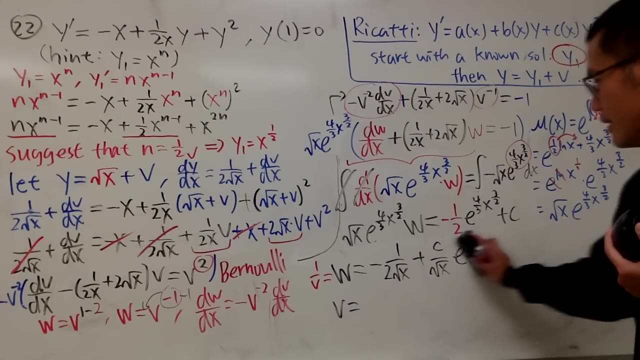 So what you have to do is well, the v will be: perhaps let's do this. I'm sorry, I'm so sorry. Perhaps let's do this, I can sorry. So this right here is what we have. 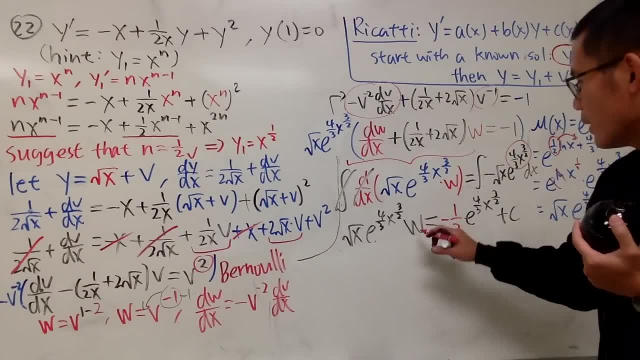 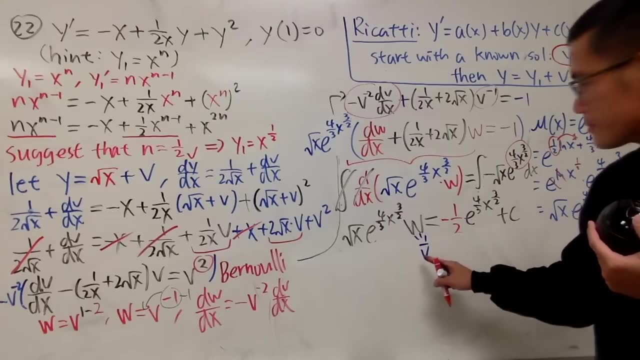 But for the w, we know it's v to the negative 1.. So I will just look at this. And we know this right here is the same as 1 over v. yeah, So what we can do is I can multiply both sides by v and divide this on both sides. 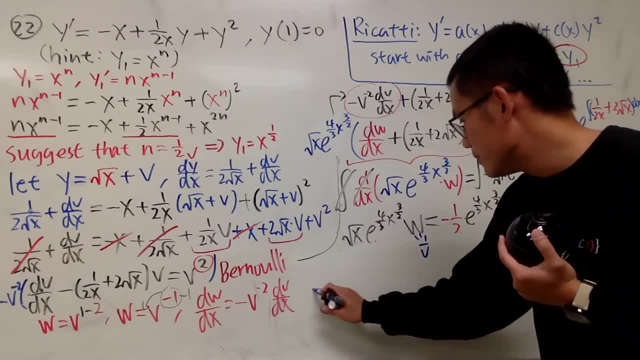 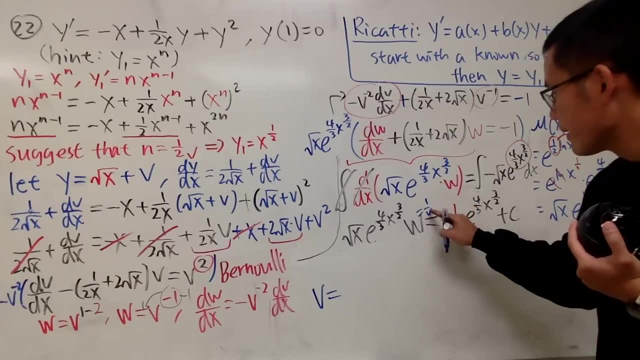 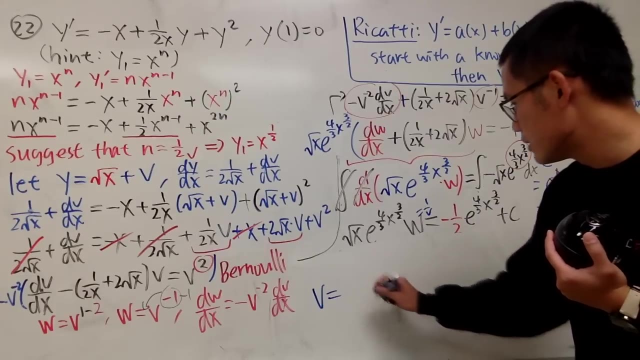 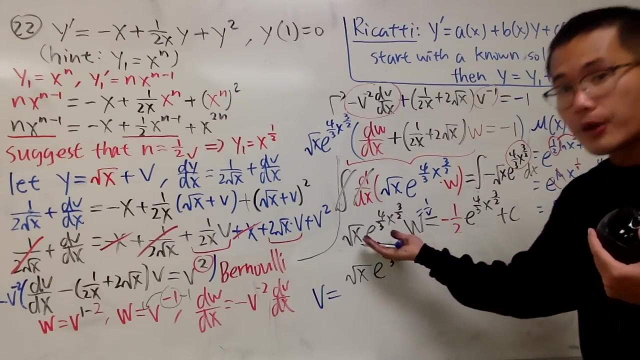 So we know v will be again. the w is the same as 1 over v. yeah, So I will just multiply the v on both sides and divide this on both sides. So on the top of this guy, which is the square root of x, and then e, 4 over 3, x to the 3 over 2, okay. 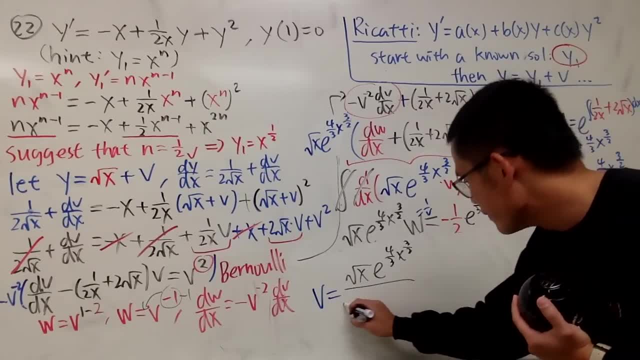 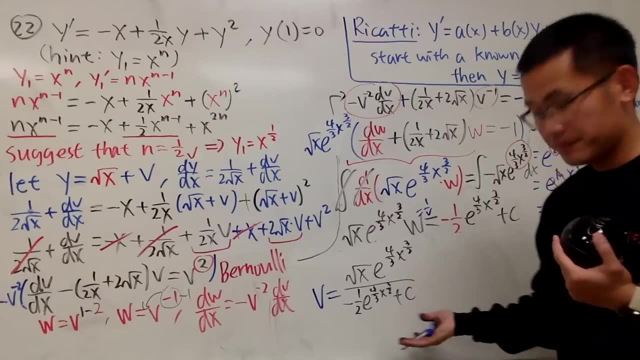 And then I will divide this right here, which is over, and we have negative 1 over 2, e, 4 over 3, x to the 3 over 2 plus c. But what's v? though? v is equal to the things that you had to plug into that. 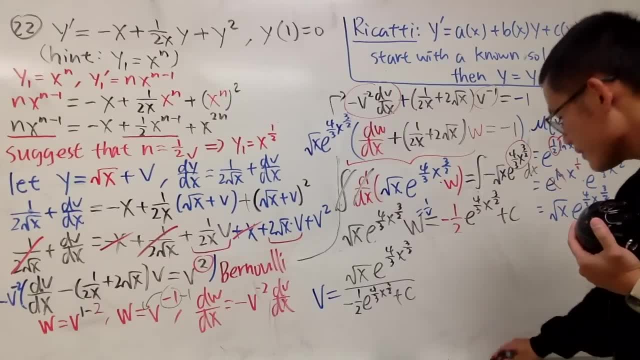 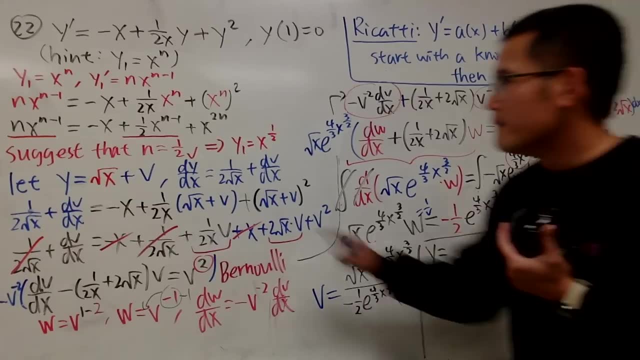 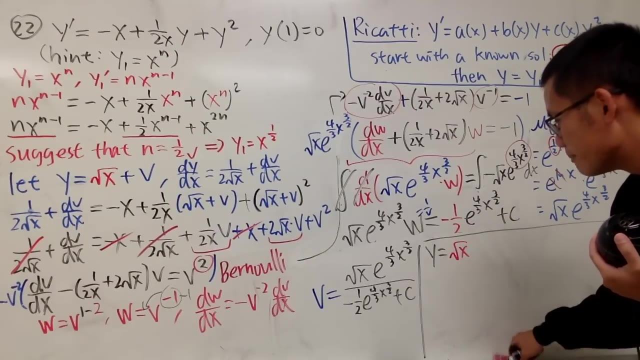 So we got a v right. So here's the deal, The solution. the solution is: y equals square root of x plus v. So we still have to have the square root of x right here, And then plus v, which is this guy. 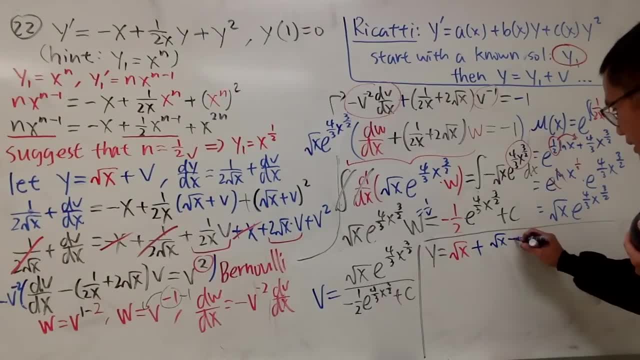 This is square root of x plus e, 4 over 3, x to the 3 over 2 over negative 1 half And uh, all the stuff. yeah, So plus v, just like this, right, Plus v. 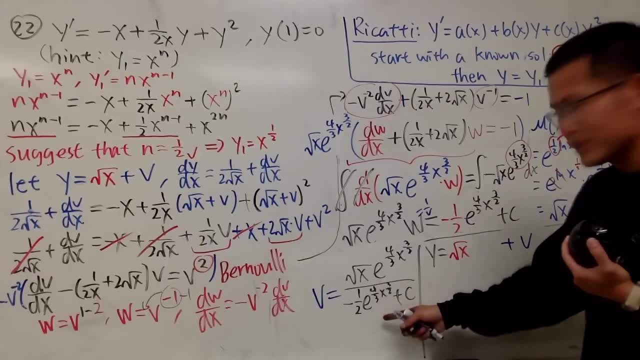 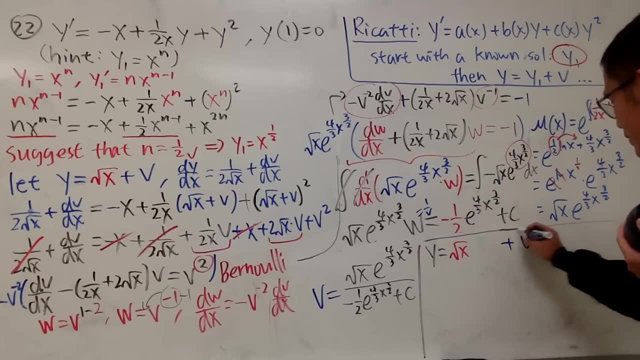 And uh, the truth is we have to get the common denominator and all the stuff. So let's just go ahead and get the common denominator And god. seriously, why did I put this question right here? to quote for myself: 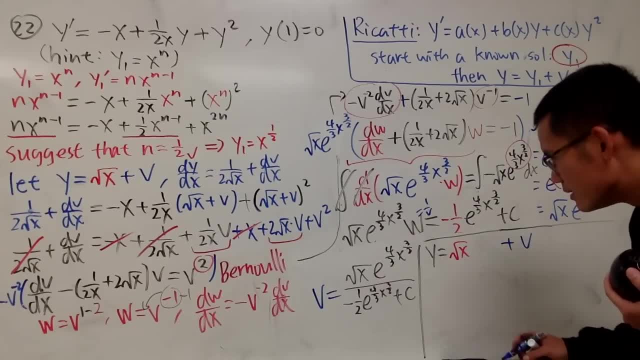 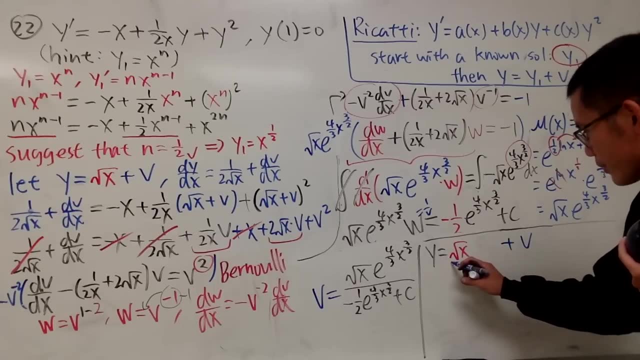 V and uh, let's see. Hmm, Okay, So I'm going to multiply the top and bottom by this, of course. So it's negative 1 over 2, uh, e to the 4 over 3, x to the 3 over 2, um plus c. 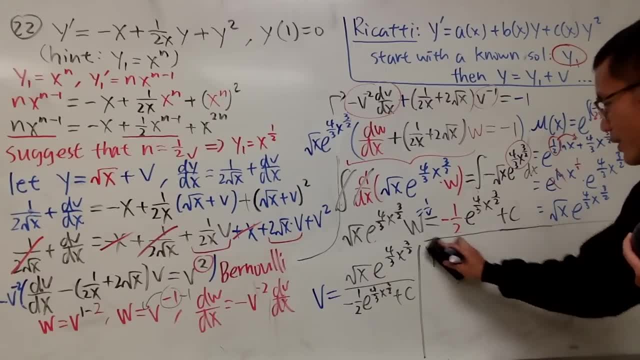 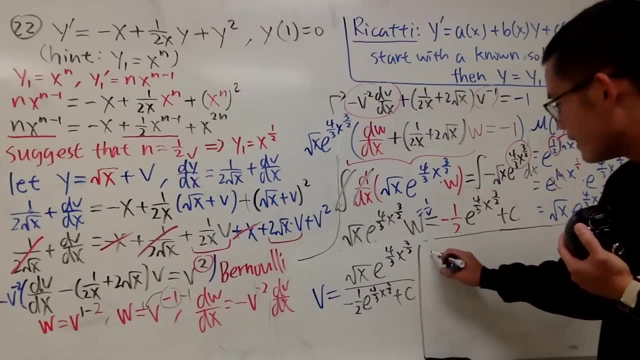 And you have, how can I? I'm going to see how can I. I know how to do it, but like I just have to make sure I can fit everything here, That would be so, so good. Okay, now let's just do things in our head. 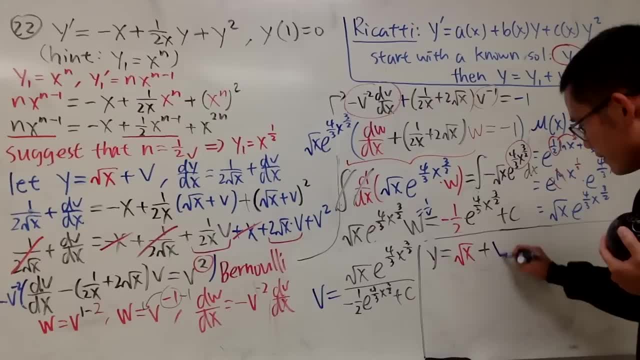 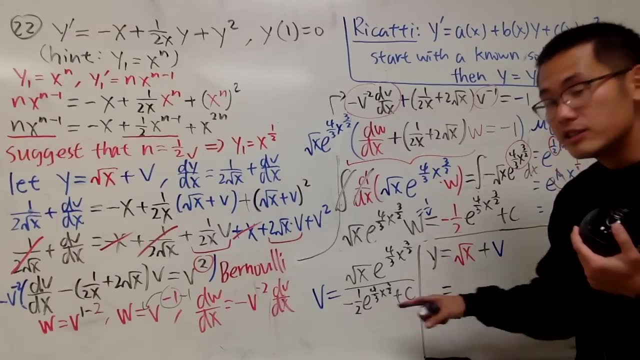 Okay, So let's do things in our head. Plus V, So now V is this, And this right here doesn't have that. So get the common denominator And we know it will be this for the bottom. 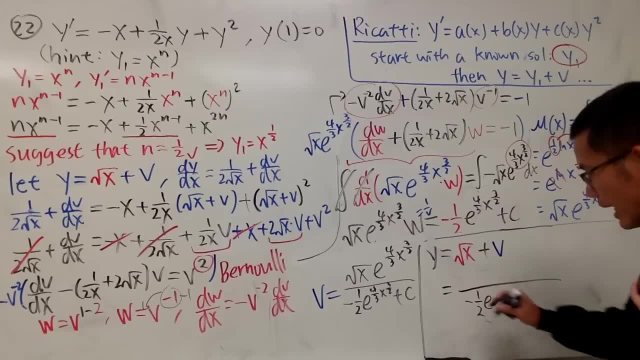 We have negative 1 half And we have e And we have, uh all that, 4 over 3, x to the 3 over 2, plus c, Like this. yeah, And then on the top here I have square root of x. 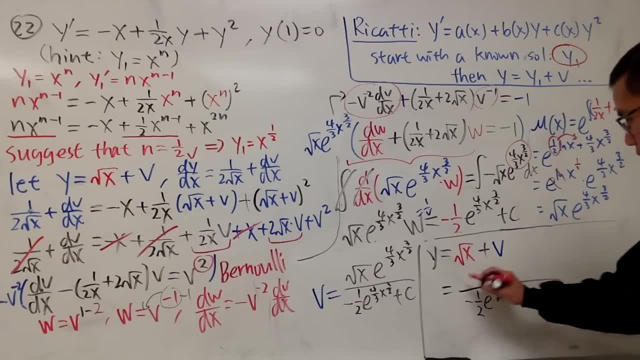 Times. So I will just have the square root of x right here, Times the bottom. So I just say it's like a bottom thing, And then plus the v, which is that part, So half that part which is the square root of x, e, 4 over 3, x to the 3 over 2.. 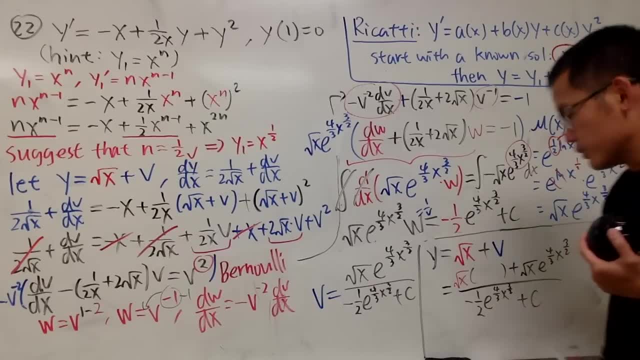 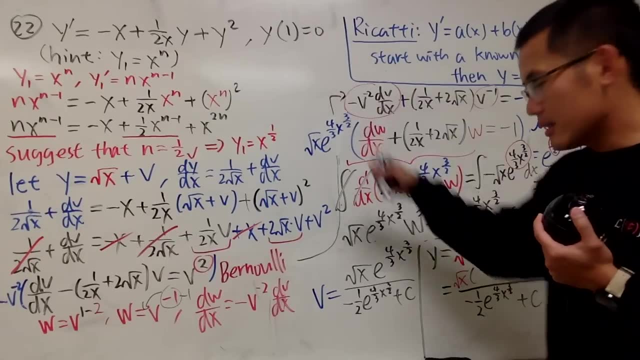 Like this, And now you see both of them have the square root. You can factor that out And I am going to just go ahead and do the um. what's that called Initial condition right now? So we want to end out with 0.. 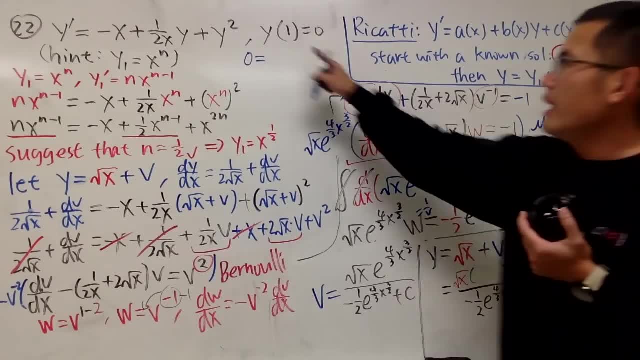 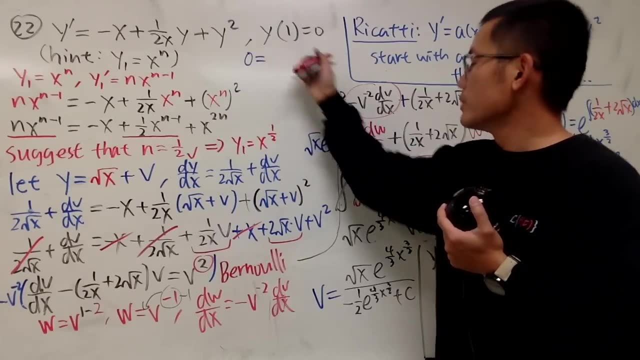 Okay, y is equal to 0.. And when x is equal to 1.. Actually, let's figure this out right: here We have square root of 1.. That's 1.. So this is square root of 1.. 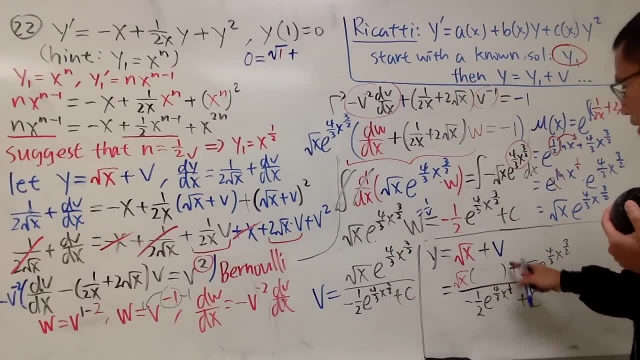 Oh man, this is not an easy question at all. And then v is all that. So I put down 1 into all the x, So we get square root of 1.. Again, just do this in your head. 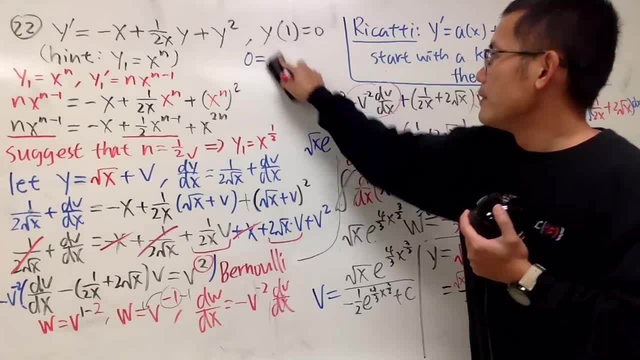 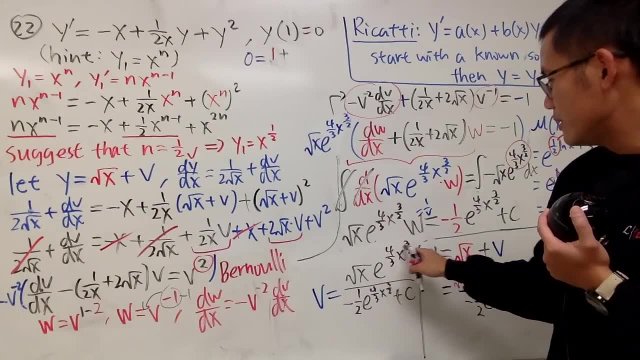 Uh, let us see 1 in red Plus uh 1 in here is just 1.. And e to this is 1.. So it's just e to the uh 4 over 3 power. 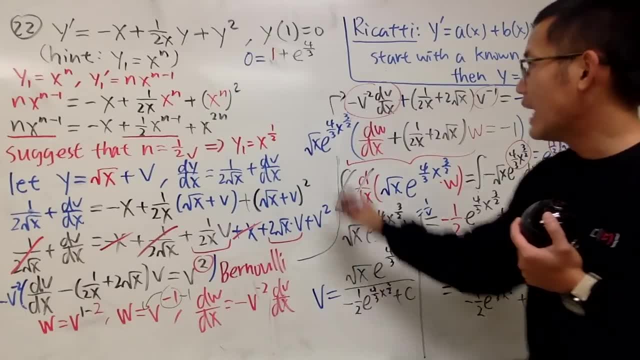 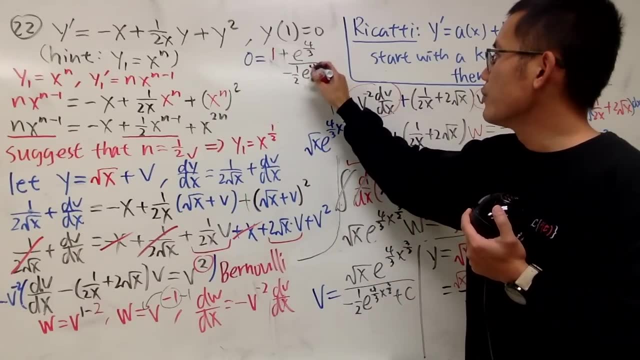 Yeah, Good huh, And then put the 1 right here, And then we have this: over negative 1 half, And then this is just e to the negative, e to the 4 over 3 power Plus c. 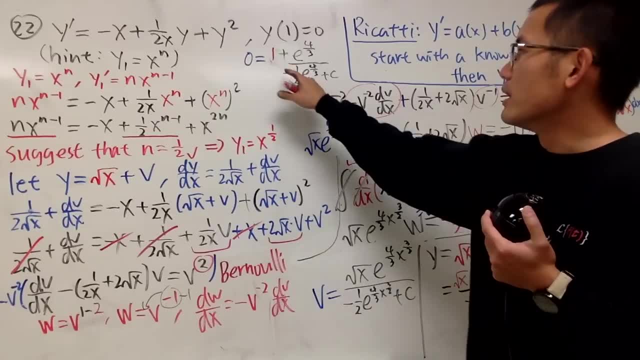 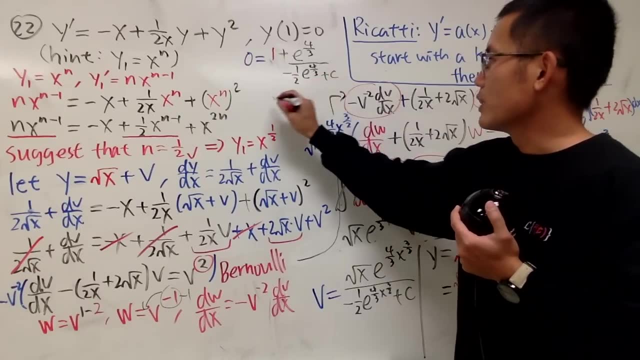 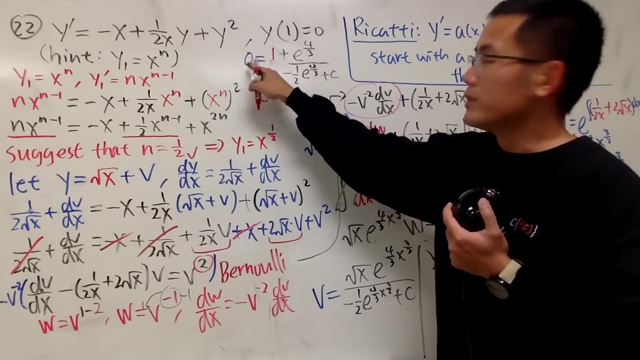 Yeah, Just like all this. Now, in order for this to be negative 1,, here's the deal I: I need to move this to the other side. That's why I said c has to be the following: Put this to the other side. 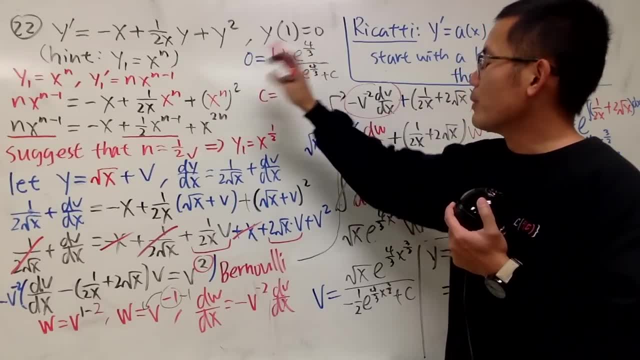 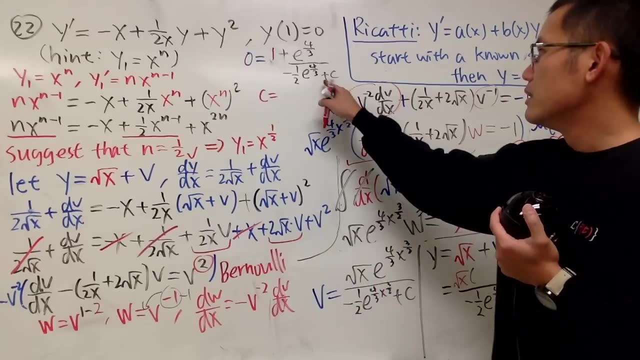 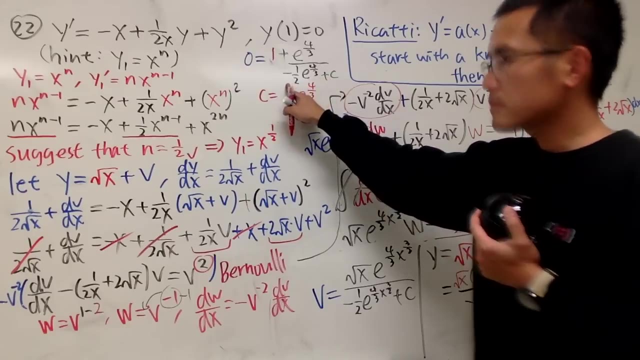 It becomes negative 1.. And then you can multiply that on both sides, Okay, okay, okay, C has to do with e to the negative, e to the 4 over 3. And then, hmm, I need to end out with negative 1.. 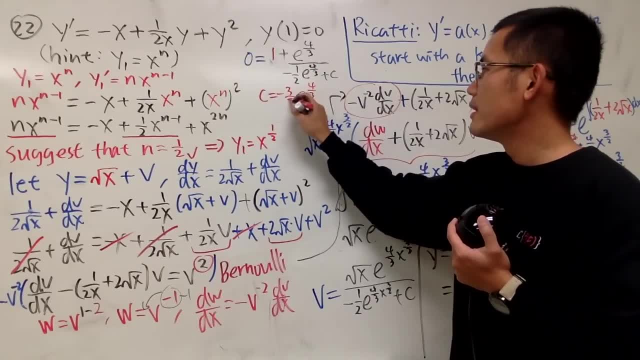 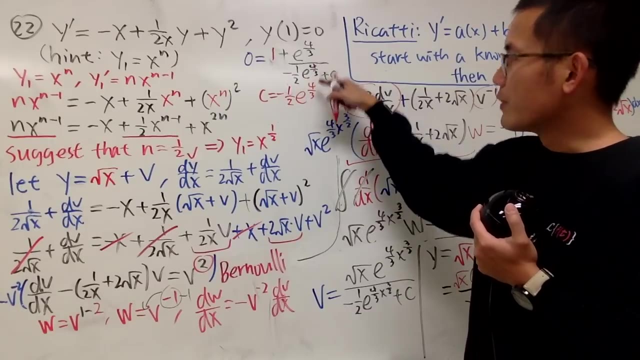 Come on, Negative 3 half, Because No negative 1 half. There we go. C has to be negative 1 half Because if you put negative 1 half here, that will be negative uh, 2 over 2.. 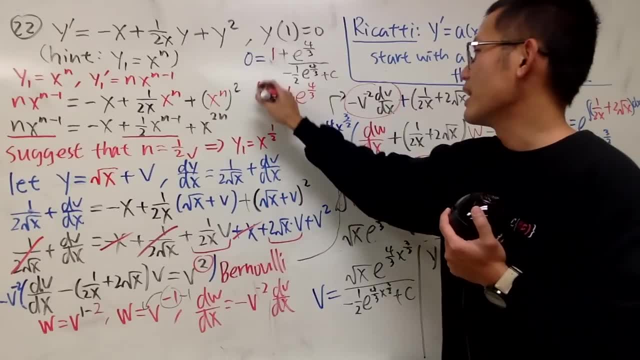 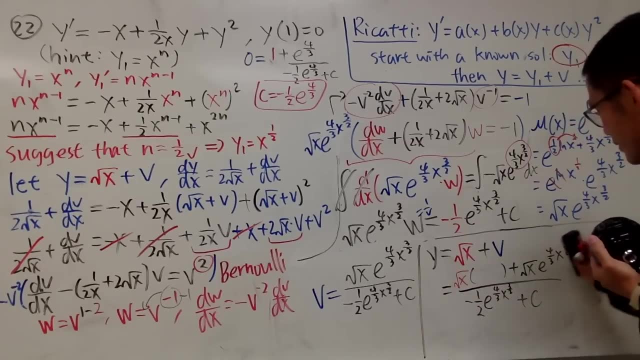 That And that will cancel. So it's negative: 1. So c is equal to this guy, Right? So that's that. So we have the c right here And I'm just going to do the following for you guys: yeah. 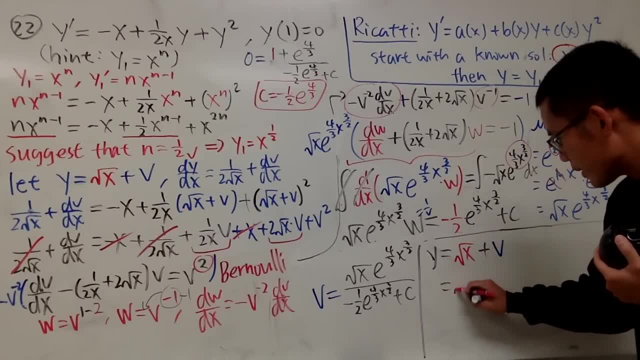 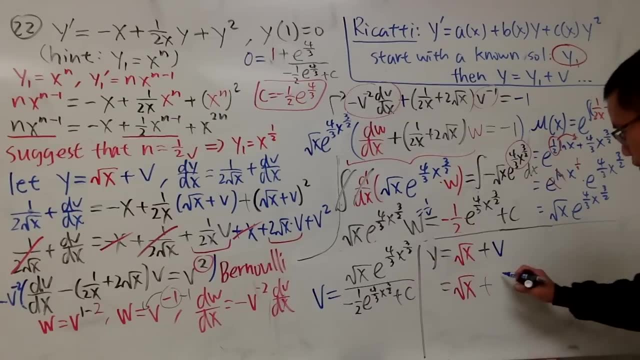 Finally, you will see that square root of x is right here, And then you add v. I don't know how many times I said v already. It's equal to this, which is square root of x, e 4 over 3, x to the 3 over 2, over. 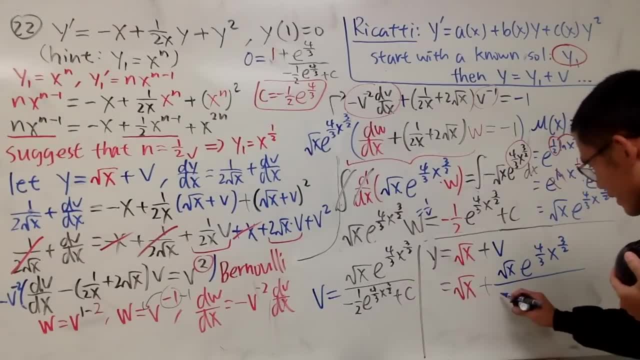 And, uh, you have this. Well, you have this, This first. Negative 1 over 3.. Negative 1 over 2.. Sorry, Negative 1 over 2, e to the 4 over 3, x to the 3 over 2.. 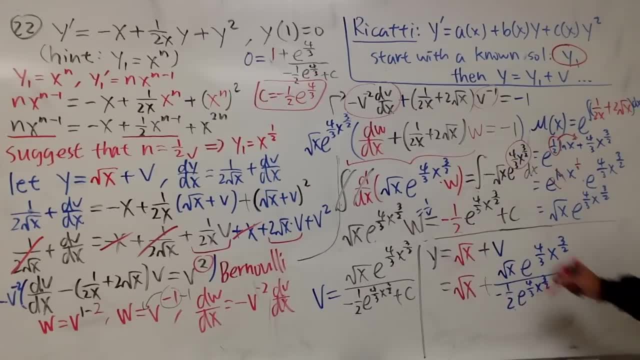 And then plus the c, which is the one that we said over there, Minus 1 over 2, e to the 4 over 3, x to the 3 over 2.. Yes And seriously, let's not do the common denominator anymore. 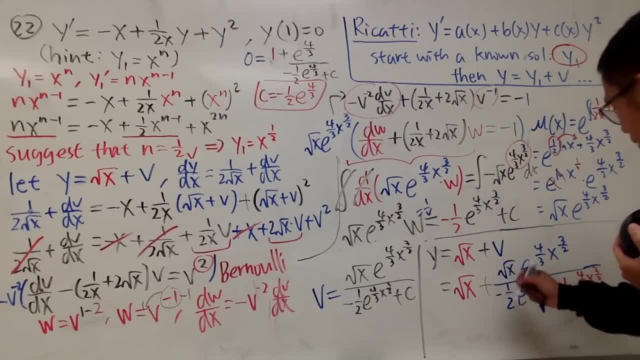 This right here will be the answer for it, Right? So I'll just write it down And you can multiply the top and bottom by 2, but uh, Please don't do that seriously. Let me see if this is the answer. 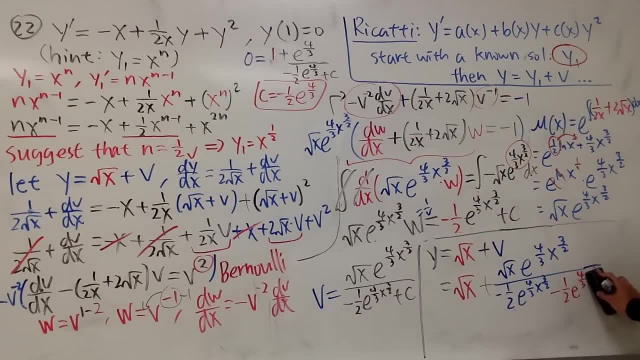 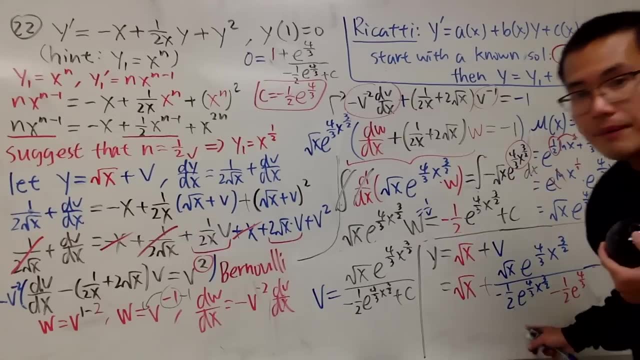 No, c is, c is just 4 over 3.. Okay, almost, almost, almost, It's just that, am I right? Good, Good, good, good, Okay. Uh, you can factor out a negative And you can bring the 2.. 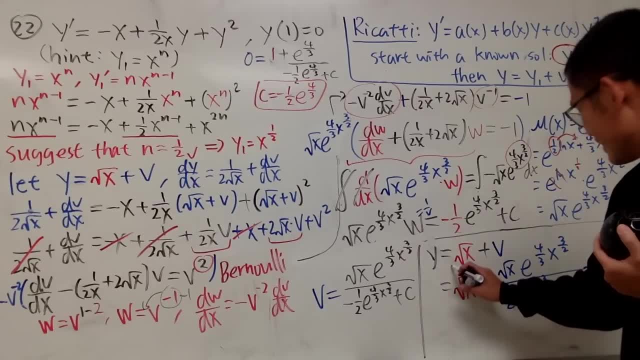 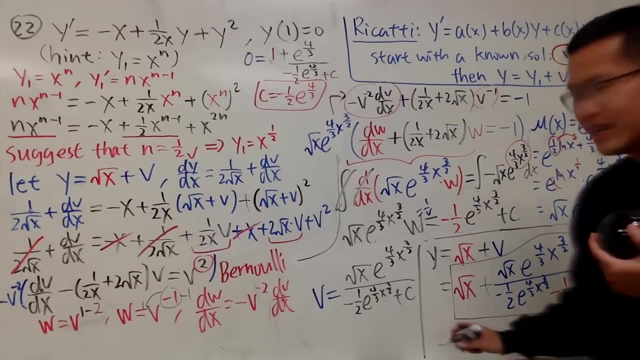 But I think I'll just leave that to you guys. Okay, Not perfect though, but I cannot run out of space. So this, right here, it's the answer, And, if you want, I will tell you, though the answer is on the answer key. 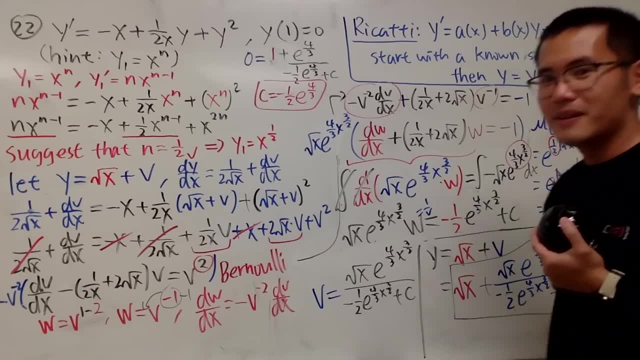 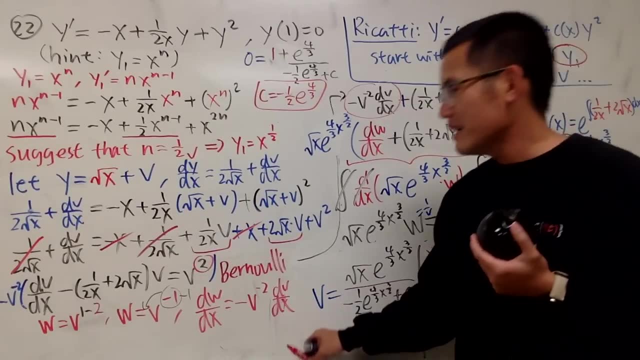 And maybe I'll just work this out another time. I'll see if I can fit in everything here- And pretty satisfying. I don't know how long it took me- Like half an hour already or so. So anyway, quick recap. 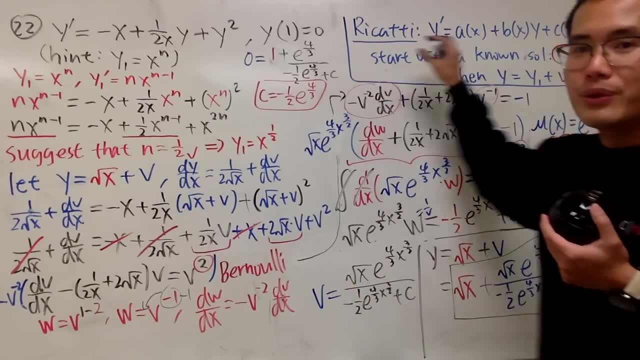 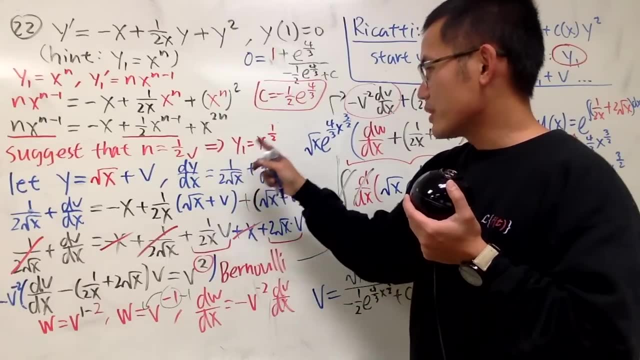 This is Riccati's differential equation, And you do the y1, and then you just continue right, And you will turn out to be Bernoulli's differential equation right here, And then it's going to be linear, And then just good luck with the integration. 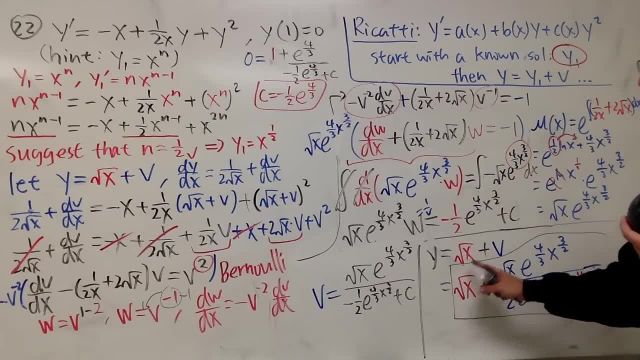 And then just put it back: Square root of x, which is y1 plus the phi, And then that's it. That's all you have. Yeah, And just to show you guys the answer, you guys can see You can actually write the answer in this form. 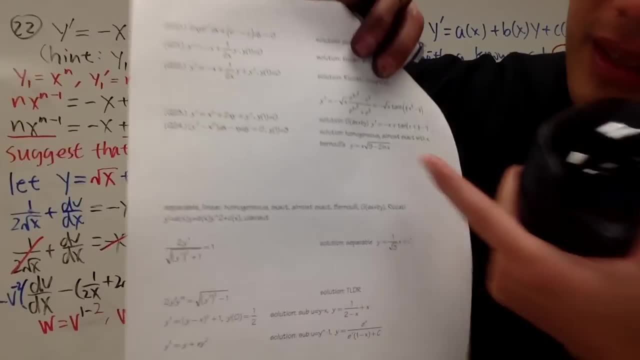 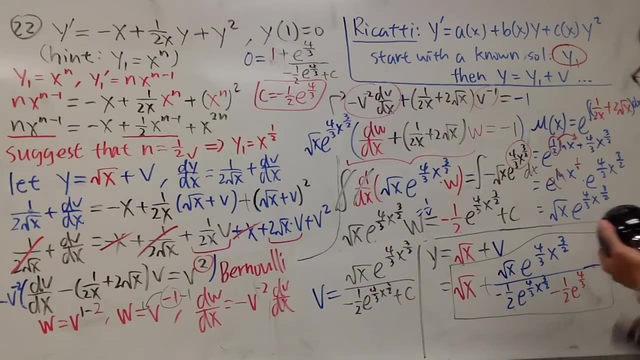 By random space, Either this or that By random space. So again, maybe another time. All right, So I'll leave that to you guys. Just get a common denominator. The rest is just algebra anyway. So yeah, 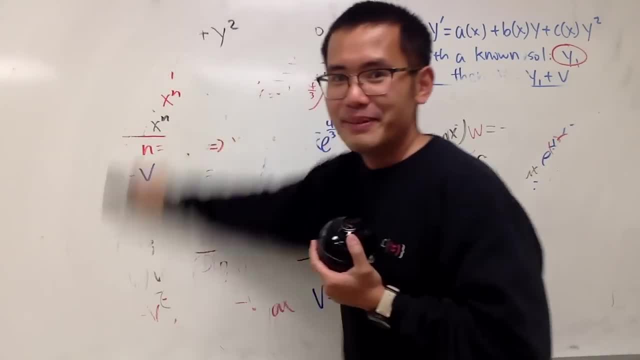 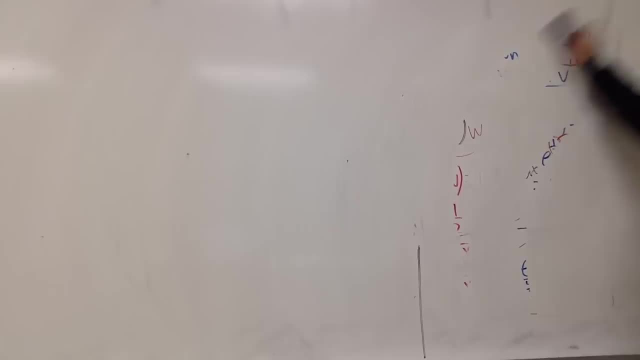 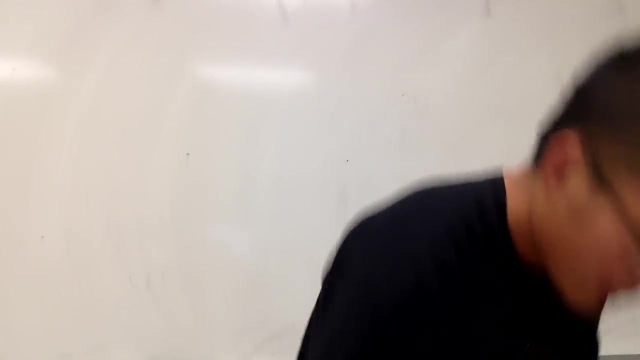 Man, very good stuff, Seriously, It's like one question takes 30 minutes. Also, I can actually use it quite often, So pretty good, All right, So I definitely use it. It's very useful if you are watching my video. 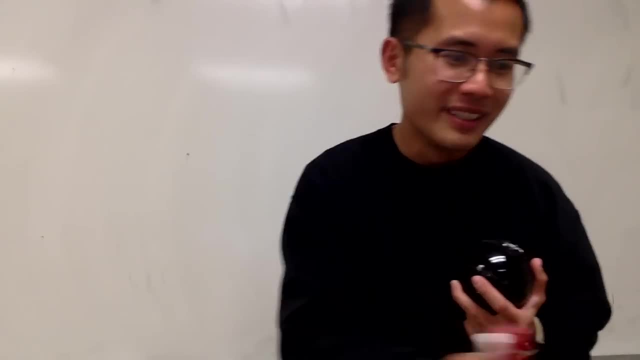 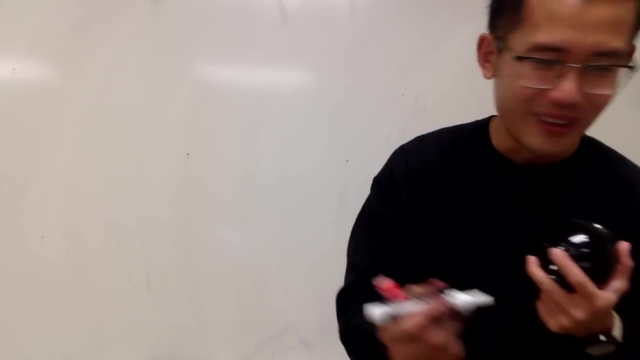 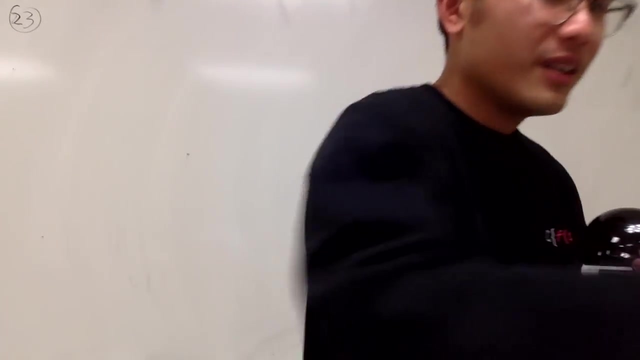 If you guys still takin the course with some of your time and maybe a short break, then I'm bummed out tonight, right, All right, Let me just reward myself with a new marker so we can be happier when we write. 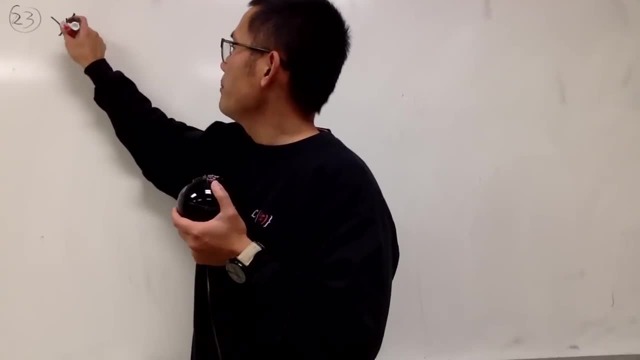 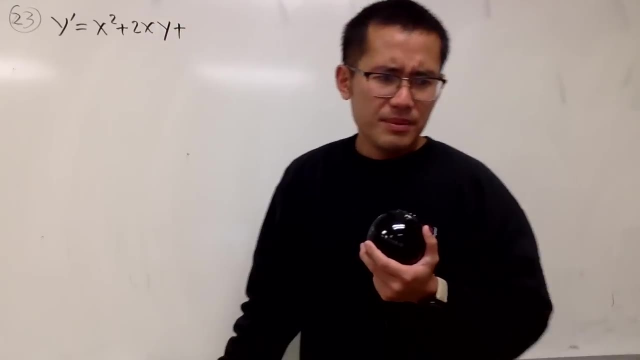 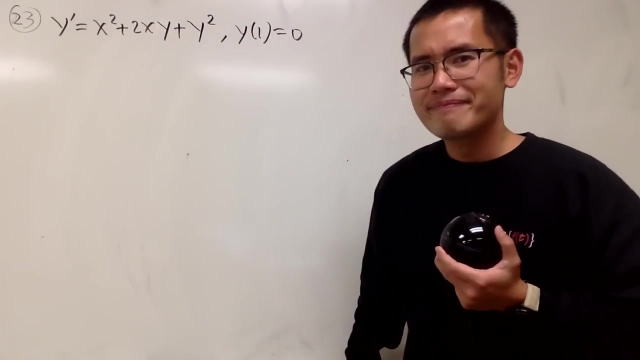 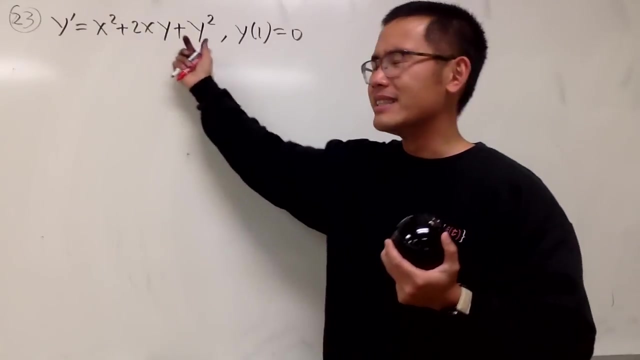 Number 23.. y' equals x squared plus 2xy plus y squared, And then y of 1 equals 0.. No, is this a Ricardian differential equation? again, Yeah, because we have the x squared plus the 2x and then the y squared. 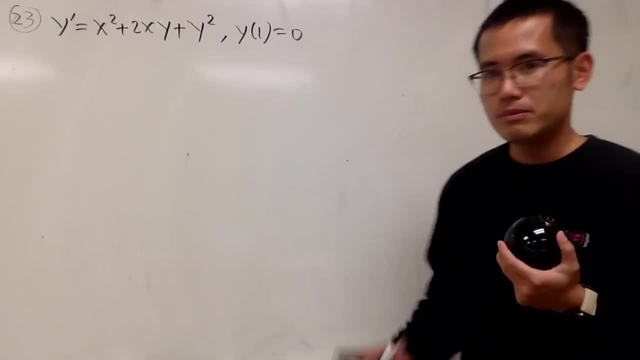 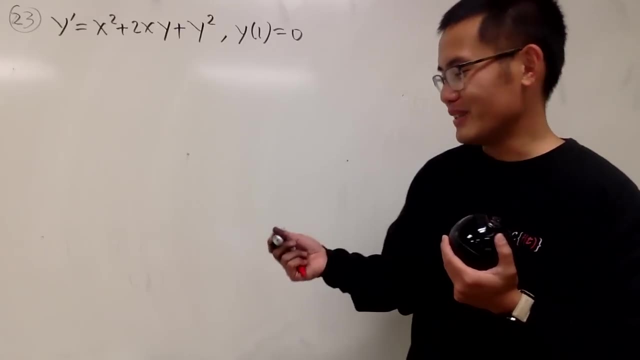 I don't want to do how I did earlier anymore. Don't worry, This is pretty good. You have a couple ways to do it, But perhaps the best way is you do the following: Can we factor this? Yes, we can. 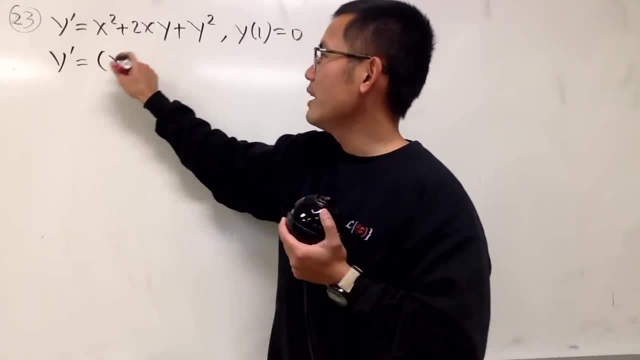 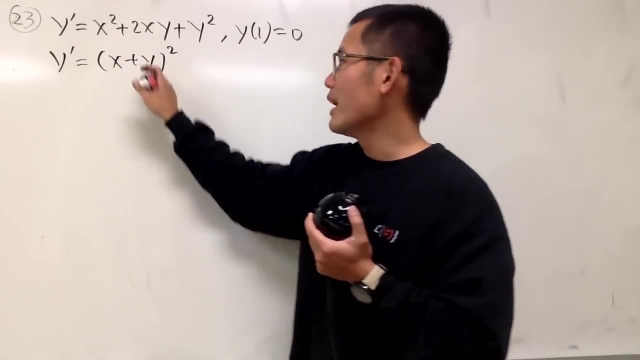 And when we factor it, what do we get? We get a perfect square named the x plus y squared. This right here is in the g of x plus y, form right, So we can just do the substitution that v equals x plus y. 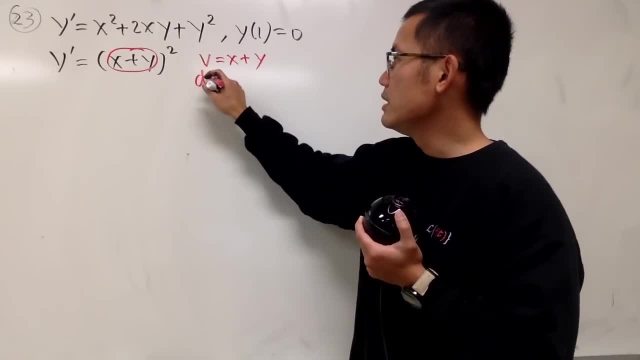 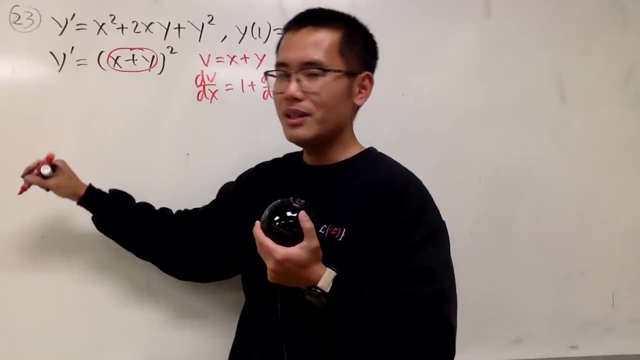 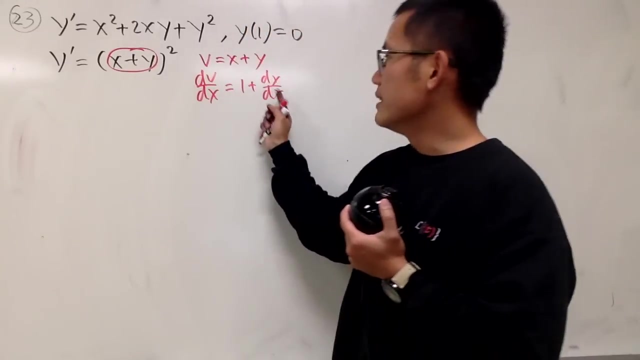 And go ahead. You can do the following: dv dx is equal to 1 plus dy dx, So of course, continue. Very nice. dv dx is this which charges to minus 1.. So it's dv dx minus 1.. 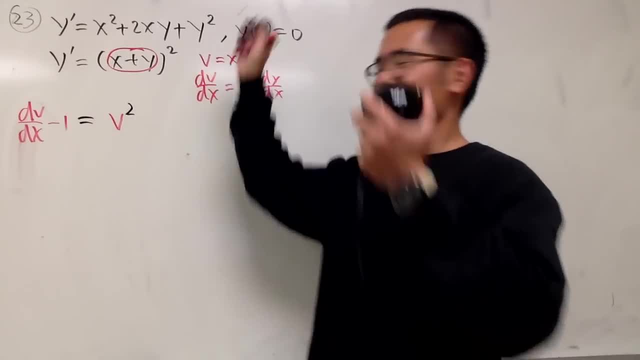 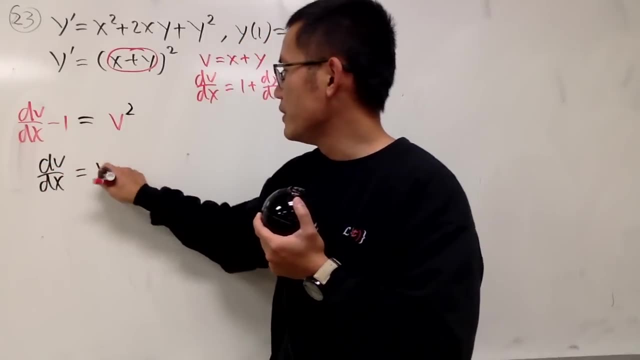 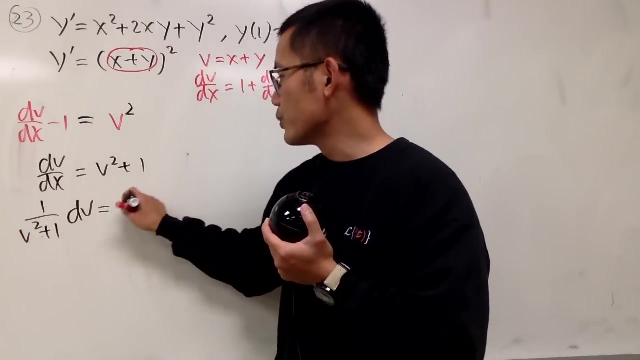 That's equal to v squared. Oh, so easy. now Add 1 on both sides, We get dv. dx is equal to v squared plus 1.. Divide, multiply, So we get 1 over v squared plus 1.. dv is equal to dx. 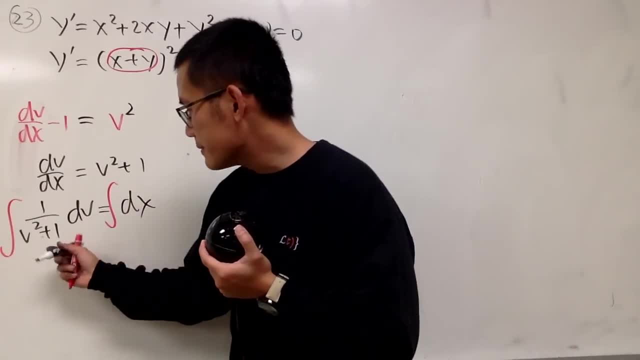 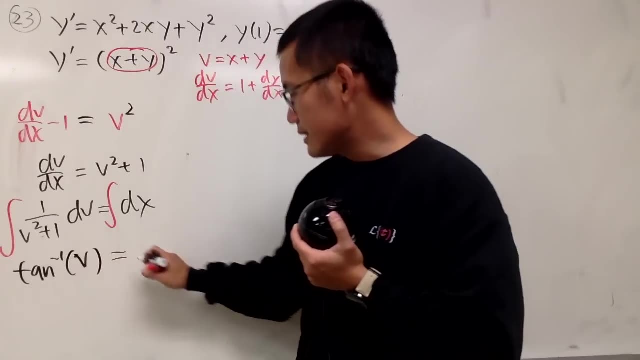 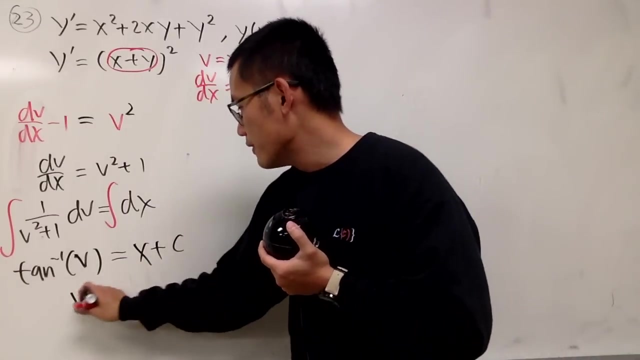 Integrate both sides, So the left-hand side, we get inverse tangent of v. Just like this, It's equal to x plus c1.. Doesn't really matter, We just need to use 1c Do the original tangent. 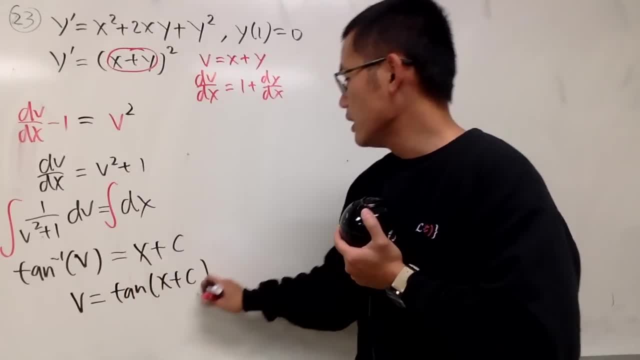 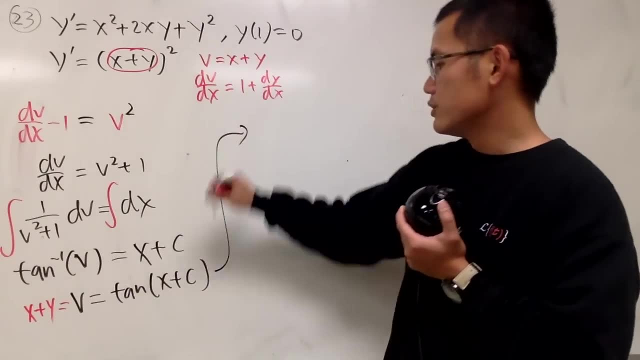 v is equal to the original tangent of x plus c And, of course, what's v, though? v is x plus y, So this right here is the x plus y To get y. well, just minus the x on both sides. 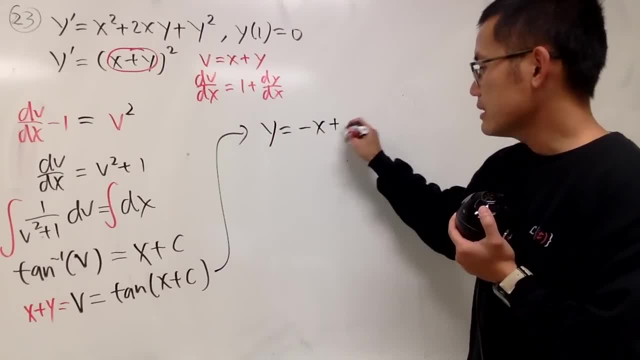 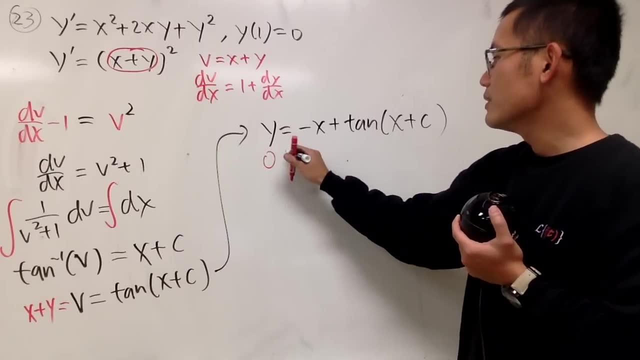 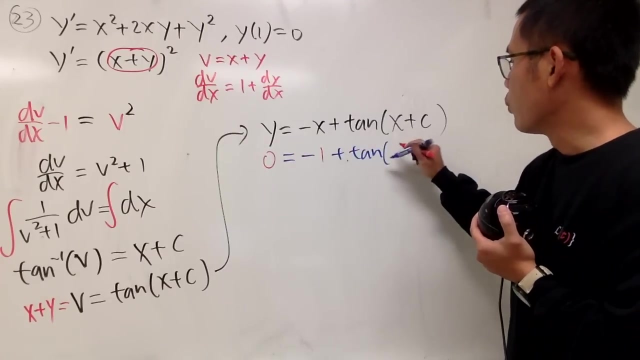 So we get: y is equal to negative, x plus tangent of x plus c. Now, with that, very easy: 0 is equal to 0, is equal to 0, is equal to negative, 1 plus tangent of 1 plus c. 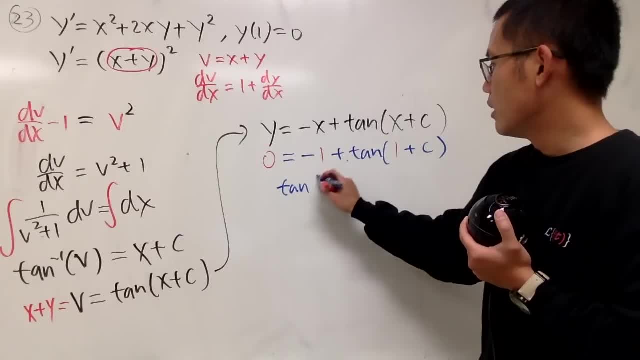 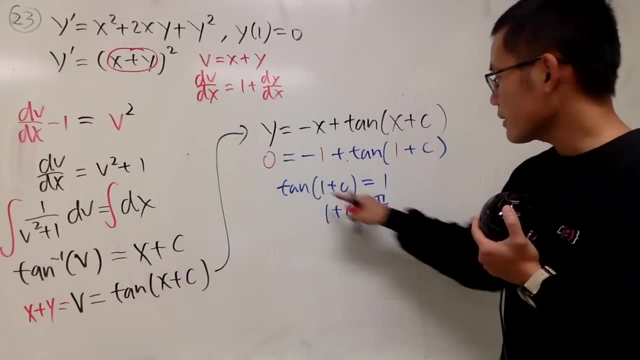 So put this to the other side, We get tangent of 1 plus c is equal to 1.. So that means the input 1 plus c should be pi over 4.. Yeah, the input has to be pi over 4.. And then of course, minus the 1 on both sides. 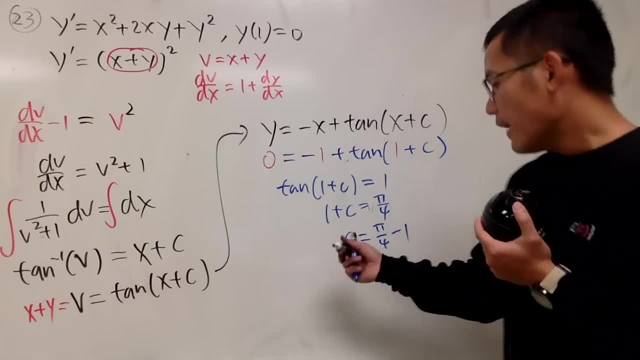 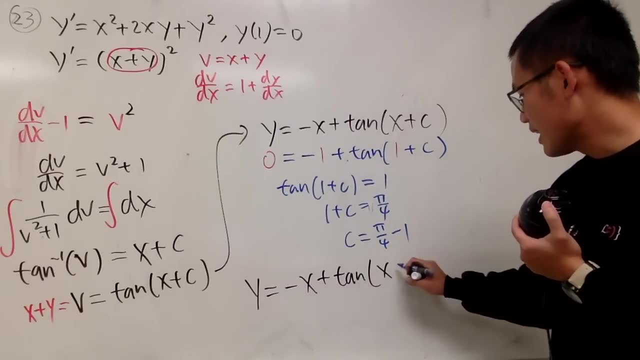 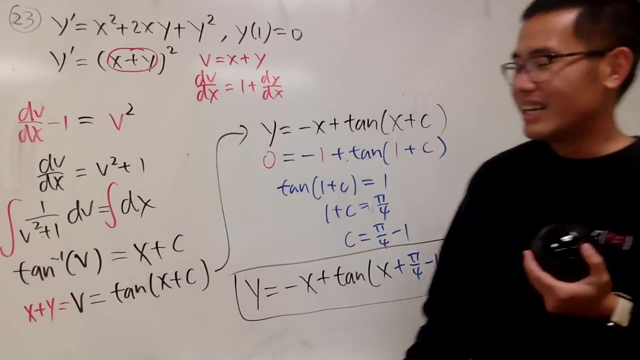 So this is pi over 4 minus 1.. Finally, y equals y equals negative, x plus tangent, x plus pi over 4 minus 1.. Like this, Very good stuff, Yeah, Whew. Okay, last one, Last one. 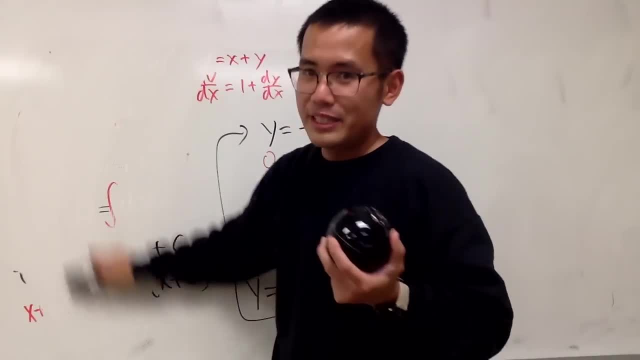 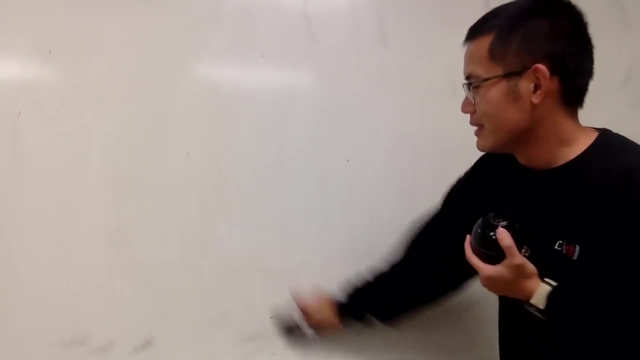 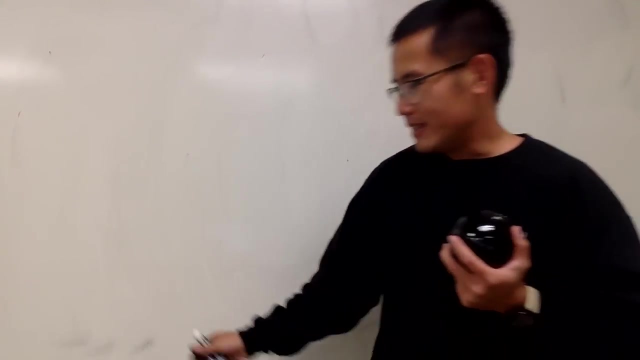 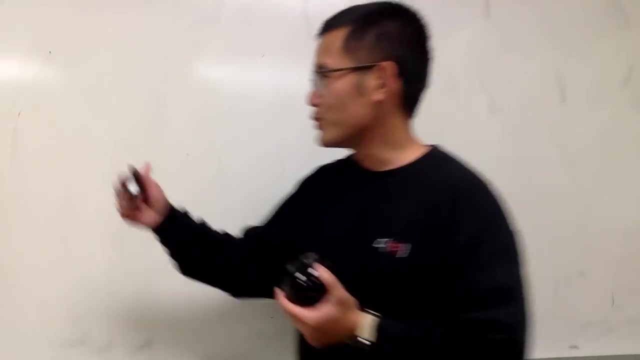 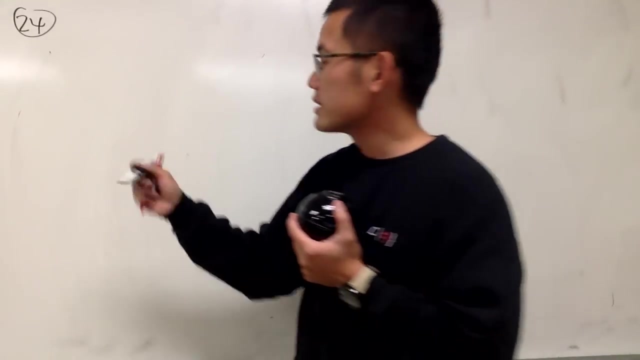 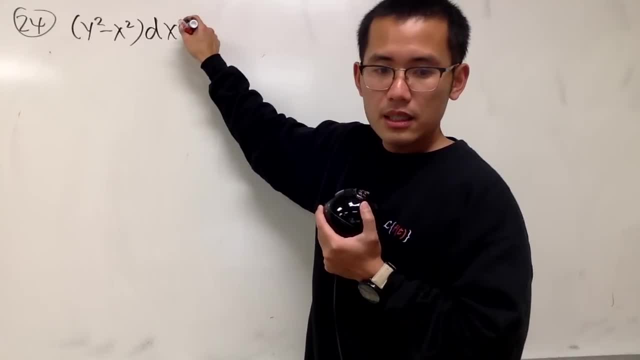 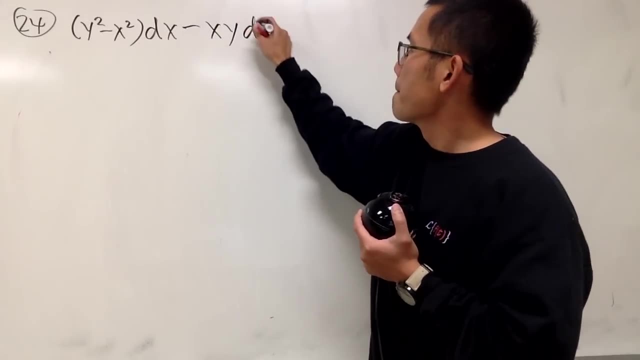 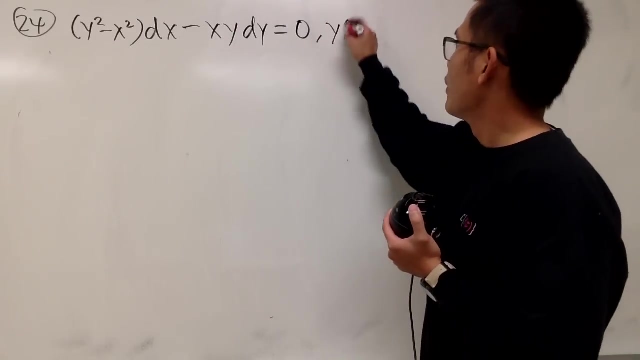 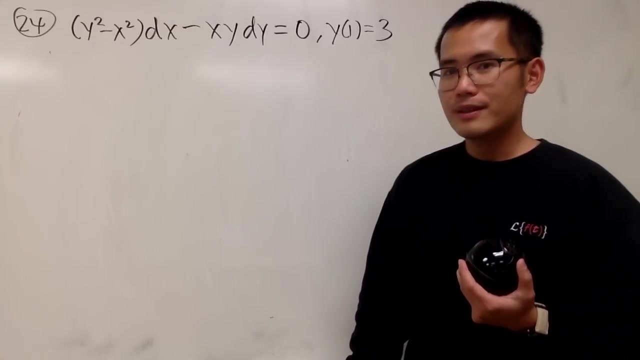 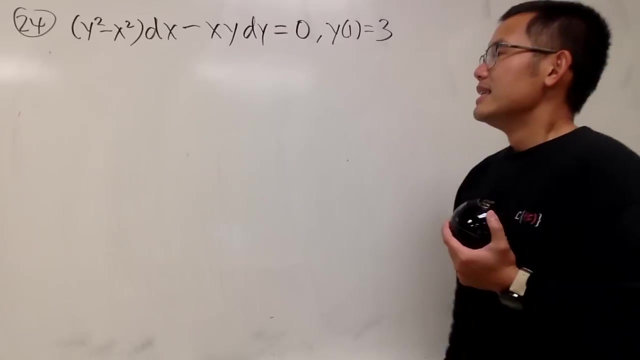 Um, Um, Um, Um, Um. x, that is minus xy, dy, is equal to 0.. Oh yeah, y of 1 equals 3.. So, all right, here we go To do this. you have a few ways to do it. 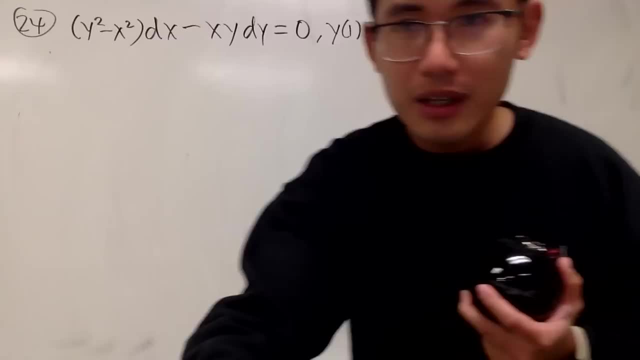 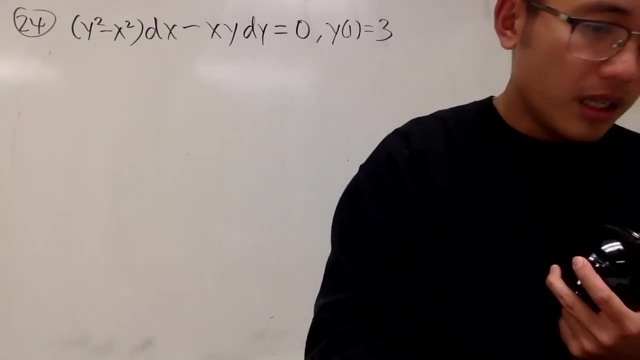 That's why I put it at the end And let's see how much time. right now it's 8 PM, right? Just that you should, that you can see it, And we have a few ways to do it. This right here. 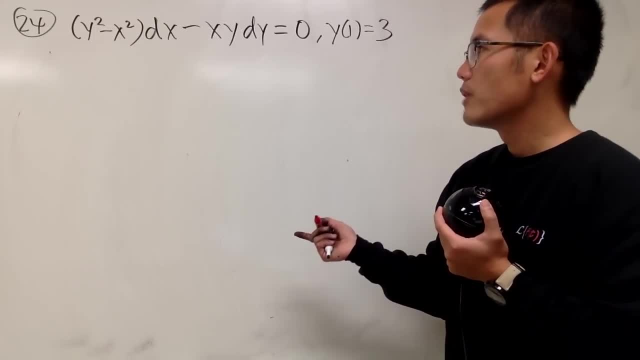 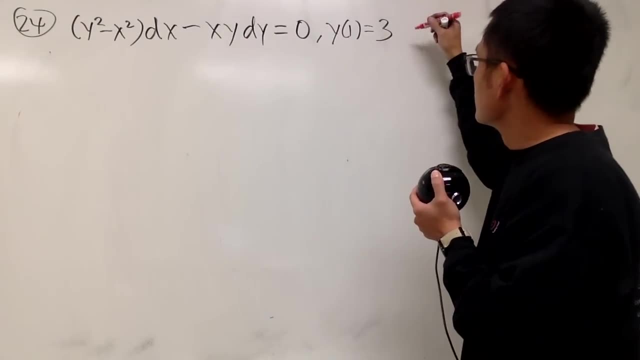 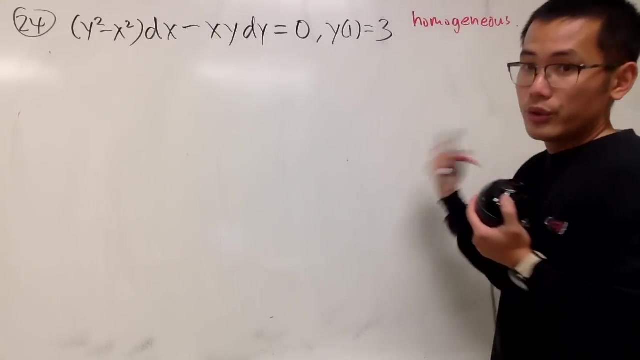 it's actually, you see, y squared, yx squared and then xy. So this right here it's homogeneous. So let me just tell you, this right here is homogeneous. So you can do the homogeneous way, just isolate the y, the x and all that stuff. 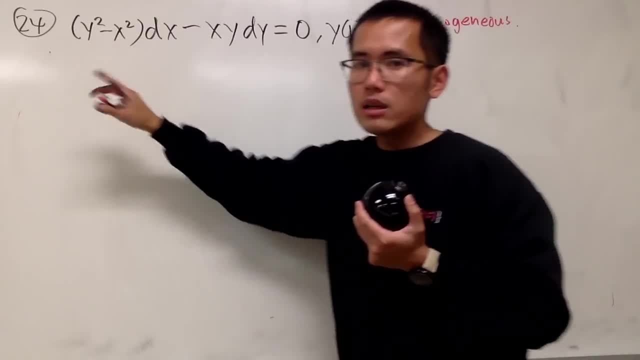 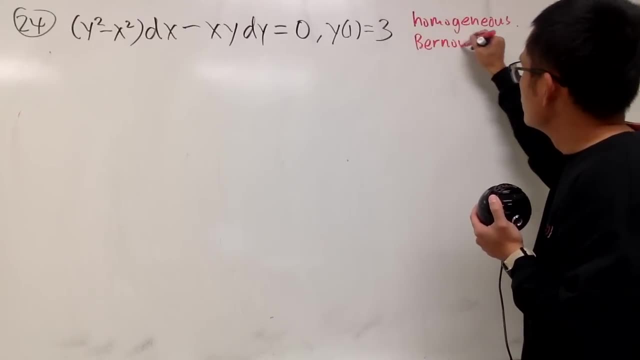 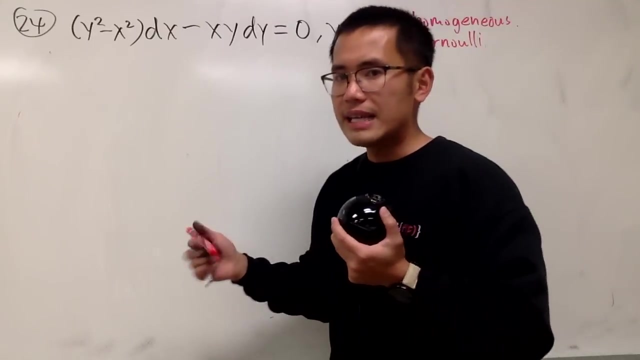 But if you look at here, you have y and you have y squared. In fact, you can actually get to Bernoulli's as well. So this is this is the Bernoulli's differential equation as well, And if you check to see if this is exact or not, 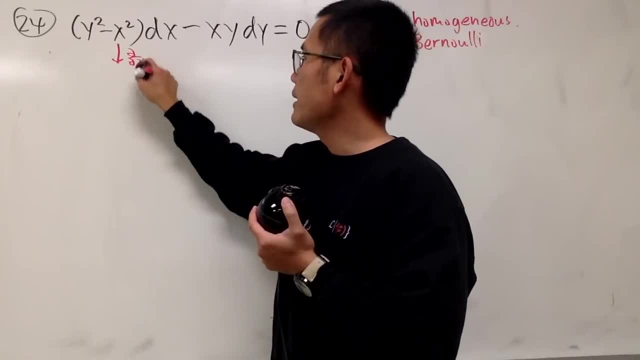 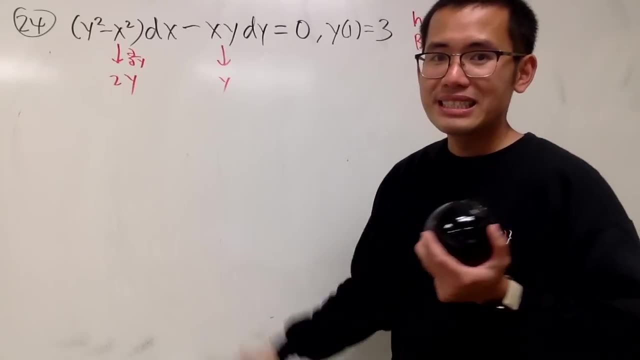 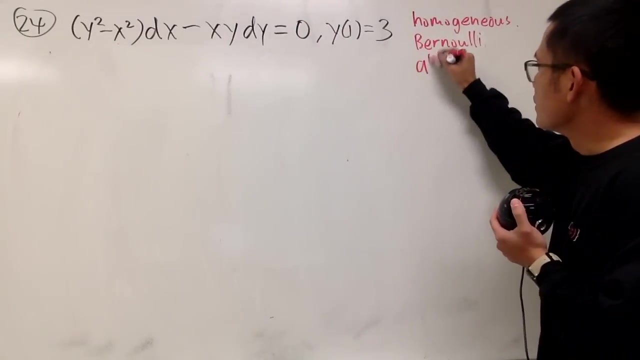 well, do the partial with respect to y, we get 2y. and do the partial with respect to x, we just get y. No right, It's not exact, but this is actually almost exact. So this right here, I'll just tell you it's almost. 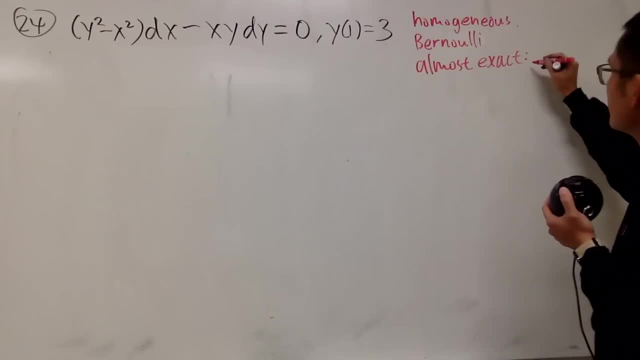 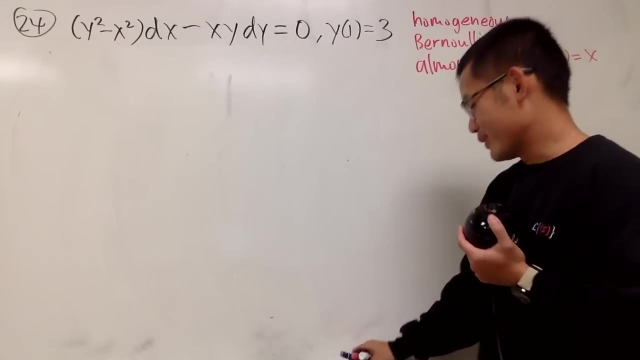 exactly, and the integrating factor that you can use is: mu of x is just equal to x. How do I know? Because I created this equation, So I'm just going to tell you guys all this. In fact, question number 23,. 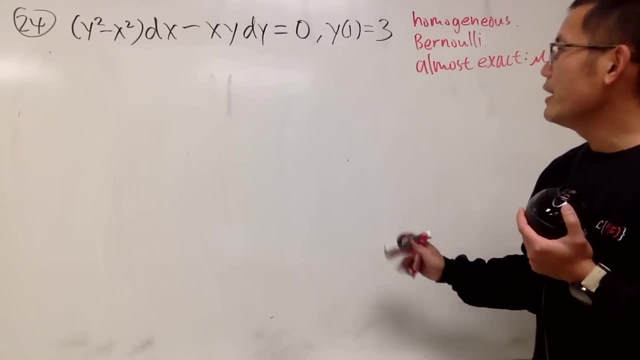 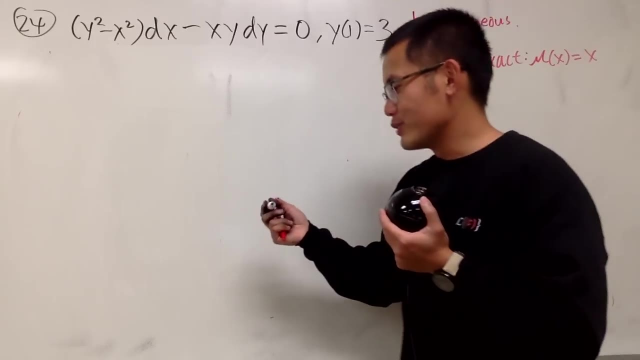 I believe it's also homogeneous, but whatever. Anyway, I'm gonna do Bernoulli's differential equation, because I think I messed up all the Bernoulli's so far. right, So I'm just going to do the Bernoulli's. so here we go. 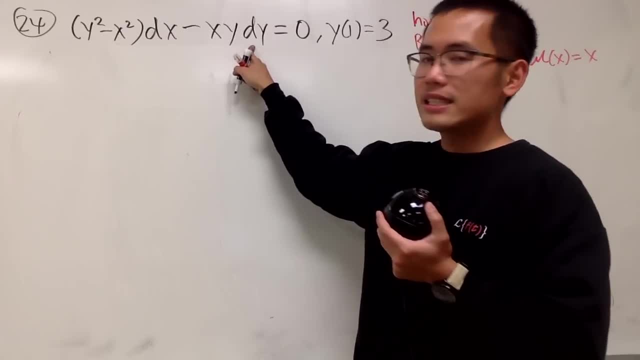 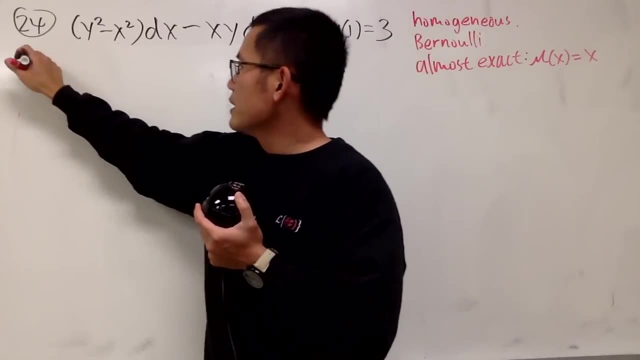 Let's do Bernoulli. for that I want to get a dy dx. I will actually do both, you'll see. Do Bernoulli first, Get dy dx by itself, so move this to the other side. But I already done first, so I have x y dy. 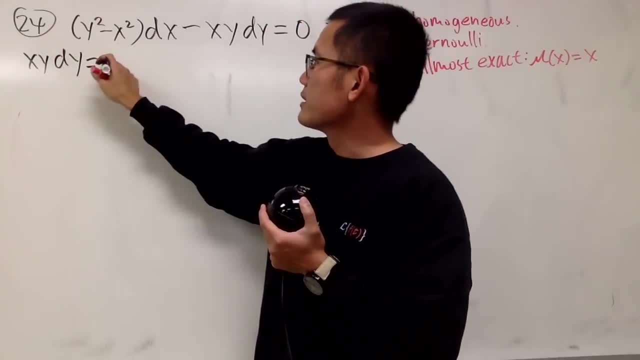 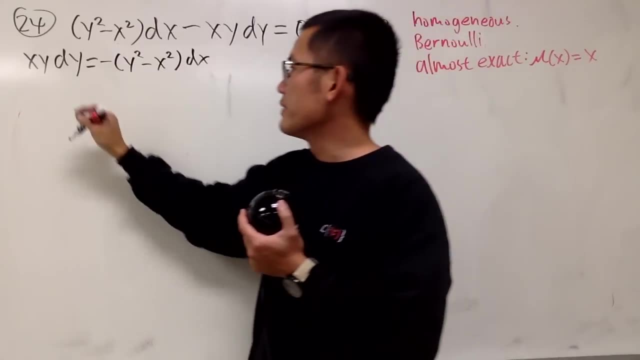 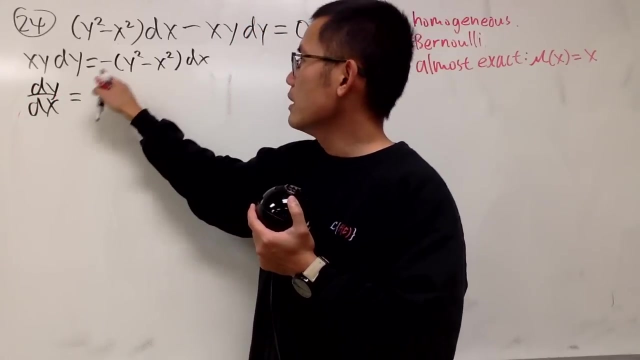 that's equal to um. move this to the other side so it becomes minus y squared, minus x squared dx. yeah, And then divide and all that stuff. So if I divide by dx on both sides I'll get dy dx and that's equal to. 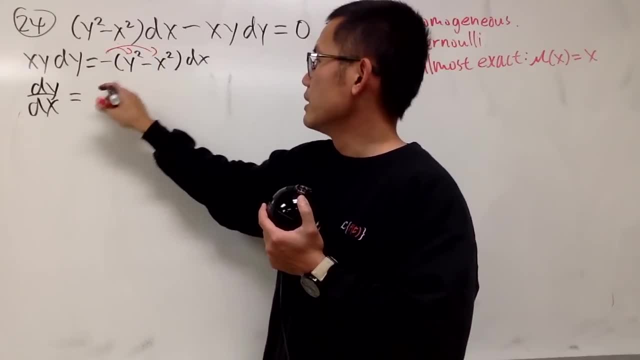 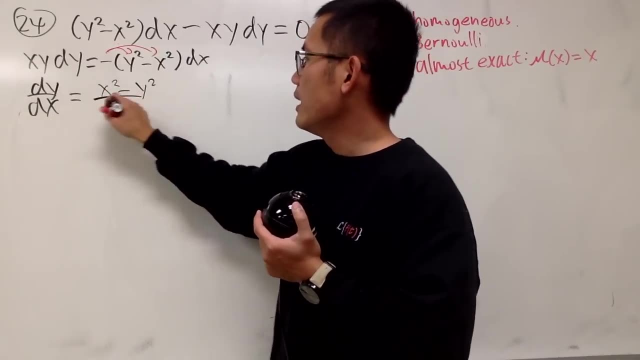 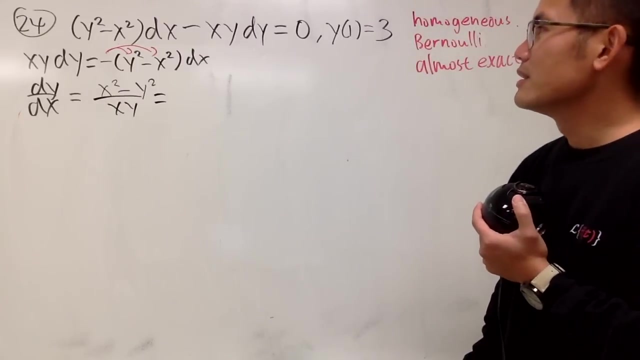 um, you'll see the difference. So I will, uh, I will just um distribute this and we have just um x squared minus y squared right, Switch the word and all that stuff, And then I will divide the x- y like this: 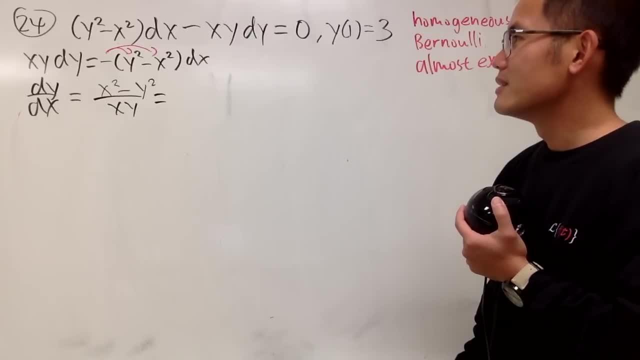 which is going to be No. this is not Bernoulli's. It's not. is this Bernoulli? Why am I messing up on all the Bernoulli's cannot be Bernoulli's. Bernoulli's is- no, just- oh. 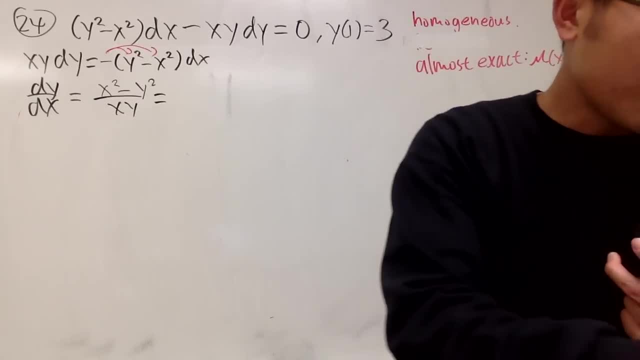 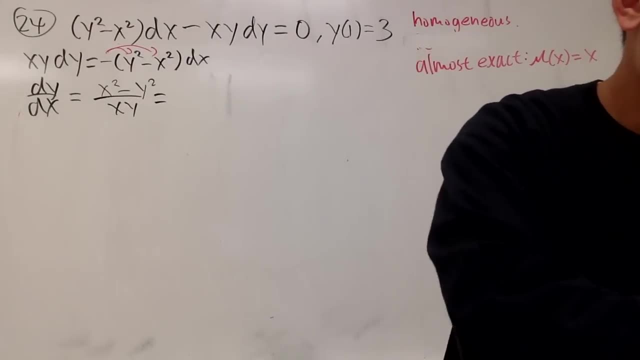 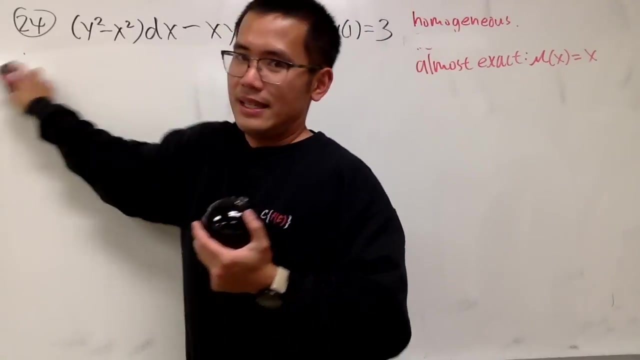 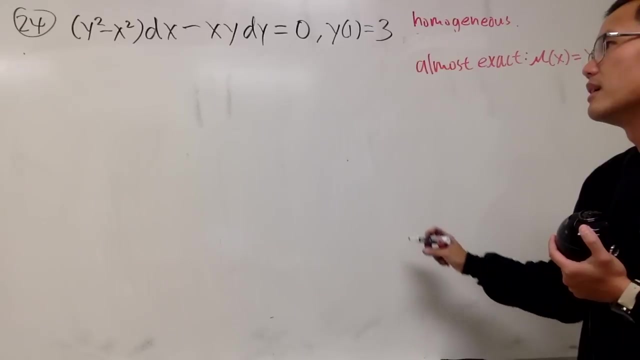 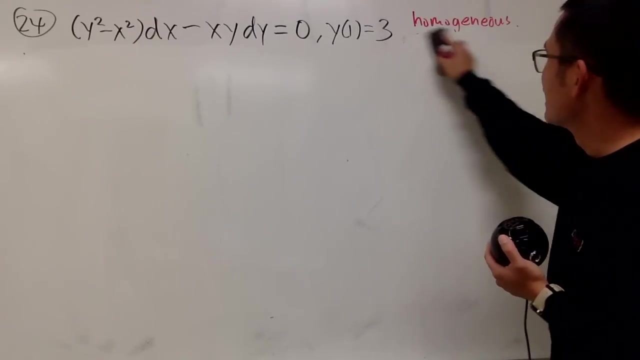 I know why it's not-. let me just double-check. Hmm, All right, I'm going to do another Bernoulli equations, uh, later on, but for this, right here, I dy dx. No, let's just do homogeneous differential equation and then yeah. 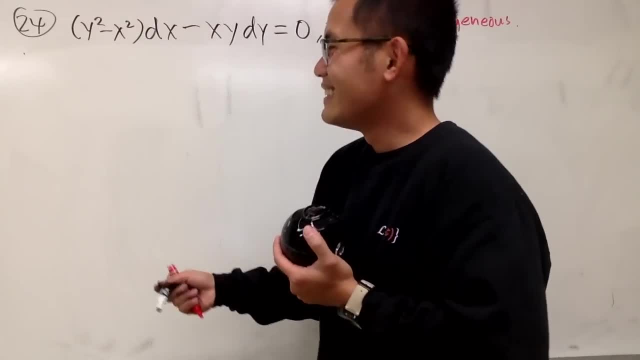 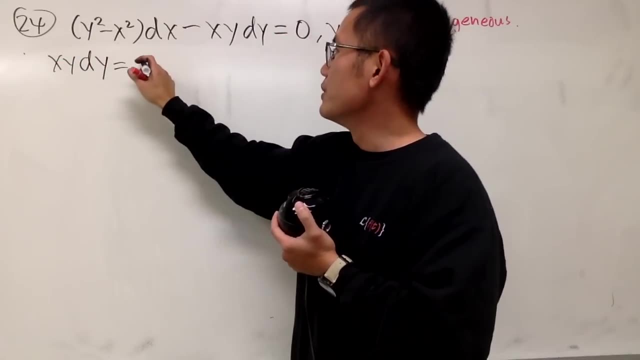 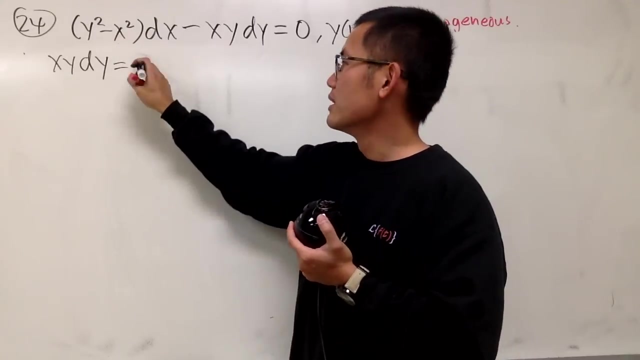 let's just do that And then, yeah, Sorry, Anyway, this right here, x, y, dy is equal to this, which is uh, negative parentheses- actually, no, That's what I'm talking about. Bring this to the other side. write down first, which is just this: 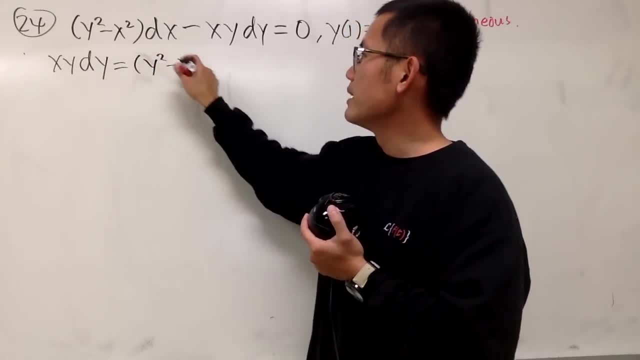 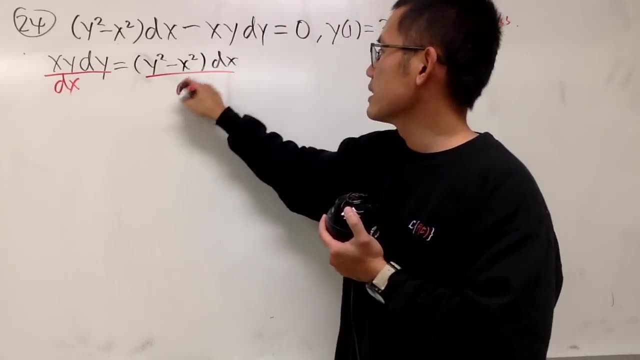 Oh yeah, I'm making a mistake earlier too, But anyway, this is just y squared minus x squared dx. Yeah, And I will divide both sides by dx, so that this right here will be over there, and then multiply-, multiply- divide by x. 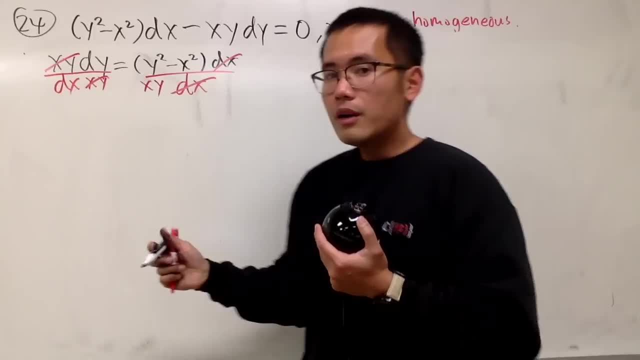 y on both sides like this: All right, So here we go. dy dx equals y squared over dx. All right, So here we go. dy dx equals y squared over dx. All right, So here we go. dy dx equals y squared over dx. 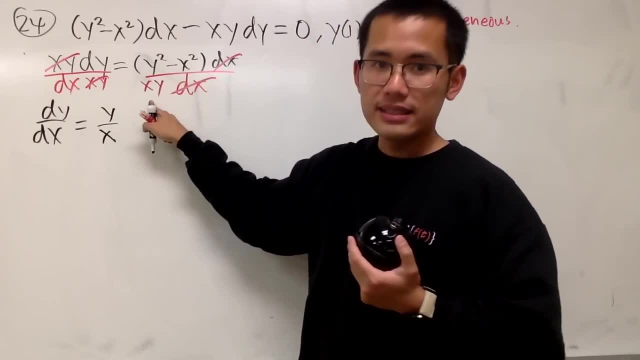 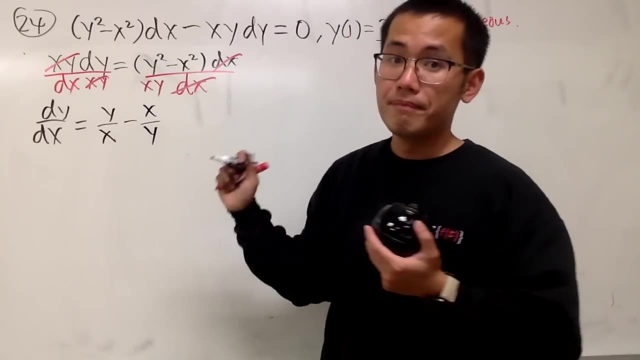 You did the math. So this y squared over dx is just y over x. yes, The other one, this over this, is minus x over y. uh, yeah, like that. all right, I believe you can make this into x が. 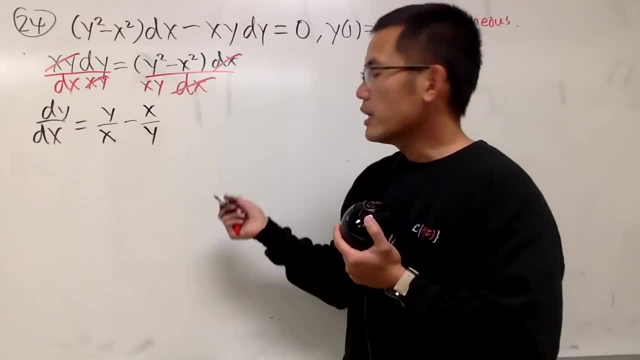 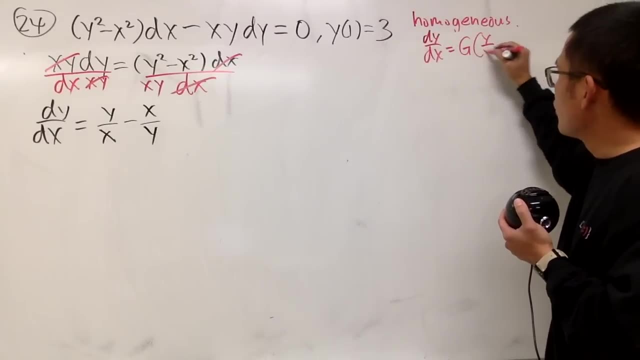 Seriously, let's not do that. So homogeneous is the way. Look at this, though: We want to get to homogeneous. This means we want to have dy dx to be a function in terms of y over x. This is y over x. 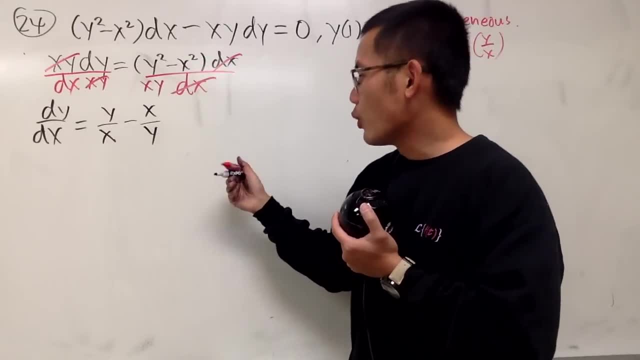 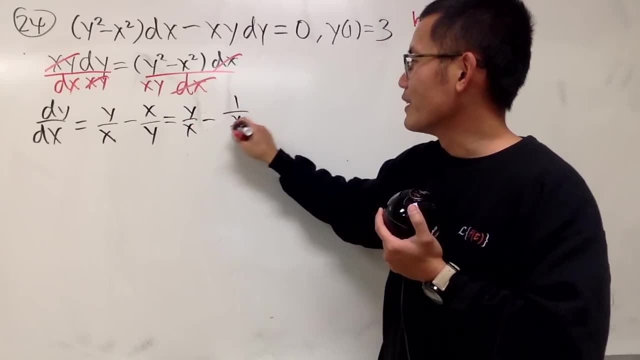 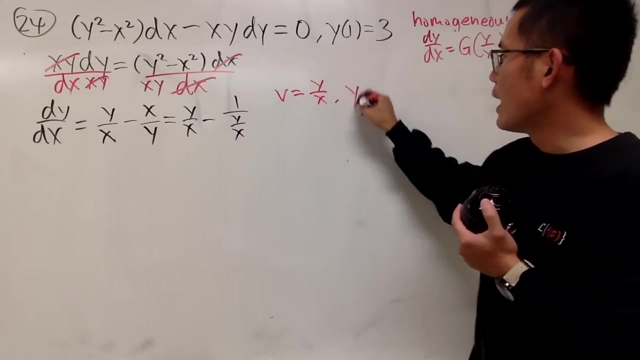 This is actually also y over x, 1 over. So what you can do is you can just write yes, y over x equals y over x, minus 1 over y over x, like that see, Alright, here we go. phi equals y over x. y is equal to phi times x. 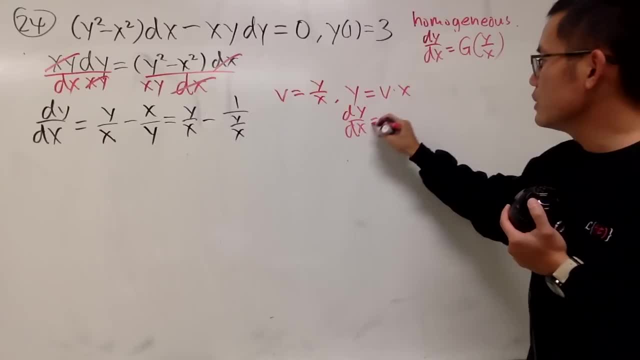 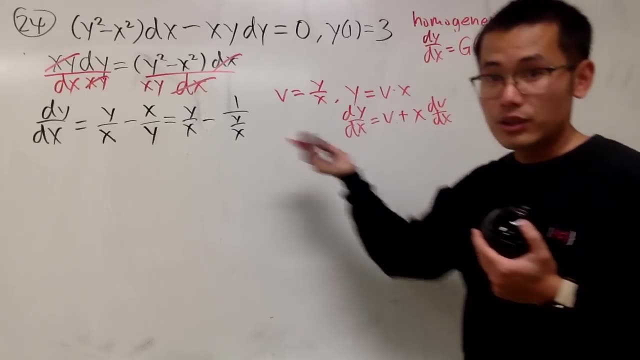 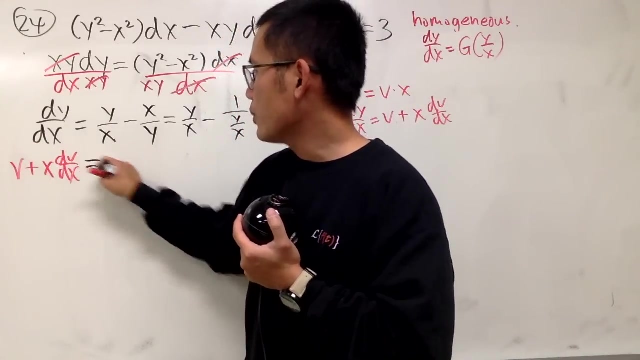 so that means dy dx equals phi times 1 plus second times the first. so dv dx like that. So go ahead. we have v plus x dv dx. that's equal to this. right here is my v, it's your v as well, it's everybody's v. 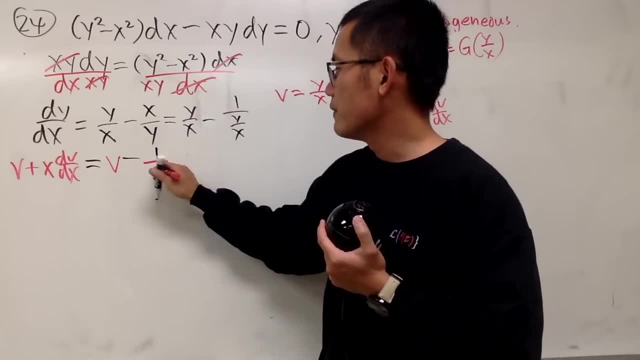 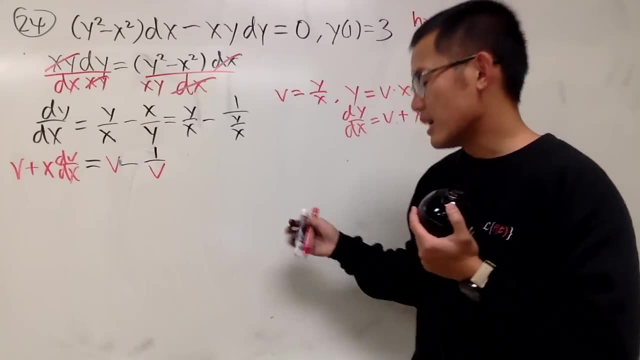 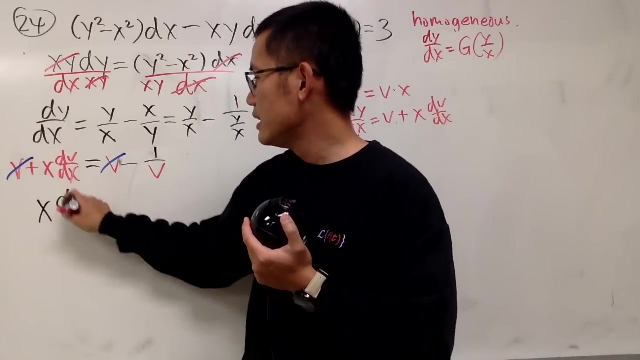 and then minus. this is 1 over v. so we have 1 over v, like that, v minus 1 over v, right? So just like that, Very nice, though, because the v's cancel the out. So now we have x, dv, dx and that's equal to negative 1 over v. 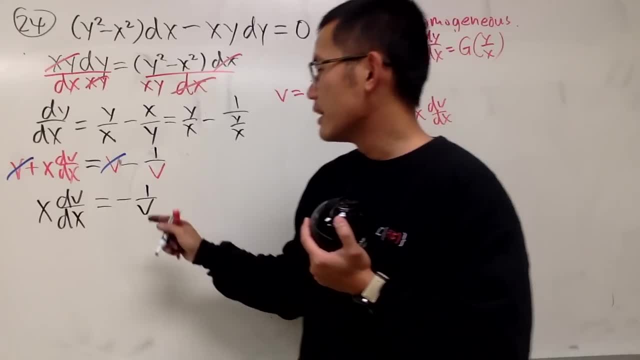 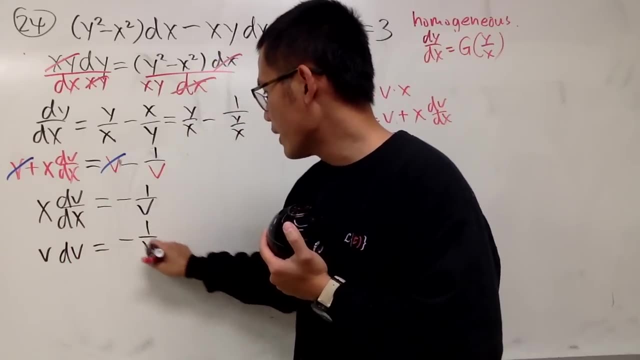 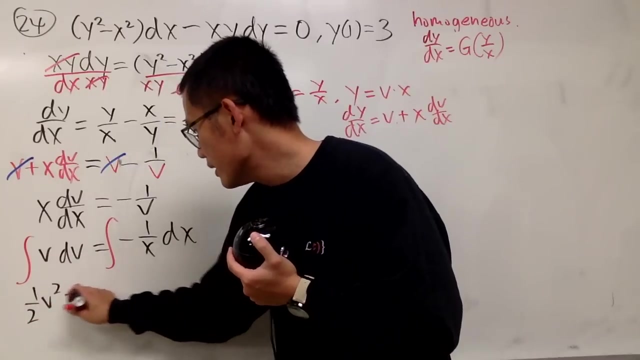 let me just make sure yes, and then let's just multiply the phi on both sides, divide, so we get v? dv equals negative, 1 over x dx, and then integrate, integrate. so when we have this right here, it's 1 over 2 v squared equals natural log. 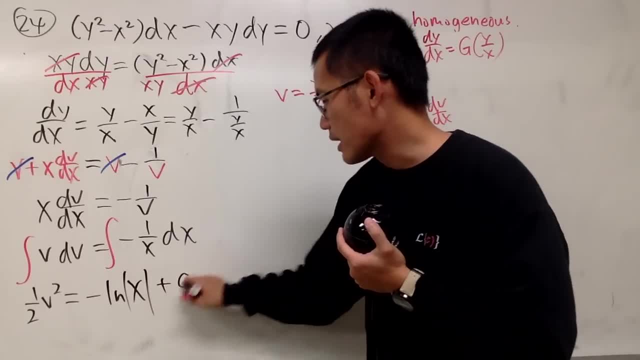 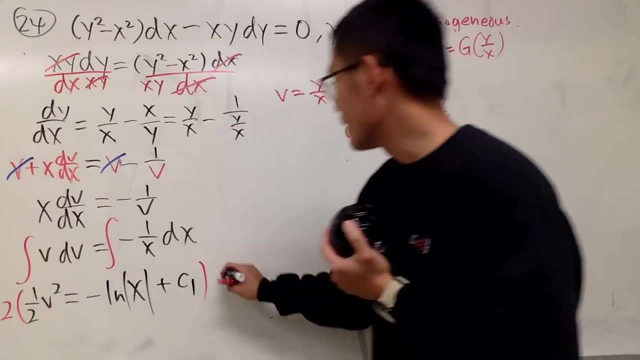 but it's negative. it's an opposite for you. maybe n plus the constant. so that's pretty much it. Well, c1, why? Because I'm going to multiply everybody by 2.. So when we multiply everybody by 2, we see that we get v squared. 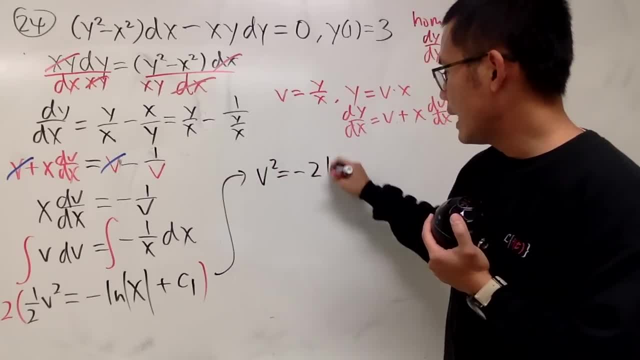 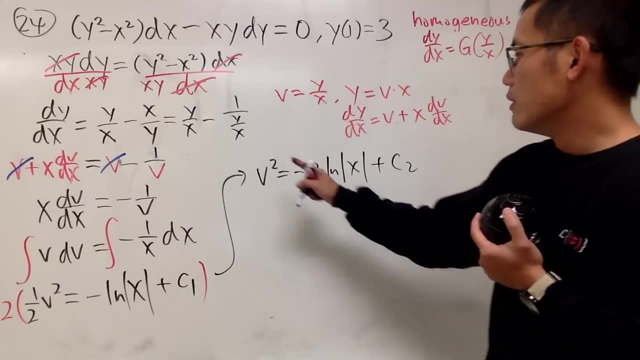 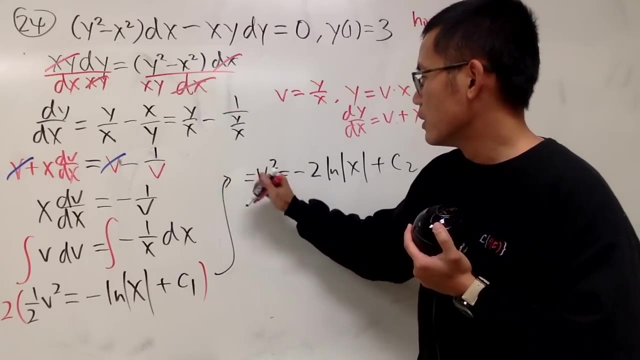 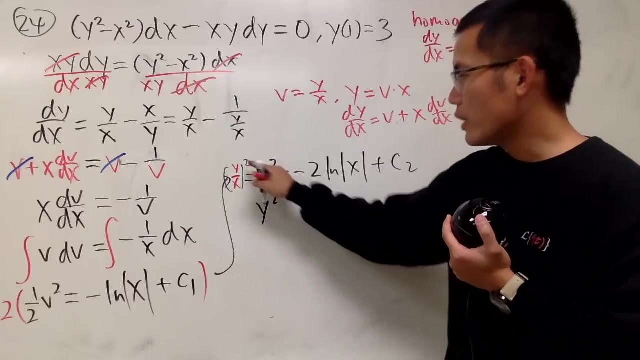 that's equal to negative 2 ln absolute value of x and then plus c2, right, So this is good. Now this is v squared. so that means we have 1 over. this means we have y over x and squared: yeah. So this right here means we have x. well, y squared on the top. 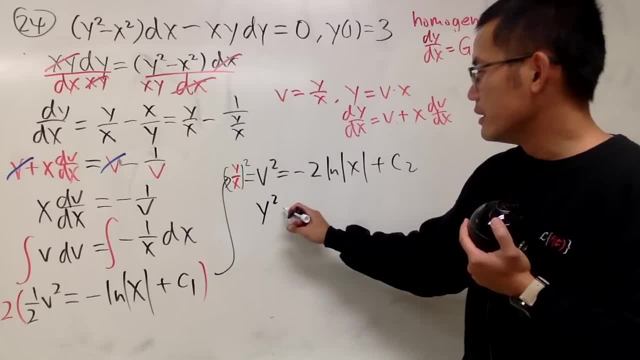 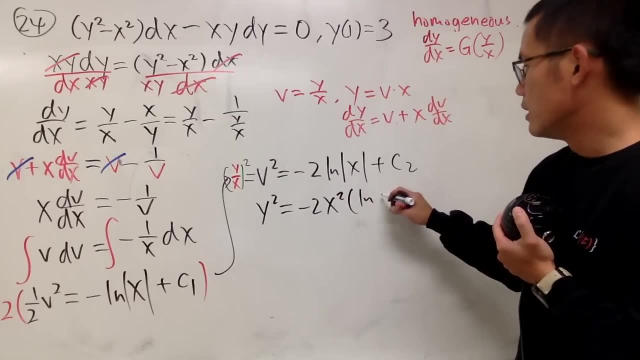 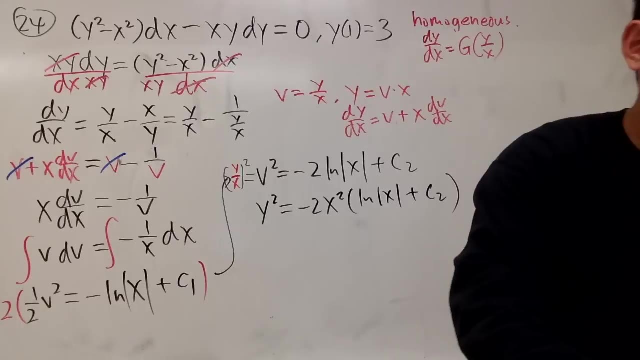 over x squared, but let's multiply x squared on both sides, so we have this: it's equal to negative 2 x squared times ln absolute value of x, and then plus c2, like this: yes, Yes, Okay so. 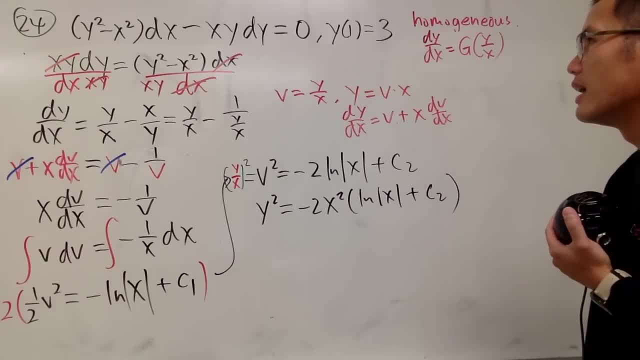 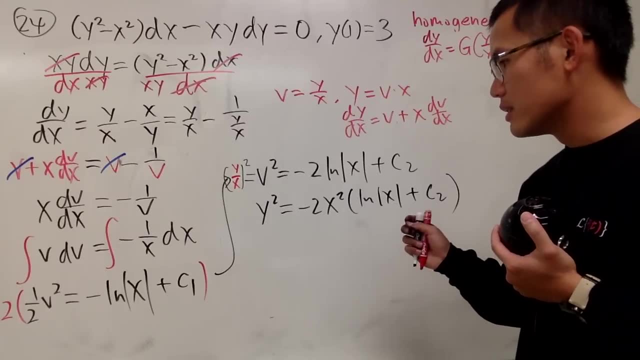 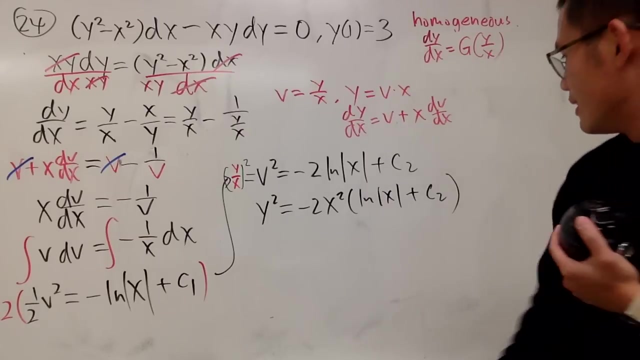 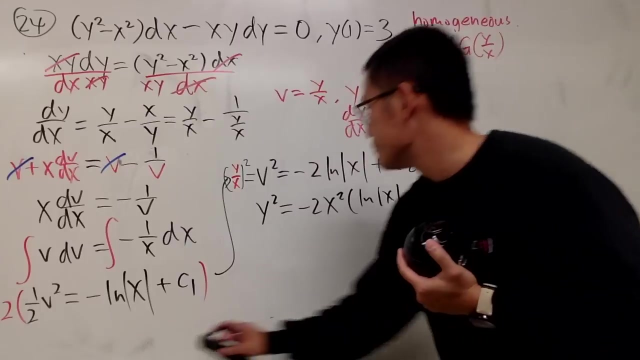 let me just double check. All right, I think that should be okay. Okay, so multiply by v to oh, yeah, yeah, yeah, yeah, yeah, it works, it works, yeah, Okay. No, the c2 should not be what the heck. 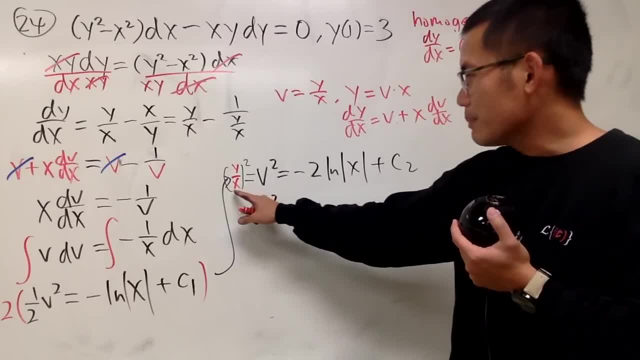 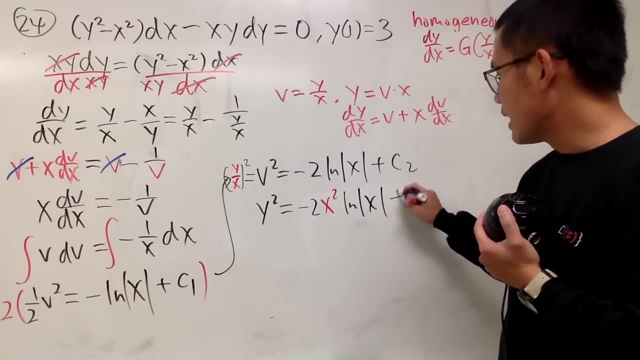 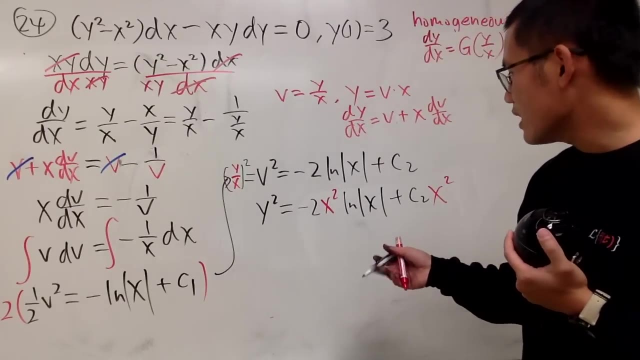 Okay, okay, okay, Multiply x squared on both sides, so we have negative 2, x squared, and then we have ln absolute value of x plus c2, and then x squared. Yeah, there we go. Oh, and then you can just take the square roots and all that stuff. 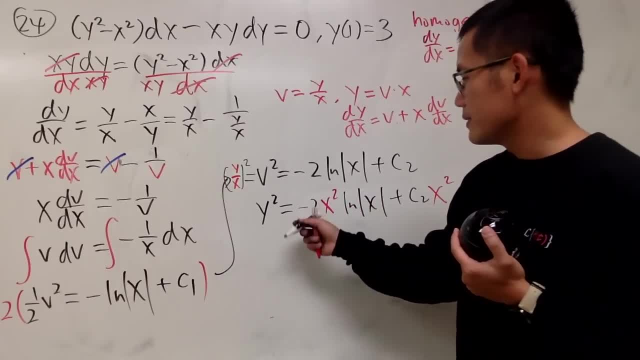 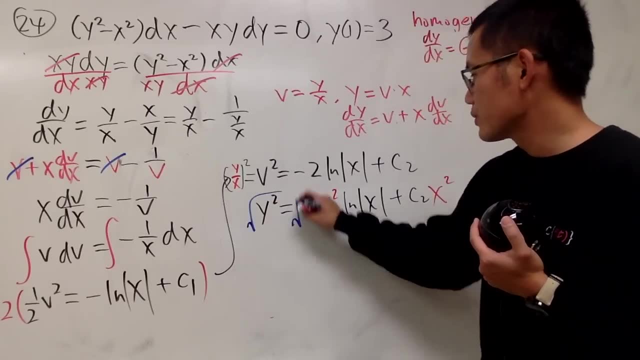 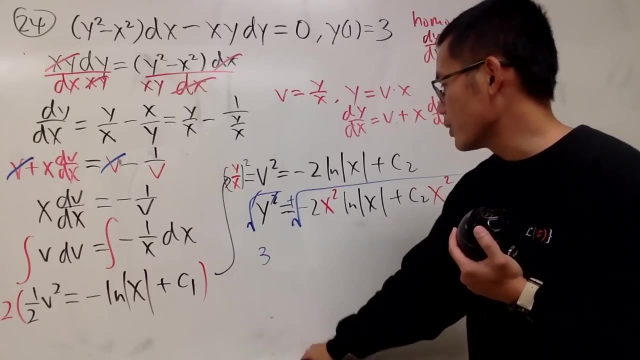 but I wanted to find out what c is. Well, so you can do the square root, of course. Square root, square root. But you want to have positive 3, right, So right here, you just take the positive square root. so this is out. 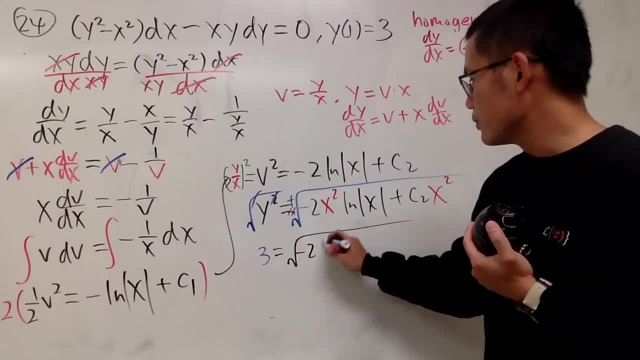 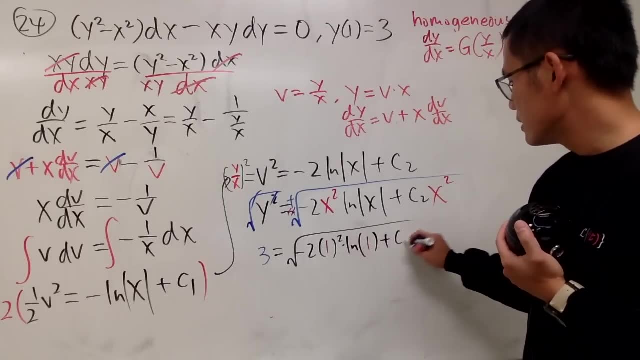 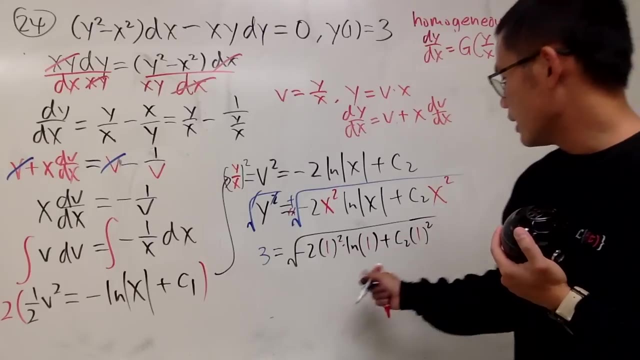 So you have: 3 is equal to square root of negative 2 times 1, square times ln 1, plus c2 times 1. squared like all that, This is 0, that's good. So you see, 3 is equal to square root of c2, which is just: c2 is equal to 9.. 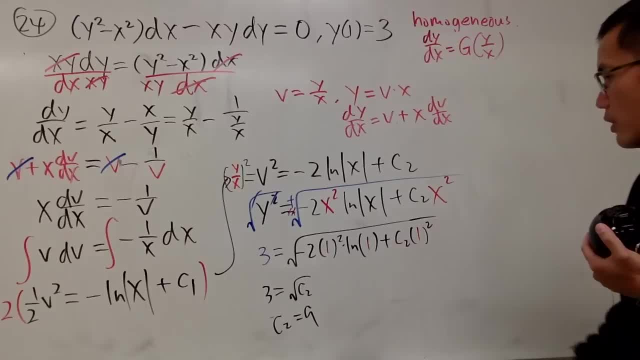 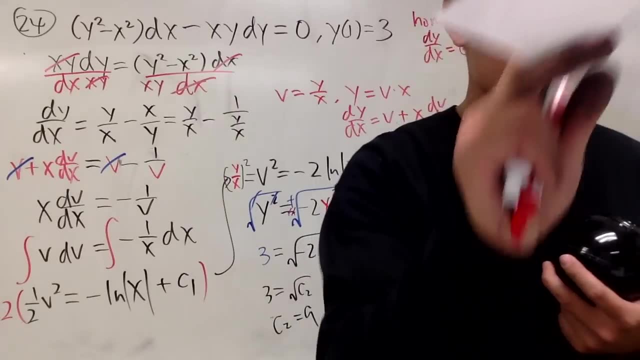 Good, Now I can just put this back here, So I will just tell you guys the answer And let me just double check that I actually have the correct answer. Okay, good, So c2 is 9.. Put it here. 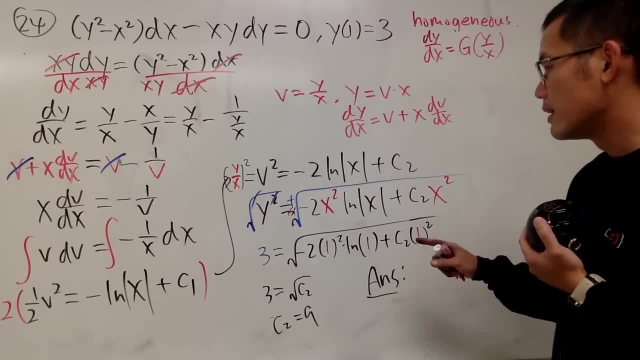 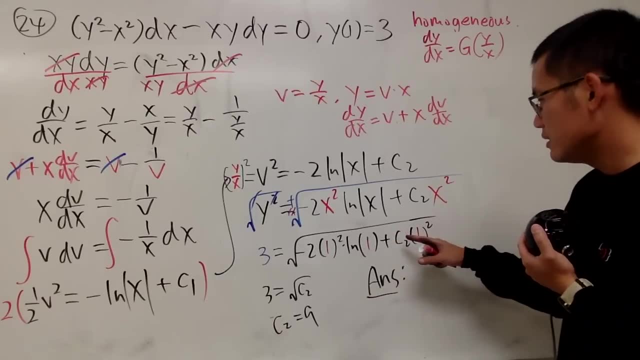 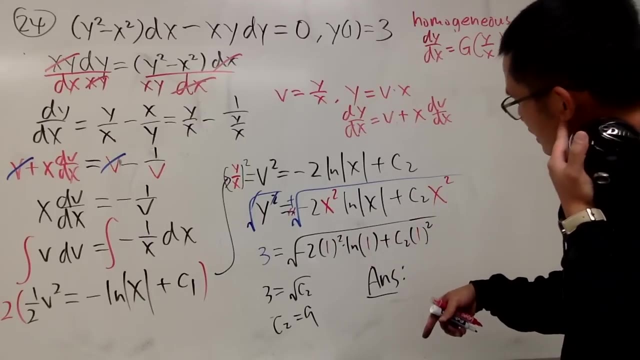 So what you can do is the following. Yeah, What you can do is the following: Just put the 9 in. You know, you can have the x squared out or the x squared in the front, so up to you. So 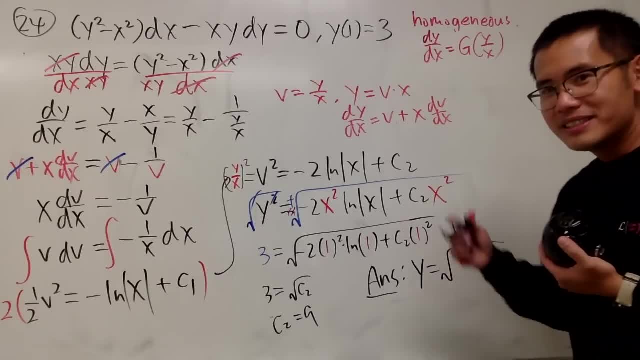 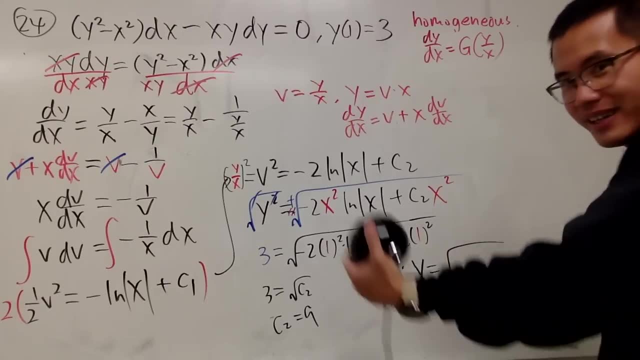 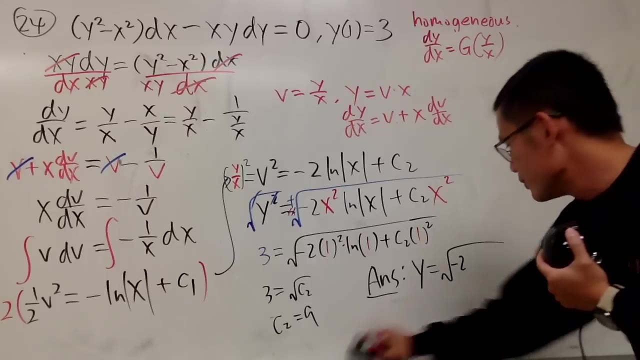 y equals square root. You can see how my soul is kind of like leaving my body slowly. Okay, 5 hours, But anyway, c2 is 9.. So you can write it like this: You have negative 2.. You know what? 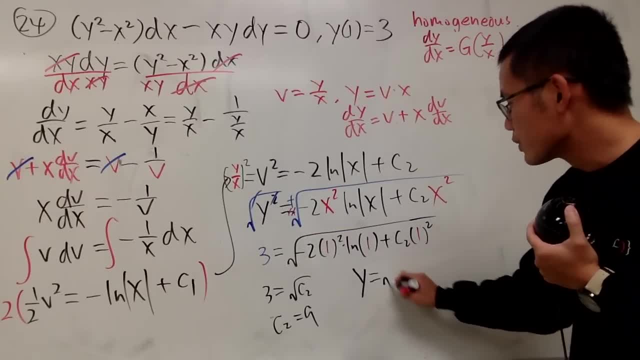 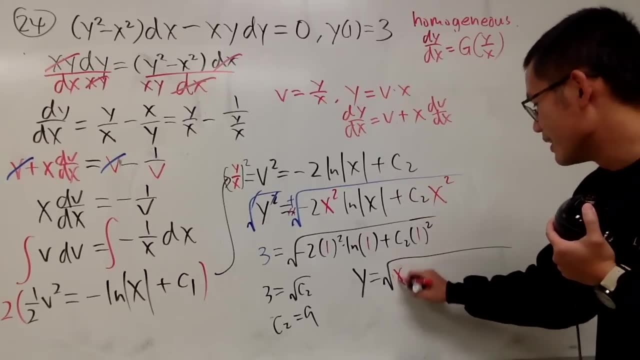 I'm going to write it down one more time: y is equal to square root. It's equal to square root. This is negative 2.. You know what? Let me actually just factor out the x squared. I don't know, I'm sorry. 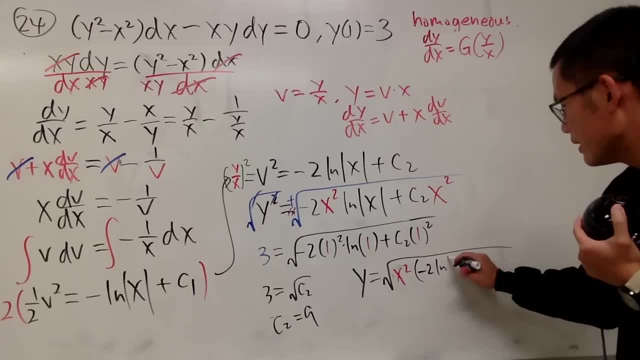 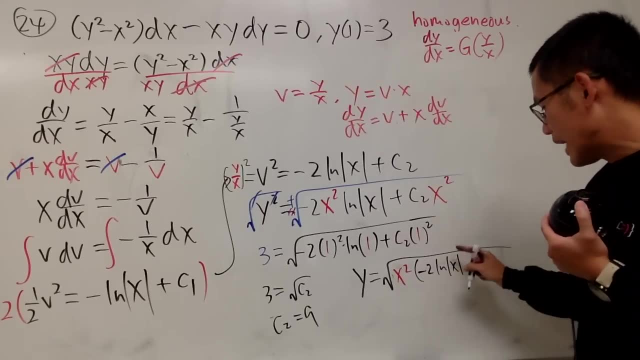 x, squared parentheses, negative 2.. ln- absolute power of x. if you wish, And technically you have x is equal to 1. You should just have ln x And then you just say x is greater than 0. But I will leave that to you guys. 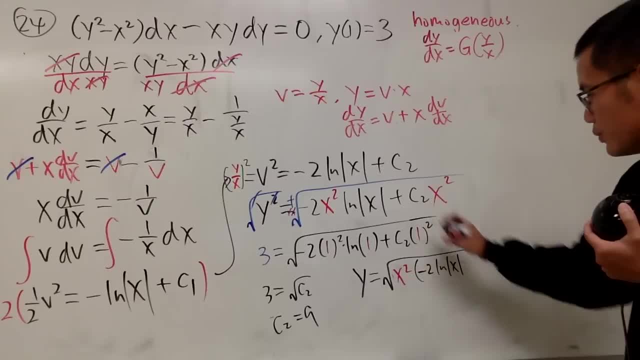 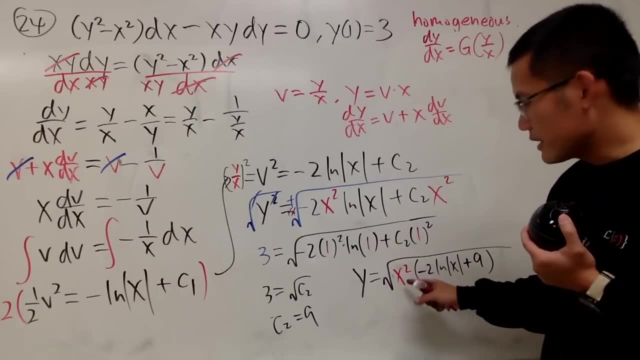 Anyway, you have this part And then you have the c2 is 9.. So you just add the 9 to it. Okay, Yeah, But the reason I want to do this is because square root of x, squared, is just x. 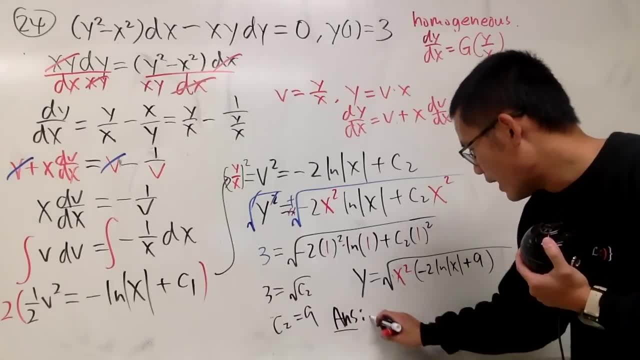 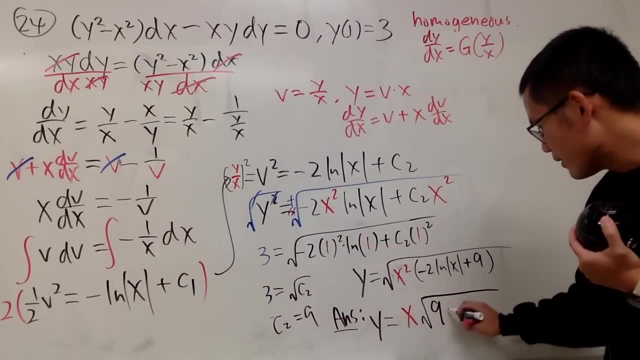 So that's why. So anyway, Final answer: y equals: This guy is just x. And then you have the square root, And let me just put the 9 down first. Minus 2 ln x, Like this: 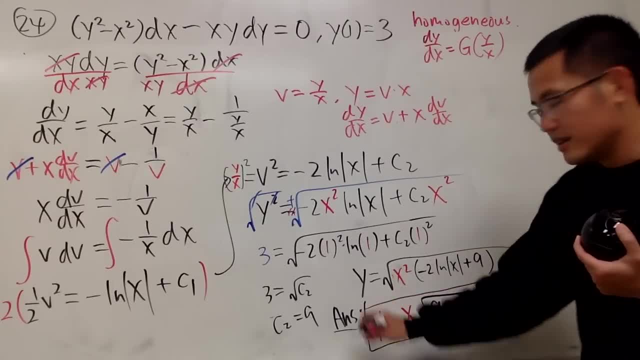 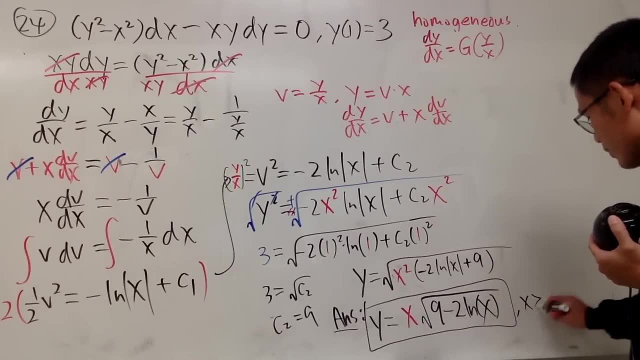 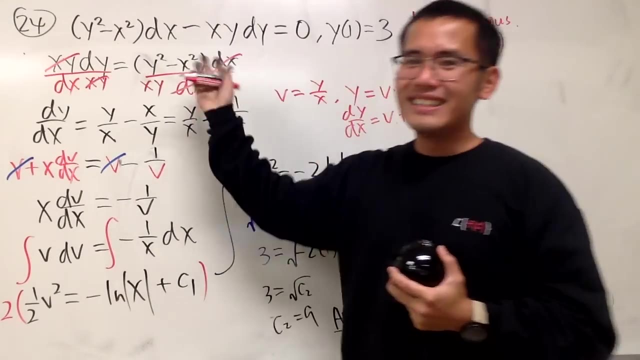 Right, Okay, So yeah, And again you can just put parentheses in and just denote that x is greater than 0. But that's it, Done, Done, Done, Done, All right, Done. So 24 differential equations for you guys. 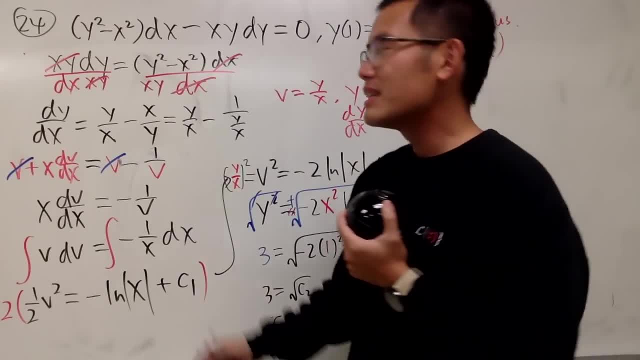 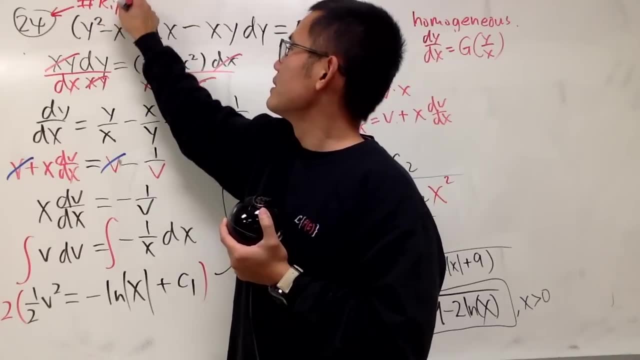 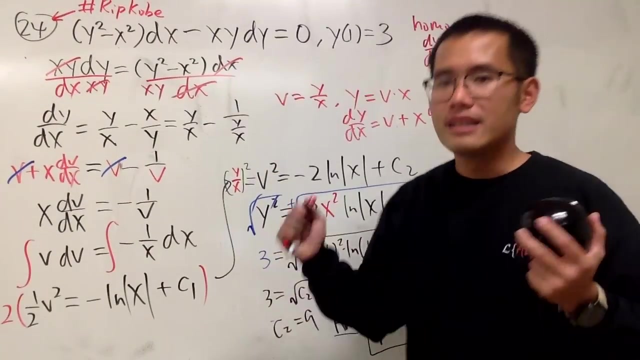 And this right here Again. hashtag: Rest in peace, Kobe branch. All right, Let me see. Okay, Done, Done, Done, Yeah. So that's it, Thank you, Bye, Bye, Bye, Bye, Bye. 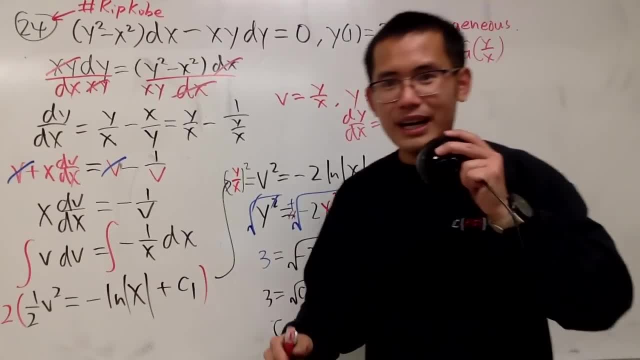 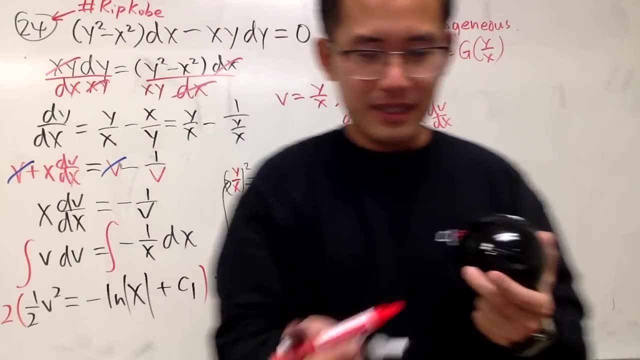 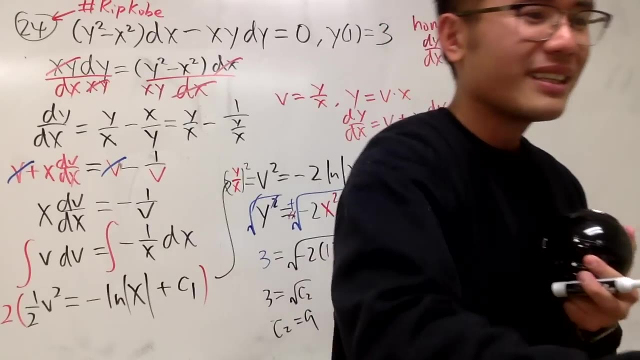 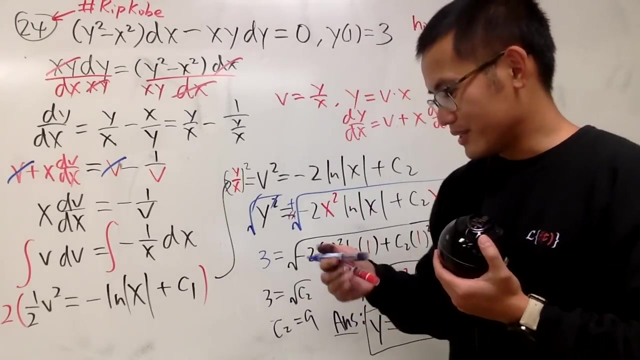 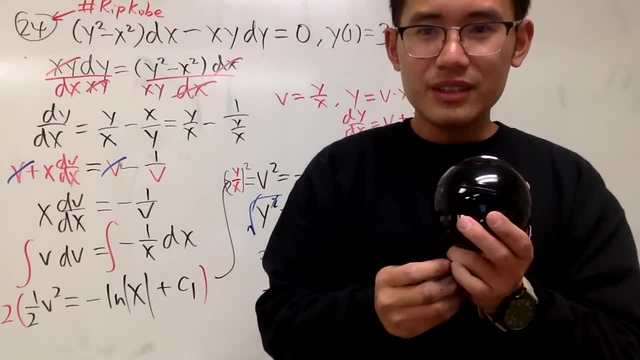 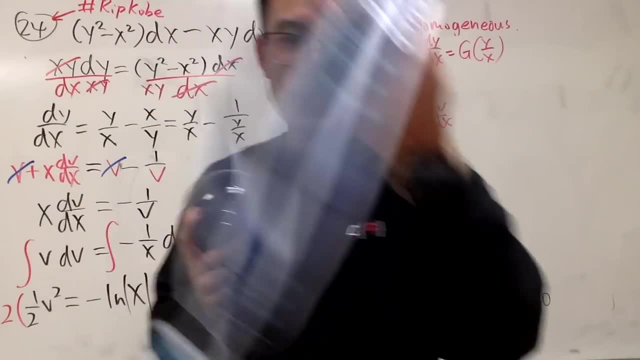 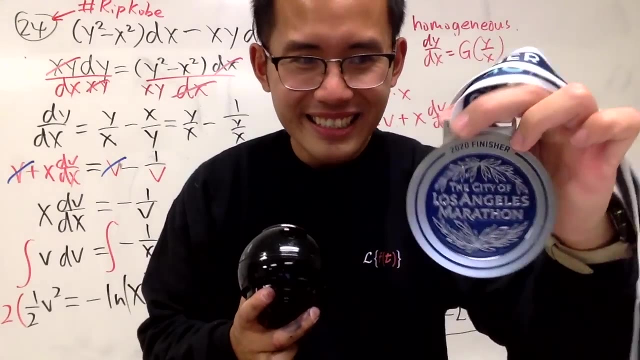 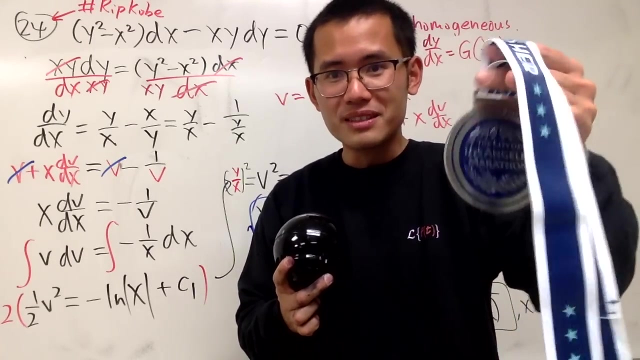